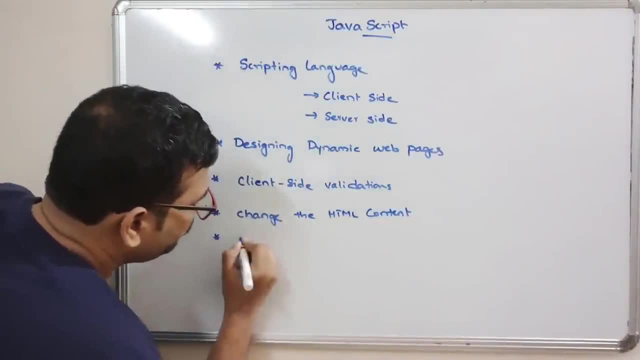 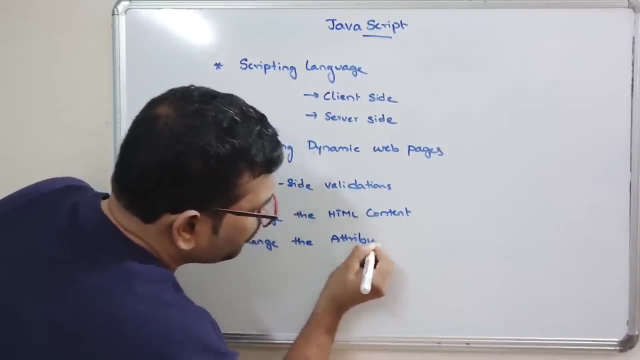 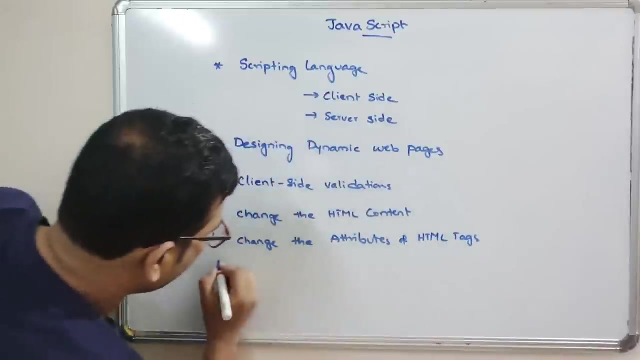 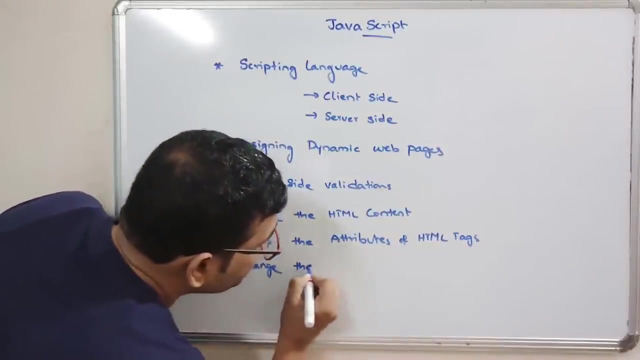 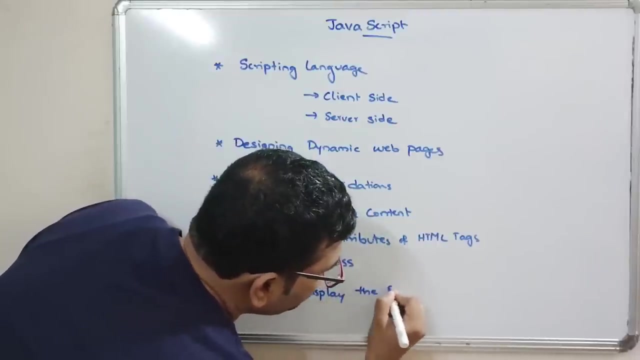 content. Similarly, we can change the attributes. We can change the attributes of HTML tags. Similarly, we can change the CSS. So already CSS also have been covered, So change the CSS. And also we can hide and display the content. Hide and display the content. Okay, So all. 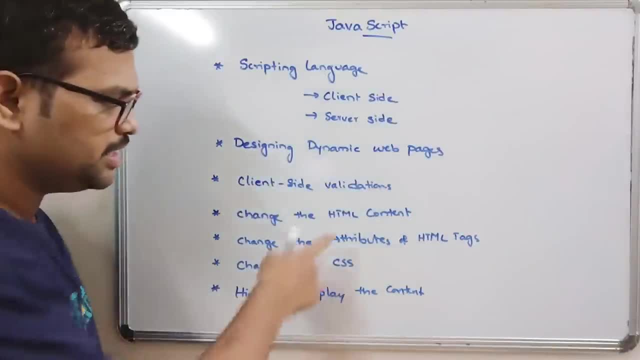 these things can be done by using the JavaScript. Okay, We can change the HTML content Similarly, attributes of HTML text, CSS JavaScript and so on. Let me know in the comment section or if you have any more questions, please feel free to ask. 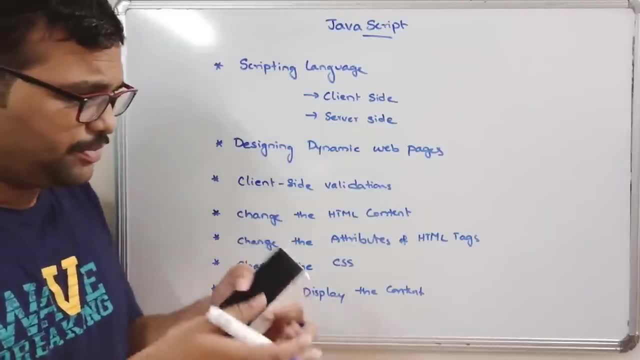 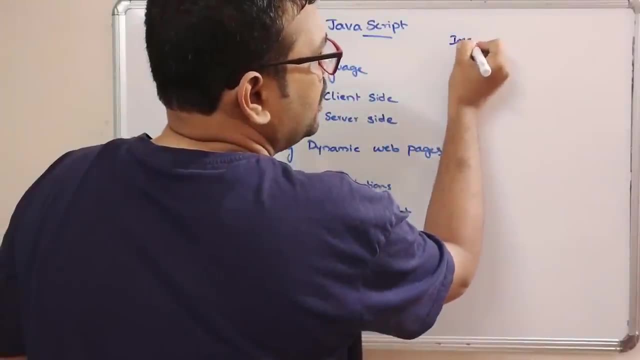 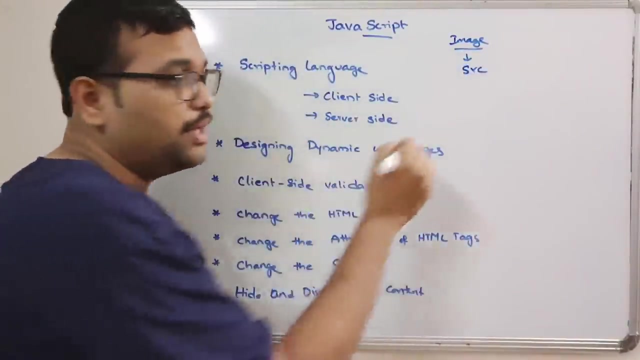 sets. we have seen different attributes. right, for every tag we are having different attributes. for example, go with the some image- okay, image tag. so in the image tag we have seen different attributes like src is the first attribute, source- okay, and then width, height, okay. all these are the. 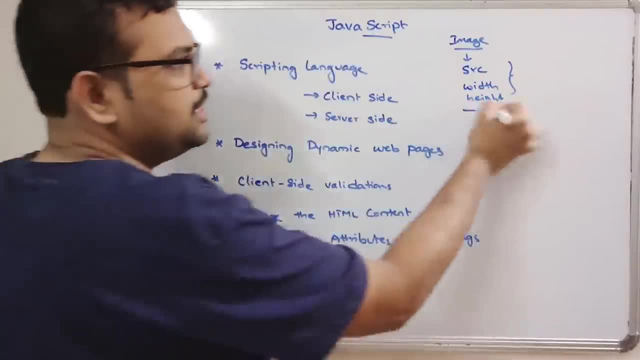 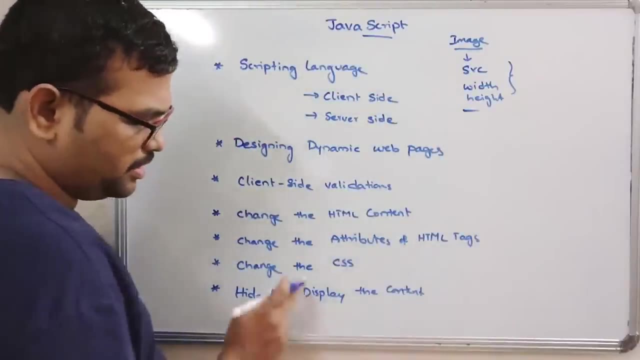 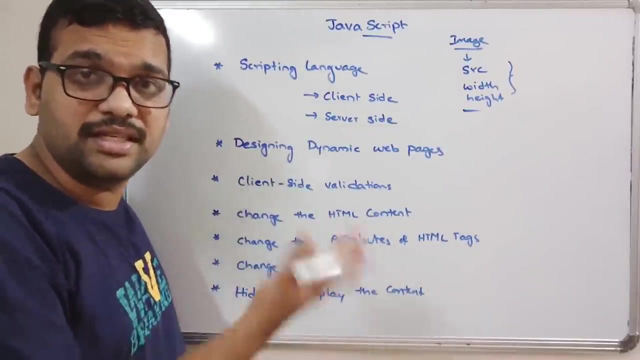 attributes. so by using the javascript we can change these attributes of this channel right. and similarly for, uh, this css. so we are having a different css right. so for front, the background and all these things, there are css, we can also change that particular css right. so for all these, 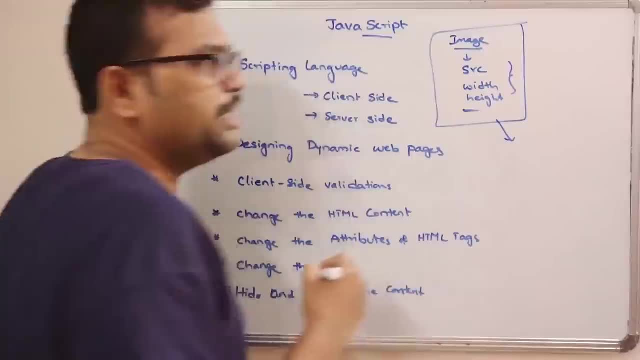 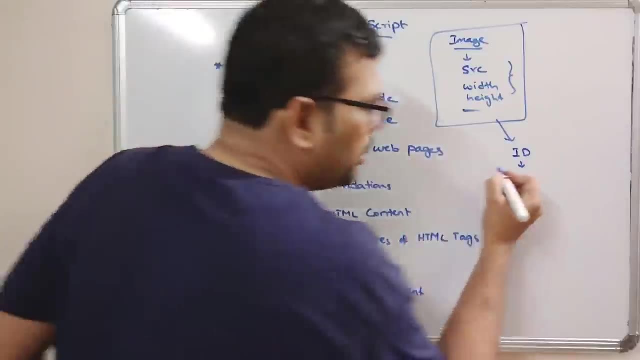 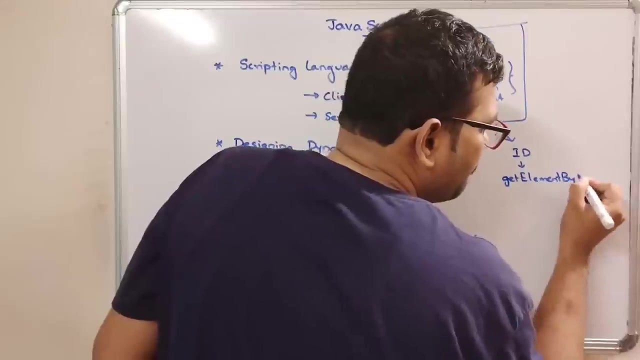 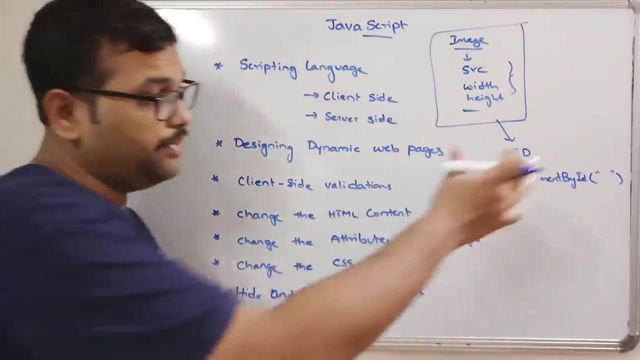 things we, we can have the content. i mean, we can retrieve the tag with the help of id. so for that we are having some function called get element, get element by id. so in in the parentheses we have to give the id, so that from here, whatever the id we are giving, 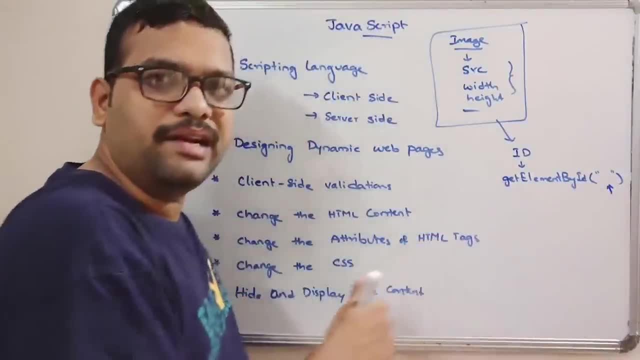 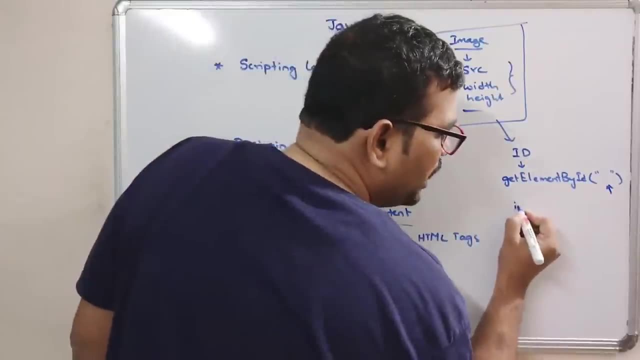 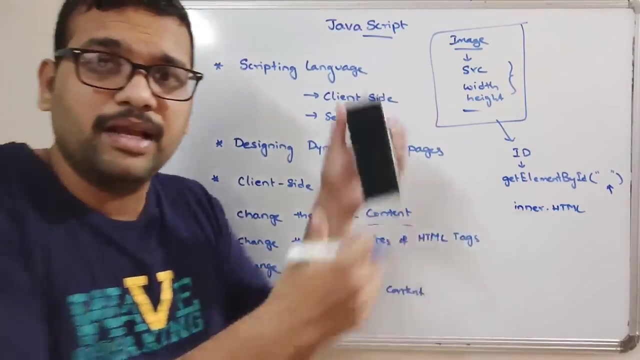 here, that id corresponding element will be written. okay, that particular tag will be written. and in order to change the html content, we are having a property called inner dot html. inner dot html. okay, so with the help of inner dot html, we can change the output right. so this is: uh, this is simply we can say: it's an output right. output statement. 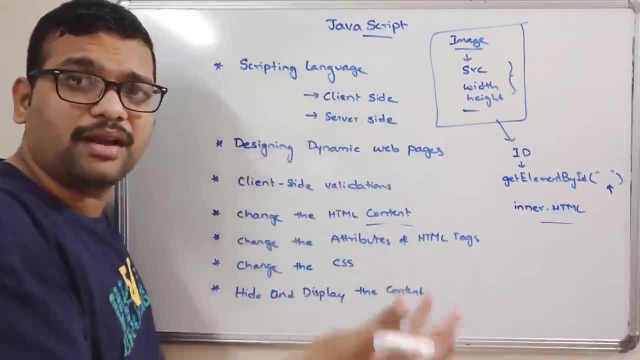 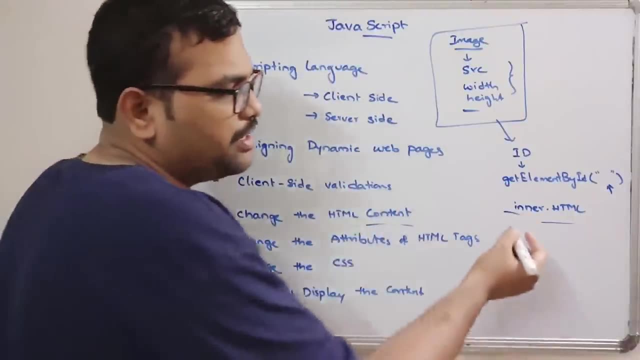 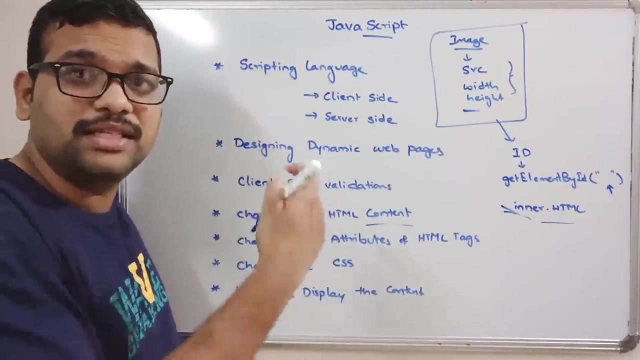 so, apart from this, we are having a lot of outputs. we can have ls boxes and all these things, but this is one, one output among all those things. so we can change the html content with the help of this inner dot html, so we can retrieve the tag, we can return the tag to which the 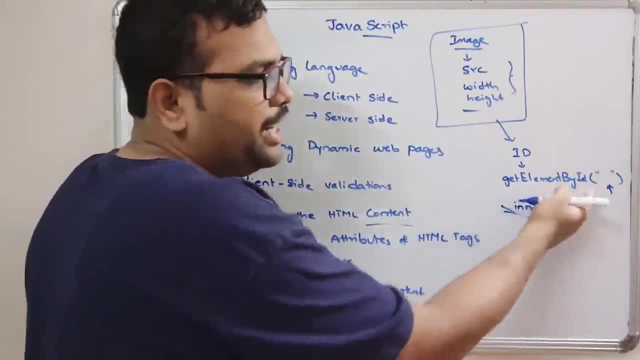 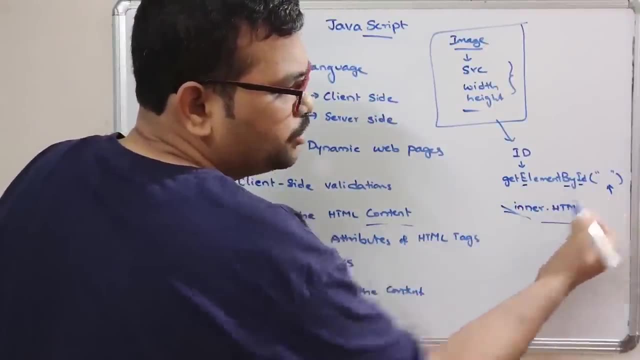 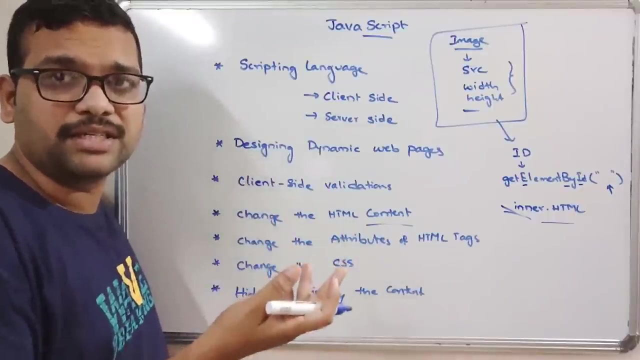 javascript should be applied with the help of get element by id function. get element by id function. okay, so here we can observe: E, B, I should be character. that means the first letter from the second word should be character letters. okay, the naming conventions. the naming conventions, because it is a function, this is a function, so naming. 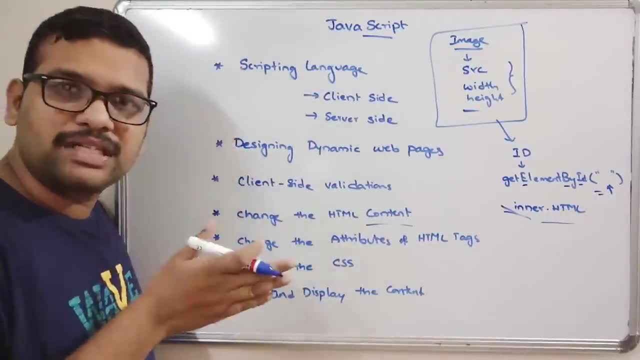 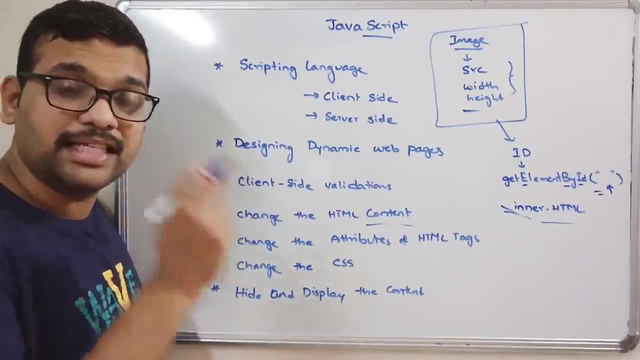 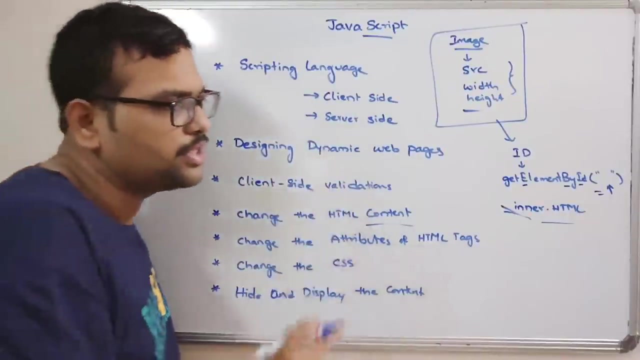 convention of a function must be: except the first word from the second word, every first character should be character. okay, except the first word, every, every first character of the second word from the second word should be a character. that's a naming convention to be followed, right? so this: 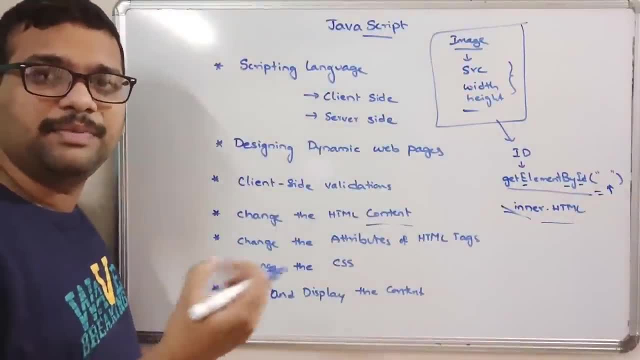 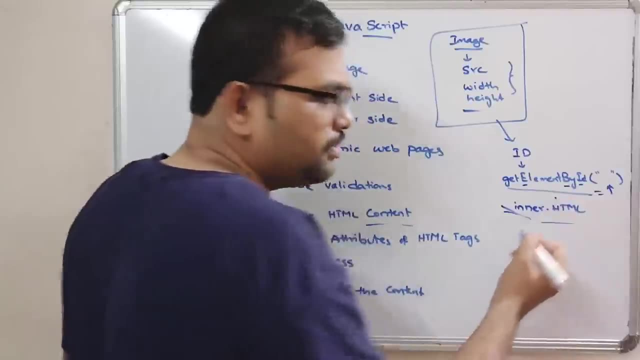 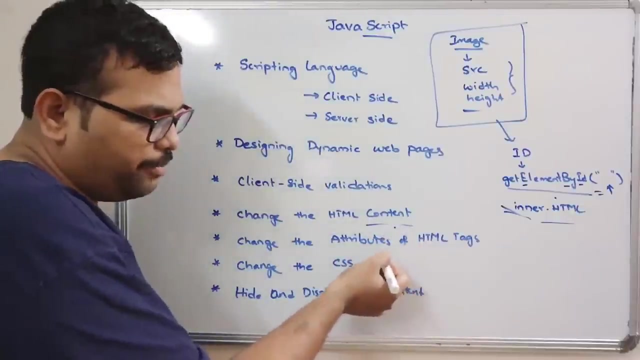 is a function. we are having to get the element. that means here the element is nothing but a tag. okay, for every tag we have to give the ID and from the from this function, we can identify the element and we can change the. I mean the stable content or the attribute or the CSS, whatever it may be, everything. 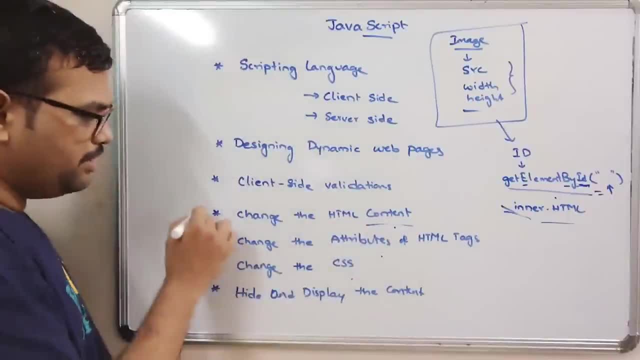 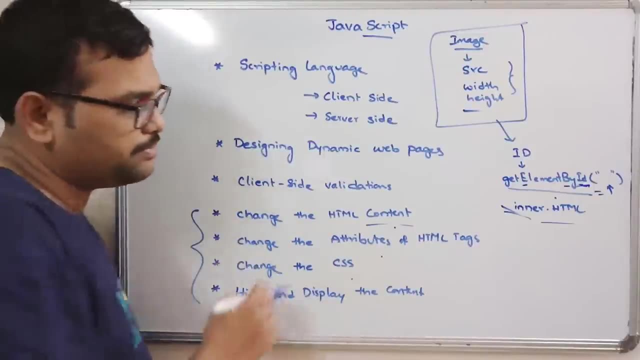 will be happens with the help of the element and we can change the- I mean itself. so I will explain all these things by executing a small code. okay, and write some small code, HTML code, and we'll explain so how the content has been changed and how the attributes of HTML tags have been changed and how the 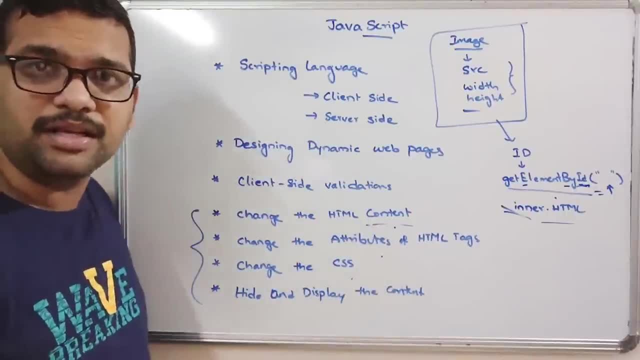 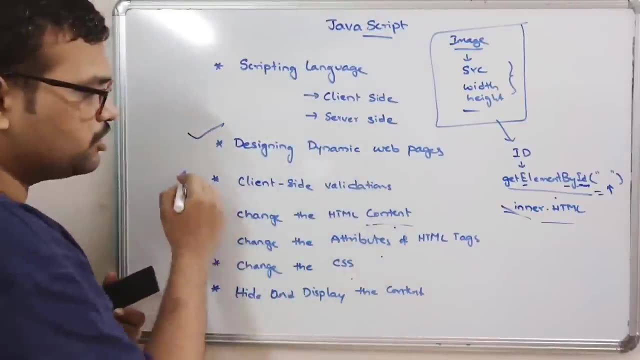 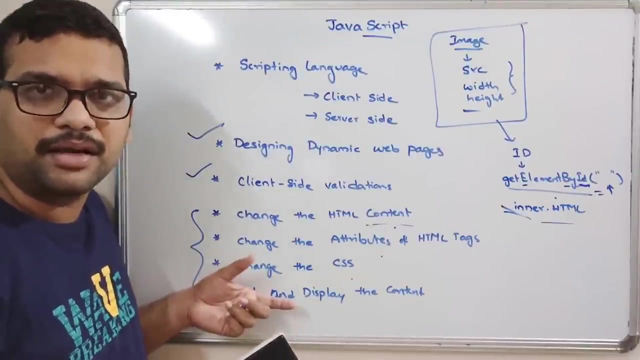 CSS will be changing and how we can hide and display the content. mainly, the JavaScript is used for designing the dynamic web pages and also for the client-side validations and offer. all the manipulations can be done on the HTML content. right, so let us move on to the computer and I. 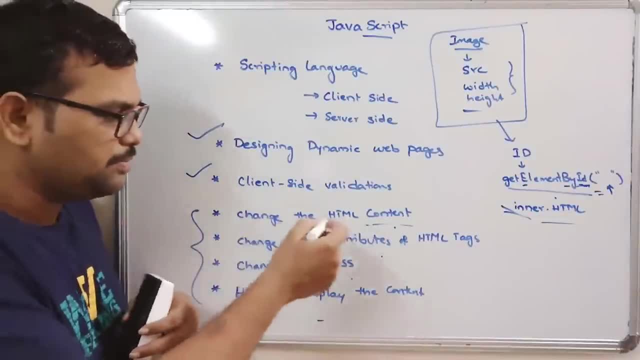 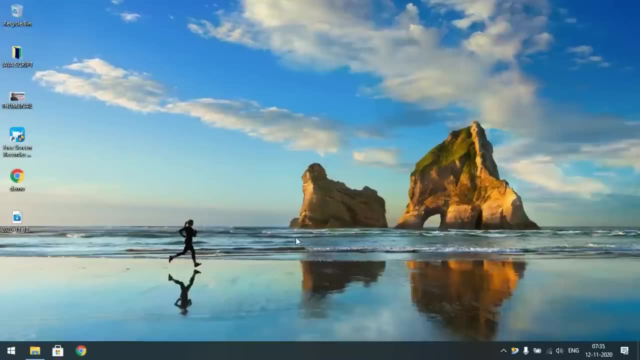 will show you all these things: how, the how the JavaScript will be changing the HTML content and all these things. let's move on to this. hello friends. so just now we have seen, by using the JavaScript, we can change the HTML content or we can change the HTML style properties, or we can change the HTML style properties, and. 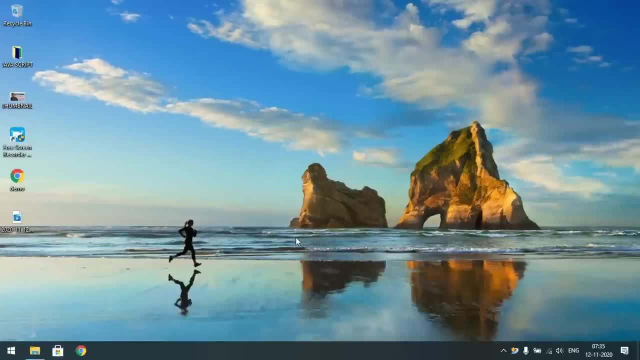 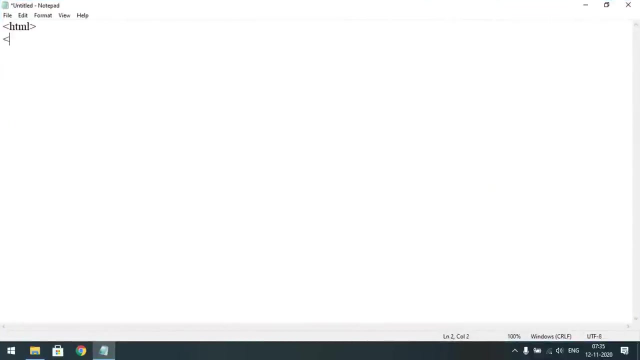 as well as we can change the attributes of HTML tags, as well, as we can display the content or we can hide the content. so all these things we will see by writing a small code. so first let us start with the HTML tag and then go with the body. 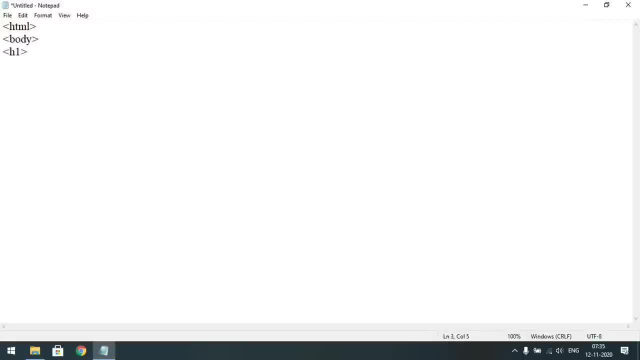 tag and write down some. I will just write down the thing first, one change and the HTML content. so first we will see the how, the how the JavaScript is used to change the HTML content. now let us write some HTML code. I'm sorry, I mean some text. okay, hello guest. 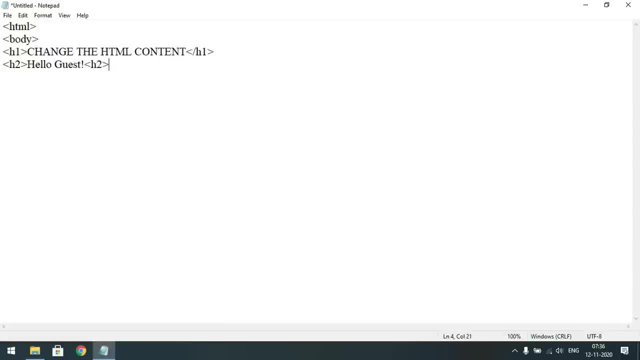 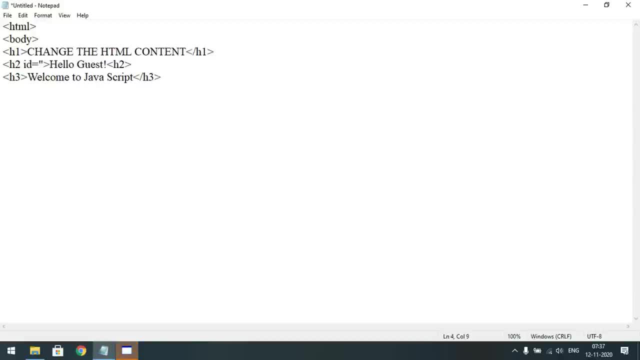 so I will go, I will give some ID. h2 ID is equal to. H2 ID is equal to, yeah, some H content. okay, it is equal to some H content. and now I have to get the ID and we have to change it. so we'll create some button. button type is equal. 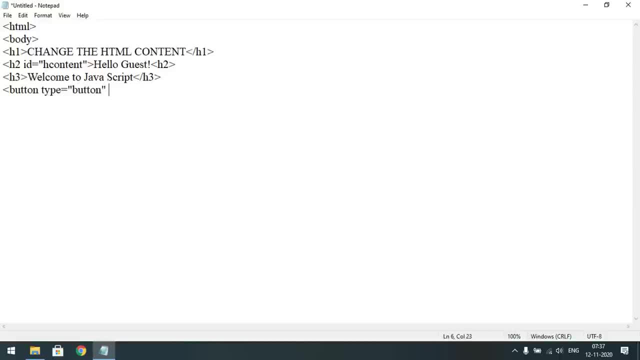 to button and on click. so after clicking on the button, what part should be done? document dot. get element ID. get element by ID and give the ID here: H content dot. how to change the HTML content. so use the attribute inner HTML. okay, change the content inner HTML. so by using that inner HTML we can change the content. 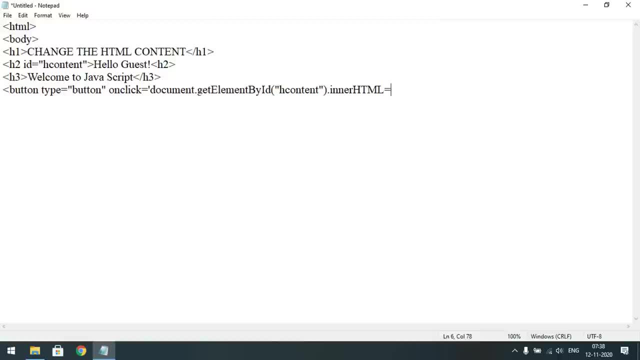 right and what we have to change. so I just want to change it as hello something. yeah, so I'm giving some name to the button. okay, I'm giving some name to the button. now I will create a one more button here and I will change some Faraday, but also I will go with the same thing. so two buttons I'm just creating. 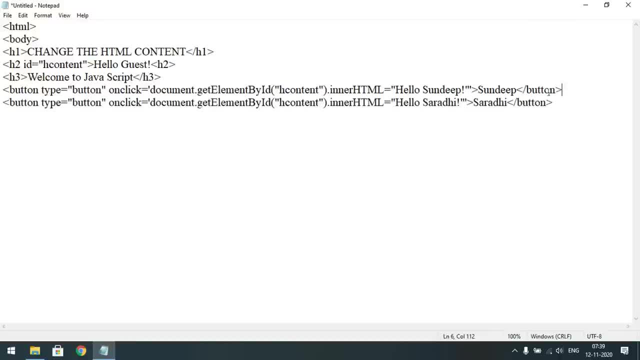 two buttons and with the names of Sandeep and Sardy. whenever I am clicking on the Sandeep, the text will be changed. okay, I will show you. so just close the body tag and close the HTML. right, so this is what we have done, so just save. 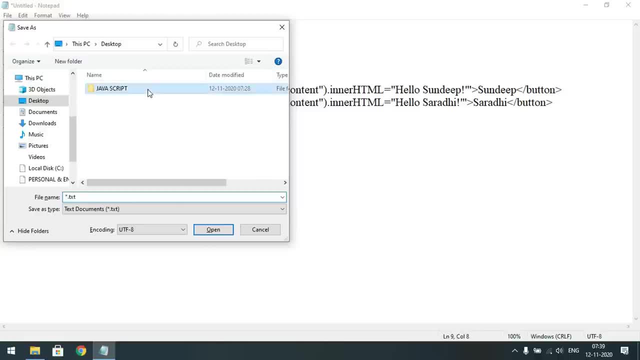 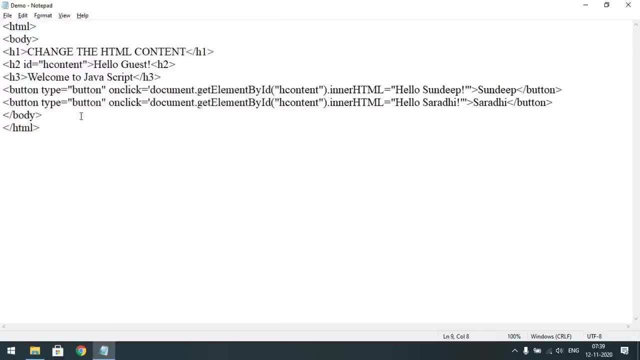 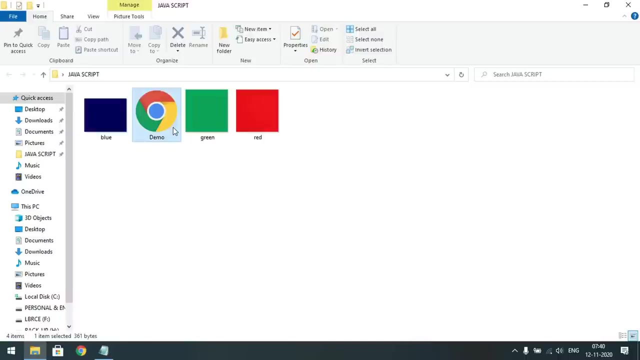 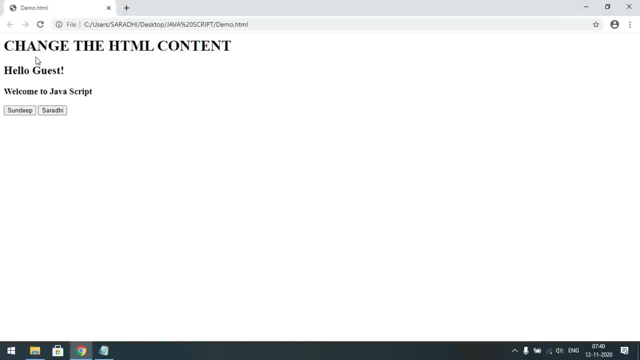 that one. so in the JavaScript, inside the JavaScript, we'll go with the demo dot HTML. okay, see, I will go with the this one. yeah, see, yeah, there is a demo dot HTML. okay, now execute this one. so by double clicking on the web thing we can get. see, you can get here, change the. 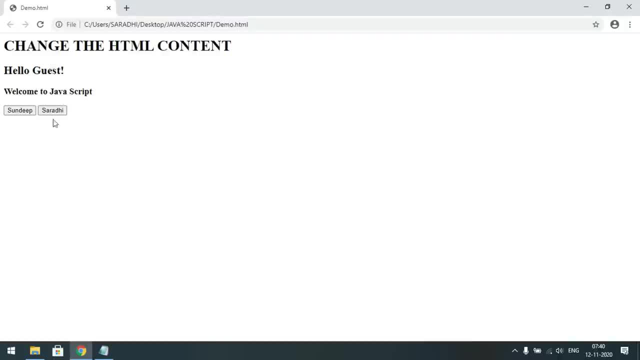 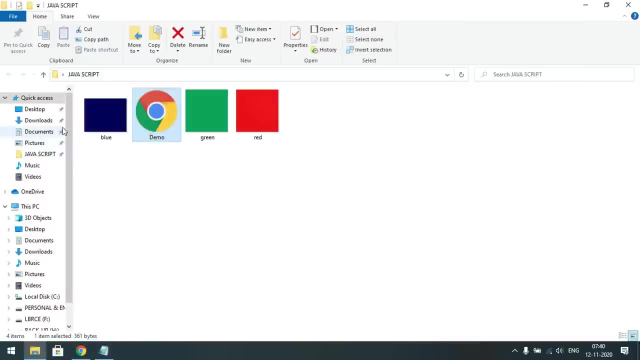 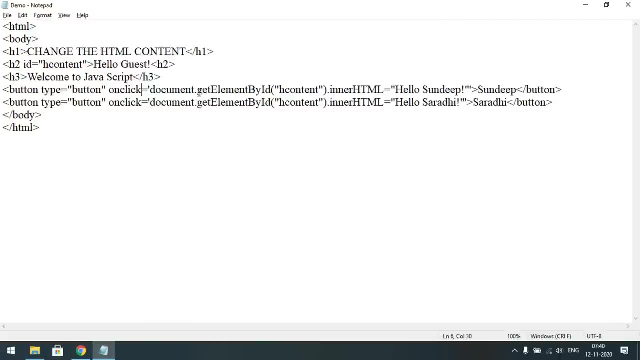 HTML content. that's a normal thing. so hello guest, welcome to JavaScript. so whenever you have created two buttons with one- Sandeep and Sardy- whenever you click on the Sandeep, so what happens here? on click, there is a method called on click and what will happen? that get the element by ID H content. so that means it will. 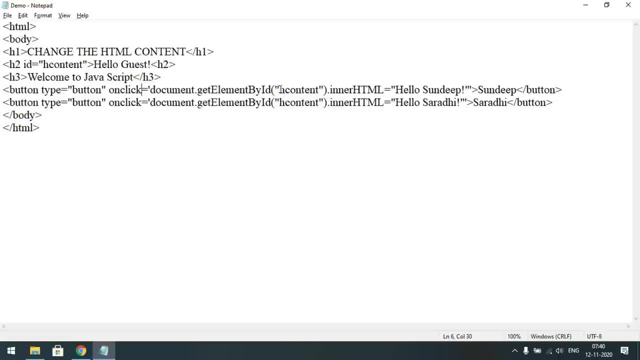 search for the element for which we are giving some H content. so this is the H content dot inner HTML. inner HTML means to change the HTML content. we will use this inner HTML so at the place of H 2, because H 2 is having the ID H content. 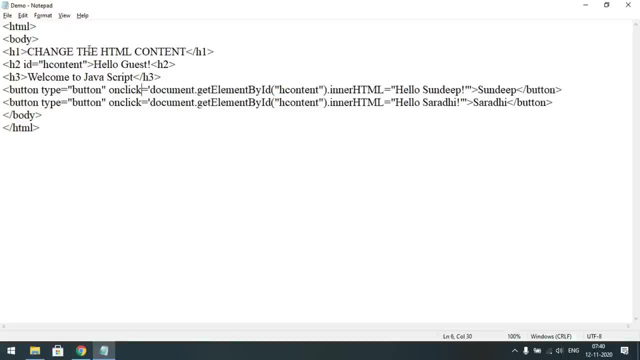 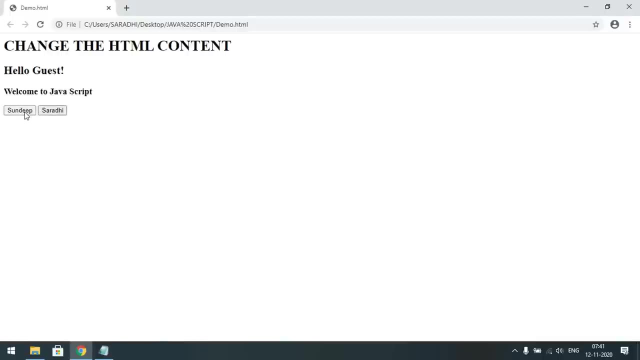 at the place of H 2. we are just changing the text from hello guest to hello Sudeep. then whenever you click on this button, Sudeep, right, so I will show you here. see, so two buttons have been created. if you click on Sandeep, you can observe the text has been changed. if you click on 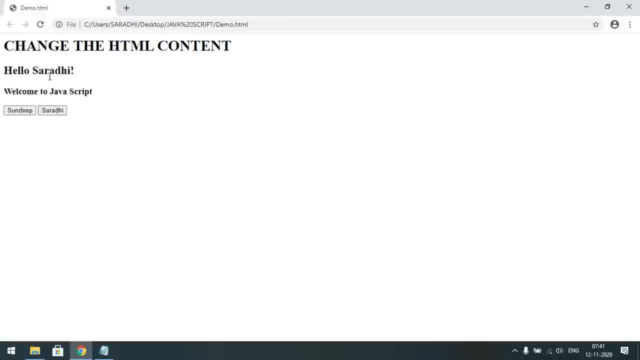 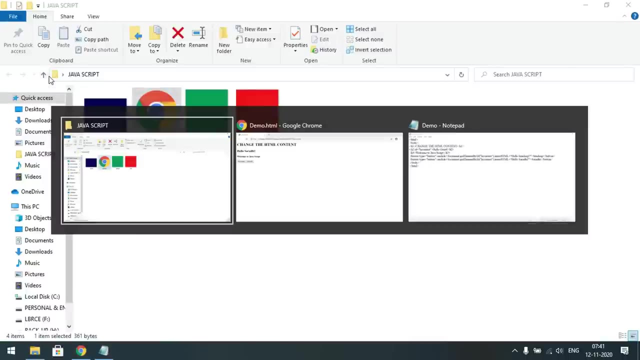 Saturday. the text has been changed, so this is how we can change the HTML content by using the JavaScript, that is, this is on click method and our get element ID and all these things basically belongs to the javascript, right? okay then, this is one thing. okay, this is one thing, and next one is: 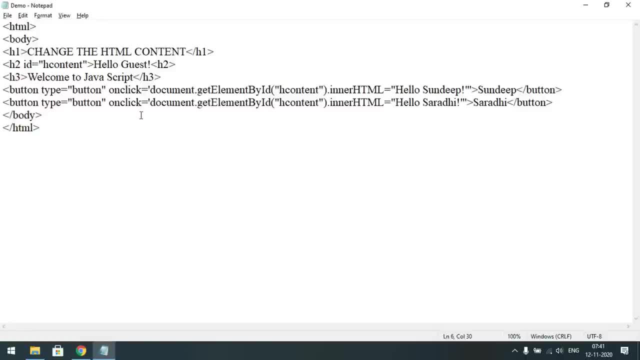 we can change the attributes. we can change the attributes of html content. so, for example, if you consider some image, we are having a lot of attributes like source or height or width, whatever it may be right. so after here also we can change that particular attribute with the. 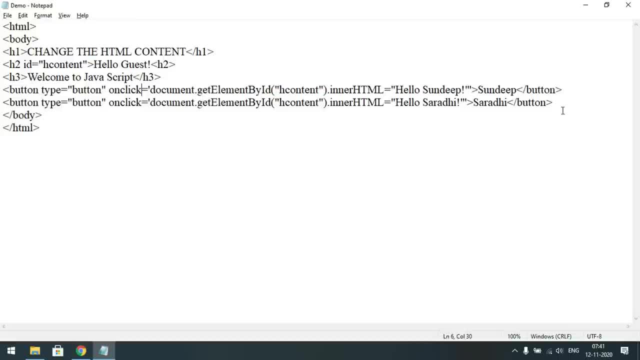 help of this javascript. so we'll see that one. okay, now we'll see that one. and the next category, next one, is h1. so change in attributes. change in attributes. okay, so let us, let us check. so we'll create one image, we'll display one image, okay, so i will go with the image src. sorry, id. 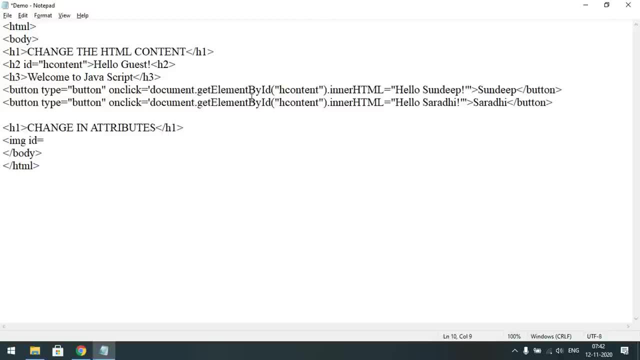 first we have to give the id, because we are using some get element by id. so with the help of that itself we are just applying the changes. so id is equal to image src is equal to. so i have downloaded three images, some blue, green and red, so we'll go with that one. so i think 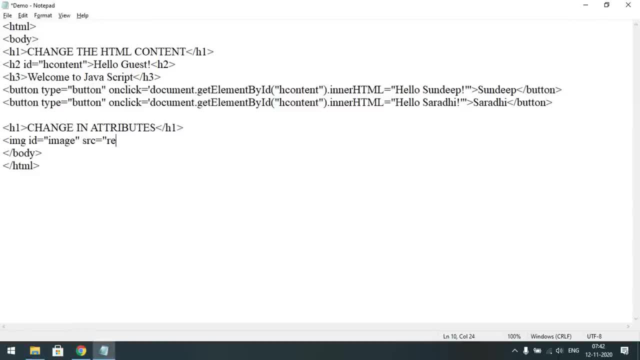 go with a red dot png. red dot png width is equal to some hundred, height is equal to some hundred. okay, yeah, just i have given like this: now use the same thing. i will go with the same thing, same code, but i will change the small changes i. 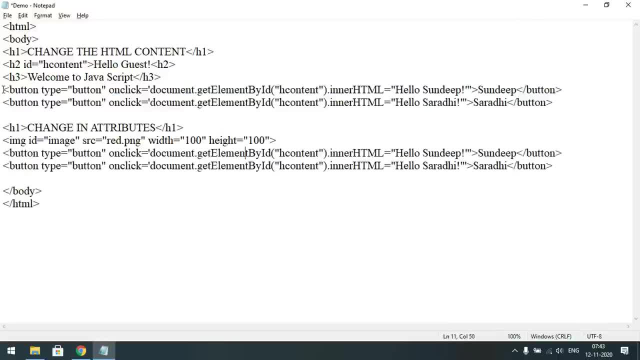 will do the small changes. so button type: one element by id. so change the element id by image. because for the image we are giving some image and here we are not changing the html content, we are just changing the attribute. so we have to give the attribute, so src is equal to. so just go with the path where which image we have to go. so green dot. 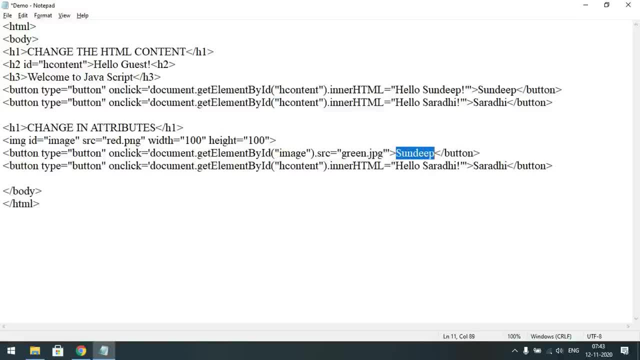 jpg and similarly green, and here also we have to go with the same thing. so remove the src, remove the inner html, give the attribute which you want to change and, instead of giving then this one, go with the blue dot jpg and give the name for the button. 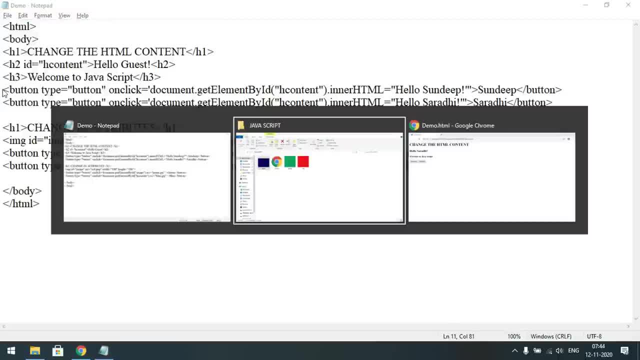 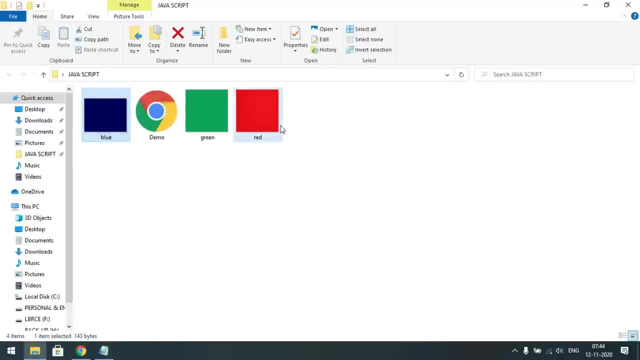 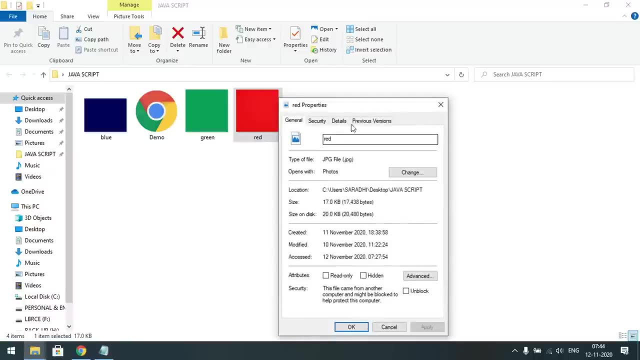 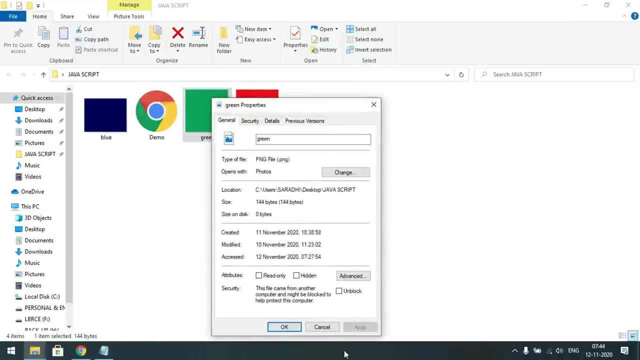 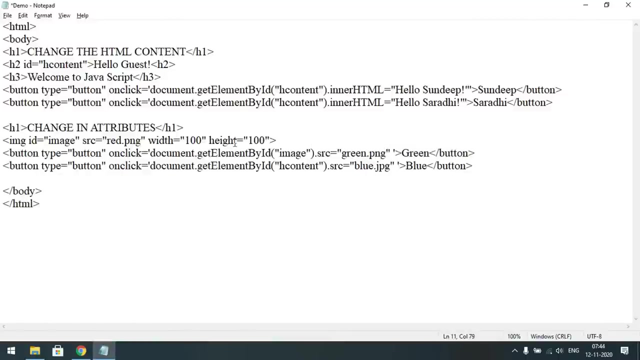 yeah, now, let us check. let us check. implement this one refresh. so i think the extension is not correct. let us check. yeah, red dot jpg. and i remember one. one color is of png. yeah, green is of png, right, let us check. so green dot png and red dot. 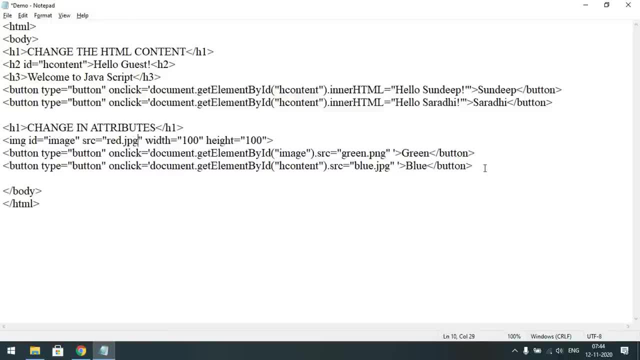 jpg, and also we will use some uh, the third, uh, third button. okay, third button, so third button is of also. yeah, here also we have not changed the content, right? so image, and here also we have to go with the image and red dot jpg, right, okay, and use some break lines. so it will be. 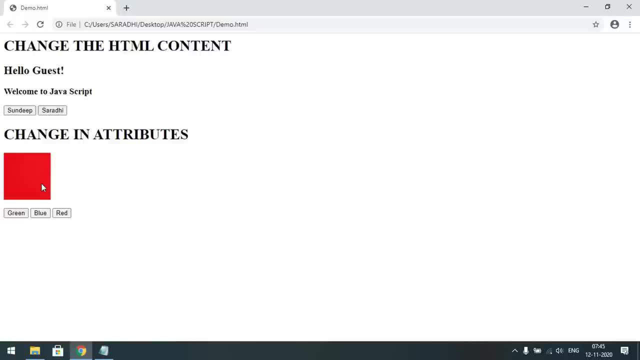 yeah, see, you can use the second thing. second category, that means changing the attributes by using the javascript. so here you can observe, we have given some image, we have displayed some image and we have created some three buttons with the different colors and if you change this one, if you click on this one by on click, it will get the ID of this. 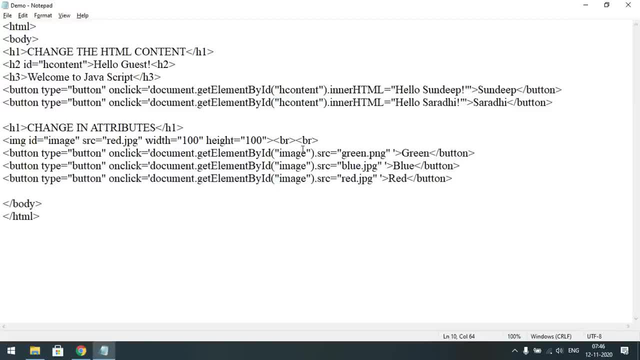 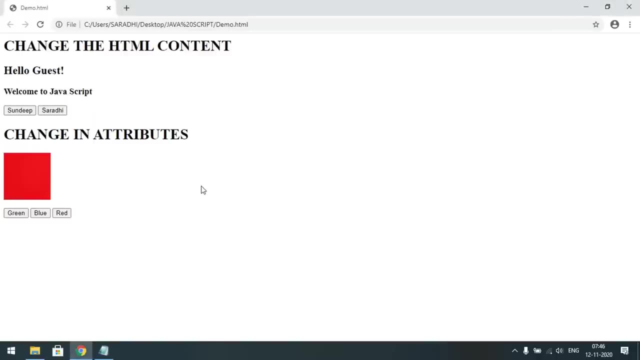 image tag. so here we have given some image image tag and dot SRC. that means the source will be changing. source will be changed to green whenever you click on the green button. source will be changed to blue dot GPG whenever you click on this blue button. okay, see, let us say so. I am clicking on the green. 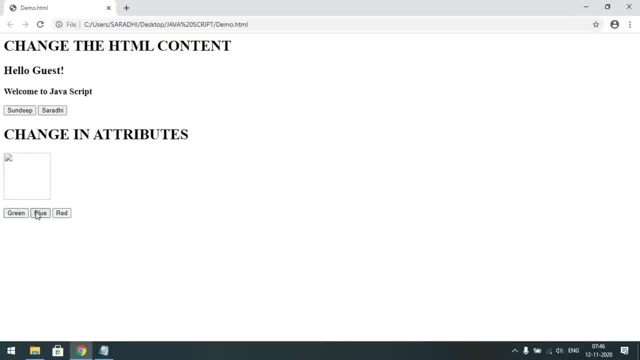 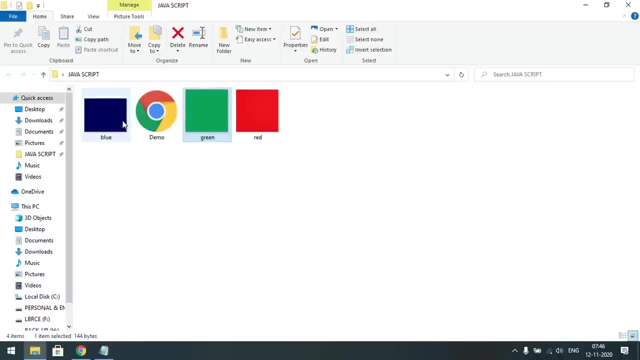 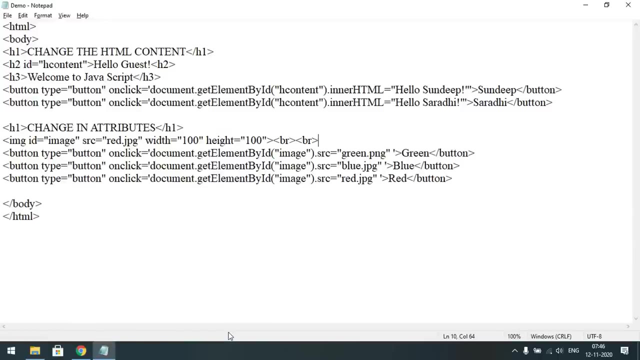 button, you can observe the green color appeared. if you click on the blue button, blue appears. okay, sorry, I think so it is also of PNG. okay, so the extension. it's a problem of it, the extension, but it doesn't. I mean there is no problem with the code. okay, yeah, you see, you can observe blue red. 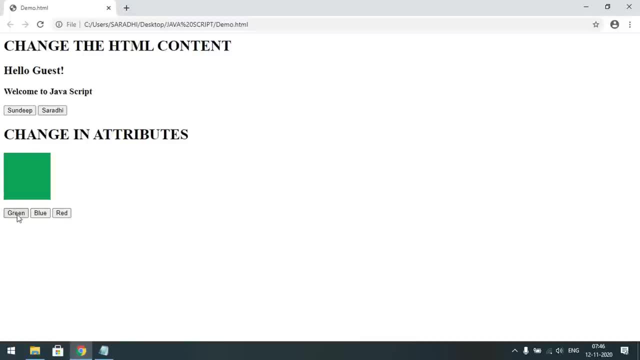 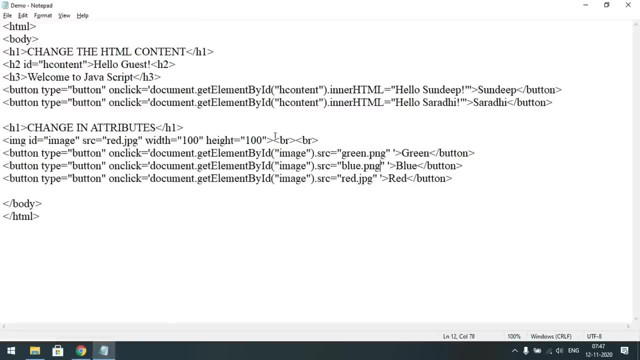 green. so like that, we can change the source of the attribute. okay, we can also change the attributes, attributes of the HTML, see. so sorry, so we will go with the third one, that is, we can also change the CSS properties. we can also change the CSS properties: see change in CSS right. 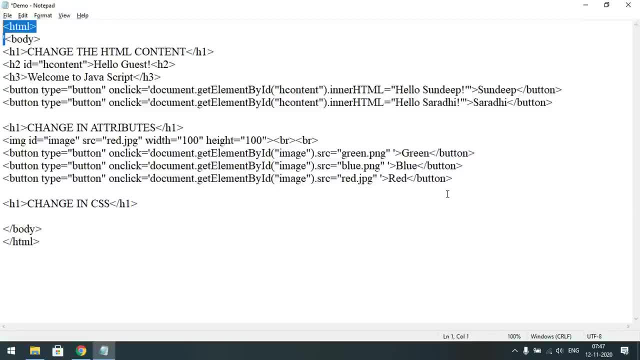 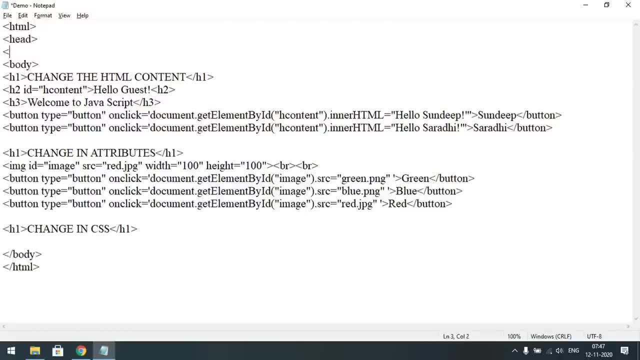 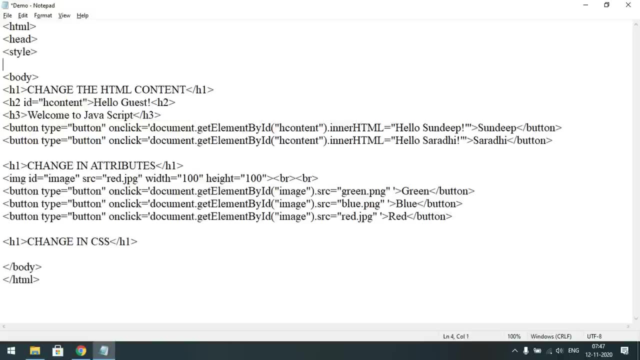 so we'll: first we'll decide one property, okay, one one CSS. okay, for that we have go to with head and then in the head. so we will go with the style property will decide some style initially, so give the ID. so in order to access the ID, we have to prefix with the hash symbol. okay, text. 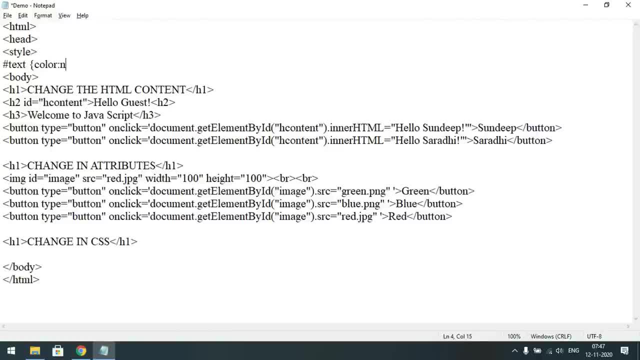 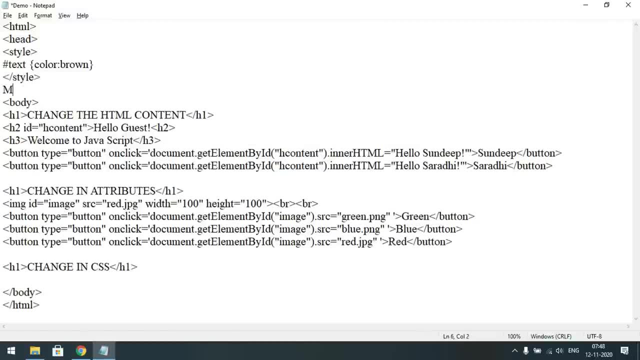 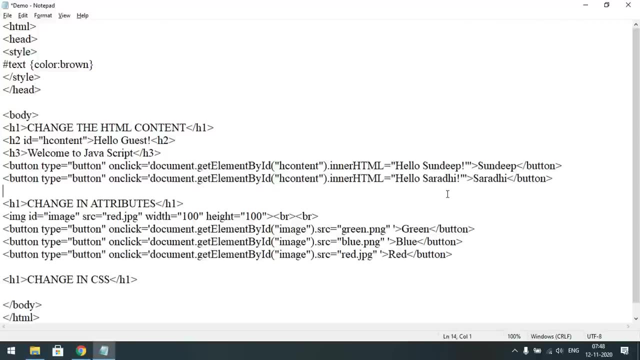 color brown. close the style head. okay, now we will create one text. okay, we can create one text. H 2- see, ID is equal to some text because here ID, we have given some text and write some text. so I'm closing the H 2 and again same use, the same thing. so we'll change the. 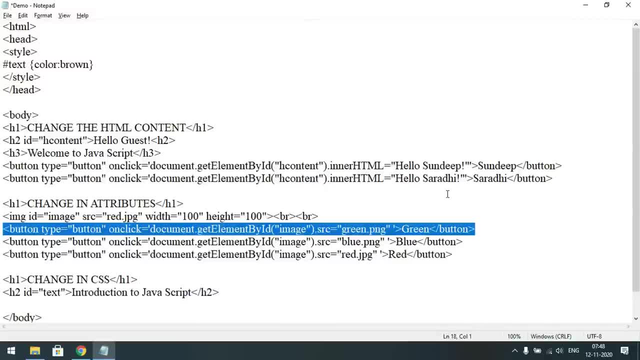 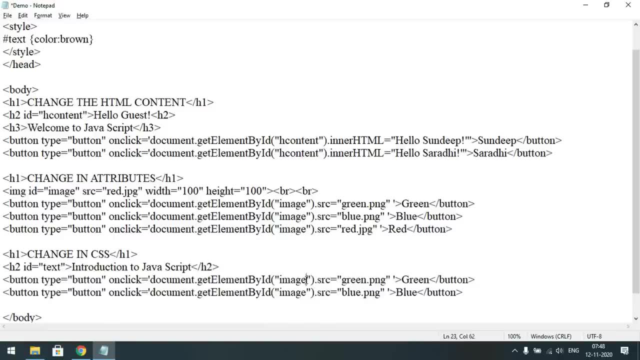 color change. we'll change the color, but here instead of image we have to give the one and two ID some text. here also we have to give the ID some text. and here it's not a source, it's a style property. so style dot font is equal to give the color. okay. 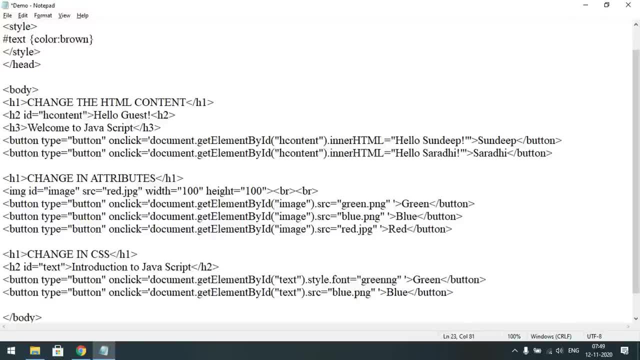 give the color. similarly, we have a single- uh, we have- works page which has a- although you see, I hope nobody is asking her, yes, yes, it's just our hers only one has been changed, and then we will give him a task and then. ok, so that's all. instead of digital layout. 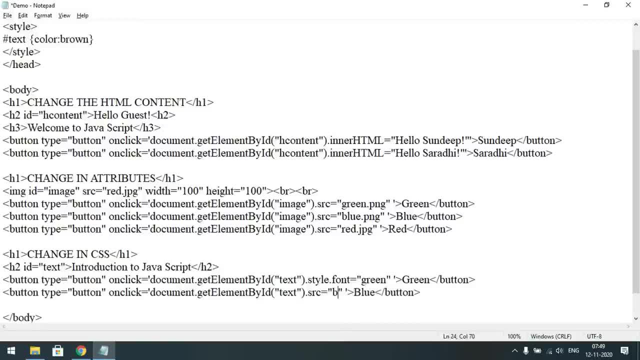 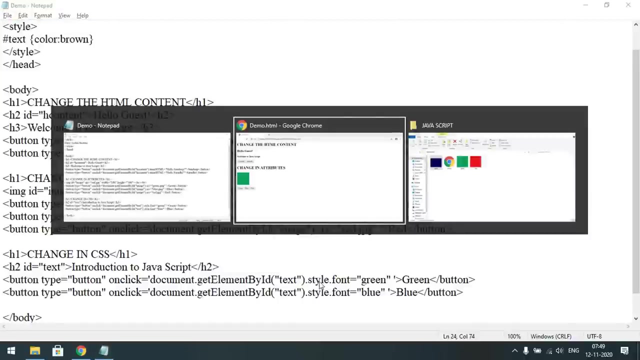 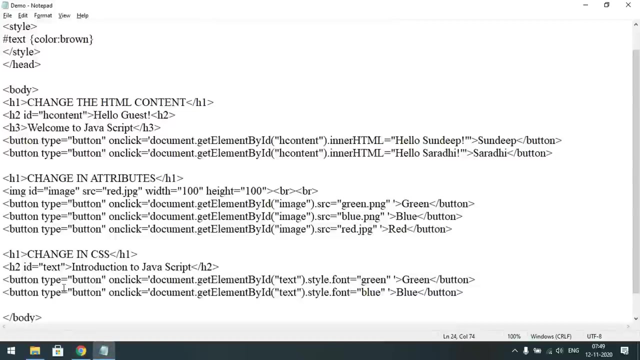 here also go with style dot font is equal to blue color. blue color- okay, one is a green, another one is blue. now we are changing the style property style- css style. okay, so let us check see, initially it was some brown brown color. okay, initially it was brown color because 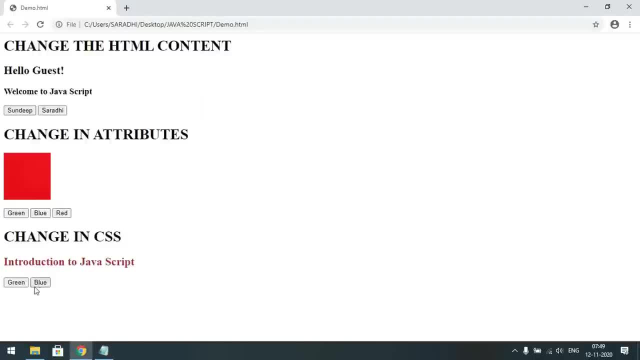 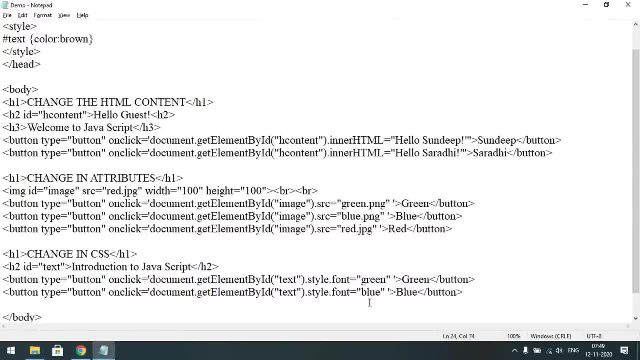 here we have given some brown right and we have created two buttons: green and blue. if you click on this green button, okay, it have to change the this one, right? so sorry, it's not a font, it's a color. however, we are changing the color, right. we are changing the color, not a font. 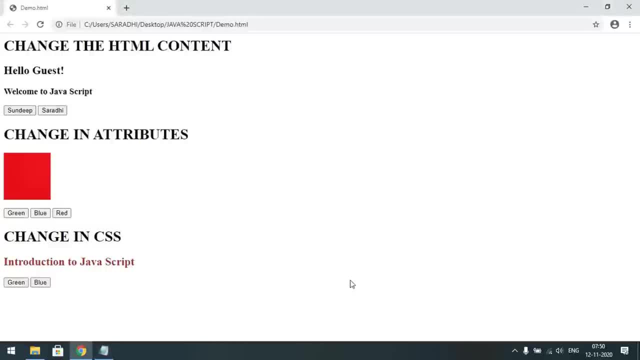 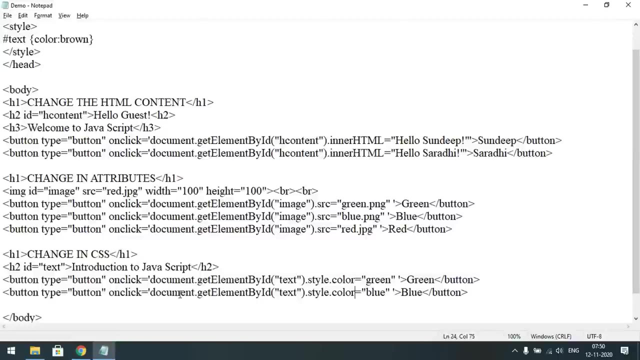 okay, sorry. yeah, you can observe. if you click on this green button, the text color has been changed. if you click on this blue button, the text has been changed. right, so like this, we can change the property of css. okay, we can change not only the color, whatever the property we are, we are. 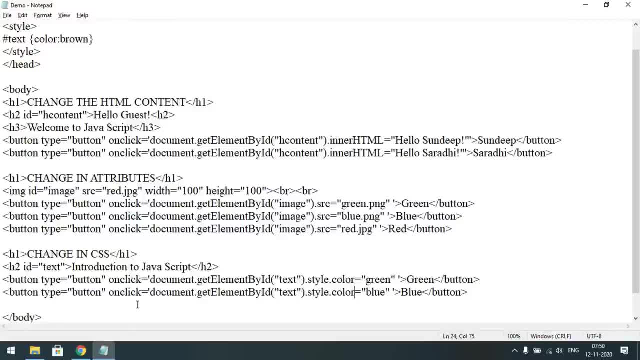 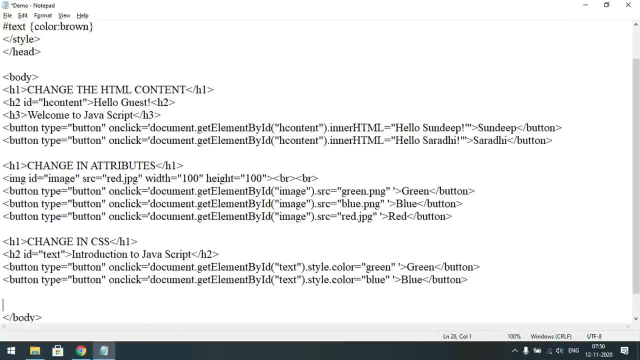 supposed to change. we have to give that in the place of here. okay, style dot. color style dot. font style dot. font family. so like this, we can give and we can change the css styles. right, and one more thing, the next one: we can also hide the elements and how we can also display the. 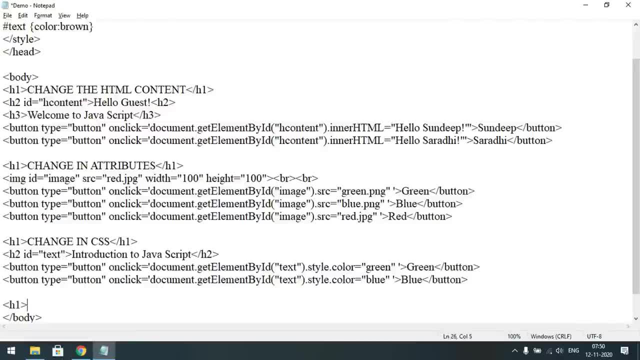 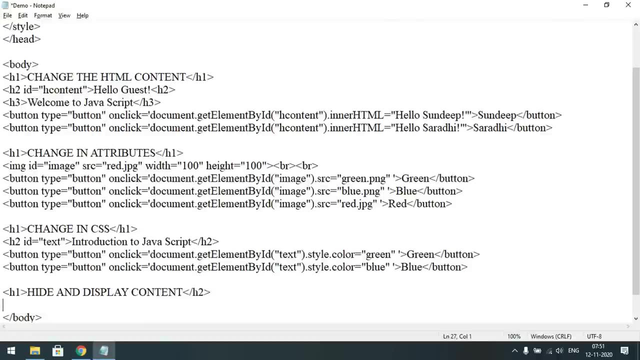 elements. so we'll see that one. okay. so h1: hide and display content. okay, hide and display the content. sorry, h1, right now we'll go with the some small text. okay, we'll. again, we'll take small text. so this is: this will demonstrate hiding and displaying content. okay, so here we have to give id. okay, i have forget it, right. 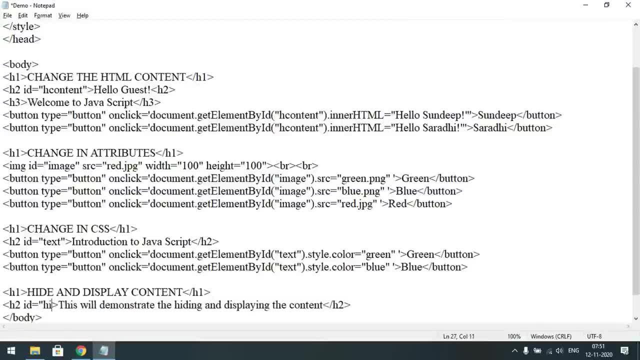 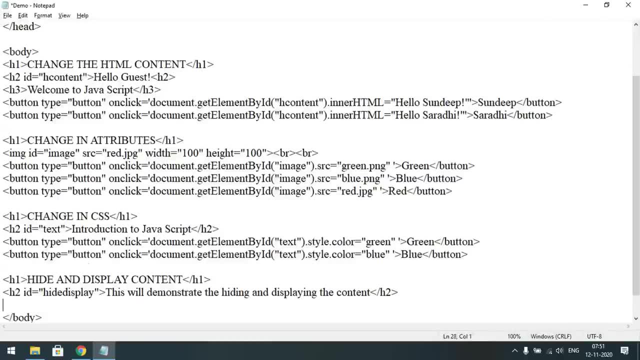 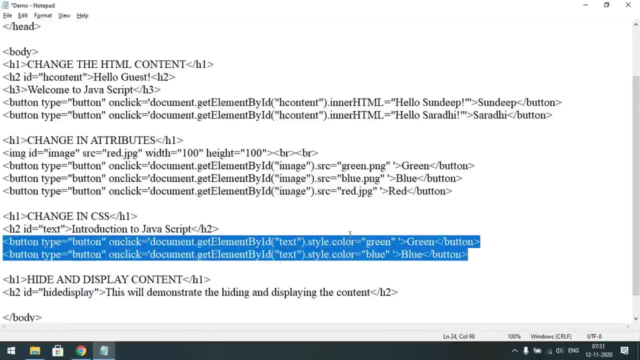 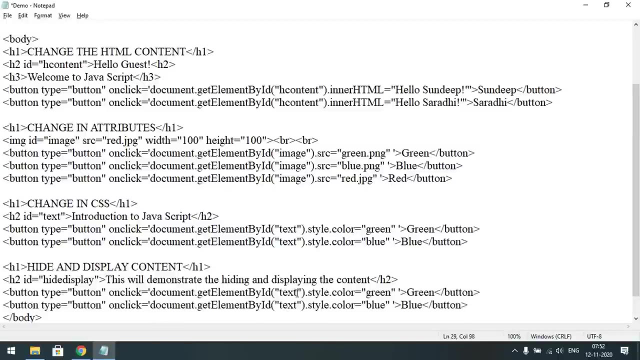 id is equal to h- hide display. okay, let us take this one. yeah, now again i will change. i will use this one. the same thing. so here element id is hide display and here also i will change it first because i will forget. okay, hide display, and then 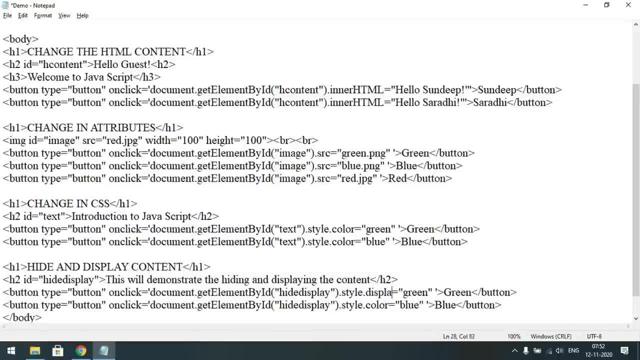 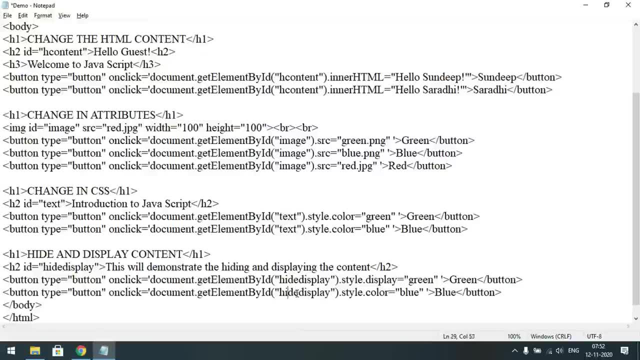 instead of color we have to go with the display, style dot display, and here also it is a style dot display. it's a small attribute. okay, style dot display is one attribute. so if you give here none, automatically it will be hiding. okay, see hide, and here display. and here if you use a block, if you use block, okay, then it implies it, so that there is 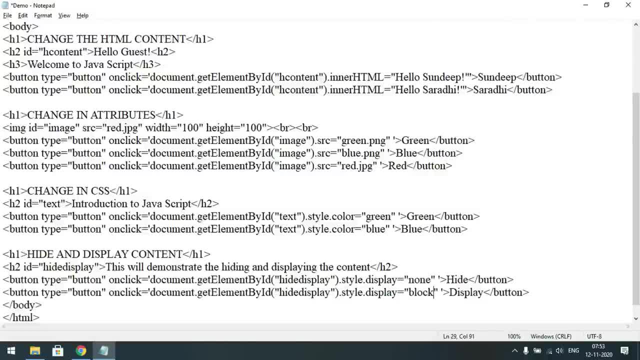 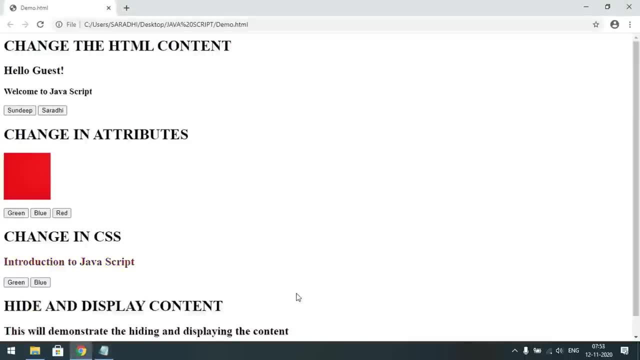 an value for the attribute called display. okay. style dot display is equal to none means the content will be hiding, okay. and the style dot display is equal to block means the display will be. I mean, the content will be displayed in block. I will show you so you can observe here. so we have created two buttons: hide and display. if 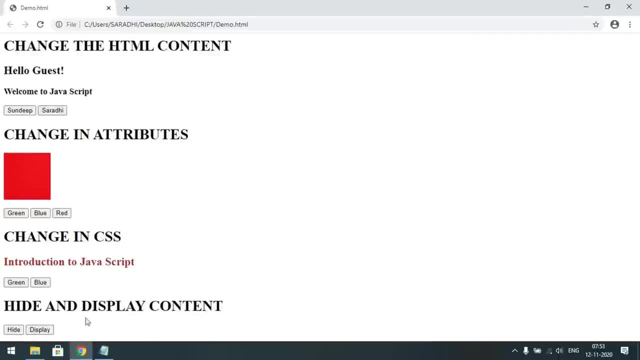 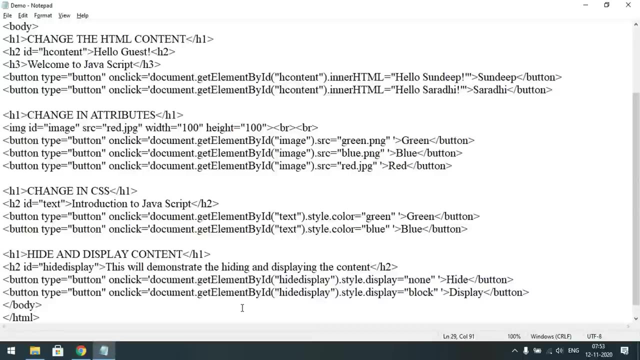 you click on this hide, you can observe the content has been hide it. okay, you can't visible this content. if you click on this display, the content is appeared, right, okay, so this is the things we can easily do with the help of a JavaScript right. the main things we can change the HTML contents. 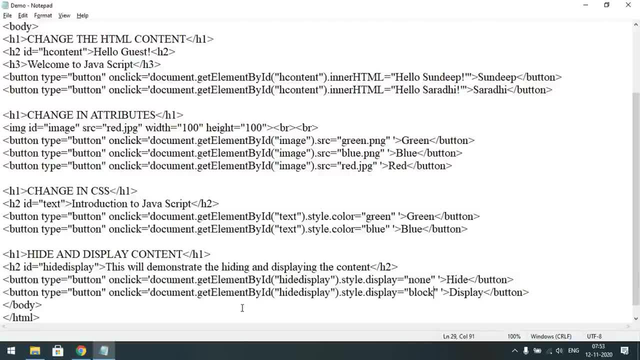 and attributes and CSS- what not so? and also we can create the dynamic web pages using the JavaScript. so here just, we are using some. on click attribute is as well as in that on clicked attribute, we are just retrieving the ID. retrieving the ID and again we are changing the either property or a. 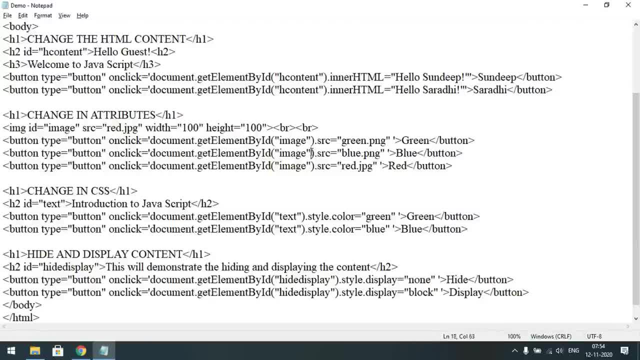 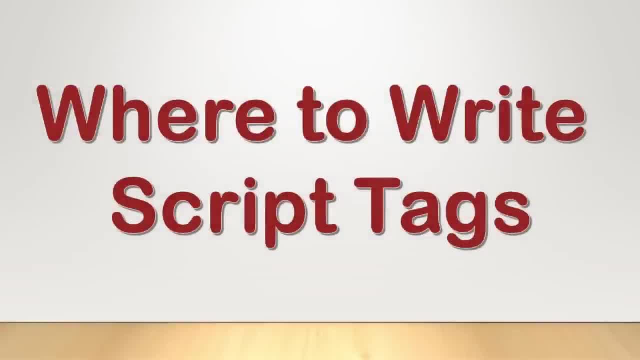 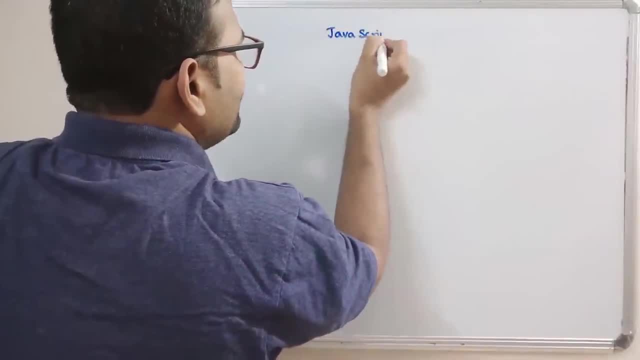 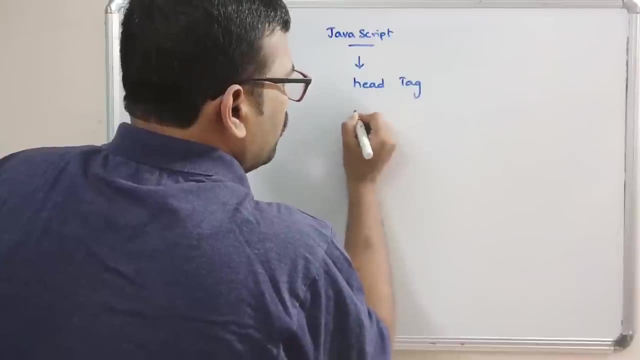 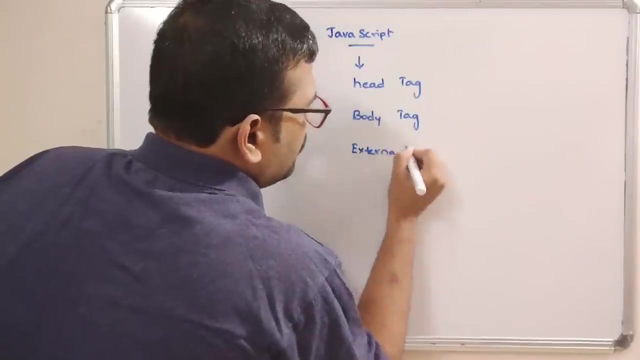 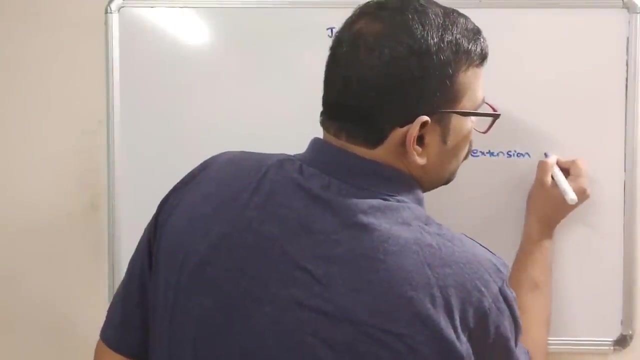 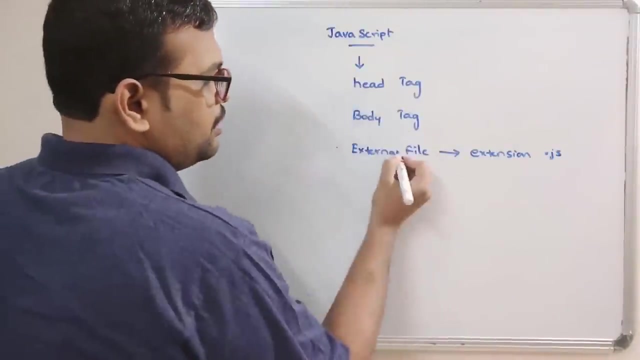 content or any CSS right. this is a simple thing, so hope you understood all you, all these things. so so this JavaScript can be written in happy tag in including in internal file. if you want, you can include any external file with an extension with an extension dot j. yes, it can extension dot j. yes, and if you, 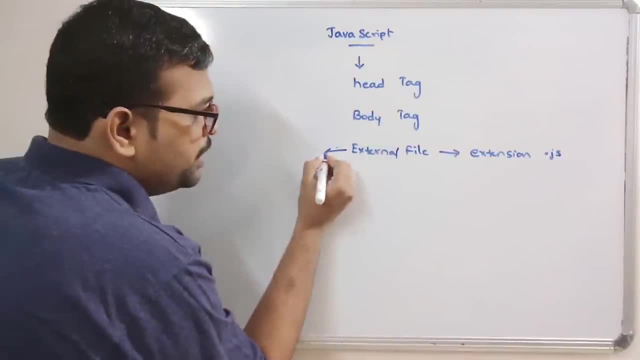 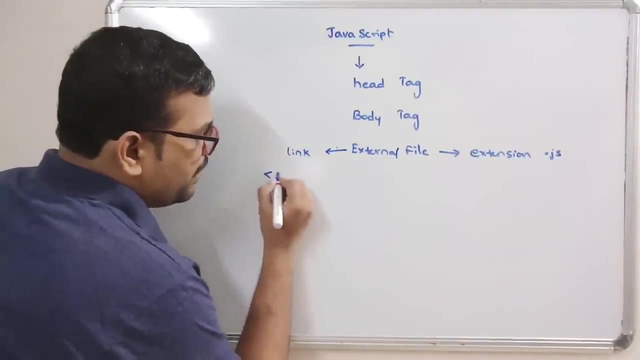 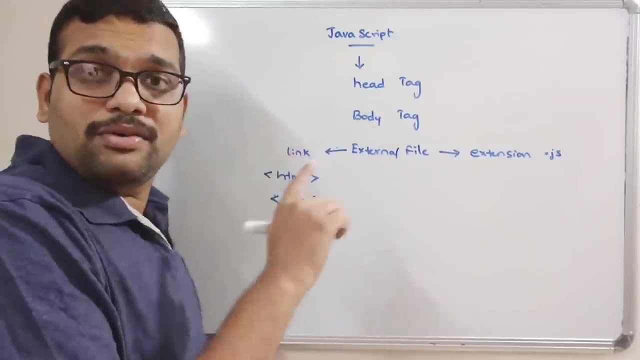 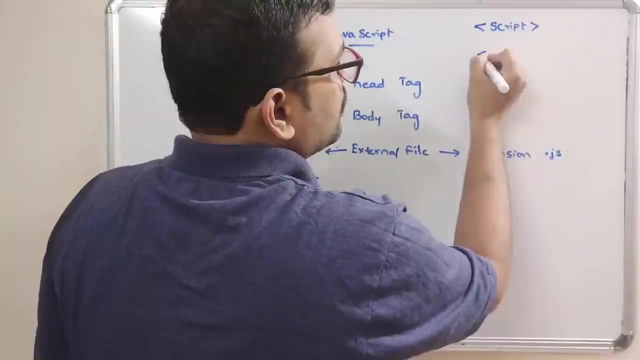 are writing this JavaScript in a my external file. this should be linked to the our HTML content. so, for example, you can write here HTML and then you can write the head tag and all the scripting. so, whatever the scripting we are writing, everything should be written in between the tags called script. okay, so in. 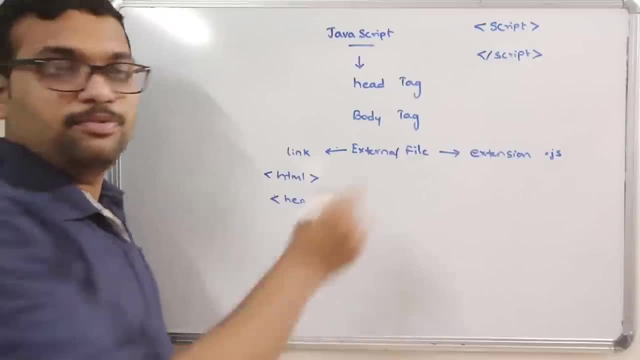 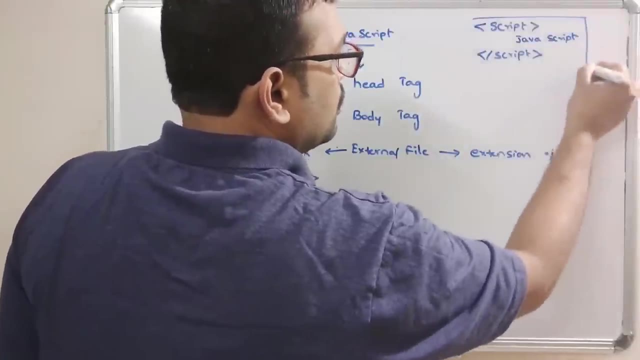 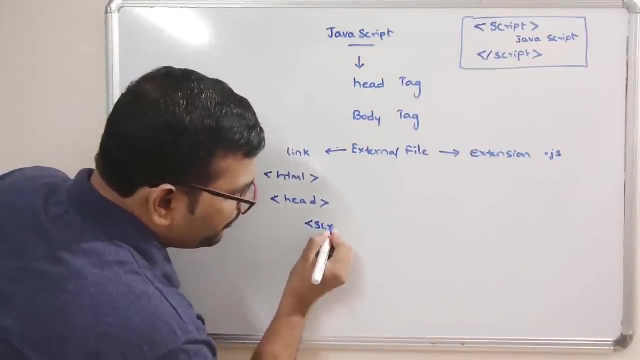 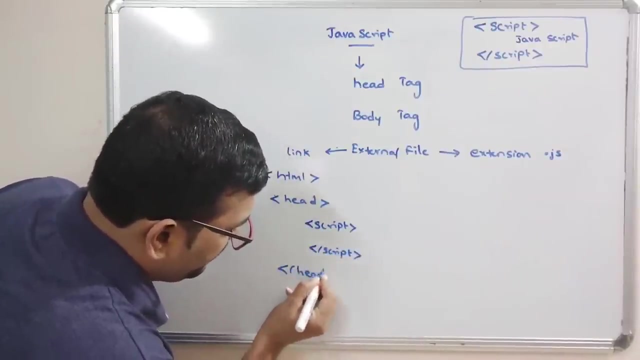 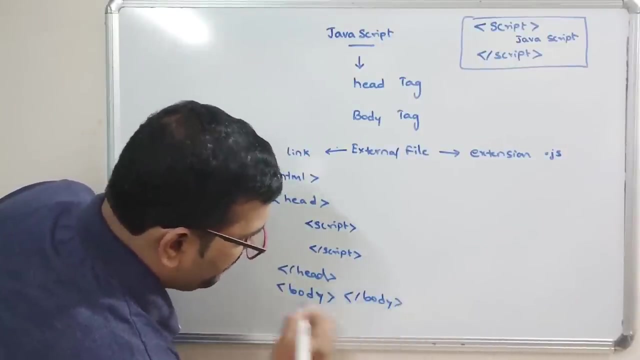 between these tags. we have to write the JavaScript which we want to return. okay, JavaScript should be written here. and this block, this block. that means this scripting block should be included either in the head tag, so in the head tag, see body and close the body. close the HTML. 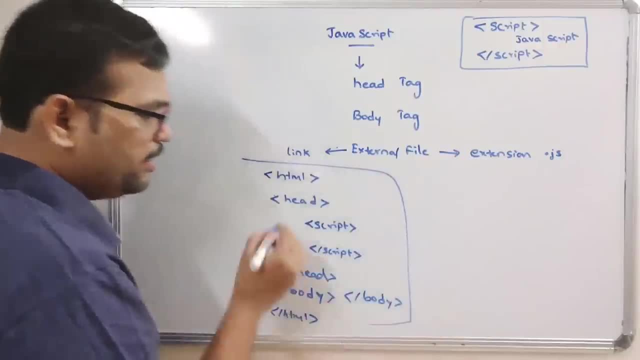 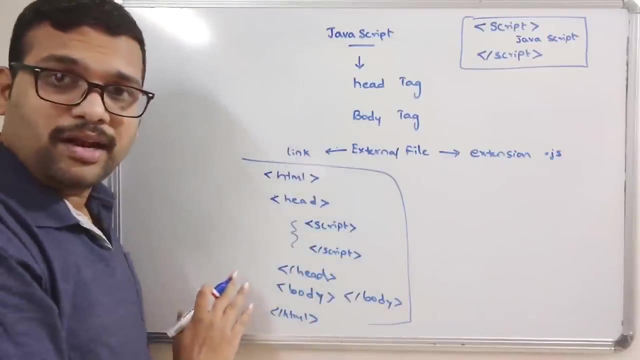 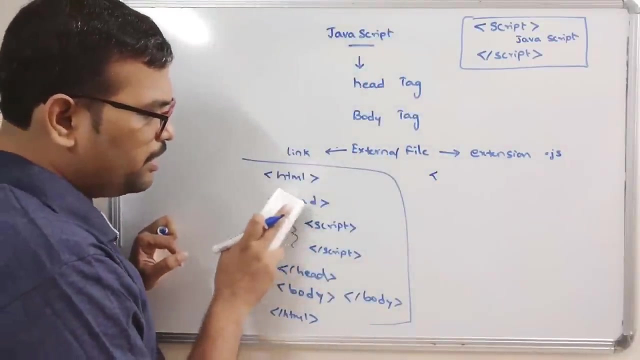 so this is the HTML content. this is the thing we can write. that means we are including this script block in head tag. so, similarly, whatever the thing we are writing, that can also be written in body tag. that means see instead of writing here, instead of writing here. 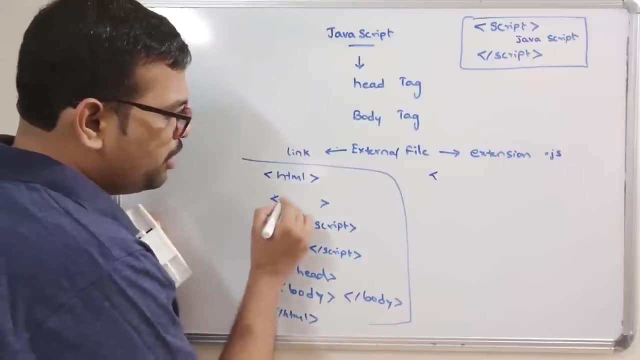 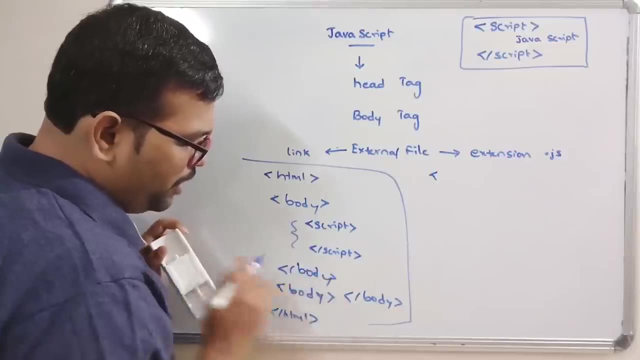 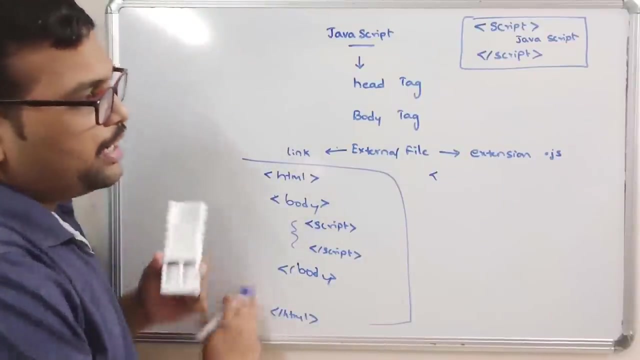 directly we can go to the body and in the inside the body we can write the script right. so close the head and go to the body and we did not write right here, so is also can be written. this is also can be written. and coming to the external, 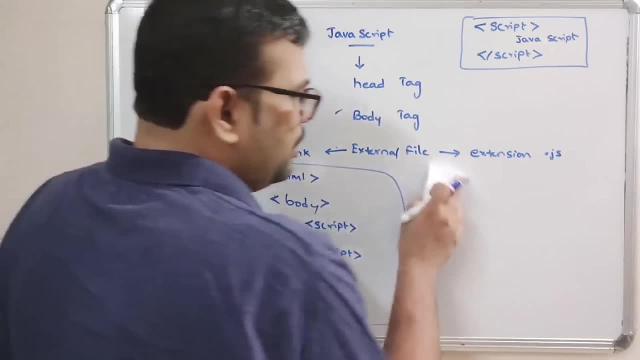 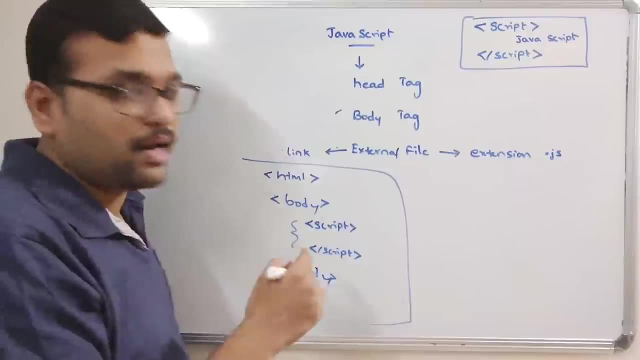 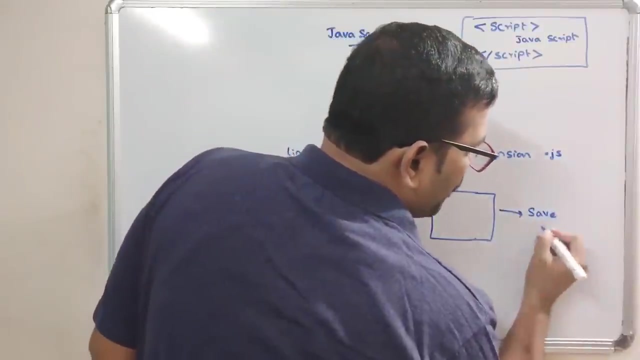 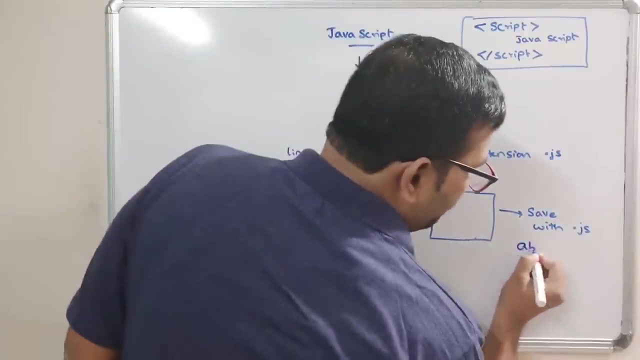 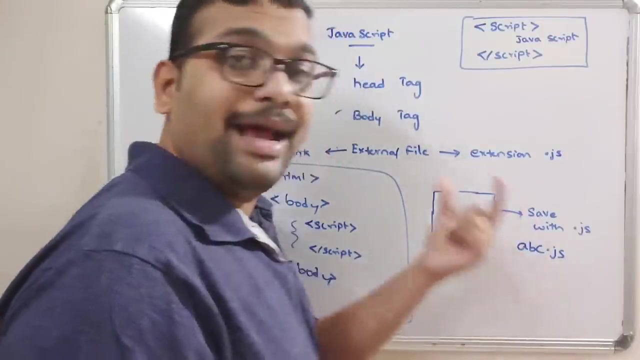 file. so this is a body type. and coming to the external file, take one notepad and give all the scripting. so, whatever the scripting, we are writing everything. write in a separate new file and sell this one with dot JS, dot JS. let it be some ABC dot J. yes, let ABC dot JavaScript. and I have to include, or how. 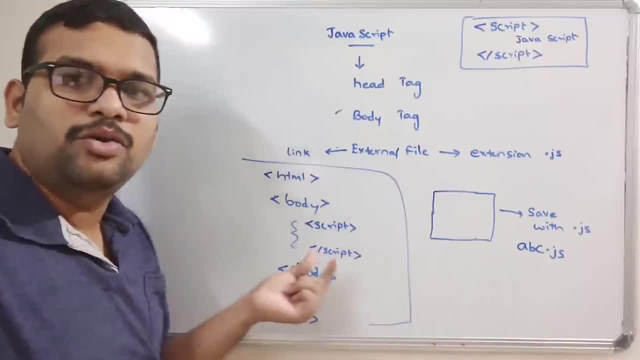 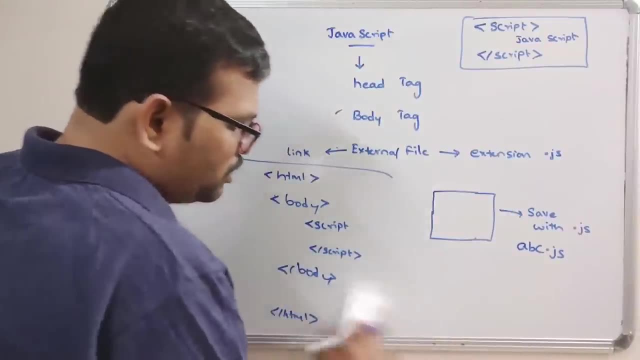 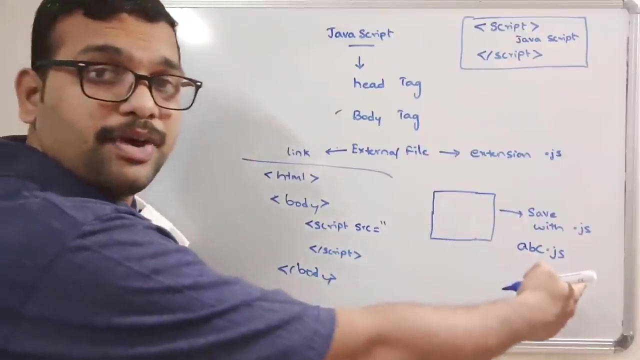 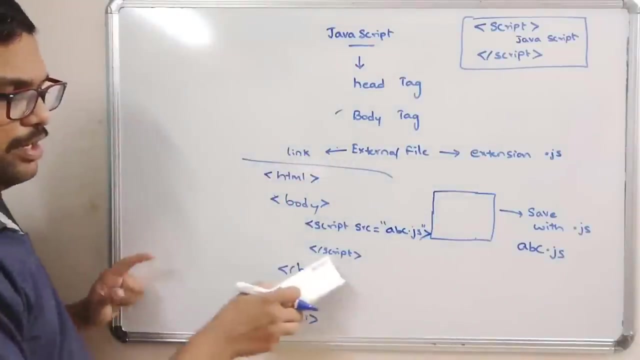 to link the external JavaScript file into our cage to my content, and this should be done in excess. so script, and then is an interview called source Script. SRC is equal to use a location where this, exactly this JavaScript file, exactly located: 87 c dot. close this one. simply close the java script automatically whenever the script is implemented. 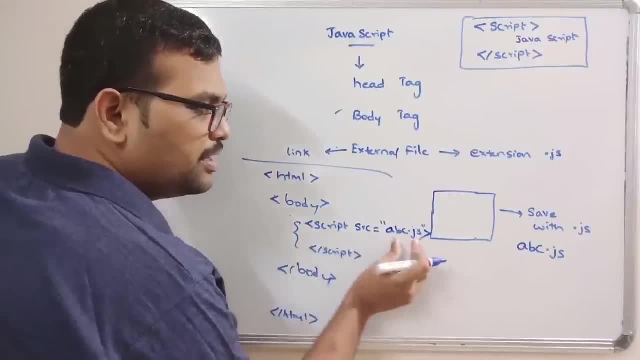 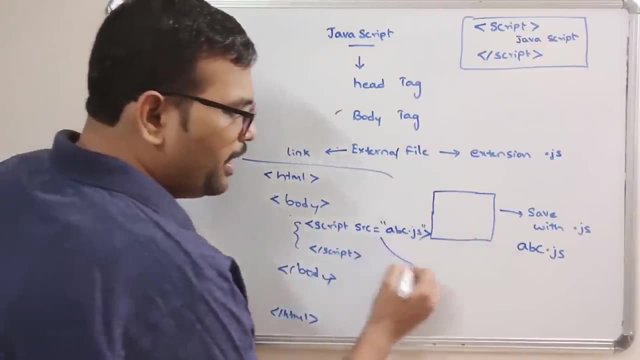 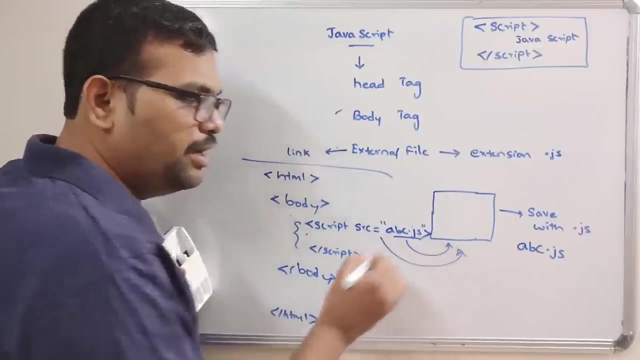 that whatever the scripting is done in this abcjs that will be implemented here, that will be executed. okay, directly, it will be redirected to the external file. whenever the scripting is executed, this abcjs will be redirected. okay, so this is how we can link the external js. 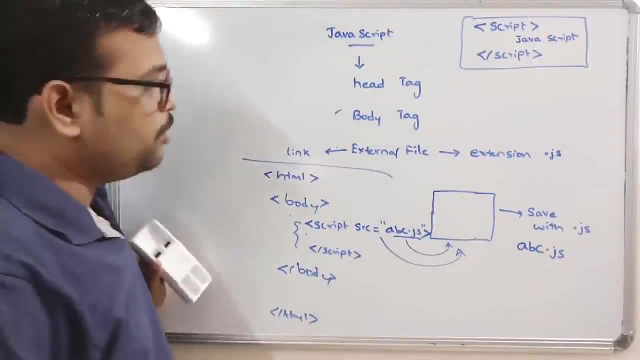 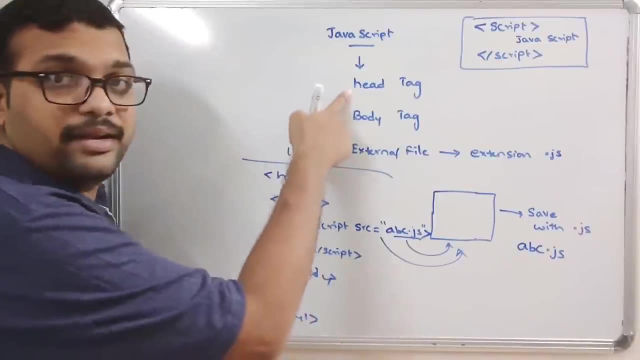 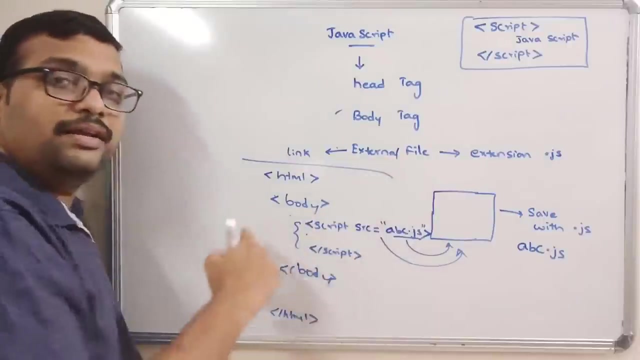 into our html content. so, no problem, i will execute a small html code demonstrating writing this script, script block, inside the head tag, inside the body tag, and also- i will explain so- writing the external file and linking this external file into our html content. right, so let us move on to the system i will demonstrate there. 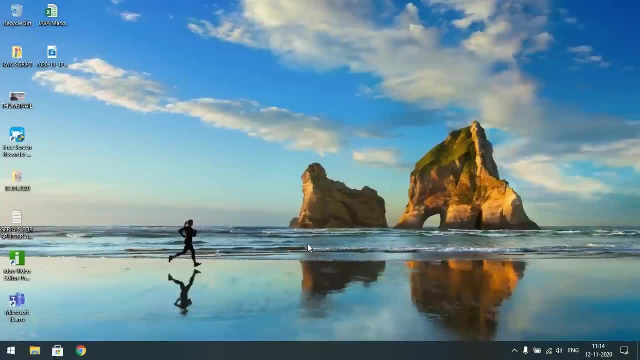 hello friends. so just now we have seen where we have to write this string scripting. so all this scripting can be written in either head tag or a body tag, or also we can write this scripting in an external javascript and we can link that file to the html content. 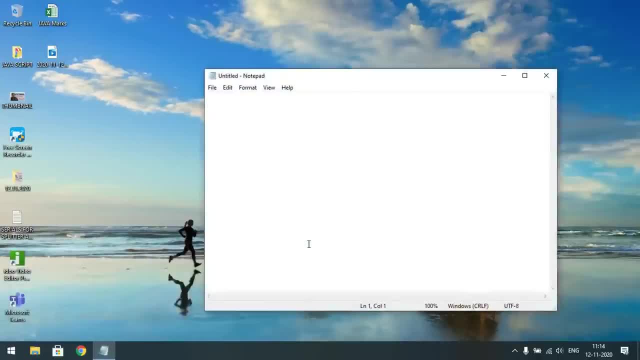 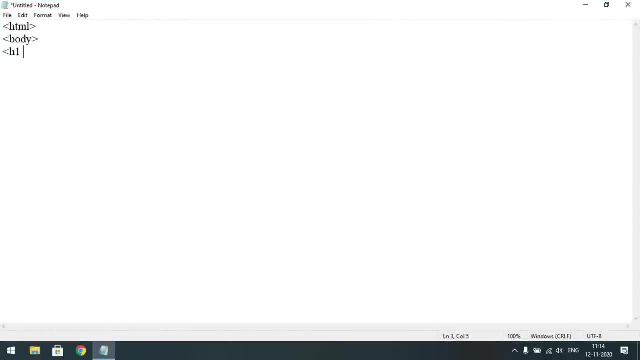 and we will see all these things by implementing a small code. so first let us write the html code, and in the html code first i will write the body and then we will go with the scripting. so h1 id is equal to, so i will give some id, some display, ok, and i will write some text. 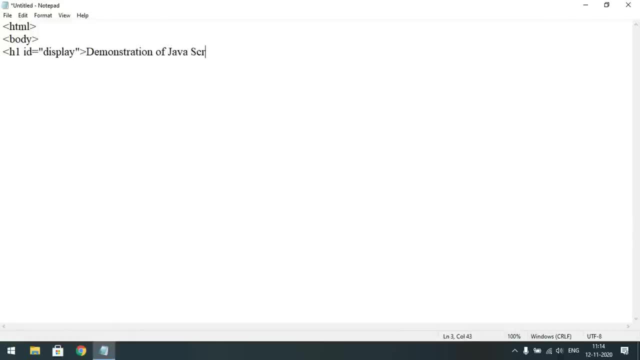 demonstration of javascript. ok, and i have written some h1 and now we will write some button, because after triggering that one, we have to change the content of html. so button is equal, button type is equal to button and on click. so after clicking on this one, what? 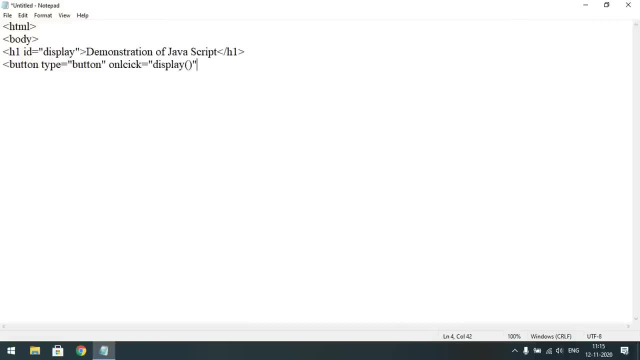 should be triggered. so i will write some display function here. ok, i will write some display function here, so. so so give the text and close the button right. next, close the body and close the html. and now we have to write the script, because after clicking on the button, what should be triggered? 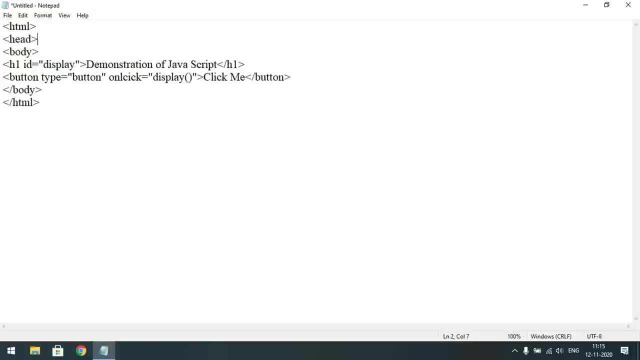 and that should be written in the script, right? so first i will write the script in head tag, so, and all the script should be written in script tag. ok, so i will write some function, so function, followed by the function name. so we have given some display as a function name and i will write here, so what should. 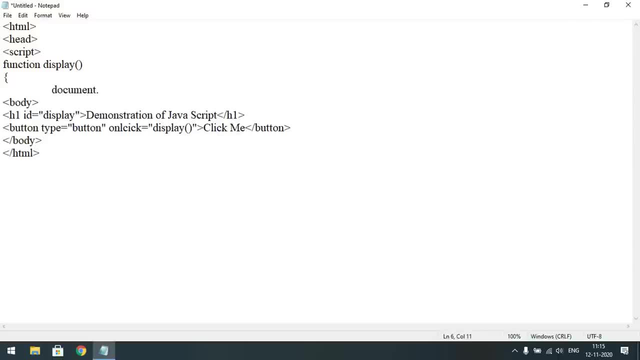 be done after clicking on that particular button. so document dot. get element by id. give the id name: ok, dot, and just changing the content. so we go with the attribute called inner html is equal to script. include ij- exist day in head tag. okay, so I have written a small thing, okay, and close the script. 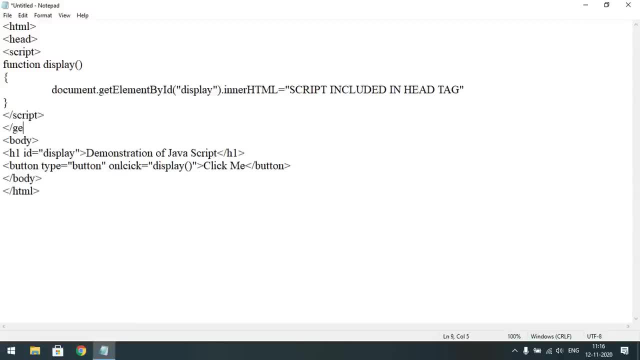 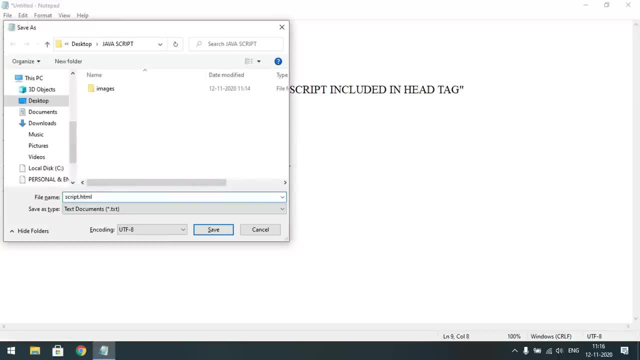 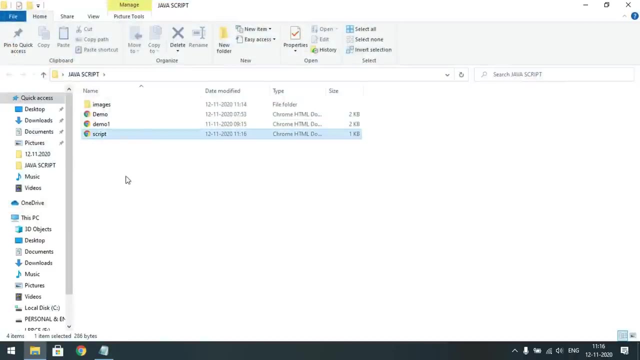 and close the head tag. save this one I will save with the script dot HTML. so in the folder JavaScript. now open the JavaScript folder and here you can observe the script dot HTML. double click on that so it will be executed and you can observe the demonstration. of JavaScript is the normal text and there. 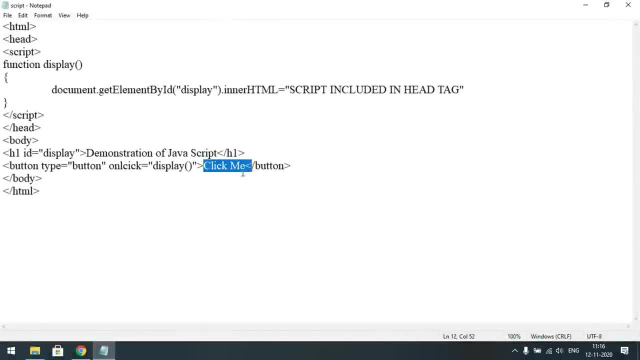 is a button and we have given the label for this button as a click me and after clicking on this button, this display function will be triggered. and this display function has been written in script which is included in head tag. sorry, somewhere we have written so. it was not thing coming, so we'll see one. we will check once. so 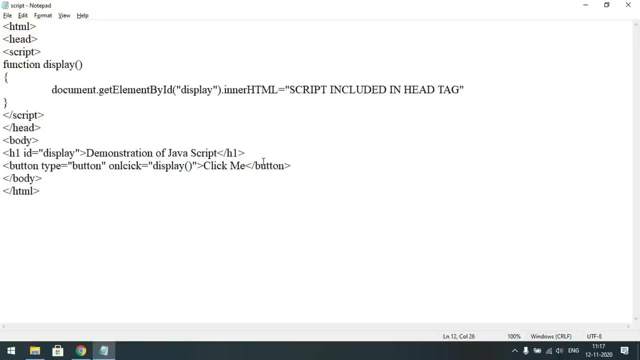 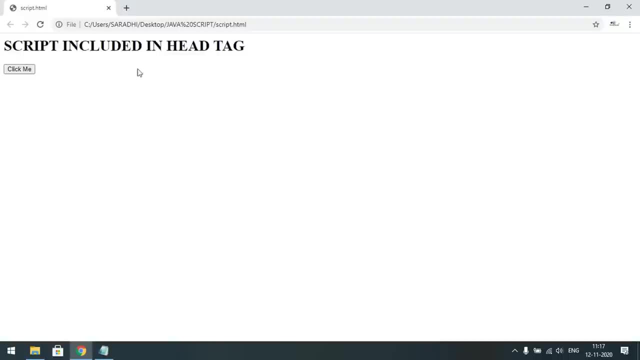 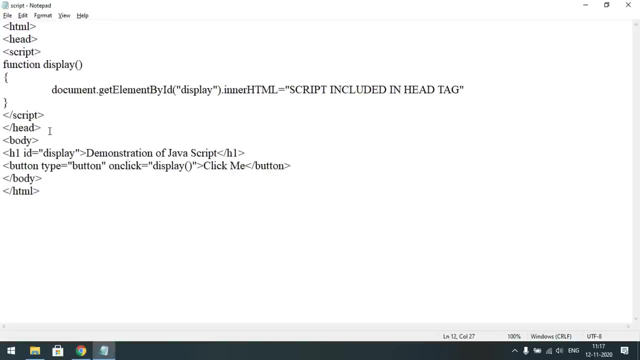 display function on click. so here you can observe there is a spelling mistake. okay, yeah, now you can observe. if you click me, then automatically that HTML content has been changed. so here, whatever the content we are writing, whatever the scripting function we are writing, that that we have included in head tag and also not. 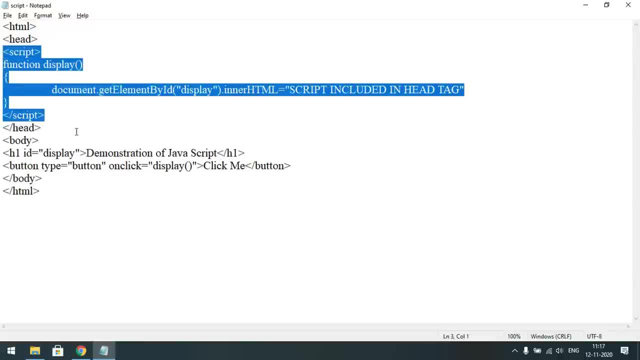 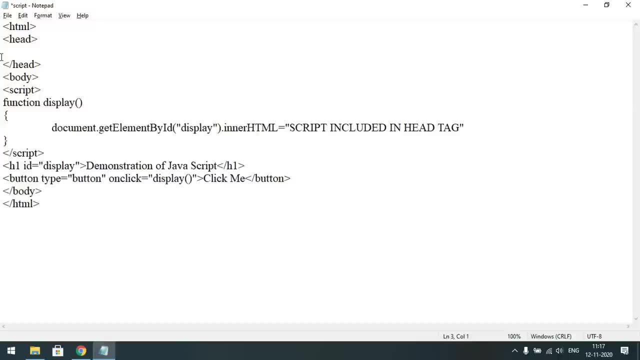 only the head tag, we can also include the same thing. okay, you can also including the same thing in the body tag. okay, just remove, and just removing the script in head tag- you can observe here- and just including it in body tag. okay, anywhere we can insert. right now I am saving this one and still I am executing. 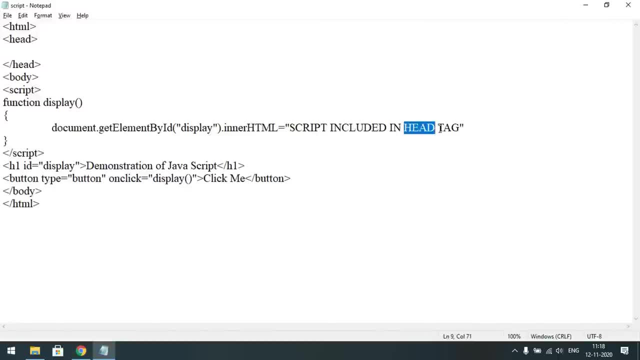 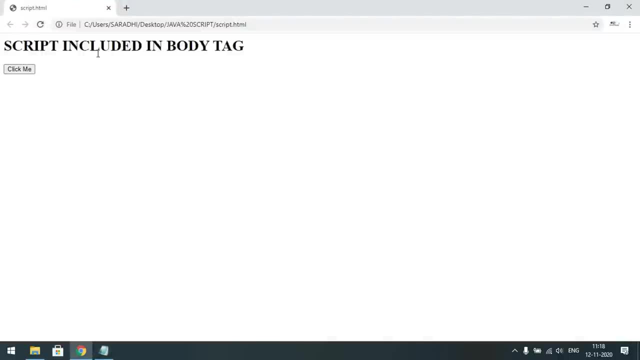 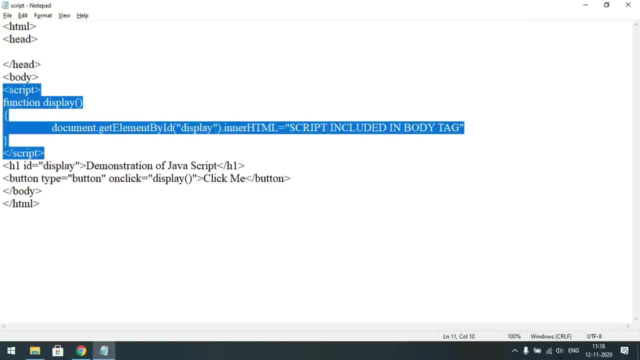 here will change in body day. okay, now execute this one. you can observe script included in body tag. ok, so we can write the script. we can write the JavaScript either in head tag or in body day, so immediately, whenever it was triggered, automatically the script will be executed, and also not only like this, we can also include this: 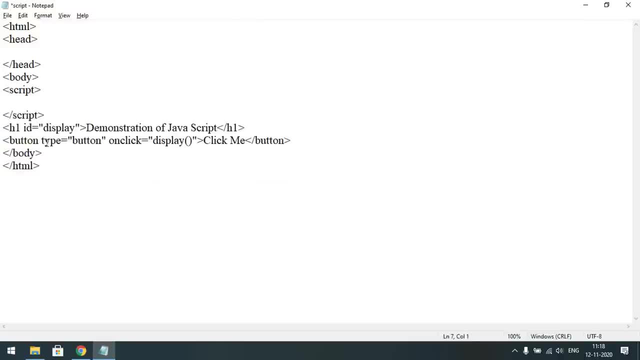 script in the body tag, and so the script which was included on body tag we have included. so any text you don't want to finalize it, the script is not possible to use and also leave bigger text, for that too, can also include this script right in a new file. ok, in a new file. see, I will include this function. 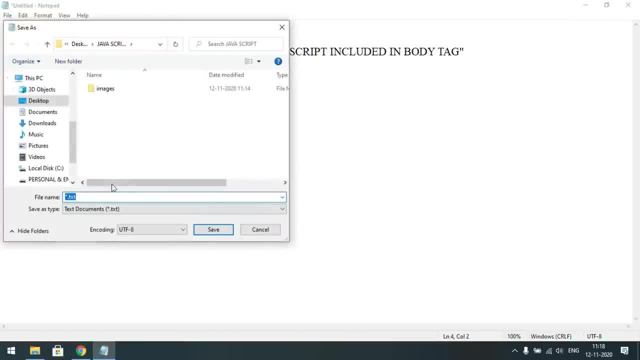 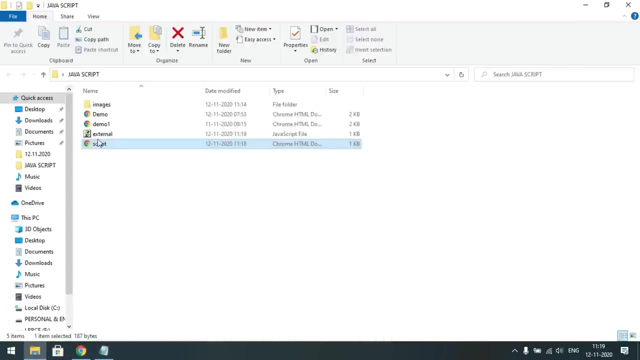 only function. ok, and save this one using dot js. all javascript files should be saved in dot js. so I will write here: external dot js, external dot js. ok, so I am saving this one and also open so you can observe here. so external, it is a javascript file, ok, and script. here we have to give the link. 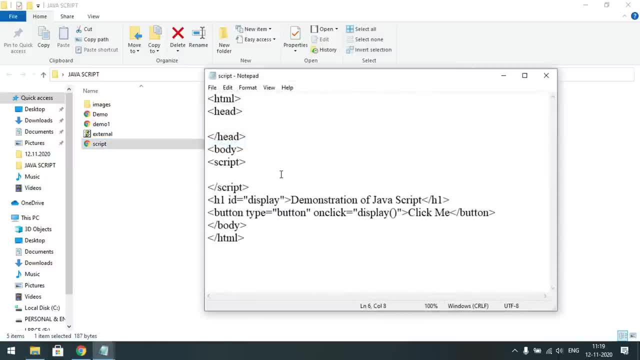 here you have to give the link in in the script script. src source is equal to source attribute. usrc source is equal to source attribute. usrc source is equal to source attribute. usrc source is used to give the link. source is equal to external dot js. ok, and you need not write anything. 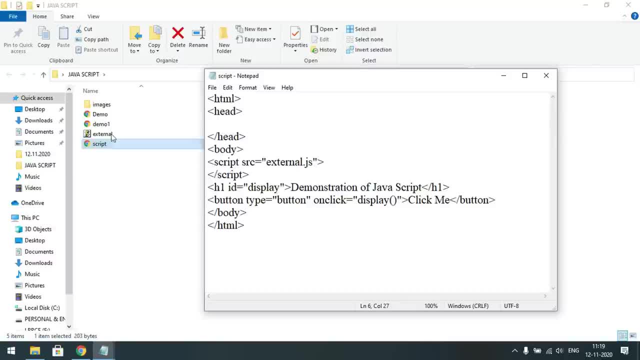 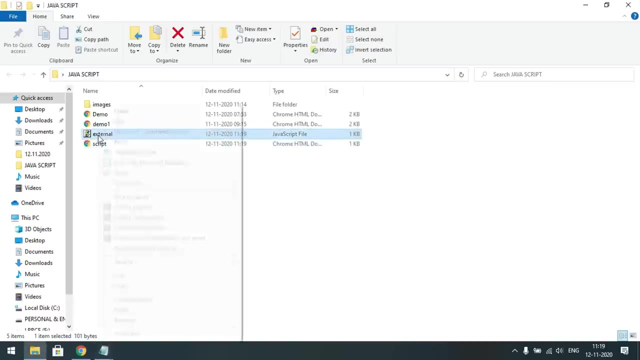 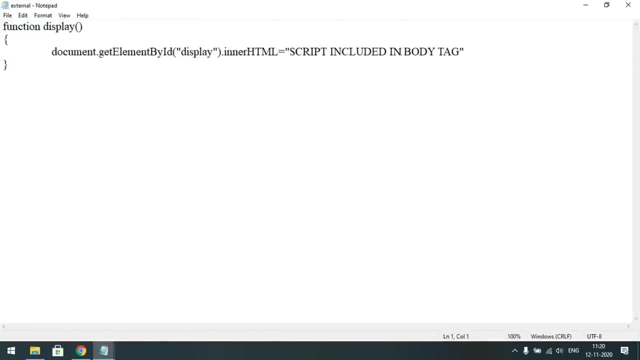 else here. so all the javascript can be written in external file and that can be included here. all right now you can observe here I am executing the same thing. I am executing the same thing, so I will change the content. ok, so instead of writing some script in, included in body tag, script included in external file so that you can. 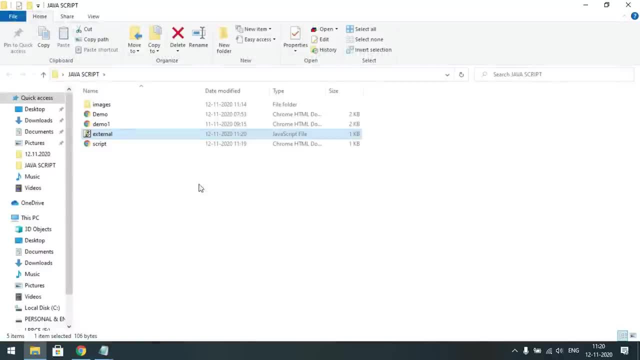 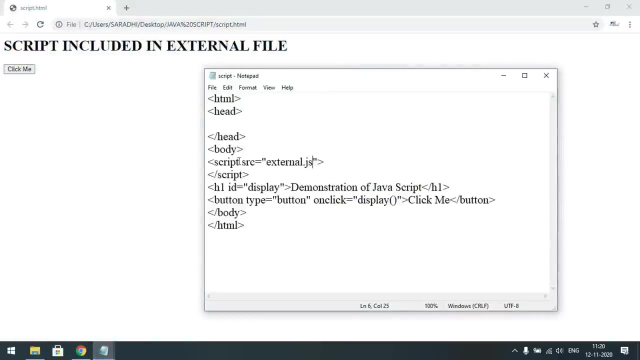 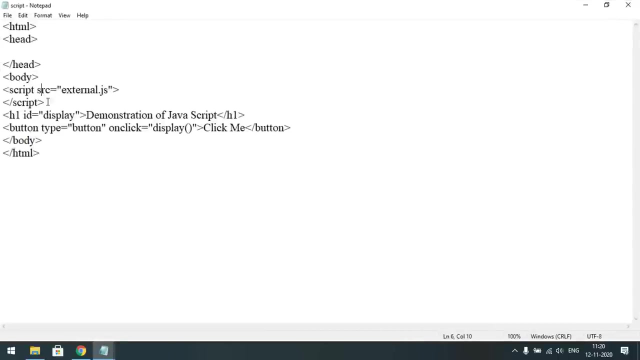 understand. ok, you can understand the difference. so I have included. now we can observe here. so just click on me. script included in external file. so here you can observe if you go with the code in this one. we are not writing any type of code, javascript code, in this source. ok, any type of code in this course, but we are just 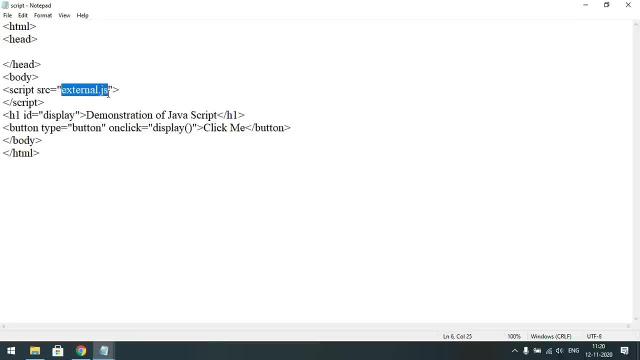 writing into an external file, and we are just linking the external file to our html content. so, obviously, whenever it executes the display function, it will go for the external, this one- and then it will execute. ok, right, so hope you understood this one where we can insert this scripting, so the scripting can be done in this way. ok, so now we are going to see. 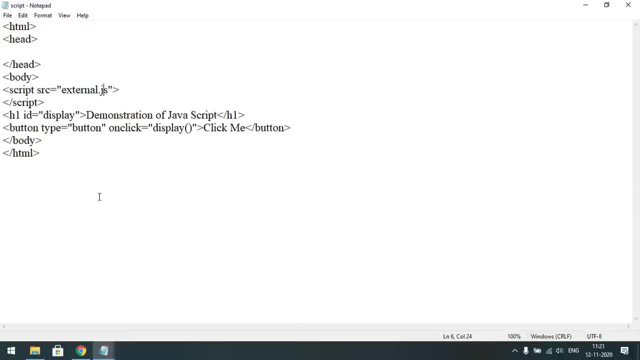 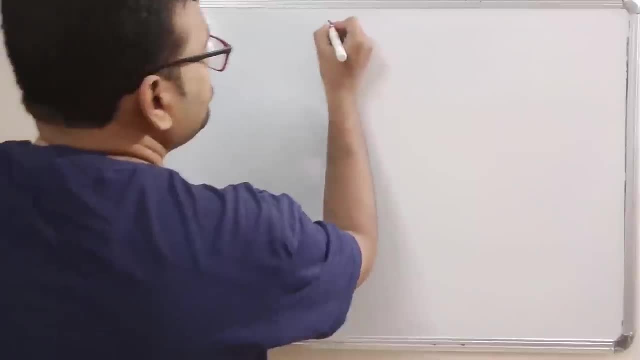 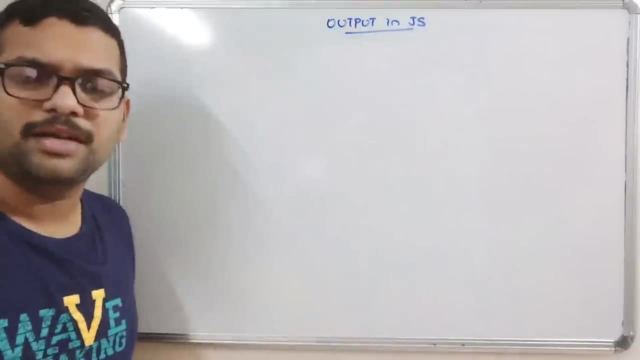 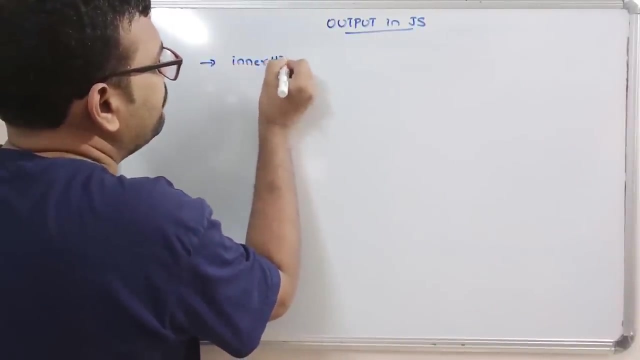 how this scripting can be written in either head or body or an external output in js. js means nothing but a javascript, right, so output the first one is inner html. so inner html is used to write the content on the html, based on the content of the content. 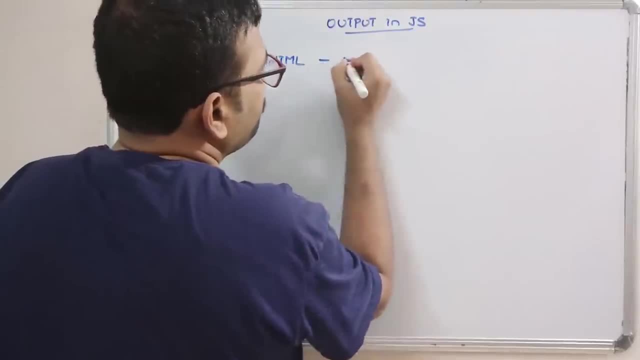 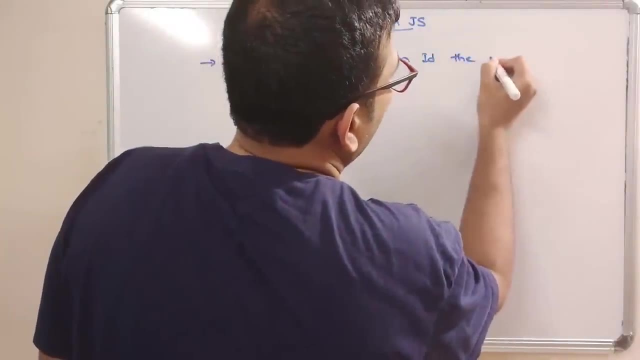 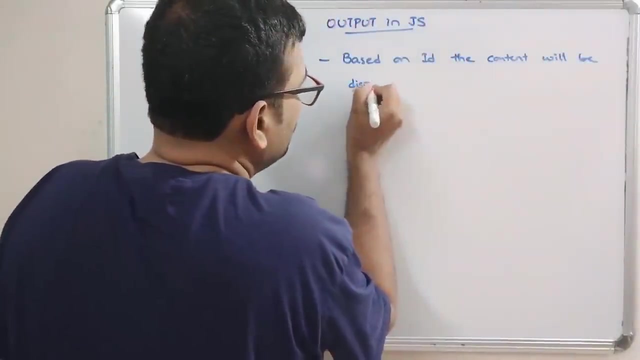 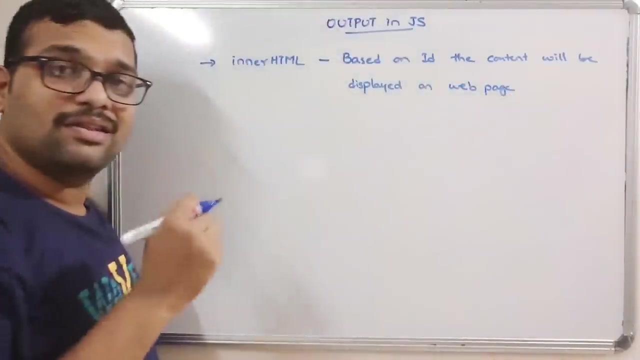 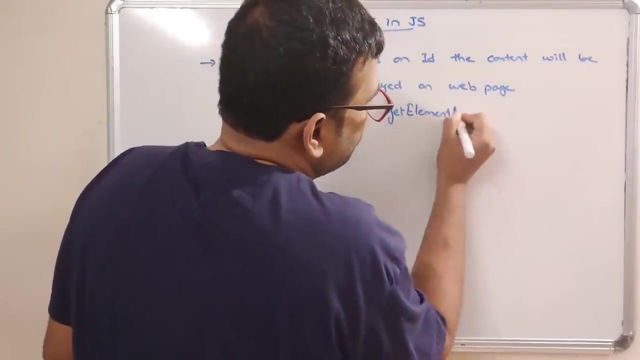 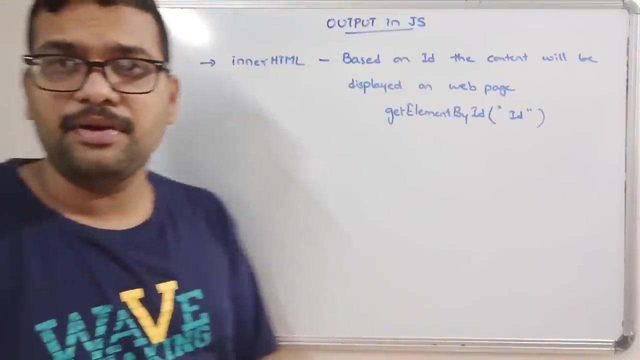 based on the id. so, based on id, the text or the content will be displayed on the web page. so so, whatever the id. so this id is written by using get element on the html and the content by id, followed by. here we have to give the id right. so this already we have seen in the 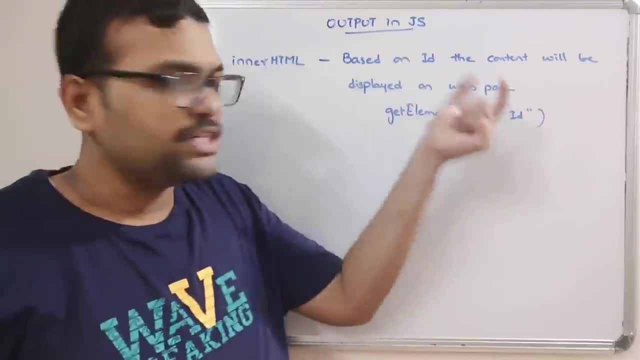 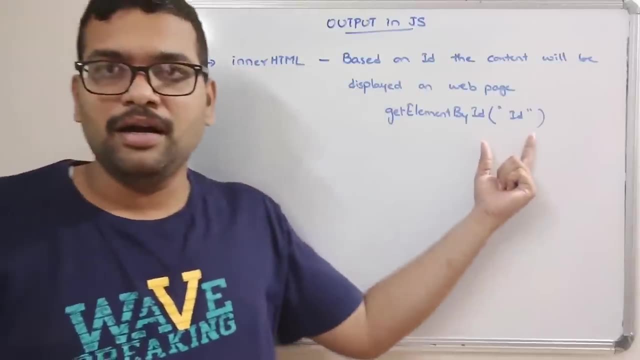 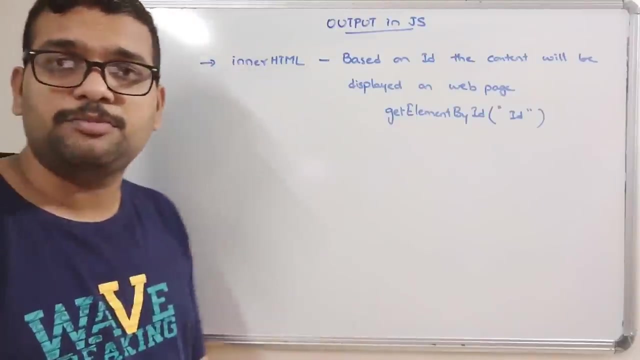 beginning session. right, so based upon the id, first we have to retrieve the element for this particular id and we can write the content in the particular id. okay, so for that purpose we will go with this inner html. okay, so don't worry, i will execute a small code demonstrating. 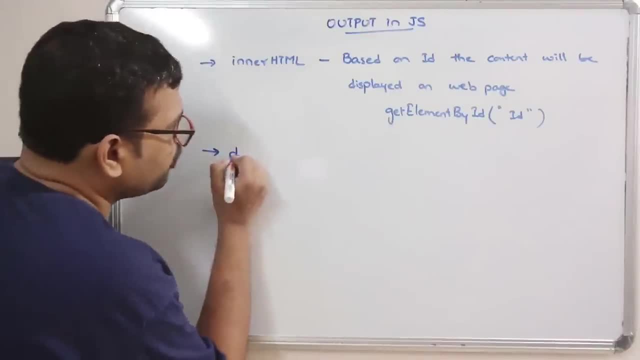 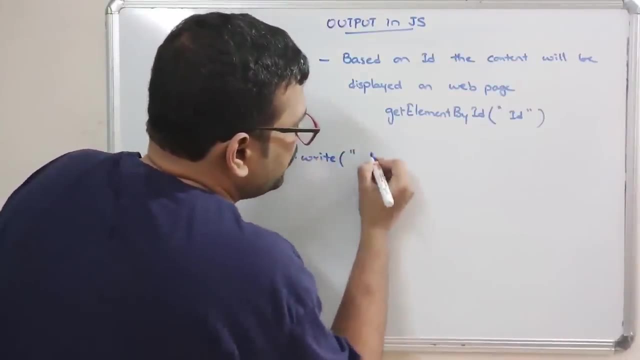 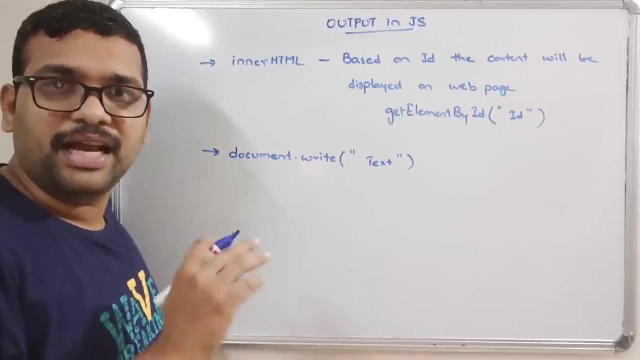 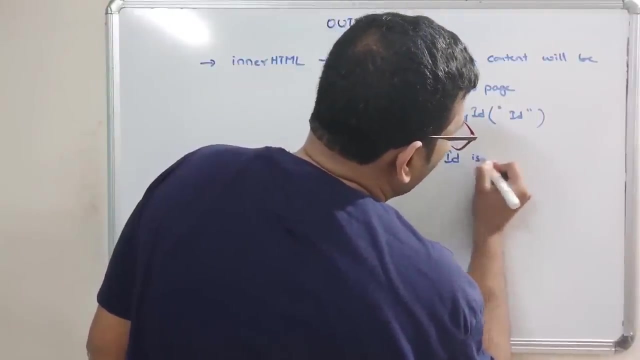 all this thing. and the second one is a documentwrite. so documentwrite function. here we can give the text. whatever the text we are writing here, that will be printed on the web page directly. so that means we need not go with id. okay, so id is not required. and director. 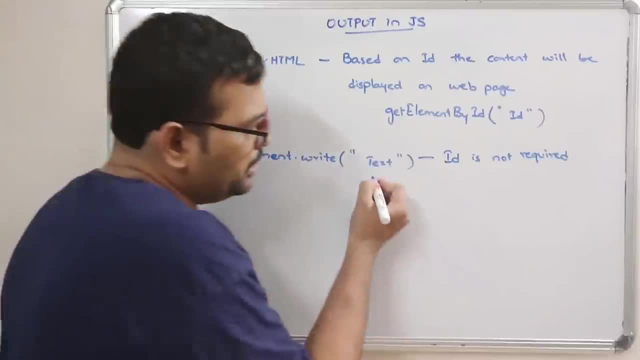 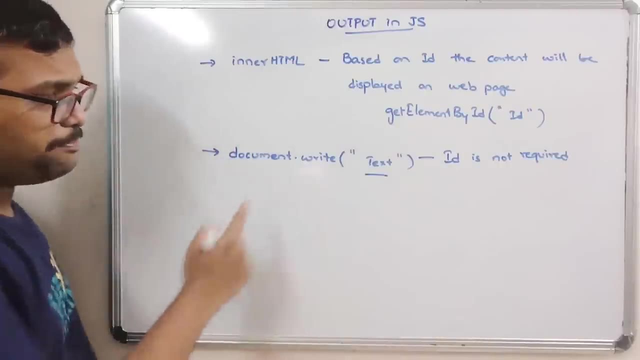 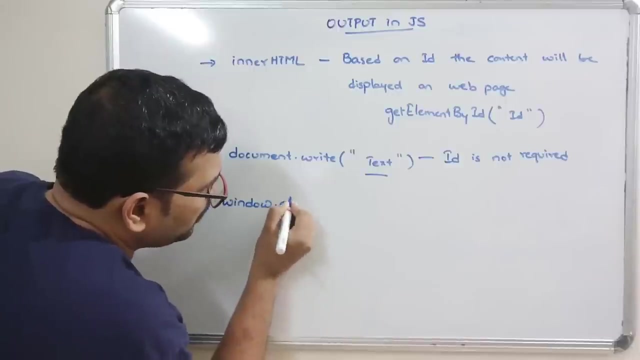 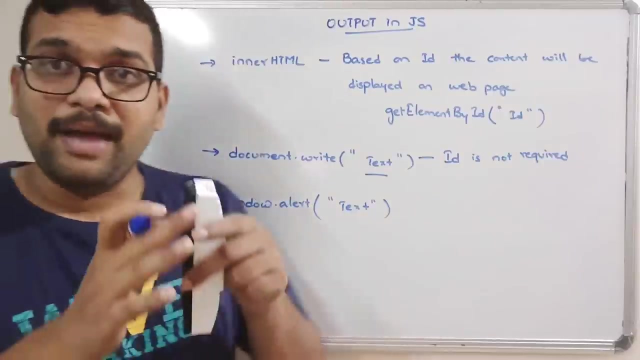 it. whatever it is, the content will be displayed on the web page directly. so whatever the thing we are writing in between the double quotes, that content will be displayed directly on the web page. that is a document dot right, and the next one is window dot alert, and again we can write some text here, right. so window dot alert means some. 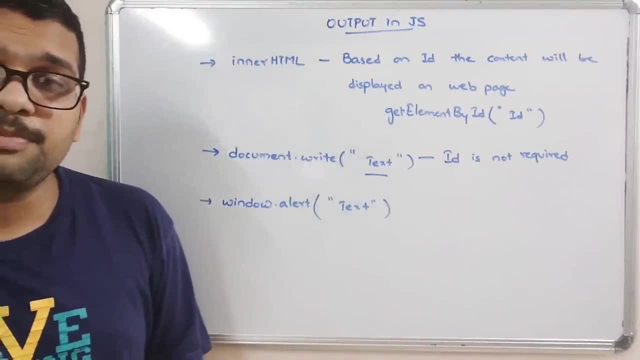 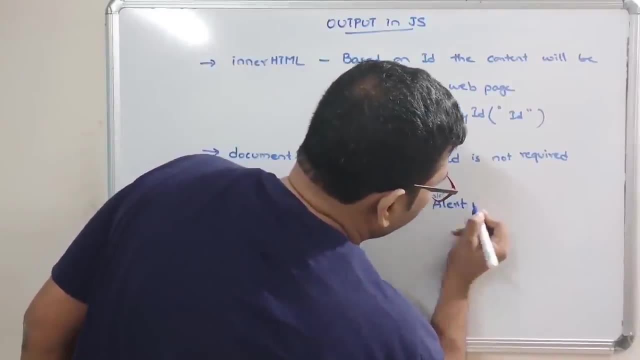 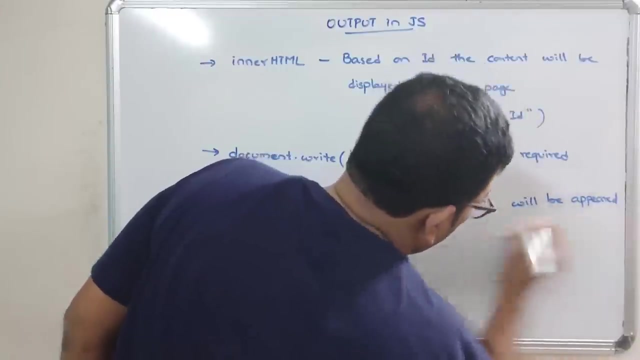 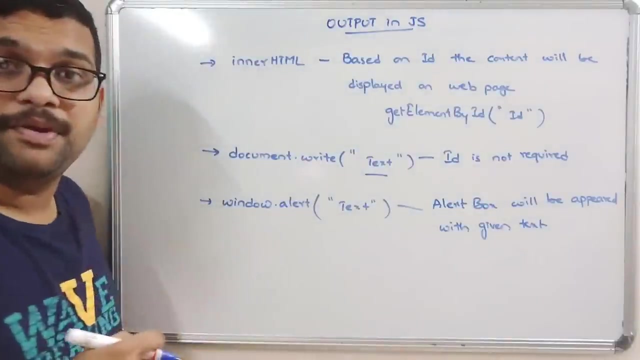 alert box will be displayed and the content will be displayed on the alert box. okay, the content will be displayed on the alert box. so alert box will be appeared with a given text. okay, alert box will be appeared with the given text. so, whatever the text, we are writing that. 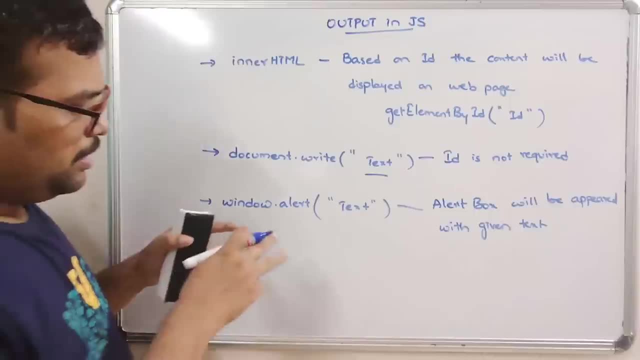 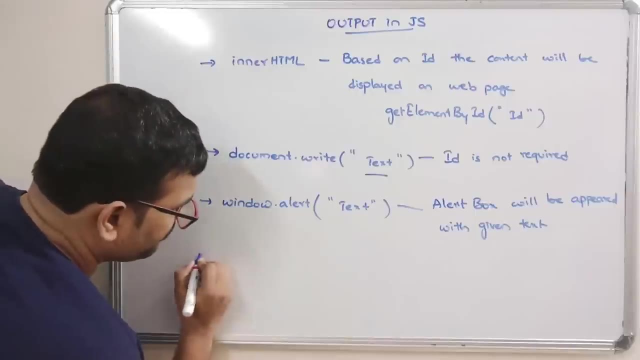 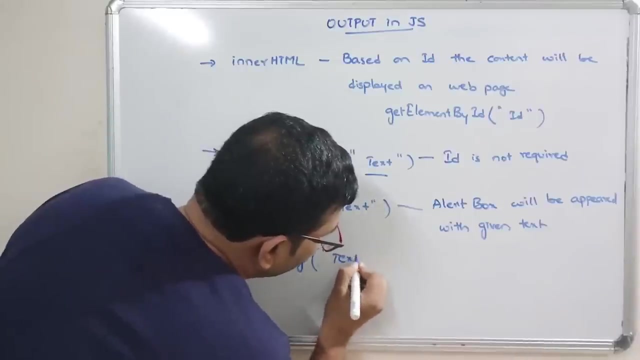 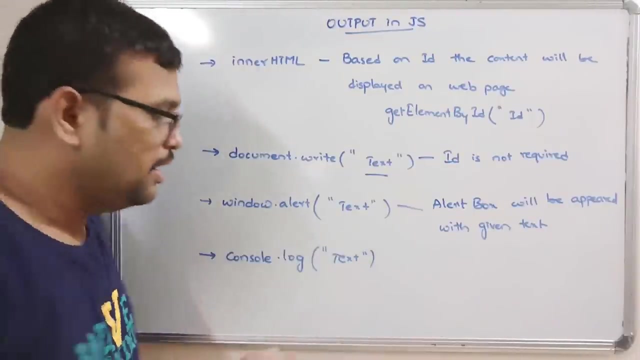 will be displayed on the alert box. okay, so i will show you the execution, so then you will be understanding perfectly. and the next one is console dot log. and here also we can write the text so this will be displayed for the debugging purpose. so directly it will not be displayed on the screen. and in order to display the text, we 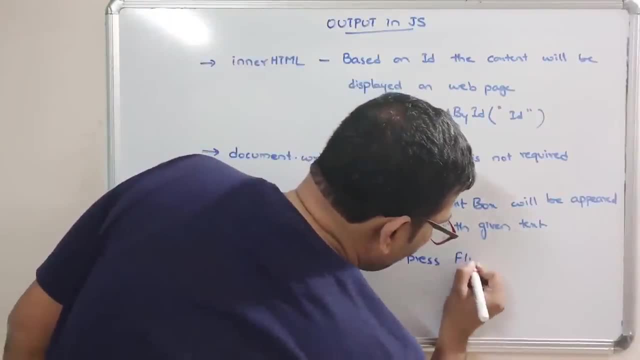 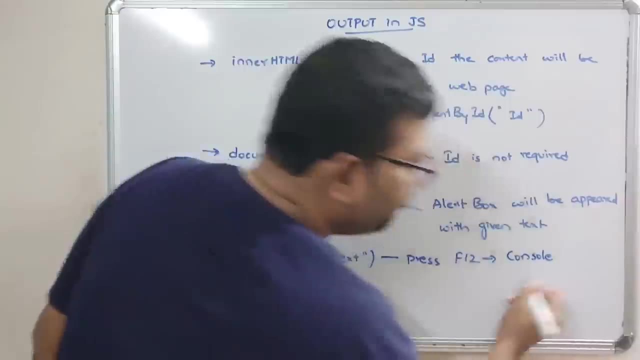 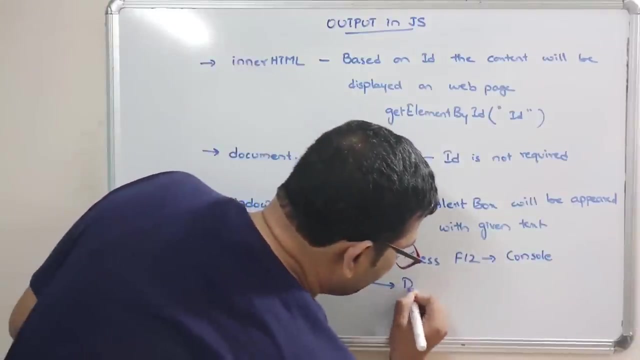 have to press f12 in the keyboard. press f12 in the keyboard and go to the console field. so in the top you can find the console, then you can find the output, then you can find the output. so this is purpose of debugging. so in order for the debugging purpose, we 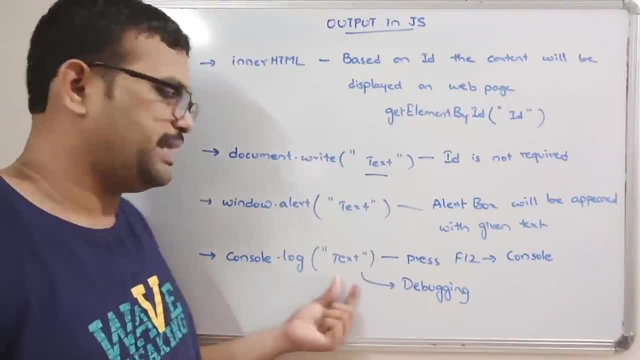 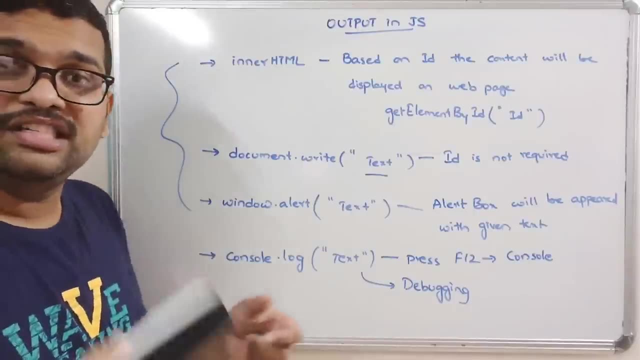 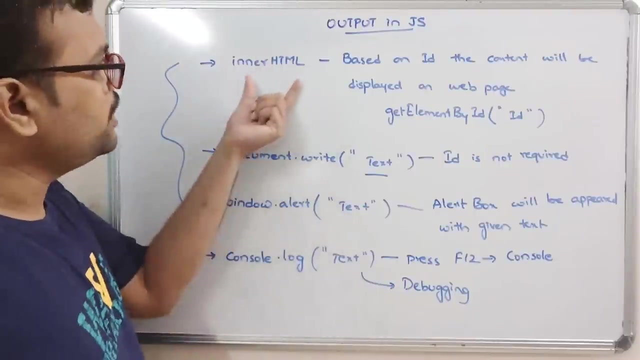 can write this function: console dot log of text. so basically we will go with these three concepts. so in the further sessions we will see how, in order to display the output, we will see one among these three. so if you want to write a function, print the data based upon the id. so we'll go with the inner html. if you want to directly print the, 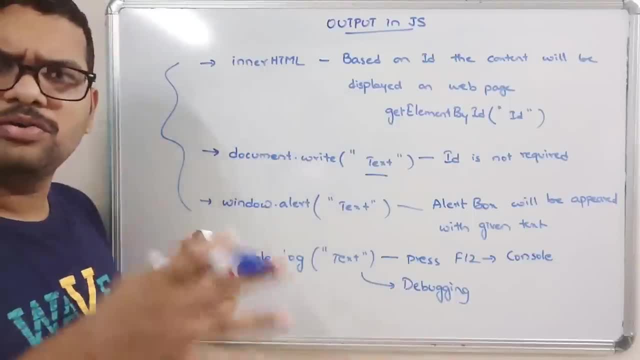 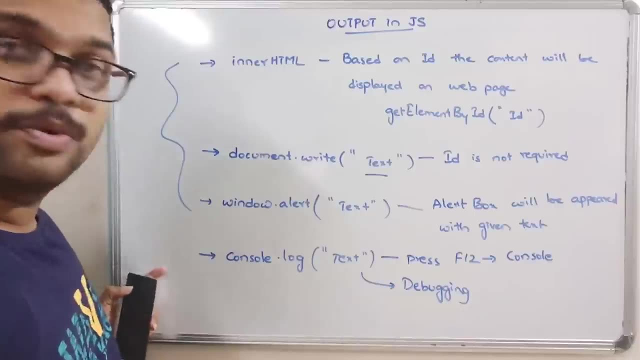 output on the web page. we'll go with the documenty, and if you want to give the alert some alert, so then we'll go with the windowalert. so these are all the different outputs, and one more function is there that is called print function. print function. 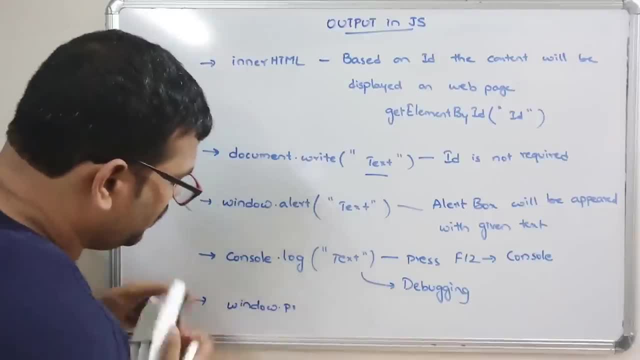 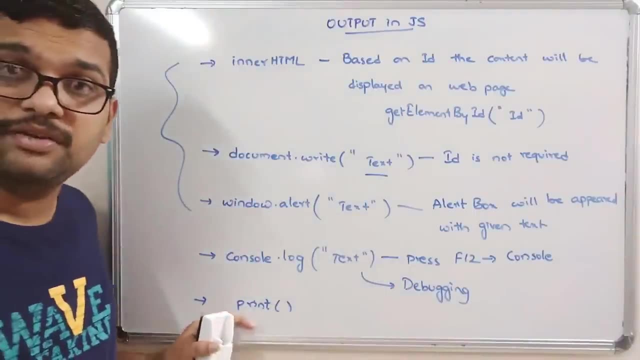 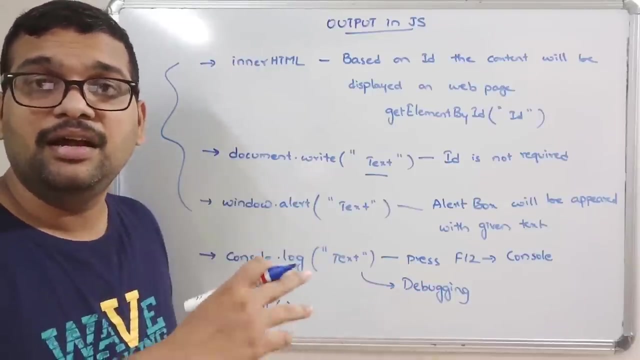 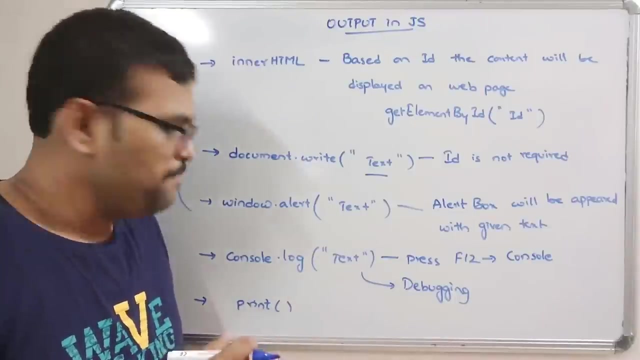 sorry, there is a direct function, that is, a print function which will give a print option to our web page. i mean the content on the web page. that will be directly redirected towards the printer. okay, if there is no printer, automatically it will be redirected to save as a pdf. so this is a function we can implement to directly print the content of the web page. 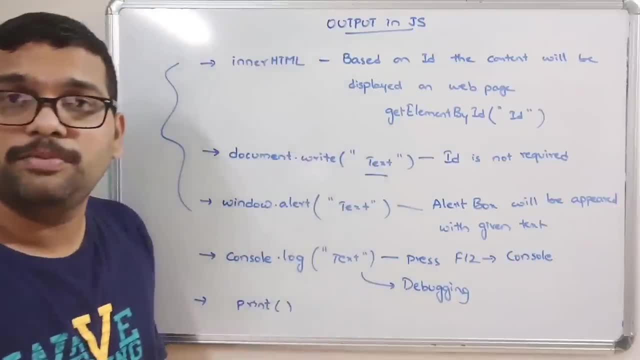 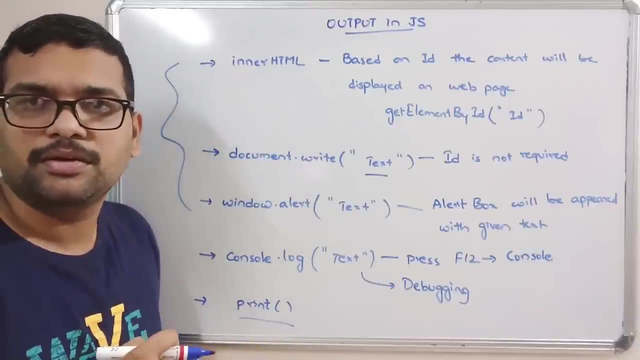 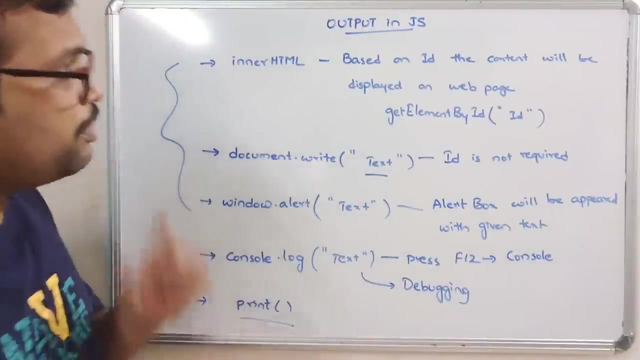 okay, i will show all these things. i will show you by executing a small html code, right, so direct print function will give the print option. it will be available to print option the complete content of the web page. right, so let us move on to the computer and we will see the demonstration of. 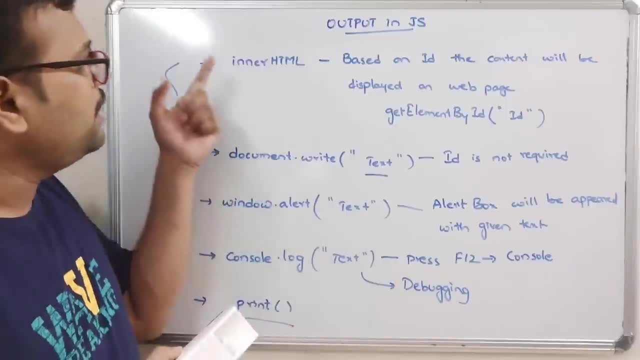 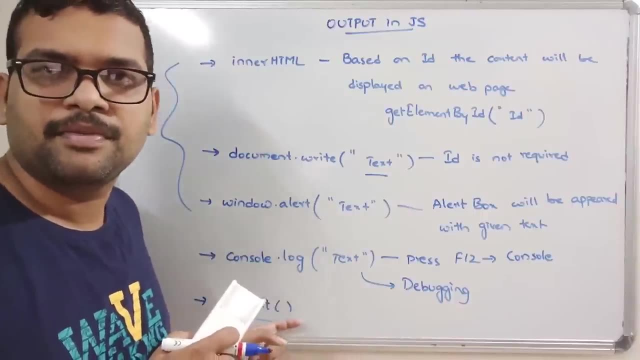 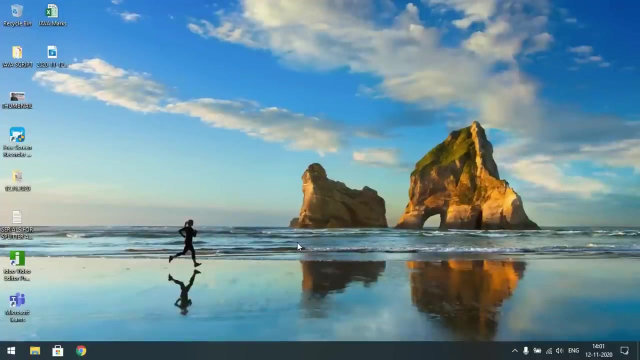 each and every output statement or a function: right inner html, documentright, windowalert, consolewalk, as well as the print. as well as the print function, well as the print function. right, so let us move on to the computer. hello friends. so just now we have seen the different. 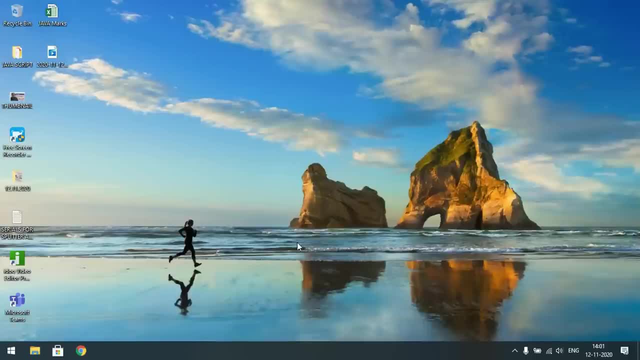 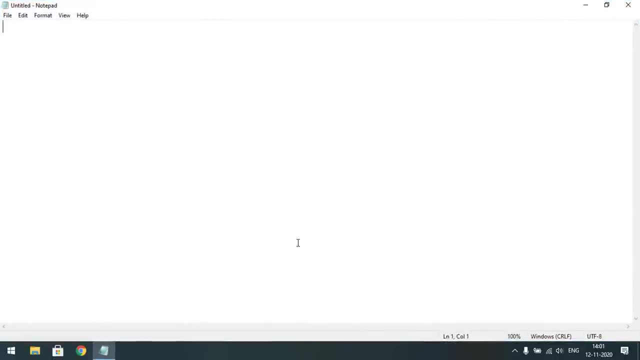 ways to print the output in javascript. so now we'll see the demonstration of all those things. so, coming to the first one, that is, the inner html. so in the previous sessions we have already seen about this inner html. so, based upon the id of the element or 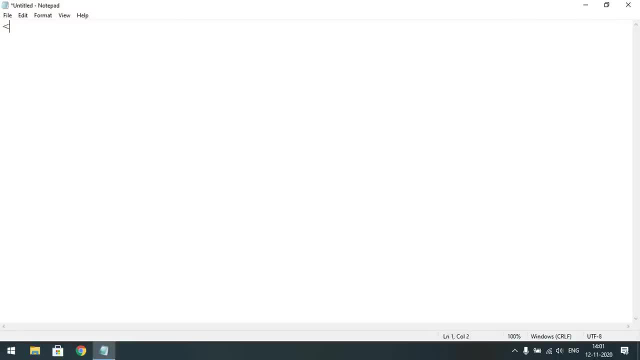 tag we have. we are just changing the content in the html, so we'll go with the html page and now go with the body and here write down: h1 is equal to sorry. h1 id is equal to give some abc id, abc. okay, i'm just giving h1, it's an empty. 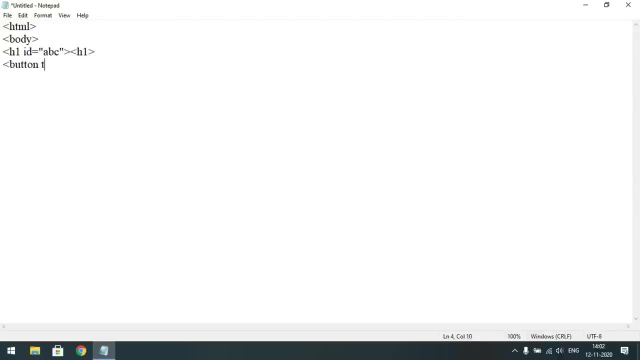 right now i will create some button. type is equal to button and here on click. after clicking this button, what should be done? so document dot. get element by id of give that id here. so dot. inner html is equal to. so give the content. okay. demonstration of in the html. 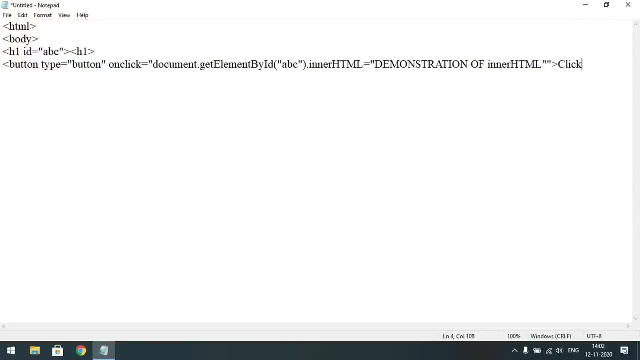 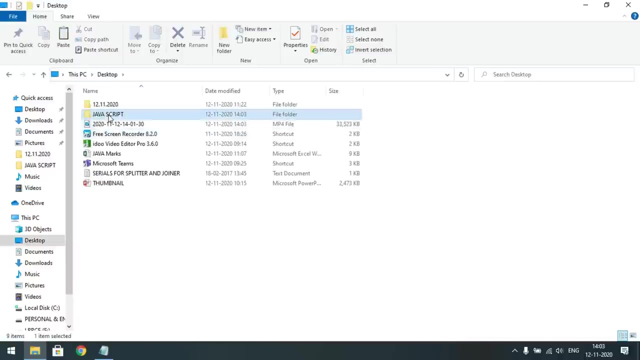 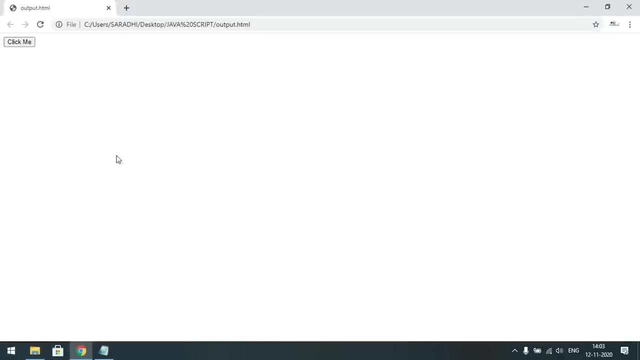 right, so write down. click me button right now. close the body tag. close the html. save this file. i will save it as output dot html, so let us open that file. so here it is the desktop which is javascript. we are having some output dot html, so double click that one so that the 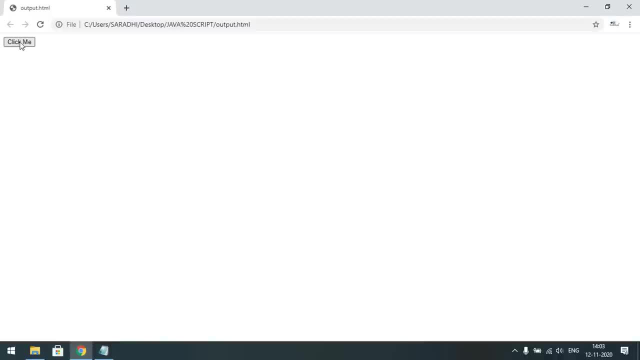 system recording will be executed. see, you can observe here, click me, by clicking this one, we will have to get this output right. so yeah, just a second. and once again, we will just use sequence, this studio. so for vocabulary example, the controlled enemy component. okay, and let's see so. 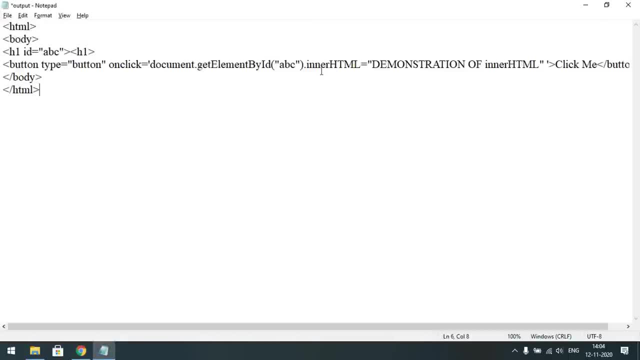 so if you want theButton under the column arrangements, the progress alpha column, your, is also used to display the content on the web page, but based upon the ID. so here, compulsory, we have to give the ID itself right. and one more thing, the second one, the second one. let us give the break row. second one, that is by: 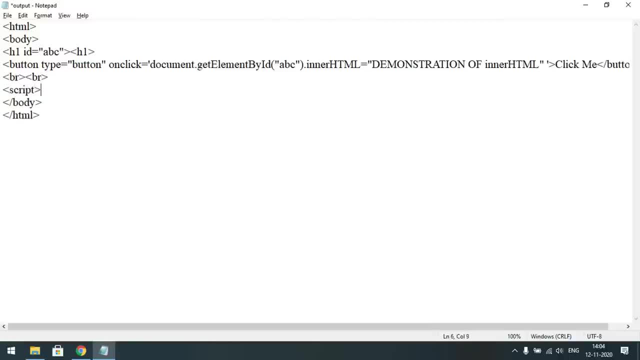 using the document dot write, so script, so document dot write function. inside the write function we can pass anything, so welcome to or simply use this one demonstration of write function. okay, so this we have done and close the script. as we have discussed in the previous session, script can be written in both. 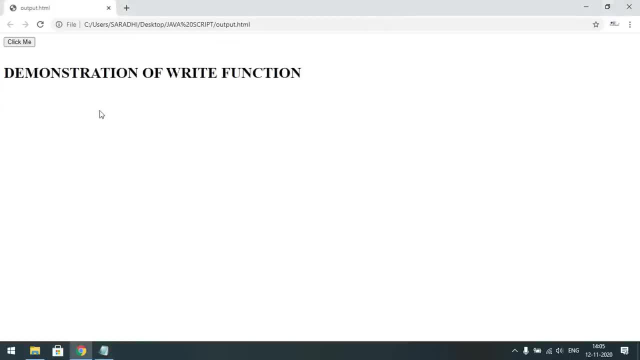 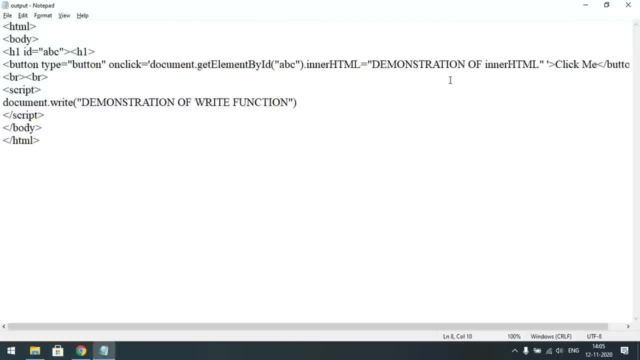 the head or body, right. if you execute this one, you can observe here, right? so if you execute this one, see first: click me is there? demonstration of write function. demonstration of write function. this, this, this is: was written in document: dot write. document, dot. write. that is written. 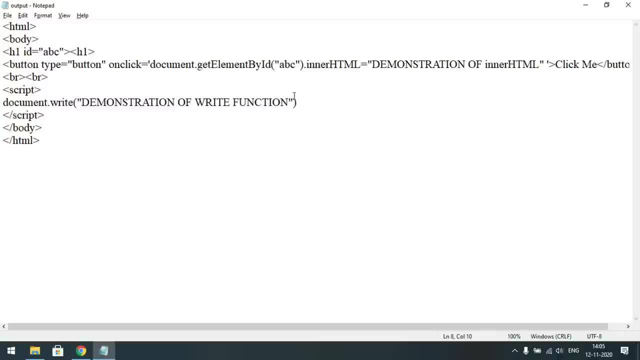 in script. this is one way. okay, this is one way. and also we can use output by using the alert messages so we can get the alert box, the prompt box. so by using that, with the help of window dot alert, we can display the message on the webpage. so 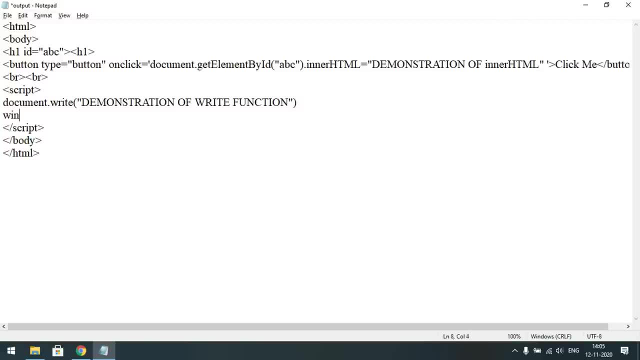 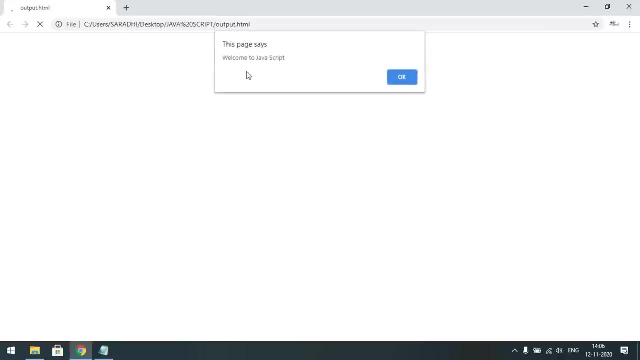 let us check window: dot alert- welcome to JavaScript right now. you can observe here: if you execute this one directly, we'll get this page alert box. okay, you can observe here: alert box, welcome to JavaScript. if you press ok, then the remaining code will be executed, so alert box will be getting right, or else you. 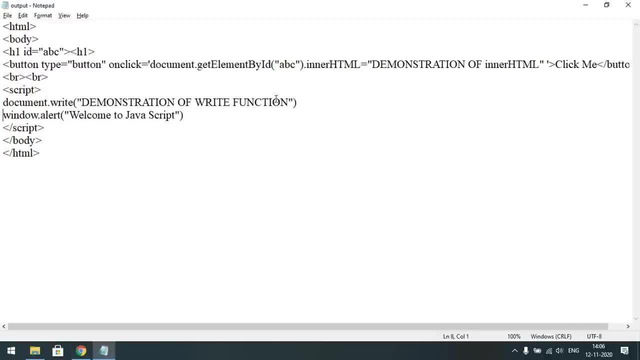 can simply use the same thing. okay, we can also combine. we can create one button and after clicking on that we can get. we can execute this window dot alert option. we can write this in some function and we can write: okay. so these are the different ways we can display the function, so one is a. 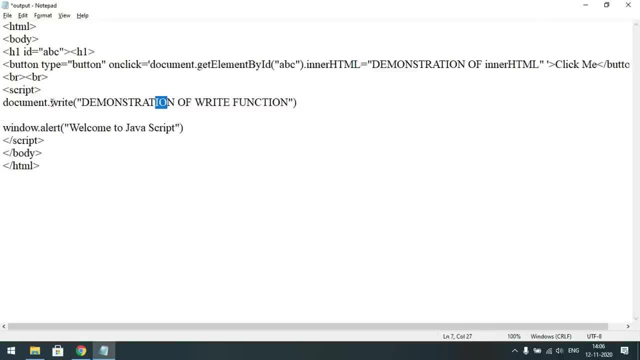 by using the inner HTML. otherwise, the second one is a right document dot right and the third one is window dot alert. and there is a one more thing, that is a console console dot log. so by using the console dot log we can also display the output. so this this will be used for debugging purpose. this is used for 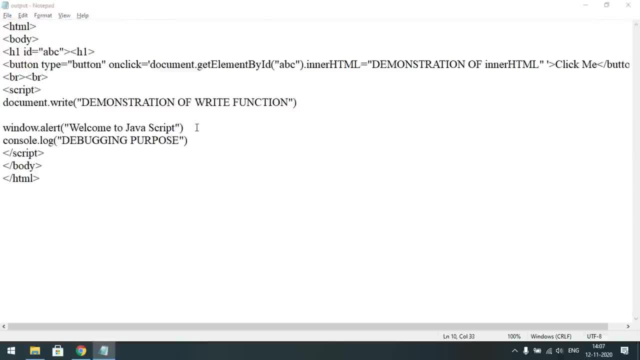 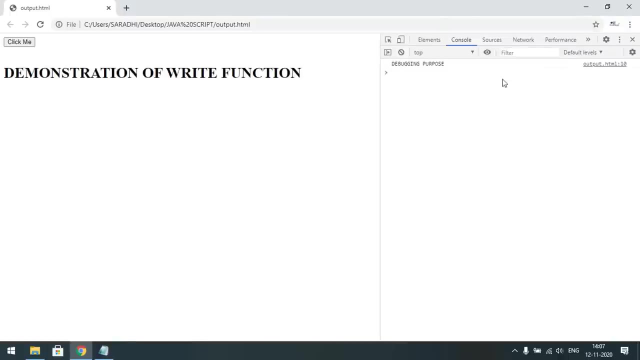 debugging purpose. so if you execute this code you cannot observe the difference. but in order to see this console dot log we have to press F12. okay, F12. if you press F12, the debugging control will be there. so here you can observe the output. debugging purpose: here you can observe. 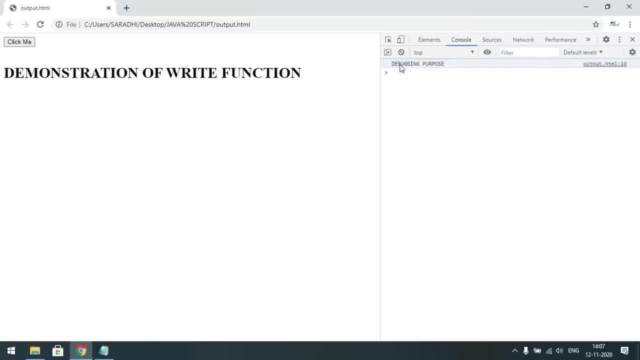 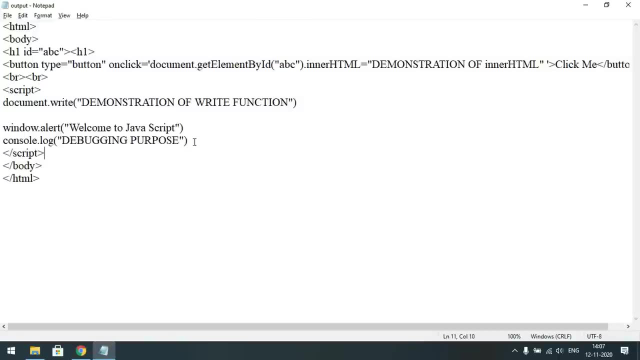 the output in the console. okay, in the console field we will get the output here right. so these are the different ways how we can display the output in JavaScript and also if you want to print the complete page. if you want to print the complete page, they simply. there is a function called print function. there is a 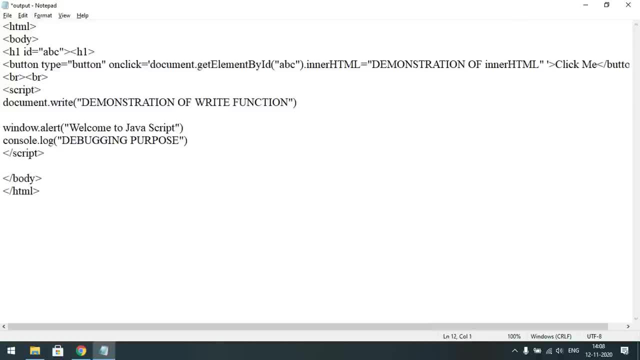 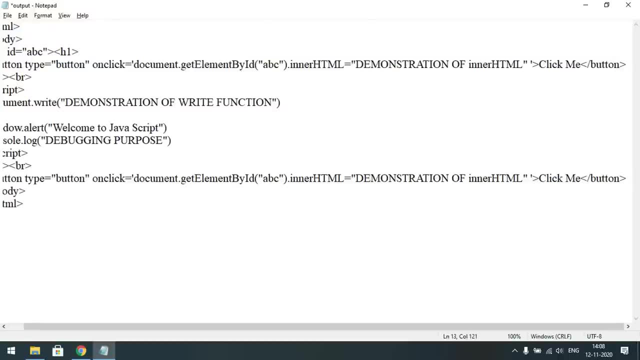 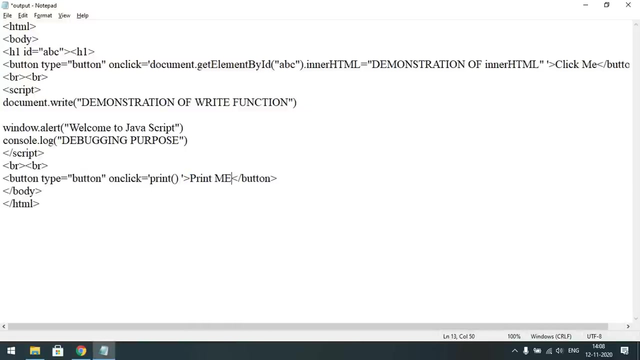 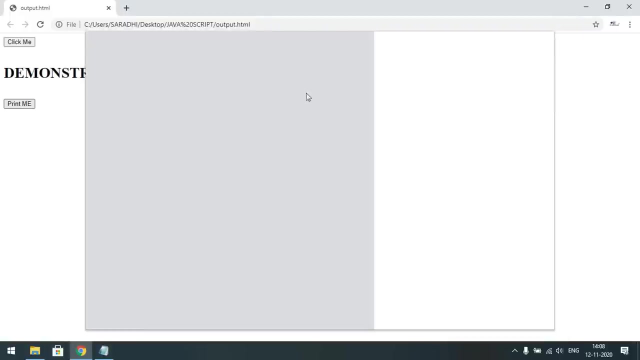 function called a print function. see, I will show you so here. instead of using all these content, go with the print function, print function, so that this will print the complete content of the page. see, if you print this one, the complete contents of the page will be printed. so this is how we. 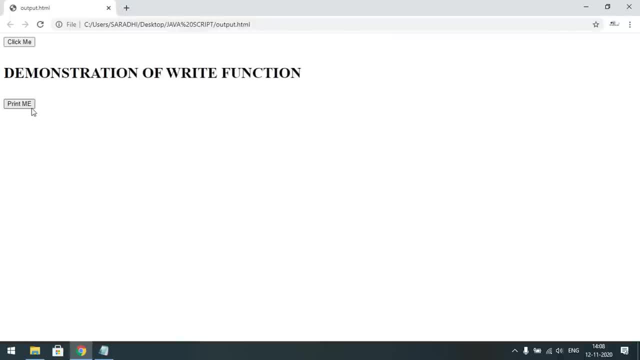 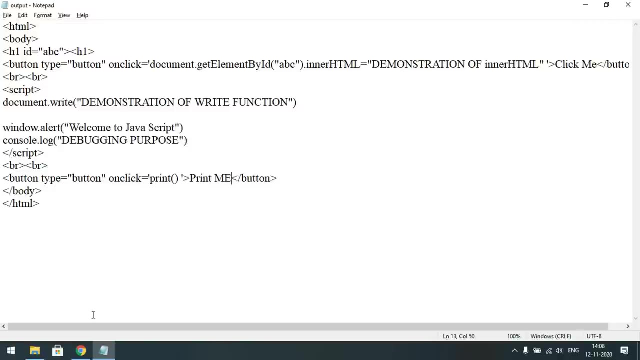 can use the print also. okay, we can also print. so it directly redirects to the printer. so if you print the complete content of the page, so here I am NOT having any printer. so it is asking about save as PDF, right, right? So these are the ways we can give the output in the javascript. one is the inner html that: 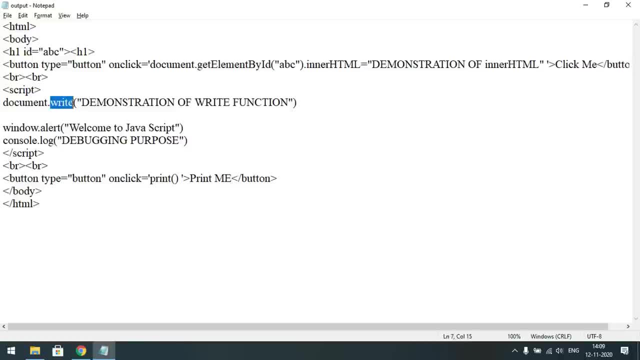 is based upon the id. second one is a write document, dot write. third one is a alert. it will give the alert box. next one console dot log. that is for debugging purpose. So for this, for executing this one, we have to press the f12 in our keyboard so that in 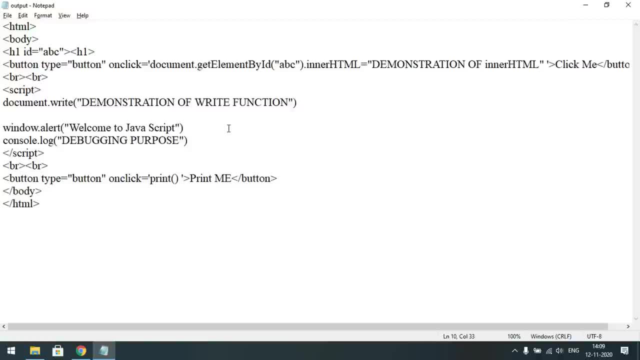 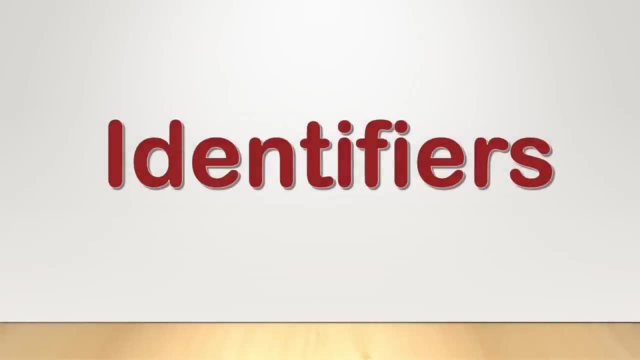 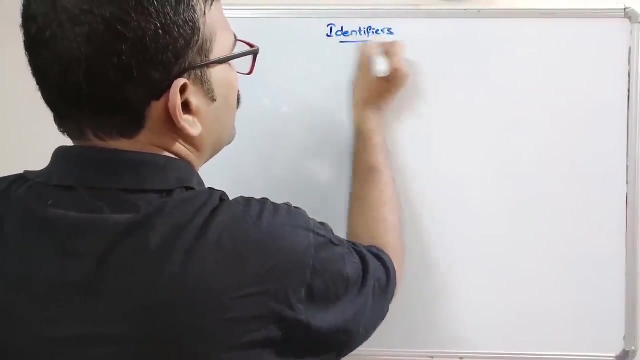 the console, I mean in the console field, we will get the output. and then there is a function called a print function, which will print the complete content of the web page, right? So the name itself indicates it identifies the memory location, right? So, whatever the thing, 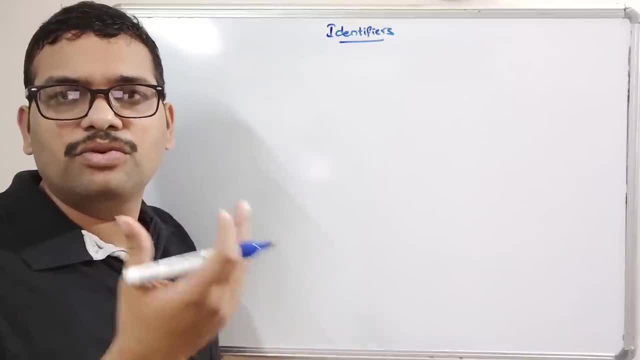 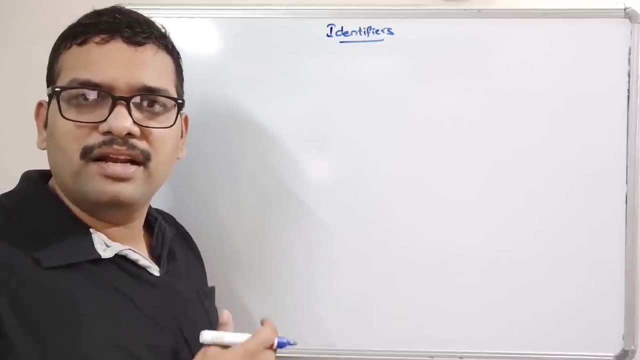 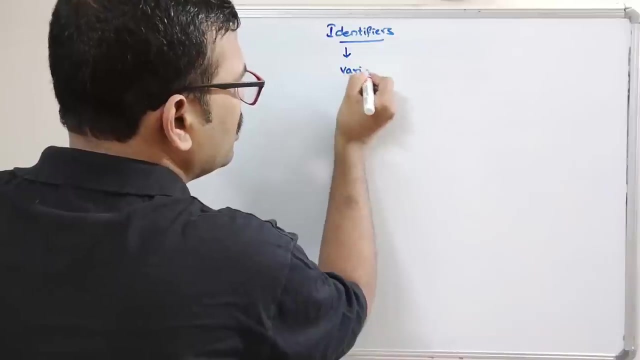 We are giving some names to the number location, those we will call it as an identifier. So best example for the identifiers are variables. okay, So what are the variables we are declaring in the program? those are called an identifiers, right? So variables are called identifiers, similarly, function names. so if you are using some functions, 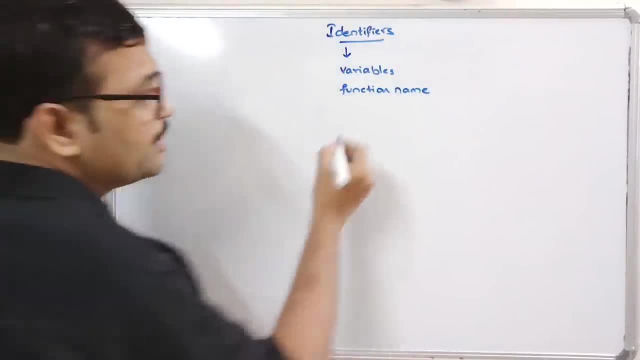 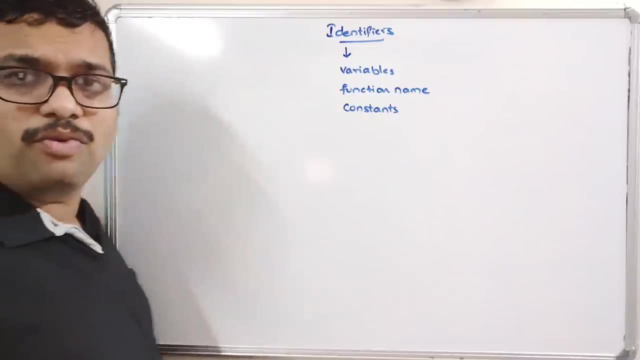 the function names can be declared as an as an identifier. similarly, constants are can be treated as an identifier. So all these things will be treated as an identifier, right? So whatever the thing we are giving some name, So those memory locations, those names will be identified as an identifier. 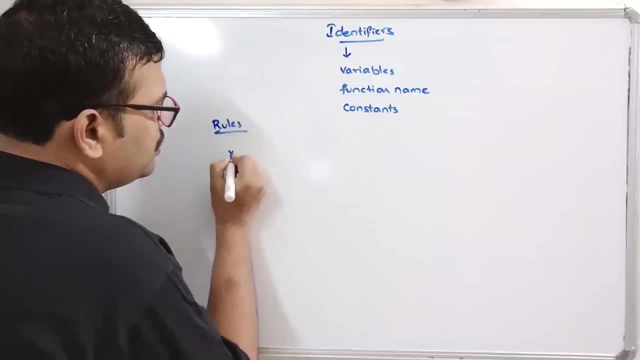 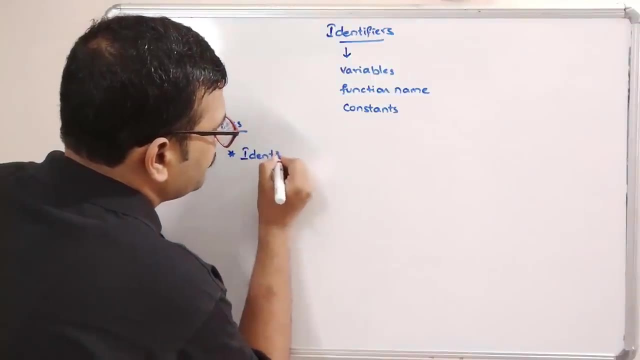 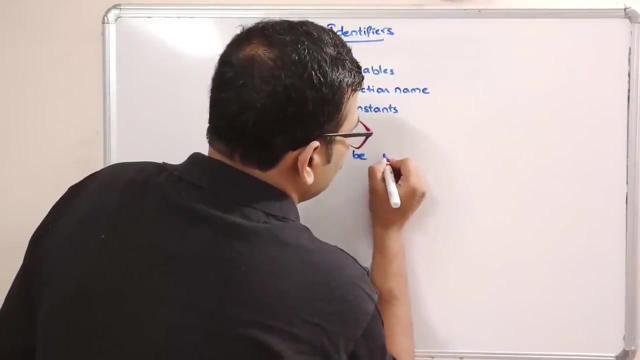 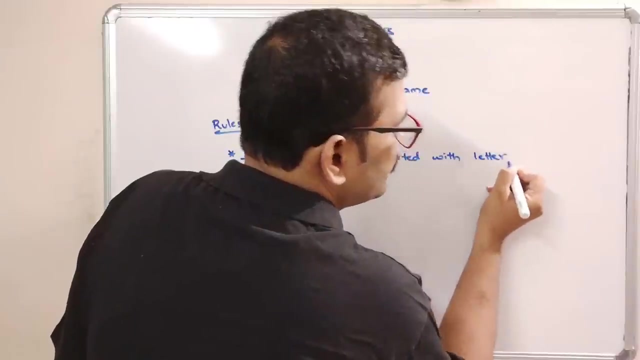 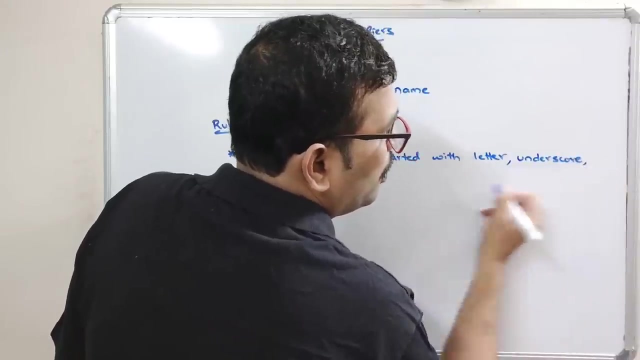 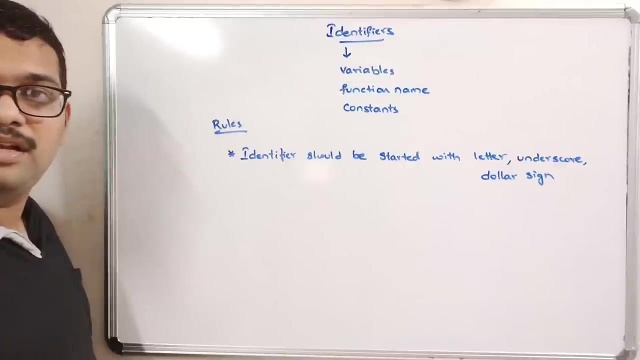 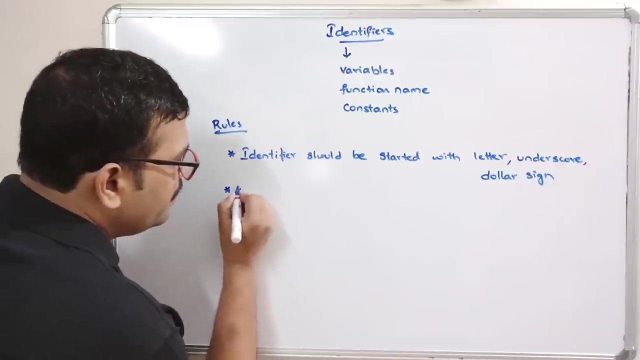 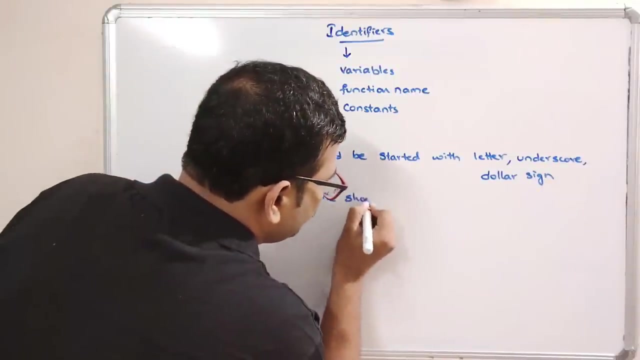 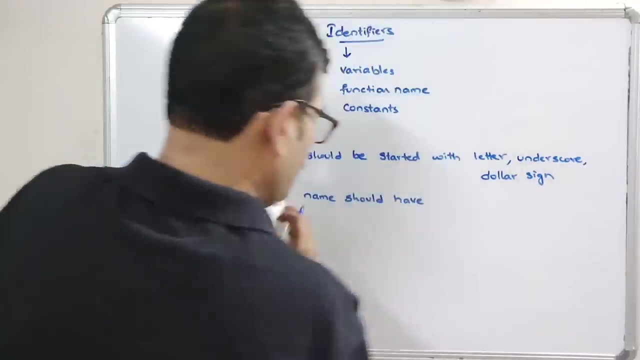 Now what are the rules to be followed? the first rule: identifier name. identifier name should be: Identifier Can be started with a letter or underscore or dollar sign, so the variable can be started with either letter, underscore or a dollar sign And Identifier Name should have: 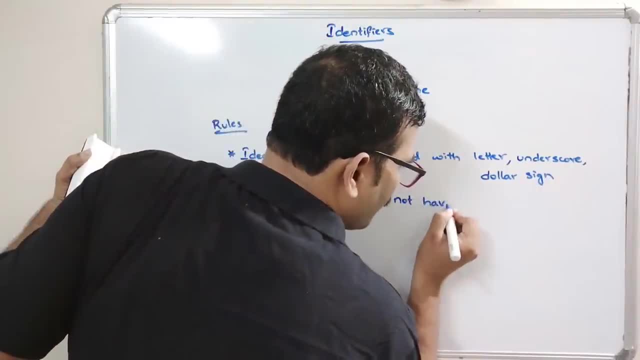 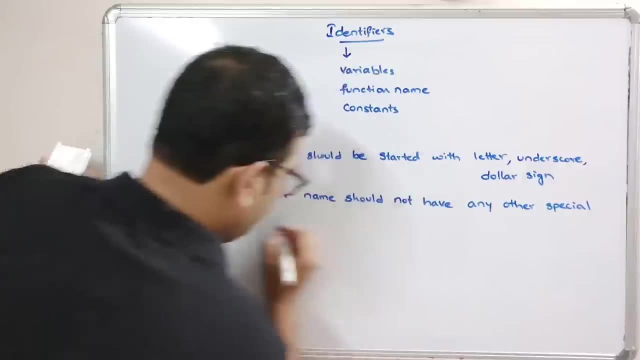 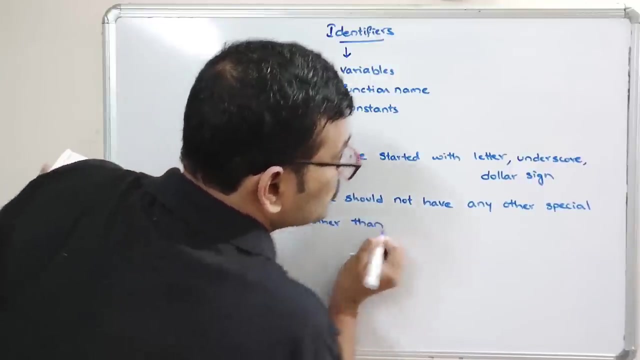 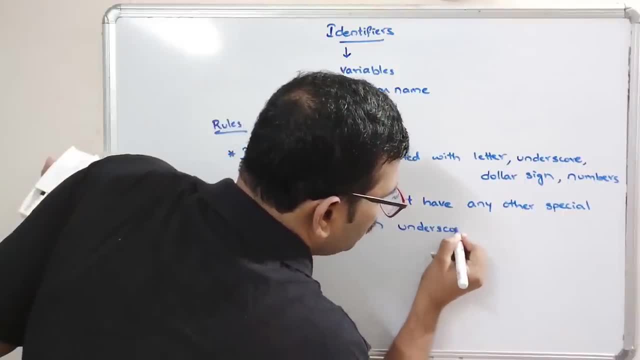 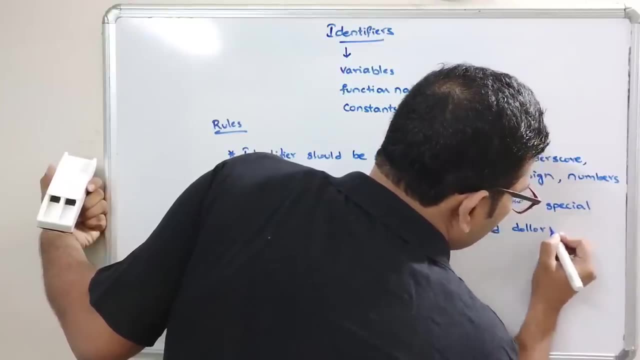 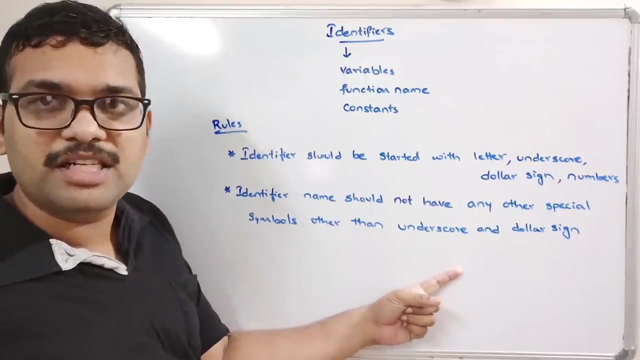 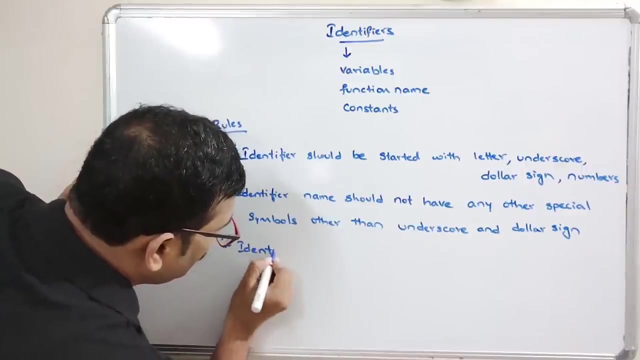 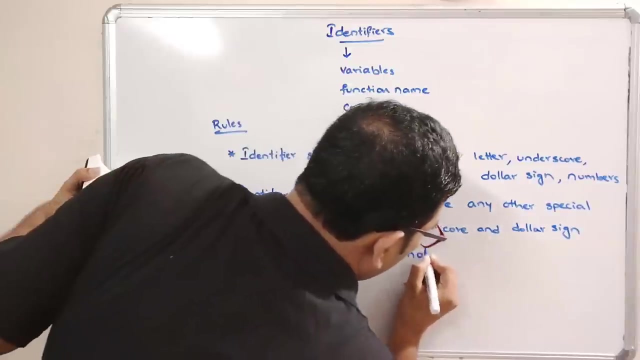 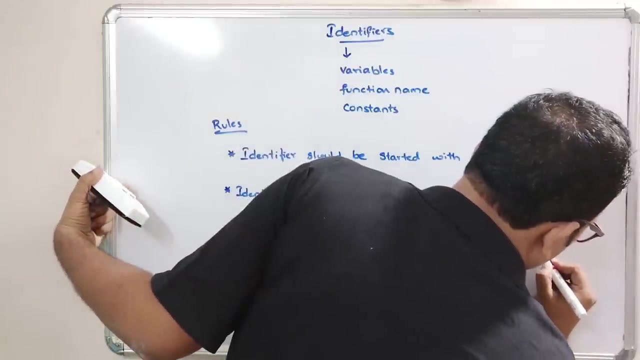 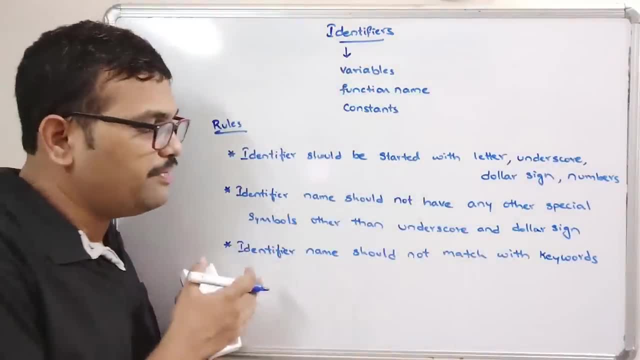 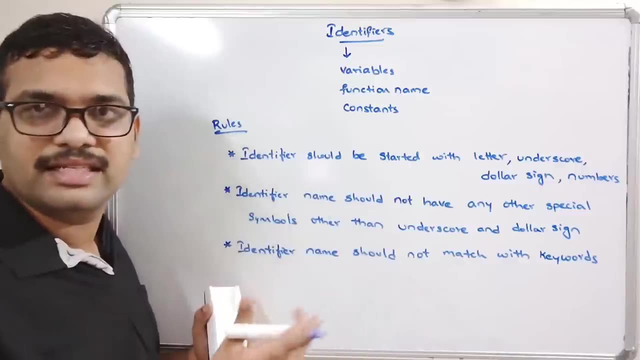 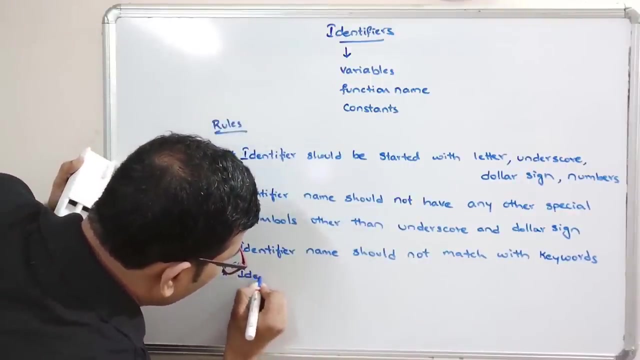 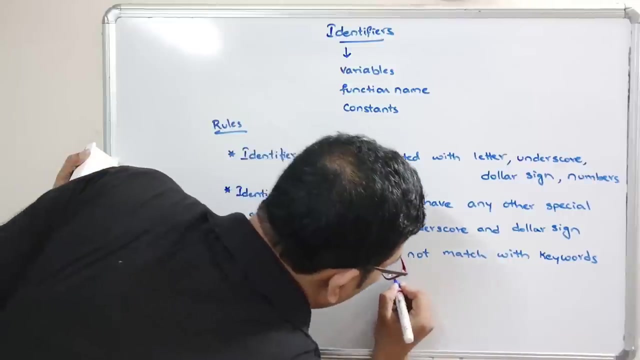 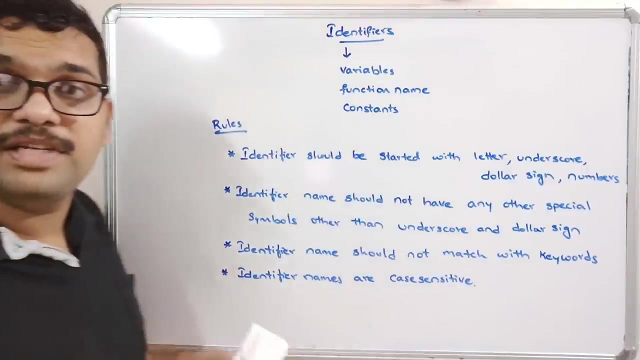 nothing but a reserved words. so these identifier names should not match with those keywords. so we have to know what are the keywords. so I will tell you the keywords in the next session, no problem. and the next one is identifier names are case sensitive. case sensitive means there is a lot of 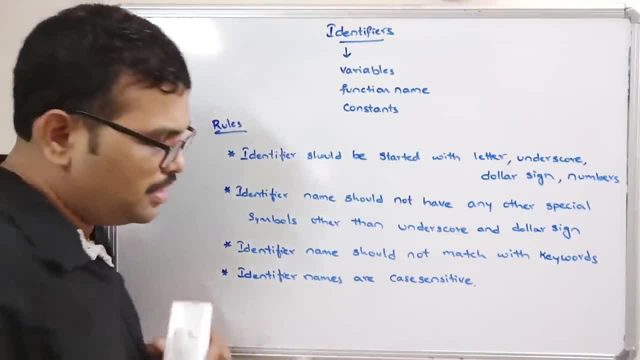 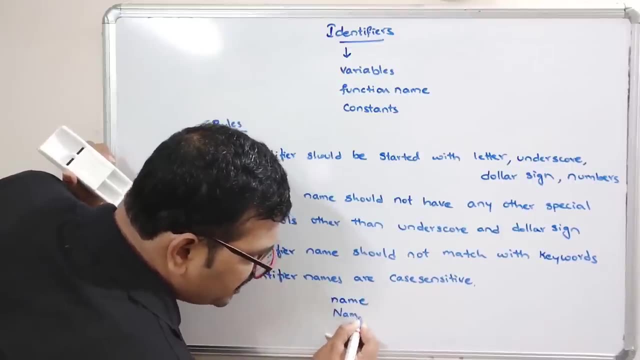 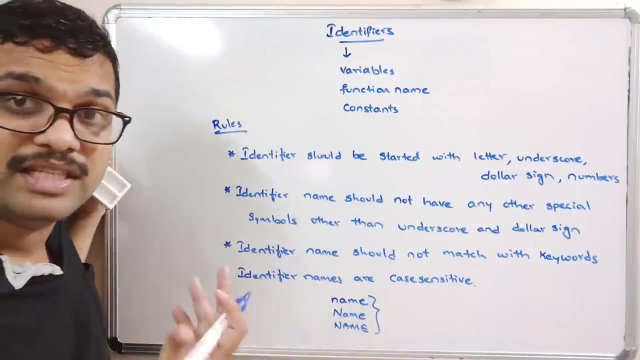 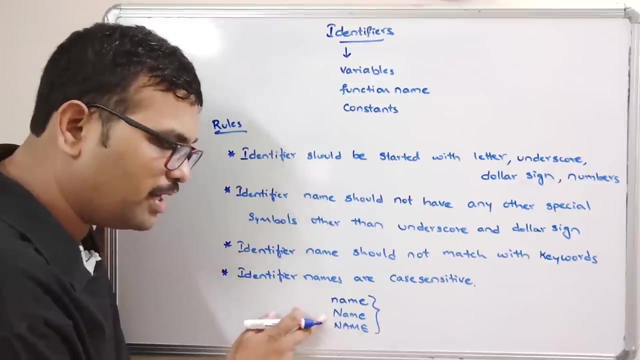 difference between the lowercase characters and the upper case characters. so, for example, if you are writing some name, so name is different, name is different, name is different, so all these three are different variables, three different variables. so even though we are giving the same thing, same variable, see, this is a name, this is name, this is name, but the 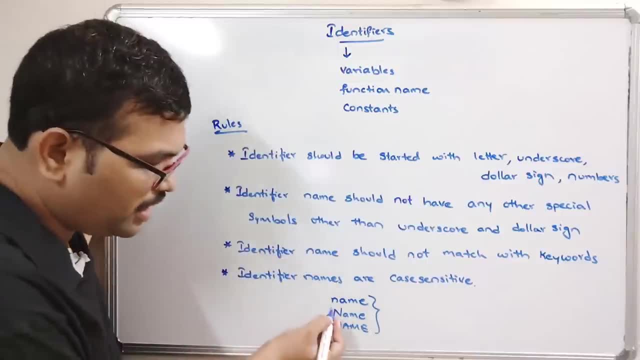 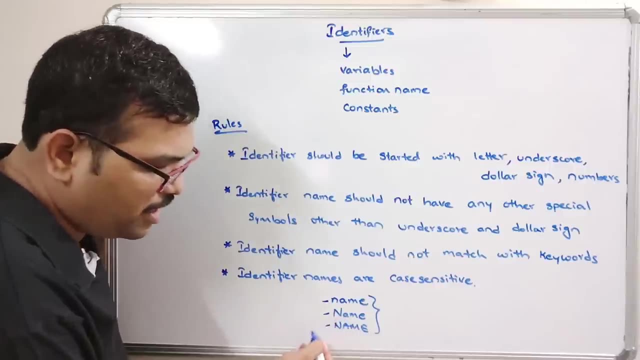 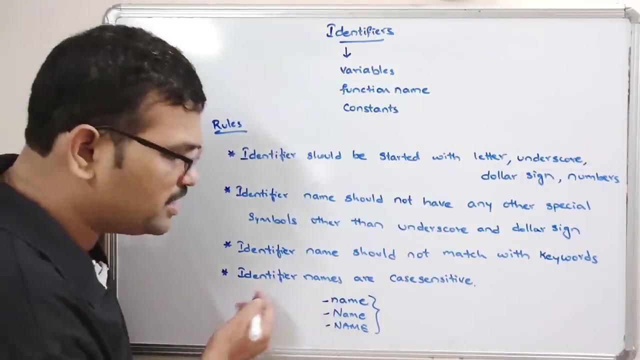 difference is between the lower characters and the upper characters. here all are the lower characters, and here the first character is a uppercase, and the remaining characters of the lower case, and here all are the uppercase character. so there is a lot of difference between the lowercase characters and the uppercase characters. so that's why these 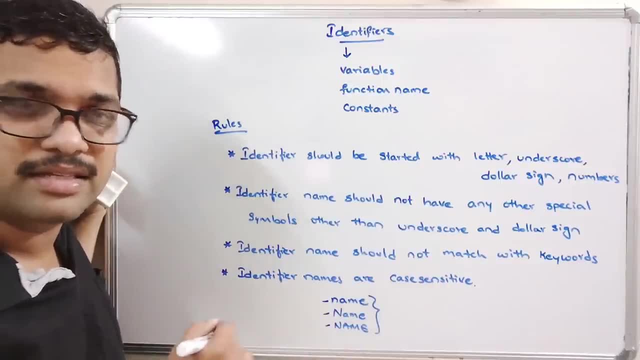 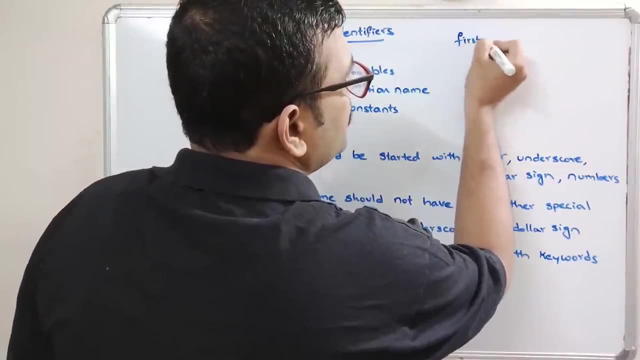 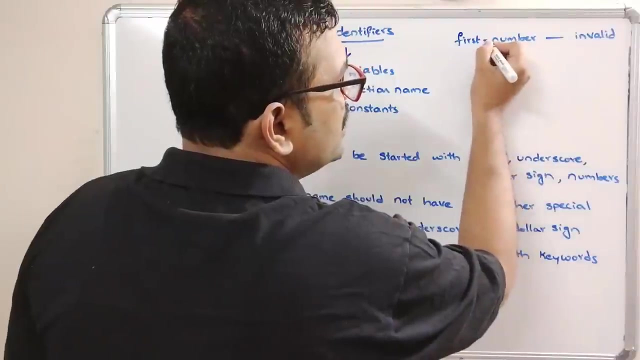 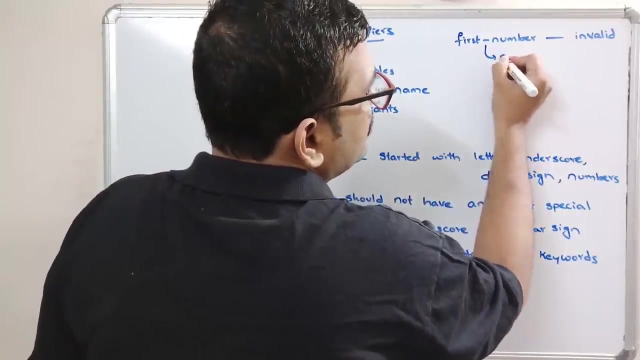 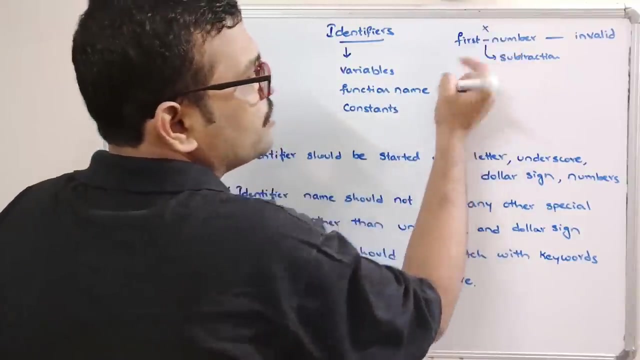 identifier names are case sensitive. case sensitive, so small examples. so if you take first number, so this is an invariant. this is an invariant because here we have given hyphen hyphen, not an underscore hyphen, so this will be treated as subtraction operator. it will be treated as subtraction, so it doesn't apply. so this: 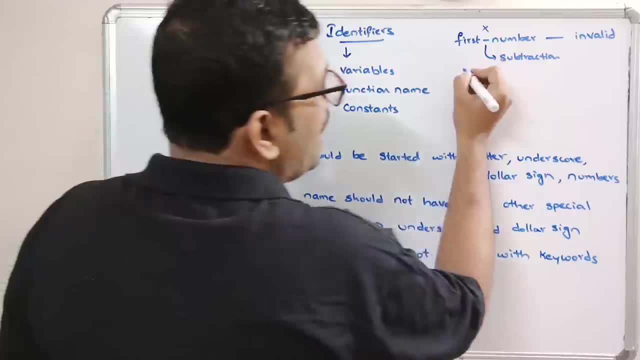 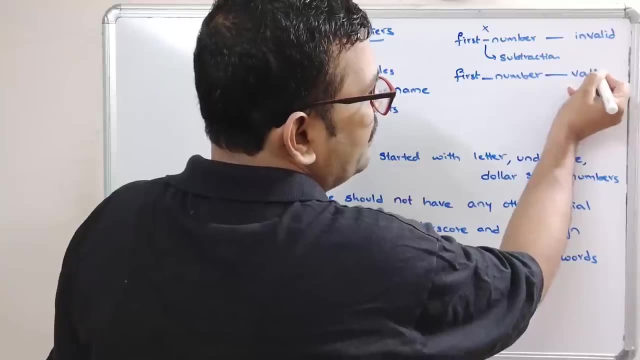 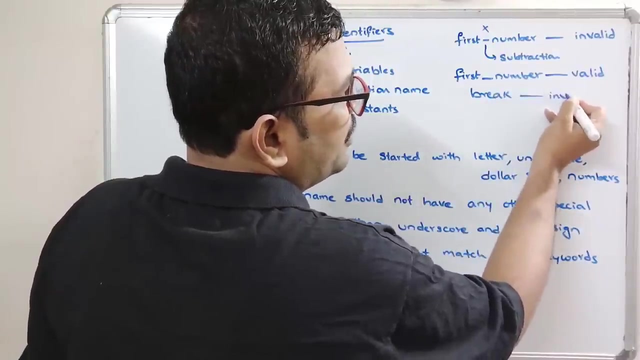 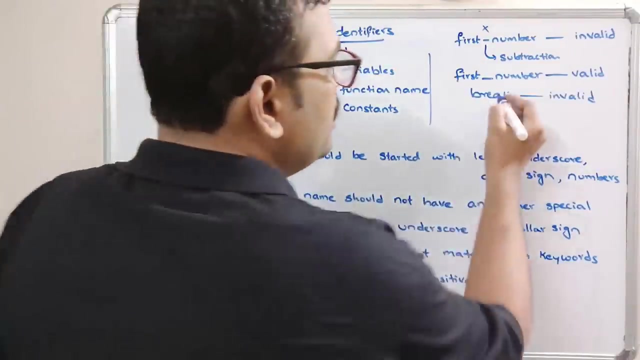 is an invalid identifier name. so the valid identifier name is: first underscore number, first underscore number. this is a valid identifier. this is a valid identifier, okay. and break is an invalid. this is an invalid, okay. so why this is an invalid? because break is a keyword. break is a keyword, so we should not use this keyword as an identifier, so break. 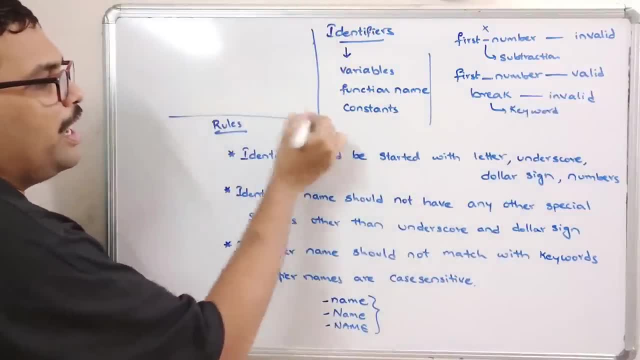 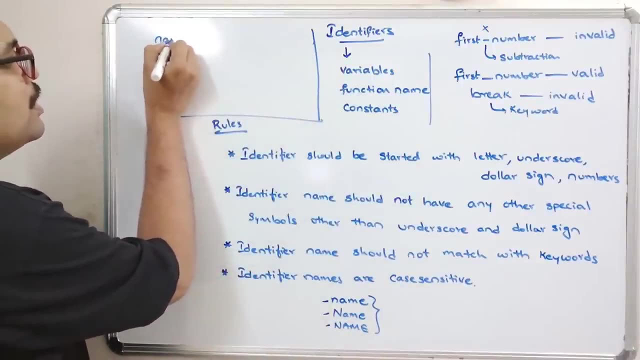 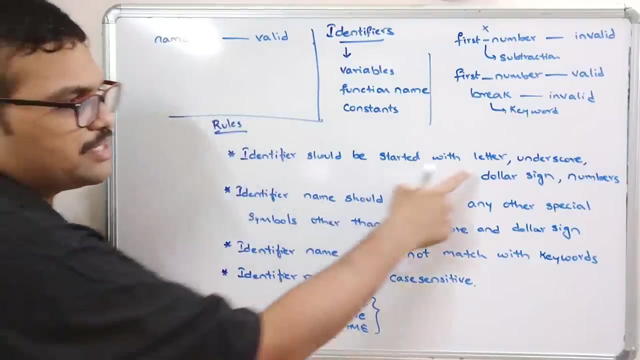 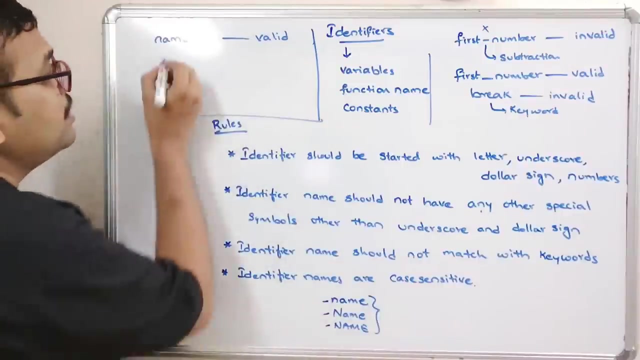 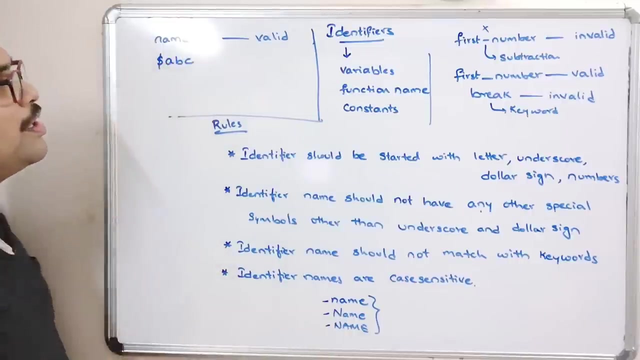 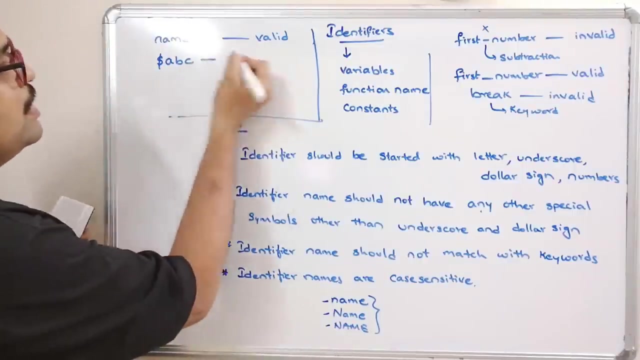 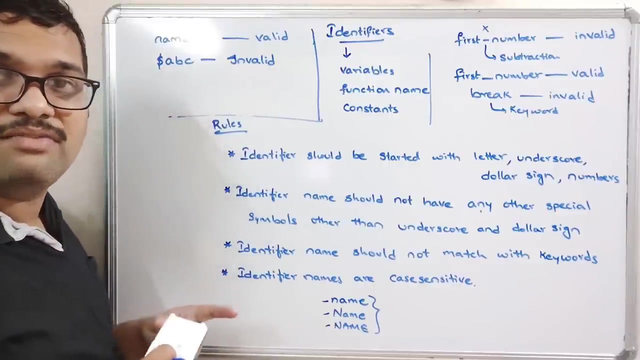 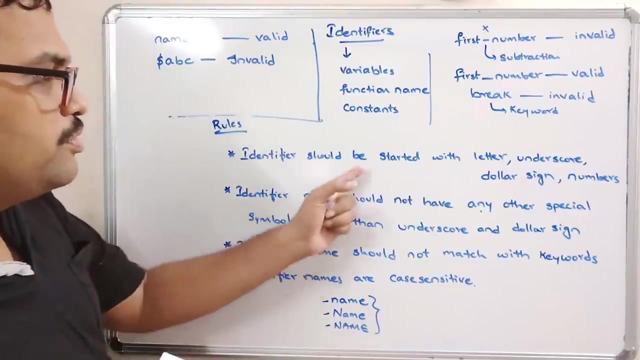 is a keyword, so I will show you the keywords, no problem. and the next one, some main one, two, three. so this is a valid because our identifier can be a valid identifier, because our identifier can be a valid identifier because our identifier can be a. This is a invariant because so our identifier name should start with either underscore or alphabets. I think we have written some wrong Name. should be started with letter and underscore. 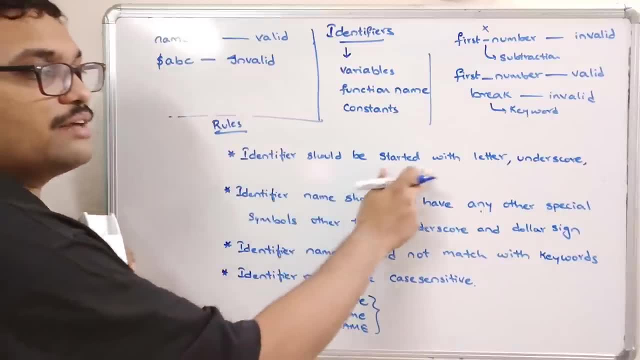 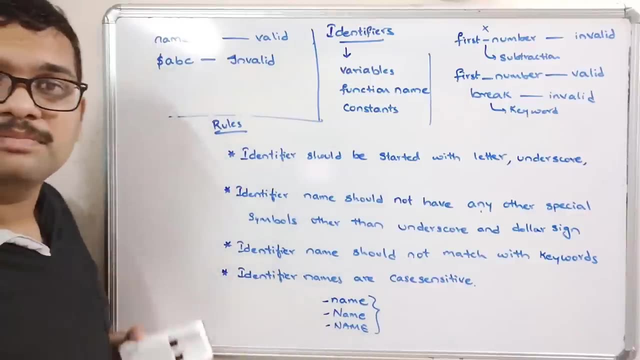 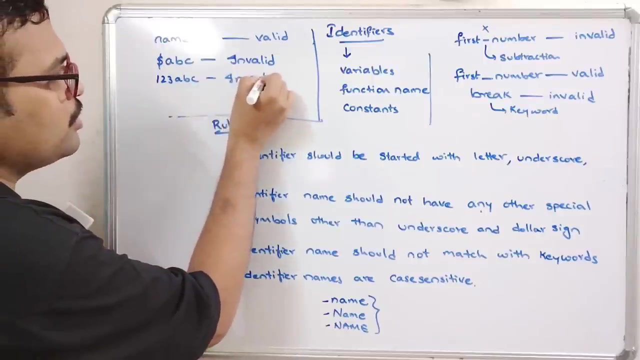 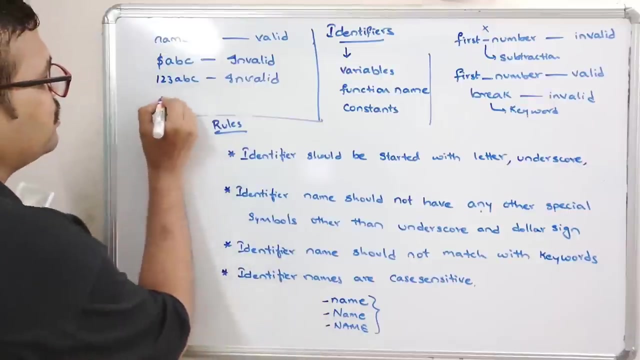 Okay. Letter and underscore. Identifier name should start with either letter or underscore. Okay, But not with number or any other symbol. Okay, For example, 123, ABC. This is also invalid. This is also invalid. So our variable name should not start with the numericals. It should start with either underscore or the letter. So underscore, ABC. So this is a valid. 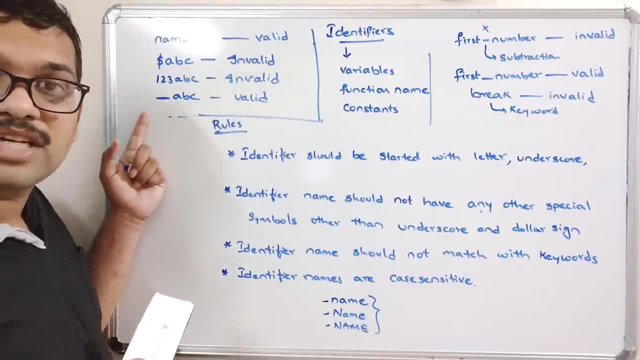 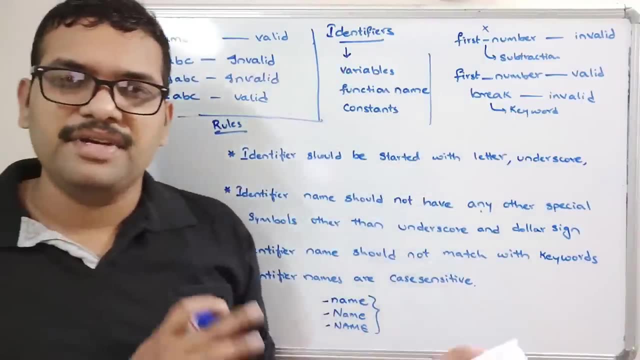 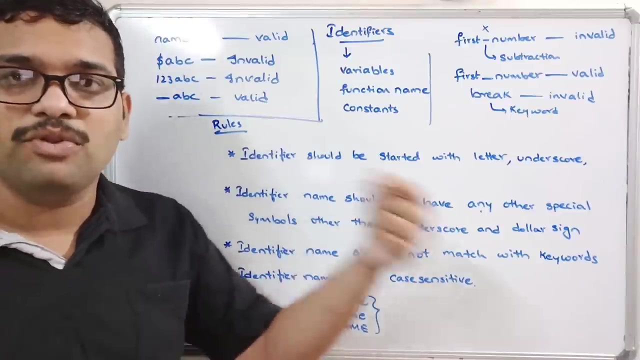 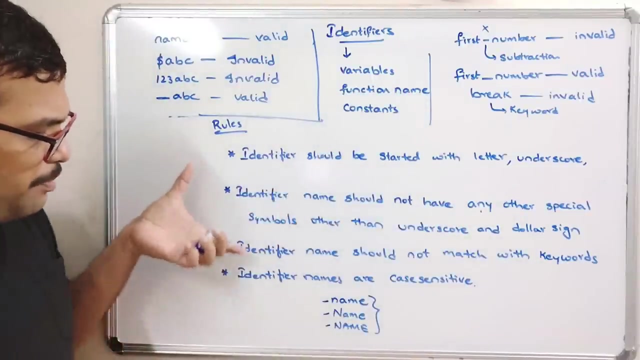 This is a valid because our identifier name starts with the underscore. So these are the few cases, just giving an example for valid identifiers and the invalid identifiers. So hope you got it. So we have to take care about all these rules while giving a name to the identifiers. Particularly, we are going to use the variable. So if you are giving a name to the variable, you have to just keep in mind about these rules. So we have to follow these rules and by applying these rules, we have to follow these rules. 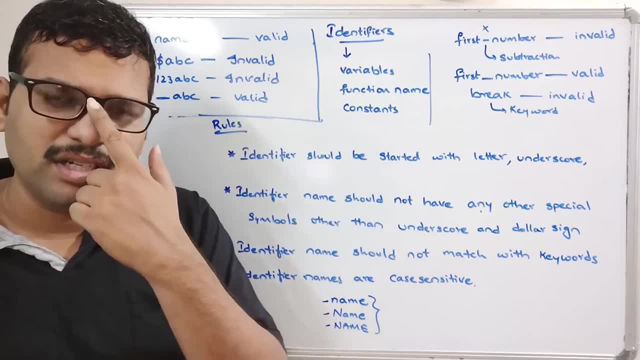 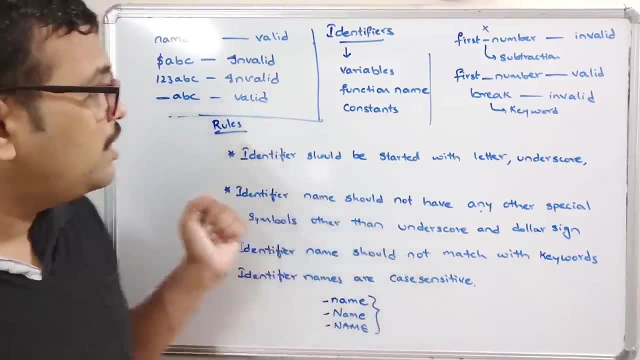 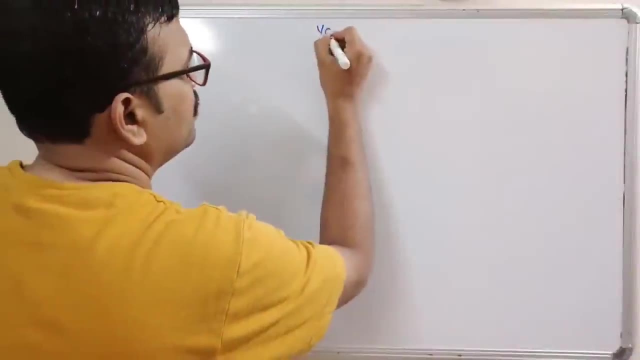 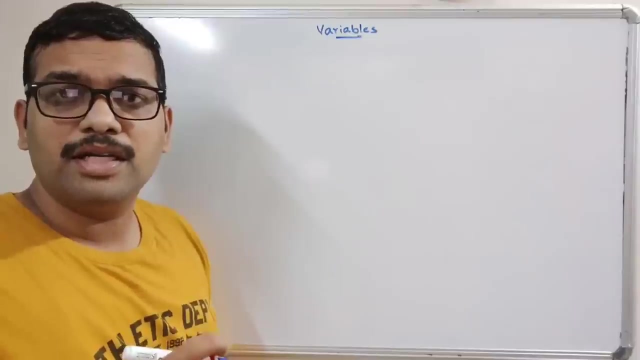 So we have to give the name to the variables, or if you are creating any function names, So for that also we have to go with the same rules, Right? So hope you understood. So we don't want to know that the variable is a memory location which holds the data. Okay, So we are supposed to store some data. 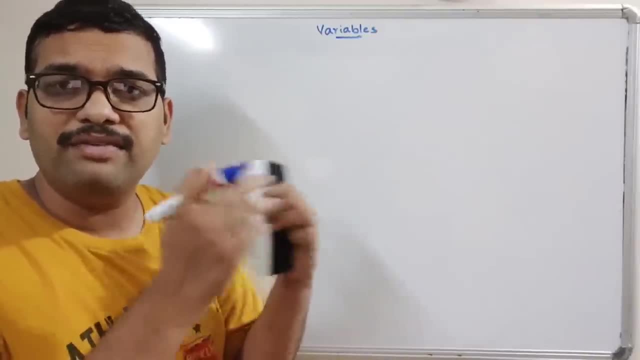 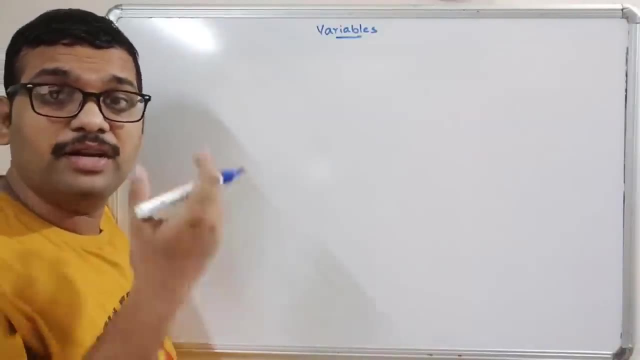 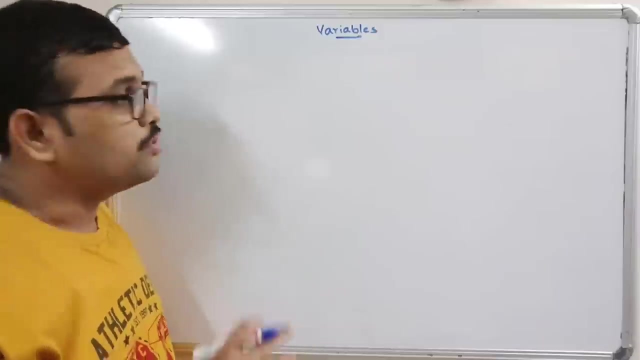 We're not going to write the data into that particular variable. So for that variable we are giving some names. Okay, So how to declare the variables in JavaScript. So in the previous sessions we have seen where to write the JavaScript. So the script tag can be written either in head tag or a body tag. Okay, So now how to declare the variables. So here we are having a keyword called VAR. 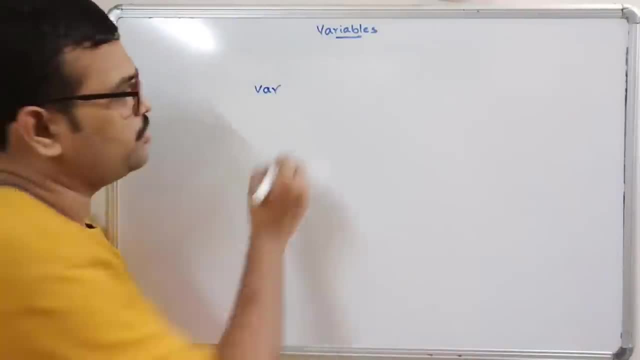 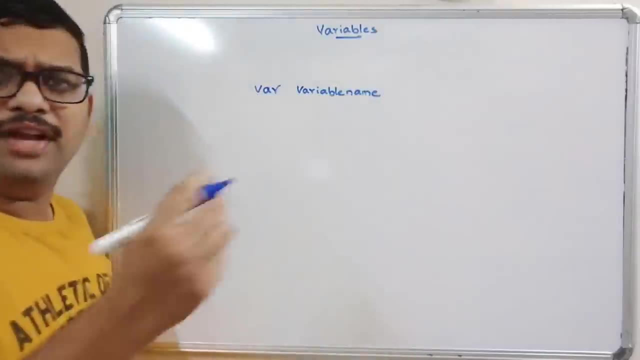 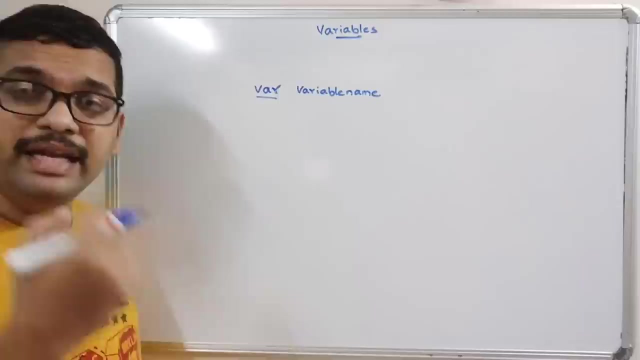 We are followed by the variable names means. So we can. we can declare a lot of variables by using this VAR Keyword. okay. So either it can be a string, It can be an integer, whatever it may be, irrespective of data type, We have to declare the variables by using the VAR. Okay, and initialization. So this is the declaration, right. 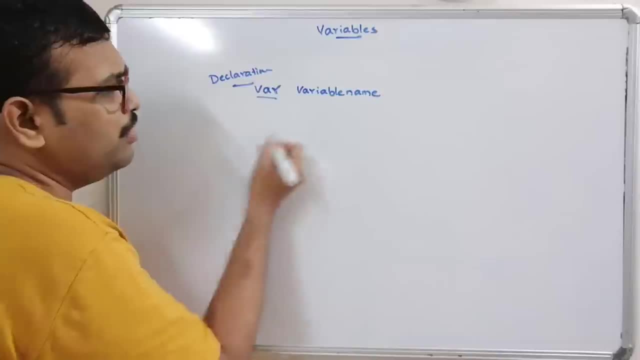 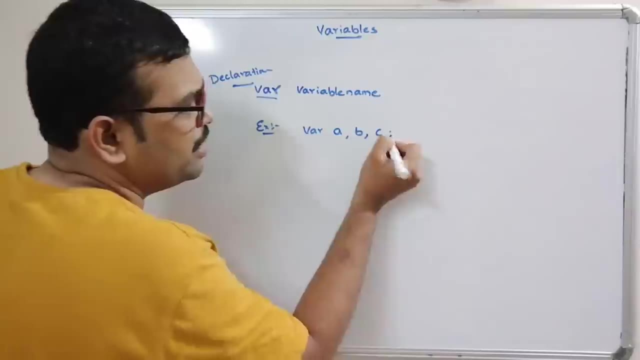 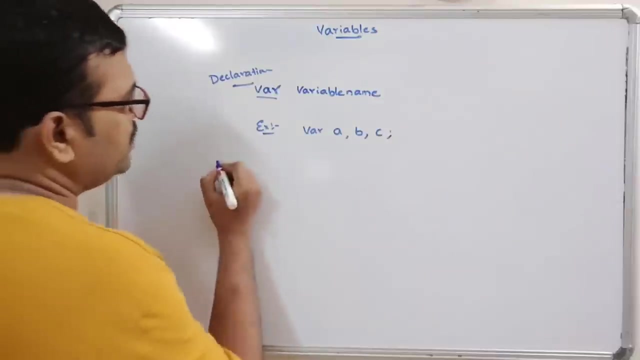 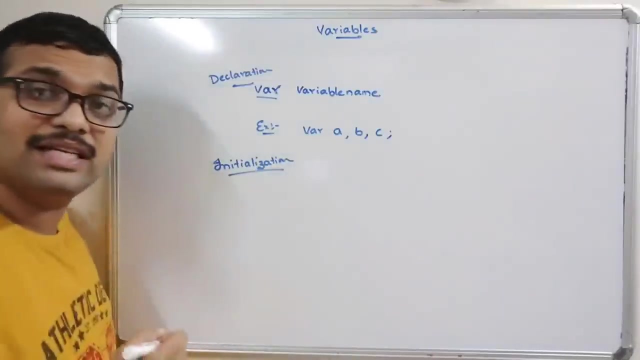 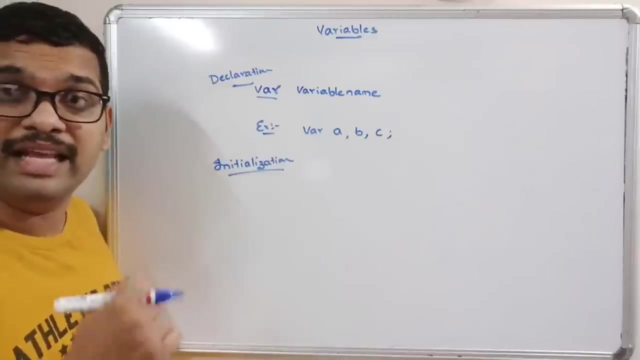 So this is the declaration. Now. so example for this declaration: so VAR: Some a, comma, B, comma, C, and here each and every line should end with the semicolon similar towards C language. now initialization, Initialization. so initialization means assigning some value to that particular variable. So we have to do some value to that variable. 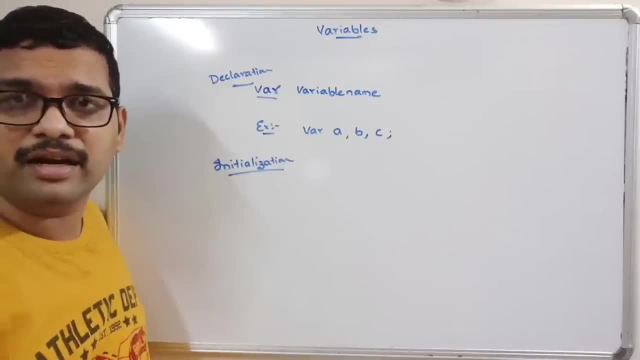 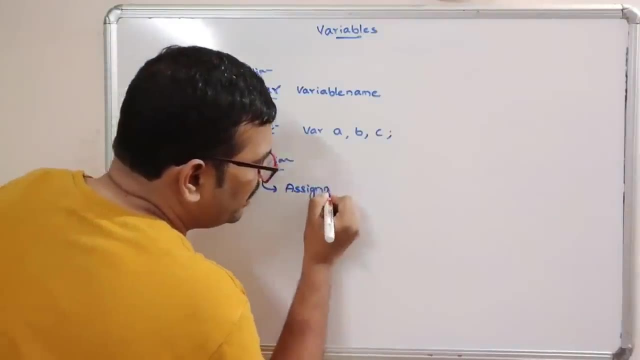 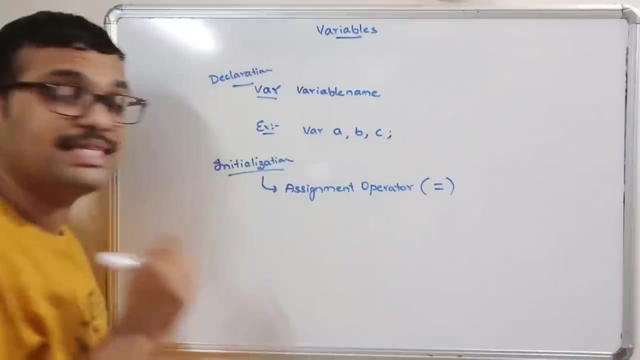 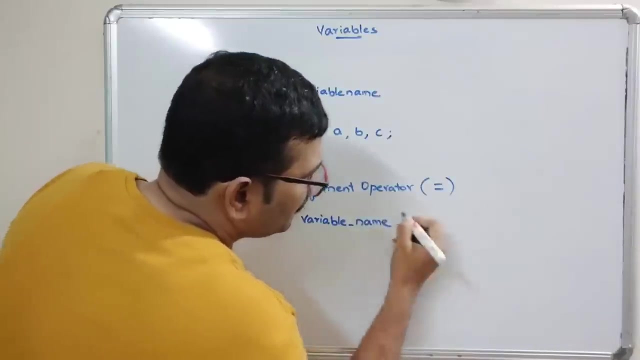 either it can be an integer or a string or any other data type, right, so this can be happen with the help of assignment operator. assignment operator. so what is this assignment operator? so assignment operator is nothing, but is equal to a single, is equal, right? so the variable name. the variable name is equal to value. 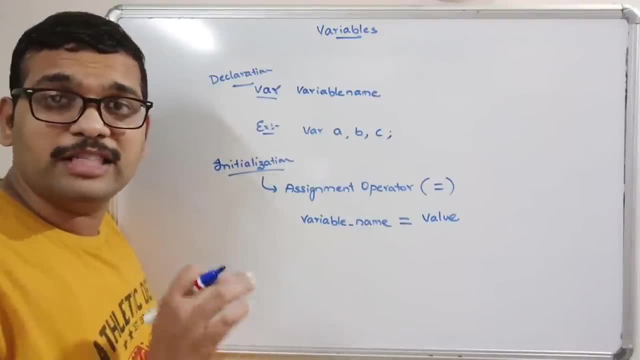 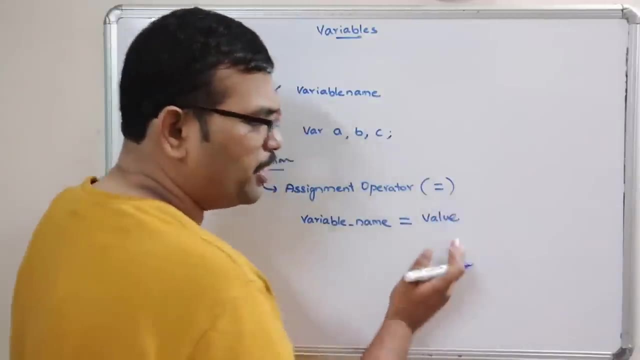 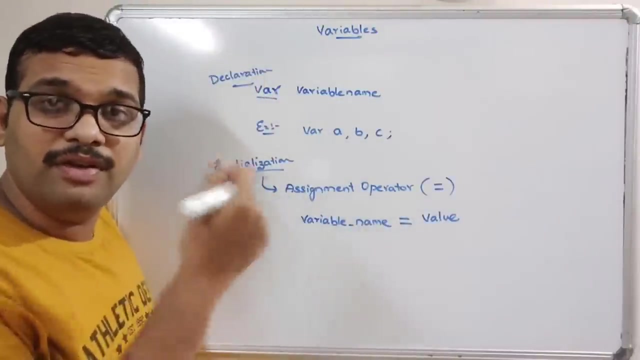 variable name is equal to value. so whatever the expression we are using, we have to use this assignment operator. so on the right-hand side of this assignment operator is the value and the left-hand side of this assignment operator will be the memory location. that's a variable name. so if you are, 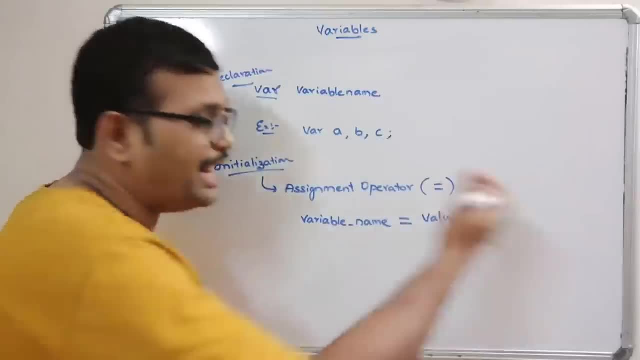 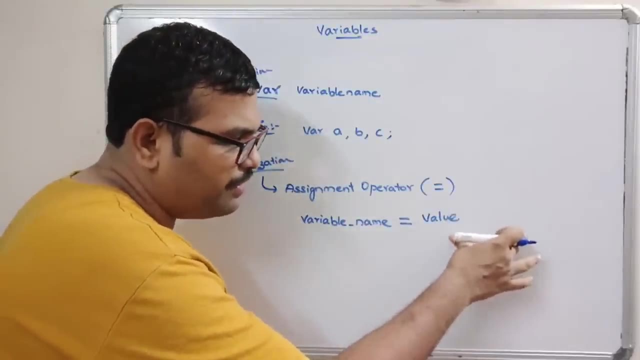 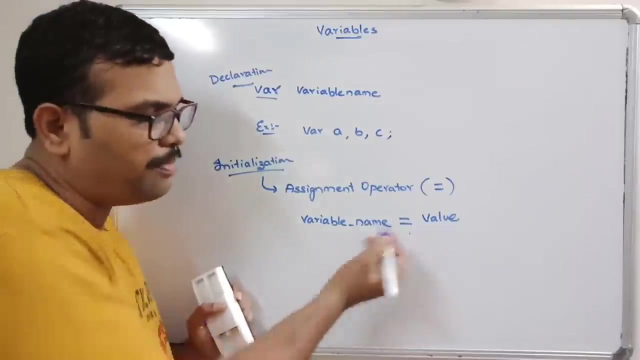 using some expression, the left hand side will be the memory location and the right-hand side will be the expression to be evaluated, right and that expression will be evaluated and the complete result will be stored on the table Variable which is given at the left hand side of the assignment operator. 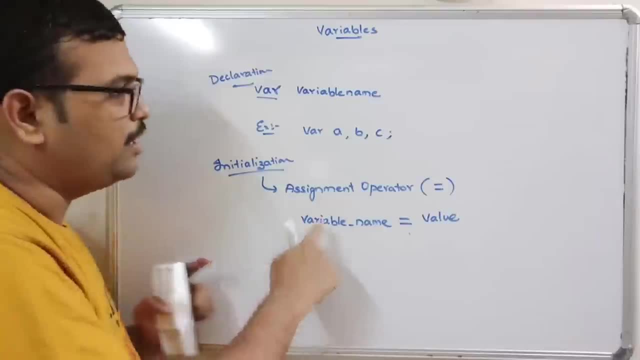 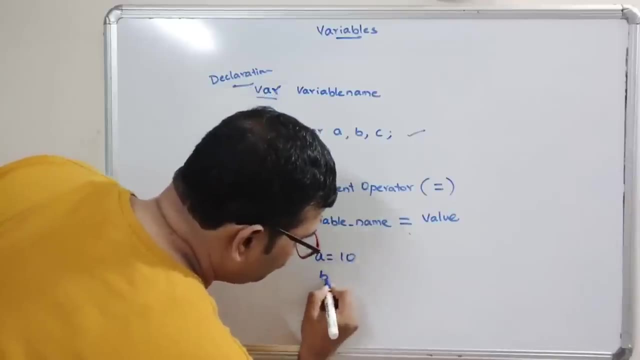 So this is how we assign the value to the variable. For example, here we have declared three variables: a, b and c. Now we can give some: a is equal to 10, b is equal to 20, c is equal to 30. 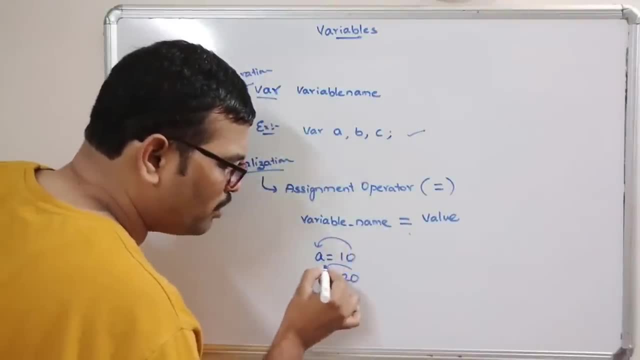 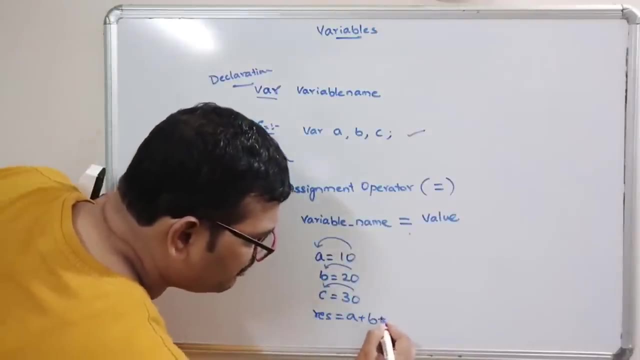 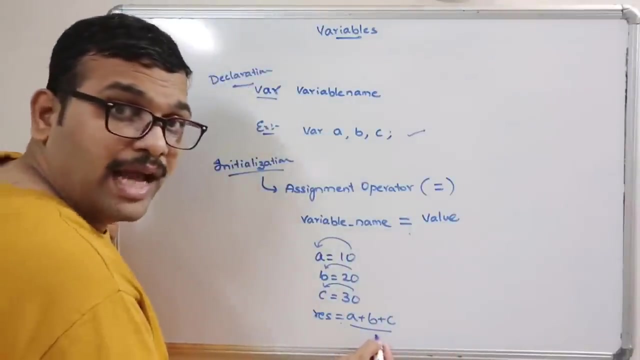 So 10 will be stored into a, 20 will be stored into b, 30 will be stored into c, And here the result is equal to a plus b plus c, So the complete addition. So on the right hand side of this assignment operator, the evaluation will be done and 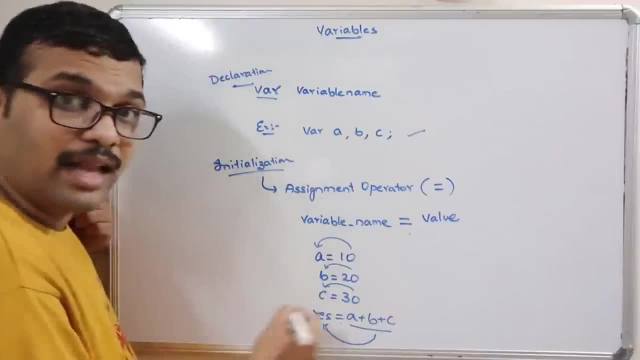 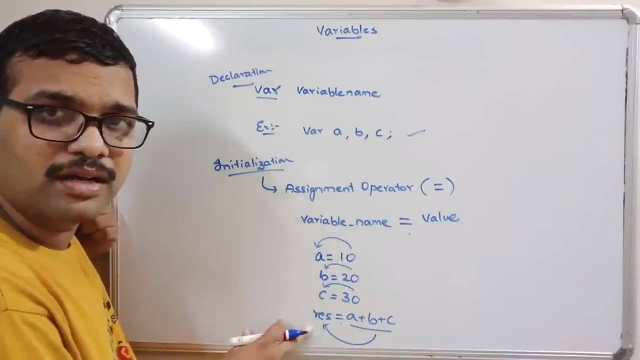 the result will be stored into the right hand side, the left hand side- variable name. That is a memory location. This is a memory location where we have to store the data. So this is how we can declare a variable and initialize a variable. 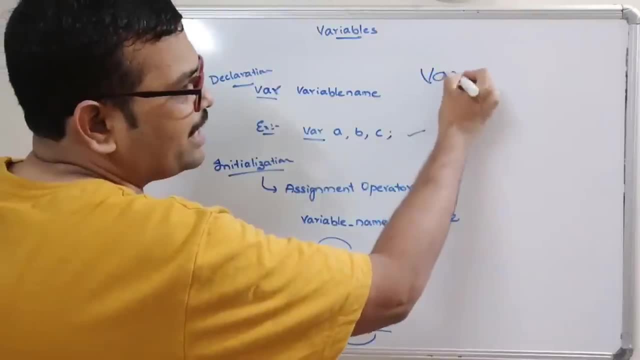 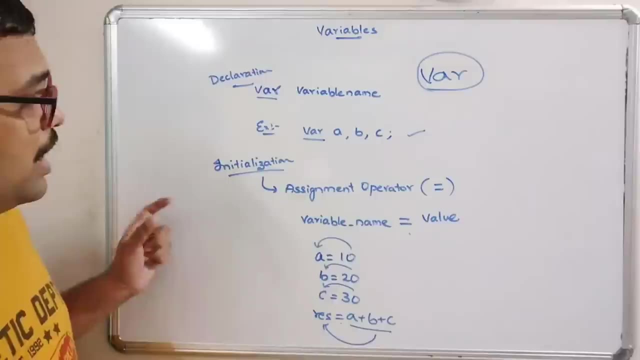 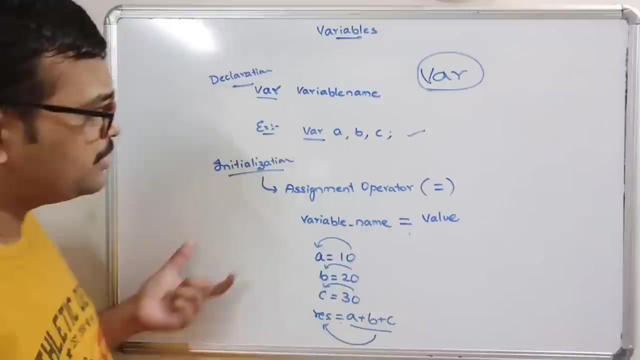 So only Only one keyword, that is var keyword. Var keyword is used to declare the variables, Right? So I will give you a small example. Let us see some addition of three numbers, So I will explain. I will write the code for addition of three numbers by initializing some. 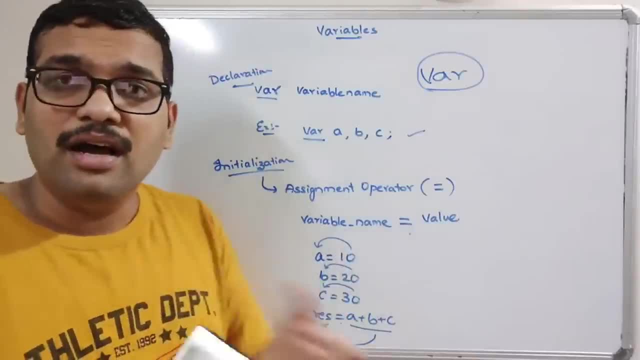 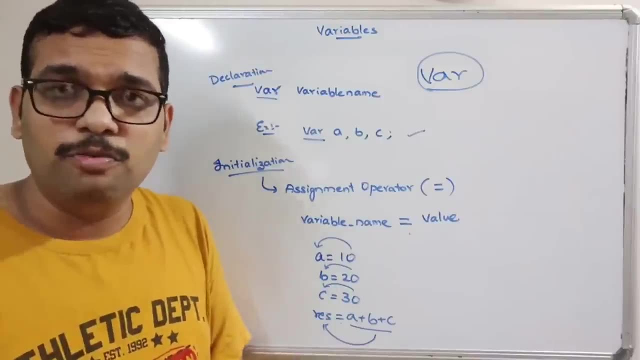 by declaring some three variables and initializing some three values, And we have already seen the different types of outputs, possibilities, Right, So how many ways we can write the output on the screen. So by using one among those output functions, we will see how to print the result on the 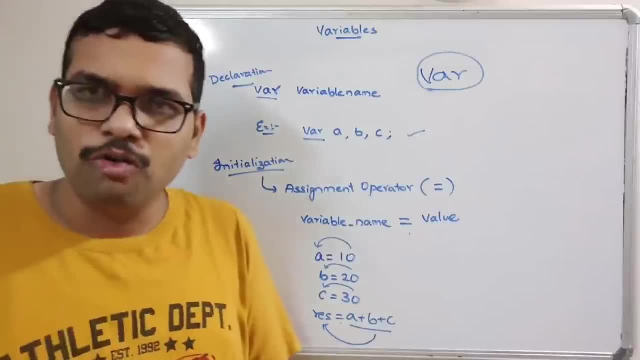 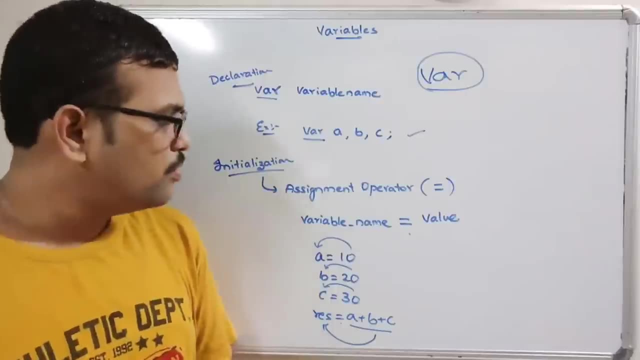 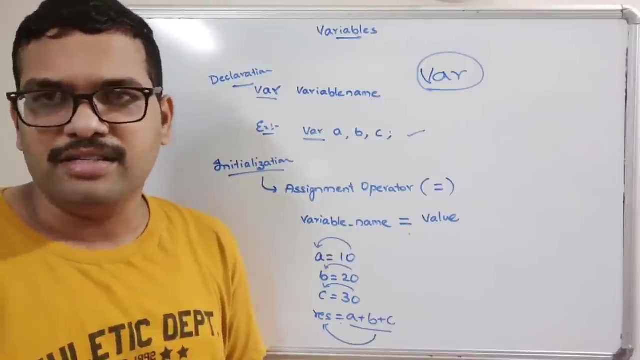 web page And I will give the link of the output possibilities in the description section so that you just follow that link and you just know about this. output functions like documentwrite, windowallet, consolelog or lrhhtml. So there are a number of ways we have seen. 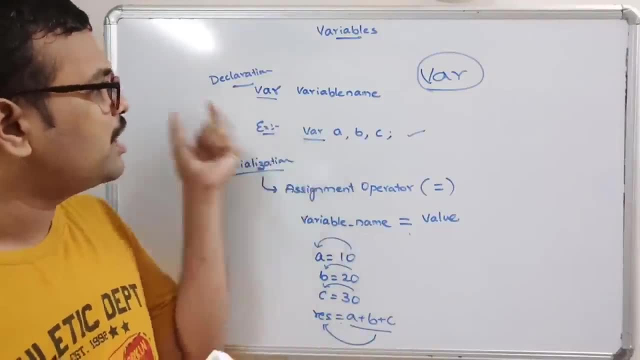 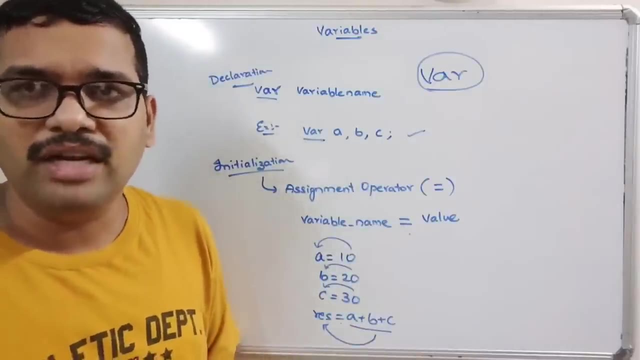 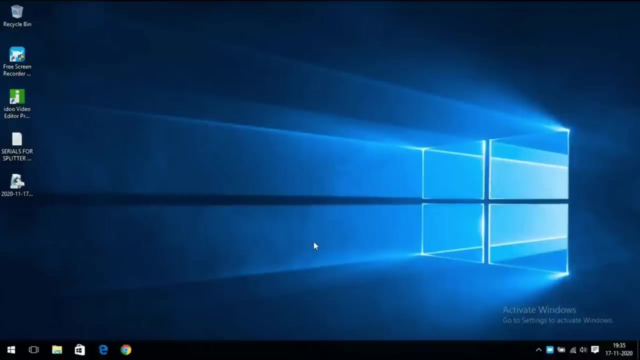 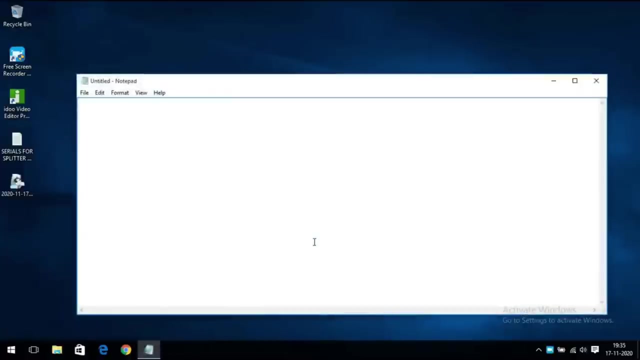 Right, So let us. Hello friends, So just now we have seen how to declare the variable and how to initialize a value to the variables. Now let us write a small HTML code. So in that we will write some scripting and in that we will declare some variables and we will initialize, and we will see. 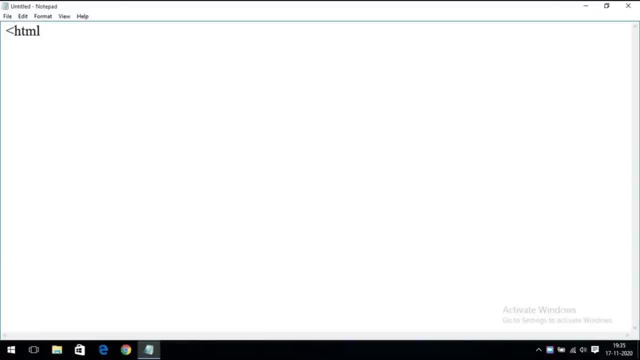 Right, So let us move on to the system of this thing. so first let us start with the HTML content, so HTML tag. so inside the HTML tag we can, we can write the script. so whatever the JavaScript that should be written in script tag, and that script tag can be included either in the 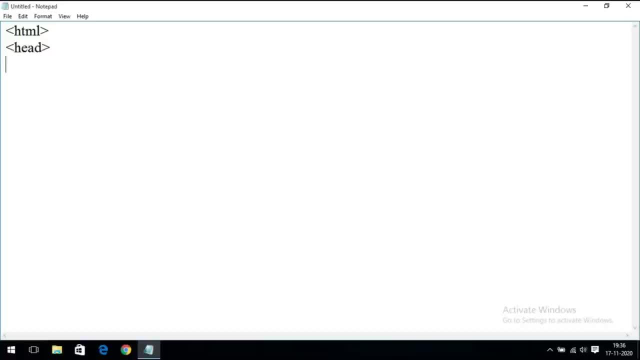 head tag or body tag. now we will go with the head tag, okay, head. inside the head will write the script and here we will write some variables. so each and every variable should be declared with the keyword VAR, VAR, followed by a, comma B, comma C. so these are the variables. okay, and keep the semicolon. so here each and. 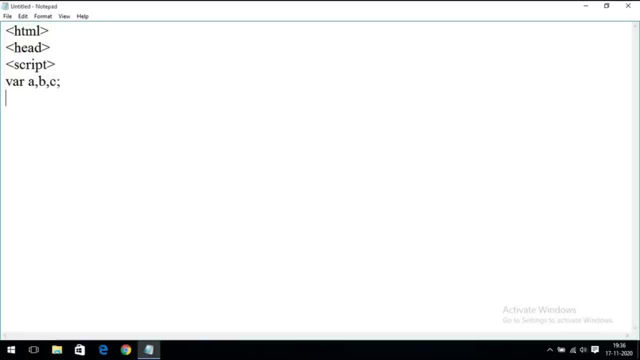 every statement to should end with a semicolon, and I will initialize some values. a is equal to some 10 and semicolon B is equal to 20 semicolon and C is equal to 30, right, so three variables, and now write the expression some result is equal to. 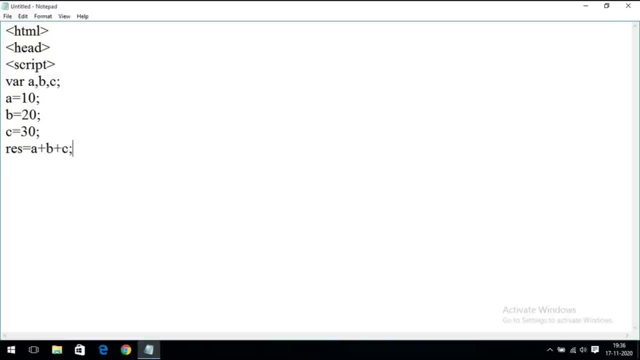 B plus C. now I just want to display on the screen so document dot write: sum of three numbers is comma. result: okay and close the script and close the head, open the body and you can write the body. so whatever the thing you can, you need, you can write. so I will write in h1. so 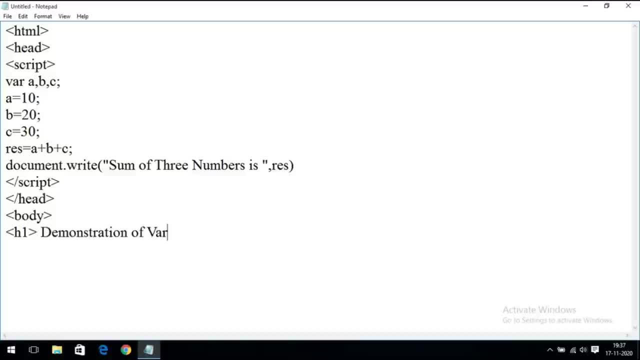 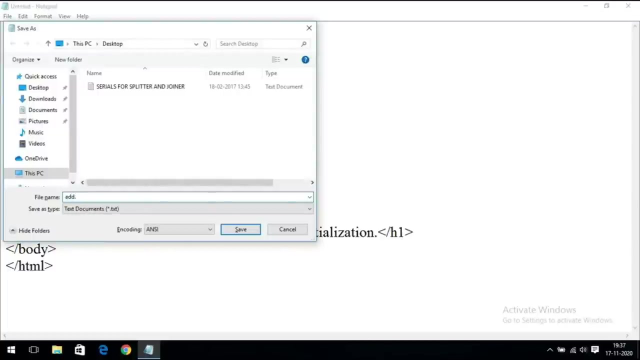 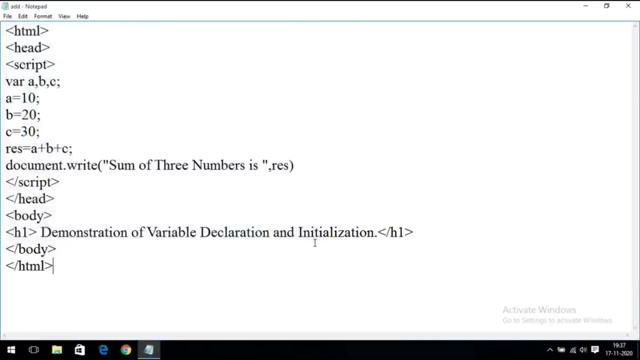 demonstration of variable declaration and initialization. and close the head tag and close the body tag and close the HTML tag. so this is a small thing in order to find the addition of three numbers. so add dot HTML. so this is a basic thing. I am just demonstrating how the variables can be declared and initialized. okay, so 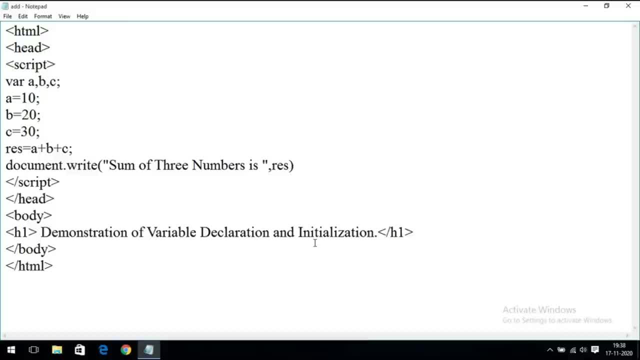 in the further sessions we will see how to get the values from the existing content, existing elements. so, for example, take some forms. so in the form you just enter the number so that that number will be initialized to some variable and that will be evaluated in the expression right. so 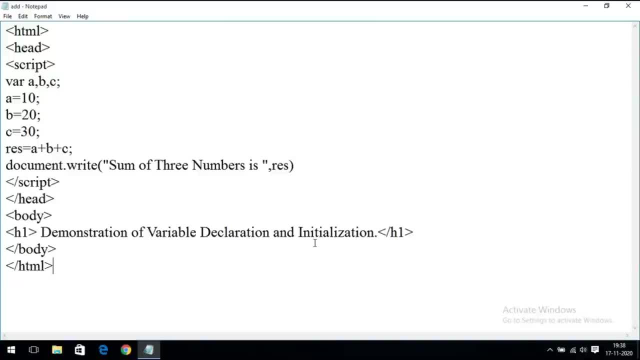 So all these things will go in the further sessions. So in this session I am just concentrating on how the variables will be declared and how the values will be initialized. So variables will be declared by using the var keyword and initialized by using the assignment operator. double is equal to. 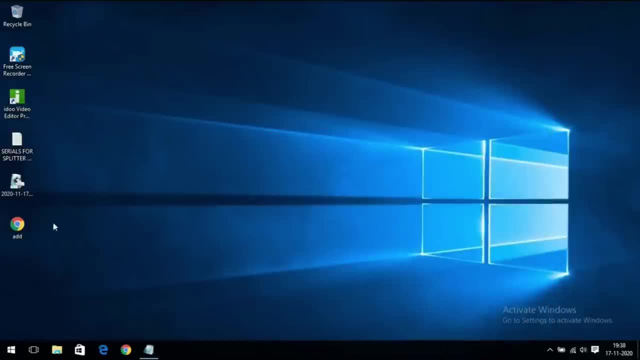 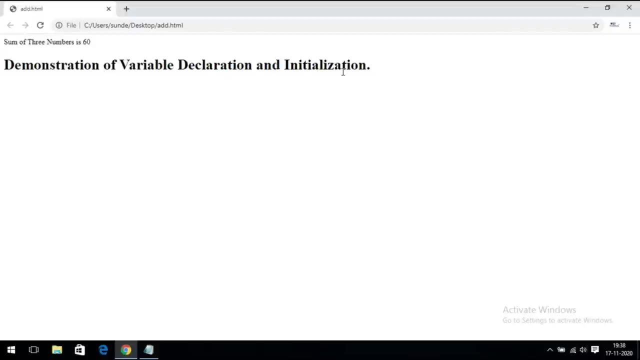 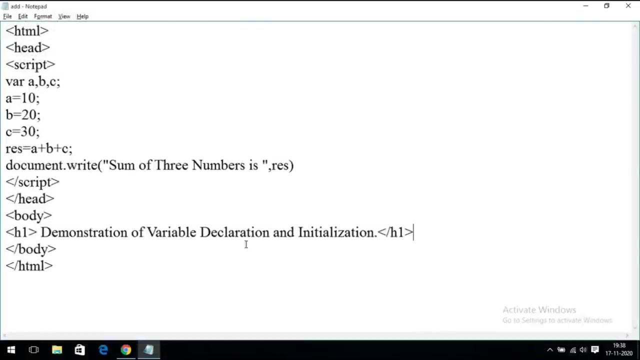 So I will save this one and let us execute this one so that the content will be displayed directly on the web page. See, you can observe here, sum of three numbers is 60. So demonstration of variable declaration and the initialization, And this we have seen. and also one more thing: we can create a button and after clicking, 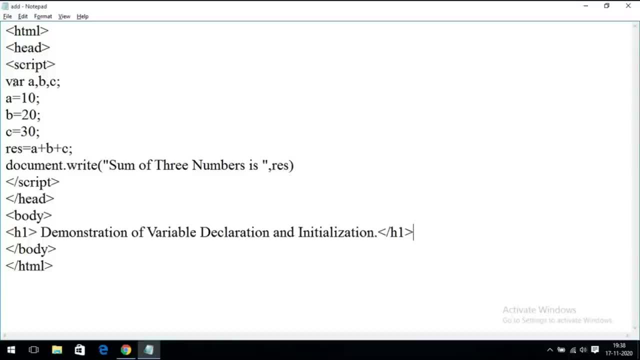 the button we can write the onClick property, So we can call the function here. So in the script we can write the function in the script, in the script tag, So implement everything in the button. I mean in the function. So function, add. So add is the function I am just calling, and after this one I am just ending the thing. 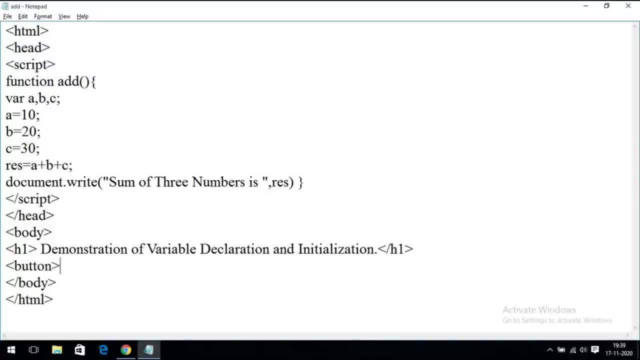 So now I will just create a button, So button type is equal to button, and go with the onClick property. onClick is equal to, So add button. Okay, Add function, So add, So just go with this one. Write down the text to be displayed on the button. 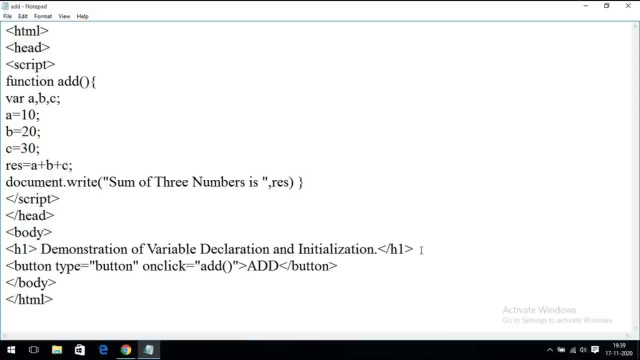 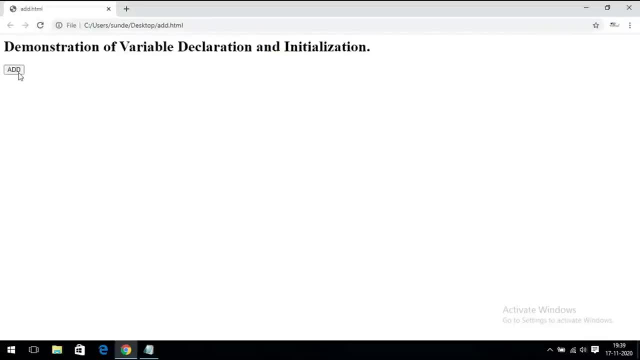 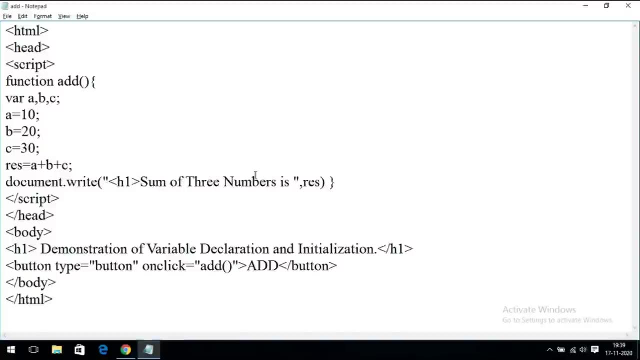 Add- Close the button tag Right Now. if you execute this one, so we will get a button here, see Add. So if you click on this add, We will get the result. Sum of three numbers is 60. So you can also apply the tags here. so h1, h1, right. 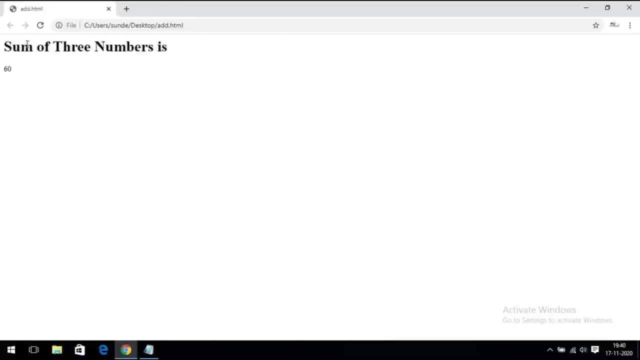 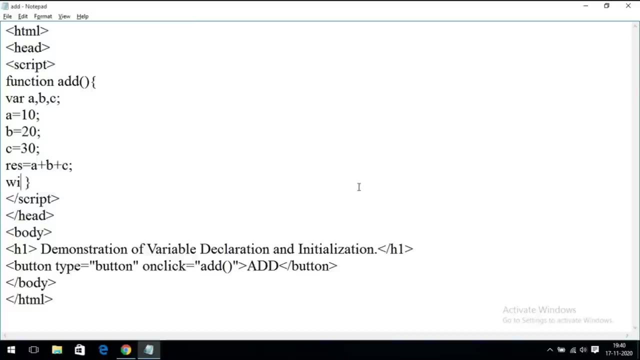 So that will be applied here itself. So after clicking on this one, you can get sum of three numbers: is 60, right? or else instead of writing all these things, you can simply go with window dot alert. So we have seen different output functions, Okay. 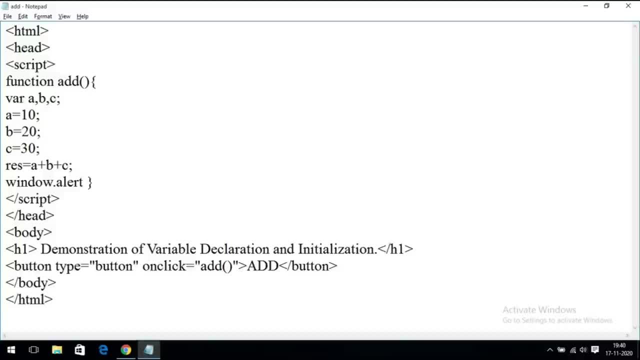 So we can also use the inner inner HTML. I have already explained all these output statements in the previous session, So I will just post the link of these output statements So in the description section, so that you just refer to that, so that you will get an. 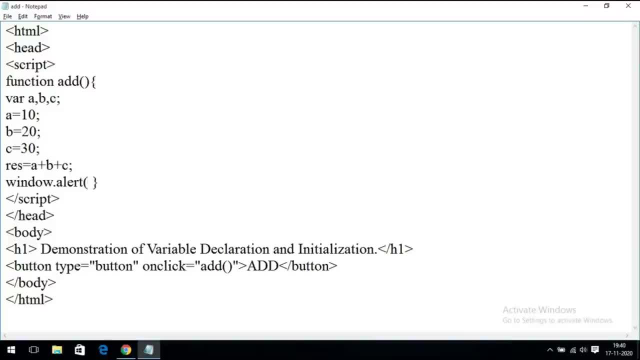 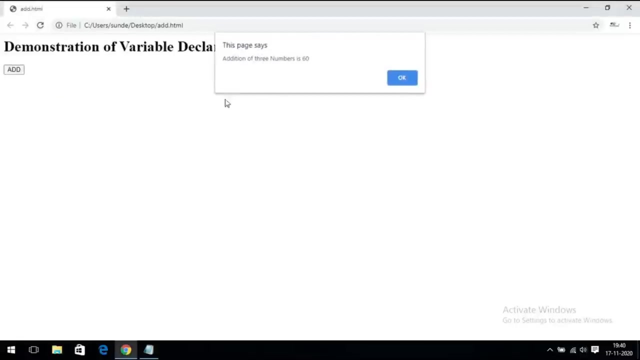 idea how many ways we can display the output on the screen Right. So window dot alert. Give here Addition of Three numbers Easy. Now you can observe here: if you click on this add, we will get an alert box. Okay. 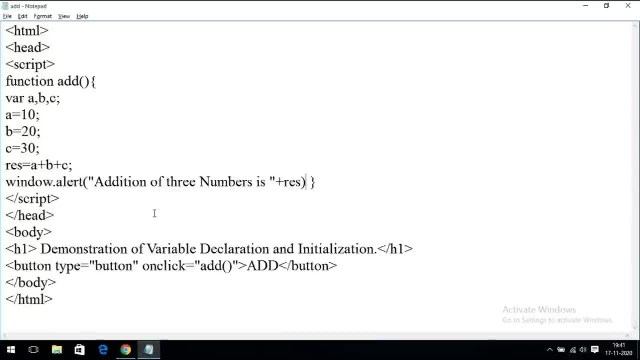 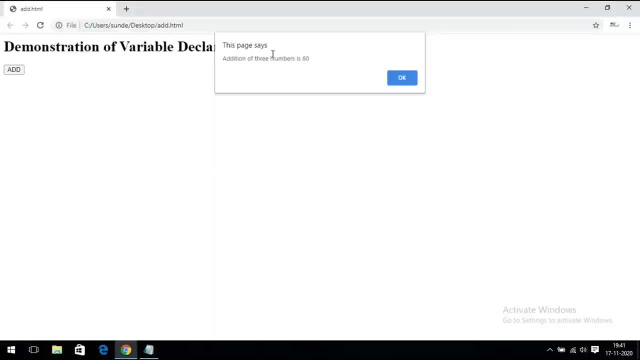 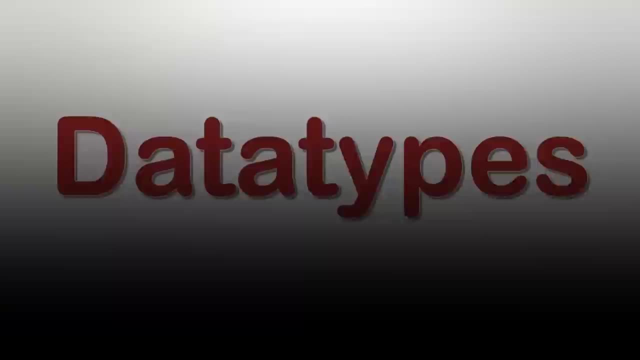 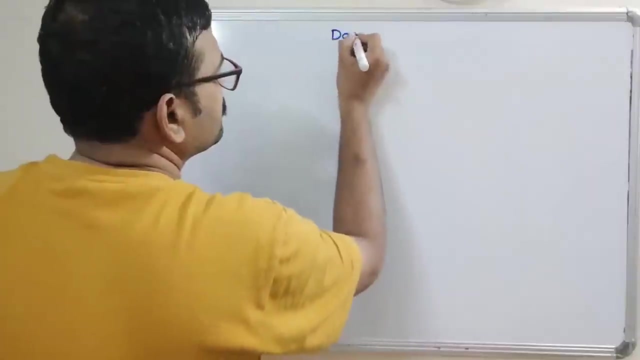 So previously we have written some document dot right so that it will directly write the content on the web page. But now, and just using the alert box- alert box so that it will be displayed here- It will be displayed here, Right. So hope you understood this session. 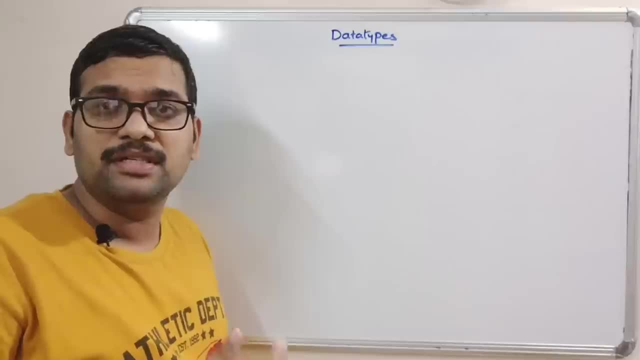 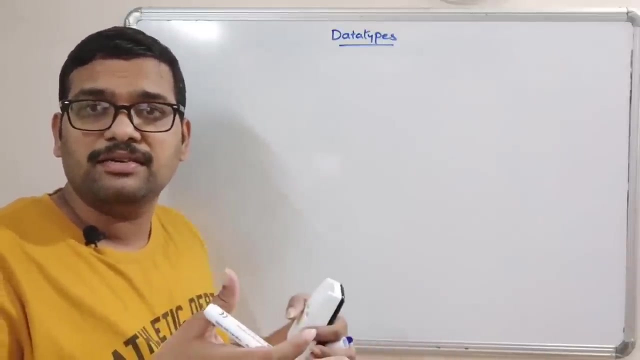 So data type means So in other programming languages. this data type is very important because so we have to declare the variable in one particular data type depends upon the value which has been initialized to that particular variable, Right? So if a variable holds the integer value, 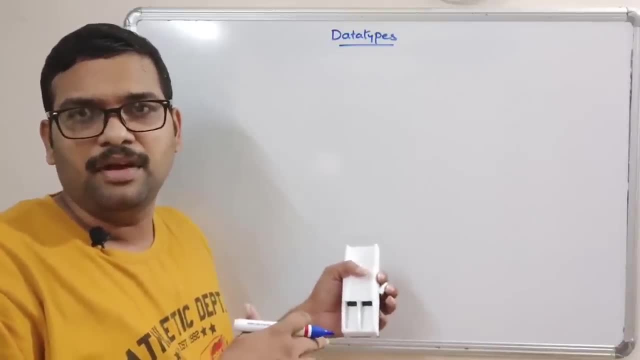 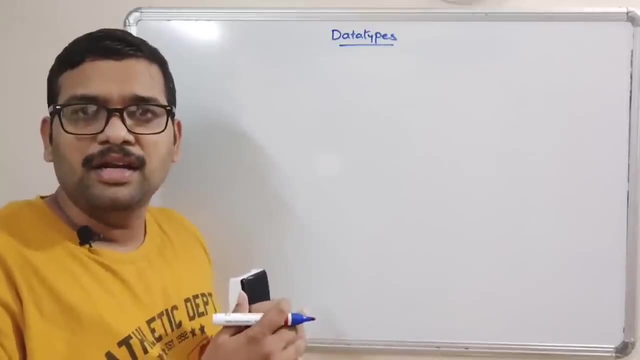 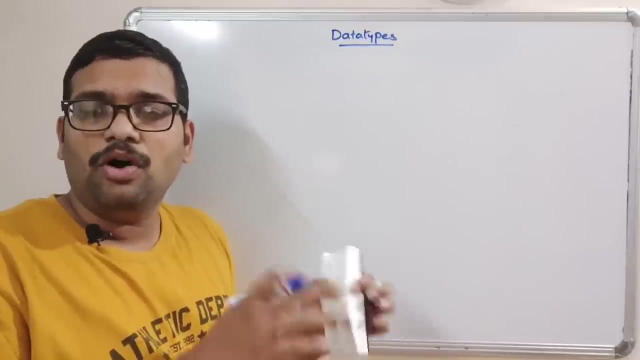 So we have to declare that particular variable using integer data type. If the variable holds the string value, we have to declare using some character data type, Right? So here, Whatever the data type, that means whatever the value we are storing into the variable, all the variables should be declared using only one keyword, that is, that, where followed. 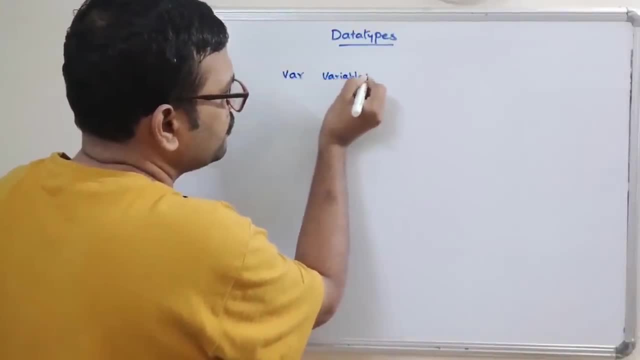 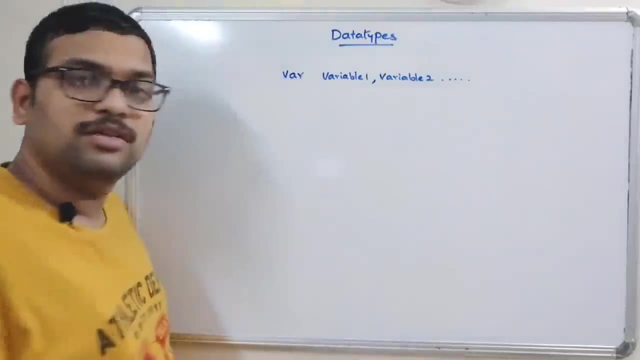 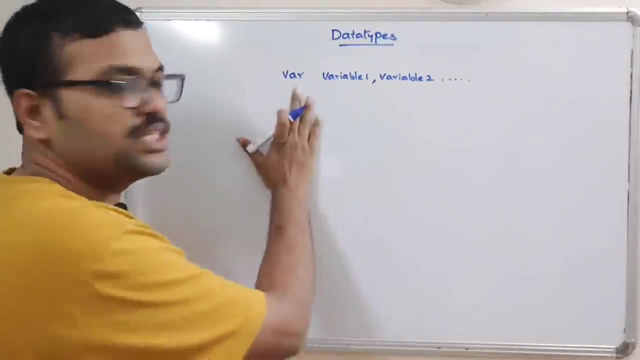 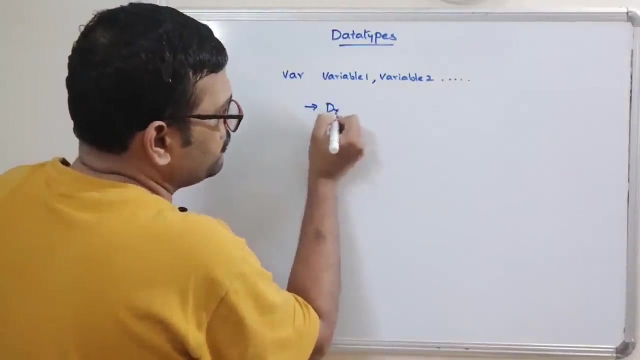 by Variable one Comma, Variable two, Etc Right. So, irrespective of the data, irrespective of the data, we have to declare the variables using the keyword that and in the in JavaScript, data types are a dynamic data types. dynamic data types. 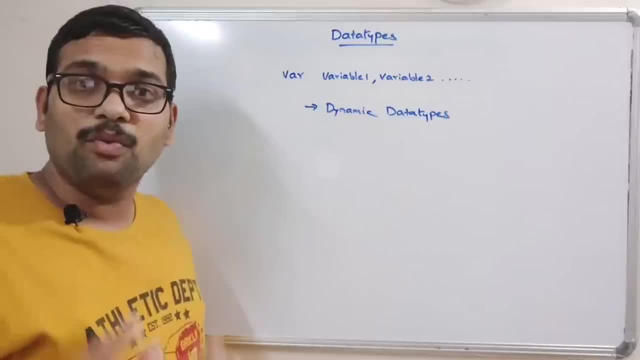 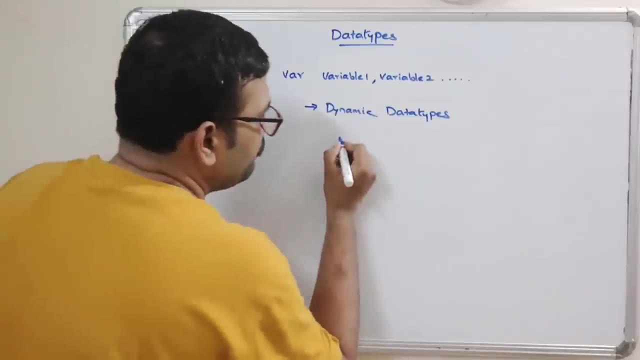 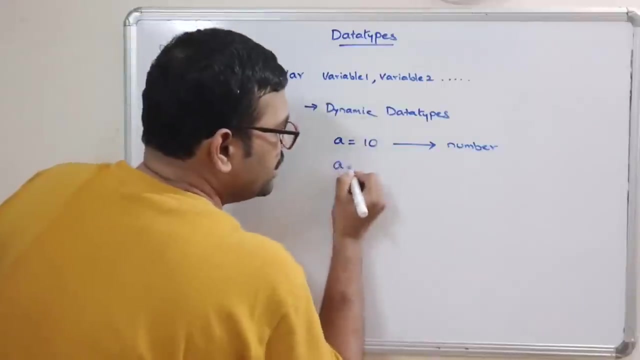 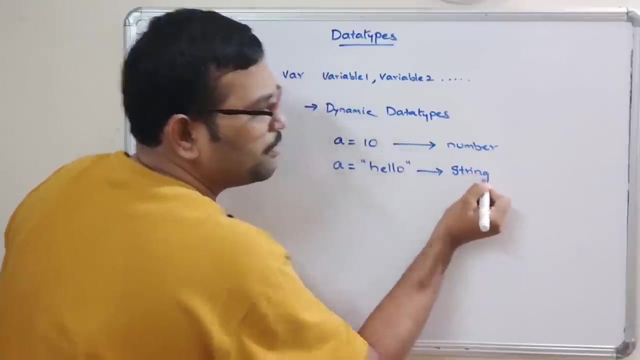 So dynamic data types means Based Upon the value assigned to that particular variable, it will be considered as a particular data type. For example, if a is equal to 10, this implies it is a number data type. If a is equal to hello, it will be considered as a string data type. 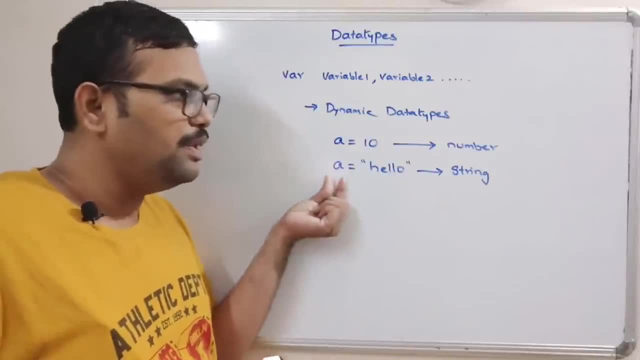 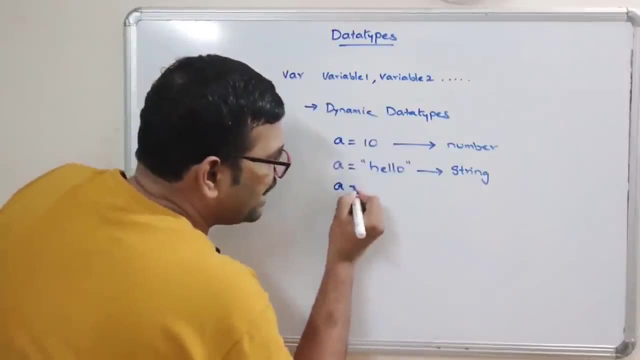 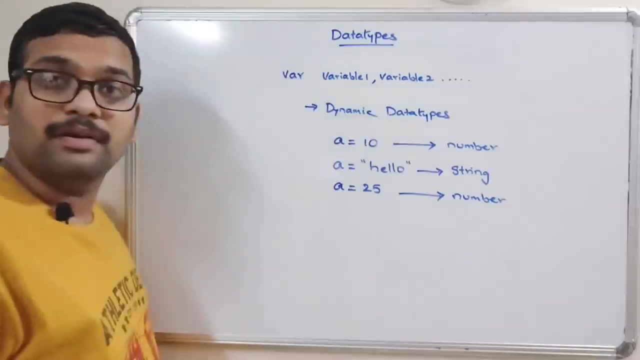 Okay, So based upon the value assigned to the variable, the data type will be finalized. Okay, And Next line: if a is assigned to some 25, again, the data type of a will be changed to number Right. So we need not declare these variables using the particular data type. 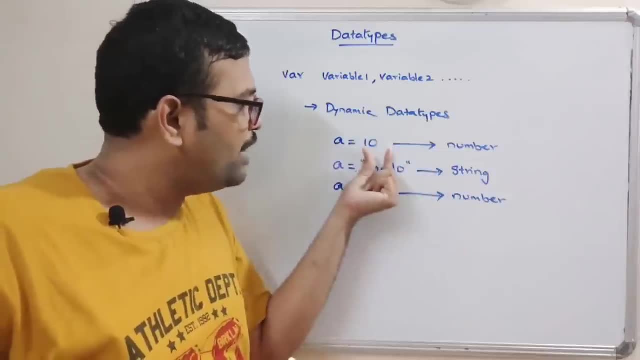 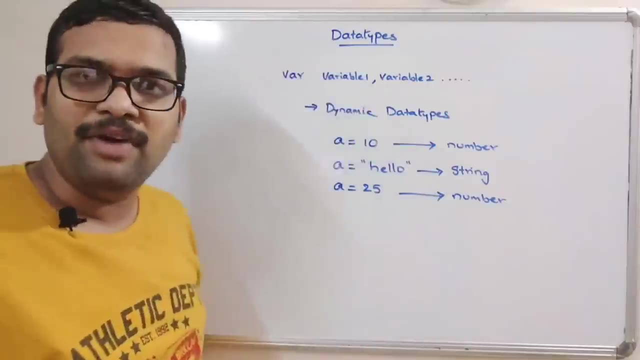 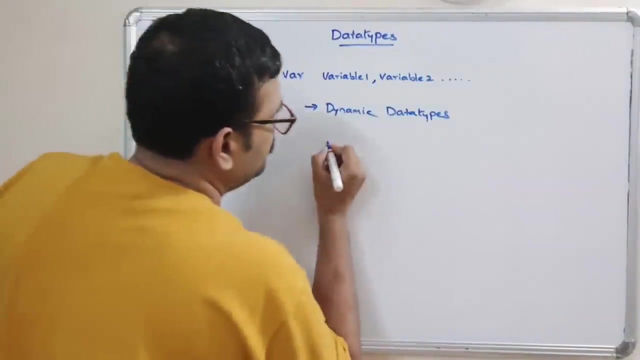 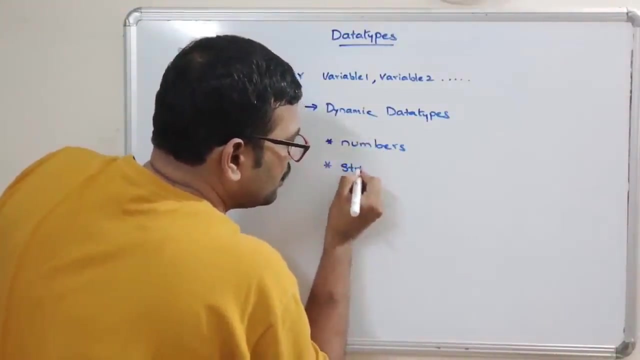 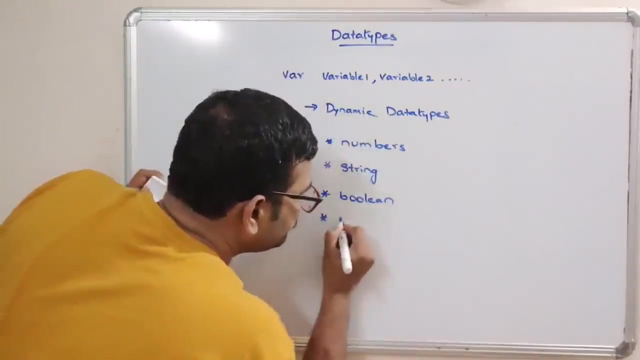 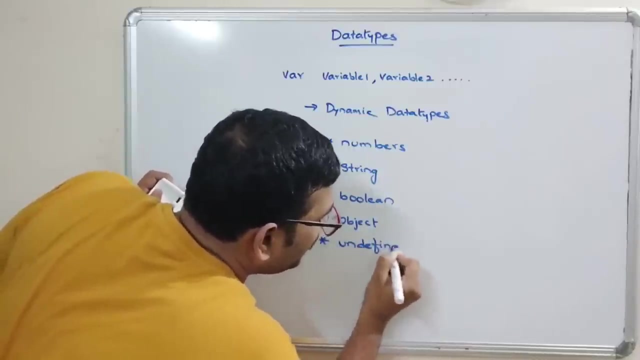 So these are the dynamic data types. dynamic data types means based upon the value assigned to the variable, the data type of variable will be fixed. and now the data types available in JavaScript are: Number, Numbers, String, Boolean, Object- Undefined- Undefined. 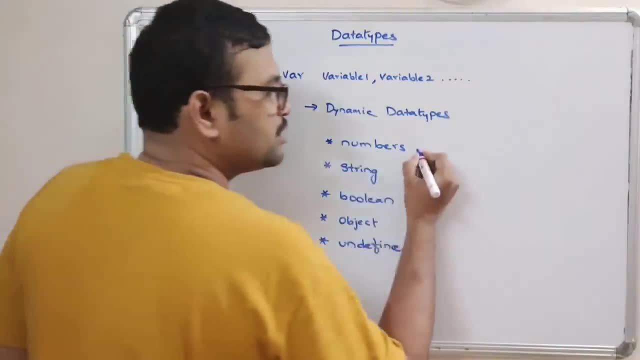 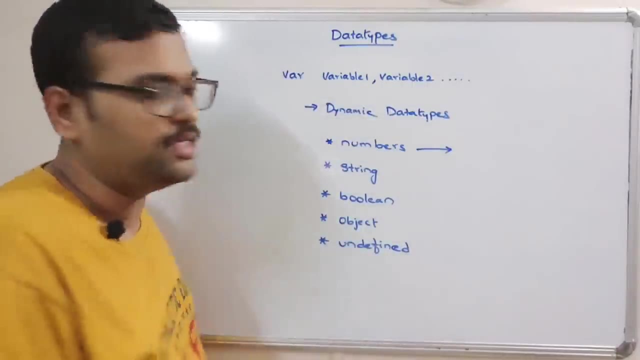 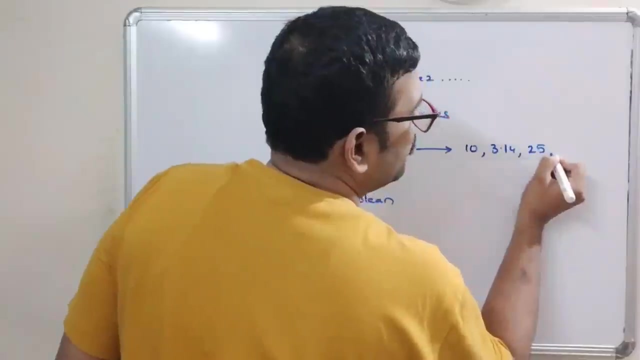 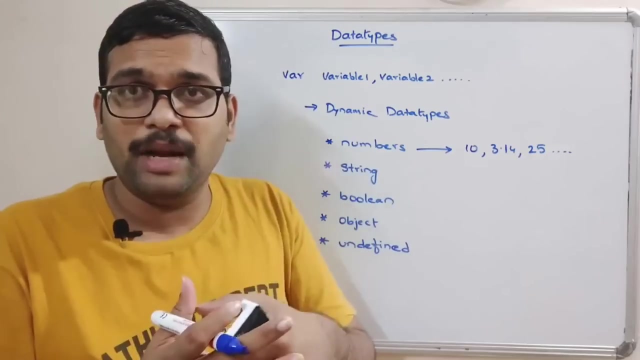 Now Headings. numbers comes with all the integers and the float values. that means the numbers without decimal points and with decimal points. so for example, 10, 3.14, 25, etc. all this comes under the number, so either it can be an integer or the float. so in other programming languages we will 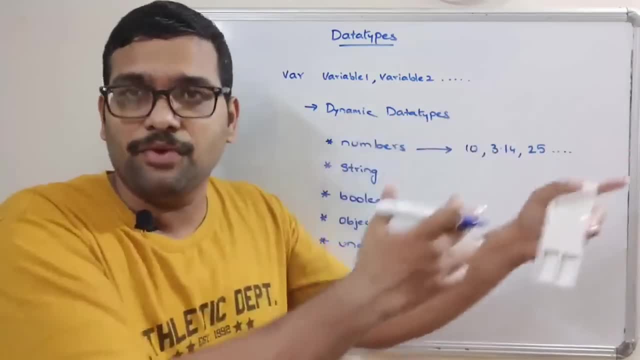 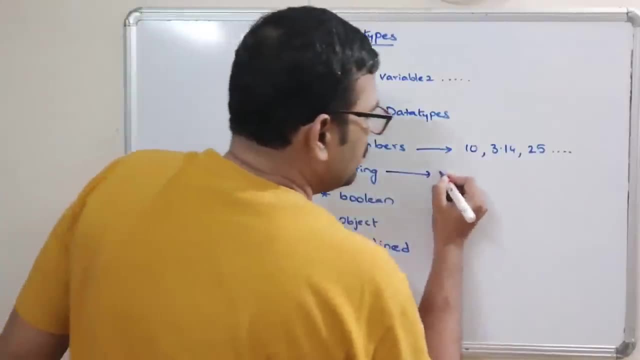 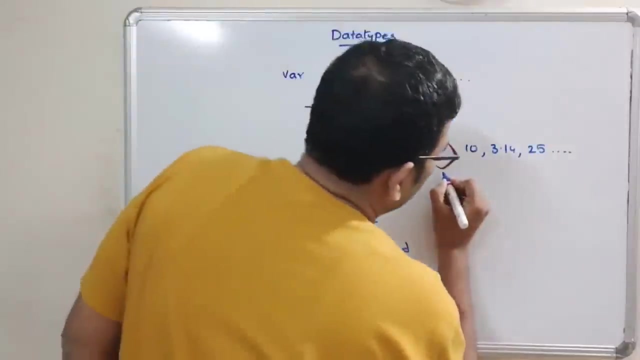 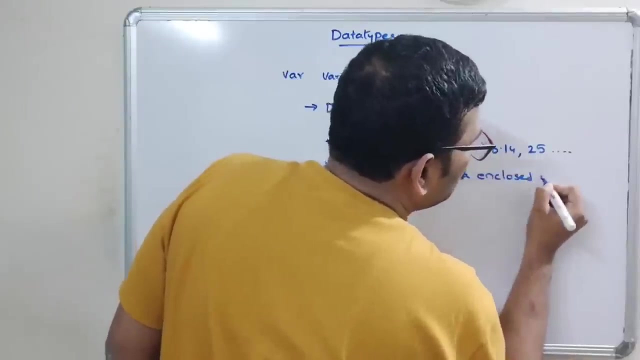 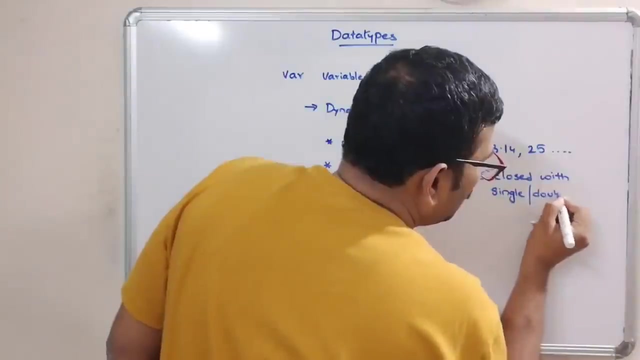 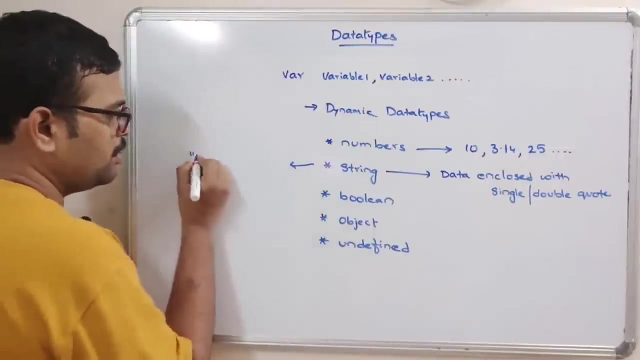 differentiate these numbers, these numbers with integers and a float right, so, but here everything will be considered as a numbers and coming to the string. so, whatever the thing, whatever the thing enclosed in between single quotes and double quotes, so data enclosed with single or double quote. so, example, this is a string, because hello is enclosed in double quotes. 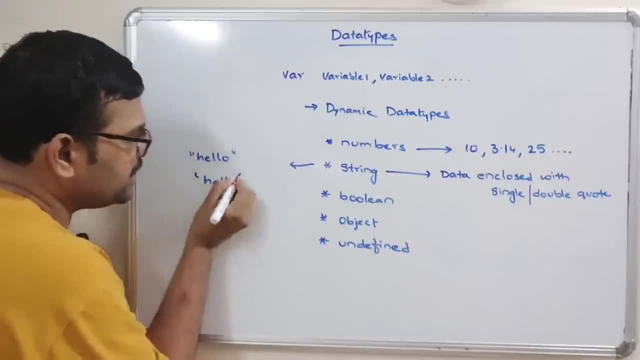 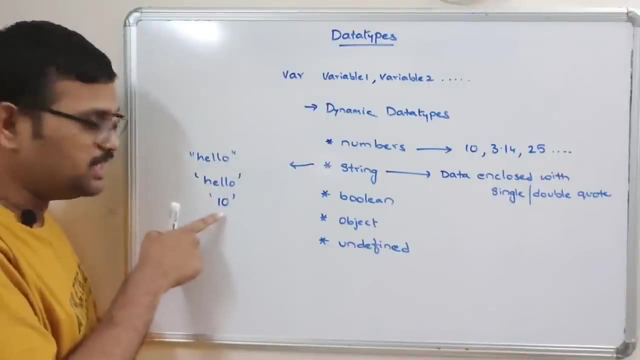 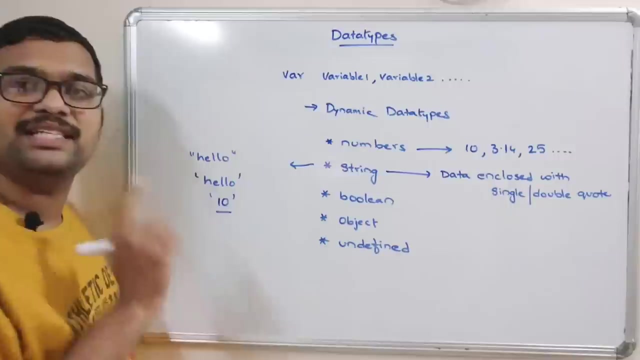 this is also a string, because hello is enclosed in single quotations, this is also a string. so even though we are giving some 10, but this 10 is enclosed in single quotations, that implies this is also a string. so, whatever the so that's why i have written the data which is enclosed with a single or a double. 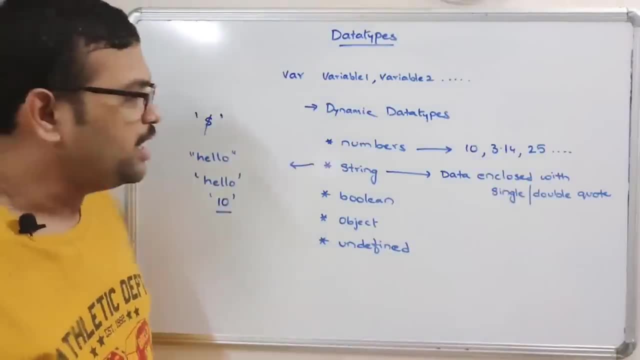 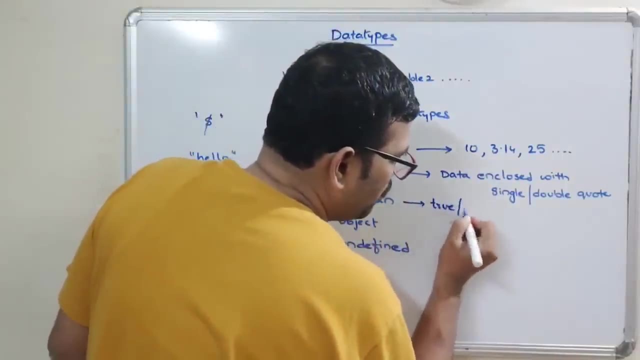 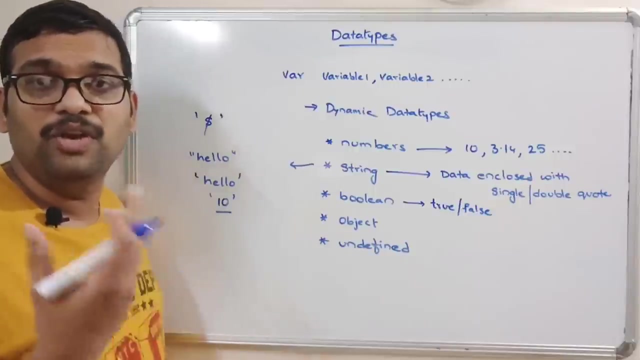 quotations that will be considered as a string right. so this is the string data coming to the boolean. boolean data type is either true or false, so whenever we are comparing the conditions, we'll get the result as a boolean result. so boolean result means either true or false. so, for example, 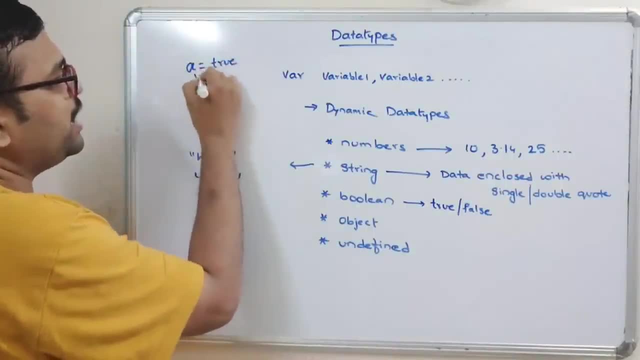 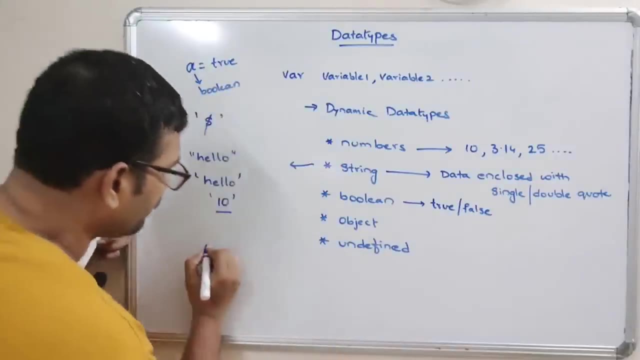 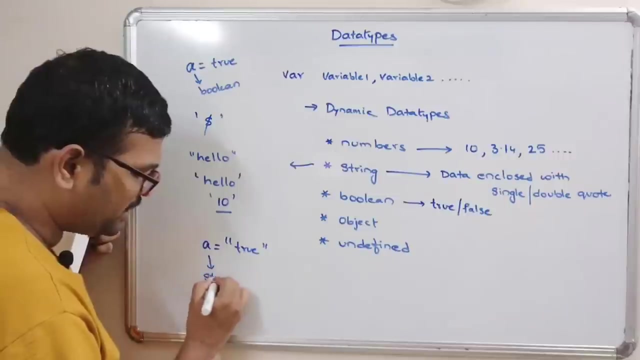 some a is equal to true. now the data type of a will be boolean. now the data type of a will be boolean. if the same thing, written like this, a, is equal to true, in between double quotations, the data type of a will be string. that's the difference, right? so if a is equal to true, this true should. 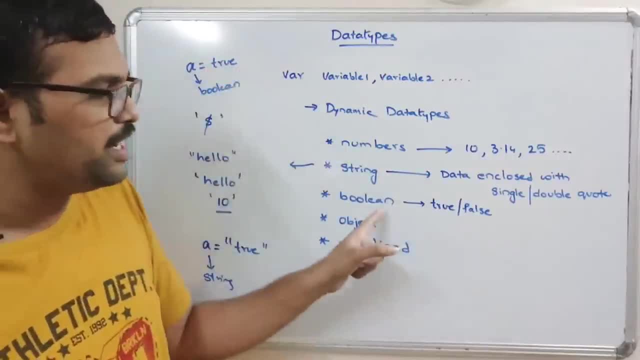 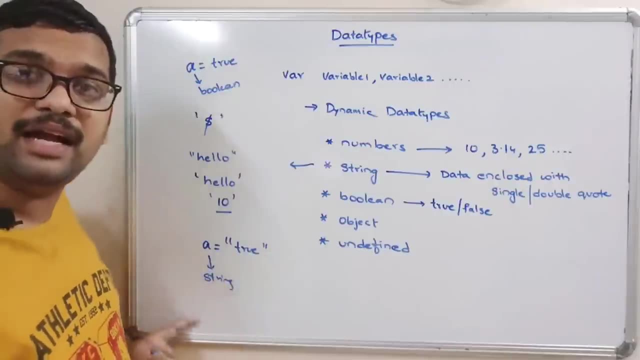 not be enclosed in double quotations, that will be considered as a boolean data type or a false or a false. and if the same true or false enclosed in double quotations, then that that that data type will be considered as a string data type. and coming to the object, 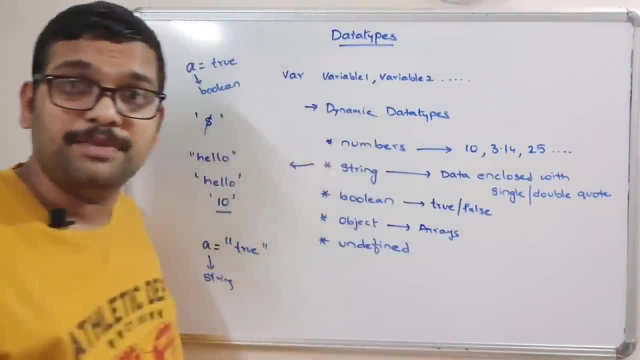 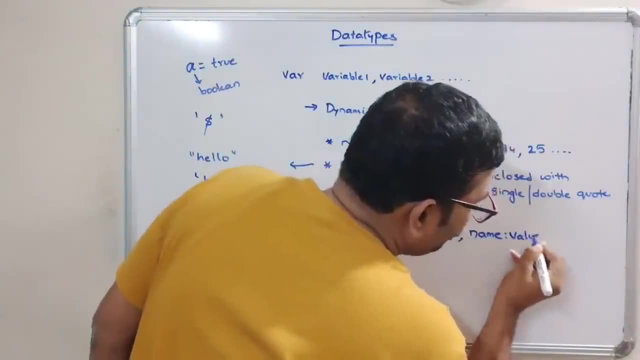 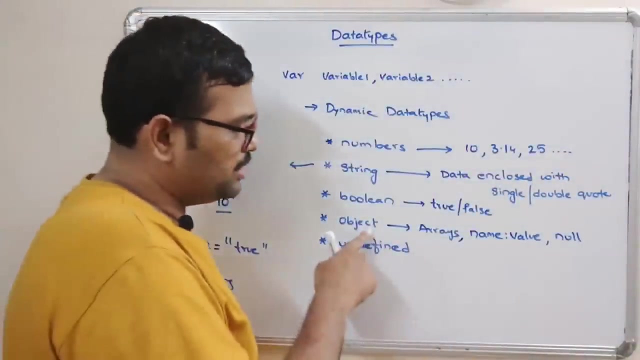 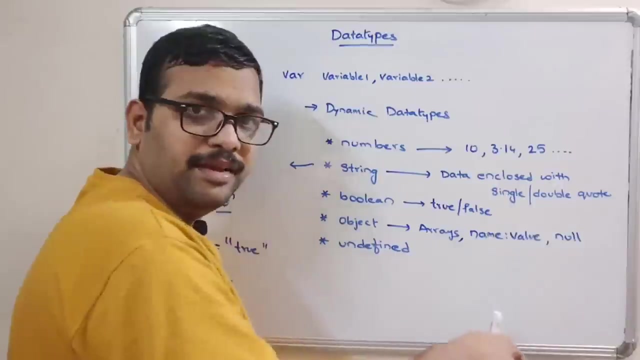 the arrays concept. so the arrays in javascript will be considered as an object, similarly name value pairs, name value pairs. similarly the null statement. the null statement will also be considered as an object. so null statement means if any one of the object is initialized null, that is an empty right, empty, then that null is also an object right. and coming to the undefined, 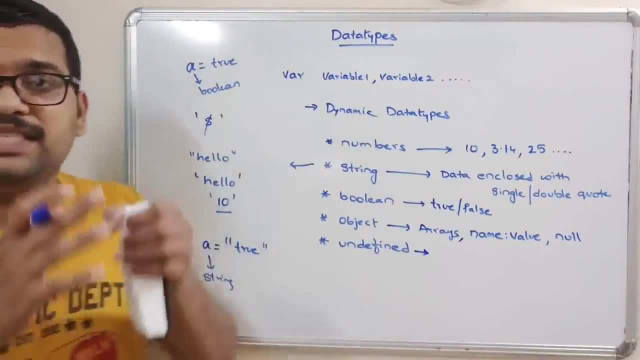 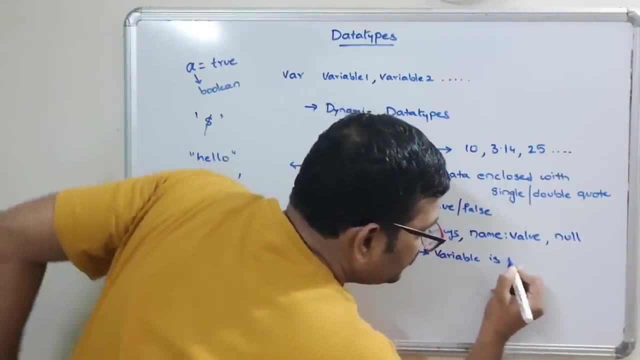 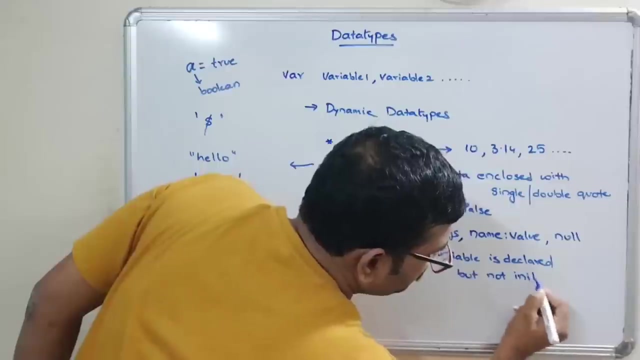 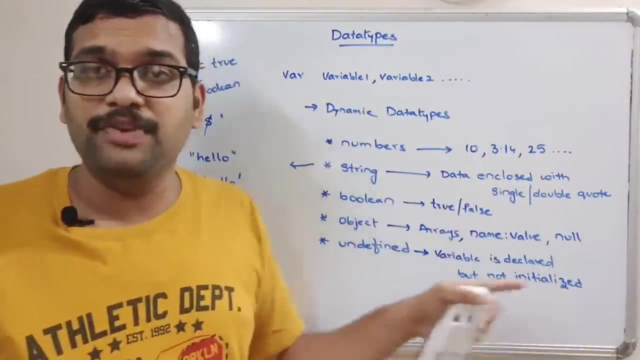 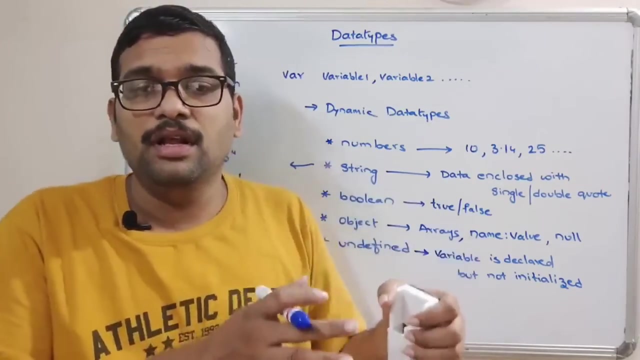 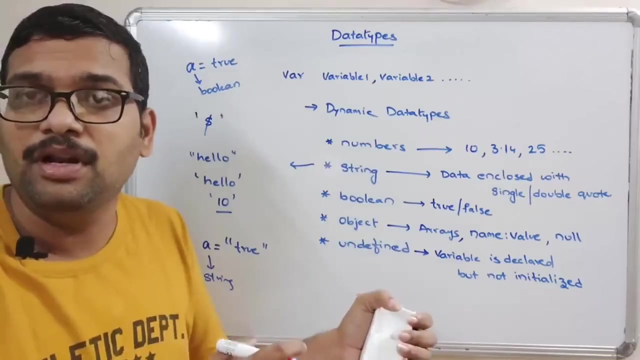 undefined means so the variable is declared but not initialized. okay, variable is declared but not initialized. okay, variable is declared but not initialized. those type of variables will be having the data type called undefined. so unless you assign some value to the variable, that variable will be of data type undefined. so whenever you assign some value to that particular variable, 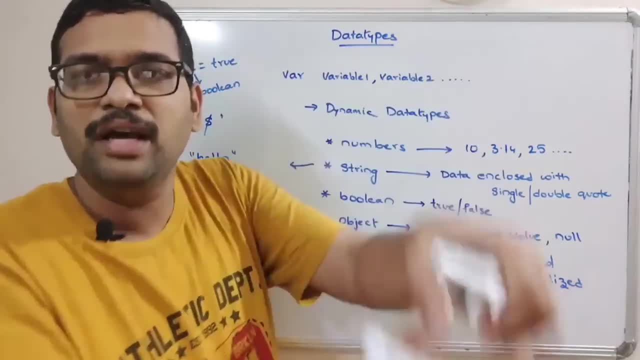 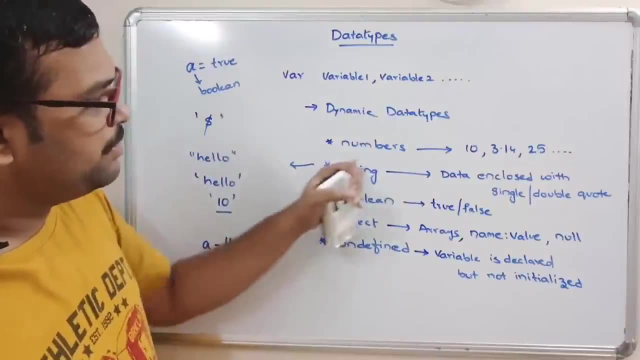 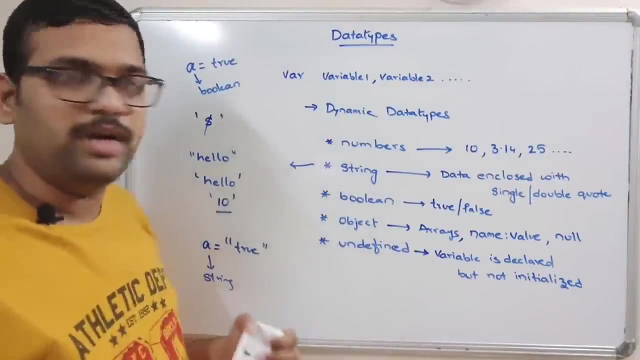 that variable will be changing its data type from undefined to the particular value which you have assigned to the variable right now. these are the different data types: numbers, string, boolean, object and undefined. so i will show you on the screen by executing a small code, demonstrating all these type of 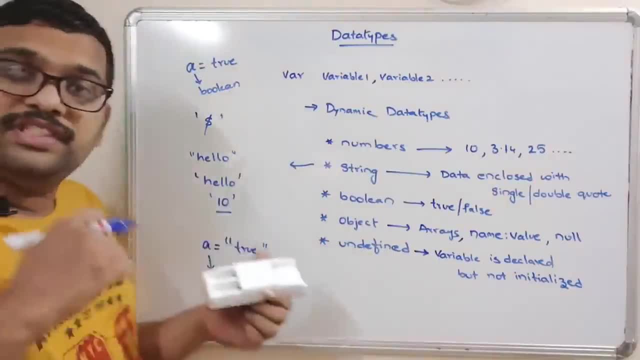 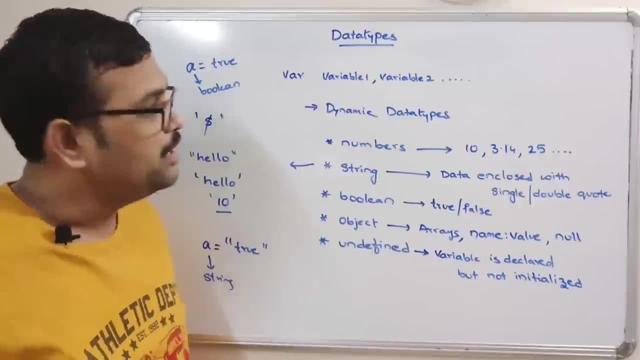 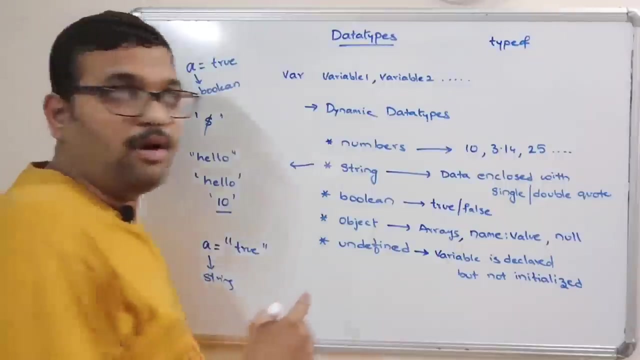 data types right, and how to check whether the particular variable is of particular data type. so finding the data type of a particular variable or a value for that. we are having a keyword called type of. so if you use this keyword, type of- and followed by the variable name, the variable name. 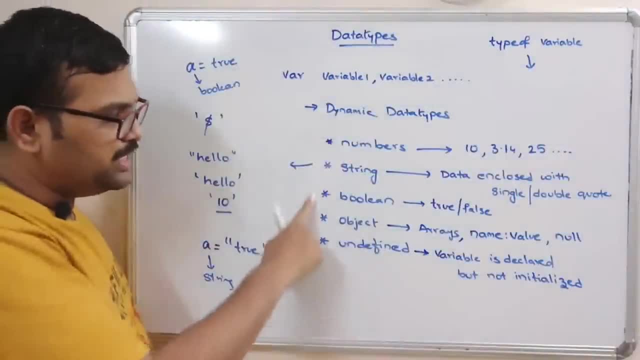 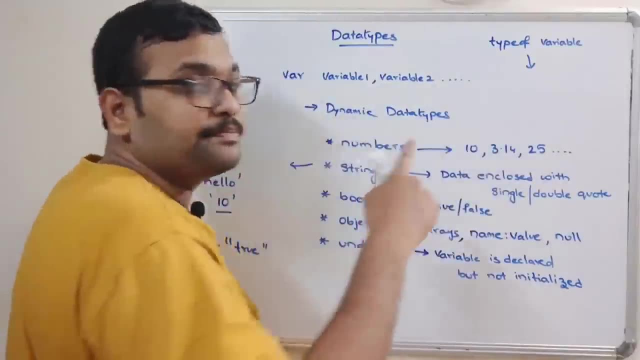 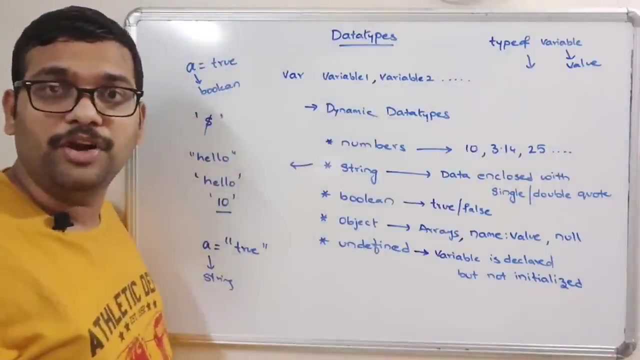 this will give the data type- one among all these data type- either numbers, a string, boolean object or undefined- right. so it will be giving like this. similarly, instead of variables, we can also give directly a value. we can also give directly a value, so you need not go with the variable you. 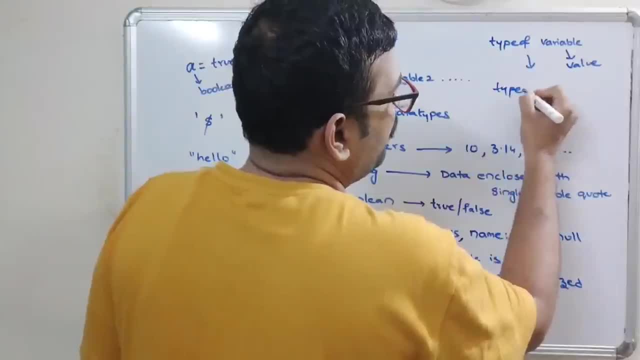 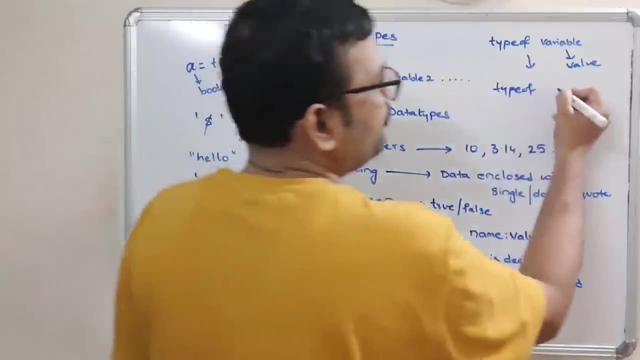 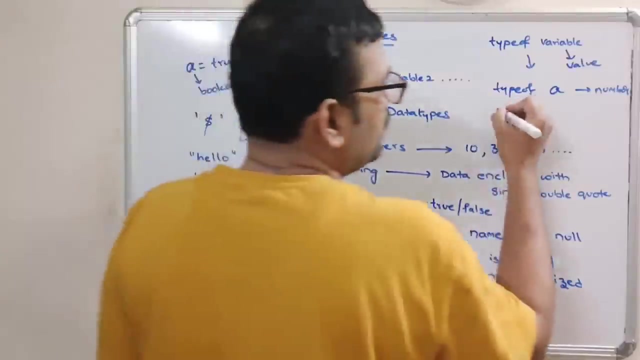 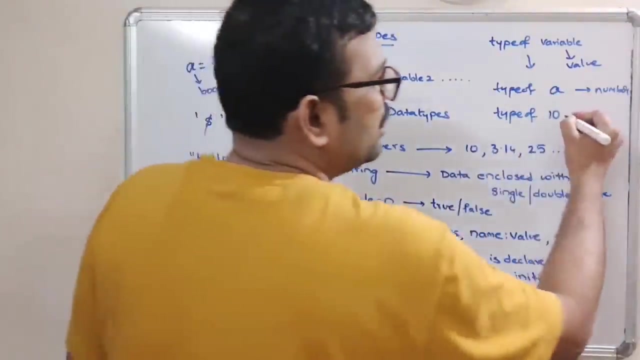 can give the value. so, for example, type of, for example, a is equal to 10. you consider this example: a is equal to 10. type of a: this give a number. the data type has number, because 10 is a number. similarly, you can also give type of 10 instead of using the variable name. you can also give the value, so that 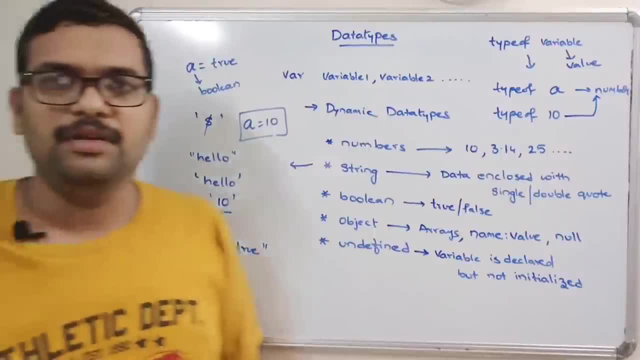 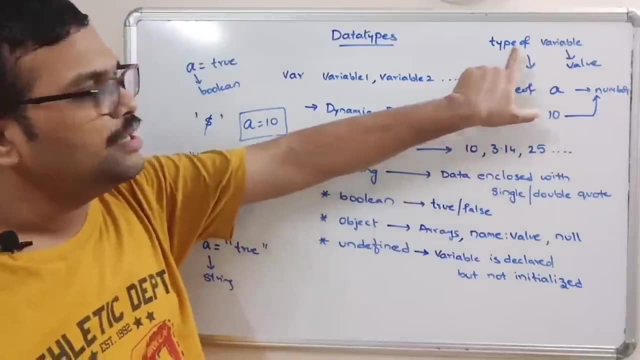 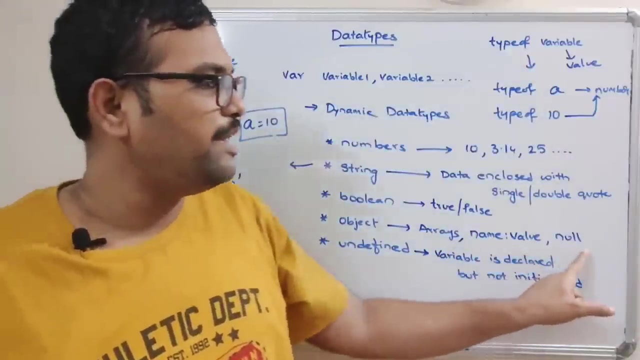 it will also give the same result as a number, because 10 is a number right. so, in order to find the data type of a particular variable, We have to use this keyword called type of, You have to use this keyword called type of, And arrays, name, value, pair and null will be considered as an objects. 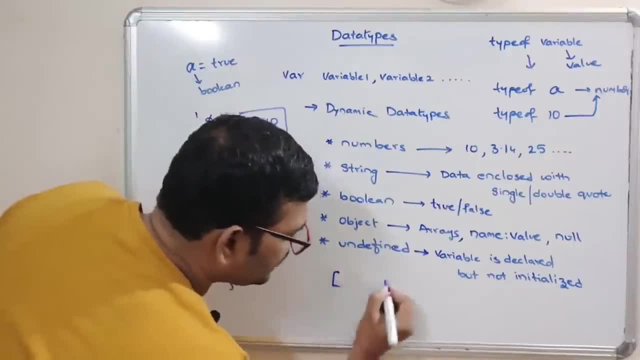 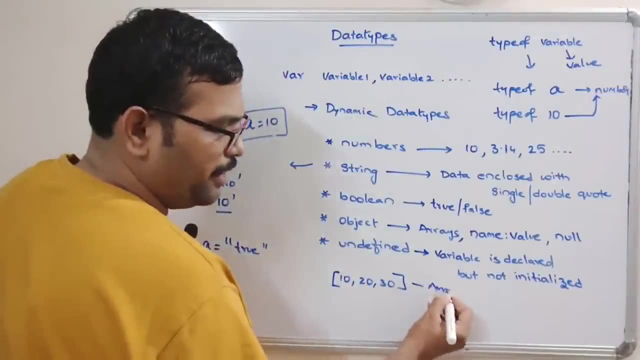 Right. So arrays means we know that. So in the subscript we have to pass the elements 10,, 20,, 30. This is an array, But here the data type of this arrays is object. This object. 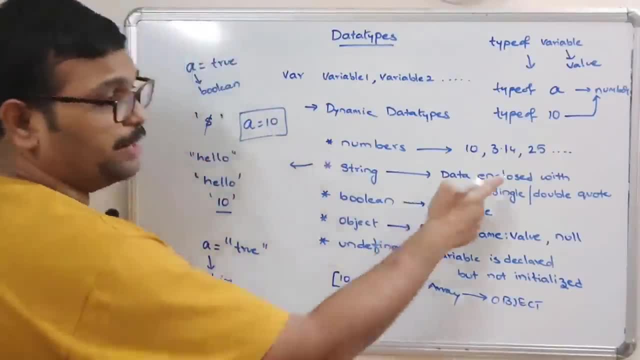 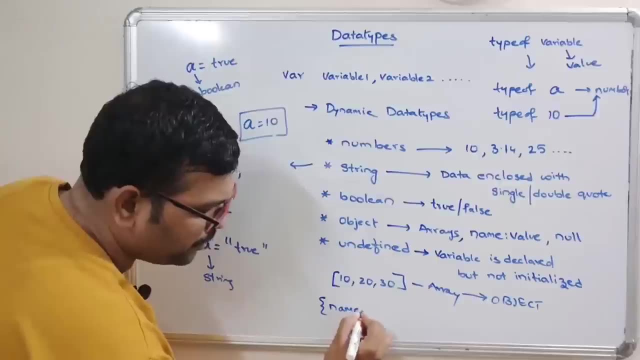 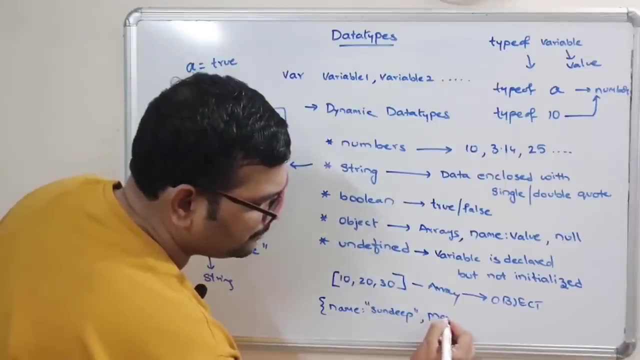 Right. So I will show you by executing a small code And coming to the name value pair: Name value pair, So you can give some name, You can assign some name And also assign some marks. So this is called an object. 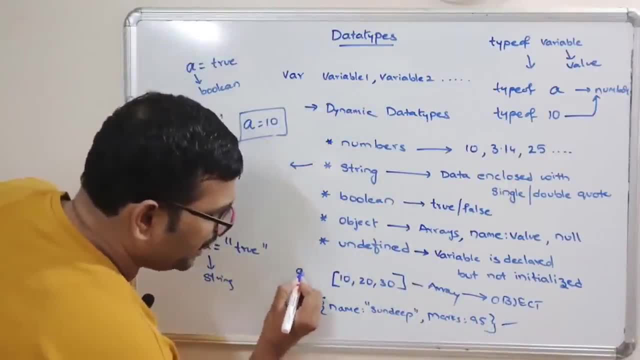 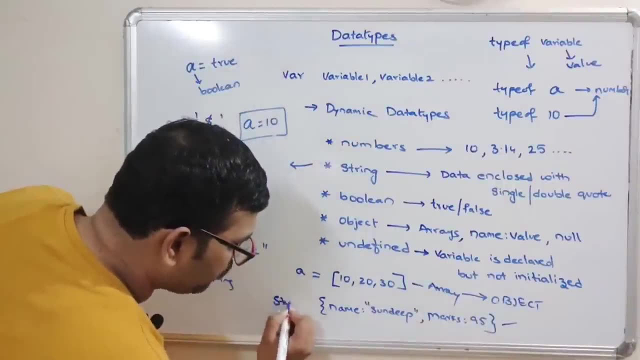 This is called an object, So you can write here some: a is equal to 10,, 20,, 30. So a is an array Which The data type is object And here the student details or anything else you can write. 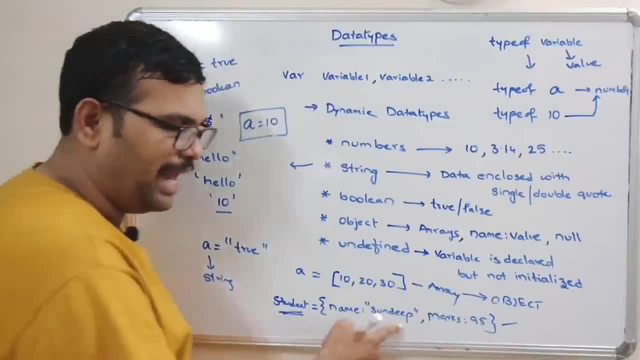 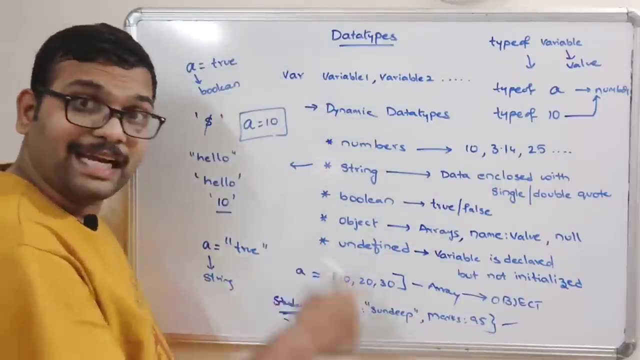 So this is a variable. Okay, This is a variable. Variable is equal to name value pair. So name Sandeep marks 95. So student is an object. The data type of this type of name value pair will also be considered as an object. 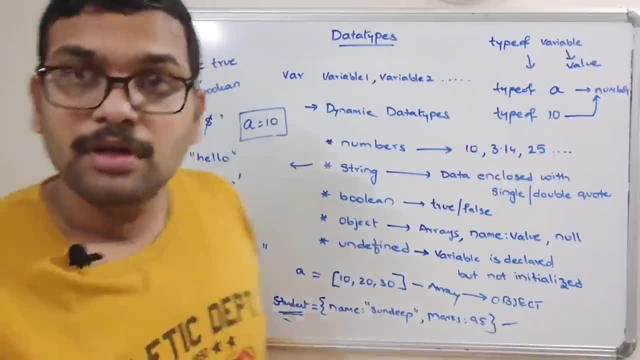 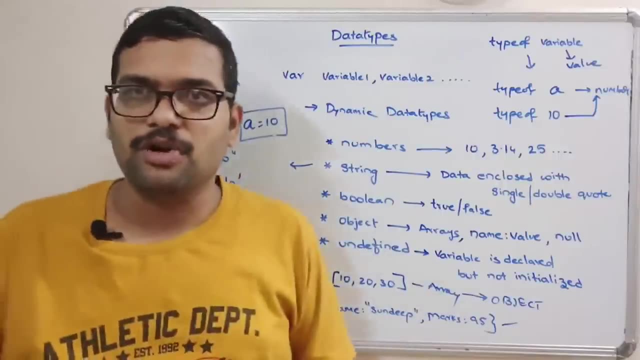 Right. So hope you understood All of you Right. So let us move on to the system. So I will show. I will demonstrate all these data type by executing a small code. So let's move. Hello friends. 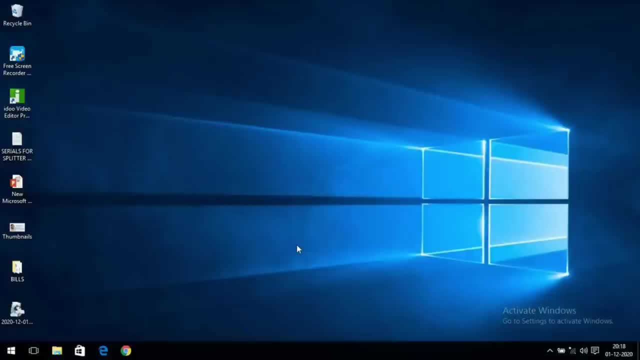 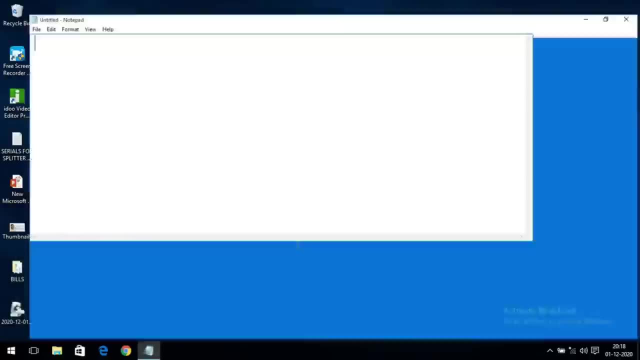 So just now we have seen various data types available in JavaScript. Now I will show you the demonstration of all those data types by writing some code. So let us open the notepad And here we can write the script in between the HTML. 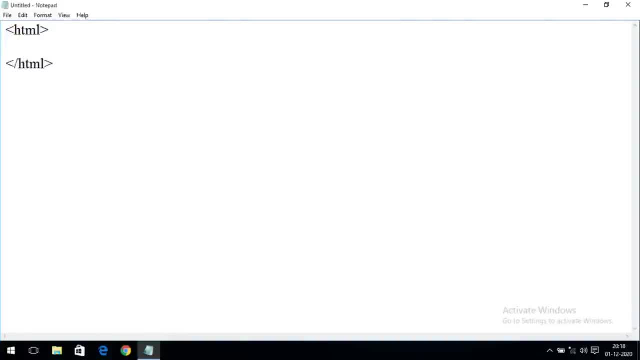 In between the HTML. So, as we have asked for our discussions in the previous sessions, So we can write the script In head tag or body tag. So I will write in a body tag. Okay, So body and close the body. 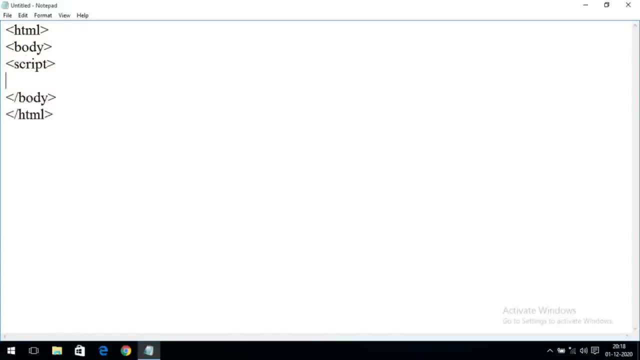 And in between that we will write the script. So in the script again we can write. we can use different output options, So which we have seen in the earlier sessions, like we can use inner HTML or documentwrite or windowalert. 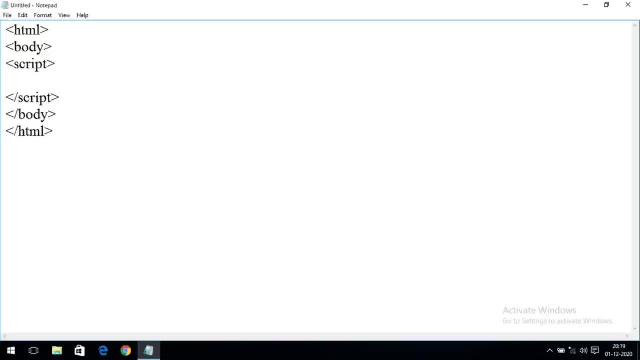 So here we will use the documentwrite to display the output on the screen. And coming to the data types, as we have discussed it just now, all the data types in JavaScript are dynamic. So dynamic means so whatever the data we are storing into the variable, those variables should be declared using only one keyword, that is, var, var. 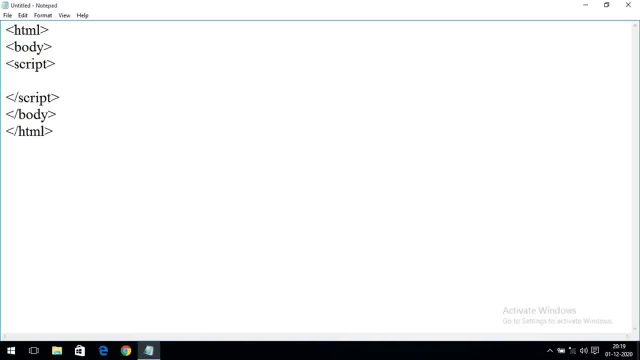 Okay, So here we have seen the data types, like string or numbers or objects or boolean. So whatever the data type, those variables should be declared by using var keyword. So then We can, by assigning a value to that variable, the script will be considered that particular variable as a particular data type, based upon the value which was initialized to that variable. 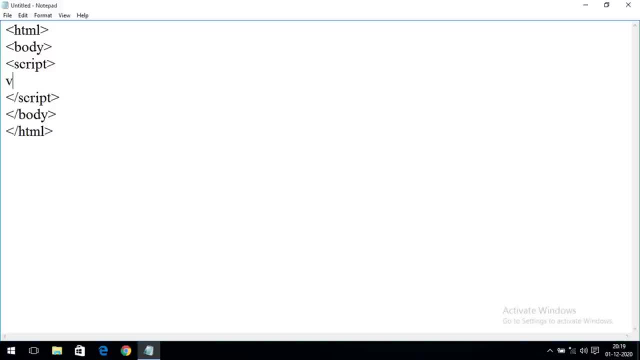 So that's why we call these data types dynamic data types. See, for example, I'm giving some var a, b, c. That means I have declared three variables. Now I'm initializing some value, So a is equal to some 10.. 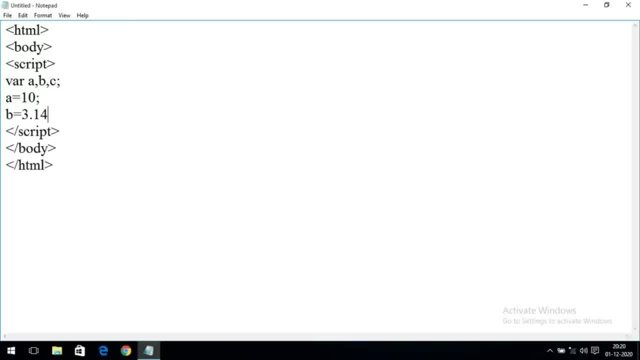 b is equal to some 3.14. And c is equal to some 7.. So here you can observe. the first a is of integer data type, b is also a float data type, But here we call the integer and the float as a common data type called numbers. 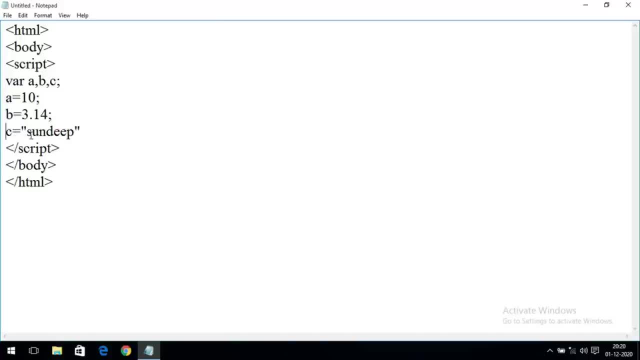 Okay, So here a and b are a number data type, c is a string data type. Okay, So in order to check the data type of that particular variable, we have to go with the type of type of keyword. Right. 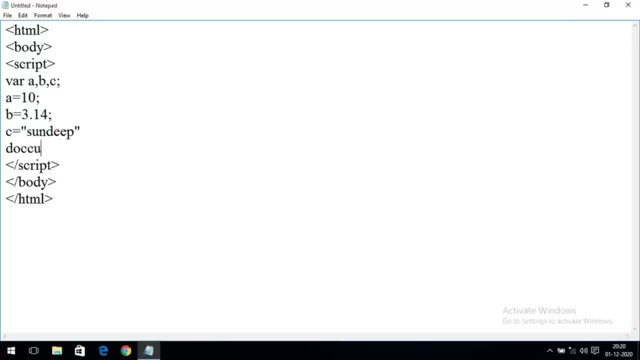 See, we'll see document: Document dot write. Let us take type of type of a: Okay, And we'll go with the document: Sorry, Document dot write of type of b. Similarly c: Okay, Now we'll check c. 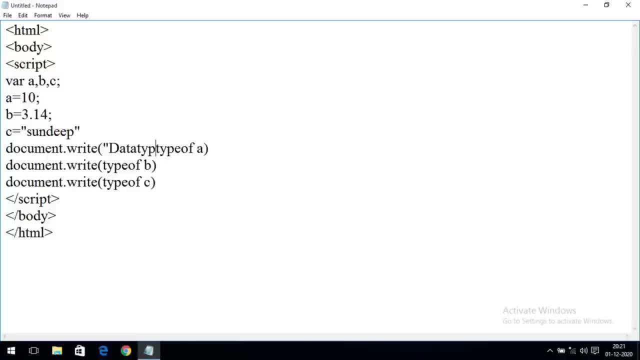 So data type of a is Just. I am writing here: data type of a is similarly, So just in order to avoid the confusions and avoid all the confusions, we can write all these things: Data type of b. Similarly, data type of c. 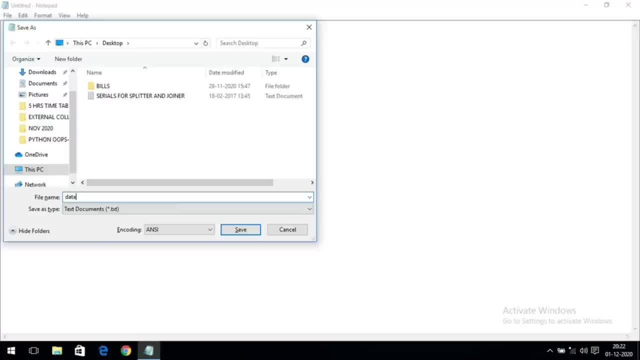 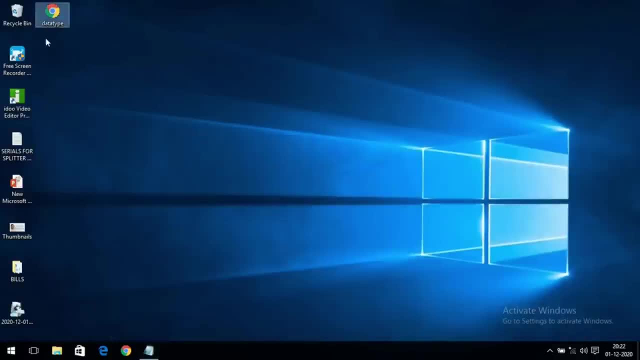 Okay, So I'll execute This one. I will save this one by using some file name called datatype dot html. So I have saved this file on the desktop So you can find here. So double clicking on the web browser we'll get this one. 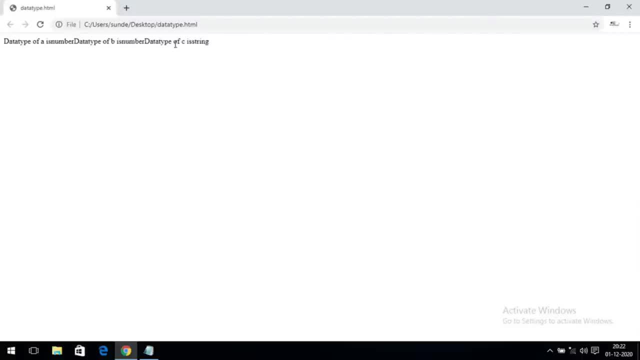 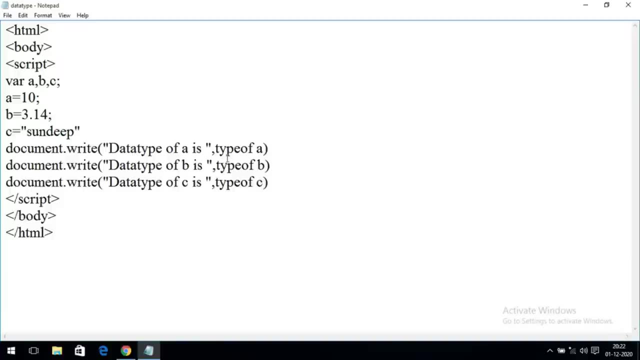 See. so data type of a is number, data type of b is number, data type of c is a string. So just give some space here so that it will be displayed here and again also use A tag. so b means break a rule. 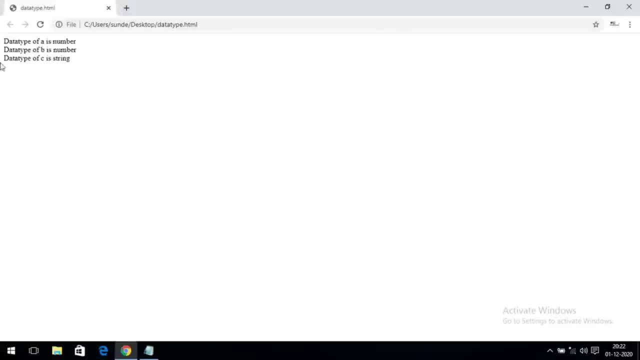 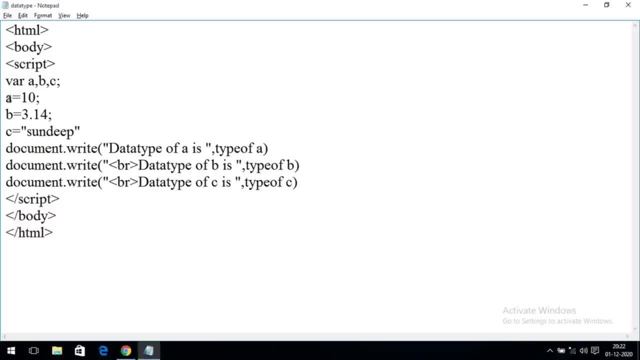 So that there will be in this different line. Okay, Everything is printed in a different line, So data type of a is number, b is number and c is a string. You can observe here a is 10 and b is 3.14.. 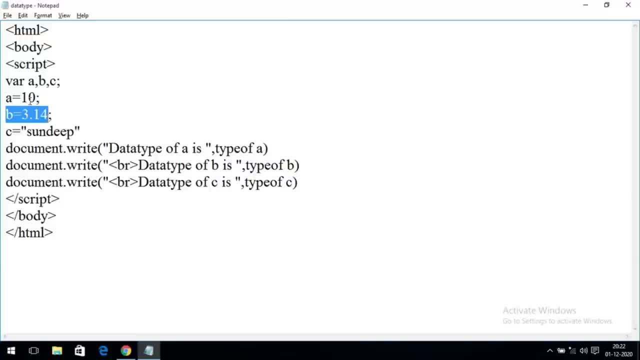 So, even though b is having some flow data type in JavaScript, it will be considered as a number. It will be considered as a number. And if you write here c, If you write the c in the same way, we will get the same thing. 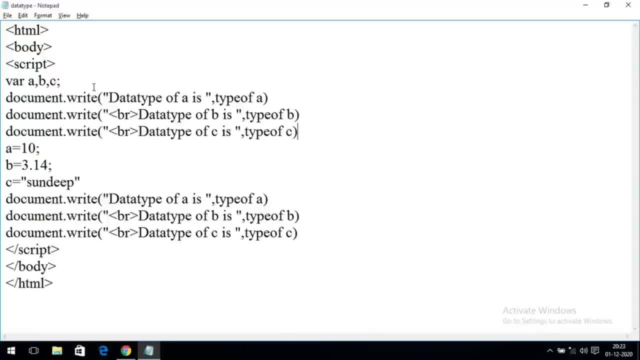 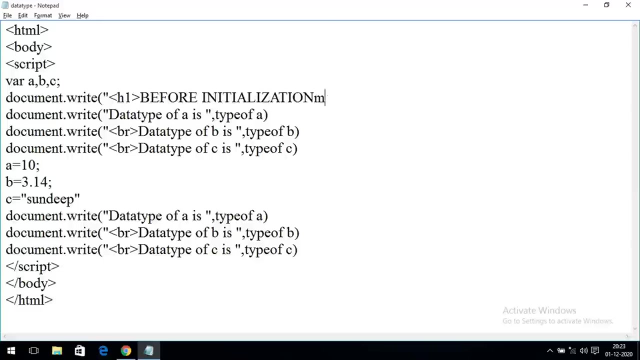 So, for example, if we take a number, c same thing here, that means before initialization. okay, before initialization. so I will write here document, dot write, see each one before initialization, each one and here after initialization, so we can go with the before initialization and after initialization. see, this is. 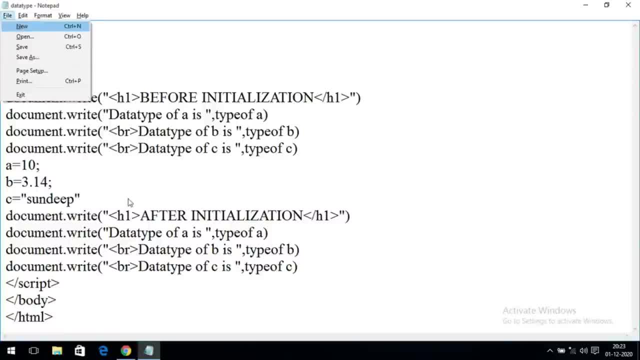 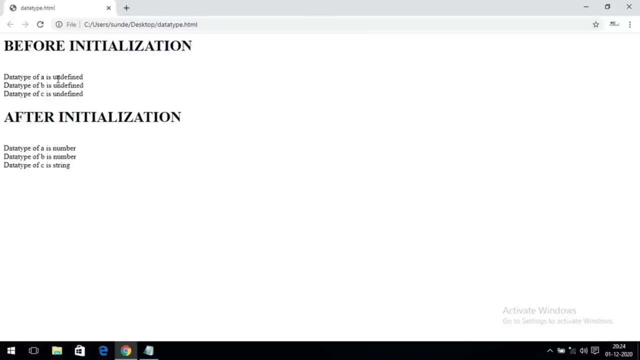 after initialization: now you can observe the difference. so I will give the break break- well, break row- so that everything will be printed in the new line. right, you can observe here now, see before initialization: data type of A is undefined. data B is undefined. C is undefined. so if you declare the 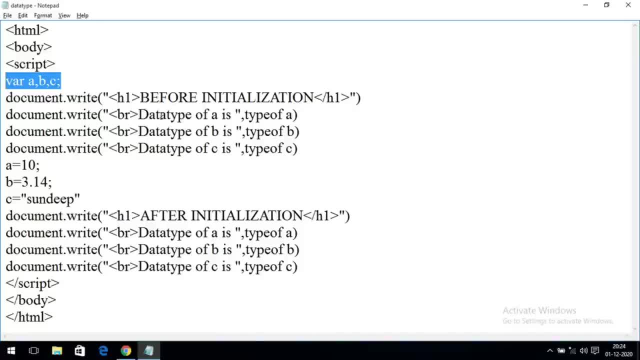 variables but not initialize it. the variable that the data type of these variables will be of undefined because no value was defined to these variables. but whenever we have done the initialization, immediately the variable will be having some data types right. similarly, let us go with one more thing. 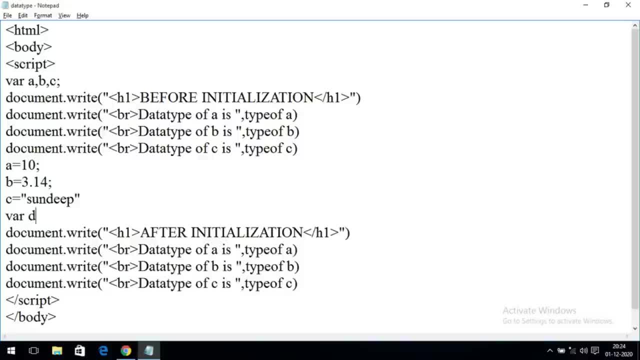 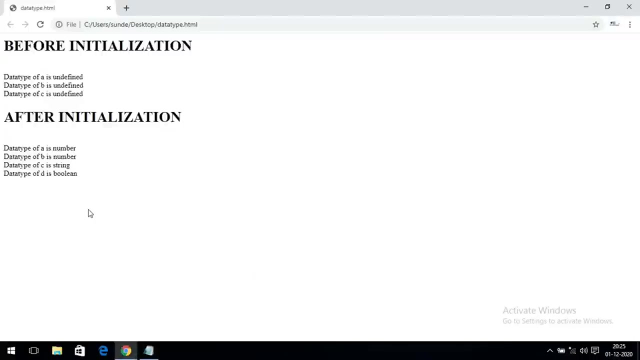 where D is equal to true, D is equal to true. now we will check the data type of D. you can observe D is a boolean, so here true is not a string. so if you place the double quotes here, then it will be considered as a string. you can observe. 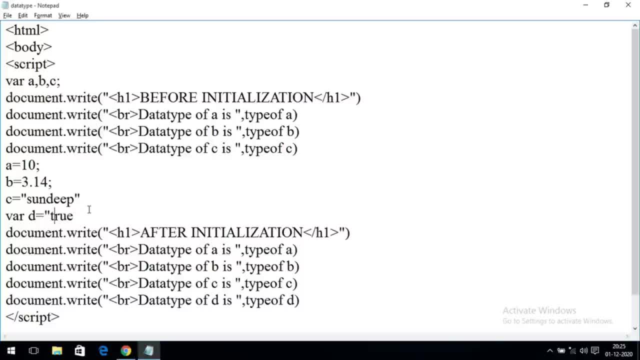 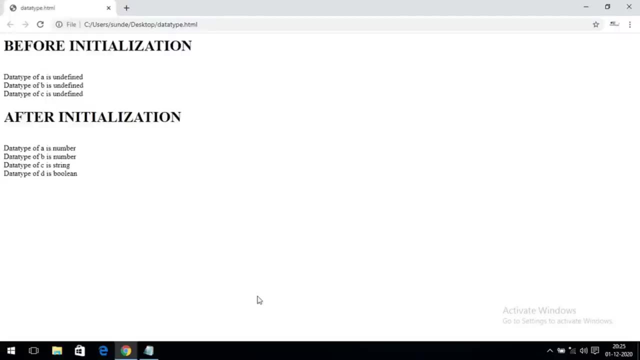 here now it will be a string. but if you are not using these double quotations, but you are initializing the value as a true or a false to the variable, to any variable, that variable will be of a data type- boolean. so that's why you can observe here: it's a boolean data type. it's a boolean data type. now, once again. 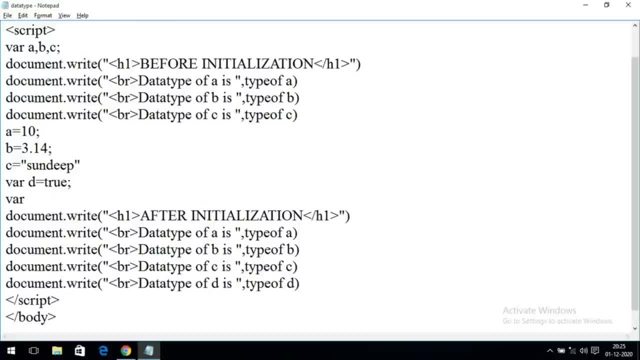 one more thing. so where some Mats is equal to true Right, So some 90,, 100,, 85,, 75. So these are the marks. So here this is called an array. So in JavaScript this is an array, Right. 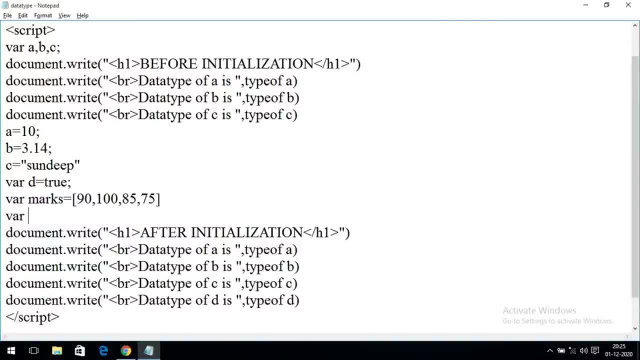 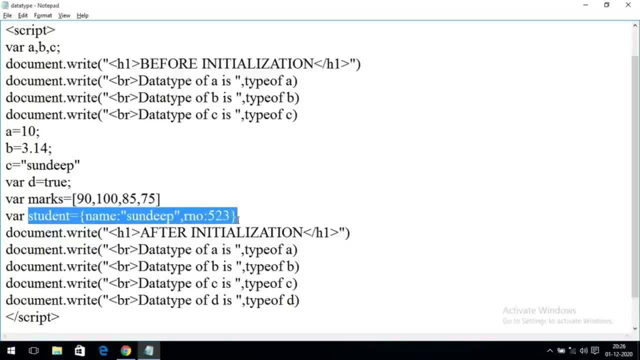 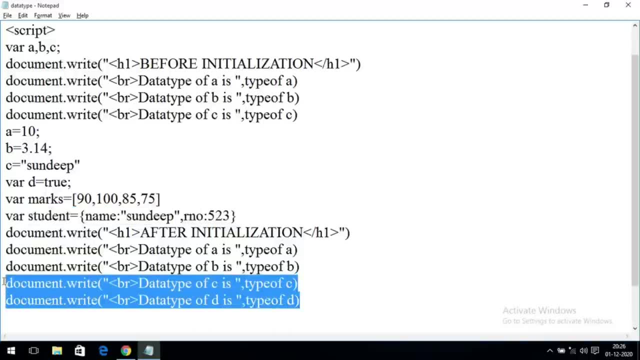 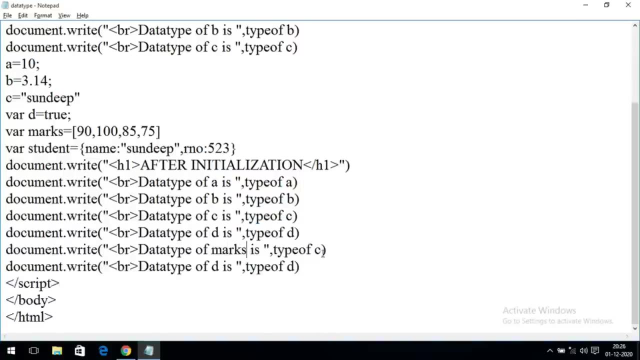 data type. i mean this type of variable is called object, object. now we'll see the data type of all these two things. that means marks and the students. see, here we'll see data type of marks and here we'll see data type of student. so here both marks and the student are. 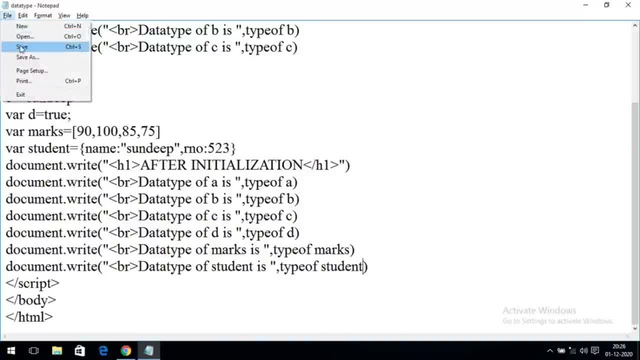 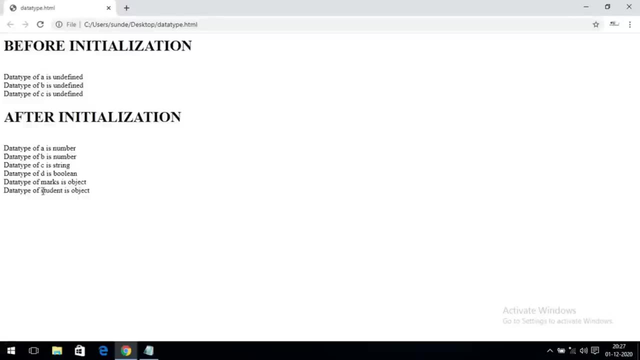 the variables, right. so here we can get here in javascript. even though it is an array, the data type of this particular array will be of object. see, you can observe here: see, data type of marks is object. data type of student is object. right, so this is the one more data type in javascript. 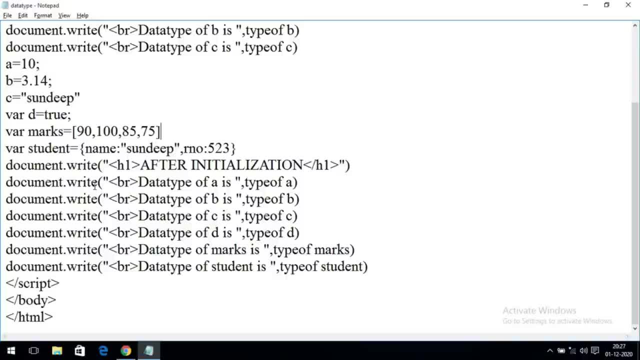 that is an object, so we can declare any variable as an object. object means a variable elements. okay, so we can use a name. I mean the key value pair, the name and value pair, as well as we can also assign the arrays concept. so if you are using 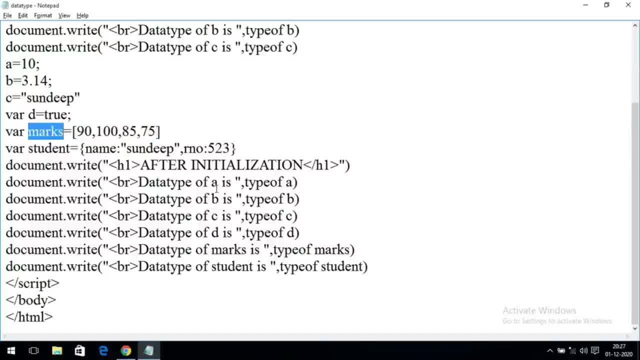 some arrays concept also, the data type of this array will be an object. right, so you can initialize or you can reinitialize this object to a null. null is nothing. okay, now means nothing. so if you go, that student is equal to null null, so immediately we will get it as a null. okay, here null is also an object. 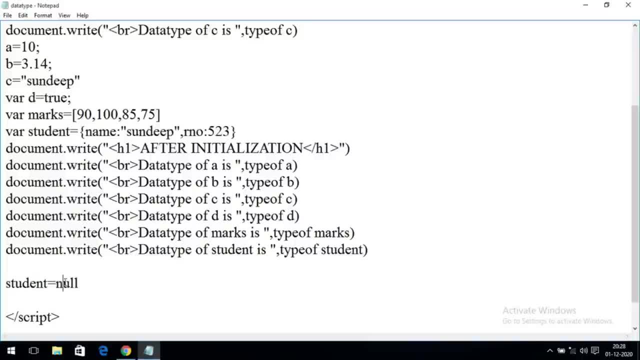 null is also an object. that means it will empty the values of particular variable. it will empty the value of that particular variable. so you can, you can observe here. so, even though it is a null, it is also an object for data type of null. so here we. 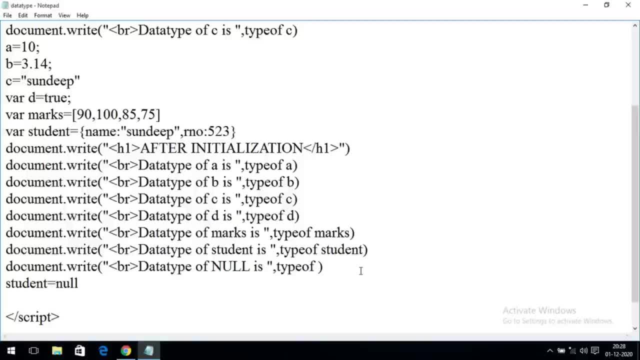 can directly view the value. so two things can be done. so if you use the type of, so you can give either a variable or the value. here I will give a value as null, small letters, null. so let us check. you can observe the data type of null is. 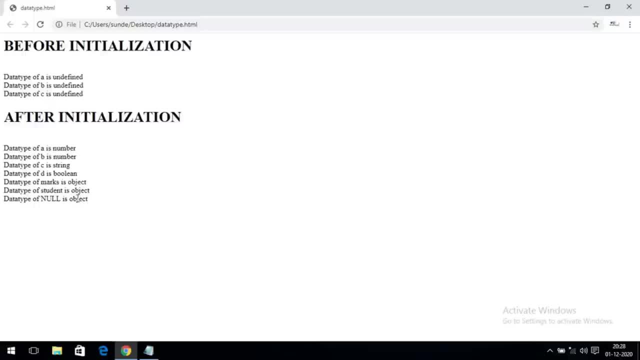 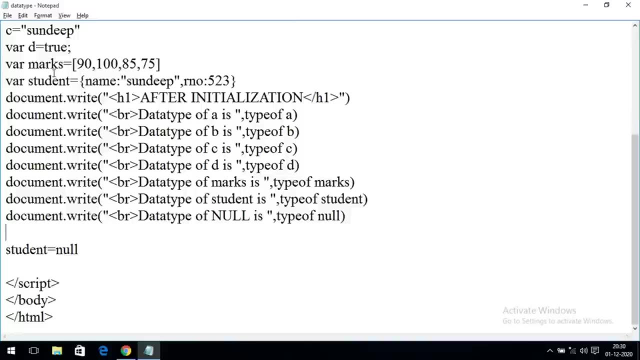 also an object. data type of null is also an object, right? so if it is an, these are the data type of null and data type of null is also an object. if you all the data types- different data types- and if you want to access the array elements similar to. 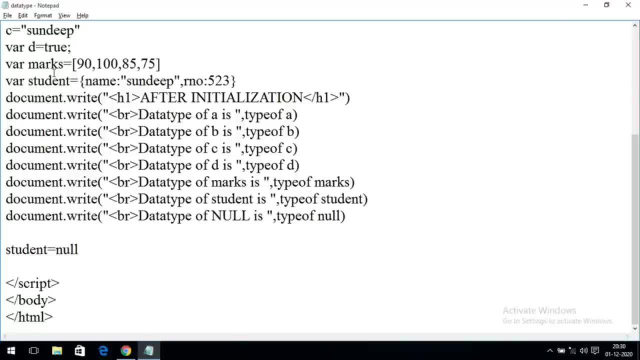 our other programming languages we can access the elements of an array by using the index values. here also the index will be starting from zero, right. so if you want to access these array elements, so directly go with this one. so document dot write dr. so marks of zero. 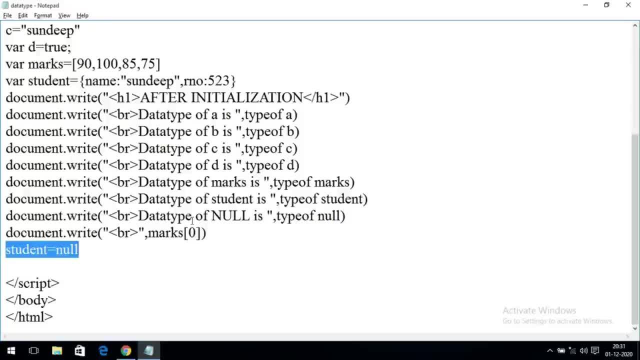 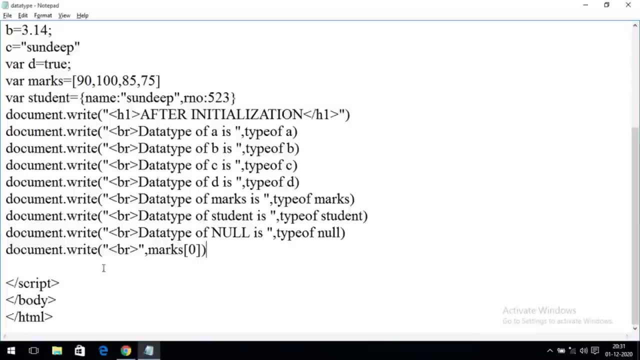 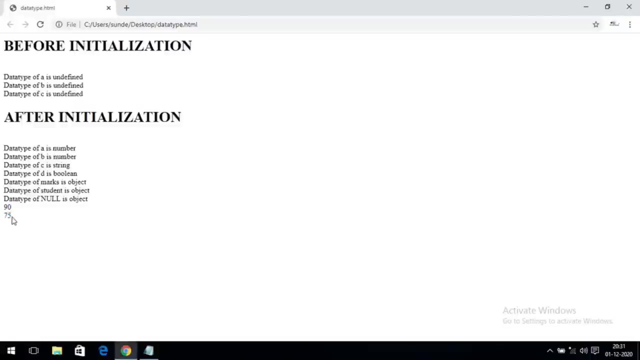 see you can observe here the marks of zero is 90, right. similarly so marks of three. so that means the zeroth index, first index, second index and the third index. so marks of three. it should be 75, so 75 will be there right. so this is. this is the way we can access the elements of an array if it is an object, see. 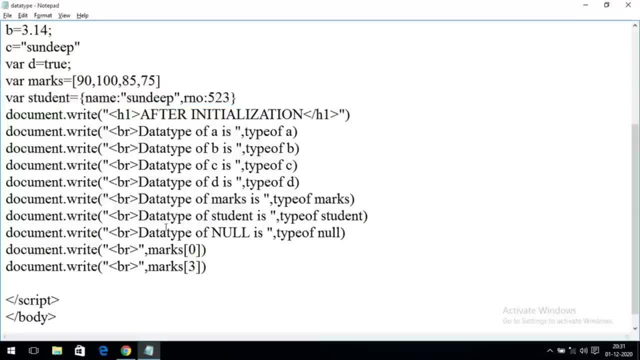 if you, if it is an object here, and how to access these elements. so similar to our structures, concept in c language. so document, dot write and if you want to access the elements of an object, so simply use the variable name. so your variable name is a student, dot the name. 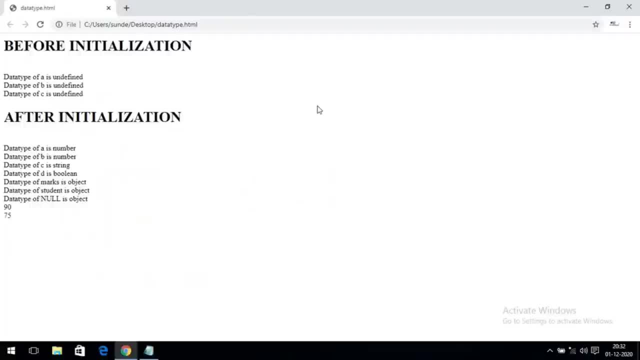 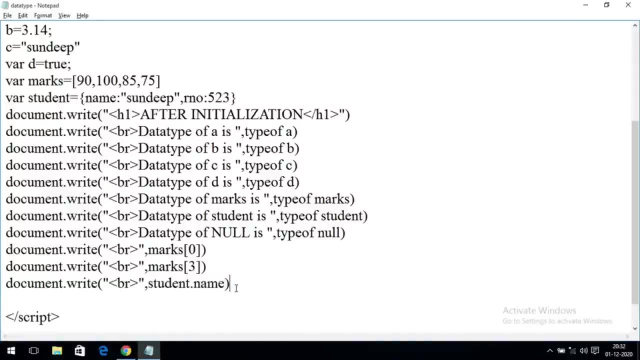 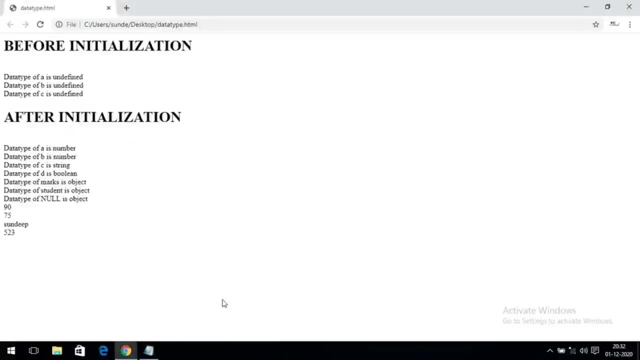 student dot name. You can observe here it will be displaying the name of the object. Similarly, if you want to get the role number, simply go with the r number, so at once we get the result as r number. So here this is an array, but the data type of these arrays are one row of an array. 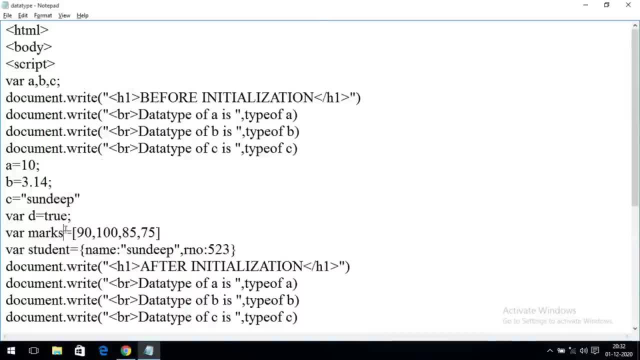 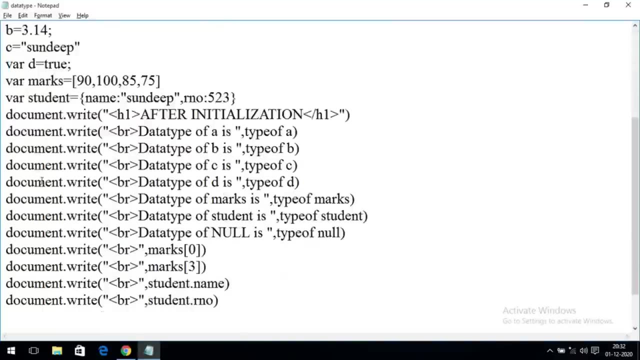 so they are an array itself that you can use here. so if you want to type these variety of is an object and this is an object and this is a boolean and this one is a string and this one is the float. but the data type of b is a number here. this is also a number and also we can. 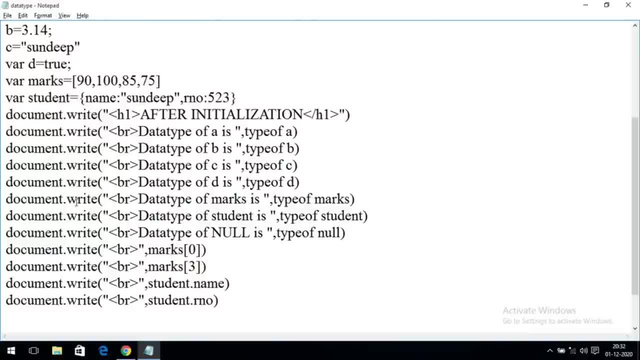 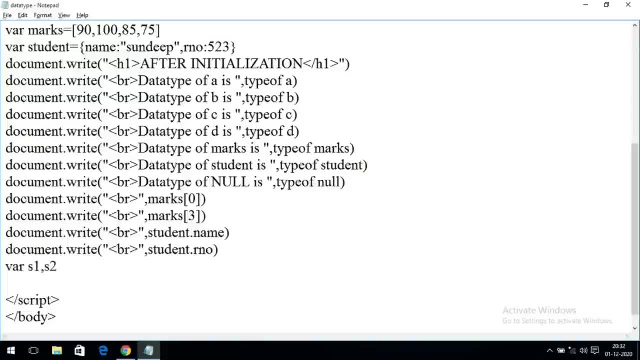 represent the string in either single quotations or double quotations, so both we can use. so i will show you. so where s1 comma, s2, two variables. i have given two variables so we can assign any value, any data type of value can it can be assigned to these two variables. so now i will go with the s1. 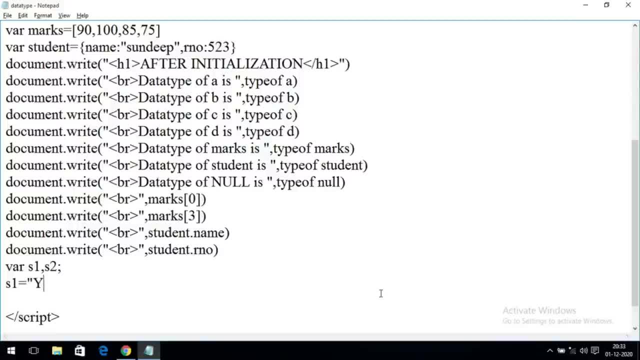 is equal to in the double quotations i will write yours. so i have given apostrophe s right, your apostrophe s. so that means i am using some single quotation here. and similarly, s2 is equal to single quotations. hello sendi, right. so inside the double quotations i have given some single quotation. right now i will print. 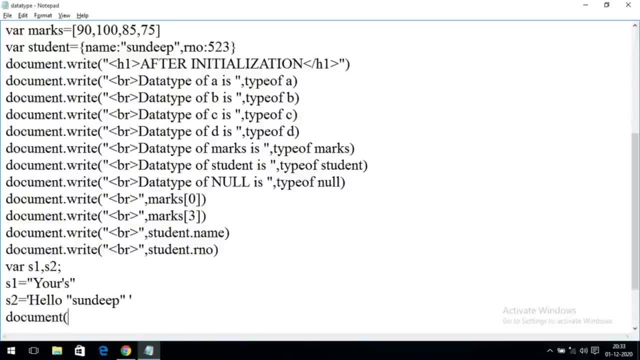 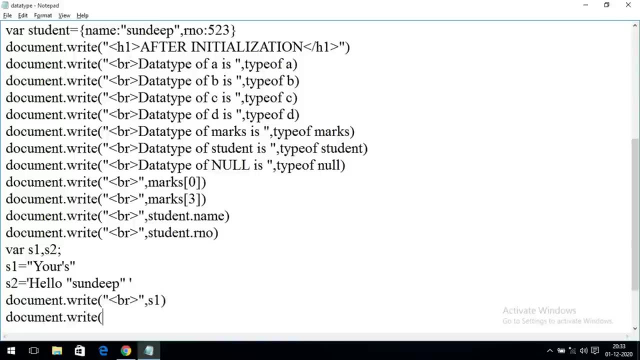 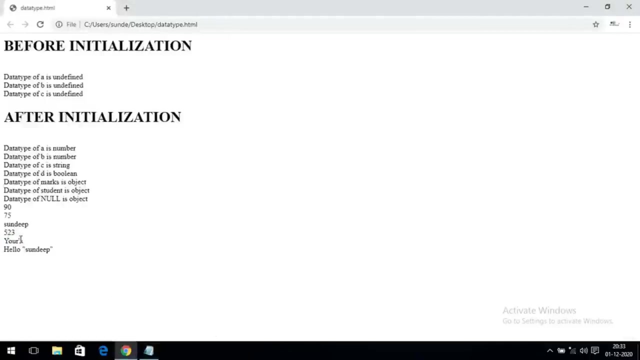 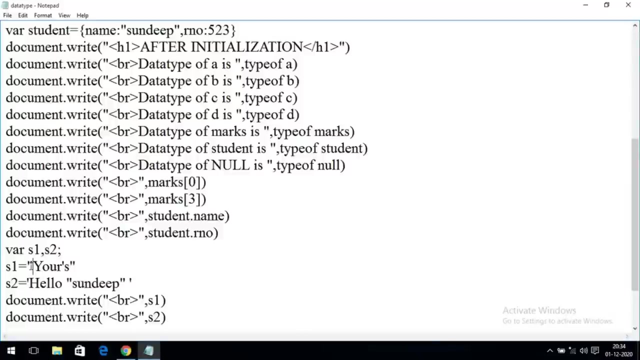 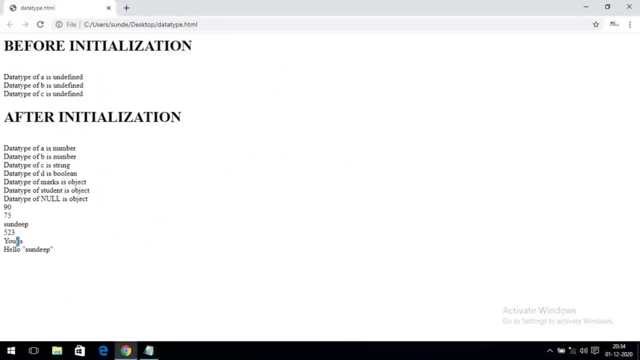 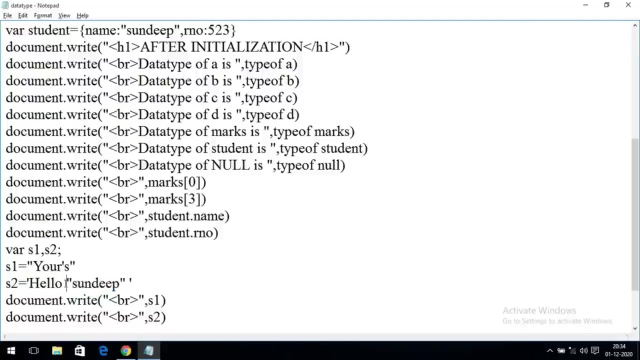 document dot- write br s1. similarly, document dot- write br s2. you can observe here, see, inside the double quotations, we can use the single quotation. inside the single quotation we can use the double quotation. right? so here you can observe, we have given the complete content in double quotations. inside the double quotations, we have given one single quotation, but that has been displayed on the output stream. and coming to the second example, the complete content was enclosed in single quotation, but the part of the content is enclosed in double quotation, right. so here you can observe, we have given the complete content in double quotations. inside the double quotations we have given one single quotation, but that has been displayed on the output stream. and coming to the second example, the complete content was enclosed in single quotation, but the part of the content is enclosed in double quotation, right? so here you can observe, we have given the complete content in double quotations. inside the double quotations, we have given one single quotation, but that has been displayed on the output stream. and coming to the second example, the complete content was enclosed in single quotation, but the part of the content is enclosed in double quotation, right? so here you can observe, we have given the complete content in double. 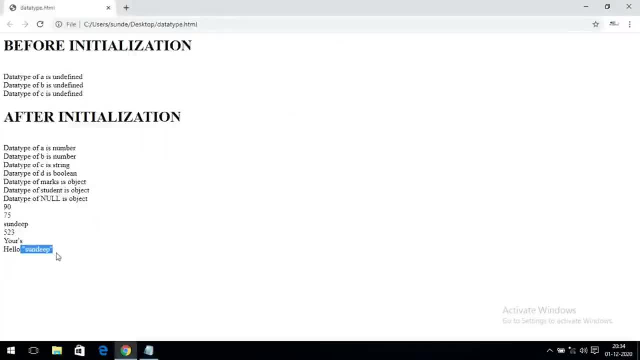 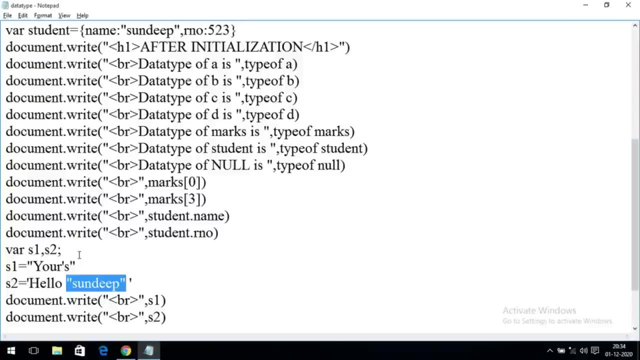 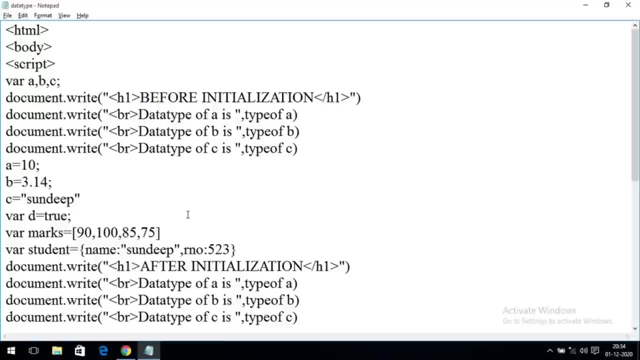 quotations so that double quotation will also be displayed on the output stream. so a string can be represented by enclosing the string, either with double quotations or a single quotations, right. so here in this session we have seen the different data types, like numbers, strings, boolean arrays or objects, and then how to find the data type of particular variable, like using type of keyword, right. so 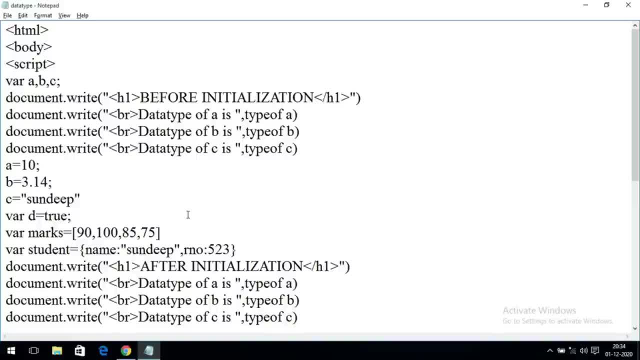 here. the data types in javascript are dynamic, so we did not use any particular data type while declaration. so we have to declare all the variables by using only one keyword, that is vr and depends upon the value or depends upon the application logic. we can assign any data type to that particular variable. we can change from one statement to another statement, right? so hope you understood this session. 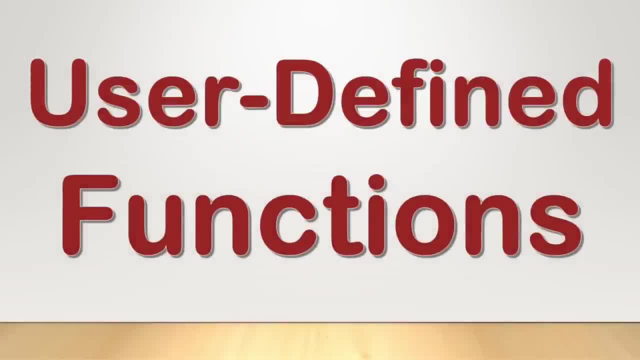 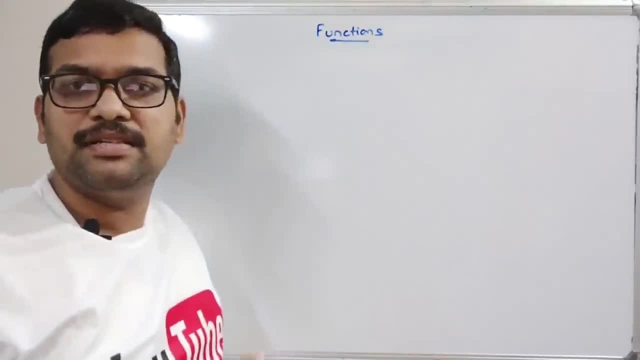 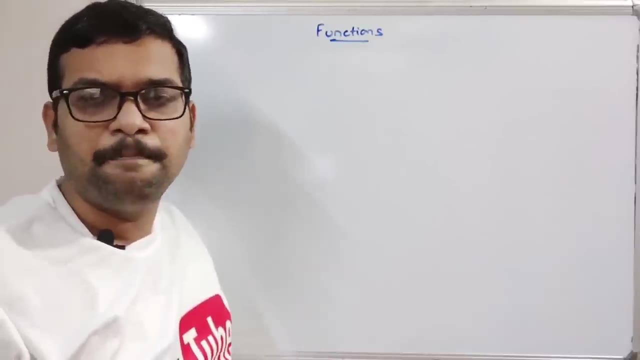 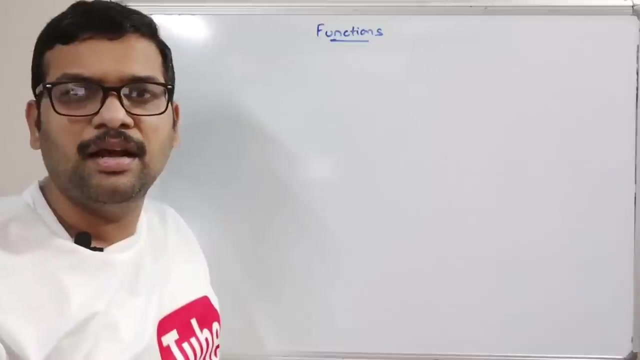 so how to implement these functions in javascript. so here we are having built-in functions as well as the user defined functions. so in this session we'll talk about the user defined functions, so how we have to write this user defined functions and how many ways we can execute this one right. so first one, 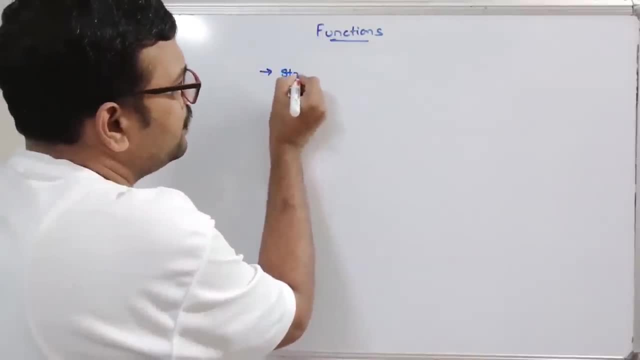 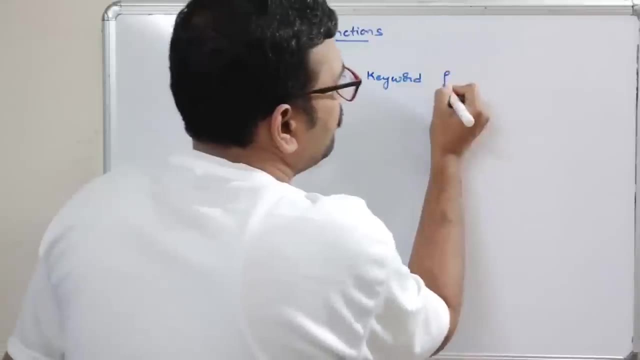 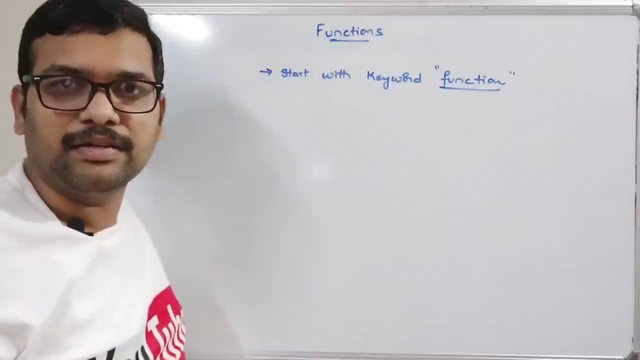 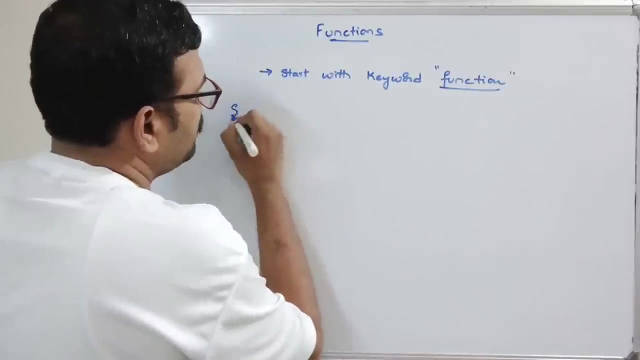 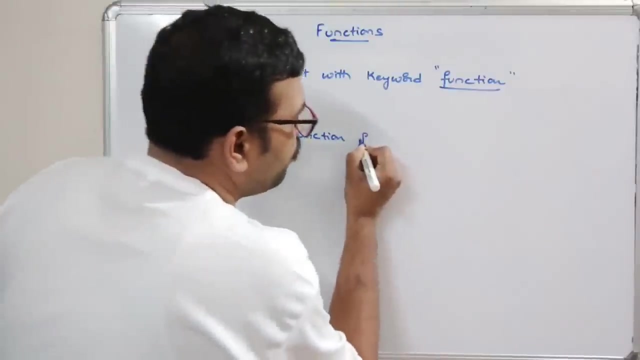 these user defined functions should should start with a keyword called function, a keyword function. so all the user defined functions should be starting with a keyword function, right? and then the syntax for implementing this function is function. so this is the syntax for implementing this function. so this is a keyword, followed by the. 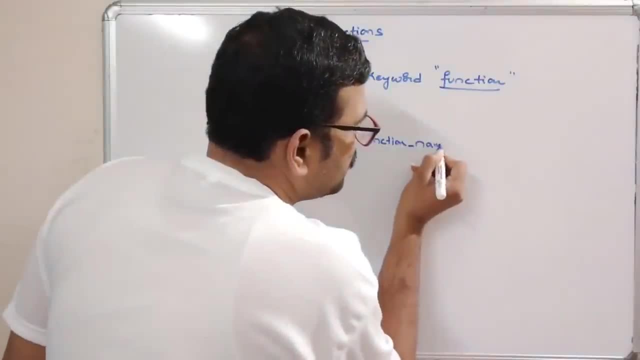 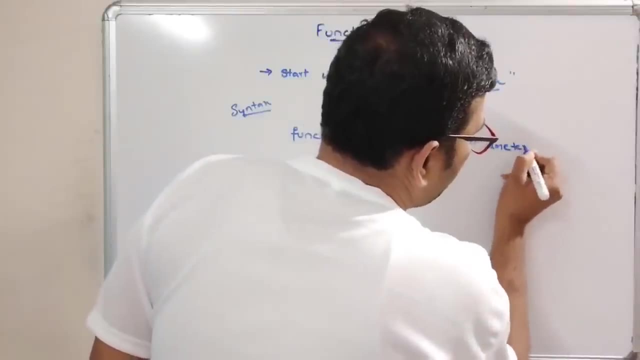 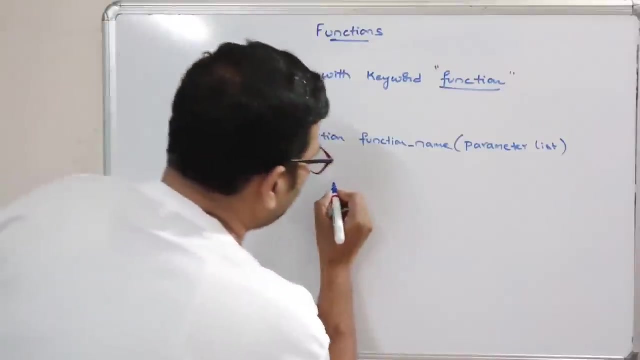 function name. so for every function we have to give some a function name, followed by the parenthesis, followed by the parameter list. so here we have to pass the parameter list. so parameter list, and followed by the curly braces. it's a block of statements, and here the statements: 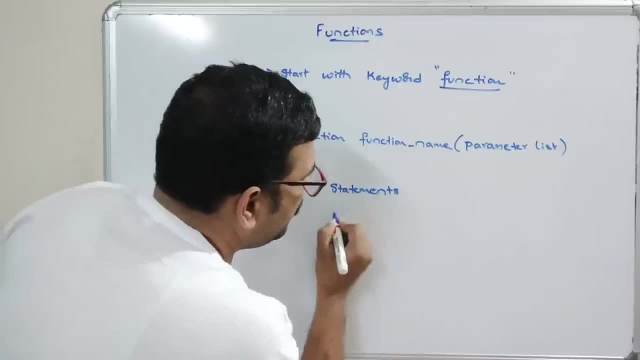 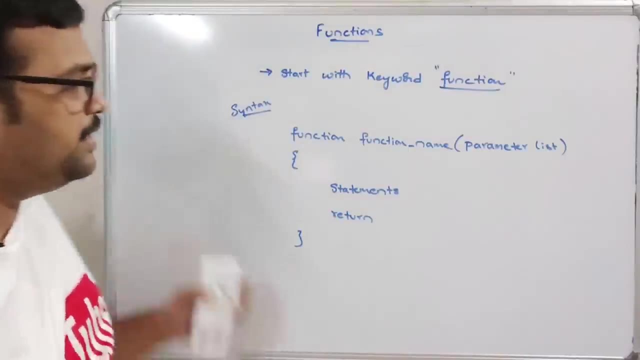 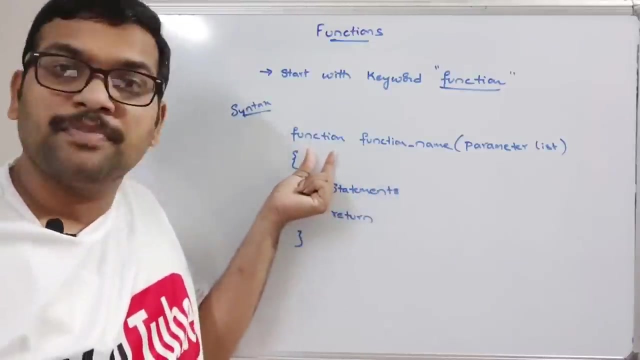 so, which we need to implement in this function, and then the return function, return type. okay, the return function, return statement, and this is a prototype for implementing any function, so the function, followed by the function name. so this is the keyword. okay, this is the keyword and this is the identifier. so we have to follow the rules. 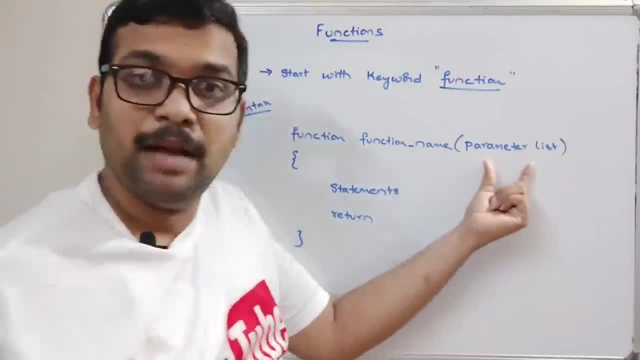 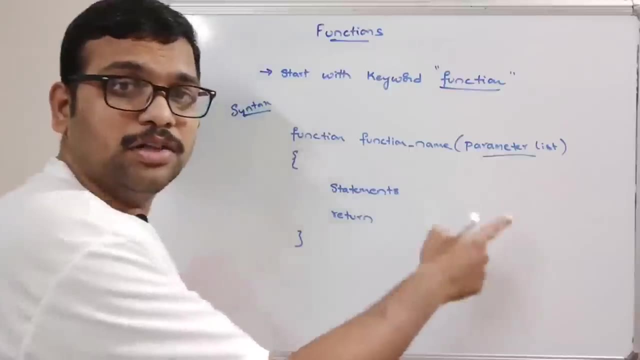 while giving this name okay, and coming to this parameter list, that is an optional, so we can give the input for this function in in terms of parameter list here, or we can also give the parameter list inside the function, right, and followed by the statements. that is a logic which. 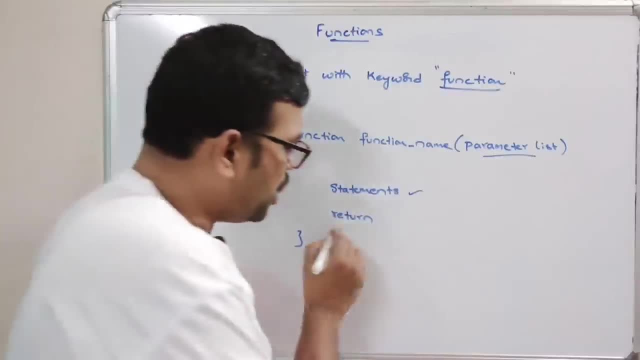 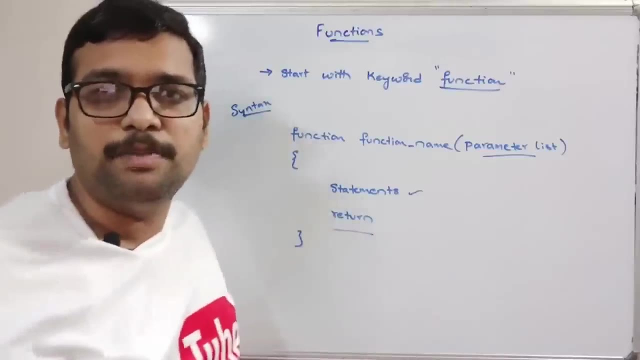 we want to implement, and followed by the return. so this is also an optional. so if you want to return any value, then we have to go with this return statement. otherwise we can directly display the output here itself. okay, inside the function itself. now, when this function will be. 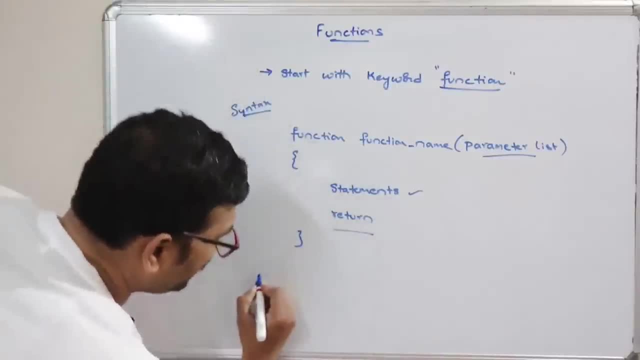 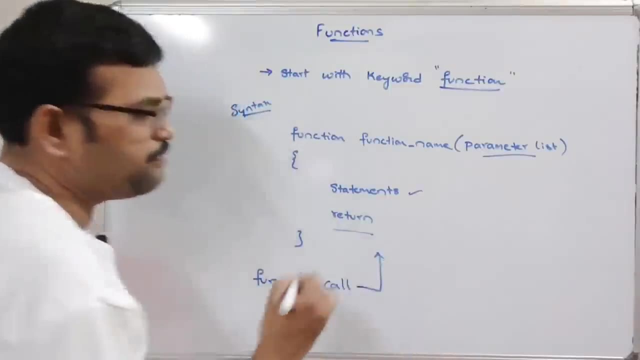 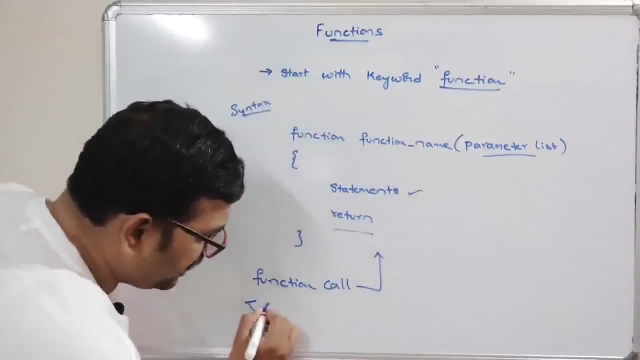 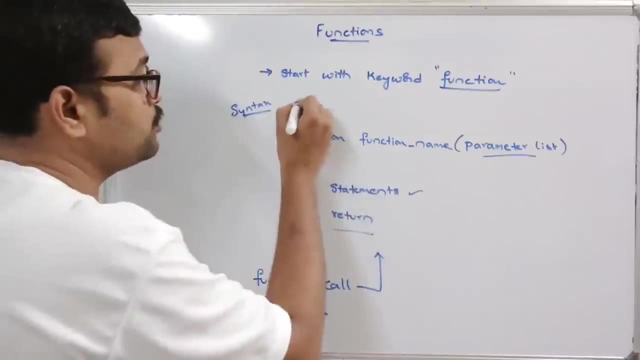 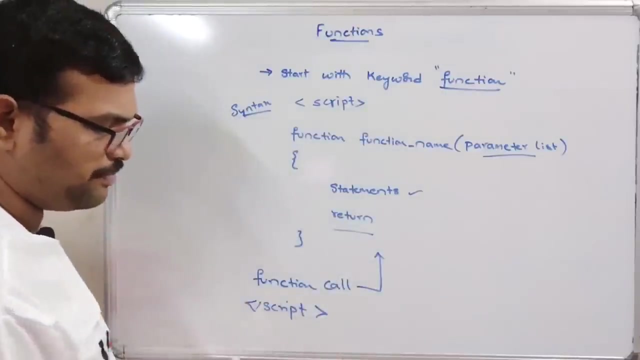 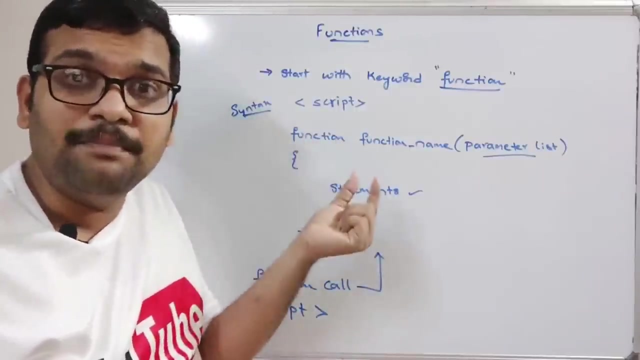 call, and this function call should be written inside the script. okay, as well as this is this function definition should also be written in script tag itself. script tag itself, right? so whenever the control executes this one, whenever the control finds this function keyword, so that implies this user defined function should be executed only after the function call. so 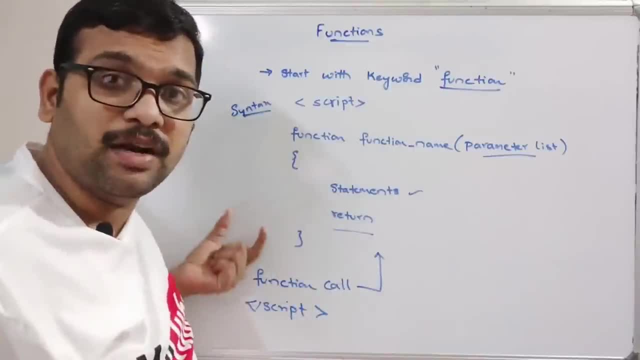 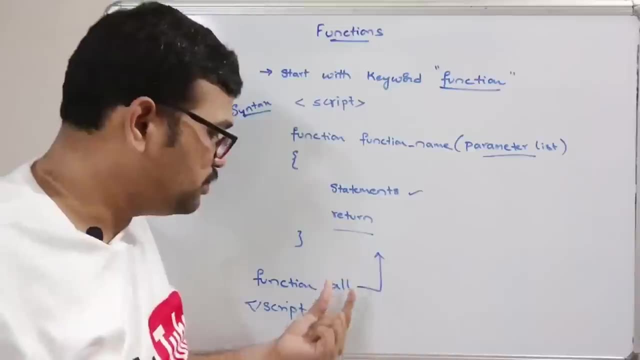 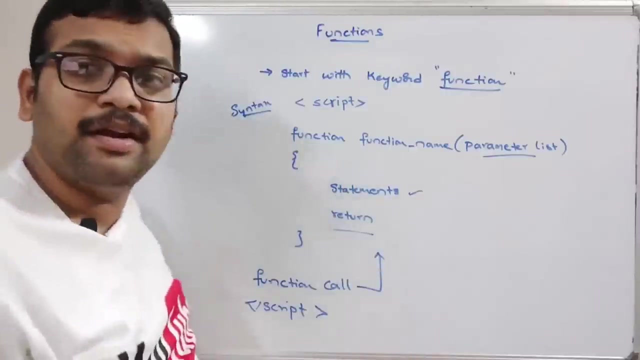 automatically it will go for the next statement after completion of this function definition. so immediately here we'll get the function call. whenever the control executes this function call, automatically it finds for the function definition and this function definition will be executed and output can be returned in a one among the three cases. so one is by using uh in. 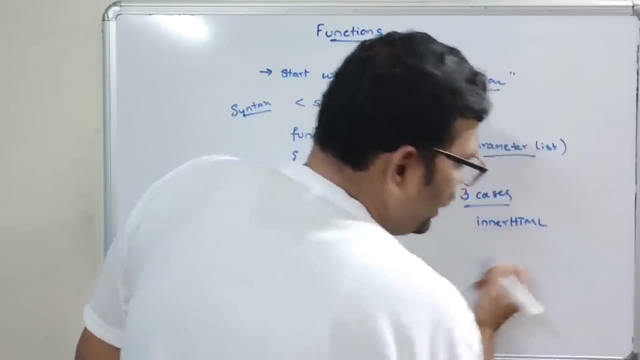 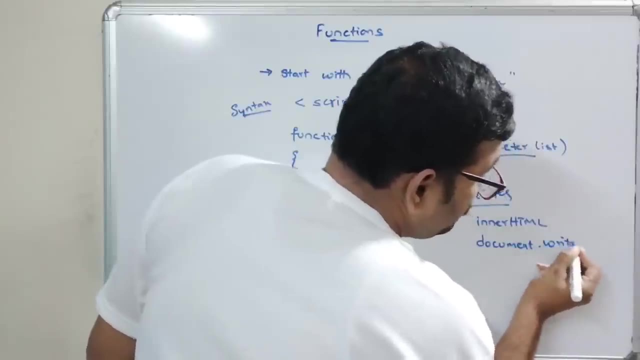 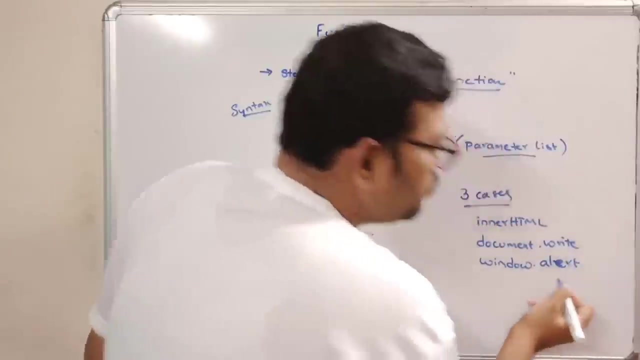 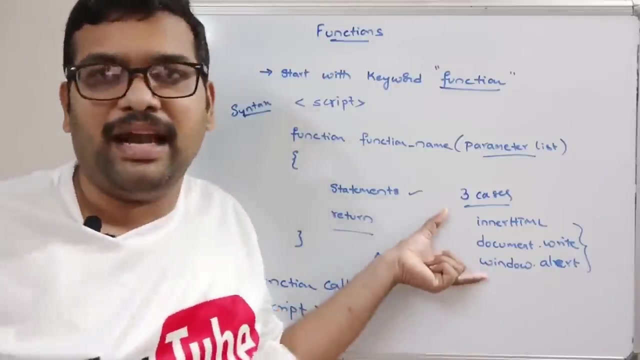 the HTML. so we have seen this one right in our HTML. and then document dot right. okay, document dot right as well as window dot alert. so we also seen this one, window dot alert. so we have to give the output, we have to display the output in one among these three. 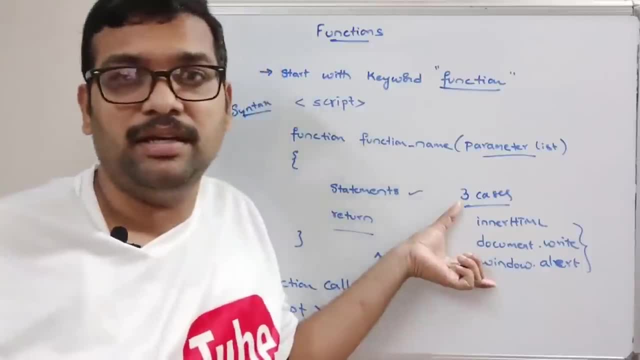 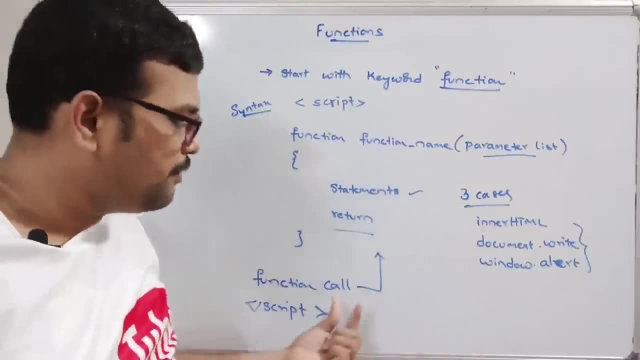 categories. okay, we have to choose any one among these three in order to display the output and passing the parameter. that depends upon the logic, so we can pass the parameter from the function call itself. so if you are giving any parameters or inputs in the function call that, 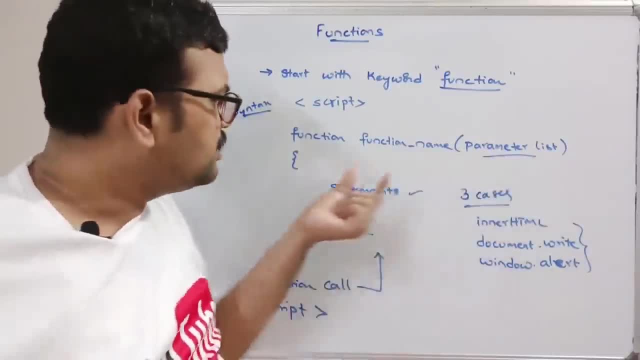 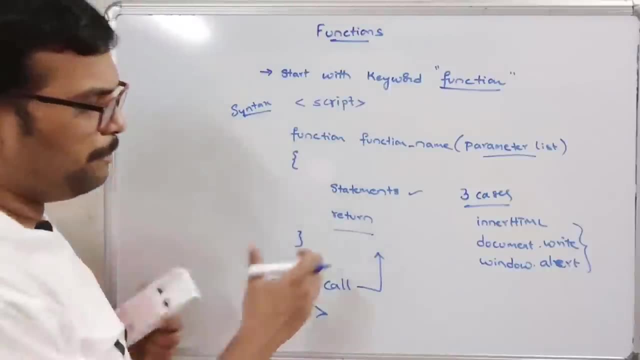 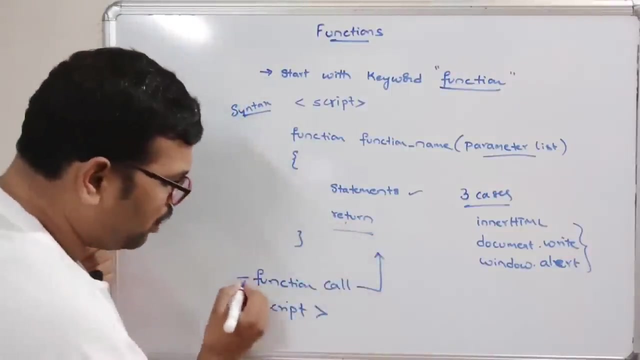 should be reflected in this parameter list in the function definition. otherwise, simply we can give the input inside the function call function definition also. and also, if you want to print the result outside the function, you have to use this return statement and that function call should choose some variable and the result of this function definition will be stored in this. 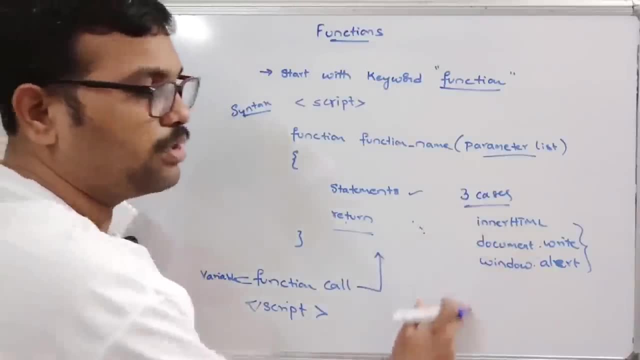 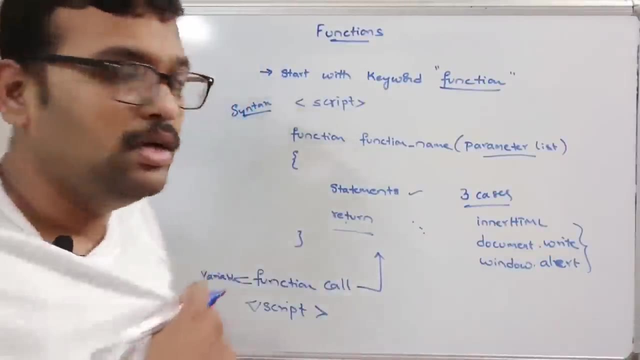 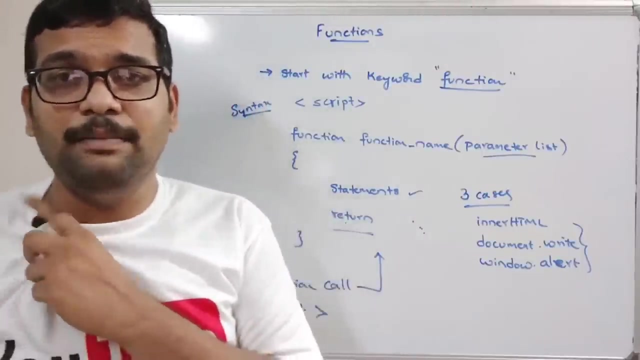 variable, so that we have to display this variable by using one among these three things. these three functions: inner HTML or document dot right or window dot alert right. so this is how we can implement the functions. okay, so one thing we have to remember, that is, so function can be: uh, returned. 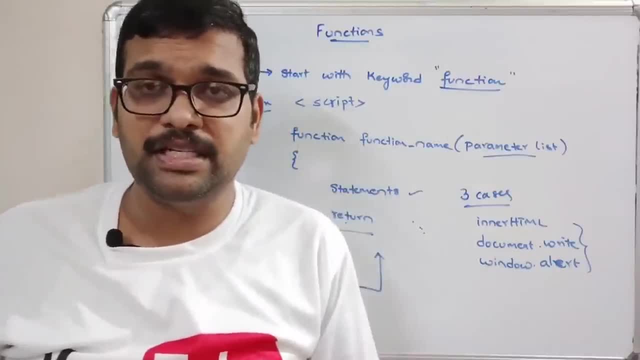 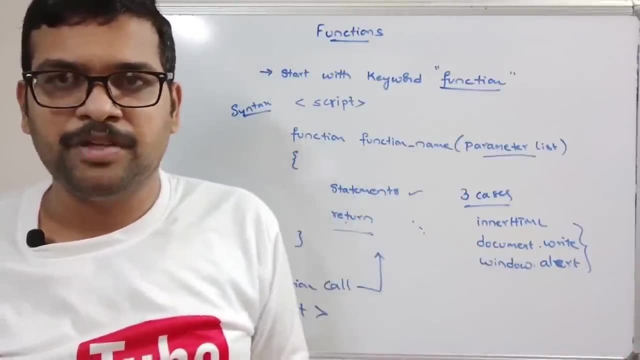 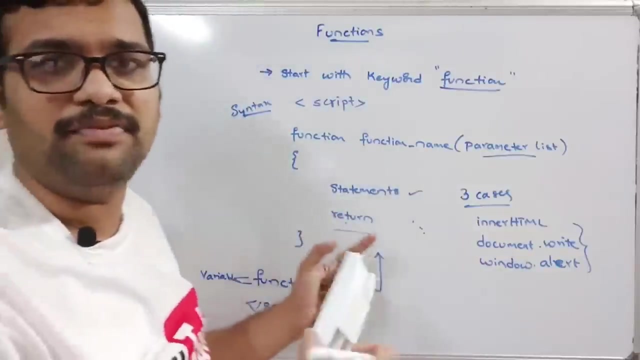 inside the script and we have already seen in the previous sessions that script tag can be included in inside the head tag or inside the body tag. so anywhere we can write the functions, anywhere we can write the script tag. so inside the script tag we have to write the functions and 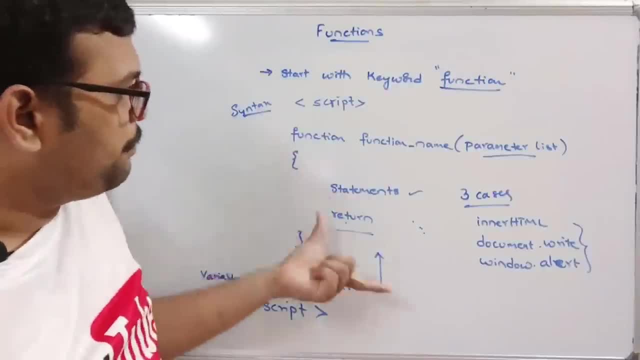 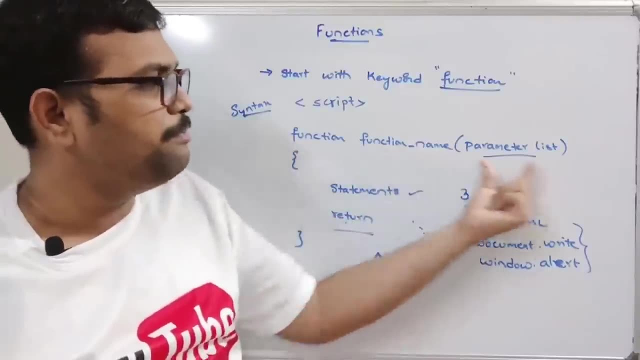 we have to implement these functions right. so this is the prototype. once again, I'm saying this: function user. different functions should start with a function keyword, followed by the identifier name, parameter list and the statements and the return. right. so now we'll move on to the computer. 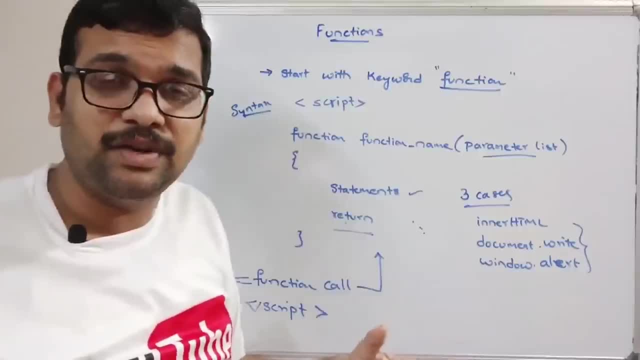 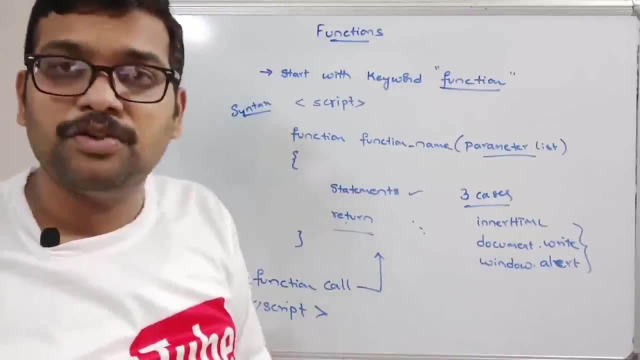 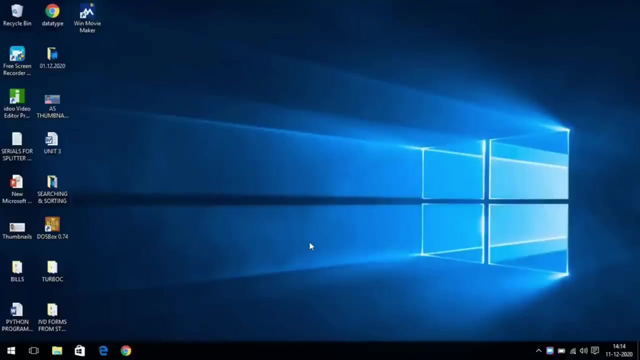 I will show you, I will demonstrate these function, how many ways we can implement this function and how can we display the output by using this. these three things, so all these things we will see by executing a small HTML code. right, so let us move on to the computer. hello friends. so just now we have seen the functions concept in. 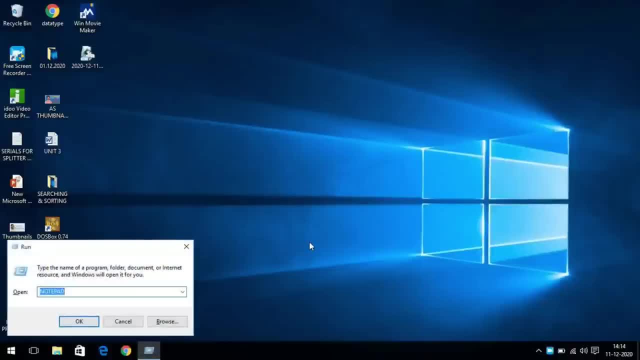 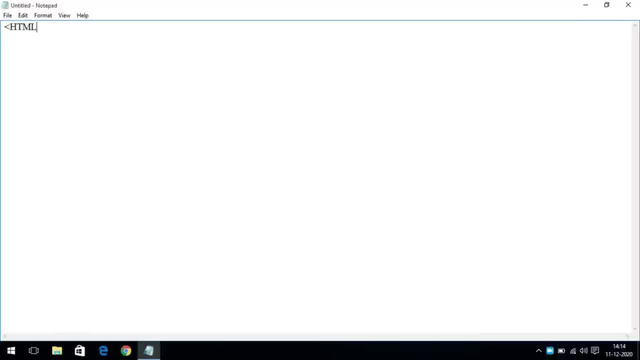 JavaScript, so how to implement the function. so every function should start with the function keyword. so let's demonstrate that. the small HTML code. so first we'll write the HTML tags. so inside the HTML I will write the complete function in the script itself. right, so we can. 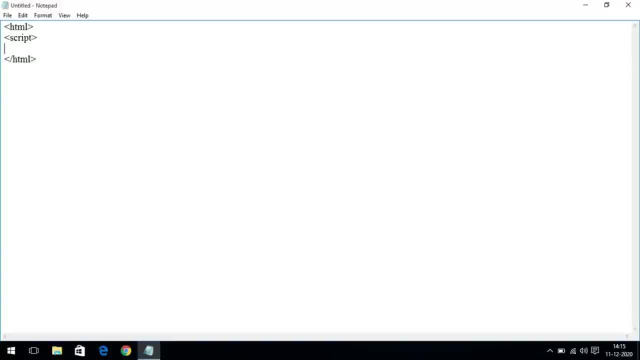 write the JavaScript in either script tag or a body tag. so I will write it in script tag. yeah, yeah, inside the script I will. first I will write the function. so every function should be starting with the keyword function function, followed by some add. okay, let us take some a comma b or x comma y, x comma y and use the curly braces and 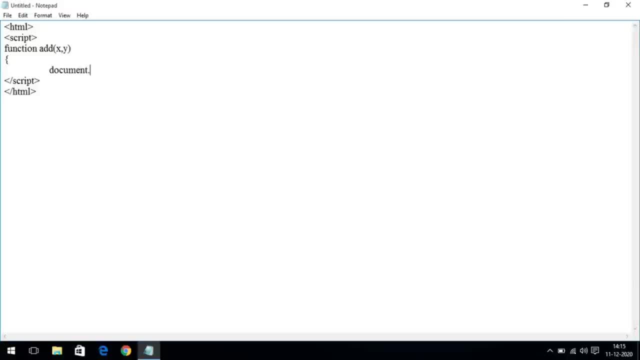 here we can write the document. dot write x plus y, so x plus y. yes, so for this we have written here and automatically, if this function is to be triggered, we have to write some function call. so for that function call we can write here the function. we will take some variables where some a, comma, b and initialize some values. a is equal to 10 and b is equal to 20.. 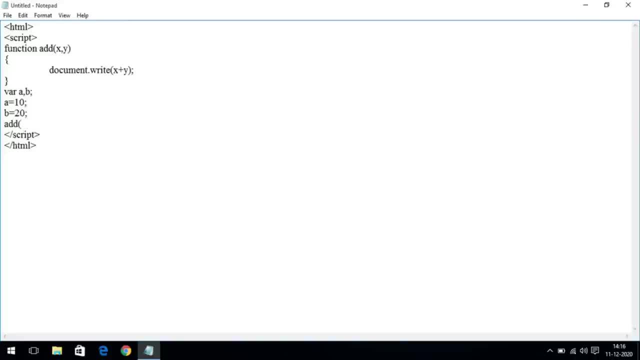 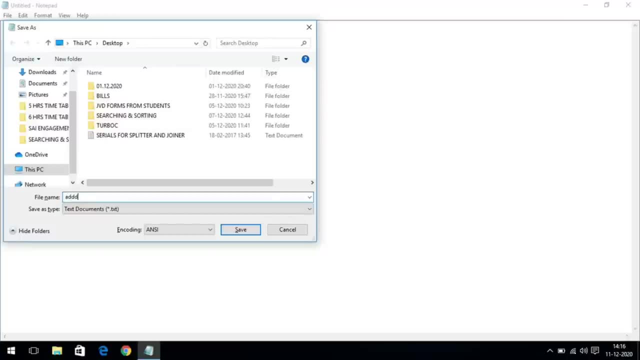 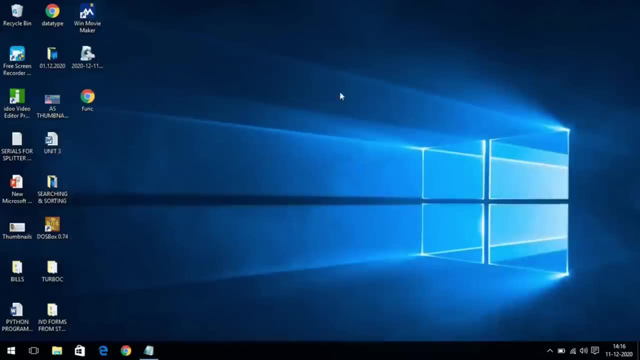 we will take a function here and write down the function: call right, add a, comma b. okay, so let us save this one with the help of one name, some. let us take some function: dot HTML. so I have saved this one in the desktop, so here you can see this file, so by double click on this. 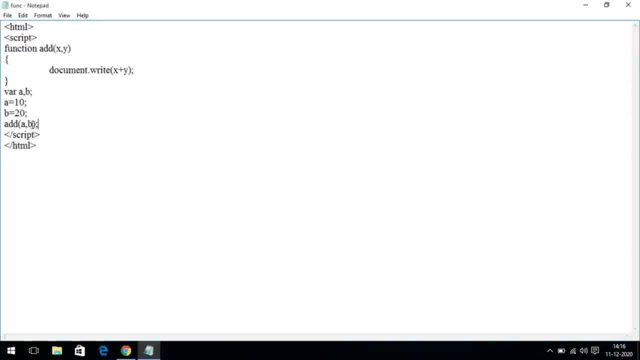 one, we'll get the result 30 right. so automatically this function call will be so only whenever an event occurs. I mean, whenever an event occurs or whenever the function call executes, then only this function definition will be executed, right. So this function keyword gives an. 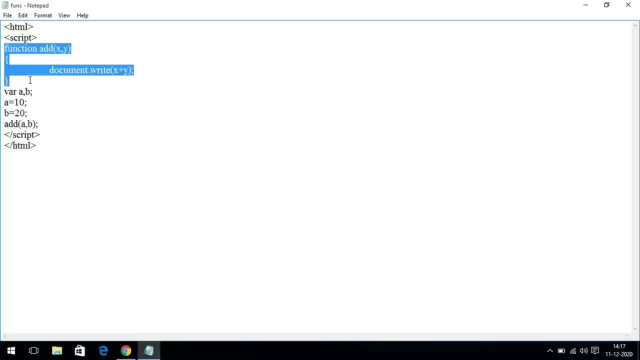 idea to the JavaScript that this is a user defined function and that is a function definition and it should be executed only when the function call is executed. So here you can write: sum of two numbers is So that complete content will be here, So you can also use the tags. 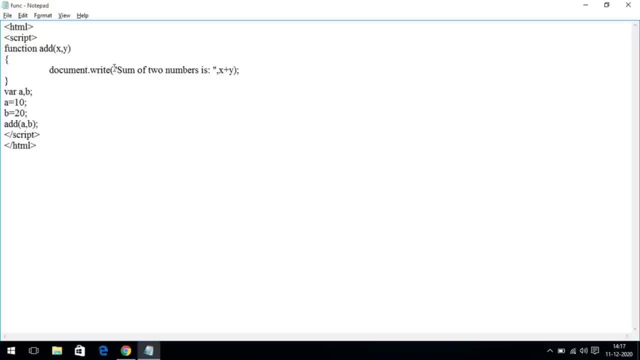 here you can also use the tags. So, with the help of tags, you can write down here h1 and here you can close h1.. Okay, Okay, See, this is how we can write this one, and so this is the function definition without. 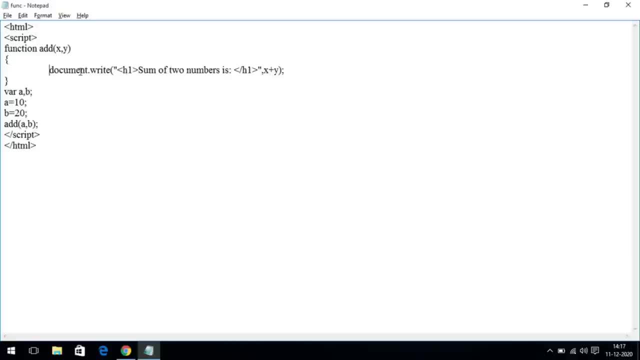 any return. So here we are not writing any return function, So directly we are displaying the output. but if you want to return some value, So here I will initialize the same thing to one variable right. So here I will give a, b comma sum. 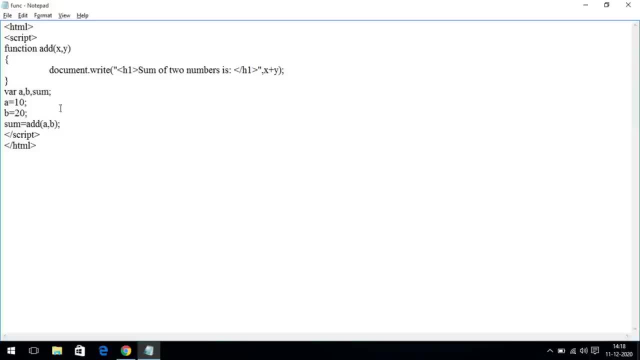 So sum is equal to add a comma b, So that here we can't write this one So directly, we can write the return statement. So we calculate the addition and we will just return the addition here, x plus y. So automatically the result will be stored in sum and after. 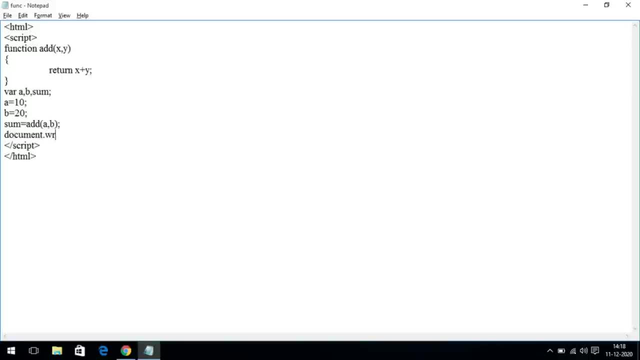 that we can write the result document dot write. So not only by using the document dot write, we can also use a window dot lth or inner his table. So we have seen the different possibilities, So we can display the output on the screen, So we can use any one among those three functions. 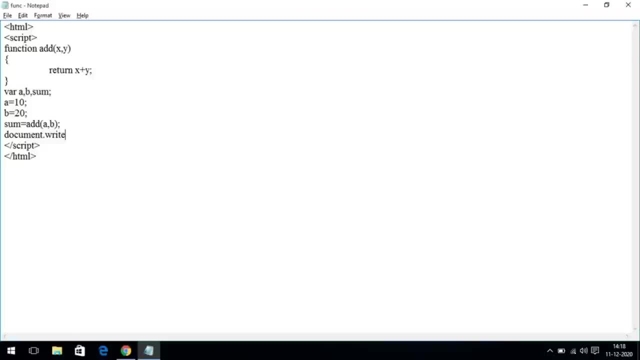 right, three categories. So by using document dot write or window dot lth or inner his table. but here I am using just document dot write, So document dot write, So you can write: sum of two numbers is and here we can give the sum, because So we are calling the function. 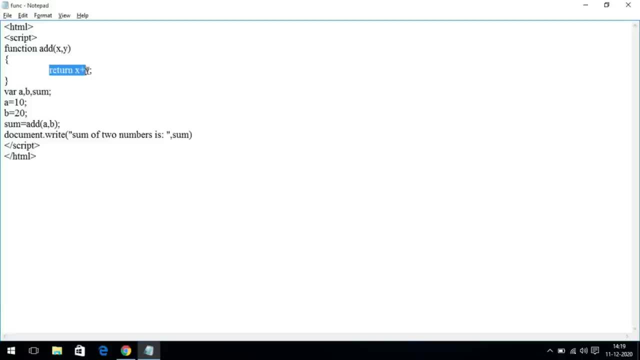 and the result. So the result will be stored in sum. So here we are returning the result. So, automatically, sum will be storing the result. So if you execute this one, So automatically, we will get the same thing. See, sum of two numbers is 30. So here we are returning the result. 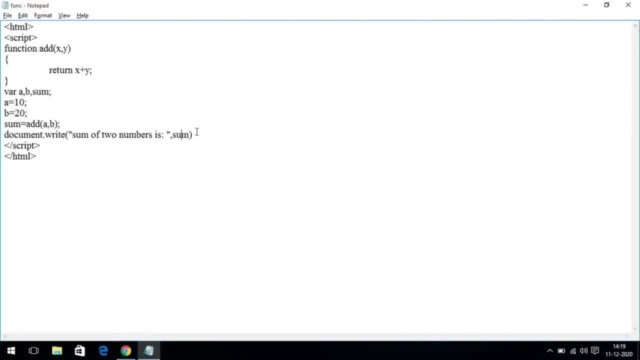 to one variable and that variable will be holding the result, So that we can directly display that result here. This is one, this is another way. So by using the return or directly, we can use that one and all these things. So, instead of writing this one, we 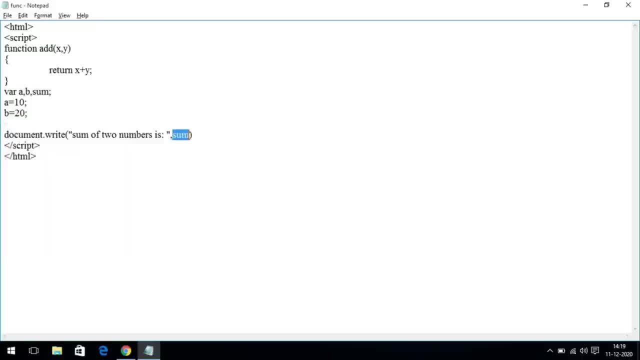 can also directly call here itself. So here itself we can call the function add of some a, comma b. So if you save this one and if you execute this one, So still we will get the same result, right? So sum of two numbers is So just we. I will change the text So. 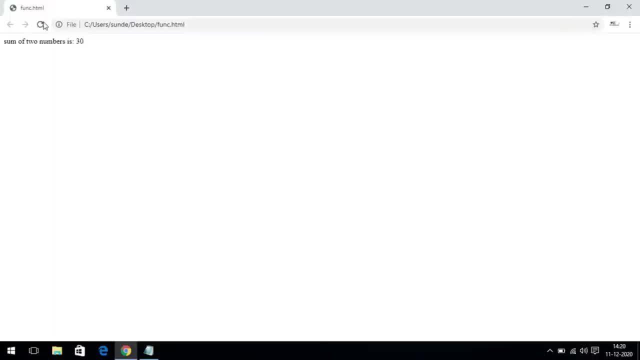 this is one. So addition of two numbers is. Now you can see the result: addition of two numbers. So we are not getting any error. So we can use the return and that return can be initialized to one variable and that variable will be holding the result and we 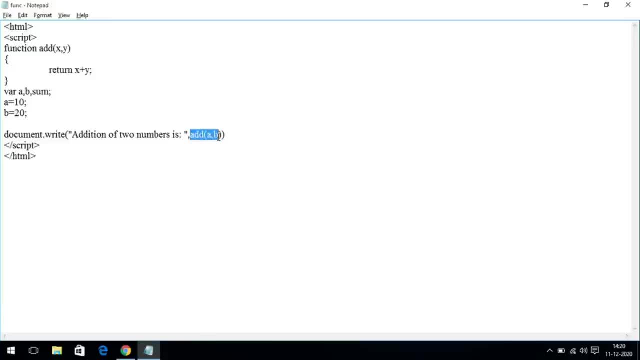 can print that variable, or directly we can use the function inside the output function, right, And this one. So with the help of this parentheses, the help of this parentheses, we can get the function definition. So another way. I will show you the another way, See. 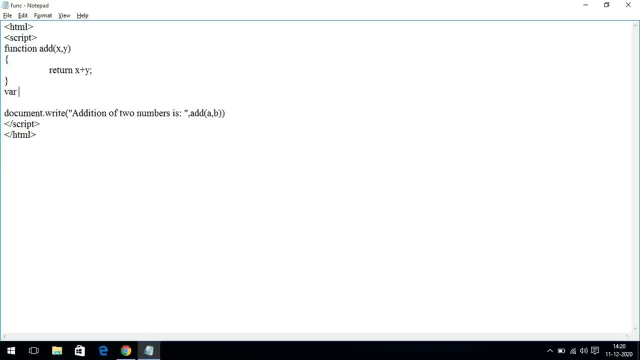 I am not initializing here, Just I am going with sum, or simply you can leave it and here itself we can declare the variables a comma x, comma y, ok, And we can also initialize the values: x is equal to 10 and y is equal to 20, and see, here I will remove this one also. 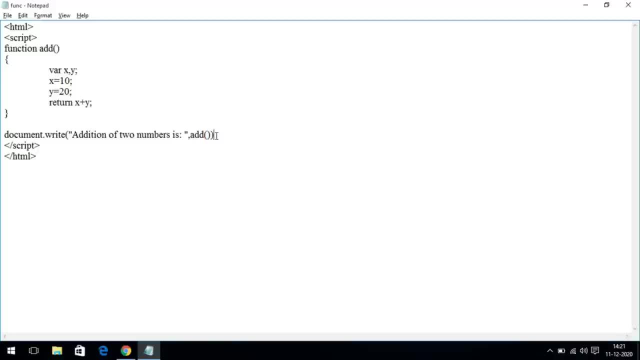 these parameters And here also I will remove these parameters. So if you execute this one, still we will get the same result. ok, Still we are getting the same result because here outside the function, we are not declaring any variables and we are not passing into the function call Directly. 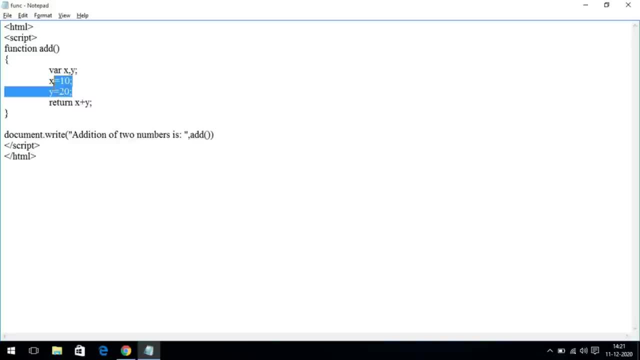 we are declaring the variables inside the function definition and also we are defining the values inside the function definition. So see, if you use these parentheses after this, one that gives the function definition, that gives the function And result. if you are not giving these parentheses automatically, it will give the function object. 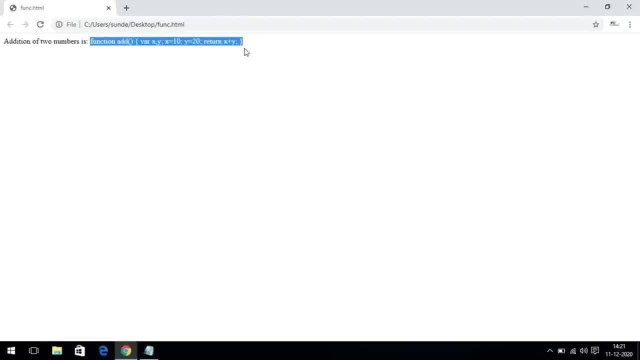 see, So this is a function object. this is a function object. we have written in the script that will be returned if you are not using the parentheses. So this is not using the parentheses for that function call. ok, So just I am using. 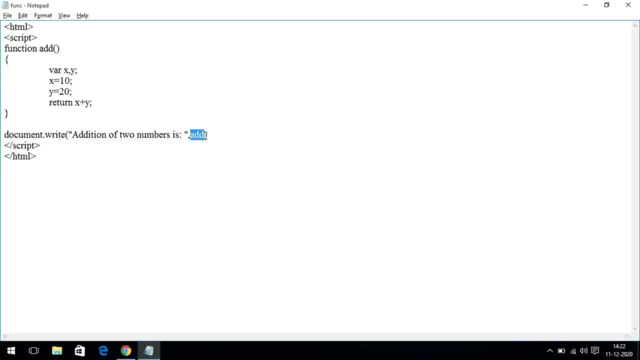 some add after that add. we are not using any parentheses. So that means it will return the function object, the complete function object, and if you use the parentheses here, it will give the function result. ok, See, you can observe the difference. addition of two numbers is 30 and the absence of this parentheses will get the complete function. 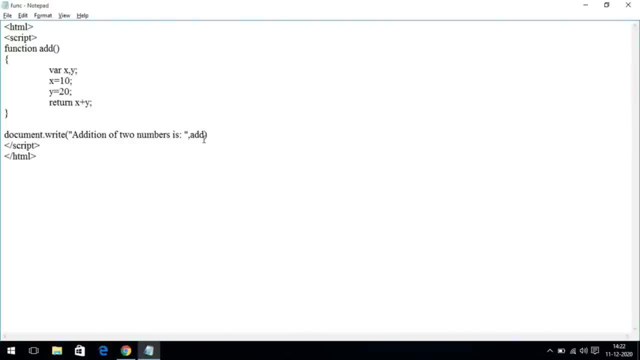 which we have written in the script tag. that is the one main thing. ok, that is the one main thing. and here, whenever we are calling about this functions concept, So we have to know about the local variables and a global variables and these variables which are declared inside the 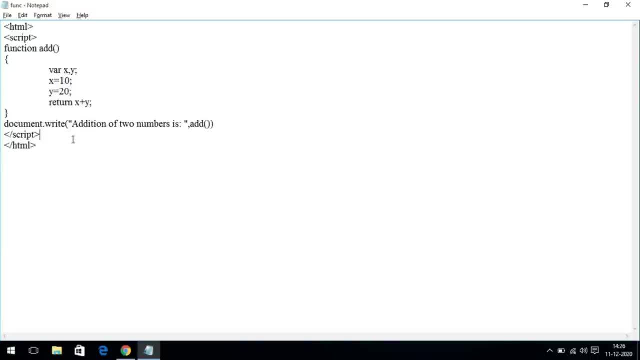 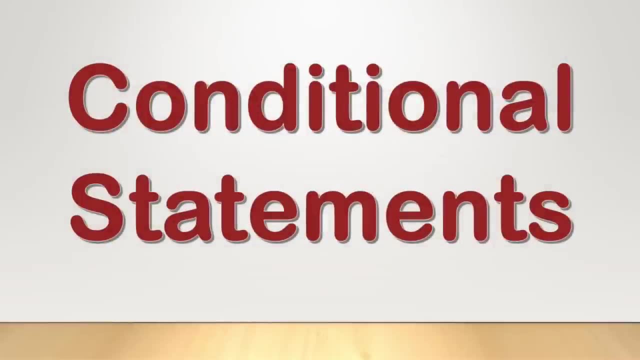 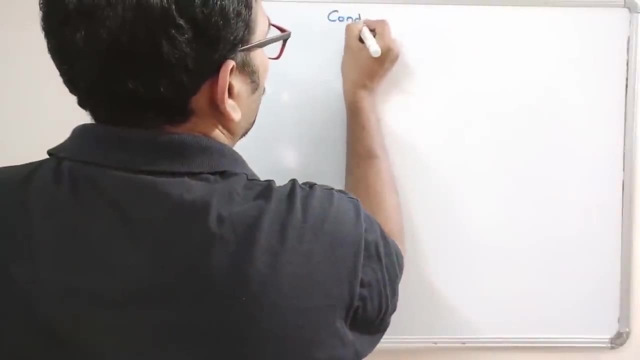 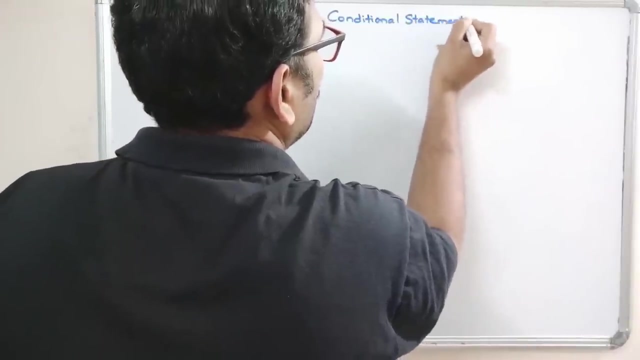 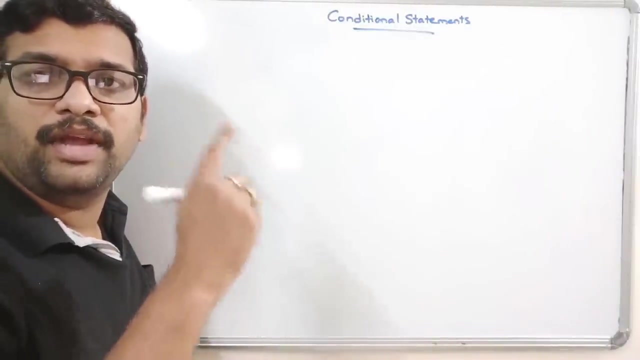 function will be treated as a local variables. This is how we can implement the functions in javascript. So hope you understood this functions concept. So here you can see that the name itself indicates based upon the result of that condition. So we have to decide which. 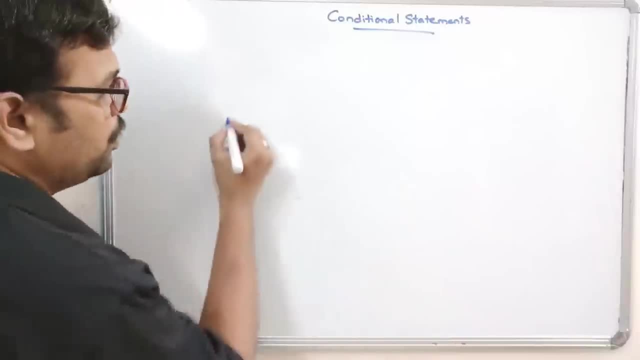 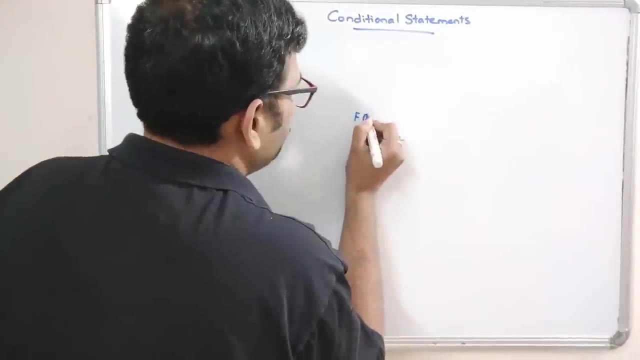 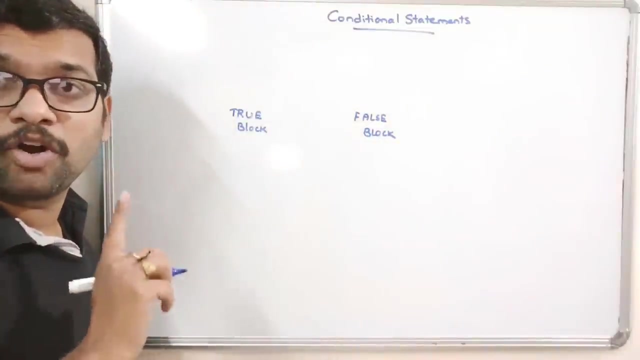 block should be executed. So here there will be two blocks of code: that is true block and this is a false block, right. So only one block of code will be executed, but not both, So that decision will be taken by the condition. 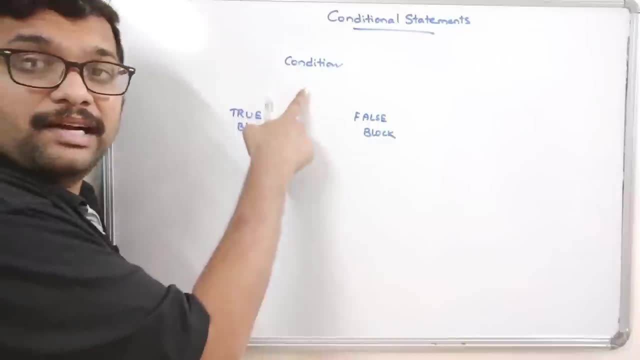 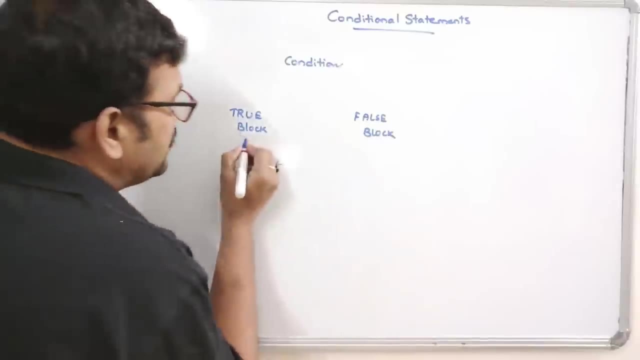 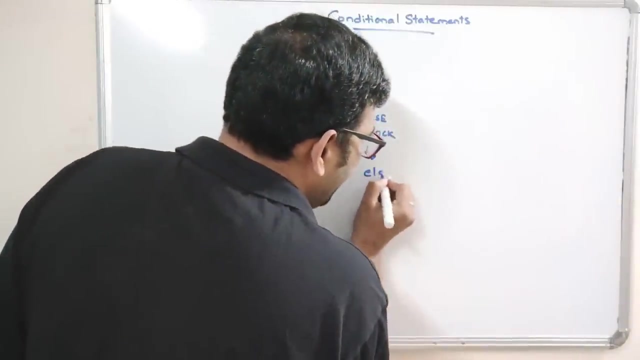 The result of the condition. So, based upon the result of condition, either true block will be executed or false block will be get executed, right, So this true block will be written as a if statement and this false block will be written as a else statement. 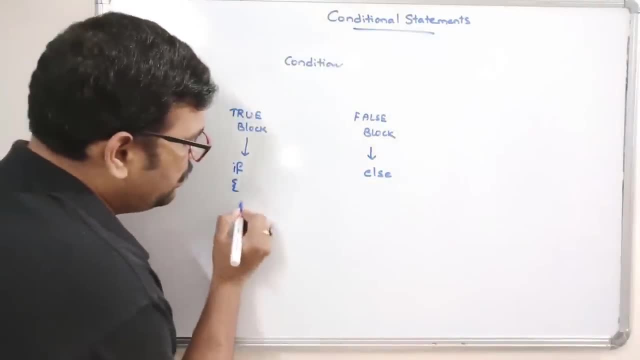 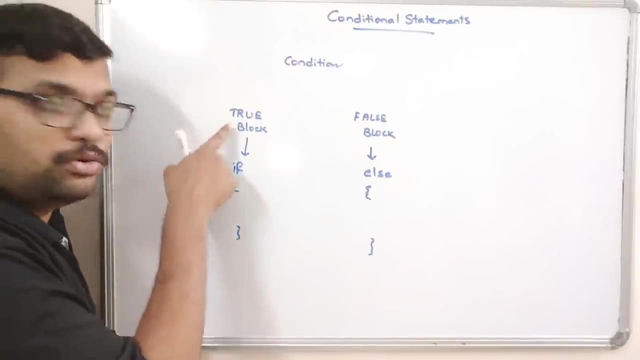 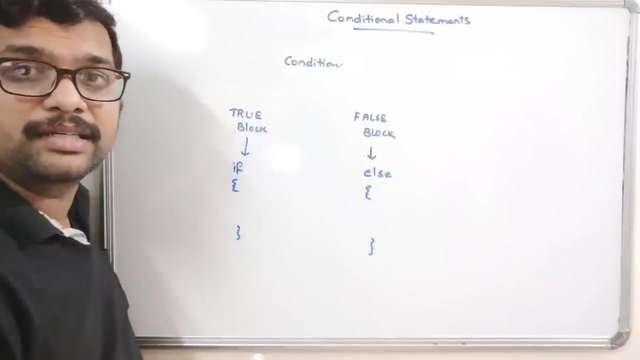 So we will write some block of codes in if and else. So this if block is represented as a true and this if block is represented as a false, And here the question is where we have to write the condition. So this condition should be written in true block itself. 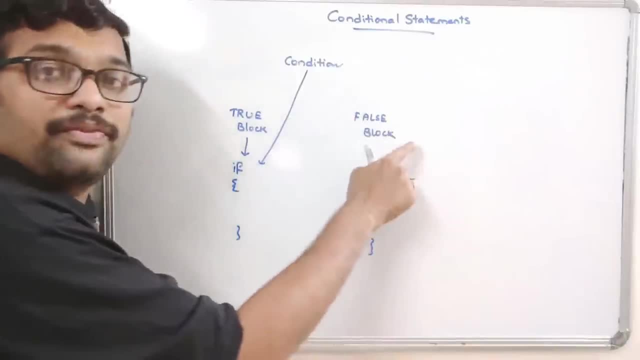 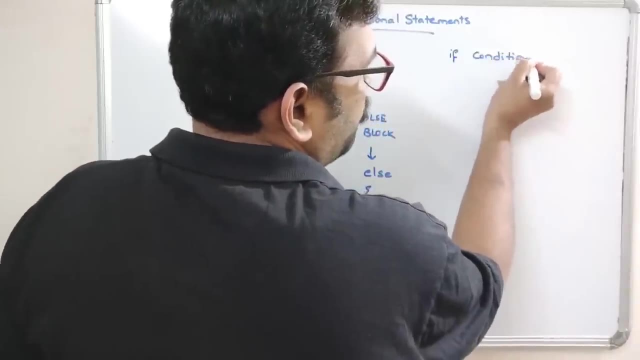 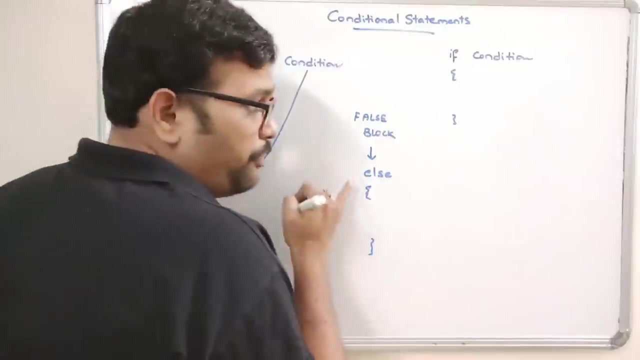 So we should not write any condition in false block. So here the syntax will be: if, followed by the condition, Followed by the condition, and write down the block. And if you want to write the false block also, you have to go to the. 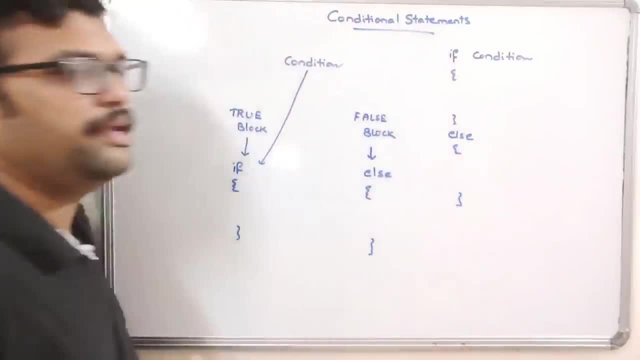 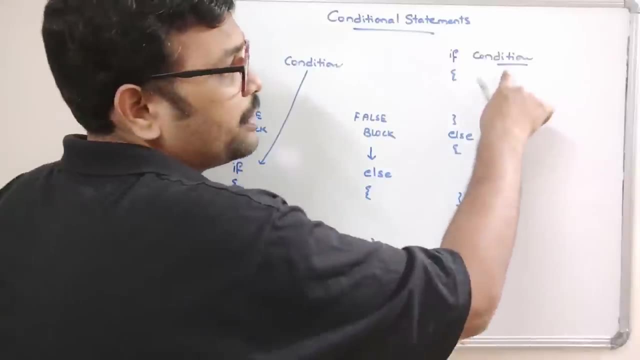 keyword else and write the code here. So, based upon the condition, if it is true, this block will be executed and this will be ignored. If the condition is false, this block will be ignored. this block will be executed, Right. 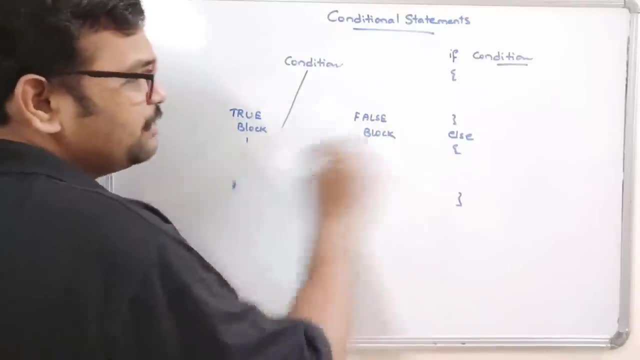 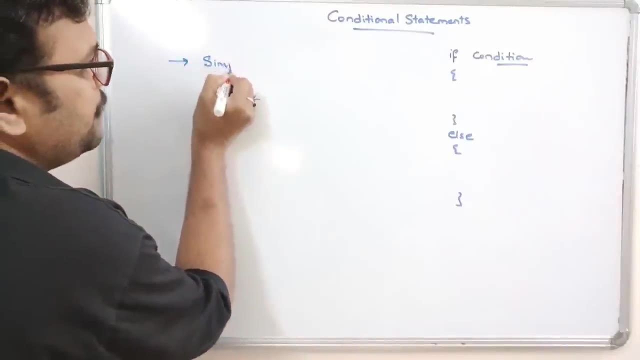 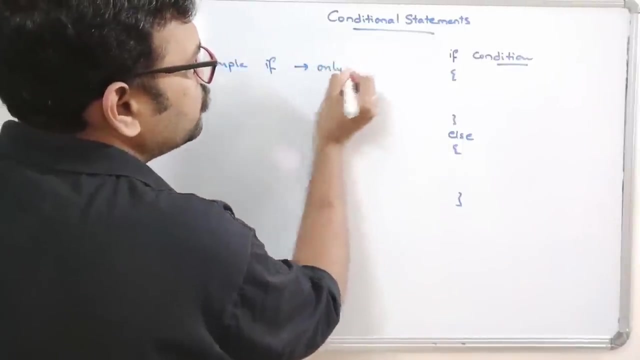 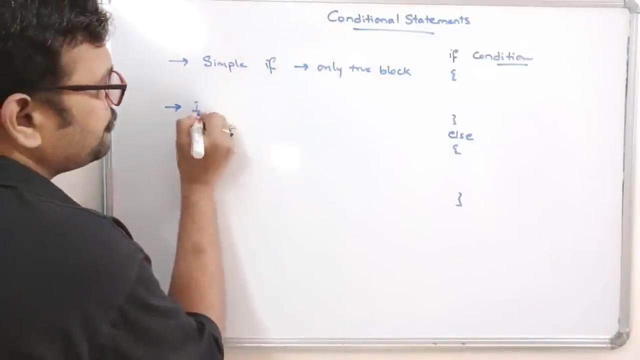 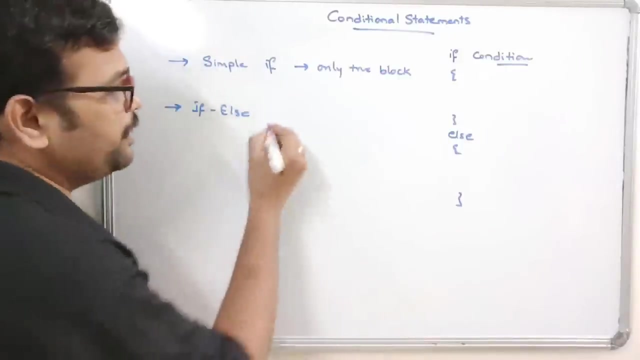 So mainly in this session we are going to discuss about the three types of conditional statements. One is simple- if Simple, if Simple if Where we will write only true block, So only true block will be written here. And the next one is if else. If else means both the true block and false block will be executed. 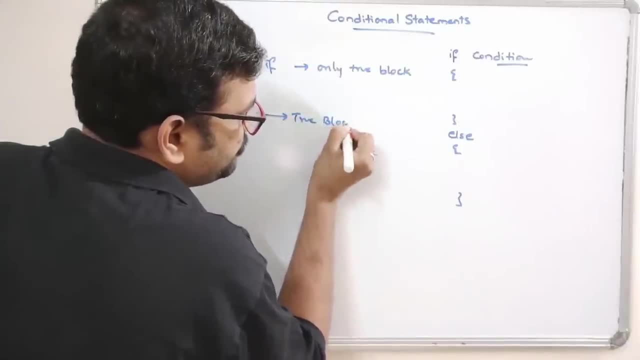 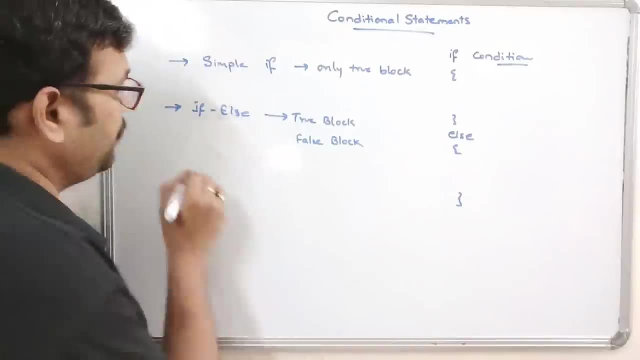 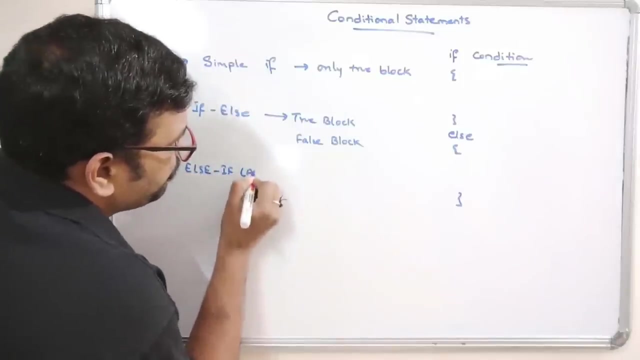 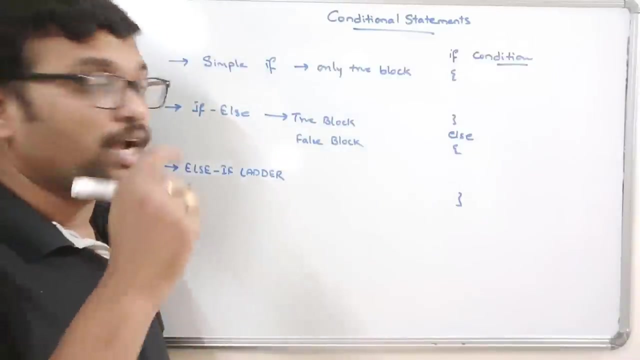 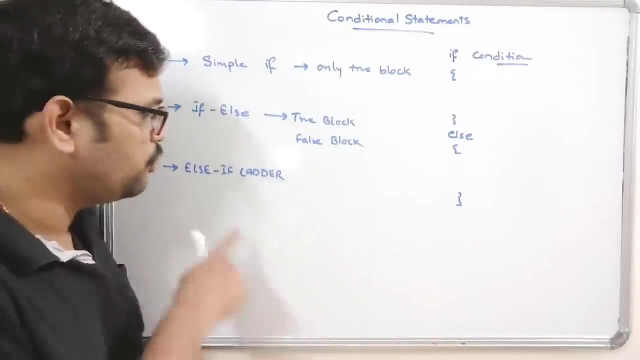 So true block and the false block, both will be implemented here. It executes only both And the next one else if ladder. Else. if ladder, That means if the condition fails. if you again want to check one more condition, that means in order to check more than one condition, we will go with this. else, if ladder. 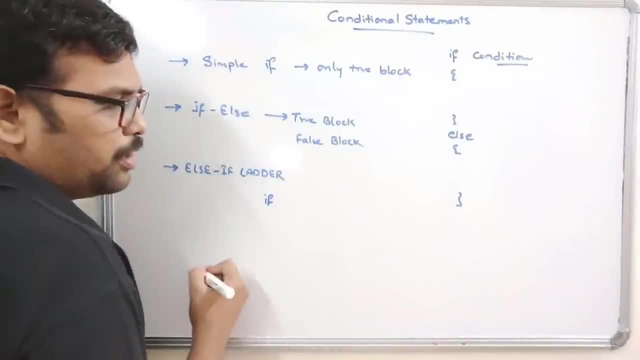 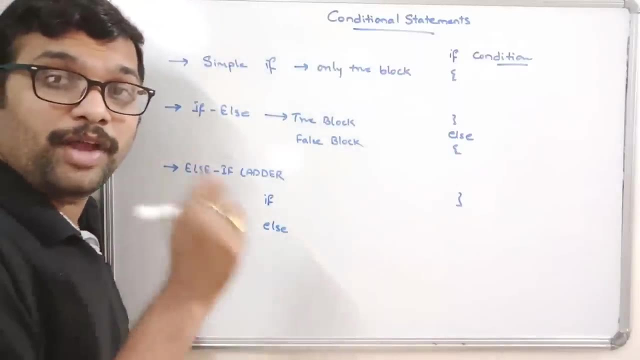 So here we will write some: if true block, Then else. And what we have just now? we have discussed about this one, So we have to write the condition only in the true block, So we should not write the condition in else. 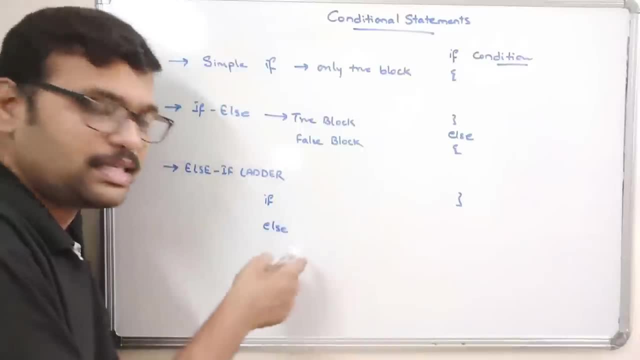 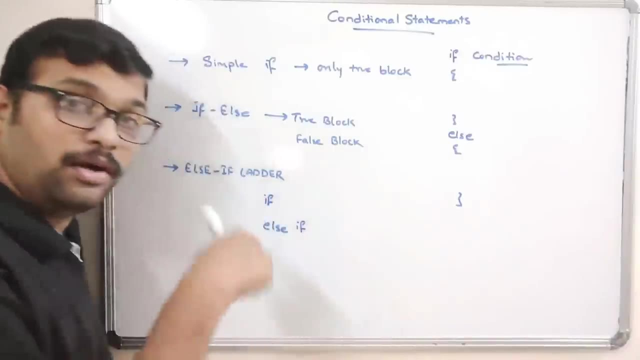 That means a false block. So if you want to check one more condition here, just include if and followed by the condition And if again, this condition fails again. if you want to check one more condition, go with another, else, if and else. 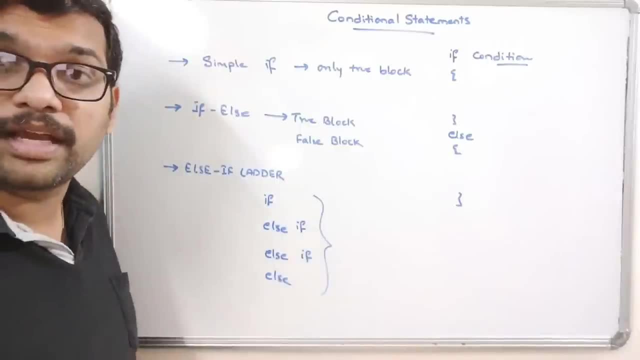 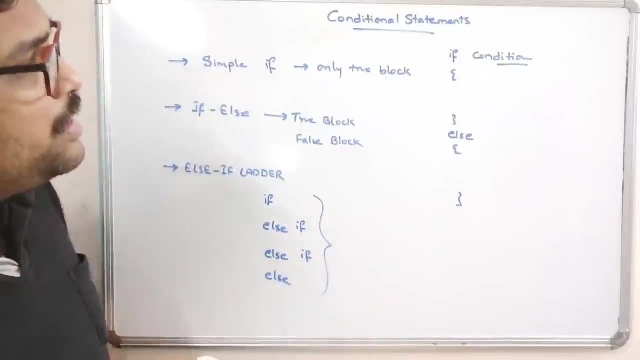 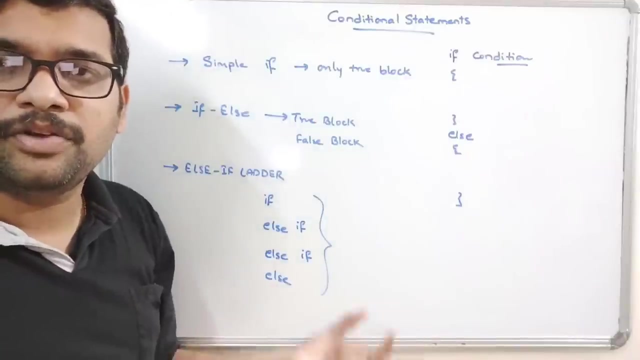 So this is the else if ladder. So we can check multiple conditions. We can check multiple conditions. So one thing: based upon the result of the condition, we are deciding which block should be executed. So either true or the false block. 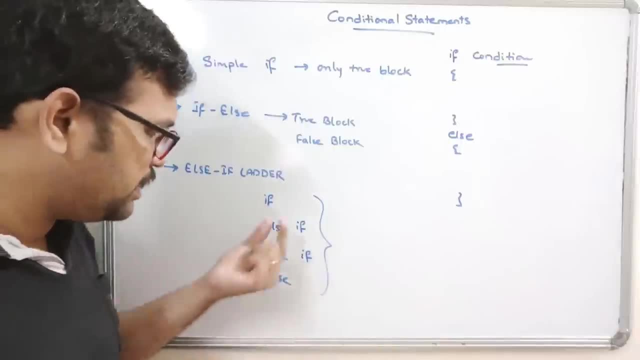 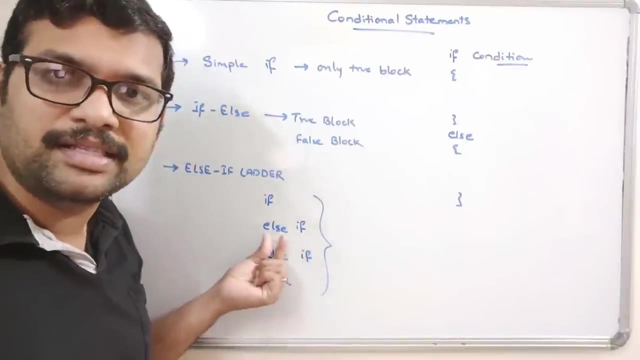 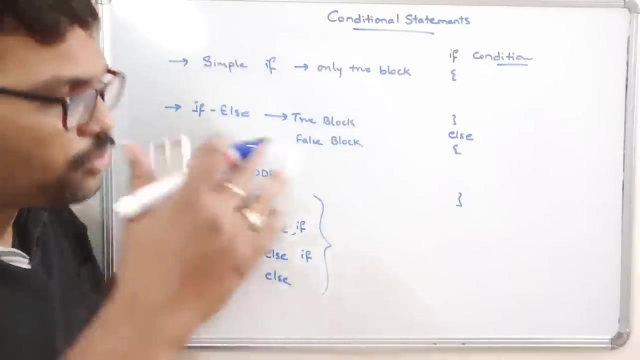 So if you want to check more than one condition, just include the true block and the false block So that forms the else if Else, if Else, if So, there must be space in between else and if Right. So this should be implemented and this statement should be implemented in script. 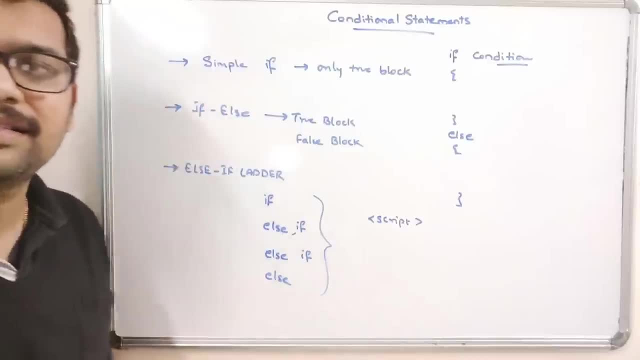 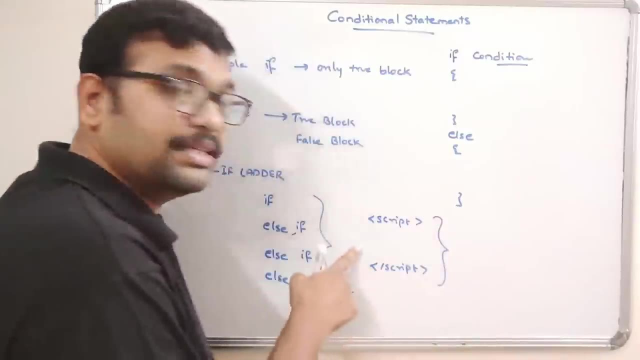 Script tag. Okay, All these are the java script, So we have to include all these things inside the script And where we have to write the script, As we have discussed in the previous sessions, we can include this script in either head. 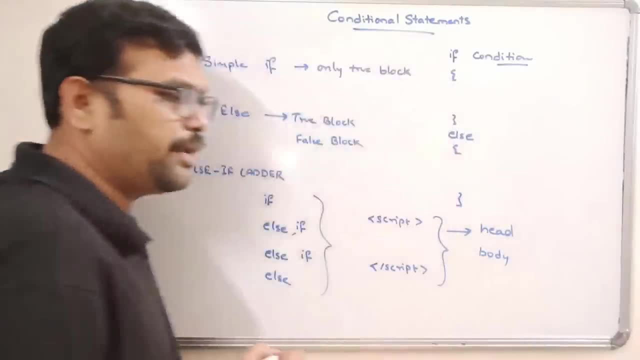 or the body, So it cannot be anywhere. In the head we can write the script, or in the body itself we can write the script. So no problem. So inside the script we have to write all these things. 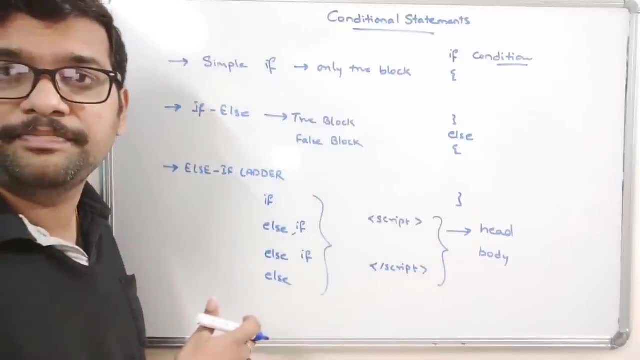 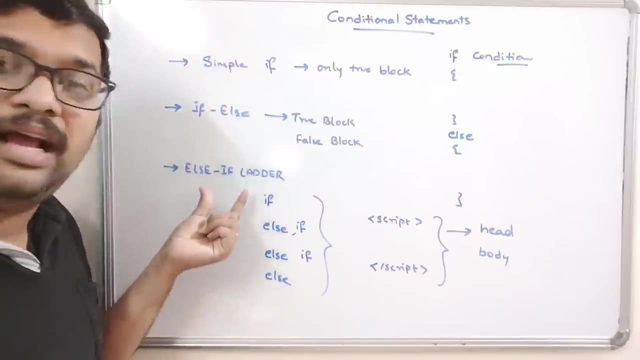 We have to implement all these things Right. So this is the basic thing, And in this session we are going to discuss about this simple if, if else and else, if ladder. So I will demonstrate all these three conditional statements by executing a small HTML code. 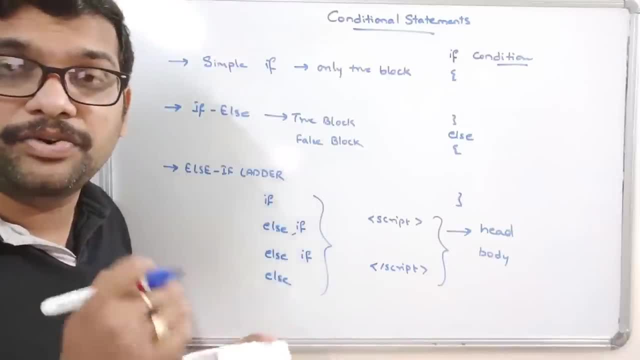 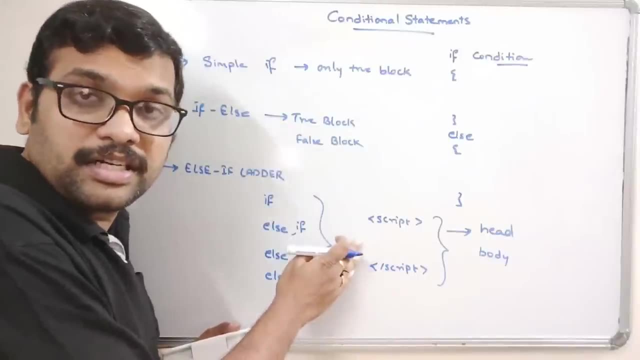 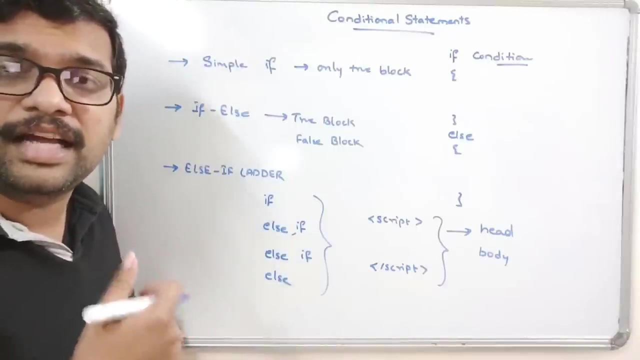 So we are going to execute a small HTML code- Okay, So we will see the script where we are writing these conditional statements, as well, as we will apply some style sheets- Okay, Some styles- to the existing tags as well as we have. we will see the output statements. 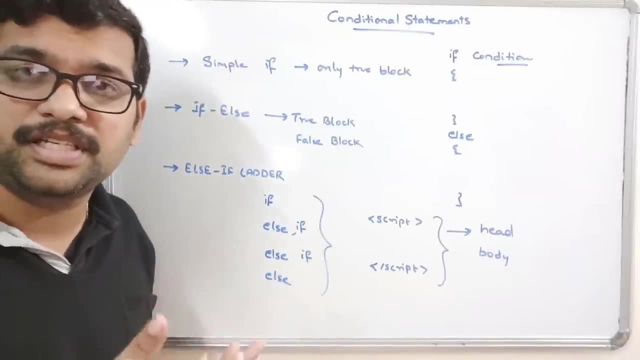 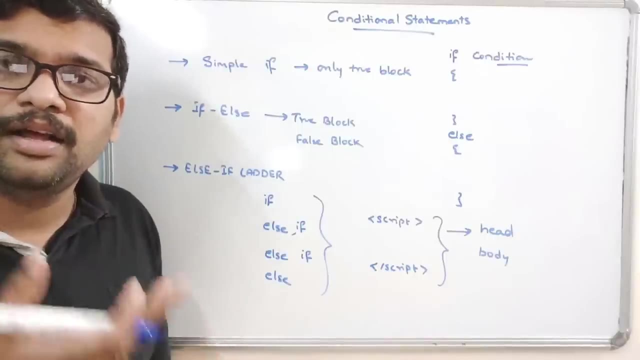 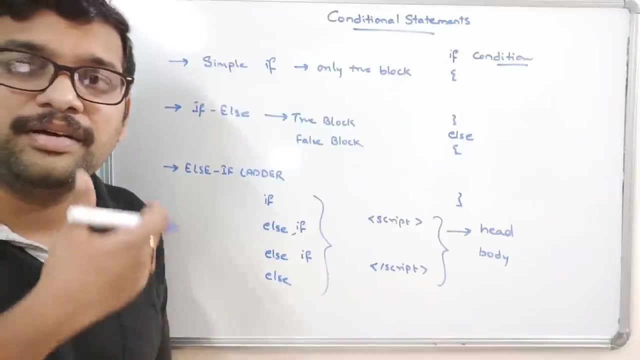 So these output statements also been covered in the previous sessions. That is three, three cases, three ways we can represent the output on the java script by using the documentwriteln or document. I mean innerHTML In the internal HTML or window dot. alert the three cases we can display the output. 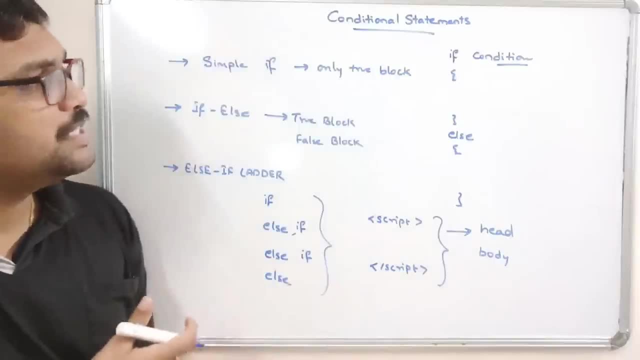 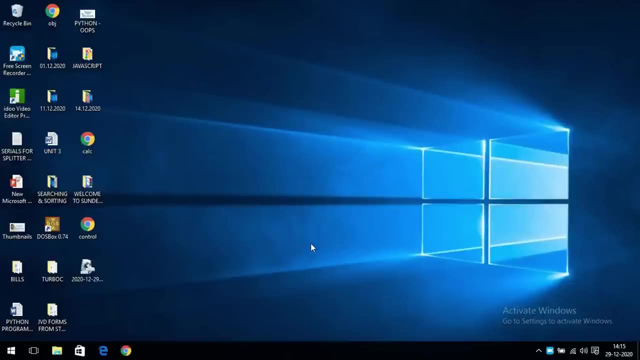 So we will use anyone among these three and we will demonstrate these conditional statements by executing a small code. So let us move on to the system. Hello friends, So just now we have seen the syntax for the conditional statements in java script. 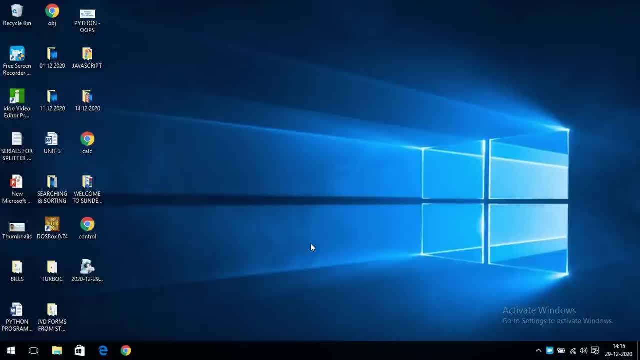 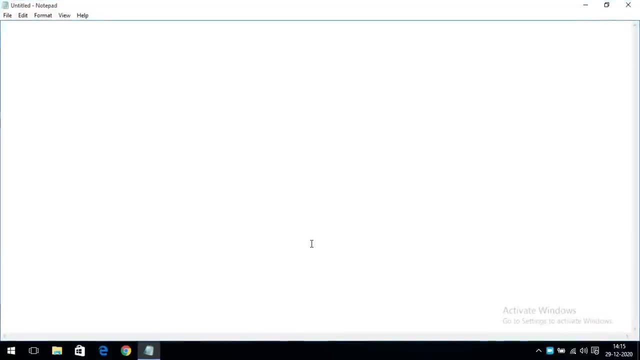 That is a simple if, if else and else, if ladder. So in order to demonstrate all these things just, we will write some code and I will explain you. So first of all, let us start this with the HTML. so in between the HTML tag, we have to: 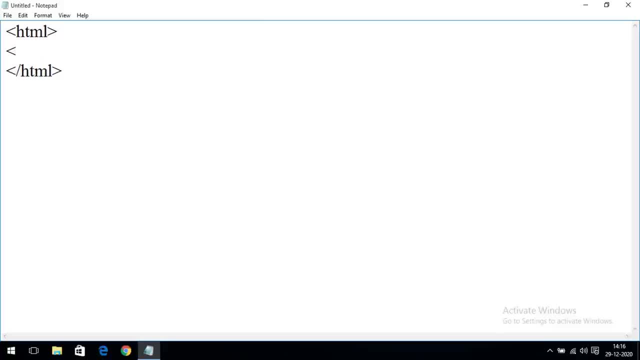 include all these things. and inside the body, first we will write one form, yeah, and here we will create one form, just we will give one text box to read the input. So for creating the text box, I am taking this one: enter age. ok, so enter the age. so 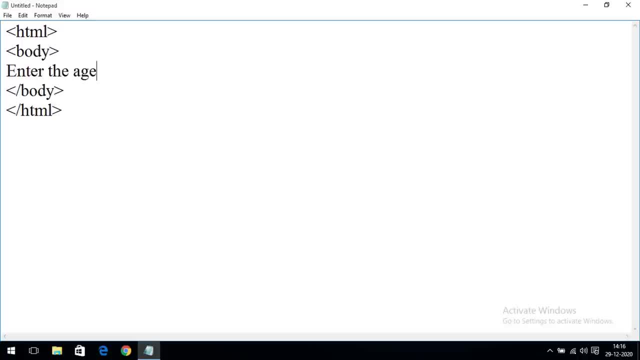 we are finding whether the person is eligible for vote or not. So here I am just giving some text box, input type is equal to text, and I am also giving some id is equal to t1.. So here I am just giving some text box, input type is equal to text, and I am also giving 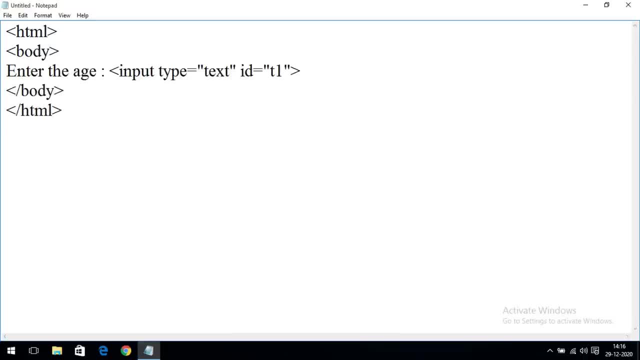 some id is equal to t1. So here I am just giving some text box, input type is equal to t1.. Then after that I am just giving some button. I am creating some button here, so button type is equal to button and here on click. 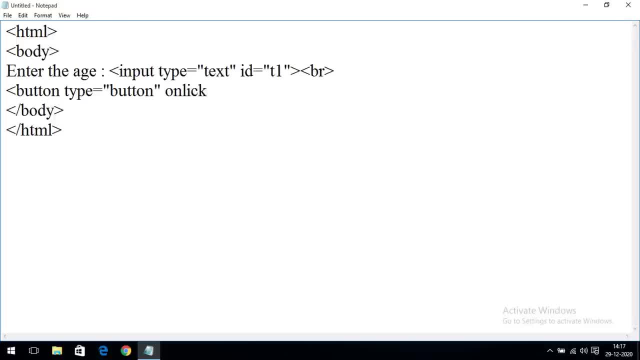 So whenever it was clicked, some trigger should be done on. click is equal to I am giving some function age, Yeah here, submit or verify. we will go with the verify. I am taking some button, I am closing the button and see. So I will save this one and we will check whether the form was created. 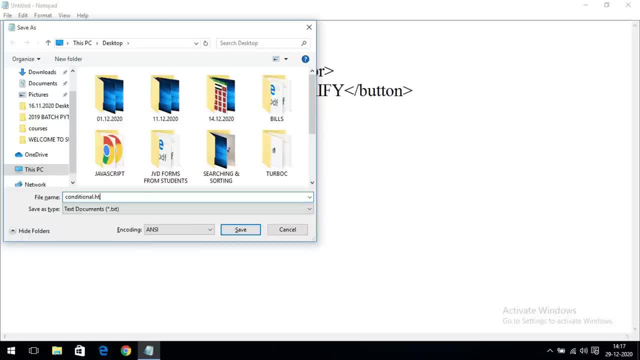 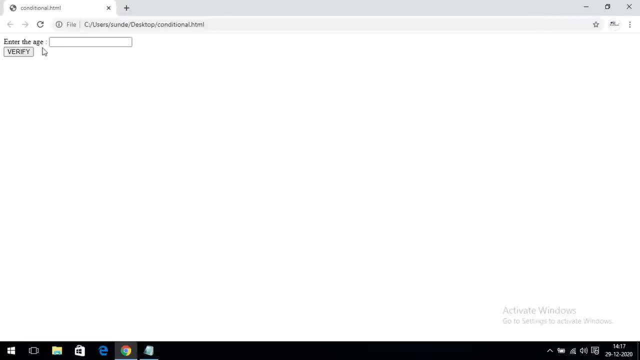 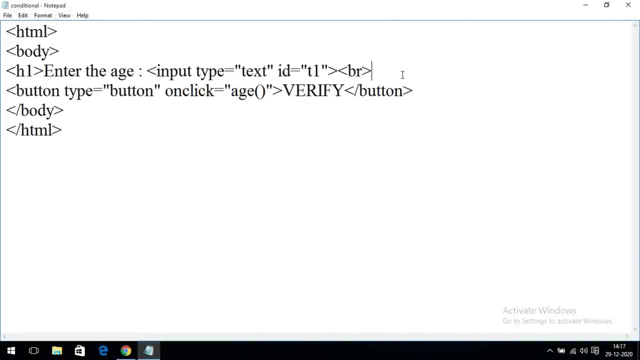 So conditionalhtml. So move with the desktop. So here you can find conditional, So you can observe here: enter the age and verify. ok, enter the age and verify and we will give some h1 because text is very small. So if you give this h1, automatically the text will. 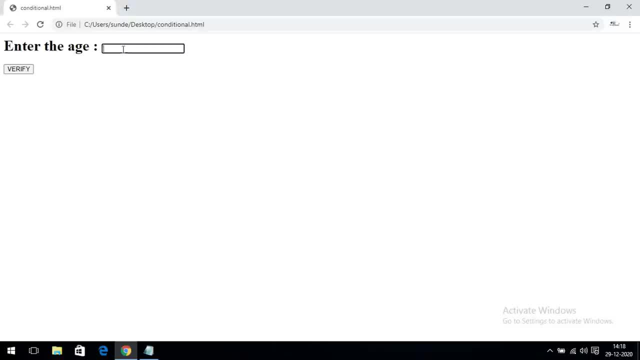 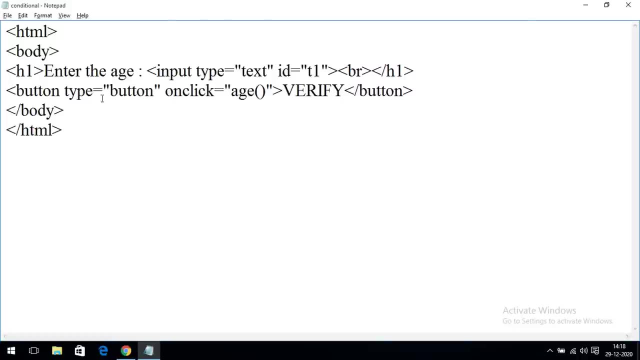 be big right. So here you are. you are supposed to give the age and we have to verify whether the age is- I mean The person is eligible for vote- or not. Now, after clicking on this age, we are giving some age function. So we have to write the function in script, because that is a JavaScript. 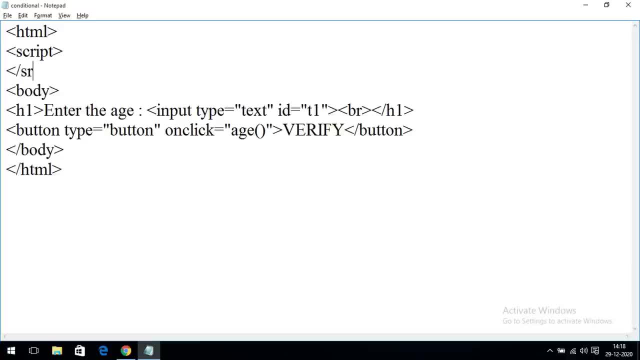 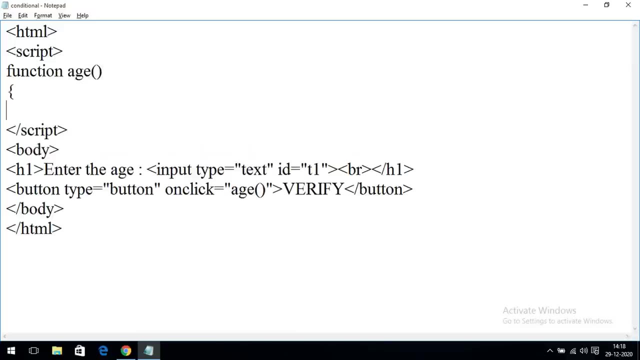 So I am just writing the thing in script tag in between the script tag. So here we have to write: So function, age. So what we have to check? We have to check whether he is eligible. that means we have to check if, if condition, So document dot get element. 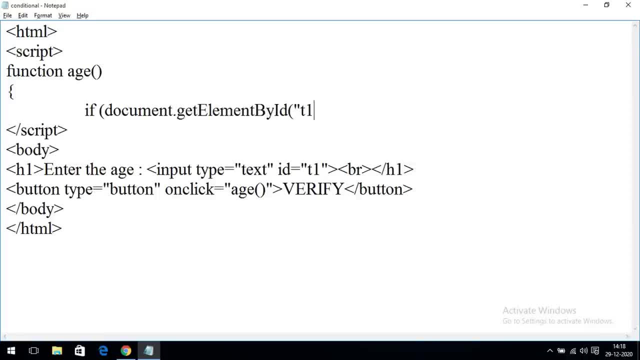 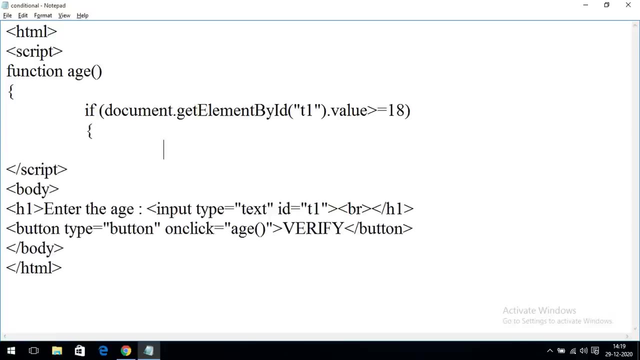 by ID of t1 dot value greater than or equal to 18.. If the value is greater than or equal to 18, obviously the person is eligible for vote. So where we have to write, we have, we have to display at some place, ok, or simply we can write some window dot alert. Window dot alert eligible for port. 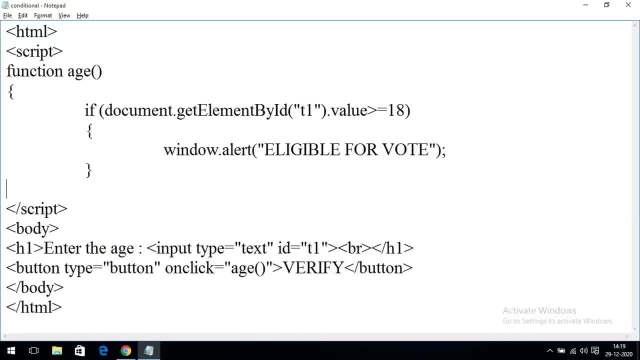 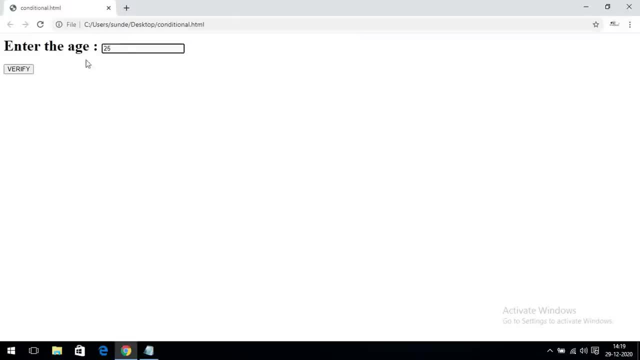 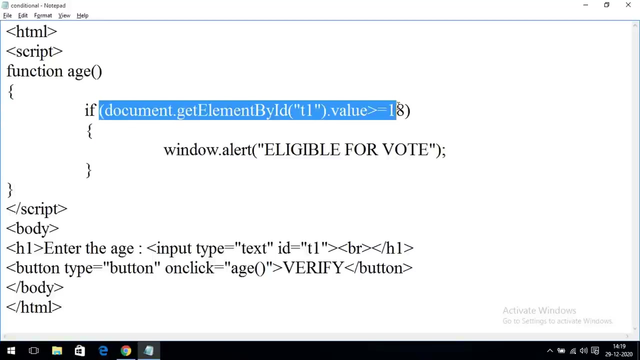 This is a small, simple if statement. simple if statement. ok. So just here, you can give some 25 and verify. we will get eligible for vote, right, If you go with some 15. if you click on verify, it does not give anything else, right, because we are writing only the true statement. 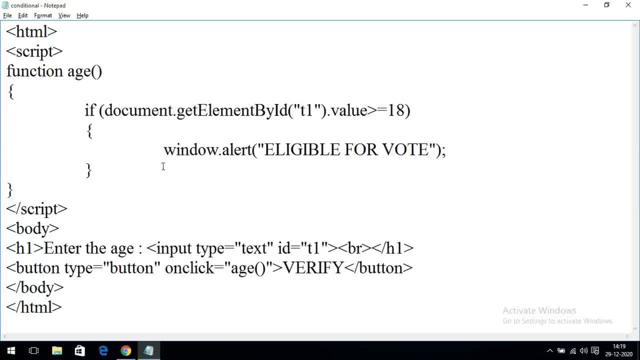 We are writing only for this true condition. If it is false, then we have to Go with the else part. ok, that is called a simple if and else. So here we can write: so: window dot alert not eligible for port Right. so this is the else part I have written. 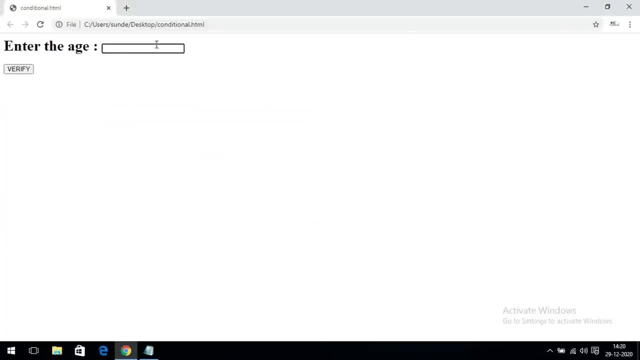 Now you can observe: we will get both the results if you press. if you give any age greater than 18, automatically we will get eligible for voting, and if you give any age below 18, we will get not eligible for voting right. So this is one way and if you want to display the same thing. 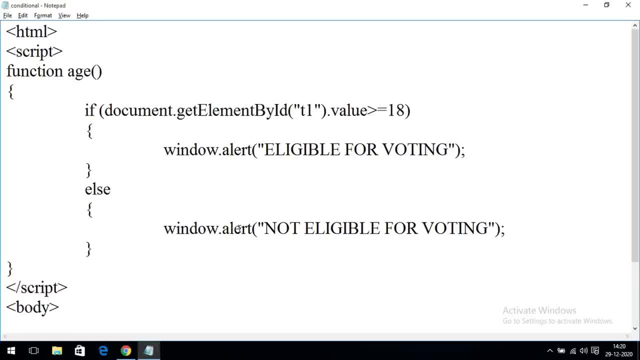 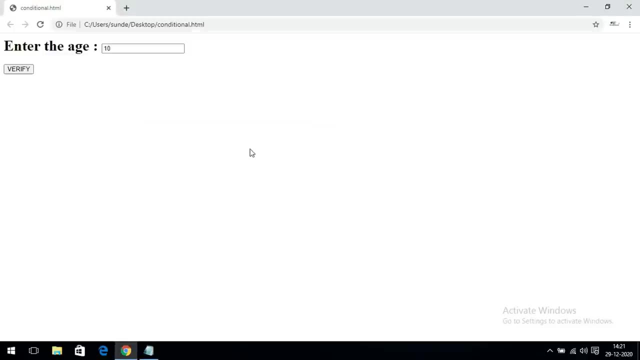 In the in the document itself, without using the window dot alert. we are having one more thing called a document dot write alarm, or we can also go with the inner html. ok, Yeah, can observe here. eligible for voting right, So otherwise we can also give some. 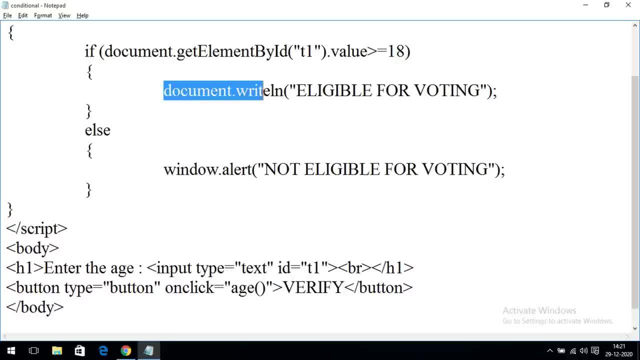 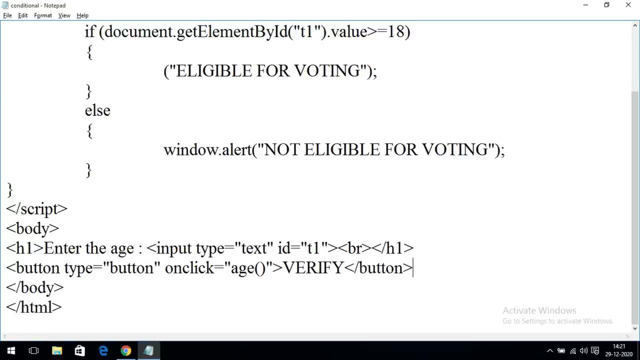 inner HTML. ok, So anyway, we can write any. we can use any output function in order to print the output. So I will go with this one, or simply we can go with the result. ok, And after clicking on the button, I will write one more thing. I will give some division. 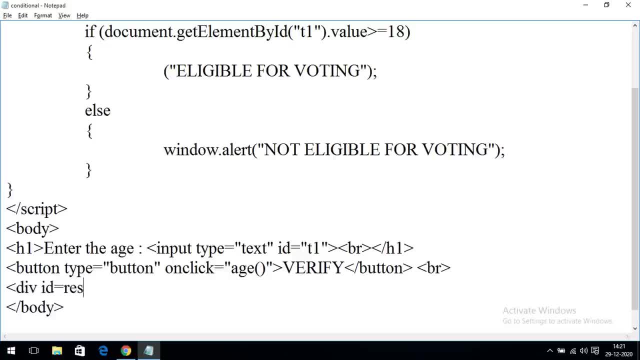 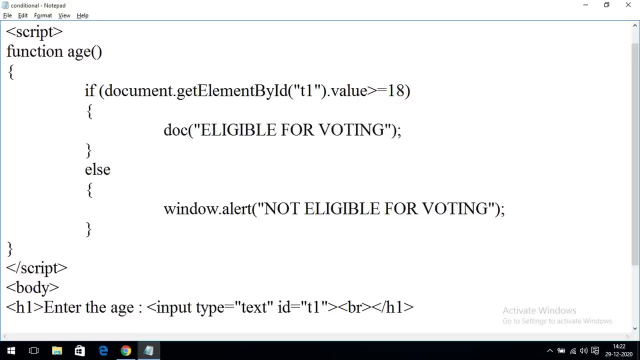 tag. give some id is equal to some result. close the division tag and here we can write. instead of writing all these things, we can write document dot. get element by id of what is the result. I think we have given some result. dot inner HTML is equal to. So you can go with this. 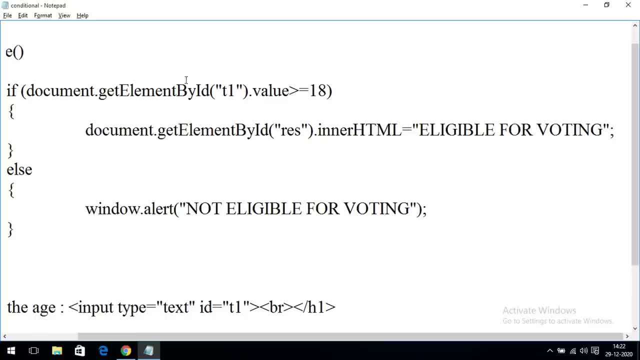 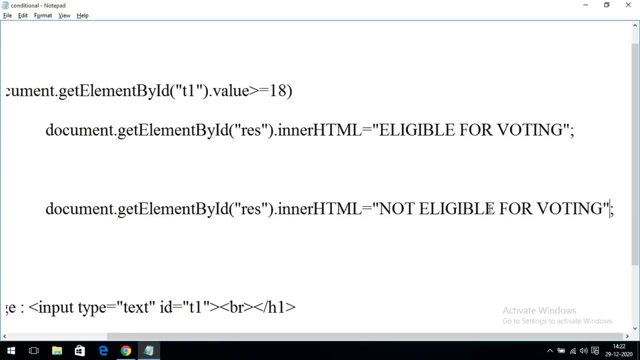 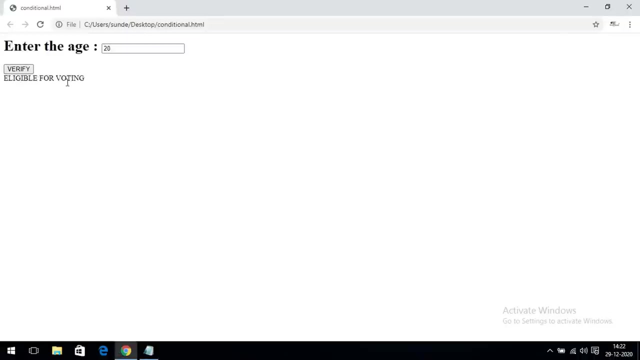 one and close the. I mean remove the this one and just copy the same thing Here also, instead of using the window dot alert, we can go with this one and remove the parentheses and you can observe here: enter the age So 20.. We will get eligible for voting in this place, in this page itself. ok, So we can use anything. 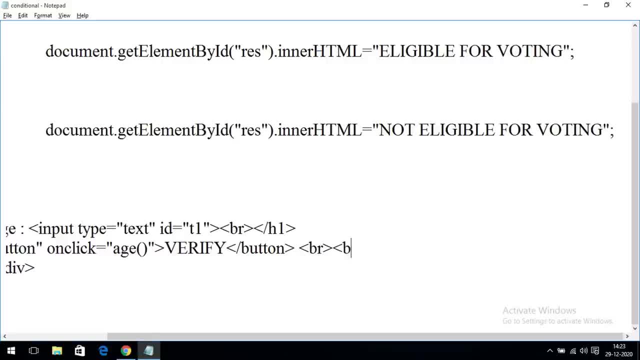 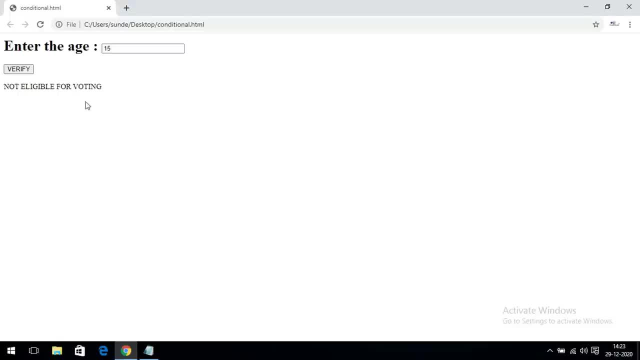 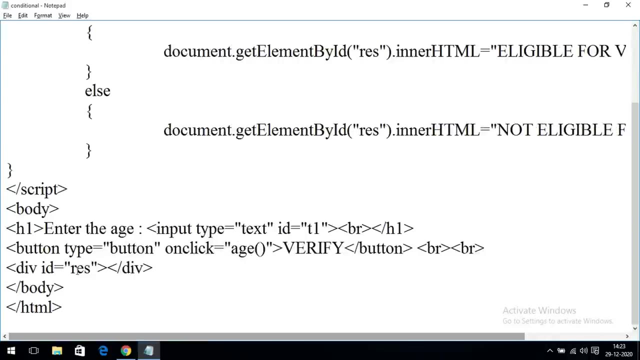 we can use anything right. See not eligible for voting. And if you want to apply the some sort of styles for this one, you can simply go with the style tag. So, inside the style, inside the this one, go with the header tag. So inside the header tag, you can go with. 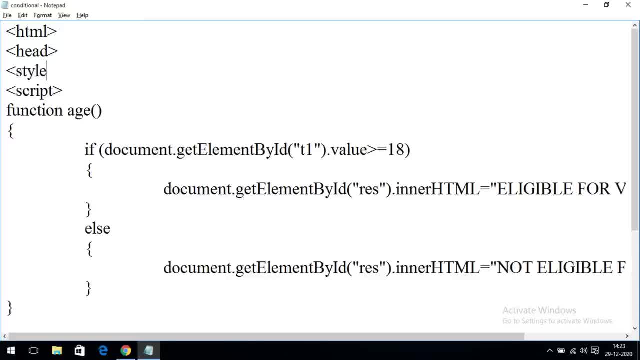 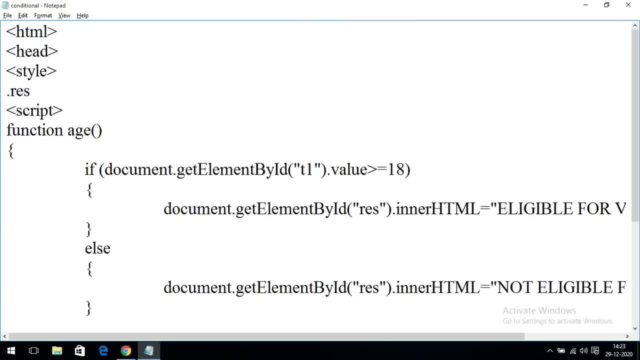 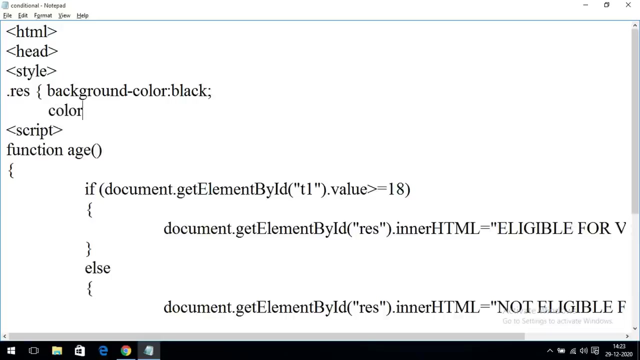 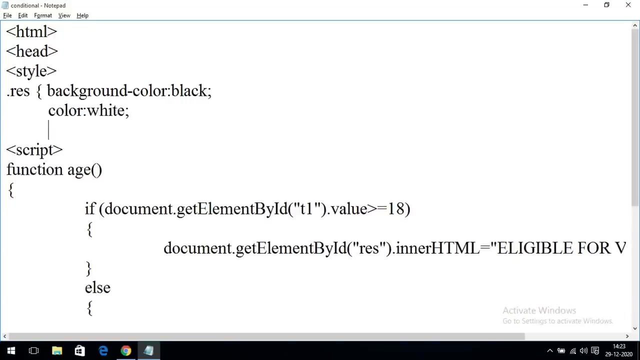 the head tag and go with the style tag and see what is the idea of this one. result So dot. result is so: background color: some black, and give some color. foreground color means font color: right, Some white, Some black, Some white And also give some width. Give some width, or else simply you can close this one and 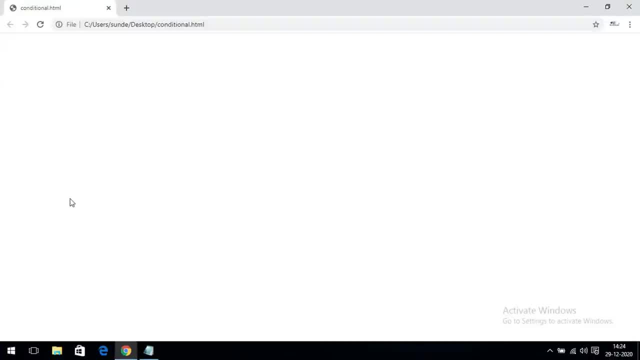 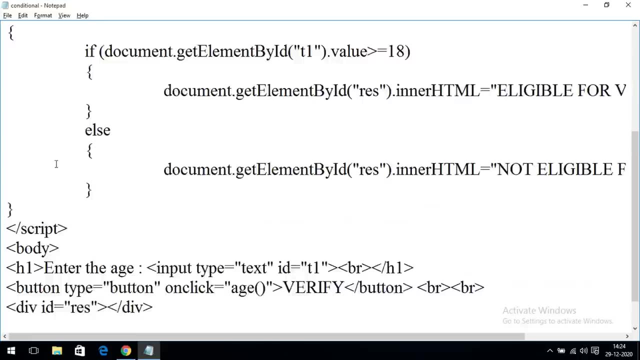 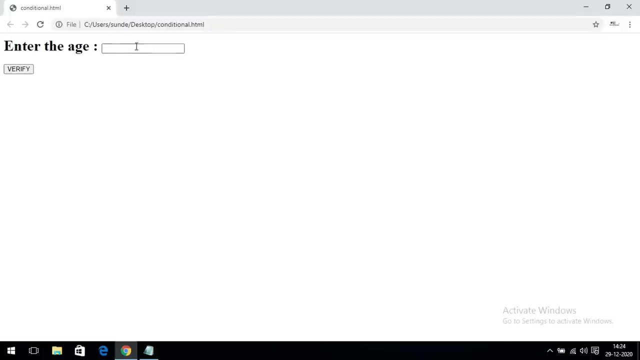 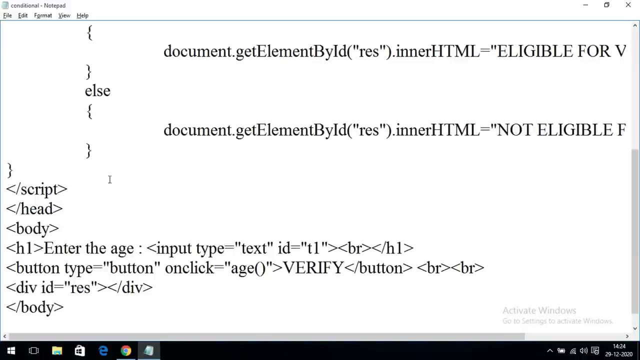 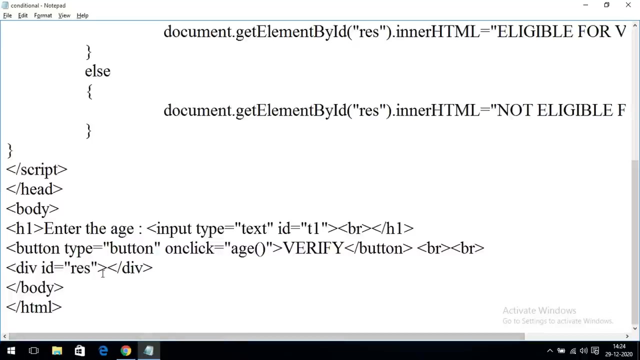 we can check over that. See, I have to close the style tag and close the head tag. ok, Now you can observe here. So if you go with the 15., We will get 15.. So not eligible for voting. yeah, Here we have to go with the hash symbol: Hash result. 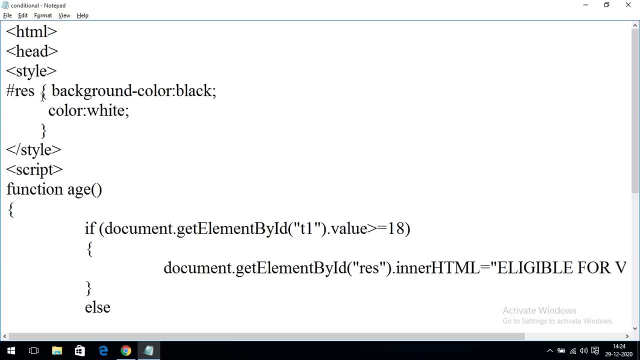 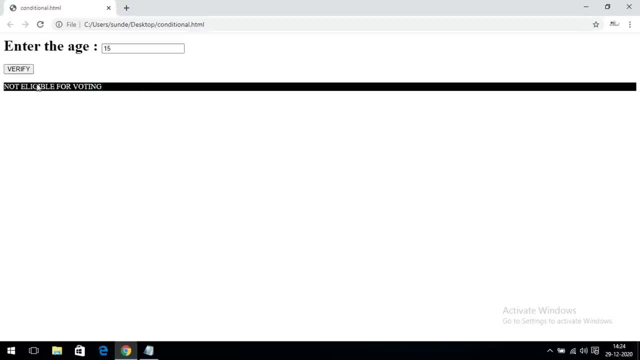 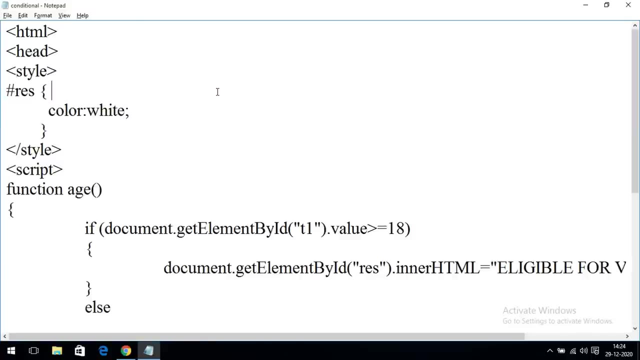 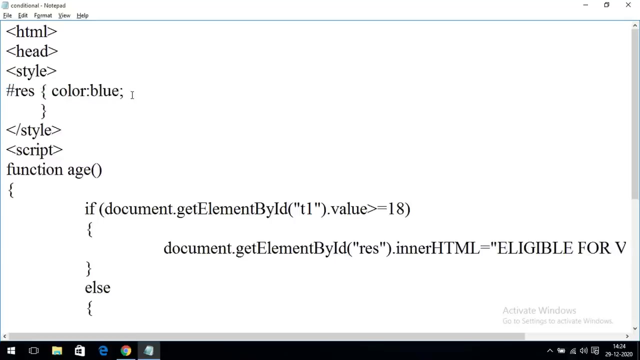 ok, because here we are using id, So we have to use the hash symbol. You can observe. So background is black and foreground is white, right? So if you, if you remove this one and remove it, it will be a very ugly color. So we have to choose a color So we can. 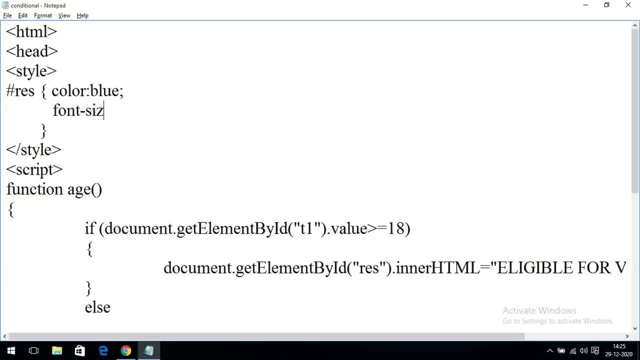 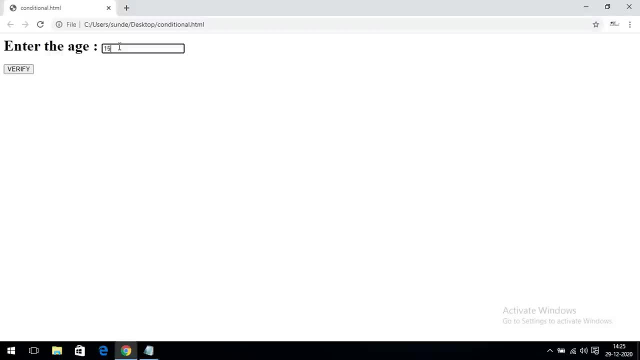 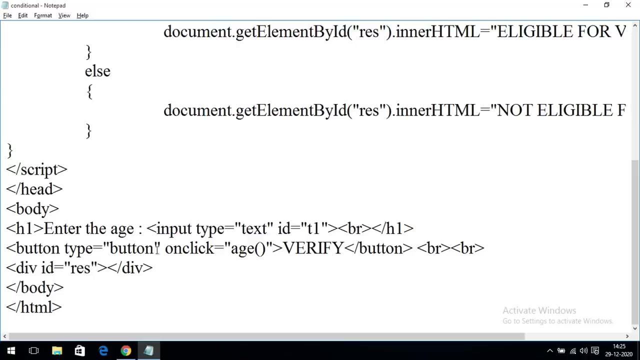 simply use the color Blue and font size: Some 10 pixels. You can check here 15, enter right 30 pixels. So you can observe here: ok, If you want color, then If you want a color here, ok. So like this we can also apply the styles. ok, we can also apply the styles for. 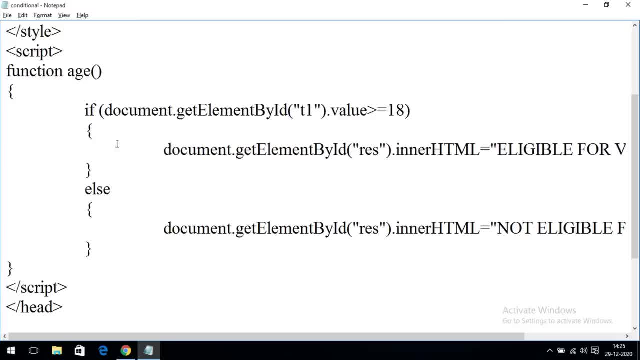 the result itself, and this is the simple if and else. So in the if block we are writing some condition and based upon the condition, it will give the result. either it may be the- I mean if it is true, the if block content will be executed, and if it is false, the else. 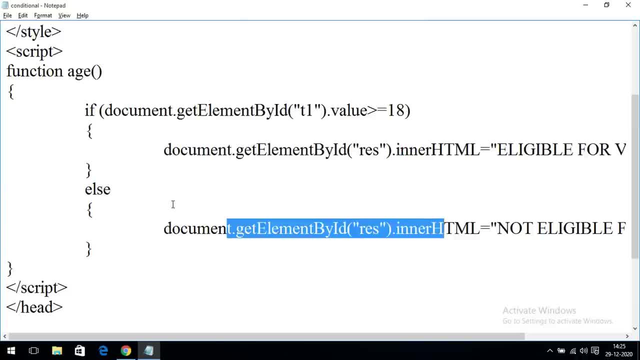 block content will be executed. And coming to the if else, if ladder that means if again, if you want to check the condition once the condition is false again, if you want to check one more condition, then we have to use the else if. So for that I will give. 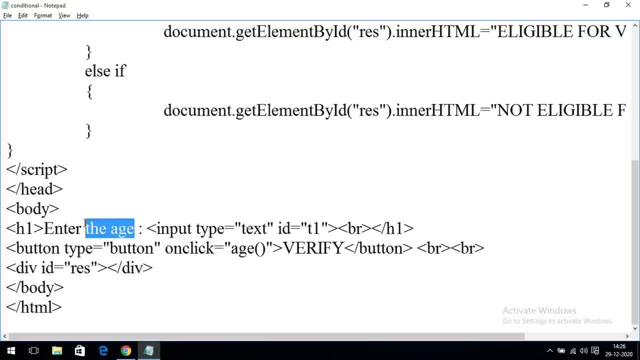 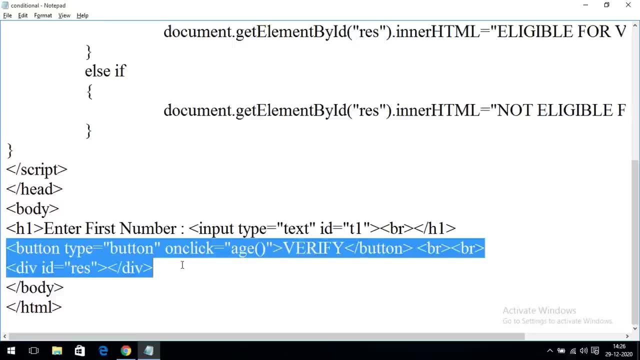 you one more thing. see, here we will write some, enter first number. and the same thing: we will write one more line, enter second number. So we are taking some two numbers and we are finding the relation between those things. ok, see, the same thing. I am not giving anything, So here I will write some relation. So here, 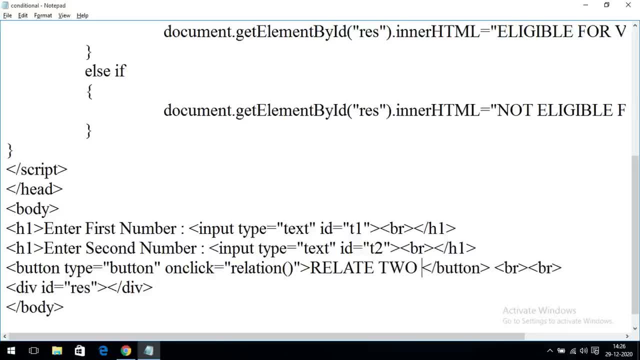 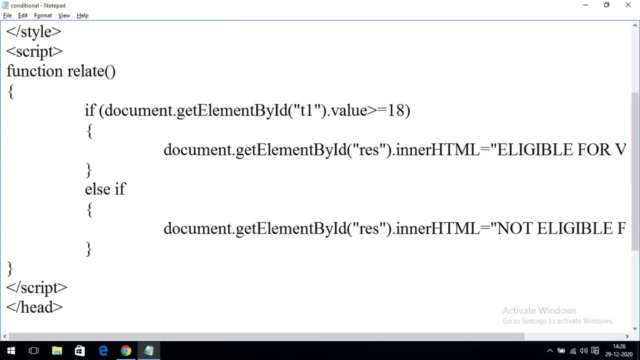 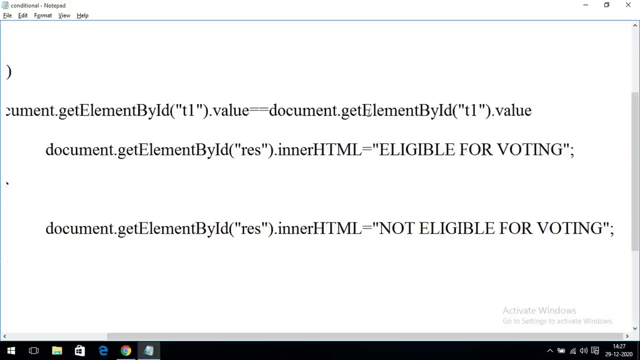 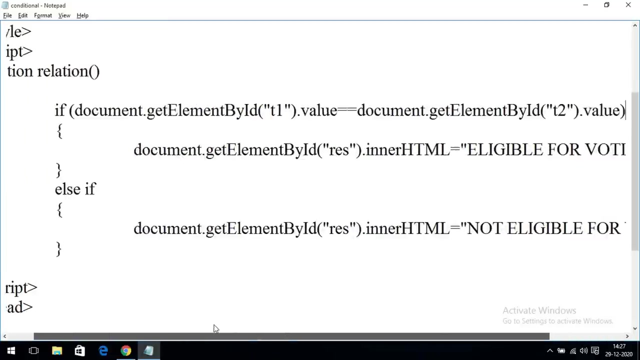 I will change. relate two numbers. relate two numbers and see I have to change the relation, This one also. So this is a relation which we have done and here write down: documentvalue: same thing if both are equal: t2.value. right, hope you understood this one. So I will decrease. 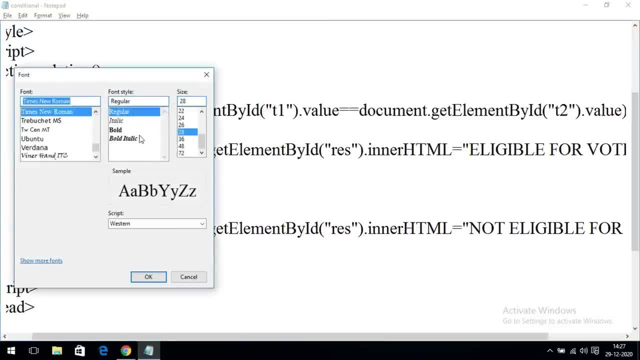 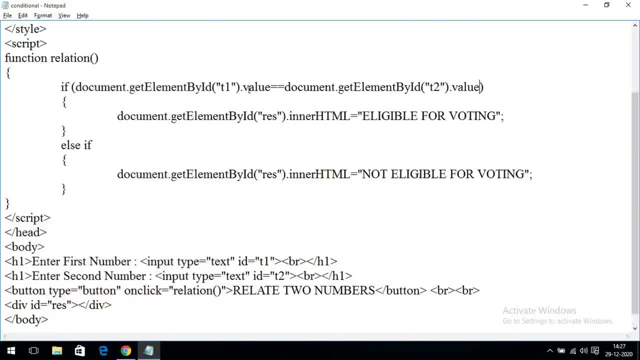 the font So that it will be readable. So I will go with 20. yeah, see, if both the values are equal, then you can write here: both are equal and else, if again, if the condition is false, and copy the same thing here. 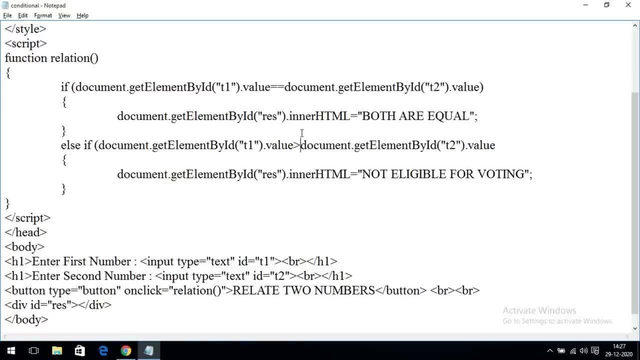 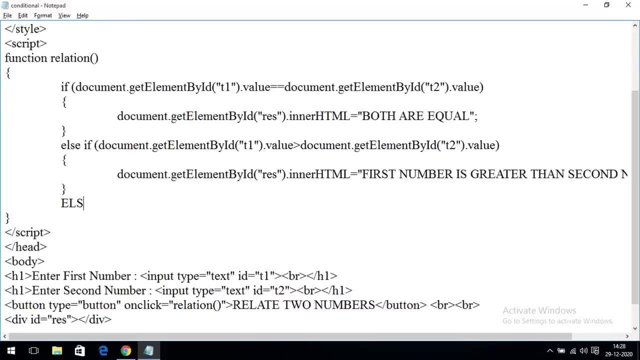 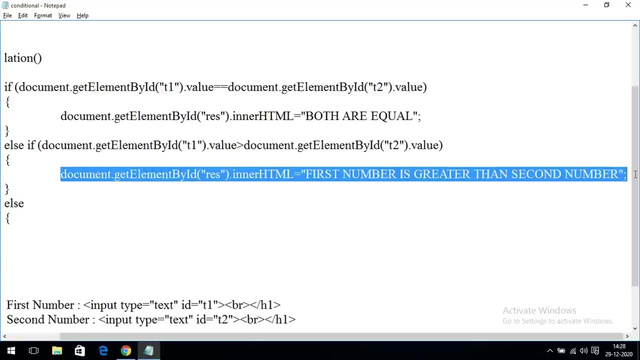 And instead of checking the greater than is equal to, we can check for the greater than greater than so. first number is greater than second number and if that condition also fail, automatically we know that The second number is greater than first number. or we can simply write: the first number is: 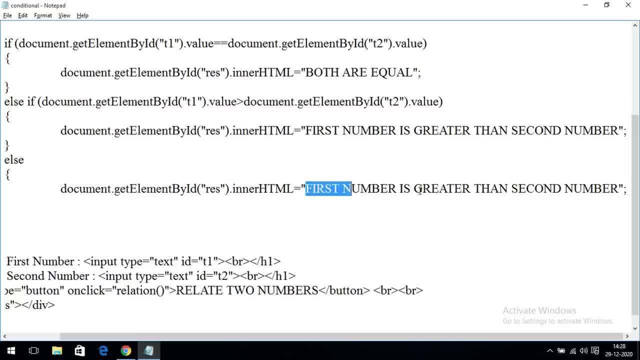 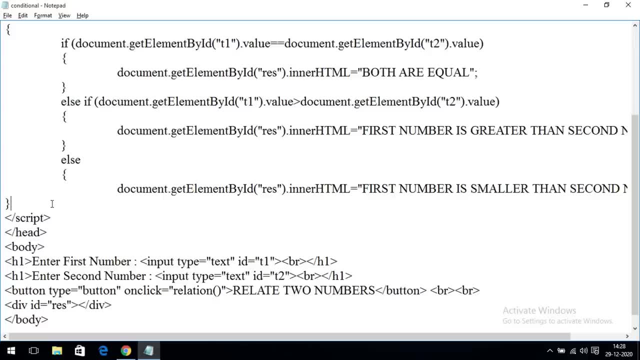 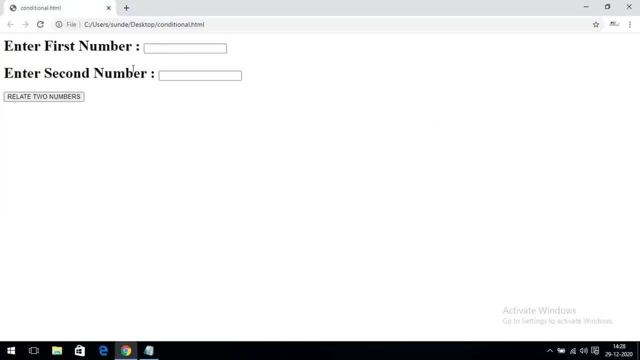 a smaller than the second number, instead of writing the greater smaller than the second number. ok, and yeah, you can observe here Now see: enter the first number. Enter the second number. first number. I will enter 10. second number: I will enter 20 and relate two numbers. 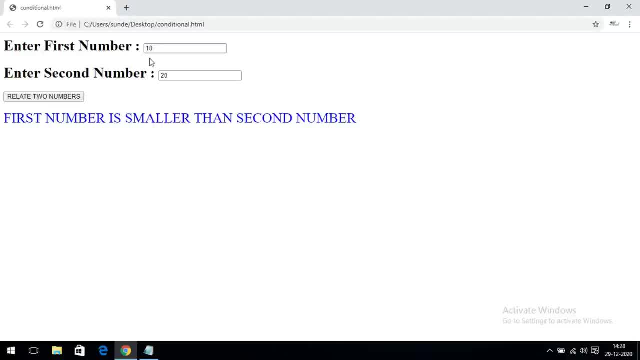 So first number is smaller than the second number. so you can observe here: 10 is smaller than 20 and you can simply go with this one. 10 relate two numbers, so first number is greater than the second number and if you give both equal, if you relate two numbers, both are equal. 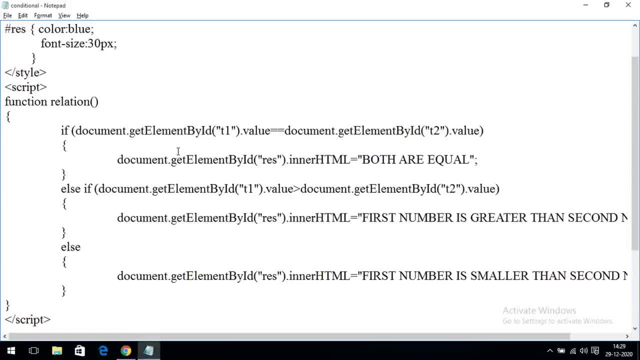 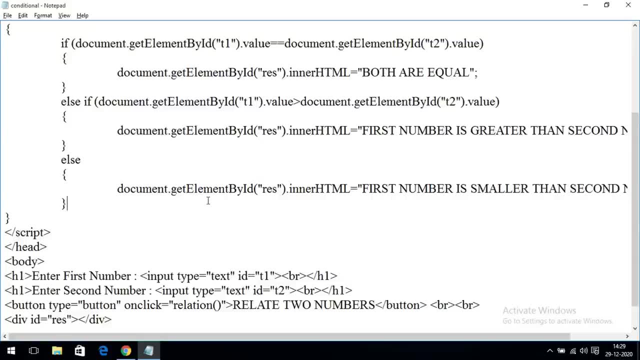 So, like that, we can use the conditional statements, We can also use the conditional statements, right? So these are the conditional statements are simple: if, if else and else, if later. So if you are only verifying the true condition, then we will go with the simple if and if. 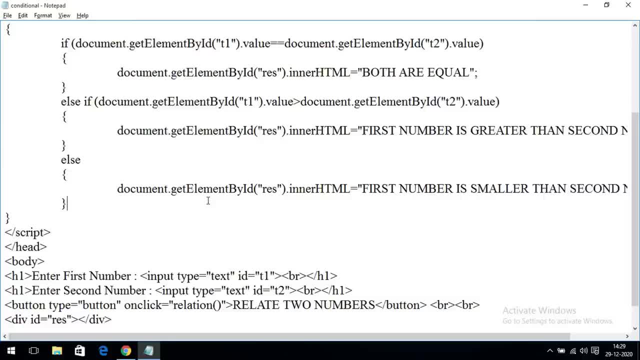 you want to display both the true condition and a false condition. I mean, if you want to display either true condition or a false condition, then you can go with the if else right. Similarly, else if later, else if later. So we should not write. 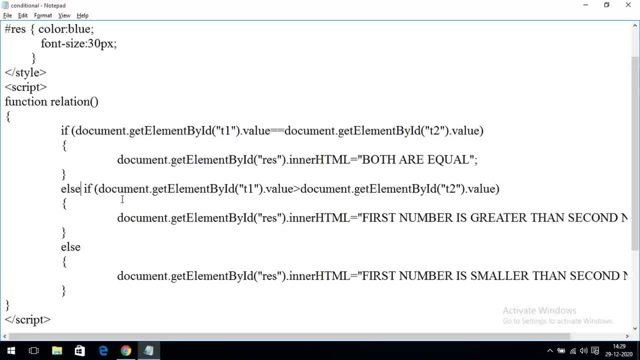 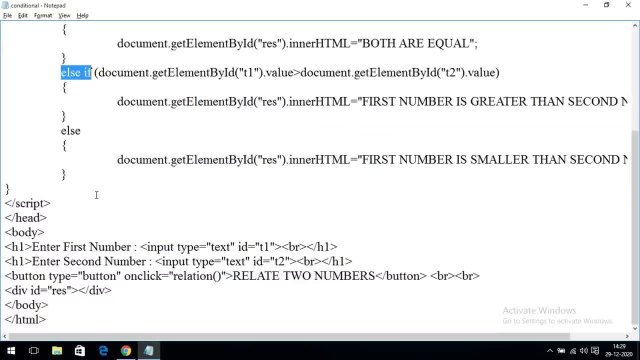 We should not write any condition at the else part. So if you want to write any condition in the else part, we have to use else. if you want to use else, if- and here we can also use the style sheets, and if you are not using the 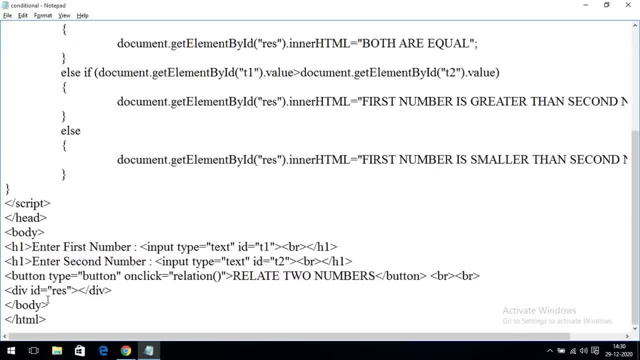 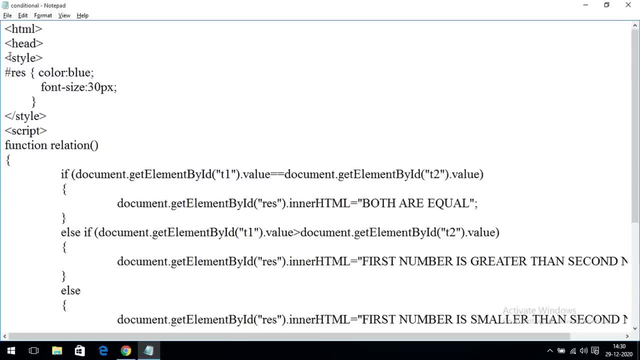 styles normal, it will print it normal. So, based upon the id or class we have to use the style sheets. If you are using some id, we have to use hash symbol and if you are using some class, we have to use dot symbol, dot symbol, and this styles should be written in between the styles. 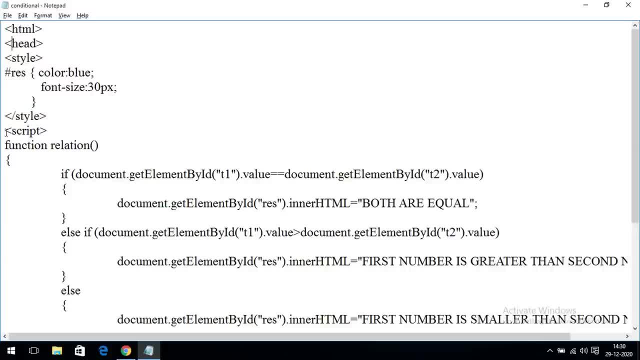 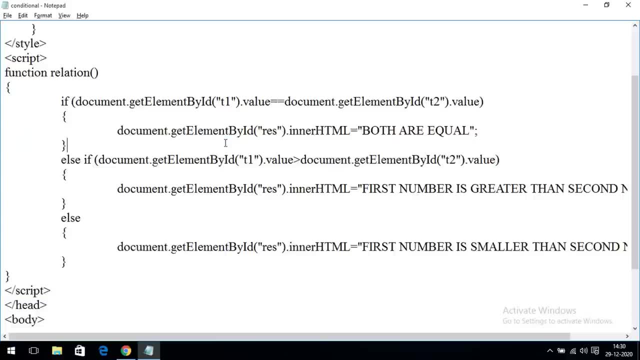 style tag and that should be included in head, and this script tag should be included in either head or body, So which we have discussed earlier, and we can display the output by using one among the three output functions which we have discussed earlier, that is, inner innerHTML document dot. 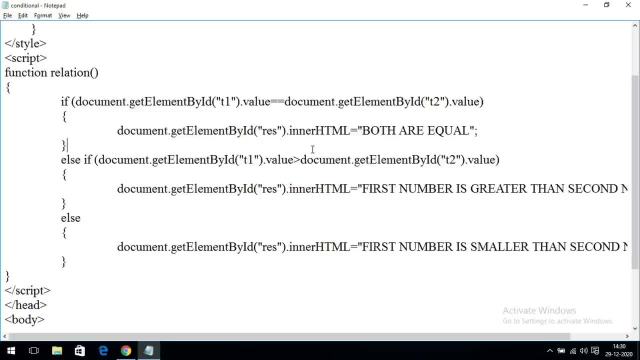 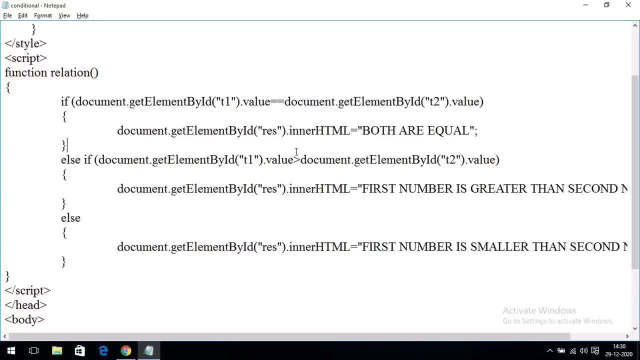 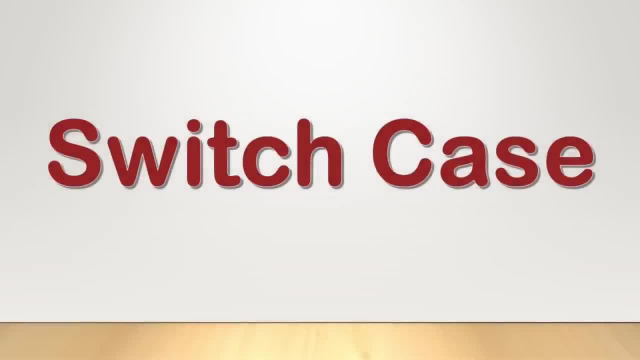 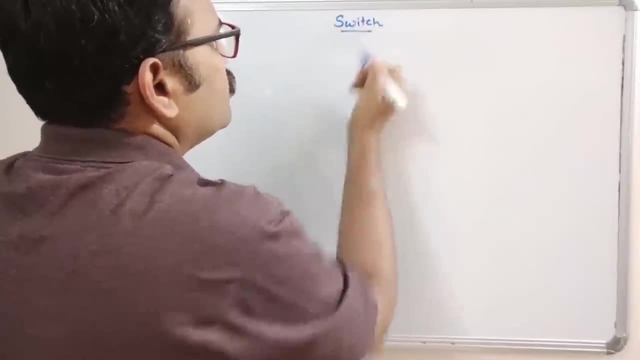 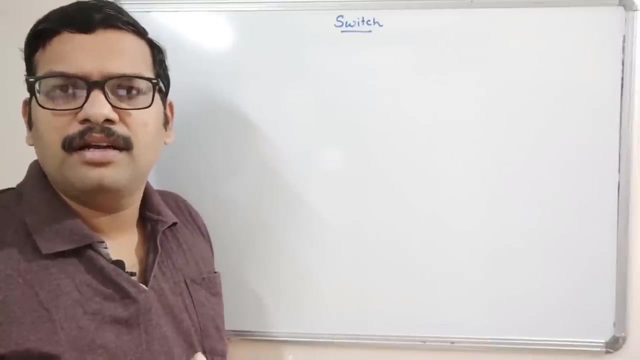 I mean window dot alert so we can go with the alert boxes, right. So hope you understood this. conditional statements. So in the previous sessions we are we have discussed about the conditional statements: if condition, if else else, if letter, and all these things. 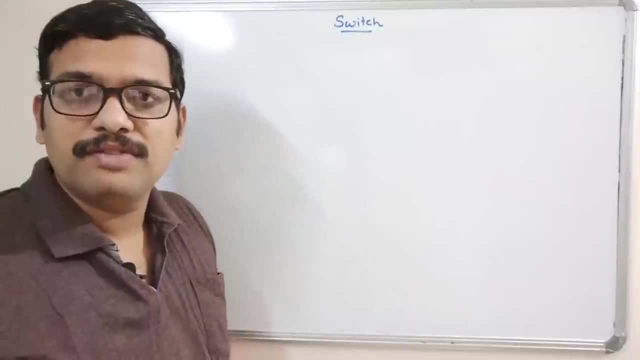 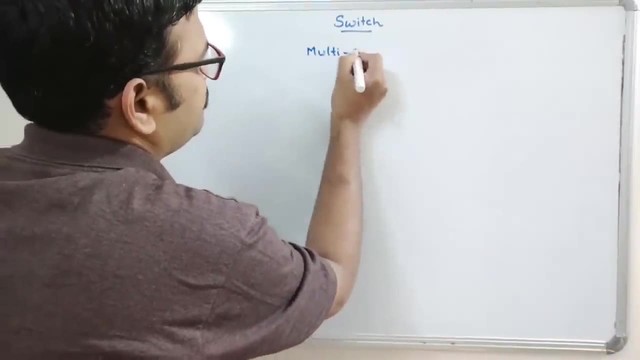 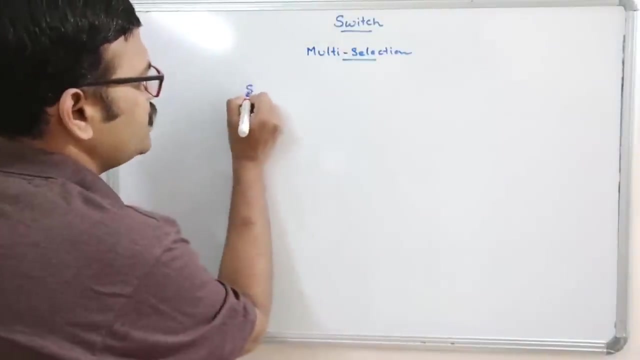 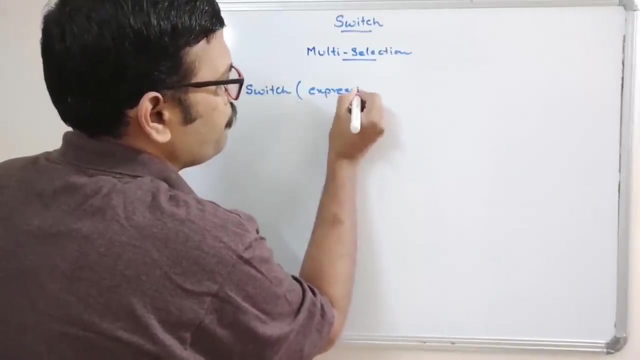 And here in this session we will just go with this switch case. that means multiple selection statement, multi selection statement, it is a multi selection statement. So here the syntax for this switch is: switch, the keyword switch, followed by the expression or a value And based upon the expression and a value. 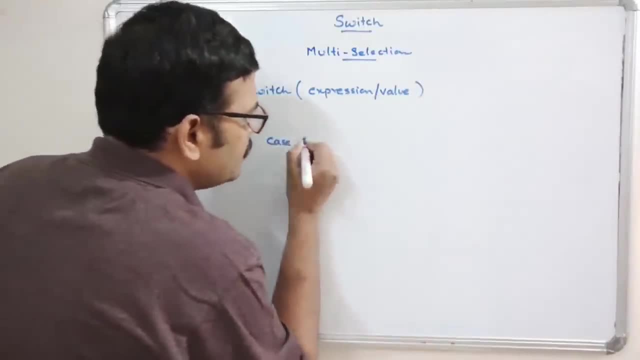 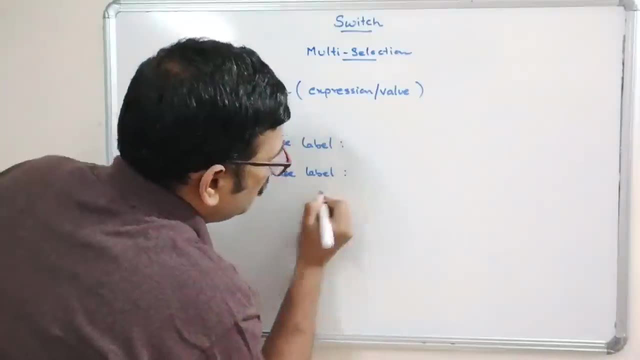 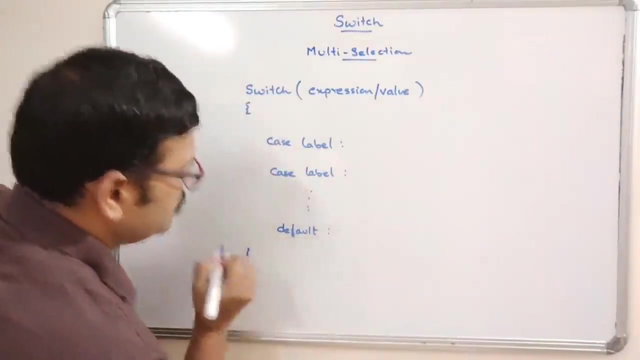 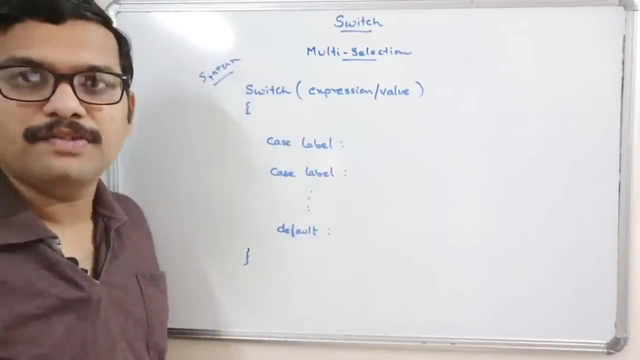 We have to write some case label colon, case label colon, and so on, default, ok and close. So this is a syntax for the switch. This is a syntax for switch statement. So here, based upon the result of this expression or the value, 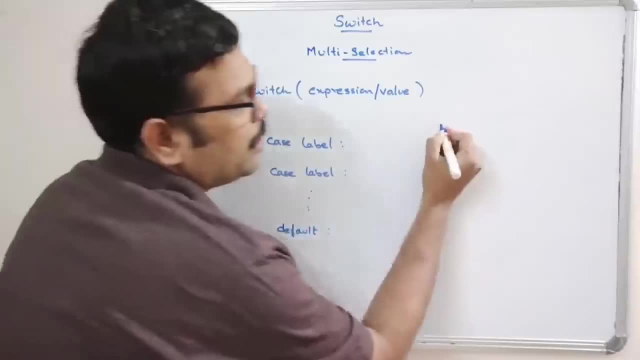 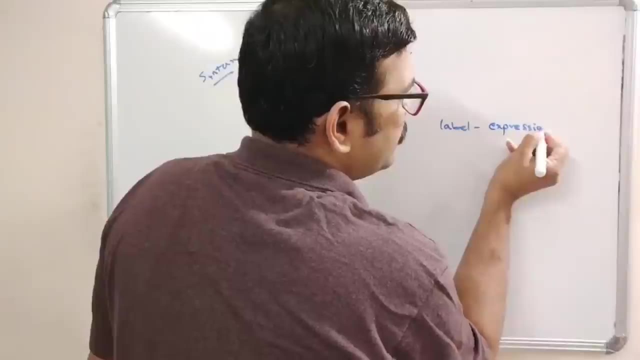 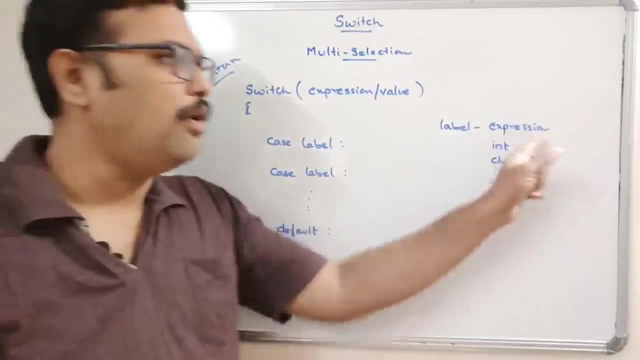 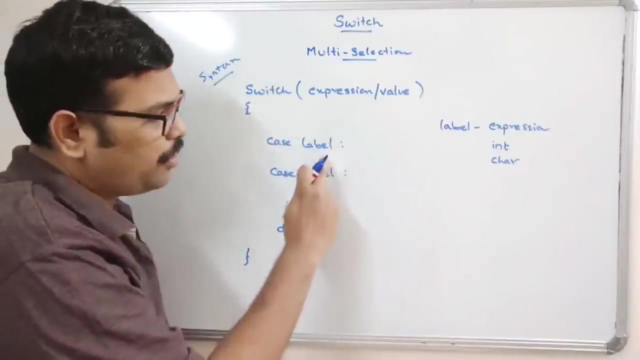 It will search for the labels. So here a label can be a label can be an expression or integer or a character. ok, an expression or integer or a character. So first the value will be compared with all these labels, So we can write n number of cases. 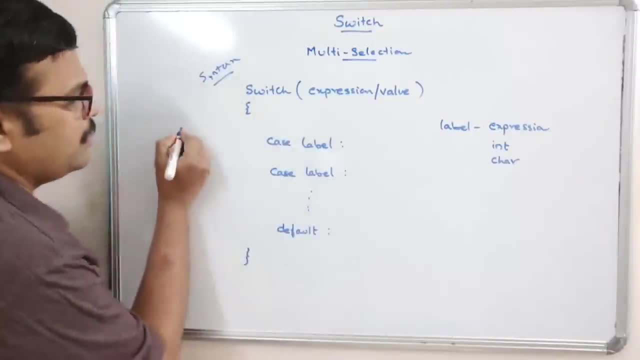 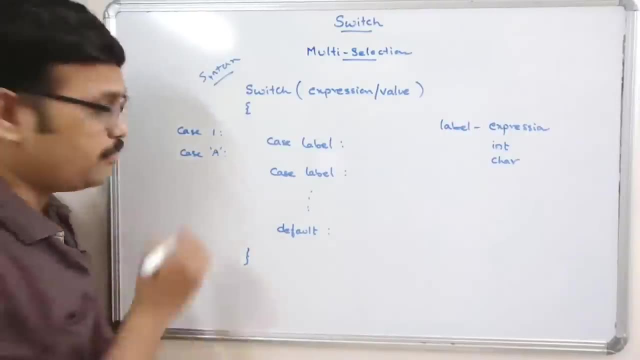 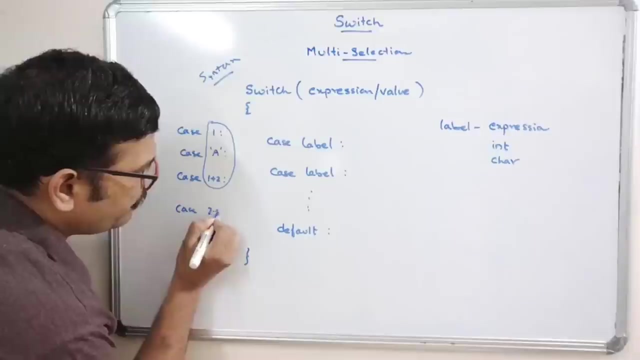 We can write n number of cases, right. So like case 1 or case a. ok, like this we can also give similarly case 1 plus 2. So this is an expression. ok, So like this: a labels can be either expression or integer or a character, and case 2.5. 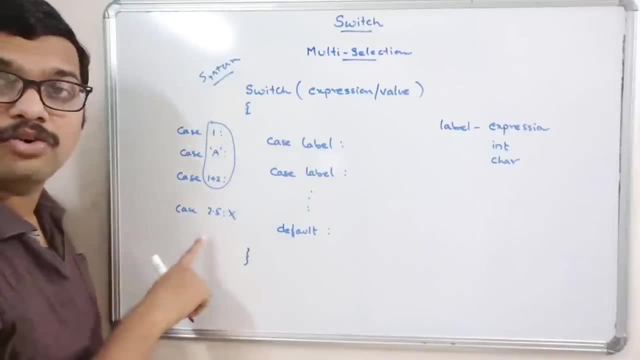 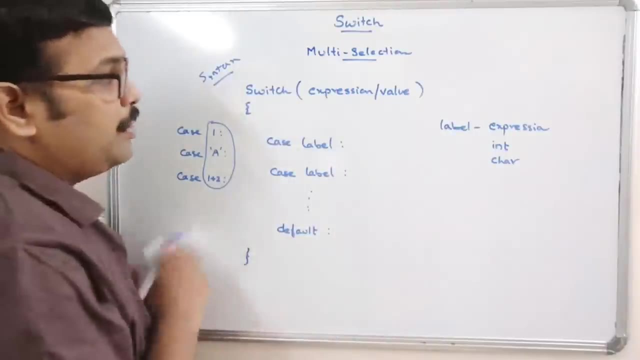 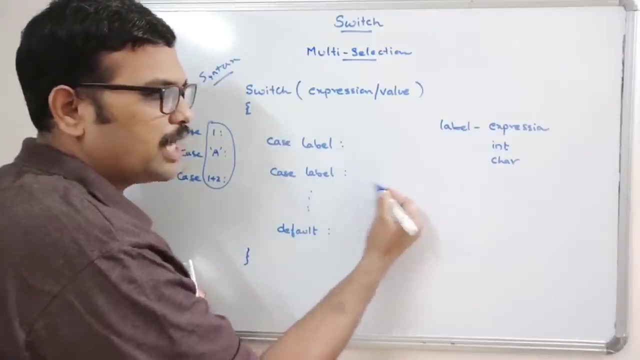 This is not valid. ok, This is not valid because it is a float, So only integer value should be here. So based upon the value first, it will check for this case labels. So if there is a match, the corresponding values, the corresponding statements will be. 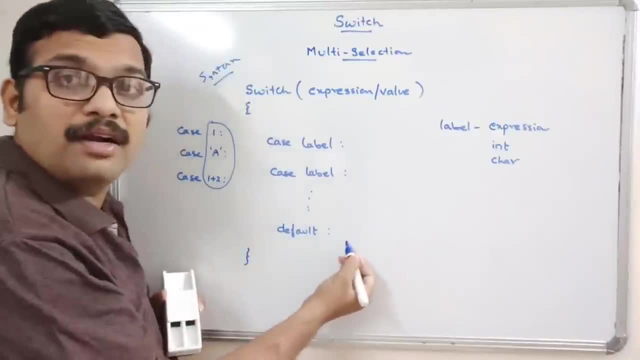 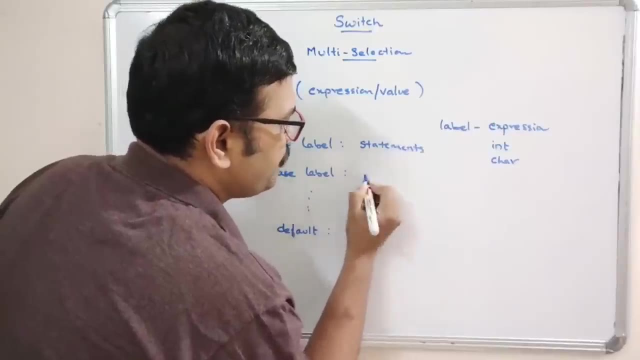 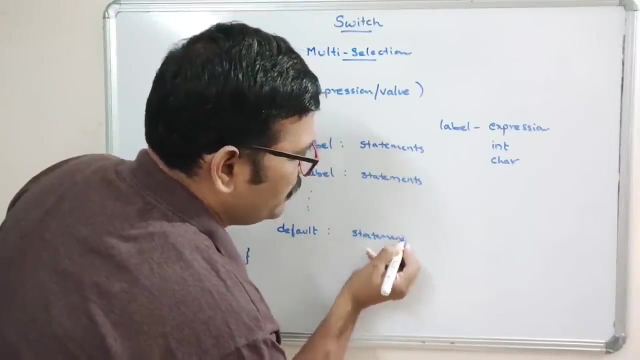 executed. If does not matches, then the default block will be executed. So here we have to write the statements. So here we have to write the statements. So in each case we have to write the statements Including the default case. ok, 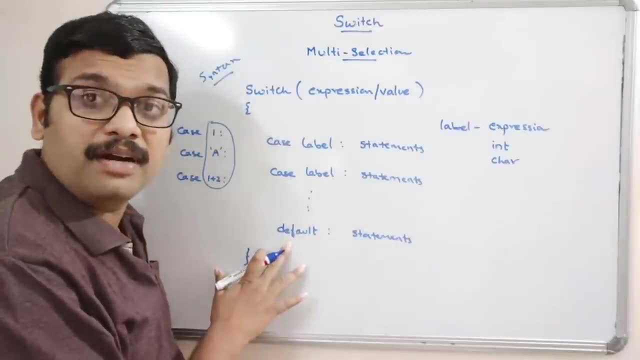 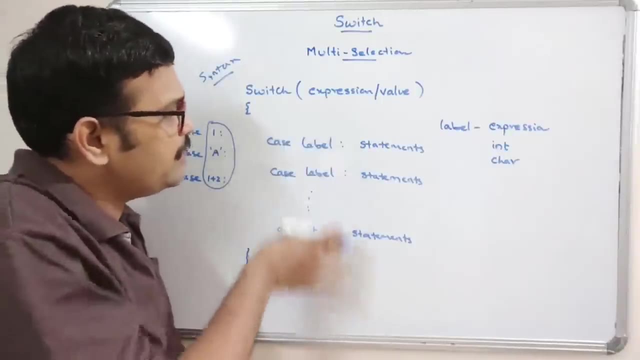 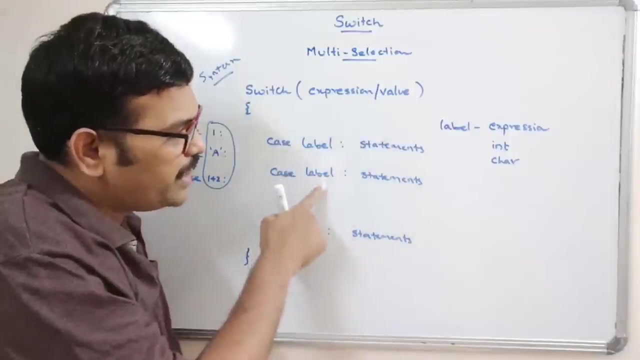 And there is a no restrictions where we have to place the default. So we can write this default statement in the first one right, So we can start writing the statements with the default also. ok, So default is a keyword, so that if the value does not matches with any one of the label, then only the default will be executed. 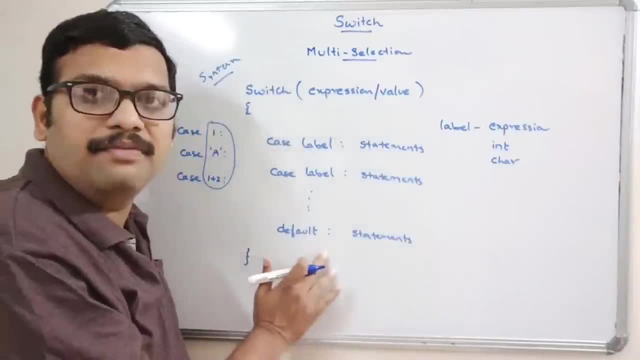 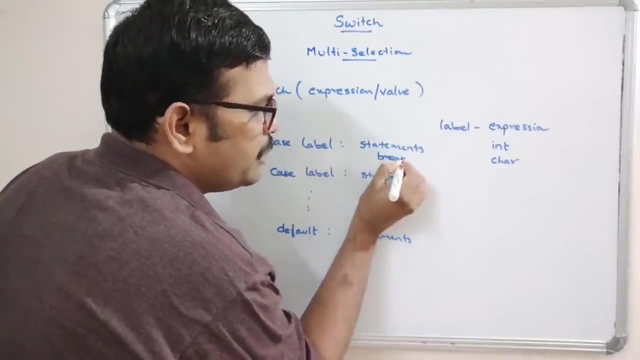 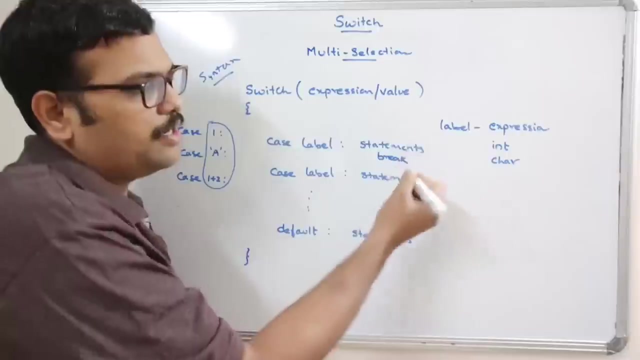 So anywhere in the switch we can write the default ok, And see, and here we will write some break statement in order to break the control, ok, So whenever the statements- I mean whenever the control- executes this break statement, immediately the control will come out from the switch case. ok. 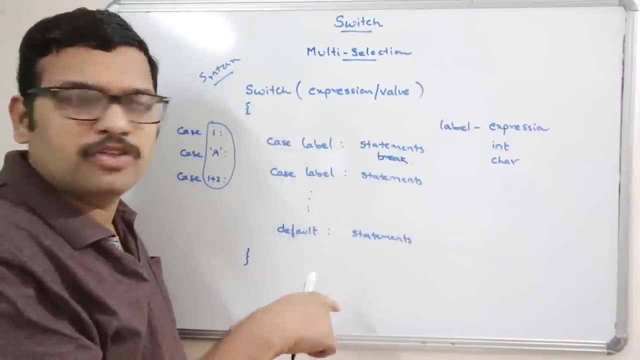 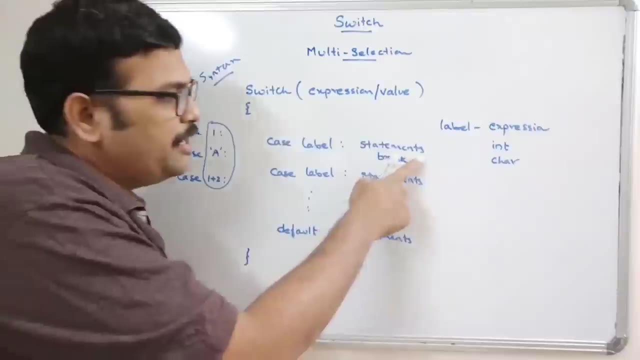 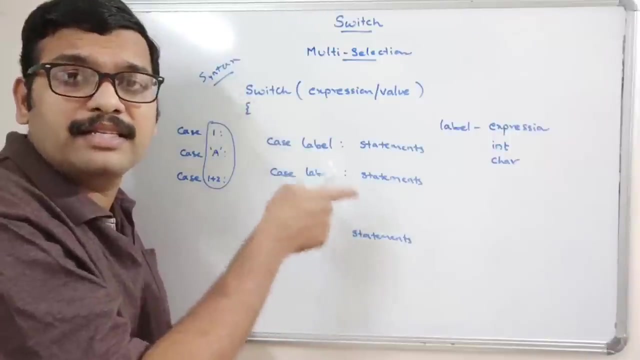 So it does not execute the remaining case labels. So that is why we will use the break. That means only one case label will be executed if you write the break. If you are not giving the break, If you are not giving any break statement, it will start continuing executing each and every case label until it reaches the break or it reaches the exit of the switch. 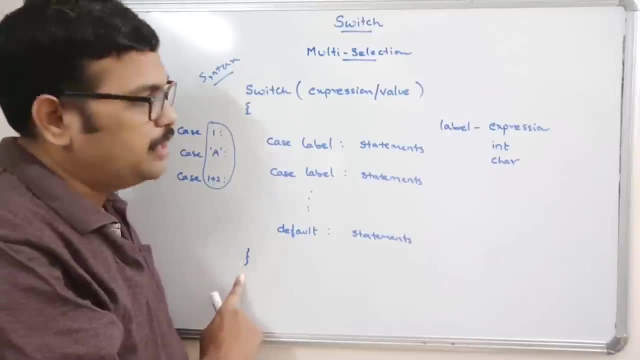 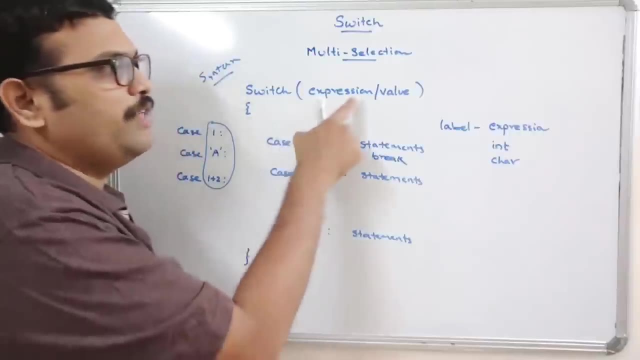 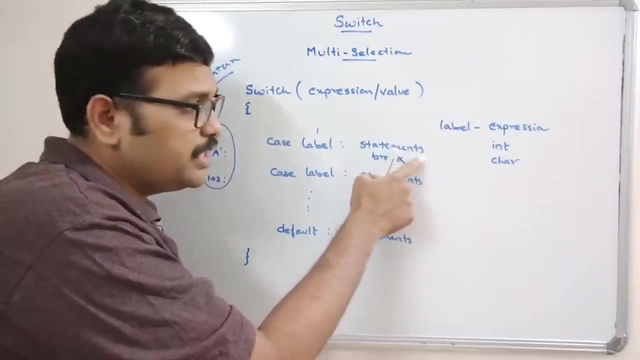 So hope you have understood. So if you are writing here break, then if so, let it be case 1.. So if the expression value is 1. So it matches with this case. So these statements will be executed immediately after executing these statements: break. 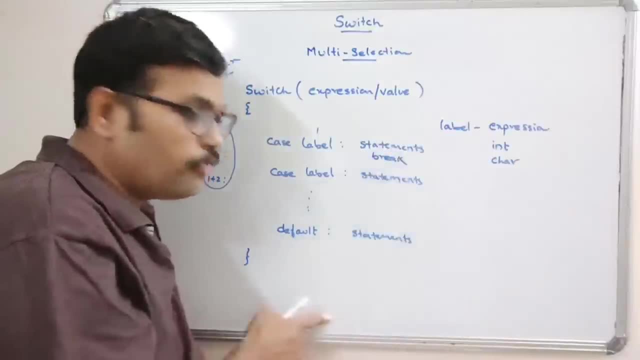 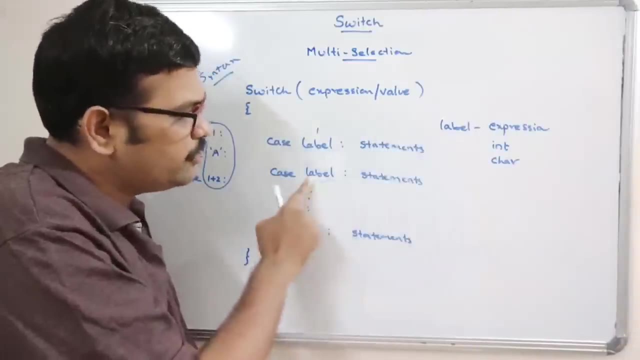 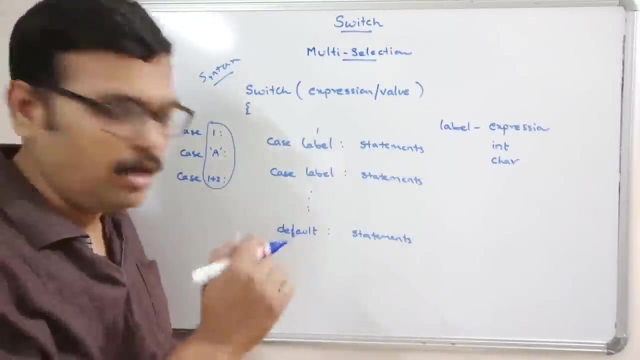 Whenever the control executes the break Automatically, the control will come out from the switch case. In the absence of this break, it will execute the statements immediately. It will again execute the second case label statements. So it will continue executing all the statements until it reaches the break statement or the exit of the switch. ok. 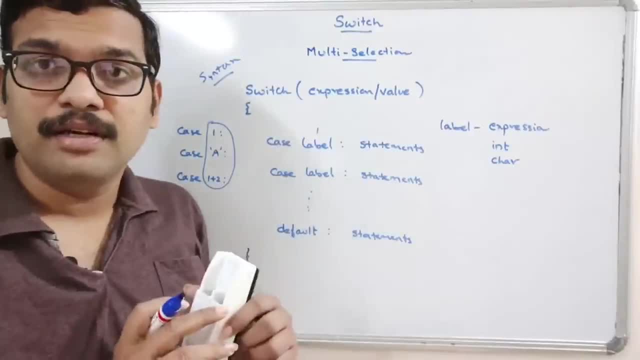 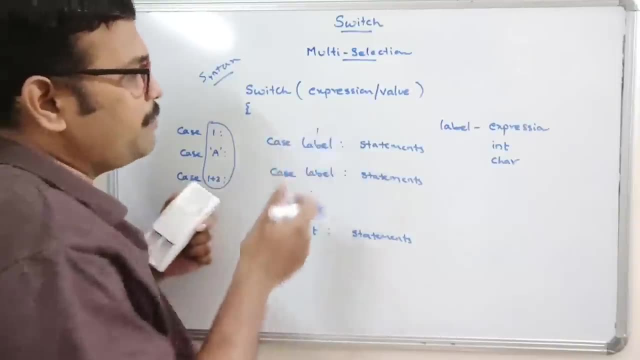 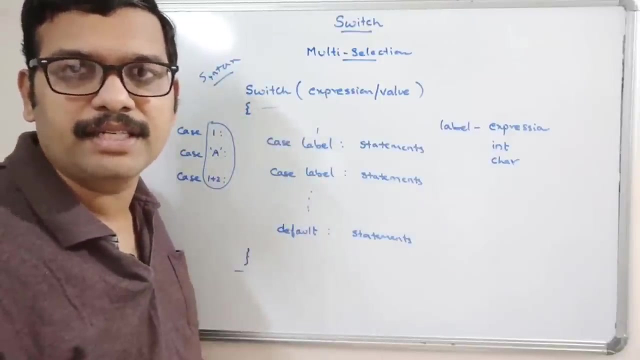 So this is the syntax for switch. So we can execute a single case or multiple cases. So if our program needs a break, If our program need to check the multiple selections, then we can go with the switch case. Then we can go with the switch case. 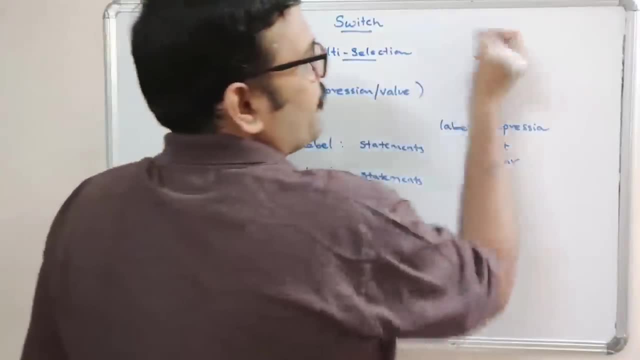 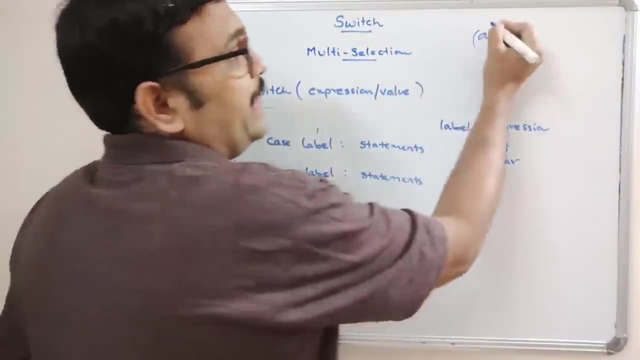 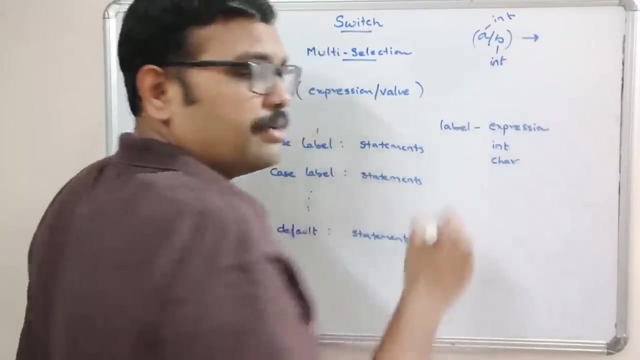 And here also the expression and a value. So here for example, a by b is an expression given in this switch case. So here if a is an integer and b is an integer in other programming languages, So that means mainly in C programming. 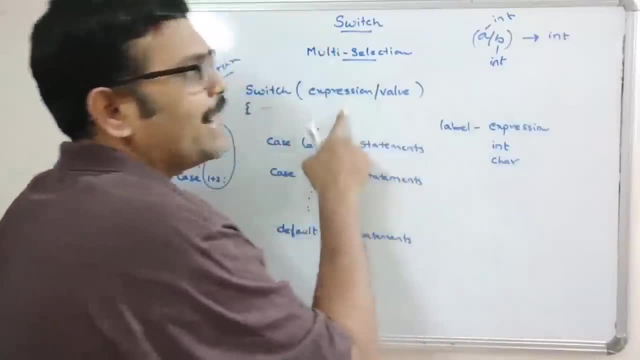 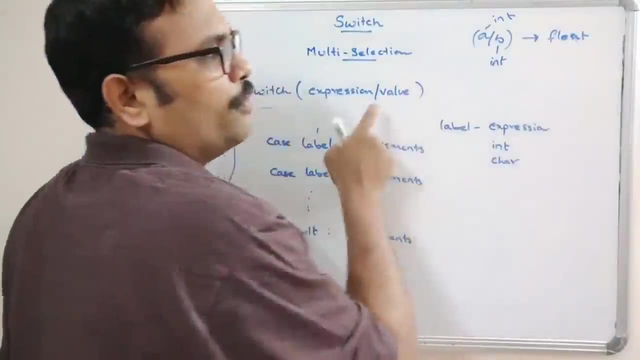 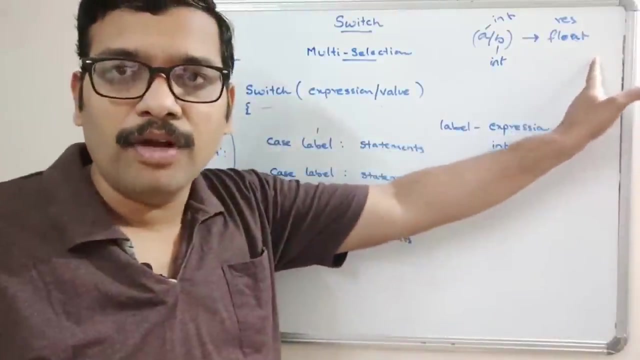 We will get the result in integer, But in javascript, we will get the result in float. We will get the result in float. Ok, So this is the result. Even though the numerator and denominator are integer, We will get the result in float. 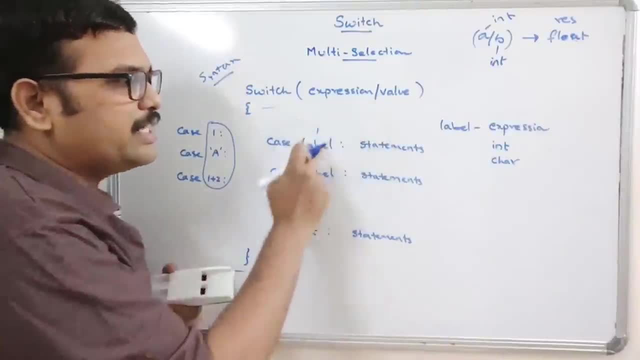 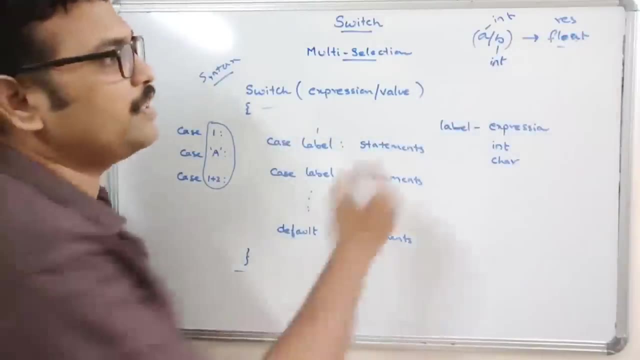 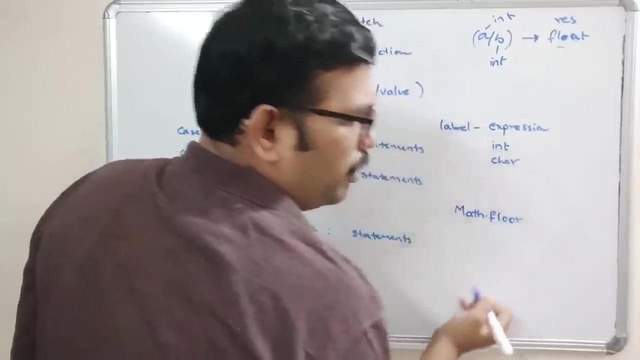 Then if we get the float here It doesn't matches with any label Right. So for that purpose we have to change this float into integer. For that purpose We are having a function called math dot floor, Math dot floor of give the expression a by b. 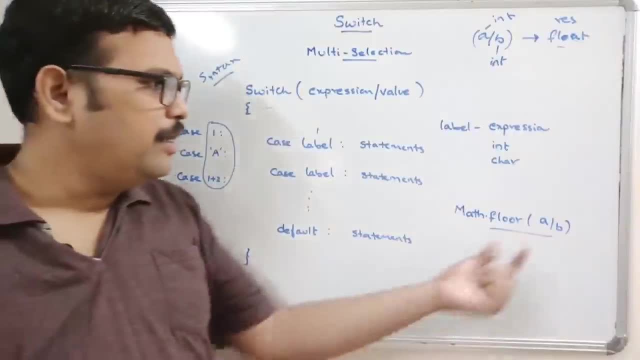 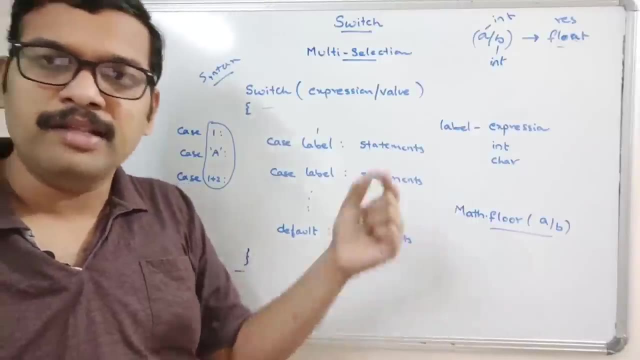 So that automatically flooring will be done And only the integer value will be displayed here, Or seal. Seal function also can be applied. Ok, Either floor or seal. So by using this function we can change the float value to integer value. 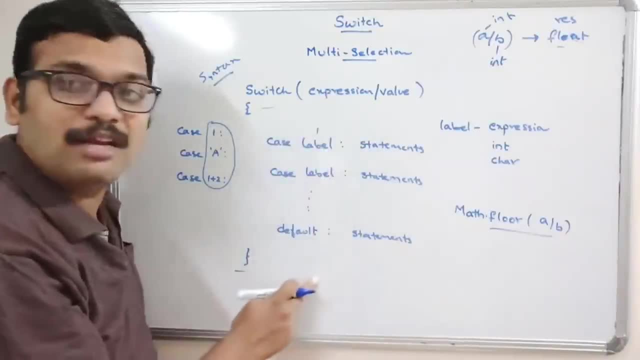 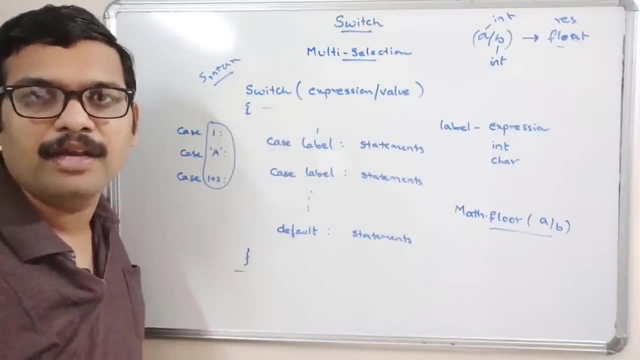 So that integer value will be compared with all these case labels And executes the particular statements where the label is matched. Ok, So hope you understood the syntax And we will say a small example. So, taking the marks of a student, 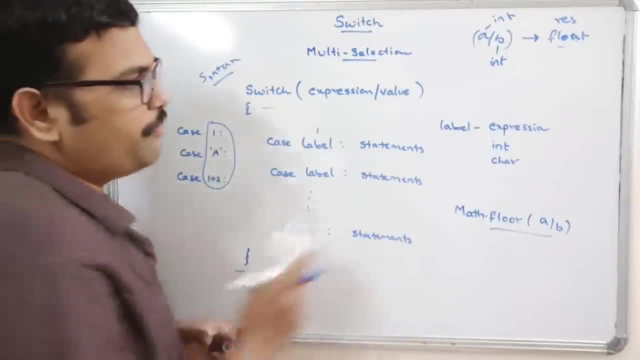 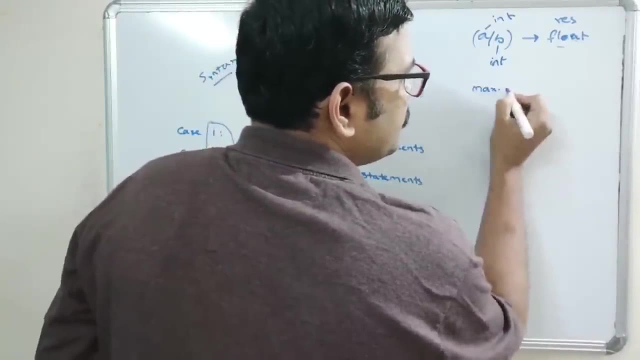 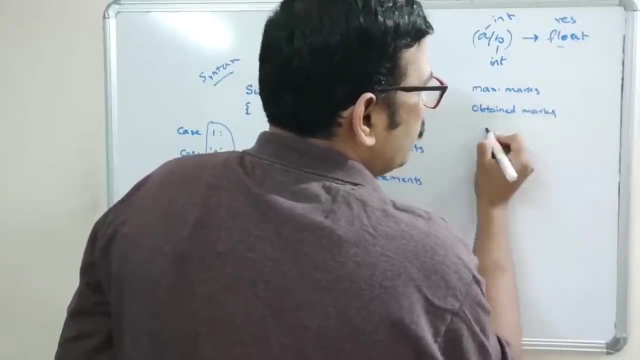 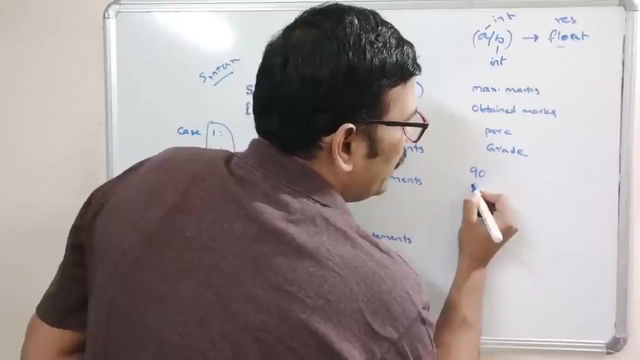 And calculating the grade. Ok, So, for example, Take this one, Take this example. So we will take some maximum marks And obtained marks, Obtained marks, So that we have to calculate the percentage and grade. So, if the percentage is 90 and 80. 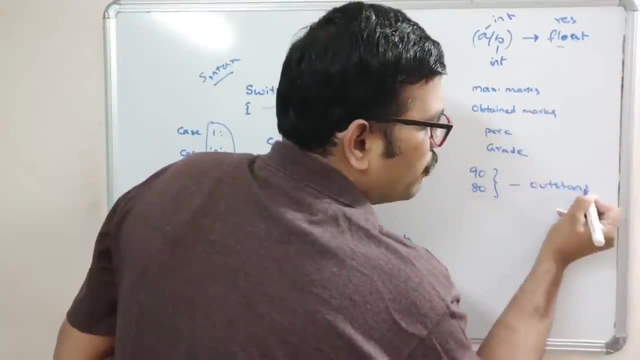 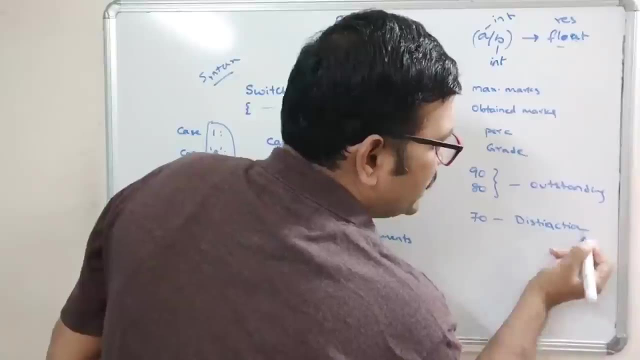 Go with some outstanding grade Outstanding. And if it is a 70. Go with the distinction. Go with the distinction. If it is a 60. Go with the good. So grade is good If it is a 50.. 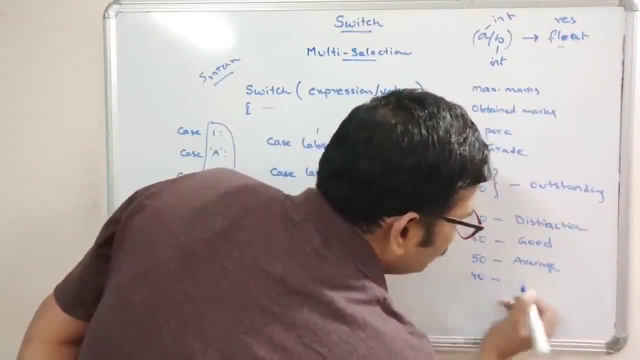 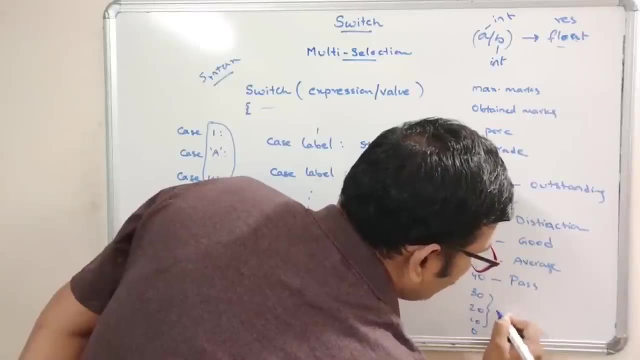 It is a average, If it is a 40. It is a pass, And if it is a 30 or 20 or 10 or 0. We get fail. Ok, So this is the grading which we want to display. 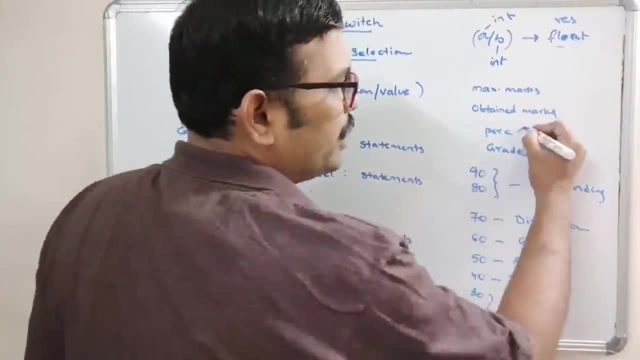 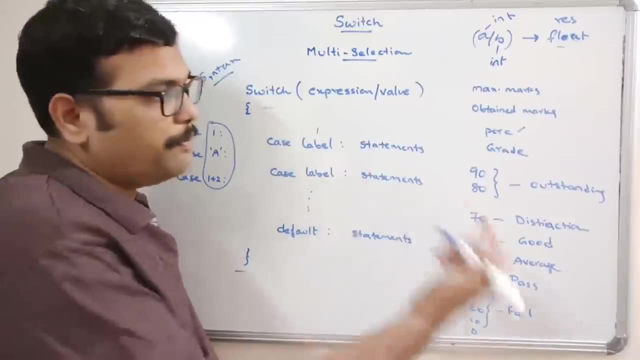 So here we can write: First we have to calculate the percentage And based upon the percentage we have to give the grading. So for that purpose we will take some percentage And divide it by 10. So that, whatever the result we are getting, 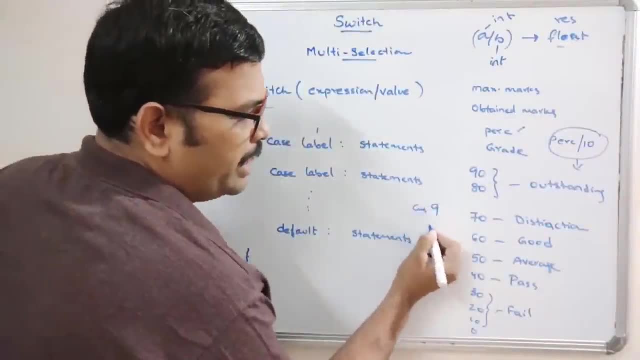 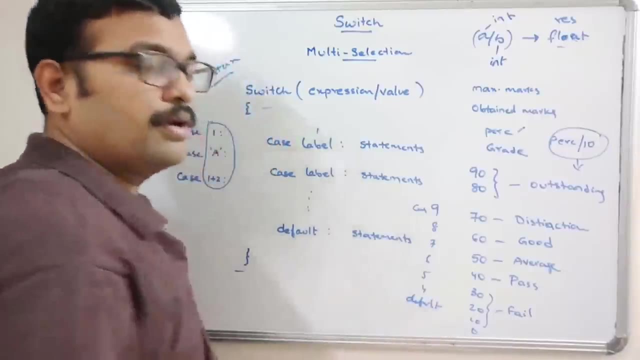 Based upon that. So we will write some case- 9,, 8,, 7,, 6,, 5,, 4- and default Ok If it is 9 or 8.. We can go with the outstanding grade If it is a 7.. 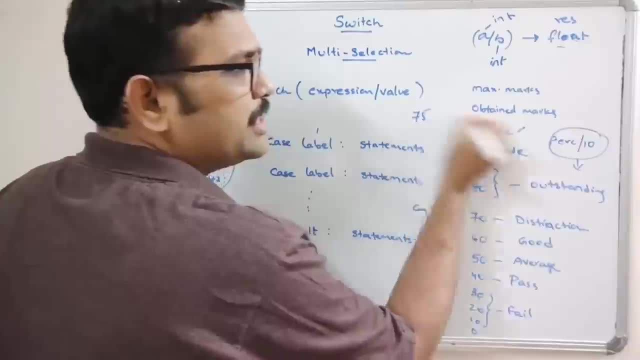 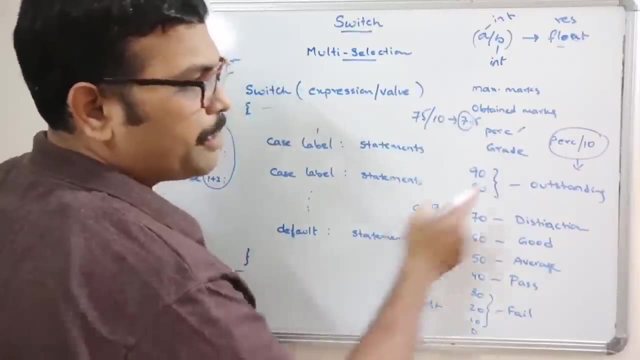 We will go with the distinction, Because if it is 75.. 75 by 10. We will get some 7 result. Ok, 7.5. And we will go with the floor function Mathfloor, So that it will be rounding to 7.. 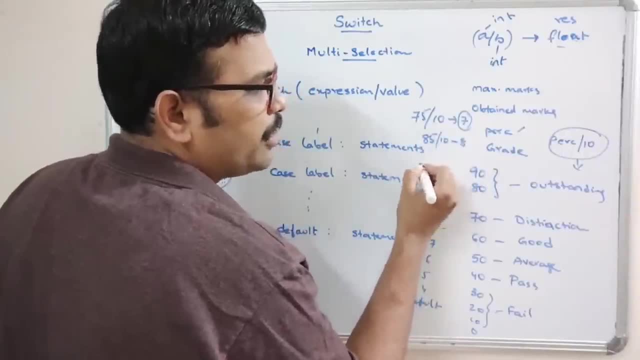 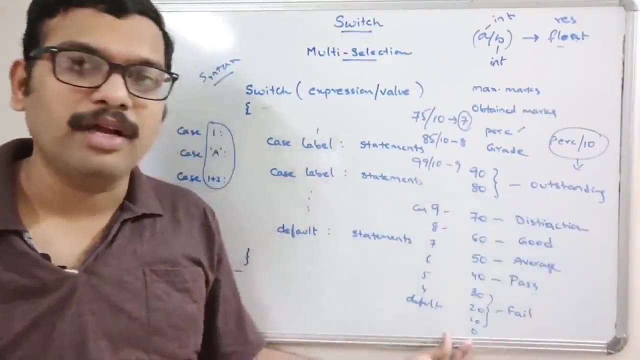 Similarly 85.. 85 by 10.. It is 8.. Ok, Some 99 by 10.. It is a 9.. So like this We can go with the outstanding. Ok, So even We will go with this one. 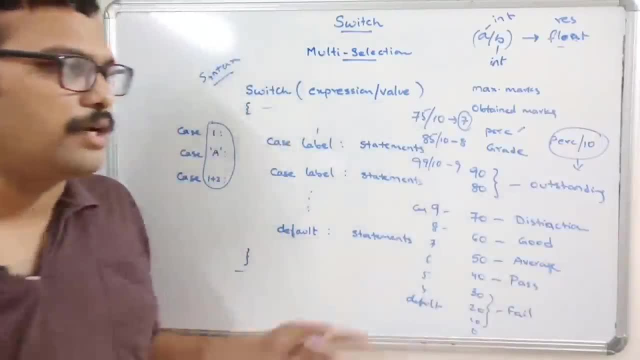 Right, So hope you understood this one. So we will execute this program in the computer By writing a small html code And I will show you. So we will go with this one, Right? So hope you understood this one. 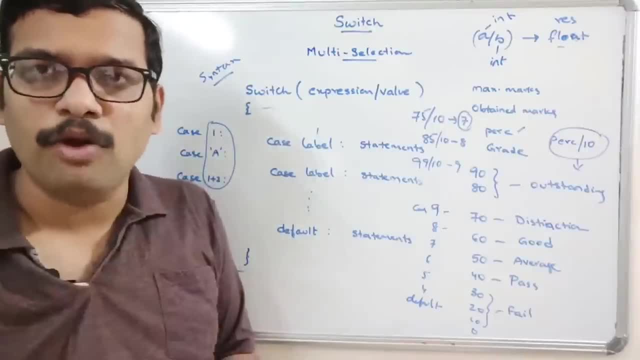 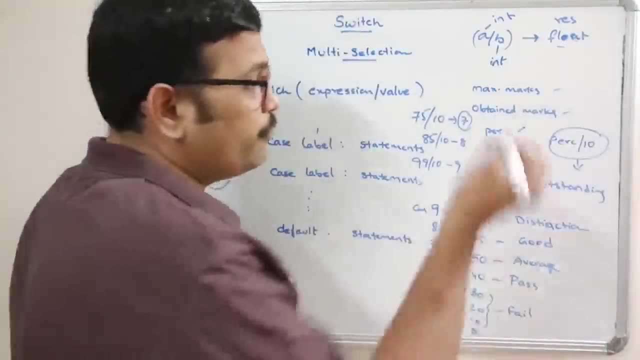 So we will execute this program in the computer By writing a small html code And I will show you. So we will take the maximum marks as input, Obtained marks as input And we will calculate the percentage and grade and those will be displayed. 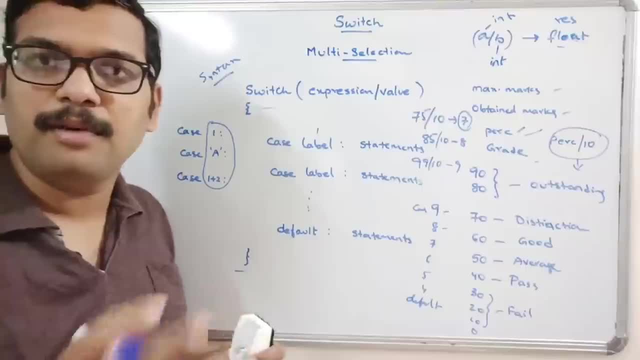 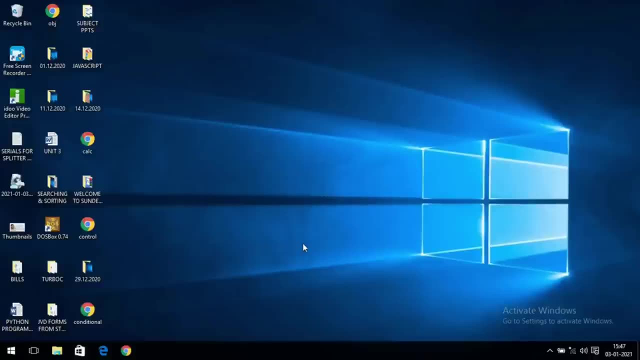 Right, So let us move on to the computer. Hello friends. So just now we have seen the syntax of switch statement in javascript. Now we will execute a small code demonstrating that switch case. So for that we will start writing the syntax. 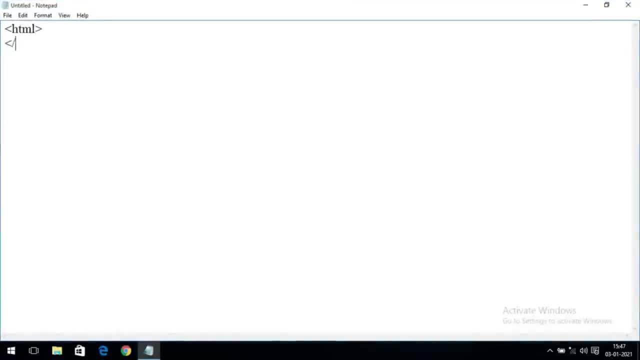 So we will write down the html code, So write down the html tags and inside the html tag, inside the body, Let us take one. So let us take two fields, that is, one is a maximum marks and next one is the obtained. 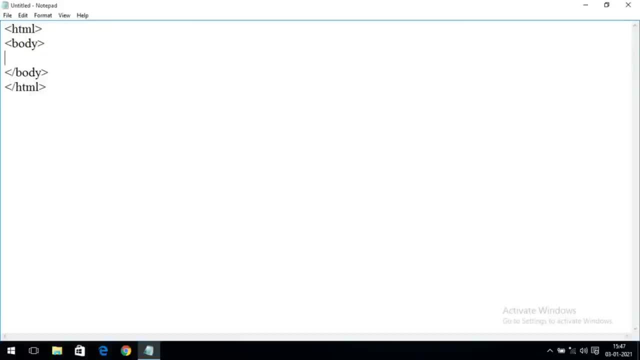 marks, So that we need to calculate the percentage and give the grade for a student. So in order to receive the maximum marks and the obtained marks, So we will create some text box Right, So let us put the heading here. 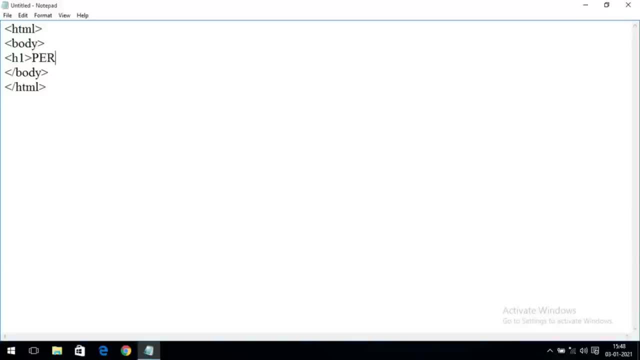 So grade, percentage and grade calculator, Percentage and grade calculator. So after giving the marks we need to get the percentage and grade. So for that purpose, first of all we will take the maximum marks as a input, Maximum marks- And for the input we will take some text box. 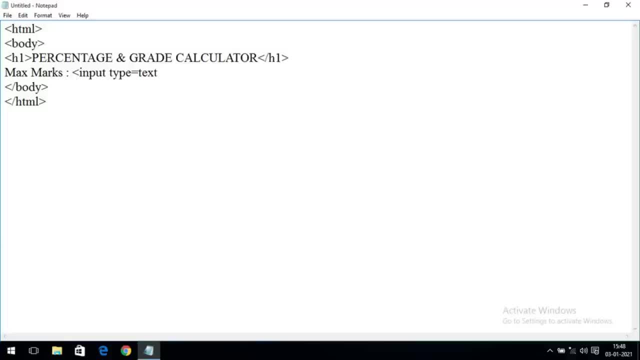 Input type is equal to text. Okay, And also we will give some id. Id is equal to some. mm Means a maximum mark. Okay, And then go with the break row So that the next text box will be printed in the next line. 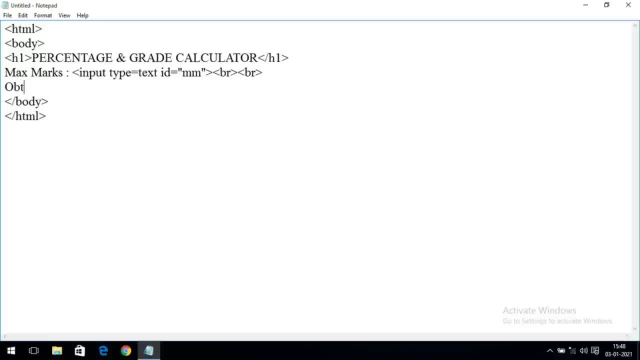 So the next text box is for getting the obtained marks- Obtained marks, Okay, So for this also we will go with the text box Right, So we will also give some id for this one. So this is for om. 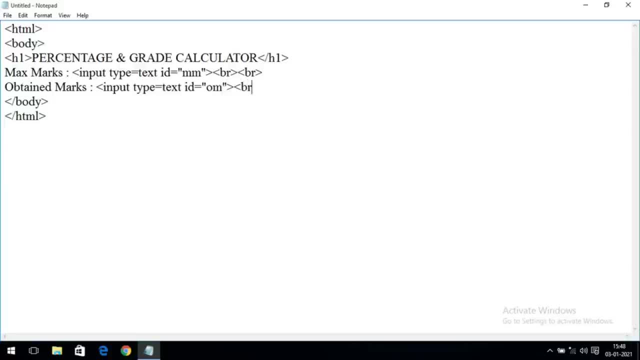 Obtained marks And again go with the break rows Again. then, just after clicking the submit button, we need to calculate the percentage and grade. So for that purpose we will create one button, So button type is equal to button And on click. 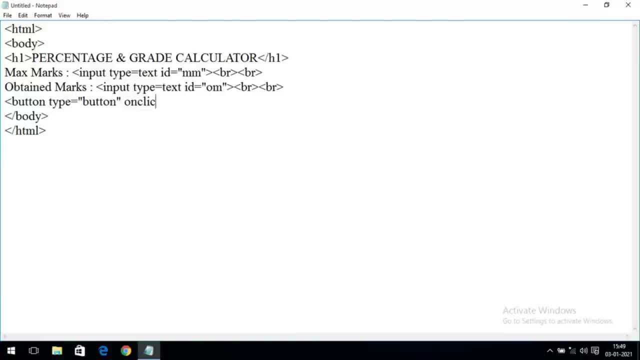 So after clicking this one, what should happen On click is equal to it should trigger one function, So that is percentage and grade PG. So let us take some PG as a function, Okay, And give the title for this button. 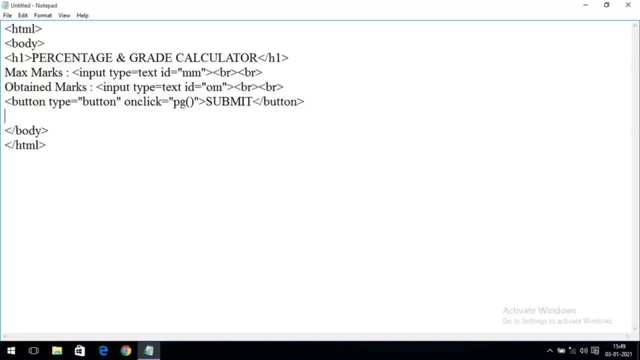 And close the button type Right So where we have to display the percentage and grade. So for that also we will create some text box So that the percentage will be calculated and the output will be displayed in that particular text box. 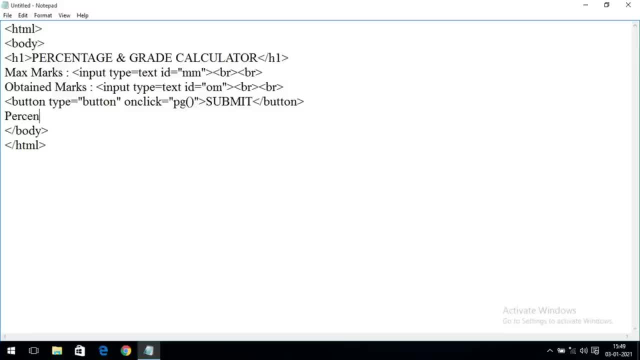 Similarly, the grade will also be calculated. So percentage, So percentage, Right. And here also we will go with the break line, Break row, Because the percentage should also be displayed in the next page, I mean next line. So here again I will go with. the input type is equal to text. 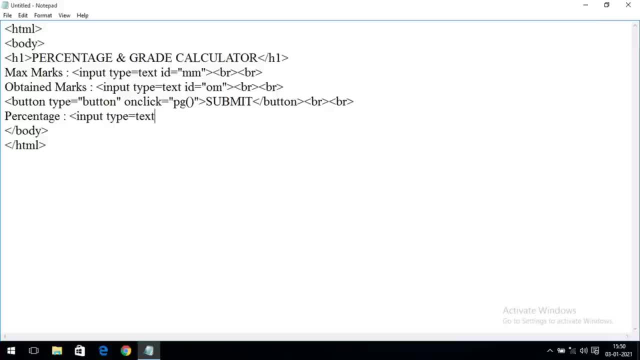 So text box where we have to display the result. For this also we will create some ID So that in JavaScript we will use this ID. Okay, For this ID we can go for that. So percentage, And So I am giving some BR. 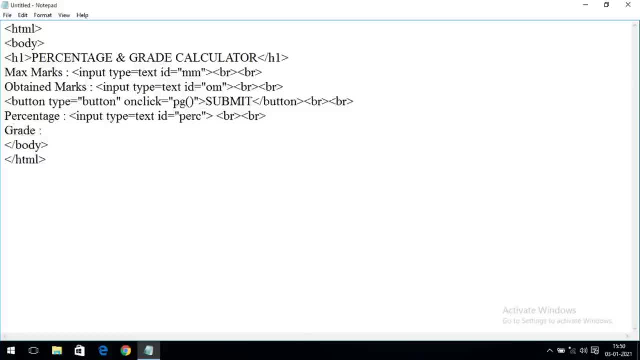 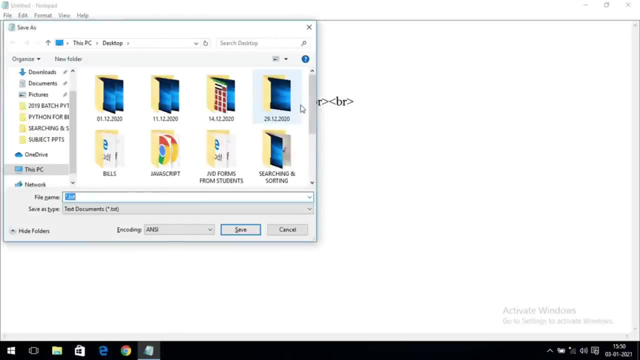 And grade, So we need to find the grade also. Grade Here also. we will go with: the input type is equal to text And ID is equal to grade. Right Now, let us save this one. So with this one, 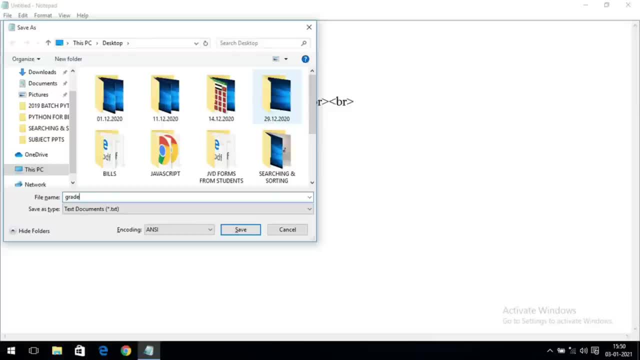 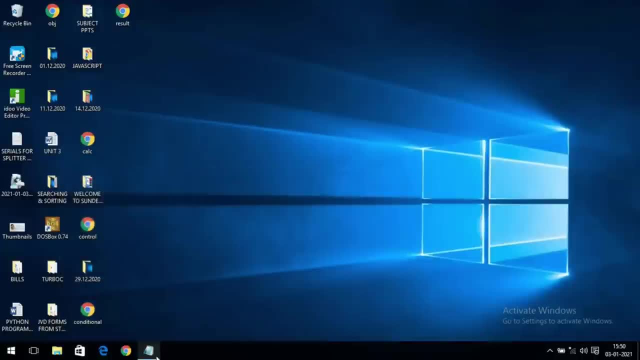 We can save this one: Grade- Html Or result- Html. Okay, Result Html- Okay. So we have saved in the desktop So you can observe here. So this is the page, So double click on that. 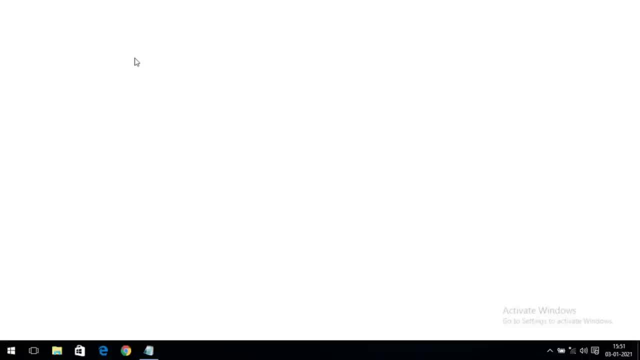 We will get the page. See, We are getting some maximum marks, Obtained marks, And after clicking on the submit, Submit button, We need to get the percentage And, based upon the percentage, We need to get the grade. Now 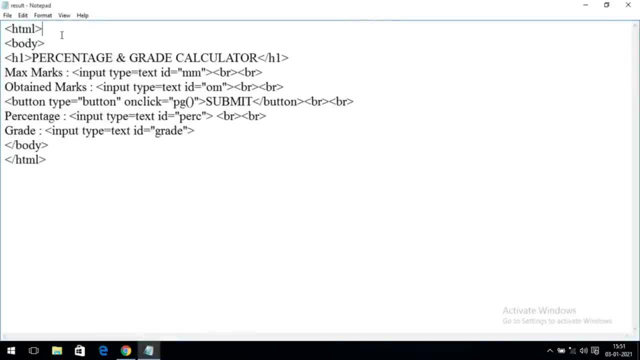 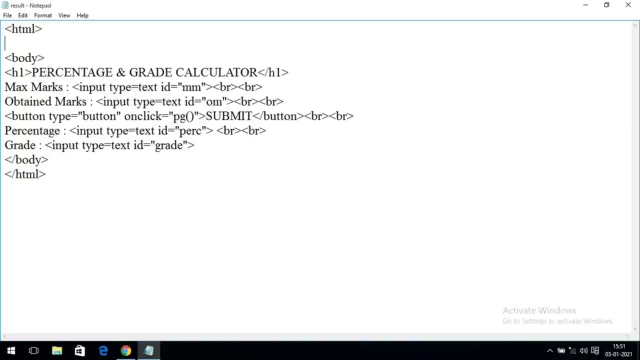 Yeah, So now, yeah, now what we have to do. so whenever the button has been clicked, that means pg function should be triggered, and where we have to write this pg, so we have to write that pg in a script tag. that script tag can be written in head or body, so we'll write in head, okay. 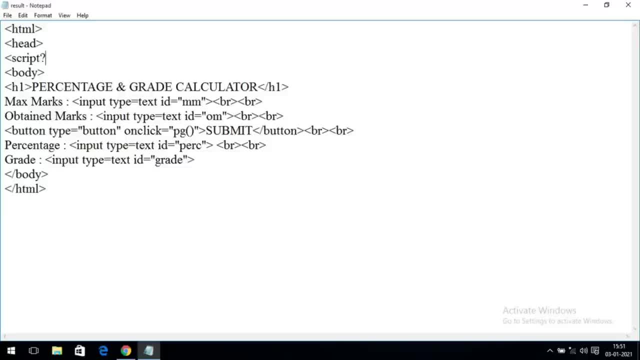 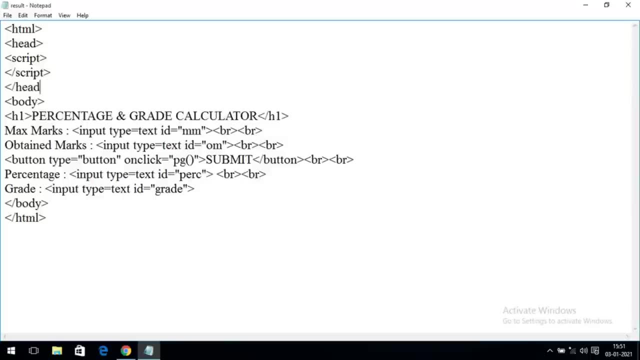 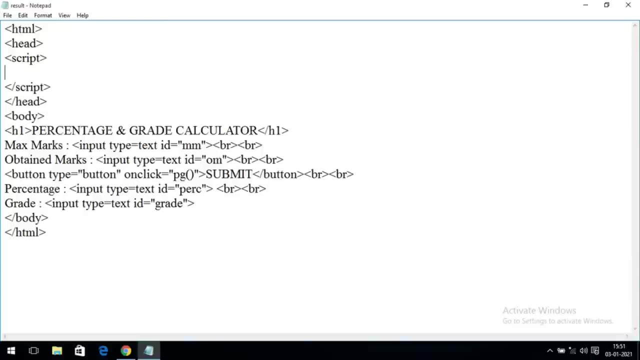 script and also we'll close that one so that we never forget to close that, and also we'll close the head right now, in between the script we'll write here. so, first of all, we need to calculate the percentage. okay, we need to calculate the percentage. so, in order to get the percentage, 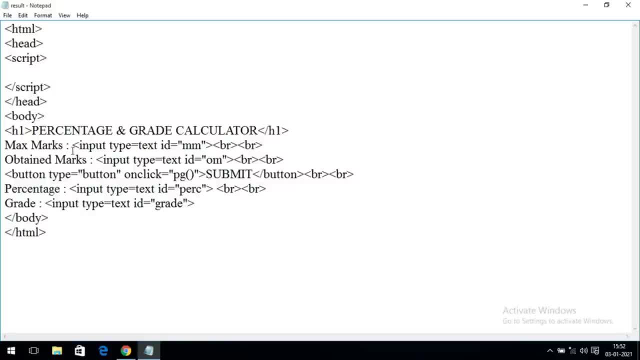 what is the formula? so obtained marks divided by maximum marks into 100. so the same thing we'll do. so document dot, get element by id of. so where we have to go with this one. so percentage. so the result, the percentage, should be displayed in here. okay, so percentage. 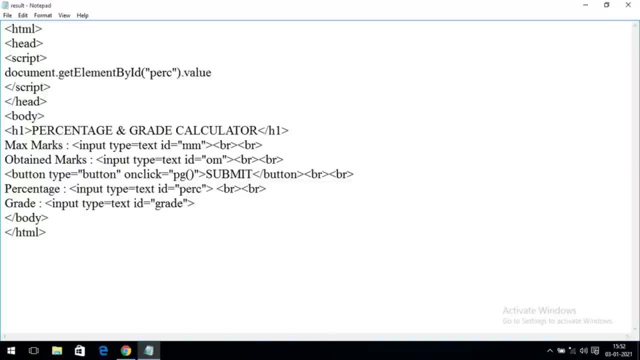 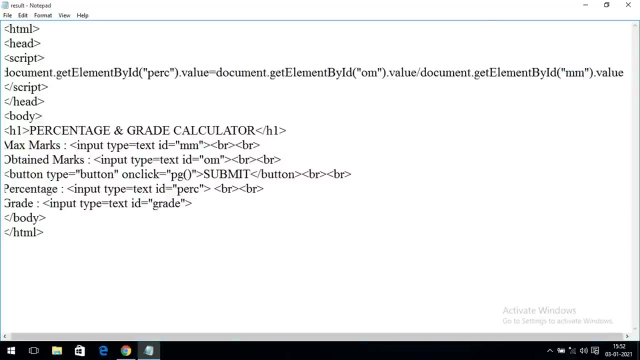 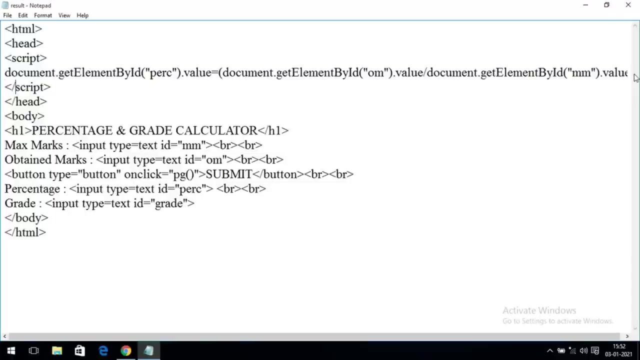 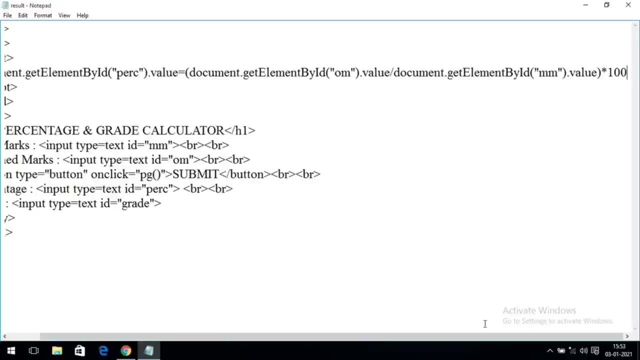 percentage value is equal to what we have to do. we have to put the division operator, so i will copy this one. so here, obtained marks, that means om dot value divided by what is this one? maximum marks, right, maximum marks. and completely we have to multiply with 100 so that we'll get the percentage. okay, we'll get the percentage. 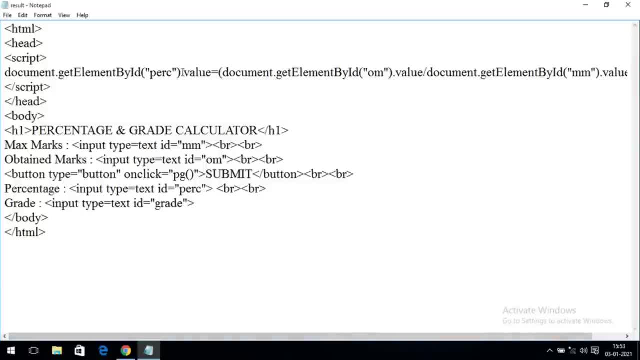 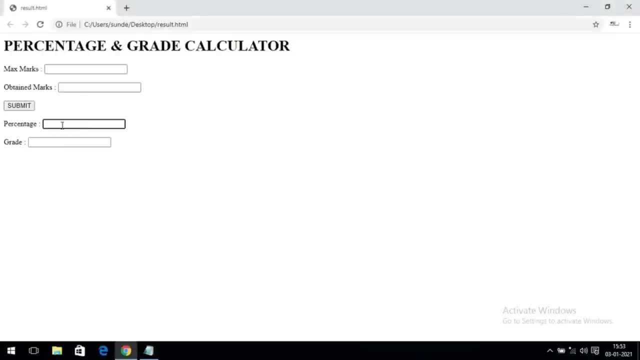 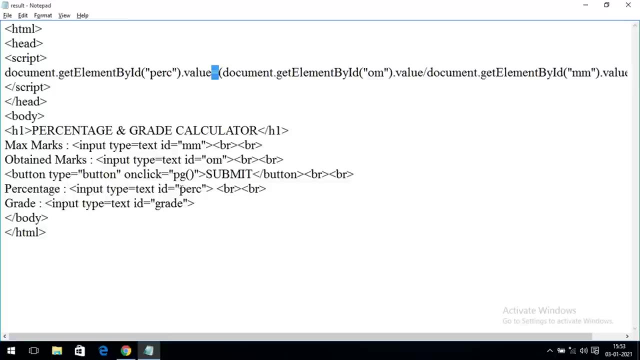 hope you understood in this one. so we- i am just giving some assignment and where we where it should be displayed in the percentage in this place we have to display the percentage. so how to get this place? so get element by id of percentage, because percentage is an id given for. 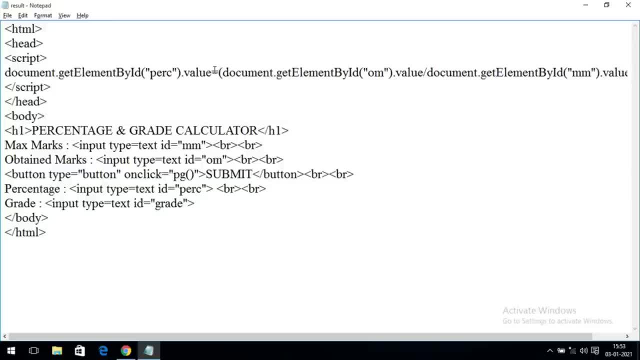 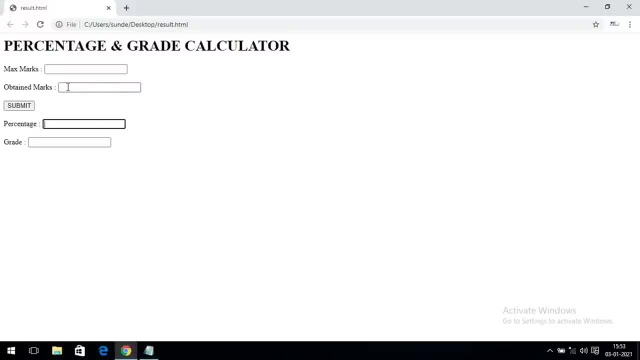 this text box. so dot value is equal to document dot. get element by id. om dot value, that means obtained marks. whatever the marks we are giving here in this text box, divided by the marks given in this text box into 100, let us execute this one. so i am giving some. 600 is the maximum mark and 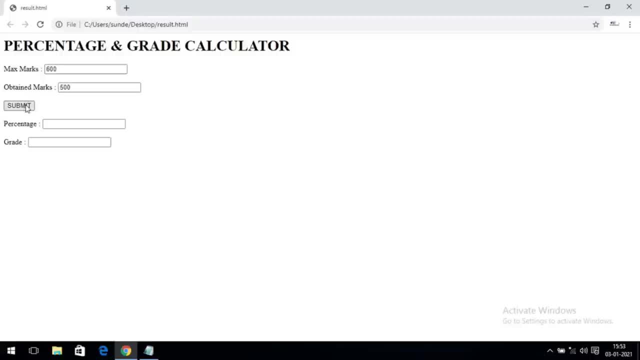 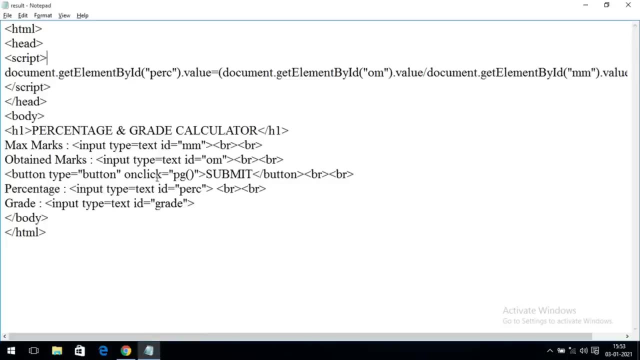 500 is the obtained mark. so i am giving some: 600 is the maximum mark and 500 is the maximum mark and 500 is the obtained marks. so submit: yeah, okay, so we are not getting here. so yeah, see, here we are giving some on. click is equal to pg. 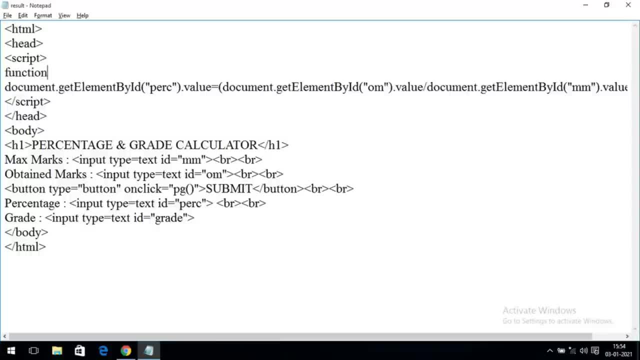 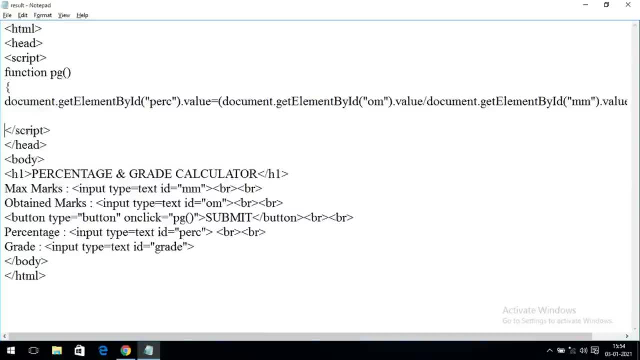 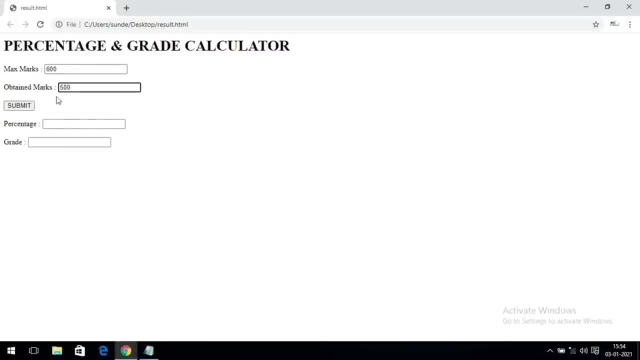 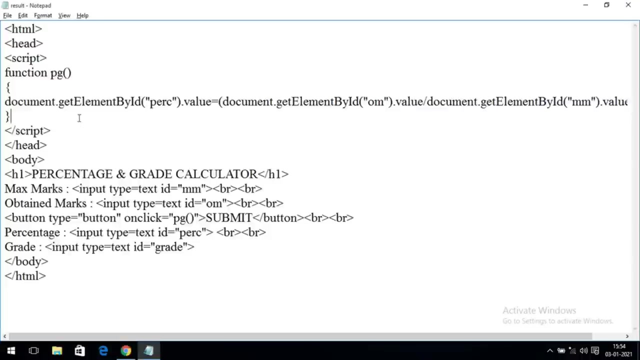 pg is a function, right? so we have to write everything in a function function: pg- open brace- oh sorry, close address. right now let us check. so 600, 500, and after clicking on the submit, you are getting some percentage here, right? so we have. we need to find the grade. so in order to find the grade now we have to check this. i mean, we have to. 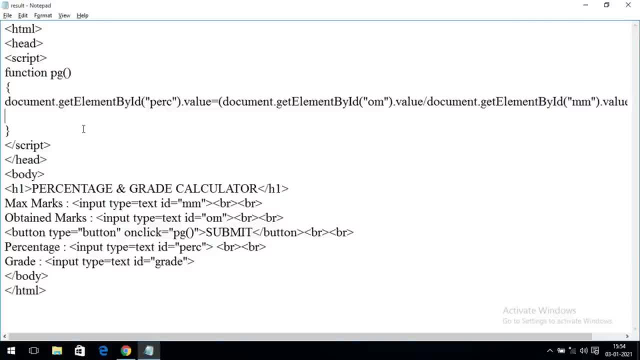 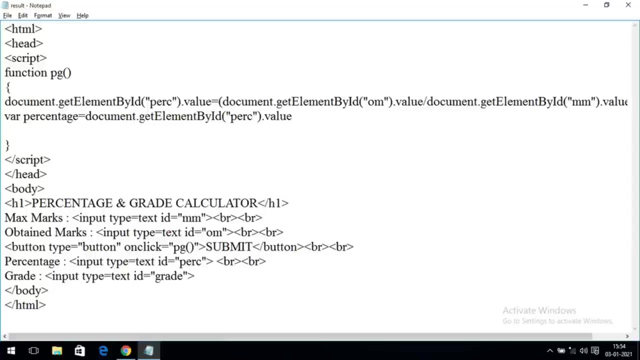 give the grade based upon the percentage, based upon the percentage now, so you can get here. so just take one variable. percentage is equal to this value. so whatever the value here, that will be assigned to some percentage. okay now, and also give some grade. give some grade here. take one variable as a grade right now. after that we have to write. 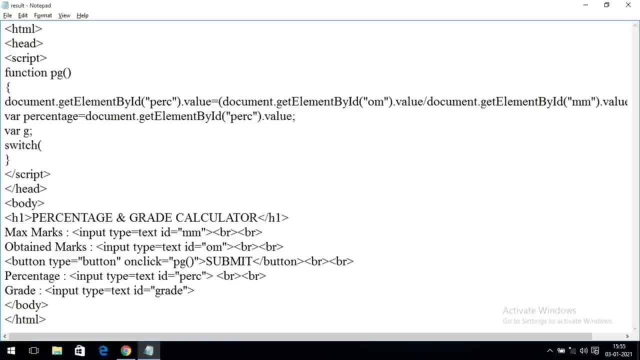 the switch case, because we need to find the grade based upon the percentage. so how we can do that. so, So how to get the percentage. So percentage divided by 10. So automatically we will get the 10th position. That means if it is a 83, we will get the result as 8.. If it is a 94, we will get the result as 9.. So based upon that, we will create a grading. 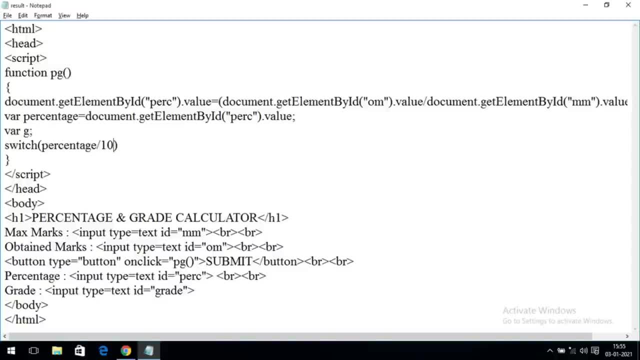 Okay, So here, percentage by 10 means if it is a 95, we will get some 9.5.. Okay, The result will be 9.5.. Even though we are getting both the numerator and denominator of the integers, we will get the accurate result in JavaScript. 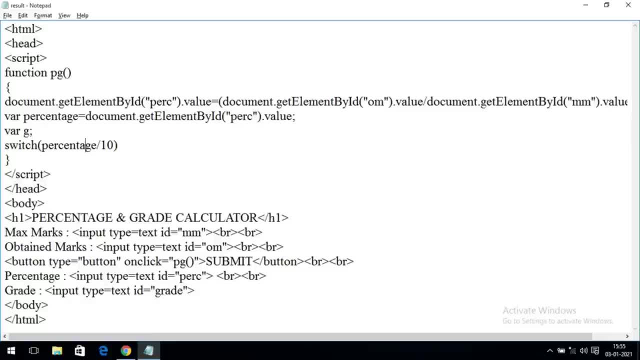 So, but switch case. So all the case labels should be either integers or expression, Right. So for that purpose we will go with the one more function called flow rate. So we have to flow rate, Okay, Math. 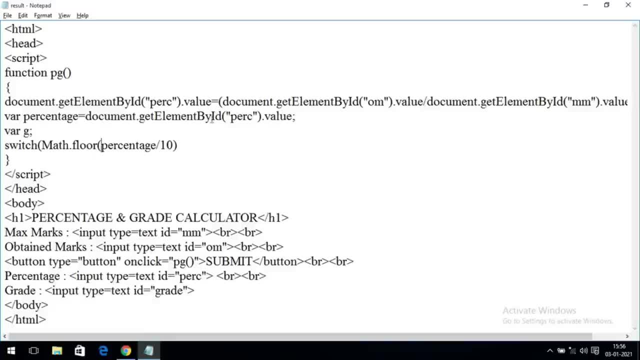 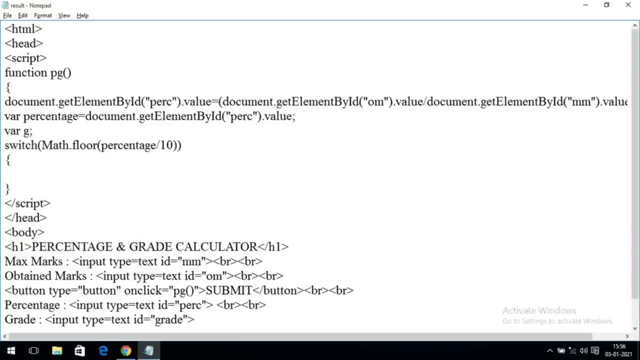 Flour of percentage by 10. So that we will get only the integer value. We will get only the integer value. So here we can write the cases, different cases. So first of all we will go with the case 9.. So if it is a 9., Okay, If it is a 9., Right, So what we will get. 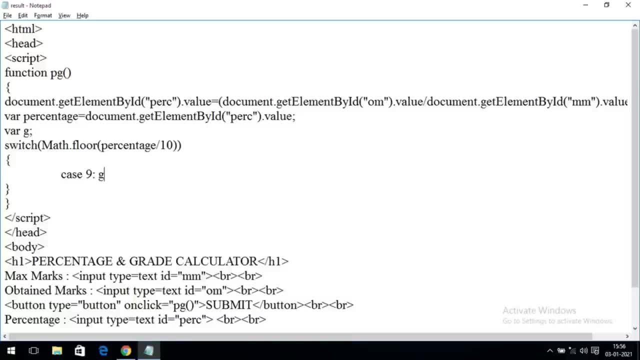 WordPress. the grade should be some outstanding. Okay, Grade should be some outstanding. So even if case 8, that means 80, if the percentage is 80, it is also outstanding Right. So I am giving some g is equal to outstanding Right And also we will go with the break. 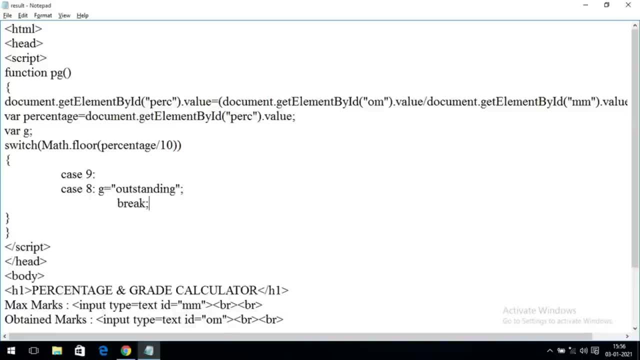 After this one, we will take the break So that it will come out from the loop Switch. Okay. So if it is, if the percentage is 70, then give the grade as very good or a distinction Okay. 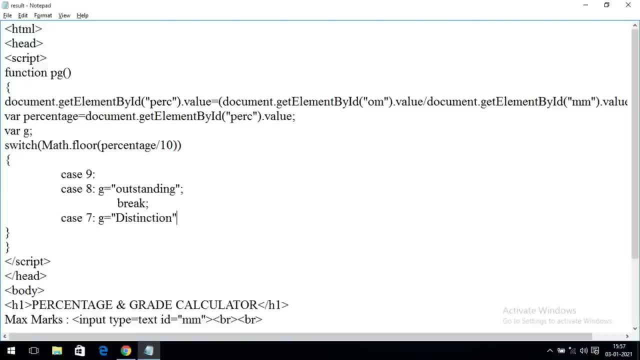 It is better Distinction Right And also give the break So that it will come out from the switch case. Whenever this condition is true, it will come out from the switch case. Case 6, if it is a 60, then go with grade is: 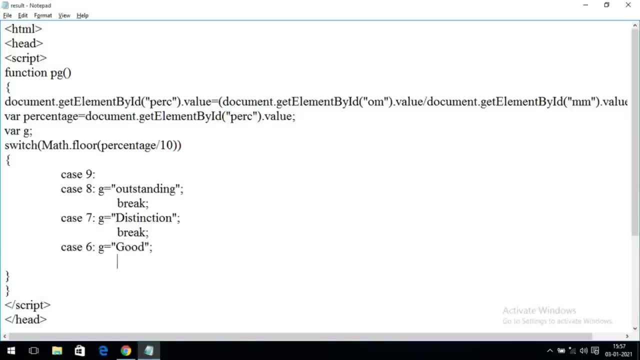 good, Okay, And also break. Next case 5 is grade will be some average Average. And also break Case 6.. Case 6. Case 6 is sorry, sorry. case 4. This is just 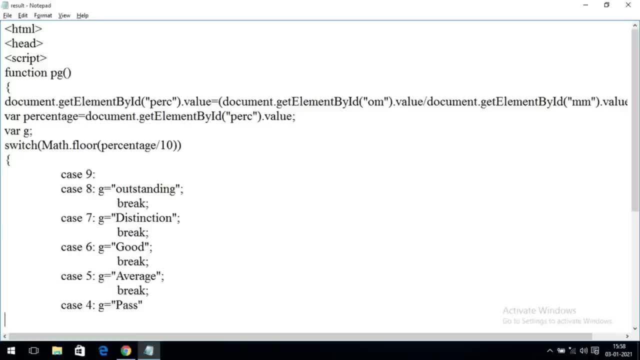 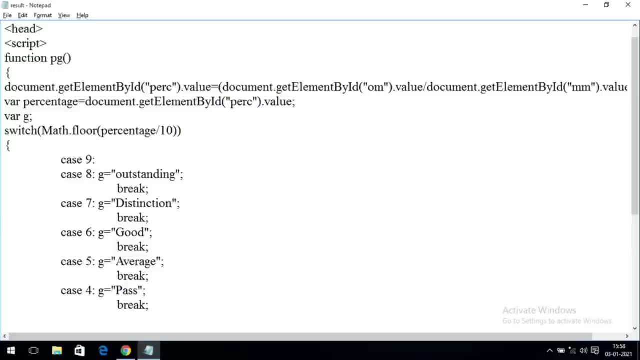 pass. Okay. G is equal to the grade is pass, And whenever we are getting the marks or percentage from 30 to 10, for everything, it is a fail. So instead of writing all the cases, we can go with the default. So, other than all these things, the grade will be fail. Fail. Okay And go with the. 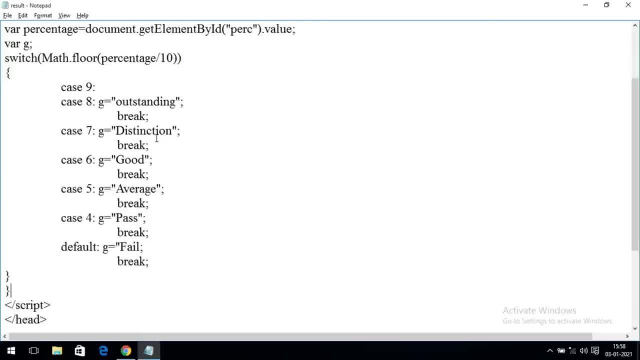 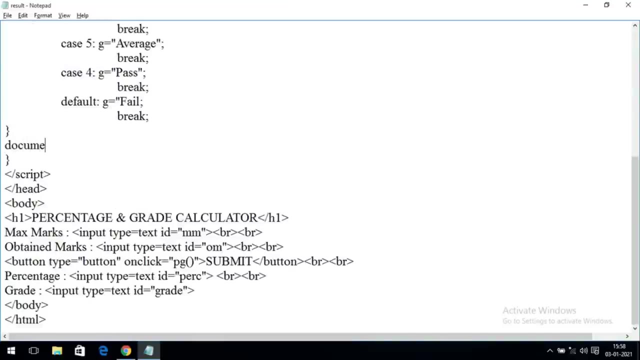 break Right And after the, after completion of the switch. so here we will get some grade and we have to display this grade in this position. Okay, In grades position. So here we have to write So document dot get element by id. What is it here? It is a grade Grade dot. value is equal to g. 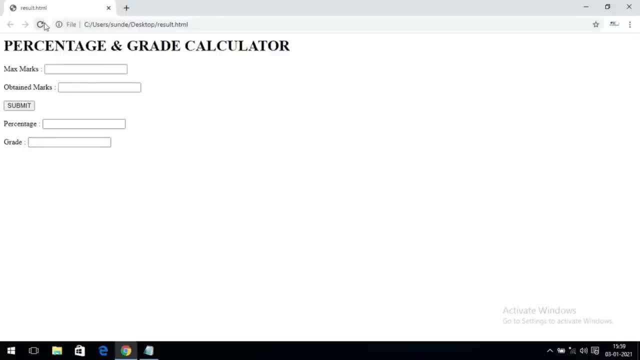 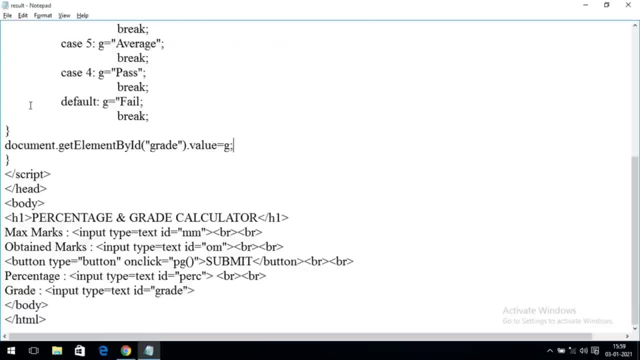 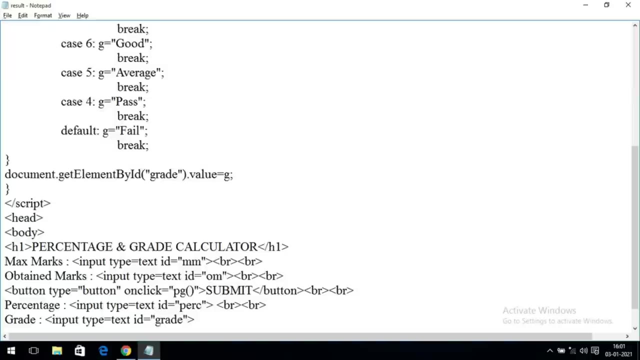 So automatically the grade will be displayed there. So now you can observe here. So if you are giving some maximum marks- 600 and a 500, if you submit here. sorry, see here, we have not given the double quotations. 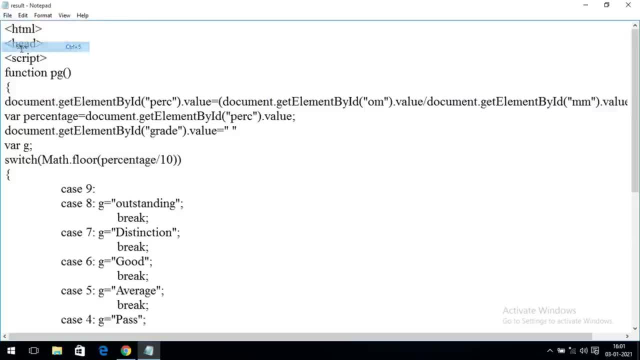 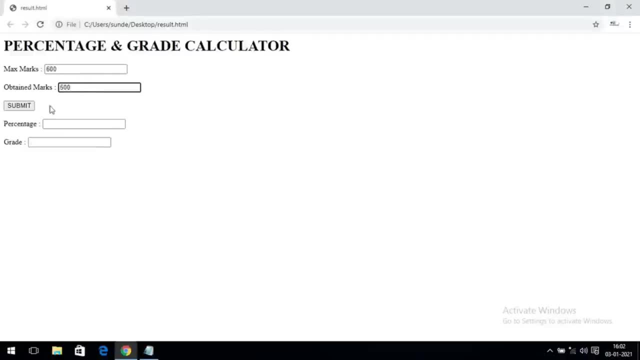 We didn't close the double quotations. Now we can check here. So execute this one, So 600, and give the 500 as obtained marks Submit. So we are getting some 83.. 8 means outstanding If you reduce the marks here, some 400.. So we will get the. 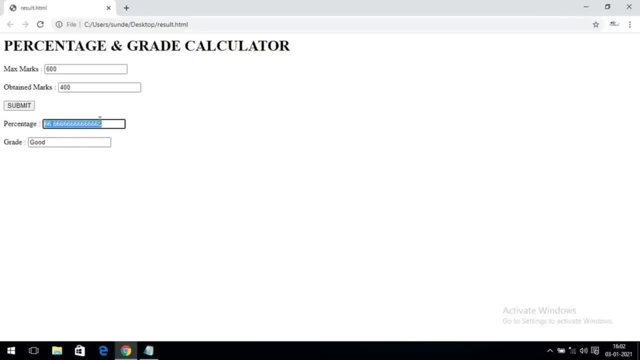 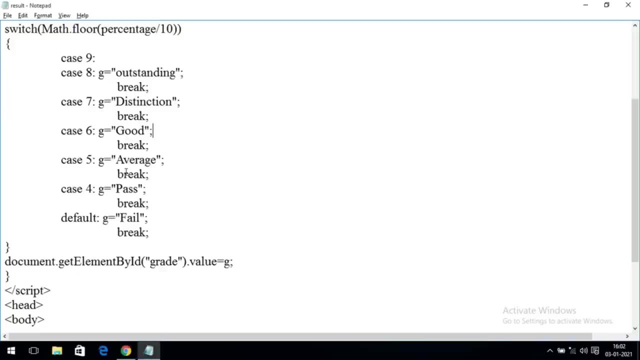 percentage: 66. So if it is a 66 percentage, the grade is good. Okay, Here you can see. grade is good. So like this, we can apply the switch case And, as we have discussed in the syntax for the switch case, So unless you give the break, 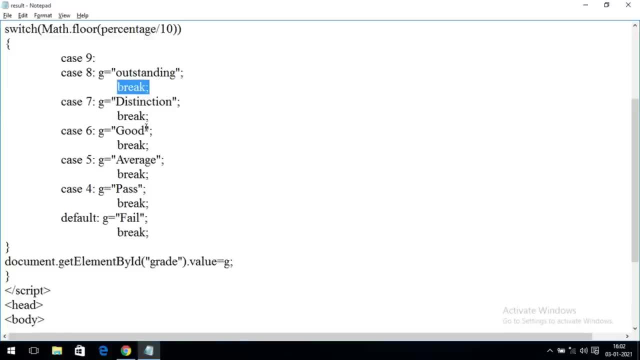 statement it will come keep executing the all the cases. So here, in the case of 9 or 8,, that means if the percentage is between 90 and 80, the grade is same. That is the outstanding. 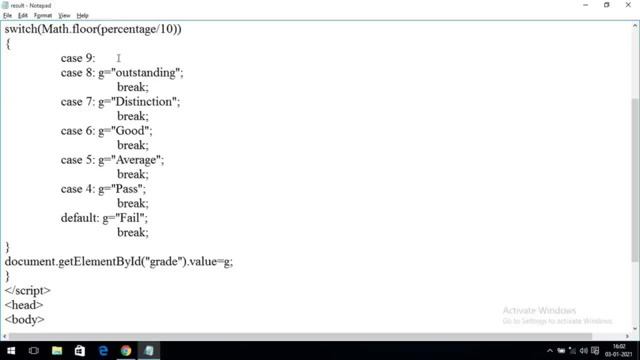 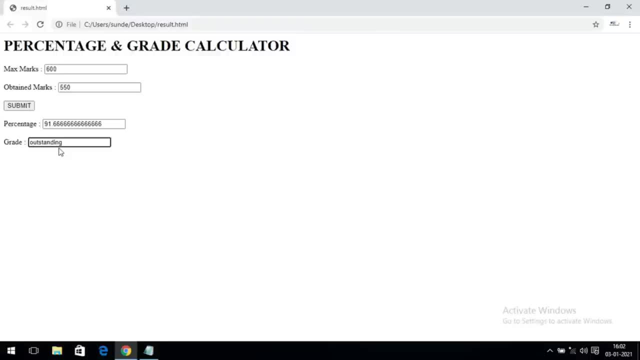 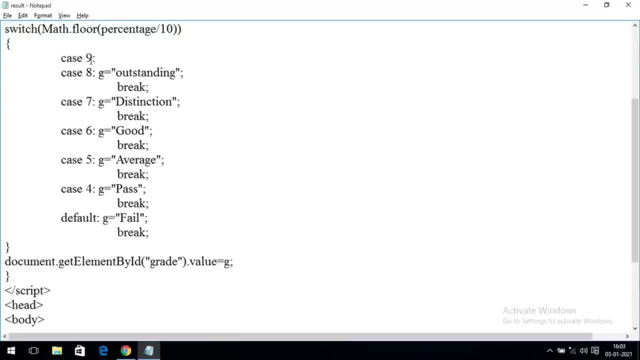 So that's why I have not written anything here. See some 550.. Then you can go with 91.. Still we are getting some outstanding. Still we are getting some outstanding. So like this, we can apply the switch key. So here, one thing we have to remember is based upon 60.. 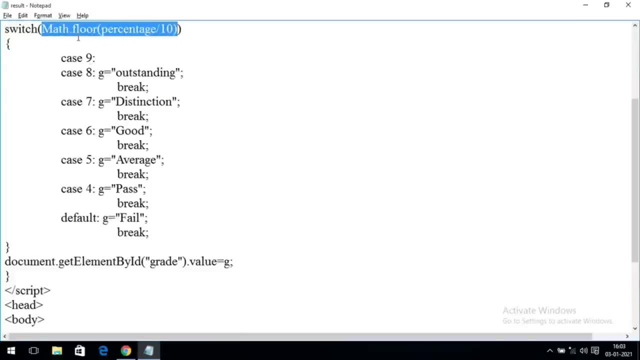 the result which we have passed in the switch statement. that will be applied for all the case labels, all the cases, different cases. So we have to include the break if you want to exit from that particular case. So if you are not giving this break automatically, it will keep. 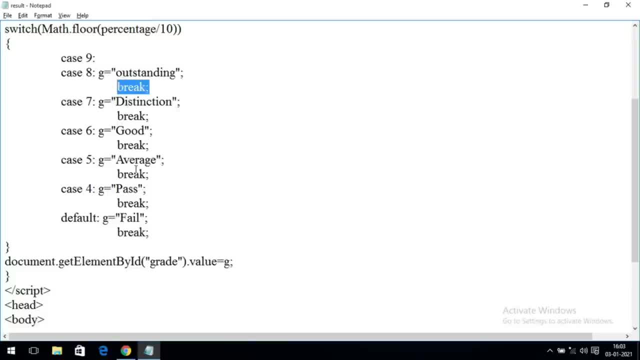 on executing the statements until it executes the break state. So here, if it is a case 9, nothing has been printed and we are not giving any break. So that is why it will go with the next case. So if the result does not match with any of the case, label automatically this default. 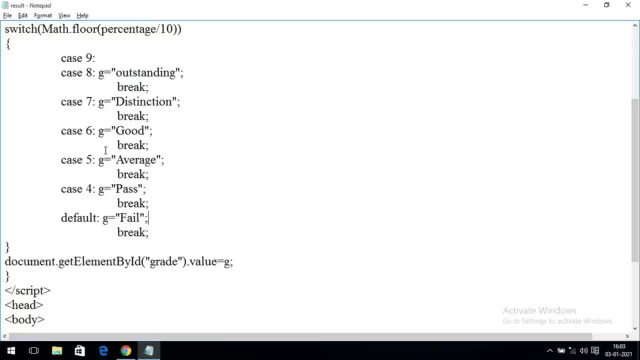 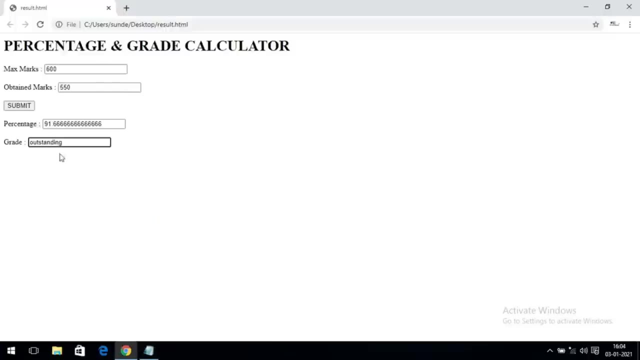 label will be executed. So that is why. so, other than these results, that means if the percentage is having the 30 or a 20 or a 10, then all those cases will get this case executed. that means a phase. okay, that will be displayed here itself. So this is how we can. 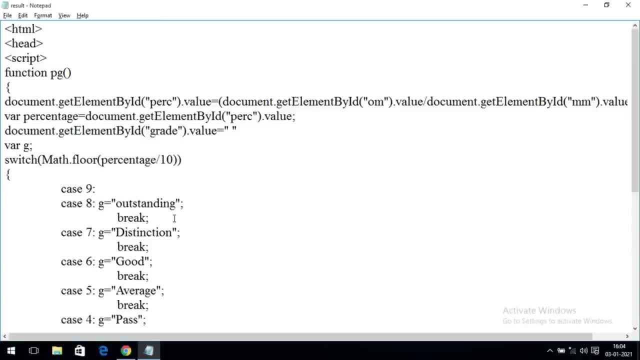 execute the break state, Use the switch case. So, in order to find if you want to give the multiple selections, multiple selections, we can go with this. this one. okay, switch case right. So hope you understood this one. 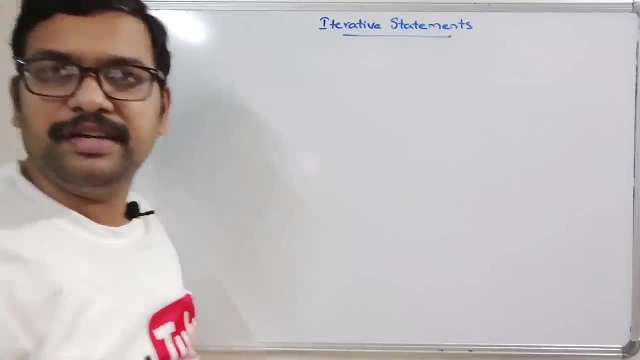 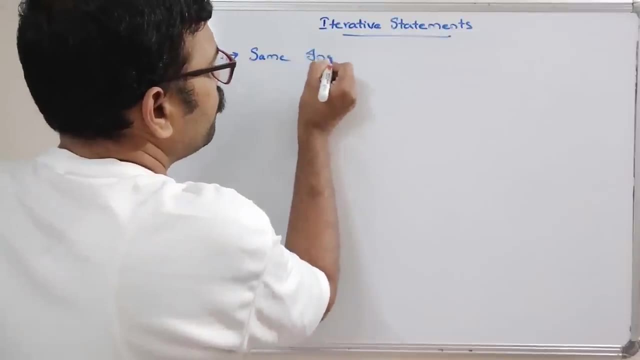 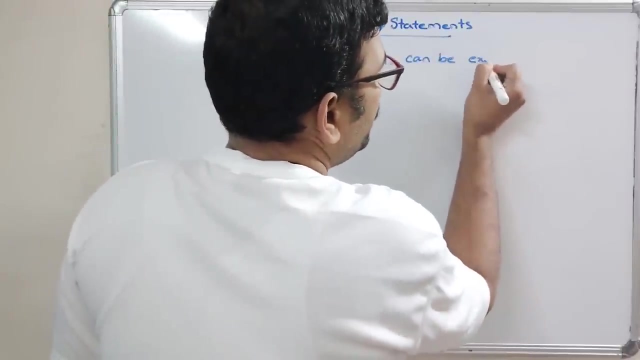 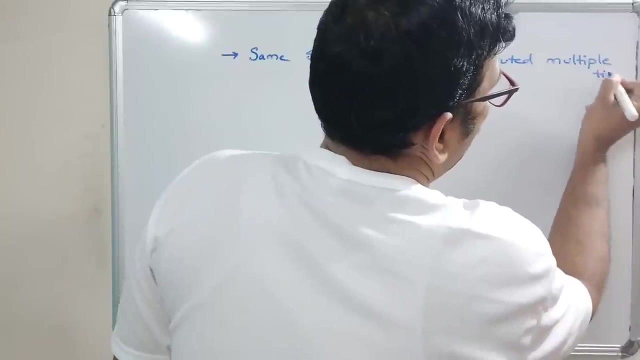 So what is the meant by iterative And what is the use of this? iterative statements? So here mainly same instructions. So whatever the instructions we are writing, same instructions can be executed multiple times. So we can execute some same set of instructions multiple times. 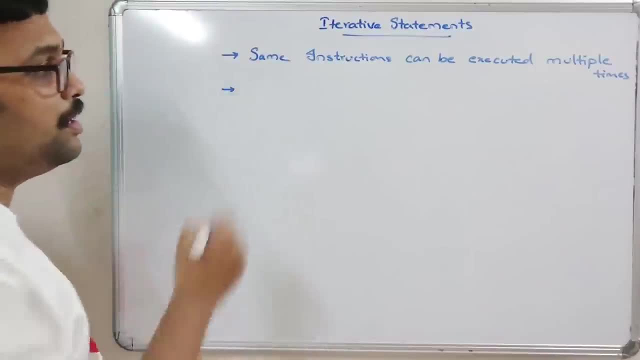 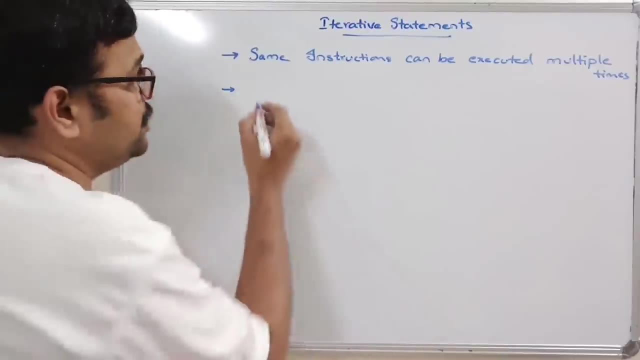 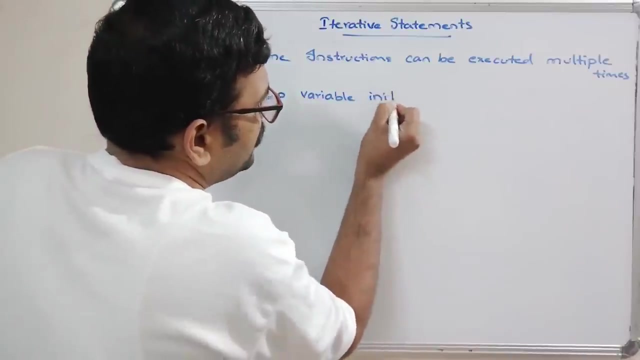 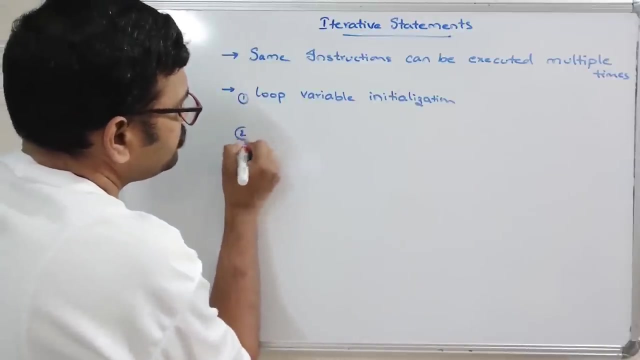 Okay, And here we will write some conditions. So, for all the iterative statements, whatever the iterative statements we are using, we have to follow the three things: One is the loop: variable initialization. The second one condition. The third: one condition. 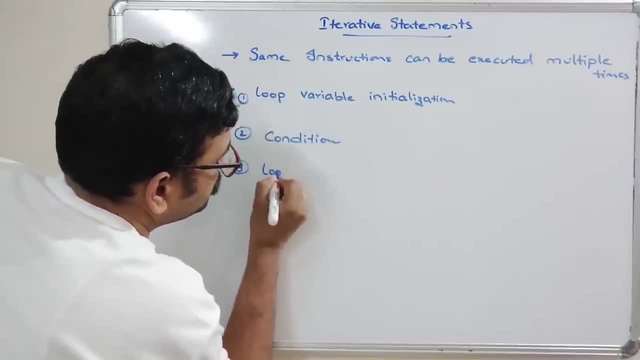 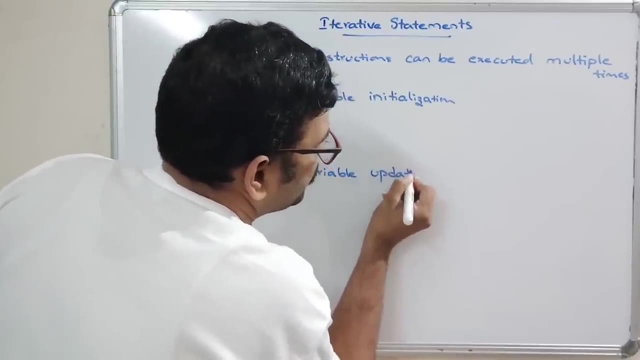 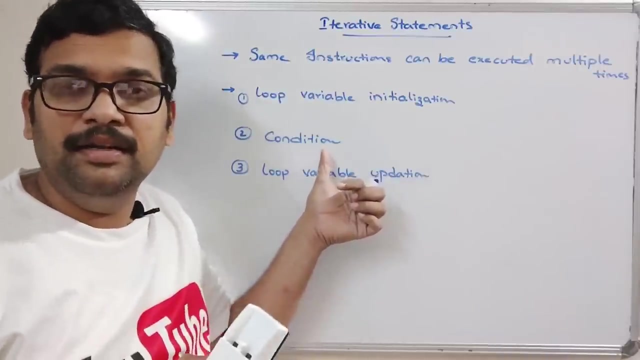 The third one condition. The third, one condition. The fourth, one condition: To do one loop variable updation. So we can, we have, we need to initialize one loop variable and then we have to write one condition. So this condition is meant for common rating, this execution, Okay So, 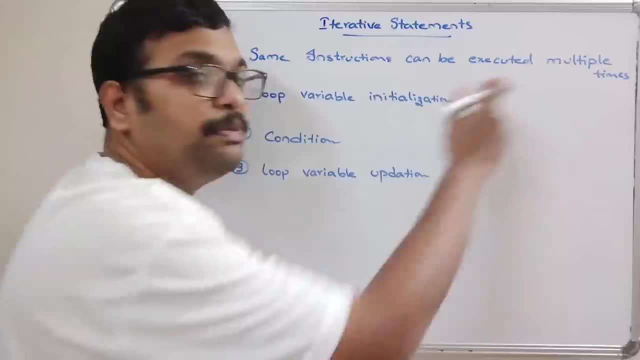 as we have discussed it now, the same instructions can be executed multiple times, So after some iterations we have to terminate it. That means what it does is it can be executed in multiple times. So that is how we can. 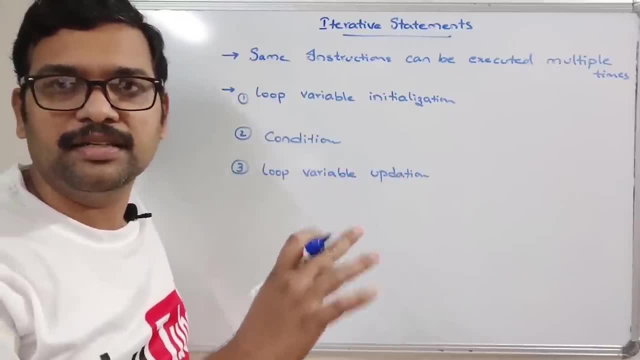 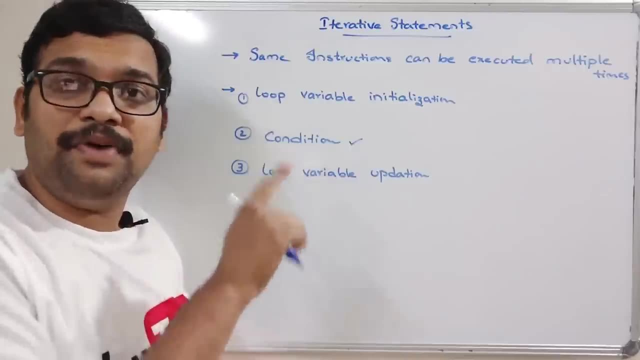 write these conditions. Okay, We can write the lotus root condition in the form of a loop means we have to stop executing the instructions for the termination. we'll write this condition so, unless i mean until the condition becomes false. okay, until the condition becomes false. 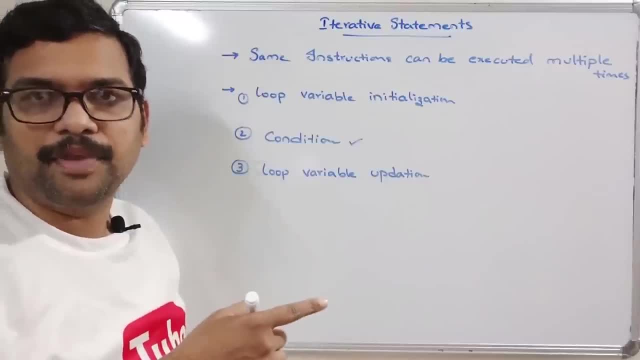 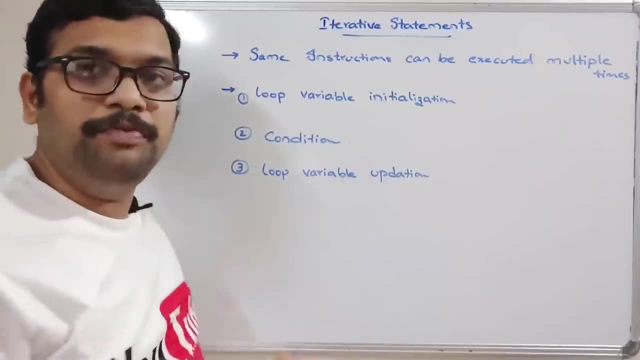 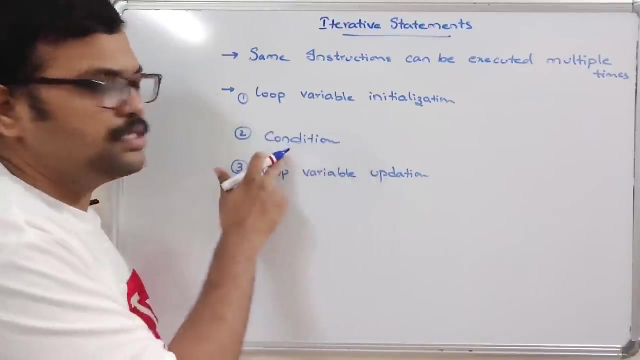 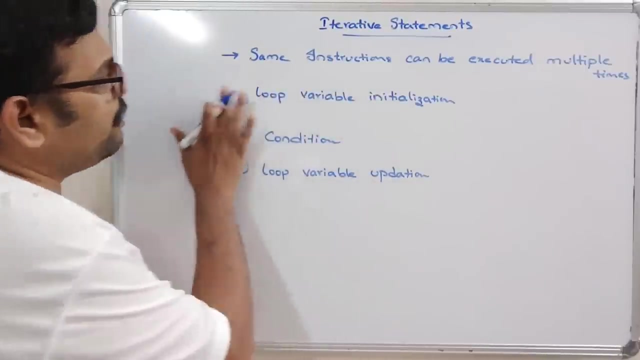 the instructions will be keep on executing, okay. so for termination we'll write some condition and for every iteration we need to update the loop variable. so we need to update the loop variable so that the at particular time the condition becomes false. so automatically the instructions will be stopped executing. right? so whatever the iterative statements we are using, we have to. 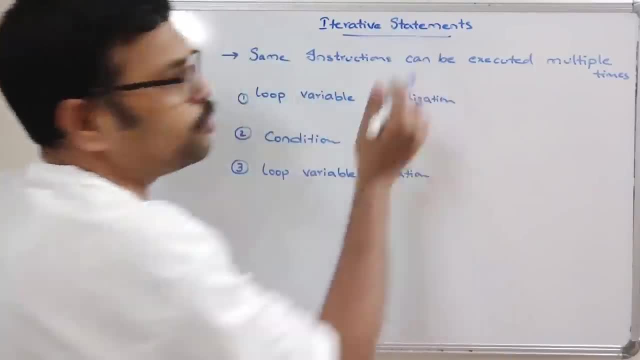 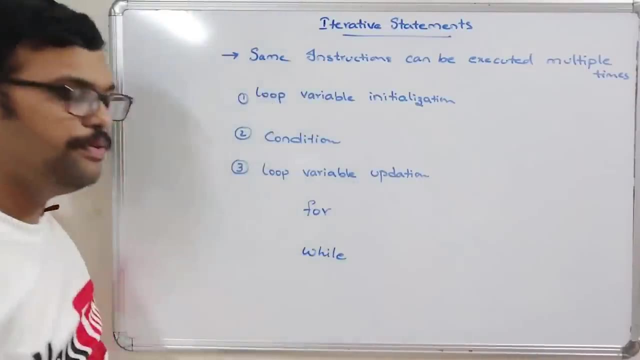 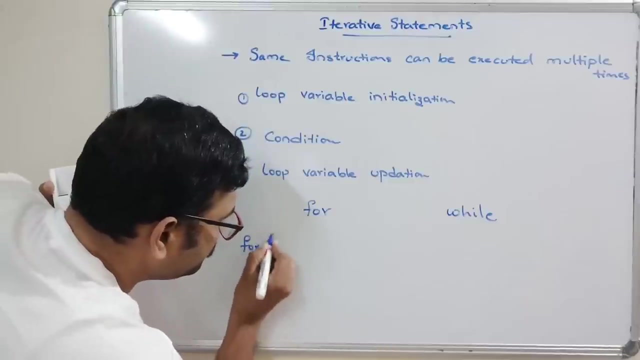 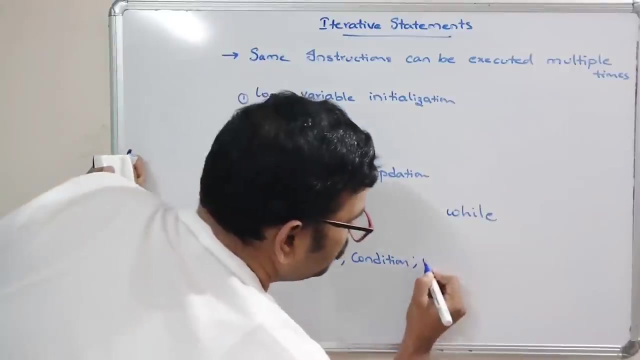 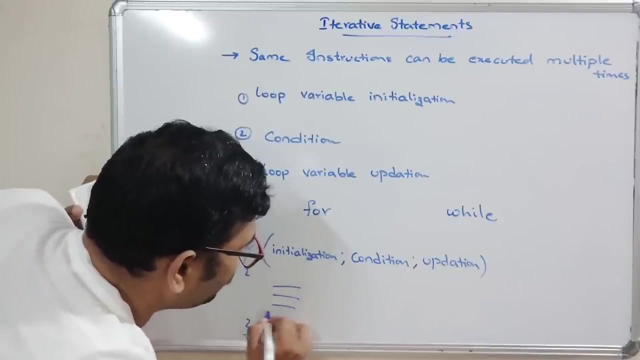 follow these three things. so there are mainly two iterative statements we are using, that is, a for and while, for and while. so, coming to the syntax for the for, for, for, go with the initialization, semicolon condition, semicolon updation, and open the block and close the block, and here we have to write the condition. 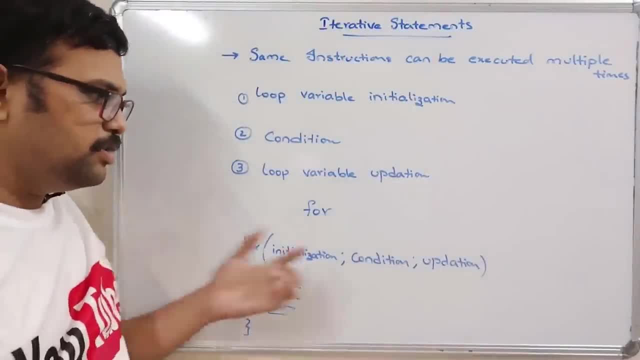 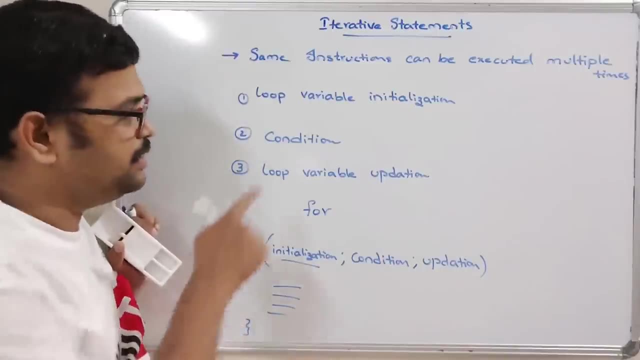 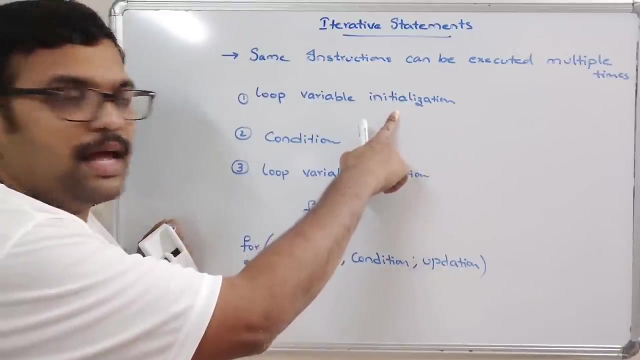 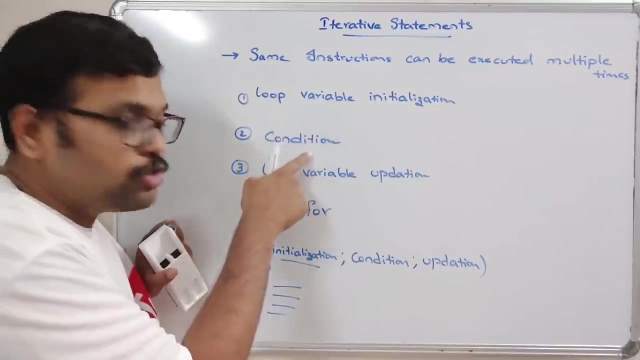 and statements. here we have to write the statements. so this is the syntax for, for. so this initialization will be executed only once. the initialization will be executed only once, that means in the first iteration, and immediately after initialization happens, the condition will be checked. so we have to check the condition. this is the second step. and if the condition becomes true, 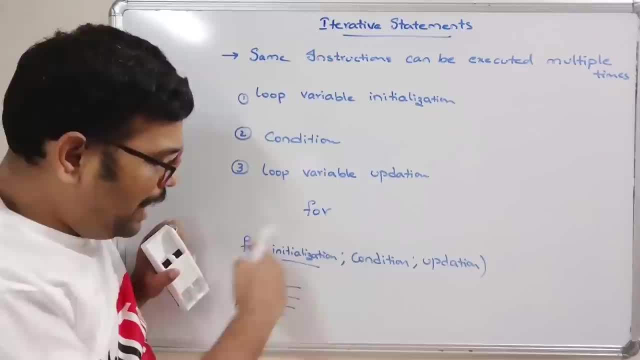 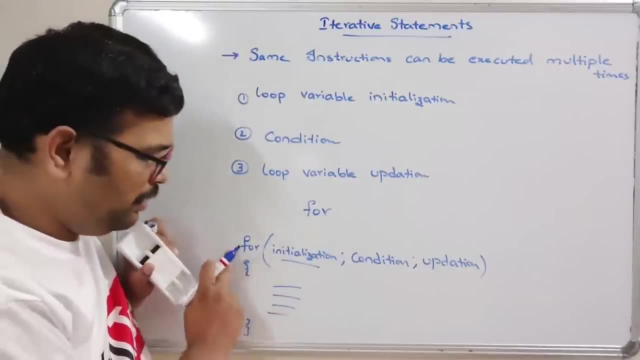 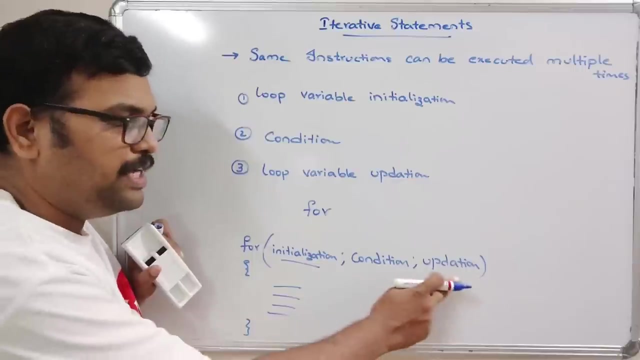 that means here: if the condition becomes true, the control will enter into this loop. okay, the control will enter into this loop and it start executing all these statements which are written in for and after completion of all these, after completion of executing all these statements, updation will be done. okay, updation will be done, and after updation again, it will check for the. 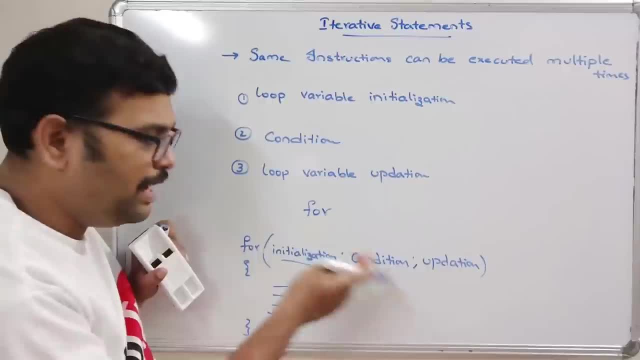 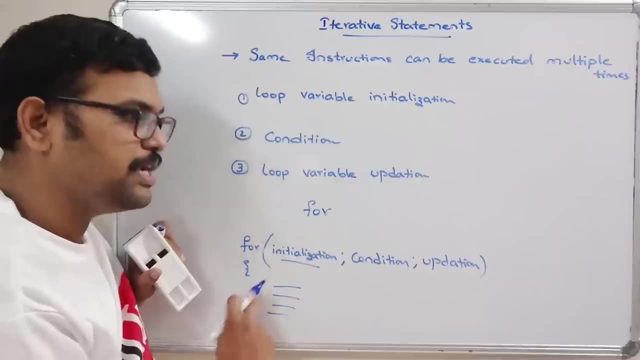 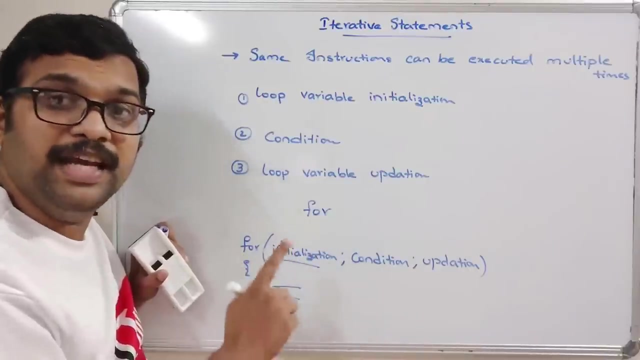 condition, whether it is true or false. if it is true, again the control will enter into the loop. it will start executing all the instructions. once it executed all the instructions, again updation will be done. and again condition: it will check for the condition. so this initialization will be executed only once at the beginning and then it will check for. 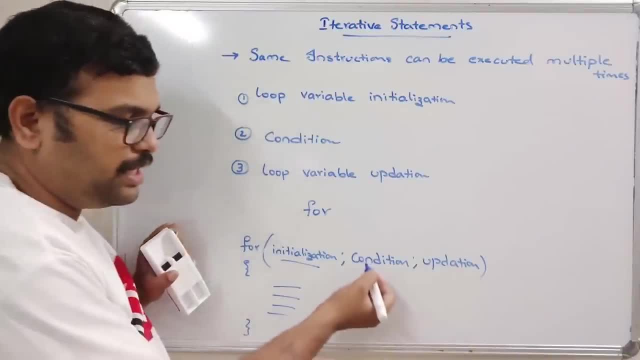 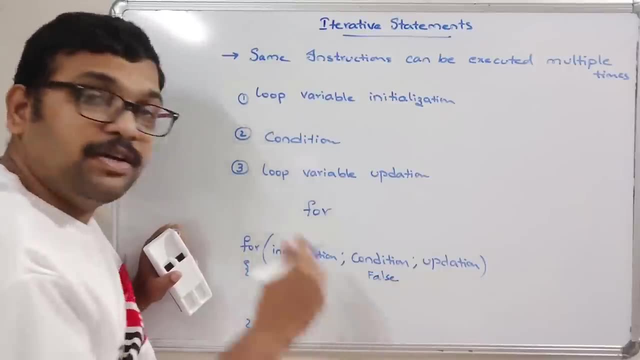 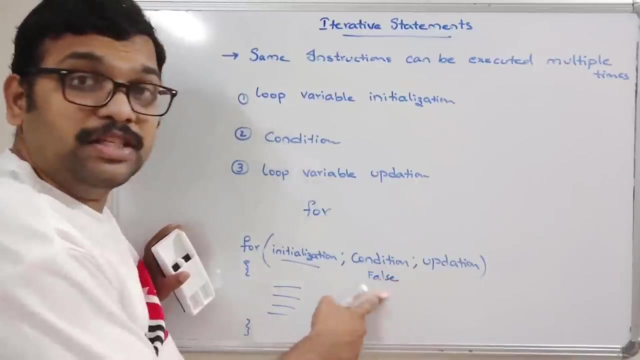 the condition. enter into the loop updation. again check the condition. enter into the loop updation. so this will be repeated until this condition becomes false. so at particular time, after some finite number of executions, finite number of iterations, so this condition becomes false. we have to write like this: so if the condition becomes true every time, so it will go with the JRT. 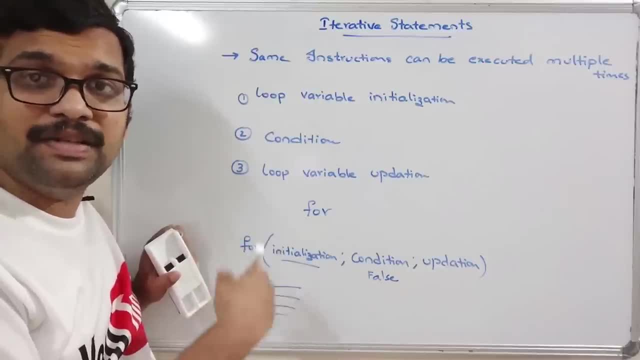 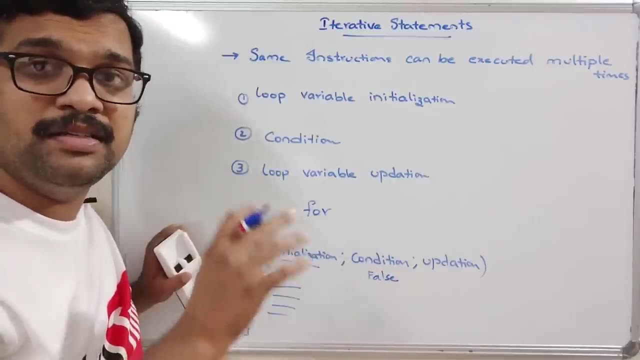 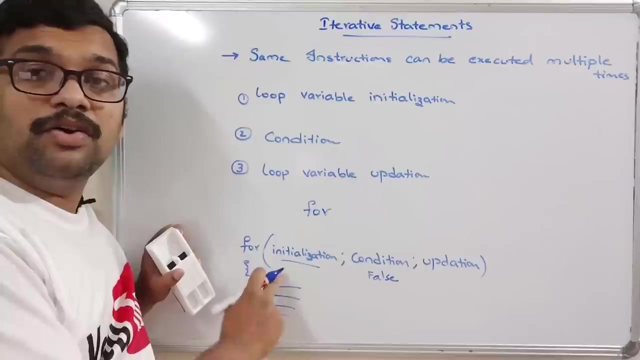 infinite loop. okay, it will go with the infinite loop. so you never stop executing these statements. so that's why we have to write the condition. so after some iterations, this condition becomes false. so whenever the condition becomes false, automatically the control will come out from the loop. the control come out from the loop. okay, it doesn't enter into the loop. so this: 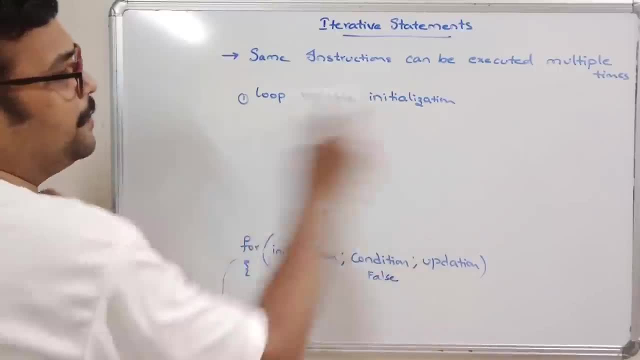 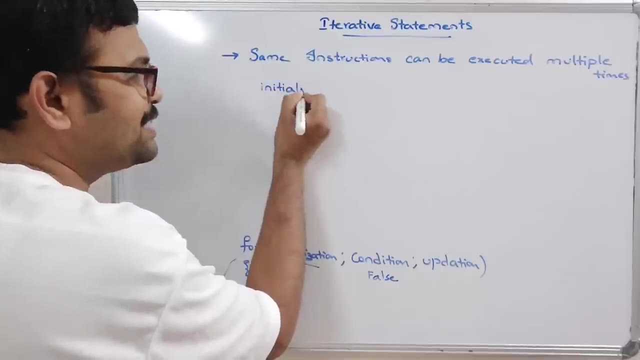 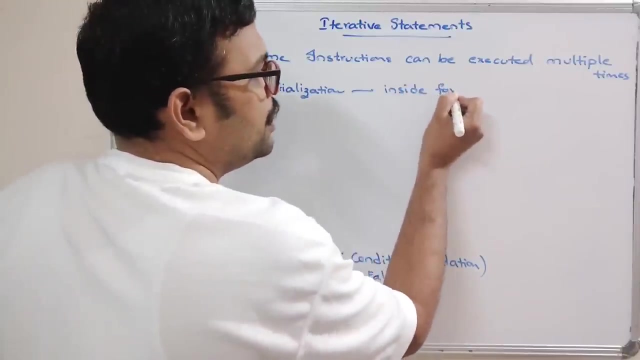 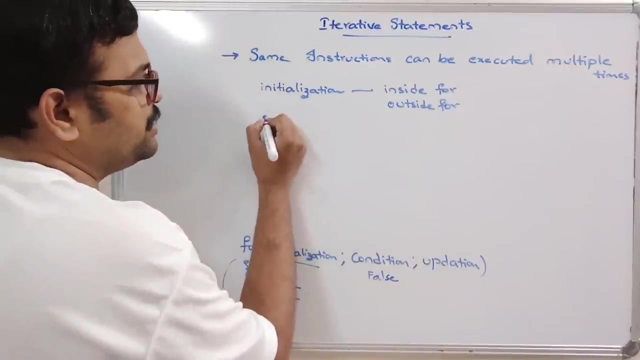 is the for loop and see, we need not follow the same syntax here. so we can also write the initialization out or inside, okay, initialization can be written inside for loop or outside for loop, inside for or outside for okay, and condition: similarly, condition condition can be given inside. 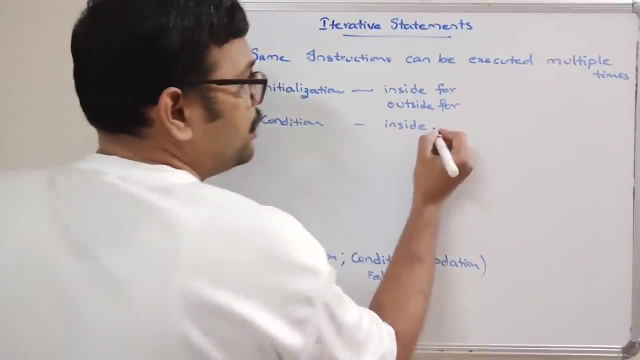 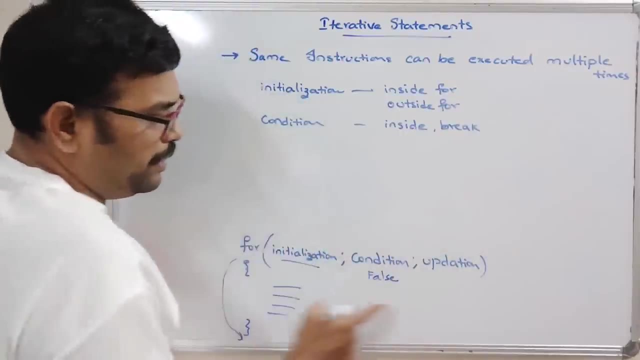 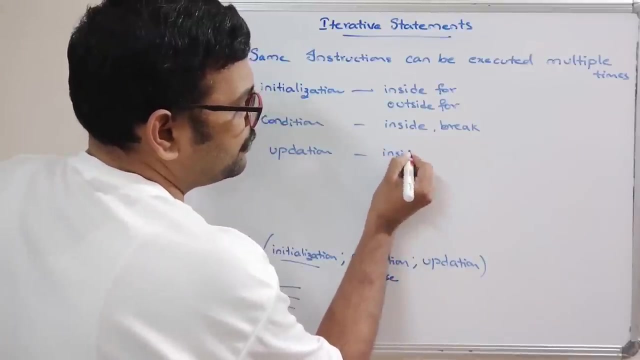 okay condition can be given inside with break, so we can use a break statement. okay, in order to terminate, we can write the break statement and then updation. so updation is also used inside, for inside for loop. okay, in the for loop or inside the for loop. similarly here: 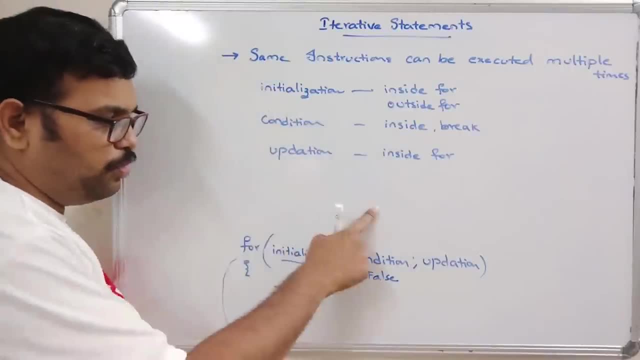 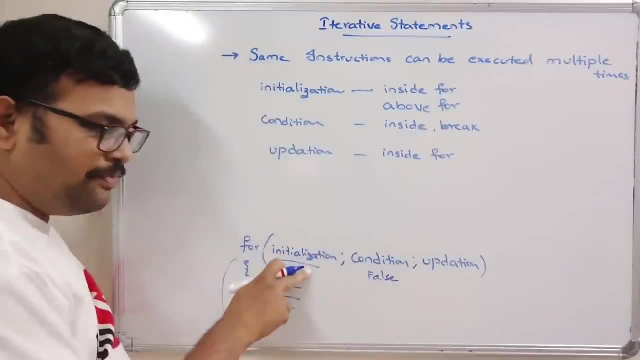 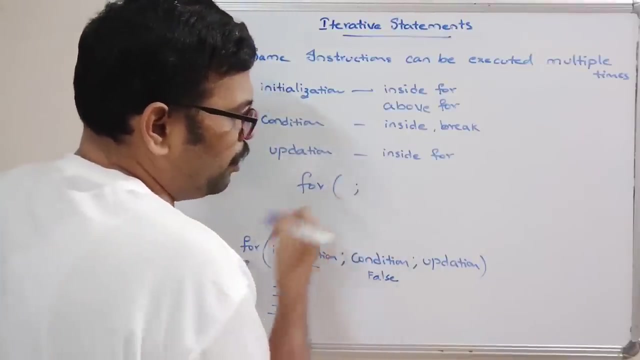 also, initialization can be done in outside the for loop. okay, outside means above the means, above the for loop. okay, above for loop or in the for loop or inside the for loop. okay, so here, like this, we can write for semicolon. so these two should be done. okay, two semicolons. 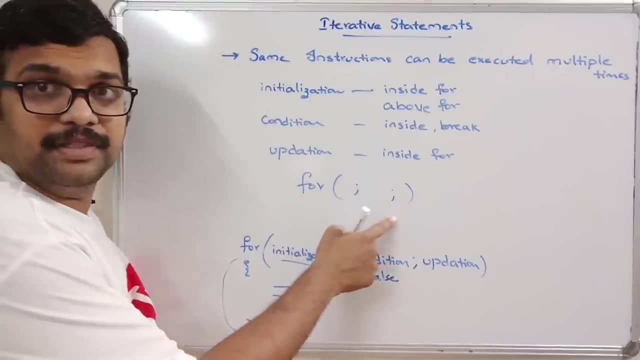 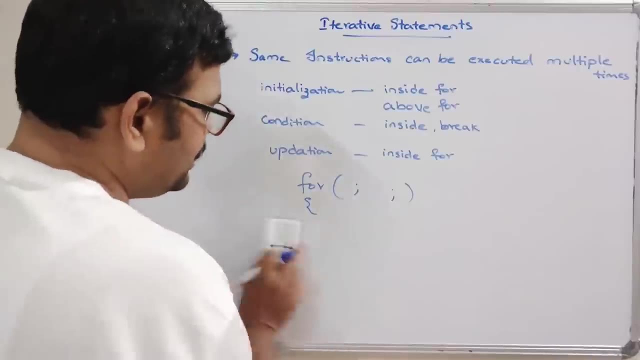 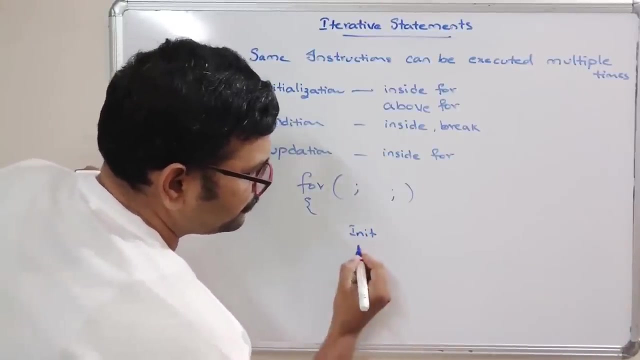 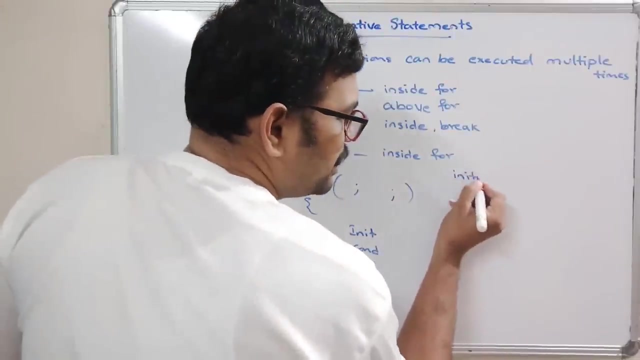 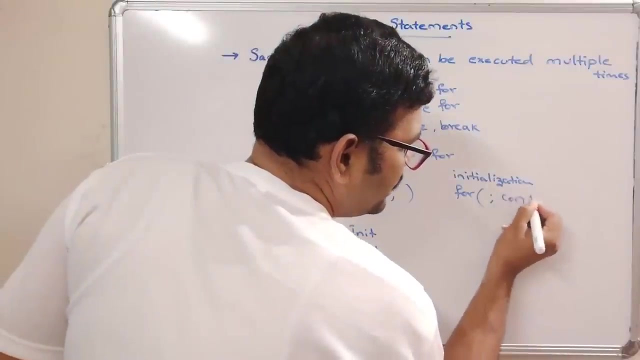 should be given here. okay, this is a syntax. this is a syntax and you can open the curly braces and you can write the initialization condition and updation here itself. so initialization- sorry- condition, updation here. this is also correct. or you can write the initialization here. use the for loop, write down the condition here. 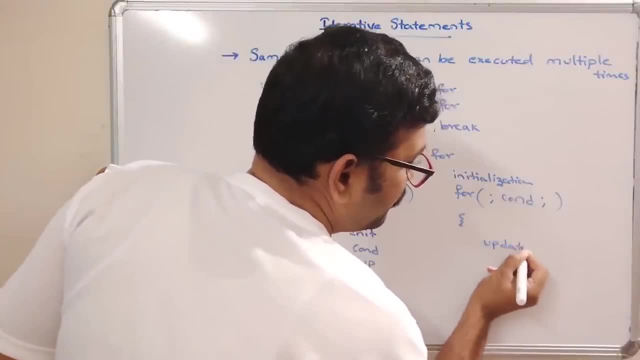 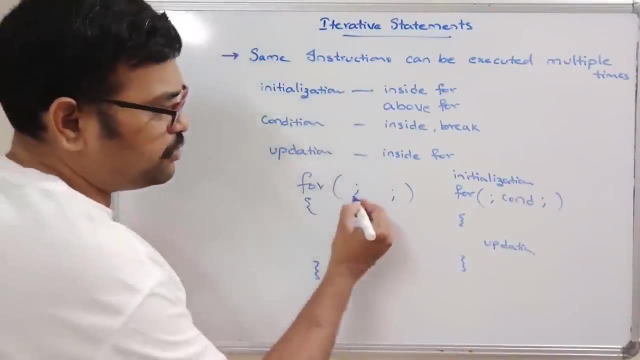 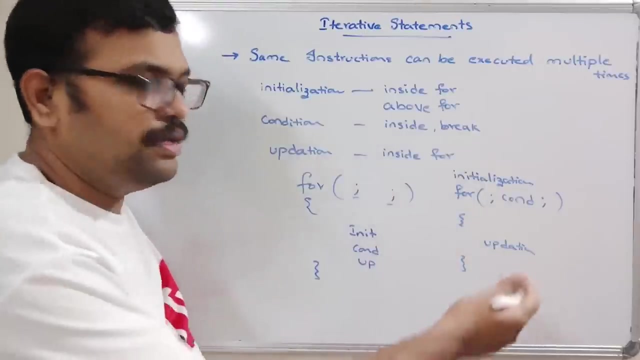 give the updation here. so this is also correct. okay, this is also correct syntax. so here the syntax is two columns separating the three things, that is, the initialization condition and updation. so these things can be written in number of cases. so i will execute a program showing all these cases, don't worry. 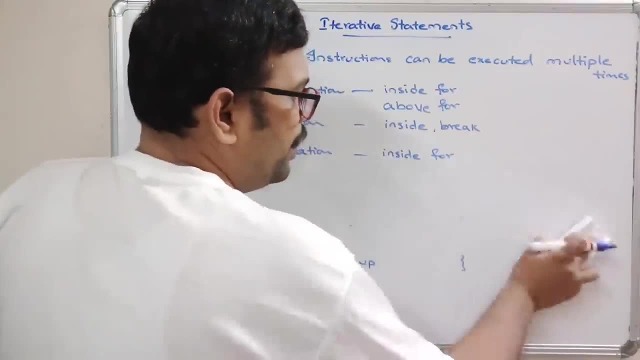 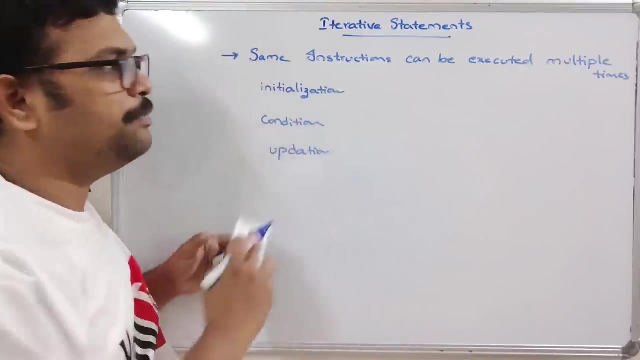 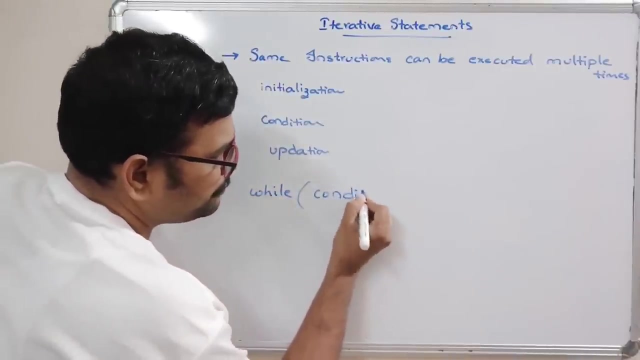 and we'll go with the while loop, while loop, so even the while loop. also, we have to follow these three, that is, initialization, condition and updation. so the syntax is correct. so we can write the initialization condition and updation. syntax is while, followed by the condition. 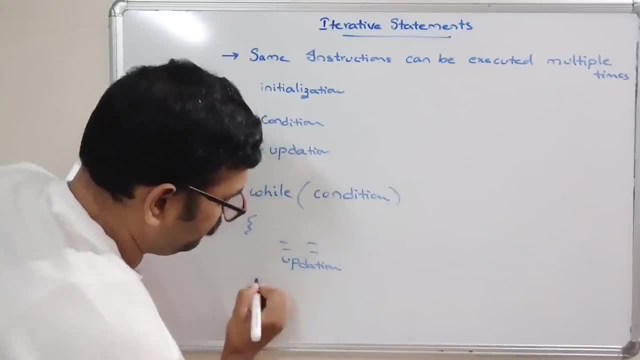 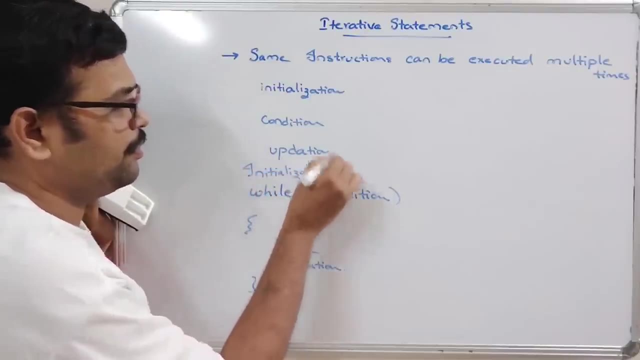 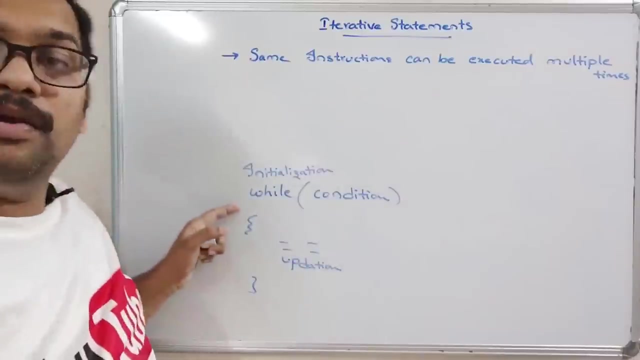 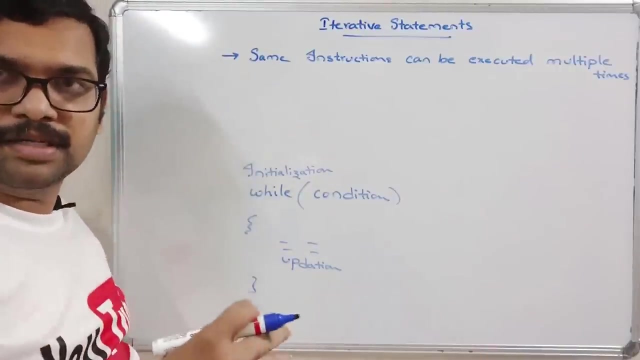 the statements and updation. so here we have to write the updation and here we have to go with the initialization. initialization. so this is the syntax for while loop. this is the syntax for while loop, okay, so just i will show you how to print the n numbers. okay, so i will go with the form i okay is. 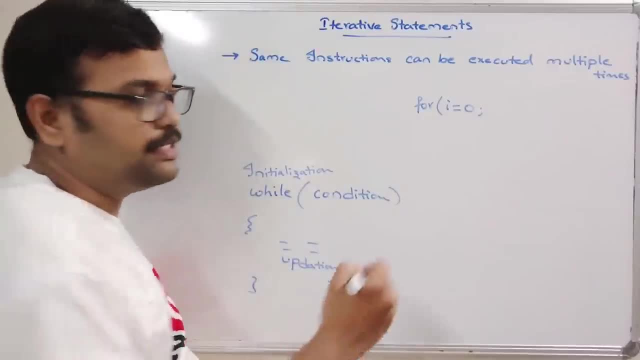 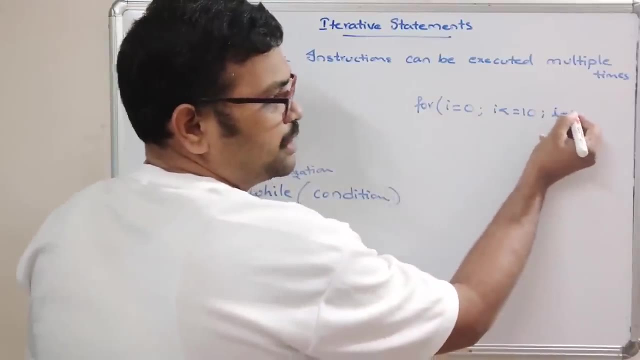 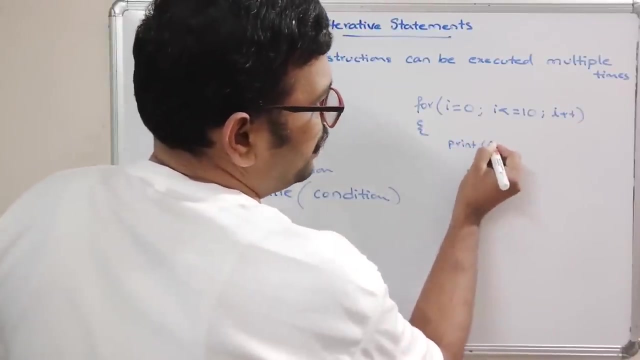 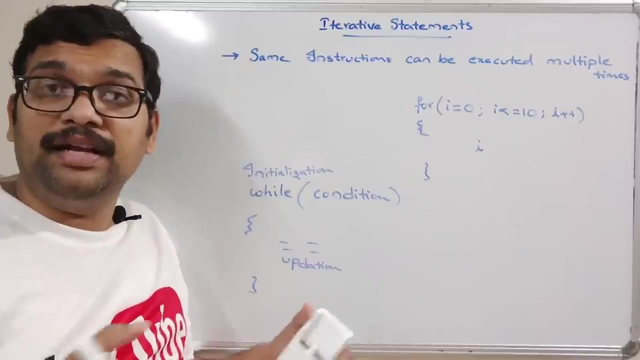 equal to zero, so i am giving some initialization. then i less than or equal to 10, condition i plus plus updation. go with here some print, i print i so in order to print i. so we have to go with the anyone that is, we are. we are having different ways to print the output. 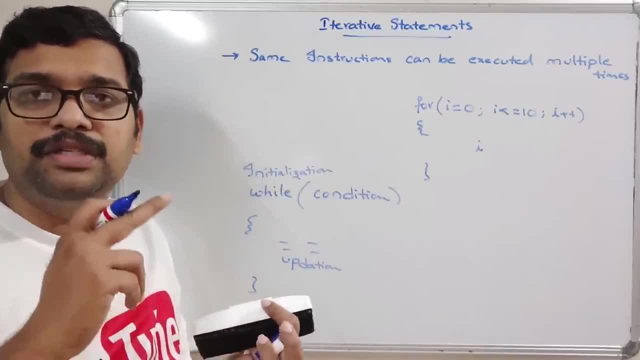 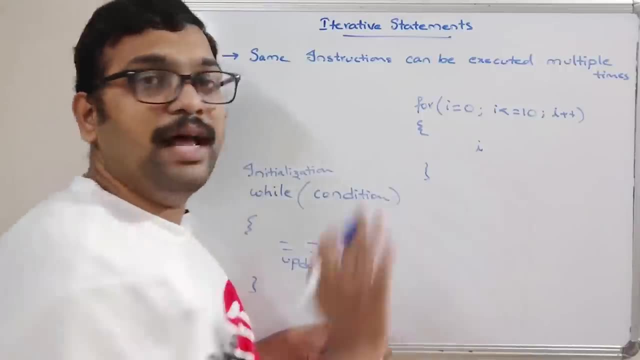 on the screen right. so we can use a inner html, we can use write ln or we can use a alert box. so whatever the thing we can use anyone among these three to print. i line so automatically for the first iteration i is zero. zero will be printed here in the second iteration, i. 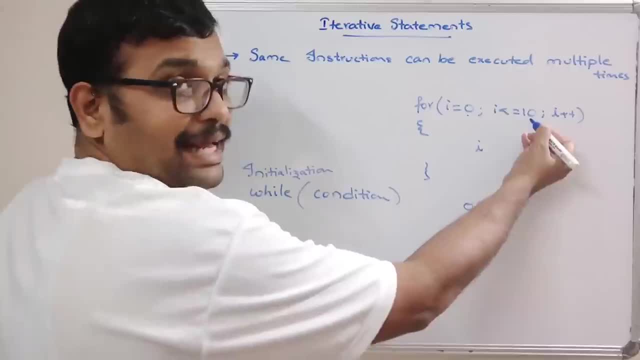 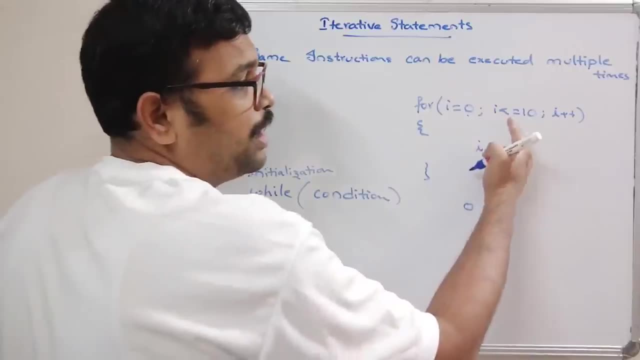 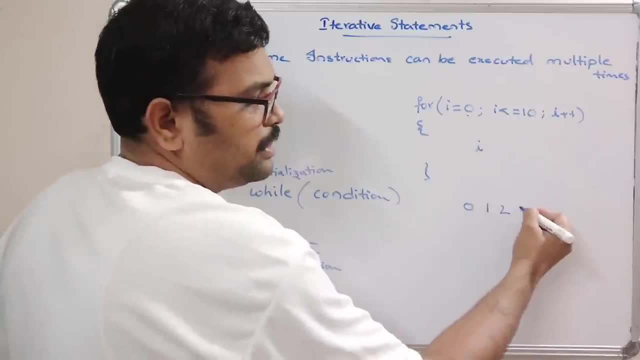 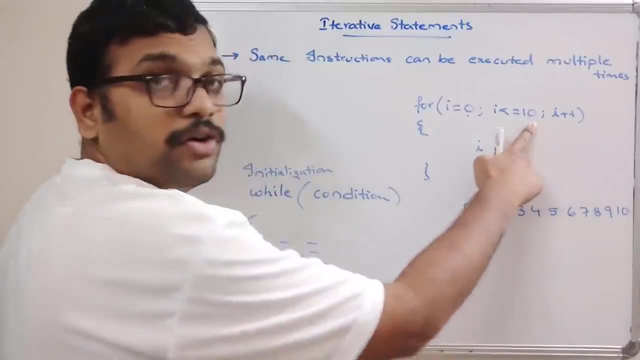 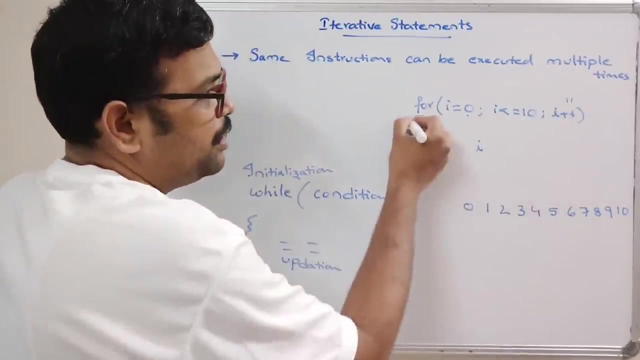 updation: two, two less than or equal to ten, three, four, five, six, seven, eight, nine and ten. ten less than or equal to ten. two, ten will be printed and updated. so eleven, eleven less than or equal to ten: false. so automatically the control come out from the loop, so like: 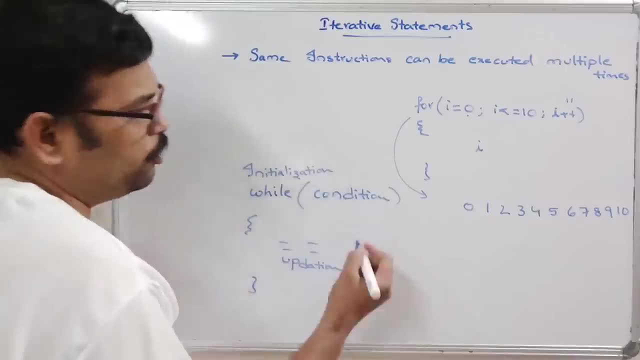 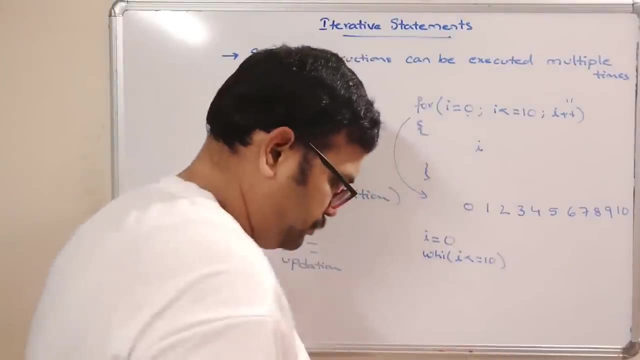 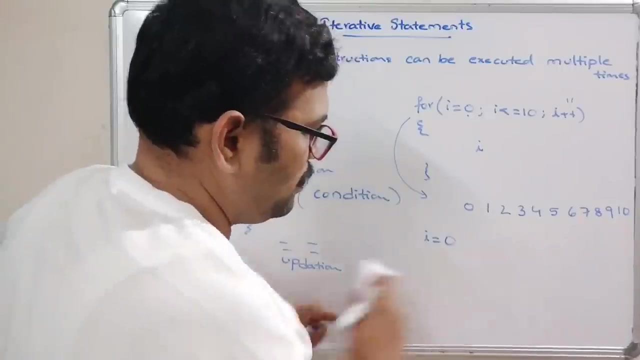 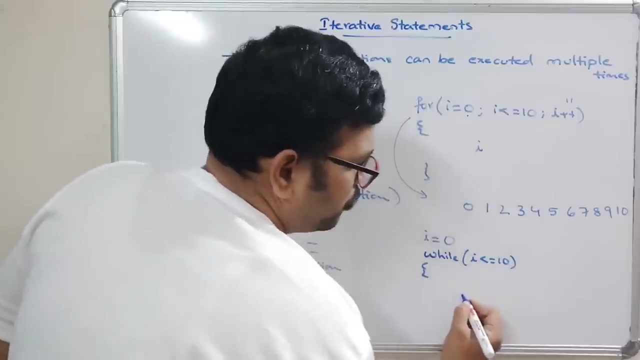 this: we can execute the n number, so we can execute the n number, so we can execute the formula similarly, while loop also. so go with the i is equal to zero, while i less than or equal to ten, while i less than or equal to ten, open and go the print i and i plus plus. okay, display. 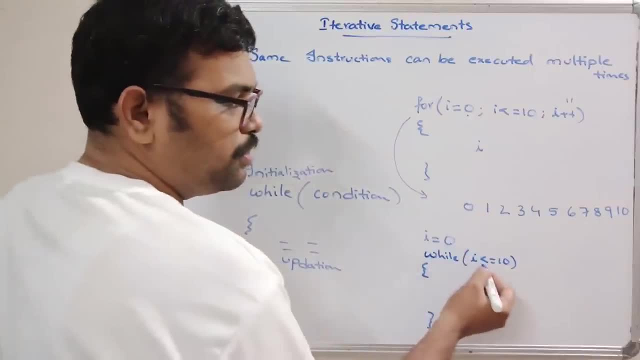 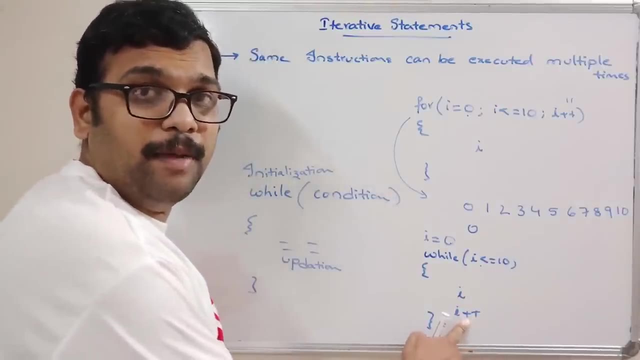 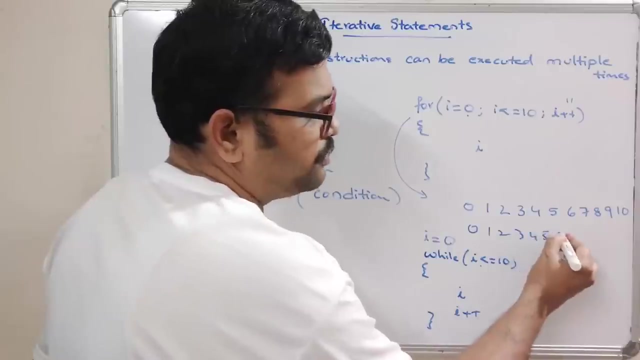 i, and i plus plus means updation, So immediately i is equal to zero, less than or equal to ten, print i, so automatically zero will be printed and updated. i plus plus means updation, so i will be updated to one. so one less than or equal to ten, so again two. one will be printed. two, three, four, five, six, seven. 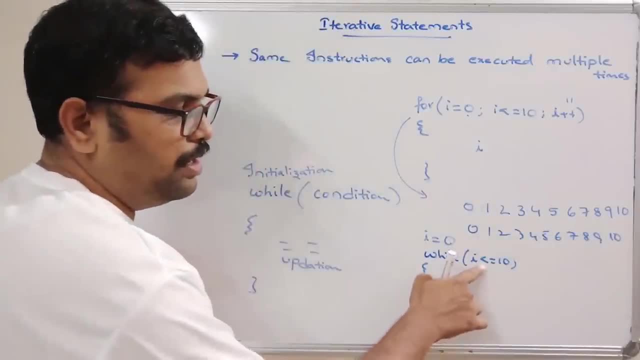 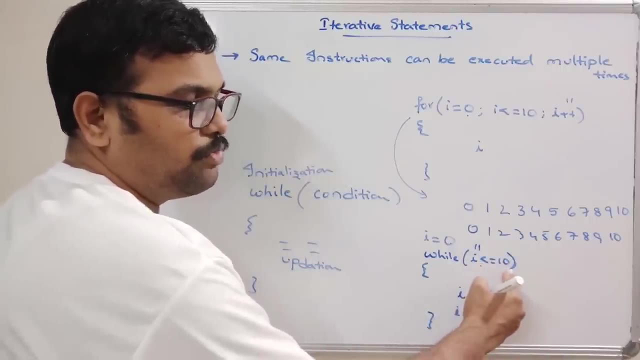 eight, nine, ten when i is equal to ten, ten less than or equal to ten, true ten will be printed and ten will be updated to eleven, and here eleven. i is equal to eleven, less than or equal to ten. it's a false. So automatically the control comes out. 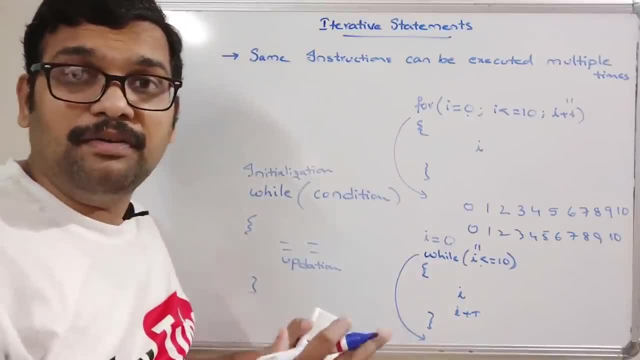 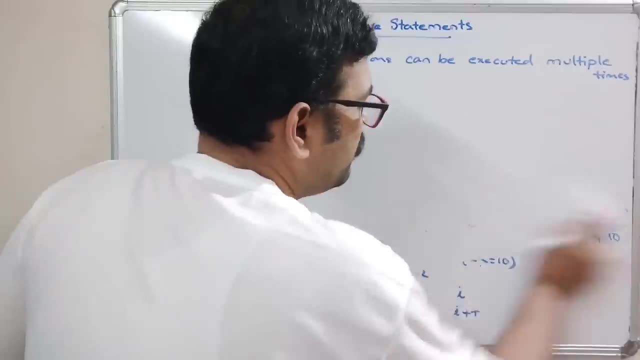 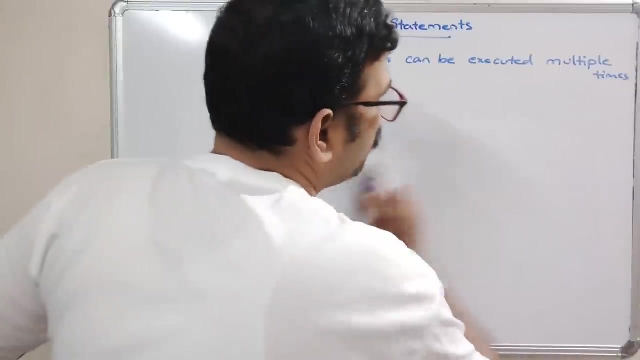 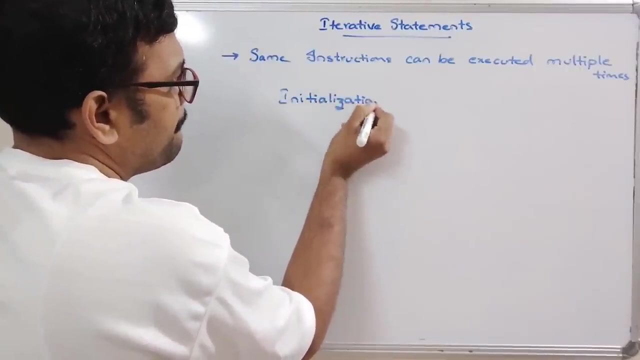 So it will come out from the loop. So this is how we can work with iterative statements like for and while. so just recalling the concept. So, whatever the iterative statements, that means either for loop or while loop. so whatever the iterative statements you are using, you need to follow the three things. that is initialization. 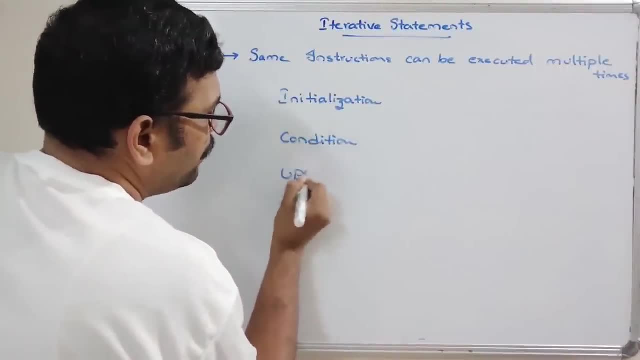 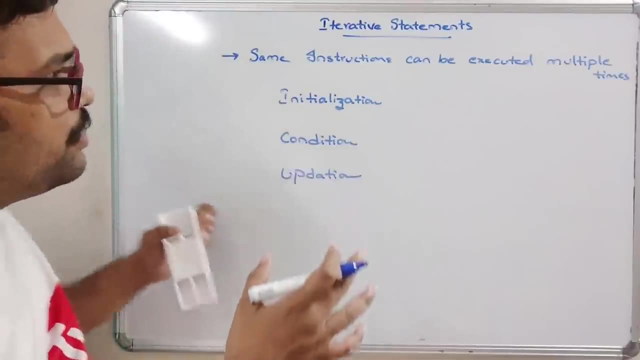 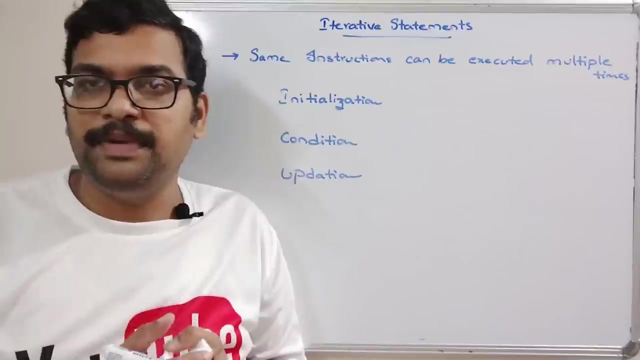 condition and updation. Okay, So these three are very, very important. these three are very, very important. So in this thing where we have discussed about the for loop and while loop, So i will demonstrate these two iterative statements by executing a small html code. 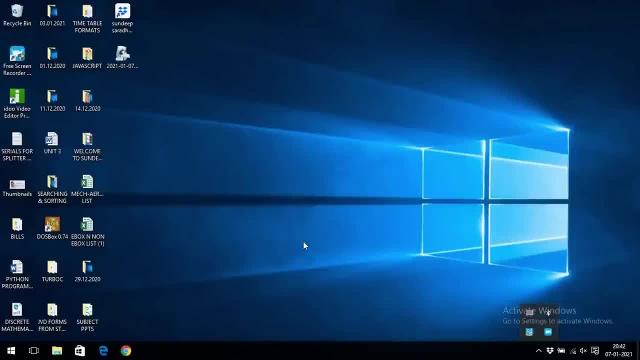 So let us move on to the screen, Hello friends. So just now we have seen the syntax for all the iterative statements, mainly for loop and while loop. So now i will show you the demonstration for this: for loop and while loop. So for that we will just start writing the html content. 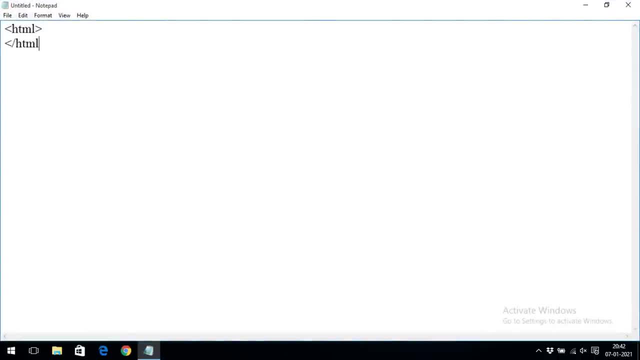 So let us start with the html tag. So in between the html tag we'll write the body and we can write the script inside the body itself. Okay, So first let us give a heading like iterative statements. So this is a heading We'll get. 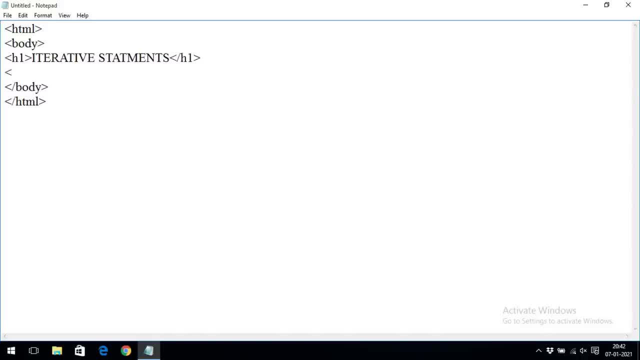 The page and we'll also write some paragraph, because where we have to display the output. So paragraph id is equal to a result. Okay, and close the paragraph. So in between, here we'll get the result, or simply we can go with the h2.. 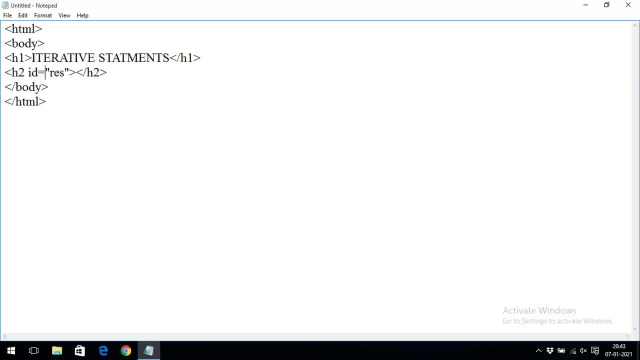 Right Now We'll write the script here. So inside the script we need to give the iterative statements. So we'll print the numbers n numbers, Some. for that. we'll first go with the for loop. First we have to initialize the value and i, less than or equal to 10, i++, and inside 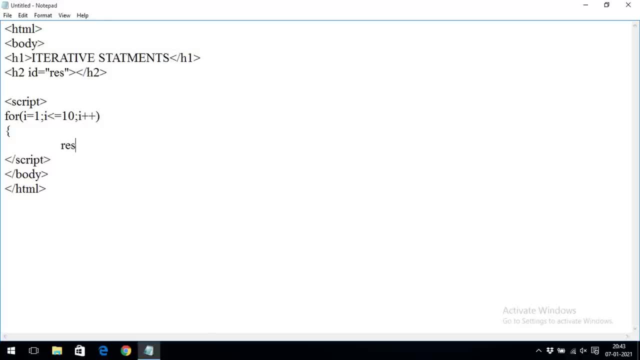 that we'll give some. result Is equal to: or directly we can print here or we'll give some here. result plus is equal to i plus space. So we'll give some space. Okay, For that we'll give some i using i value and similarly, result is equal to some empty string. 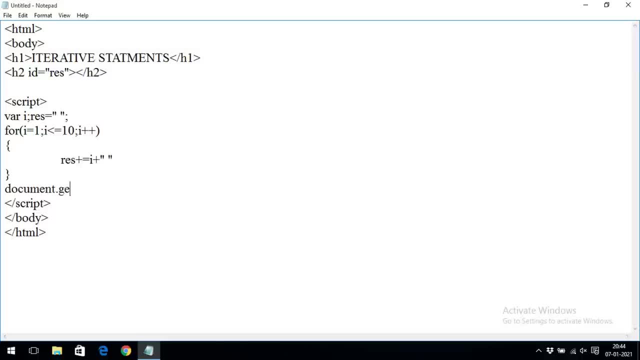 And after the for loop we'll print this one Document dot. Get element by id result. result is the id where we have to display the output. So inner html is equal to in the result. here it is. So now we'll print here: 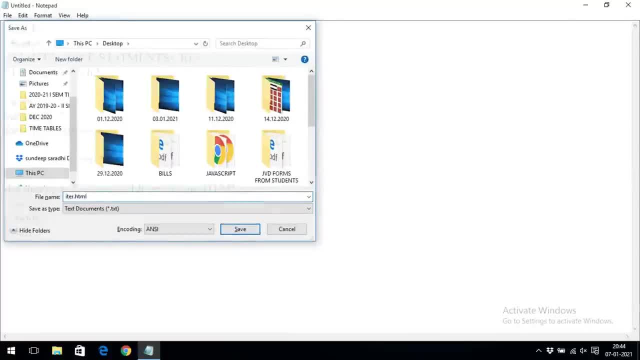 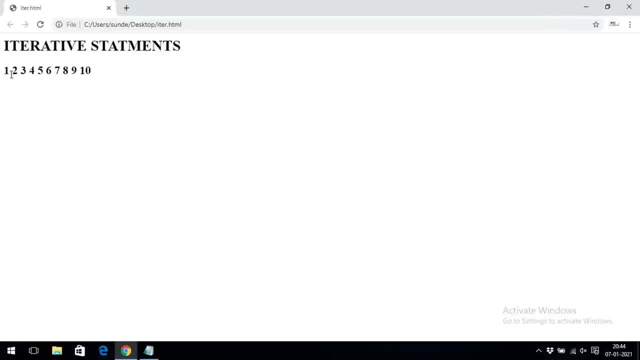 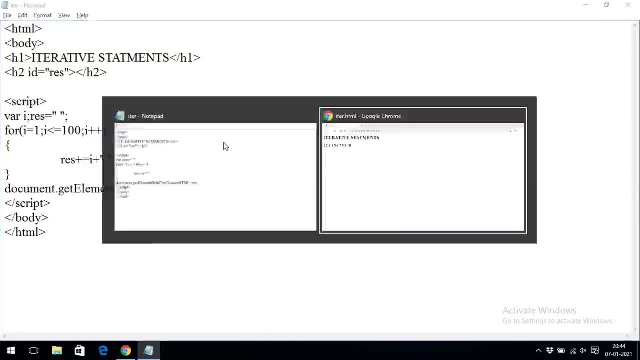 So I will save this one as iter dot html, and now we'll execute this file so that we'll get the result. See, you can observe here one, two, three, four, five, six, seven, eight, nine and ten Right. So if you place here hundred, we'll get the result with hundred, right? 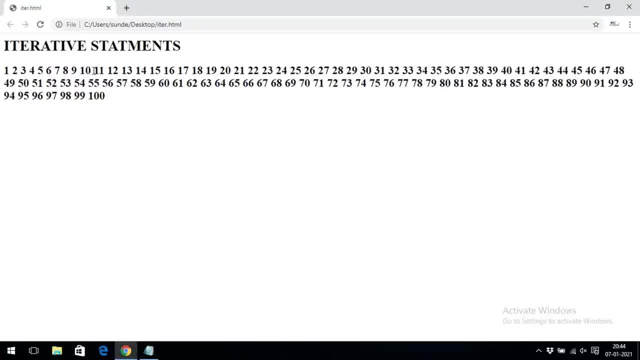 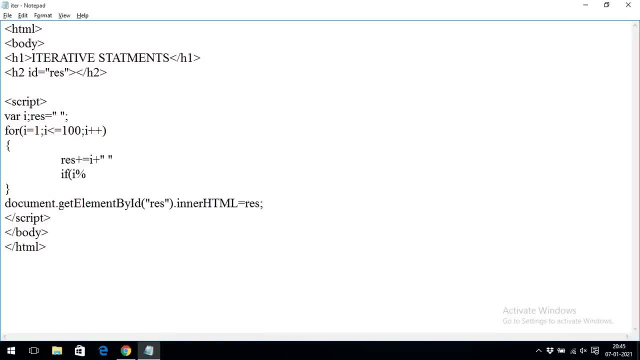 And if you want to divide each and each, I mean ten numbers in a row- we'll write some condition here. If i mod ten is equal, is equal to zero, then what we have to do We have to do: result plus is equal to br. br means break row. 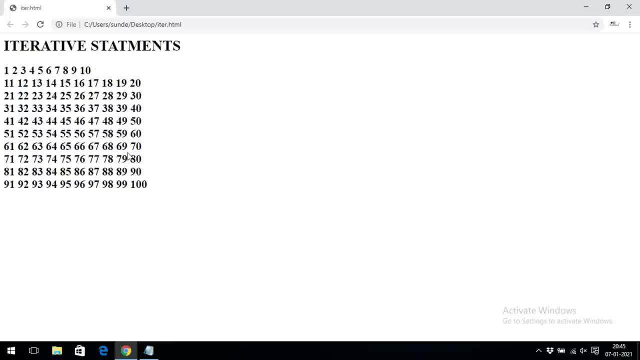 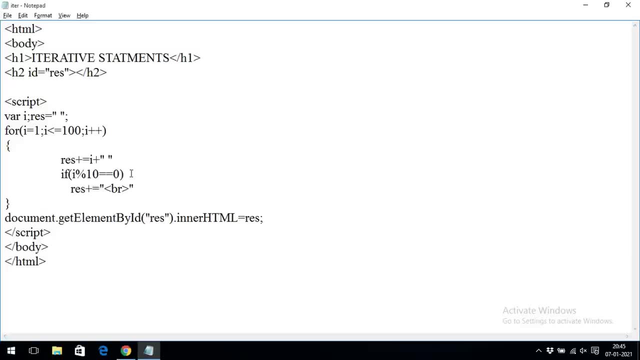 Right? Okay, You can observe here, right? So for every ten numbers we'll get, we'll start printing in the second line, right? So this is how we can demonstrate the for loop. So first, initialization condition and the updation. So for the first time the initialization will be done and immediately it will check for. 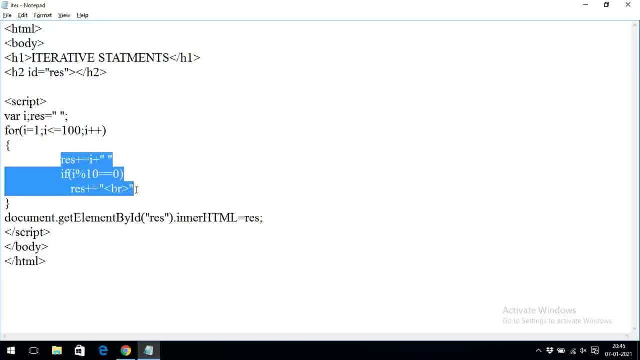 the condition. If the condition is true, then this complete body of the for loop will be executed and after executing this one Again, updation will be done. And after updation again, it will check for the condition. That means this initialization will be executed only one time. that's the only first time, right? 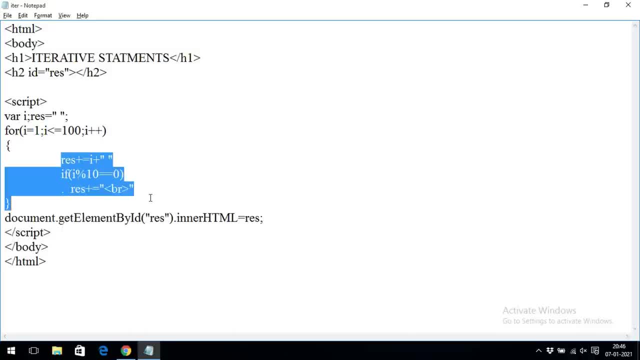 Next condition: if condition is true, it will enter into the loop. it will start executing all the statements into the in the for loop and after completion of this execution it will again update the loop variable and again check the condition. So this is the happens in the for loop. 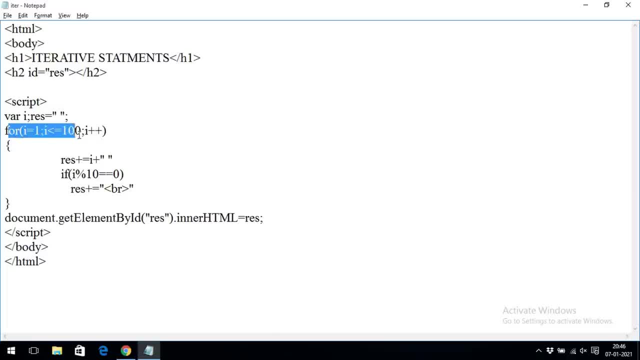 And now similarly just replace this for loop With a while loop. So in the while loop also we have to use a loop variable. So here we'll take some loop variable, as i will initialize the loop variable outside the loop, So I will initialize here and here. instead of writing all these things, we'll write simple. 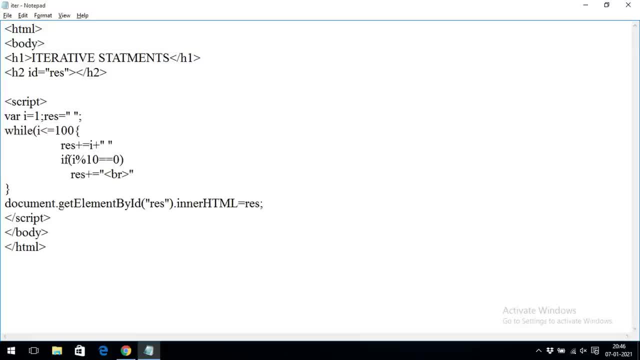 condition, while i less than or equal to 100. right, So updation. we need to updation. So we will update the variable. Right, We will inside the loop. We will update the loop Next. you can observe. the content is here, okay. 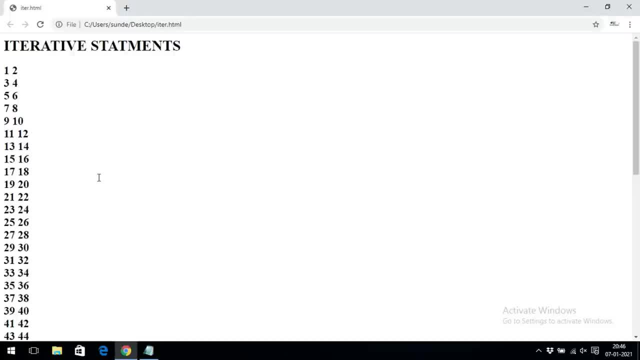 And also, if you go with the two, see, so for every mod two is equal to zero, we will get the break row. okay, After every even number, we will get the break row. So we can consider the first line as a odd numbers and the second line as an even numbers. 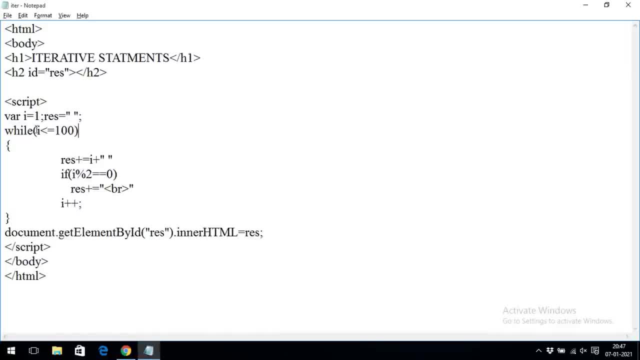 right. So this is how we can use the while loop. So, whatever the iterative statement we are using, first we need to have one loop, variable initialization, and then the condition and then the updation. So in for loop, in for loop syntax, we are taking all the things in the single line. okay, separated. 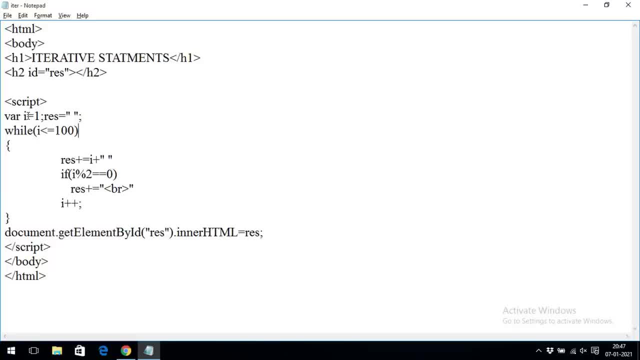 with the semicolon initialization, semicolon condition, semicolon updation. But coming to the while loop, we can initialize the value outside and we can. we have to write the condition And we can update the value inside, even in for loop. also we can write the initialization. 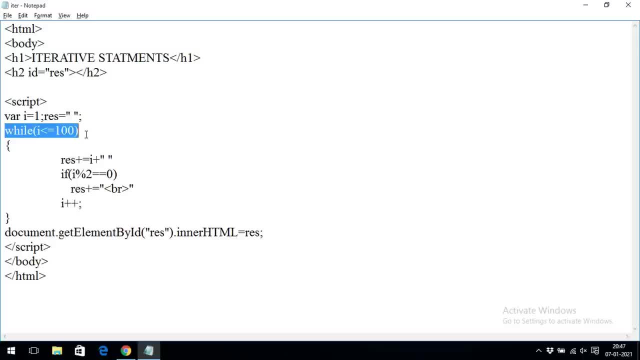 outside and updation inside. okay, So let us check for that. So for, and this syntax is should be followed: right semicolon and i less than or equal to hundred column close. see till we are getting the same output, we will change this one. So I am taking again i mod 10.. 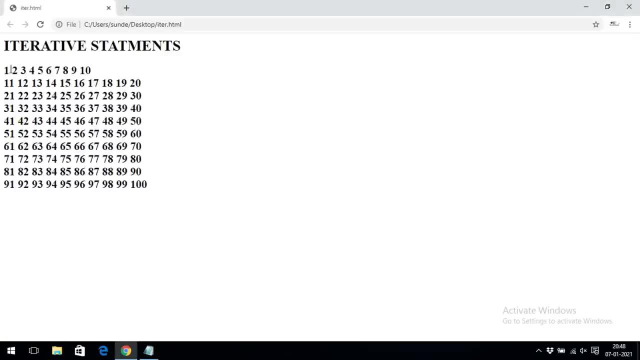 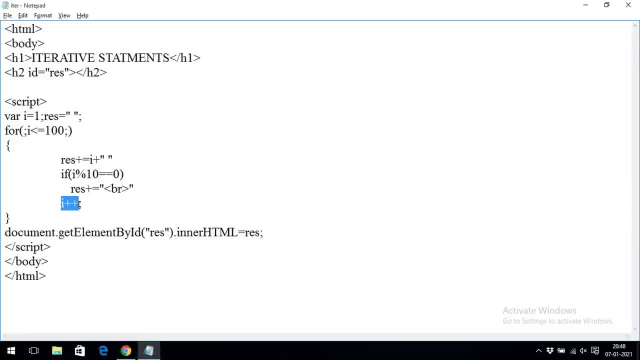 So that 10 numbers will be printed in a single line. So you can observe here that change. there is no change. but here we are using the initialization outside the for loop, updation outside inside the for loop. okay, Here we are not using all the three statements, we are using only condition. but we have to. 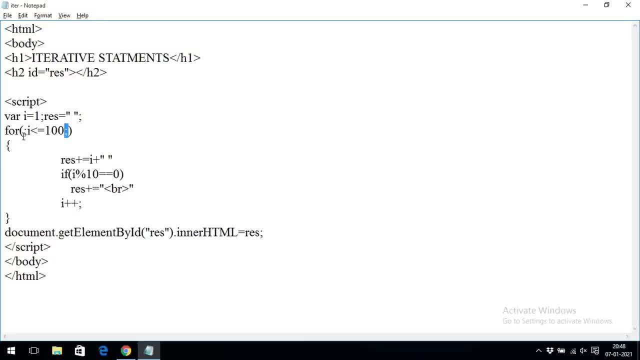 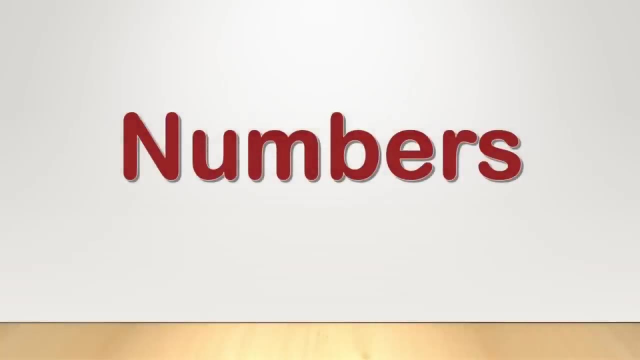 separate with the semicolon. two semicolons must be there. okay, So two semicolons must be there, right? So this is how we can use the iterative statements. That is a for loop And while loop. So hope you understood this one. 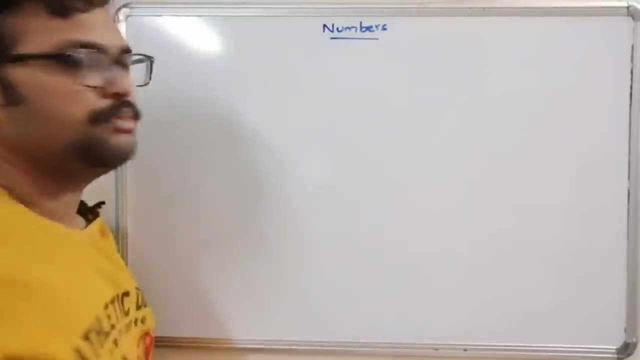 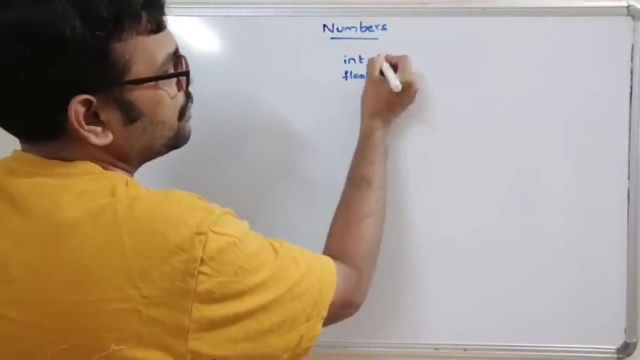 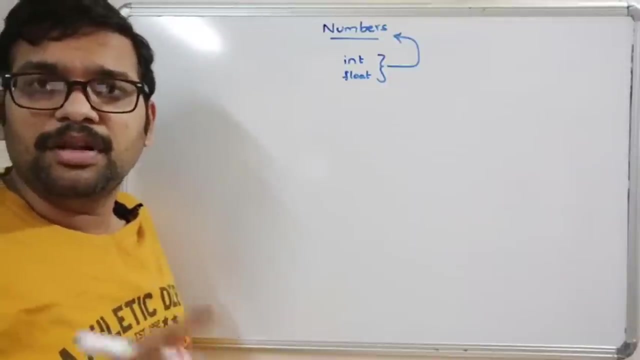 Now coming to this numbers. So what comes under this numbers? So in JavaScript we can have the integer and a float, Okay. so whatever it may be, that can be treated as a numbers. So in other programming languages, if you want to declare a variable, we should declare those. 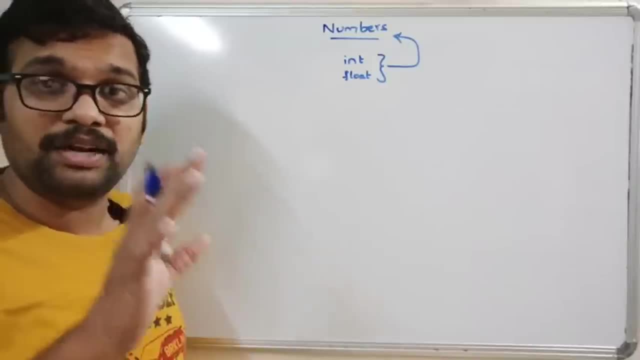 variables with the help of a data type. So in other programming languages, if you want to declare a variable, we should declare those variables with the help of a data type. That means what, whatever the data we are supposed to store into that variable, we have to declare. 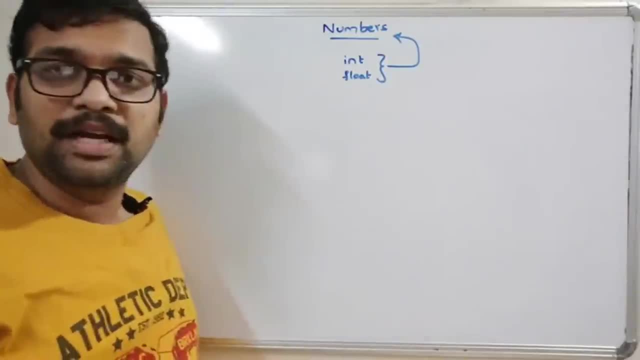 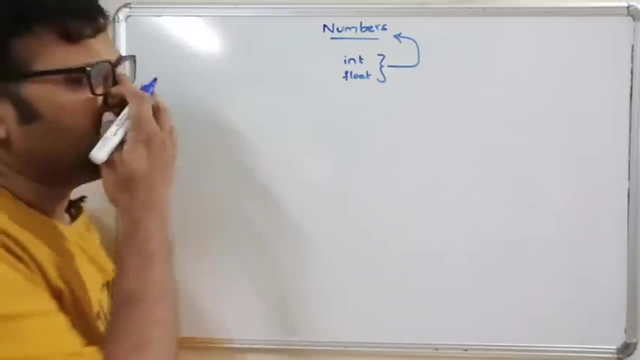 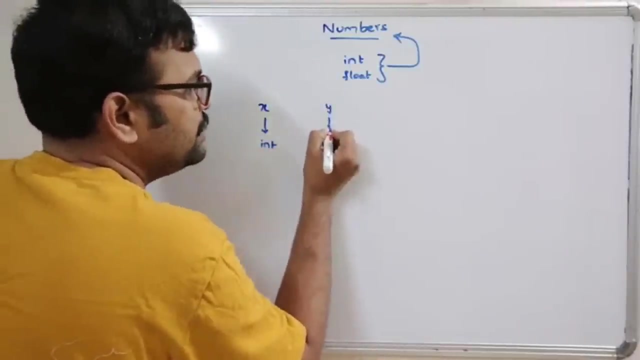 that variable with that particular data type. But here in JavaScript that doesn't require. So irrespective of the data type, we can declare a variable and we can initialize the values. For example, let us take some: x is an integer, y is a float, z is a string. 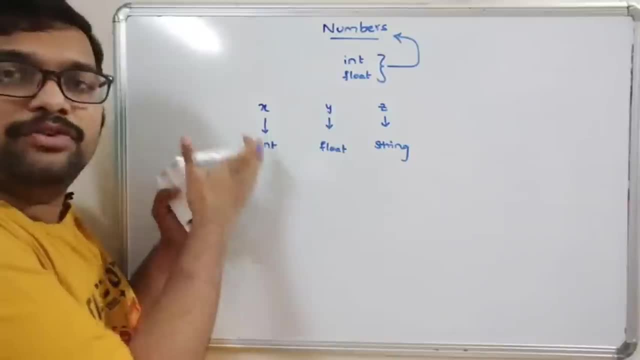 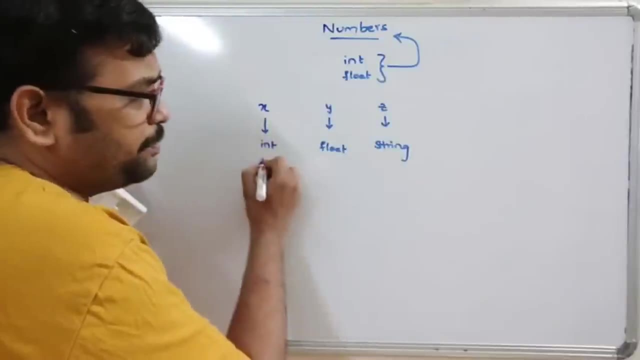 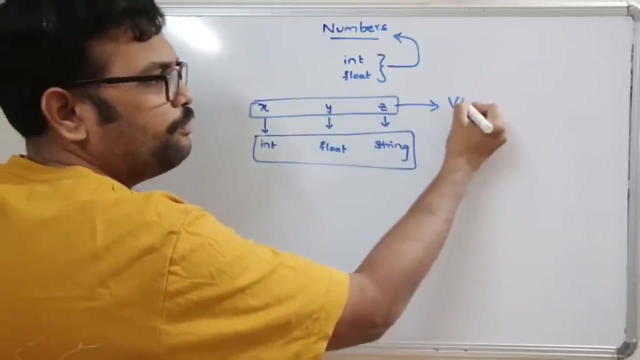 Okay, Okay. So we want to store some integer value in x, float value in y, string string in z. So, irrespective of these data type, irrespective of these data types, we have to declare these variables, These variables, with the help of var, var, keyword, right. 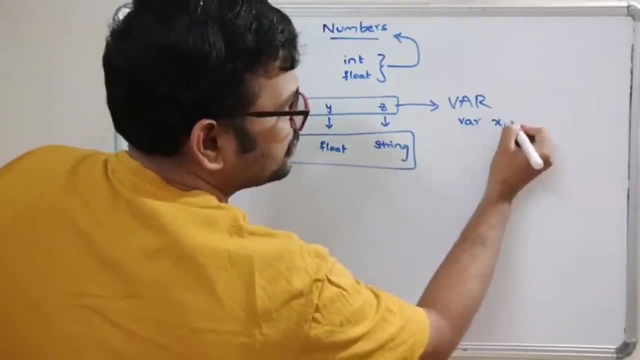 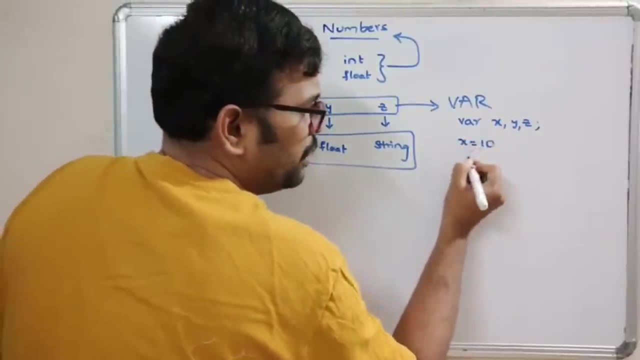 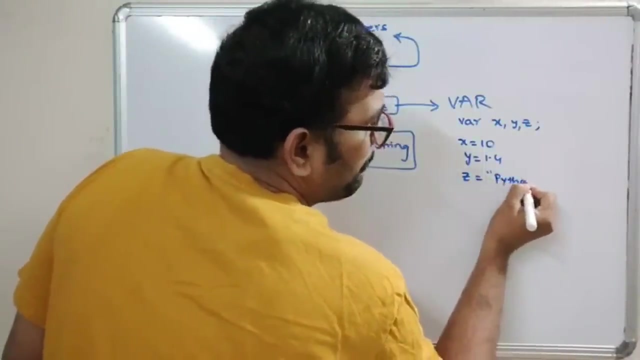 So, with the help of var keyword x, comma, y, comma z and later, we can initialize the value. That means some x is equal to 10.. y is equal to 1.4, z is equal to some phython right. So like this we can initialize the values. we need not bother about the data types. 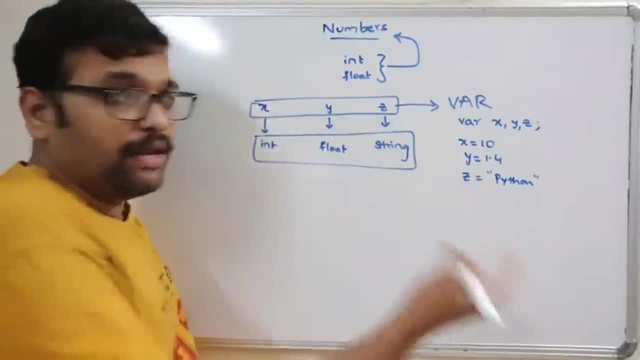 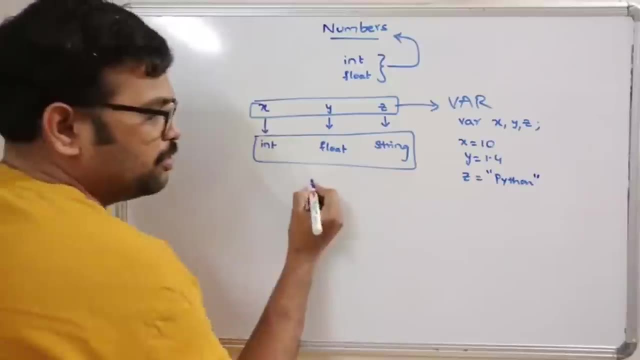 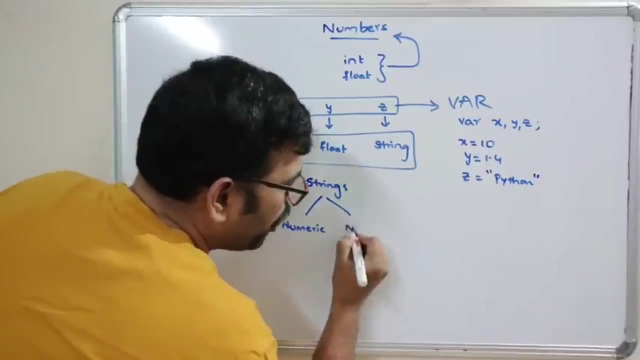 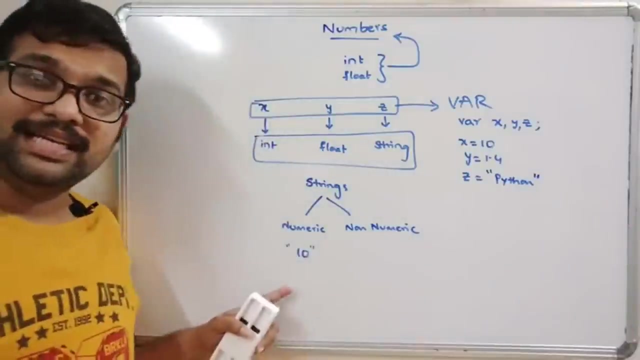 And see one thing we have to remember: if we, if we are saving some string to the variable, we have to enclose that in double quotations. So strings can be of two things: One is a string and a non-numeric. non-numeric, for example, n enclosed in double quotations. 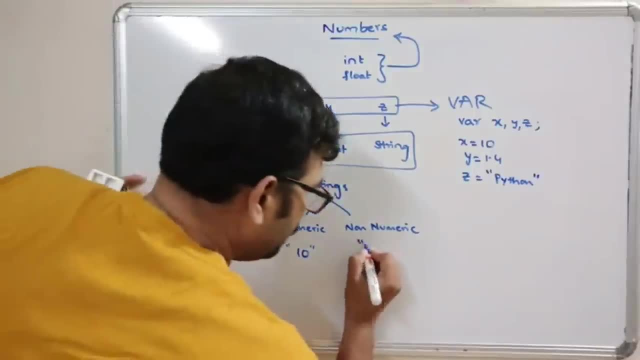 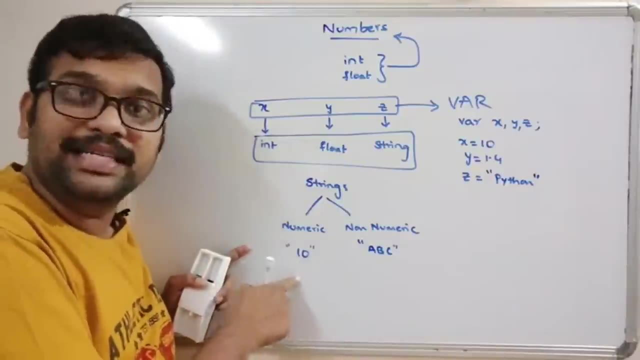 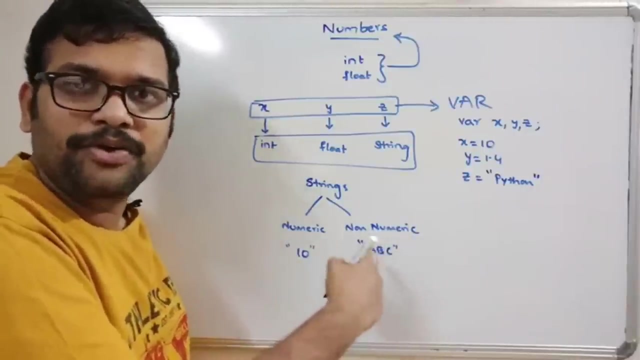 is a, 1, 0, okay, this is a string, and some a, b, c, that means this is a non-numeric string- okay, both are strings, but here we are having the digits, so that's why we call it as numeric strings, and here we are not having the digits, so that's why we call it as a non-numeric. 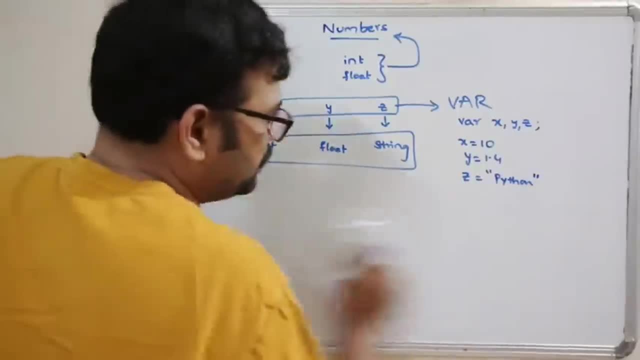 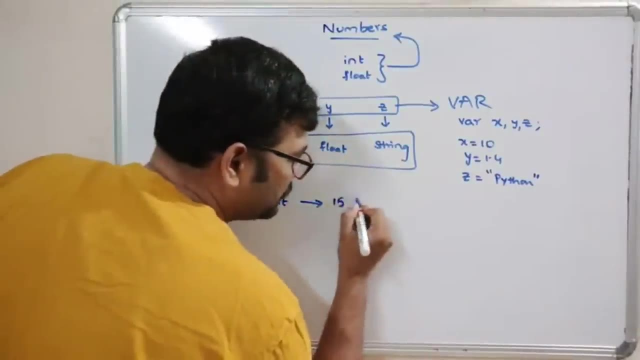 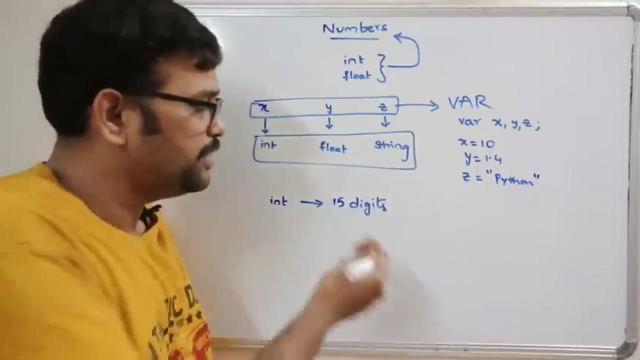 strings right, See. Now coming to the numbers, the integer. the integer will be having the accuracy till 15 digits. 15 digits, So if the number with the 16 digits, where, if you give, initialize a value with the 16 digits, automatically the accuracy will be lost. 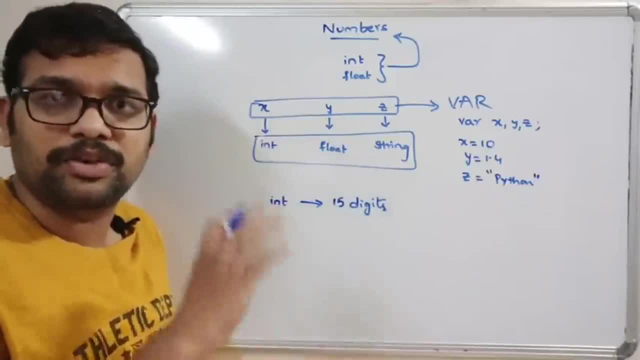 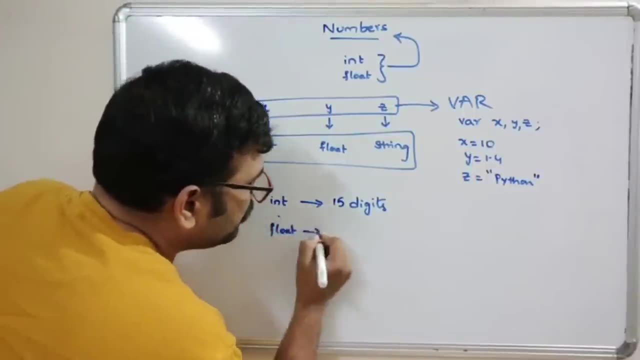 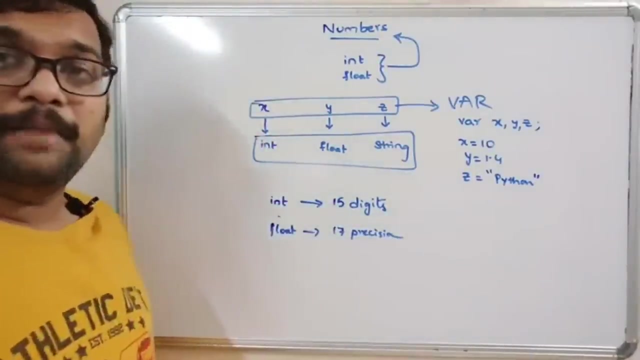 So I will show you the example on the system so that you will be understanding right. So integer will accept up to 15 digits only. And then, coming to the float, Okay, It will give the accuracy till 17 precisions. 17 precisions, okay, but usually the float doesn't. 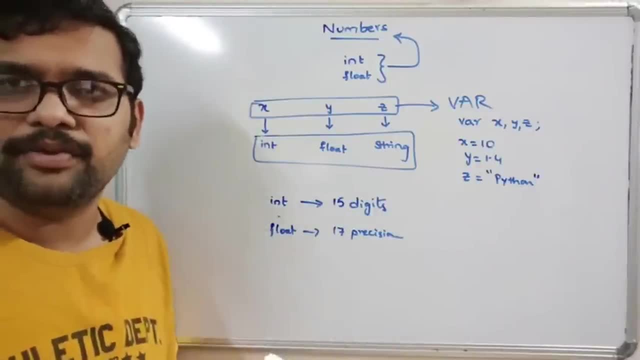 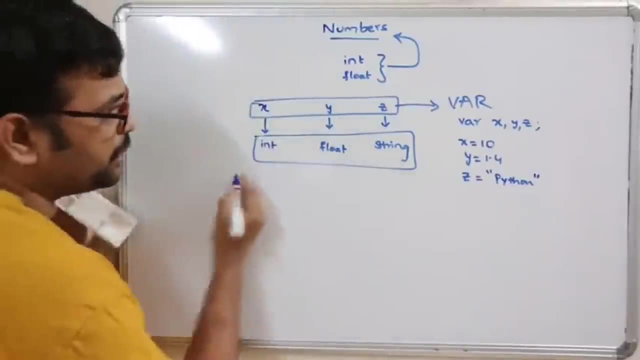 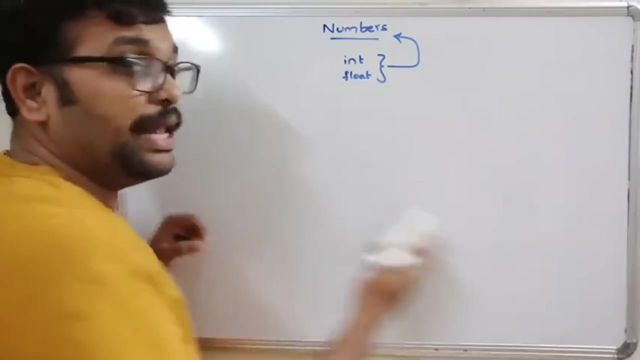 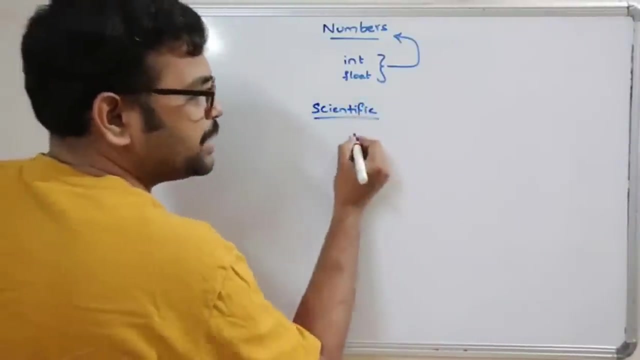 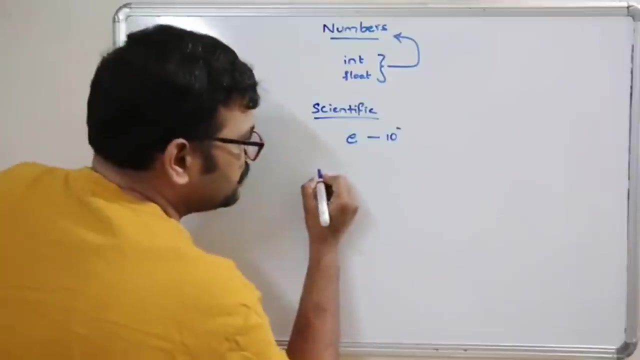 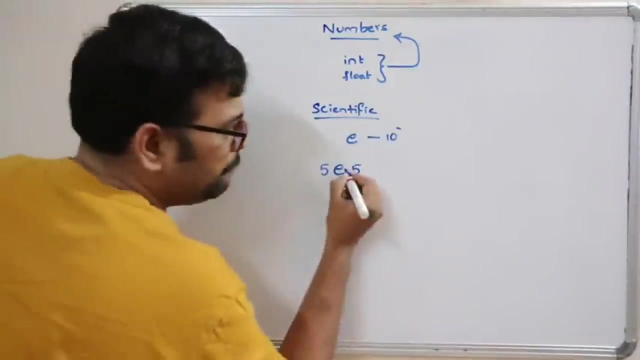 give any accurate value. anytime, it doesn't give any accurate value, right? Next, coming to the arithmetic operations. arithmetic operations, see, and also we can represent a number in a scientific form. Right, So that means exponential. exponential means a 10 power, right? So if a number represents some 5 e, 5, okay, 5 e plus 5, that implies 5 into 10 power, 5.. 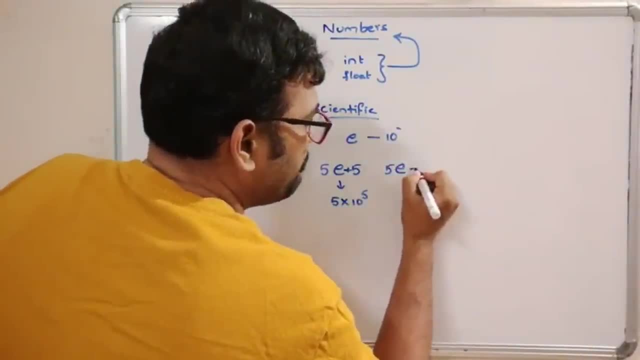 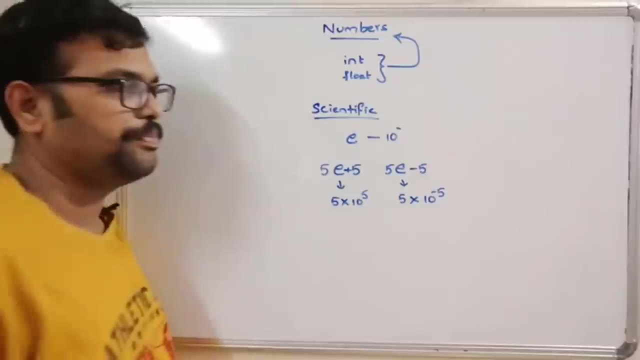 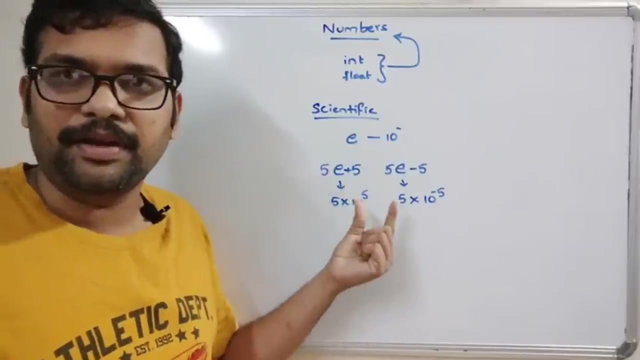 Okay, If 5 e minus 5 minus 5.. Okay, So that means 10 power 5.. Okay, So this implies 5 into 10 power minus 5. okay, 10 power minus 5.. So this is how we can represent a number in a scientific way, scientific way, okay. 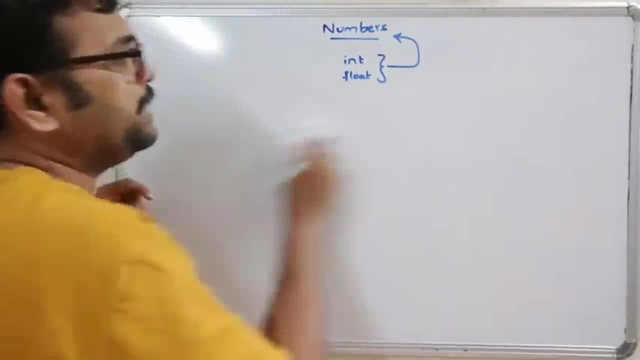 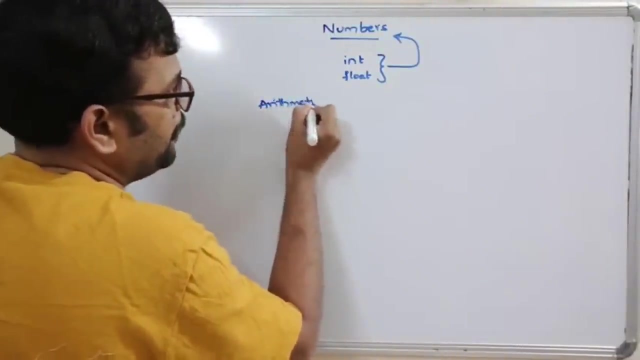 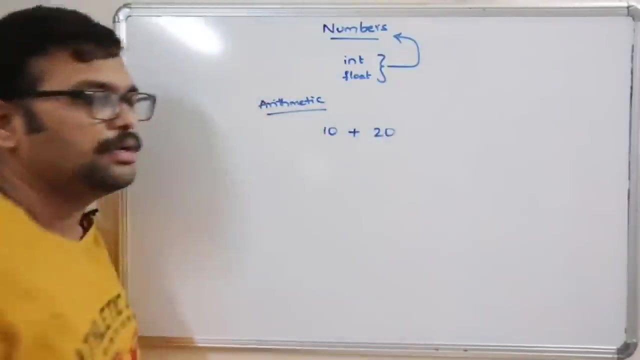 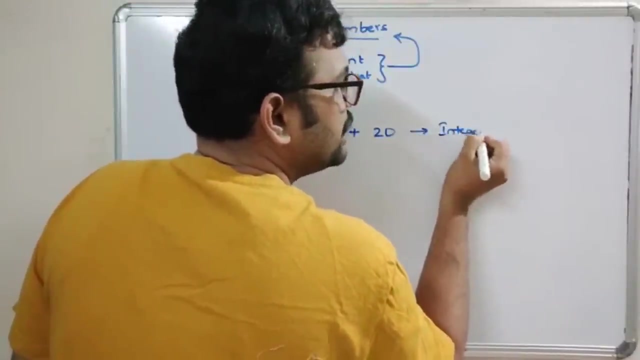 Then I will show you by executing a small code, no problem, and then working with the numbers and strings. So coming to the arithmetic operations. arithmetic operations, So if 10 plus 25.. Okay, If you are taking two variables, both are integers. we will get the integer result. integer result. 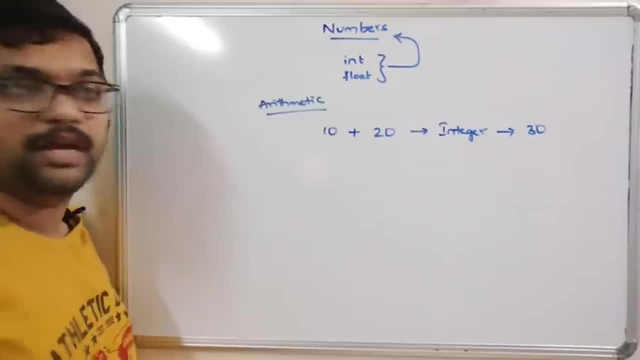 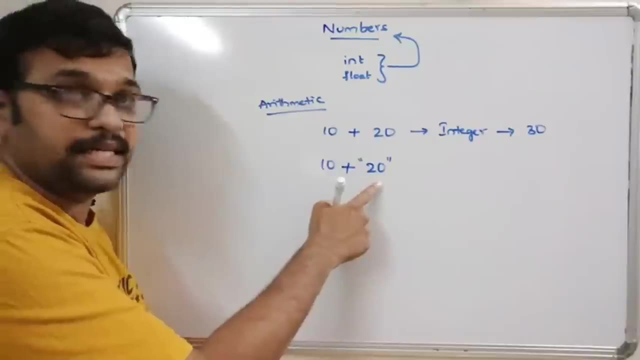 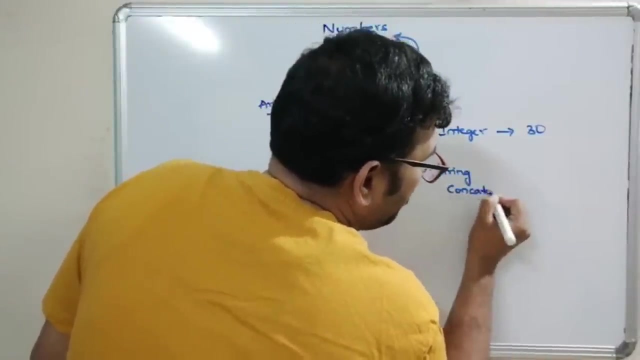 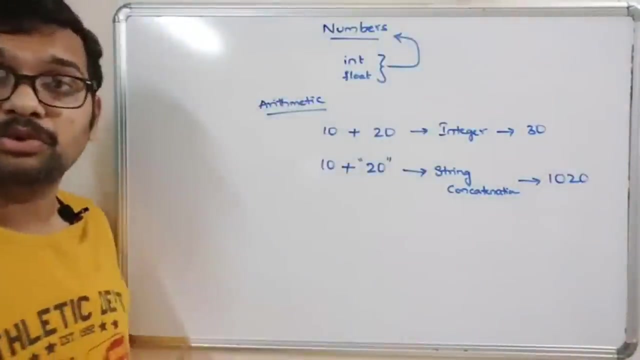 that means 30, 30. okay, if 10 plus 20- here 20 is a string, here 20 is a string- then it will treat as a string. So concatenation will be done. concatenation. So if it is a concatenation, What is the result? 1020, we should not call as 1020, we should call it as 1020. 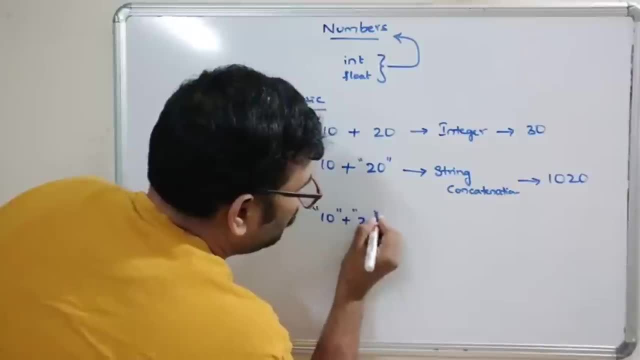 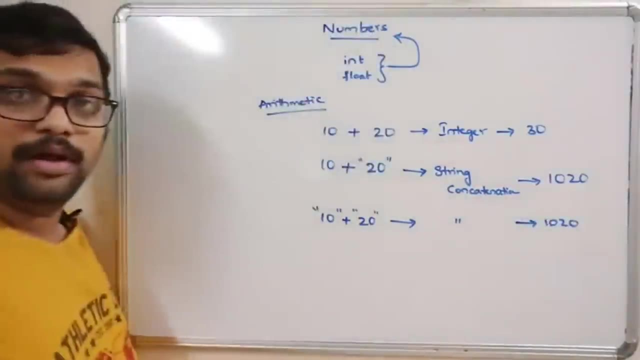 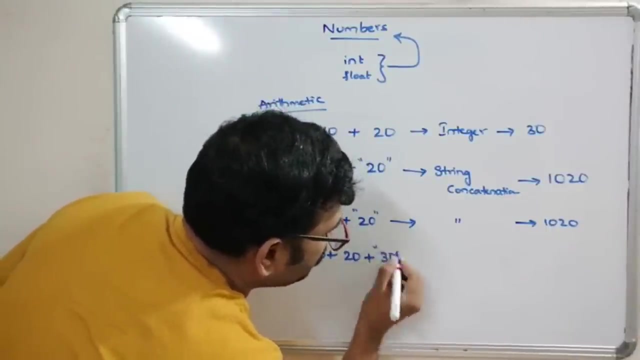 Then if both are strings, if both the inputs are strings, still we will get the concatenation 1020 and see 10 plus 20 plus 30.. Okay, 10 plus 20 plus 30.. Okay, 10 plus 20 plus 30.. 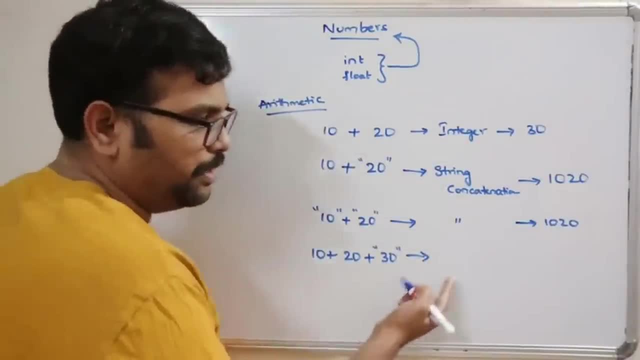 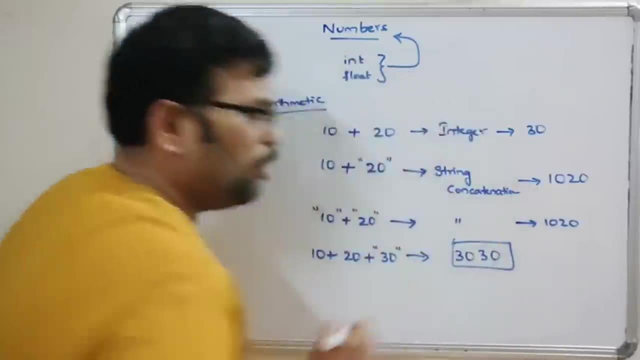 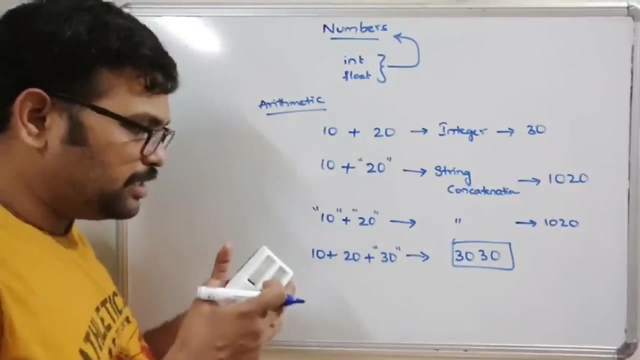 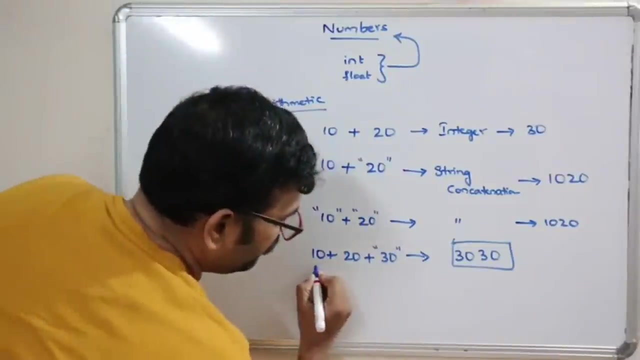 Then the result will be 13030. this is the result why we are getting this 3030. always, the JavaScript interpreter will execute from left to right. okay, consider, and it will execute from left to right. So first, it will execute these two things, these two values. what's the value both are? 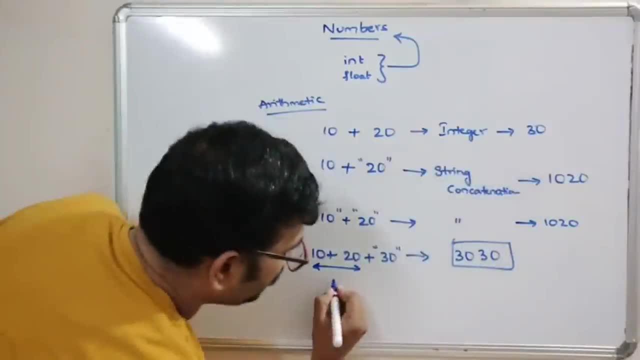 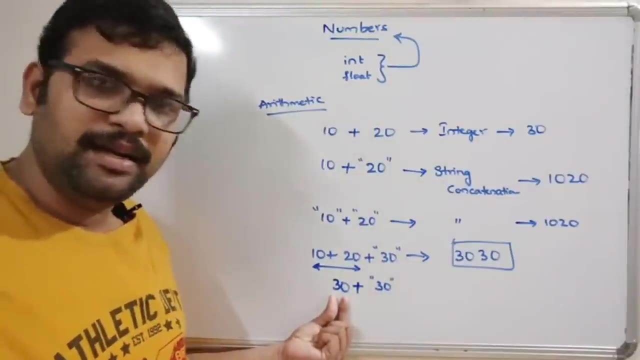 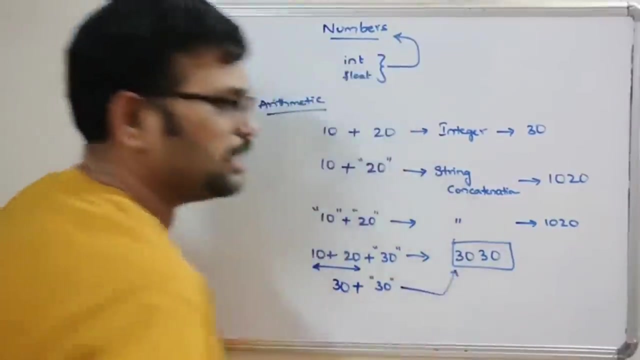 integers. If both are integers, We are getting the result. so 30 will be the result plus 30. so again we are getting one integer as well as one string. so then it will be considered as a string concatenation. So that's why we will get the result as 3030- 3030- we should not call it 3030, it's a 3030. 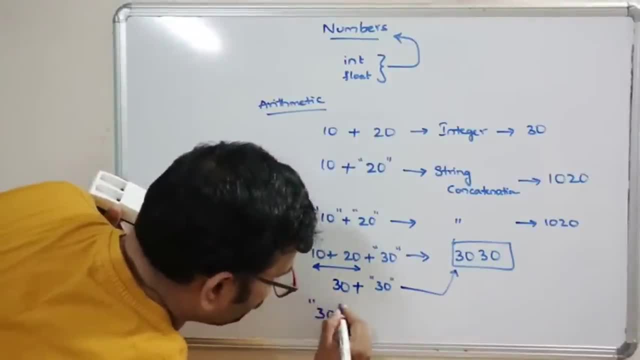 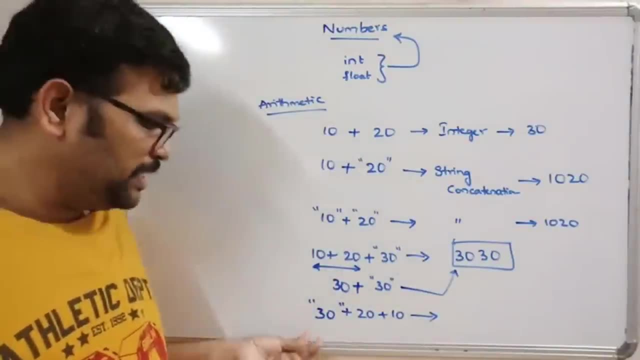 then see same case: 30 plus 20 plus 10.. So we are getting the result: So 3030, 3030.. If the expression is in this way, That means the first argument is string and the further two arguments are integers. then 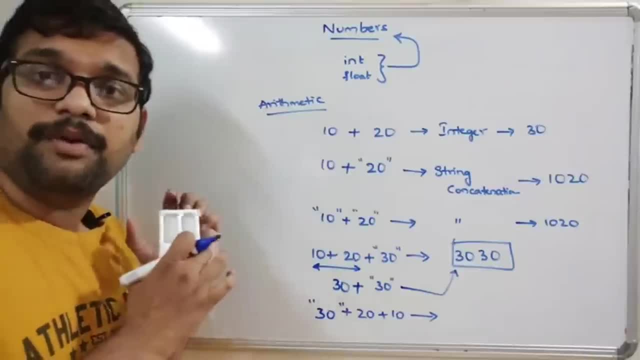 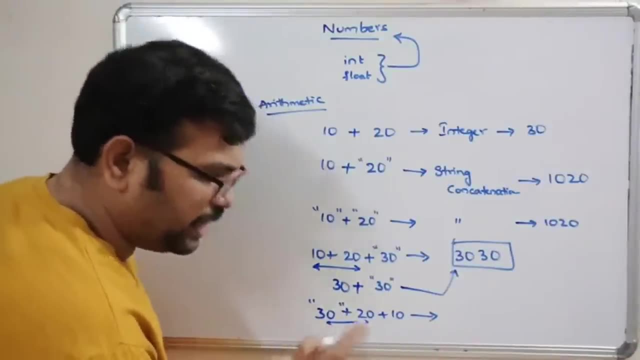 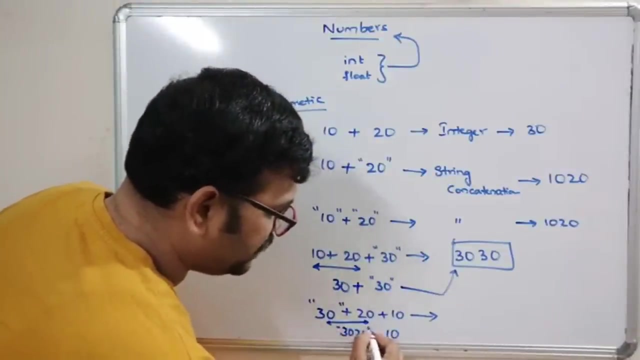 then also the JavaScript interpreter will execute from left to right. So first these two will be executed, these two will be executed. what's the results of these two? one is string and another one is integer. So concatenation will be done again, 10.. So this is a string, right? 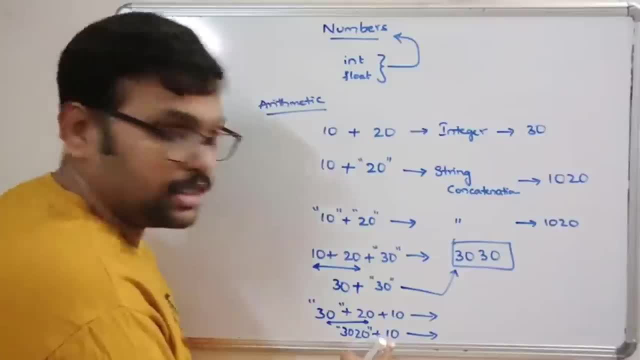 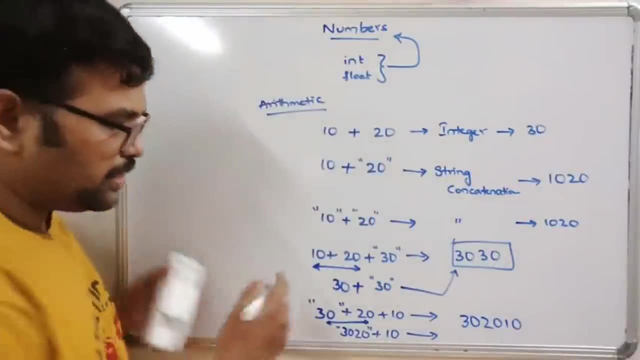 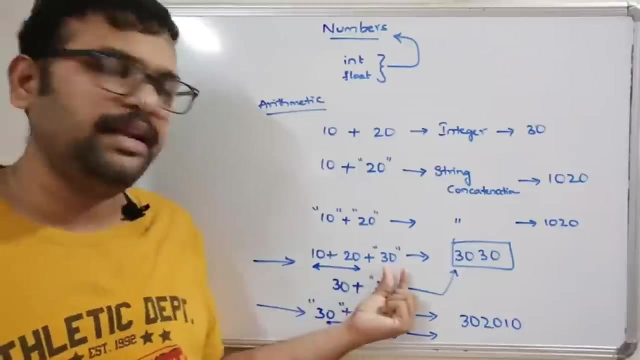 This is a string. So what is the result? one is string and another one is integer, So the result is 302010. see, both are same. You can observe here both are same, but the order is different. first we are giving the integers and then string. here, first we are giving some string and then integers. 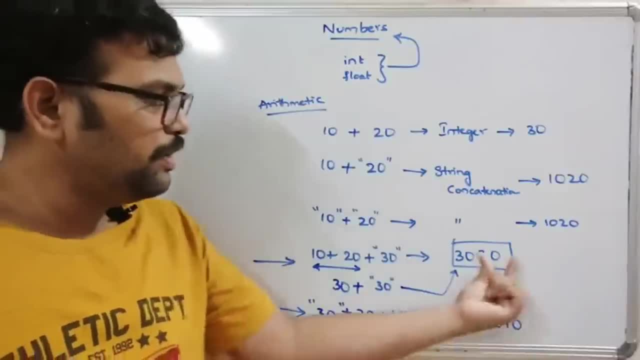 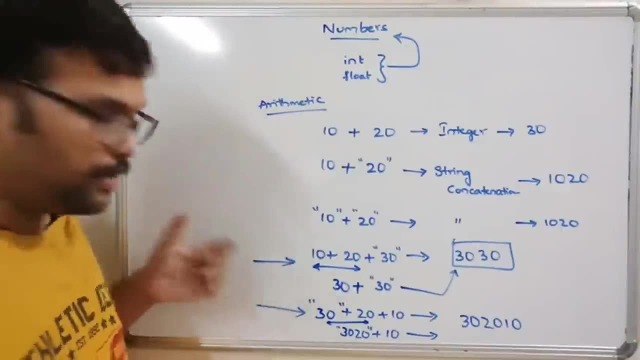 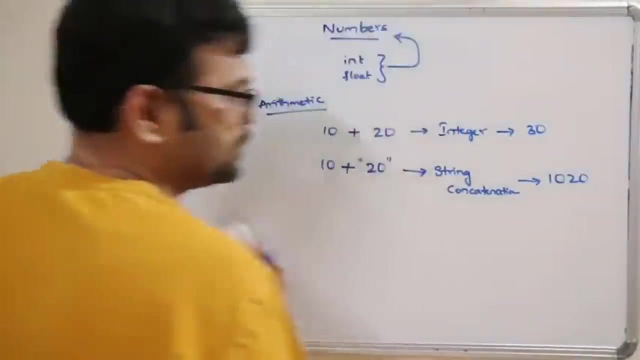 So interpreter will execute from left to right, So that's why we will get different answers for this type of expressions. Right, Right. So hope you understood this one, Right. Next, Other than addition, what about the remaining arithmetic operations other than addition? 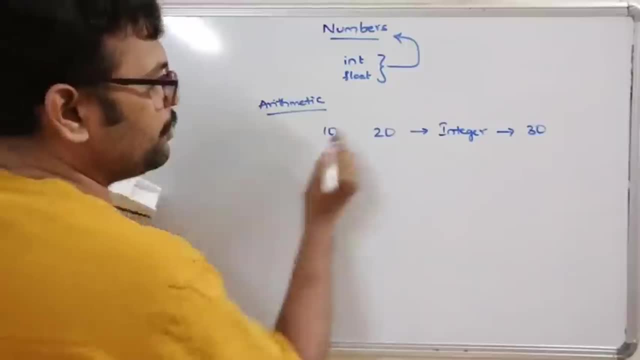 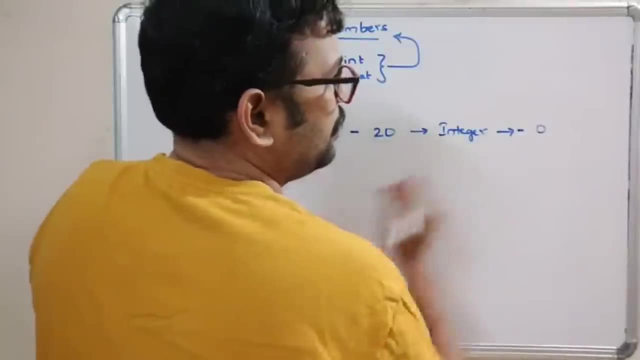 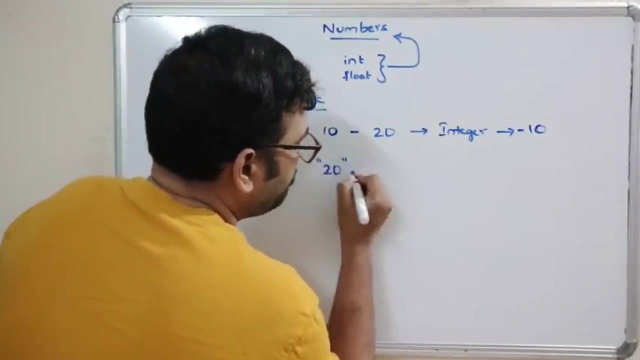 So, for example, for example, in place of addition, if you give minus, the result will be minus minus 10, minus 10.. Right, And if 20 minus 10. Right, Right, Right, What is the result? So this is a string. 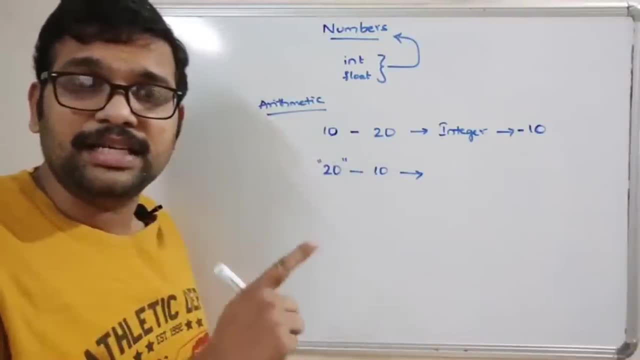 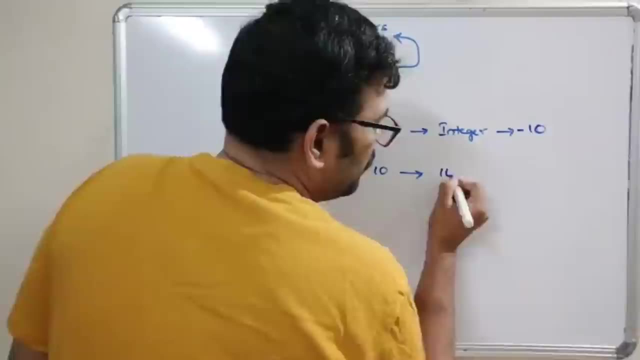 This is an integer In such case, other than the addition, in such case the string will be converted into numerical. Okay, The string will be converted into numerical, So the result will be 10.. Integer itself: The result will be integer itself. 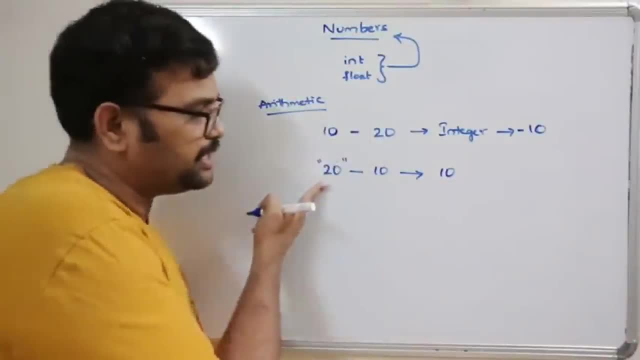 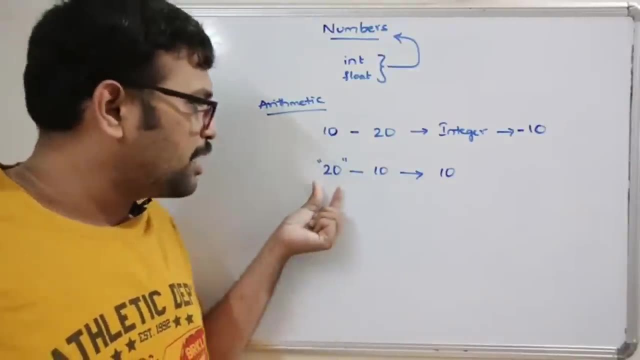 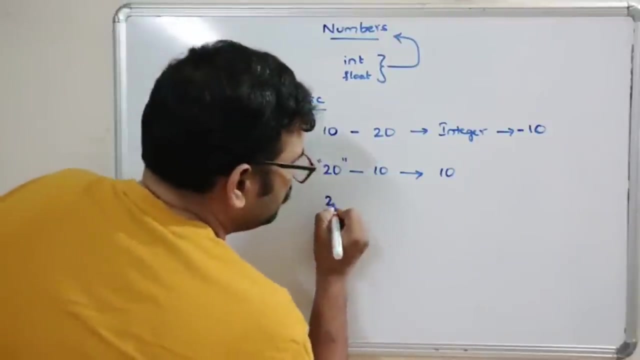 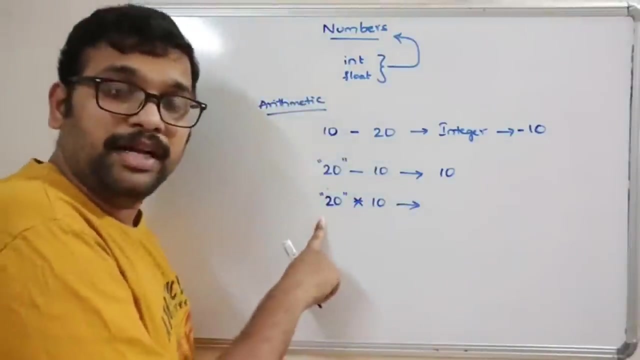 So if one is a string, another one is an integer. If the operator is other than the addition, then it will. then the- I mean this string- will be converted into number. Similarly, Similarly, 20 into 10 again will get the number. 20 will be converted into number. and. 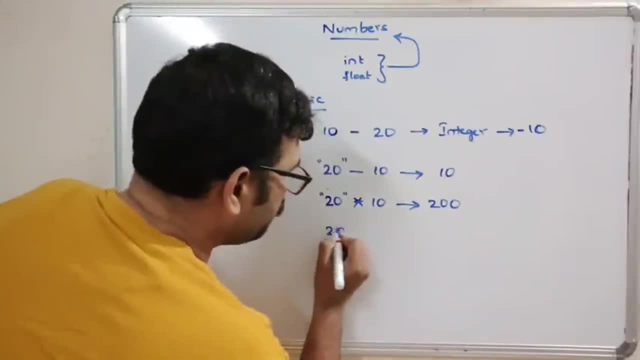 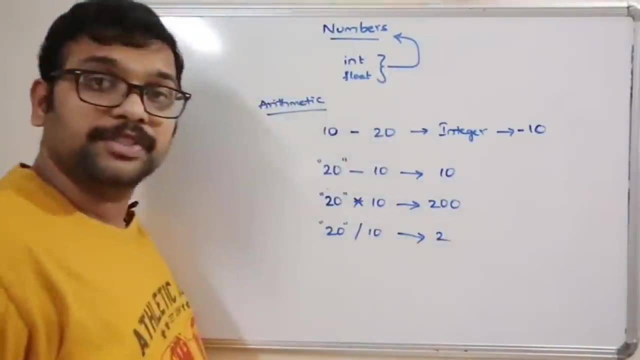 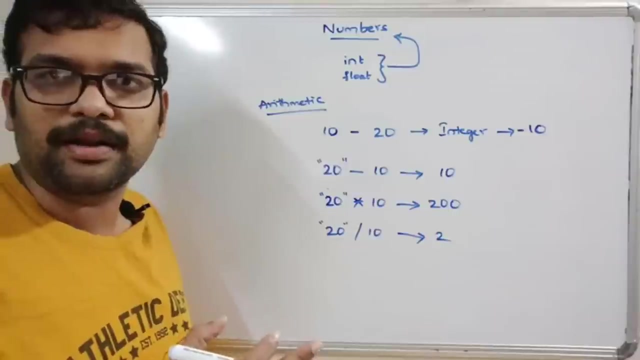 10.. That means 200.. Similarly, 20 divided by 10, again 20 will be converted into number, So the result will be 2.. Okay, Only for addition, the string will be concatenated, So plus will be acting as a concatenation operator. 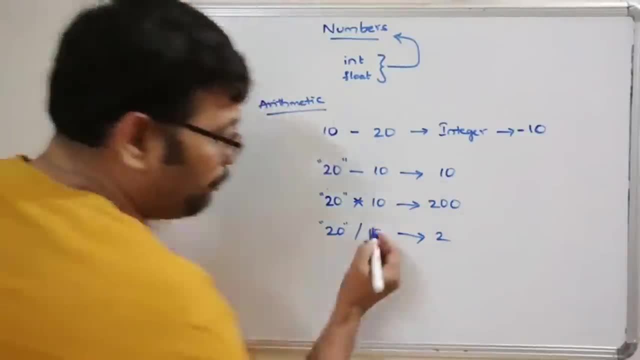 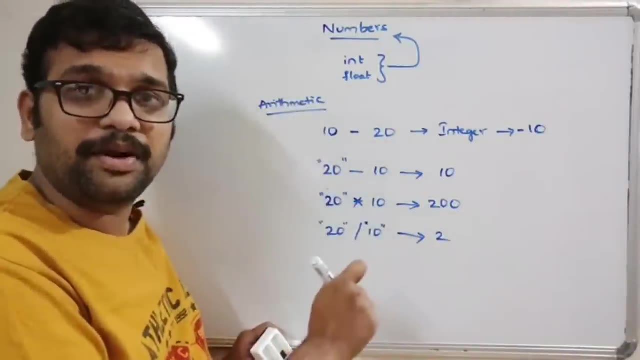 Right, Hope you understood this one. And if both are strings, then also we will get the same result. Both are strings. also we will get the same result, Other than the addition operator. For every other operator the string will be converted into number. 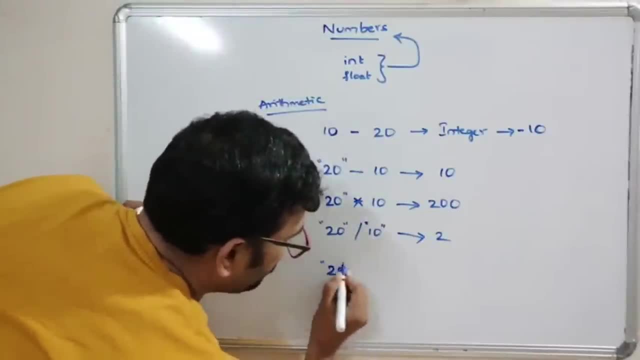 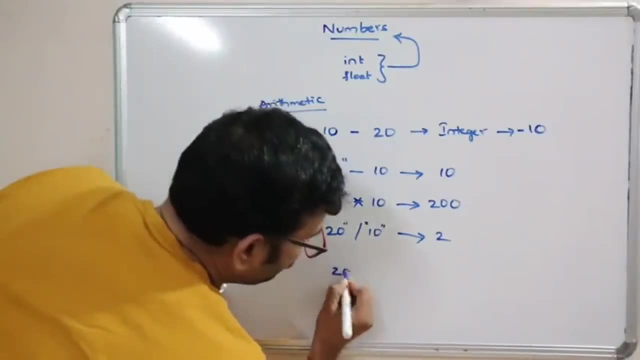 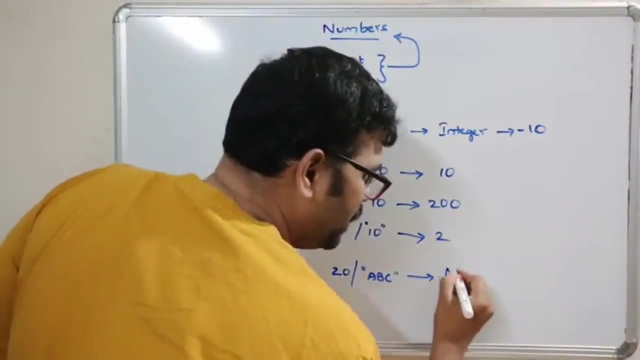 Right And see, in such case, one is a string, Another one is, or one is an integer- Okay, One is integer, And another one is some string- Okay, Another one is a integer, Okay, So some string. automatically, if the result will be n a n, the result will be n a n. 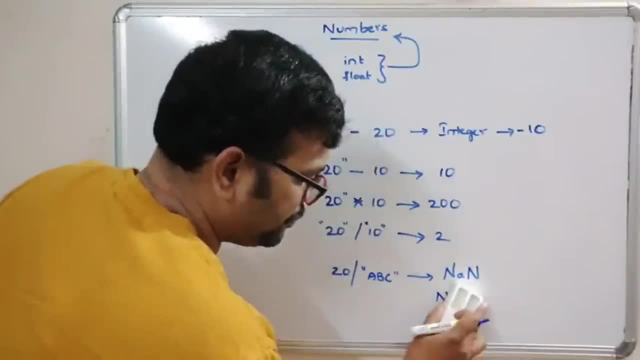 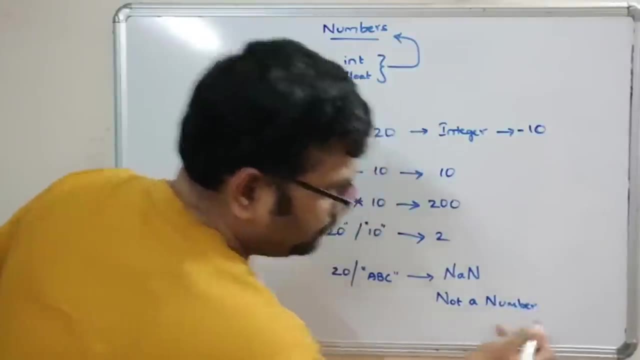 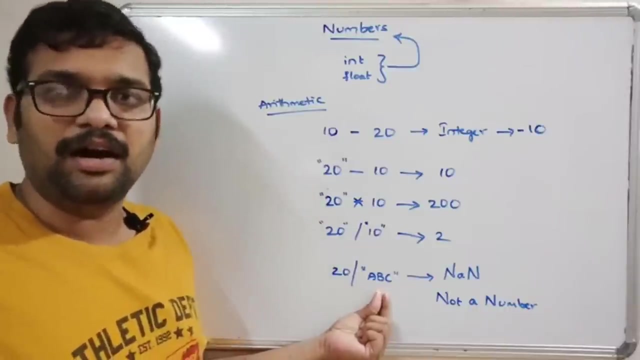 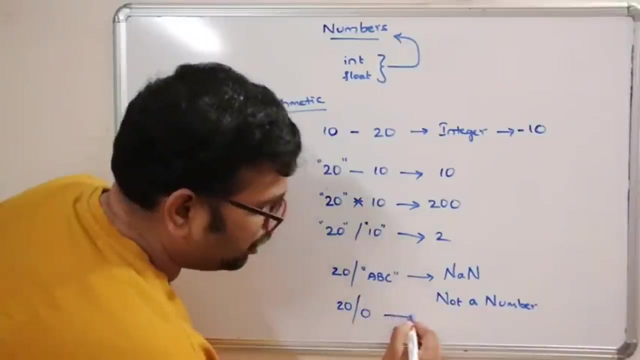 n. a n means sorry, not a number, because this is a non-numeric string. So if any expression is having a non-numeric string, automatically will get the result as nan, not a number. And, for example, if you are having 20 by 0, we will get the result as infinity. 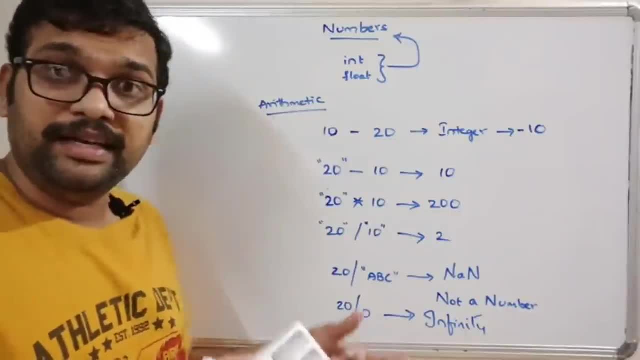 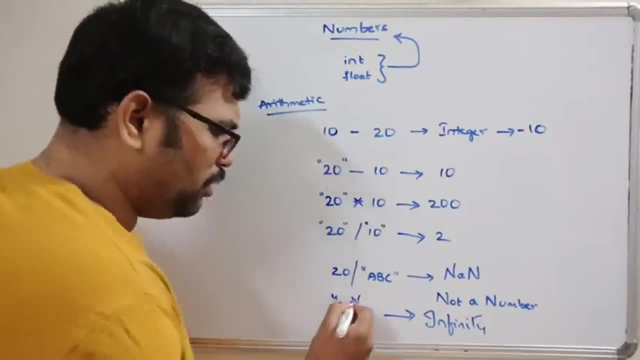 Infinity. So we know that anything divided by 0 will get the result as infinity. So in such cases we will get the infinity. So if it is a string, also we will get the infinity. If both the numerator and denominator are strings, then also we will get the infinity. 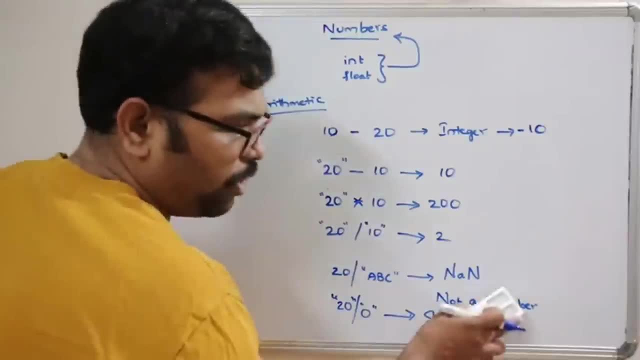 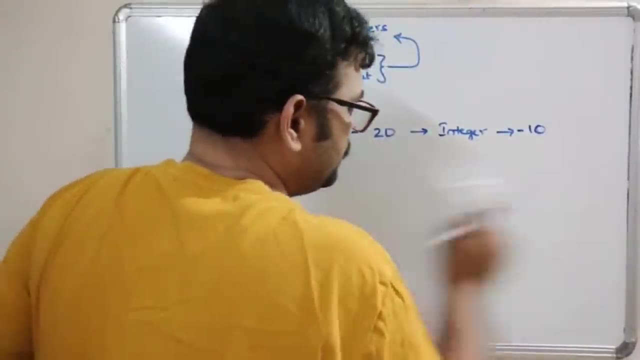 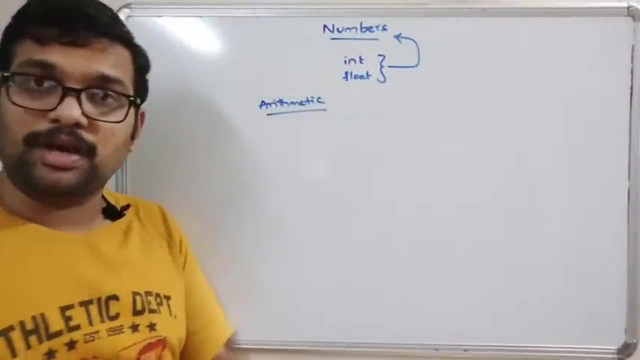 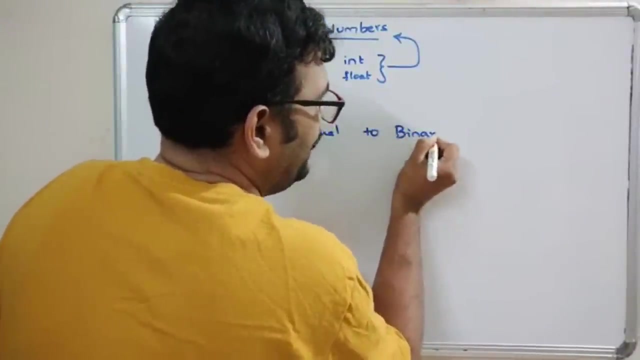 Okay, So this is one case, not a number and infinity, Okay, Okay. And the next one is number conversion, Number conversion. So, in order to convert one numbers conversion from one type of number to another type of number, That means decimal to binary, octal, hexa. 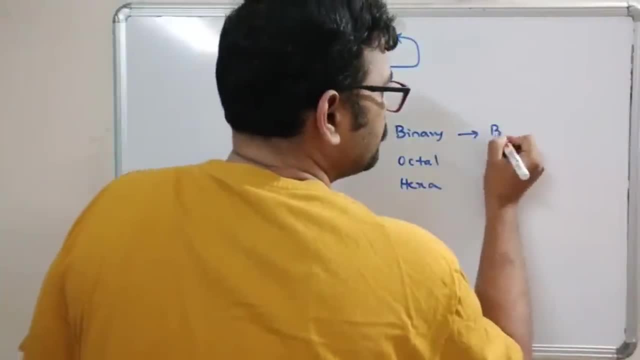 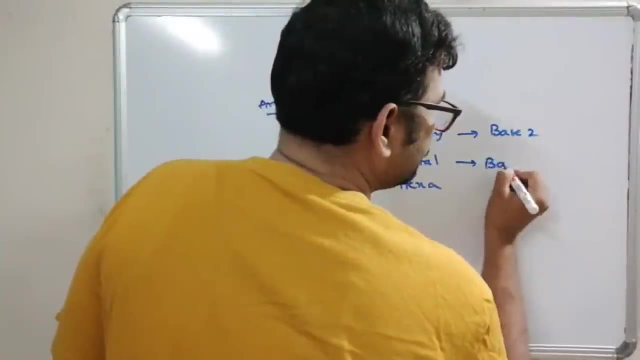 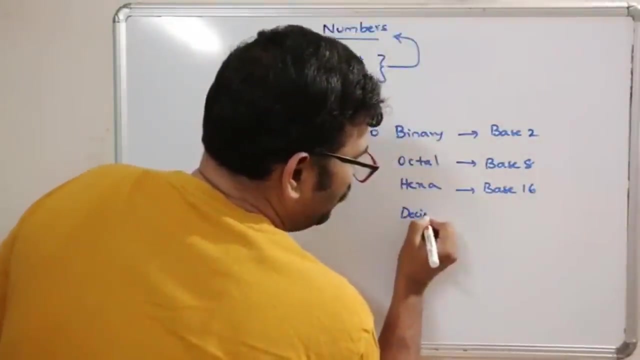 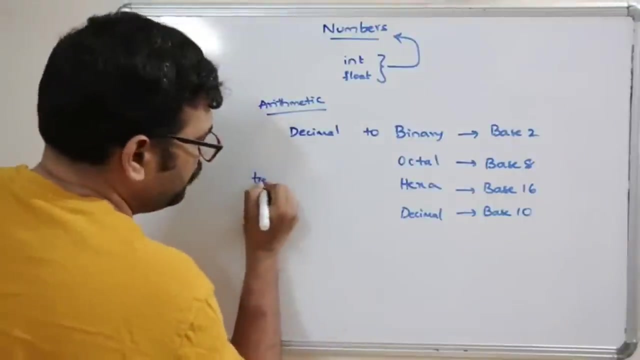 Okay, Hexadecimal. For binary, the base is 1. 2. okay for octal, the base is 8. for hexa, the base is 16. for decimal, the base is 10, right, so there is a function called to string. to string, here s is capital, right? so here we have to pass. 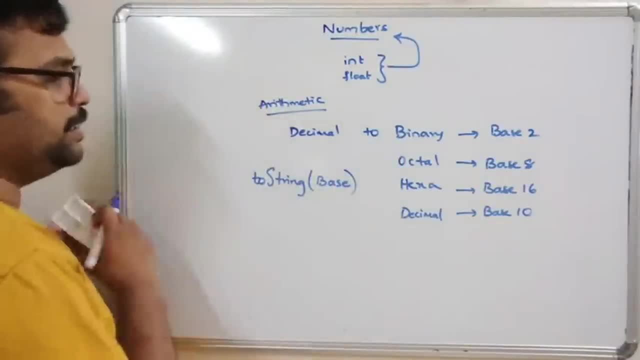 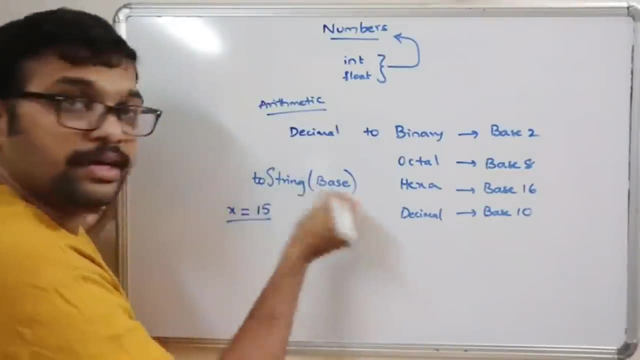 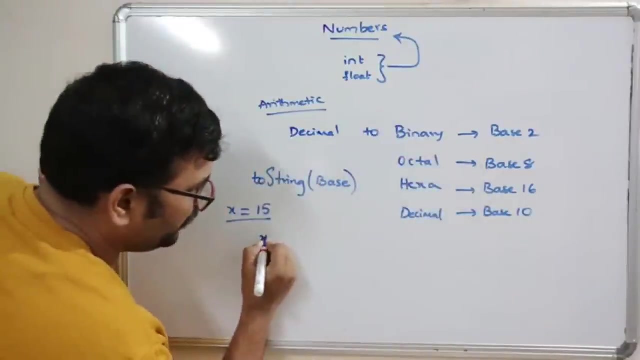 a base to which we need to convert right. see, for example, x is equal to some 15. x is equal to some 15. now we need to convert into another number system. so this is nothing but an integer which is a decimal value. so if you want to convert into binary, so we need to do x dot to string. 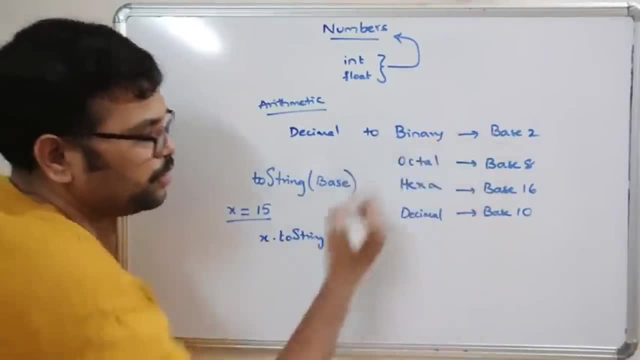 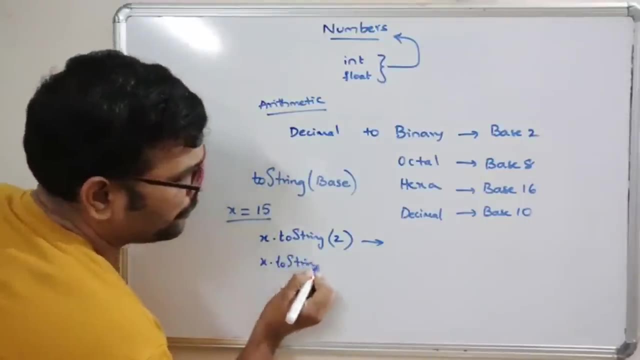 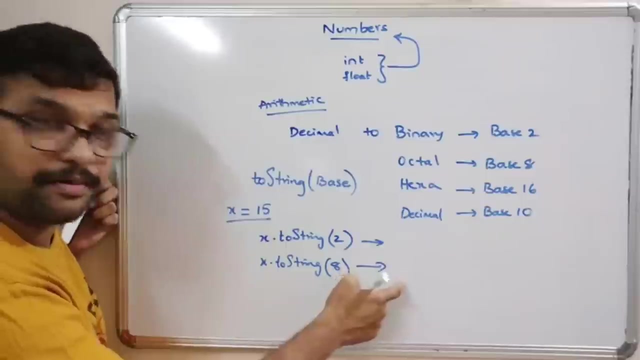 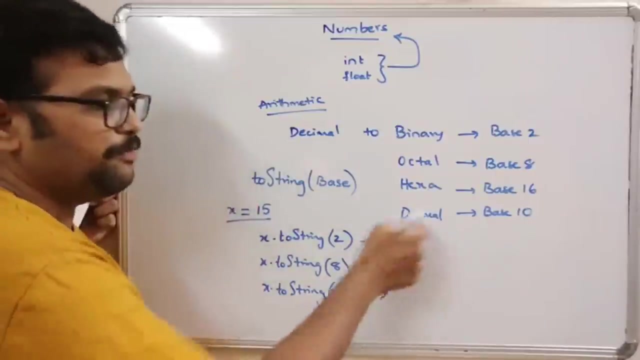 of base. what is the base for binary 2? so automatically the binary result will be applied and similarly x dot to string of 8. the octal representation, the octal value of 15, will be displayed here. similarly, x dot to string 16, the hexadecimal value for this 15 will be displayed here. 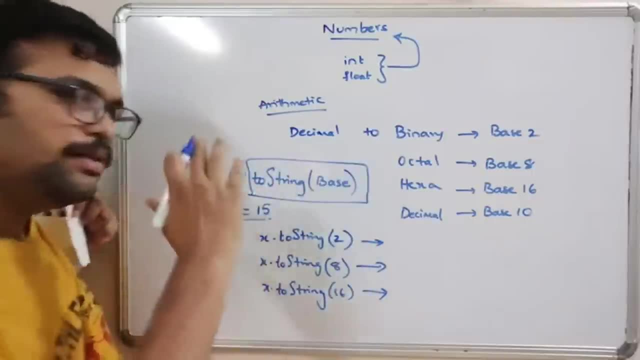 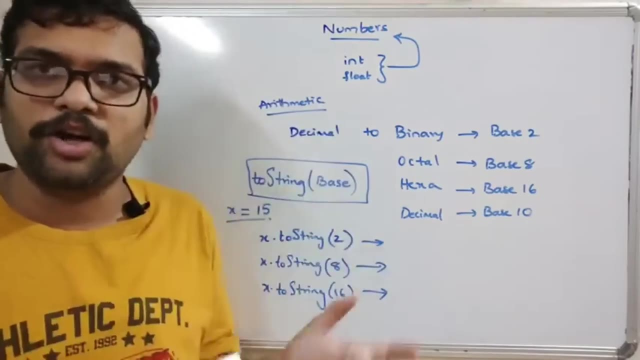 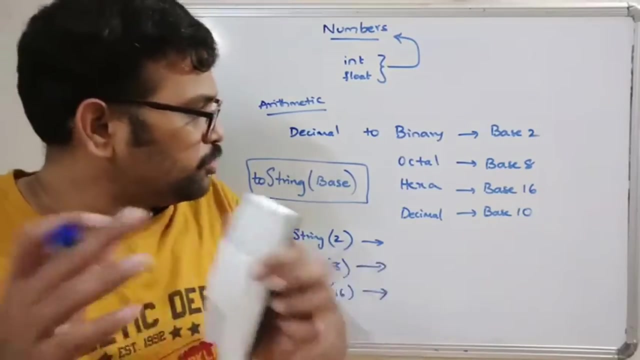 so this is a function to convert from one number system to another number system, right? so hope you understood this one: the numbers and the arithmetic operations between the numbers and strings. working on working with numbers. so let's stop here and i will show you each and every. 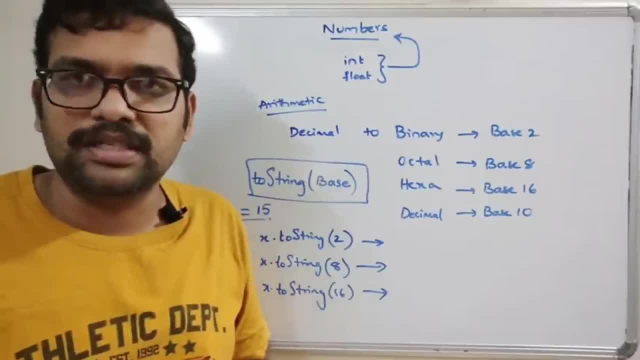 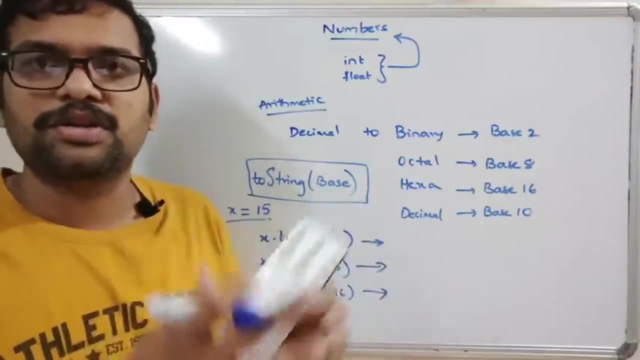 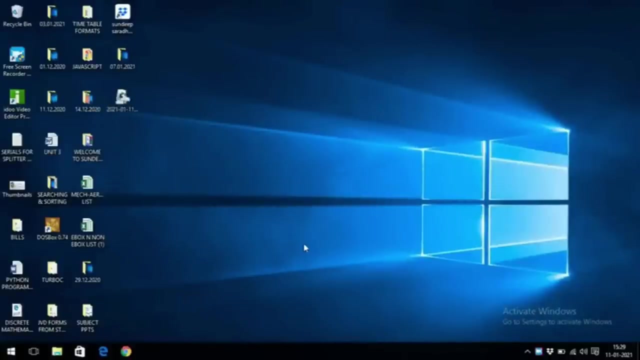 explanation demonstrating using a small code on the system. so let us move on to the system and write some html content so that, if you are still having any doubts, those dots will be carried. so let's move on to the system. hello friends. so just now we have seen working of numbers in javascript. 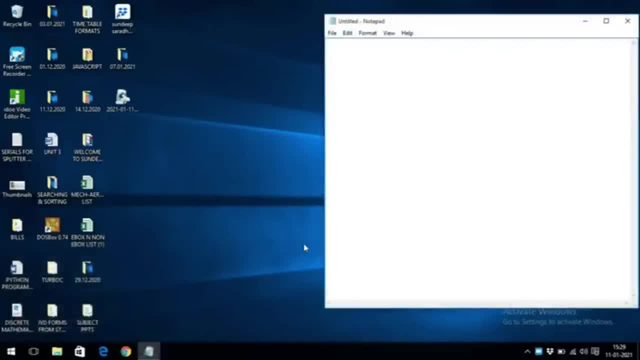 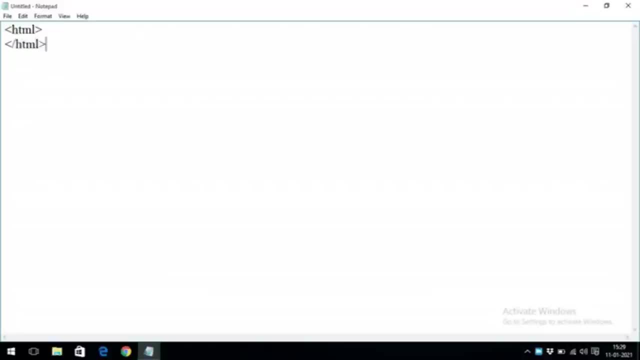 now i will demonstrate this thing by writing some HTML code. so let us start with the HTML content. so let us take some HTML tags and inside the HTML we'll write some body. so we'll write some title here, heading, some h1 numbers in JavaScript. now we'll take some paragraph. we'll take 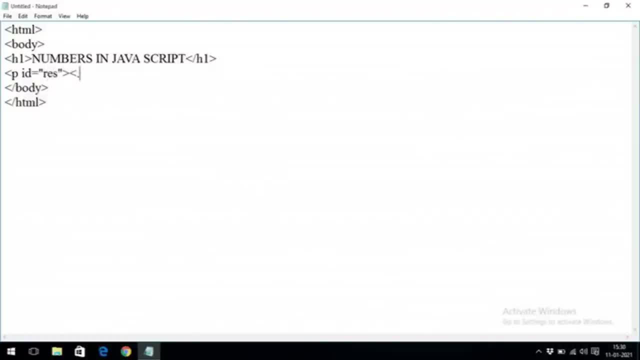 some ID is equal to some result, so that our result will be displayed here itself. okay, we'll write some script inside the script. we'll write all the things. script right now. the number of tags: we'll write some number of tags. we'll write some number of tags. 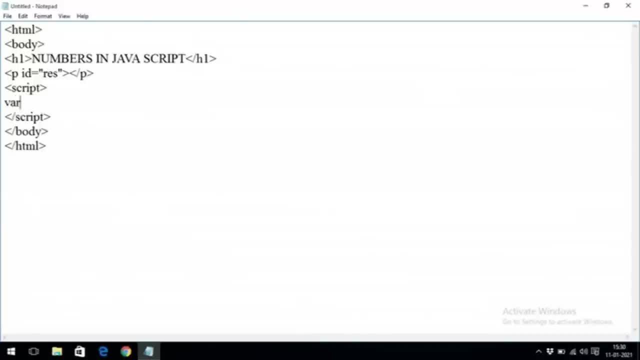 numbers. let us consider the numbers. so: variable X. so here there will be no data types. okay, you, based upon the value assigned to that variable, it will be considered as a data type. some X is equal to some 3.14 and variable X Y is equal to some 20. then we display here: so get document dot. get element by ID. 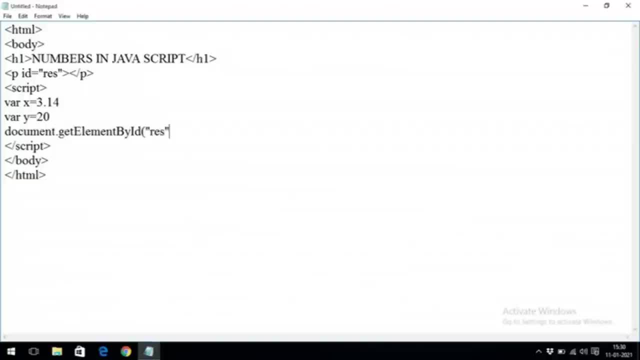 of what is the value. result: dot inner HTML is equal to some. see some X. let us take some X. I will save here with the numbers dot HTML and we'll check. we'll execute this one whether it was displayed or not. we can observe here. so 3.14, and if you display Y here, we'll get some 20 right now. that's clear. 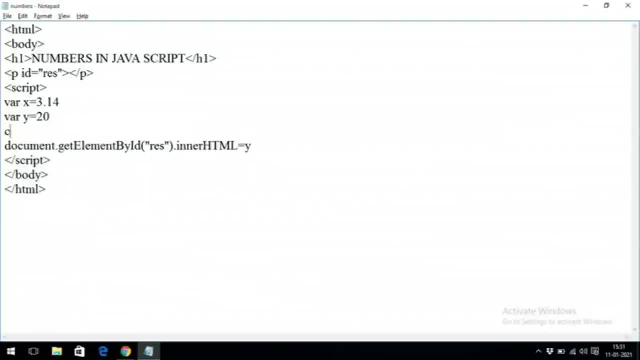 now we can also represent this one in a scientific notation somewhere. scientific notation means exponential right. some Z is equal to some 5 e 3. 5 e plus 3. e plus 3 means nothing but 10 power. 3. that means a plus 3 means 10 power plus 3 if 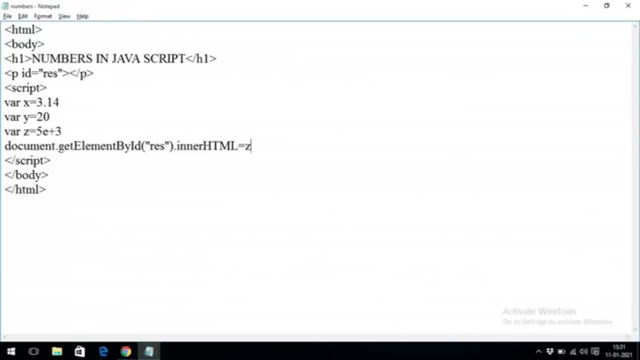 it is a minus 3 will be 10 power minus 3. now you just go with the Z value, you can observe here, see 5000. so 5 into 10 power 3. if you go in here with a 6, can observe okay, 5 into 10 power 6 and if it is a minus 1. so 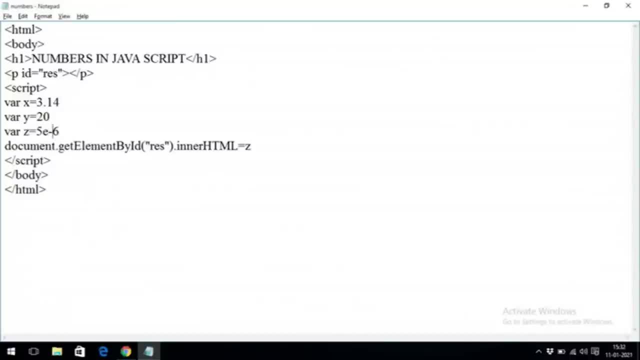 the real part will be having only one value and everything will be in the decimal part, right, so simply 5 into 10 power minus six. now you can observe here: 0 point 0, 0, 0, 0, 0 file right, so we can also represent any, any value in the 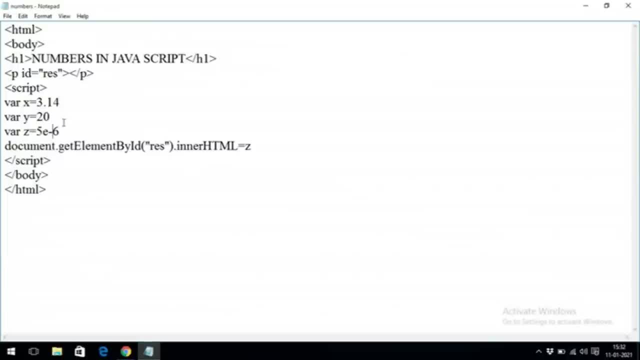 scientific format also. and next is the Precision's. so here not only the float values, we can also have the precisions for integers. that means in javascript the integers will be having an accurate result of only up to 15 digits. if the number exceeds, with the 15 digits, automatically the result may vary. for example, you can observe here some 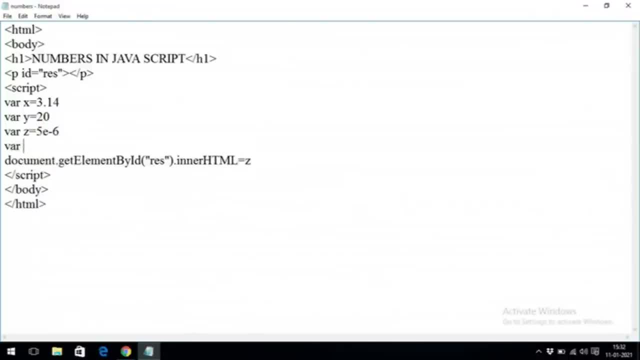 where n is equal, to see 1,, 2,, 3,, 4,, 5,, 6,, 7,, 8,, 9,, 0, right? so total 10 digits are there. so here I will display some n you can observe here. so we are getting accurate result, accurate result, right. 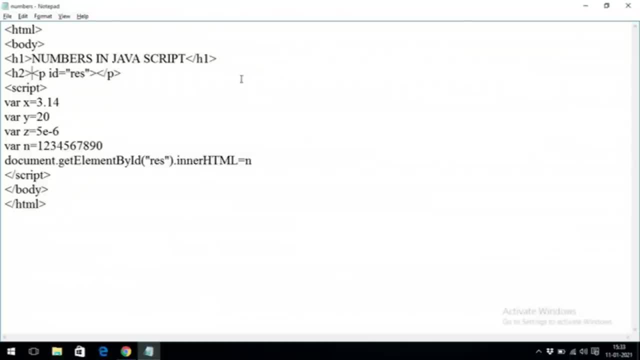 so let us do some heading so that it the text will be appears bigger. okay, right see, now I will add a few more. so 1, 2, 3, so that total 13 digits, 14 digits. I will give 14 digits now we will see: yes, 14 digits. 15th digit. let us check. yes, 15th digits. 16th digit: okay now. 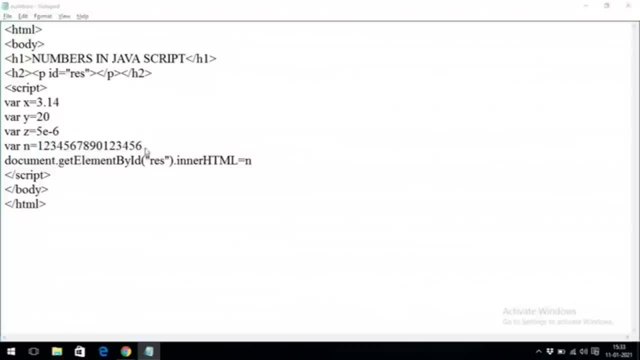 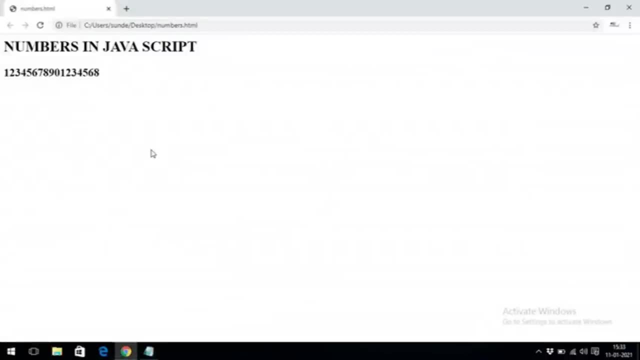 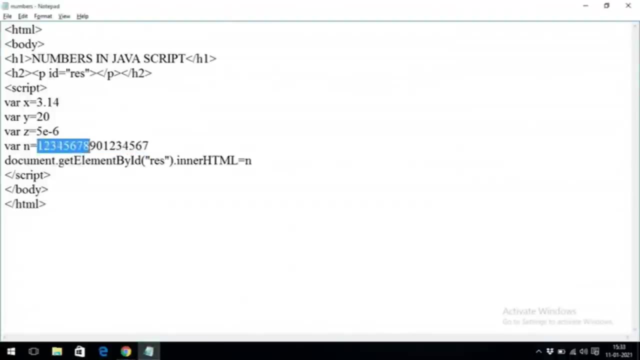 the digits. the number of digits for this number is 16 digit number. now you can observe here, okay, 16. see from the 16th digit you can observe if it is a 17 digit. here we are. we have given the number as 1, 2,, 3,, 4,, 5,, 6,, 7,, 8, 9, 0, 1,, 2,, 3,, 4,, 5,, 6, 7, but we are getting some 8 value here and if you go, 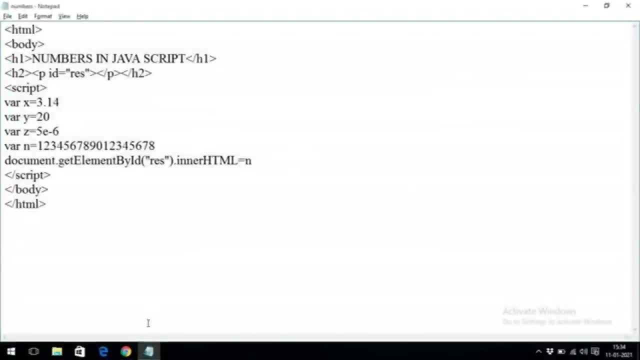 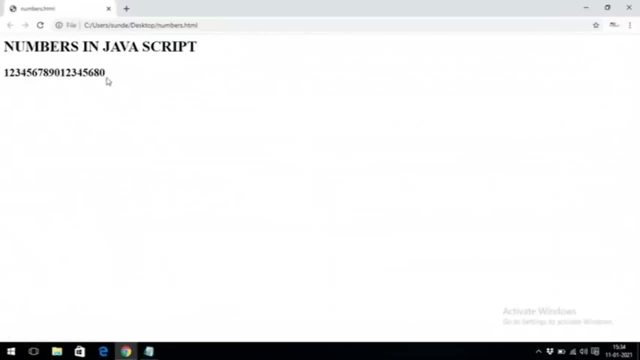 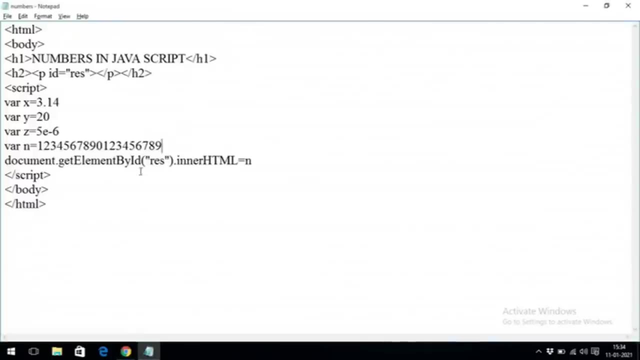 keep on increasing the digits. sorry, once again, we will execute this one. if you keep on executing the digits, you can observe the result will be varied. okay, so the precisions, the precision, the maximum number of digits equal accept with the accuracy, is only up to 15 digits. 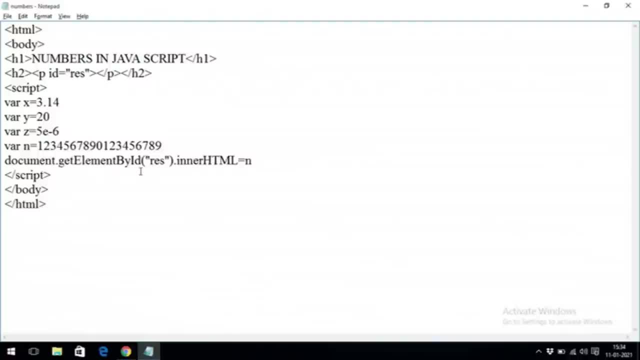 okay, if the number exceeds with the 15 digits, automatically the thing will be: the number will be automatically inaccurate, right? similarly, we will go with the float values. float values means so it will maximum, it will take around 17 decimals. it will give the accuracy up to 17 decimals. for 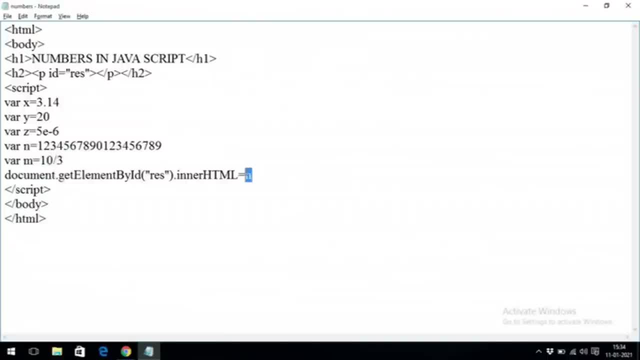 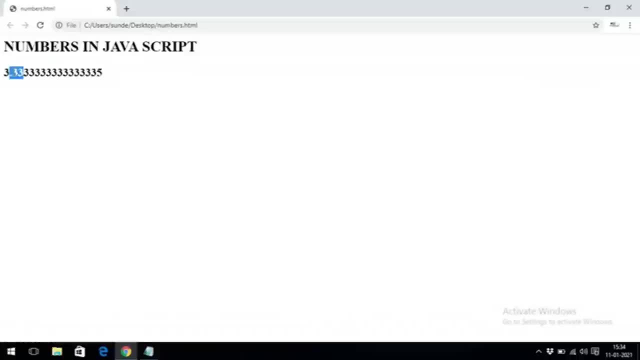 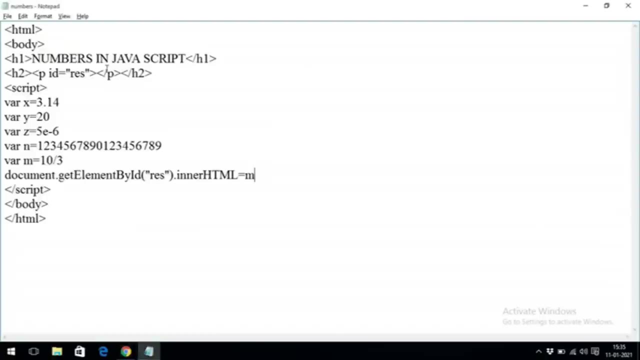 example divided by 3. it is a never ending right. So if you give m, you can get it here. see. So up to 16 digits is it was equal and for the 17 digit we are not getting any accuracy. it is an inaccurate right, So the float values will always be inaccurate, that is. 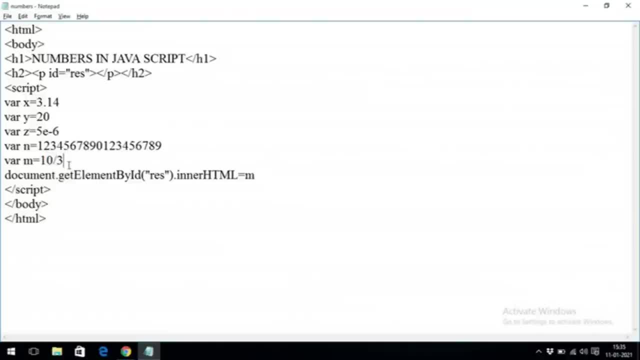 one thing to be remembered, right? So here the float values will be almost inaccurate. Now, see, we will see the working with numbers and strings, or combination of numbers and string. So I will remove all these things. we will take two variables, x and y, and we will check. z is equal to. 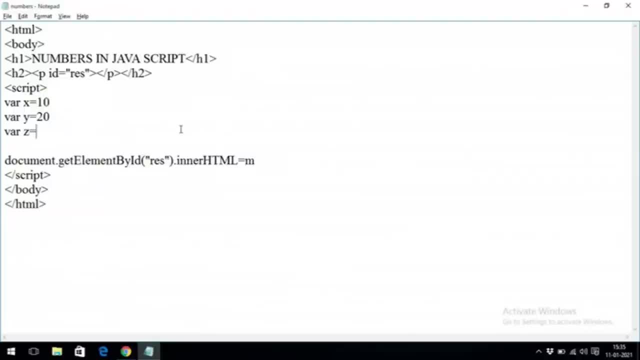 So if it is some 10 and a 20, if it is x plus y and if you are printing some z value, see we will get some. result is 30. that is good. both are integers. we are getting The integer result if both are strings. So remember that all the strings should be. 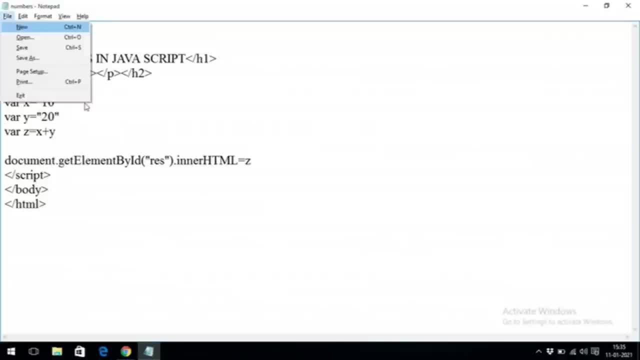 enclosed in double quotations. either it may be a numeric string or non-numeric string. So this is a numeric string. So if the string consists of only digits, we call it as a numeric string. So if digits does not have any numerics, we will call it as a non-numeric strings. see. 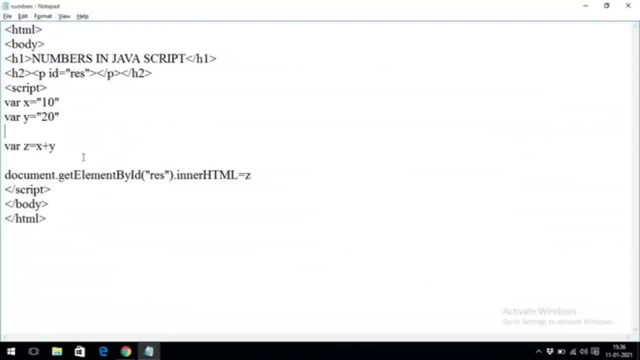 Now what is the result here? the concatenation. the result will be the concatenation if both the variables are having the string data type. So if you use the addition operator, automatically the result will be the concatenation. So the result is not 30, it will be 10, 20, 1, 0, 2, 0. and then if, what is the issue with integer and string? 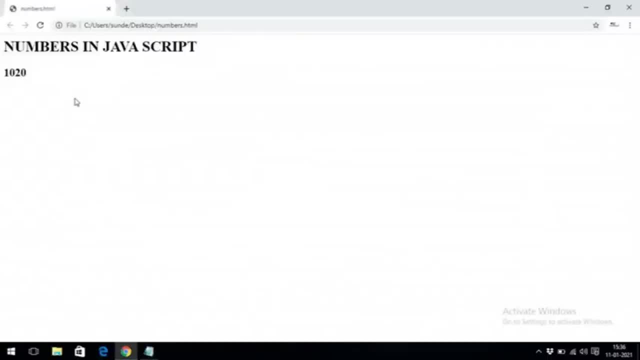 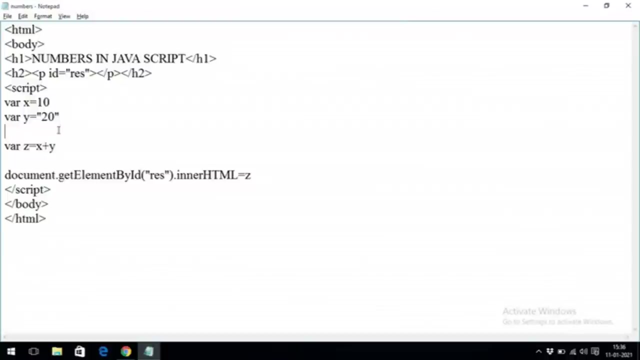 So 10 and a 20. if you execute this one again, we will get the concatenation right again. we will get the concatenation. ok, So 10, even though one is integer and another one is a string, we will get the concatenation as a result. Now we will. we will check x, y and where some r is equal to. 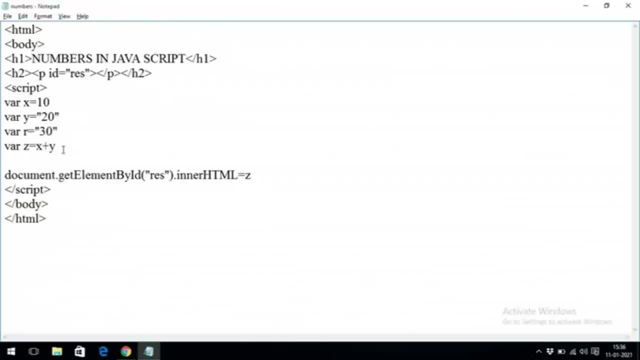 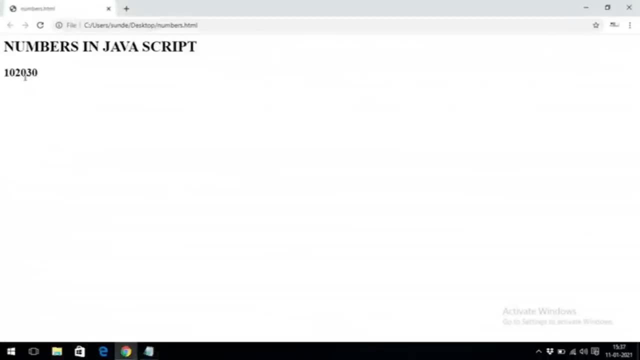 30. ok, r is equal to 30, we will. we will see x plus y plus z. sorry, r is not a z, it is a r. Now check: we will get 10, 20, 30, 1, 0, 2, 0, 3 0. we should not. 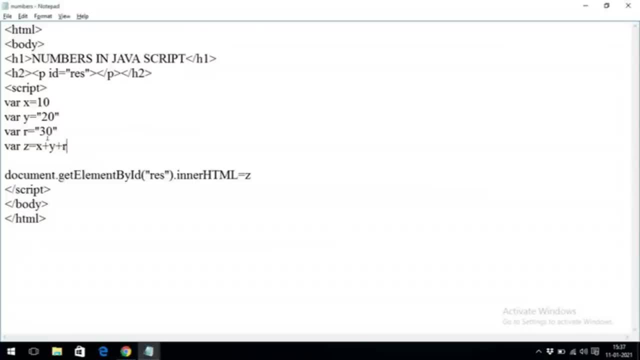 call it as a 10, 20, 30. we should call it as a 1, 0, 2, 0, 3, 0. that is good. And what if the expression is like this: So x and y are integers and r is a string. 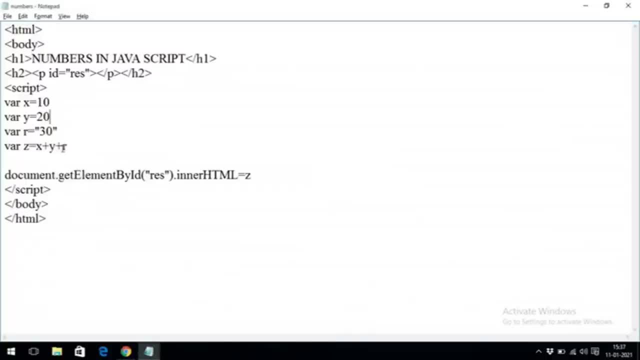 now what is the result? it will be 3 0, 3 0, because here these two are integers in JavaScript. the expression will be evaluated. arithmetic expressions will be evaluated from left to right. So left to right means first x plus y will be done, and then that result will be added to the r. 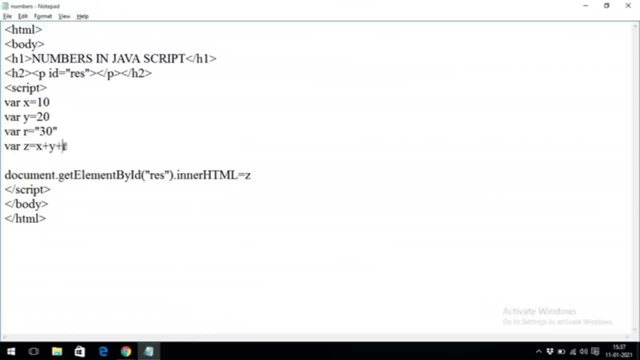 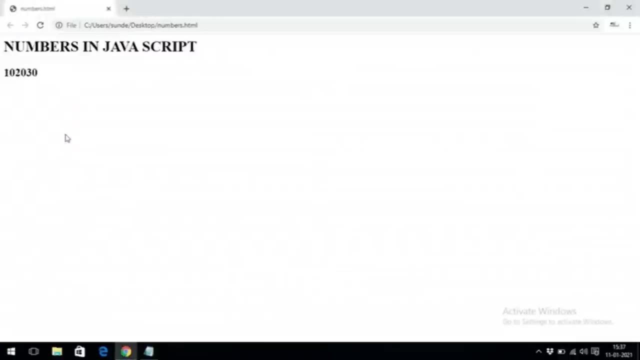 So here, x and y are the integers, So 30 will be added and r will be the string. So automatically it will be concatenated. See, the same thing I will show you in another case. if the first one is a string and next two are integers, then we will get the concatenation. 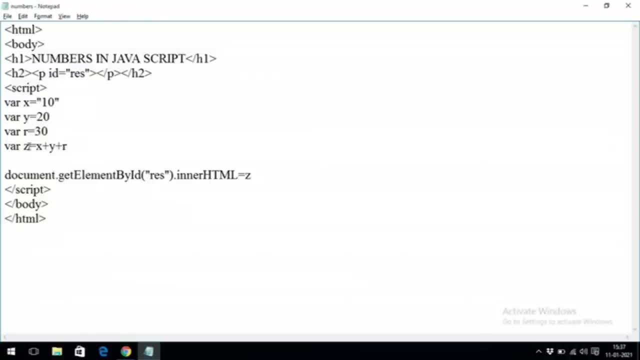 because left to right, the java script, the expressions will be evaluated. the interpreter works from left to right, So left most, with 10, which is a string, x, the and y is a integer, So both will be having the result of string concatenation: 1: 0, 2, 0. 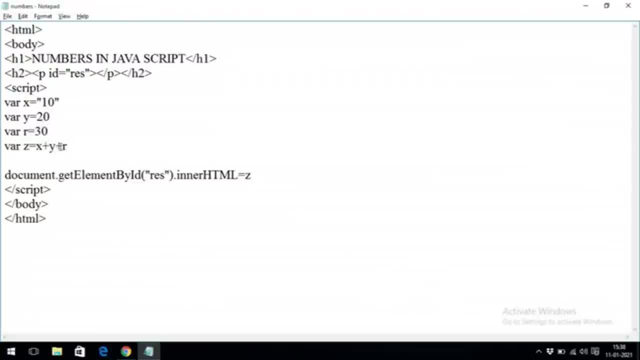 Again, it is a string, So again we are adding 30.. So 10, 20, 30, that means 1, 0, 2, 0, 3, 0 will be the result, right. So this is this is one thing you have to remember. the interpreter works from left. 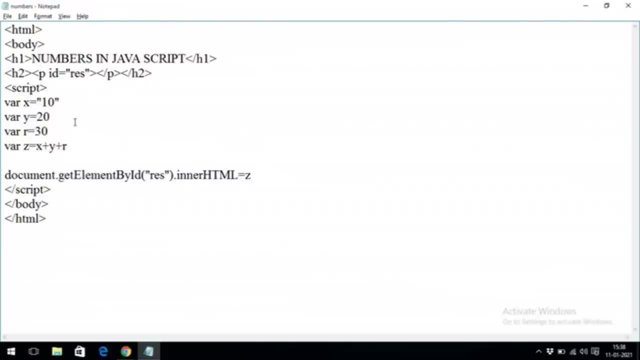 to right. yes, Now what about the division? dividing two strings: dividing two strings, If you go with the 10 and divided by 5, it is a string. again, it is a string, right? So so if x and y, now if we add, if you do add operation, it will be concatenated. 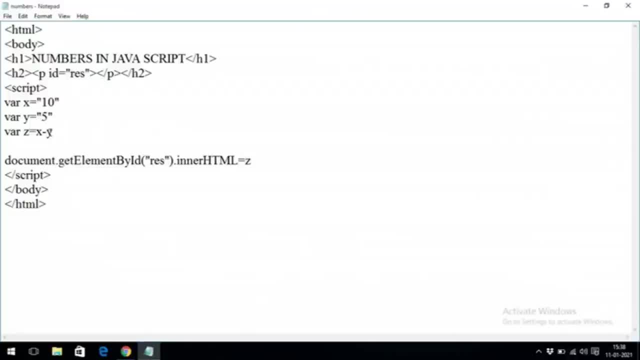 If you go with the minus minus, automatically java script will convert the string to numbers and you will get the numeric result. So 10 minus 5 it will be 5, and if it is 2, 10 minus 2- it- sorry, it is 2, the 10 minus 2- it will be 8.. So obviously, if both are strings, even though both 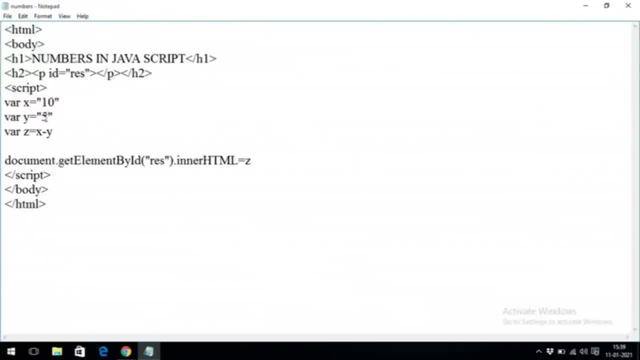 variables are strings and we are applying other than the addition operator. the strings will be converted into numbers and again you can observe x divided by y. again it will give the result at two. So 10 divided by 5- numerics, okay. and even 1 integer and 1 string will also give the same result. 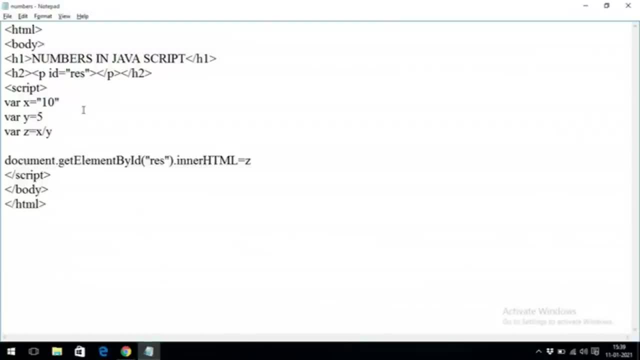 okay, So other than the addition operator, other than the addition operator, all remaining arithmetic operators. for all remaining arithmetic operators, the strings will be converted into numbers. right? And what about this case? js divided by j s. So this is a numeric string. this is a non-numeric string In such cases. 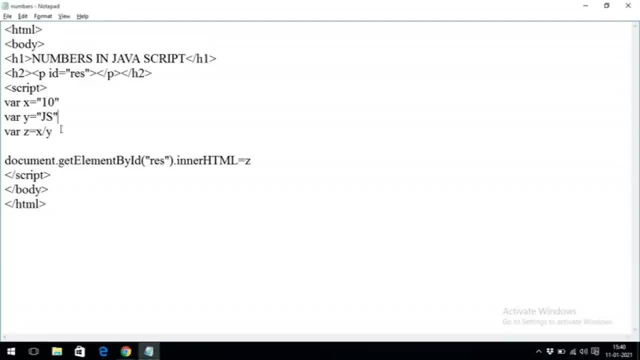 we will get a, not a number, not a number. n, a, n. So here any expression is having- with a I mean any arithmetic expression- is having a non-numeric string, automatically we will get the result as nan. that is, a, not a number, not a number. So here you can observe: x is 10,. 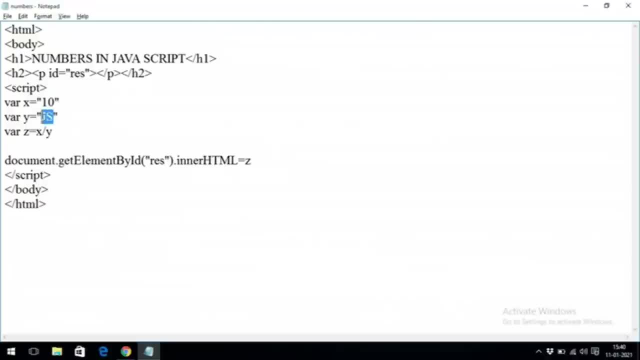 it is a numeric. y is also a string, but it is a non-numeric. So obviously we will get the result as not a number. And what happens if it is 0?? What happens if it is 0? We will get infinity. either it is a negative value or a positive value. divided by 0 will give. 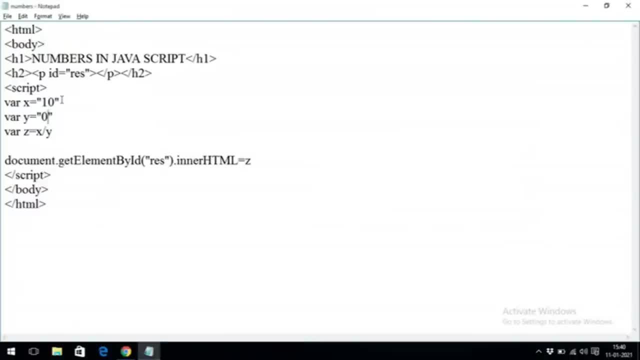 the infinity. ok Now, and one more thing. it is a number conversion, So we can convert any number from one system to another system. If you, if you are having some x is equal to 10, we can convert it to see. 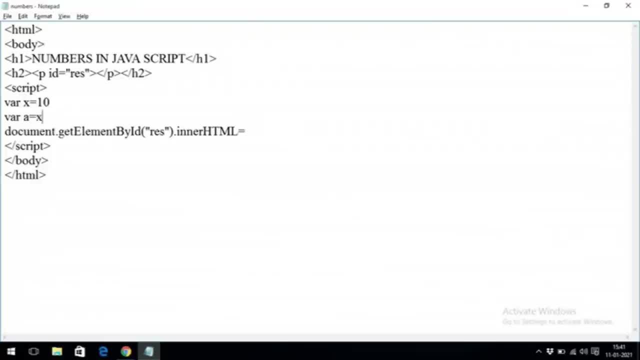 where a is equal to some x dot, there is a function called 2 string, 2 string of 2.. If you give a 2 as an argument here, if you give the 2 as an argument, the result will be in a binary form. 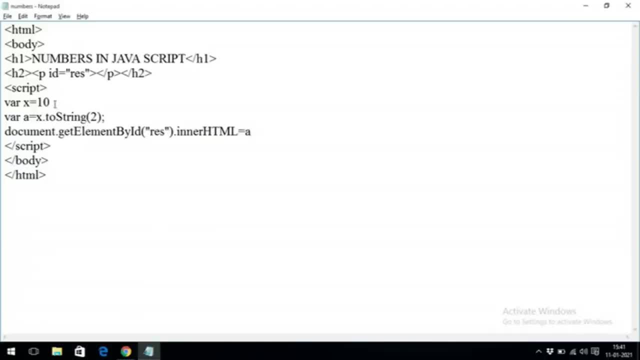 you can observe. ok, This is a binary format for 10.. If you increase this one- 15,, you can get the 15, binary format. And if you want to convert into another way, so octal, just give the 8 as a. 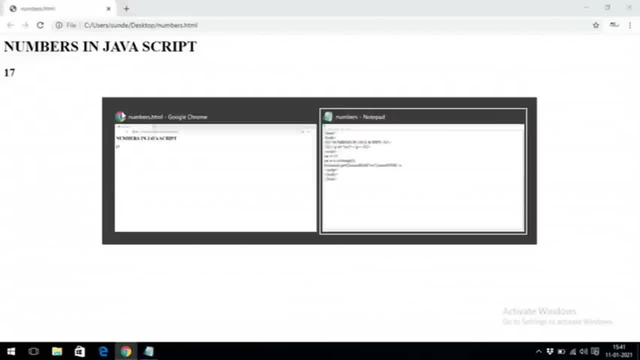 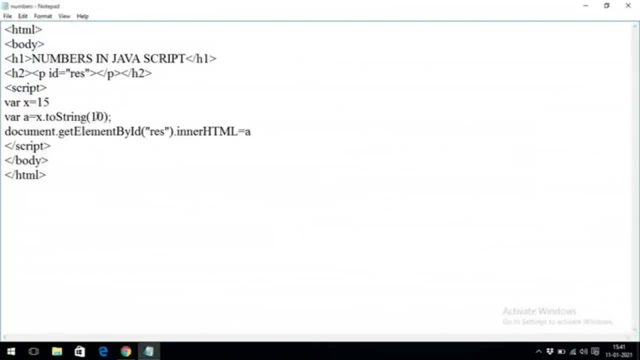 argument 2: string argument 8, it will return octal value. So 15 is a integer value, 8 is an octal value And the decimal value is normal 10,. ok, Decimal value is 10, base 10.. So that base. 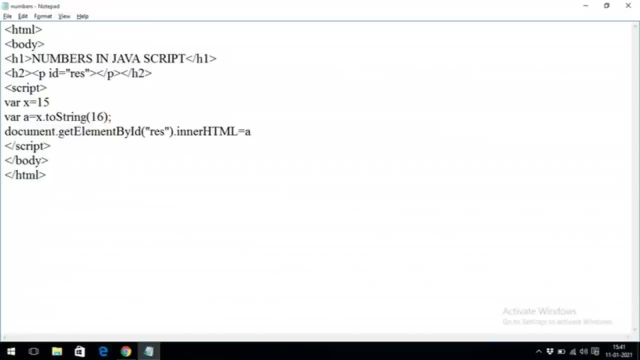 should be given as an argument to the 2 string. So this is a binary format for 10.. So if you want to convert it to a string function, if it is a 16, so 16 is a base for hexadecimal. So 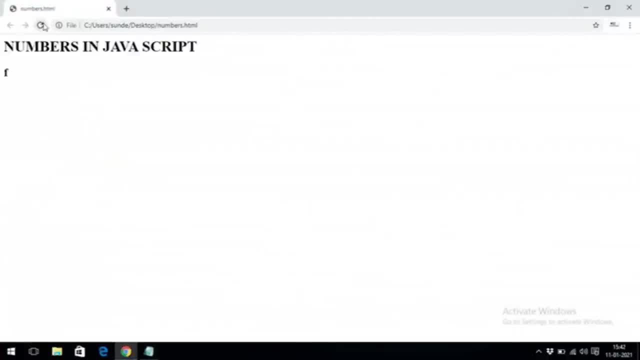 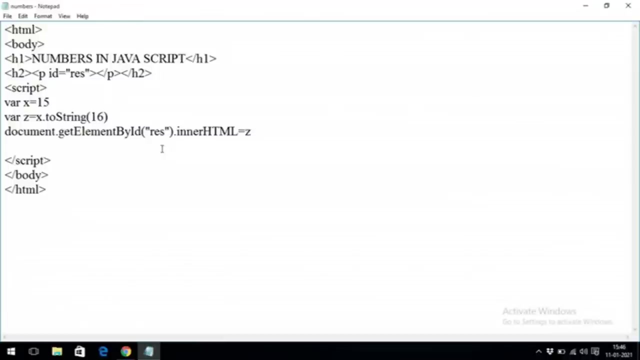 15 will be displayed in hexadecimal right. So this is the function 2 string to convert from one system to another system. Hope you understood this concept. So working with the numbers. so we have seen the integers, float, scientific notation in the precisions and the combinations. 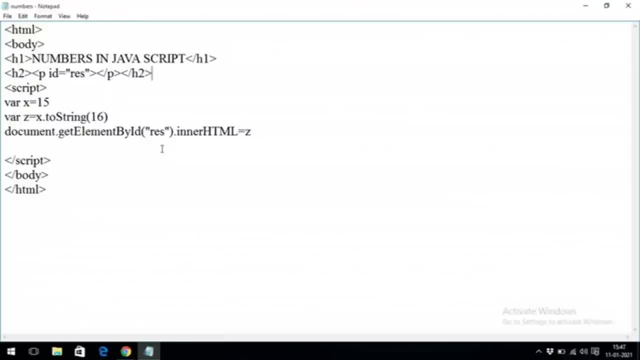 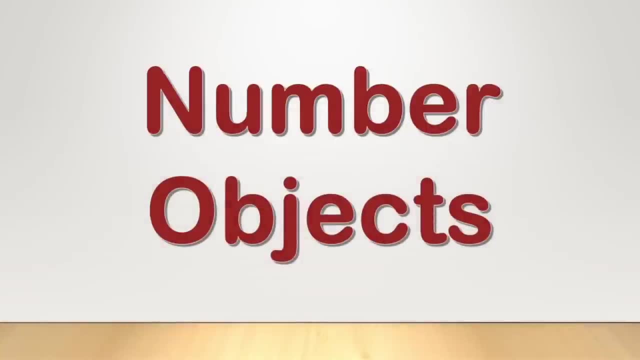 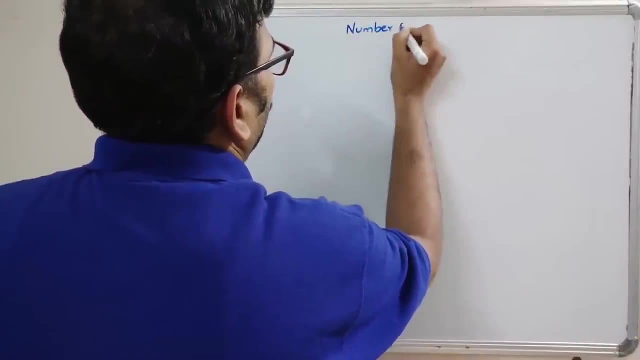 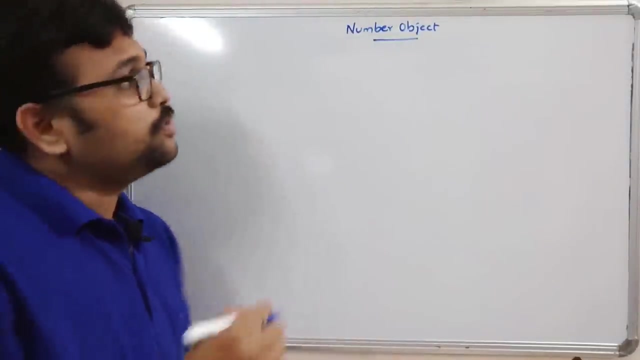 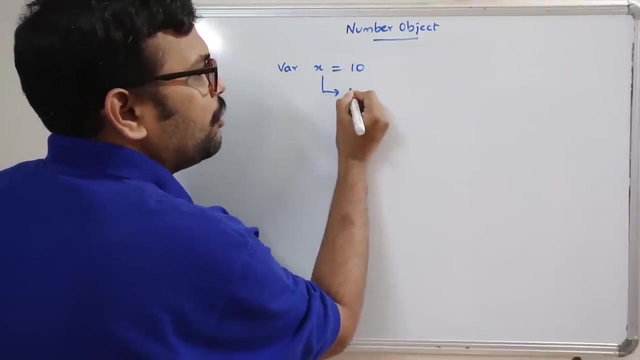 of numbers and strings, and also not a number and the infinity and the number. these are called the set-conservative, set-conversion- See coming to the number of objects. so it is completely different with the numbers. ok, So if you are creating some variable, some x is equal to 10, so this x is of type number. Similarly, 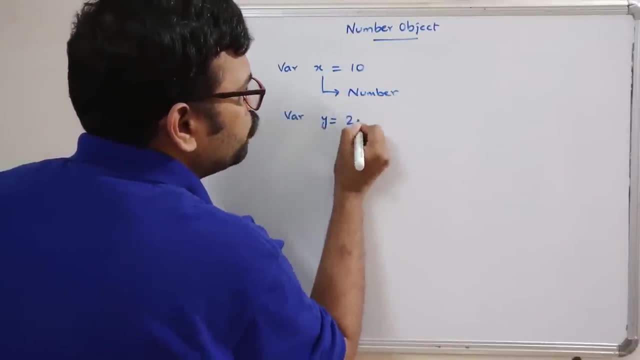 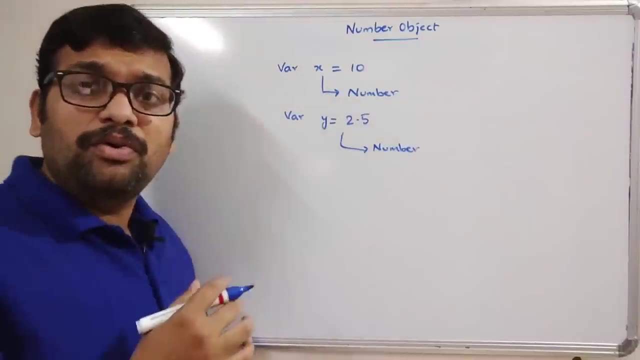 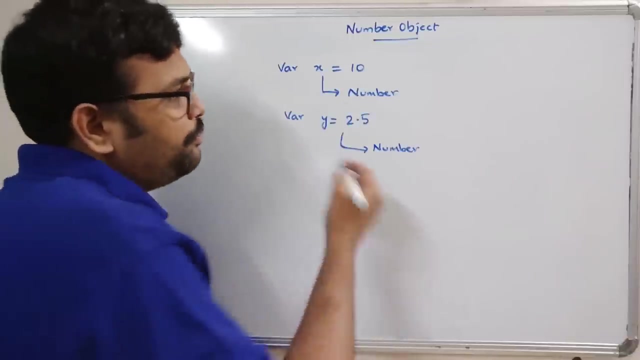 if you are declaring some variable with y equal to some 2.5, this will also be of number. so one thing: how? how can we know whether the given variable is of which data type? that means either it is a number or a string. so for finding this one, we are having a small keyword called type of. so by using this type of 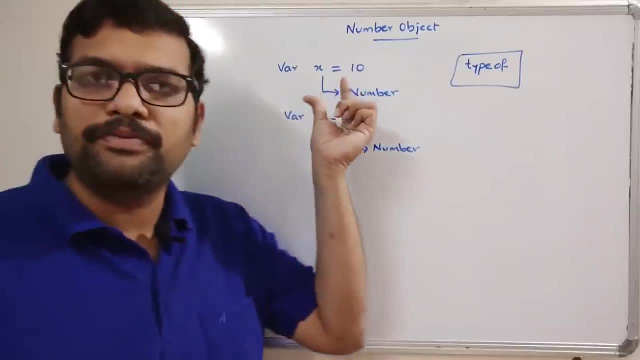 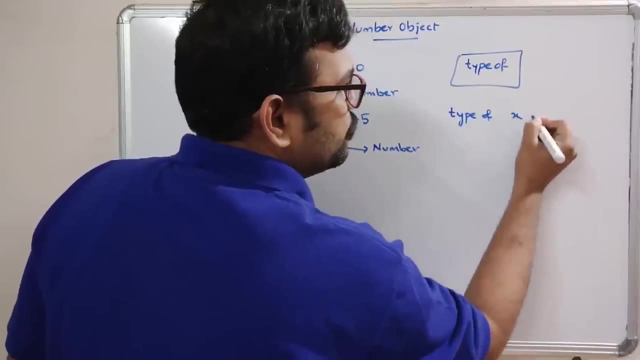 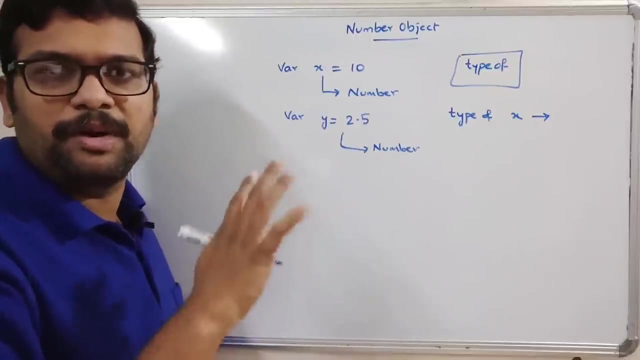 we can know what exactly the data type of the particular variable. so if you want to check the x, we have to go with type of x, so it will give either number or a string, or it's an object. okay, number, string or object, whatever it may be, the data type of this variable will be given here. 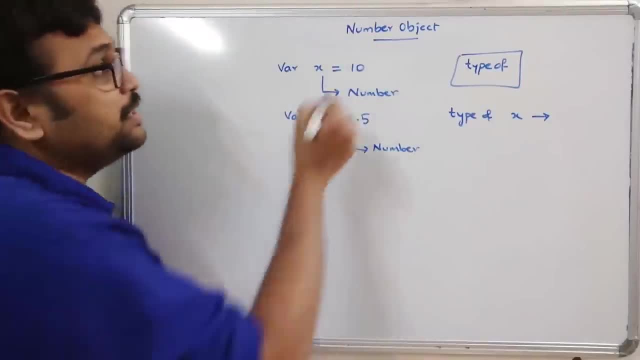 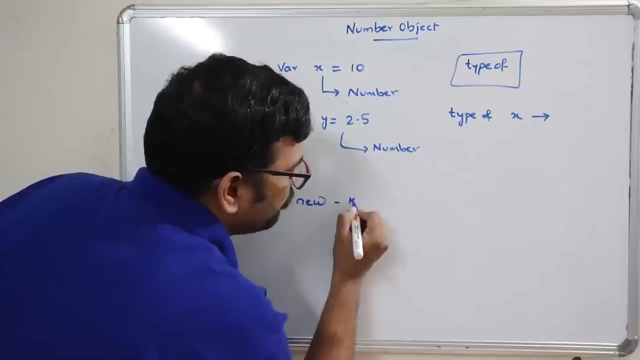 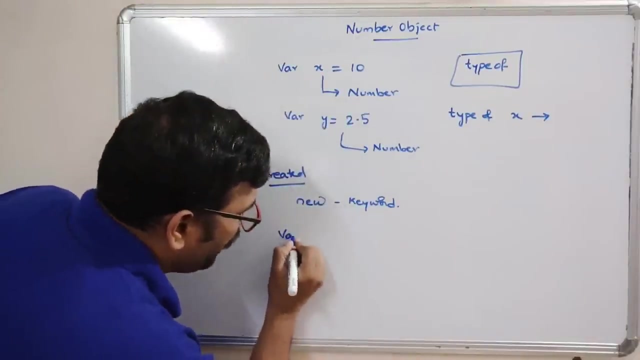 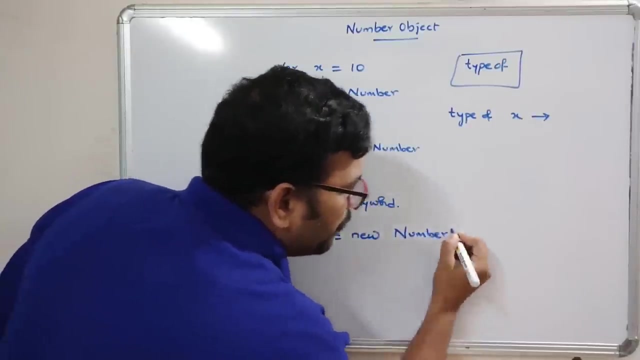 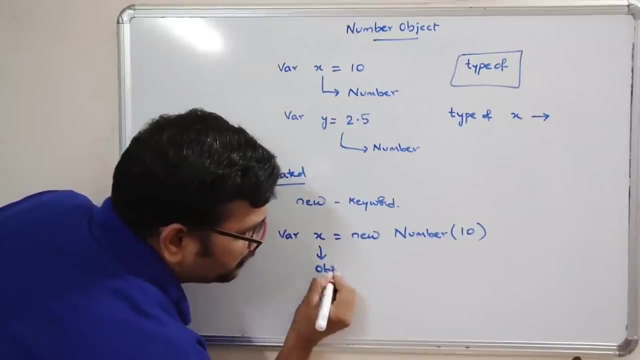 so if you want to create a number object, then this number object can be created by using new keyword. new keyword: okay. so how to create a number object? similarly, where x is equal to new number, n should be capital here. number of. give the value here some 10 right now. the type of x is an object, it's not a number. 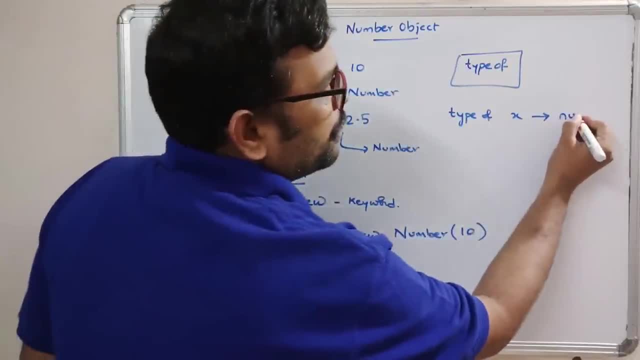 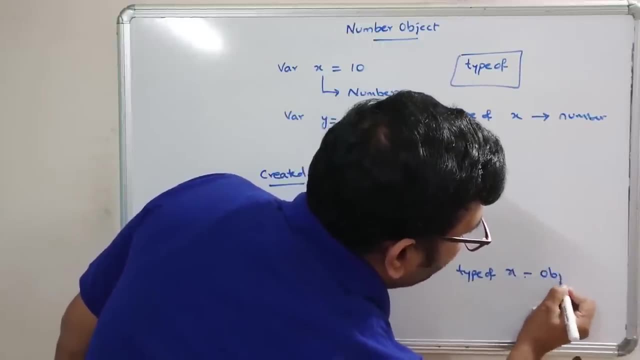 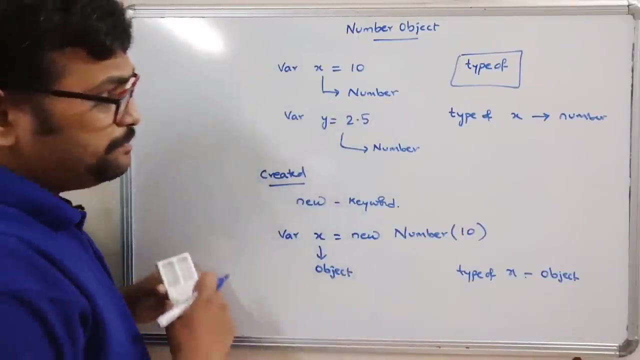 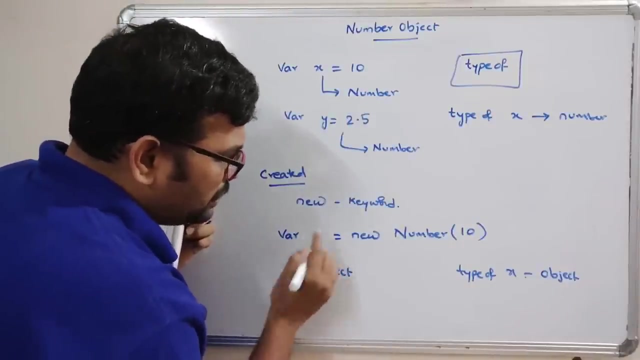 in this case the type of x is number right and in this case, type of x will be object object. so objects will be created with the help of a new keyword. right now, if you compare these two things, okay, if you compare these two things, for example: consider y here. okay, consider y here. so x is equal to 10 and remove this one. 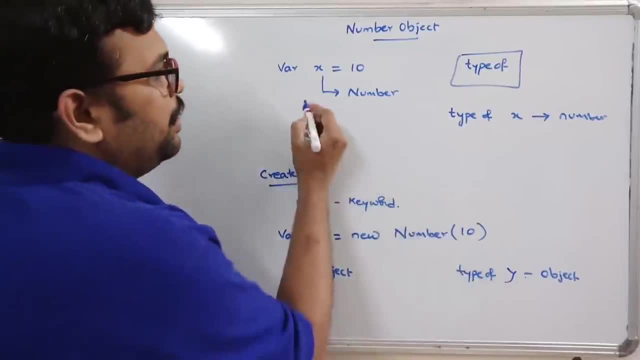 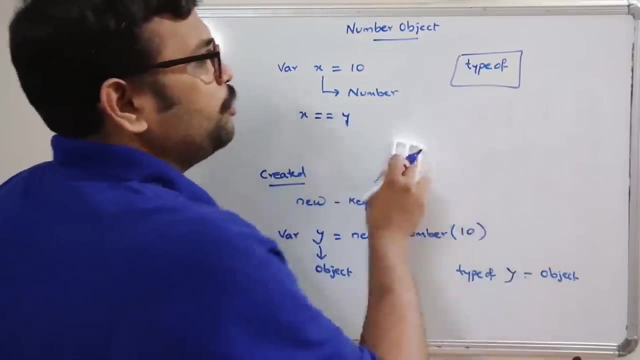 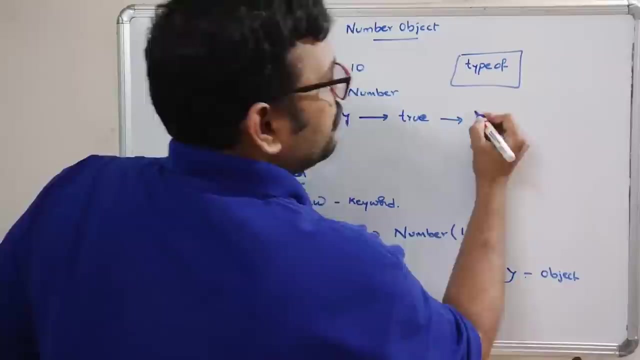 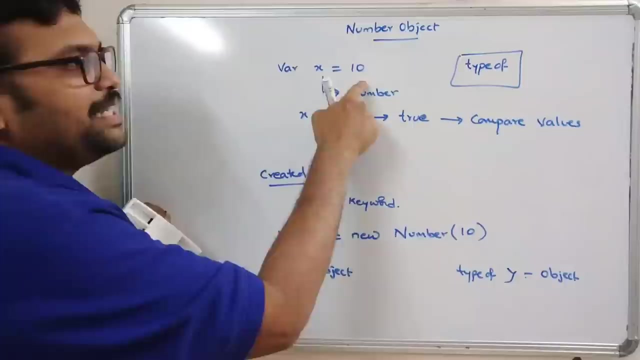 x is equal to 10 and y is equal to 10. if you compare, x is equal to is equal to y, x is equal to is equal to y, automatically this will return true because- because it will compare the values, compare values. okay, so the value of x is 10 here and here also the value of y is 10, so x. 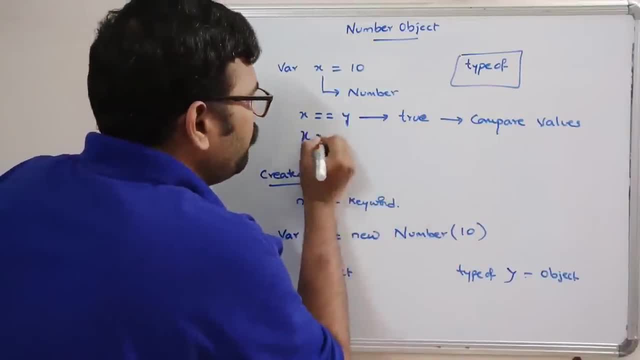 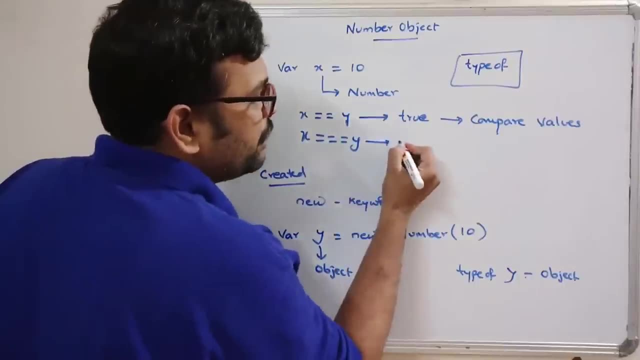 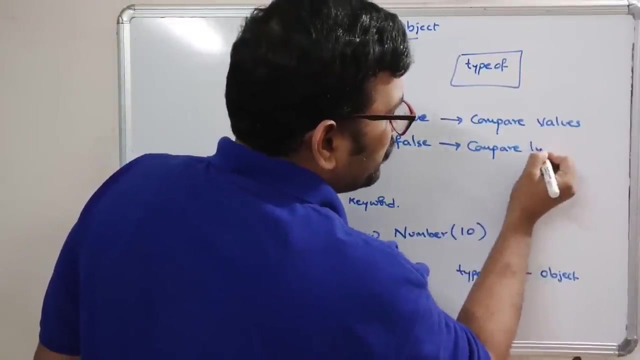 is equal to, is equal to. y is true, and if you go with triple is equal to, so here there is a one more operator called triple is equal to, so triple is equal to, then it will return false, because it will compare data types. so it will compare types. so here x type is number, y type, 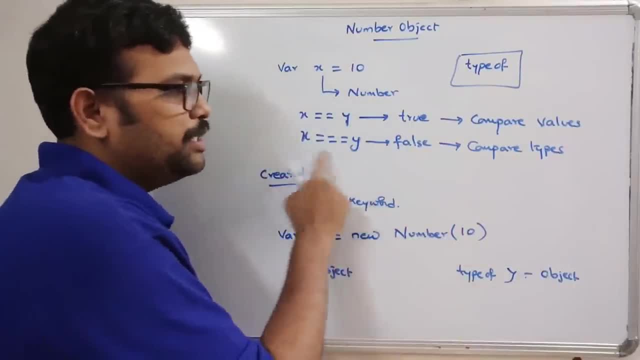 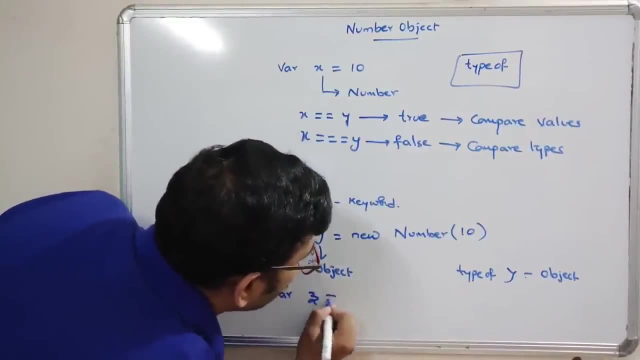 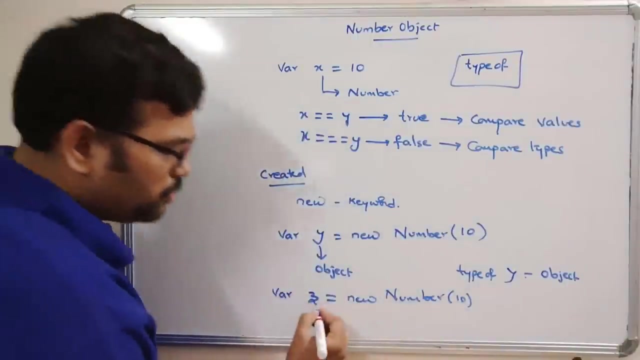 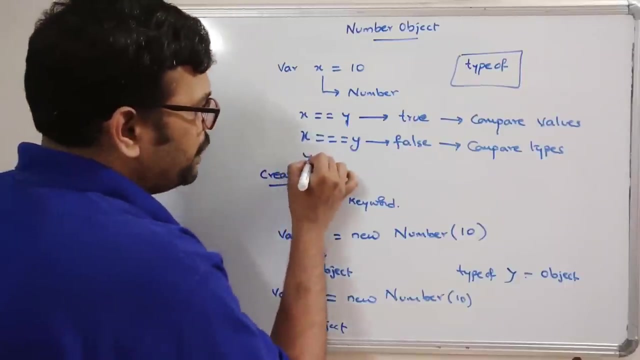 is object. so both are different. so if you compare these two, we'll get the false as a result and similarly see where z is equal to some new number of 10. so here you can observe. so here z is also an object right, z is also an object, y is object, z is object, and if you compare these two, y is equal. 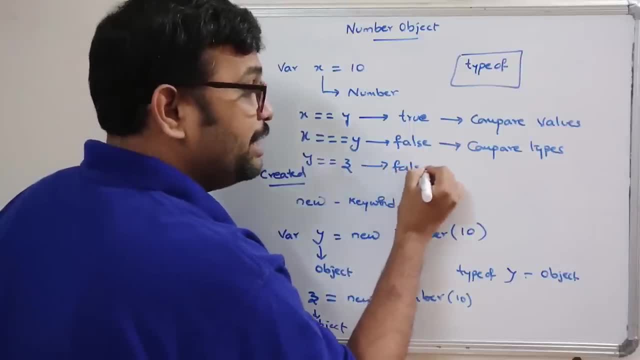 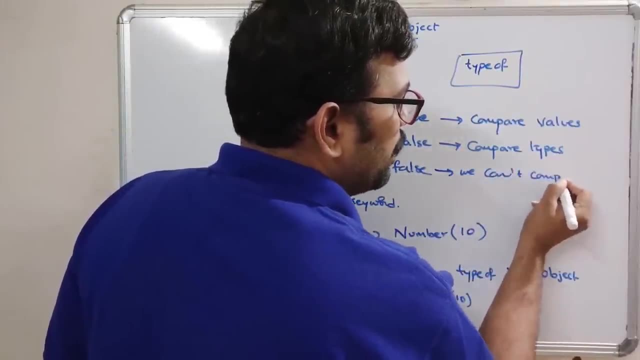 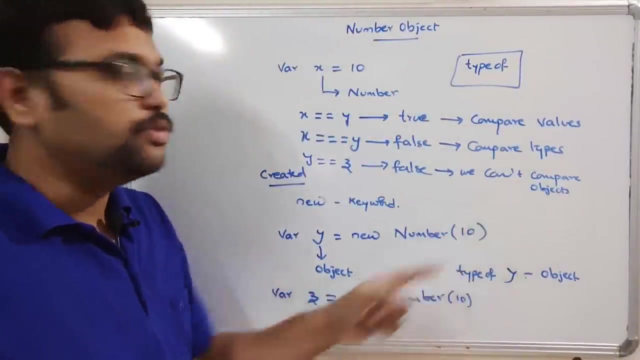 to is equal to z, it will return false. and it will always return false because we can't compare. we can't compare, compare the objects, so objects should not be compared. okay, we can't compare the objects, so this is the difference between all these things. okay, this is the difference between all these. 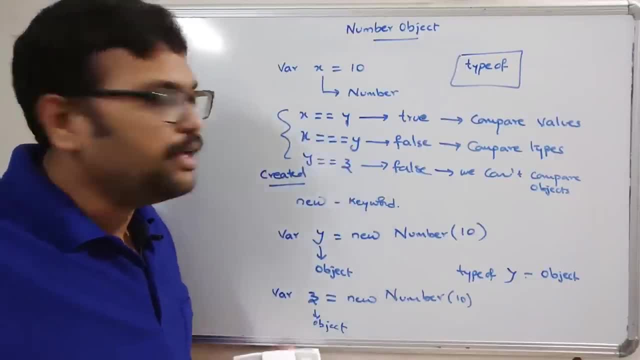 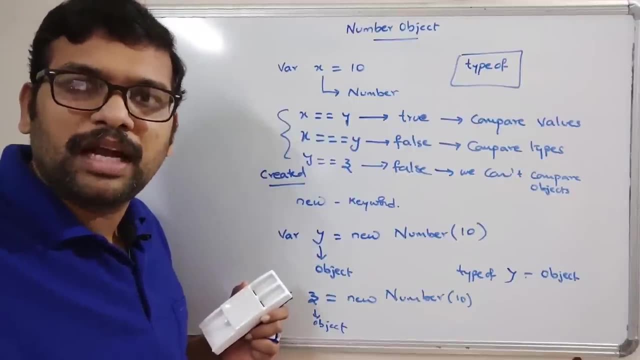 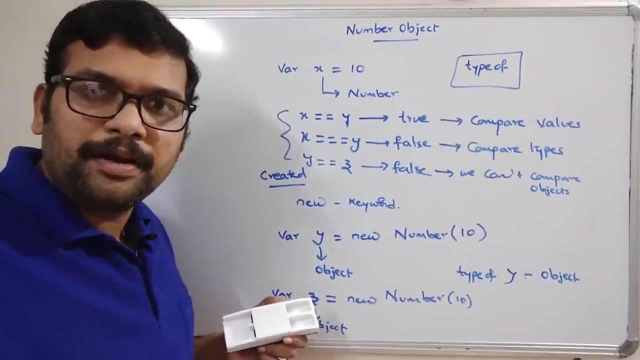 things. so is equal to, triple is equal to and again equal to. so if both are values, then we have to use a double is equal to. if both are types, if you want to compare the types, we have to use a triple is equal to n. objects should not be cut there. now let us move with the methods. so there are a few. 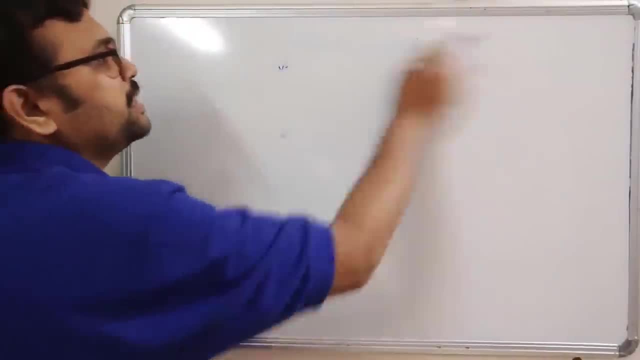 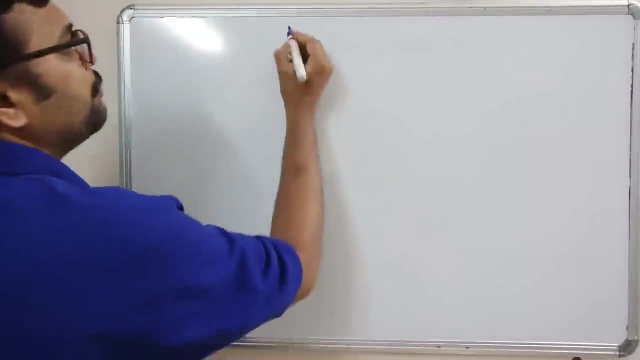 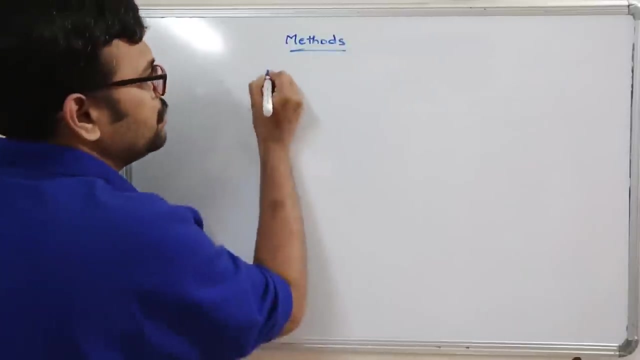 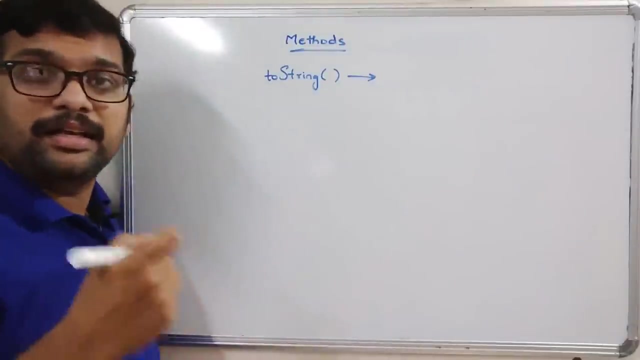 methods that can be applied on these numbers and the number objects. so now, number methods will go with the number methods. so one method we have seen in the previous session, that is a two string, two string. so this two string will be, uh, returning the string from any other variable. 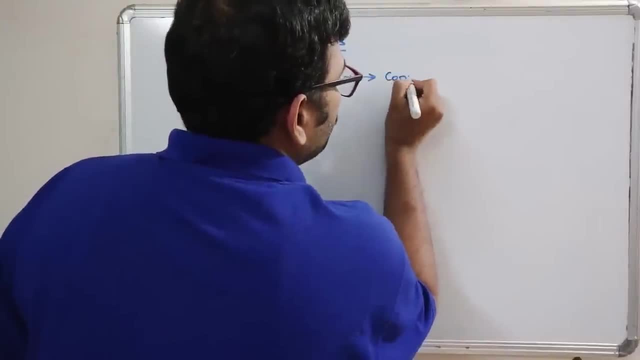 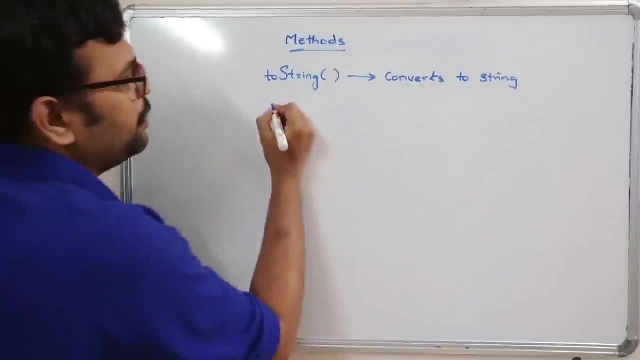 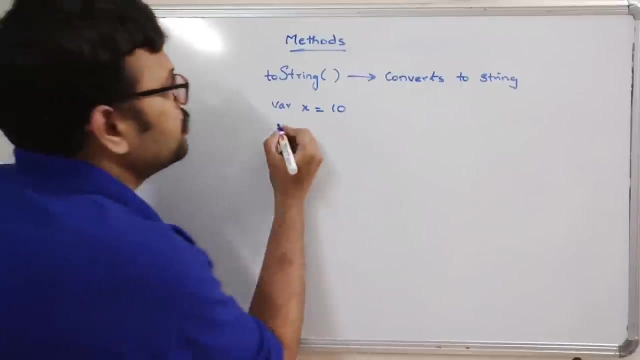 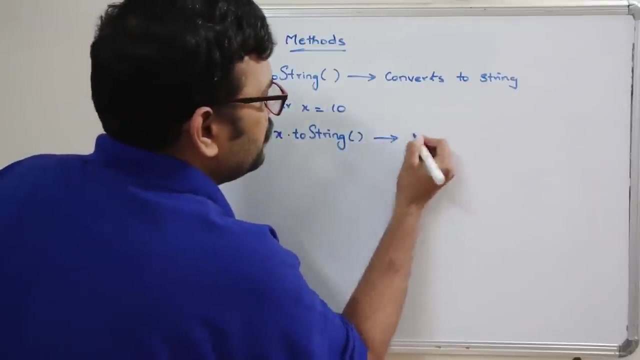 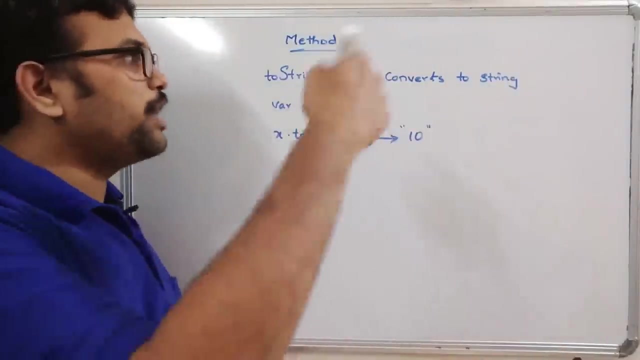 right, so converts to string data type. converts to string data type. for example, where x- is sorry for, where x is equal to 10. here 10 is a number, so x dot two string. so s s is a capital. right, s is a capital. it will return 10 as a string, 10 as a string. similarly, some float value can. 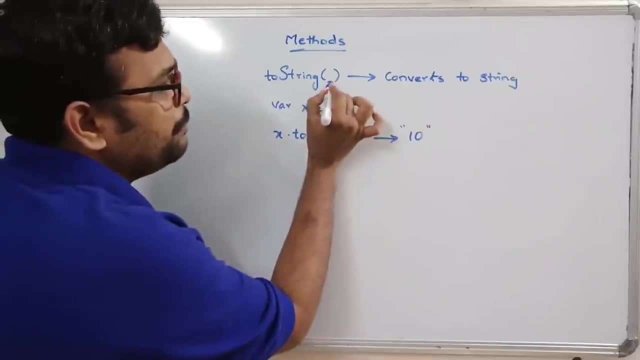 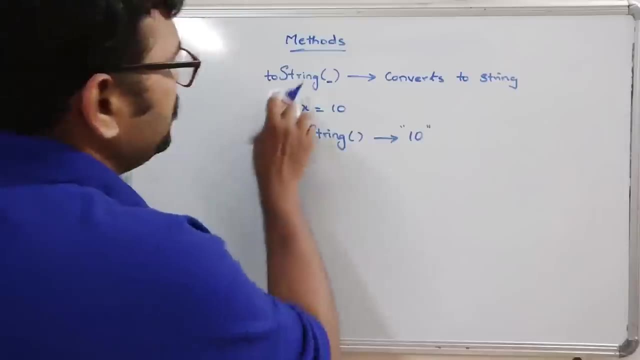 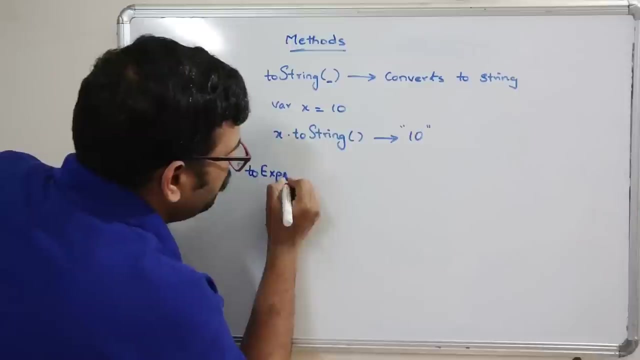 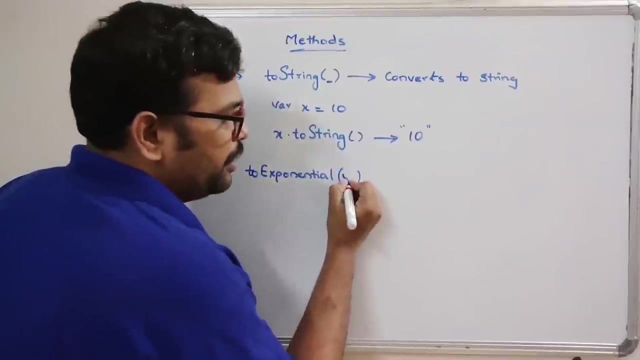 also be converted into a string. and also, if you give any base value here, automatically it will convert from one number system to another number system, right? so this is one method. and the second method is to exponential to exponential. so here we have to give the value here, and whatever the value we are given, that will. 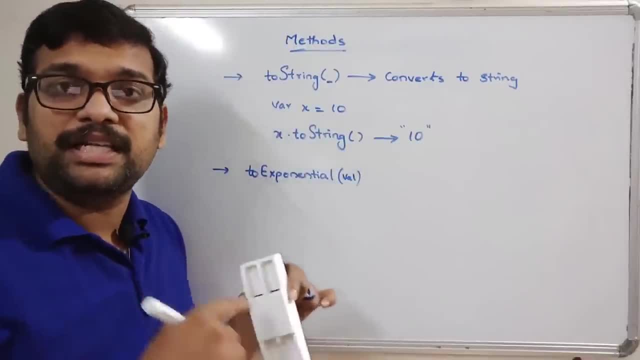 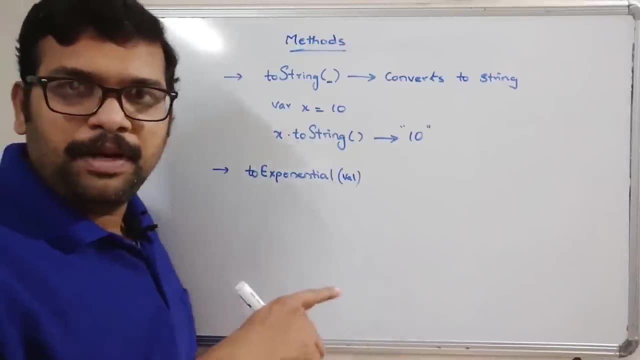 be applied to the number and that number will be represented in a scientific manner- that means exponential- with the help of exponential right. so i will show you an example by executing small code. and there is a one more example by executing small code. and there is a one more example by executing small code. and there is a one more. 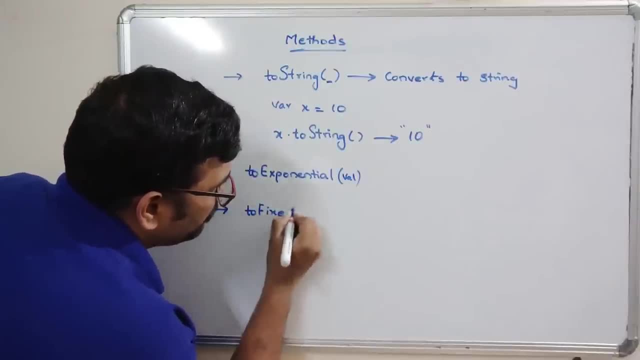 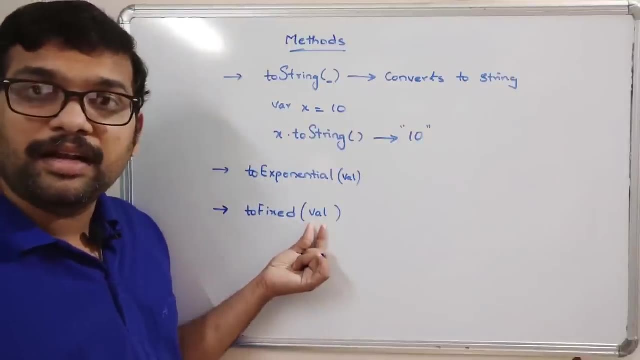 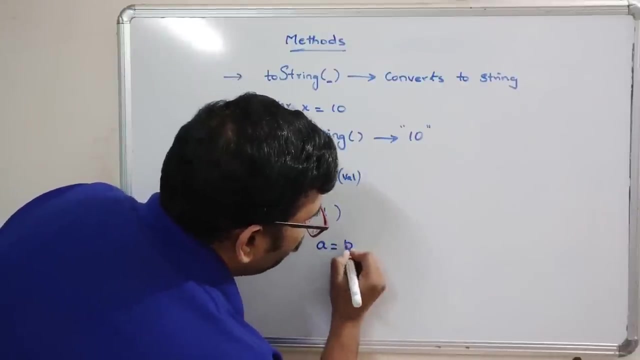 method called to fix it. to fix it, and here also we have to give the value so that the value will be taken consideration and it will be rounding up the number right. for example, if a is a is equal to 5.4567, and if you are 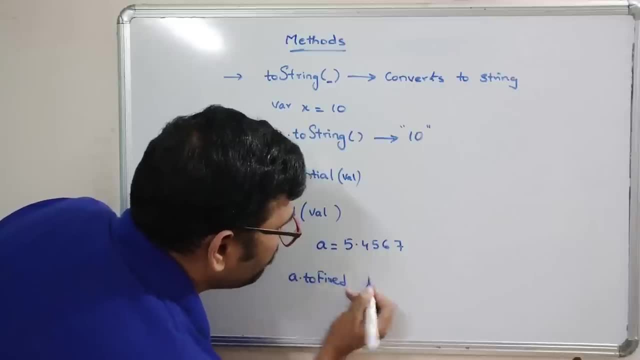 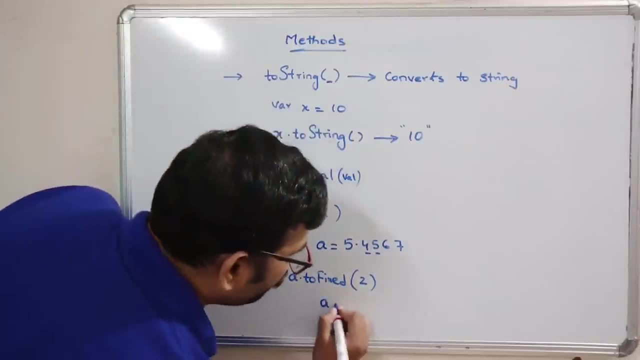 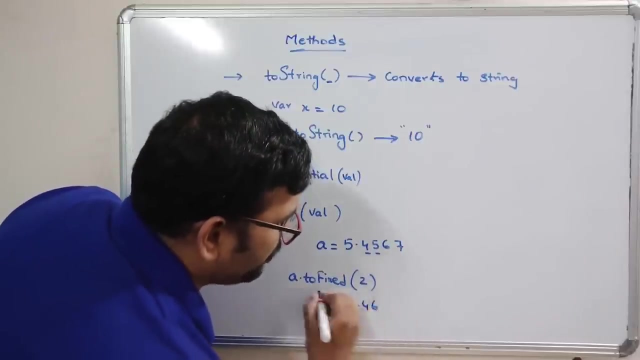 doing a dot two fixed f is capital here, two fixed of two. so only two decimals will be taken up to two decimals, so a value becomes after executing this one: five point, four, five. so four, five will be rounded, so four, six will be printed here. four, six will be printed. okay, so five point four, five, six. 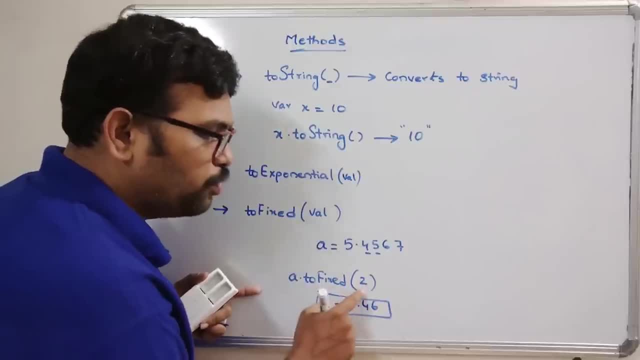 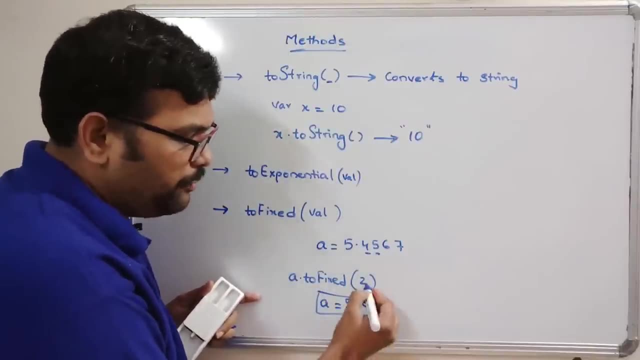 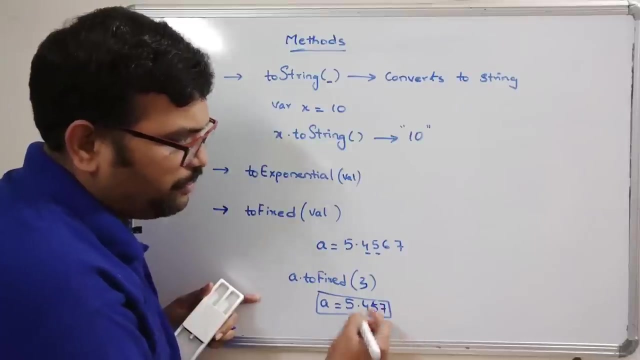 seven. so a two, a dot, two fixed of two. that means it will round up to two values. so four, five, it will print display four, six, right, if you are giving three, then four, five, six. so it will print four, five, seven. it will round up the third up to third value. so i will execute the program so that 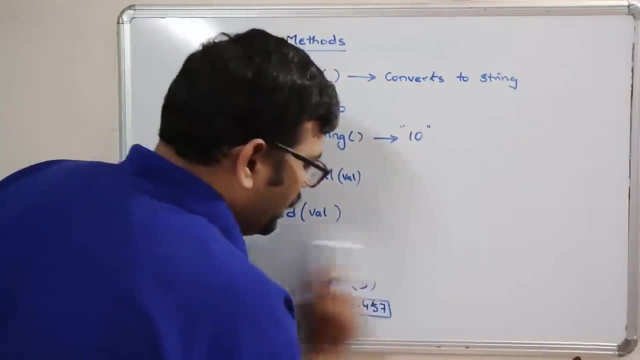 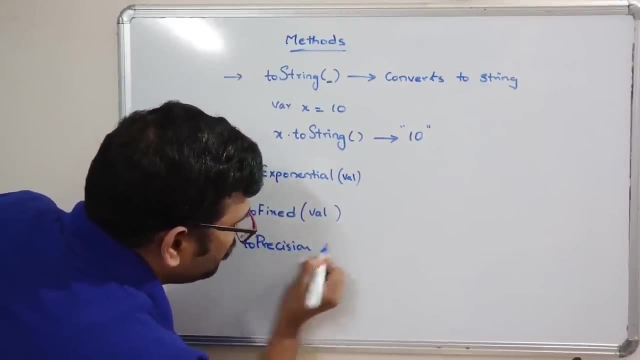 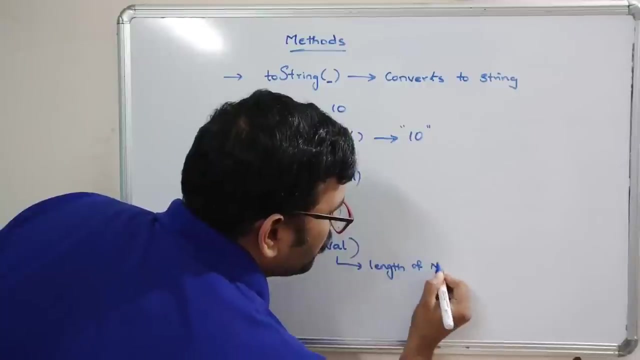 you will, uh, your doubts will be clarified right now. again. there is a one more function called to precision, to precision and give the value, and this gives the length of the number, length of the number. so how many numbers, how many digits should be, uh, accepted, for example? similarly, 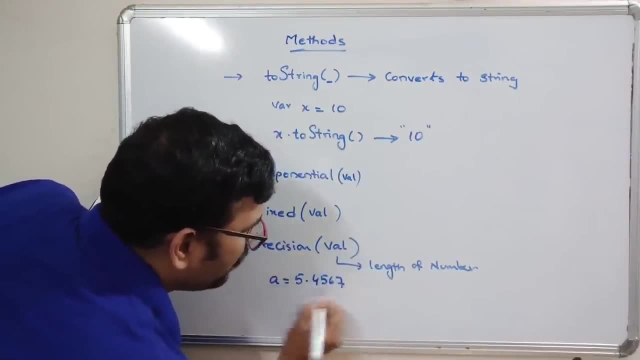 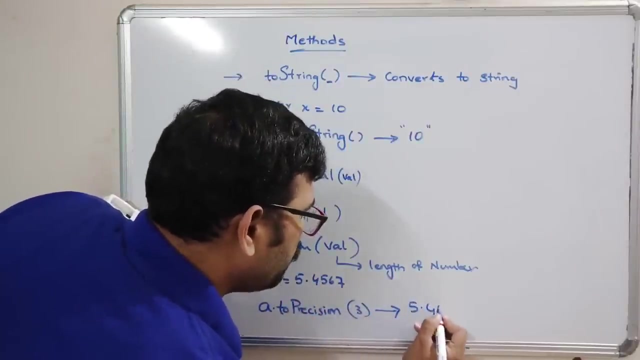 a five is equal to five point four, five, six, seven and a dot two precision, a dot two precision of three. so it will return only three. the length of the value should be three, so it will return so five point four, five. so total values are five oh three. okay, total number of the length of the. 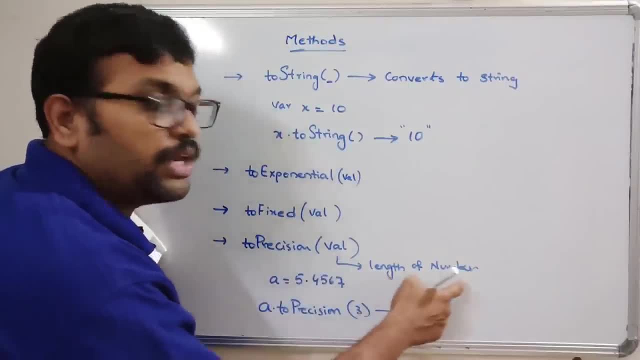 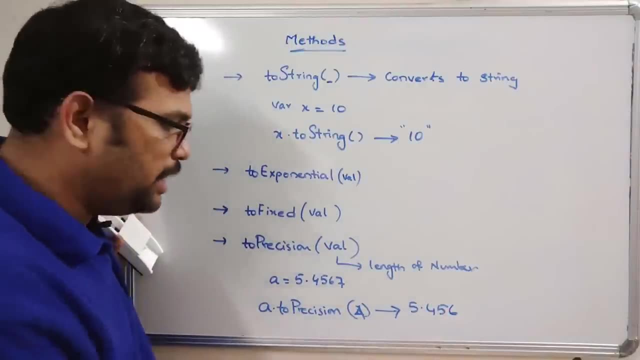 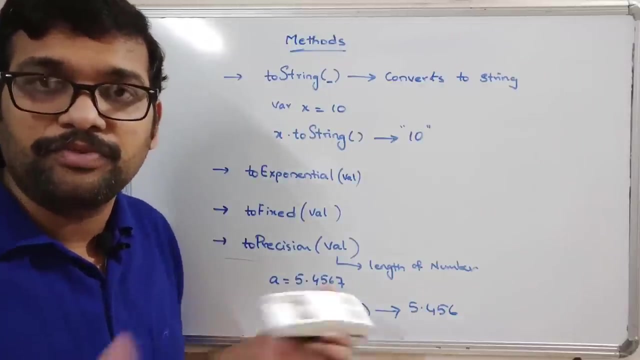 number is three, so this value represents the length of the number. okay, if it is a four, so automatically four, five, six, so total length is four. so, like this, we can use this to precision, to reduce or increase the value, the length of the value, the length of the number. right, so i will. i will execute all these. 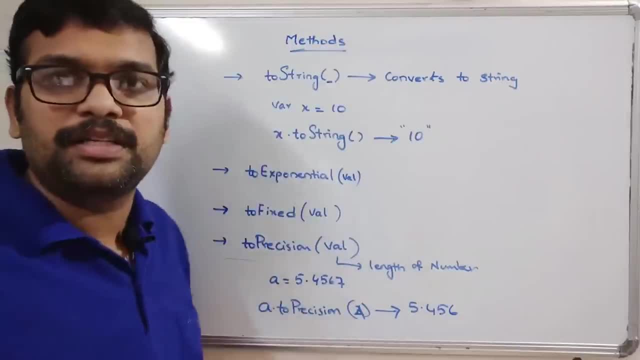 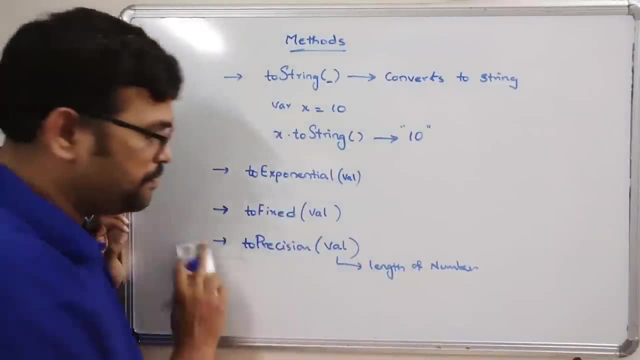 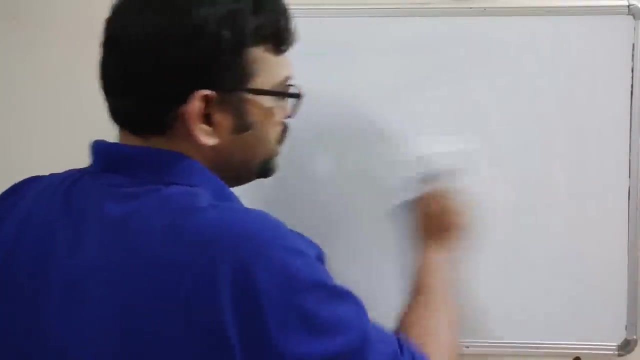 functions. these are the methods available and i will execute all these methods by uh. in the in the html code, we write some html code and i will execute all these things and after the methods now. so, whatever the methods we are using, uh, either two string or two fixed or two exponential or two precision, the written state. 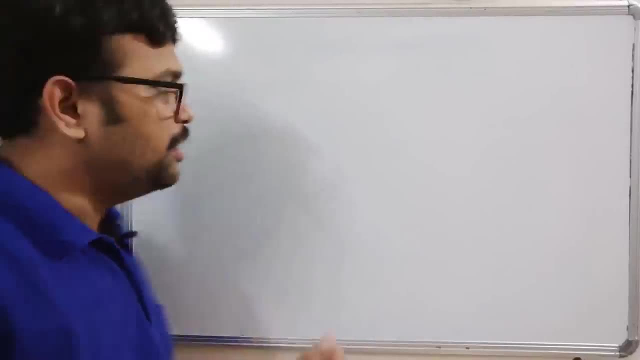 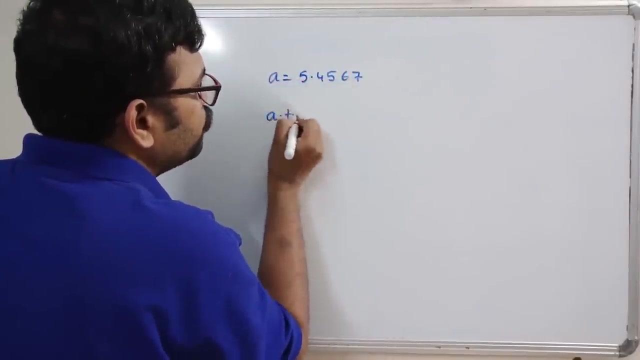 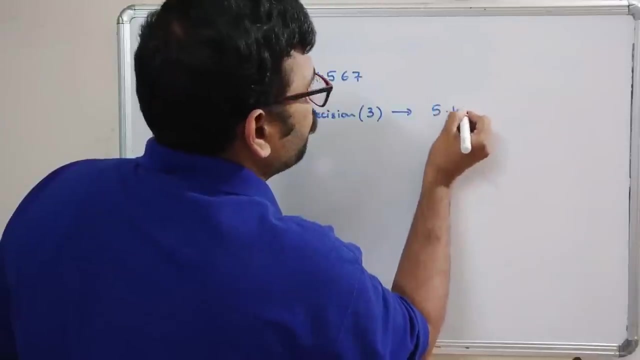 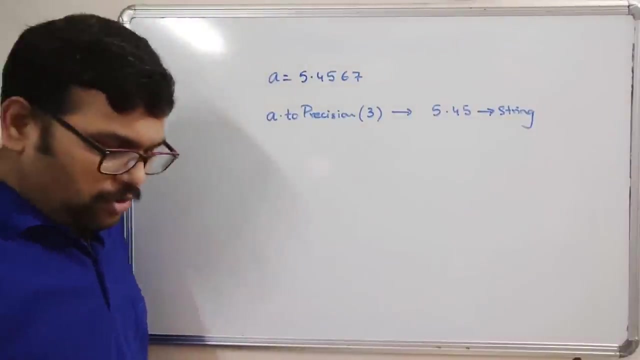 the written value will be in the form of string. okay, so, for example, some a is equal to five, point four, five, six, seven and a dot two, precision two, precision of three, the result will be 5.45 and this is in the form of string. this is, this will be in the form of string, so we need to convert into: 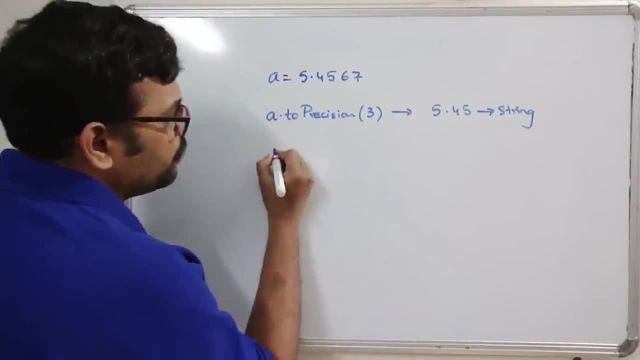 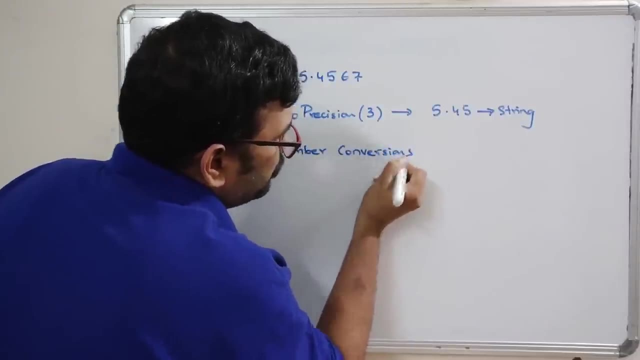 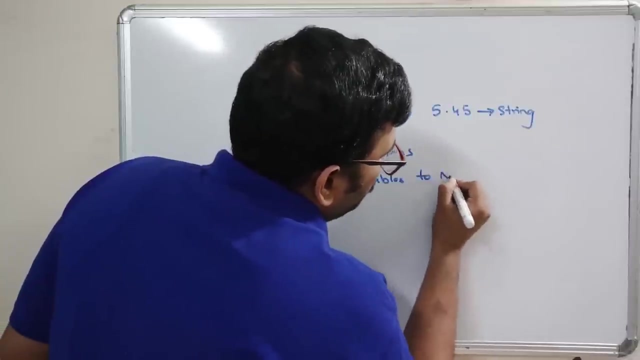 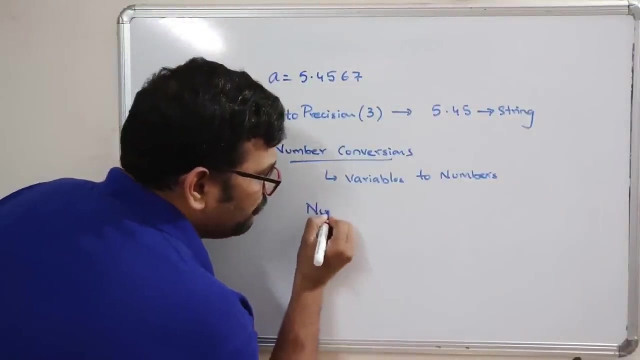 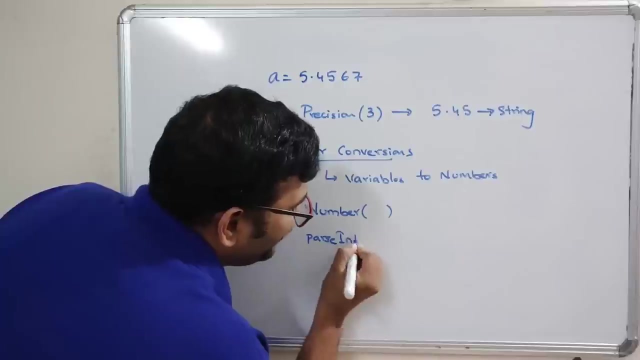 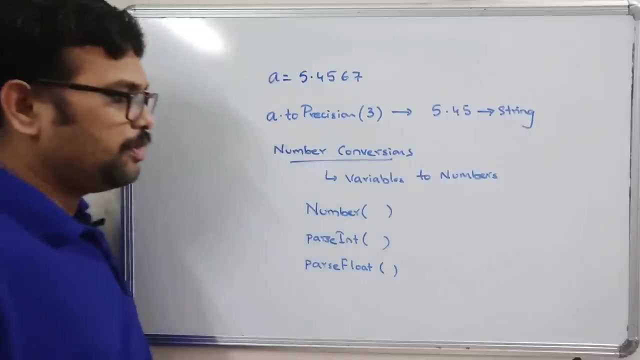 numbers if you want to convert into your numbers. there are some number conversions, there are some number conversions, so, which will convert the variables to numbers, variables to numbers. so for this we are having the functions called number, parse, int, parse, float. okay, so these functions will convert the variables to numbers. so 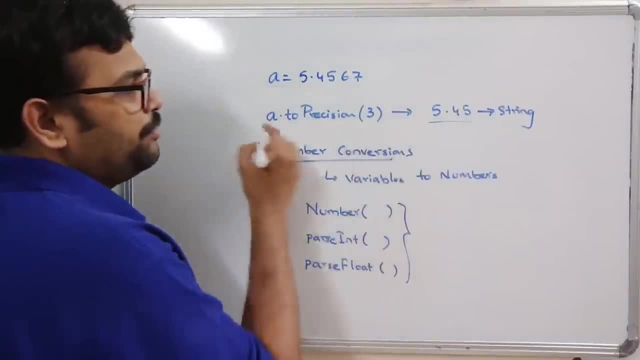 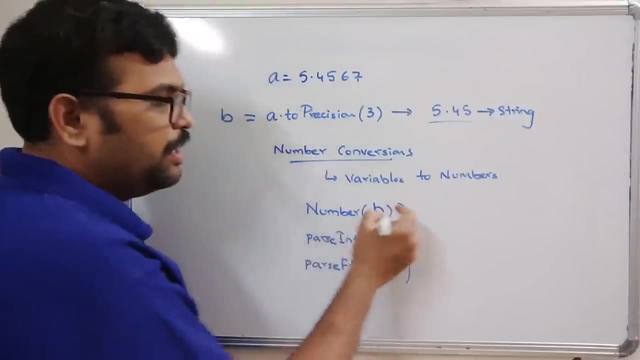 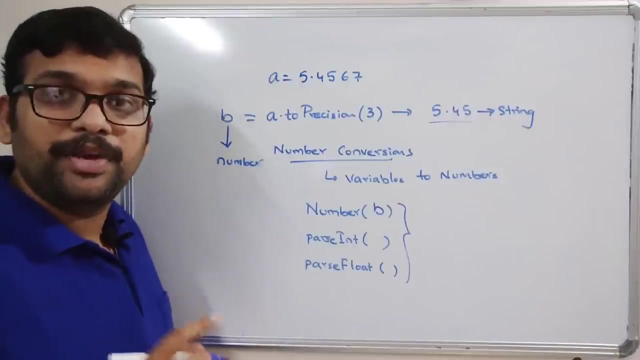 for example you, you take this one and if you initialize it to any other variable, so b will be having some 5.4 file. if you pass this b here, automatically the data type of b will be number. the data type of variable b will be changed to number, so initially now. so whatever the uh. 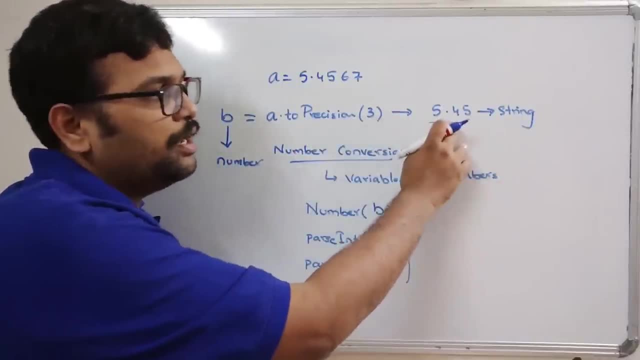 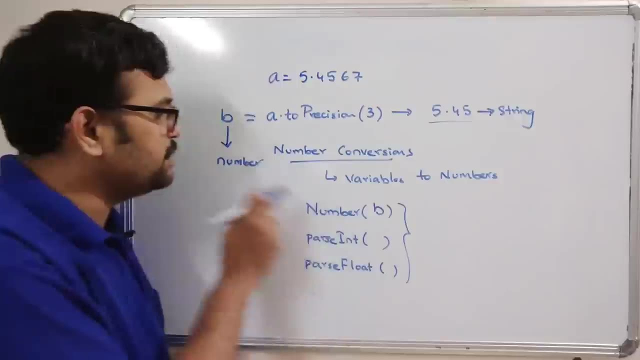 i mean value. we are applied to the precision. the result will be in of string. and again, if you are passing the value to the number function or parsing function or a parse flow function, we will get the result as a number. so this will give the result as 5.45. it's a number and if you 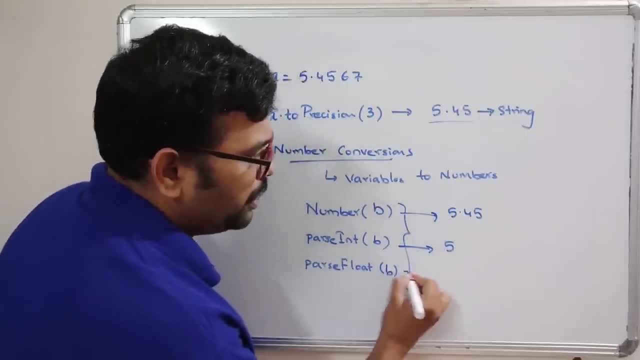 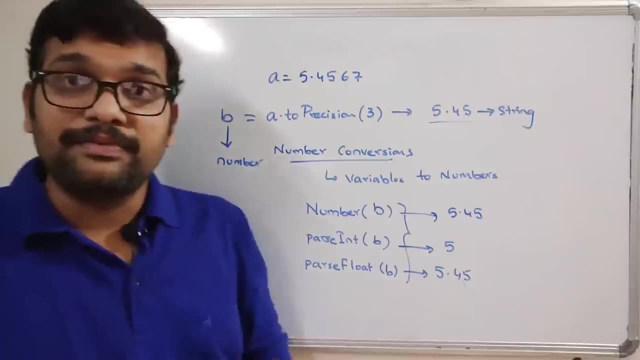 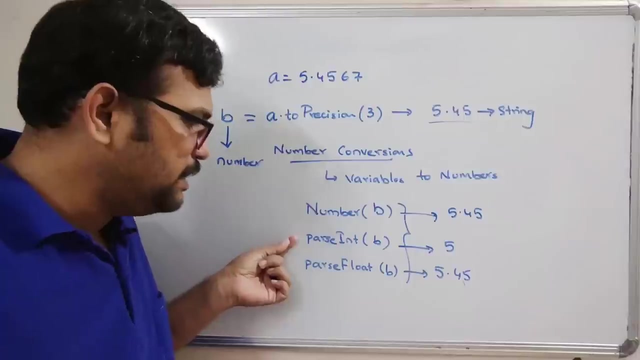 give this here, it will return only 5.. if you give here, we will, it will return 5.445 right. so like that, we can convert the variables to numbers by using one among these three functions: number function, percent and a parse float right. and apart from these conversions, we are also having some. 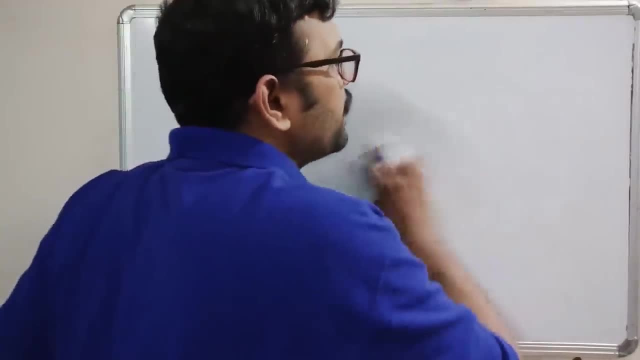 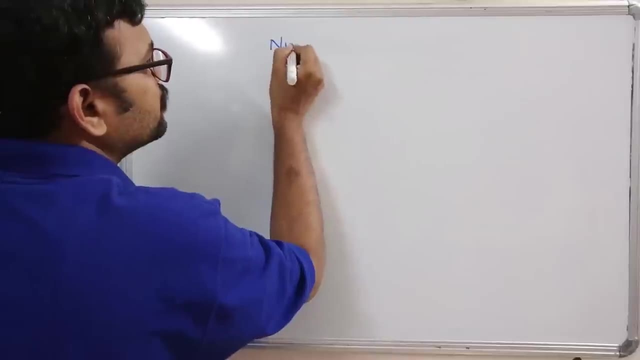 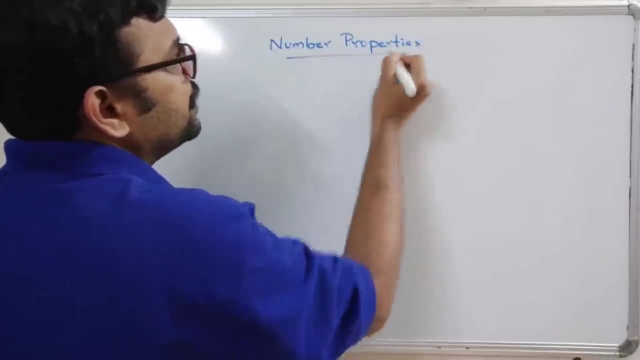 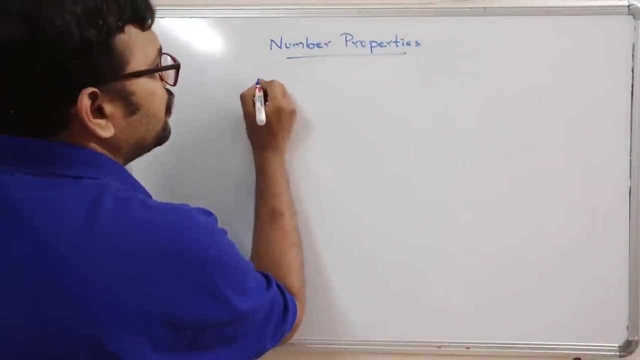 properties, number properties. so for variables we can't apply these properties. for only the numbers we can apply the properties. so there are different properties. those are called number properties, number properties. so this can be applied only for the numbers right. so the first one is capital letters, min underscore. 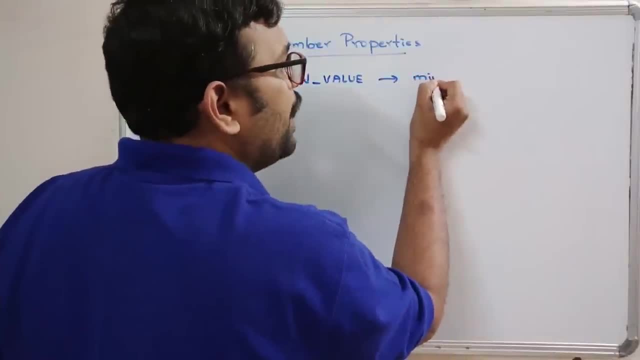 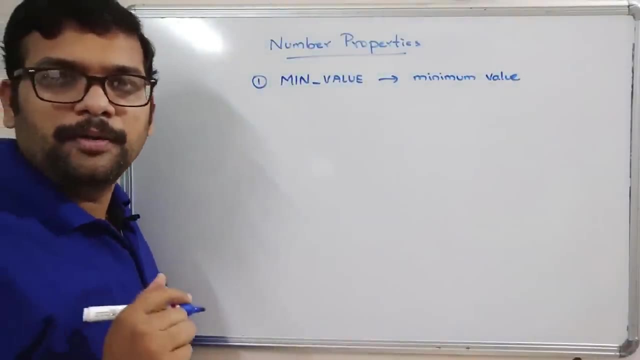 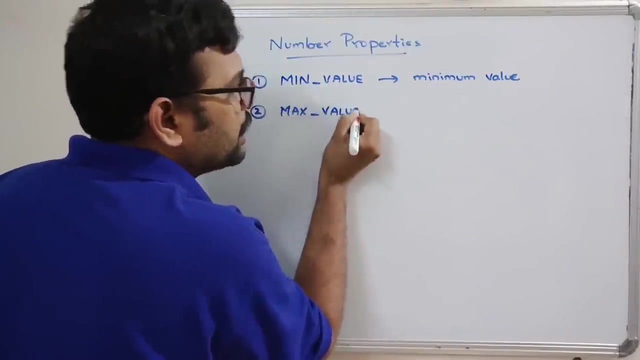 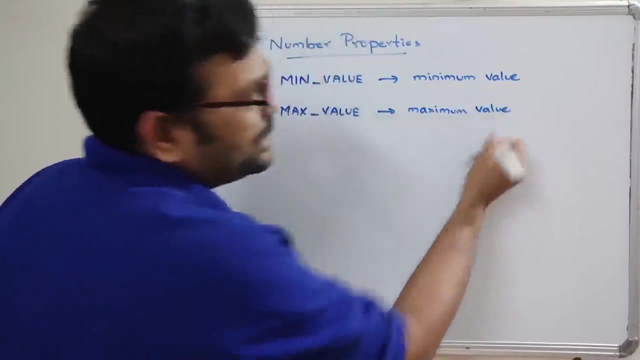 value. so this will return the minimum value, minimum value that the javascript variable will hold. okay. second one is a maximum value, max underscore value. all are the capital letters. this will give the maximum value that a variable can store in javascript. okay, that a variable can store in javascript: a maximum value. 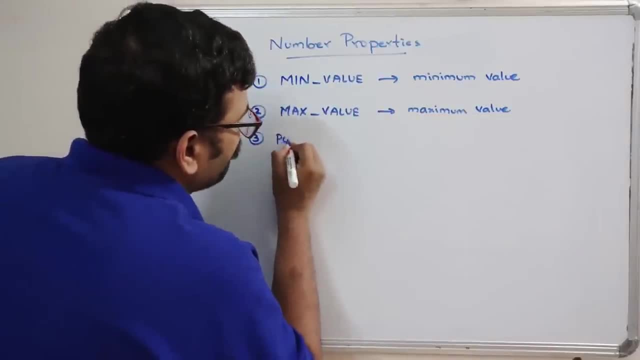 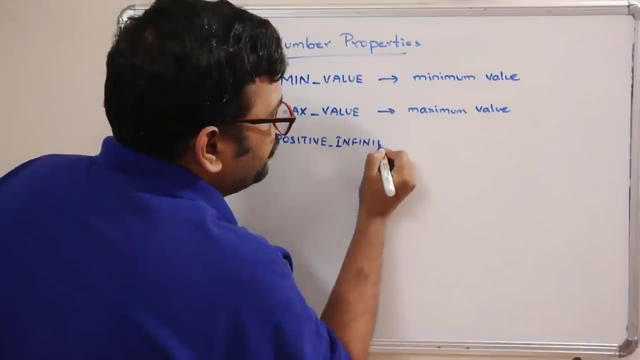 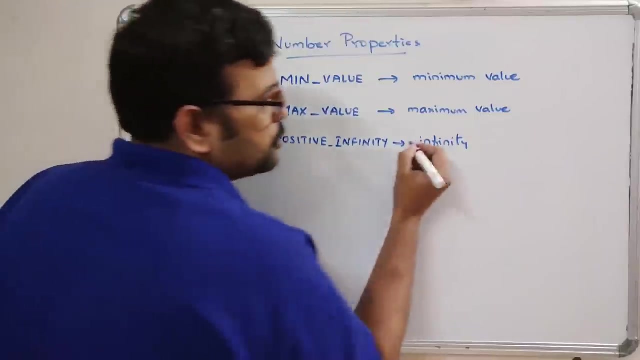 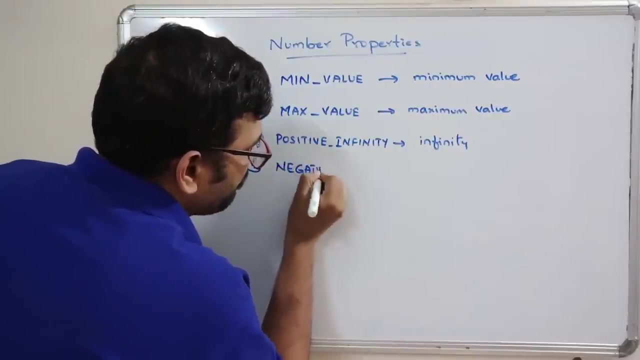 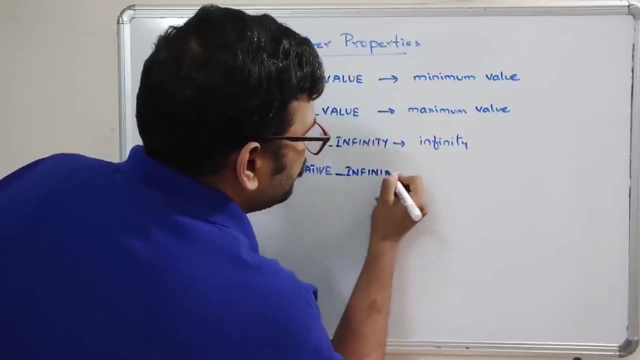 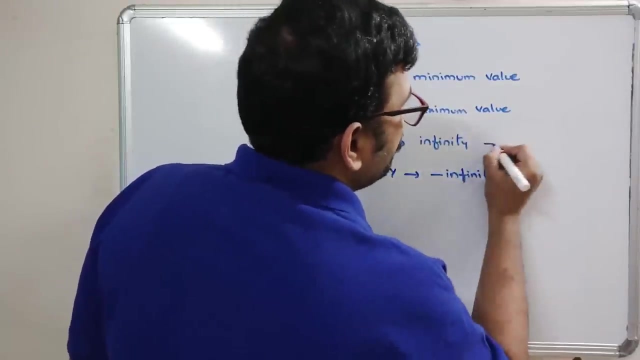 and a minimum value. and the third one, positive, underscore infinity. so this will return the infinity value. infinity that means divided by 0. okay, so this is a plus positive infinity and next one is a negative infinity. all our capital letters. this will give negative infinity. see, for example- this is an example- 10 divided by 0, it will give the positive infinity. 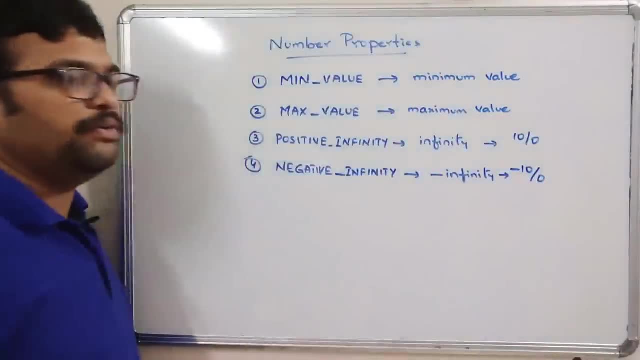 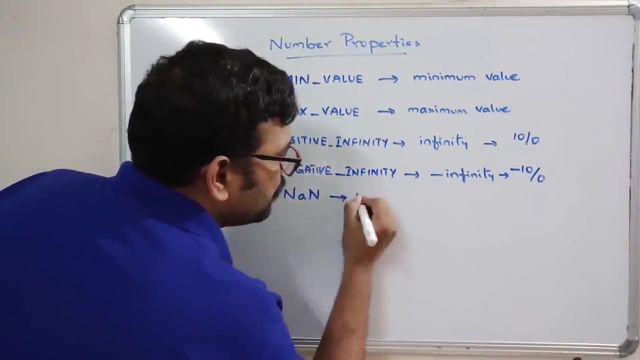 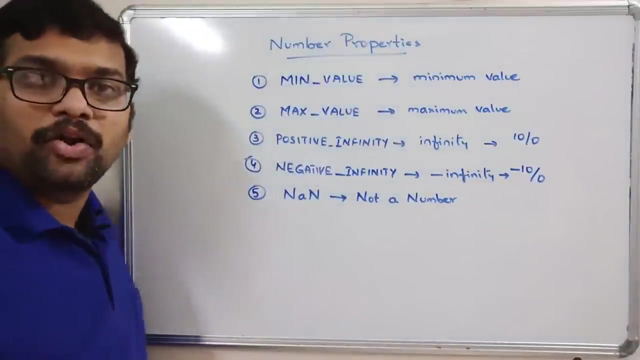 minus 10 divided by 0, it will give the negative infinity. so this is a negative infinity and the last one is nan. it is nothing but not a number, not a number. so i think in the previous session we have gone through this: none not a number. so if any expression is having a non-numeric string, 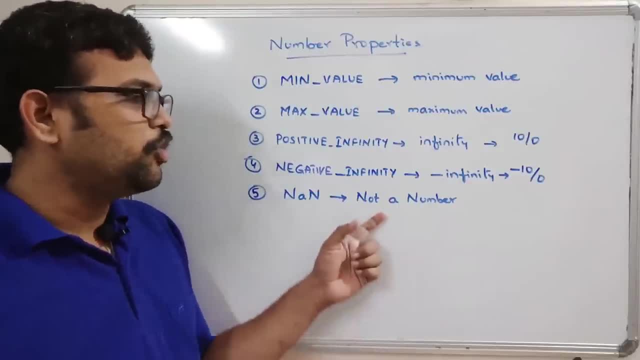 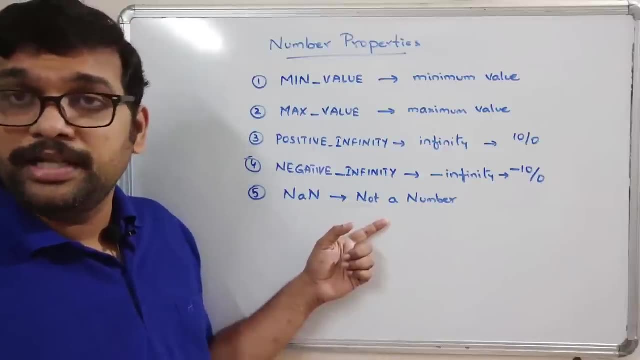 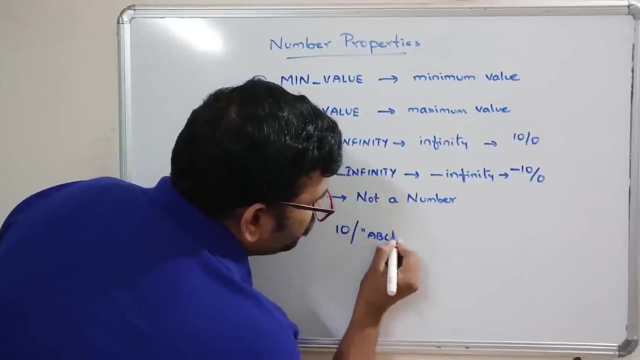 and it is applied to the automatic operations, then we'll get this, not a number, non-numeric string. that means the string should not contain any alphabets. sorry digits, right? for example, some 10 divided by a, b, c. so this is a non-numeric string, but applying some arithmetic operation, similarly 10 plus. 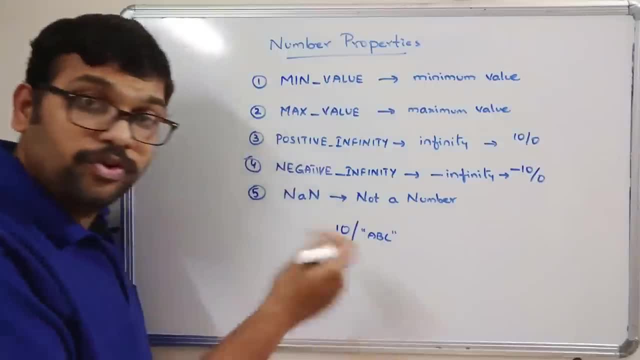 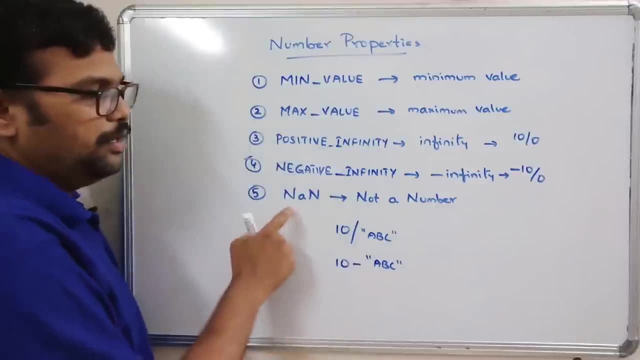 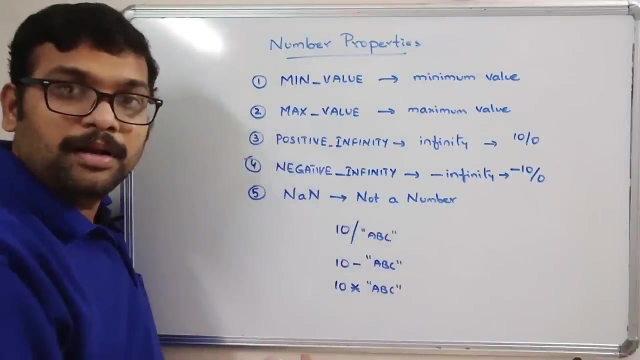 sorry, not not the plus. so if you use a plus, automatically it will use a concatenation 10 minus ABC. this will also give the, not a number. similarly, 10 into ABC, this will also return the non, not a number. but if you give 10 plus ABC, 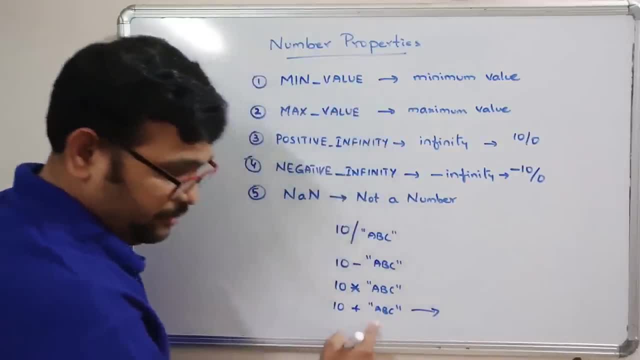 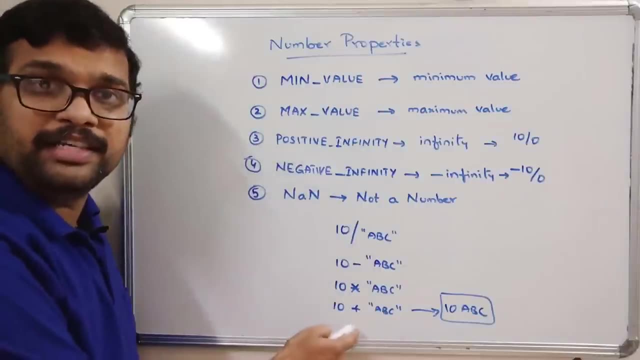 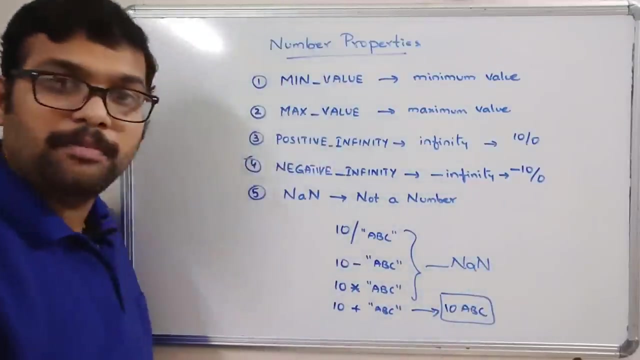 what is the result? in the previous session we have seen can concatenation will be done, so 10 ABC will be the result here, in this case, only in the addition, arithmetic addition. so all the remaining cases will get the result as not a number, not a number, right. so these are the number properties and these 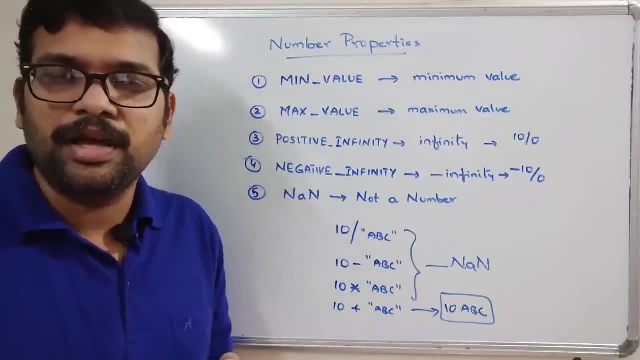 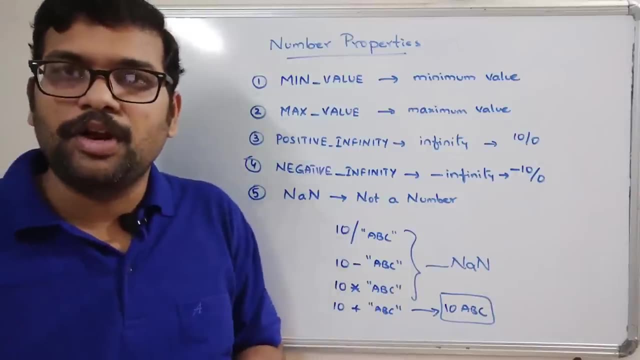 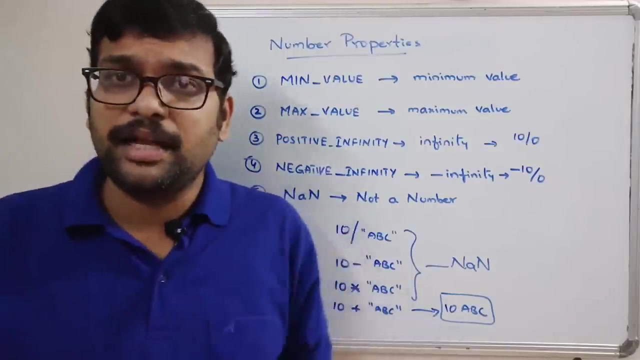 properties are only valid for numbers. okay, only valid for number object. it doesn't suitable for variables. it will not be applied for variables. okay, right. so hope you understood this one. so let us demonstrate. I will demonstrate all these things by executing a small HTML code. so let's move on to the system. 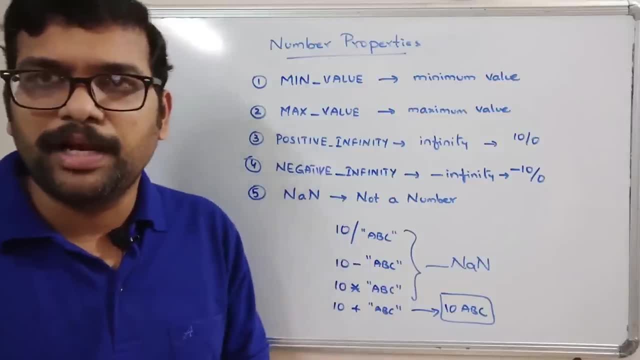 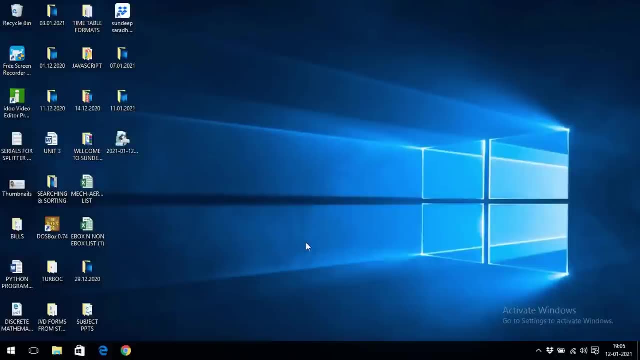 so that if you are still having any doubts, all the doubts will be clarified once you see the program right. so let's move on to the system. hello friends, so just now we have seen the number object, so how to create a number object and how it differs from the normal number and then different. 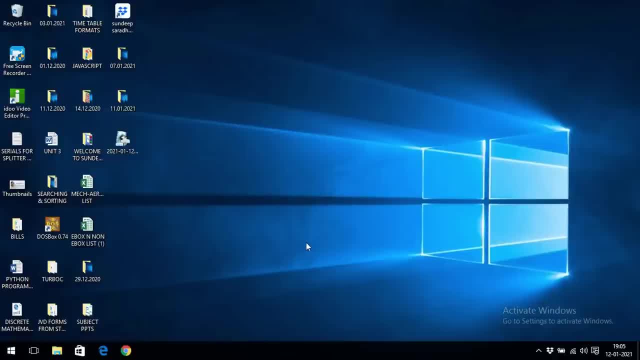 number object and how it differs from the normal number, and then different methods available in this number object. and also we have seen different conversion functions. that means number function, parsing function and a parsed load. and also we have seen the properties of number object. right now, let us demonstrate all these things by executing a small HTML code. so let us 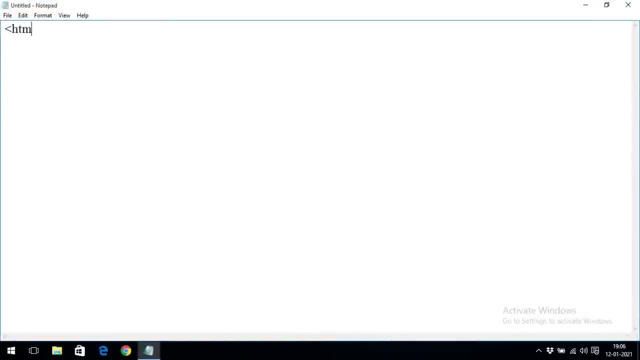 start writing the HTML code. so let us start with the HTML tags. so inside the HTML tag we have to write the body. so inside the body we can write the content. so body tag. so yeah, put the heading here. I just have a view, the heading as number objects right now, so here I will write. let us write the script here. 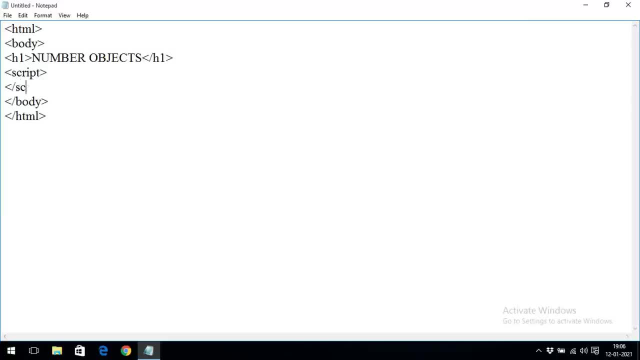 inside the body, so inside the script, we can write all the things. so first we will create a number, a normal number, and the number object. so in order to create a normal number, and we can go with a VAR, some X is equal to minus, x is equal to. 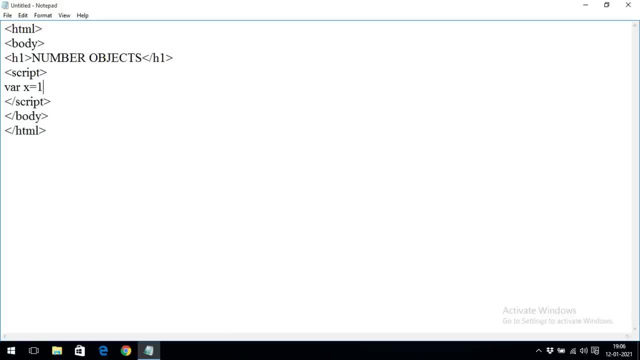 equal to some 10 or 15, right, let us take some 15 and let us create an object. so object is created with the help of a new keyword. so y is equal to some new keyword, followed by the number, and whatever the number we are giving here we have to pass. now you can observe, here i have given. 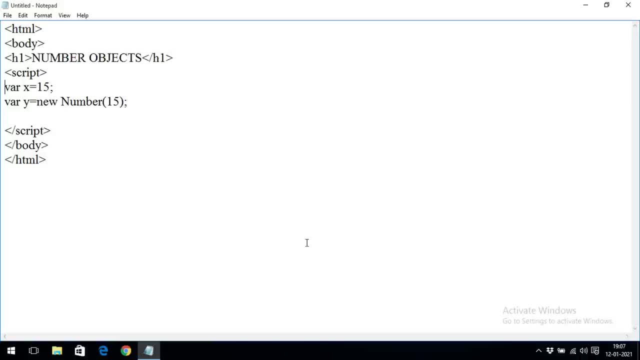 the two things here: x is a number and y is an object. so x is a variable and y is an object. so how to know whether x is a variable or object, that means how to know the type of that particular variable. so here we can have- we are having one keyword, that is a type of. so by using this type, 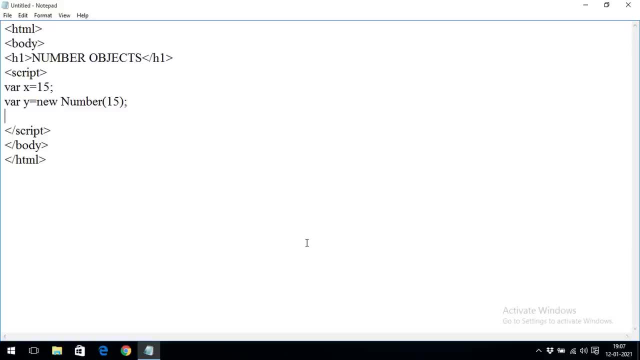 of statement. we can know whether the x or y are variables, the variables of particular data type. so let us check with that one. for that i will go with a. some z is equal to sorry, so document dot write l, and so i will write some this function to print the output. so here i will go with the type of x. right, so i will write. 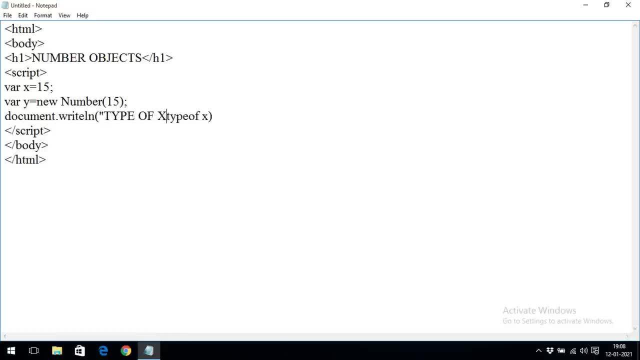 here. type of x, right now, sorry, yeah, and, and, and, and, and, and, and. then also write the same thing in order to know the type of y. okay, type of y, type of y. so we will get the data type of x and a data type of y here. let us save this one with the. 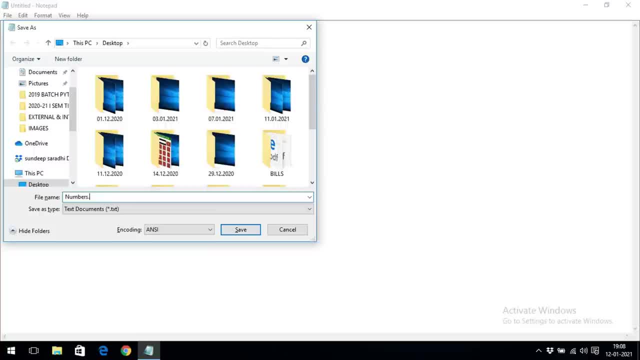 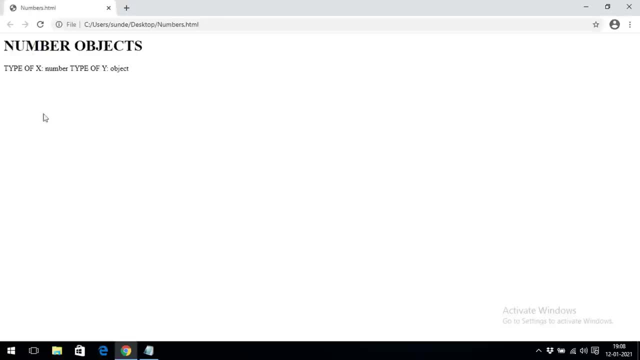 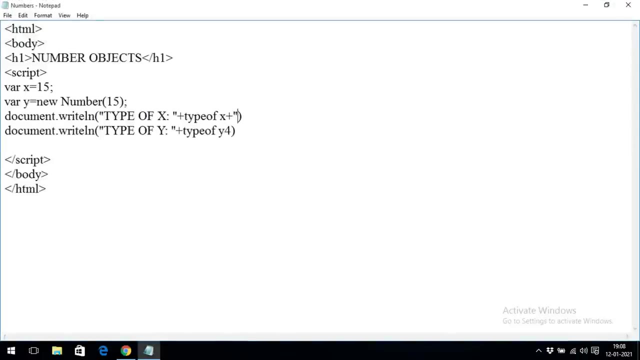 help of numbers dot html, right, so we will save this one, the numbers dot html, so you can find here, by executing this one we will get the data types. so you can observe here: type of x is number, type of y is object. So we will take br, that means a break row, and also here I will include this one because 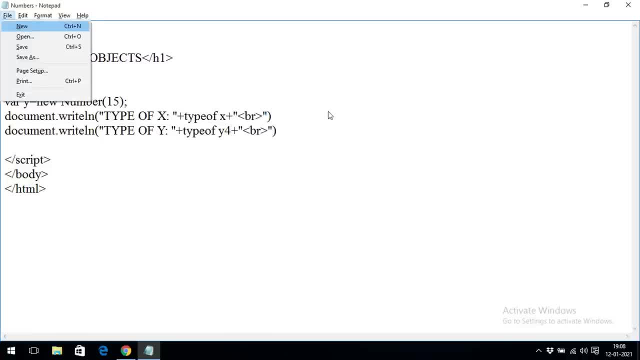 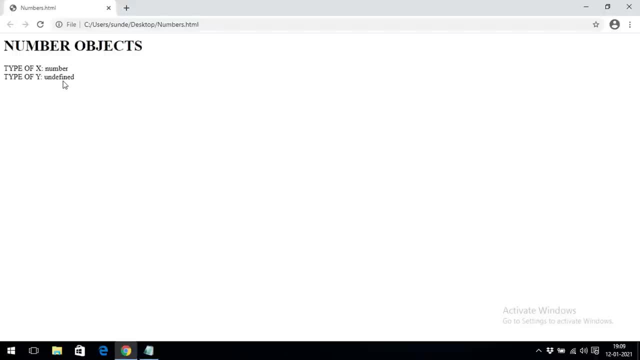 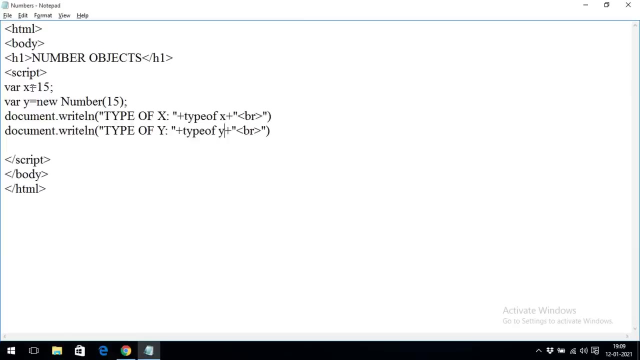 whatever the thing we are printing in the next lines, that will be printed in a new line. So just refresh it. So type of x is number and type of y is undefined. Here y4, now you can observe- type of y is object. So here x is having 15 and y is having 15.. 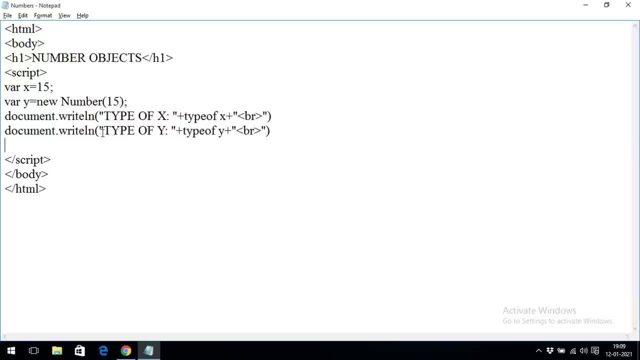 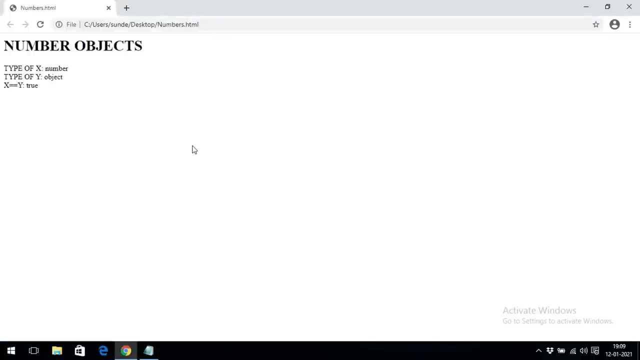 And if you are comparing the things, see, if you are comparing the things, write the same thing. See, x is equal to is equal to y. That means so, instead of writing here, just write x equal to equal to y. Now, what is the result? Observe here, So we will get true. What is the result of here? 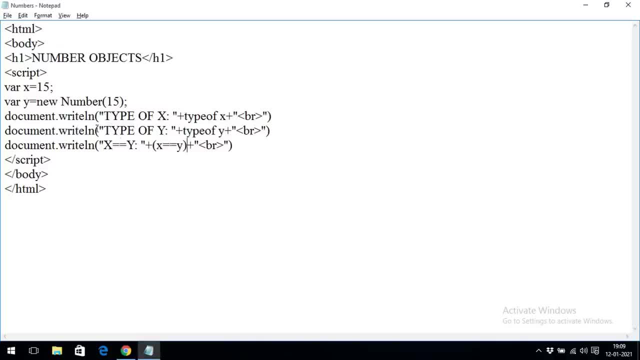 It is a true. x is equal to. y is true, right. So because here double is equal to, is an equal is nothing but a relational operator. Whenever you are using this, double is equal to. it checks the value. So value of x is. 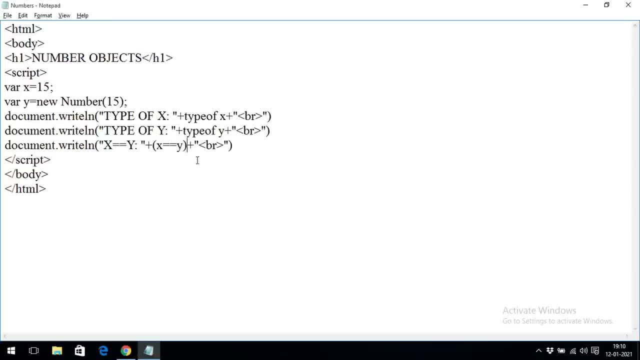 15 and y is 15.. So it becomes true. And if you go with the triple, equal to triple is equal to. that implies it compares the types, not the values. okay, So here type of x is in. 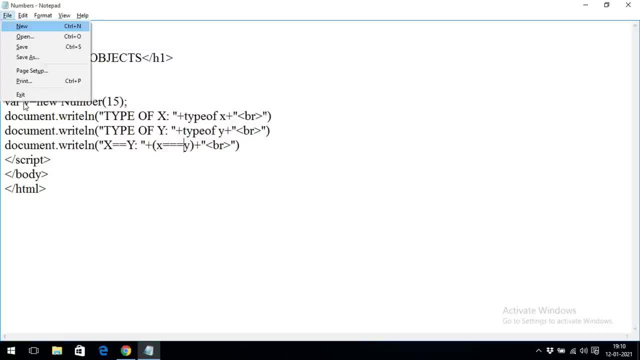 Number and type of y is object: Now we will get the result as sorry see, I will copy the same thing and I will go with the next. So here we will go with. the triple is equal to Now the result. 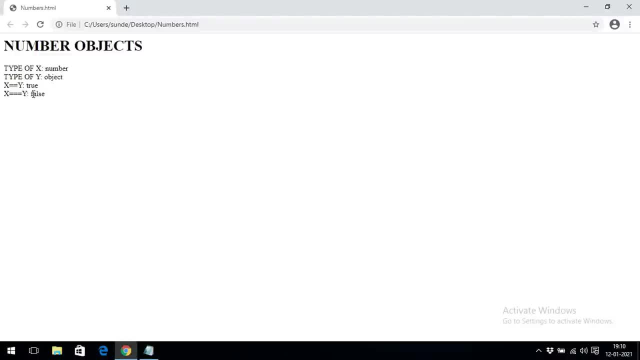 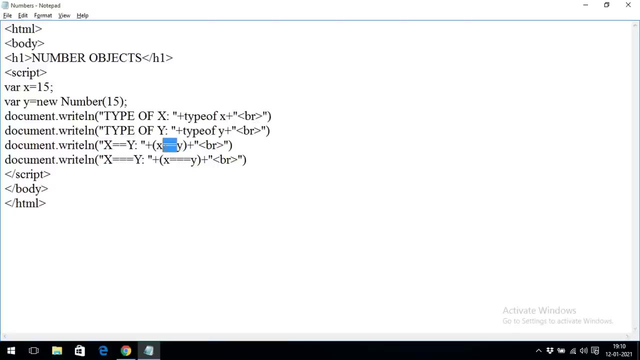 will be false. The result is a false here: okay, The result is a false here. So here the result is a false. Why it is false? Because we are using some triple is equal to, Which means it compares the data types. Okay, If it is double equal to, it is a. 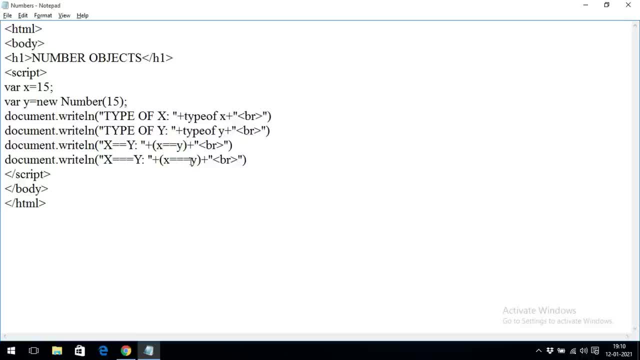 values. That values will be compared. If it is triple is equal to, the types will be compared. And one more thing: we cannot compare the objects. So, for example, you take the same thing, You take one more variable here, some z, some z. z is equal to 15, and also you can. 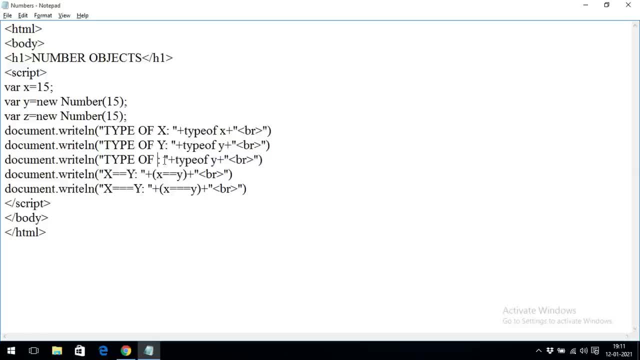 print the type of z. okay, The type of z is nothing but an object, right? So type of z is an object because we are using some new and if you compare the same thing, if you compare the same thing with z, y and z, So you can observe here both are objects. 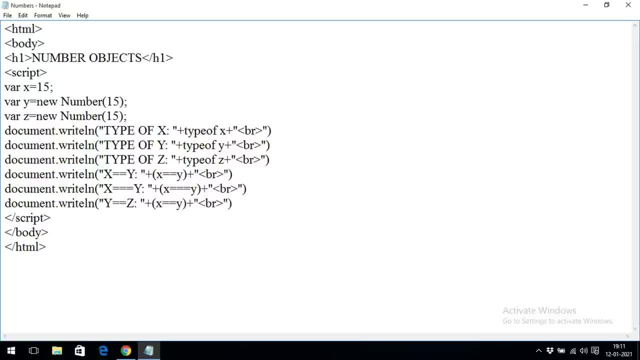 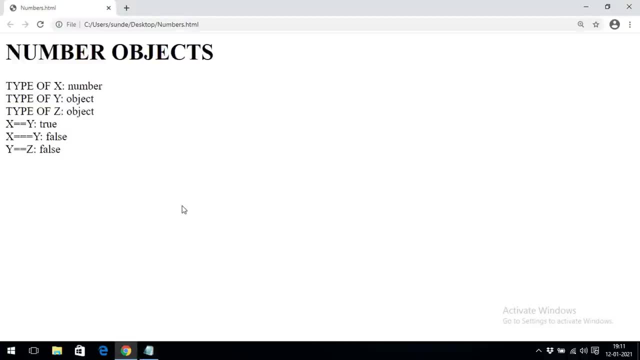 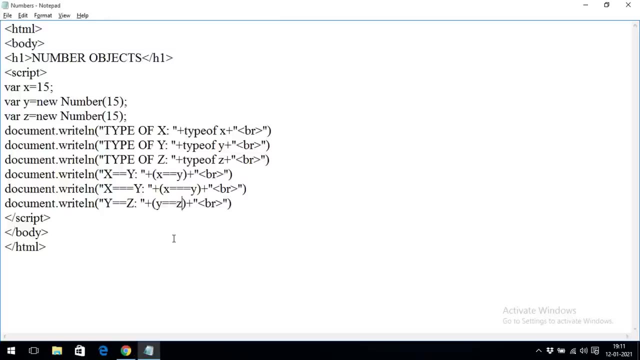 So here I am comparing y and z, So even though both are objects, we will get the result as false Because two objects can't be compared. So this point should be remembered. two objects can't be compared, So this is a number object. So like this we can create: 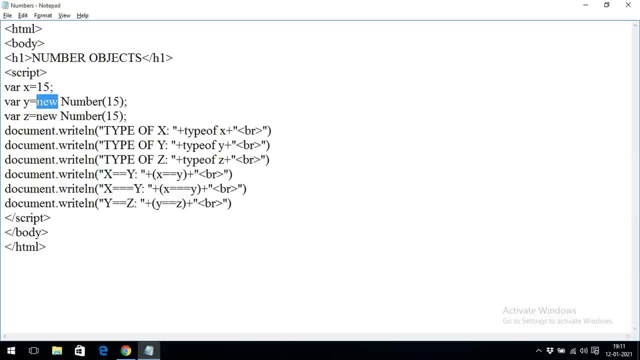 an object. that means by using the new keyword. Now there are different methods available in number object that is first. one is a toString. So already we have seen in the previous session that is a toString in order to convert from one base value to another base value, So that base value 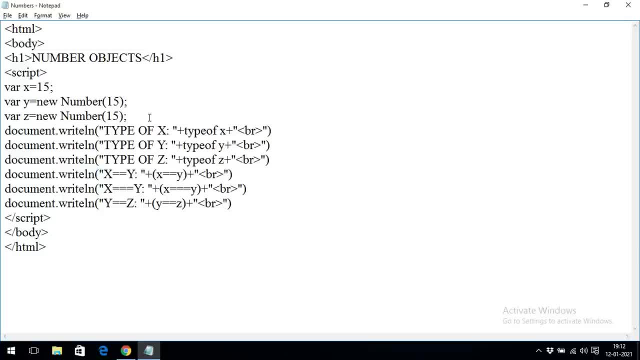 will be given as an argument to the toString function. So if you are not giving any argument there, the value will be converted into a string data type. So here you can observe, x is nothing but a 15, and now, where s is equal to write down xtoString. So automatically s is a type of 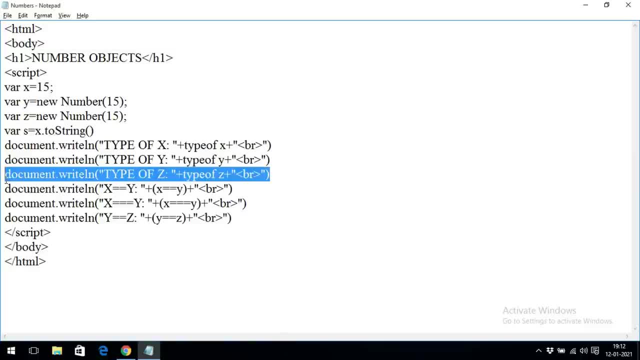 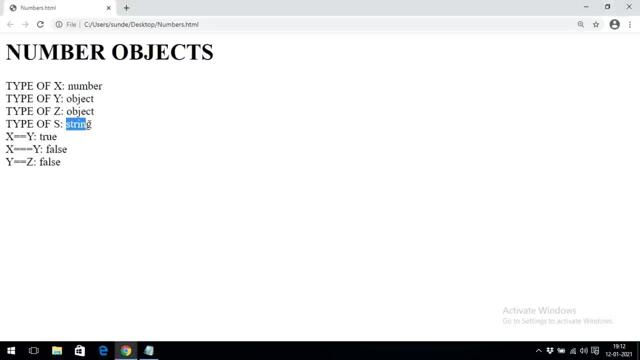 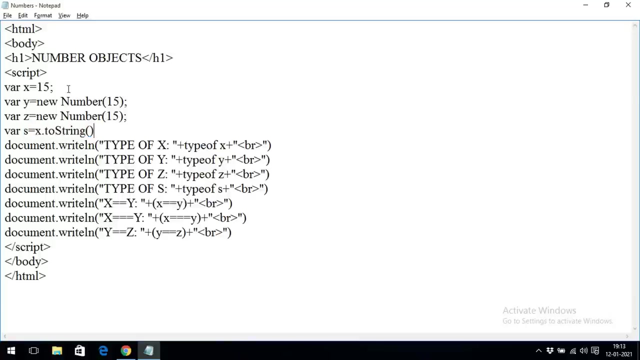 string, So 15- will be converted into a string type. So you can observe here. So here, type of s, You can observe here. type of s is a string, So s xtoString means whatever the number we are giving, either integer or a float numerical value will be converted into a. 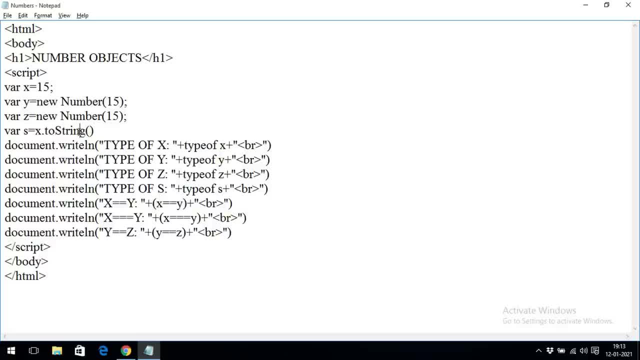 numeric string. It is a numeric string now. Then there is one more function called toExponential, So we can represent any value with the exponential form. See, you take the same thing, So were some. e is equal to exponential, So 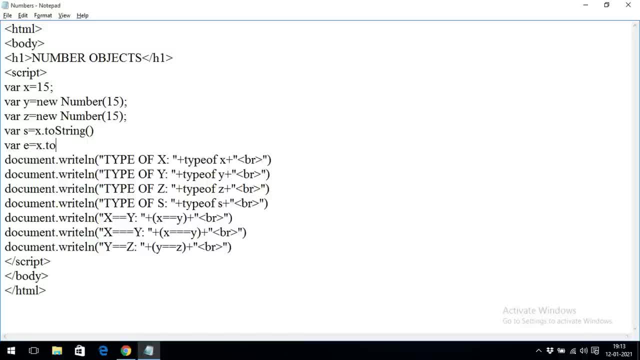 will consider 15 itself xtoExponential And give the value to which it must be exponented, So 2.. I will give 2, and I will print e value. here will print E value. so I will remove all these things. okay, I will remove these. 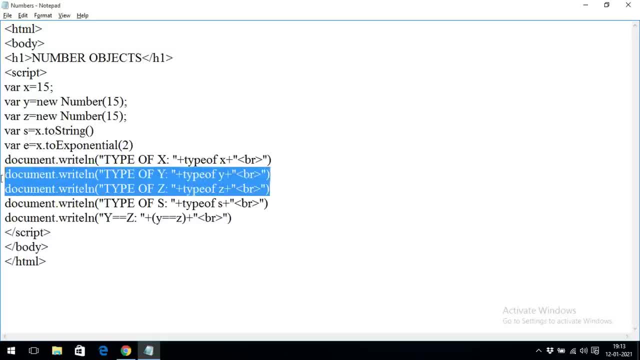 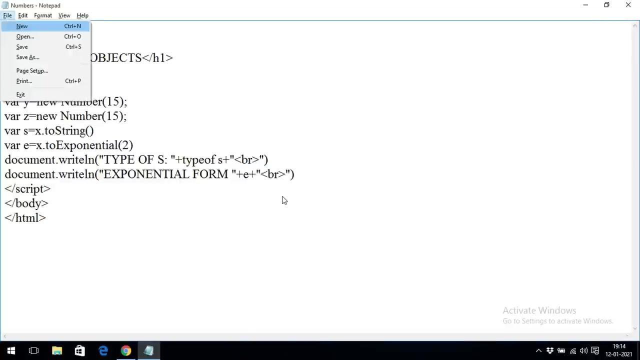 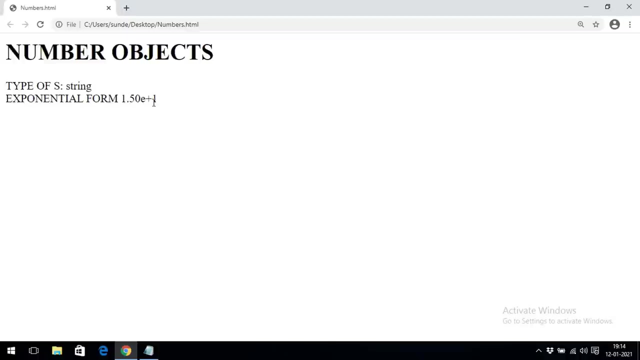 things and also, yeah, I will remove these things so that there will be no confusion for you. so instead of giving here exponential form, it's nothing but E. so if you print E will get the value in exponential form. you can observe here the exponential form: 1.50 E plus 1, right. so 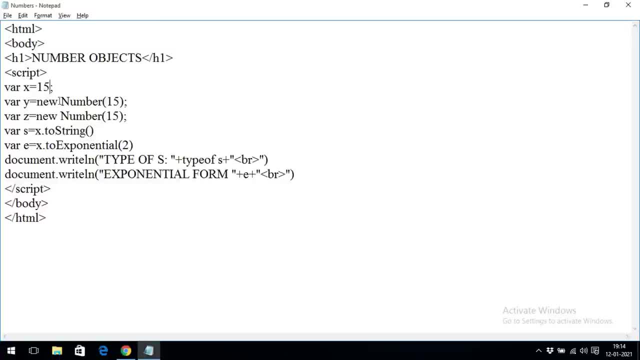 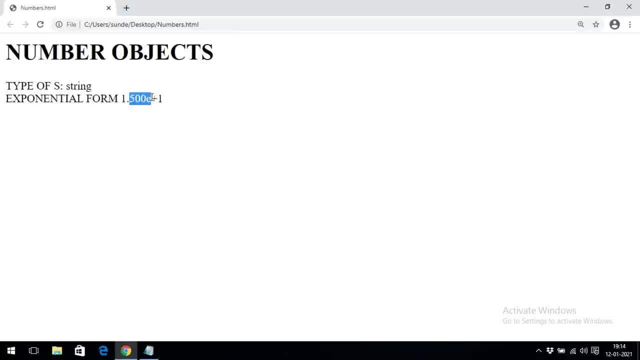 representing the value, the representing the value in terms of exponential. if you go with the 3, you can observe here: so 3. this is a 3. you can observe here, so 3. this is a 3. you can observe here. so 3. this is a 3. 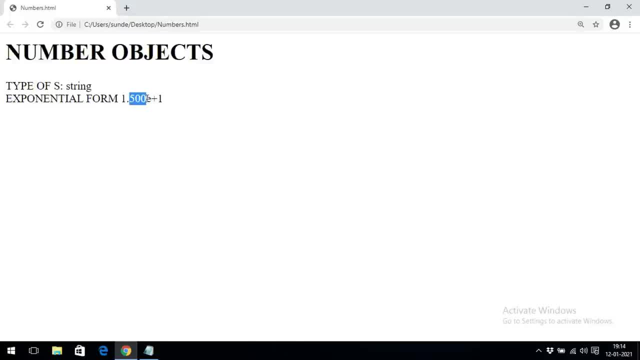 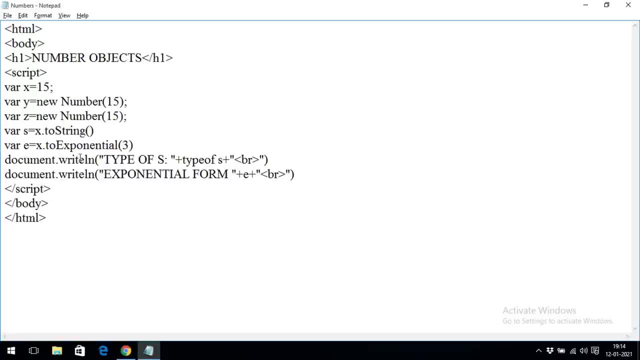 precisions: right. 3 decimals, 3 decimals with exponential value- right. so this is how we can convert any number to exponential form. okay, now there is a one more function called fixed to fixed to fixed function will returns a string and gives the number of decimals. it will restrict to the number of decimals. so if 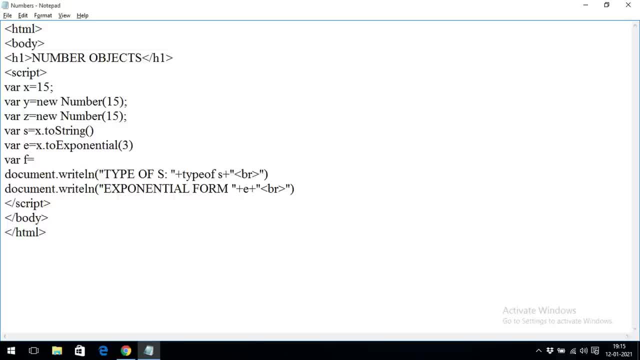 you go with the, where F is equal to the X dot to fixed off. give the number of decimals. let us take some three decimals here and let us print here. that is good here. so to fix it up, function right, so I will print here. yep, you can observe here, so let me intent it to print here: F will get the number. 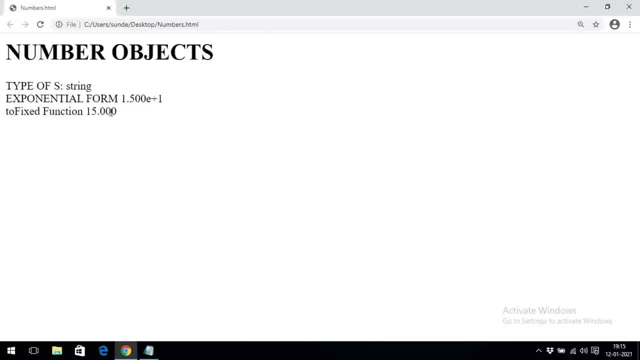 So we will print it to F. so F, you can observe here, F zero or true. first option should be F, right, so I will print here: yes, you can observe here. if you have norou, if you have already got an answer here, two fixed is 15.000.. So that means we are restricting to three decimals, So automatically. 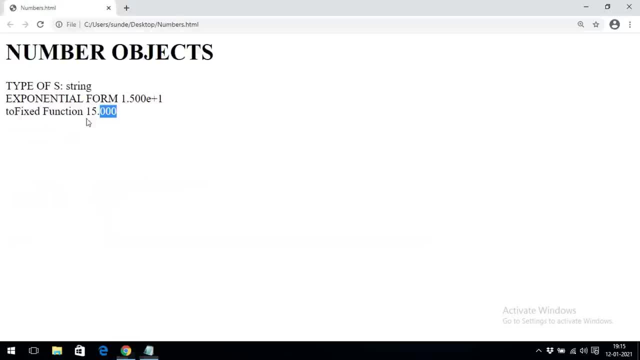 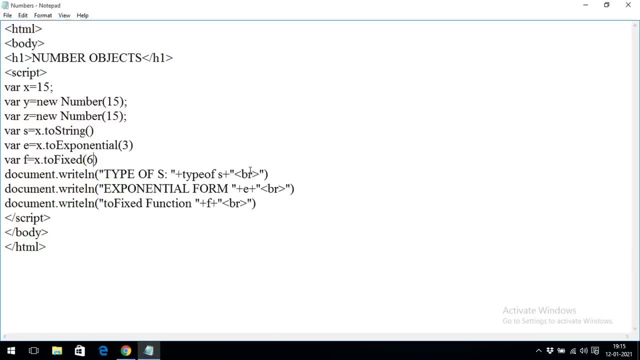 three decimals will be added right. So initially x value is 15 and now it is a 15.000 because we are restricting to the three decimals. If you go with the six decimals, automatically it will be printed with the six decimals. So if somewhere n is equal to 5.345678.. Now, if you restrict this, 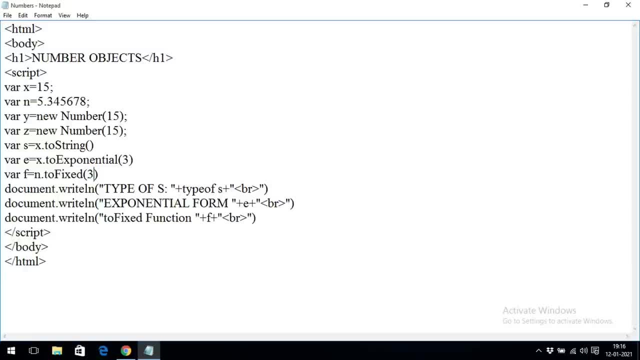 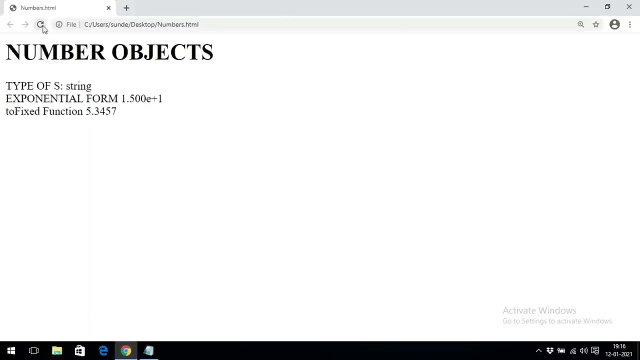 one n dot to fix it with three. So you can observe, here it is: the result is 5.346.. It will be rounding up. Okay, it will be rounding up to the three decimals. If you go with the four decimals, 5.3457.. We will get this one 5, 7.. You will get 3, 4, 5, 7, right. So like this, in order to restrict. 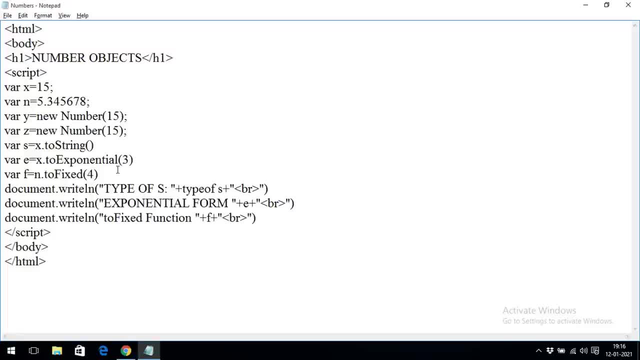 with the decimal values. we will go with this two fixed function And there is a one more function called two precision. So total number of length, the length of the value can be restricted with the help of this precisions. Okay, p is equal to 5.345678.. Now, if you go with the four decimals, 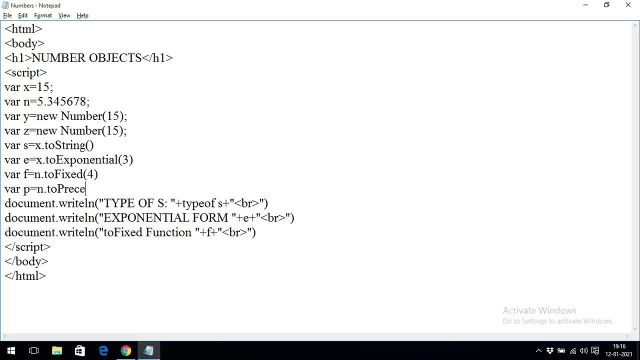 n dot to precision of. So if you consider this length, that means number of digits: 1, 2, 3, 4, 5, 6, 7 digits are there. So here you can restrict with the three digits, You can restrict with the three. 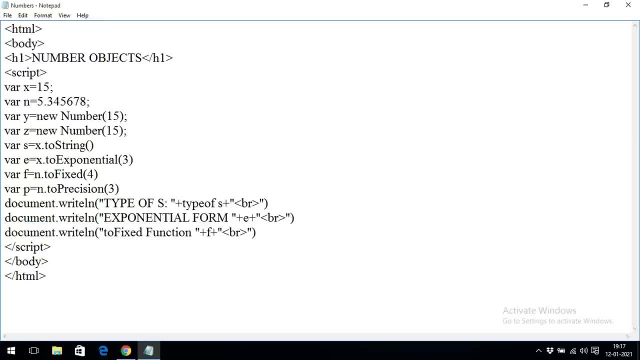 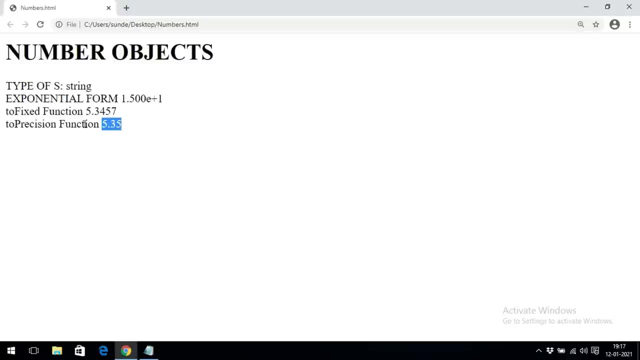 digits. Now you can print the p value here, So see precision function, and here, instead of f we have to give p, And if you execute this one you will get the value. the length of the number will be 3.. And you can one one important thing: the result of all these functions are string. So if you go with the 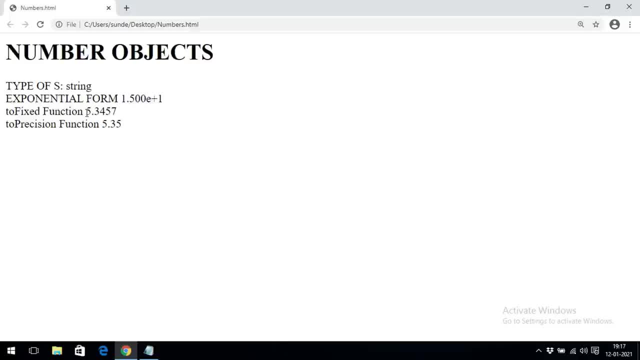 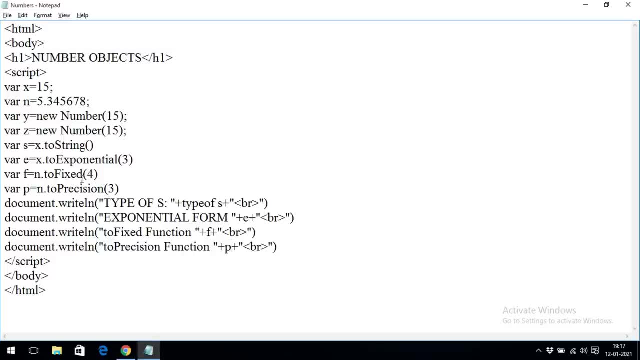 exponential form. this is not a number, this is a string. And two fixed function. this is not a number, this is also a string. And two precision function. this is also a string, Right see, And you can observe here. So I will let us check whether the type of this one. So, type of p. Okay, type of p, And you can observe. 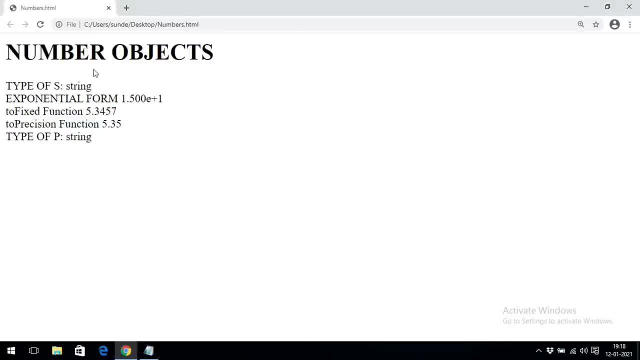 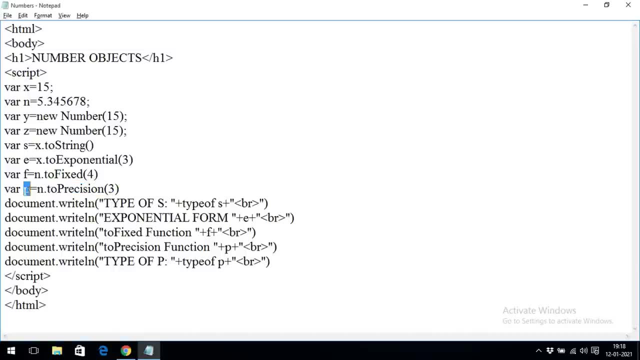 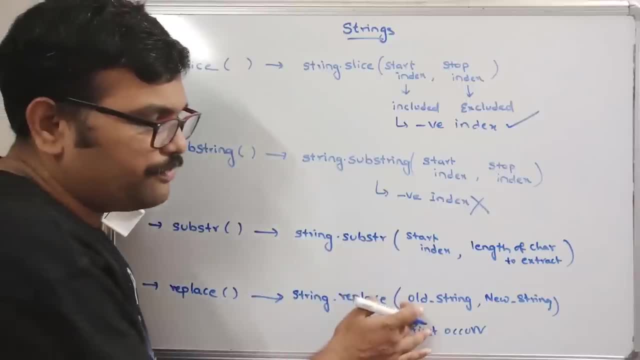 means two fixed function. So then of course you can observe that p is a string, And if it is f, that means two fixed function. So then of course you can observe that p is a string And if it is f, that first character. So whenever it finds this old string, automatically that old string. 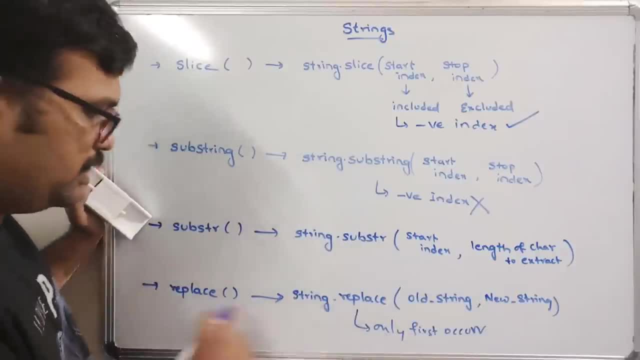 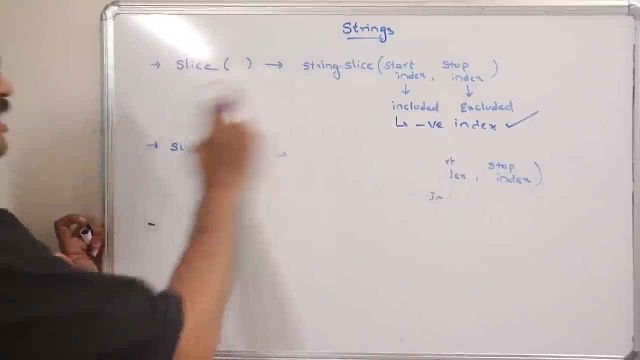 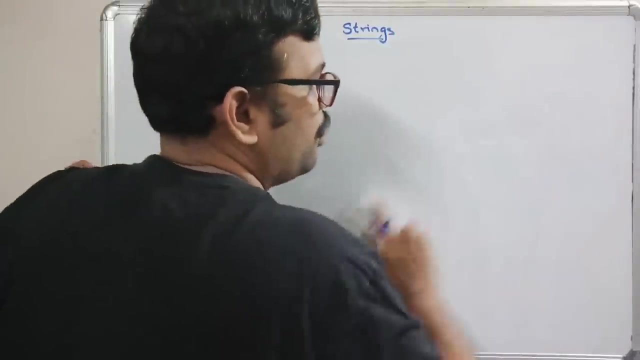 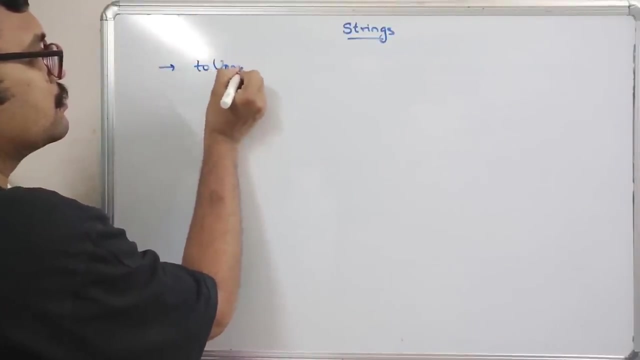 will be replaced with a new string. So this is a replace function And there are a few more functions available. So, in order to convert from lowercase to uppercase and uppercase to lowercase, so we are having a functions called to uppercase, to lowercase, To uppercase. 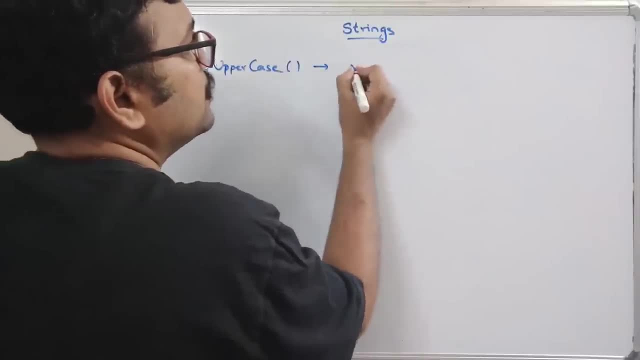 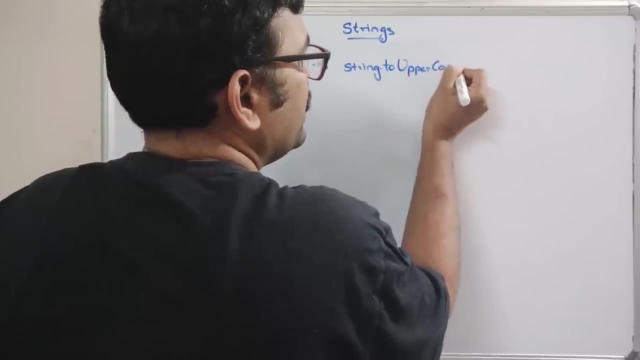 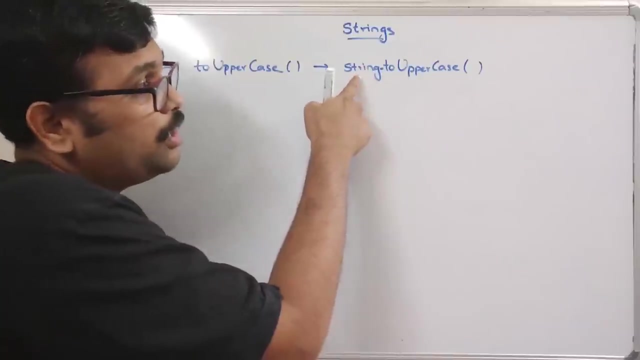 function. So the syntax is: string dot to uppercase- Okay, automatically. whatever the string available in this string, the all string dot to uppercase- Okay automatically. whatever the string available in this string, the all the lowercase characters will be converted to uppercase. Similarly, we are having the one more. 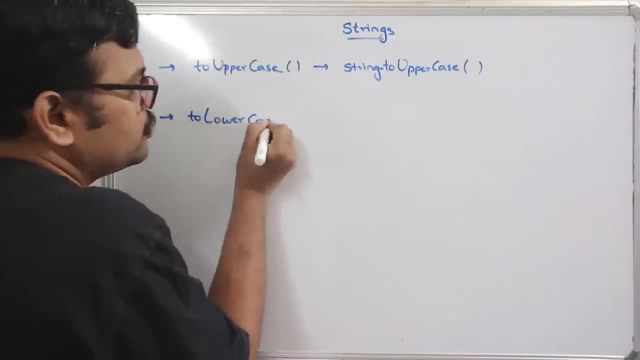 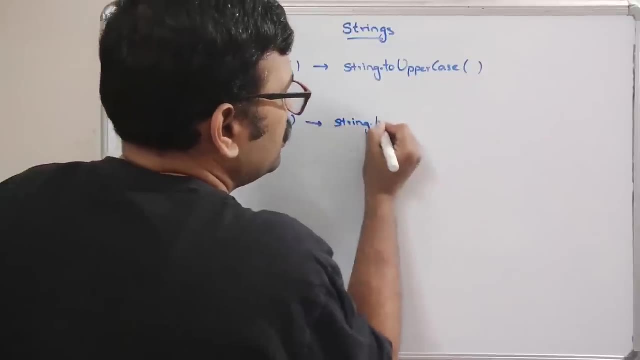 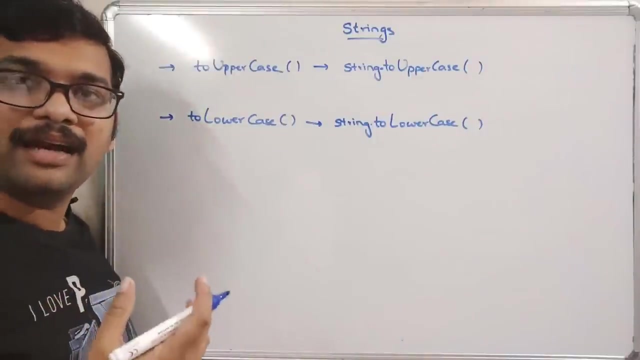 function called to lowercase. So don't worry, I will execute each and every function and I will show you Okay. So I'm just giving the syntax here: string dot to lowercase, So automatically, whatever the characters- uppercase characters- available in this string, that will be converted. 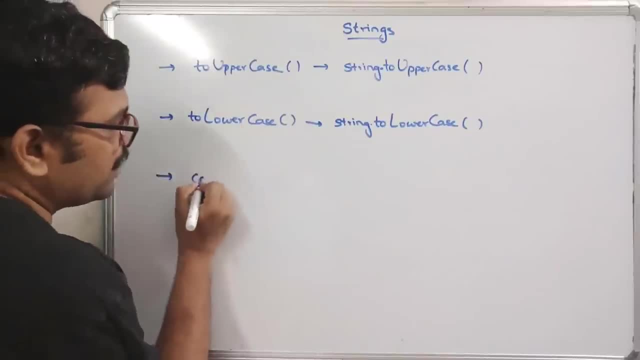 into lowercase And there is a one more function called to lowercase. So automatically, whatever the characters, uppercase characters- available in this string, that will be converted into lowercase. And there is a one more function called to lowercase And there is a one more function called con cat Este. con cat means concatenation, so it 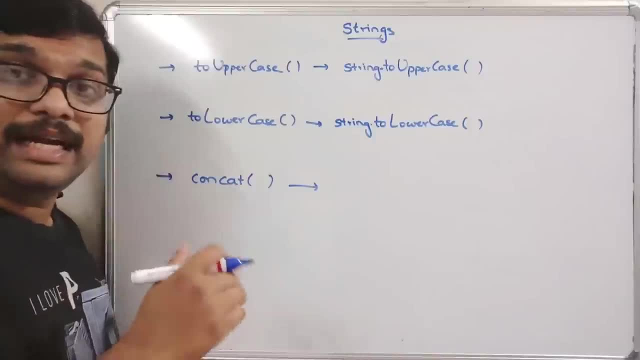 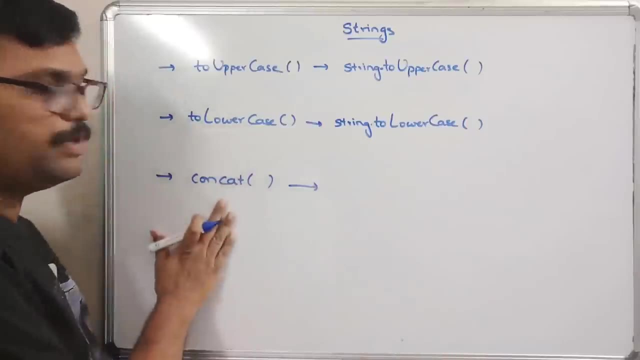 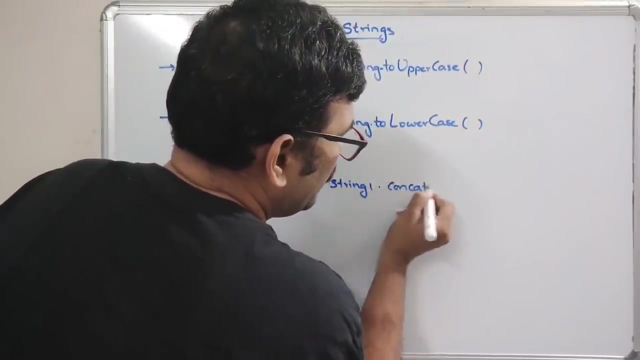 tees concept understand con cat. con cat and Latin means concatenation, So it replaces the plus operate. So generally, plus will be used as a concatenation between two strings that can be replaced by using this concatenation, So string one dot con cat. 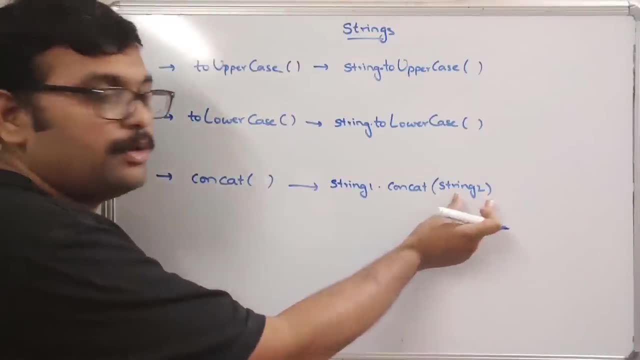 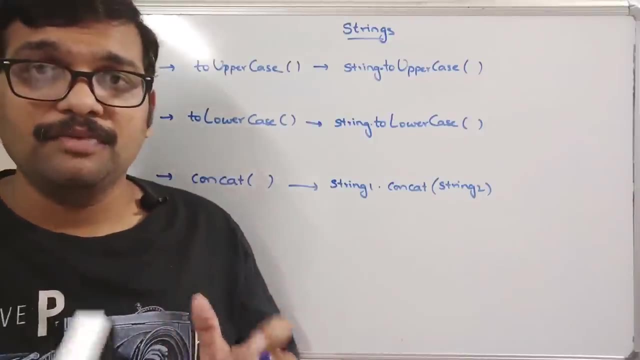 from two. automatically, whatever the string available in string two, that will be concatenated to string one. So one of the three other things that we used- chili, you need toне thing i need to say here. so whatever the thing we are creating, everything will be creates a new. 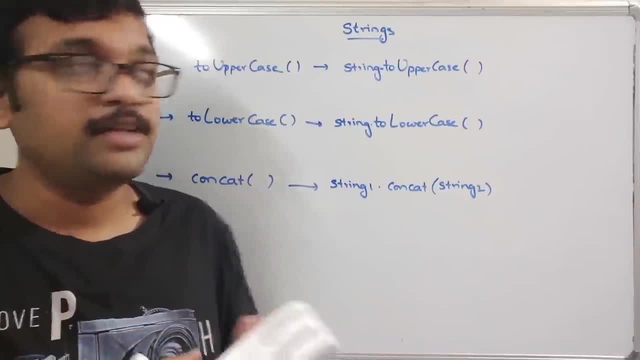 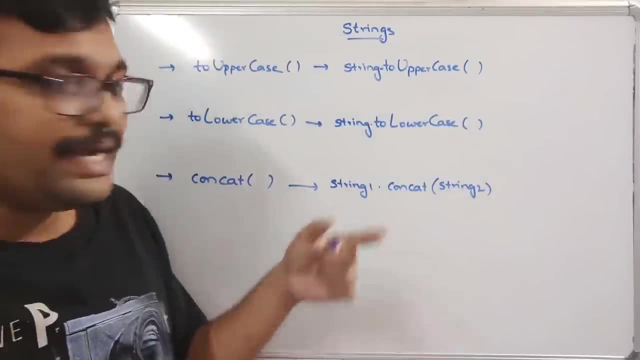 string: okay, the original string will not be affected. so if you convert some lowercase to uppercase, the original string will not be converted. right, so a new string will be created. similarly, concatenation: also: a new string will be created. the old string will not be updated. right, so a. 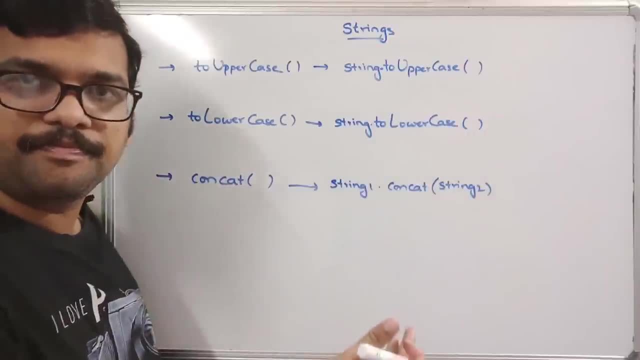 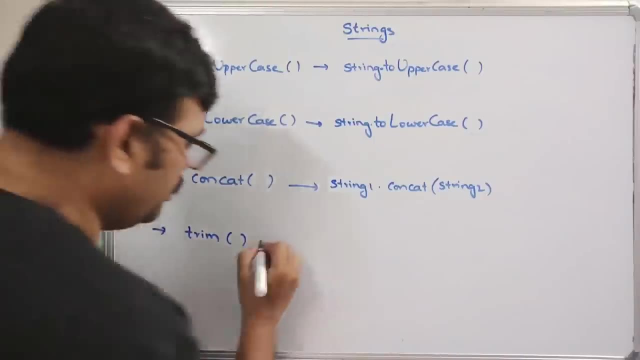 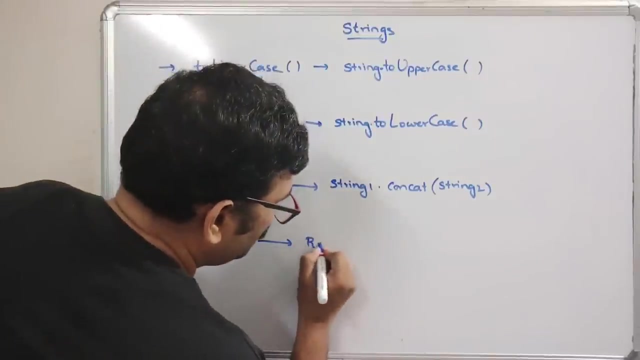 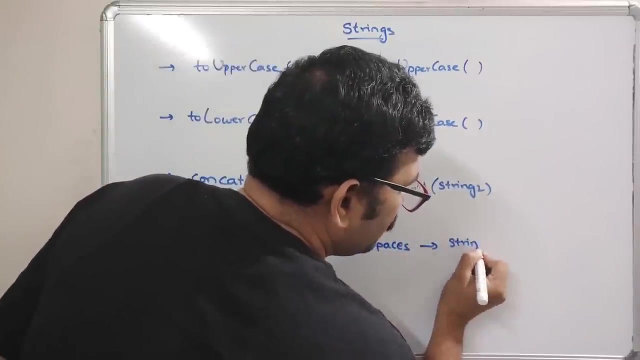 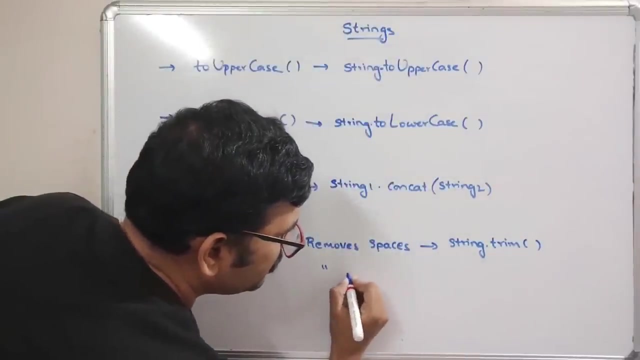 new string will be created by applying these functions right. next one: trim function. trim function. it removes all the leading and tiling spaces, so it removes the spaces and the syntax is string dot. for example, we are having some spaces, three spaces, and we are writing some javascript. 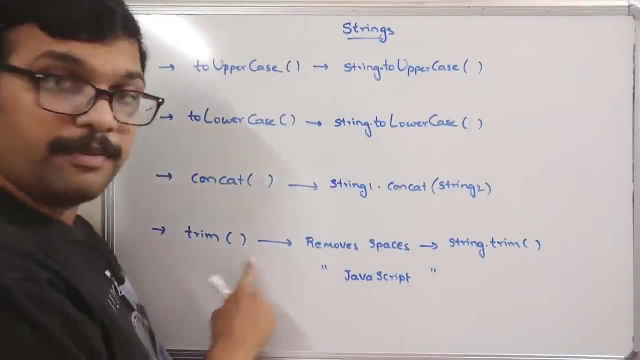 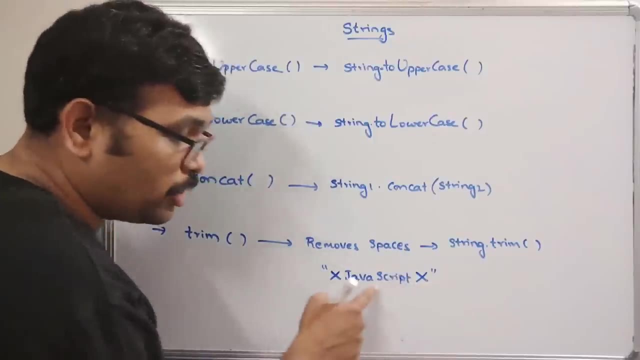 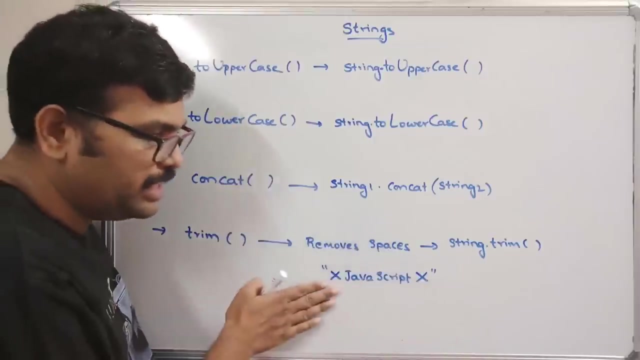 and three spaces here, and if you apply this trim function, it will remove all these spaces, all these spaces- leading spaces and tiling spaces- but not the spaces in between the string. okay, it doesn't remove the spaces in between the string, it only removes the leading spaces and tiling spaces. so the result will be directly so, without 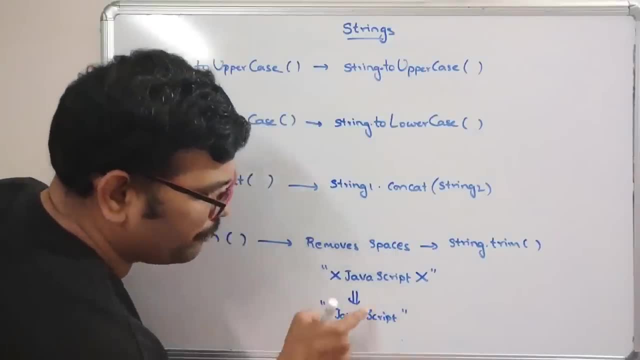 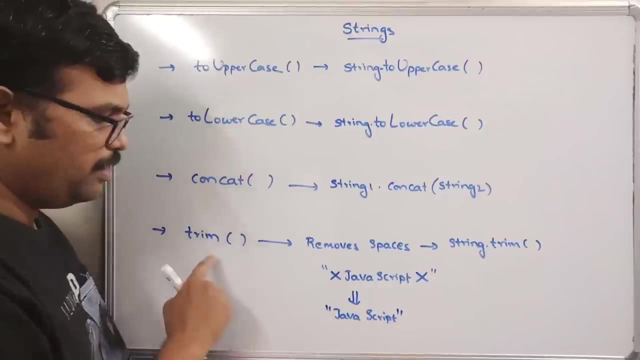 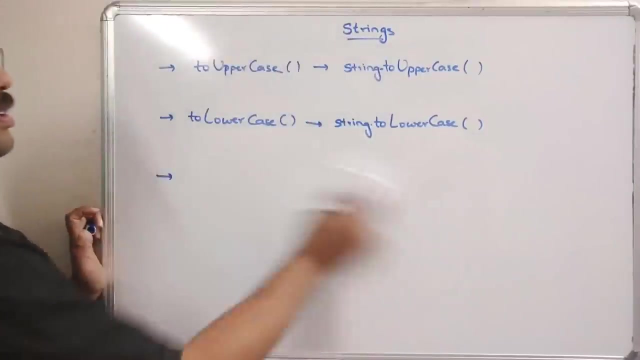 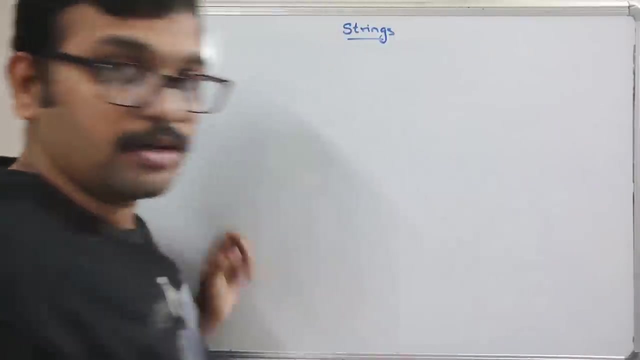 the leading spaces. we will get the result: so this space is common. okay, this space is common. it will remove the leading spaces and tiling spaces. so this will be the result for trim function: it will remove the spaces then. so how to extract the characters from the position? okay, extracting the characters. 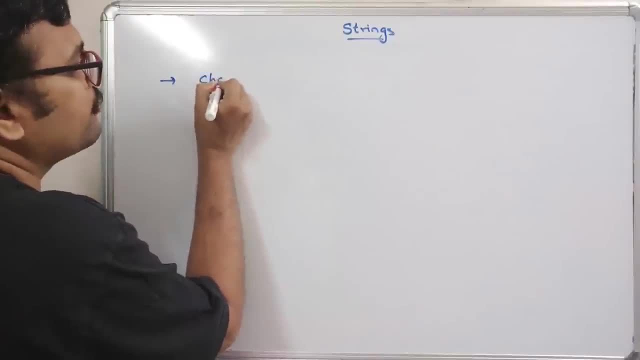 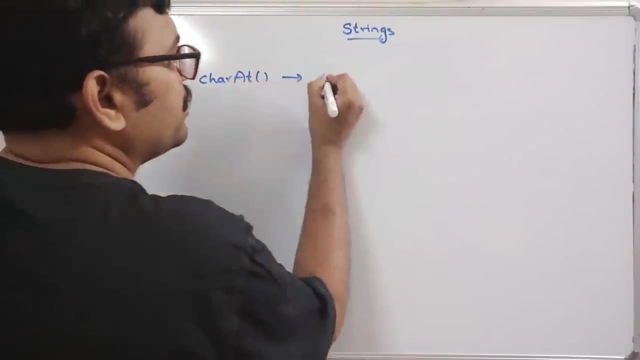 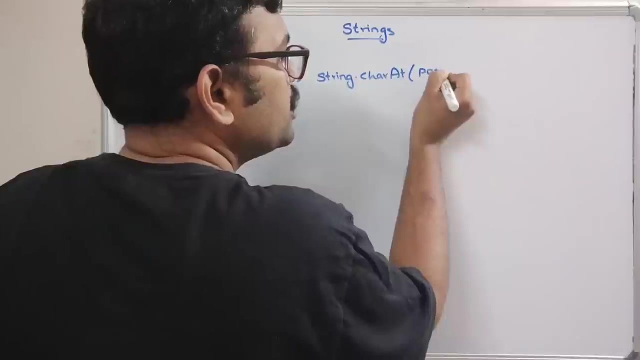 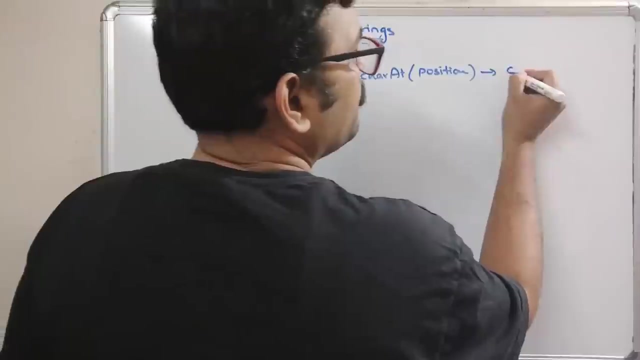 from the position. so for that we are having the function called char at function. so char at means character at. so string dot char at and here we need to give the position or index, whatever it may be. so whatever the character available in that position, that will be returned. okay, it will return the character at position. 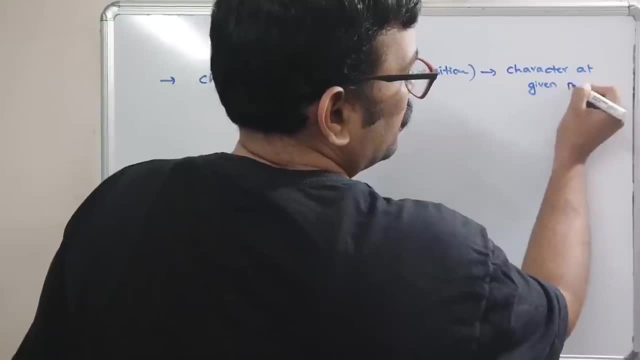 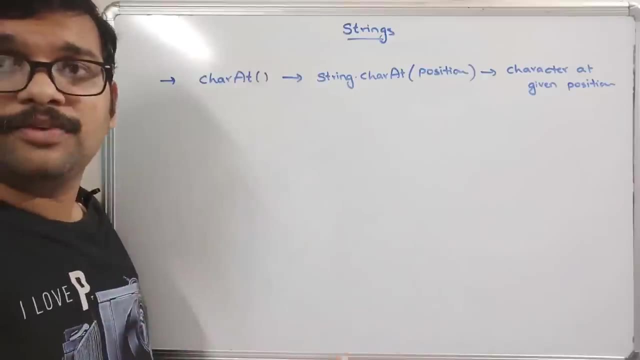 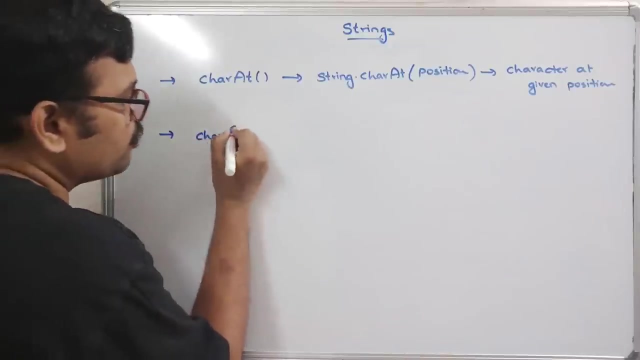 character at given position, right, so we need to give the position. so if the position is beyond the length of the string, nothing will be printed. so i will show everything. okay, and there is one more function called char code at. so here c and a will be characters. 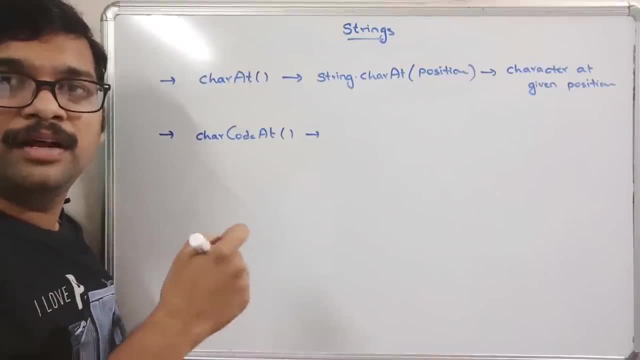 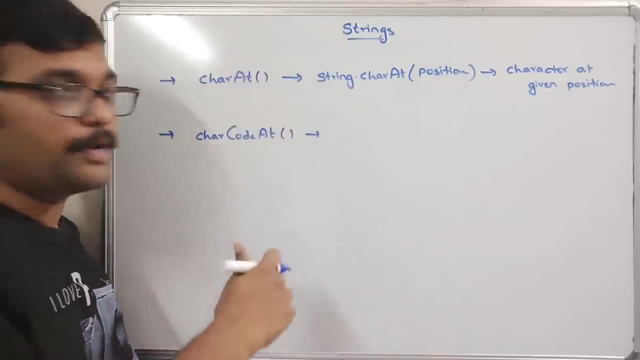 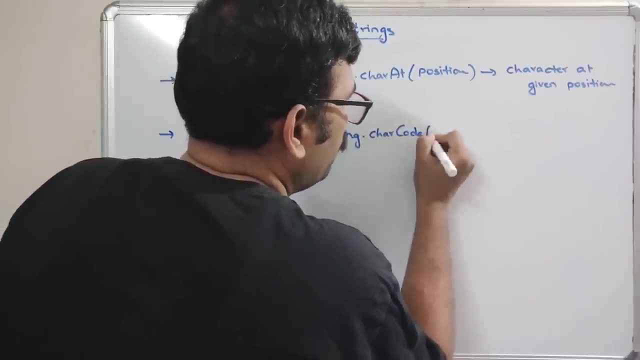 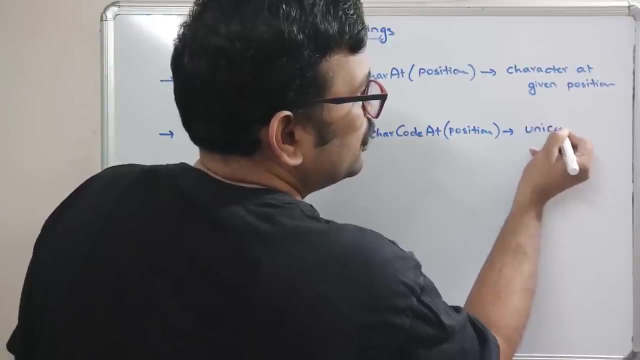 char code. so it will return the unicode of the given character. okay, first it will. it will get the character for that position and it will return the unicode for that particular character. so string dot care code x position, it will return a unique code. so generally we are having a different. 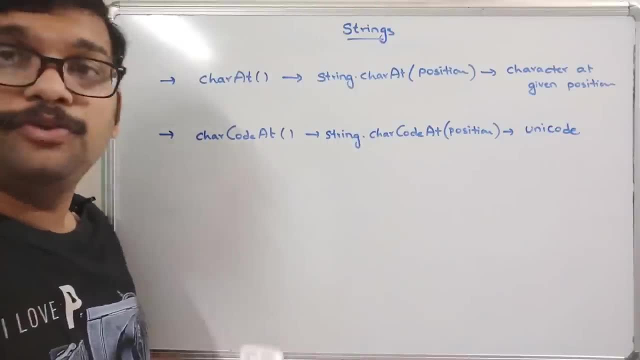 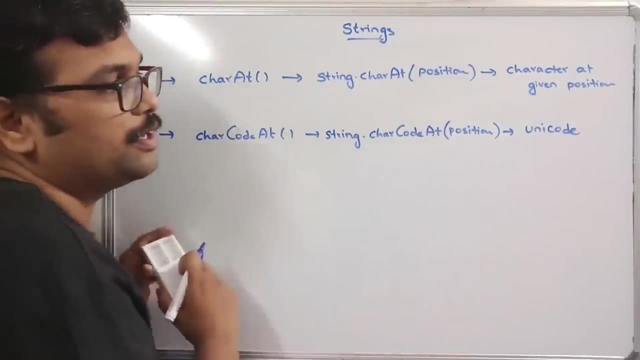 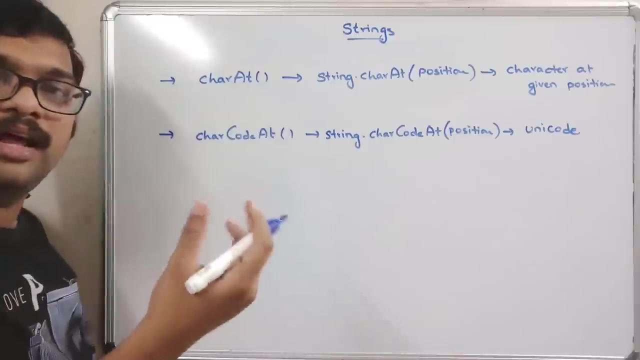 code formats, that is ASCII. we know that ASCII, so this is a unique code. so it will return the unique code of the character which is available in this position. okay, unique code for the character available in this position. right, so these two. by using these two, we can extract the character. that means we can get the character or the code at the given position. 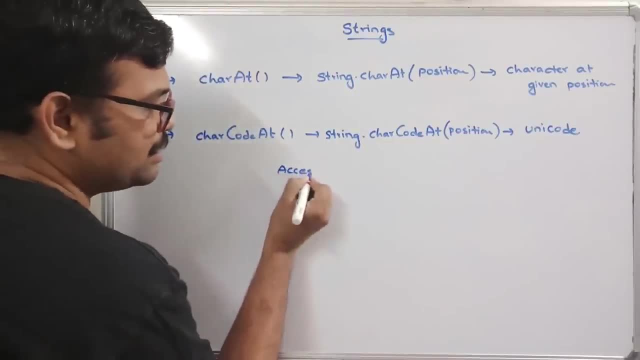 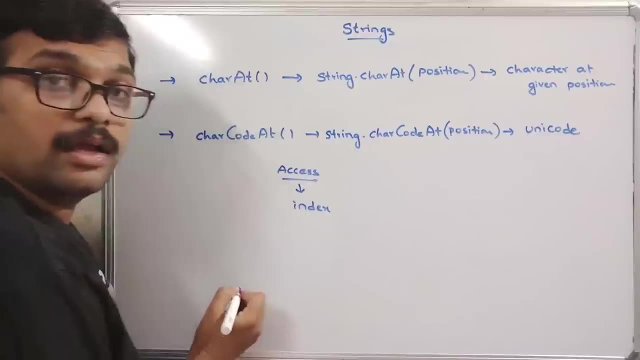 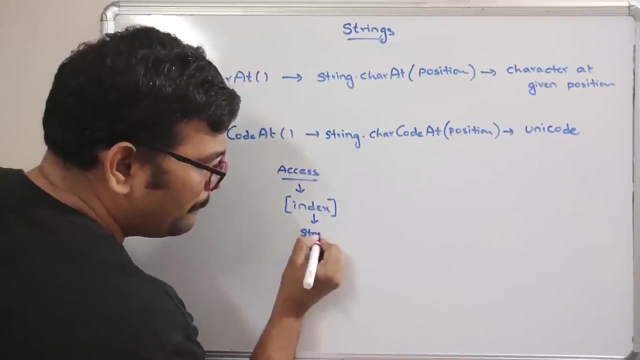 right. the next one is accessing. so how can we access the string characters? so this accessing can be done with the help of index value. okay, in between the subscript. in between the subscript. so index value always starts with, starts from 0, right. for example, s is equal to. 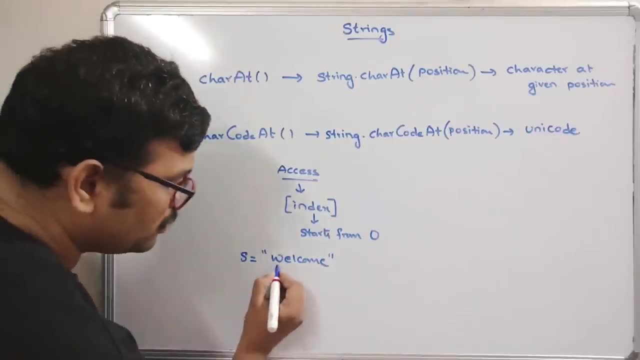 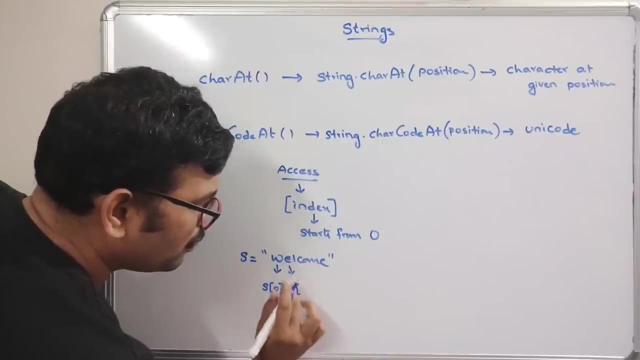 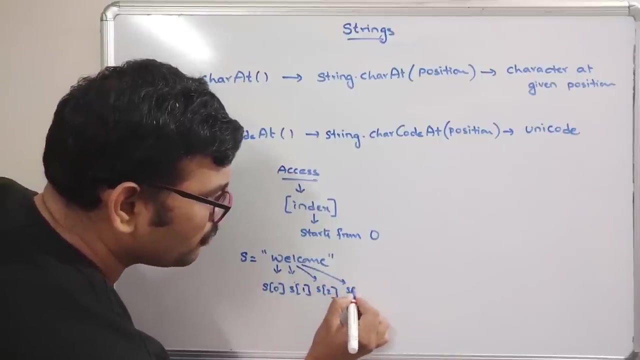 some welcome. so index value is 0, so this can be represented as s of 0, and this can be represented as s of 1, and this can be represented as s of 2, and this can be represented as s of 3, and so on. right? so each and every character will be having some index value and we need 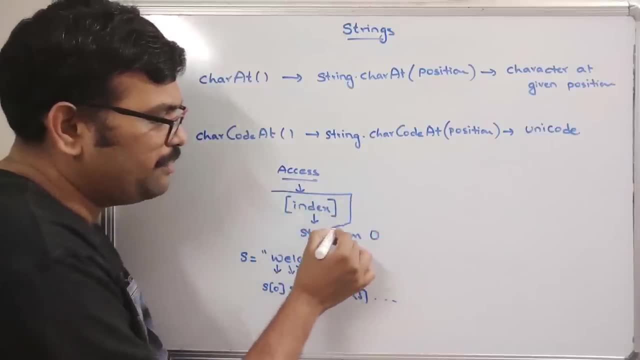 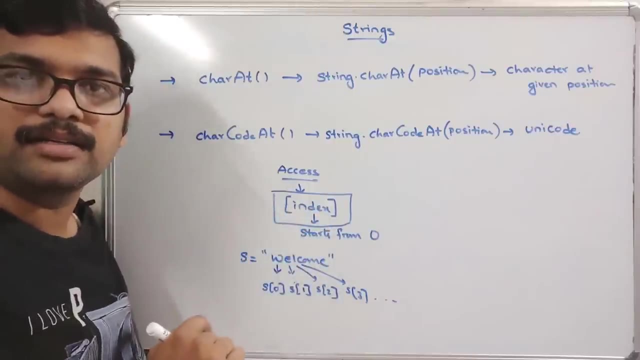 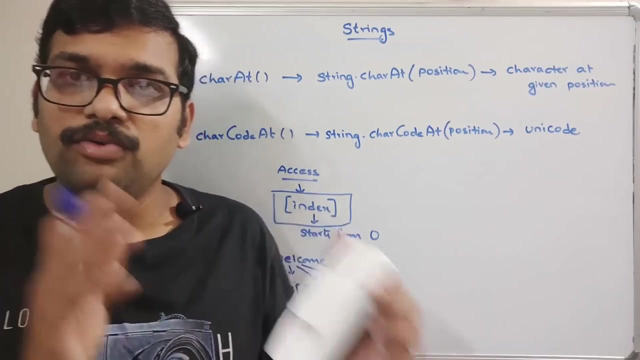 to access the characters with the help of index given in subscript, given index in substrate. so by using this we can access the characters. so hope you understood this one. so i have given the complete information about the strings: how to create a string, how to create the string object and how. what are the different methods, the syntax for different methods available. 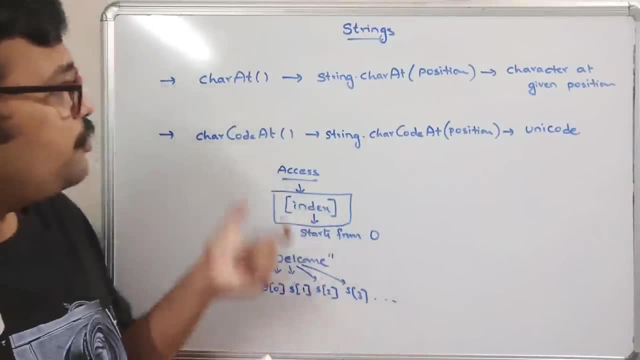 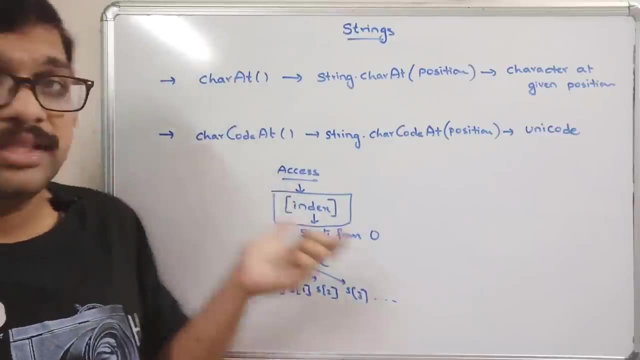 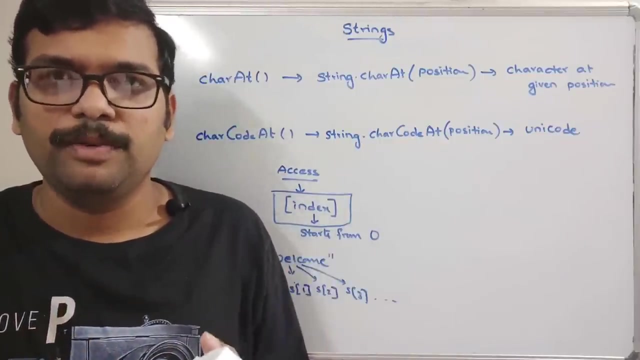 in the strings javascript. now we will execute each and every method. so we i will show you how to create a string, how to create a string object and how to execute all these string methods in the program by executing a small program, right, so that if you are having any doubts, those doubts will be. 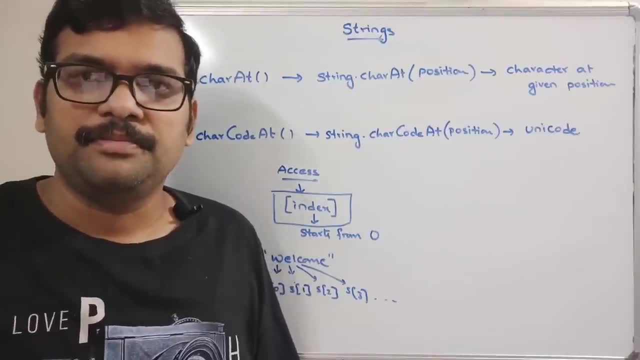 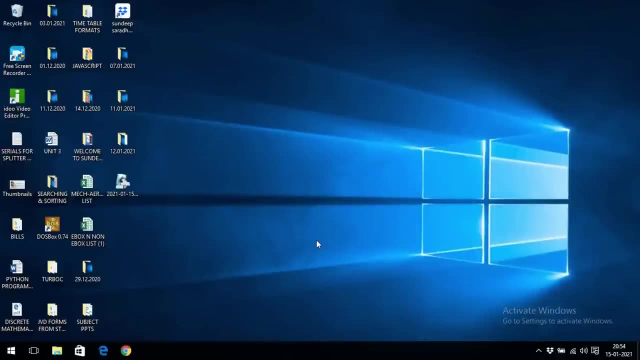 clarified. so let's move on to the system. hello friends. so just now we have seen about the strings- introduction, and then string object and string methods. now i will demonstrate each and every method of the string. so by executing a small html code, we will execute small html code. so 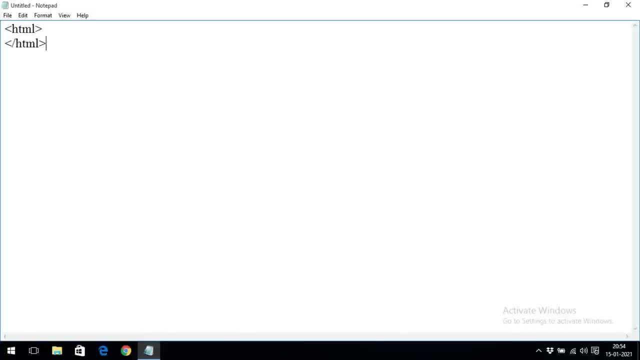 begin with the html tag. so in between the html tag we will create a body and in the body we will write the content, right, yeah, so we'll put the heading first of this topic, that is strings. so this is all about our strings. and now, uh see, string, strings, and then 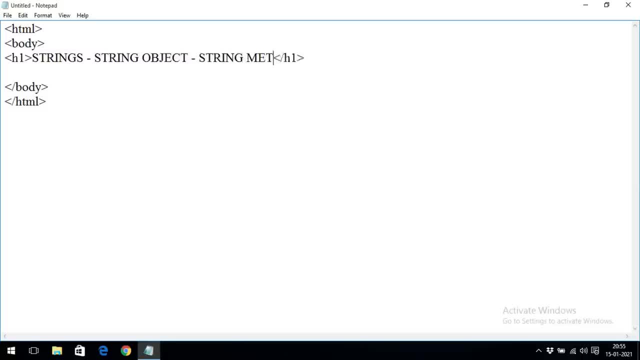 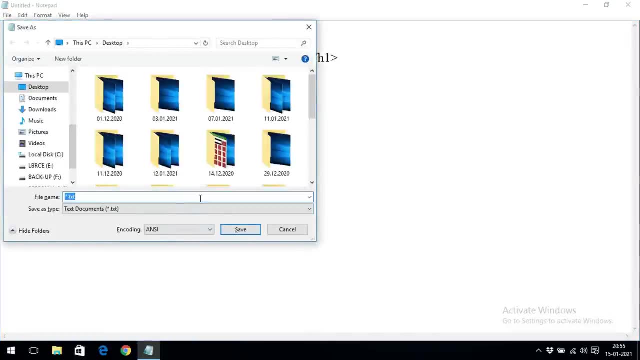 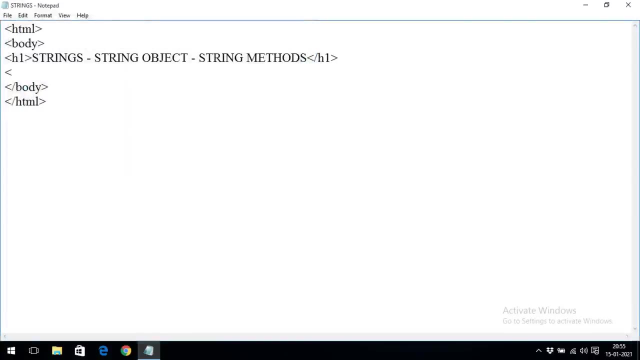 string object string methods: right, so this is our concept now. so inside this we'll write the scripting. right, so string dot html. i'm just saving it. so inside here we can write the script. so inside the script we will create one string. so string can be declared by using the where s1 is equal. to see here we can write here: 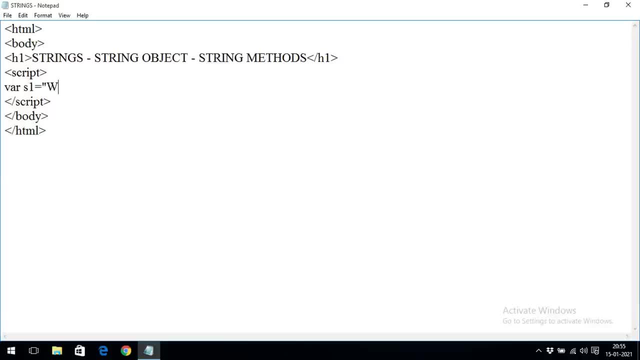 the double quotations. so a string is a number of zero or more characters enclosed in the quotations. so either it can be double quotations or a single quotations. so i am writing welcome to strings in javascript, right? so this is the string we have declared and now we'll display it. so for 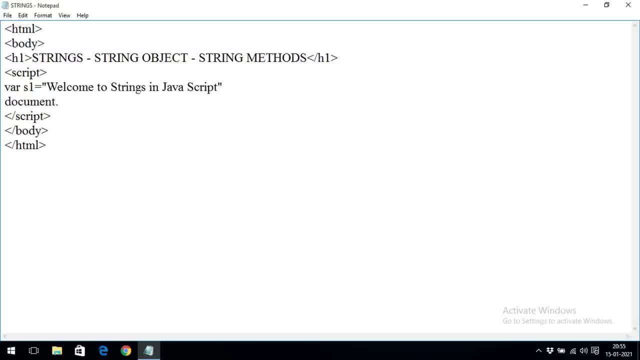 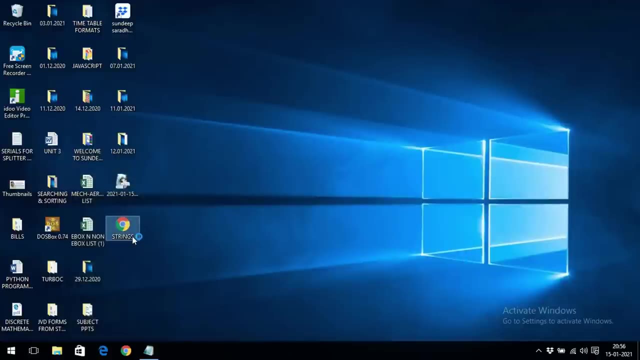 display. we will go with the document: dot write ln s1. okay, so let us execute this one. so i am saving this one. so this is the file, and if you double click on these strings, you will get the string that we have declared in javascript. the file see: 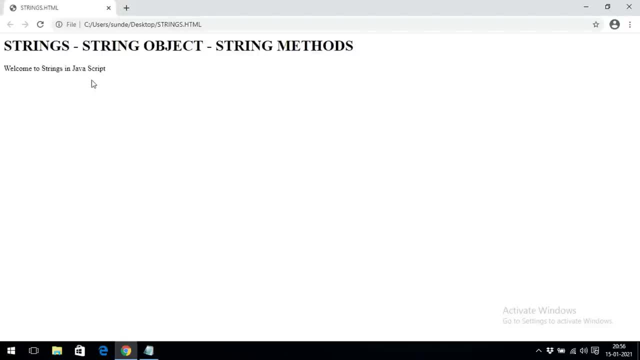 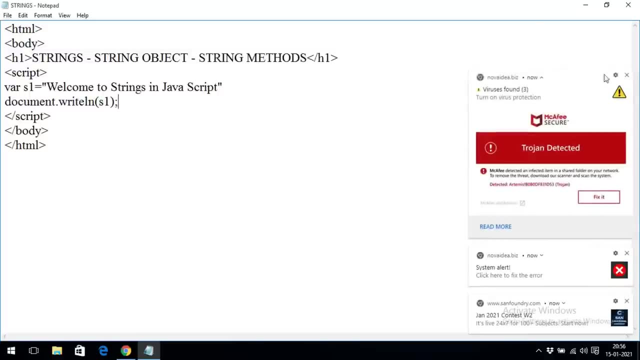 so heading. this one is a heading and this is a text, right? so welcome to strings in javascript. that one, that's what we have written here now. usage of double quotations and single quotations. so even uh string can be used in a single quotation. so see where s2 is equal to. 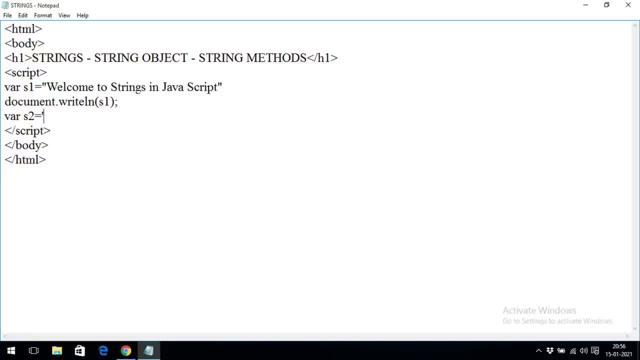 instead of single quotations i have double quotations. this is giving a single quotations string with single quote. so again i will display the same thing. document dot. write ln single quoted string s2- right? so i will do the same thing here for better understanding, right? so instead of single, here it's a double quoted. 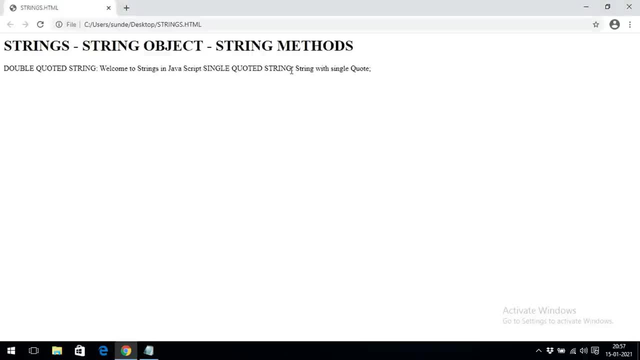 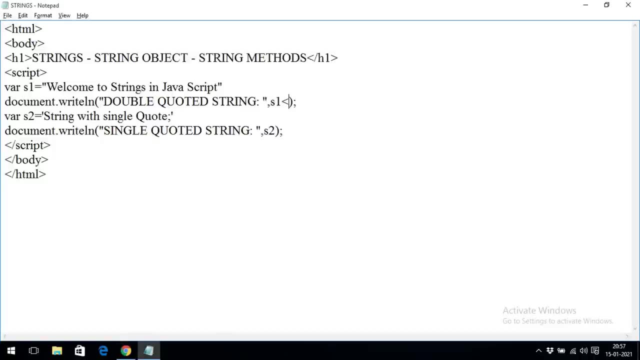 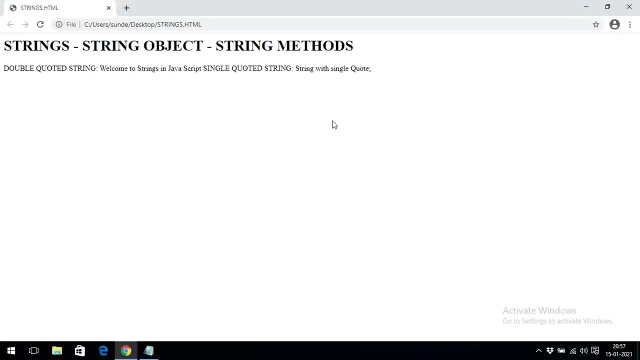 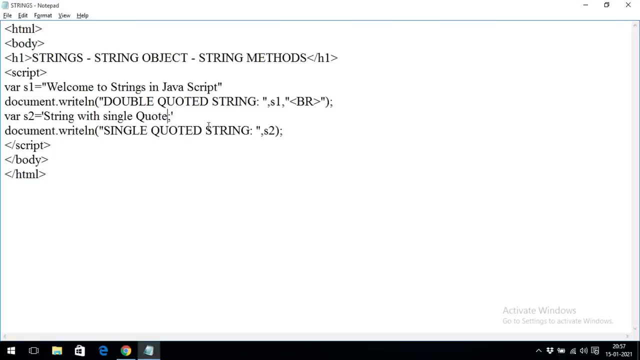 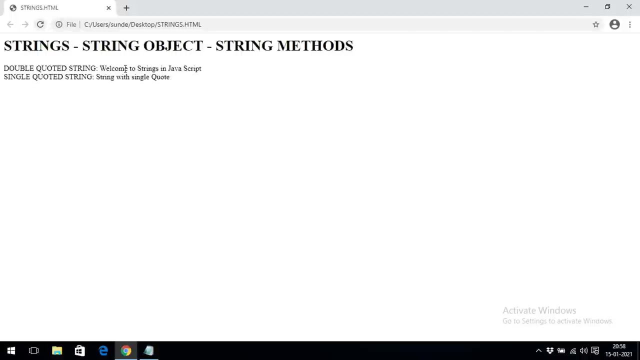 you can observe here: see double quoted string. single quoted string. just a second, so here we can break row. we can give the break row so automatically. it was displayed here right, so double quoted string and single quoted string. this was right now. if you want to insert any double quotations or single quotations. 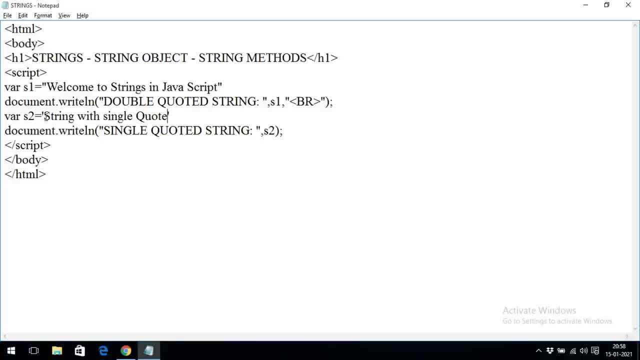 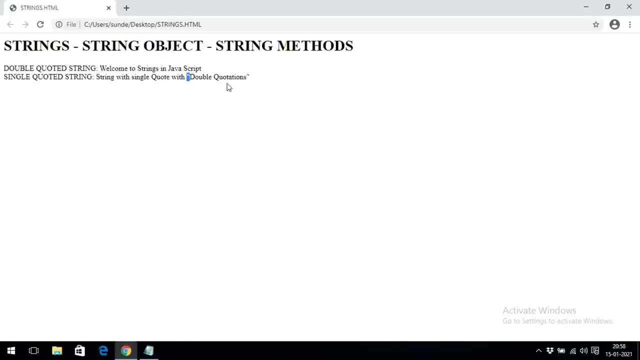 inside the string, so we need to give here. so inside the single quotations, see, inside the single quotations, we can give the double quotations. see, i will write here with double quotations, so i will write here. i will keep this one is a double quotations and let us execute here. see, if you observe here. so it includes the double quotations. okay, the double. 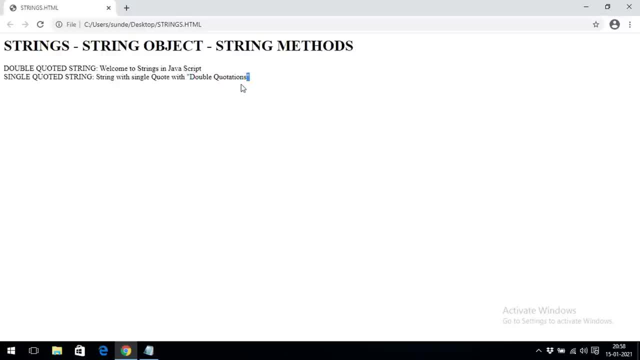 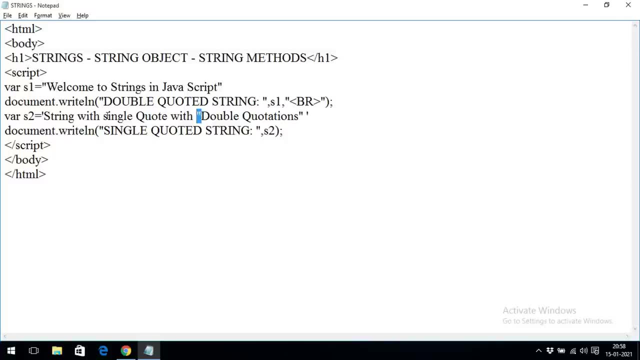 quotations will are included here in double quotations, right, hope you understood. so inside the single quotations we can use the double quotations. similarly, inside the single double quotations we can use the single quotations. right, see, i will show you javascript. i will keep this javascript in a single quotation, you can. 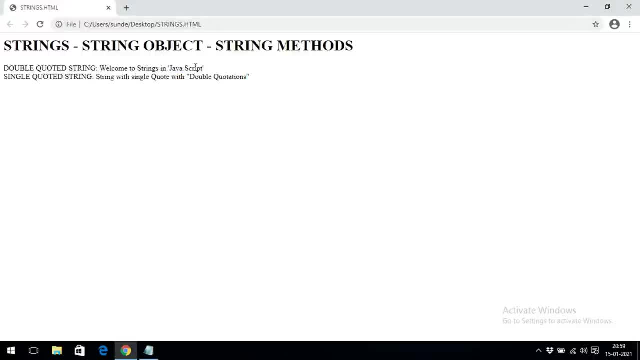 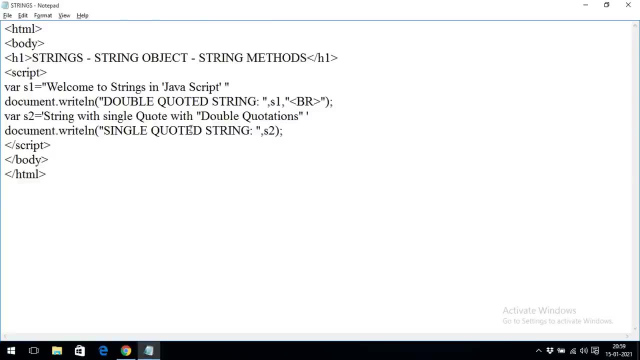 observe here so you can observe in the output. we will get the single quotation right so that that is the usage of uh: double quotations and single quotations. so a string is a is zero or a more number of characters enclosed in a quotations. either it may be a single quotations or it may. 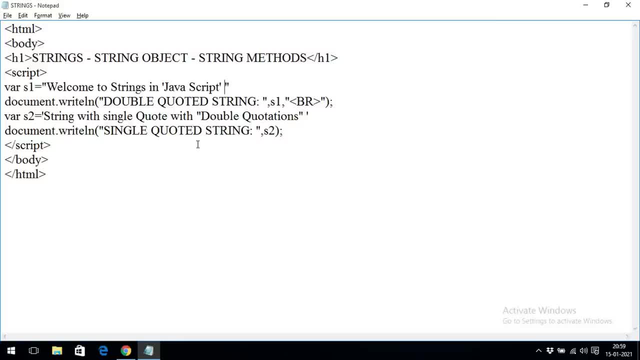 be a double quotations, right then. and the next one, uh see, we can have, uh, the string object, how to a string object. so this is a normal string. we can have the type of a thing, see document dot. so instead of this one, i will give type of yes to, yes to okay. 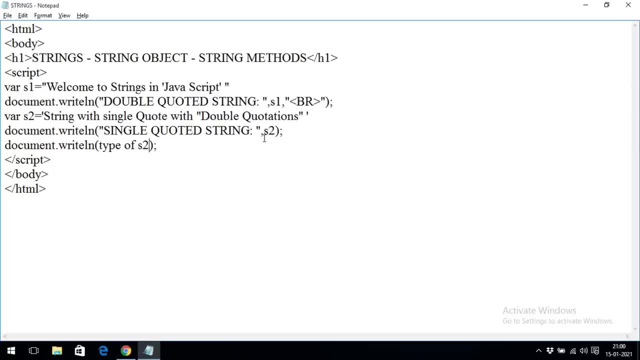 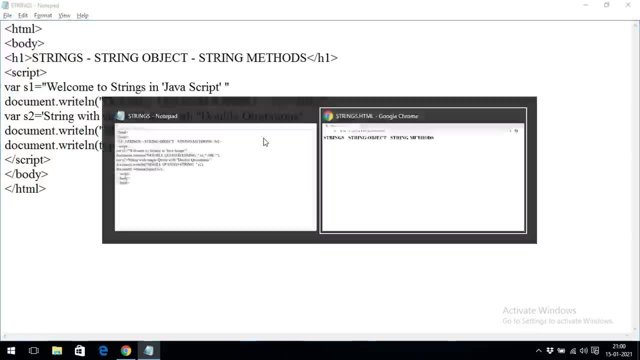 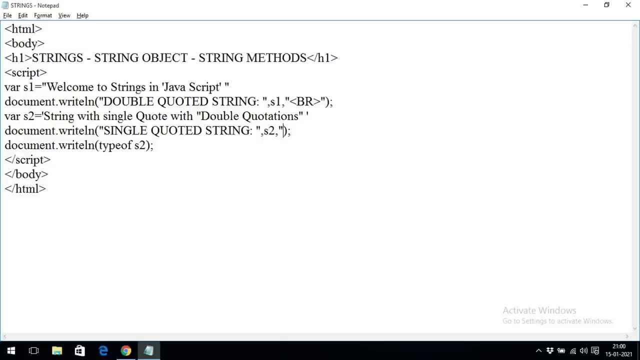 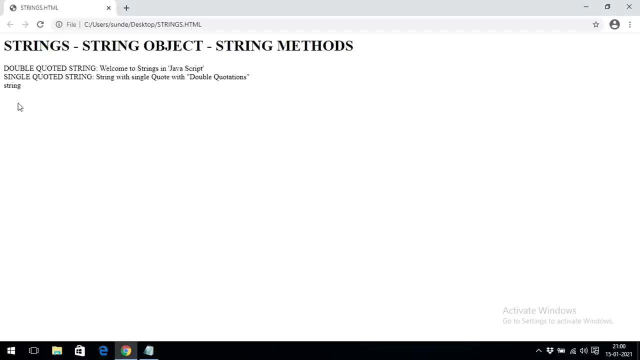 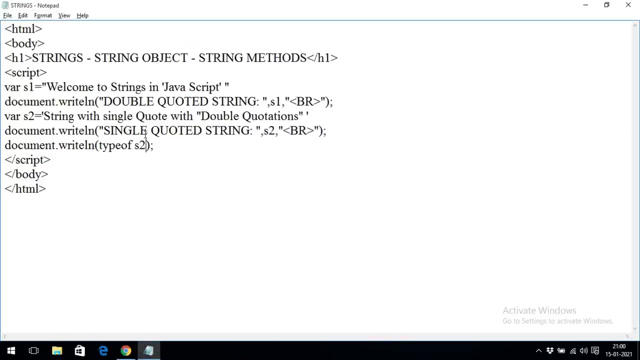 you can observe. sorry, yeah, you can observe, it is a string. see, you can observe here string. okay, you can observe here string. right, and if you create a string object, so where we can create a string object, s3 is equal to, we have to use a new keyword and followed by string. 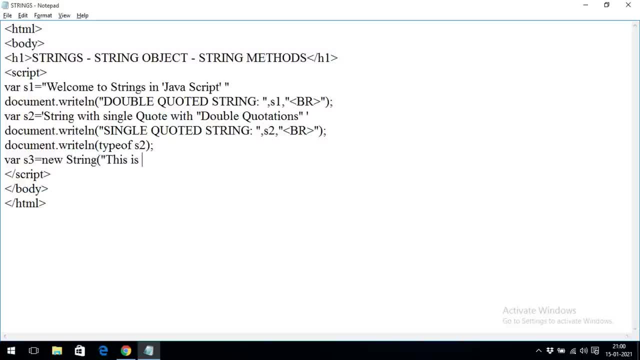 and pass the string here. so this is string object. right now, document dot write ln. yes, three string object: s3. right, so here you can go with vr. you can observe here string object. so this is string object. and now you can check with the data type. so here you can observe type of s3. 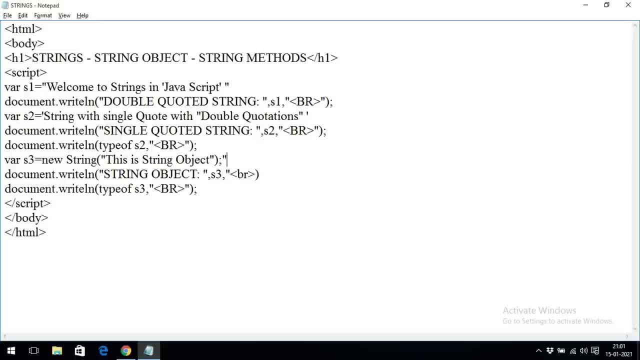 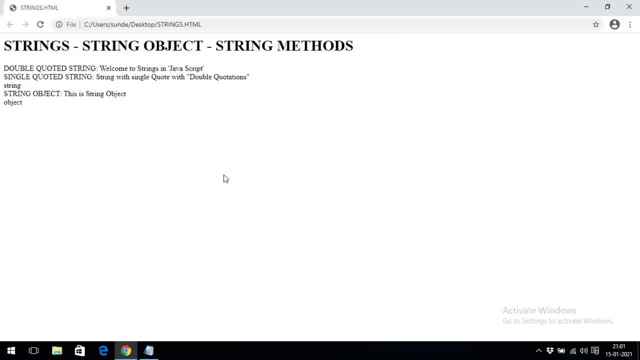 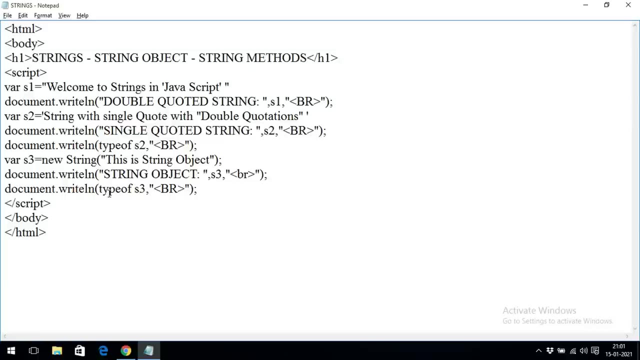 type of s3. you can observe here, type of s3 is an object, so whatever the operators we have seen in the numbers, that means double is equal to, triple is equal to. the same can be applied in the strings also, right? so if you are using, double is equal to we. 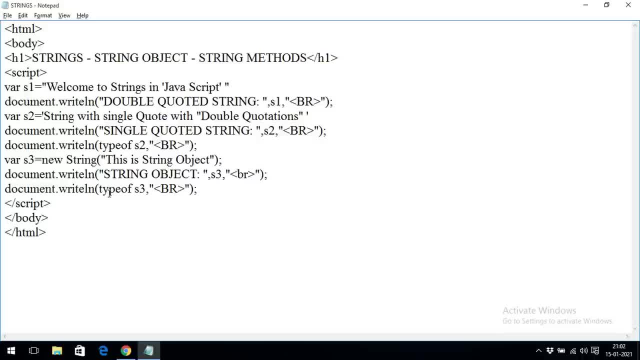 will get the. i mean the values will be compared, and if you are comparing, using triple is equal to the values. the number is the same. you can see. so the important thing in the a's, both of the a's, as always, right, so let's go back toار. 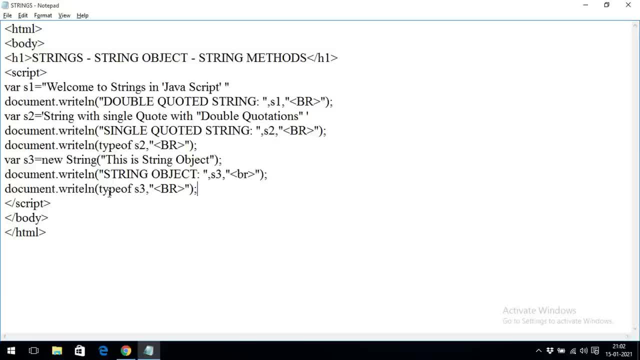 triple is equal to the types and values will be combined. The same thing here, And this is how we can create the objects and strings. Now we will see the method. So we will see the method. So what are the different methods? So I will give you the document dot. I will write the heading. 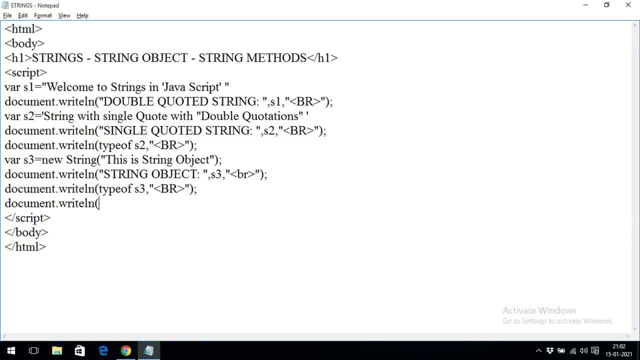 here: write ln instead of. I mean, if you want to write a heading in the script, we have to put in the document dot, write ln, right? So h1, string methods. See, you can observe here string methods. 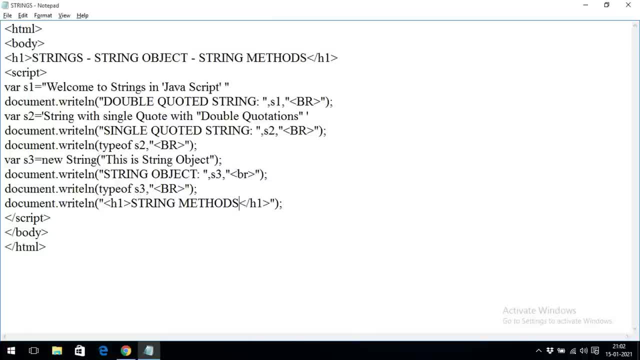 right. Now we will see one by one. So what are the string methods? The first one is index of index of right, So index of means. so we have to pass one argument and we will get the string. So I will. so we are having some s1,. 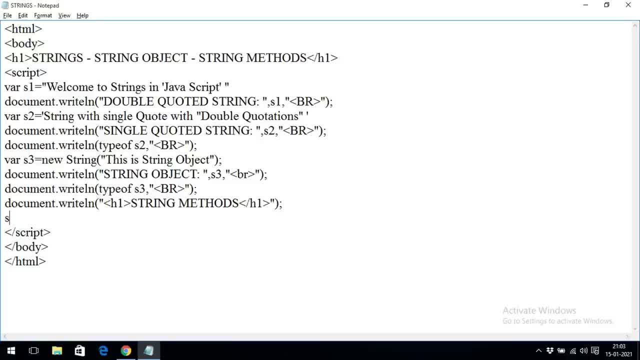 s2, and s3.. So we will see that document. dot write ln. So here we will see what is the function: Index of. So we will write here: index O, capital of Index of function. ok, right now the syntax is: what is the syntax? so string dot, that means s1 dot. so i just want to. 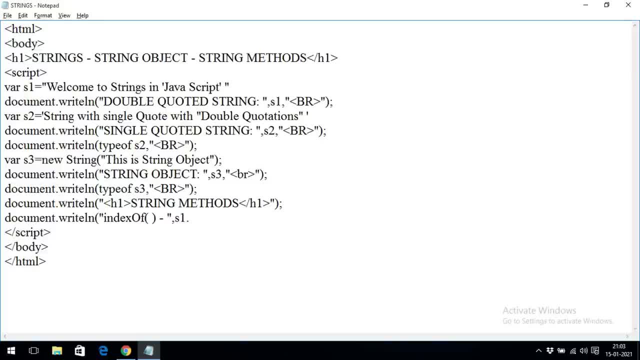 identify the index of some character or a string of s1, so i have to write s1 dot. if you want to find out the index of any character in the s2, we have to write s2 dot. so like this s1 dot index of give the string here. so either it may be a character or a string. so i will go with some. 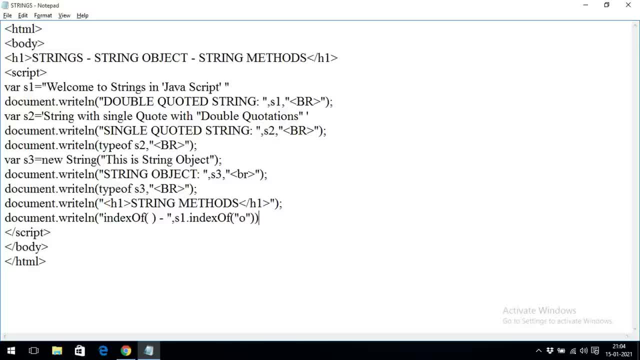 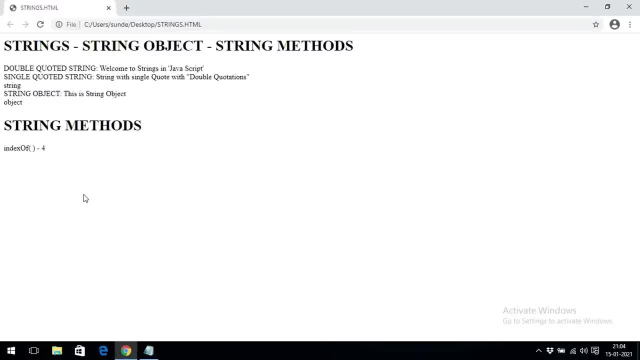 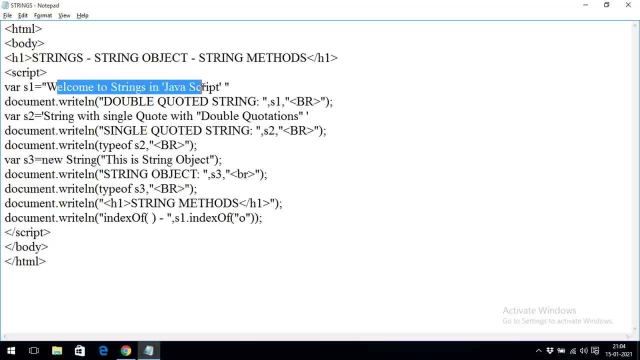 o, so it will give first occurrence. okay, it will give the first occurrence. we'll check. see index of index of is 4, that means index of o. so here we are checking o. what is the in the s1? what is the s1 here? so you can observe: s1 is a welcome to string in javascript. so in that we are finding the index of. 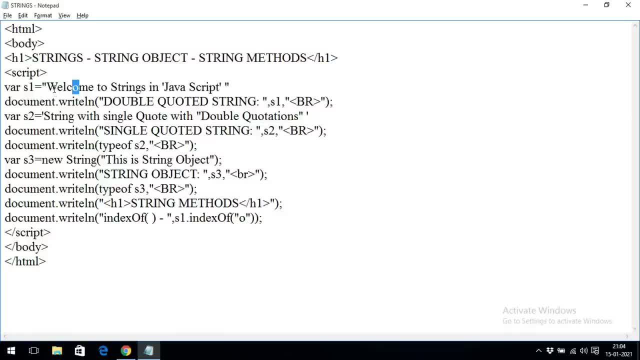 o. that means this one: like: what is the value? the index starts from 0 itself, 0, 1, 2, 3 and 4, so we got the result as 4 and if you are giving any string which is not available, so i am giving. 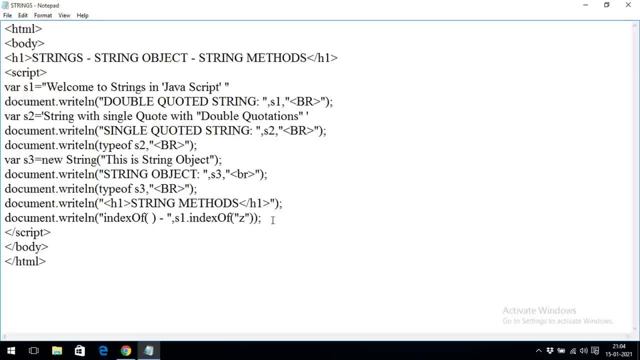 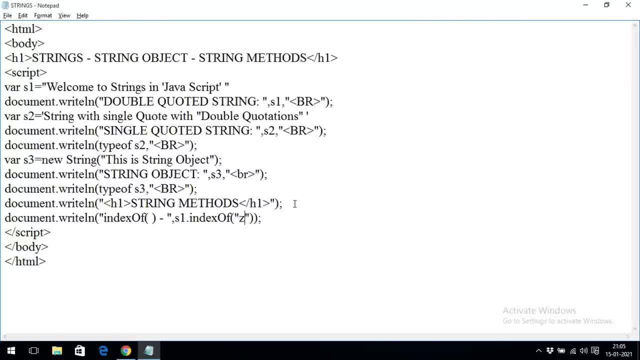 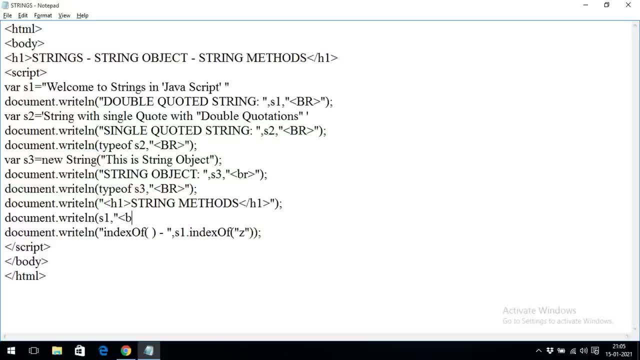 s1 comma see. so just for representation, i am giving s1 comma s1. i will go with the br. next, s2 is equal to s2 and also I will display the s3 also. okay, and we will go with the br. br means break row. okay, s3 is equal to s3 and also we will go with the br because 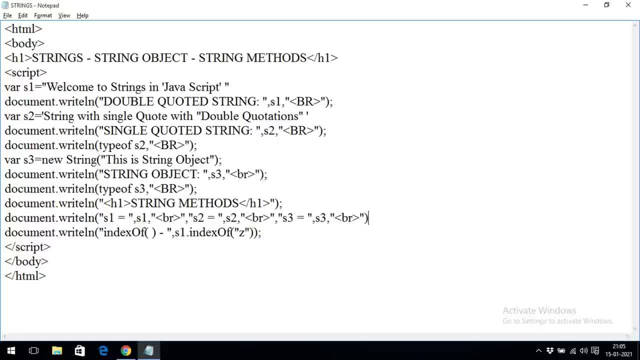 for every time we are supposed to print the output in the next line. now you can observe s1, s2, s3, okay, so here we are getting. we are finding some z in s1. okay, position of z in s1. so index of function. position of z in s1. 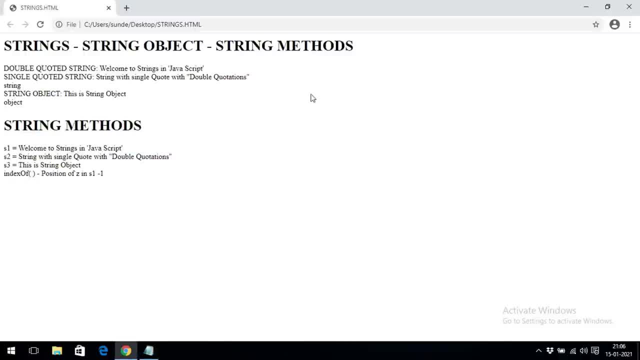 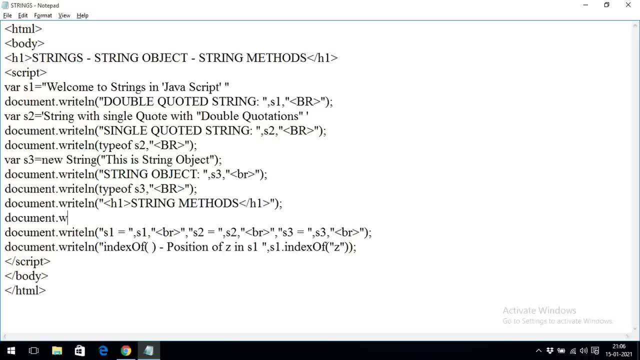 so you can observe, here, right at the next, see the index of position. so always here you can observe, we have to pass one string or any character so that it will display the index of that particular character or a string. and there is a one more function called 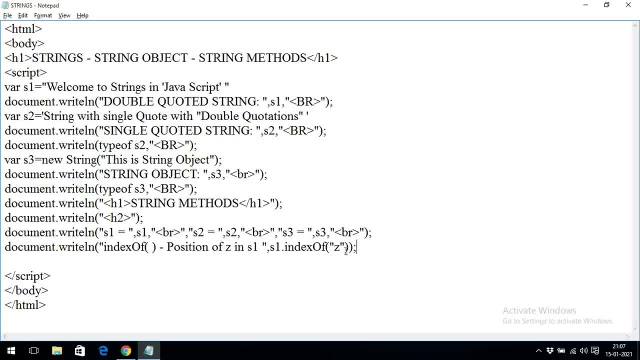 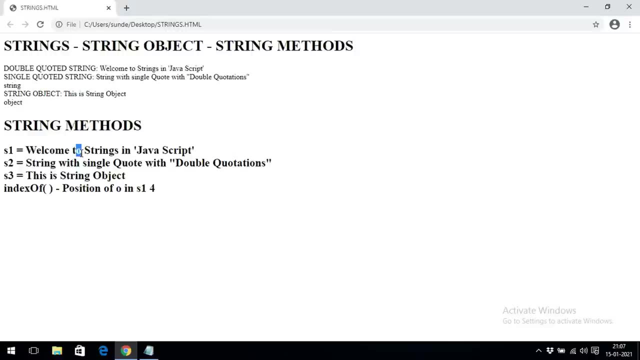 last index of. so here this is in from the first occurrence. okay, so if you go with the o, so that is a first occurrence position of o in s1, so you can find. so you can find here s1 it is having one, two, so two o's right so. but here we are getting the index value as four. that means 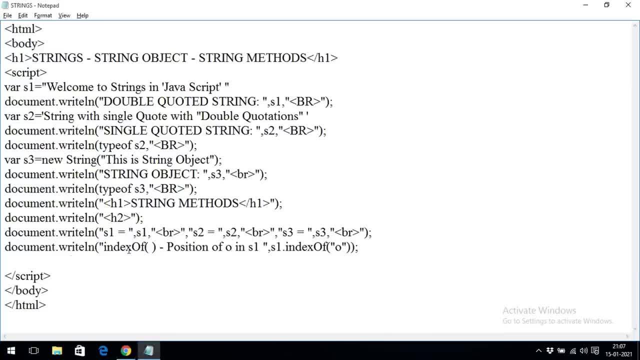 it is a first occurrence. if you want to get the last occurrence, we are having the same function. yeah, there is a one more function called last index of, last index of. so in the last index of will, i will be the capital, i will be the capital and o will be the capital now. position of o in s1. it is a last index. 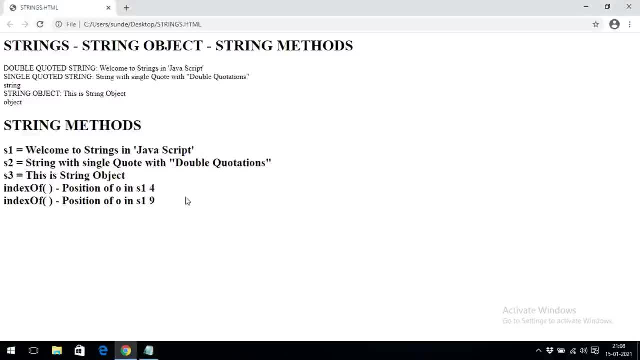 okay, now we will check the result. so you are getting some value as nine you can observe here: zero one, two, three, four, five, six, seven. zero one, two, three, four, five, six, seven, eight and nine ninth, one right. so position of o in s1. last index of. this is the last index of. it is not. 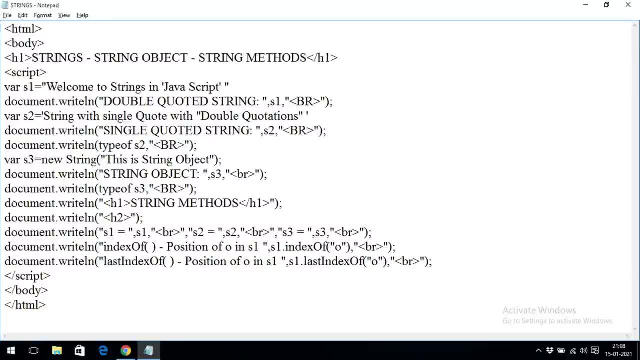 index of last index of o is nine, right, so hope you understood from the starting position. if you want to check the index, we will go with the index of. that means the first occurrence and if it is a last index of function it will search for the position of event substring from the last. okay. 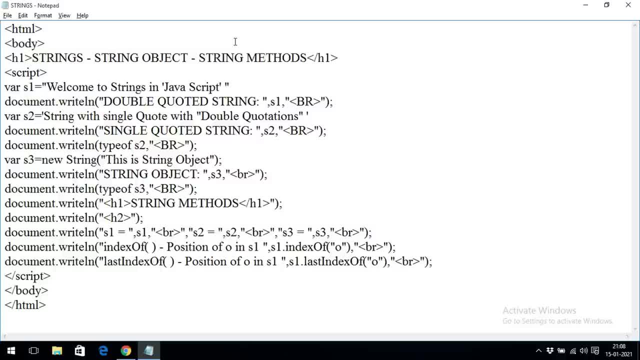 from the last, last occurrence, that means the last occurrence, first occurrence and last occurrence. and here we can also give a parameter. the second argument, that is a starting. that means where we have to start from, where we have to start, index of with one argument, with one argument. so i just 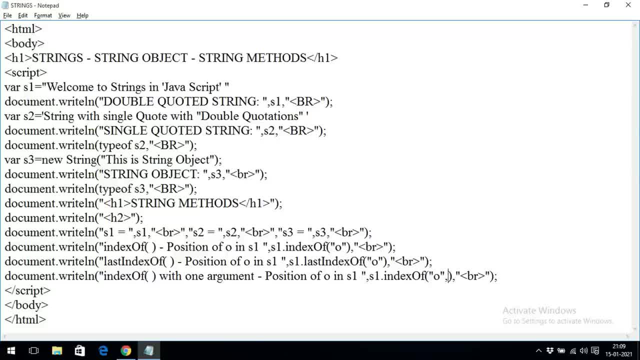 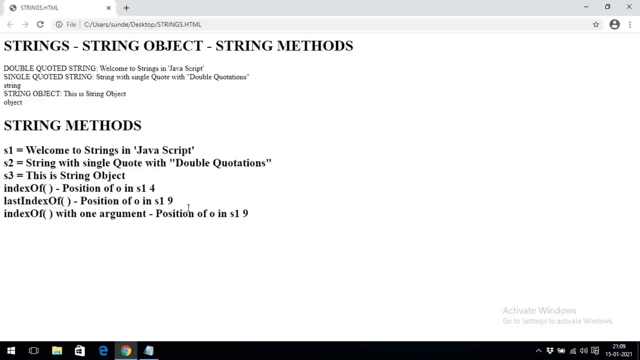 want to find the value of o, index of o and i need to search from the position, some six onwards. okay, from six onwards, see index of. with one argument, so i have given from sixth, so sixth position, from the sixth position it will search for the whole as a first occurrence. so zero, one, two, three, four, five, six from here onwards. 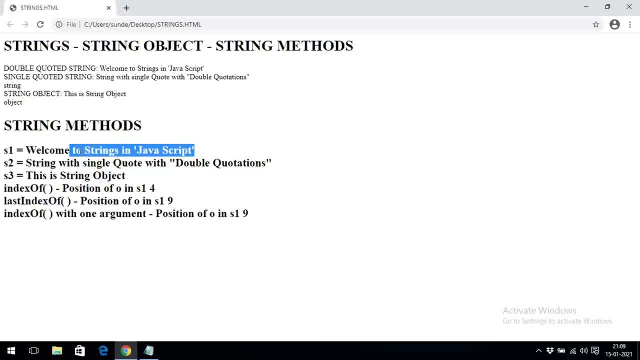 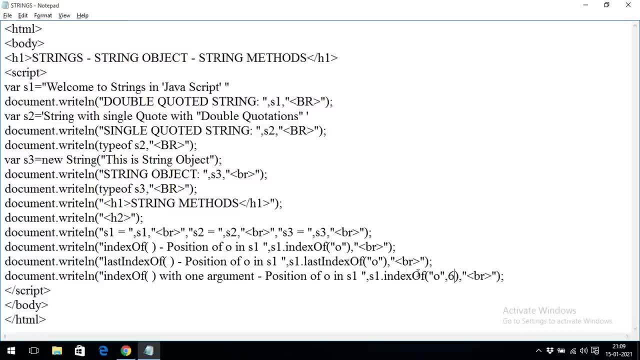 it will search for the first occurrence of war. so you can observe here: the position is nine, position is 9.. Okay, If you, if the index, I mean if the value- is not available, automatically it will return minus 1.. So you can see So instead of o. if you check for z. if you check for z. 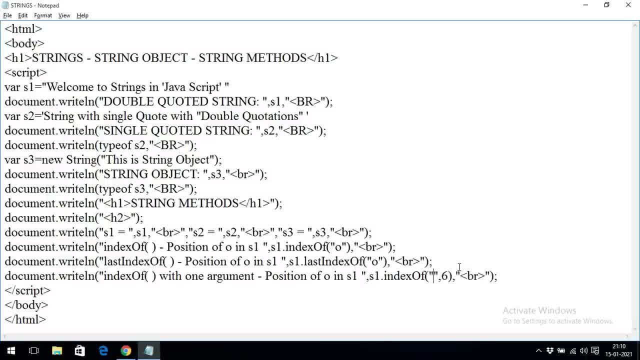 we will get a minus 1.. Okay, So hope you understood this one index of and the last index of. Now there is a one more function called search, So we can search whether the string is available here or not. So next one is a search search function: Search. 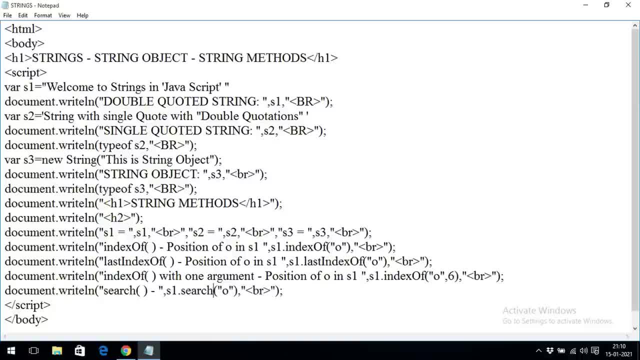 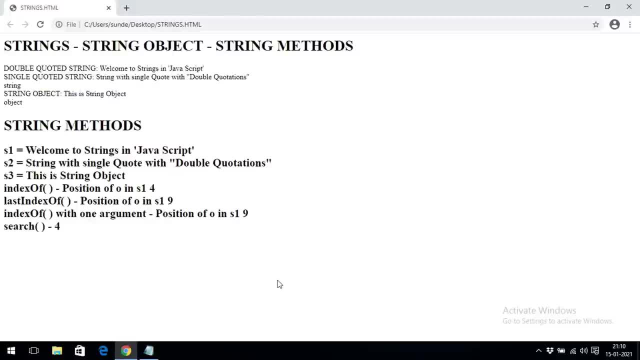 Here I will search o in the given s1.. See 4, 4.. Okay, So here search will also give the same thing. Okay, There is index position from where it has been started, But the only difference is: 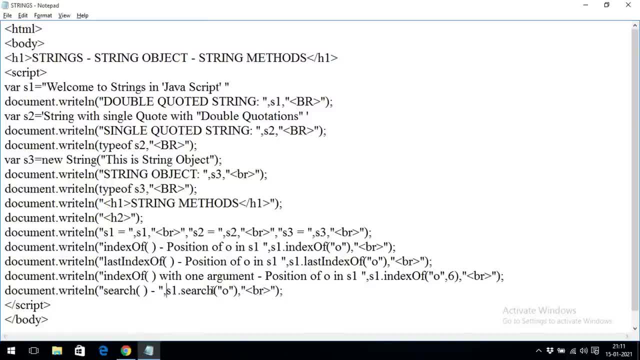 in search function we should not give the arguments, We should not give the second argument. Okay, So in index of we are giving the second argument. that means where we have, from where we have to start the search. So here in the search function, we should not give the. 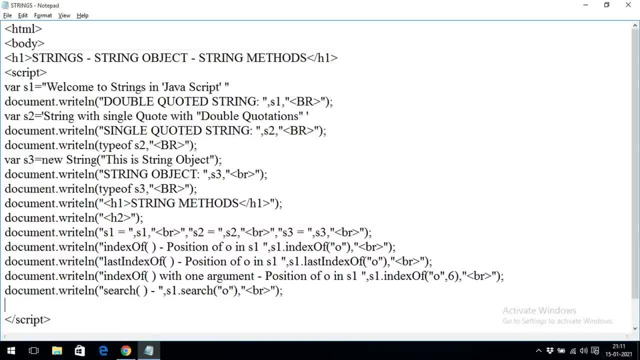 second argument. We are, we are not supposed to go with the second argument. That is the only difference between search and index of, And then slicing, So extracting some portions of the string. So then we will go with the slicing. So first method is a slice method, Slice method. 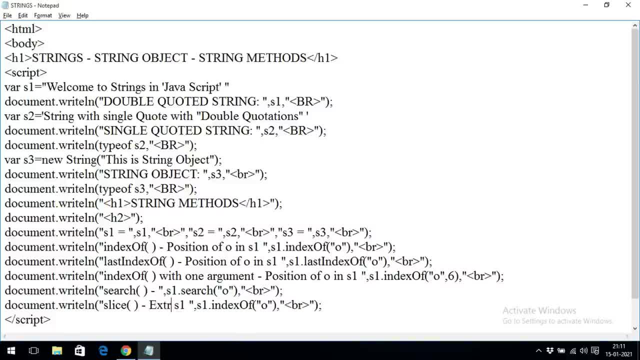 Okay, Extracting from s1. From s1.. Right, So here you can go with s1 dot slice. So here in slice we need to give the starting index and stop index. Okay, So we will give some 0th index to 7th index, So 7 will not be. 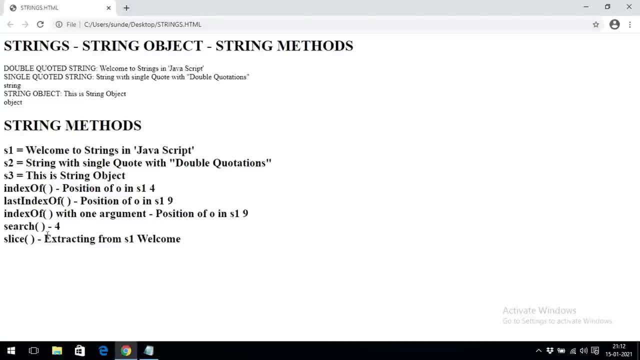 included. 7 will not be included. So you can observe here: So extracting from s1 slice, So from 0 to 7.. 0th index is here: 0,, 1,, 2,, 3,, 4,, 5,, 6. So it should not include the 7. It will. 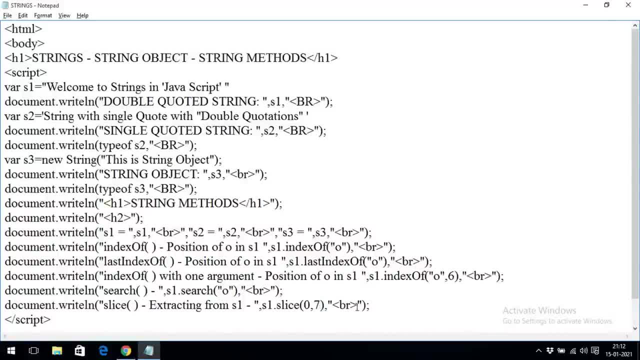 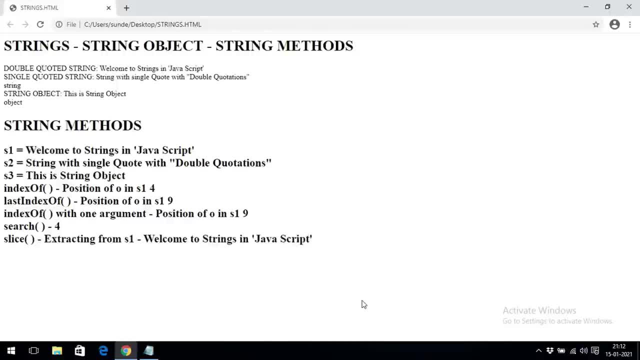 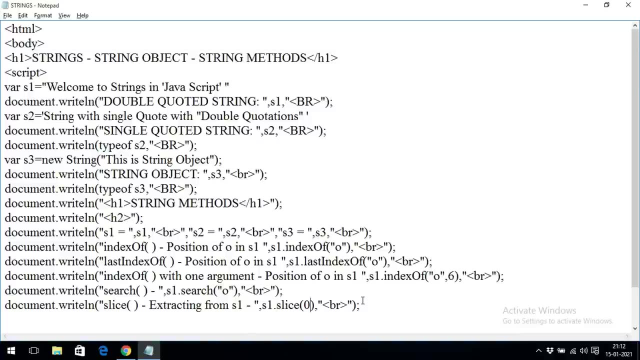 go with the 6 itself Right And see, we can. if you are not giving the second argument in this slice, we will get the complete string. Okay, It's an optional. The second argument, that is, a stop index, is an optional If you are not giving the stop index automatically. 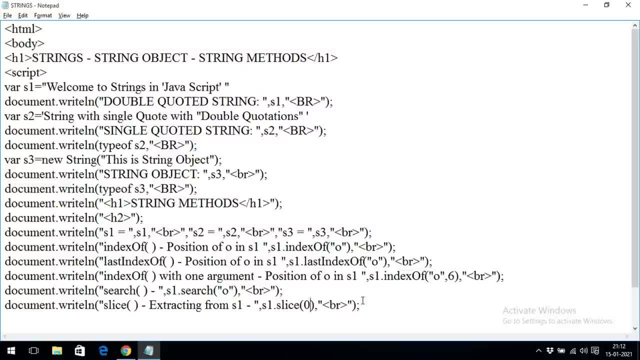 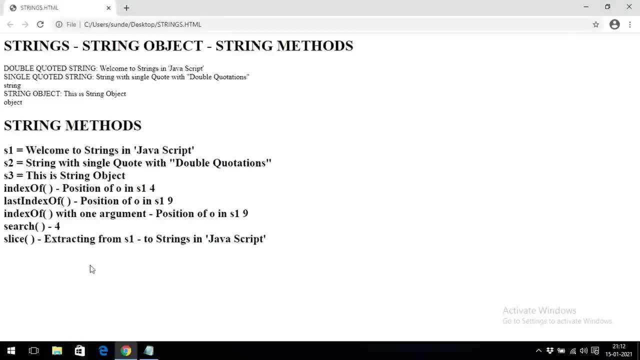 it will start extracting from the given index value to the end of the string. So for example, if you go with 7, it will start extracting from the 7th index. So you can observe here, from seventh index it start executing. and if you go with some 17, it will start extracting from. 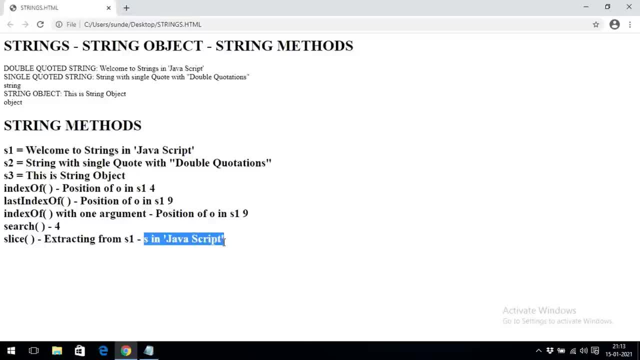 the 17th index value, so this is the 17th. okay, so like this, this is an optional thing, so if you go with the 0 to 17, so you will get up to here. okay, up to here. 0 to 17. so this is the 0 to 17, right. 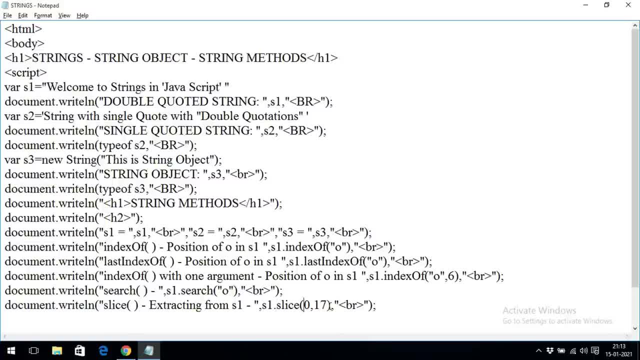 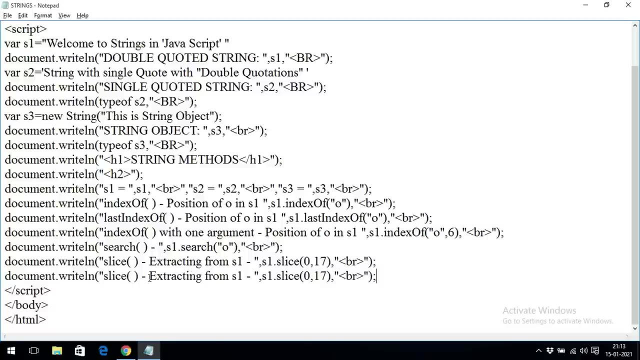 and here we can also give them negative indexes. so if it is a positive index, it will start from the left to right. if we have give the negative index, it will start with the right to left. okay, see, I will go you, I will explain you this. with negative 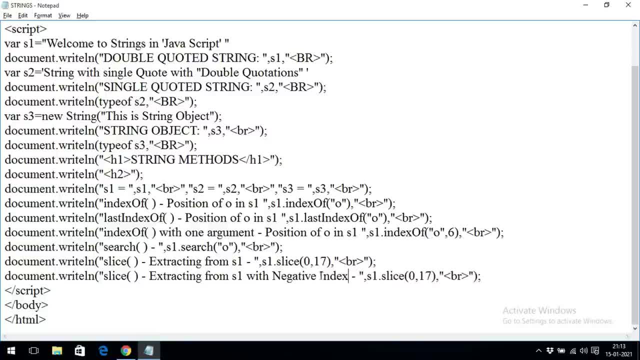 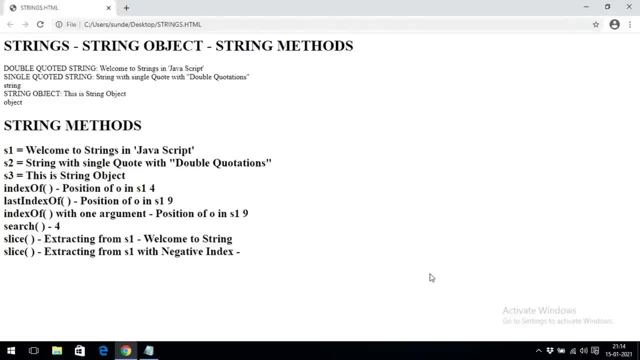 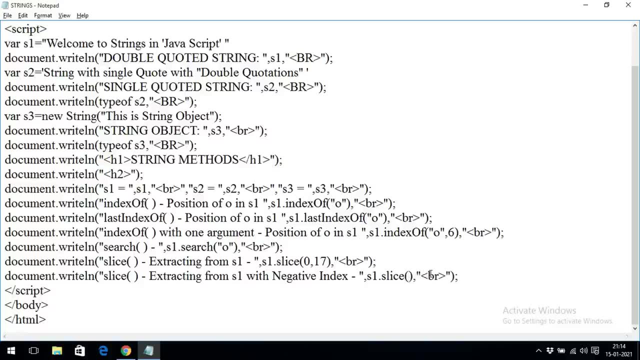 index. it's a negative index, so I will go with the negative index. right, so minus 1. so here the minus 1 is the index of last 1. minus 1 is the index of last 1, so I will go with some 5 minus 4, 2- sorry, minus 17, 2. 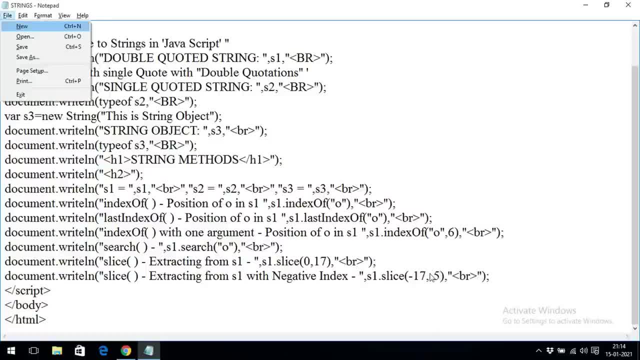 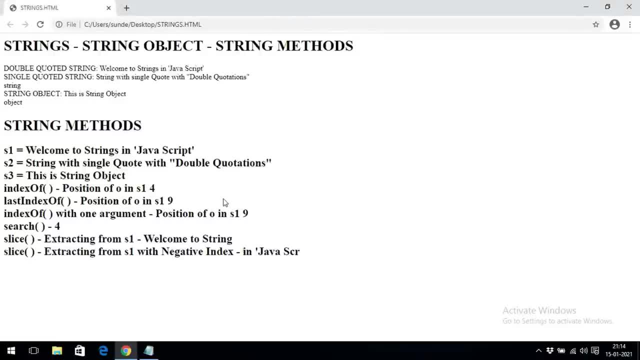 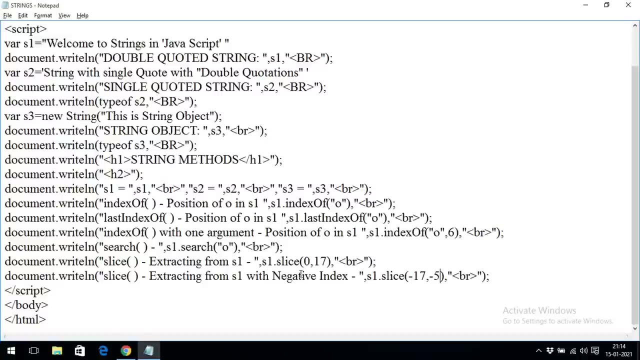 minus 4, 5.. Okay, You can observe here minus 17 to minus 5.. So minus 17 to minus 5 means you can observe here. So this is the this one. So always it will start from. the negative index will start from. 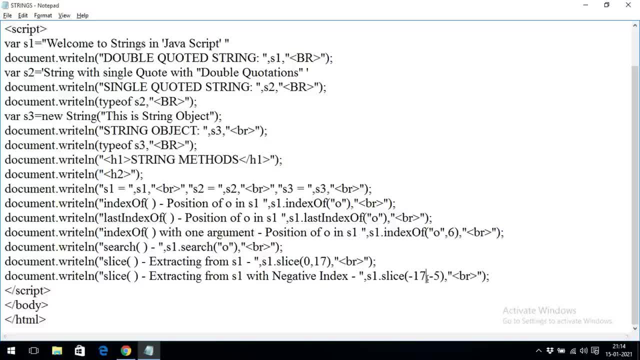 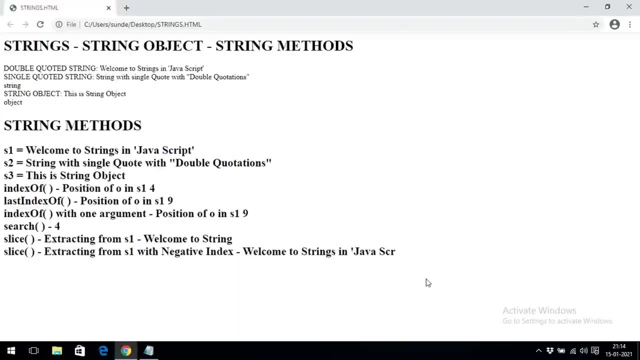 left. Okay, Left onwards, Sorry, right, right, most The last index value. the index value for the last element is minus 1.. Okay, The index value of the last element will be the minus 1.. You can observe here 0 to minus 5.. That means up to here it will get. Okay, So here minus. 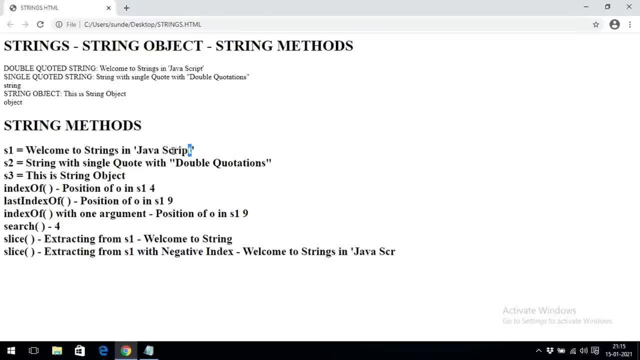 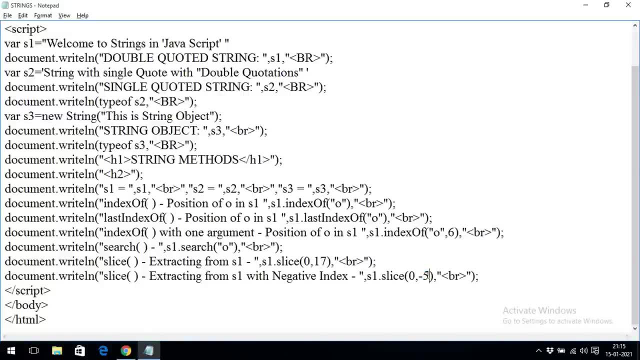 last: minus 1, minus 2, minus 3, minus 4, minus 5.. Okay, It does not include the minus 5.. It does not include the minus 5.. Hope you understood this Right Negative index. And the next one is substring, Substring, So similar to the slice. 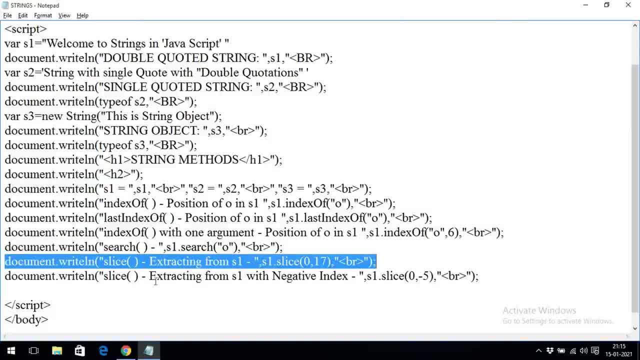 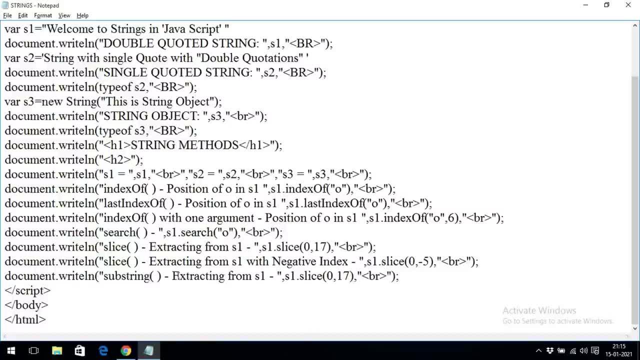 function. we are having a one more function called substring, See. Substring is a single term, So we should not give any capital letter: S1, dot, substring. So here here also the same thing, So we will. 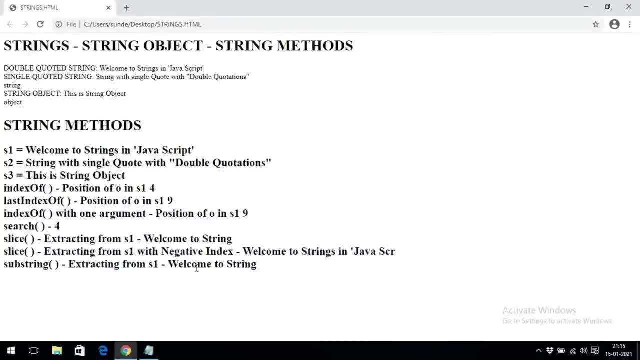 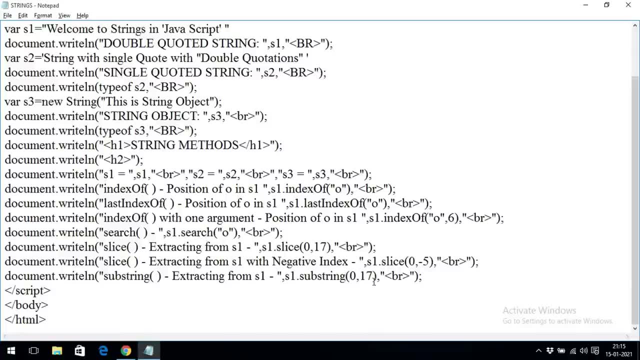 We will give some starting point and ending point. So starting from some welcome to string. So that is 0 to 17 index. So what is the difference between substring and slice? So slice will accept the negative index, but substring will not accept the negative index. That is the only thing. 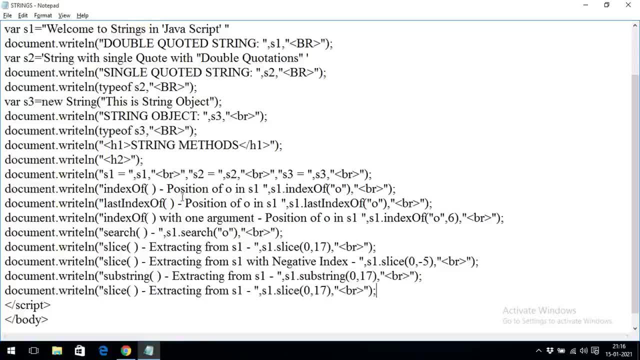 And then come into the, there is a one more thing called substr, Substr. So what is the difference here? Instead of giving the substring, So substr, So it will start. the first one is the starting position and the second one is the length of the string you need. 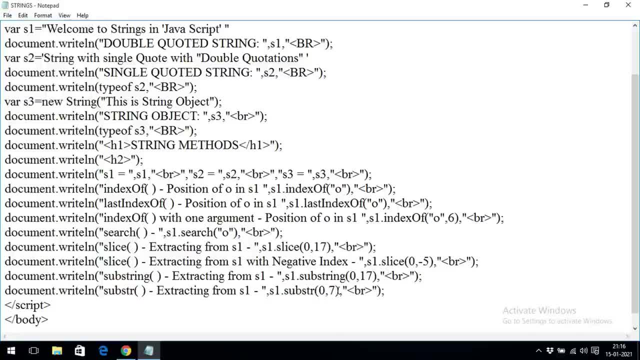 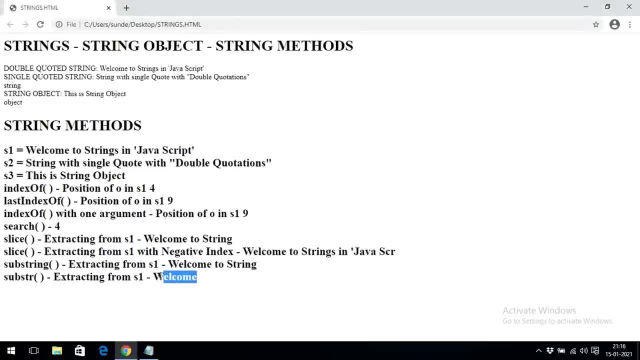 to extract. For example, if you go with the seven, seven characters, it will extract the seven characters. You can observe here seven characters: 0, 1,, 2,, 3,, 4,, 5,, 6,, 7 characters, If you want to. 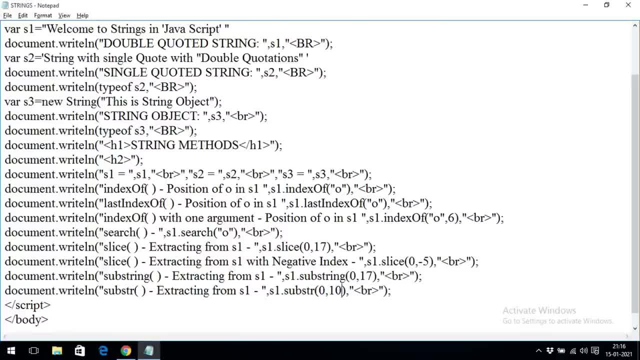 get the 10 characters you will go with here, 10.. So that will get the 10 characters Right. So that is the thing. And here also it will accept the negative index. Substr will also accept the negative index, Right. Then there is a one more function, that 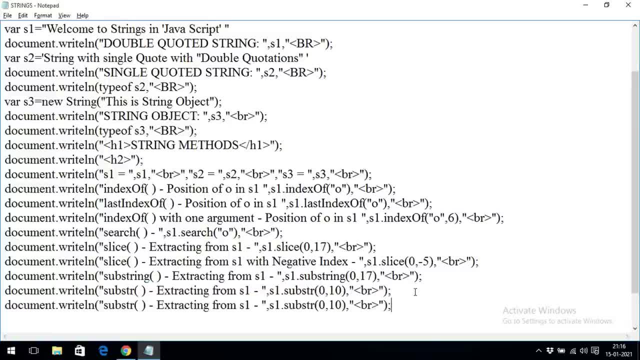 is a replace function, Replace function. So replace function will take the two arguments: One is the old string and the next one is the new string. Okay, So not extracting replacing: See replacing S1.. I will go with the replace. What is the S1?? Welcome to strings in JavaScript, So I will give. 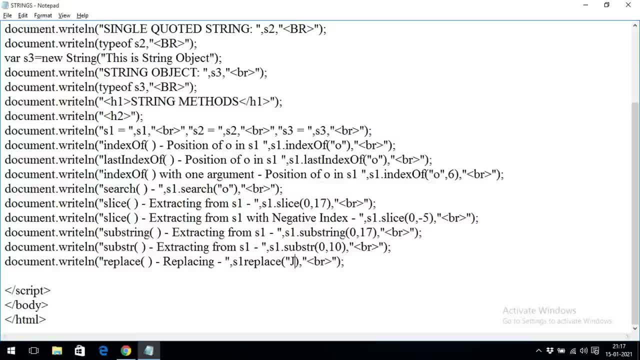 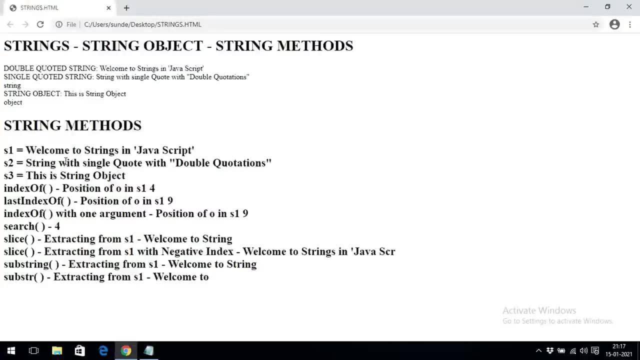 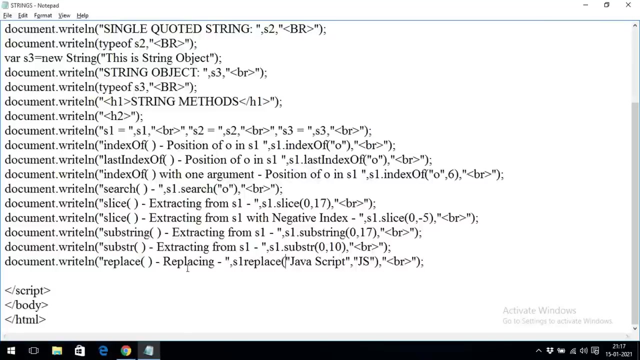 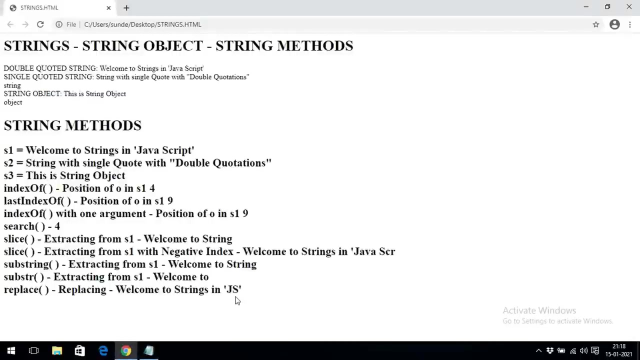 the JavaScript Right. So I will give the old string and new string is JS. Okay, JavaScript is replaced with JS. Now you can observe here: S1.replace. Right Now you got it. Welcome to strings in JS. So one thing we need to remember. 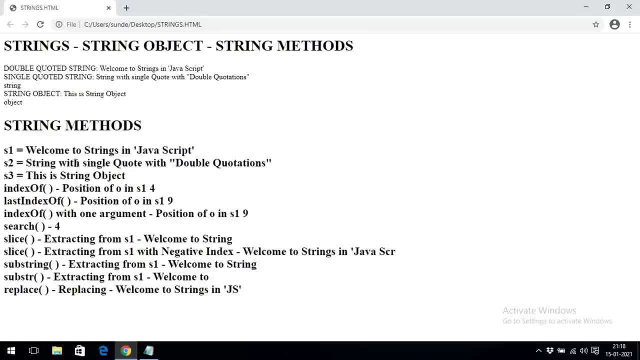 whatever the thing we are doing, it will create a new string, but the original string will not be modified. here The original string will not be modified, Right? So replace means old string, common new string. So it will replace only the first occurrence. 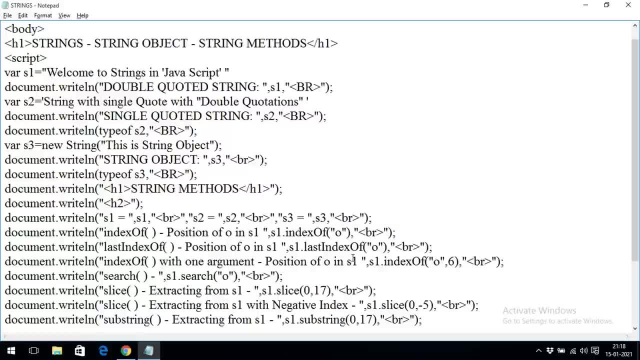 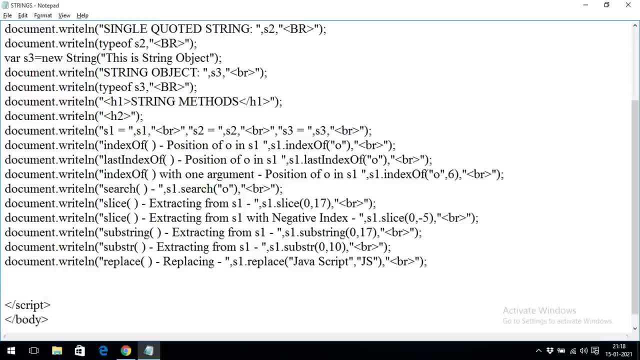 If our string is having a more number of occurrences, it will replace only the first occurrence. Right There is a replace function And there are a few more functions called lowercase and uppercase. So I will give you somewhere S4 is equal to. I will take some. 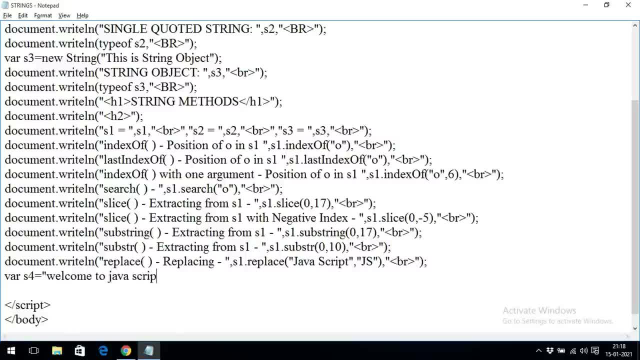 see welcome to JavaScript. All are in small letters, Right, So I will do here document. Sorry, I will take one more variable. S5 is equal to S4.toUppercase, So this is a function to uppercase. It will convert everything in a uppercase character. Now you can. 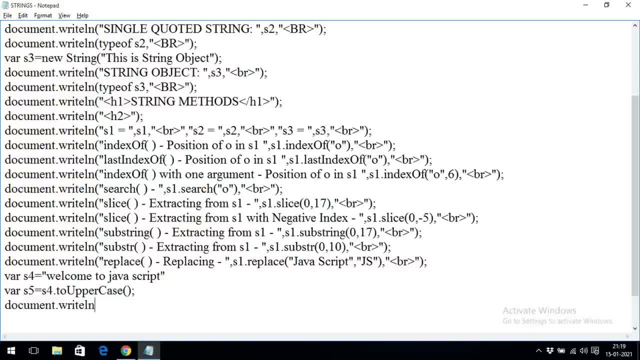 go with the documentwriteln S5.. Okay, Comma vr, because So for every function, we are giving it a display. See, you can observe. Welcome to JavaScript. This is a uppercase. Now we know that S5 is having the uppercase. 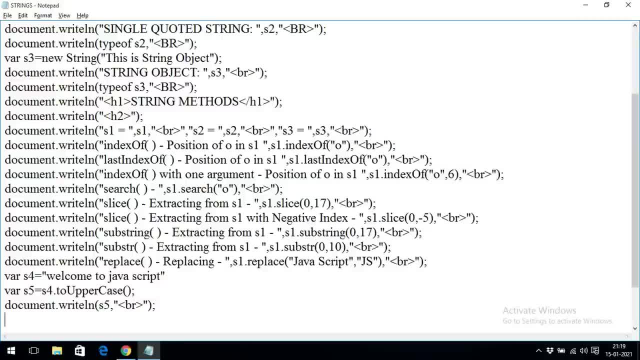 Now I will show you one more function. So documentwriteln S5.toUppercase. So all the lowercase characters will be in, all the uppercase character will be converted to lowercase character. So this, these are the two functions: two uppercase, two lowercase. So u and c is capital. 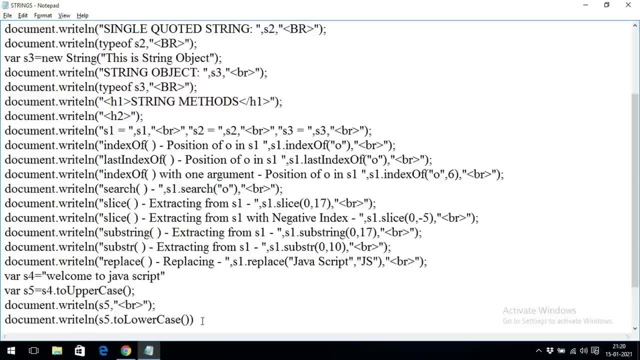 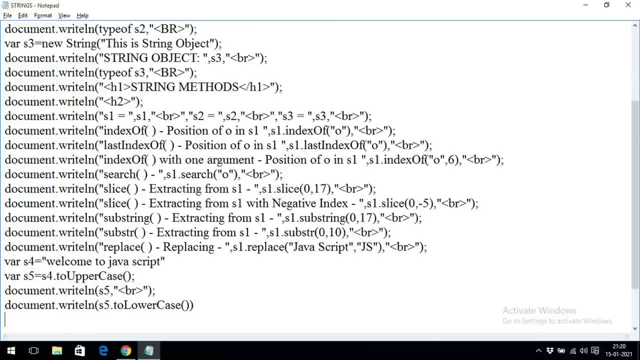 here l and c are capital here, right. And then we are also having the concatenation. okay, we are also having the concatenation function will be, which will be concatenate, two different strings. That means this is a replacement with replacing of a plus operator. 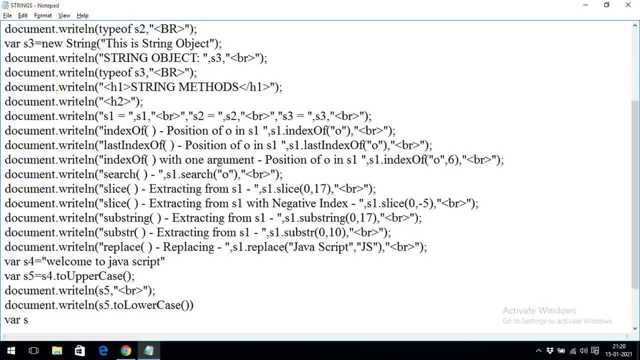 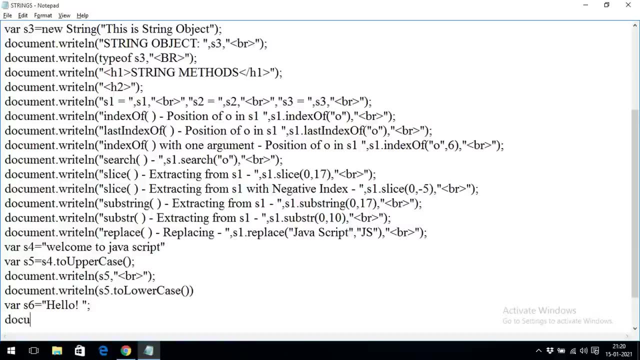 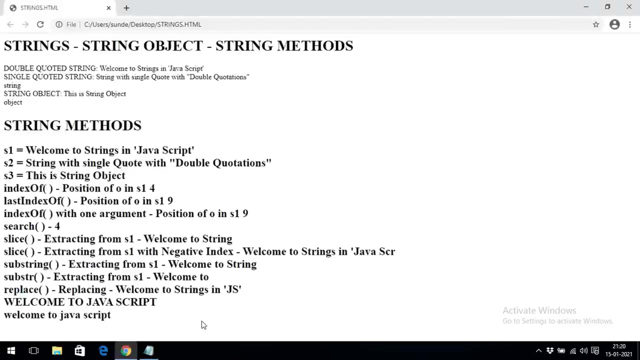 plus operator right. So where s6 is equal to, I will take directly. I will give the string so hello. So now I will concatenate documentwriteln concat of s6 comma s4. So that both will be concatenated. both will be concatenated, right. 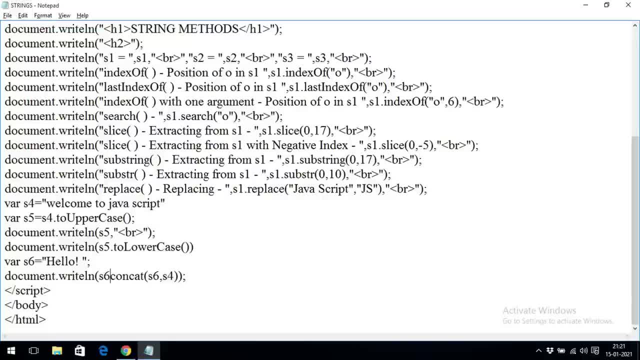 See where we have to concatenate. sorry So here s6 dot, it should be concatenated. you can observe: hello, welcome to JavaScript, right? So here I will give the break line. yeah So, hello, welcome to JavaScript. Or simply, you can go with the. 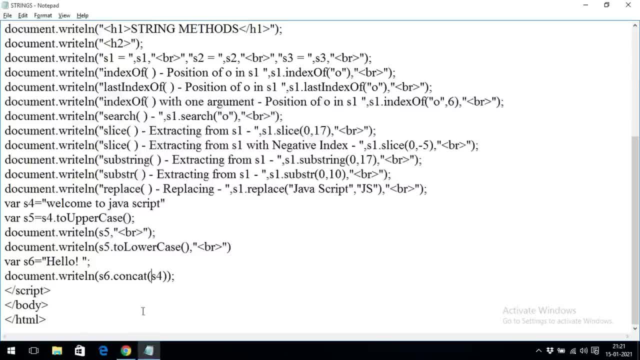 remove this one, So you will get the same thing: s6 dot concatenate s4. So that s6 dot concatenate. whatever the string we are having in s6, it will be concatenated with the s4. So that is why we 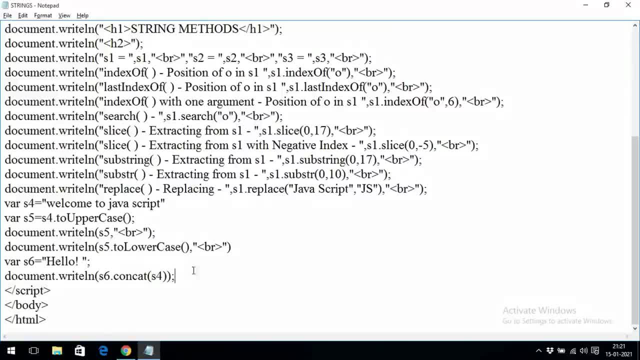 are getting some hello. welcome to JavaScript, right? So hope you understood this one. And there is a one more function called trim. function trim, So see where s7 is equal to. I will give three spaces and I will give some JavaScript. okay, Again, three spaces and close. 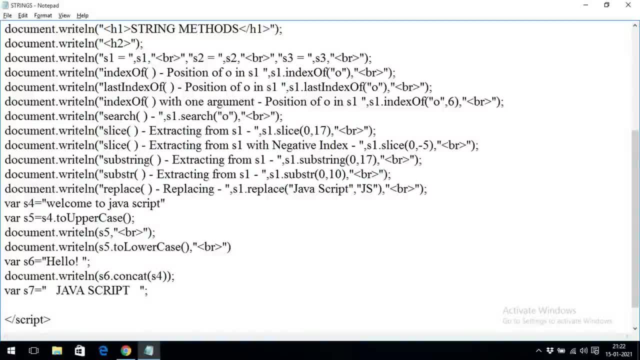 Now. so you can observe here the length of the thing, the length in order to find the length of any string. we are having the length property, So directly we can go with the length property right. Here you can go with the s7 dot length Directly, we will get the property right. 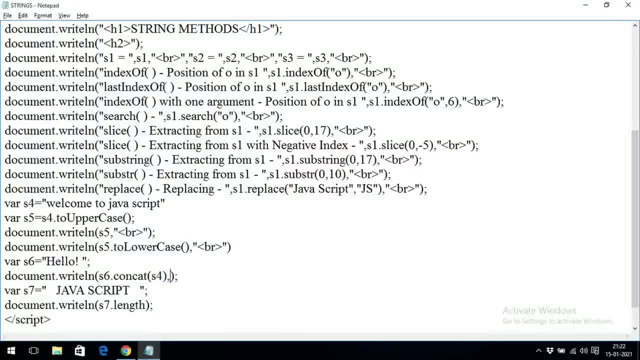 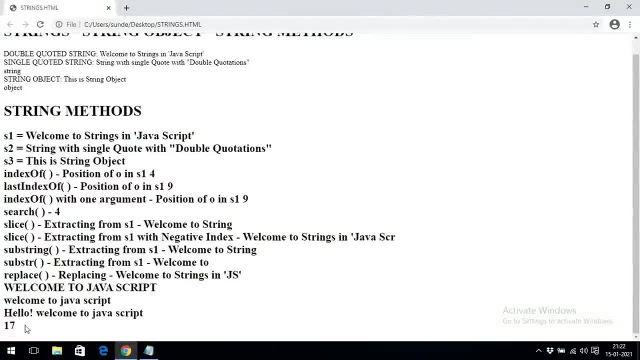 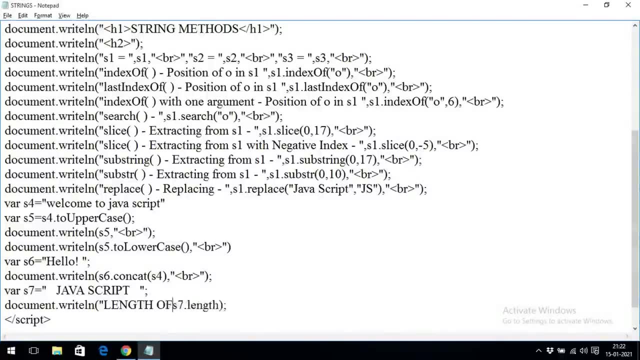 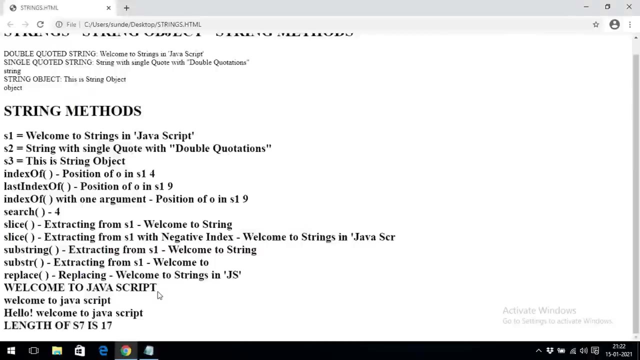 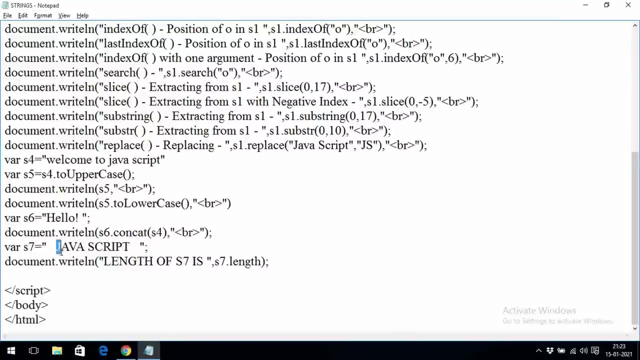 Here we need to give the break row so that you can get the length is 17,. okay, Here you can go with the data. length of s7 is yeah, length of s7 is 17.. Now that means we can observe here: So 4,, 5,, 6,, 7,, 8,, 9,, 10,, 11,. 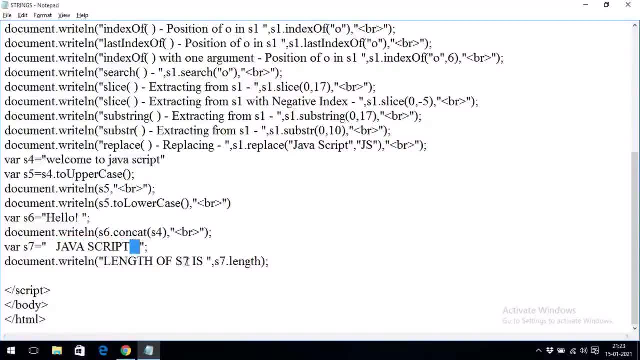 and here three spaces, and here three spaces, So 17.. So now I will use a function called trim. Okay, we use a function called trim. So where s8 is equal to s7, dot trim function, so that 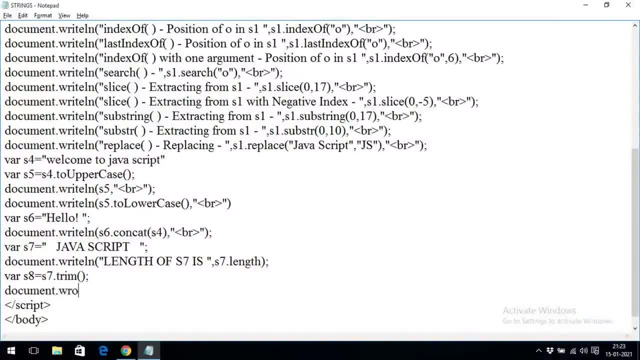 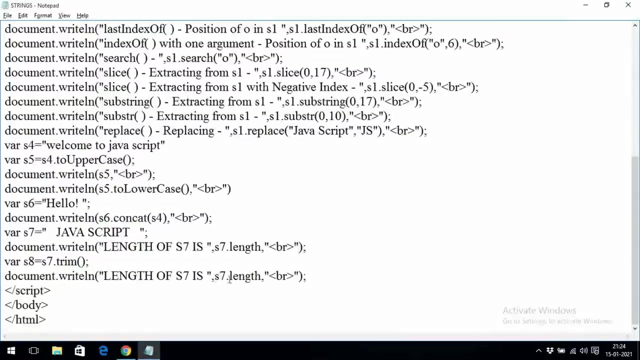 it will trim the value. So now we will check the writeln and I will. I will take the everything here. Yeah, I will go the same thing here also. Now we will check, You can observe. Yes, because we have. 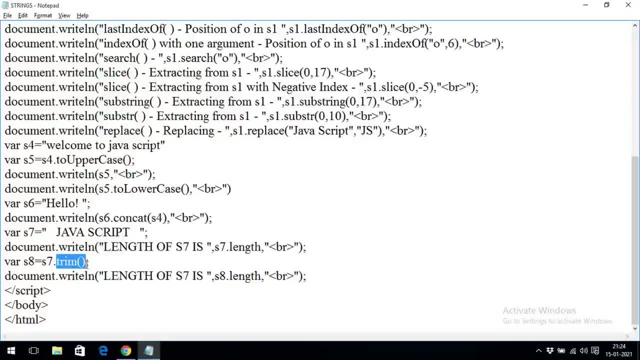 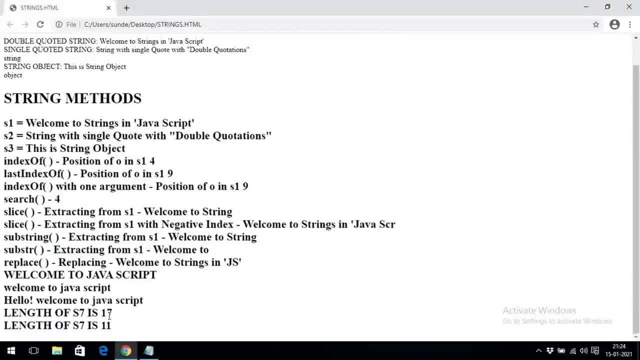 the trim function. so trim function will remove all the spaces. okay, leading and trailing spaces: it will remove all the leading and trailing spaces. you can observe, here we got a 7, S, 8. here it is not a 7, right, yes, 8 is 11 because it. 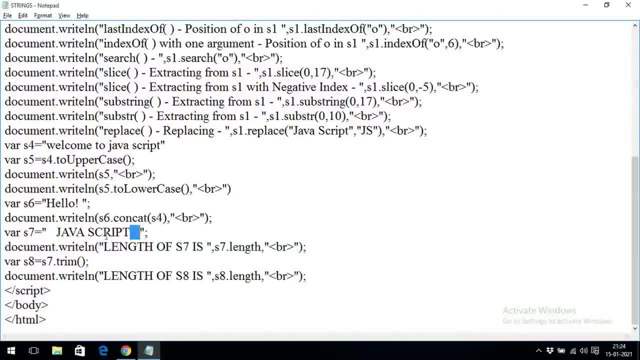 removes the spaces only leading and trailing, but not in between the string. okay, so we are having some three spaces- leading spaces 3 and trailing spaces 3, 6- and in between the string we are having one space- total 7. but this trim function only removes the leading and trailing spaces, okay, so that's why we 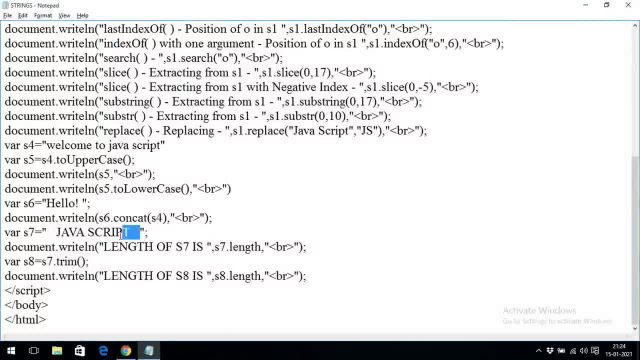 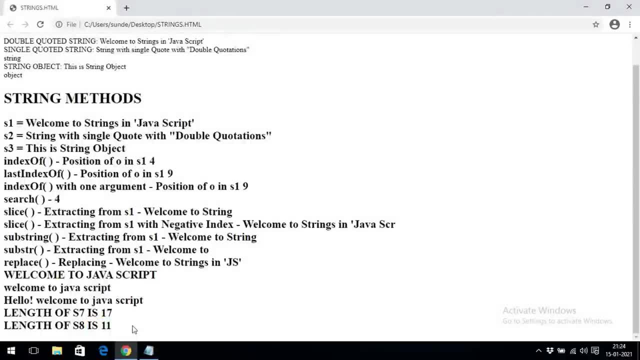 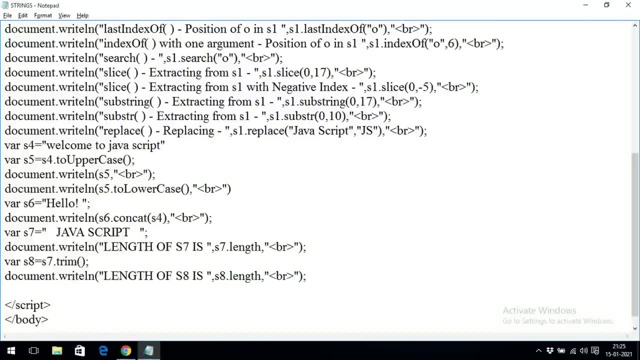 got 11. that means it removes the leading 3 spaces and trailing 3 spaces. total 6 spaces has been removed so that we will get the result as 11 right. so hope you understood this one. it removes the leading and trailing spaces. now there are two more functions. 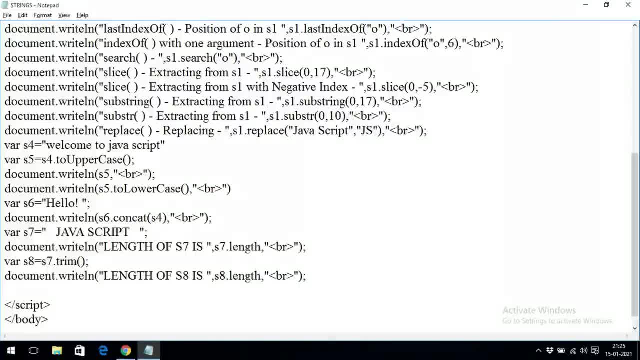 there is a care at car at function. care at function means here we need to give the position so that it will give the character at that particular position. so we'll go with the right document dot, right LN. so here care. okay, now we'll go with the S 1 or S 8 dot. 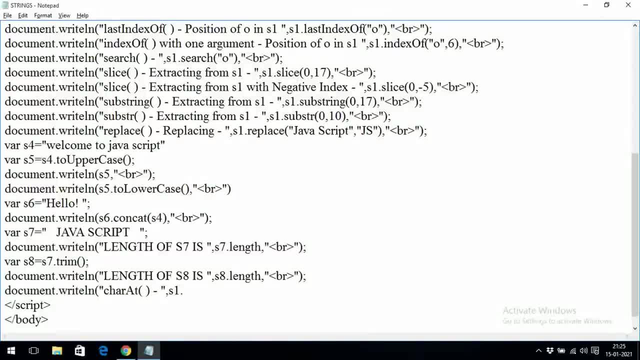 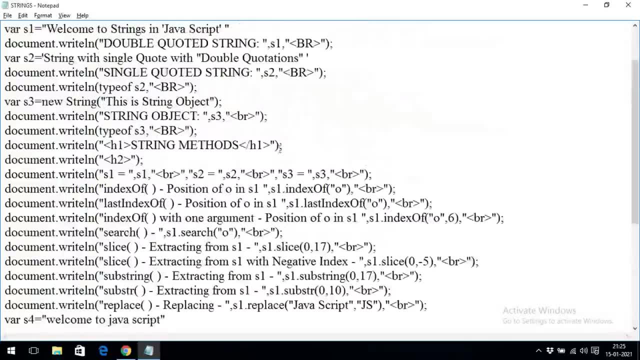 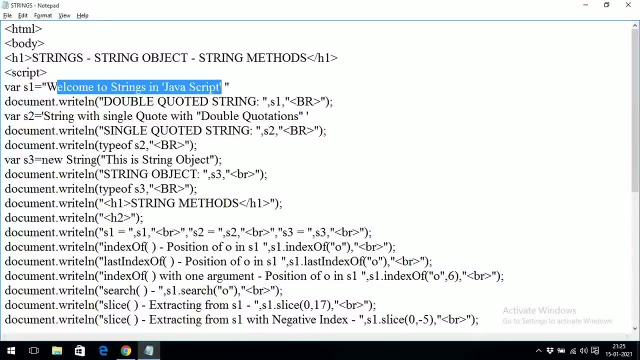 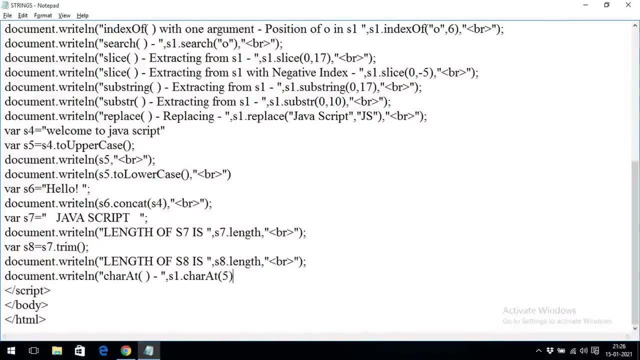 sorry, we will go with the s1 dot. okay, char, yet of what is a s1 data? so welcome to strings in JavaScript. so we'll go with the O. okay, some four, four or five, okay, we'll give anything, no problem. see, care at five is young, you can observe. 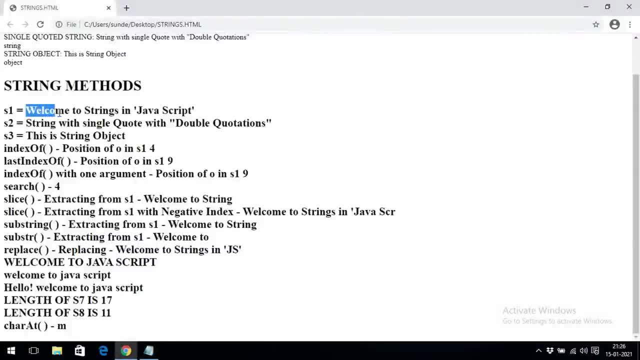 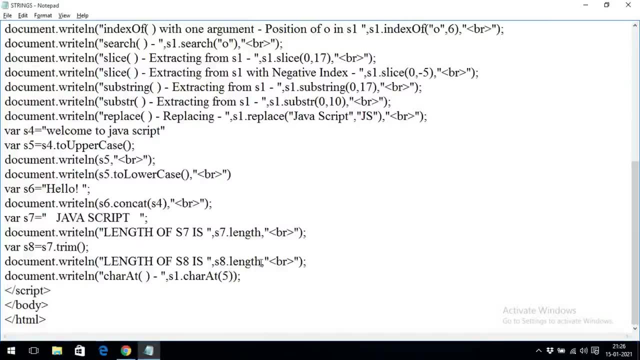 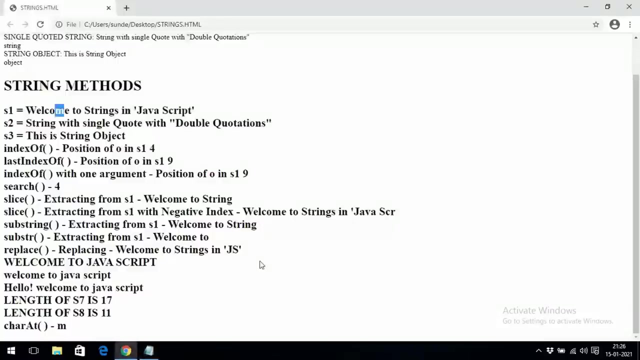 here: zero, one, two, three, four and five, the position five, position five: the characters here. now we can also know that length of this one. so we will check the length. okay, we will check the length and we'll give the position beyond that length. okay, so, document dot write a length, yes, one dot length. what's s1 dot length 36. now 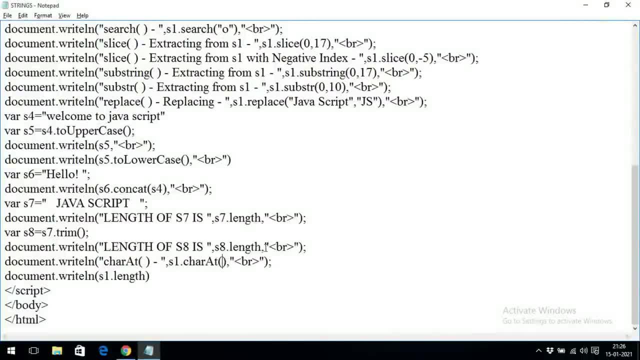 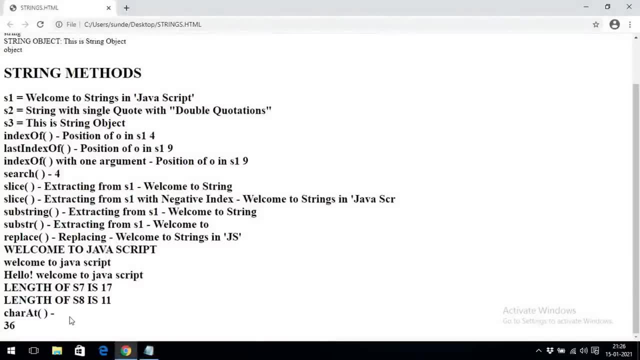 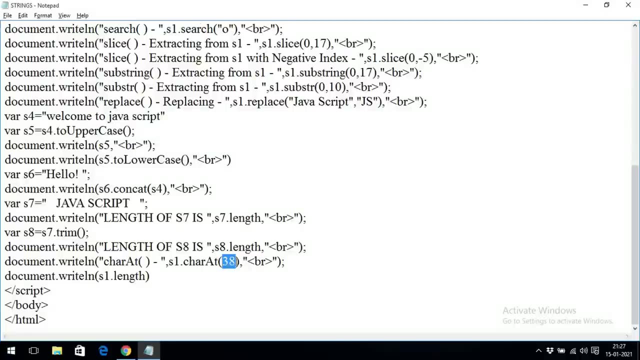 you give the value 38, what's the result here? another empty, okay, it will not return anything. it doesn't return anything if the position goes beyond with the length right. so if you go with a length 3, we'll get the result as the third character seat right now. there is a one more function called 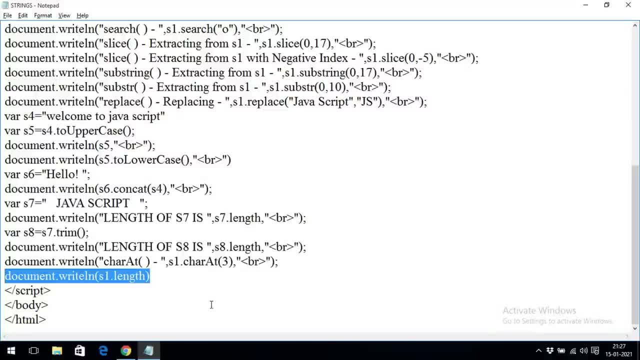 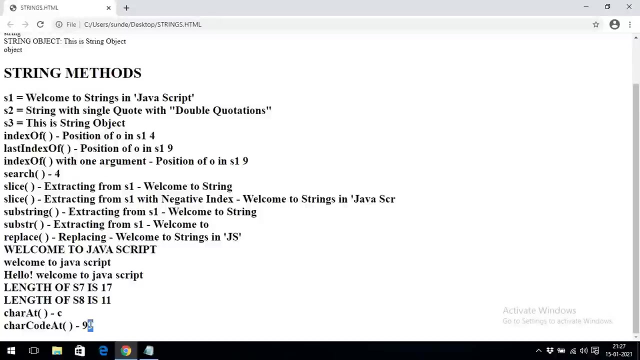 care, Char Kodak chair coded. so these things will be saved in a different format, that is, a Unicorn format. so normally we know all about ASCII format, but here it will store in a unique code, so it will give the Unicode value of that particular position, right? So I will take the same thing and we will check the unicode of this one. Okay, Car code 8.. C and A capital: Okay, Car code 8 of this one. So you can get the car code of C is 99.. Okay, Car code 8 of C is 99. 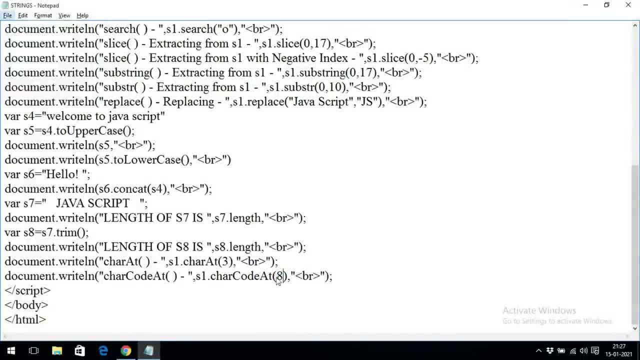 And if you go with some 8, you can get the car code of position 8.. What's the value at position 8?? You can check Position 8, T is T, So T value will be 1163.. This is the unicode value. Okay, This is the unicode value. 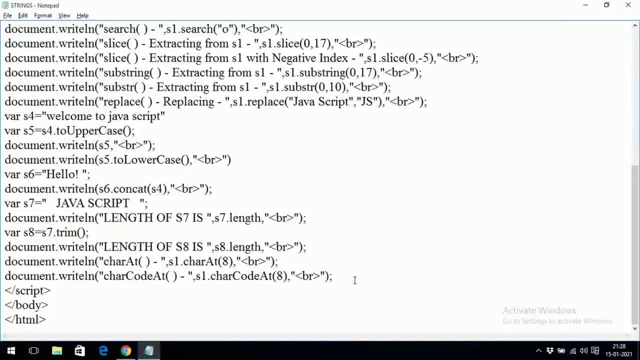 And now there is a one more thing. So how can we access the characters of a string So directly? we can go with the index value, So we can use a subscript and index So that we can access the characters Right. So I will show you that. For we will use a one loop. I is equal to 0.. I less than some S1 dot length, or we can go with the S8.. Okay, S8 dot length, I plus plus, and go here. 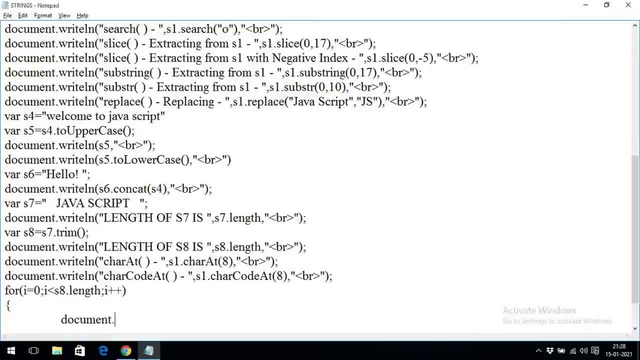 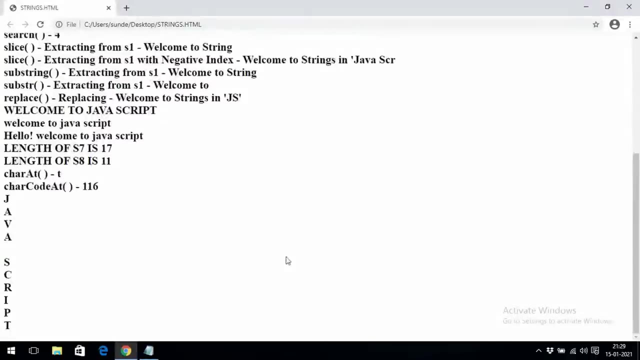 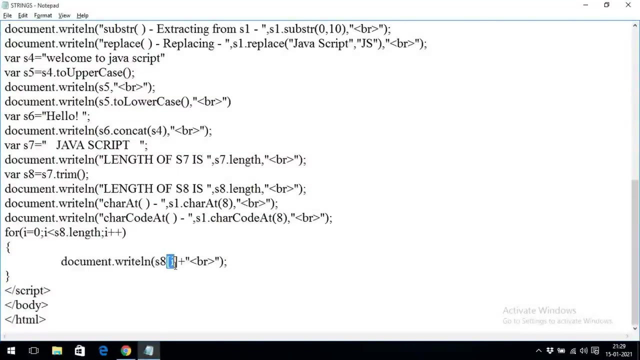 So document dot, writeLn And take S8 of I Give the index value in the subscript. Okay, Plus. So each line, We will go with each line. Okay, So it will print each character in a single line. You can observe here JavaScript. Okay, So this is how we can access each and every character, by using the subscript, followed by the index value. 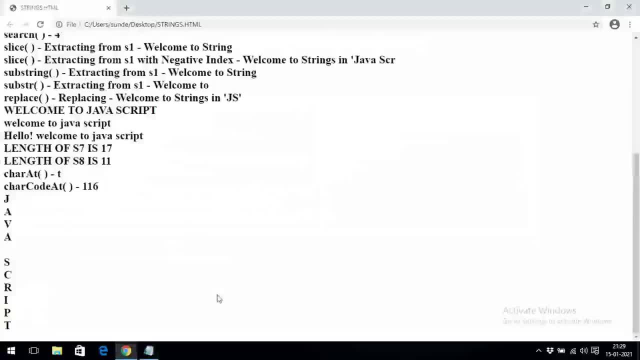 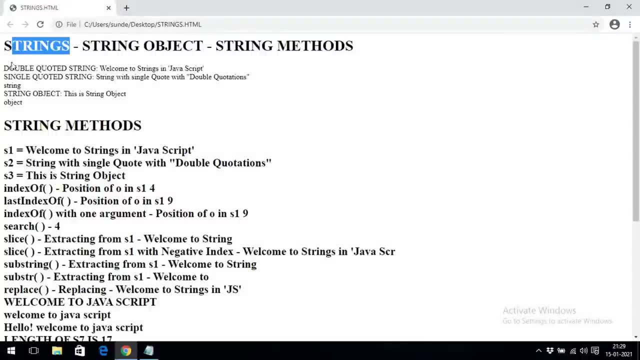 Subscript followed by the index value, Right. So hope you understood this one. The string. So what are the strings and how can we use this? double quotations and single quotations, and then how to create a string object and then different types of string methods. 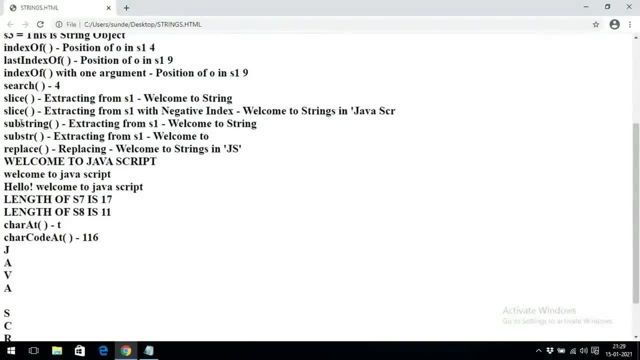 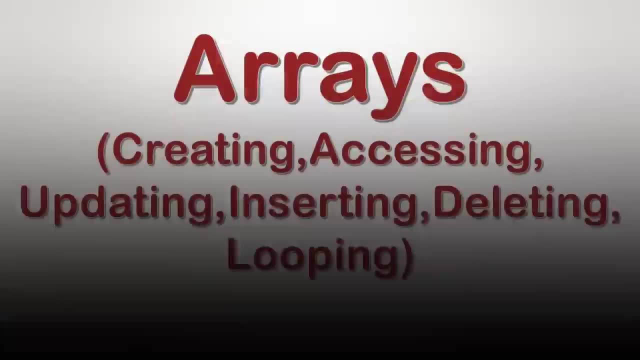 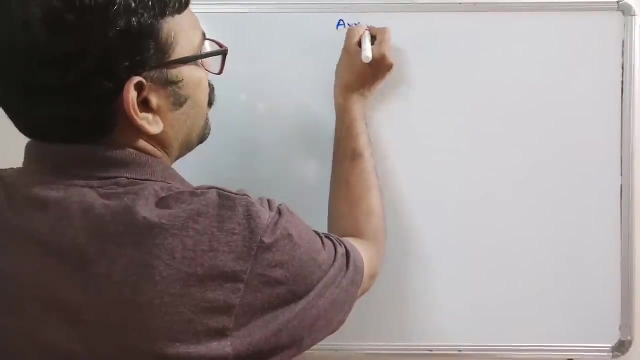 So index of last index and search slice: substring. substr replace two uppercase, two lowercase and the concatenation length property caret carecoded. And how can we access the characters of a string? So till now we have seen as normal variable which can hold only one value. 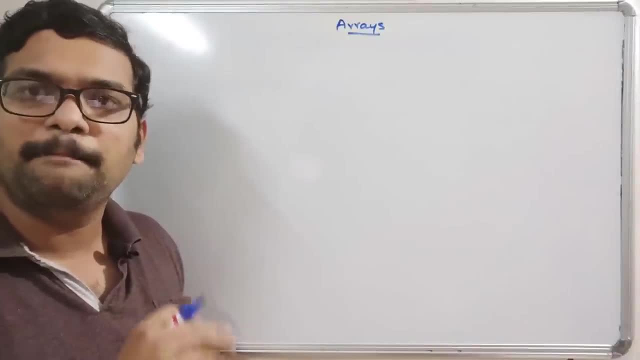 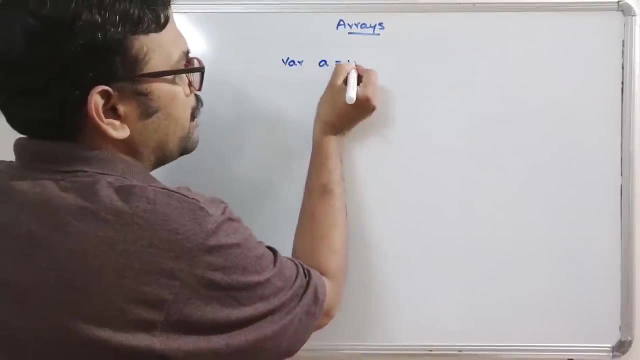 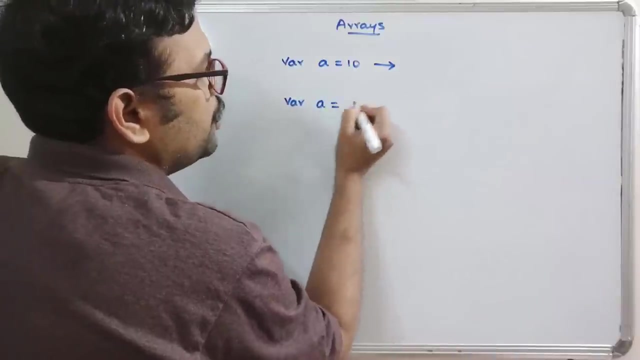 But arrays is another type that can hold multiple values under same name, For example if var a is equal to 10.. So this is a normal variable Which can hold only one value, and if var some a is equal to square braces, comma separated values. 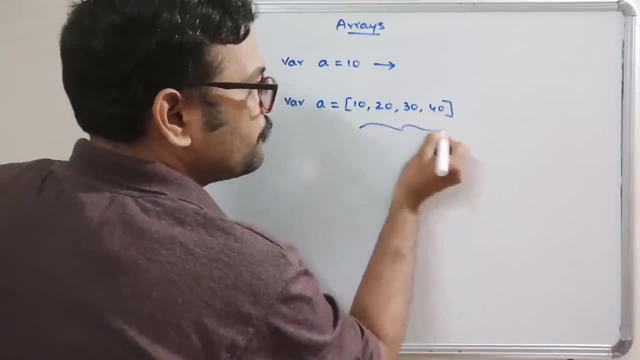 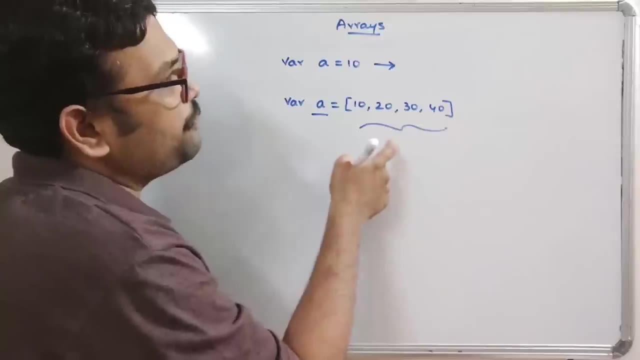 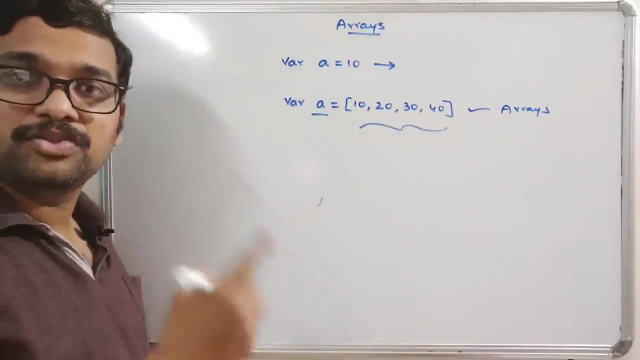 So this gives an array That means all these four elements will be stored under the same name, under the same name. So this type of thing we call it as arrays, Right, So these arrays can have not only the same data type, but it can also hold a multiple data types. 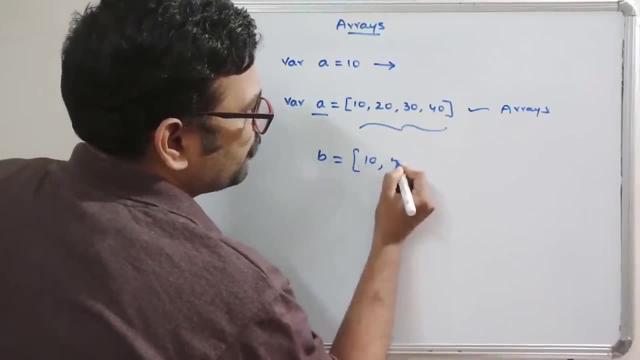 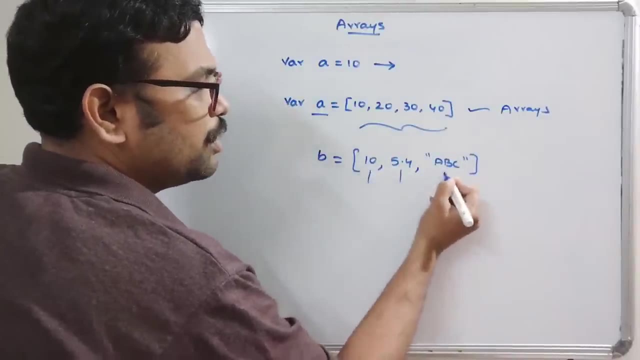 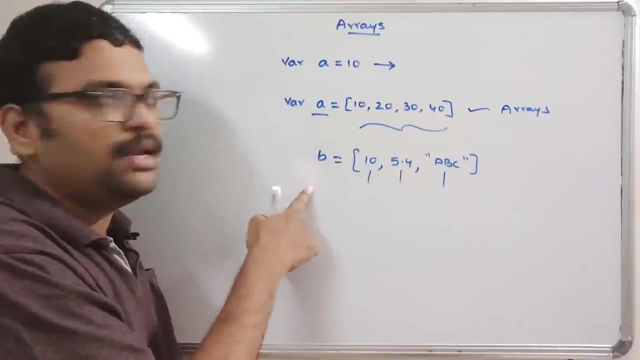 For example, b is equal to sum 10, 5.4 abc. So that means here we are having integer float string, So we can save all the different data types under the same name, Right? So this is called arrays. 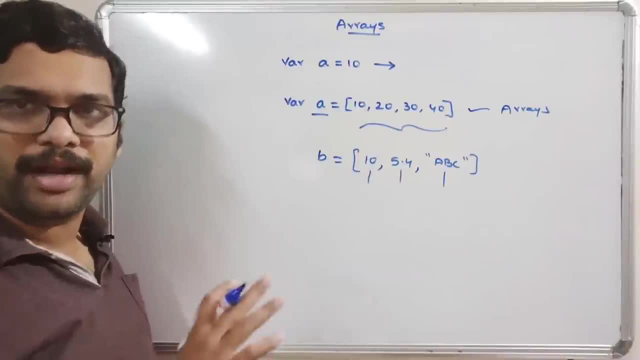 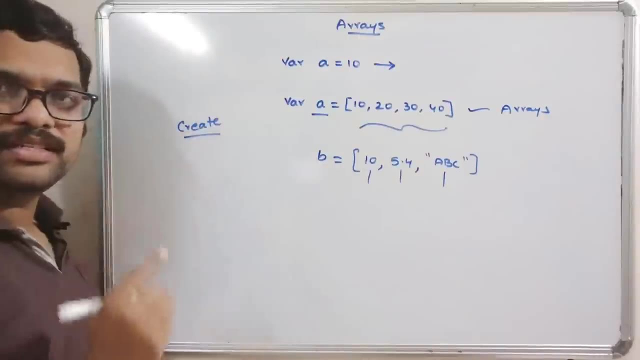 That means a variable which can hold a multiple values is called an array. So how to create an array, How to create? So an array can be created in two ways. One is with the help of declaration, at the time of declaration itself. 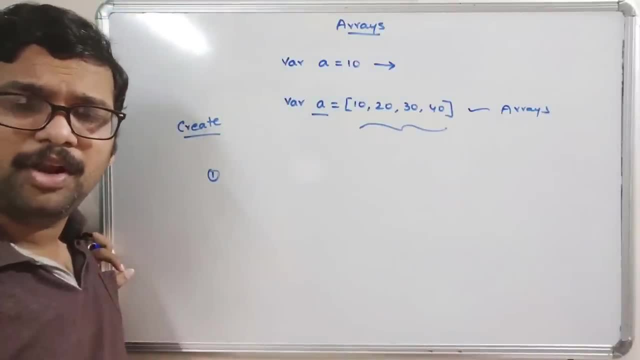 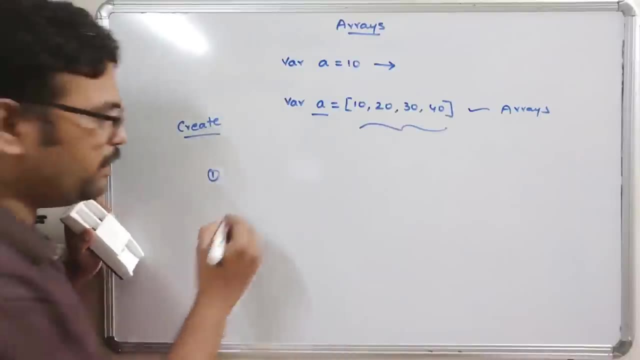 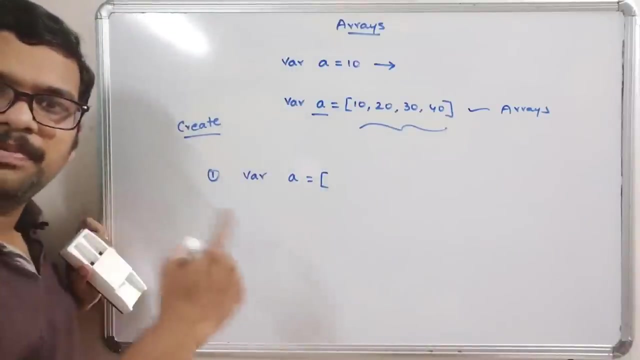 So any variable. So it may be a array variable or a normal variable that should be declared with the help of var keyword. So the first way to create an array is var some a is equal. to open the square braces and do the multiple elements comma separated elements in the square braces. 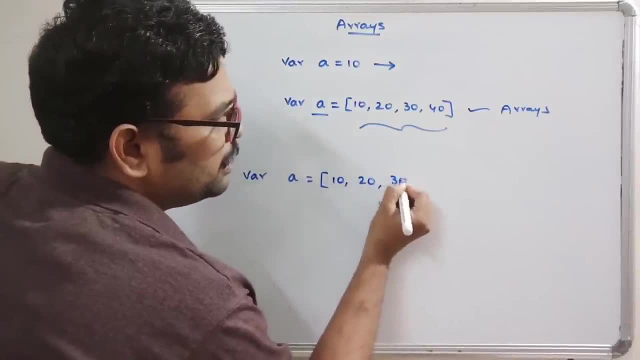 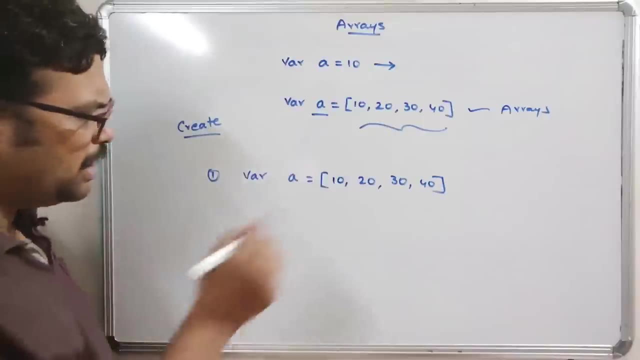 Right, So 10, some 20, some 30. And some 40. So total of four elements are available in array en. So this is one way to create an array. Otherwise you can also go with an empty array. 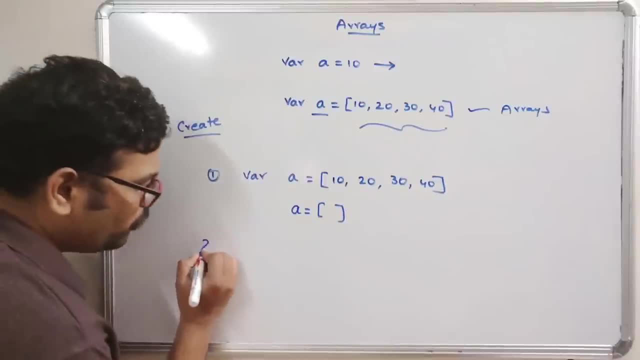 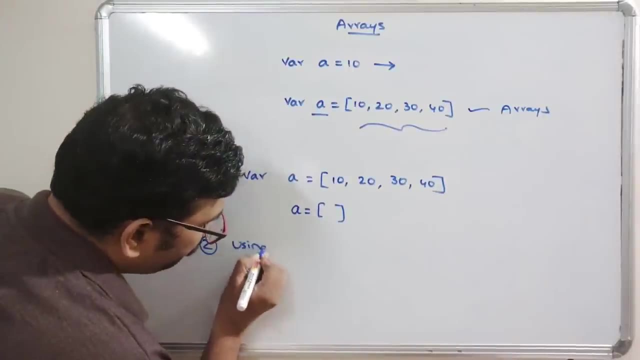 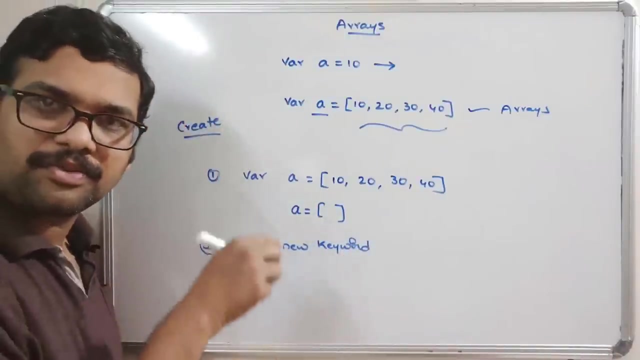 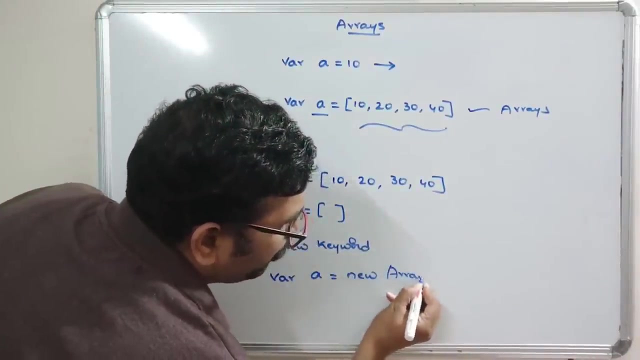 So this will create an empty array. Okay, And the second way to create an empty array is so using a new keyword. So using new keyword, So similar, which we have discussed in the numbers concept. So where, So where a is equal to new array of, here you can pass the elements. 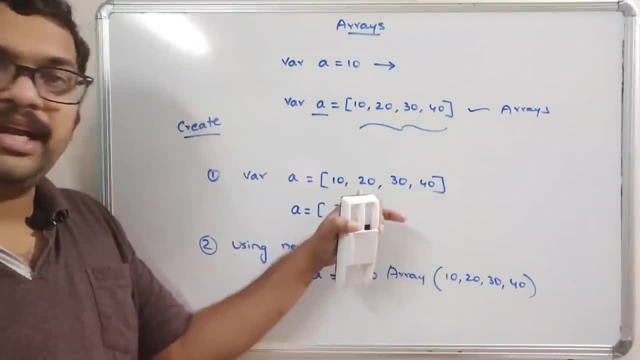 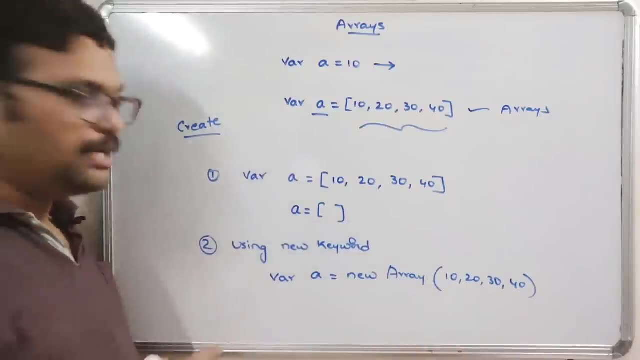 Right, So this is also an array. Okay, This is one way to create and this is another way to create. So, even though the data type of a is array, but in JavaScript the data type of a will be treated as an object. 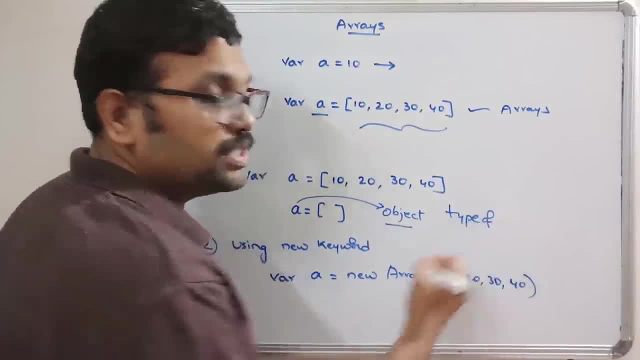 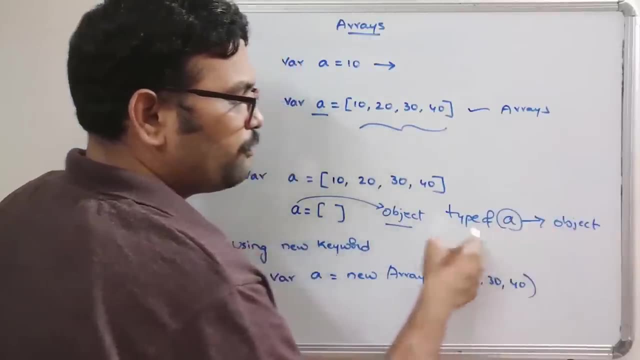 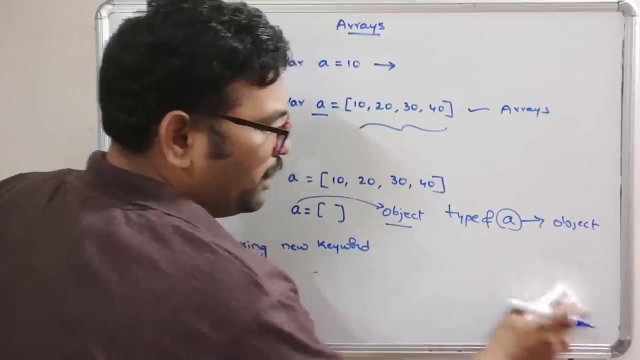 So if you go with the type of a- So we have already discussed about this type of Type of a- that will return as object. So even though the a is of array, it will return an object. Right Now, how to create an empty array. 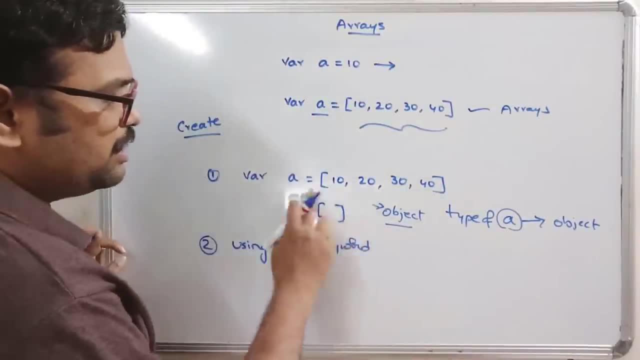 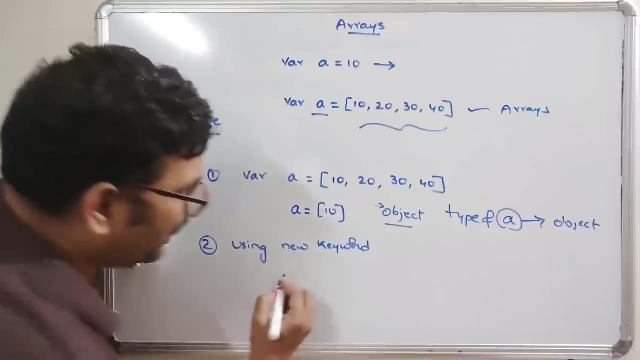 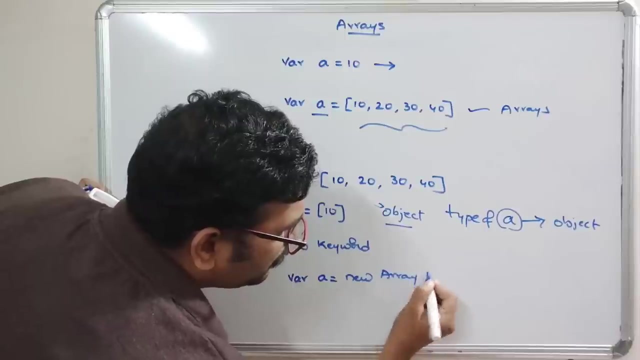 So single element. So if you consider the in the first case, if you go with, a is equal to 10, that implies array holds only one value, that is, a 10.. And coming to the second case, Where a is equal to new of array of 10.. 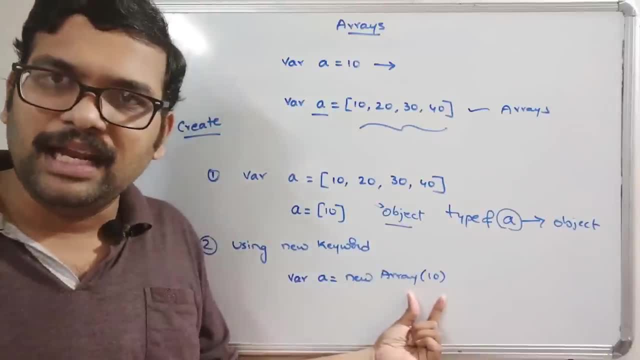 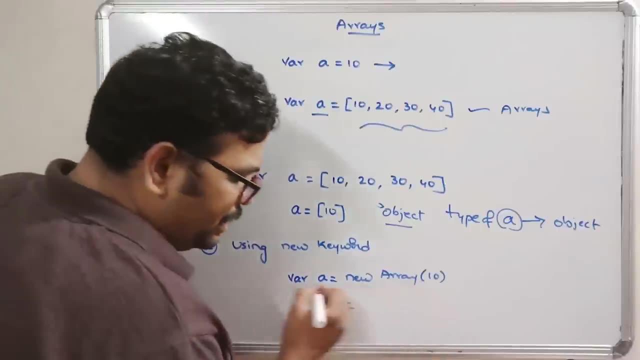 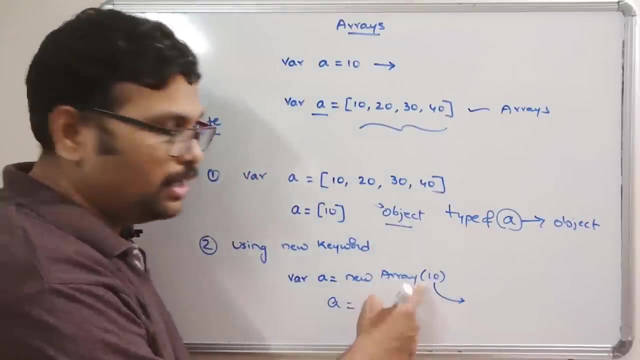 So this doesn't mean a single element, So it will create an empty array with 10 elements. So here, in this case, that means in the second case, if you give only one argument in the in the array function, that will treat as a length of the array. 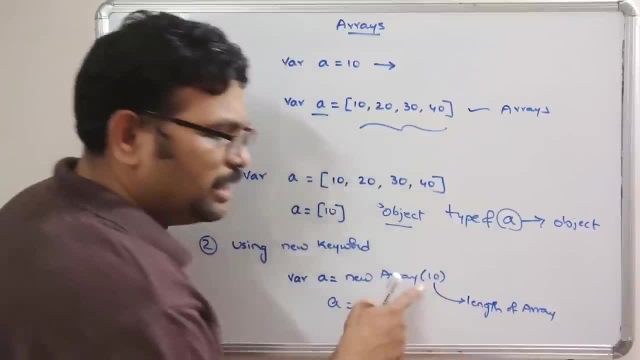 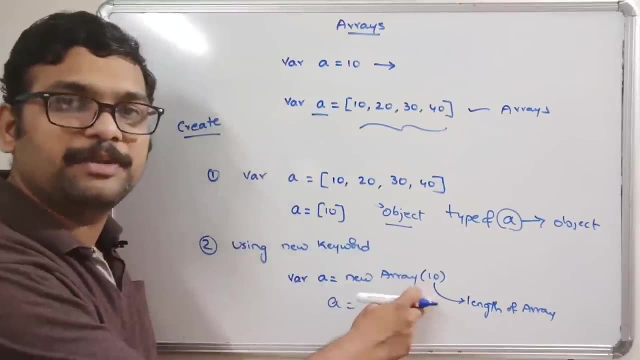 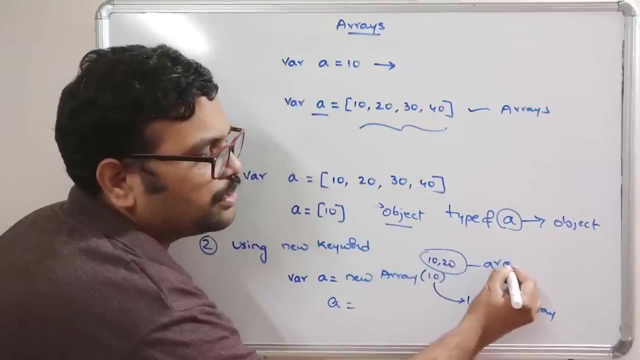 Length of array. So that means the JavaScript will consider it as a 10 elements. So maximum of 10 elements. The size of the array: It will specify the size of the array. If you go with a 10 comma- 20, then it will be considered as an array with two elements. 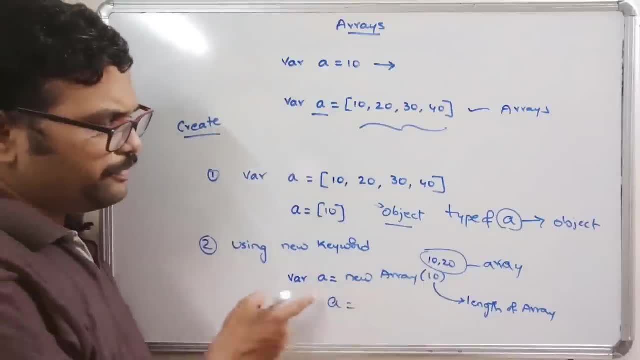 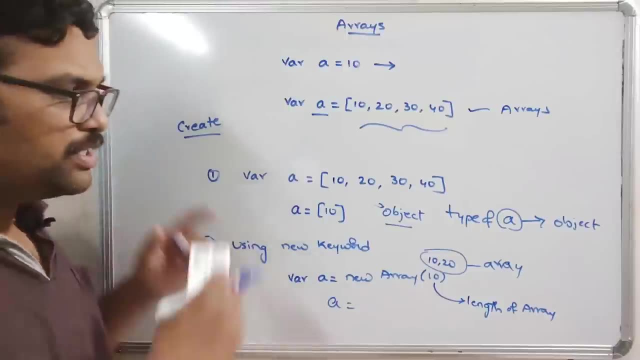 Array with two elements, Right? So that is the difference between the first way and the second way. So I will show you by executing a code in the system. Okay, So once I will, This syntax has been completed. Then we will move on to the system. 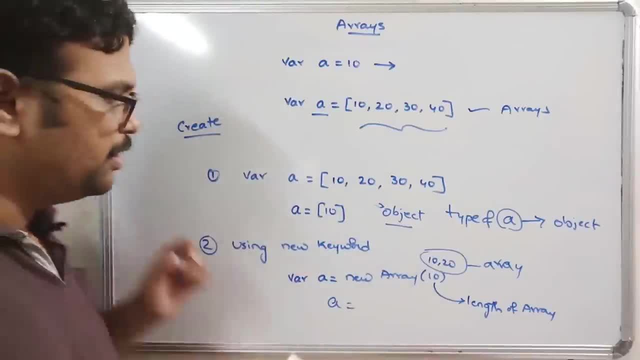 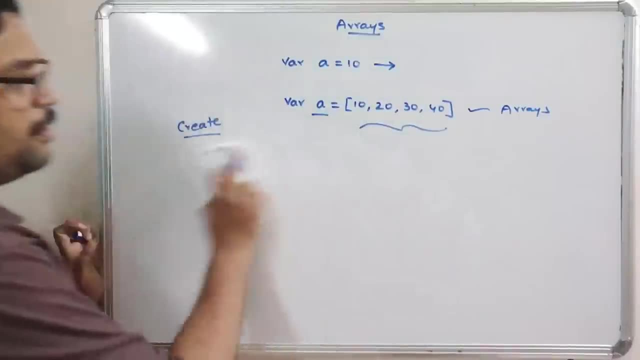 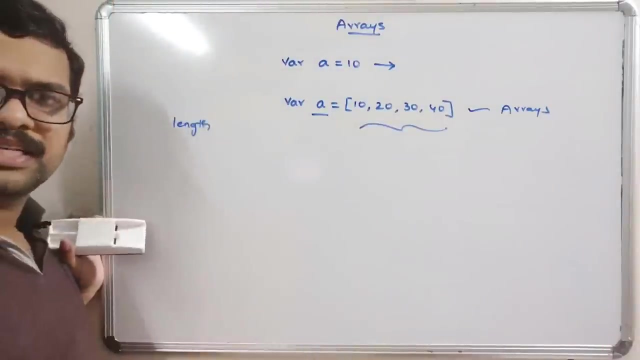 And I will show you the execution of all these things. Right, Yeah, So these are the two ways to create an array. Now there is a property called length property. This also we have already seen in the string function. So length property. 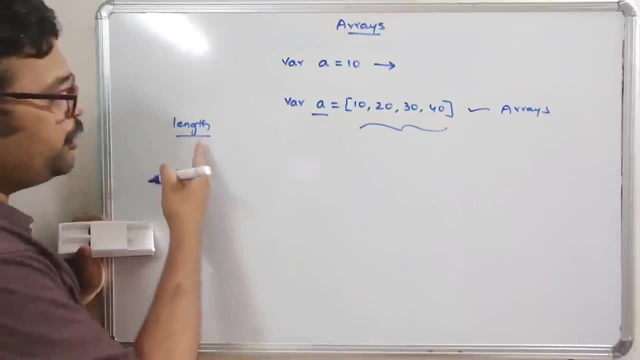 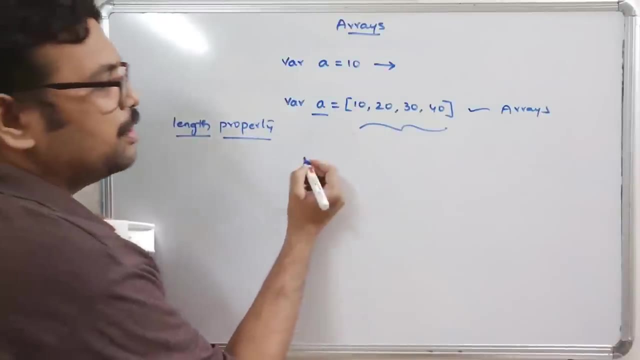 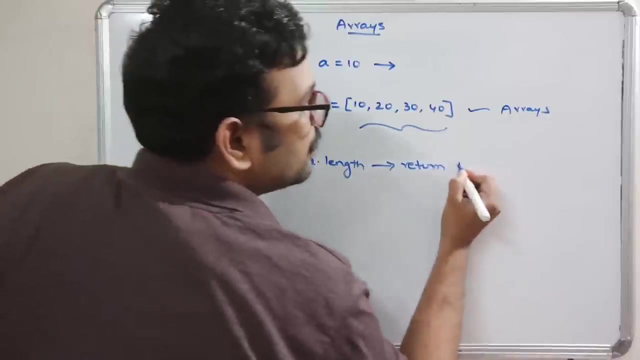 So, in order to know the size of the array, we need to go with this length property. Okay, Length property, Right. So, for example, if you consider this one, we have to go with the a dot length. Automatically it will return the size of the array. 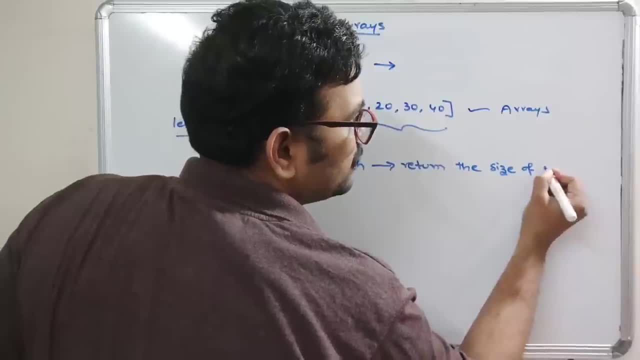 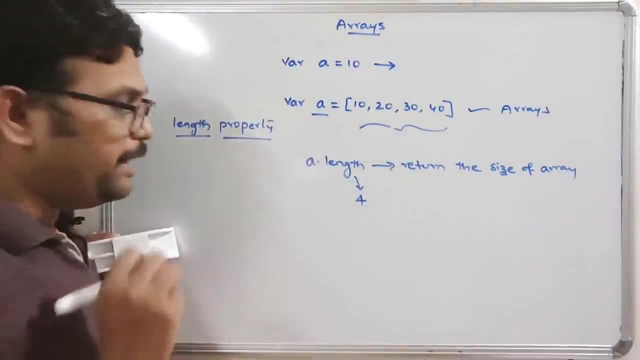 That means how many number of elements available in that array, Size of array. So in this case, it will return four. It will return four, And so this is a length property. Now the next question is how to access the elements. 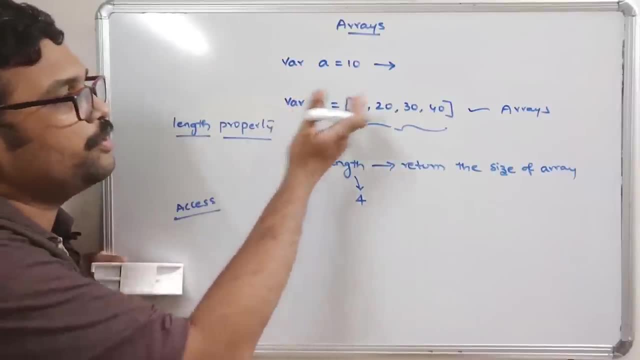 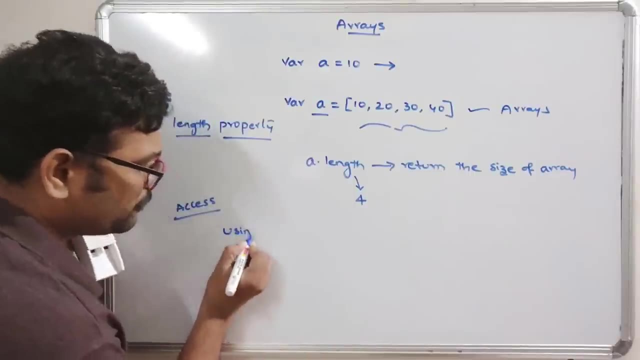 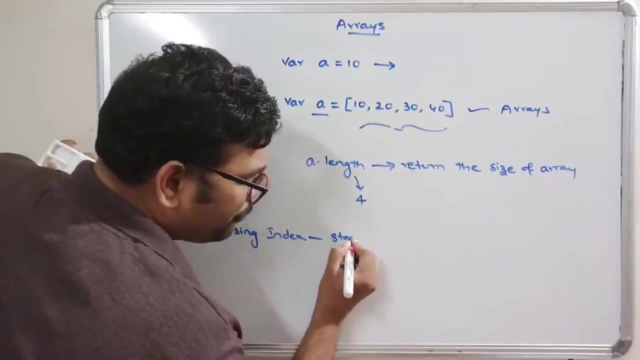 How can we access the elements? Because only one variable can hold a lot of elements, Right, So how to access the elements? And these elements can be accessed using index values. Using index values. Okay, So these index values always starts from zero. 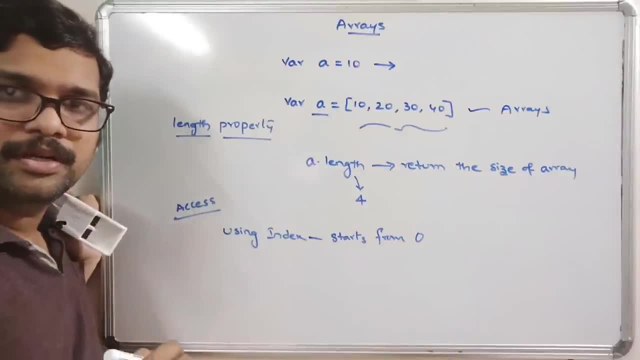 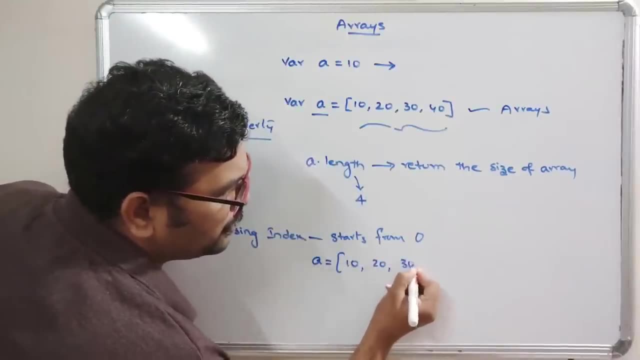 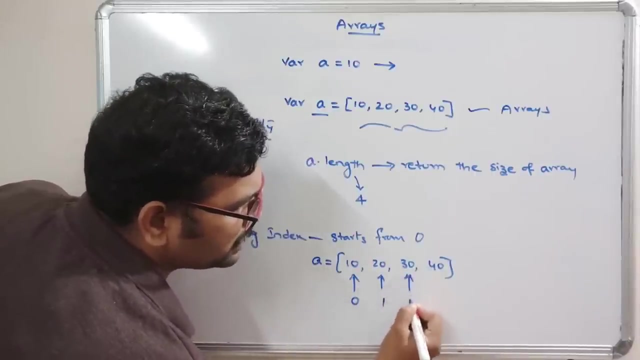 Zero onwards Always starts from zero onwards Right. So if you consider this one, 10,, 20,, 30 and 40. So this is the index value zero, This one index value one. This is the second index. 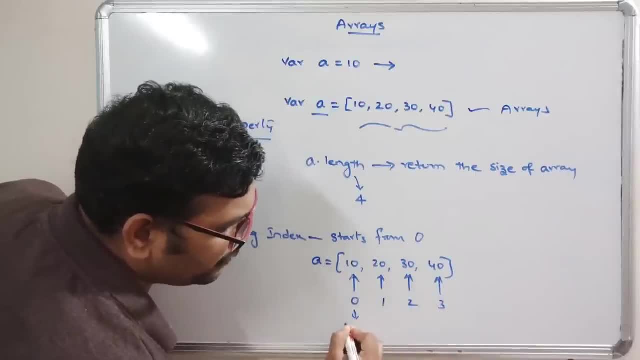 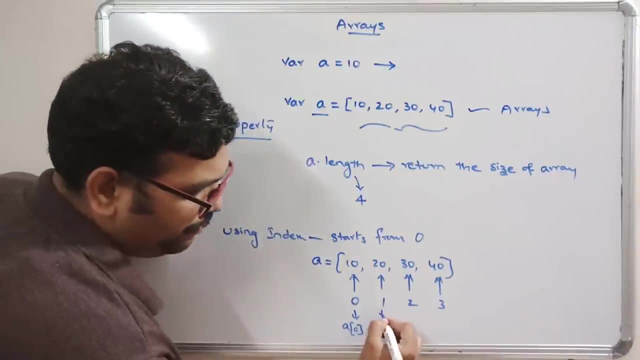 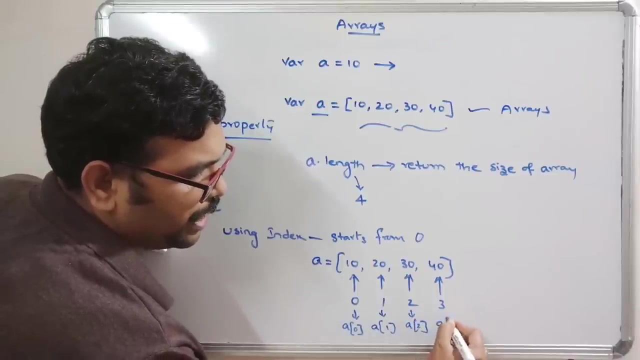 This is the third index, So this can be accessed with the help of array name, subscript, index number. Similarly, array name, subscript, index number. Similarly, array name, index, subscript, index number. Array name, subscript and index number. 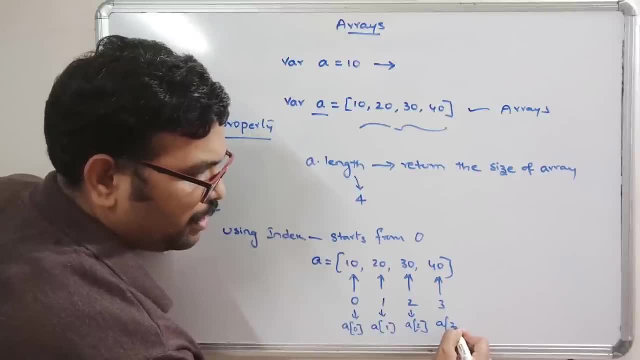 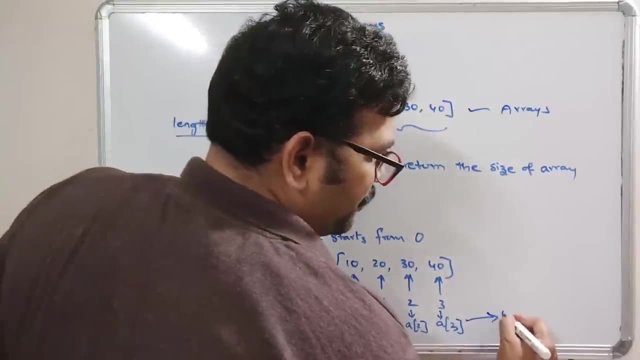 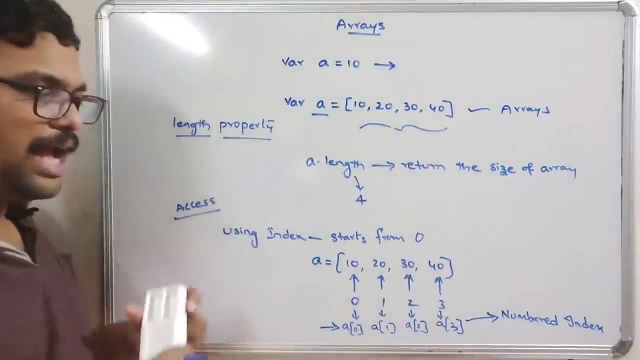 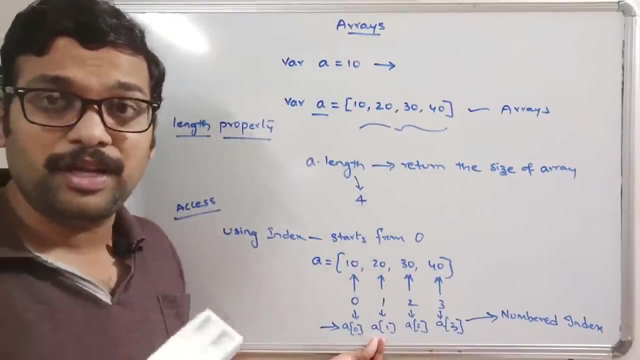 Okay, So this is how we can access the elements. So this is called numbered index, Numbered index So because as a number, I mean the index will be considered with the help of numbers, numeric values. So that's why this type of things we call it as a numbered index. 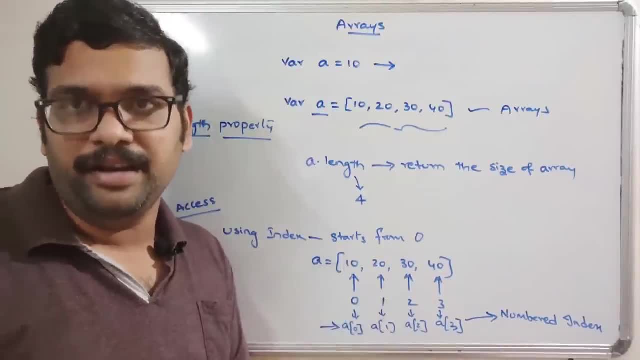 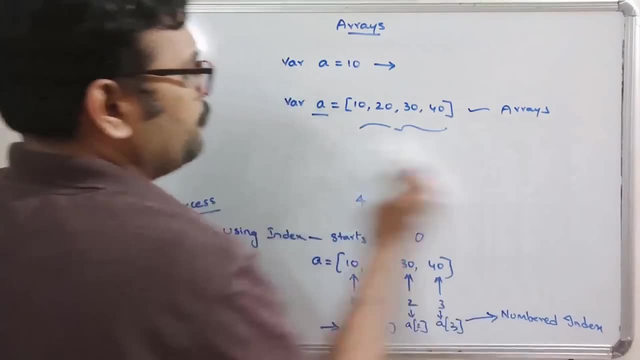 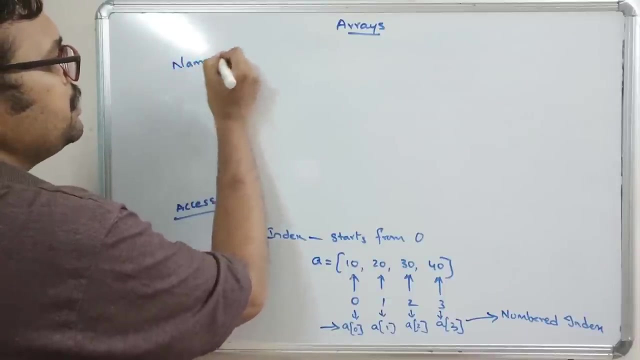 So we can also access the elements with the help ofiveness. Okay, named index. so that means, instead of using the numbers, we can also use names. so that is how we will see now, for that purpose, for that, named indexes. okay, named index. that means in order. 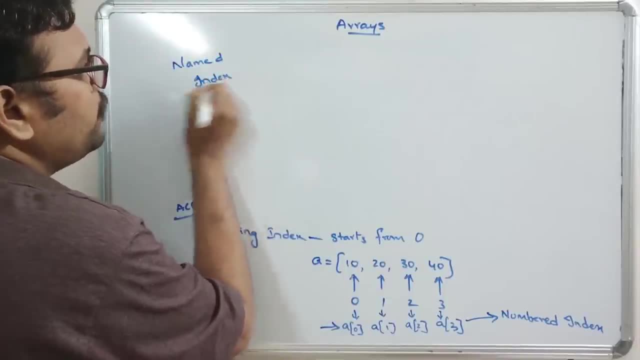 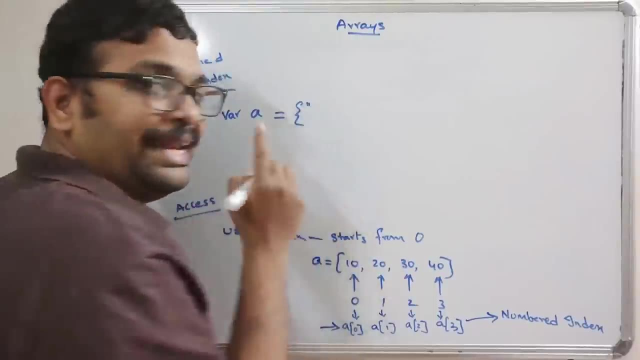 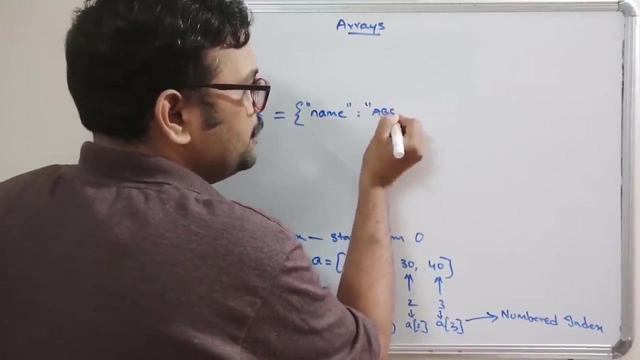 to access the elements by using the named index. we need to create an array in such a way that where a is equal to curly braces, so give the name for the element. okay, we can give the name for the element. colon. give the value here some a, b, c and second element. give the name for second element. 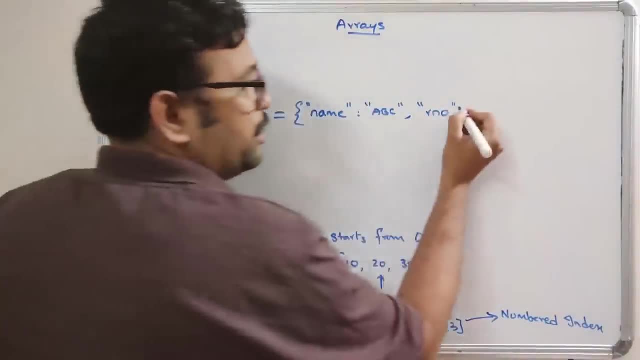 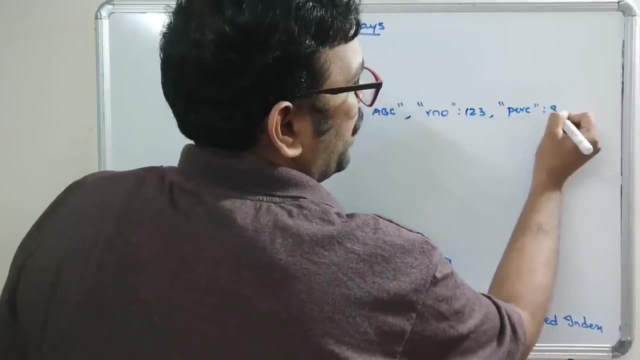 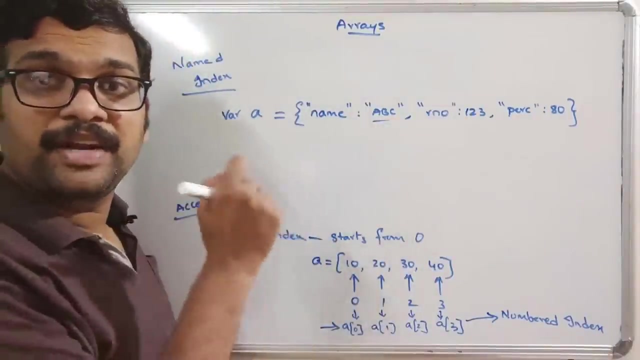 so if it is a string, you have to enclose in quotations, right? so some one, two, three give the third element some 80, right? so this is an array now how to access this element. so this element can be accessed with the help of named index. so a dot name, a dot name, it will give. 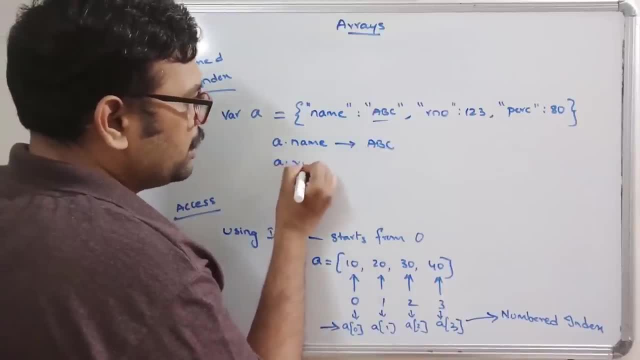 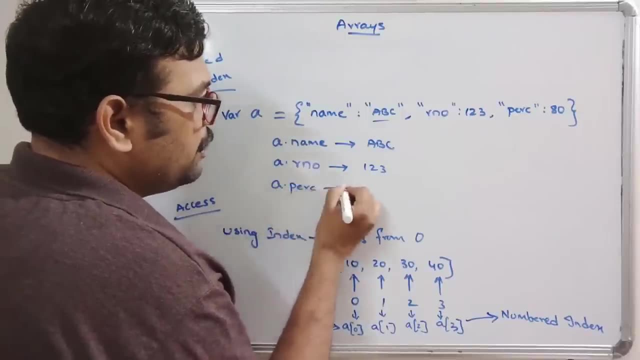 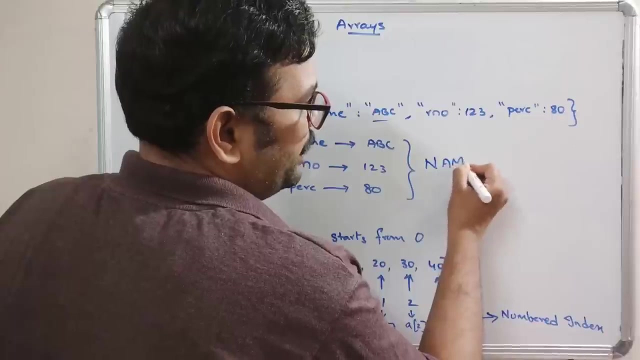 the result as a, b, c. similarly, a dot r number, that means roll number- it will give some 123. so similarly, a dot percentage: it will return 80. so these type of accessing the elements are called as named index, with the help of named index. so this is a numbered index and this is a named index. 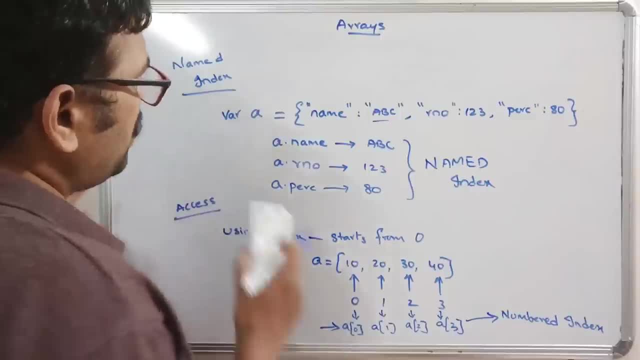 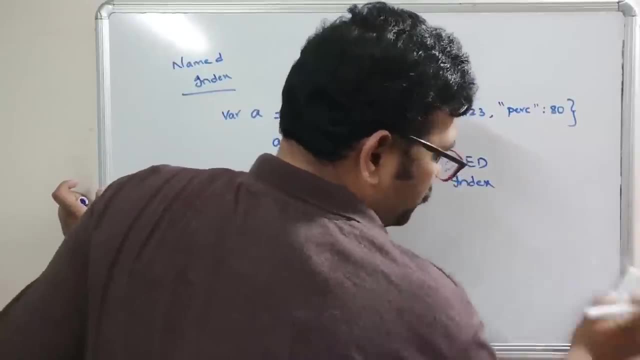 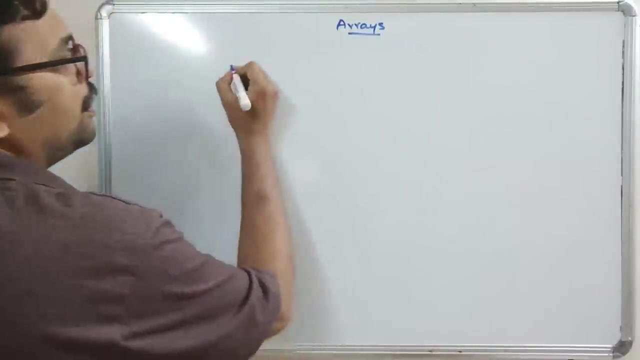 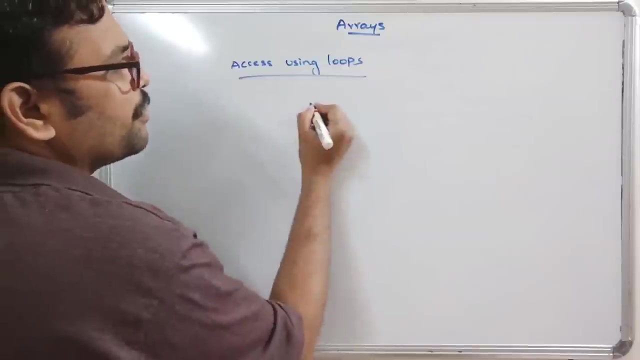 so i will show you by executing code. no problem, right? so this is how we can access the elements. now, how to access by using a loops. okay, access using a loops. using loops simply. for example, if you consider some variable, a is equal to some 10, 20, 30 and 40. 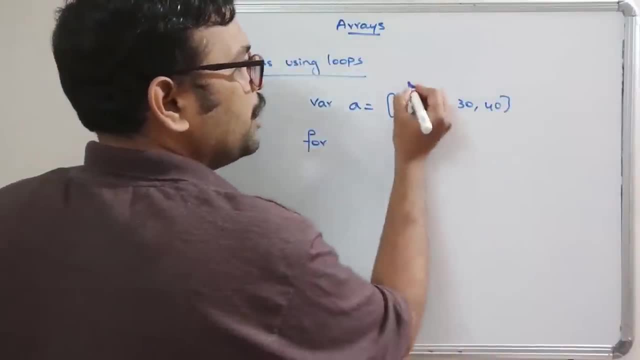 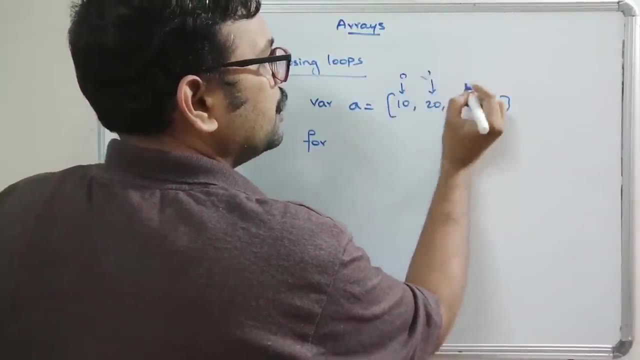 and go with the loop. for so here you can know, the index value is 10 and the index value is 10. value of 10: 0. the index value of 20: 1. the index value of 32. index value of 43. so far you know. 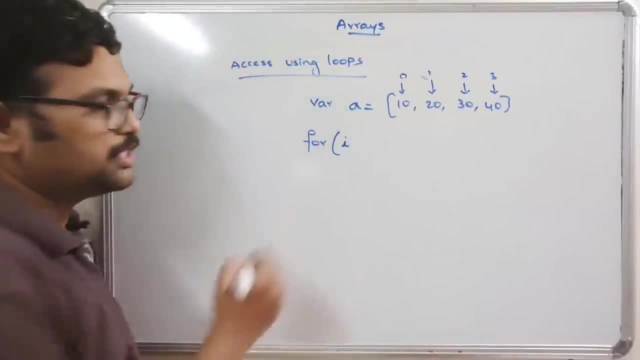 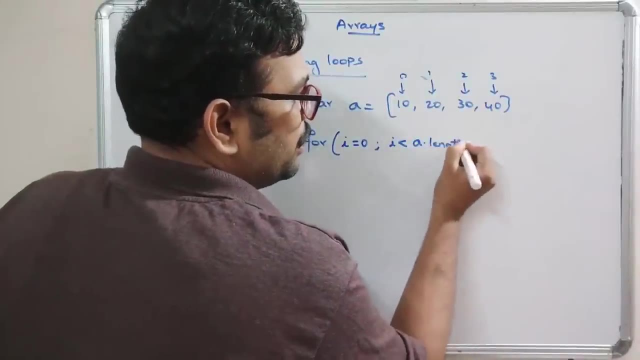 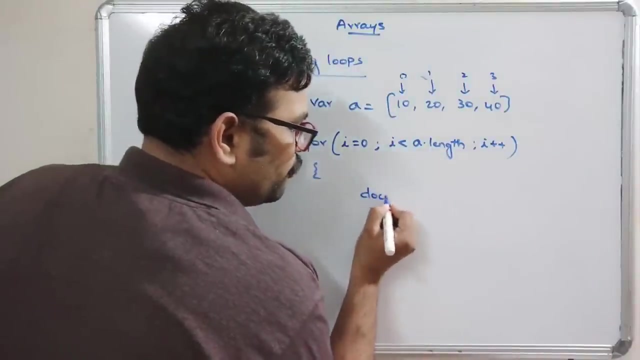 the syntax for the for loop. give the in loop variable initialization: i is equal to 0, i less than a dot length. okay, a dot length i plus plus. so immediately you can print here some. you know, we know the output statements. so document dot, write ln or windows dot alert or document dot. 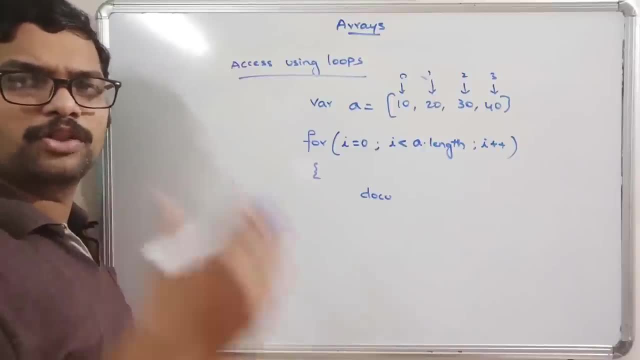 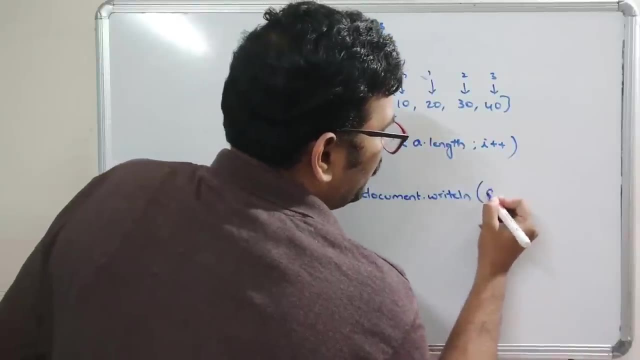 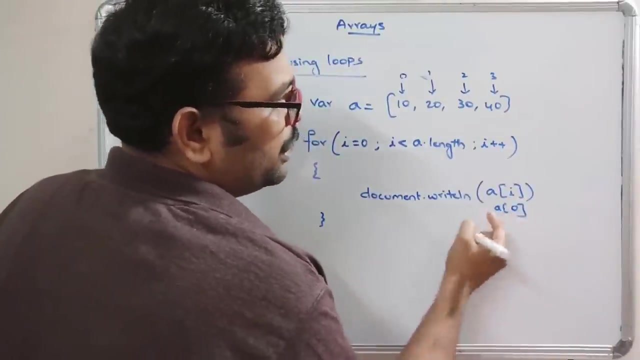 get element by id. so one, use one among all those threes. so just use the output statement. i will go with the write ln and print a of i, a of i. so for the first iteration i become zero. so it will be a of zero, i will be incremented and immediately i a of one, a of two and a of three. 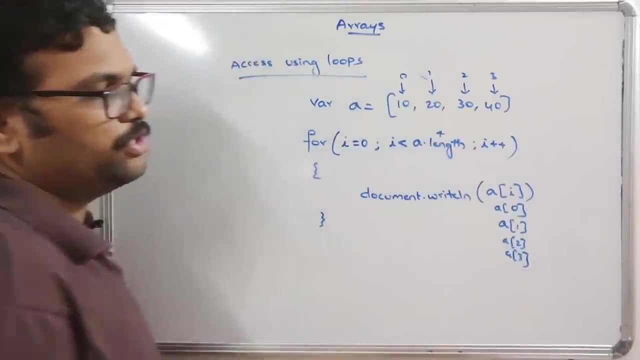 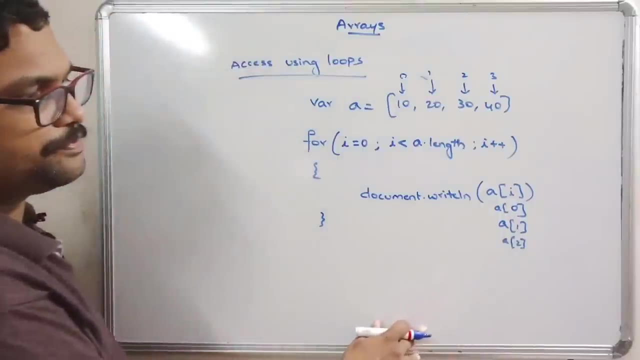 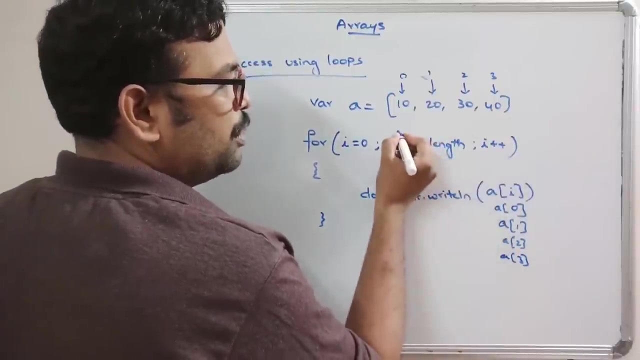 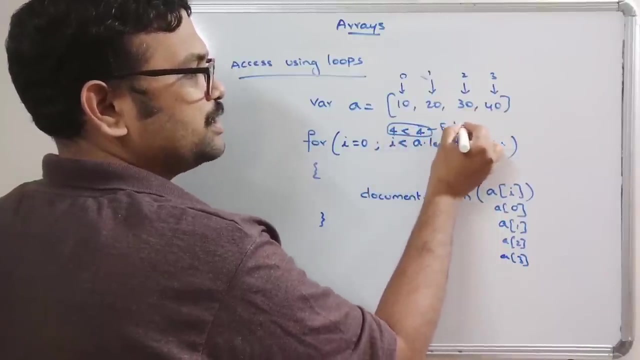 whenever i is incremented. now four, right, a value is a four. sorry, sorry, so here it will print everything. yeah, it will print everything. whenever i becomes three, three plus plus now i becomes four, so four less than a dot length, four. so four less than four is a false. four less than false is a. 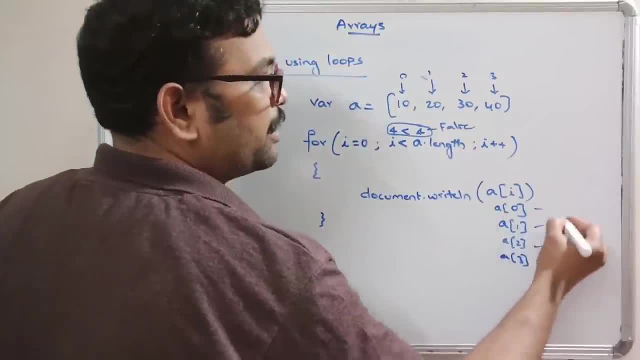 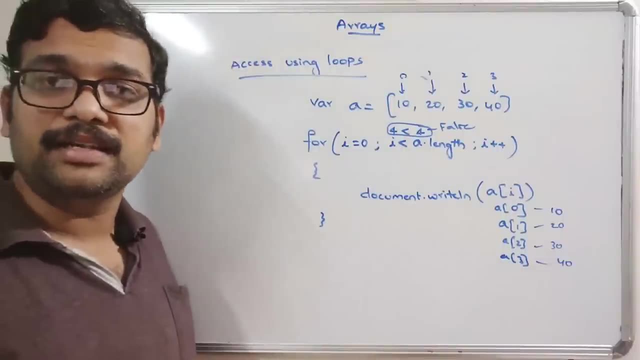 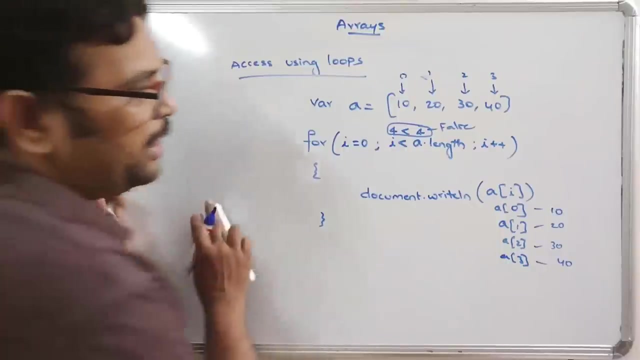 false, so automatically it will print these elements directly. so in the next iteration 20, next iteration 30, next iteration 40 will be printed. so this is how we can access the elements by using a looping statement. you can also use the file while loop also, okay. so this is how we can use, and then the next one is how to change the elements. how can we? 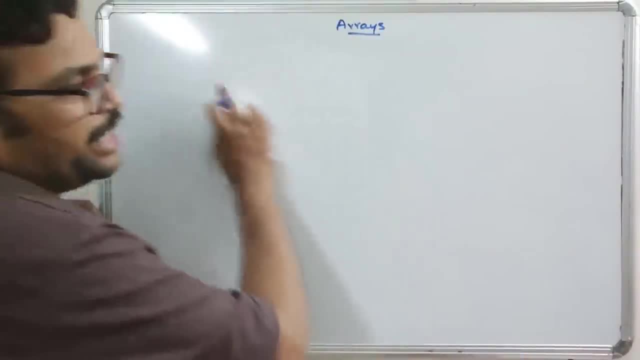 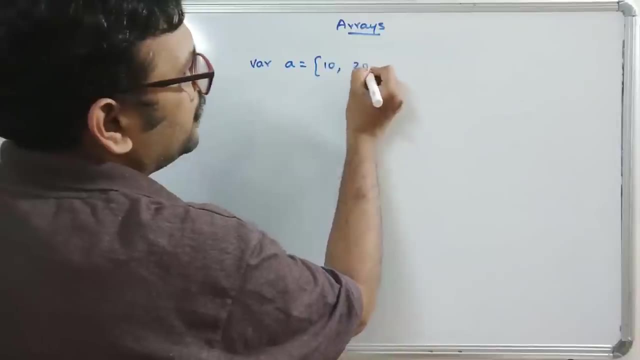 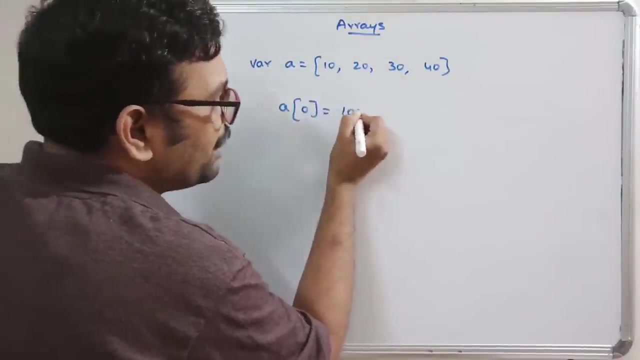 change the elements. so changing the elements means reassigning the values. for example, consider the array: a is equal to some 10, 20, 30 and a 40. so if you go with a j of zero is equal to some hundred, automatically, whatever the element. 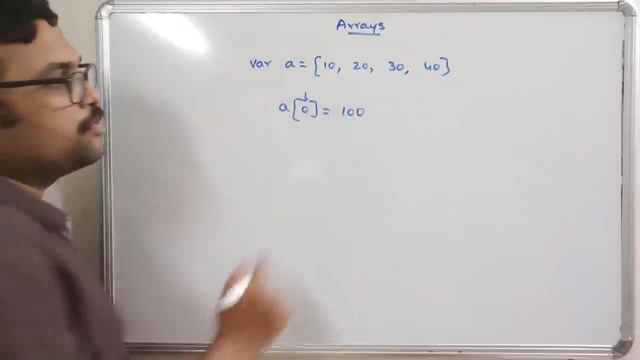 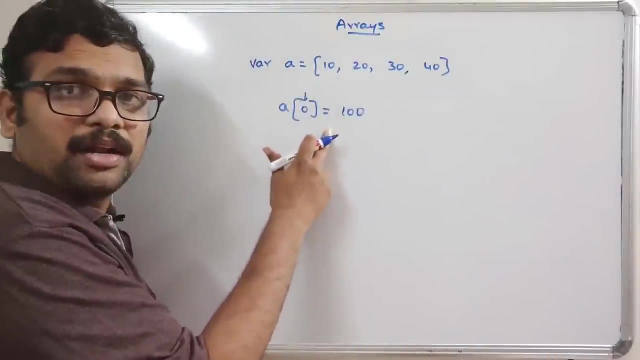 available in this index. that will be replaced with a hundred. so now you can observe. so a of zero means 10, right, a of zero means 10. so here we are using some assignment operator. so if you are using an assignment operator, whatever the computation is done on the right hand side, that will be computed. 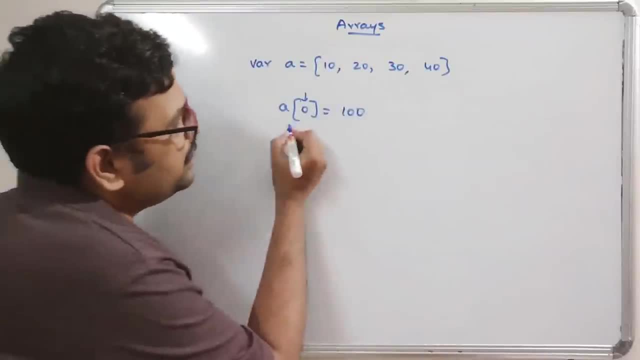 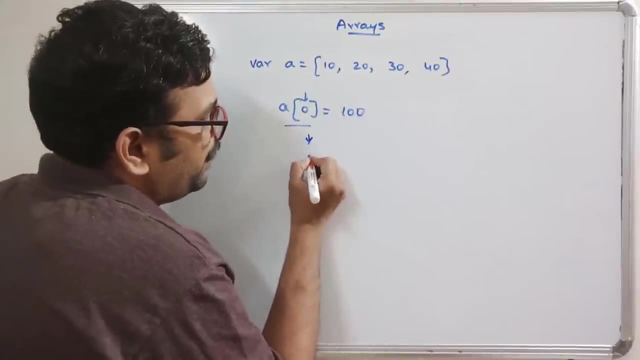 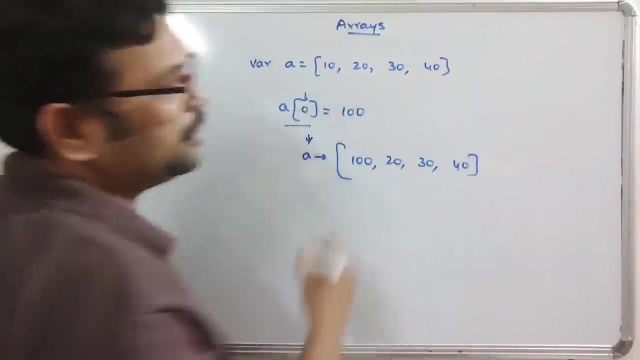 and the result will be stored on the left hand side. so left hand side is a of zero. so automatically in the place of zero the index 100 will be placed. so if you print a, automatically we will get some 120, 30 and a 40. this will be displayed, okay, and see if you go with a of. 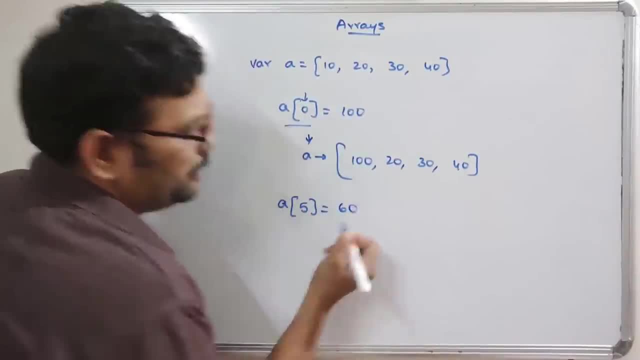 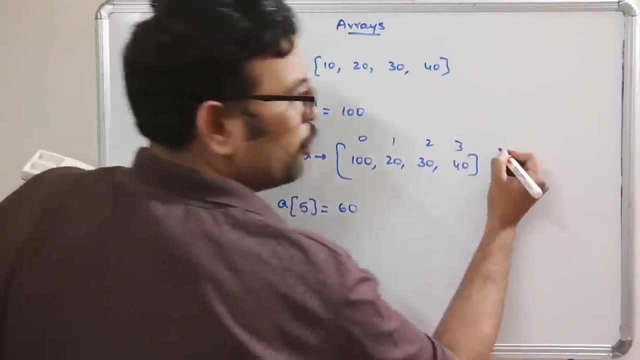 five is equal to 60. yeah, 5 is equal to 60. you can observe here: the index values are from zero. one, two and three. okay, there is a no fourth index. there is one second now, so we are not going to get to the next point. okay, we are going to get to the next point. 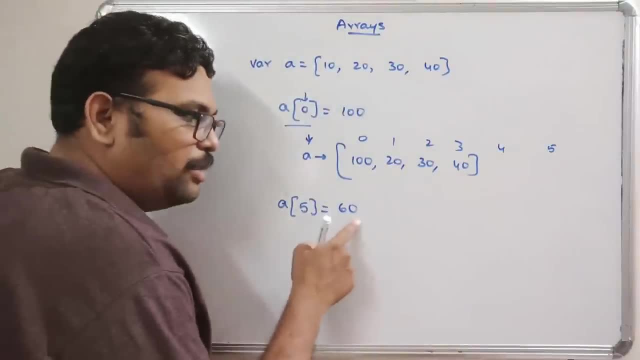 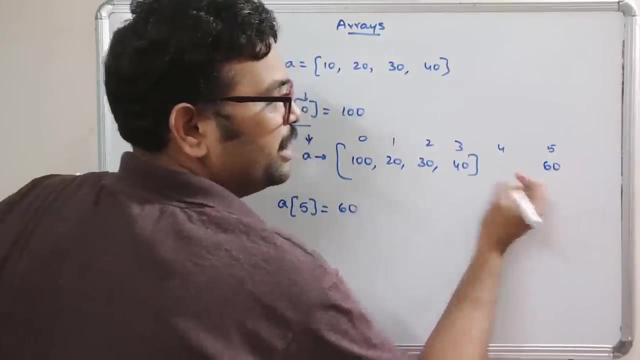 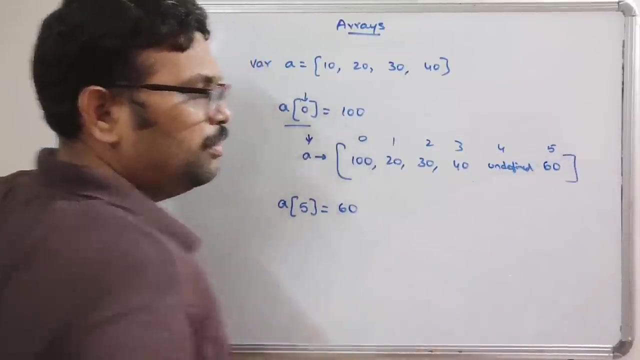 is no fifth index, right, but still we are assigning a value to the index file. so automatically it will go with the index file and it will store 60 and coming to the four, it will be undefined- okay, undefined. so now the value for fifth index will be 60, and without the four we can't go with. 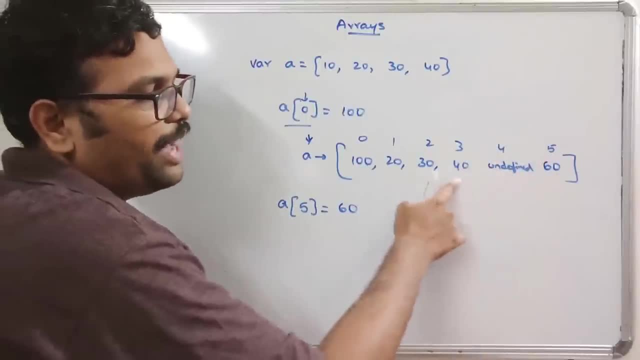 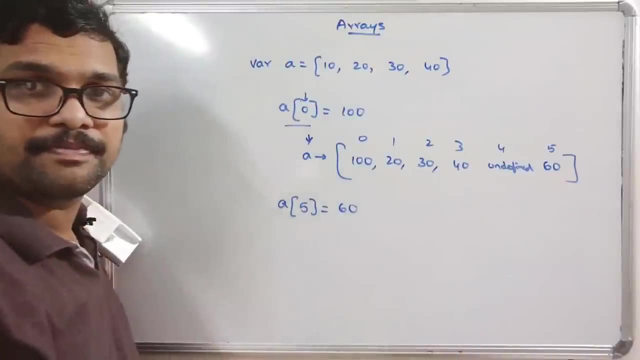 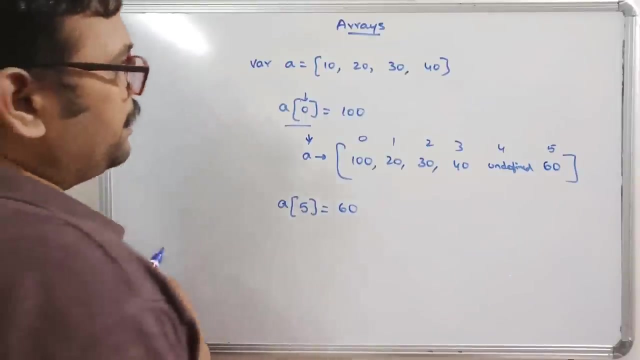 the file. so five fourth index will be created and the value will be undefined, and immediately the fifth index will be created and the value will be stored in the fifth index, right? so this is how we can assign a value beyond the length, also beyond the length, right then? so this is all. 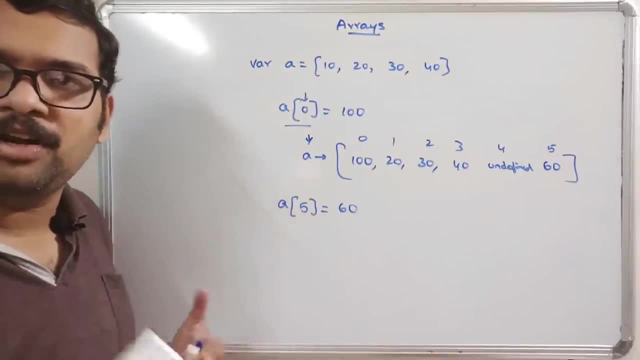 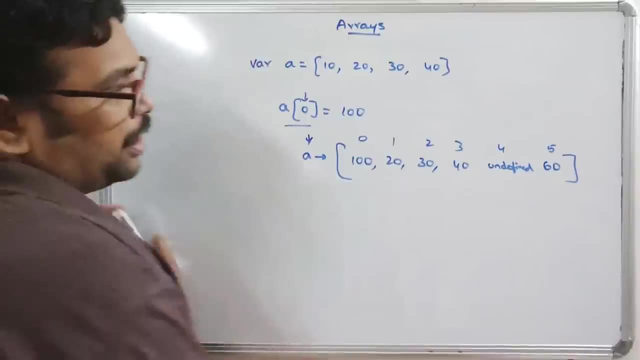 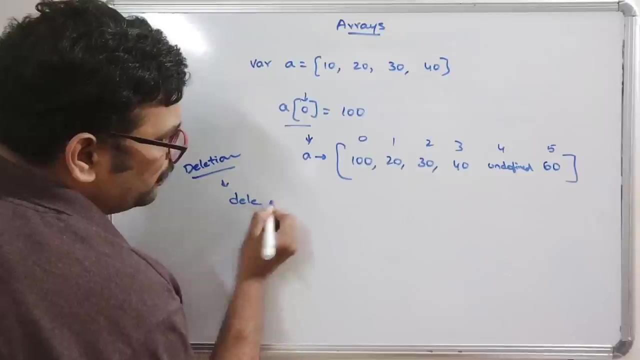 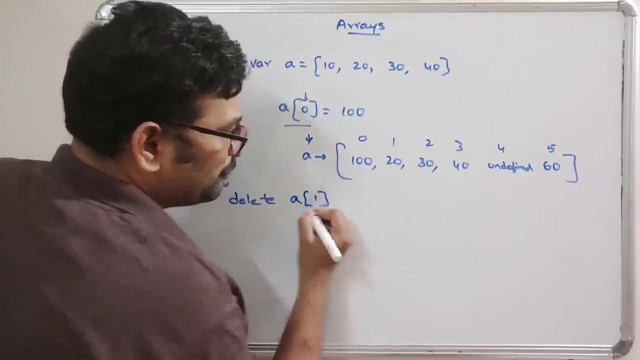 about our reassignment. okay, reassignment, or adding the elements, we can also add, or we can reassign the elements and coming to the deletion. coming to the deletion, so how can we delete? so, by using delete keyword, so delete, give the add the array name and the index. so a of one, a of one, automatically. 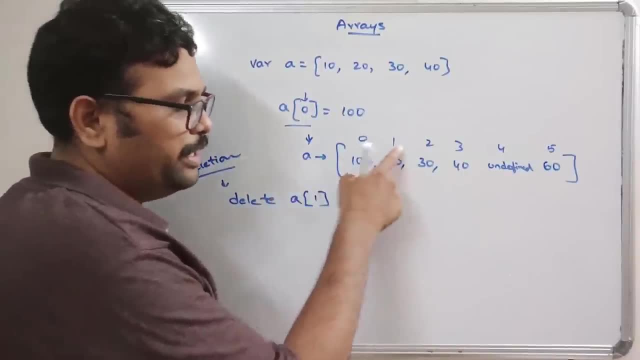 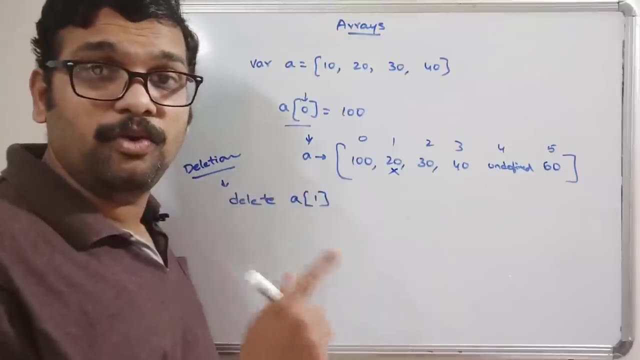 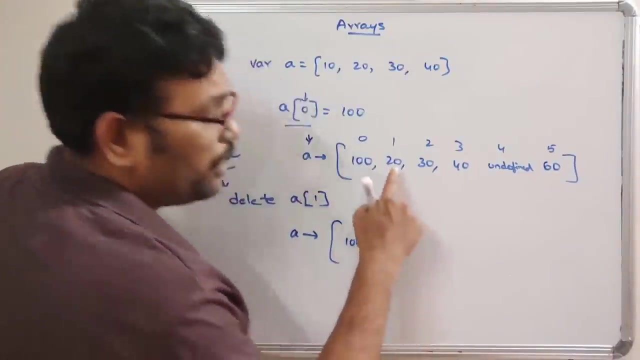 from the array a. whatever the value available in one index, one that will be deleted. so this will be deleted, the space not will be. i mean, the space will not be deleted, only the value will be deleted. so if you print a, we will get the result as 100 and we have removed the value at the 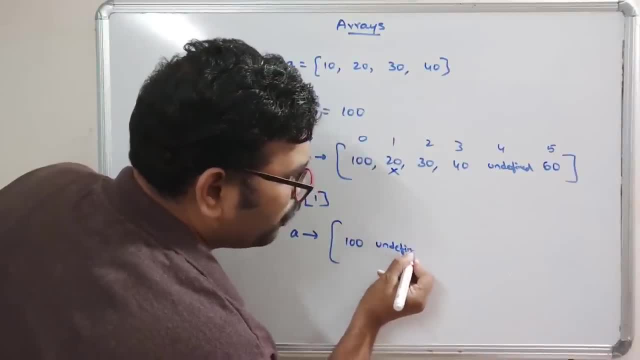 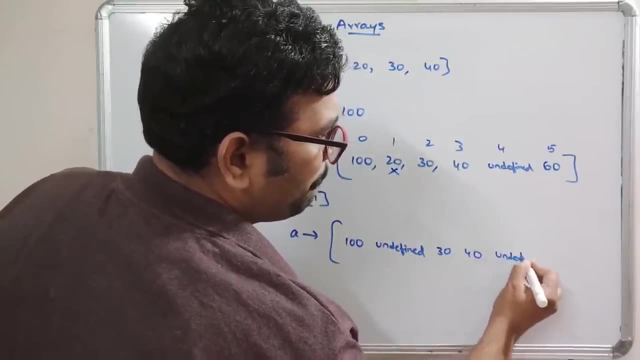 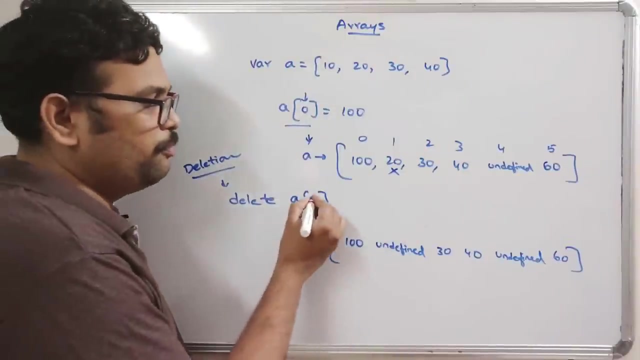 space one. so we will get undefined. so the value or the space will not be deleted. so next to 30, next to 40, again undefined, undefined, 60. so this will be the result after deleting the element at first index. and if you move with the second index, so 30 will also be deleted and in place of 30 will. 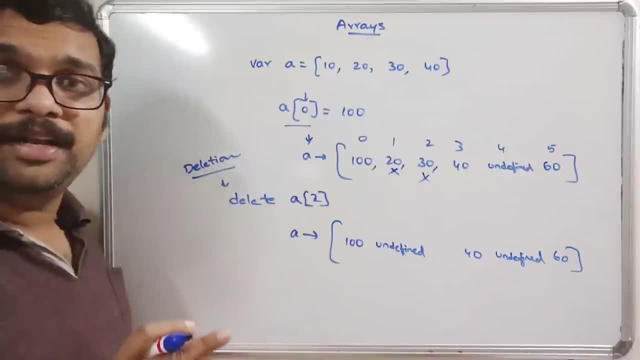 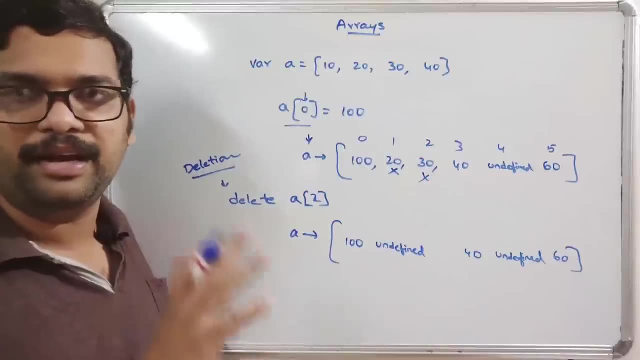 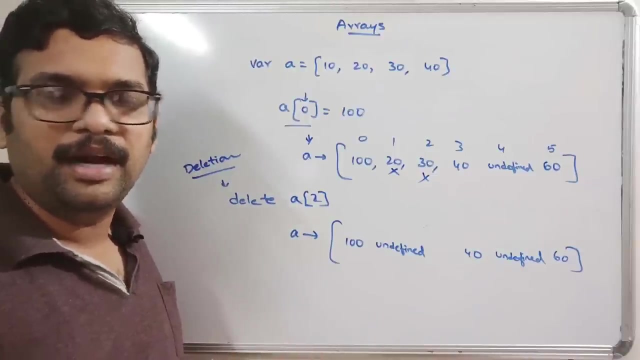 get undefined, another undefined right. so only the element will be deleted, but not the space. okay, the memory will not be released. the memory will be allocated with the undefined symbols. undefined, okay, unless you you add an element in that particular index, it will show the undefined right. so this is how we can delete the. 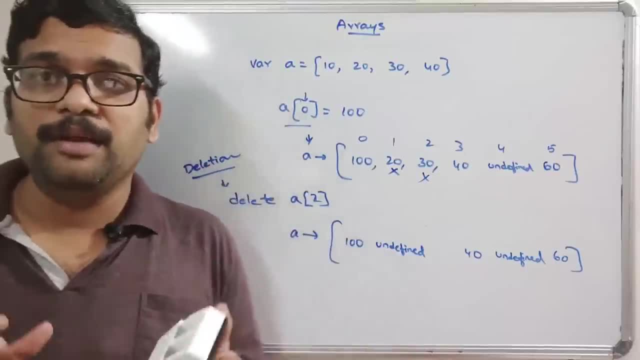 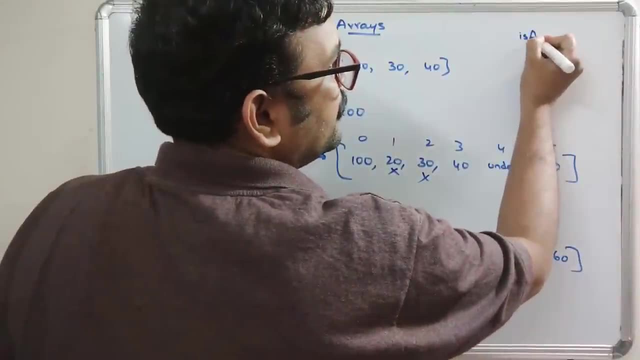 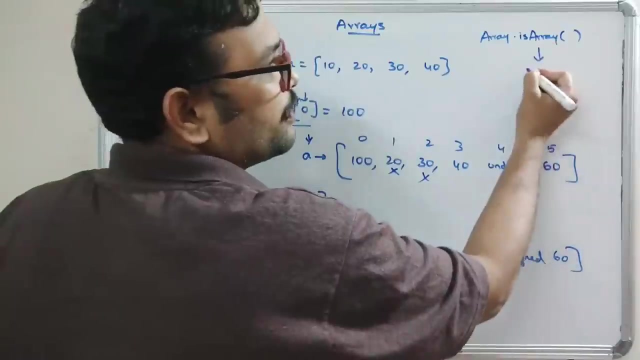 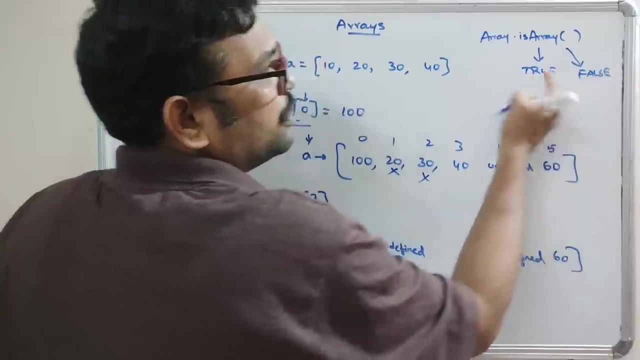 element now how to know whether the variable is an array or a normal variable. so for that purpose we are having a function called is array function is array, so is array function. so array dot. array dot is array. this will give a true or false right. so if this function returns true, automatically, here we have to give. 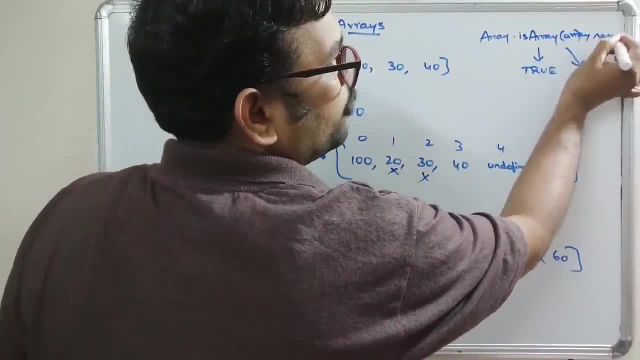 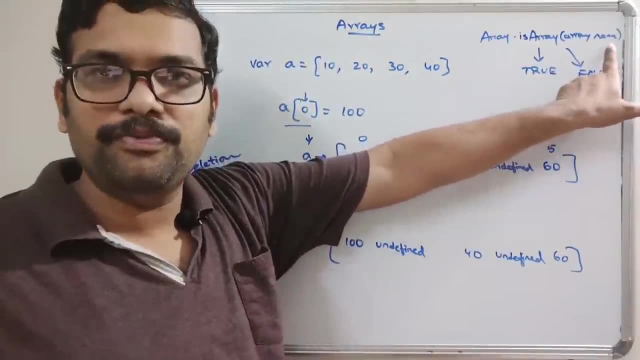 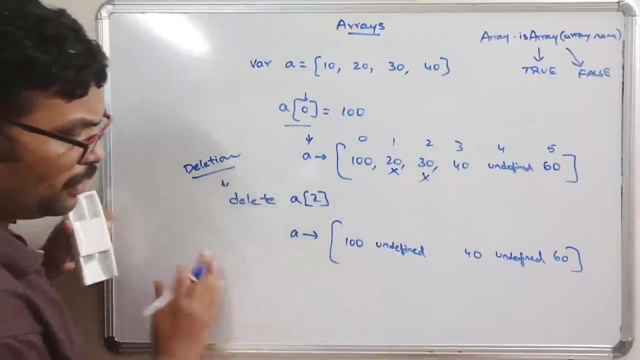 some array name. array name should be given here. okay, array name should be given. so if it returns true, that implies the name of the variable given here is an array. if it is false, it's not an example. example, see. so here we have created some a right, here we have created. 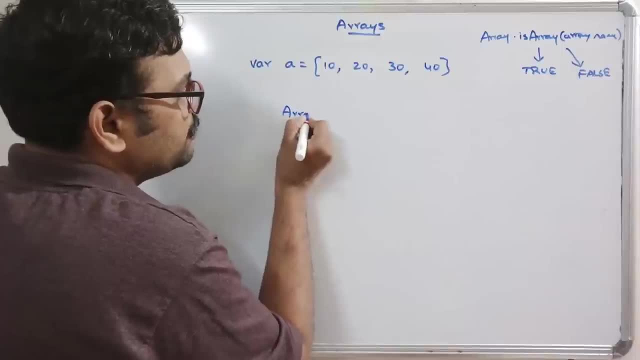 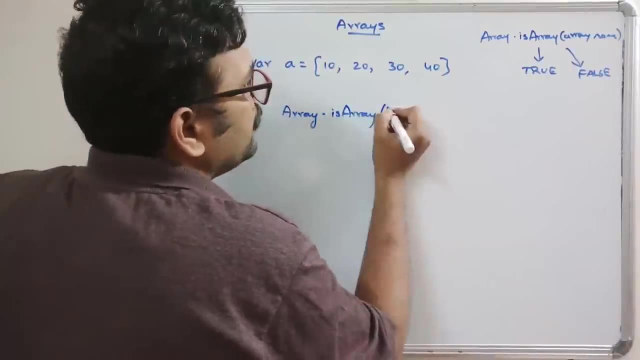 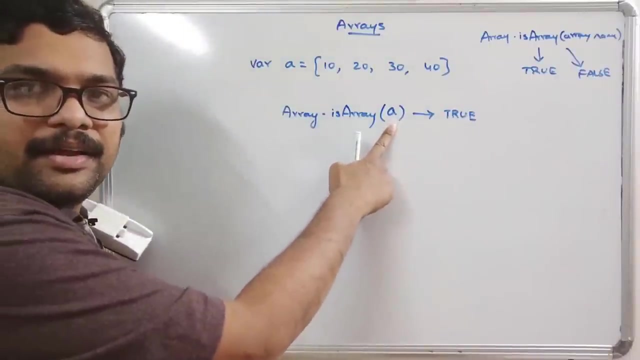 some a. now we can check array. dot is array, so is array. in his array we must be listed of a, so this will return true. so that implies a is a array. so if you go with the type of, if you, if you check with the type of a, it will return as an object. 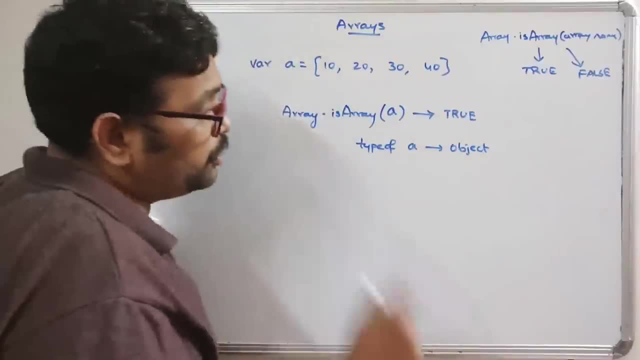 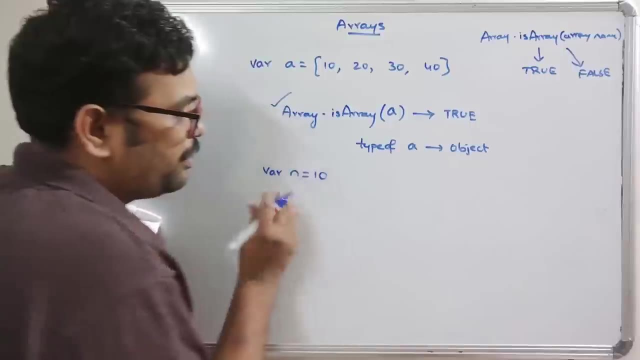 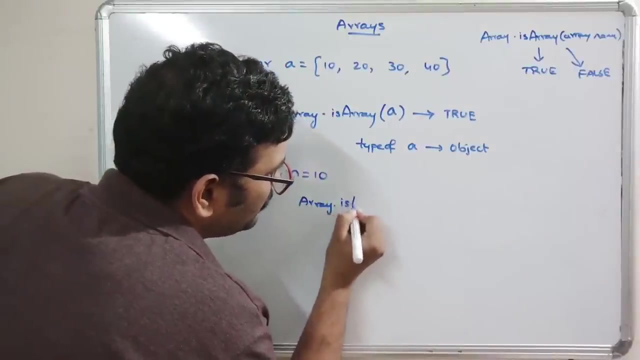 even though it is an array, it will return an object. so in order to check the- whether it is an array or not, you have to use this function. and for example, variable n is equal to 10. that means n holds the numbers. now, array dot is array of n. it will gives as a false. 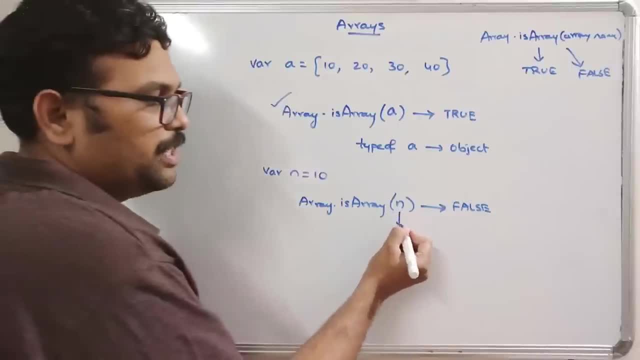 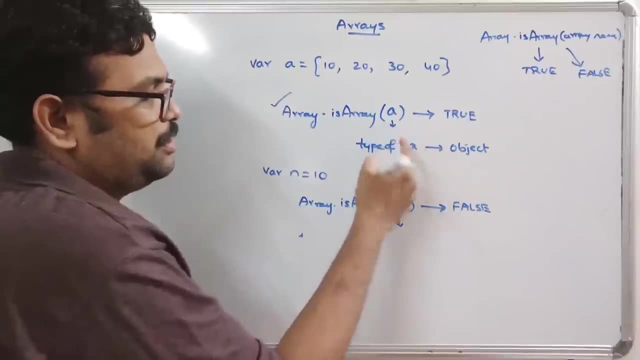 it will return false because the argument that means the name of the variable. this is not an array, this is a number, so automatically we'll get a false as result. but in this case, this is this is an array, so automatically we'll get the result as true. so this is how we can check whether 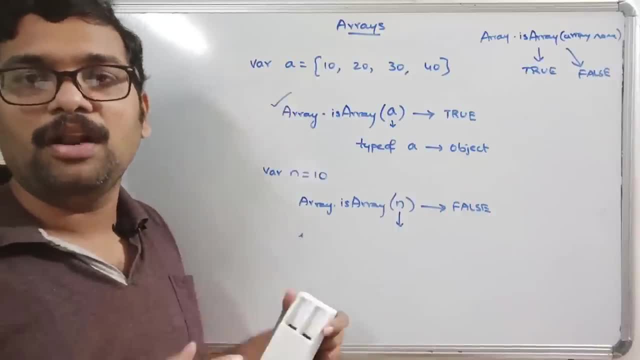 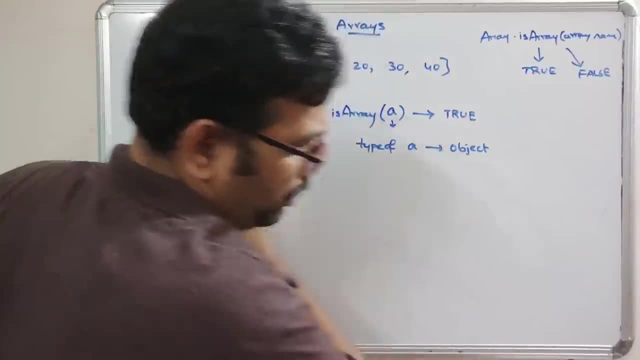 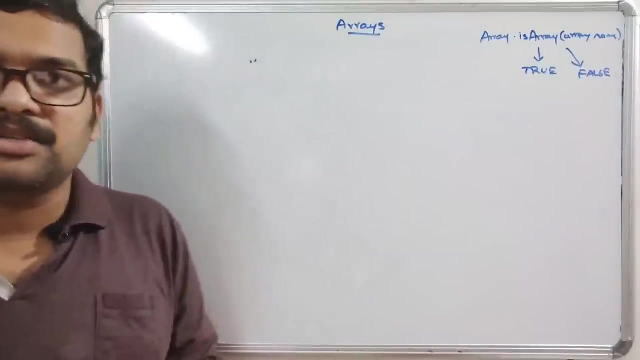 the given variable is an array or a normal object or the any number, right? so hope you understood this one, all of you. let's stop here, and in the next session we'll discuss about different methods of array. and now we'll move on to the system, and i will demonstrate all these things by executing a. 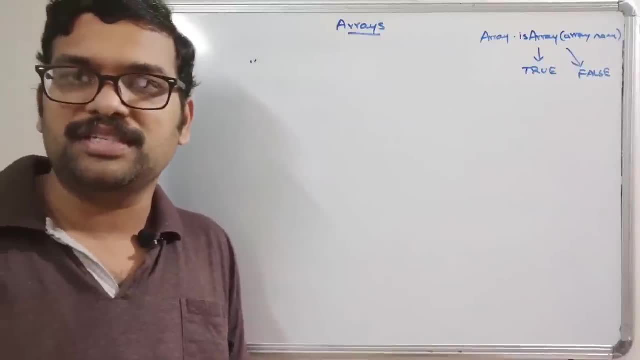 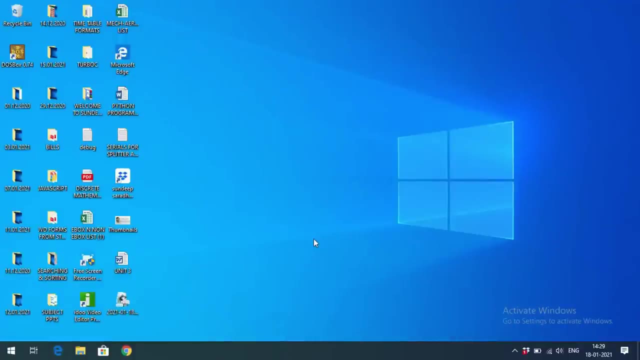 small html code. right, so let's move on to the system. hello friends. so just now we have seen the theoretical part of array introduction. that means how to create an array, how to access the elements and how to get the length of the array and how to add more number of elements and how. 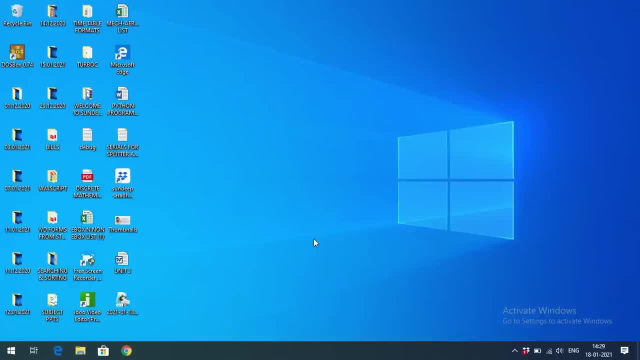 to delete the elements. all these things we have seen now, theoretically. just now we'll see the theoretical part of array introduction. that means we'll demonstrate all these things by executing a small code. so let us take the notepad and let's start writing the code with the html tags. so 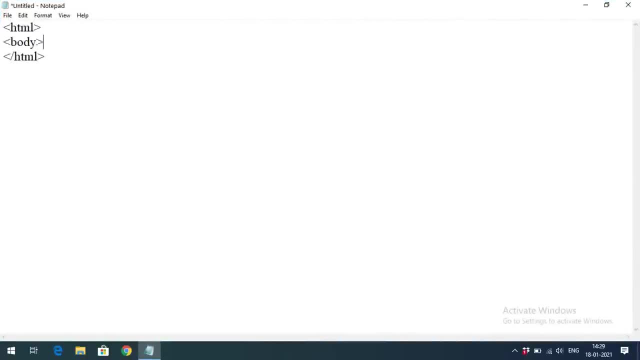 inside the html tags, we need to write a body and inside the body we'll write the script. right? so inside the body, just go with the heading. so we'll give some heading arrays and then start writing the script. now, inside the script, First let us create an array. So, in order to create an array, the creation of array will 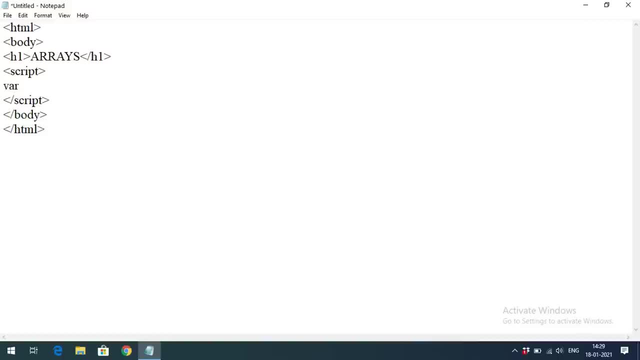 can be done in two ways. So one is without using a new keyword and another one is without using a new keyword. Let us check it. where a is equal to open the square braces, give the comma separated values and close, and you can go with the document. dot write ln and. 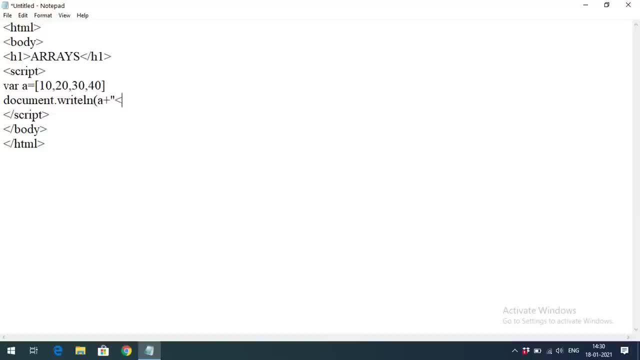 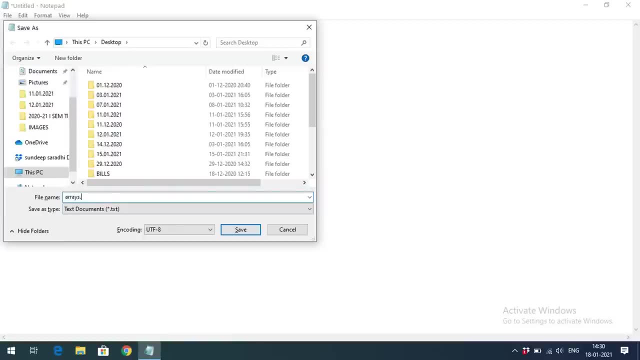 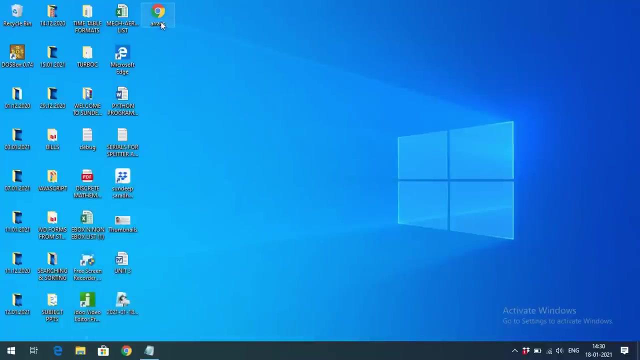 go with the a and also give the break row, So that our next execution will be printed in the next one. So first save this one. So I will save this one with the arrays dot HTML So that it was displayed in desktop So you can observe here. just double click. 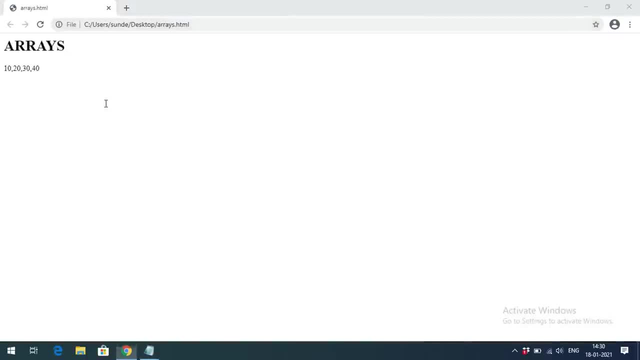 on this will execute. will get c. this is the array. Now, what is the type of this array? So in order to get any variable type, we are using some type of type of keyword. So we think in the previous session we have seen that. Now we will check type of a plus give. 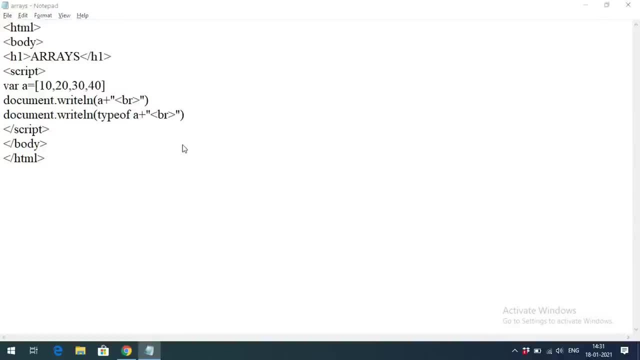 the break row for the next right Now we will get the output as object. So in java script, arrays will be represented as an objects itself. So even though you are creating an array, it will be created as an object. Next, the second way of creating an array is array. 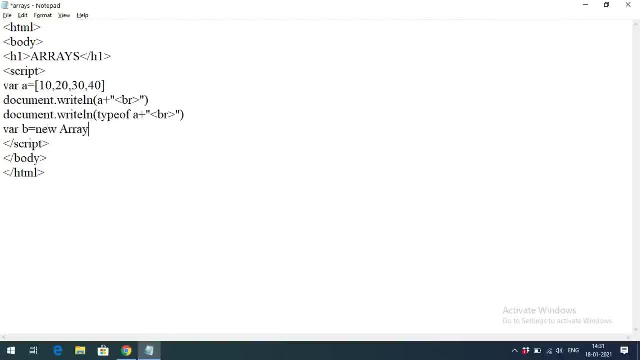 a is b is equal to using a new keyword. So I will show you the difference, why we have to go with This one and all these things. So 50,, 60,, 70 and 80- ok, So here also I have created. 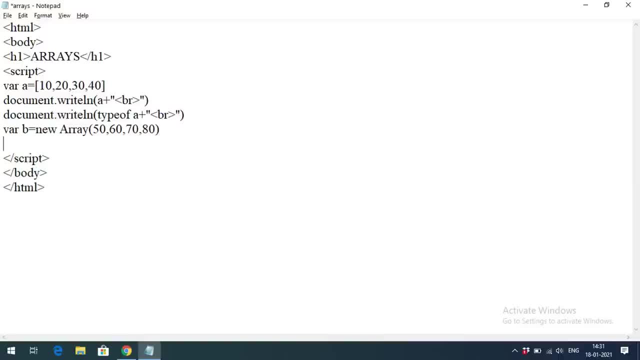 some four variables, So four values in that array. right and here also you can print document dot, write ln, b plus go with the break row. for the next output, see 50,, 60,, 70,, 80. again there are, If you want to create a single element, single element where the variable c is equal to single. 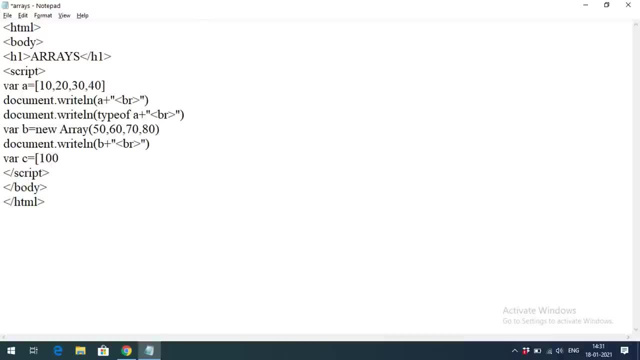 element some 100. ok, 100, I am giving some 100.. Now go with the same thing. So document dot. write ln, c plus go with the break row for the next output, c. What is the value? 100? perfect, And go with the d is equal to new array of elements. So if you want to create a single, 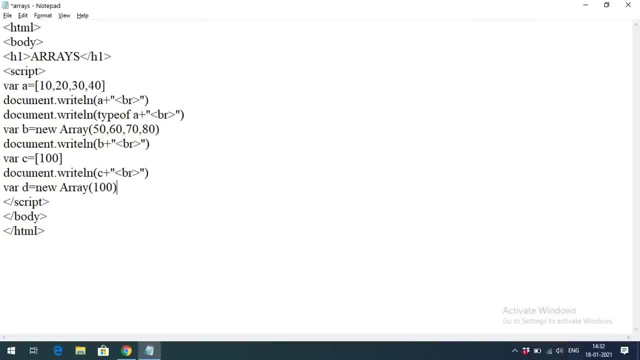 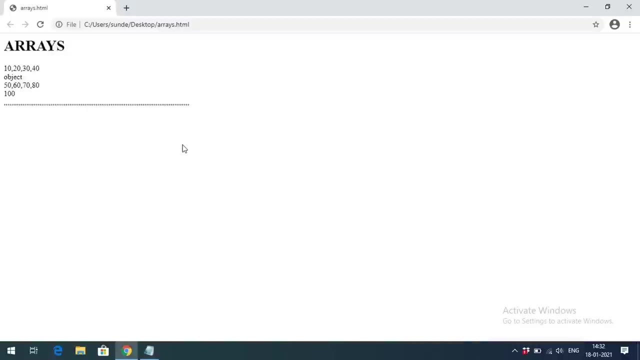 element, single element where the variable c is equal to single element. some 100, ok, 100.. Now just go with the this one document: dot, write ln, d, plus give the break row for the next output. So you can observe here. So what we got: all commas. all commas because 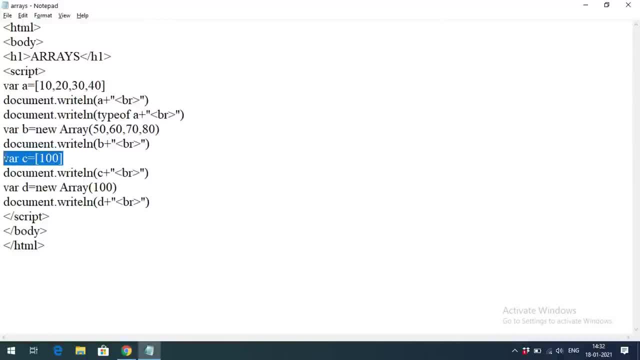 this statement, So particularly this statement- will create a single element for the array. but if you are using new keyword, It will create 100 elements, 100 elements with a undefined values, 100 elements. So this is the size in this statement: 100 is a size. it will treat 100 as a size, right? So if 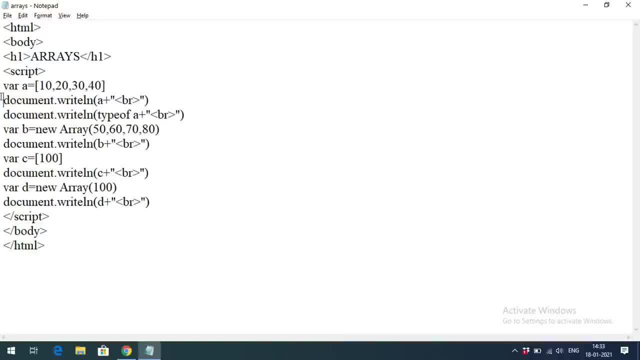 you want to add a more number of elements, we can go with this one. So this way we can create this way right And for inserting. we are having a lot of functions. we are having some few, So we are having a lot of functions. we are having a push function and a pop function. 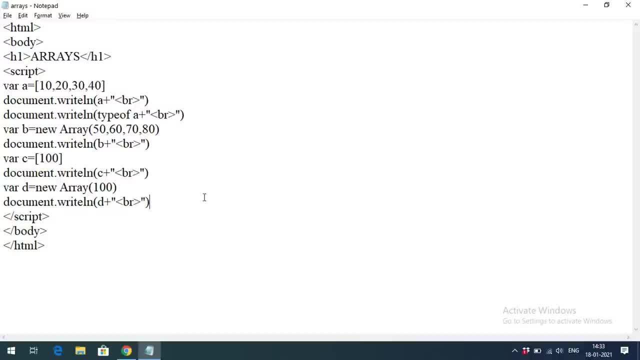 that we will discuss in the next session. So this is how we can create an array by using a normal way and by using the new keyword. And now how to get the length length of the array: simply go with the length property, write ln. So here we are having some a. a is equal to 4 element, So a dot length, or 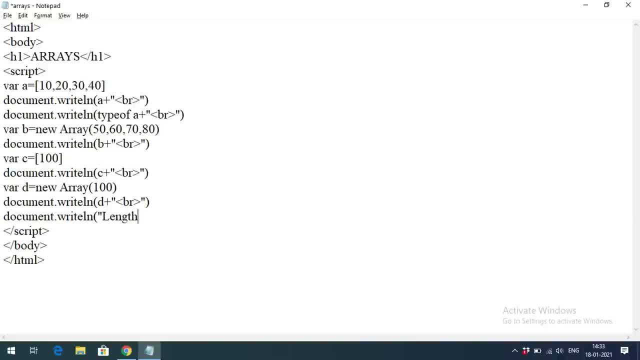 simply give the text a is and go with this one plus a dot length. this will directly gives the length of the array and give the break row for the next output. So you can get here. length of array is 4,. 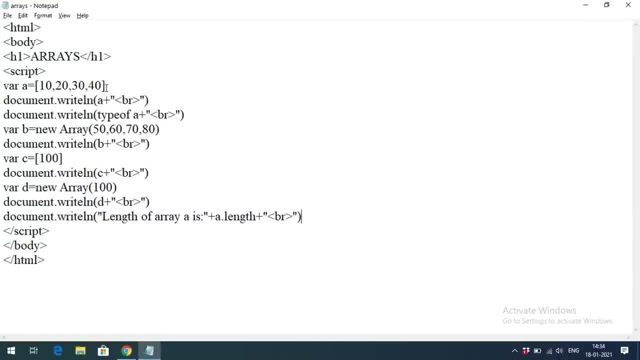 length of array a is 4.. So you can observe 10,, 20,, 30,, 40. So total 4 elements are there. So this is how we can find the length of the array and then how to create a, how to access. 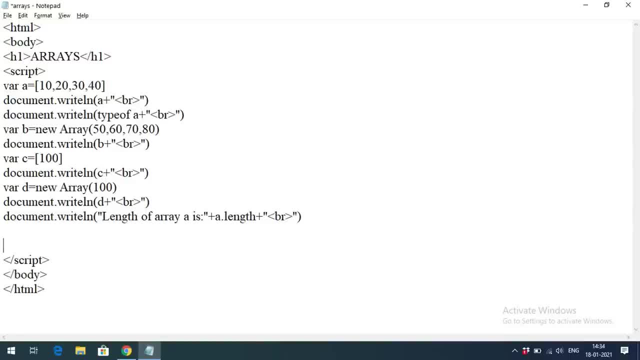 the elements. how to access the elements. So we can access the elements with the help of index values. Here also there will be index values and index values will always start from 0. So by using the index values we can access the arrays. So let us check here. So document dot. 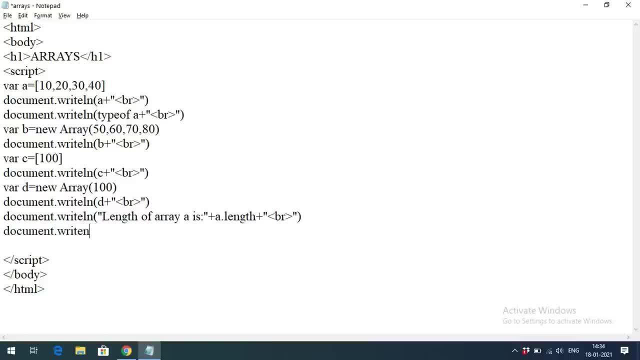 write ln and here elements plus. or we can simply go with the first element, First element plus. how we can give a of 0 will give the first element plus, give the break row for the next. So first element 10.. So give some space So that we will get the. 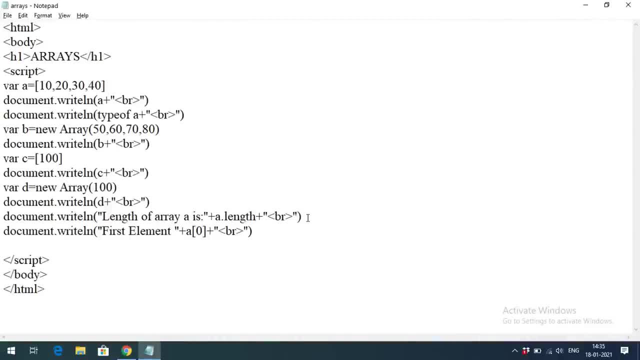 clear, right. First element is 10, right? Similarly, we can if you go with the second element, if you want to go with the second element, what is the second element index? It is a 1, 1. So second element is 20 and the third element will be 30,. fourth element will be 40. So second element is 20 and the third element will be 30,. fourth element will be 40. So second element is 20 and the third element will be 30,. fourth element will be 40. So second element will be 40.. 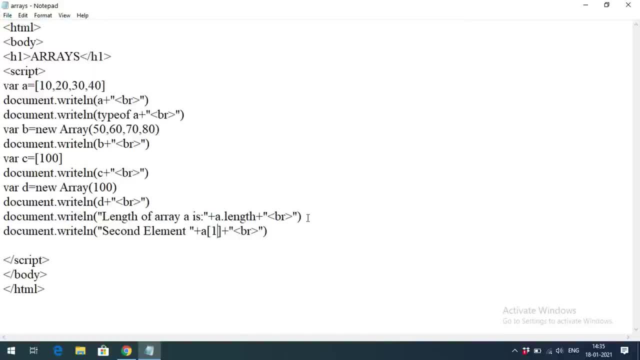 30,. fourth element will be 40. So, like that, by using the index values, by using the index values, we are supposed to access the elements. And now how to print this one, How to print that one? So, simply by giving this one, we can print the. 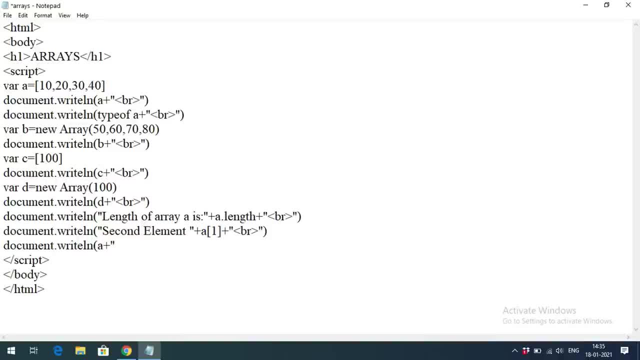 complete array. So simply by you giving the array name we can get the complete array. And And there is a one more way to access the elements, that is a named index, values, named index. So these are called numbered index, because with the help of numbers. So 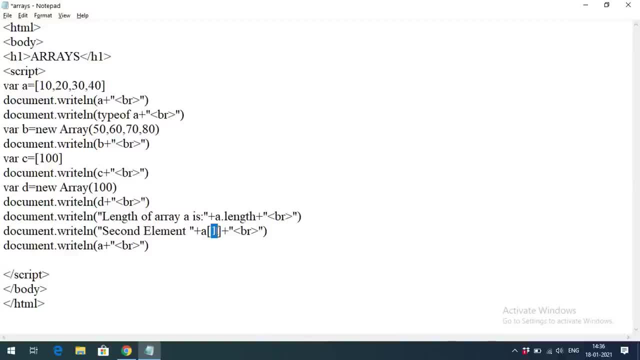 in the subscript we are giving some numbers. based upon the numbers we are accessing the elements. So there is another way to access the elements, that is, a named elements. So in such for that purpose, we will have to create the array in such a way where e is equal. 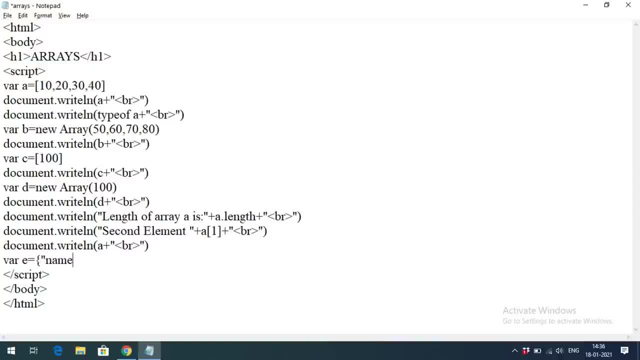 to open the curly brace. So give the name. give the name instead of using index values. we are giving some name for all the elements, some a, b, c, and give the roll number. So if it is a string, we need to give in the double quotations. So 1, 2, 3, ok, and go with the percentage. 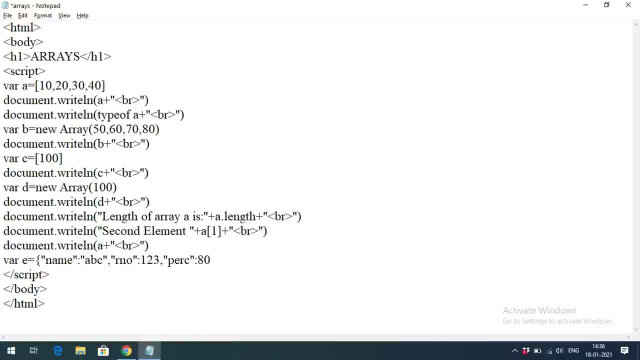 colon, give the percentage some 80 and close the curly braces. So this is also an array. ok, this is also an array, But here, If you go with this one, write ln of e. see, you will get some object. ok, here you will get some object. 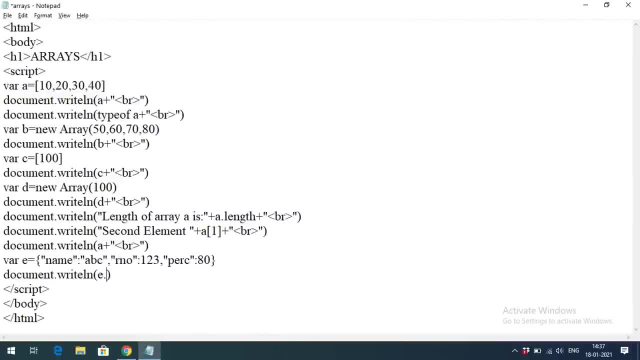 If you want to access the elements, go with the named index: e dot name. e dot name. it will give the name of the element. ok, name of the particular element plus break row. So in the next will be added here. So e dot array, dot element name, named index: ok. similarly. 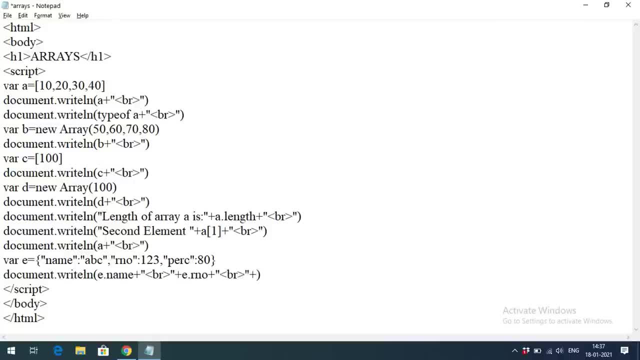 again go with the break row So that the output will be printed on the next one. So e dot % plus, give the break row. Now you can observe we can get the elements with help of named indexes. So this is a named index, ok. whereas here this is a numbered index. So with the help of numbered 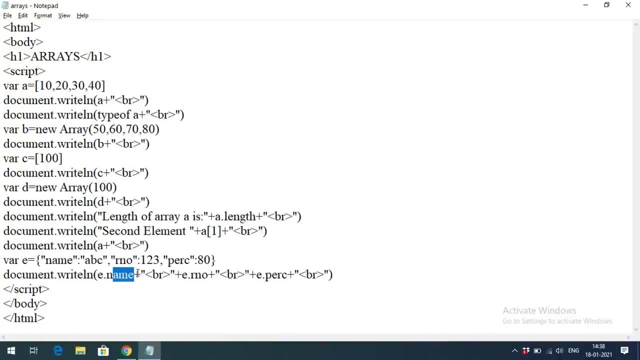 index. we are accessing the elements, but here we are using some names in order to access the elements right. So preferably it would be preferred with the numbered index right. So the next one is the looping. So how can we display all the elements one by one? 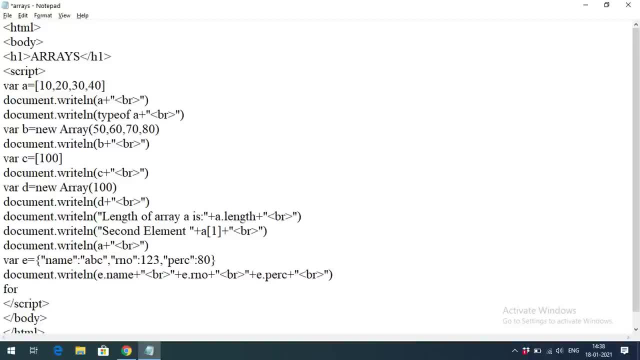 So use a statement. So here you can have for loop i is equal to 0 and you know the property length, property i less than a dot length. So you know a is having some 20, 30 elements. So 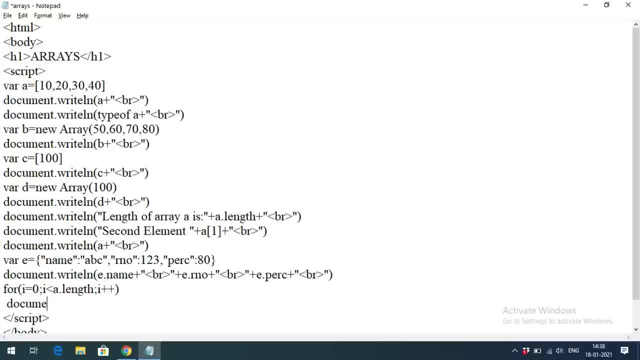 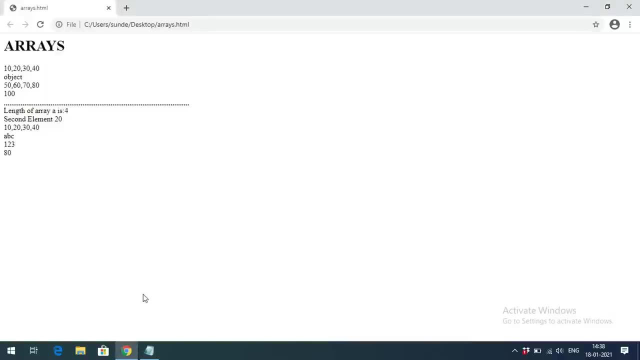 i++ and just print here: documentwriteln: go with a of i plus, so each and every element will be printed in a new line here. So you can observe here. so each and every element will be printed in a new line. So you can observe here. 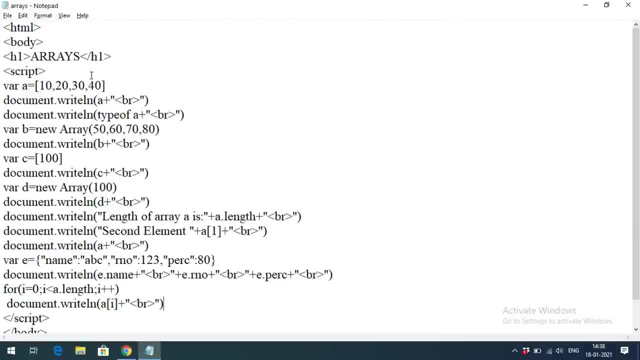 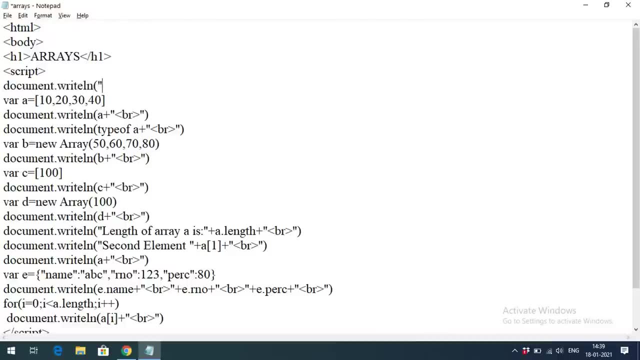 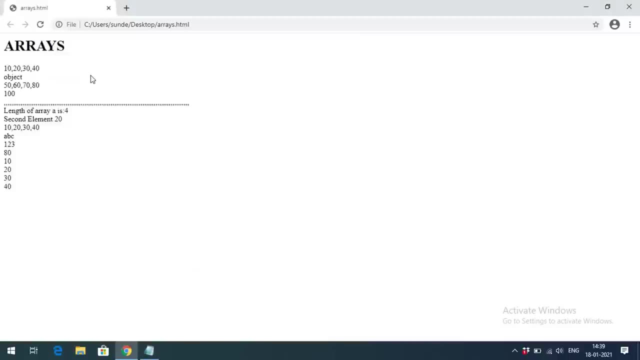 10,, 20,, 30, 40. ok, just I will increase the font size. document dot write ln h2, h2. yeah, so you can get it right. So 10, 20,, 30, 40. so these elements will be printed in a line. 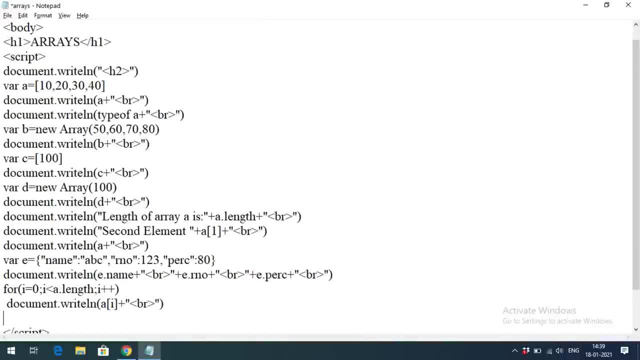 by line. that is, we are using some iterative statements and we are printing the elements of a array, right? So how to change the elements? that means a reassignment. how to change the elements, that is a reassignment. So we know that. so, document: dot write ln. write ln. a is 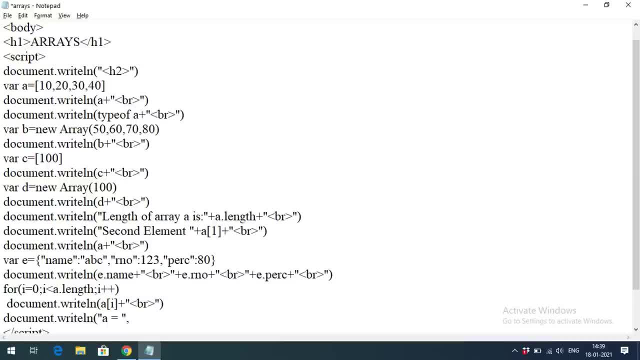 it. a is equal to see. here we will go with a plus. Now you can observe here. so a is equal to some 10,, 20,, 30,, 40, right? So here we will go with this one, ok, instead of going this one, we will write here, right? ok, So just remove. 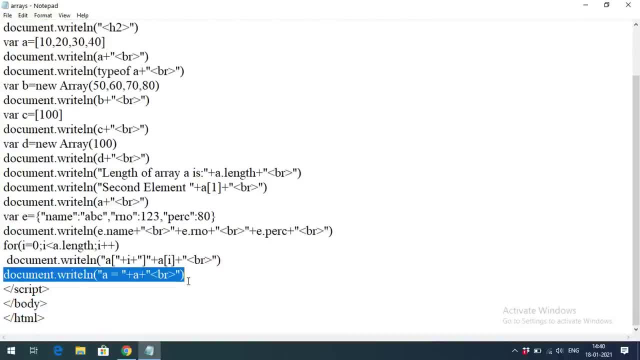 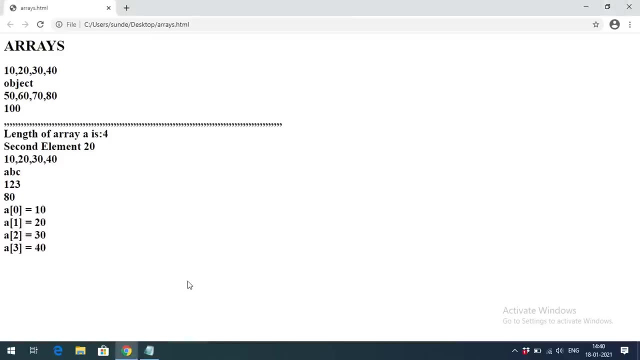 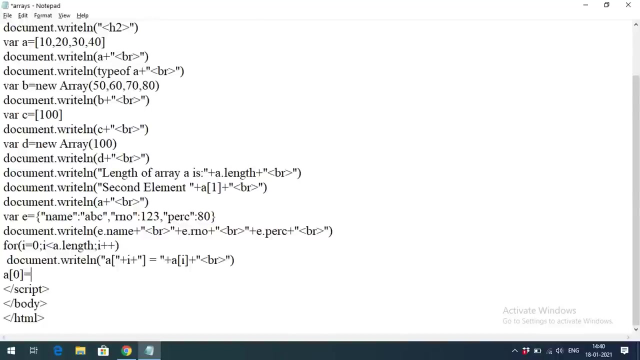 this one, So a of 0. now it is 100, right, So previously it was 10. now I have reassigned the value, So automatically the element which is available at 0th index is replaced with the 100.. So 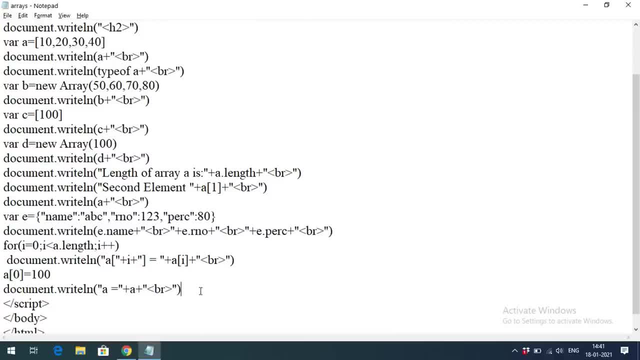 the updated array is 100,, 20,, 30,, 40. So this is how we can update the element. that means change the elements, change the elements and how to delete the elements. So you should delete any element. so we can delete the element by using the delete keyword. So delete give. 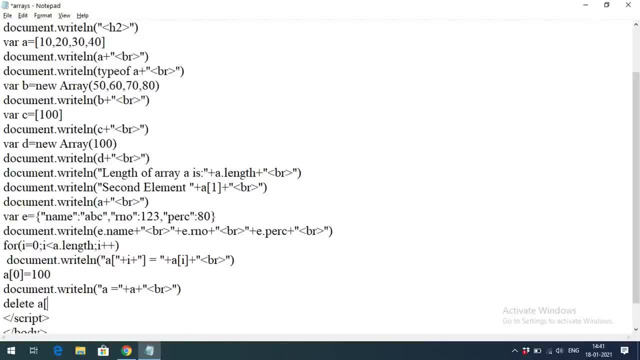 the value. that means give the specify the element, So delete. So delete the elements means give the specify the index, So a of, for example, 1.. So the element present at the index value 1 will be deleted and the space will not be removed. That means some undefined space will be. 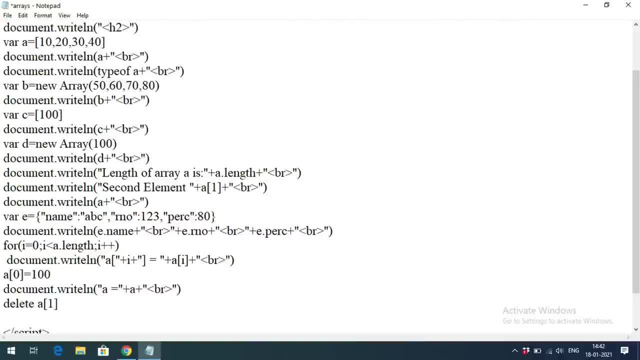 available there itself. It just only deletes the element. So now I will show you. So first we will get the length of a length of array a is a dot length. This is the property in gth property and go with the break row. 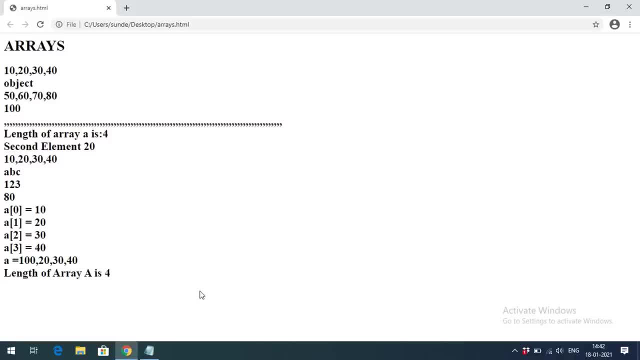 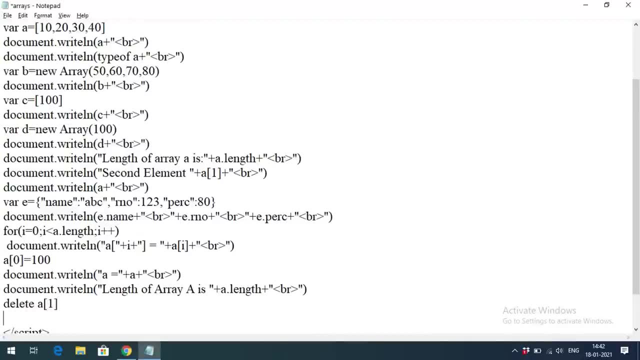 Now you can observe the length of the array. a is 4.. Now I am deleting the element delete a of 1.. So just this statement will delete the element present at the index value 1.. Now if you go with document dot, write ln and the same thing, just copy the same thing. 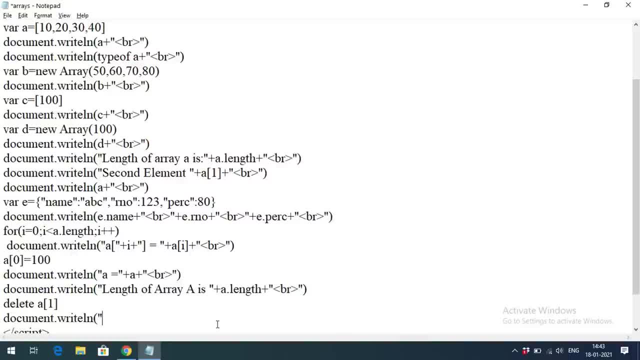 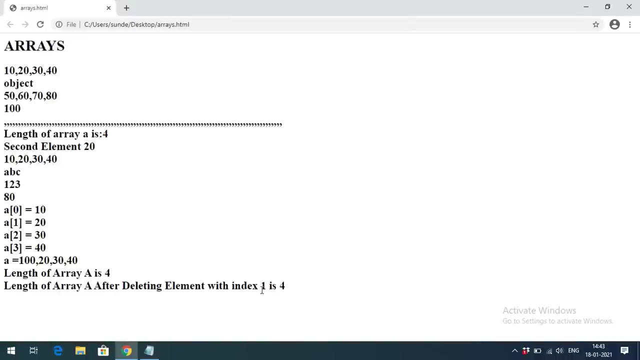 a: after deleting, after. after deleting element with index 1.. Now this is the statement we are giving: after deletion, Still the length is 4.. Still, the length is 4.. Now, you can observe. So what about the? 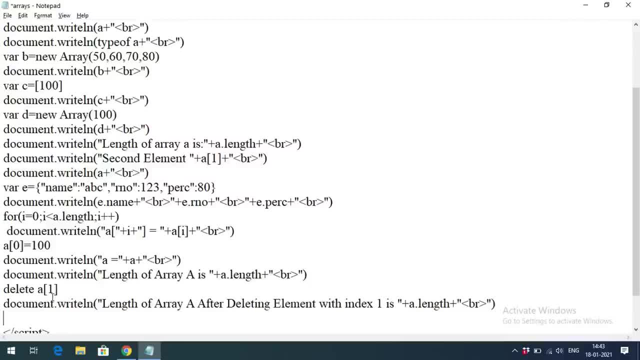 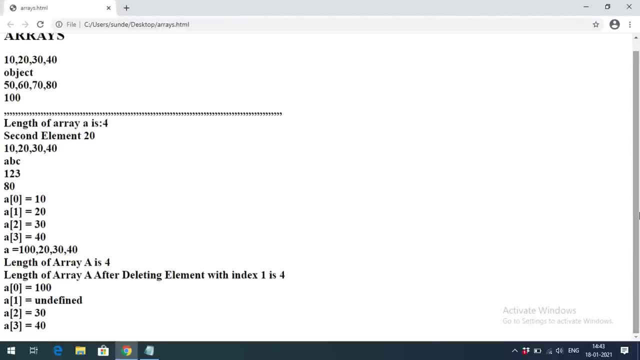 what is the value of a of 1?? Because we have already deleted it. We have already deleted it. Now, if you observe here, just go with the same statement So that we will get the values of a. You can observe here: a of 1 is undefined. That means the space will not be removed. So 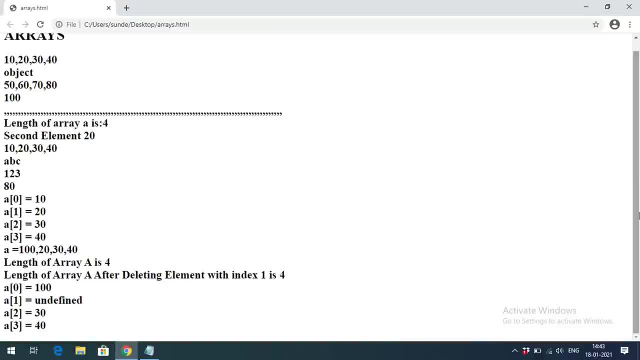 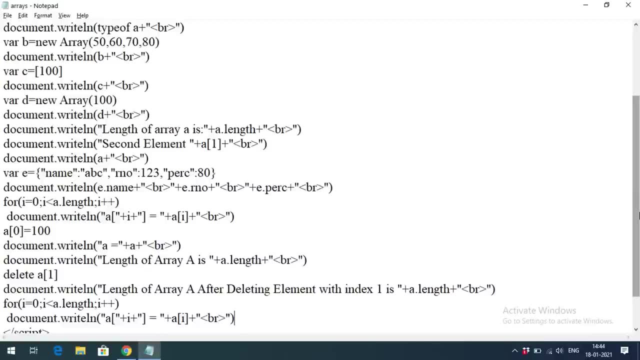 the space remains the same, So only the value will be deleted. So the value will be deleted and it will be as it is. I mean the space will be as it is. The reference, I mean the space reference- will be as it is, And we can also insert a more number of elements, Like 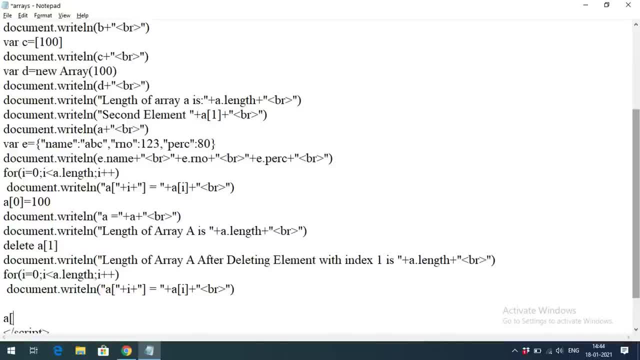 for example, a of. so a is having around 4 elements, index 3. If I go with a of 5 or a of 6 is equal to some 200, automatically 6th element will be 200. And previously we are having only 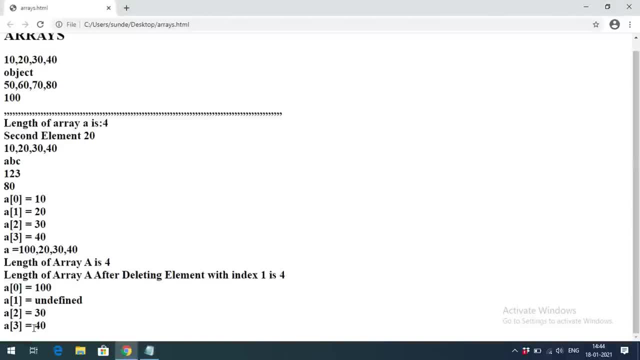 4 elements. right, only 4 elements. That means the 4th, 3rd index. Now I am inserting some index 6, the element at index 6.. So what about index values 4 and 5? Automatically it will be. 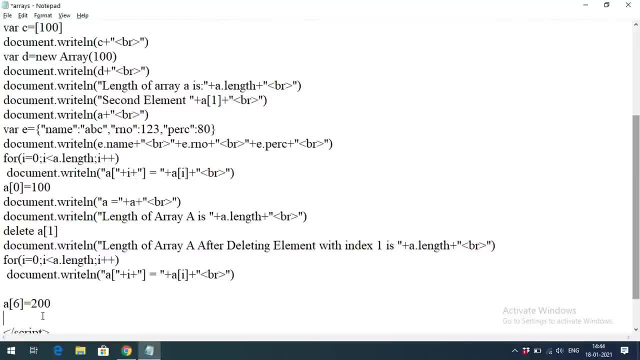 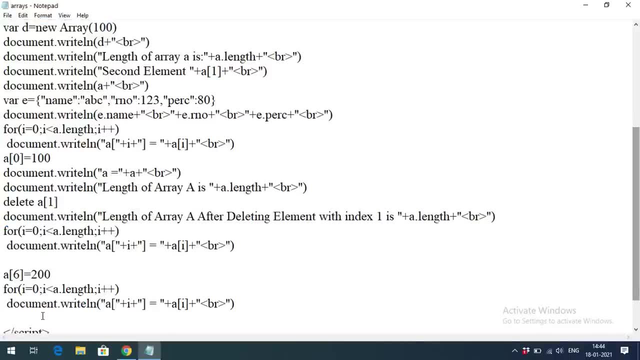 fixed with a space. That means undefined values will be occupied, right? So see again. once again I will go with this one. You can observe here: See a of 6 is 200, I have given So here we can write: go after inserting element at 6th element. 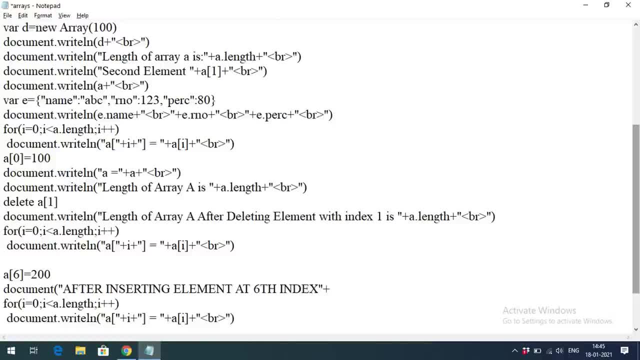 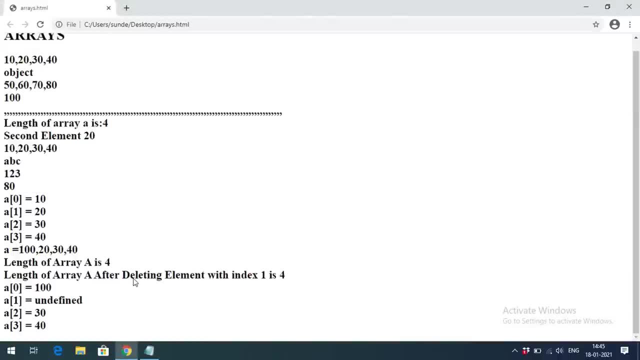 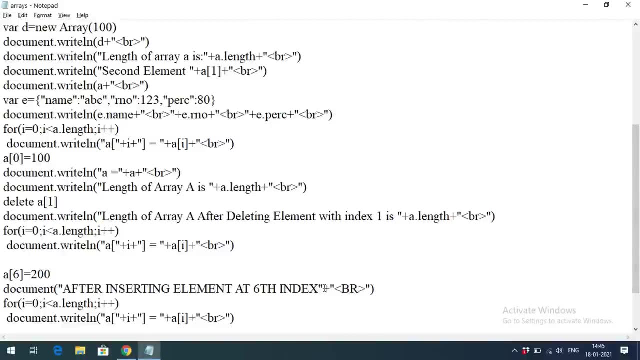 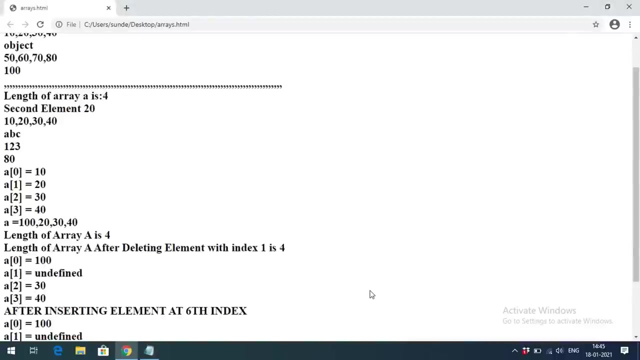 index. See, you can observe here. So after again, I have given a wrong statement here. document dot. write element. Sorry, write element And here we will go with this one, So you can observe After inserting. 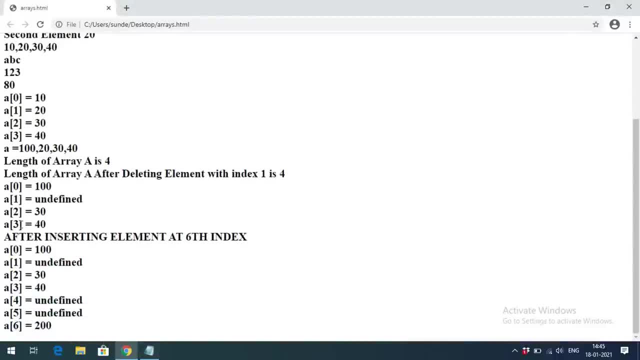 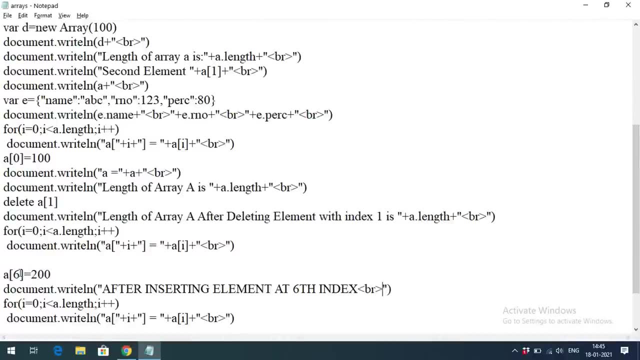 element at 6th index. So you can observe: previously, only 3rd index is the last element. Now I have, we have created some 6th index. We are inserting some element in the 6th index. 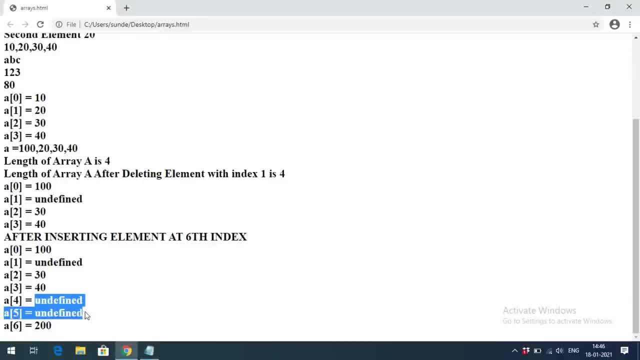 So what about the 4th index and 5th index? So those will be filled with undefined values. Ok, Now array is having some 7. 7 elements with a 3 undefined values and a 4 defined values. right, So this is how. 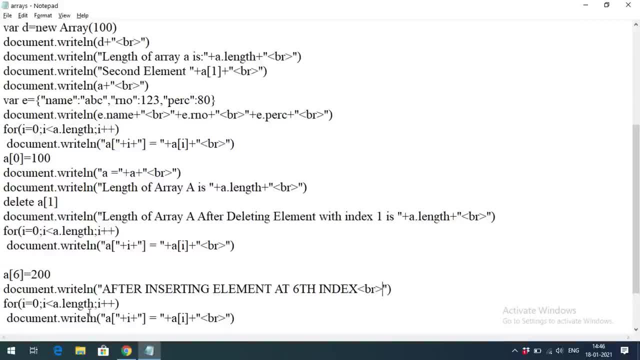 we can use the elements We can delete. So if you delete the element by using the delete keyword, the space will remain same, The count of values will be remain same. right And here, how to know whether the variable is array or not, Because even though it is an, 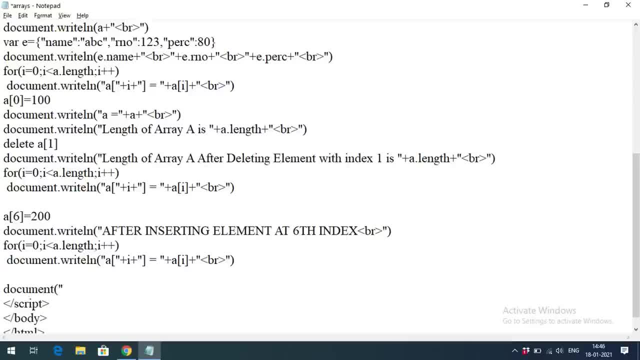 array what we have done. So we are getting some obj As a data type, right, So we know that type of a is array. ok, We know that type of a is array because we have created. So if anyone wants to know whether what is a data type, 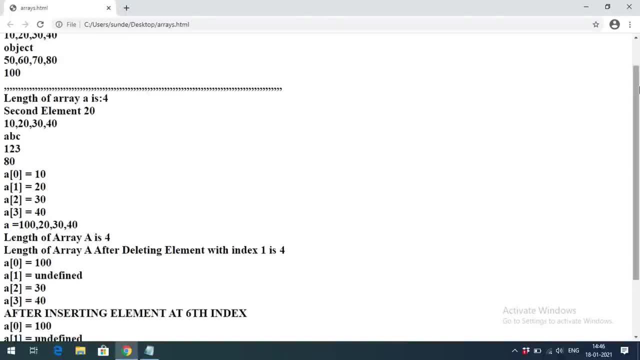 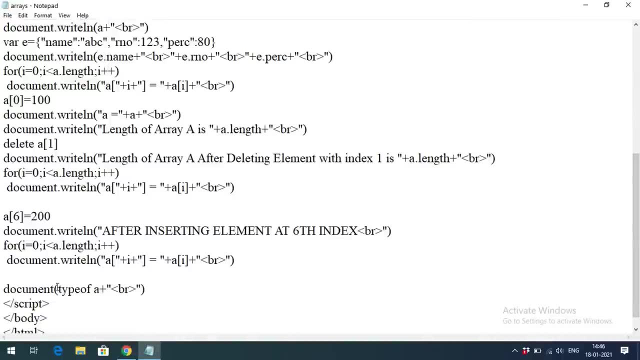 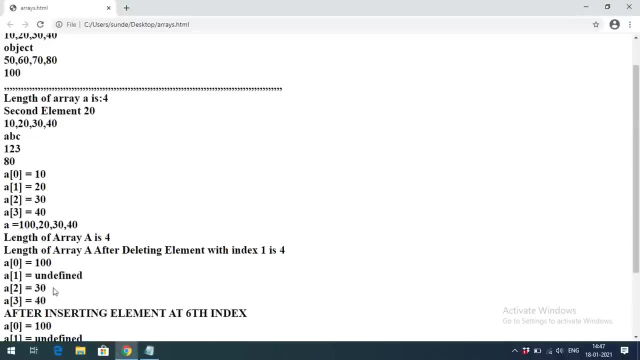 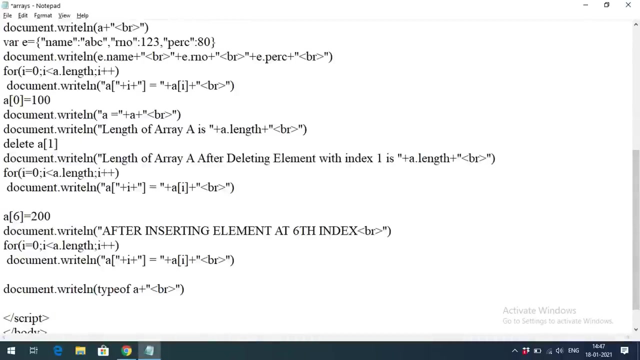 of array a, then if you go with the type of a, we will get the array as dot write element, So we will get the result as Object. right Now there is a function called is array, So if it is an array, automatically. 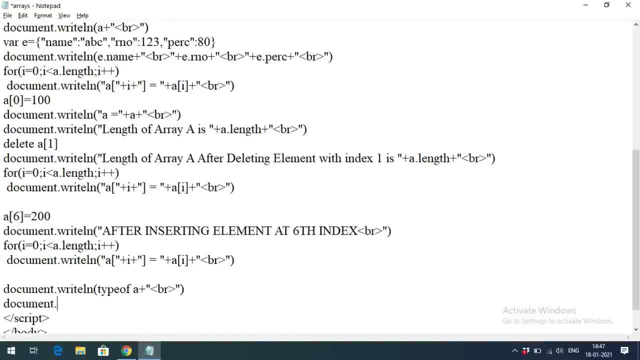 it will return true. Otherwise it will return false. You can go with document dot. write l: n. We can go with array: dot is array of. you have to pass an argument that means a, So it will check whether a is an array or not. If you go with here, you can observe. 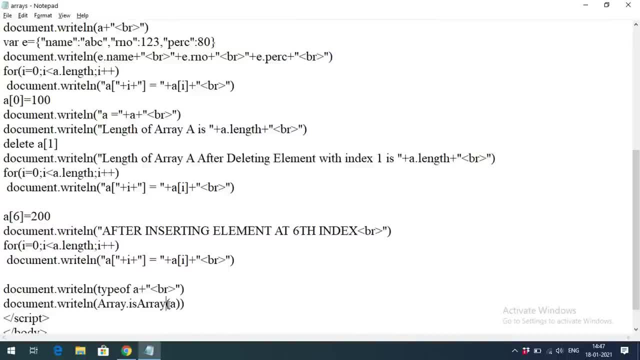 true, right, Thank you very much. Thank you. So here the array should be given in the parentheses as an argument, So it will check whether this given name is an array or not. ok, And here you can observe we have created. 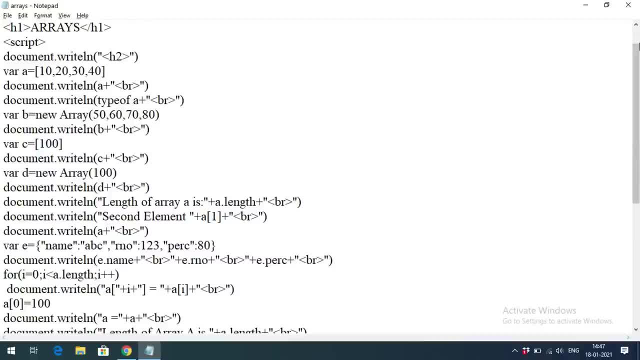 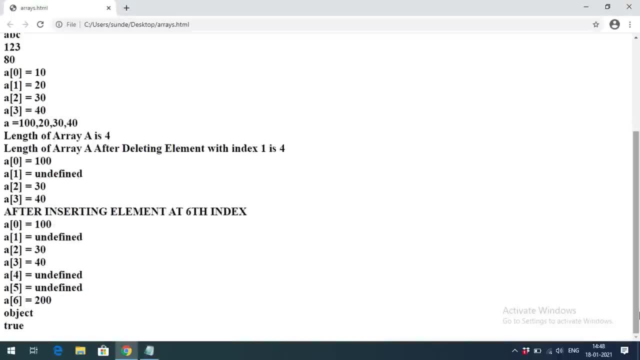 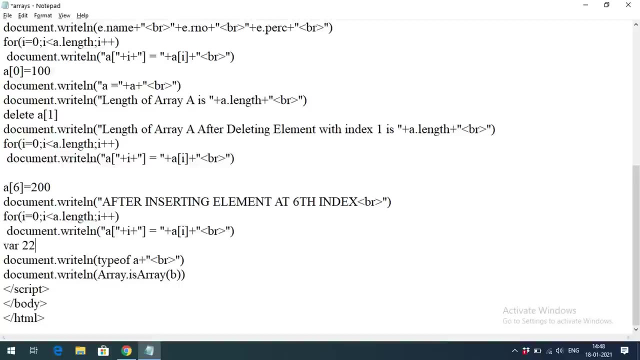 some b, right? So we will check whether b is an array or not. See it is a true, right? So if it is an array, it will return true. see where e, for example, where some n is equal to some 10, right? So let us check whether n is an array or not, So you will get some. 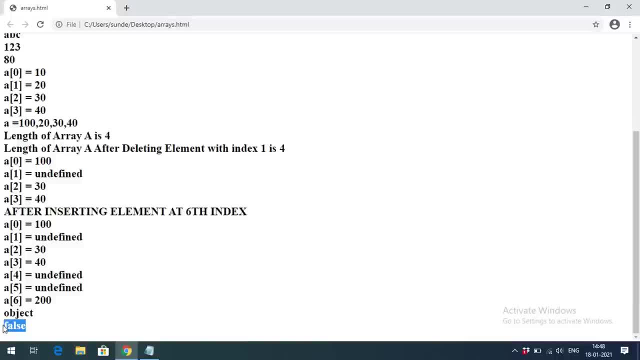 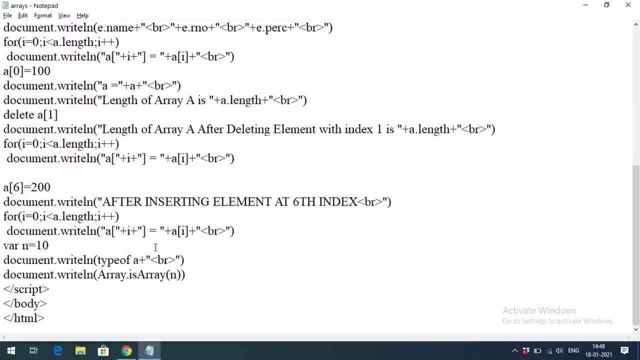 false because, see you can observe here- false because n is not an array, n is a number, right, So that is why we are getting some false as a result. So this is the function in order to check whether the given variable is of array, data type, array or not. So by default. 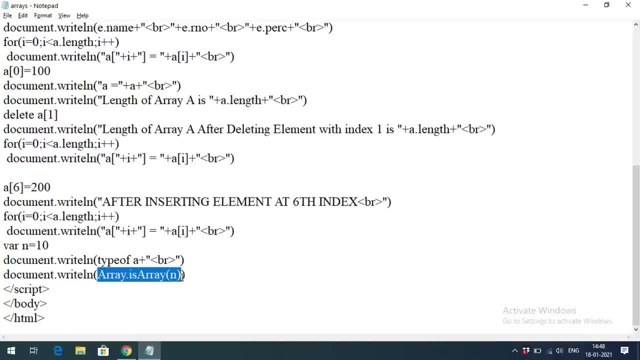 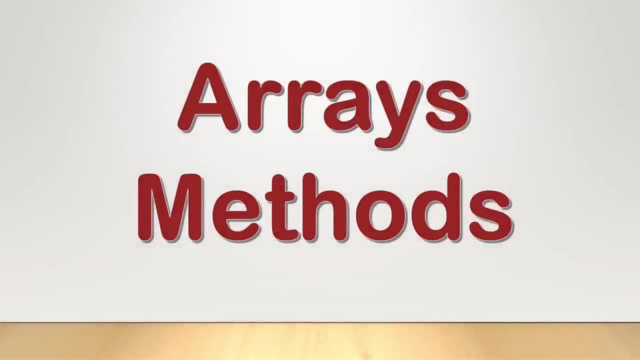 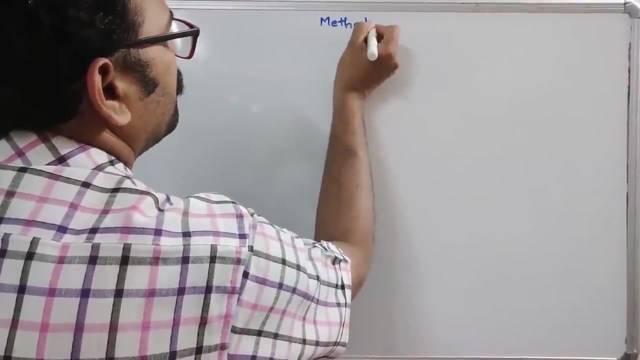 the array will be treated as an object. That is why we are supposed to use this function to check whether the variable is an array or not. So hope you understood this one. So in the previous session we have seen about the arrays, the introduction to arrays, How. 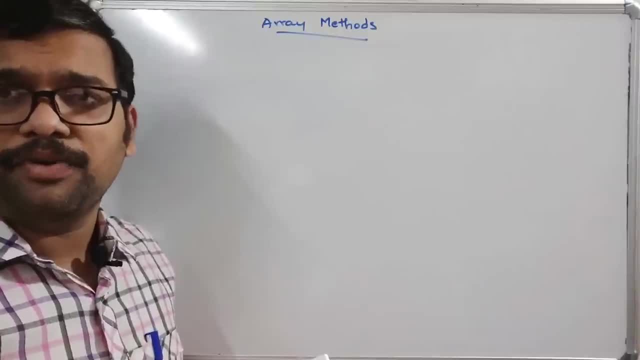 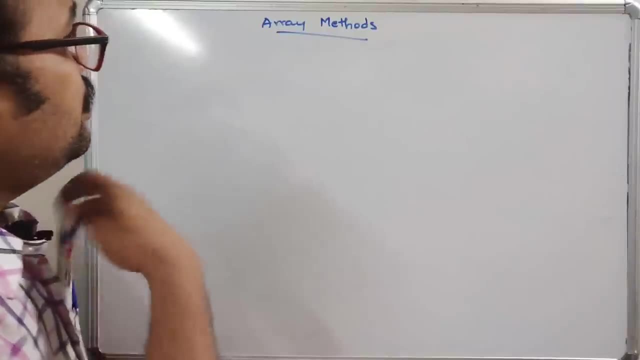 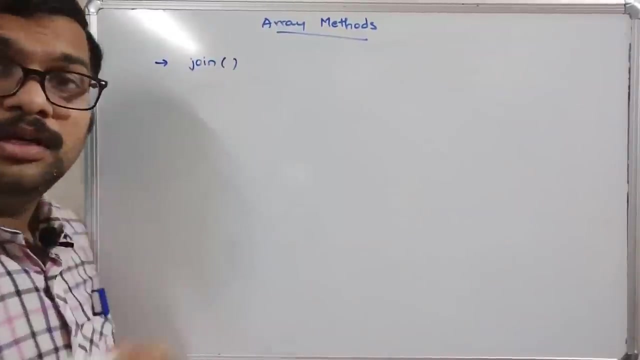 to create the arrayed in arrays and how to access the values of arrays right. So now in this session will see some methods available in arrays right. First one: it's at JOIN, JOIN JOIN function. So we know that a array consists of a multiple elements of different. 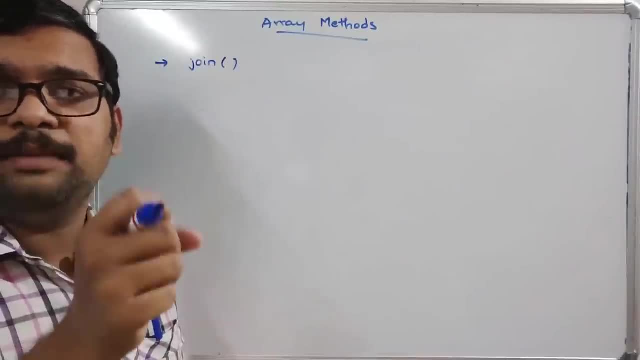 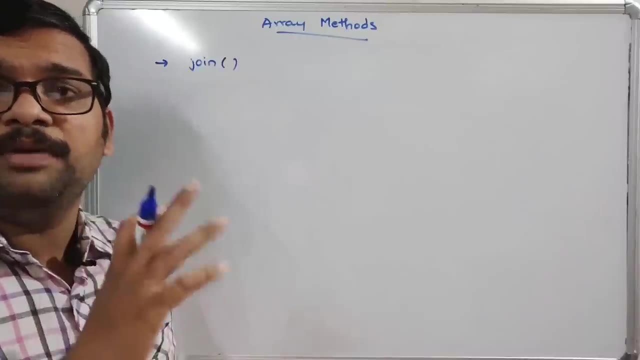 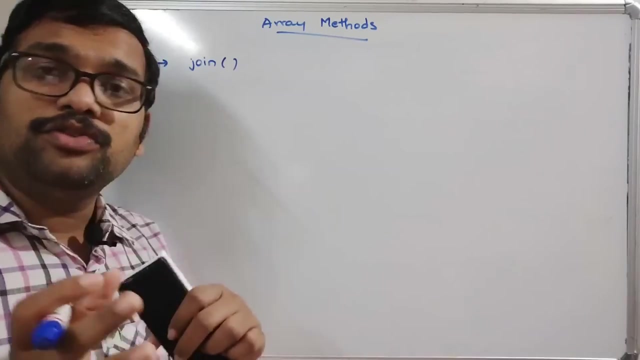 data types right under the same name, So we can join all those elements with some delimiter, So that delimiter should be given in this function. That means we have to give the delimiter as an argument to this function and that delimiter should be enclosed in double quotations So that the values of I mean 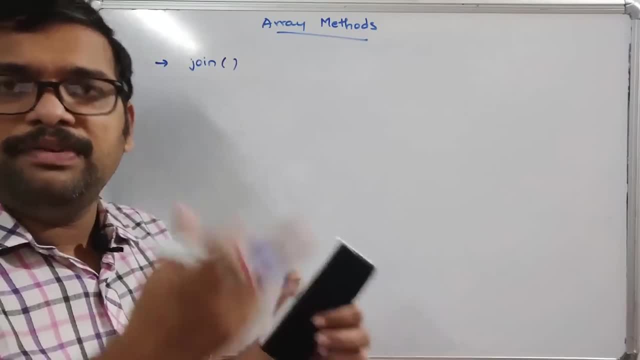 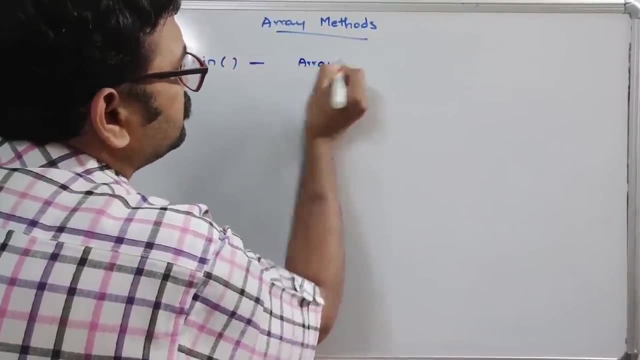 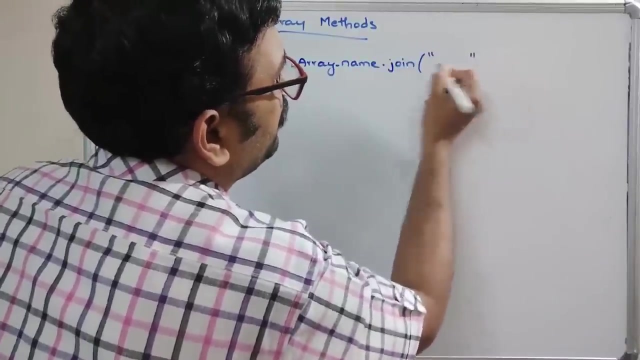 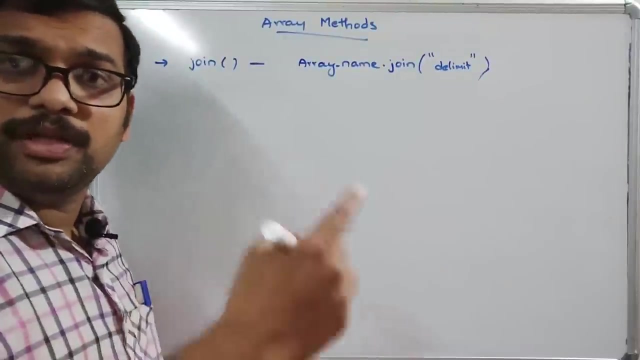 the values or elements of the array will be joined with the help of this delimiter. So the syntax is: array name, dot, join and give the delimiter here, Delimiter here. So if you give some space, all the elements will be printed with the help of space differentiating with the space. If you give. 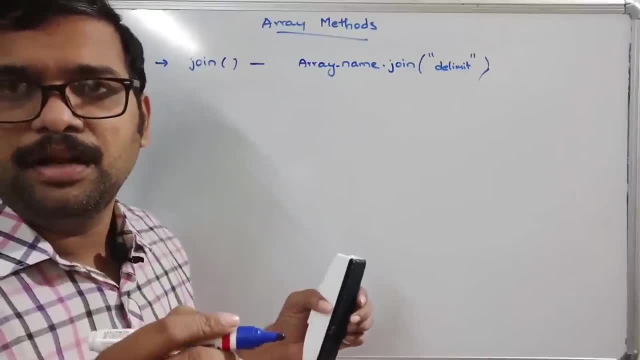 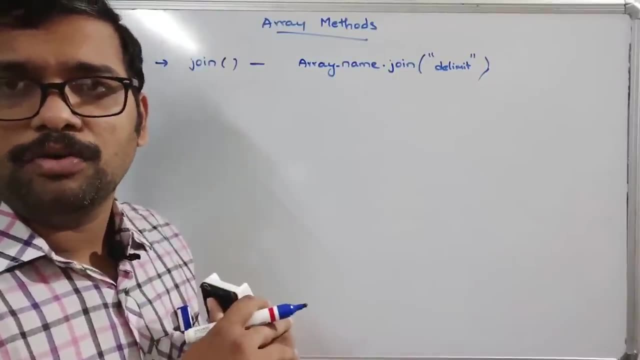 some hyphen, all the elements will be differentiated with the hyphen symbol. So I will show you the syntax here and I will show you the syntax here. So I will show you the syntax here and I will demonstrate all these methods by executing a small code. So this is a syntax for join. So with 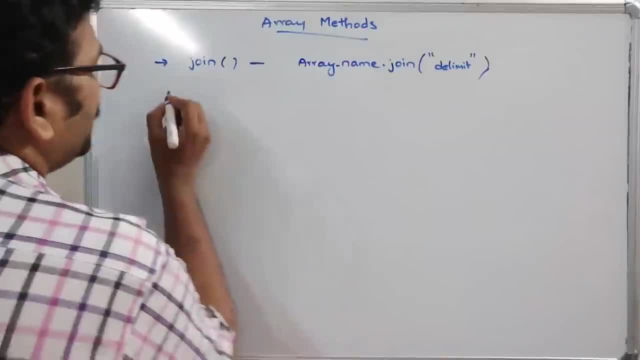 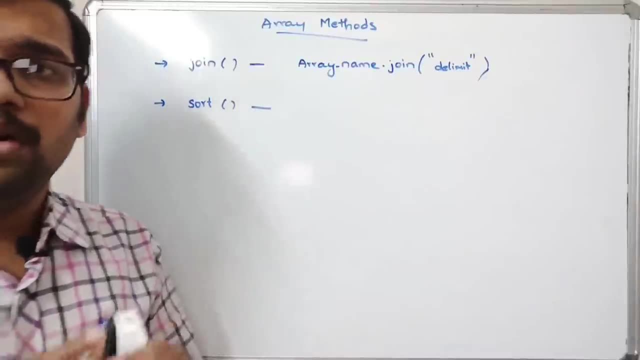 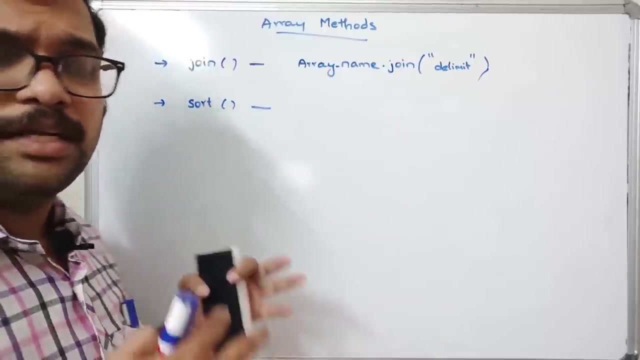 the help of this delimiter, the elements will be joined. Next sort is used to arrange all the elements in a sorting order. That means from lower value to higher value, as any order, And this particularly works on the character arrays. So if the array consists of all the strings, 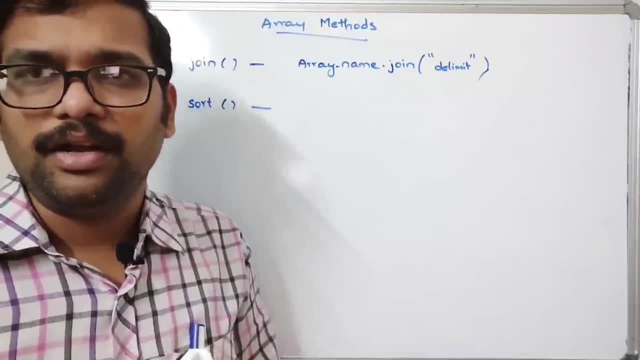 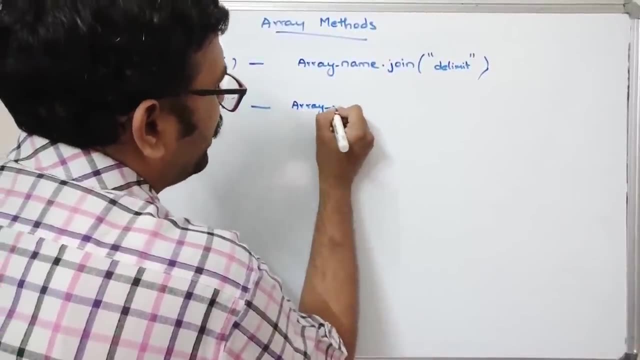 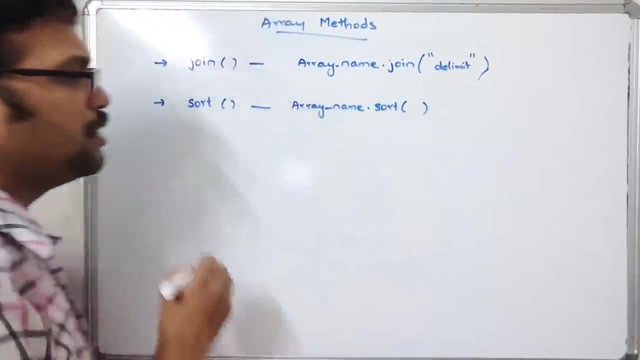 then all the strings will be sorted in alphabetical order. So the syntax for this one is the same thing: Array underscore name. So whatever the array, we are taking that array name dot sort function. Similarly, there is one more function called reverse, So this can be applied in any. 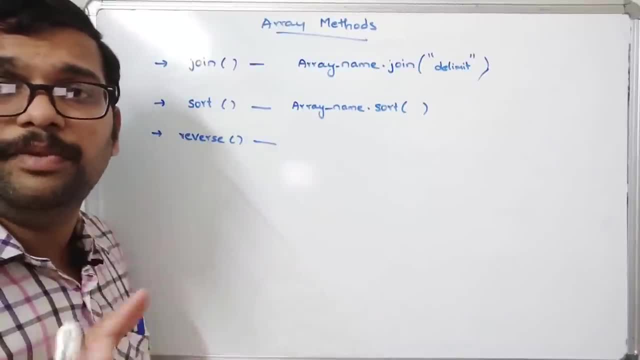 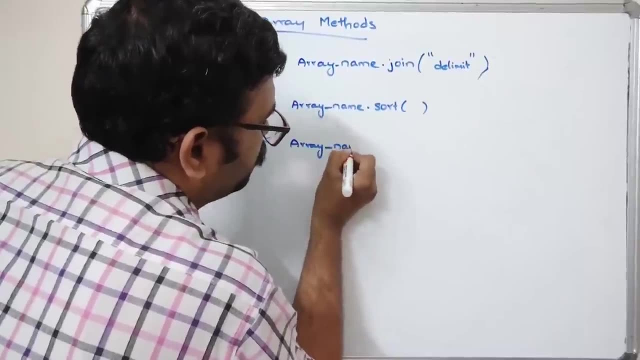 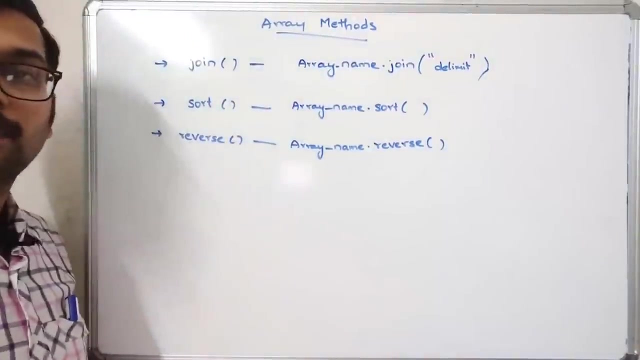 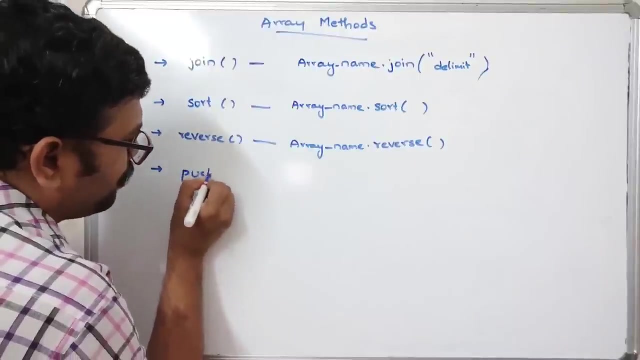 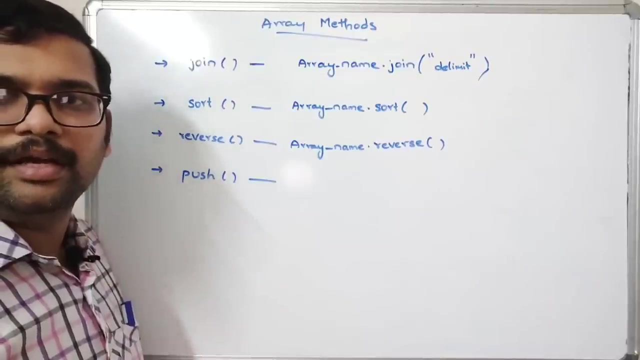 kind of array. So, as the name it self-indicates, the elements will be arranged in reverse order. Okay, So the syntax is: array, underscore name dot reverse. Okay So, array- name dot reverse. And the next function is push function. So this push function will insert the element. Okay, It will insert the. 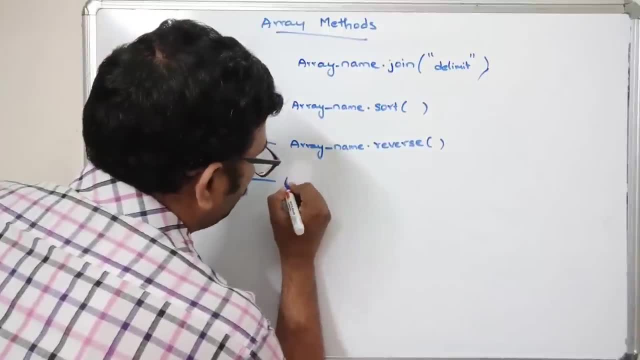 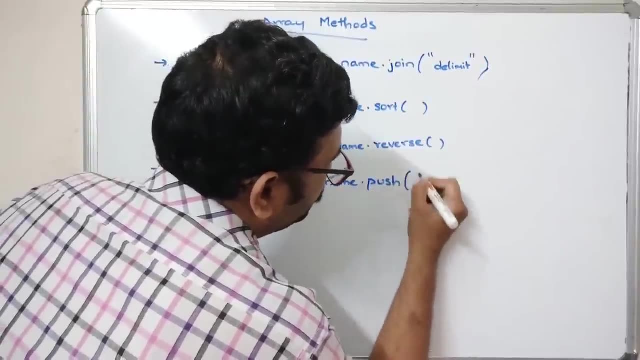 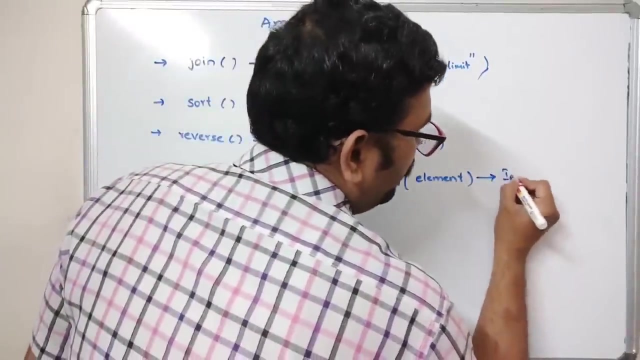 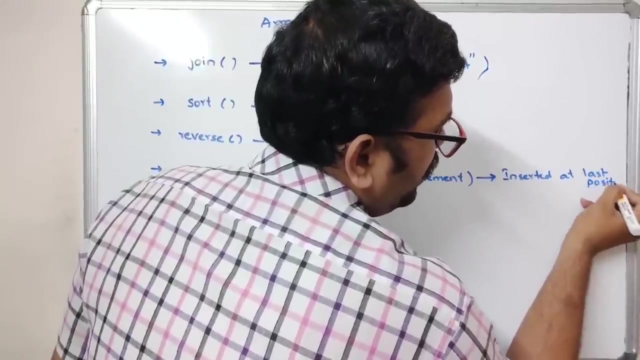 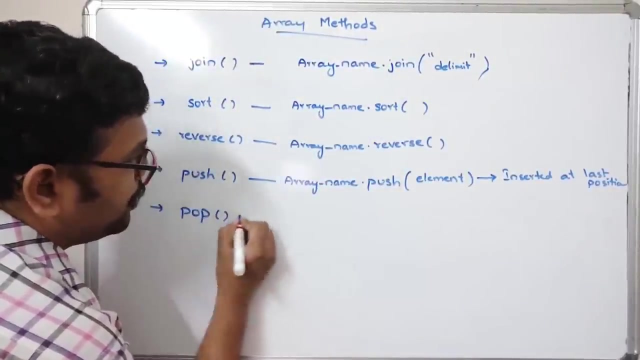 element at the last position. So here the syntax is: array name, dot push, give the element here. So we need to pass the element as an argument So that it will be inserted at last position, At last position Right. Similarly, there is a function called pop function, So here the syntax is: 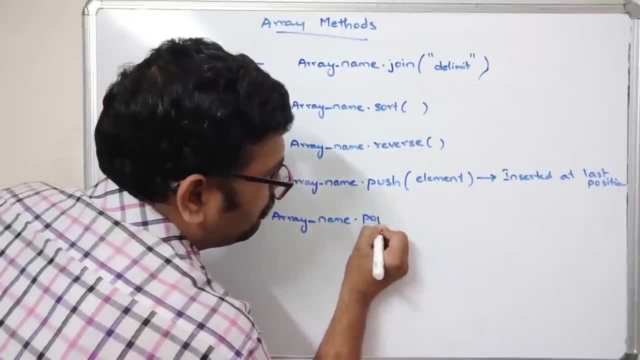 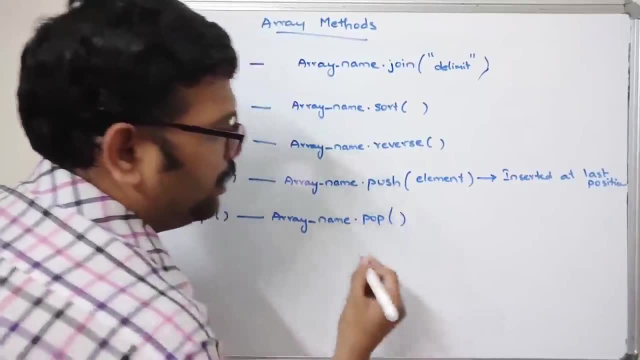 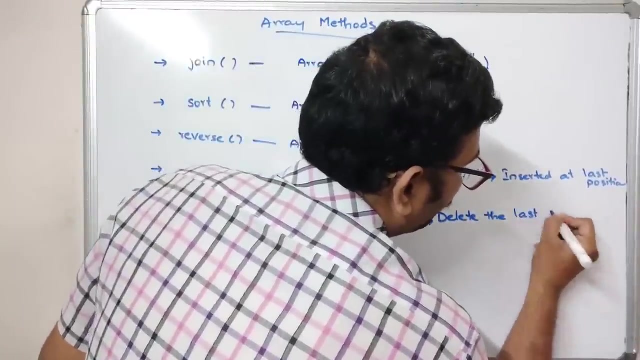 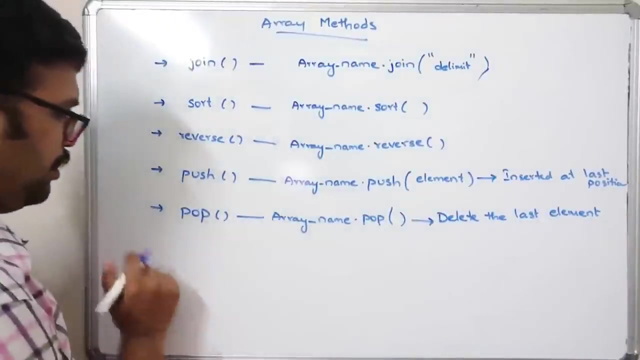 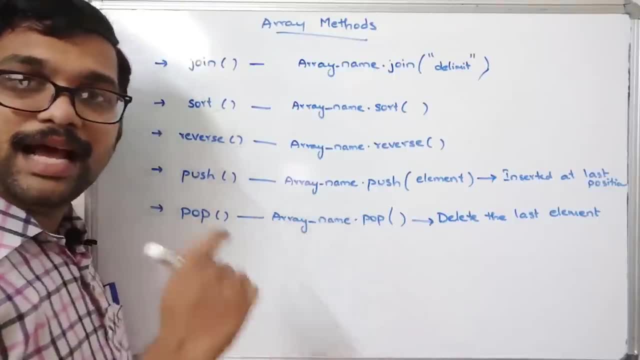 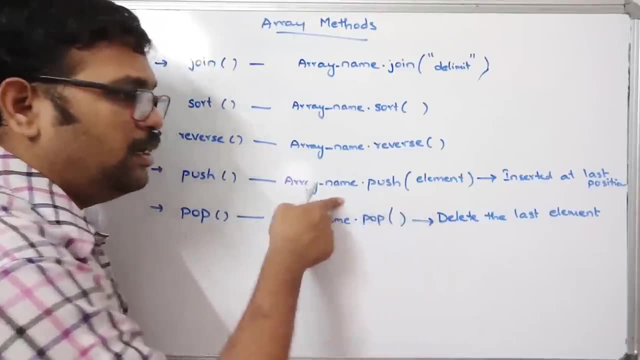 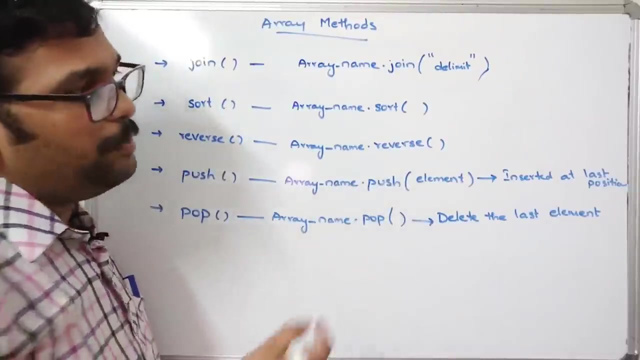 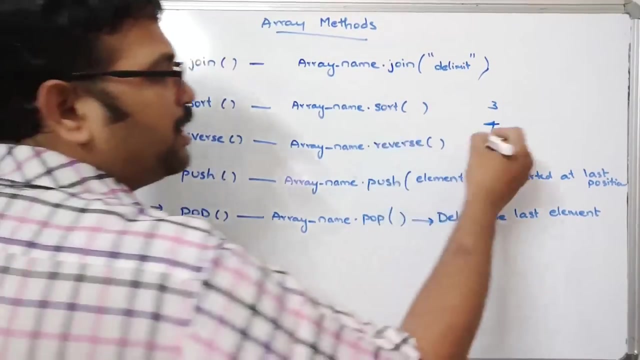 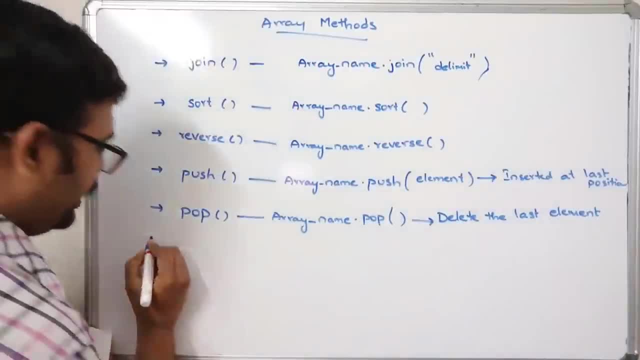 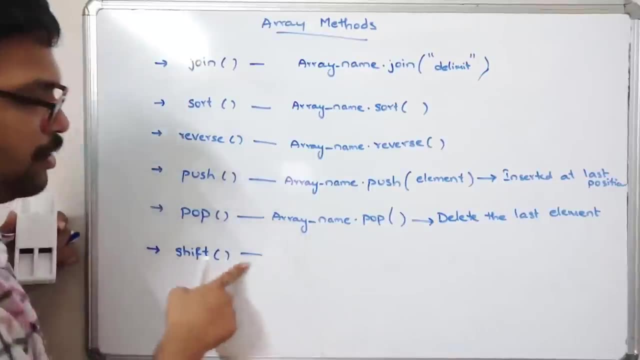 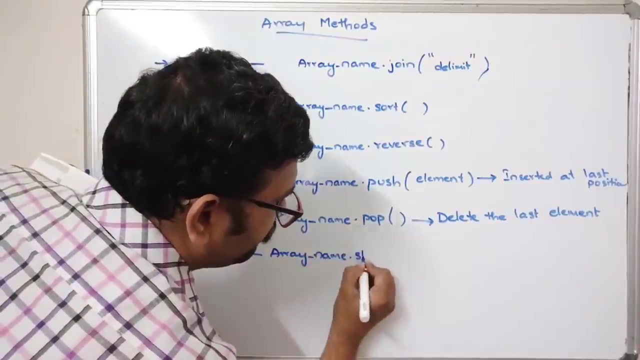 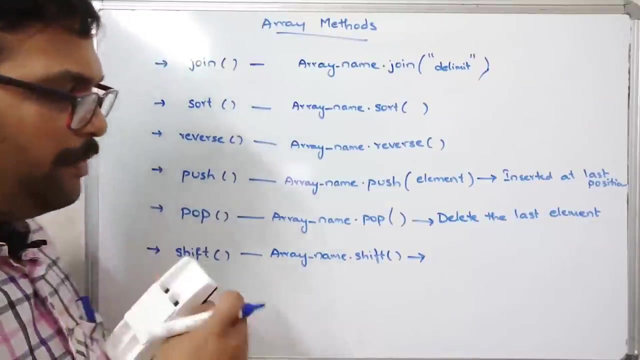 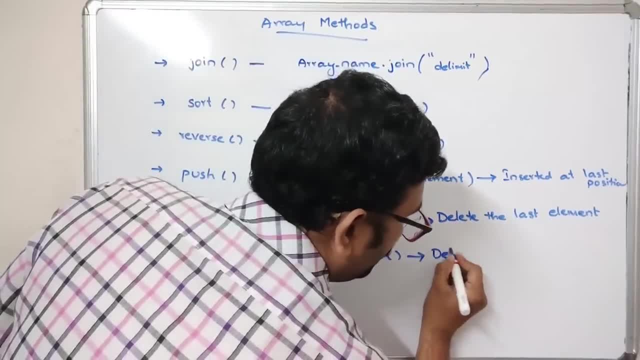 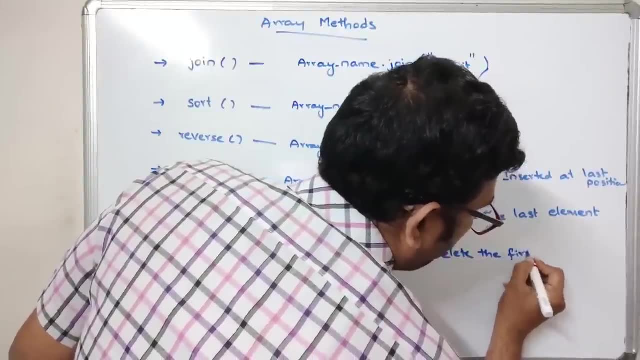 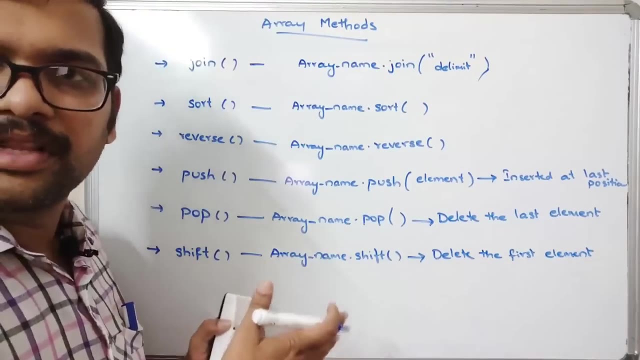 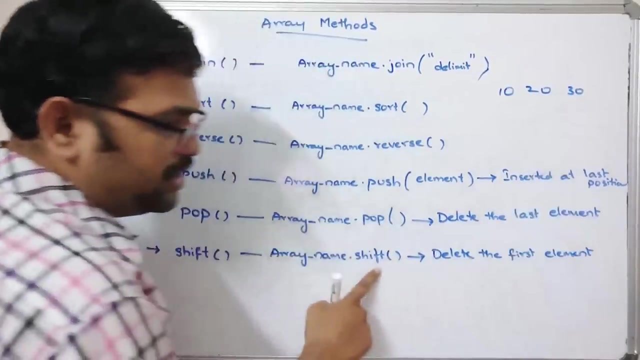 element from the starting position. so here it will delete from the last element. here the delete the element, the first element. it will delete the first element and all the remaining elements will be moved towards its left. that means it will occupy the lower indexes. for example, there are three values, so if you apply the shift operation, the 10 will be removed. 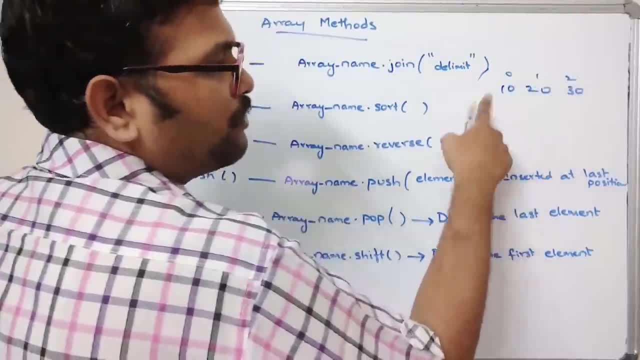 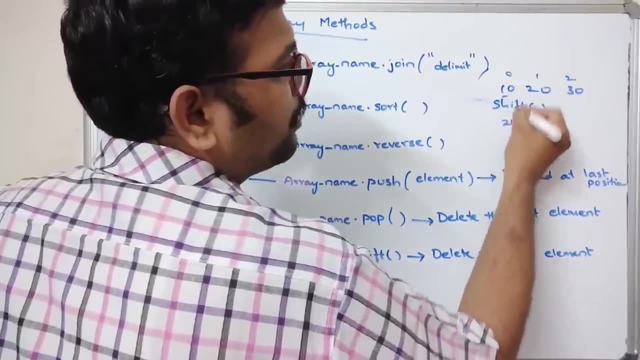 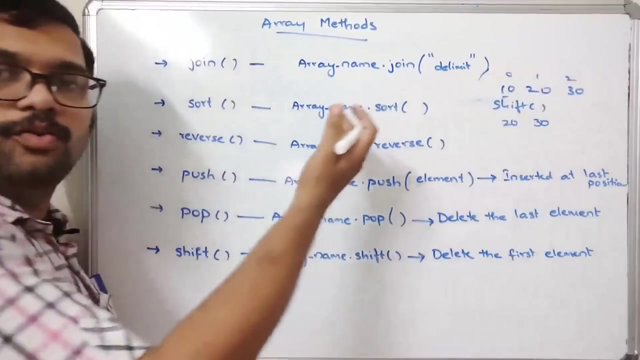 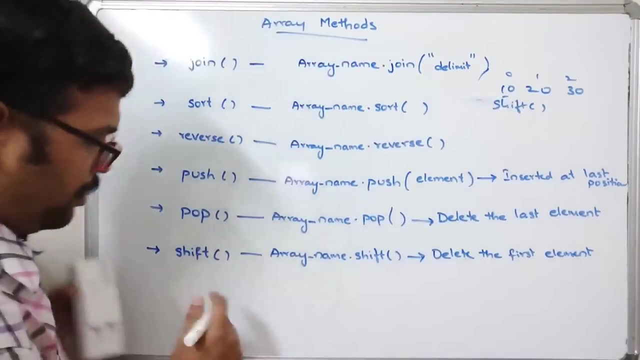 ok, initially 0, 1, 2. now after shift operation. ok, after shift operation, 10 will be removed, 20 will comes at the index 0 and 30 will come at index 1. so the elements will also be shifted towards its left position. that means lower index values, right and next one. so shift is. 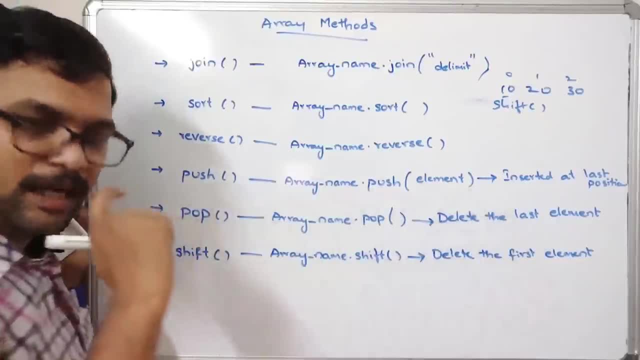 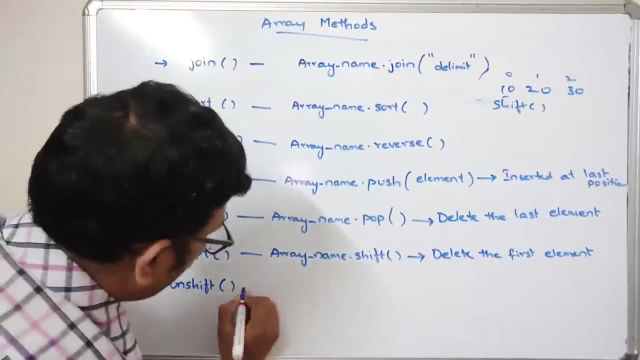 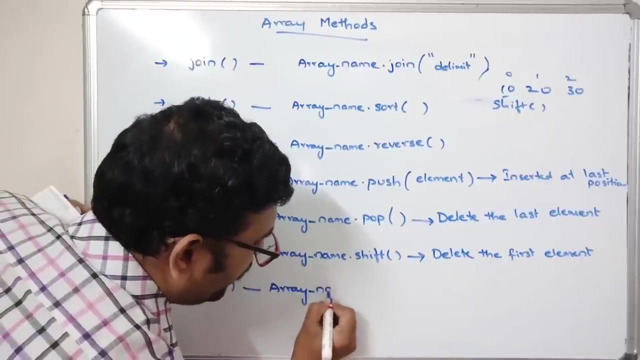 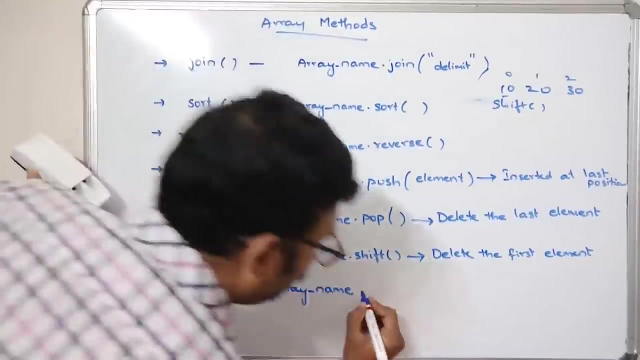 to delete the first element. pop is to delete the left position. Ok, last element. and there is a one more function called unshift, unshift, right. so unshift function. the syntax is array name. so whatever the array name we are giving- some a or s or array or whatever the name we are giving that array name, dot unshift. 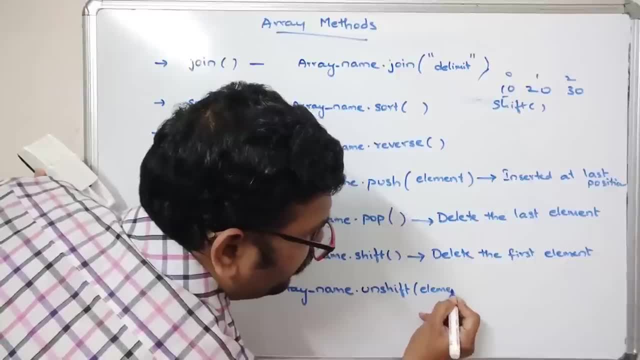 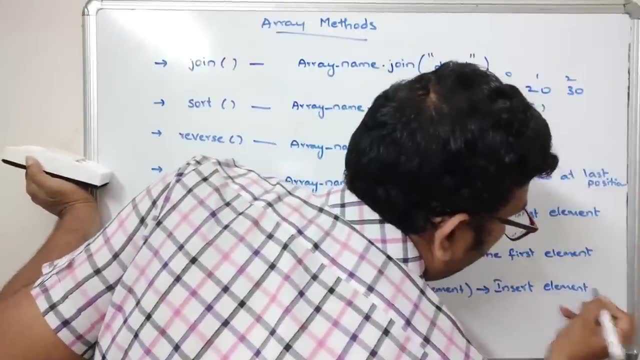 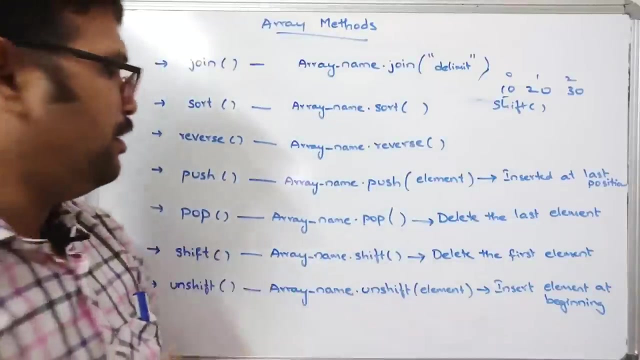 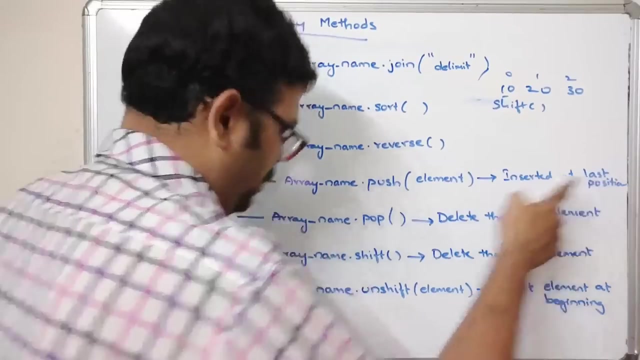 unshift, give the element here, give the element here. so this will insert element, yet beginning: insert the element at beginning. so if you use the push operation, if you use the push operation, the element will be inserted at the last position. if you use the unshift operation, the element will be inserted at the beginning. 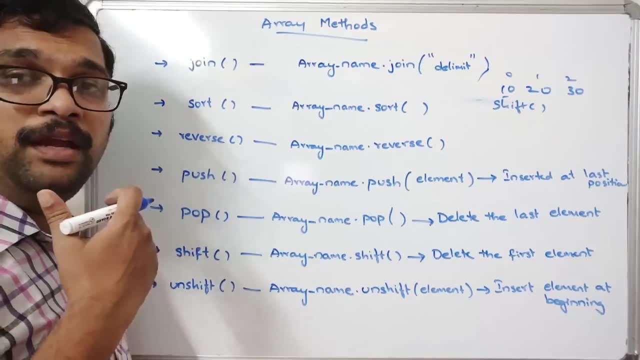 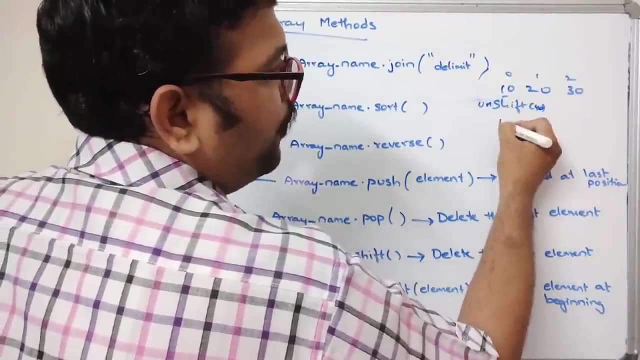 and automatically the element will be inserted at the last position and automatically the elements will be moving rightwards. so for example, if you go with the unshift some 40, then 40 will be occupying at first position. that is 0, so 10 will be moving to 1. 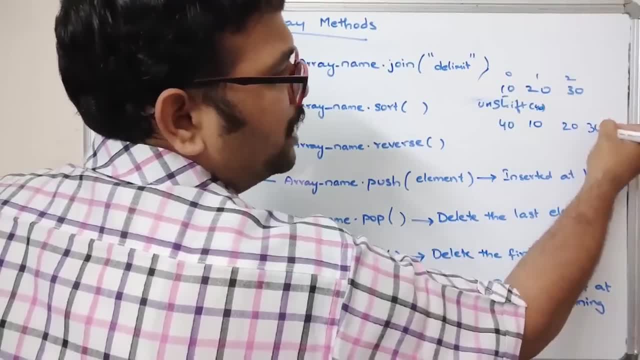 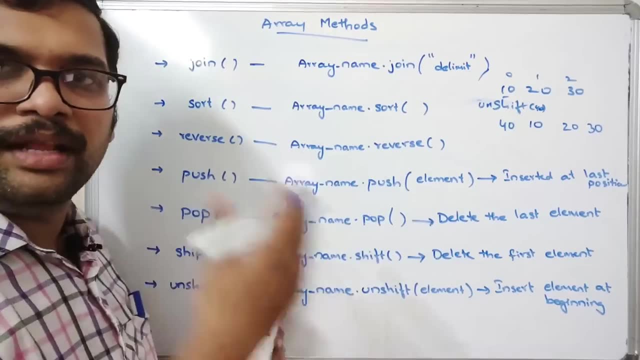 20 will be moving to 2 and 30 will be moving to 3. right, so the elements will be moving towards its right side. okay, it will increase the total length of the element and it will be moving right side. so that is for unshift, unshift. 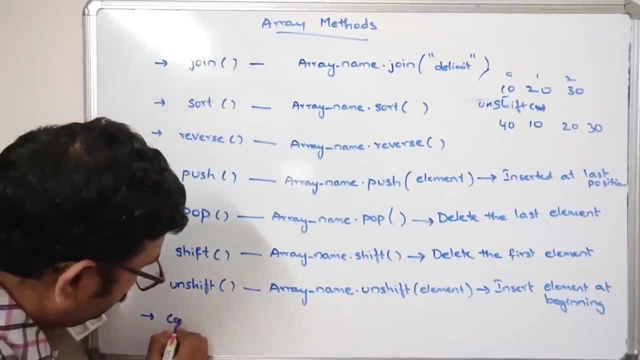 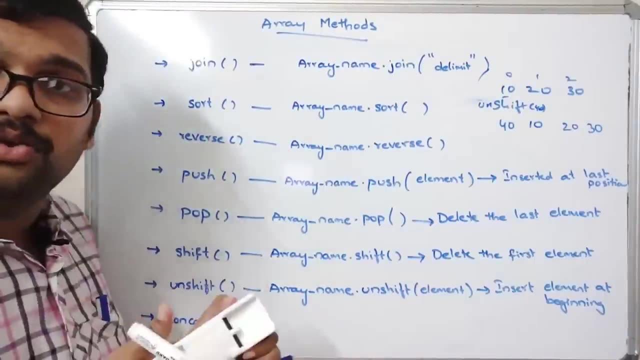 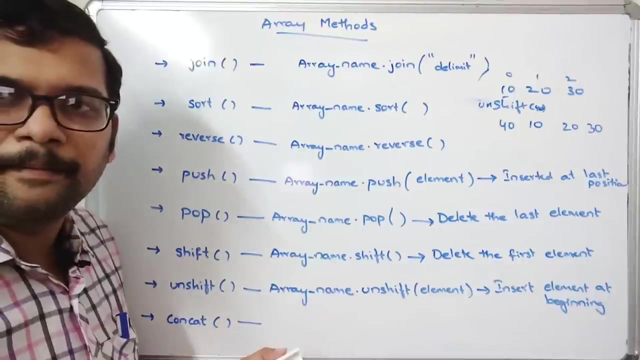 and then, and then concat function, concat function. so this concat function is used to concat two different arrays. not only the two different arrays, so we can also concat the element to the existing array. okay, so not only the, it's not restricted to two arrays, we can also concat three arrays. 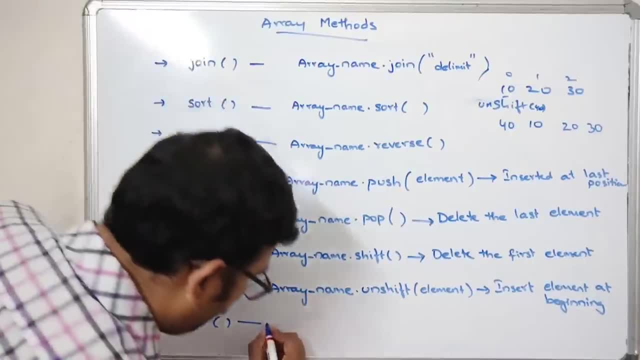 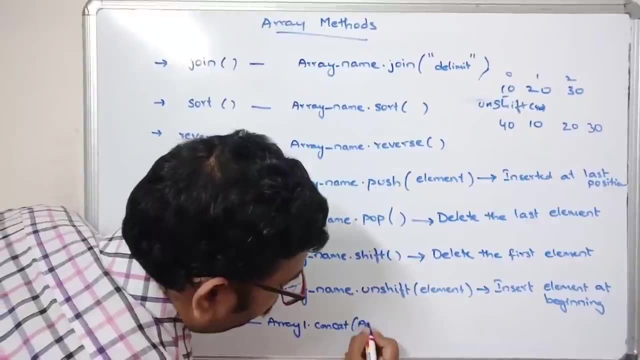 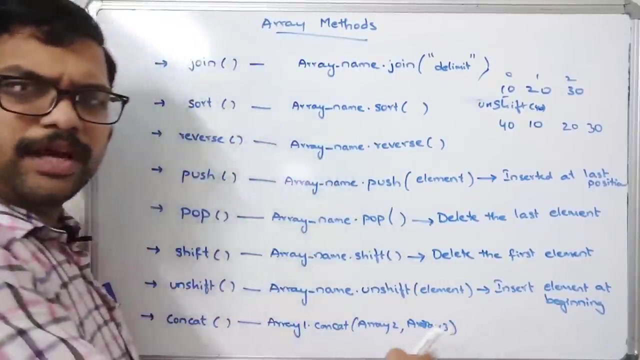 we can also concat four arrays, right. so here, here and, and here we have the entire array name: Array 1, dot. concat. array 2, comma: array 3.. Ok, So on, we can. we can concat any number of arrays. Ok, It will merge. 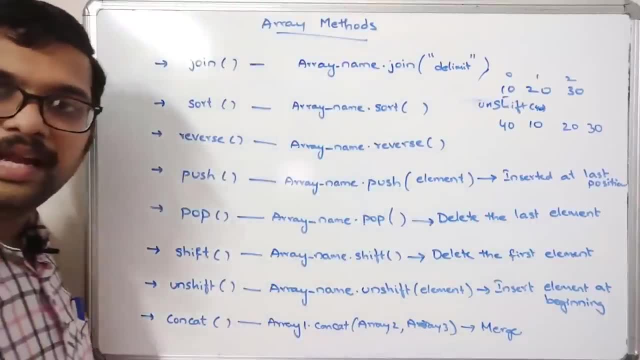 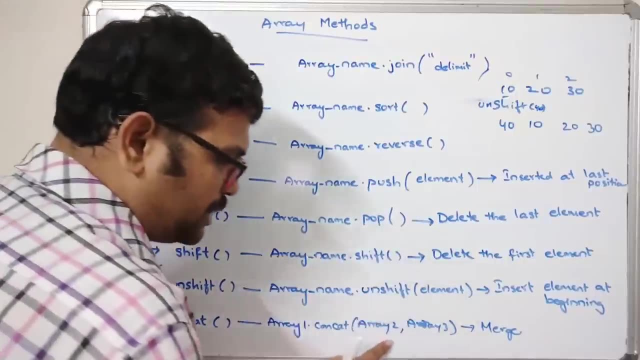 Simply, we can call it as a merge, Merging of array elements. So here, instead of using the array, we can also use the elements. So whatever the elements you have passed as an argument to this concatenation operation, those elements will be concatenated to the this array. 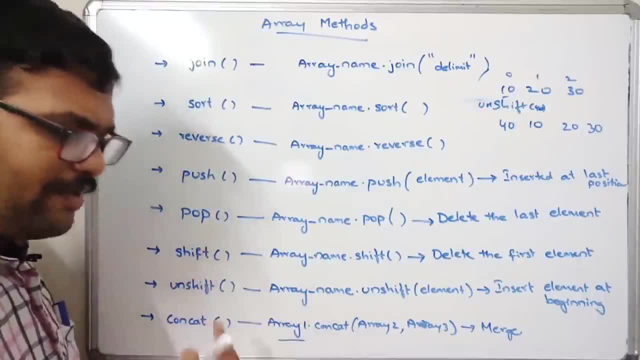 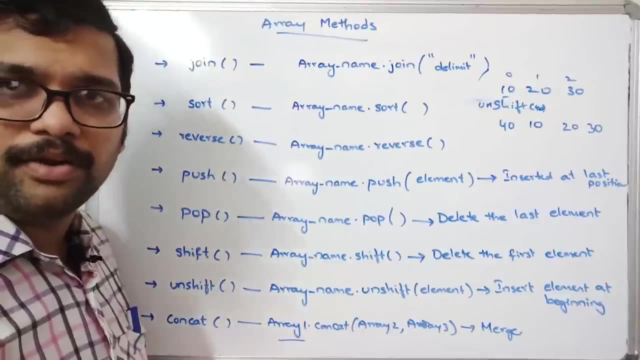 Ok, Hope you understood. So if you are still having any doubts, just wait for a while. I will show you execution of all these functions so that your diets will be clarified. Ok, Right, So this is about the concatenation function. 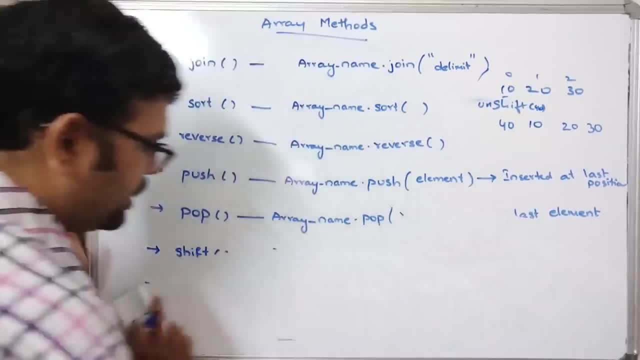 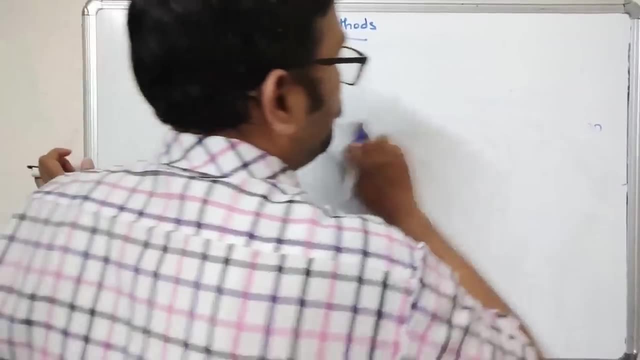 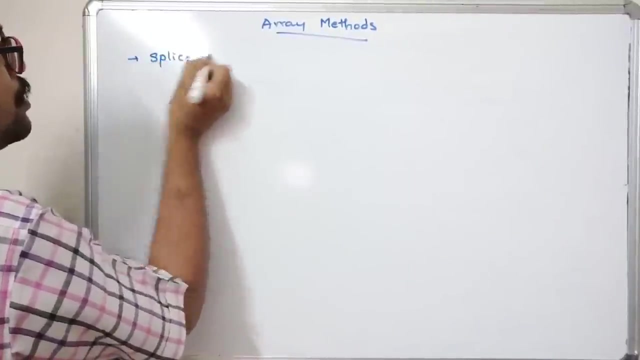 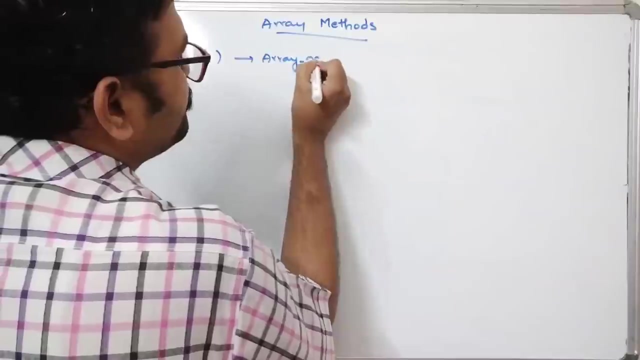 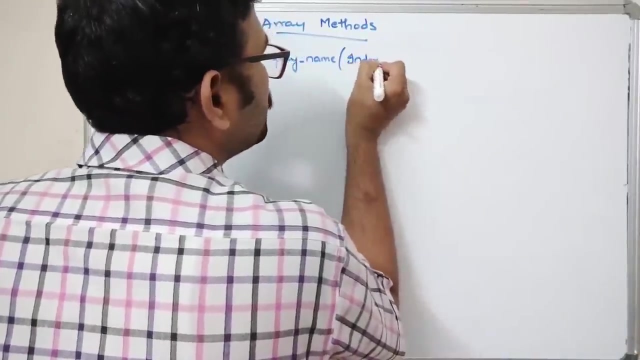 And there are two more functions available, that is, a splice and slice, Splice, slice, Splice function. So this splice function will take three arguments. Three arguments: The first argument is index, starting index, where we have to insert, and the second one is: 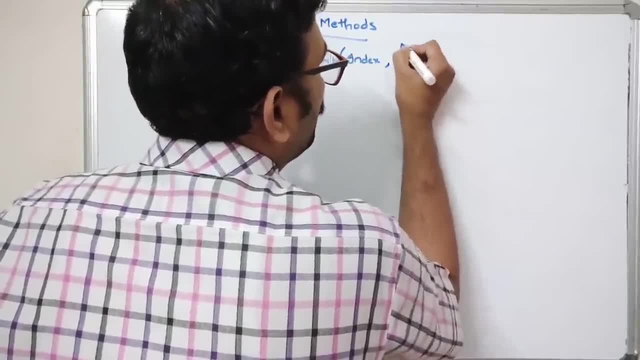 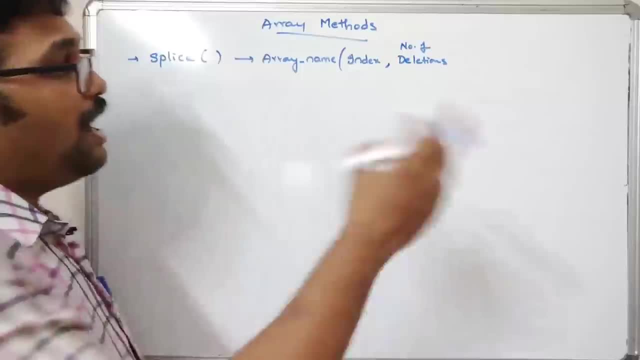 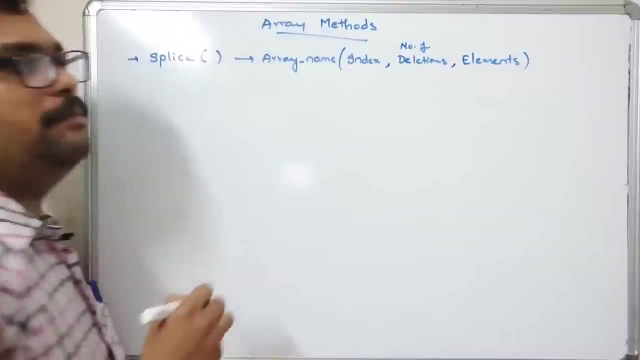 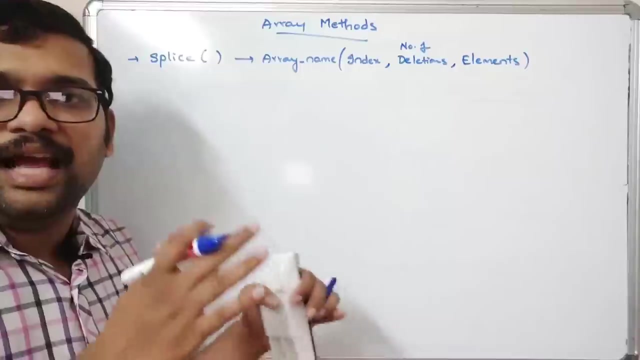 number of data, Number of data Deletions, Number of deletions: How many elements should be deleted after inserting this one? And the third one is elements Elements. So, whatever the elements we need to insert, So this splice operation can be used for both insertion as well as the deletion. 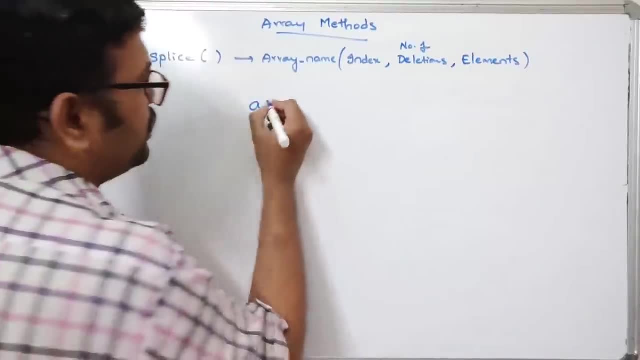 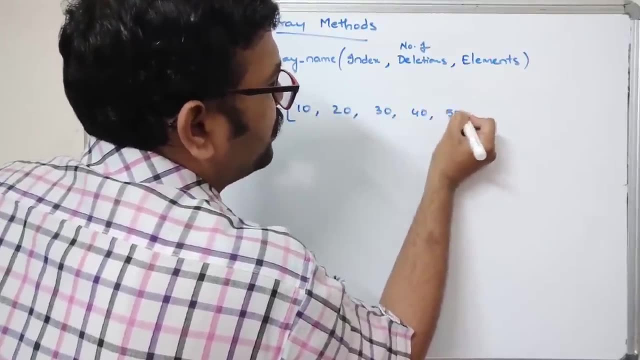 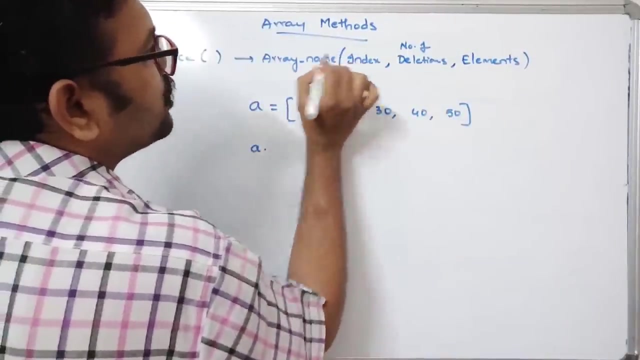 So if you go with some, I will show you the example so that you will be understand. So some a is equal to 10,, 20,, 30,, 40. And a 50. Let us take this one. So here, yeah, aarranamesplice here. I have forgotten to write this splice. 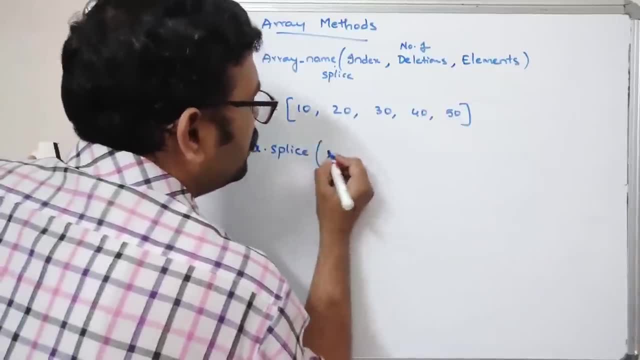 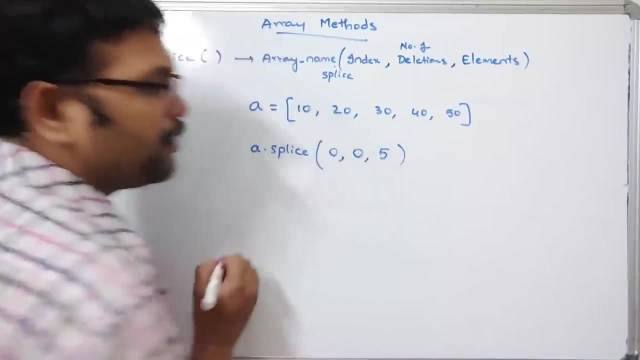 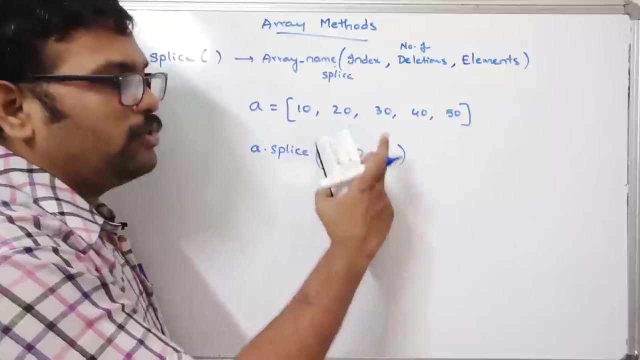 So asplice of, I will give some 0. ok, 0, I will give 5. right, So this means the starting index is 0 and we should not delete any elements and we have to insert the 50. 5th element. 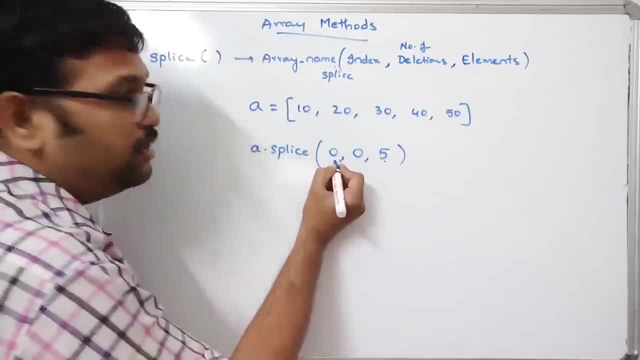 5. Element 5. So 5 should be inserted at index 0. So the result will be: The result will be 5, because 0th element means here 0th index. So you can observe here: 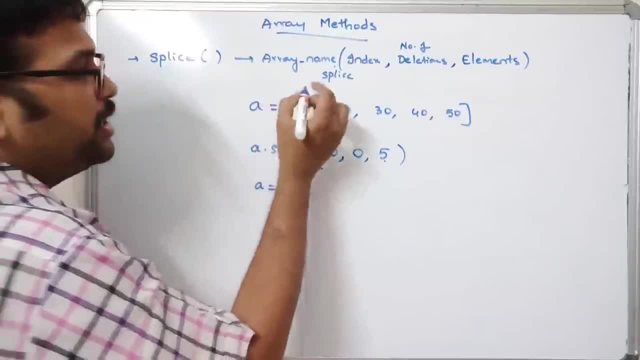 0,, 1,, 2,, 3 and 4.. These are the index values, So 5,, 10,, 20,, 30,, 40 and a 50. See once again I am writing the splice. 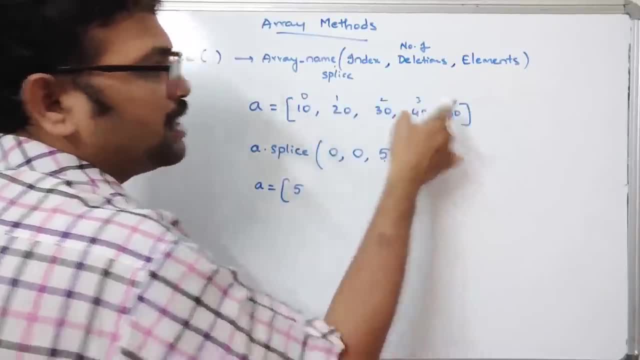 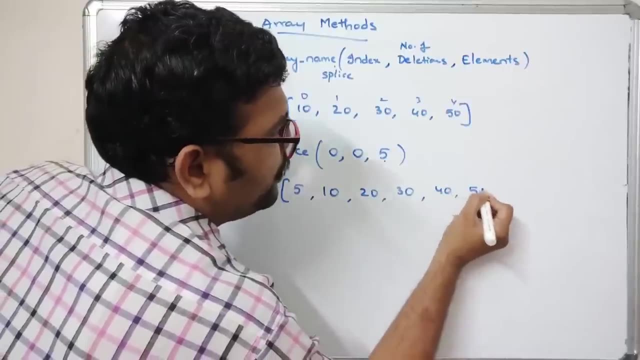 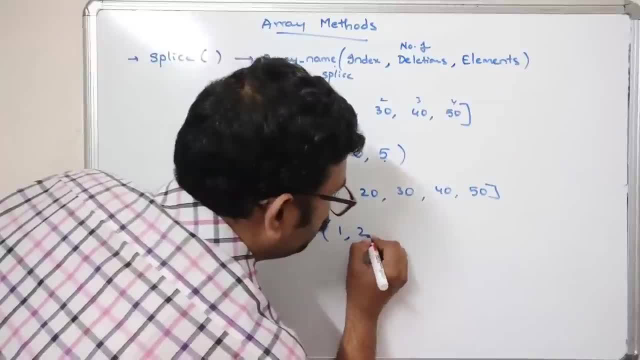 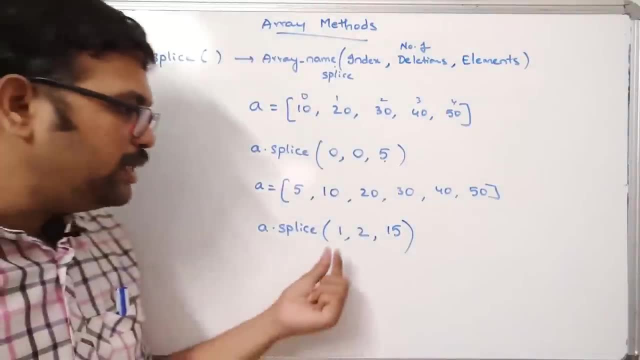 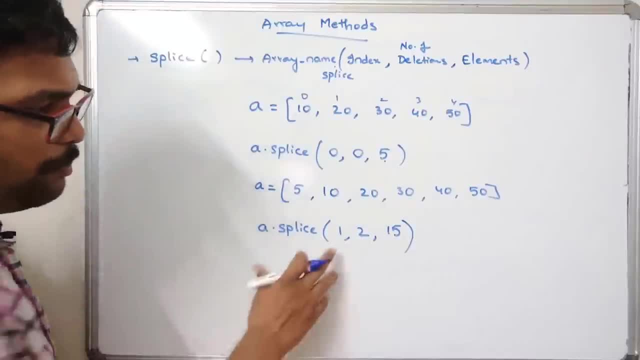 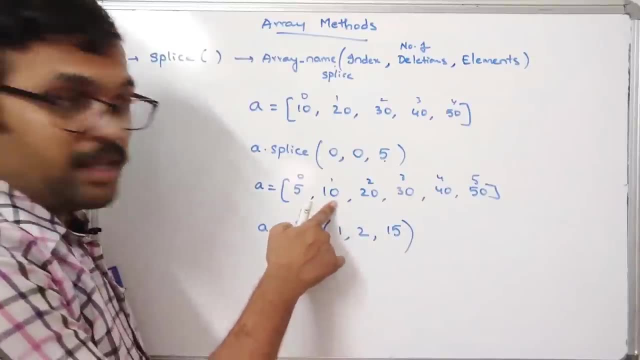 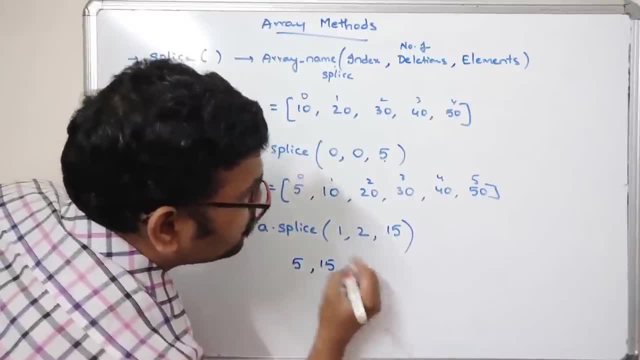 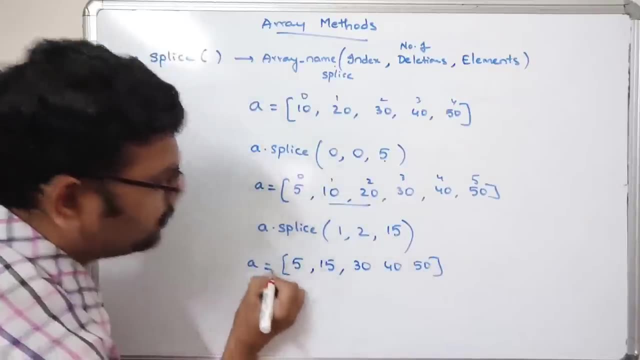 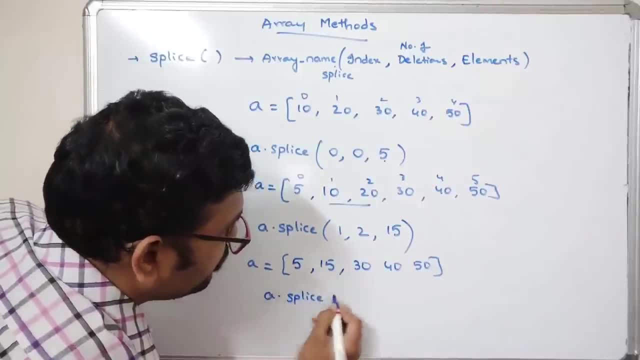 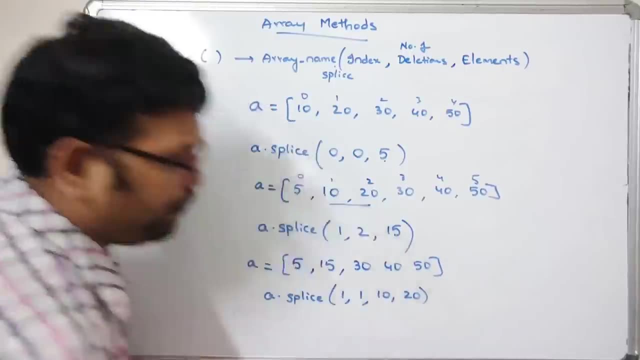 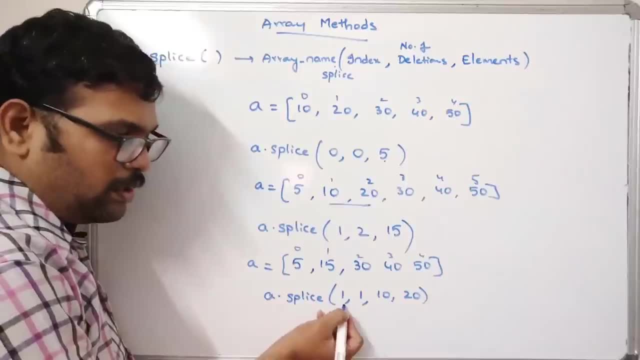 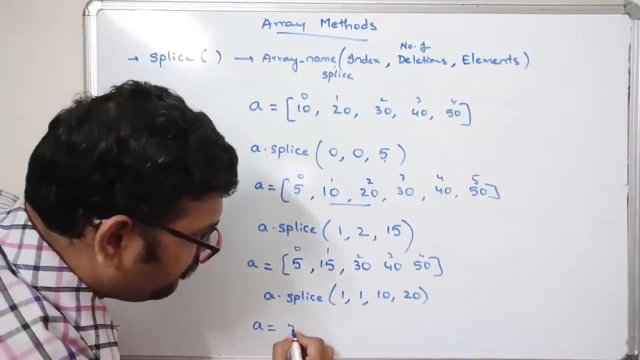 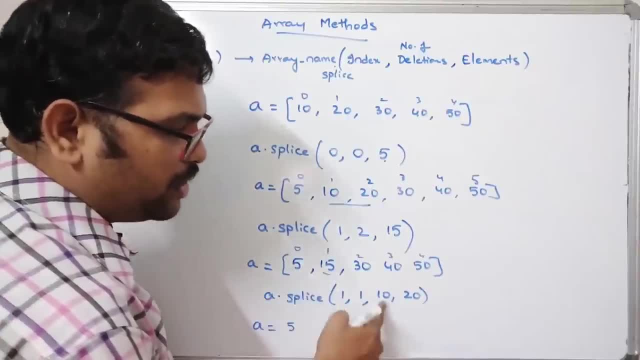 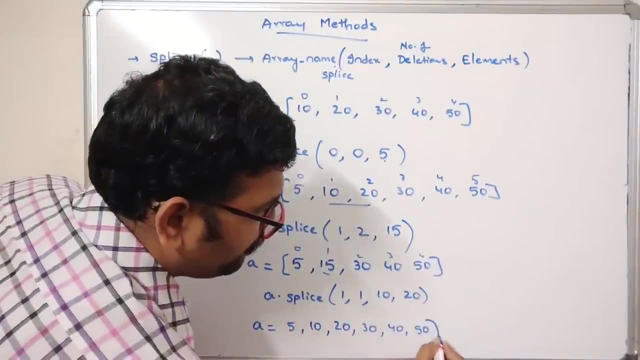 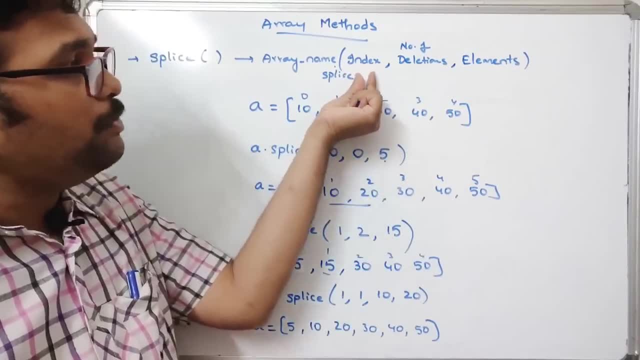 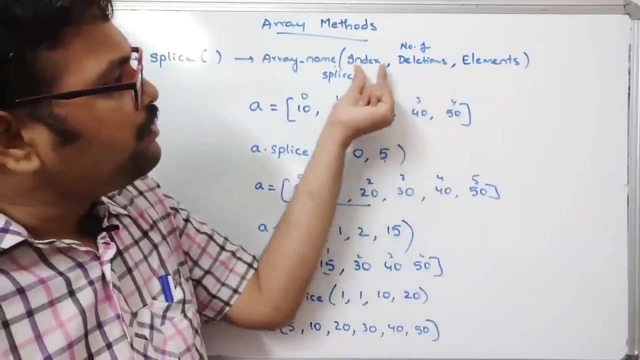 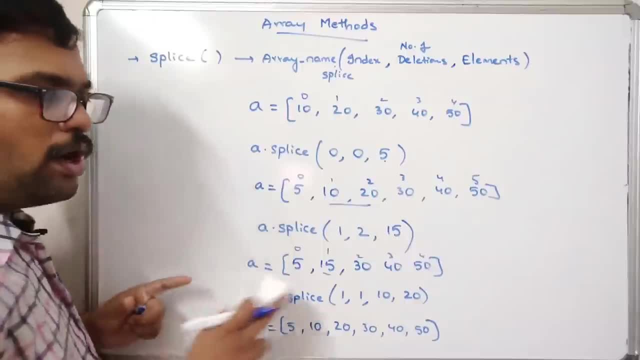 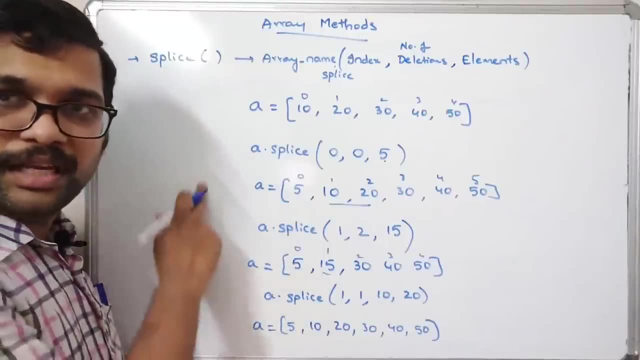 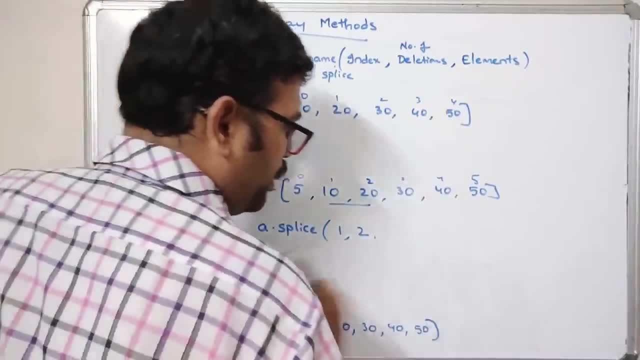 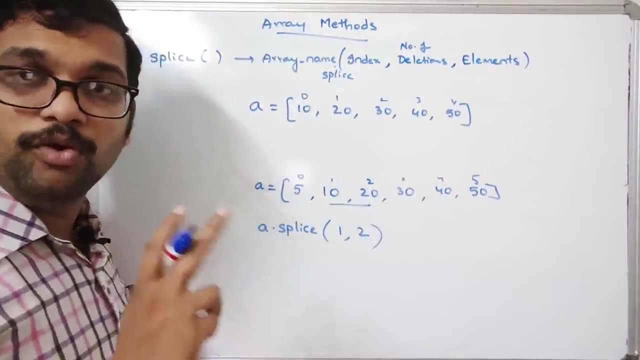 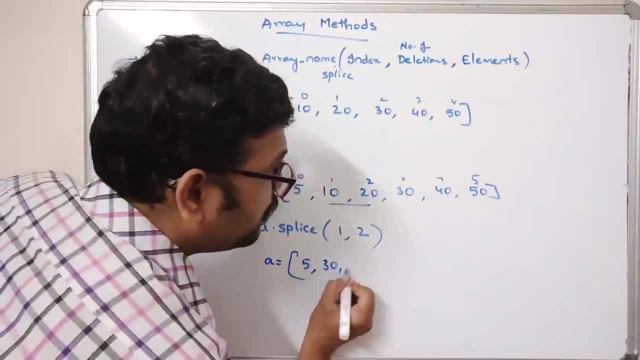 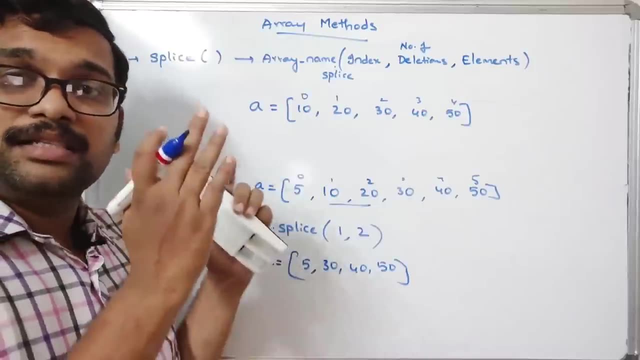 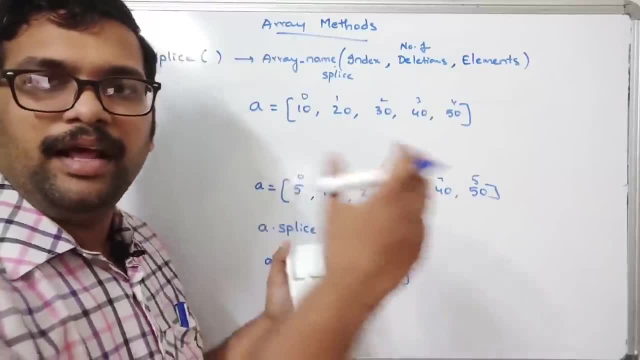 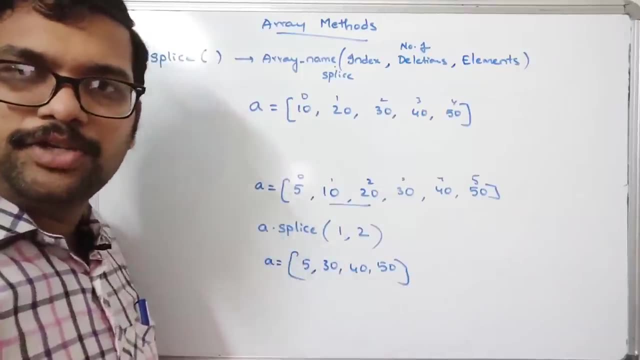 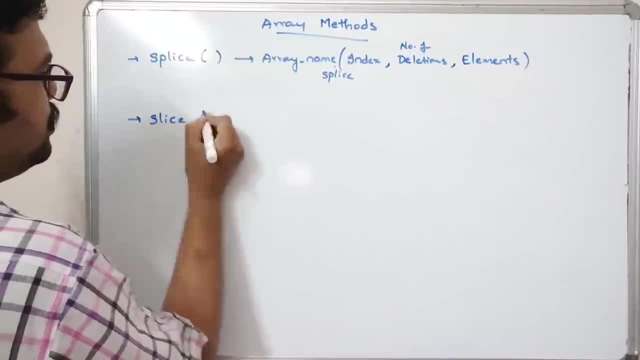 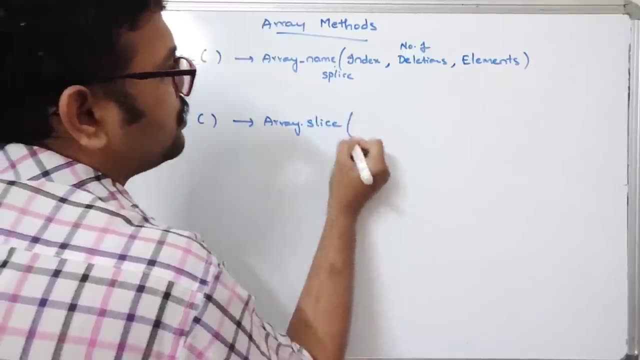 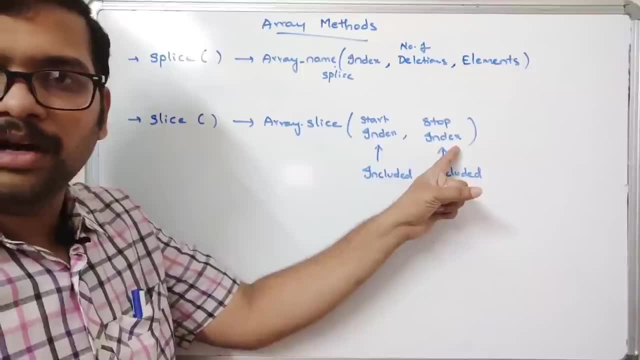 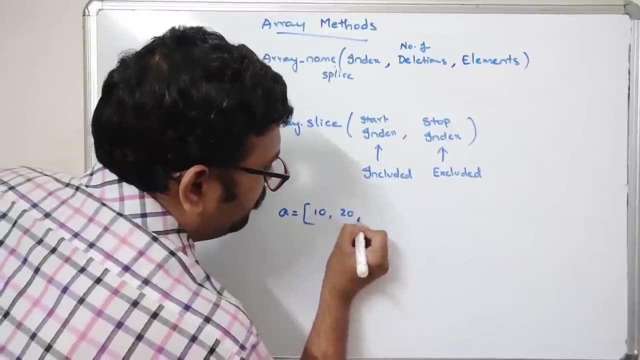 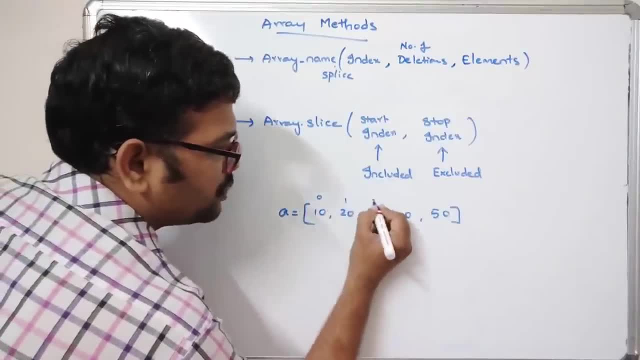 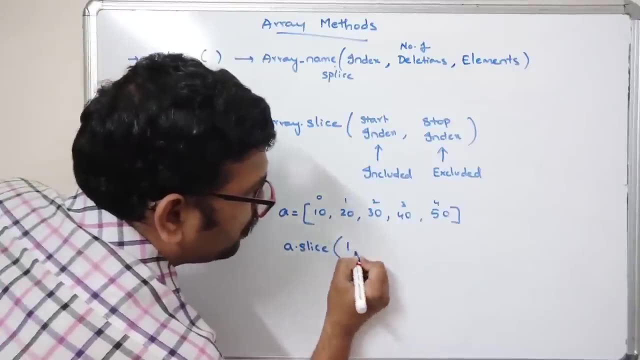 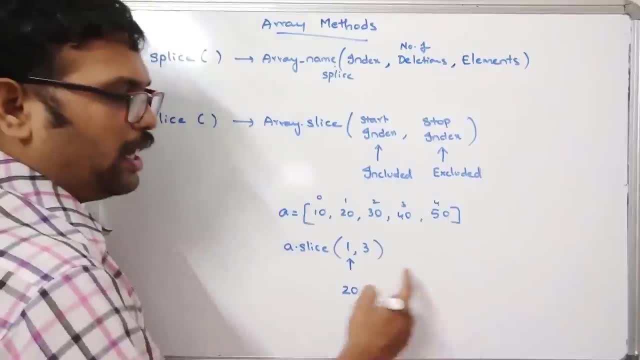 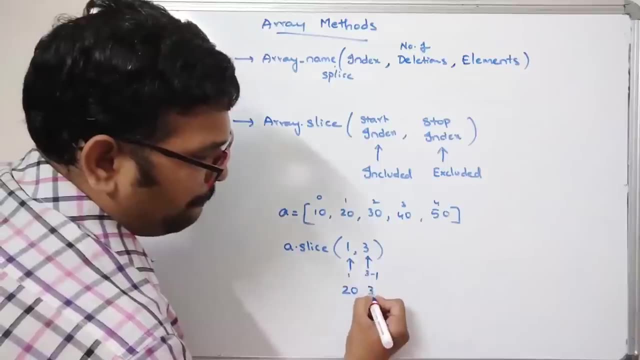 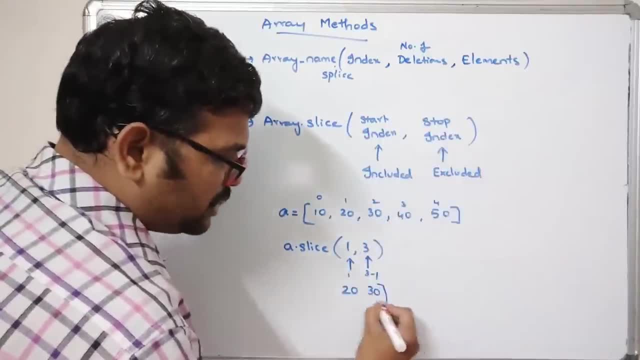 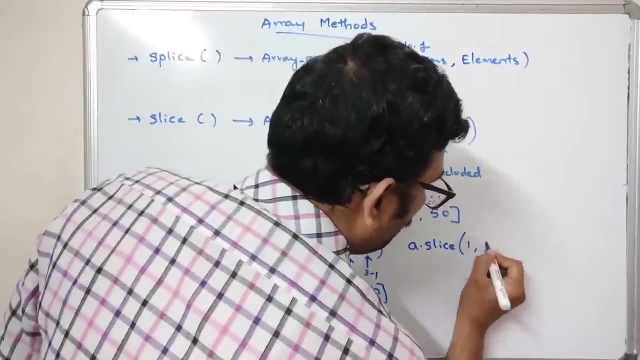 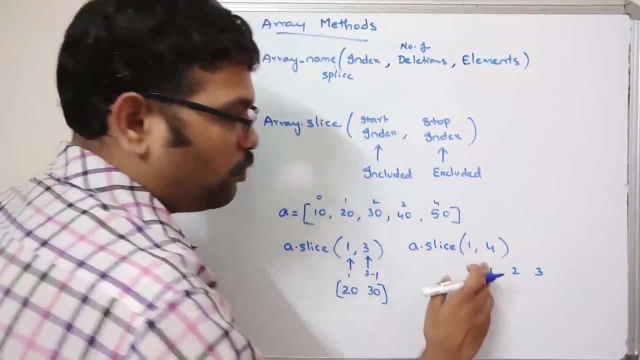 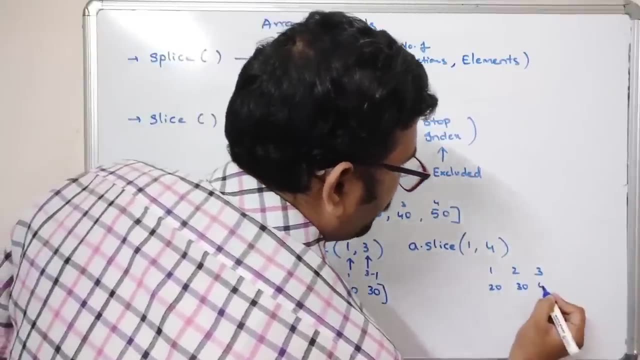 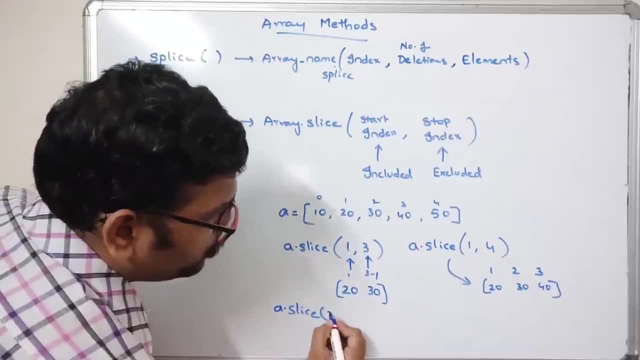 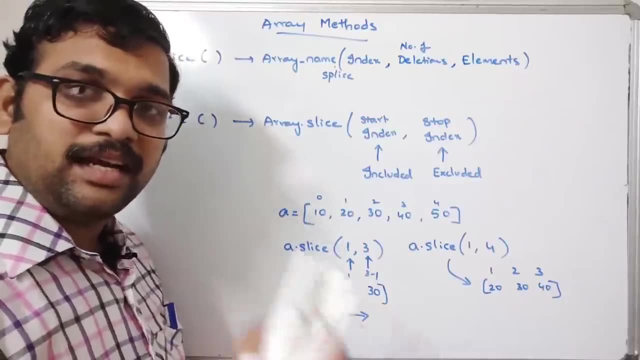 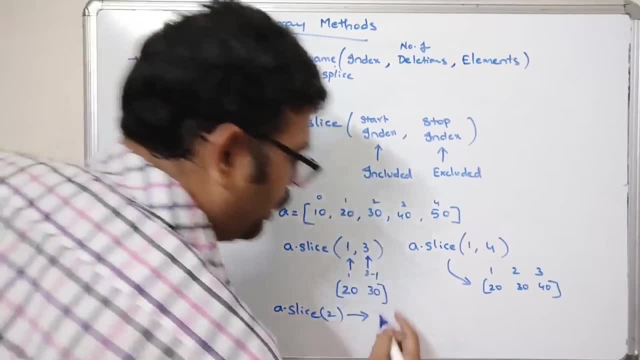 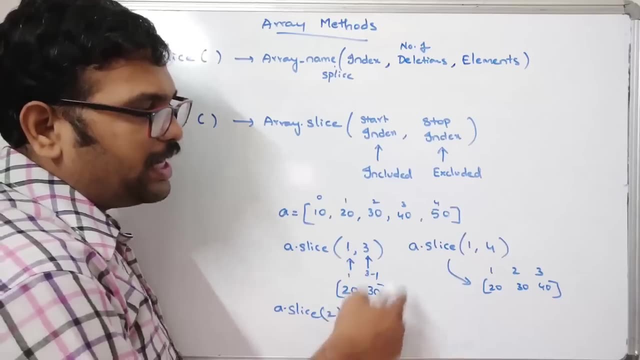 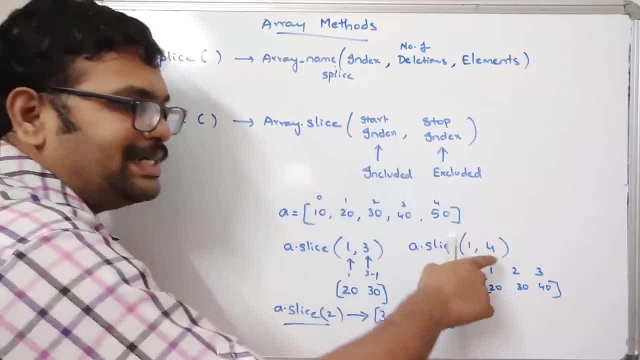 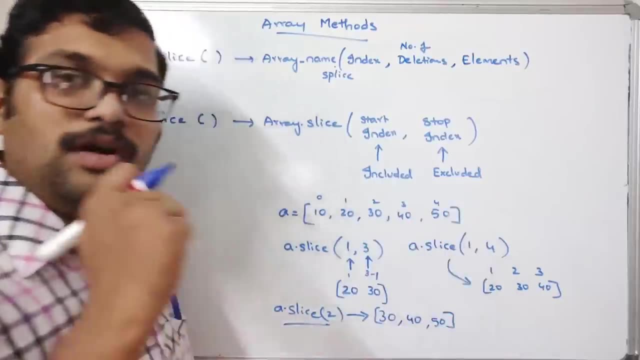 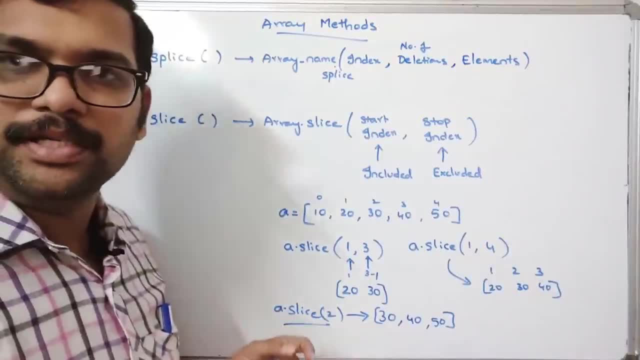 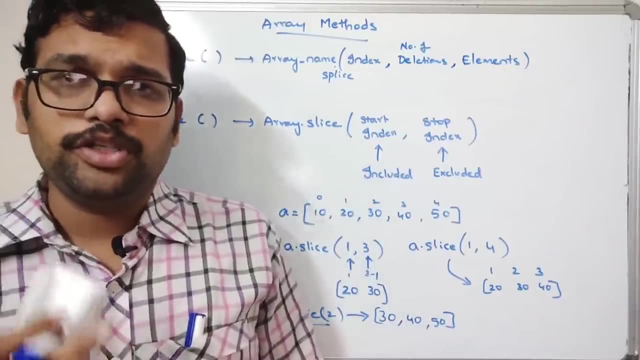 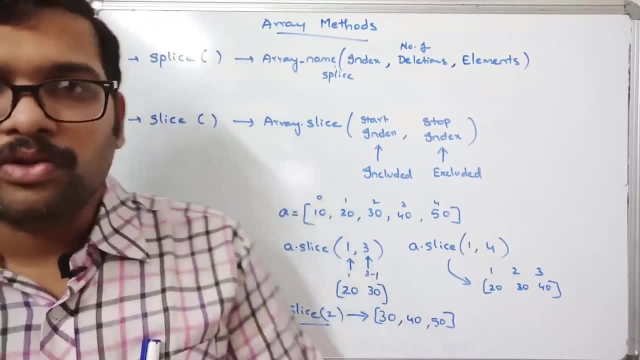 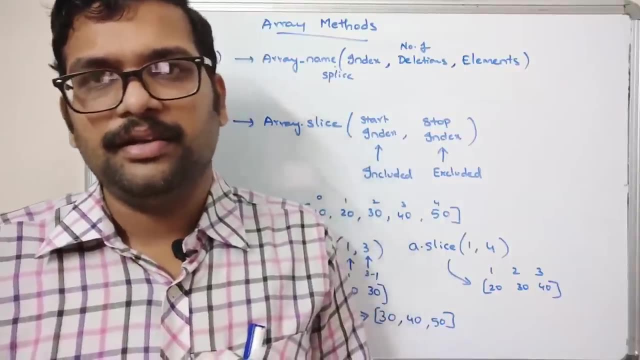 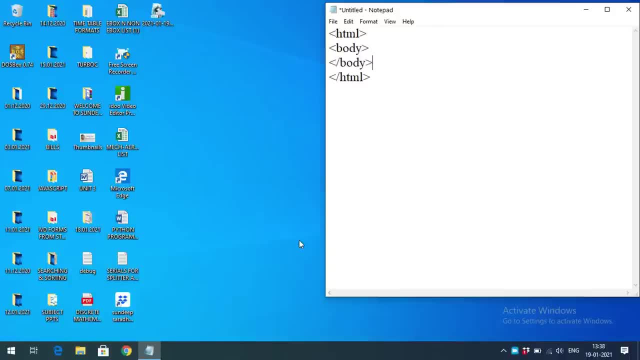 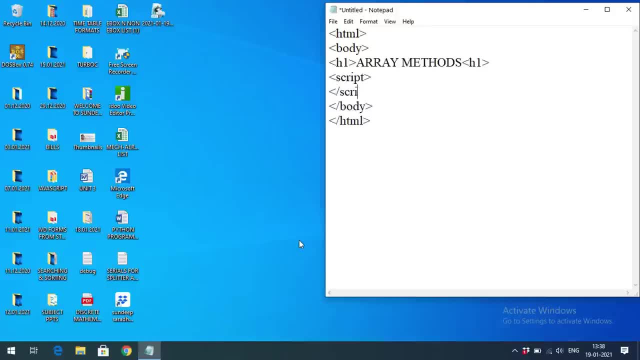 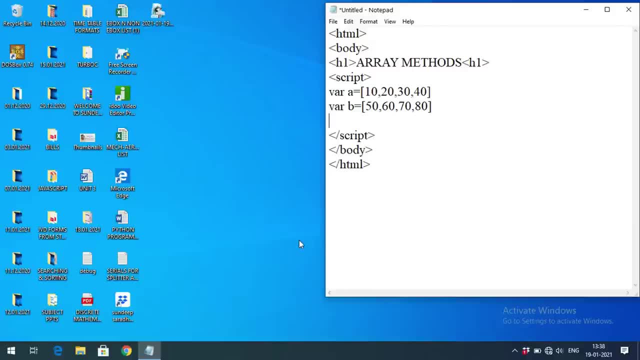 so joining means joining all the elements of an array. for example, if you consider some array A, there are four elements. we can join all those three elements by using one delimiter right. so we will check with this one document: dot write a length, so A dot join and give. 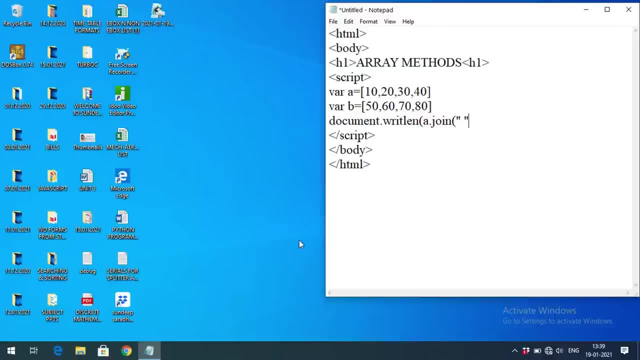 the delimiter. here you can give any delimiter, so not only the symbols or not only the space, you can also give the text also. so I will give the break row for the next output to be printed in the next line. so, dr, yeah, now you can observe. here I have given some. 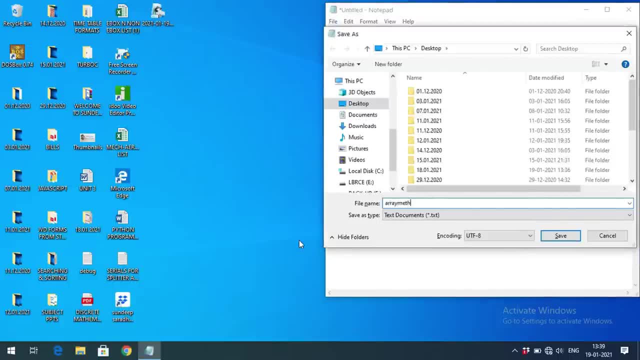 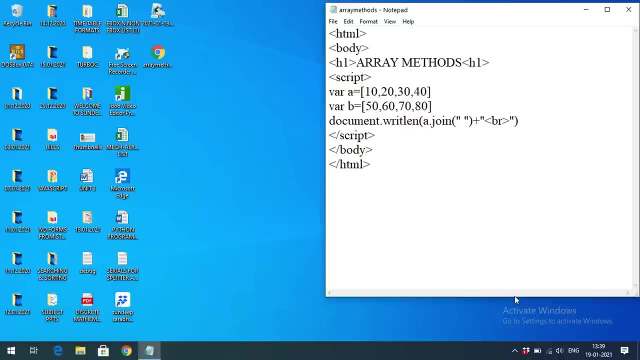 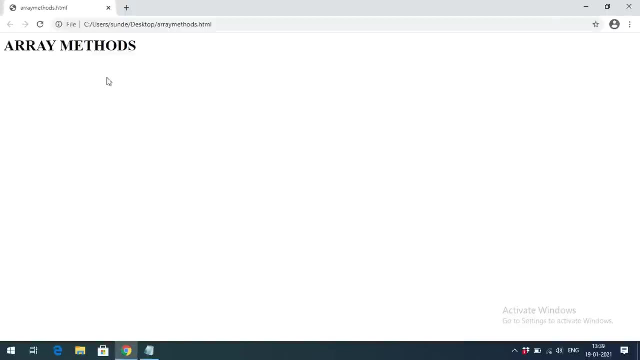 space, right. so now I am just saving this file with array methods, dot html, so you can find the file has been generated here and you can execute the right. so now I am just saving the file. so this is the array methods and write a length. so spelling mistakes. 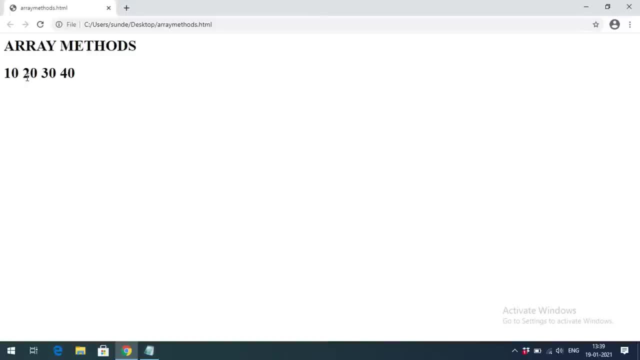 so you can observe here: now we get the content: 10,, 20,, 30 and 40, right, so this is how we can use the thing. so we can print the thing. so, instead of giving the space, if you give. 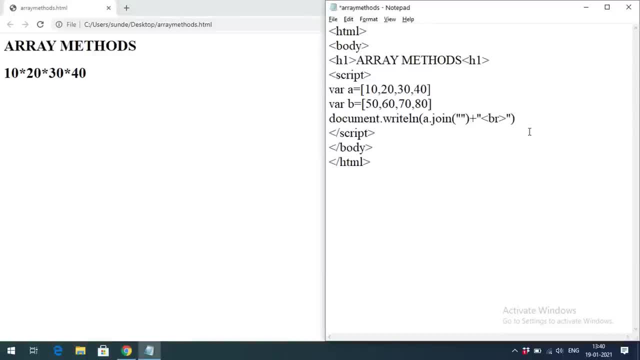 the space. the star will be printed in between the elements instead of star. if you use some dollar symbol, the dollar symbol will be added in between the elements of the array and also you can give the content. the text can be also given. so 10, given text, 20, given. 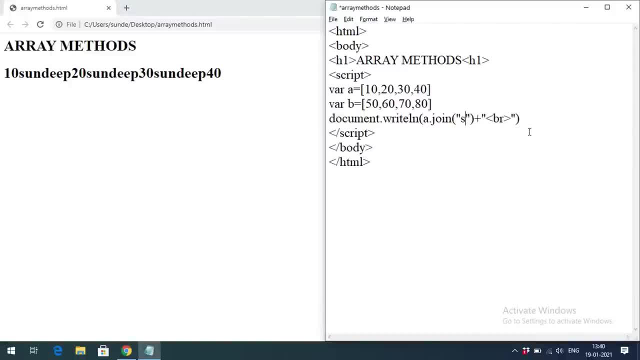 text 30, given text 40, so not only the symbols. we can give any value here. so that is why we call it as a delimiter, and that delimiter should be enclosed in quotations so that we can join all the elements of array with the help of the elements of the array. so 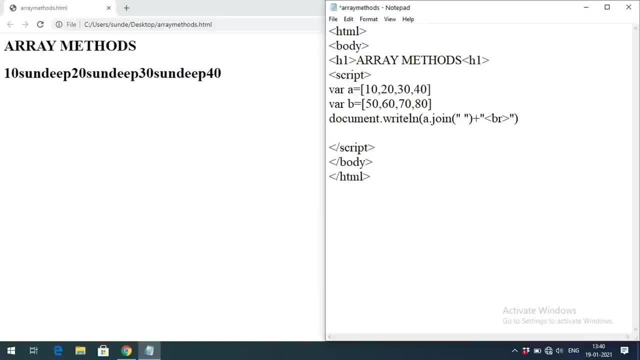 delimiter given in the join function. so that is all about our join function and then we will go with the sort function. so we will take some string, some c is equal to give the string some x, y, z, and then g, h, i, next d, e, f, a, b, c. so I have given this. 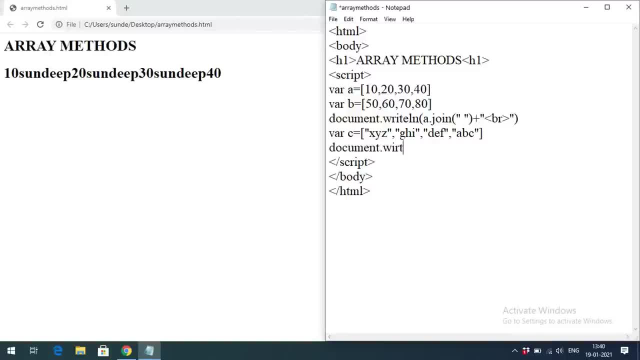 one. now we will sort the elements. So sort function will sort out the array elements in alphabetical order. right, so a dot, sorry, sorry, c dot, sort. you can observe here and also give the dr for the next output to be printed in the next line. so you can observe here. see, this is the elements a. 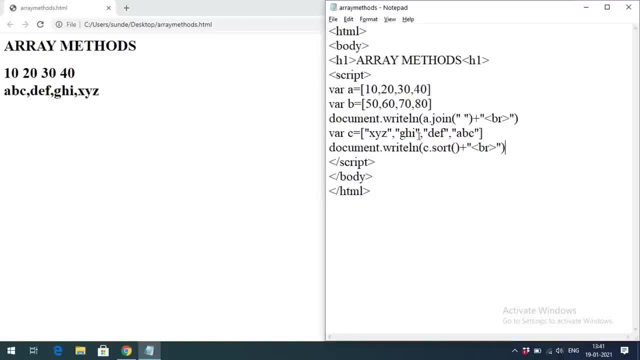 b c, d e, f, g, h, i and x y z. so here we have given x y z, g, h, i, d e, f and a b c. 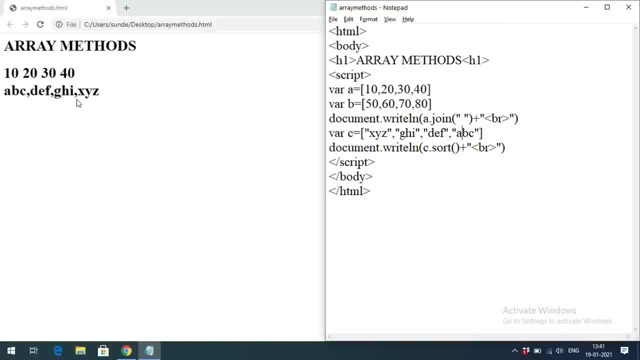 Correct order is in this way. correct order is in this way, right, and also we can have the see. I will change the order now. ok, I will change the order now. now also, it will be same. and now I just want to reverse the elements. ok, I just want to reverse the. 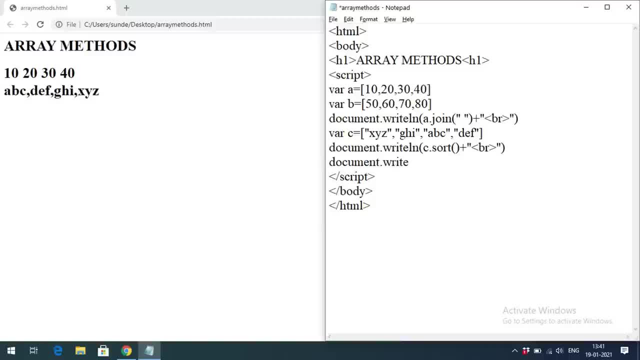 elements. we can reverse the elements in a numerical array or a string array. ok, so a dot reverse function, Reverse function will print all the elements in a reverse order. ok, see, you can observe here. so actually the elements of a is 10,, 20,, 30,, 40 and m. I have just implemented. 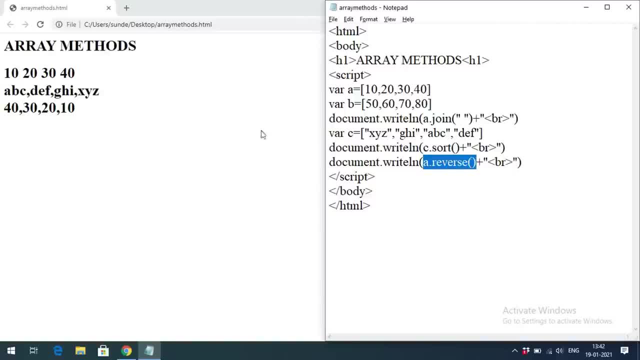 some reverse function. so the elements are 40,, 30,, 20 and 10,. right Now I will print both the arrays: document dot, write ln. I will give the a is equal to plus a plus and go with the break row and use the same thing for printing the next second. 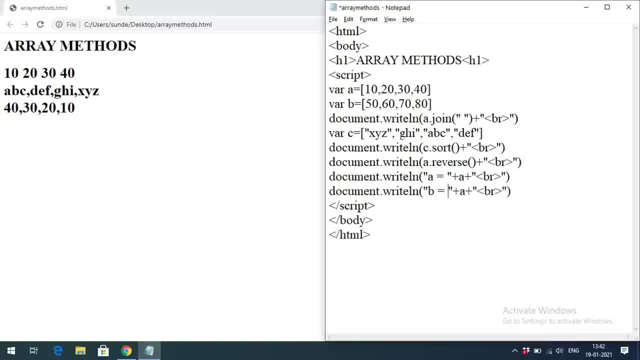 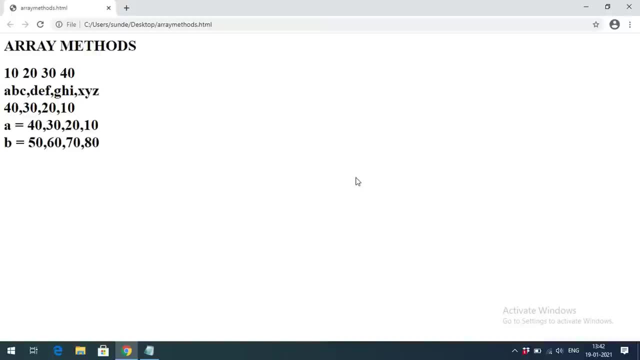 array. also, that means b is equal to, because further we are going to discuss about the push and pop function so that you need to know what are the elements should be pushed and what the elements should be sorted. so you can observe here a dot reverse means. 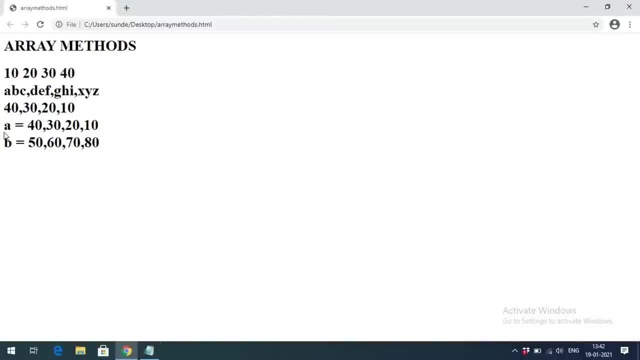 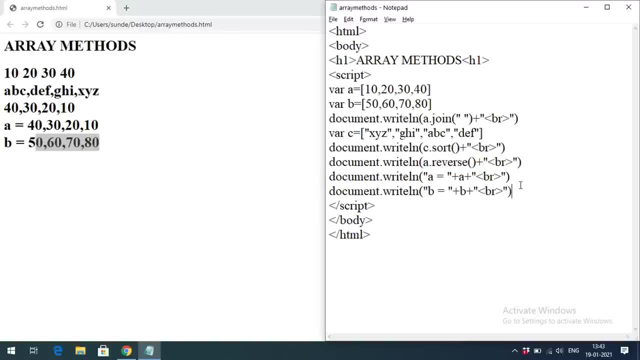 the complete elements will be reversed and it will be stored in the same array. so that is why we got the same result: 40,, 30,, 40,, 10.. And here 50,, 60,, 70,, 80,. now we will move on with the next function, that is a pop function. 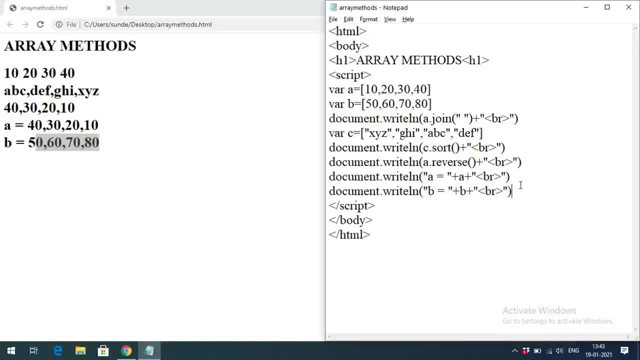 pop function. So, coming to the pop function, pop function will remove the last element. so you can observe here: dot vent, dot write ln. so we will pop the element from a, so a dot pop and also give the br for the next output. 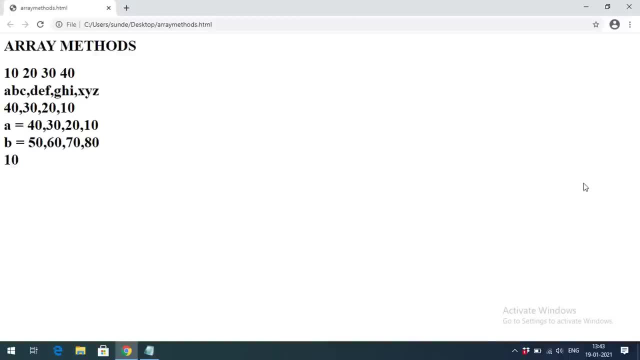 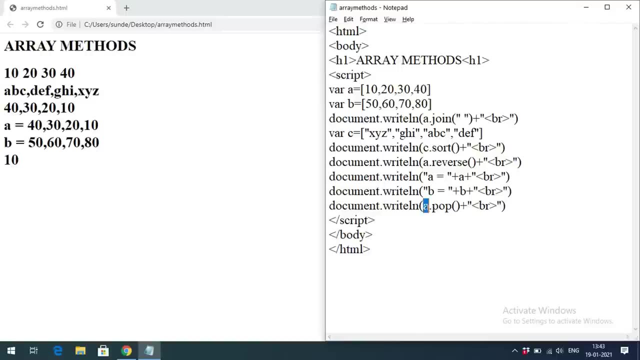 So you can observe here: It will return the element which has been deleted, right? So actually pop function will delete the last element. So here I am giving some a dot pop. So consider the array a, If you can, just the array a. the array elements are 40, 30, 20, 10 and from that the last element is 10. that will be. 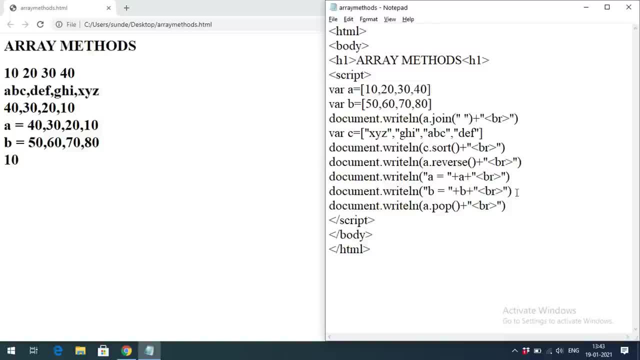 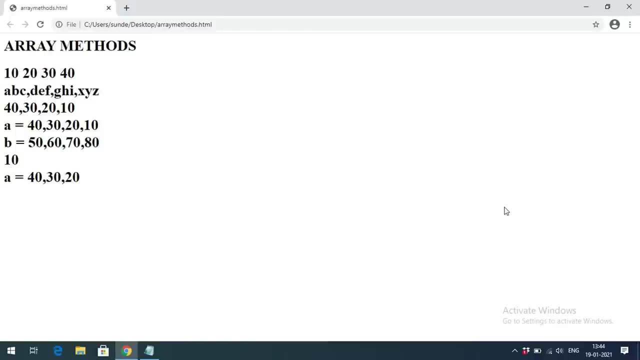 Removed and that element will be displayed here and after the pop function. if you still display the a Array a, you can get the elements here: See 40, 30, 20,. that means we are deleting an element, but we the complete space is also deleted. 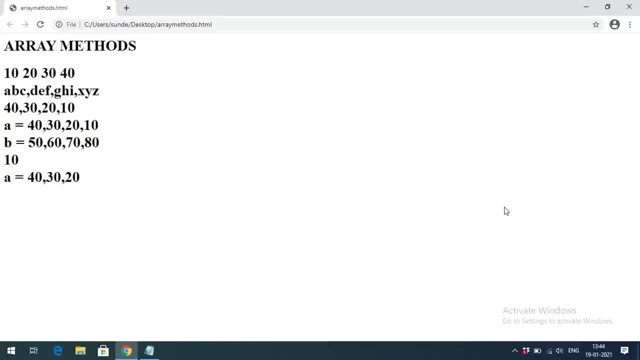 So in the previous video we have seen the delete method. So in order to delete the element by using the delete keyword, if you delete that, one space will be defined. So Space will not be deleted, The element is only deleted and that space will be filled with the undefined symbol, right. 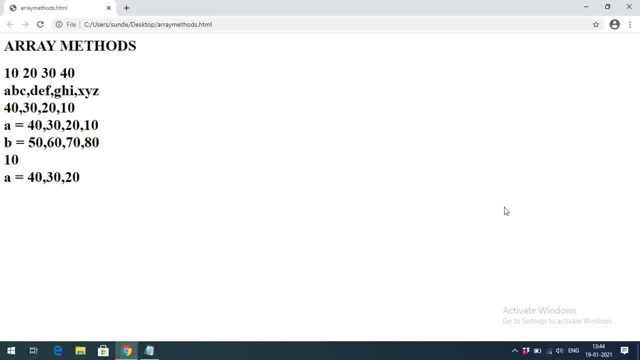 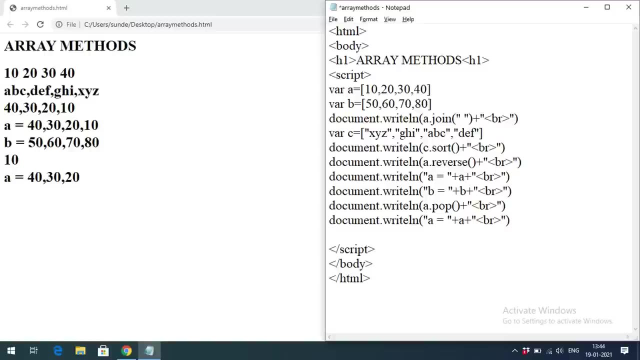 But here the pop function will delete the complete element. Okay, the space will also be, the memory will also be deleted. So only Three elements are there now. Now, this is all about a pop function. If you pop, the last element will be deleted, and next one is a push function. push function means inserting the element in order to insert. 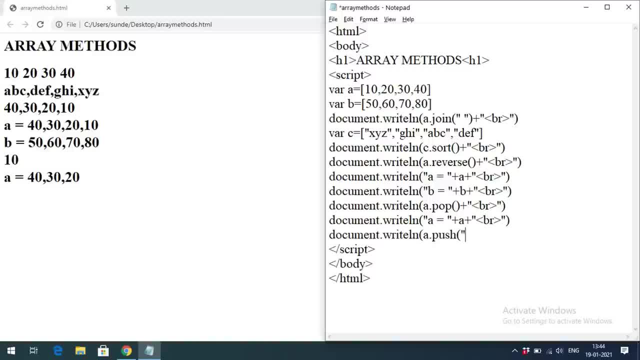 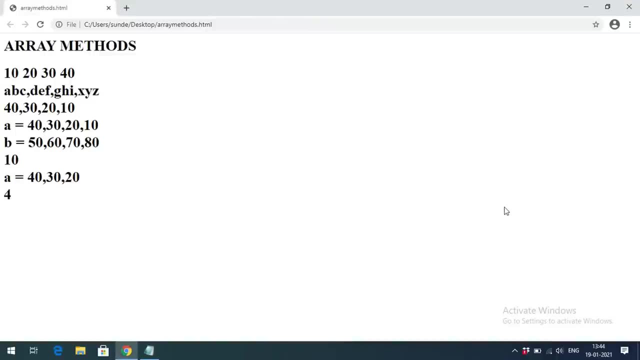 The element. so a dot push and give the element as an argument here. Give the element as an argument here, I will give some 10.. Okay, I'll give some 10 Now. you can observe, it will return the length of The array. so if you push the element it will return the length of the array. 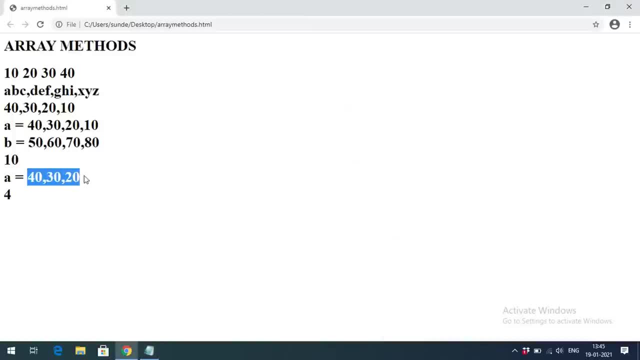 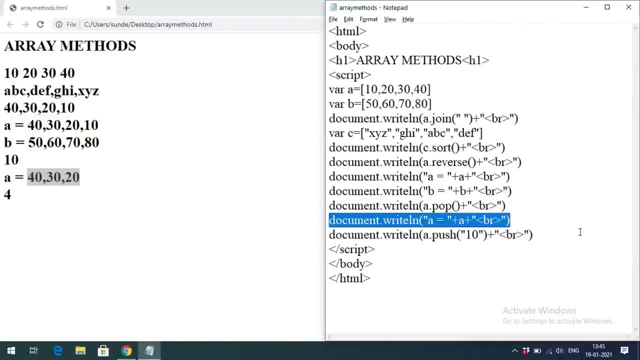 so you know that after deleting an element we are. the length of the array is a 3, but Now you have pushed one element, automatically the length is 4. now again, If you just print the value of a will get the four elements here: 40, 30, 20, 10. 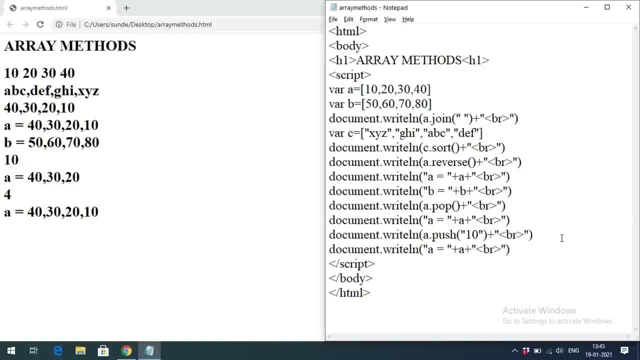 Okay, it will push the element at the last, last position. Okay, So pussy pushes to insert the element and pop is true, The element. and now there is a one more function called a shift Shift. shift will also delete the element, but the first element will be deleted. 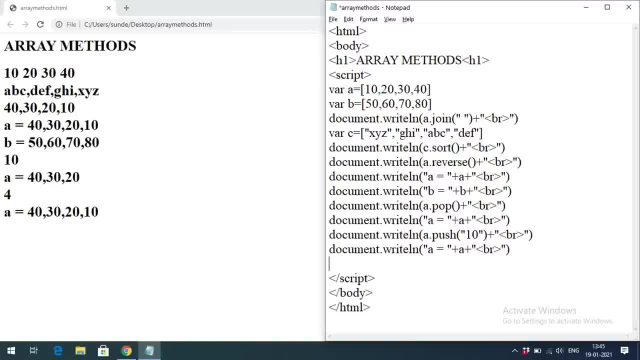 So, coming to the pop function, the last element will be deleted. Coming to the shift function, the first element will be deleted and all the remaining elements will be moved to the lower indexes. So now I will check. let me show that right. Ellen, It a dot Shift, Okay plus. 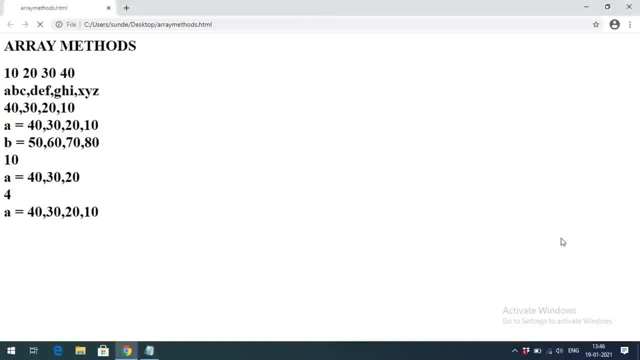 Yeah, Now you can observe here It will also Give the return the element which has been deleted. No, You can observe here. a dot shift means the 40 is removed. That means the first element, the beginning element, will be deleted and all the remaining elements will be moved towards its lower positions. 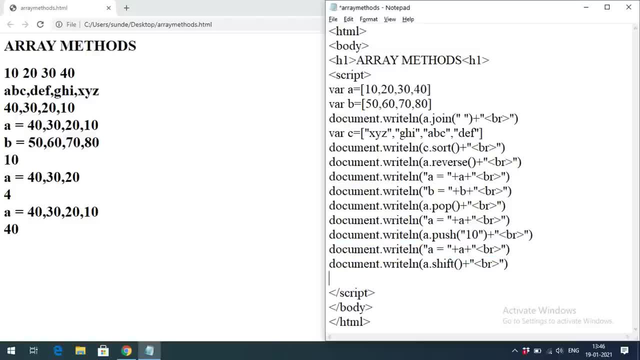 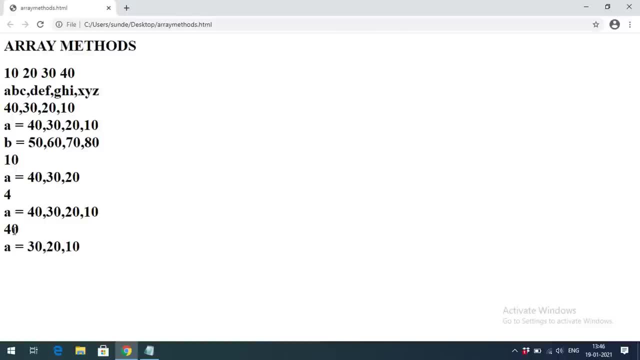 After that you can observe the a array a, which is having the three values shifted towards left side. So you can observe 30, 24 for 10. So before shifting the 40, The 40 is in 0th for index. 30 is in first index. 20 is in second index. 10 is in third index. 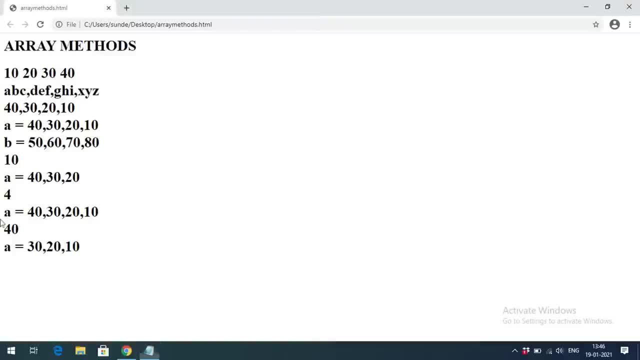 Now, after deleting this one, that means after using the shift operation, the 40 will be shift, 40 will be deleted and all the remaining Values will be shifted towards left. So previously 30 is in 0th first index, now 30 is in 0th index. 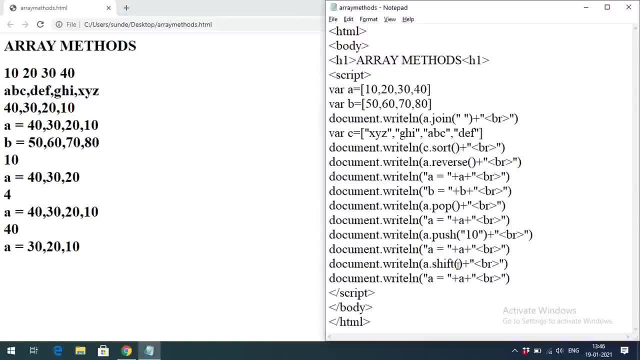 Similarly, 20 will be moved to left and 10 will be moved to left. So that's called a shift operation. and there is a one more operation called unshift that will insert the element At the beginning itself. so that will will check document dot. write ln. 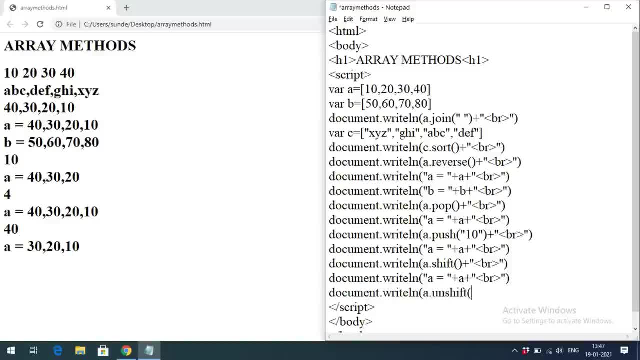 A dot unshift, so unshift and pass one argument, So argument, that argument is a value that should be inserted, right? So I will give 50. So where it will be inserted, it will be inserted at the beginning of the array and again the elements will be moved towards. 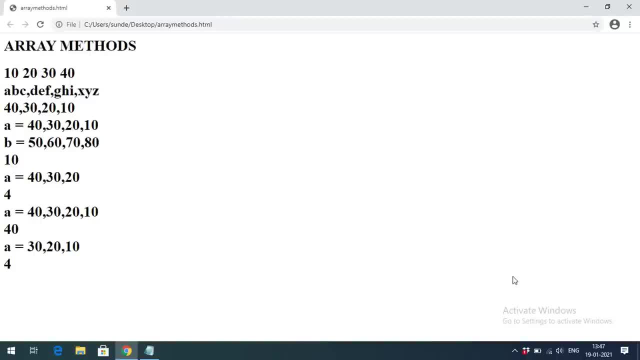 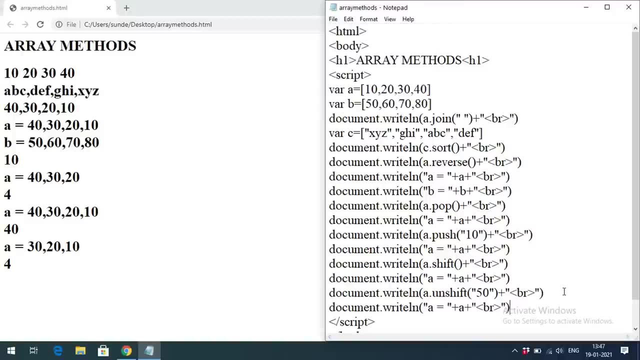 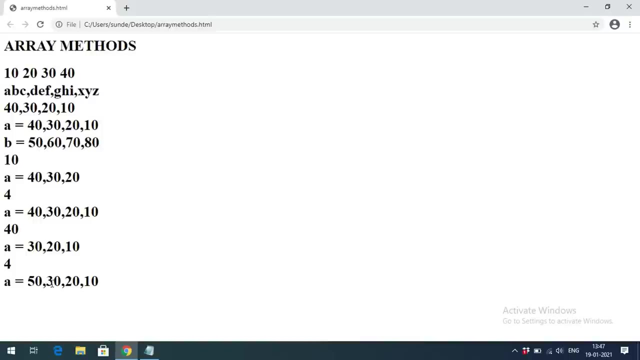 Then observe here Again, the length is Four, right, So previously we are having three. the length is four again. if you print a value, You will get the elements you can observe here: 50 is Inserted and all the remaining elements are shifted towards its higher indexes. the move moved. 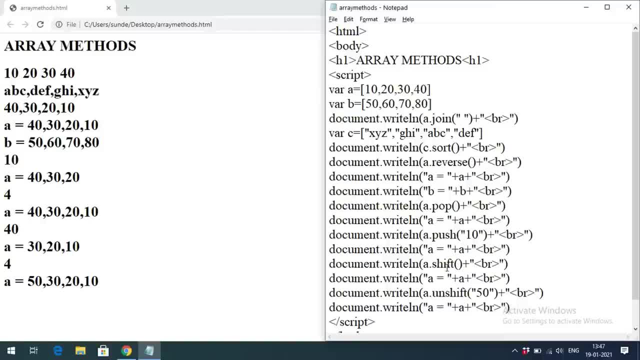 Okay, So that is the purpose of unshift. shift is for deleting the element at the starting position and moving the elements. unshift is to insert the value at the beginning of the beginning of the array. That means inserting at the Starting position and the all the remaining elements will be moved towards its right side. 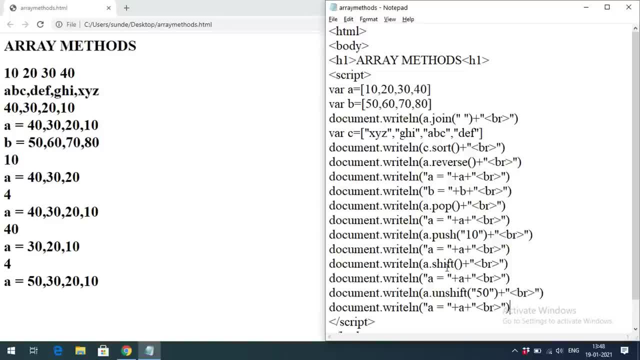 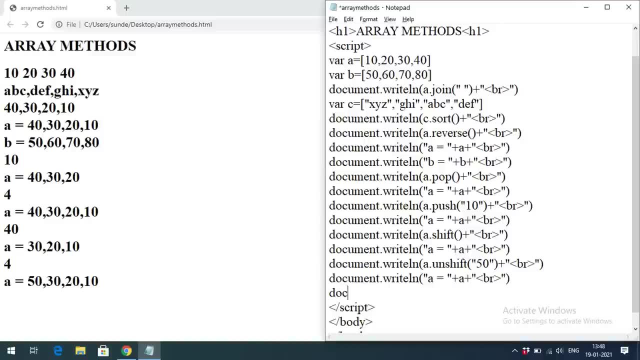 Hope you understood this one right. next, Concatenation. so now we will see the concatenation. concatenation means combining both the elements. so we can use here so document dot, write ln, and You can concatenate here. so a dot, concat of B, so that B will be concatenated to. 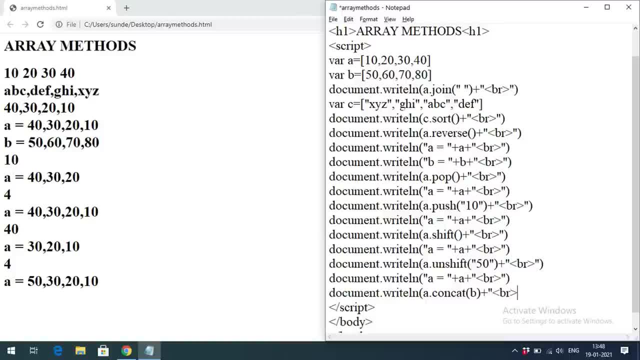 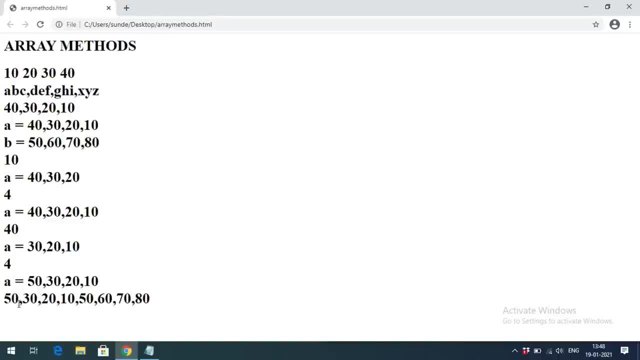 A. so let us check the result. So after applying this one, You can observe here. So the elements have concatenated. So this is the elements of a: 50, 30, 20, 10, 50- you can observe here Right- and next 50, 60, 70, 80 are the B elements. So we elements are: 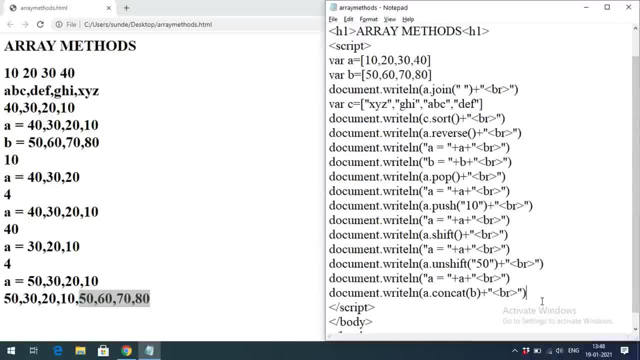 Concatenated to an array, a, so that this also called as merging. Okay, merging two arrays, and also we can not only the complete array, We can also concatenate this particular elements. so if you observe here document dot, first let us print a value. see a is. 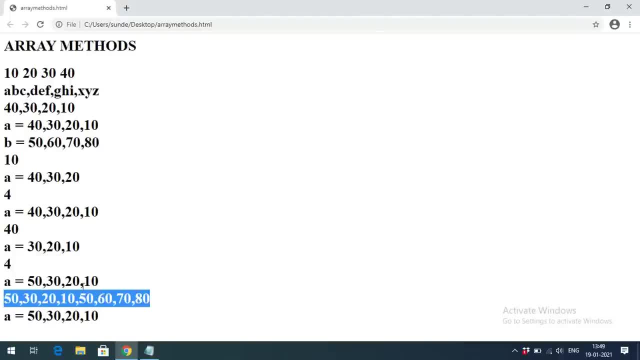 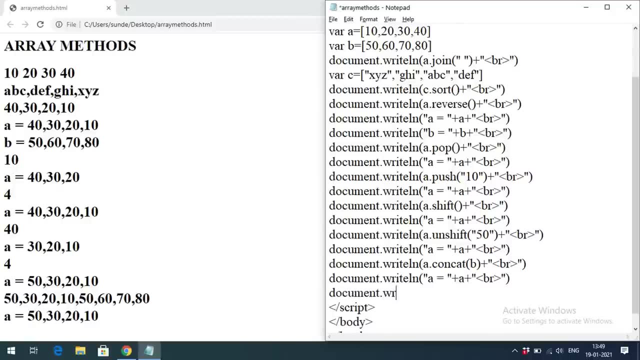 equal to 50, 30, 20, 10. that means a will not be updated, so a new array will be created. okay, a new array will be created. now let us check. so: document dot, write ln, a, dot, concat. and instead of giving c here, I will give some only one element. 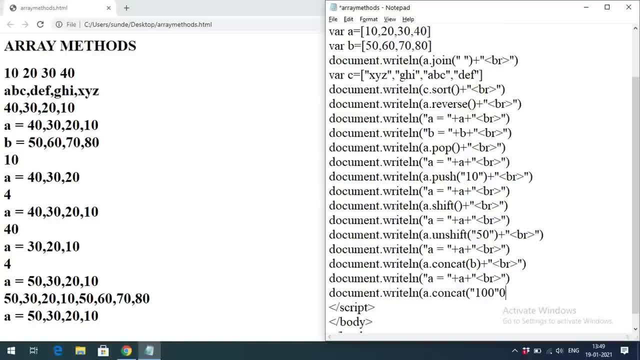 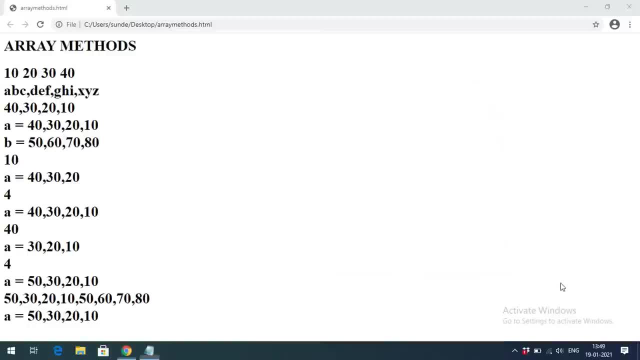 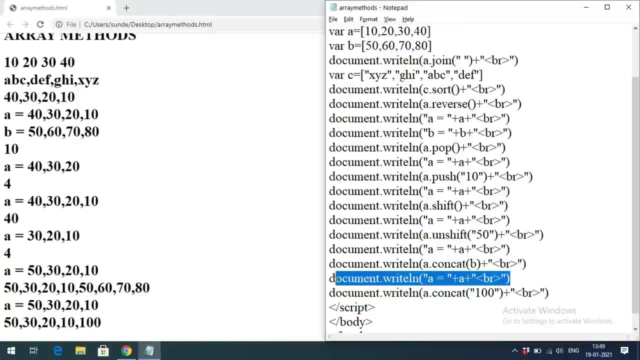 okay, one element, I will give some hundred so that element will be concatenated to a. let us check so we are can observe, see 50, 30, 20, 10 and hundred. okay, a concatenated. and after that you can also observe the a, whether it has been changed or not. you can see here, a is not changed. 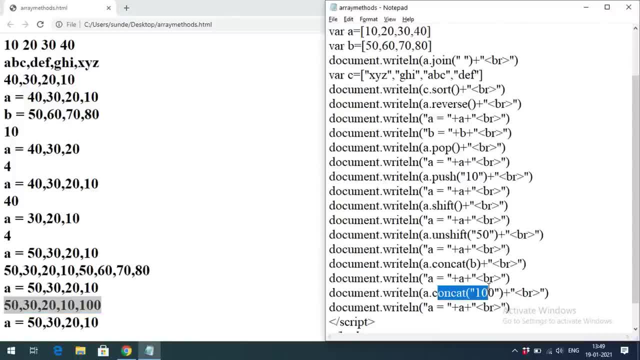 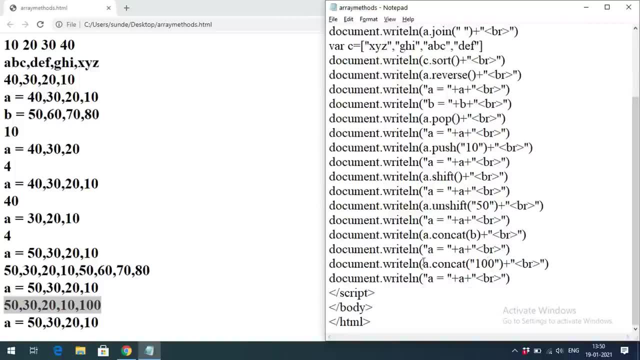 okay, a new array will be created. so for concatenation function, it will be added and a new array will be returned. so unless you saved the new array into a particular variable, it doesn't save the values. okay, so the original values will not be changed. hope you understood this one. so after concatenation: still, if you, 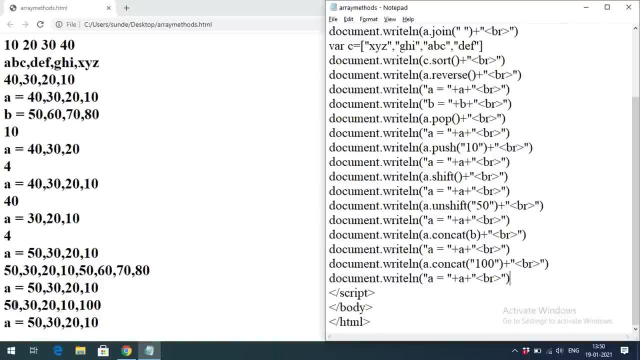 are printing here. we are not getting the concatenated value because this returns a new array right. so that is a concatenation and splice. you can also do anything here. you can run the and create a automater call and this want to neurologic smoking and we can run as you're ripping a local. 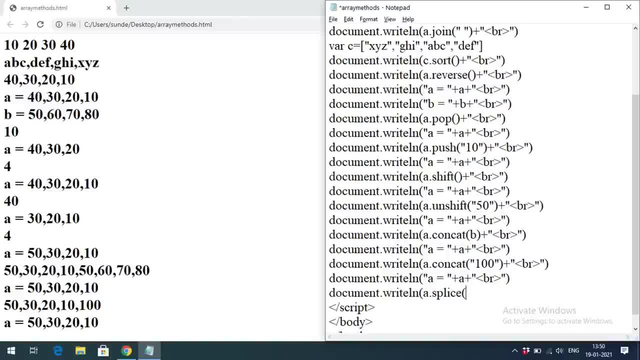 inside un谷 Emmy Christ property and say that this is who is gonna define, and the last, the next, next, followed by a new array, will always bequeath basic to not only the ability to be added to every object, I don't mean even the item, the. 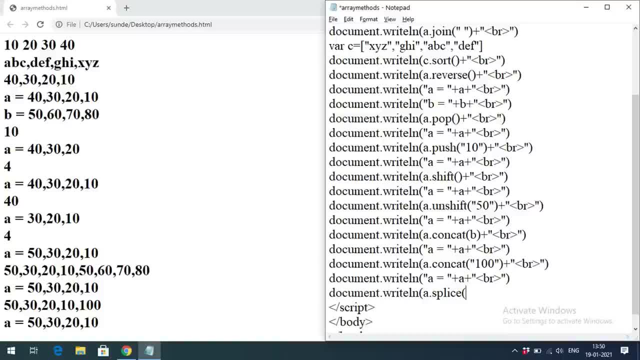 largest object you can have. once again, I will add 40. that means the index value of 40. so I just want to add 40 here, right? so 40 here means the index value is 1 and I don't want to delete any other elements, even though we are. 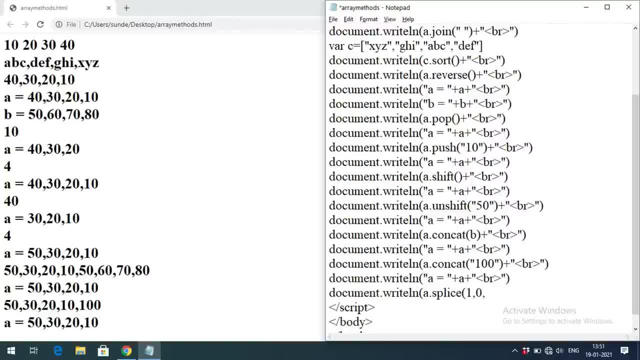 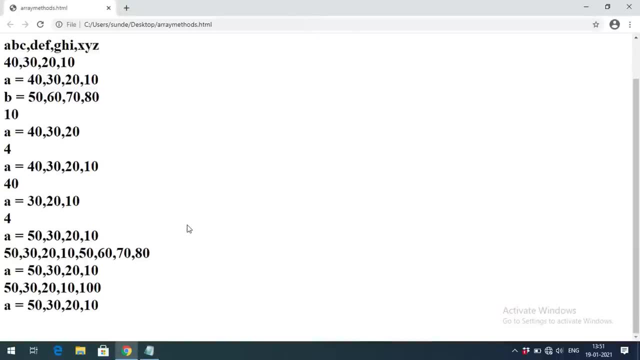 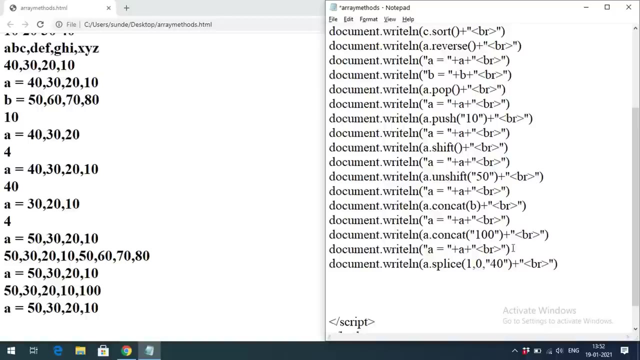 adding the elements I don't want to delete. so zero number of elements should be deleted. and what element should be added here? so 40 should be added here, right? so nothing will be printed because no element has been deleted here, right? so after that, if you print the value of a, we will get the added element here, so you can observe here. 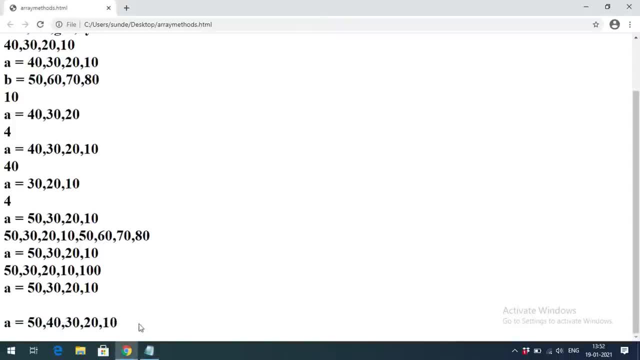 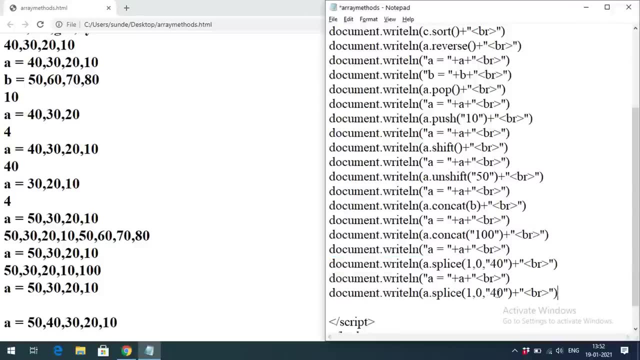 a is equal to 50, 40, 30, 20, 10, and if you want to delete the elements, so we can give the position from where we have been waiting for that value to happen, right, so from where we how to add? okay, not only the 40, we can also go with the multiple elements. so if you add some, 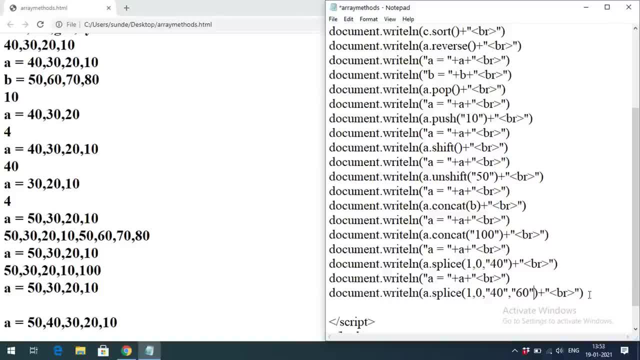 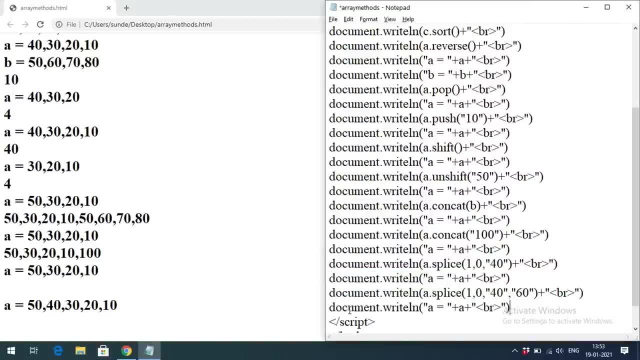 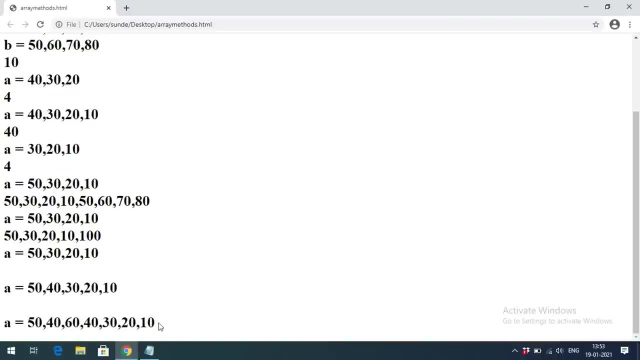 40 comma 60. so two elements will be added here, right, so you can observe here again: nothing will be printed, and after that, if you execute, if you print the value of a, we will get the two more elements here. so see 40, 60, 40, 30, 20 and 10 right at one position. zero element should be deleted. 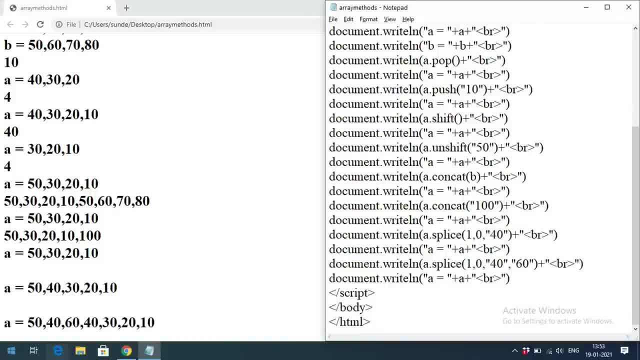 and if you want to delete some two elements, now you can observe, the value of a is here. and if you want to remove this one, what element see here? here you can observe. I just want to add some 70 and I just want to remove two elements so I can go with here. I just want to add some 70, okay, and I just 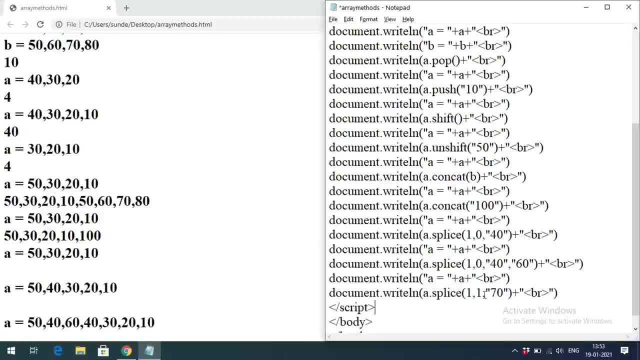 want to remove one element and where I have to get the 70- zero, one, two, three. third index. see here you can observe zero one, two, three in the third index. I just want to remove 40 and I want to get a 70. so here you. 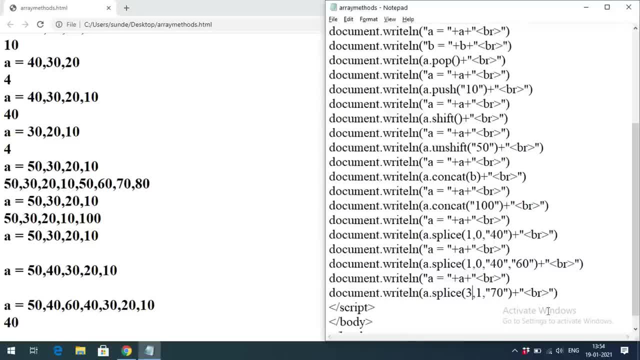 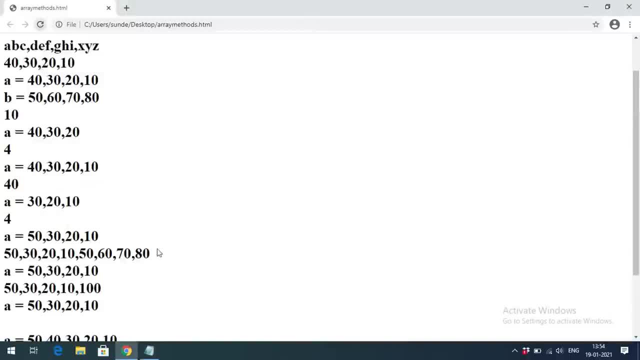 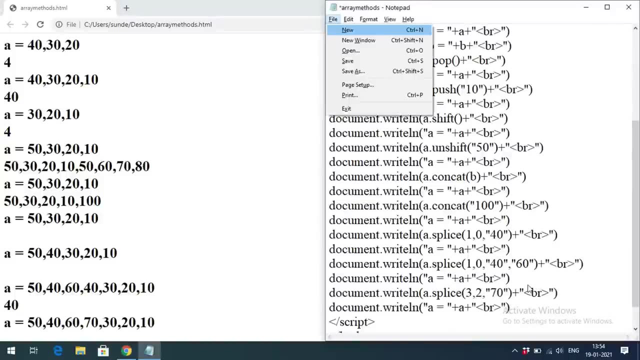 can observe. so if you put this one, the 40 is removed and you can observe here. so it will return the element which has been deleted, right? so after that, if you print a value, you can observe the 40 is replaced with the 70, and here, if you want to remove two elements, the two elements will be deleted. here and those two. 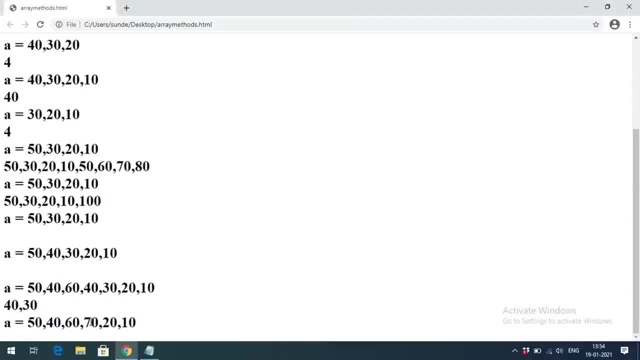 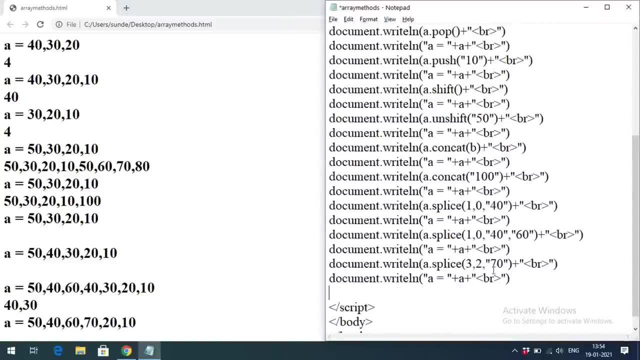 elements will be printed here. so you can observe here. the 40-30 is deleted here instead of 40-30-70 is inserted. so here, if you don't want to insert anything, if you just want to delete the elements, then also you can use this splice function. it doesn't give any space, so you can observe here. so 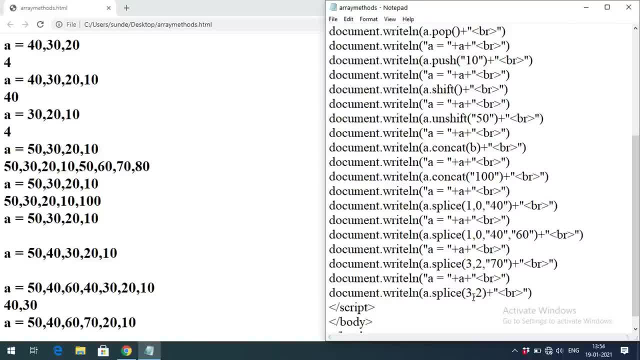 give the two arguments, that is, where, from where we have to start deletion and how many elements to be deleted. So 3, that means. so you can observe here, 0,, 1, 2, 3, here from here the third index, two values, that means 70 and 20, will be deleted by executing this. 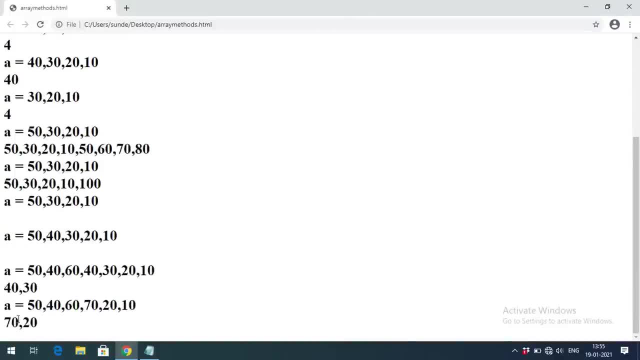 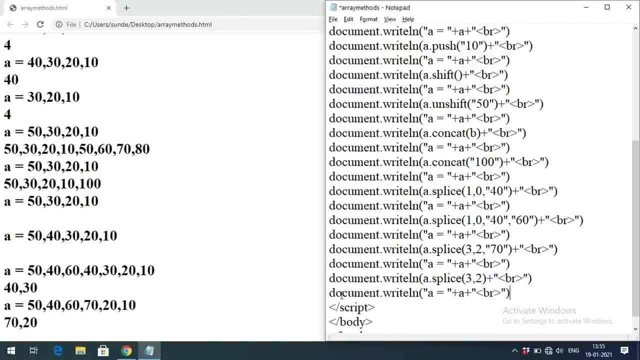 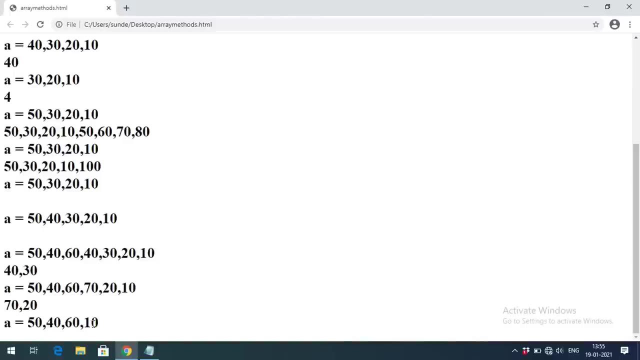 statement you can observe here: see 70 and 20 will be deleted, So it will return the elements which has been deleted. So after that, if again, if you want to print the a value, you will get the elements after deleting 70 and 20.. So the elements of a are 50, 40,. 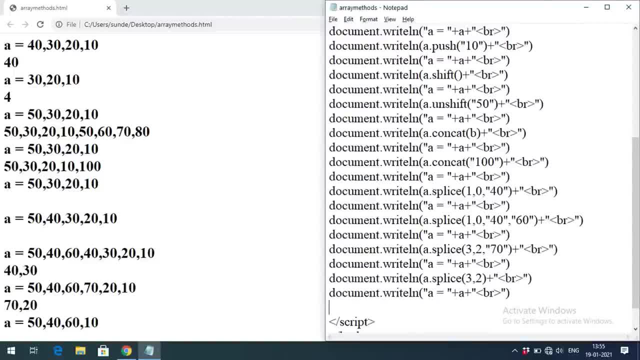 60 and 10, right, and I just want to replace some with a 30,, 10 with a 30 again, go with the splice function and use the splice. So 0,, 1,, 2, 3 from 3. delete one element and insert. 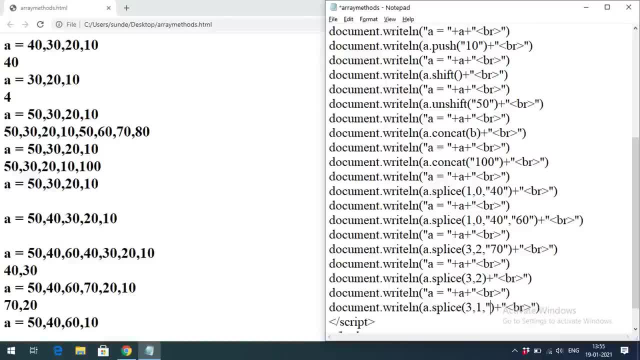 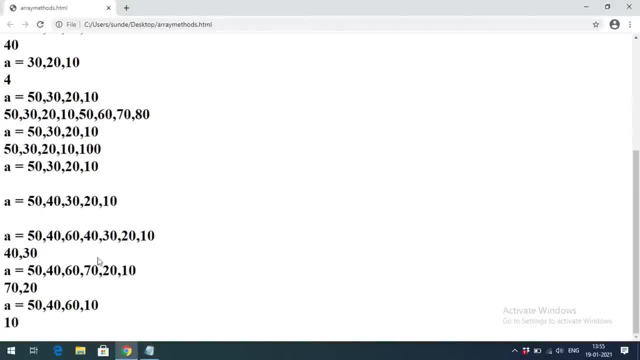 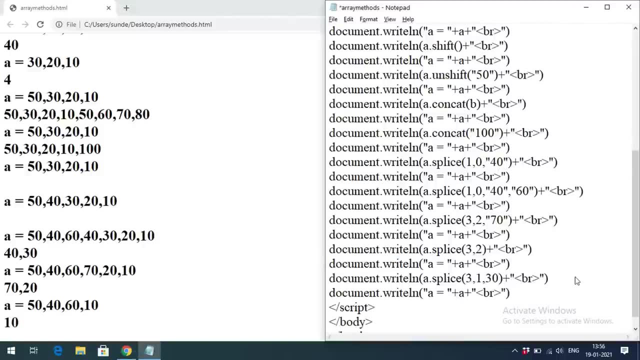 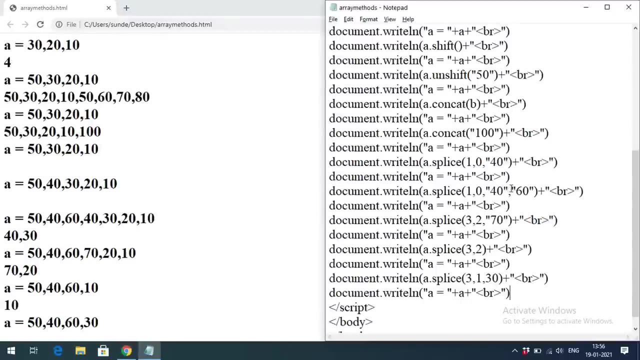 some 30,, some 30.. So 30 element will be added here. ok, 30 element will be added here. So 30 element will be added here. ok, 30 element will be added here. See, 10 is deleted here and if you go with the a, 30 is added here. right, So in you can. 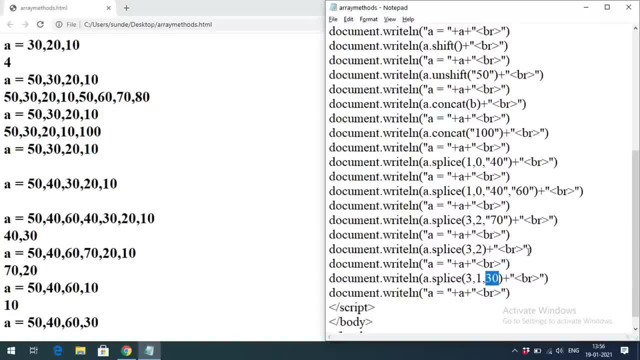 enclose in a quotations, or simply you can go with this one, because this is a numbers right. So even though the strings are here, it will be treated as a numbers in here, other than the arithmetic addition right. So 3, 1,, 10, 30 means from 30 to 30. So 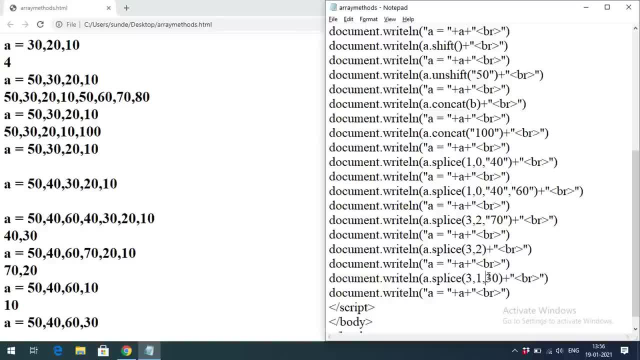 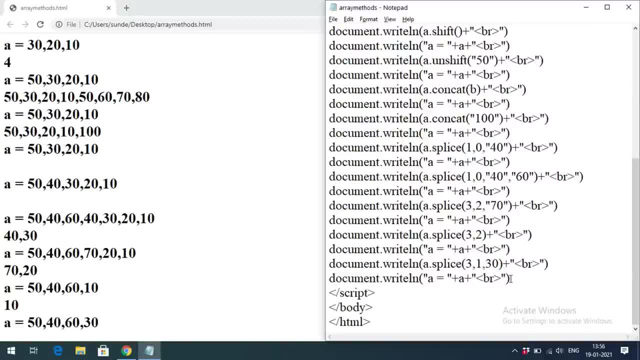 from third position, one element will be deleted and instead of that element we are adding some 30. So that is why 50, 40, 60 and 30, right? So hope you understood this one. and also we can have the slice operation. So slicing means extracting the portion, right? 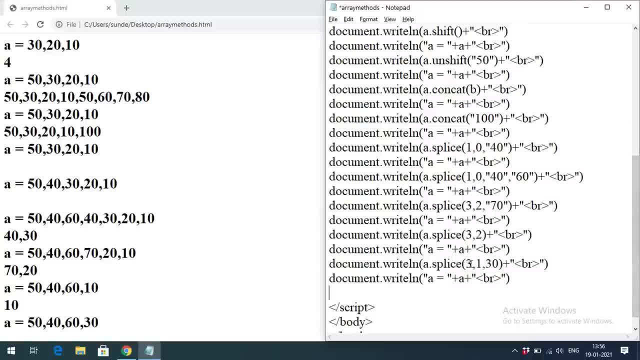 So, splice, I think you understood this splice function. The first one is the index, from where we have to start, and the second parameter is how many elements should be deleted. ok, how many elements should be deleted If you want, if you do not want to delete the elements. 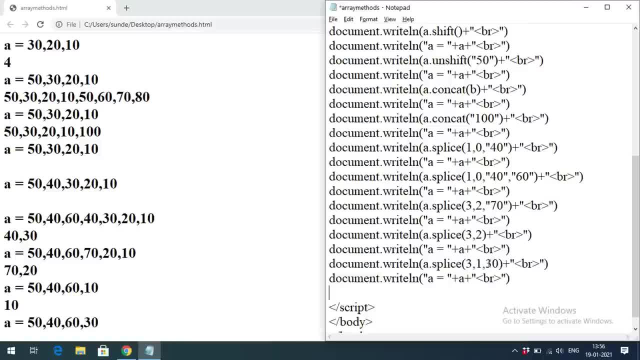 you just place 0 there, ok, And after that, what are the elements to be added, how many number of elements to be added? those elements should be inserted here using a comma right, And then the slice operation. so slice operation means extracting the portions based upon the index value. So I will go. 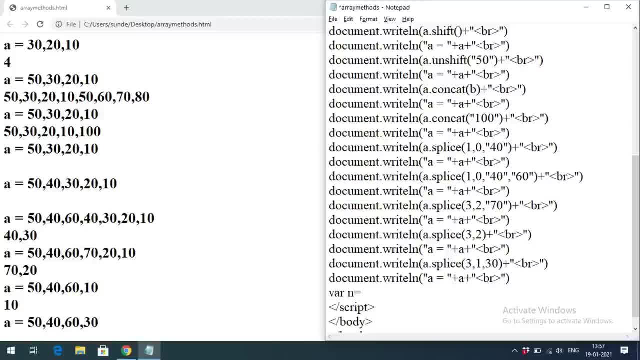 with some. where n is equal to, I will go with the 10,, 20,, 30,, 40,, 50,, 60,, 70, right. So now let us check document. dot write ln go with the. So I will go with a dot. sorry n n dot slice and give the index range the starting index. 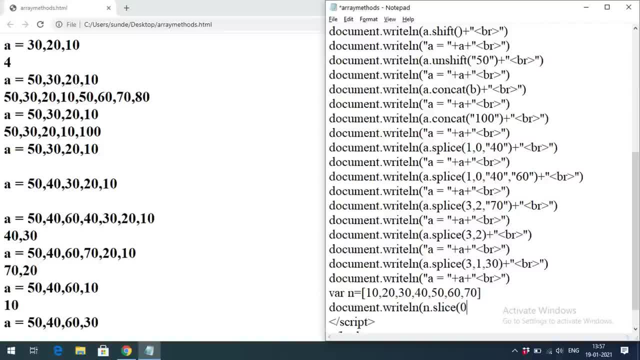 and the end index and index will not be included. I will go with 0. that means the extract, the portion from the index value 0 to 5,. 5 means 4 up to 4. it will be deleted. ok, it will be extracted. 0,, 1,, 2,, 3 and a 4. last stop index will not be included. So you can observe. 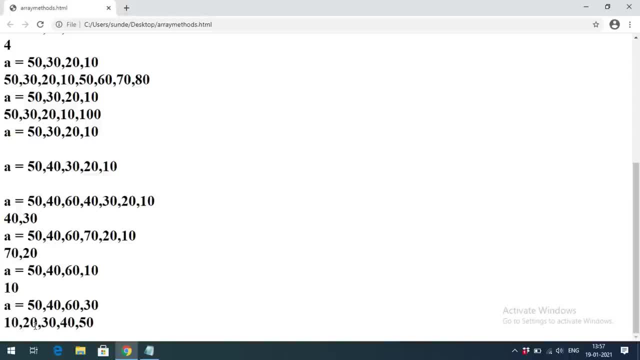 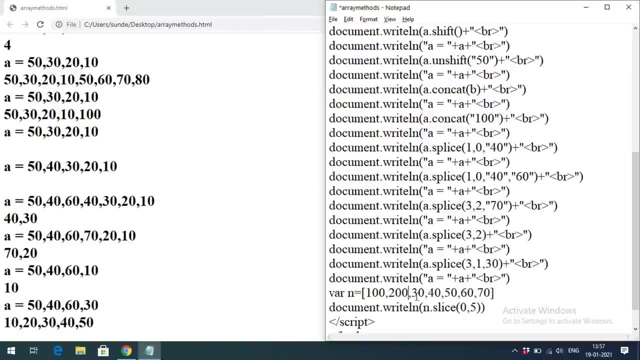 here it will return the elements So you can observe 10,, 20,, 30,, 40 and 50. So let us give some 100.. So there will be no confusion for you. So I will change the elements: 300,. 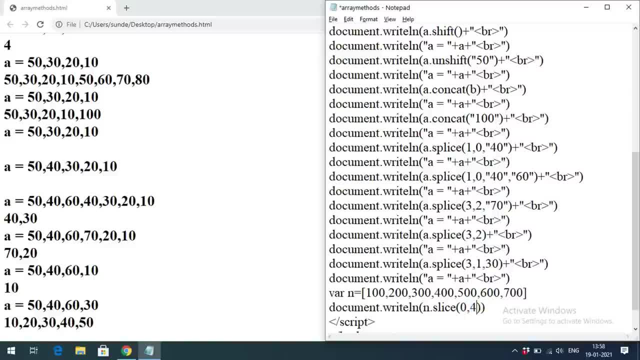 400,, 500,, 600, and 700, and I will give some 4. that means 0,, 1,, 2,, 3.. So before that I will print the value of n so that and the output, we can know that n is equal to plus. 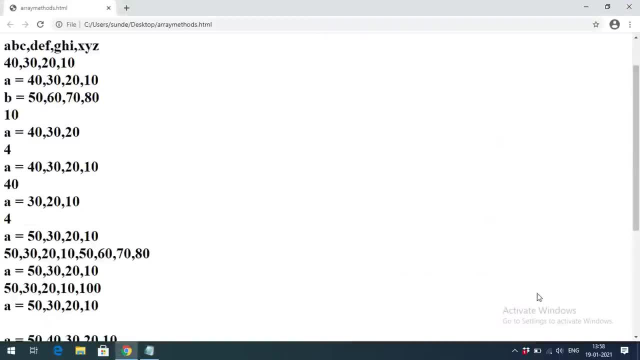 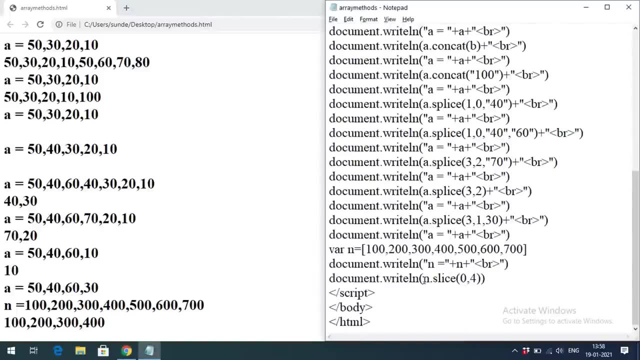 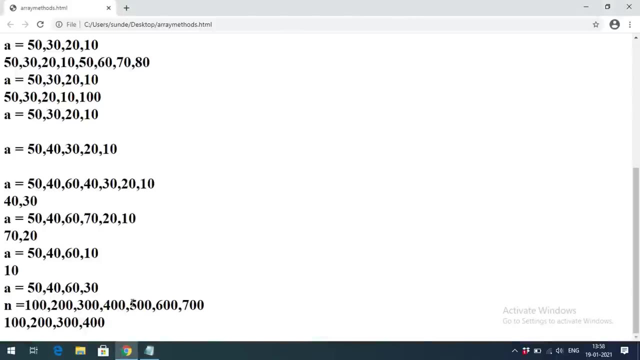 n plus dr. here n is equal to 100,, 200,, 300,, 400,, 500,, 600,, 700 and coming to the slice. So here, 0th index to 4th index, 0th index, 0,, 1,, 2,, 3 and a 4.. So 4th index is not included. 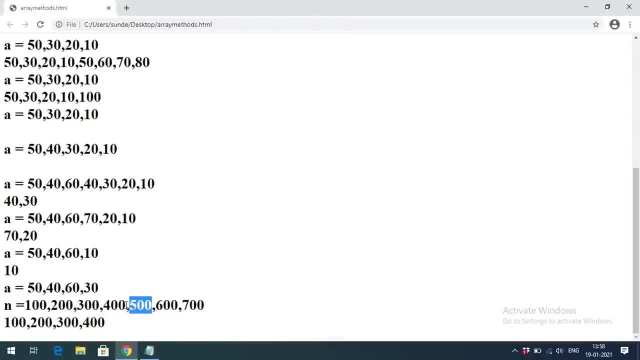 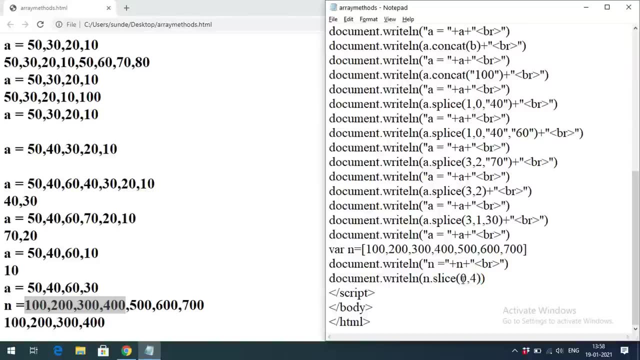 because the last index will not be included. So 4 minus 1, that means up to 3,. 3rd index, it will be printed right. So here the slice function will accept the two arguments: one is the start index and the second one is the last index. And if you are not specifying, 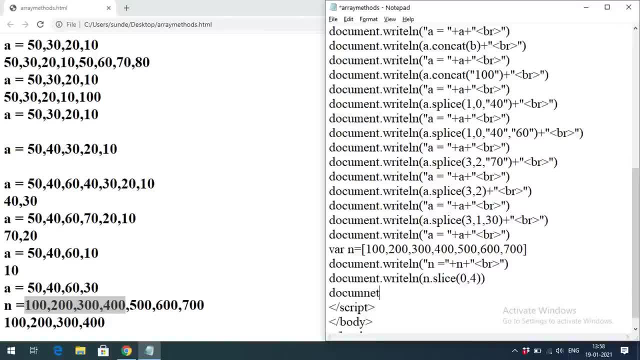 the last index, automatically it will print the rest of the array, ok, from the given starting index. So n dot slice. so if you go with only one argument, that is, a 3, it will start extracting from the 3rd index to last element. You can observe here: see 3rd. 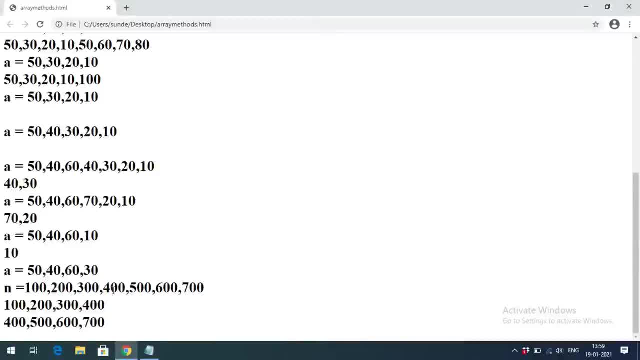 index. I am given 3, right. So 0,, 1,, 2,, 3. that means from 400,. we are not giving the stop index automatically. it will stop. So 0,, 1,, 2,, 3, that means from 400,. we are not. 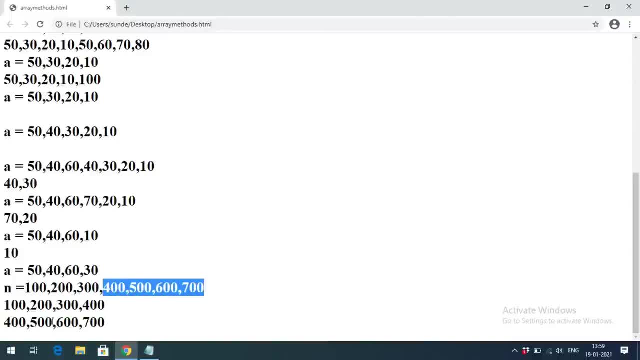 giving the stop index, So 0,, 1,, 2,, 3, that means from 400,. we are not giving the stop index, so it will start extracting the all the values from the given index value, So 400,, 500,, 600 and 700.. So like that we can use the slice operation to extract some portion. 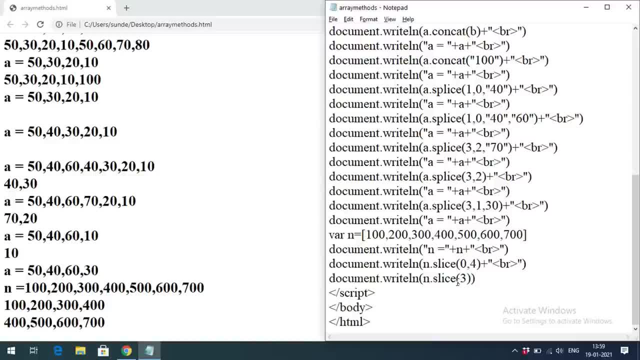 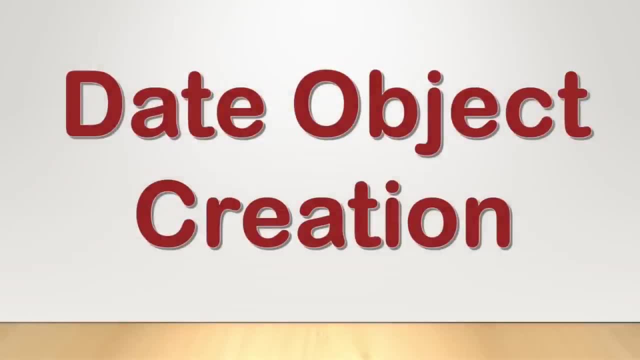 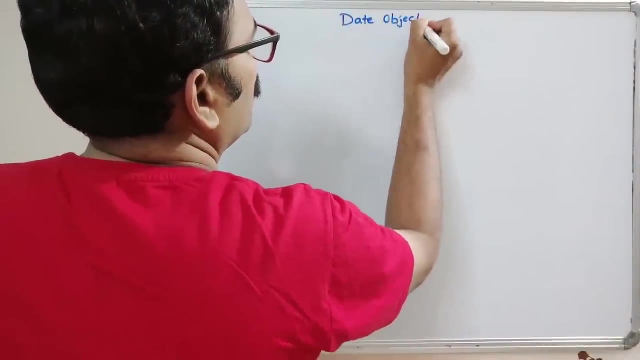 of the elements right, So hope you understood all these methods. So we have seen a join, push, pop, shift, unshift slice, concatenate slice, sort operation and reverse operation. So in the previous sessions we have discussed about how to create an object, So any object. 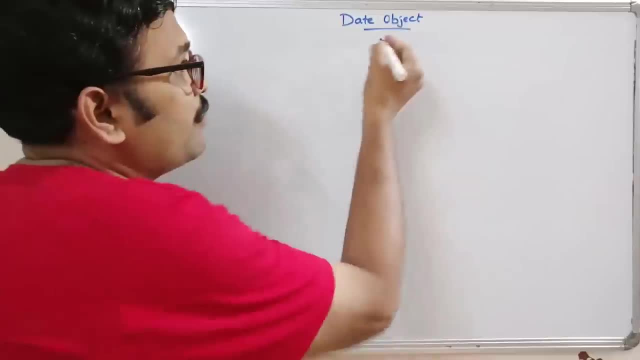 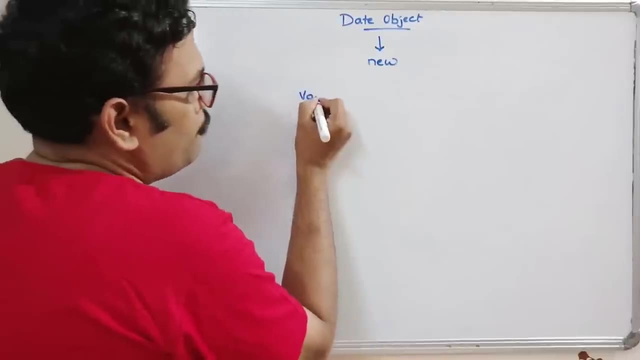 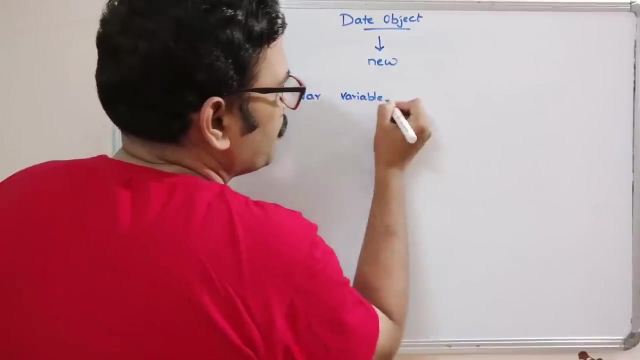 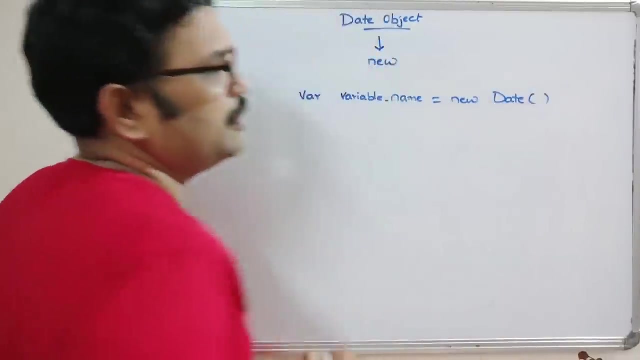 can be created by using a new keyword. So for creation of this data object also, we have to use new keyword, right. So where some variable name right, some variable name, right, Okay, Okay. So this is called a new is equal to new. date. Date class, okay, Date class. So this will. 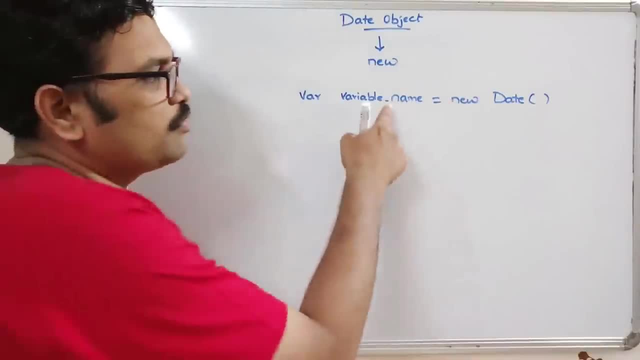 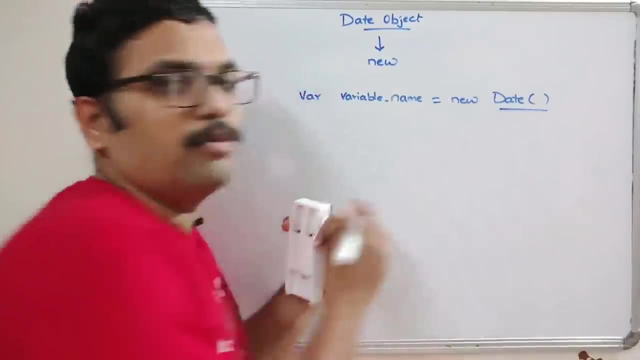 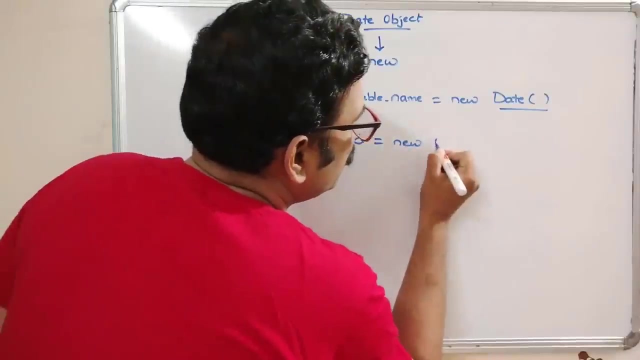 create a variable of date class. That means this is called an object- date object. So in order to work with the time and date, we need to go with this date object right. So, for example, where some D is equal to new date. So this function will give content. 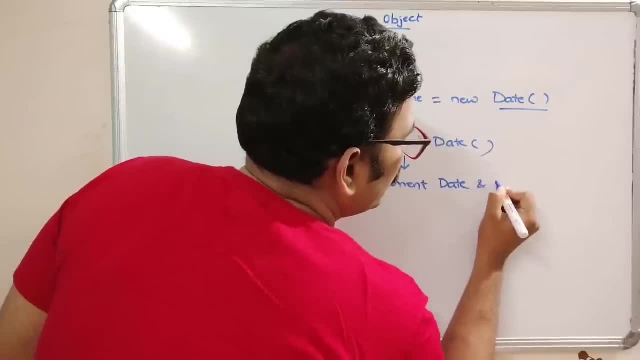 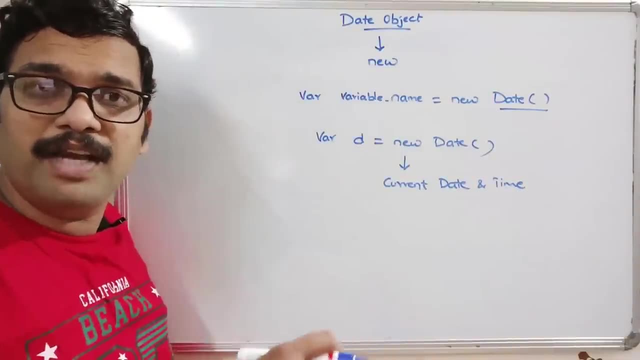 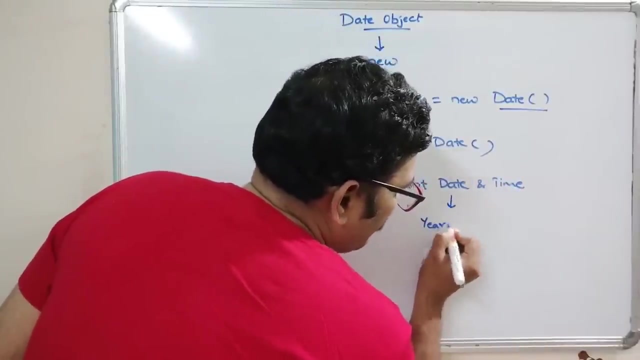 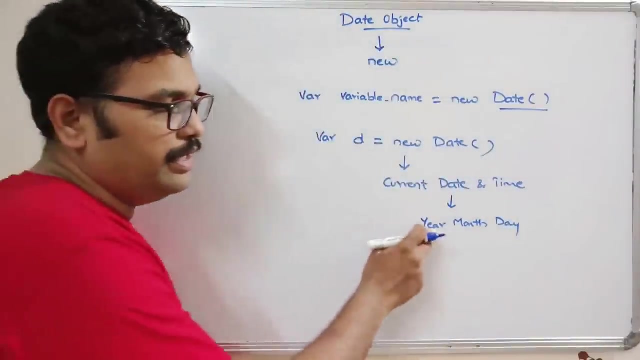 current date and time. current date and time: okay, so this will be a dynamic. so whenever you refresh the page, automatically it will return the current date and time. so in terms of date, we'll get year, month, day. so three attributes for date: year, month and day for. 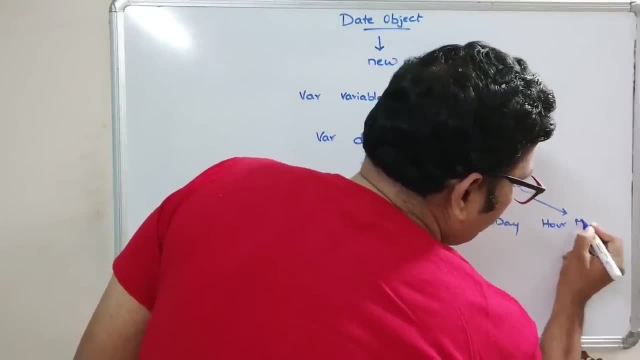 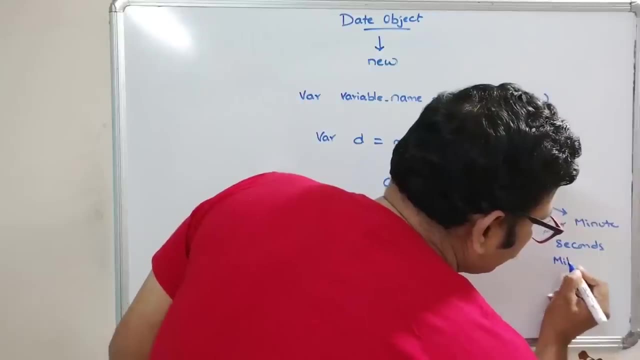 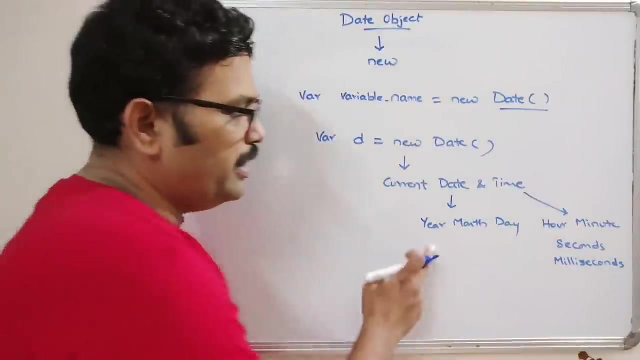 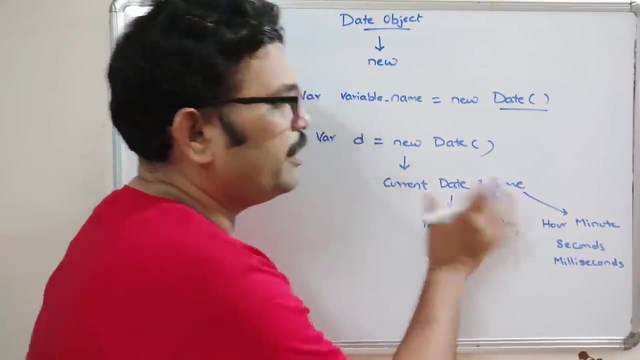 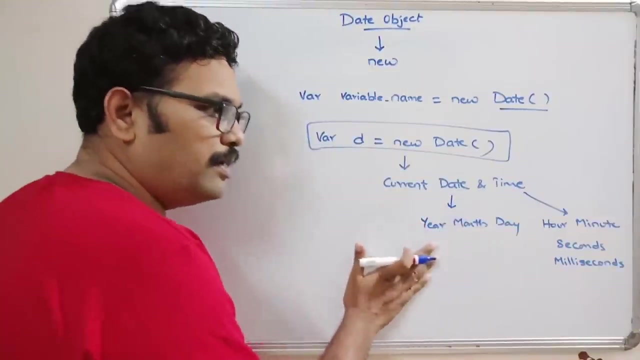 getting a time, we'll get hour, minute seconds, milliseconds. so four attributes for time. okay, so year, month, day, hour, minutes, seconds and milliseconds. so these are the attributes for date and time. so if you go with this statement immediately, we will get the date and time: the year, month, current year, current month, current day, current hour, minute seconds. 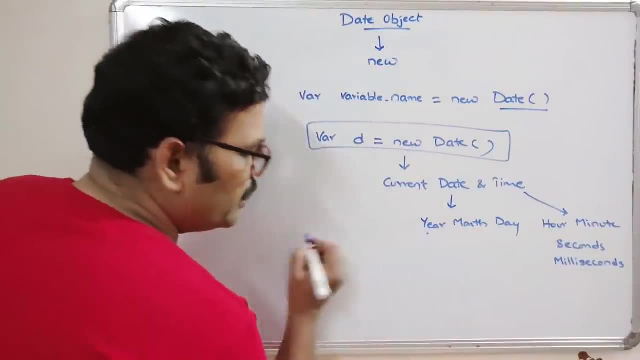 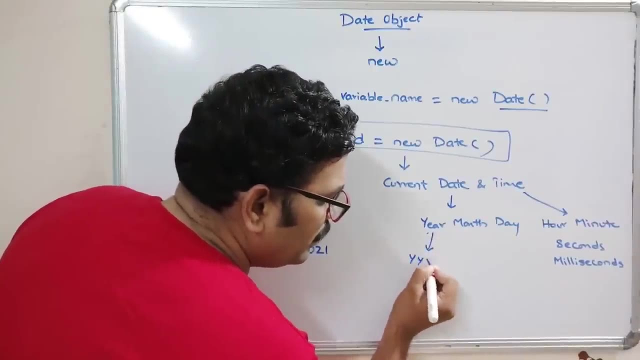 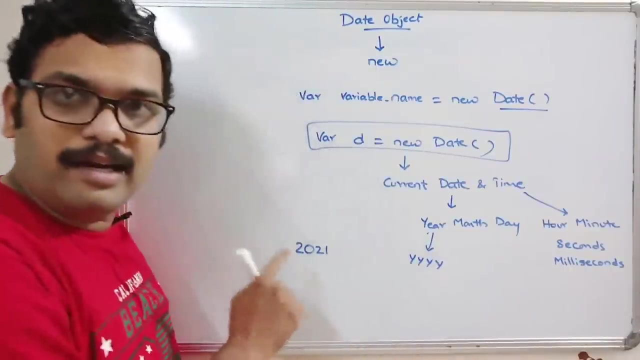 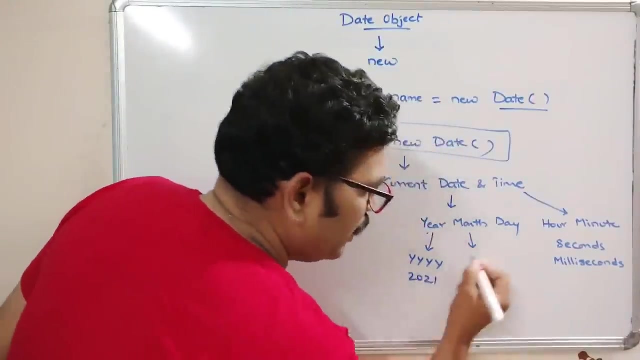 and milliseconds right. So, for example, here is some 2021 month, So here. so this will be 4 digits right, 4 digits right, and this will give the current date and year right. So this month, month will be so this is 2021 and this is January and this will. 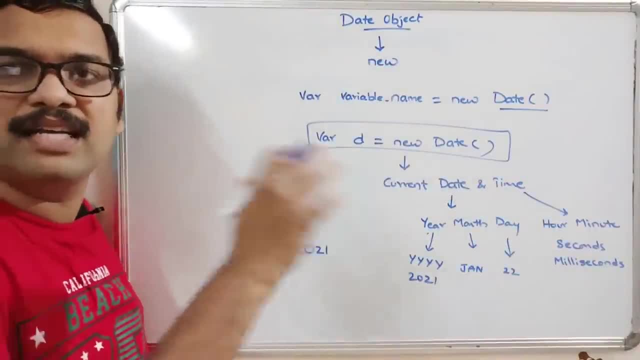 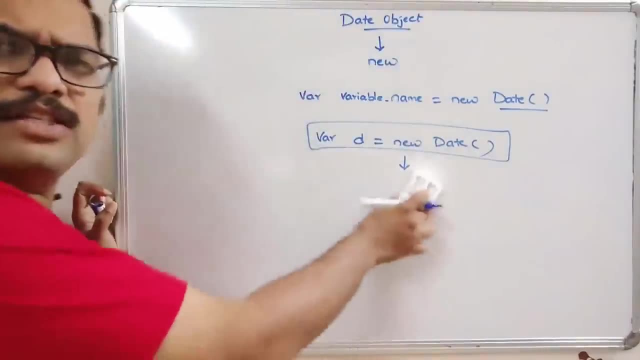 be 22 and hour minute seconds. present hour minute seconds will be displayed here, right? So this is one way to create the date object. So there are different ways to create the date object. One is by using the date method, right? So we have to use this one. So we 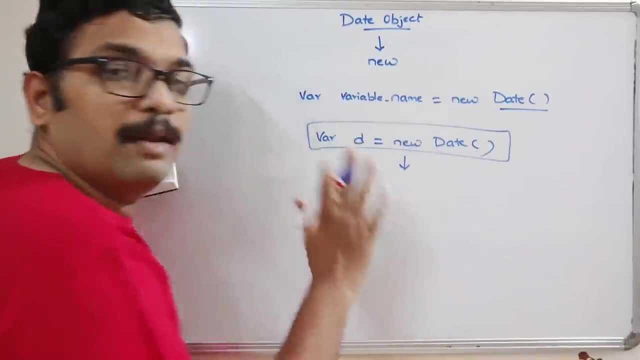 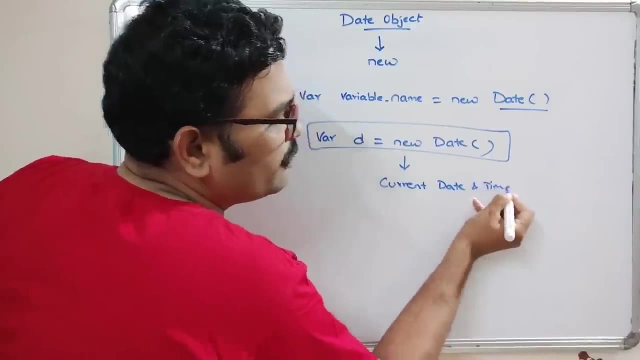 should not give any parameters inside this one. So if you do this, you should get the date of the month. So what did you learn? So are not giving any parameters automatically. it will give the current date and time. current date and time, right. so this is the first way. the second way, similarly, where d is equal to new. 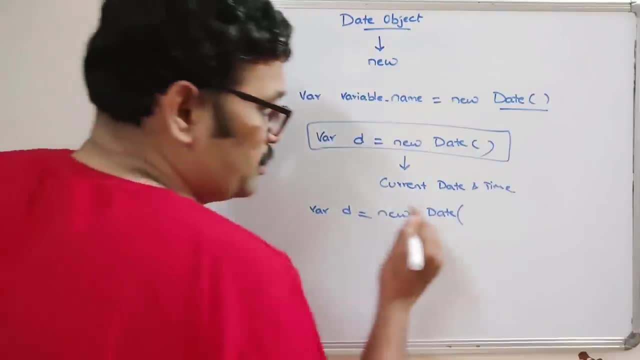 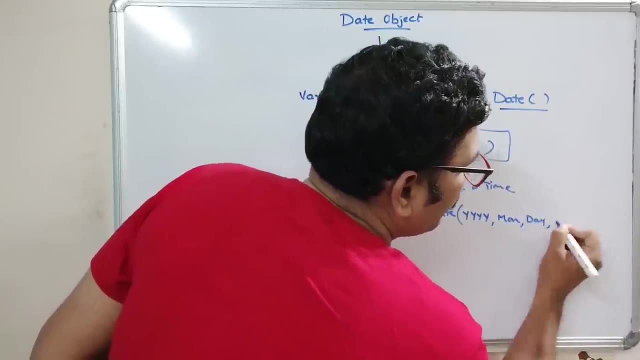 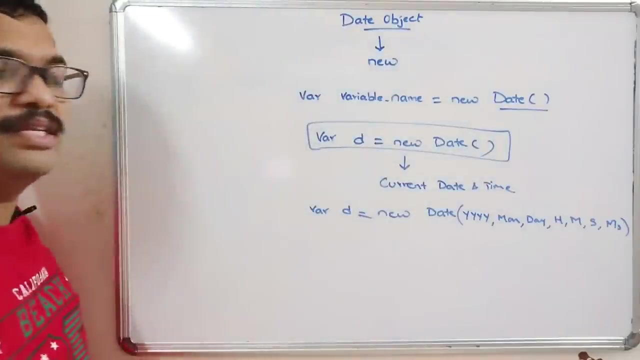 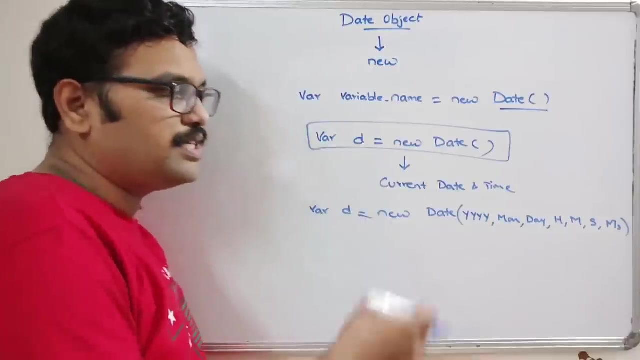 date of here you can give all the seven parameters right. so year, month, day, hour, minutes, seconds, milliseconds, milliseconds, so all the seven parameters we can give here so that this is a static. that means whenever you refresh this page you will get the same date and time, because 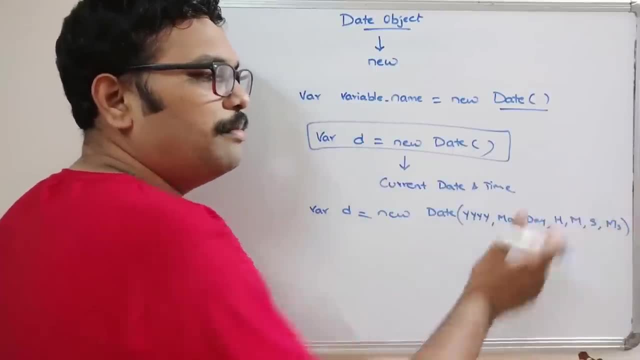 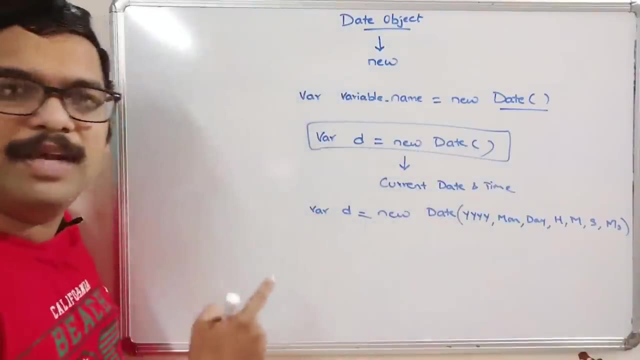 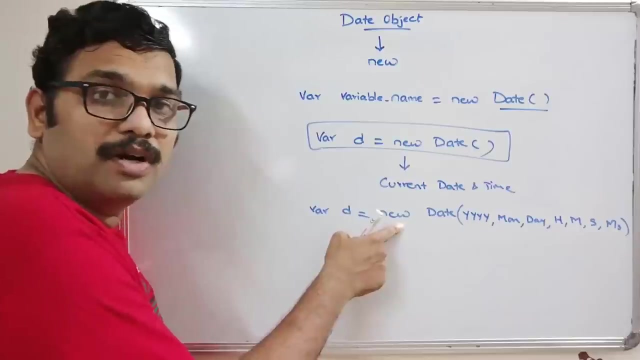 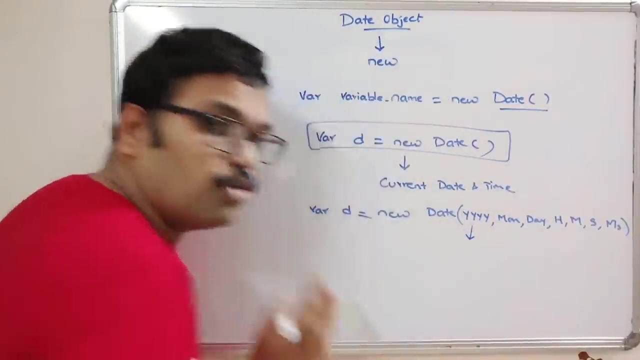 we are fixing the year's, month, day, our minutes, seconds and the milliseconds. so whatever the thing you are giving as a parameters here, that date will be assigned to this d object. okay, so here d is an object because we are creating d with the help new keyword, so d will be the object, right? so here here will be the four digit, and if you give the 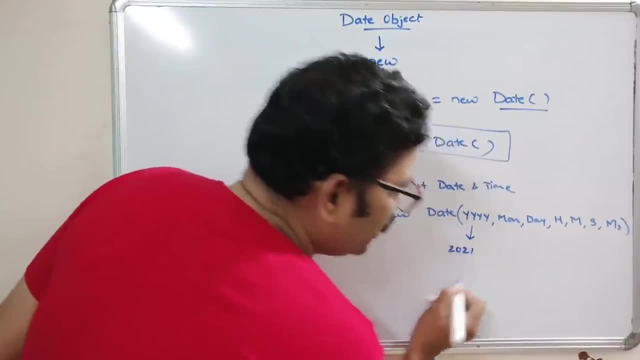 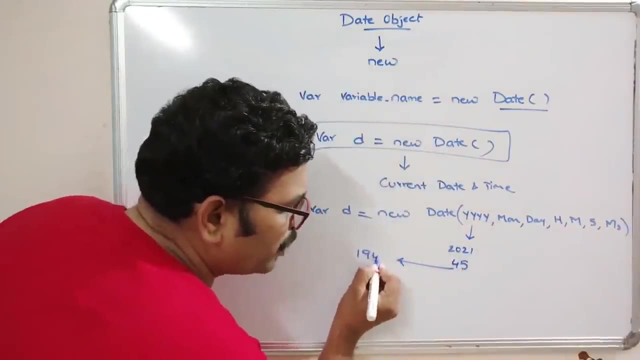 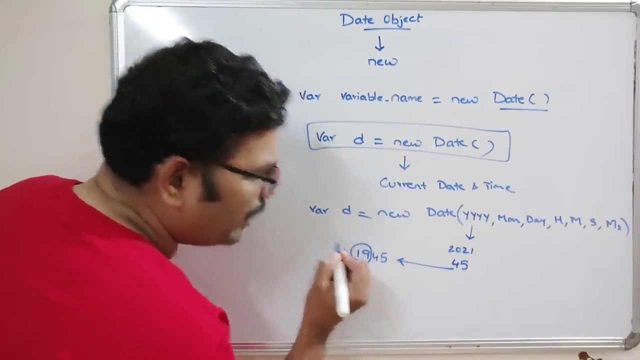 two digit. if you give the two digits. so if you give 2021, that will be the final year. otherwise, if you give some 45, this will be considered as 1945. okay, this will be considered as 1945. if you give the two digits, it will go with the. it will add 19. so if you go with some 65, it will return. 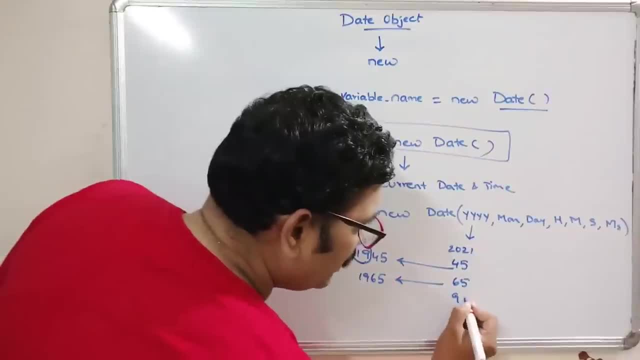 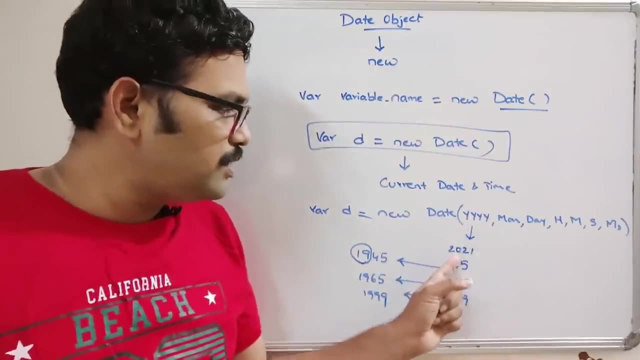 as 1965. okay, if you go with the 19, 9 again, we'll get the year as 99. so this year should be four digit. if it is 2000, so and so, and so from 2000 year onwards it will give four digit, and if you. 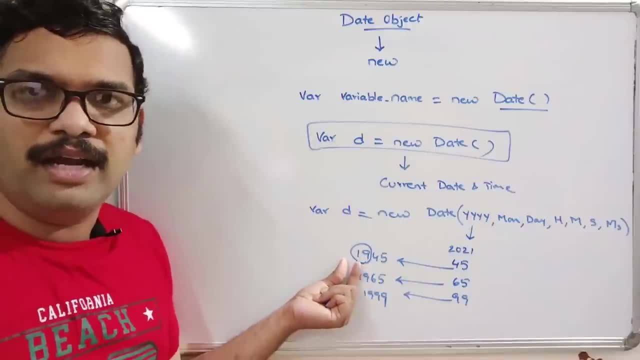 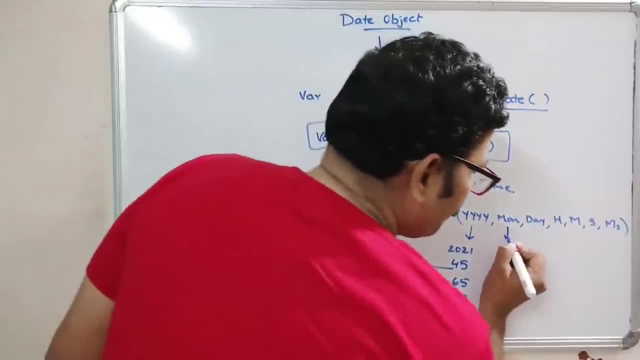 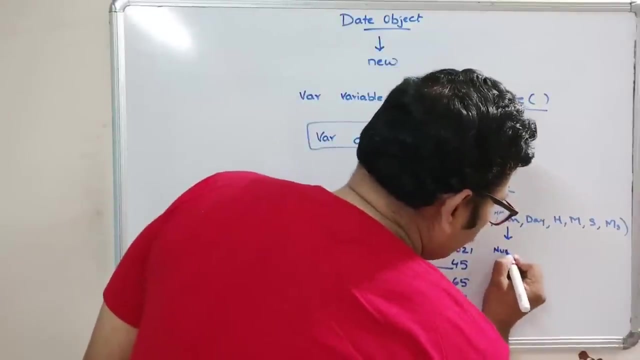 give only two digit, automatically it will go with the 19 000, 1900. okay, 1945, 1966, 1969, so and so. and coming to the month, coming to the month, so here the month will be represented in terms of numbers. okay, it will represented in terms of numbers. 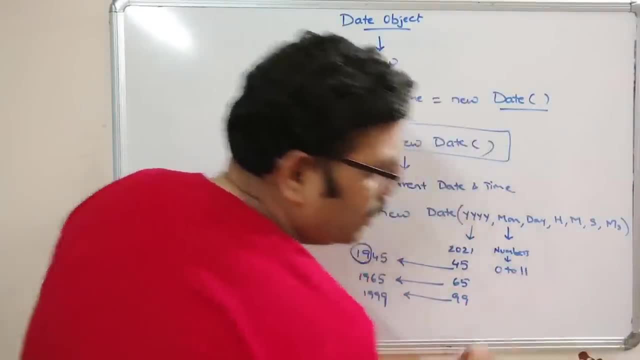 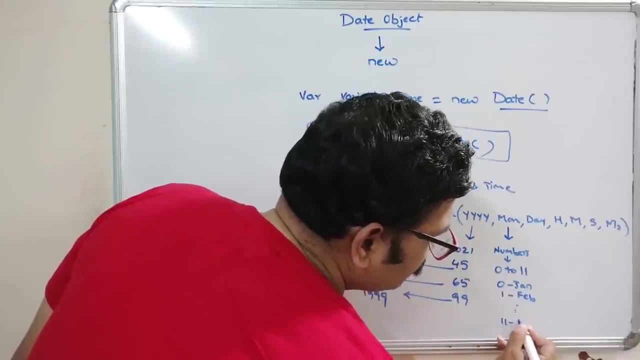 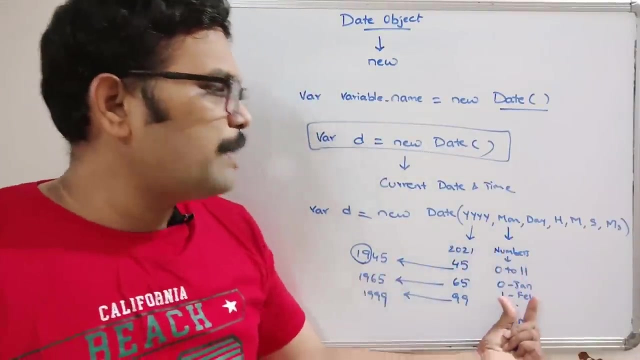 so these numbers can be from 0 to 11. so 0 is for january, 1 is for february, and so on. 11 is for december, 11 is for december. so like this, this numerical representation should be given for this month. okay, and there we know that the day can be represented in terms of. 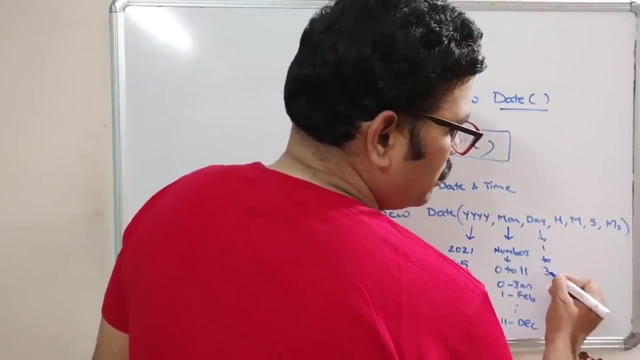 that the one day can be represented in terms of hours. that day can be from 1 to 31. okay, the day can be 1 to 31, and similarly hours. hours, so 24. 1 to 24. 0 to 24. and similarly Zoom浩. ok, they can be one to 31, and similarly hours. hours, So 24. 1 to 25 inches difference. 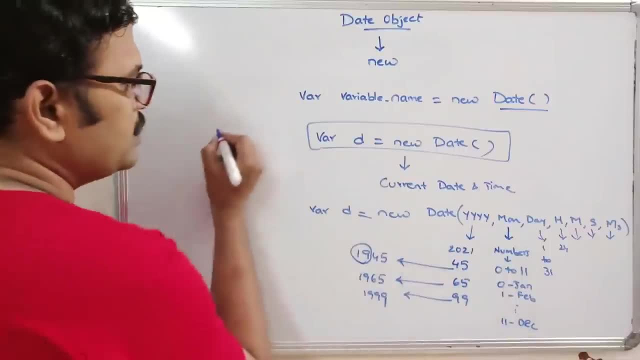 minutes, seconds and milliseconds. so we know that milliseconds means thousand. milliseconds is equal to one second right. so we can give accordingly, we can give the value accordingly. so don't forget how you change every case executing a small January means the day is possibletu. 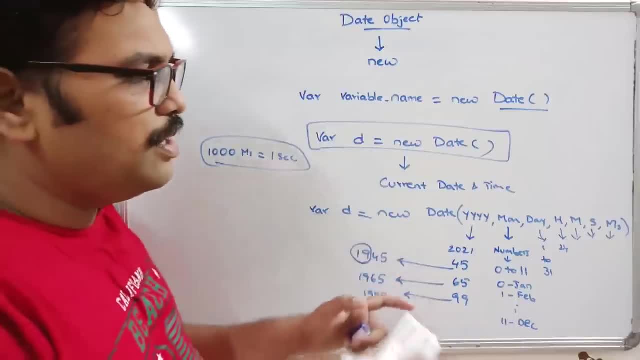 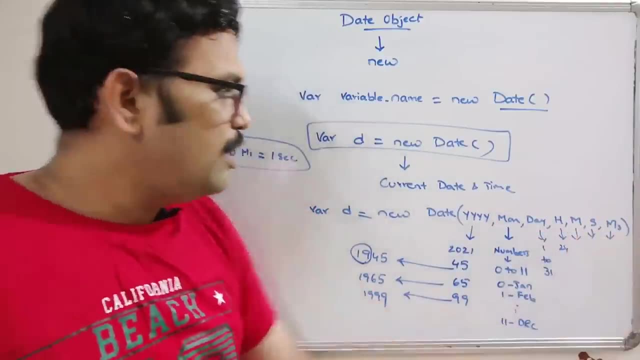 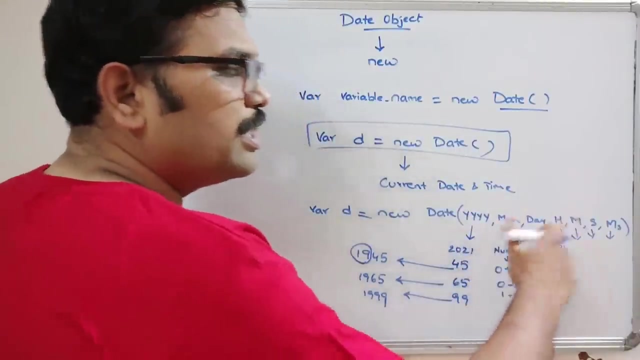 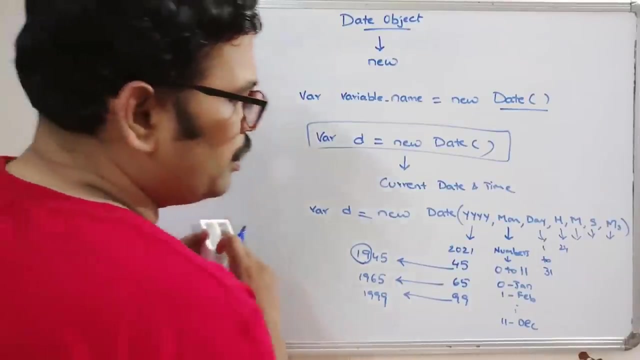 by executing small code. right? so this is the syntax for creating an data object in another line. that means we have to give these parameters different parameters, and we can also restrict these parameters. we may not give the seven parameters, and if you give only three parameters, the remaining parameters will be set to zero. okay, so that means if you give here the year as 2021, 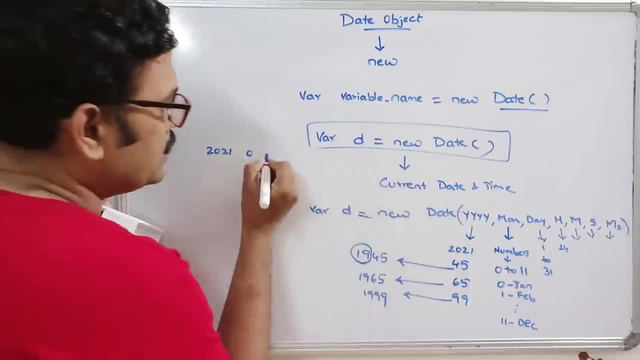 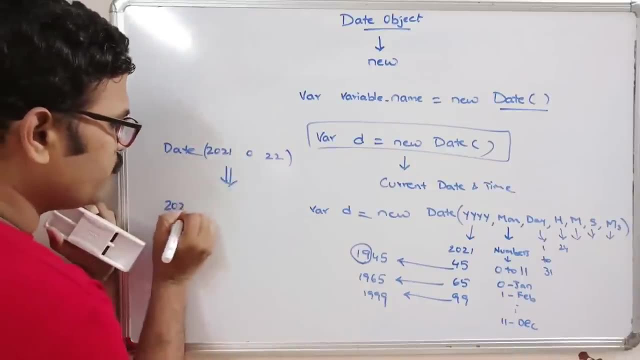 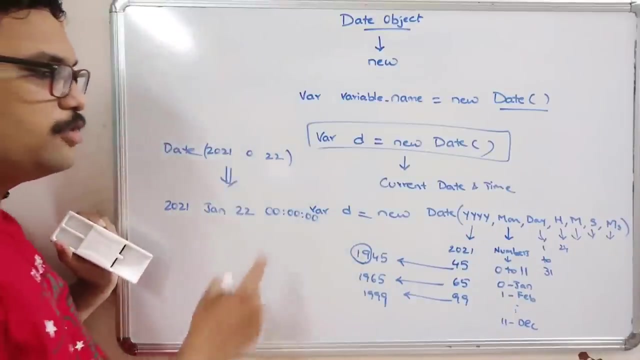 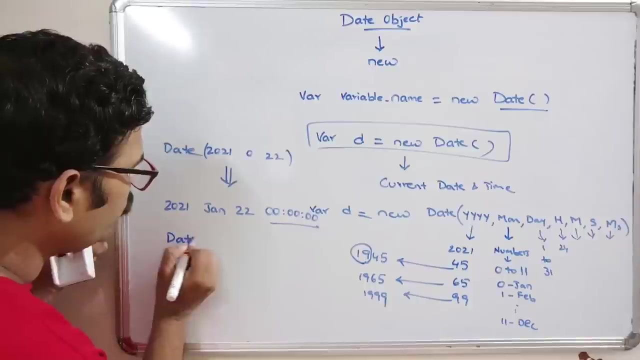 and a month as a zero and day as a 22, and that's all right and that's all date function. so this will return 2021 january 22: zero hours, zero minutes, zero seconds. so because we are not giving any other parameter right. so that's why it will set to zeros and if you go with some, only two. 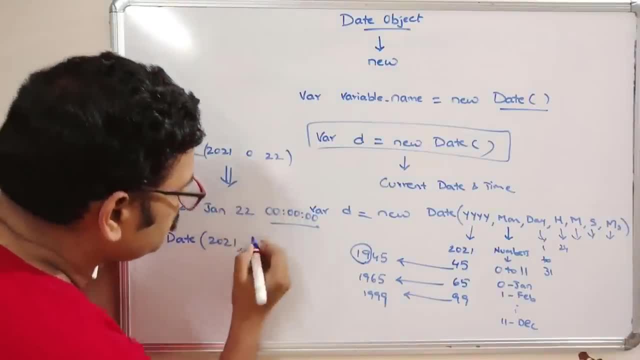 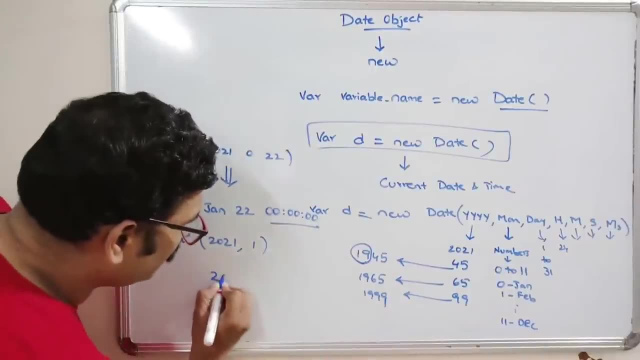 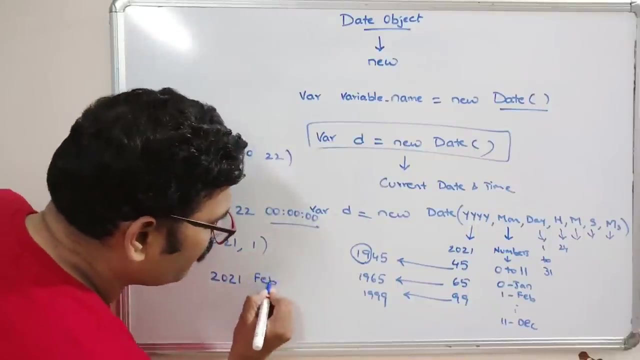 parameters: 2021 and some one okay, so we are giving only two parameters. first, one is a year mismanagement month, so here it will return: 2021, jan. sorry, one represents the month right. one represents the month february- february, and we are not given date here, so that's why, by default, it will be one. 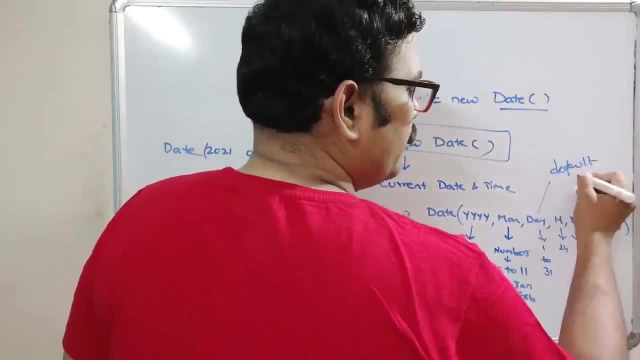 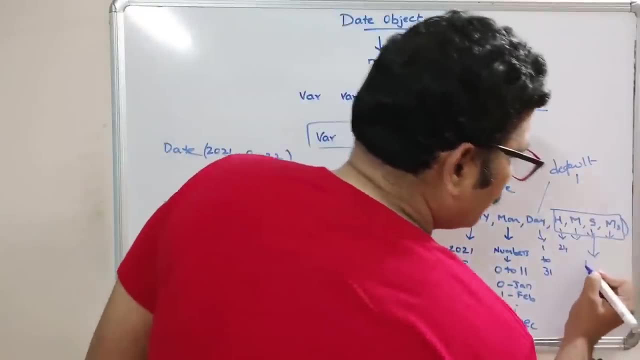 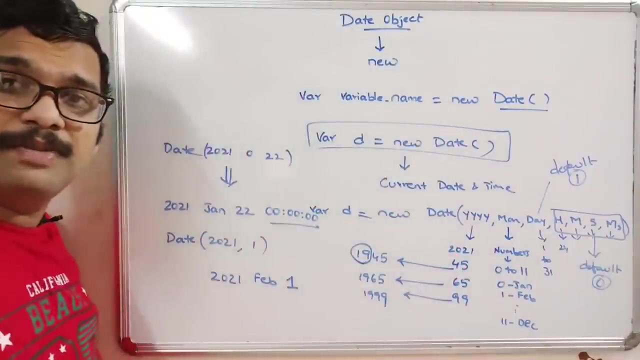 so the day? by default. by default, it will be one. by default, it will be one. what about all these things? by default? default, it will be zero. okay, by default, these hours, minutes, seconds and milliseconds will be zero. so if you are not giving any parameter here, automatically it will be set to zero if you are. 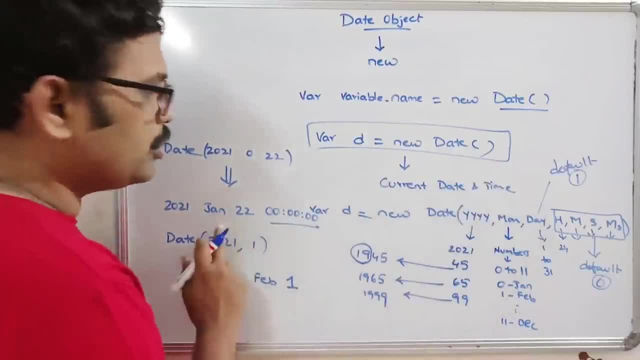 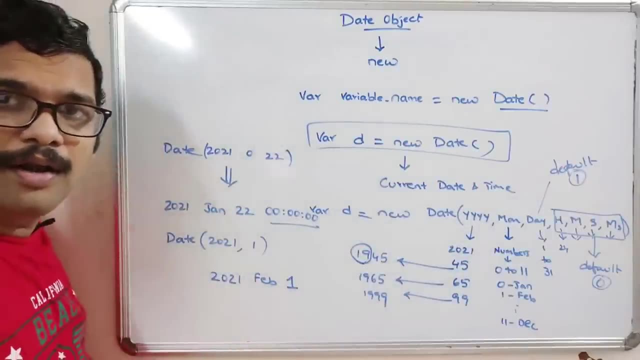 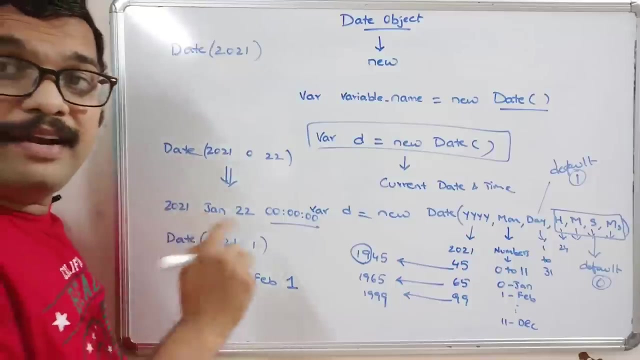 giving any parameter, that will be set right. so for month also, if you are so sorry, for day also. if you are not giving any number, it will by default it will be as one, okay. and if you give only the thing date, some 2021, this will be treated as a millisecond. so this one parameter, it doesn't. 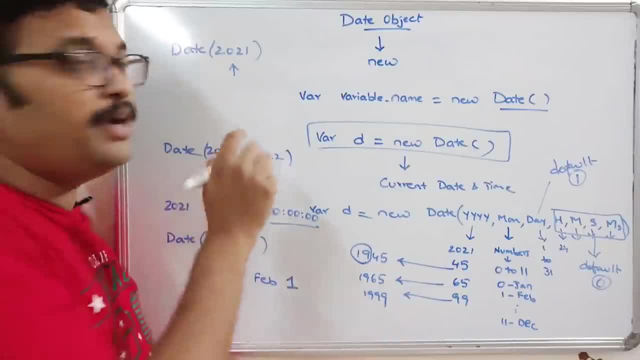 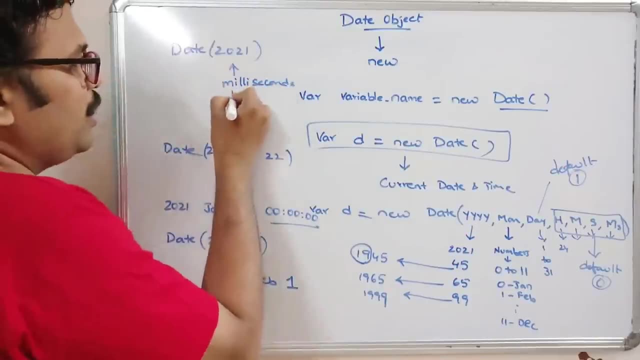 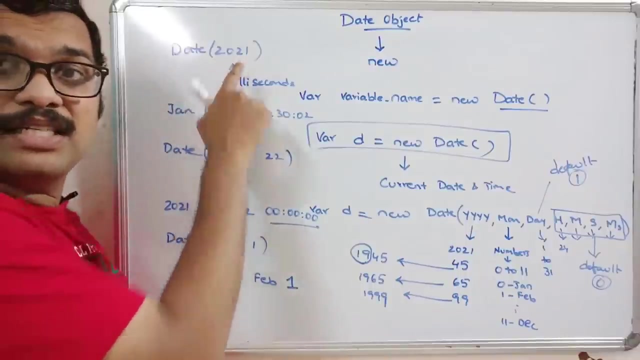 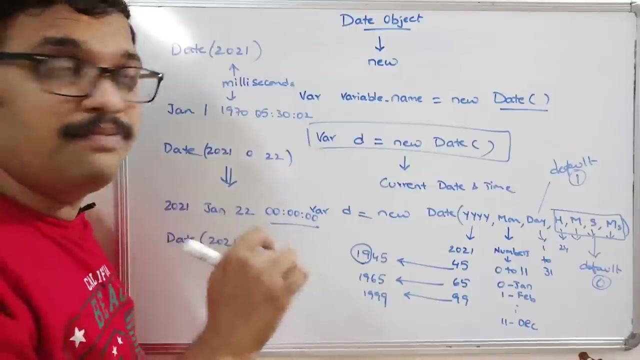 i mean consider this as a year. so if you give only one parameter, this will be treated as milliseconds, milliseconds, right. so automatically we'll get the result as january 1 1975, 30 02, because 2000 milliseconds is equal to two seconds. so that's why this two seconds will be here. okay, hours, minutes two. so by default, by default. 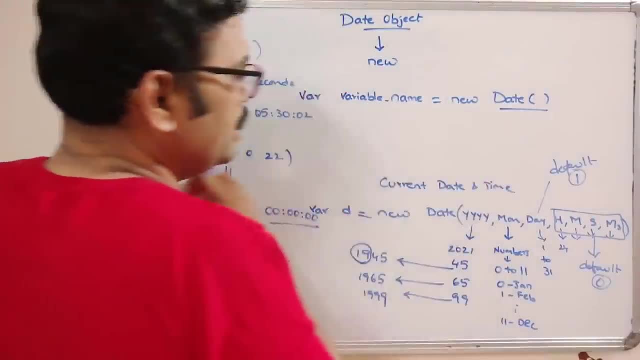 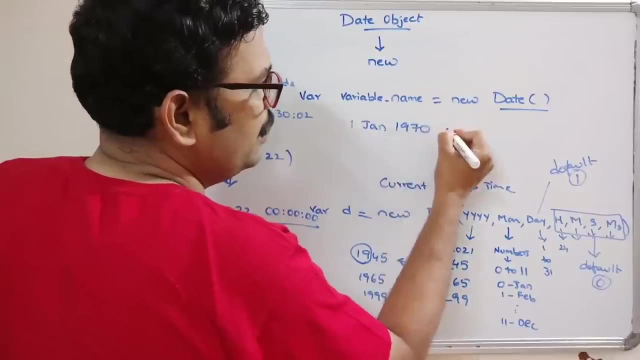 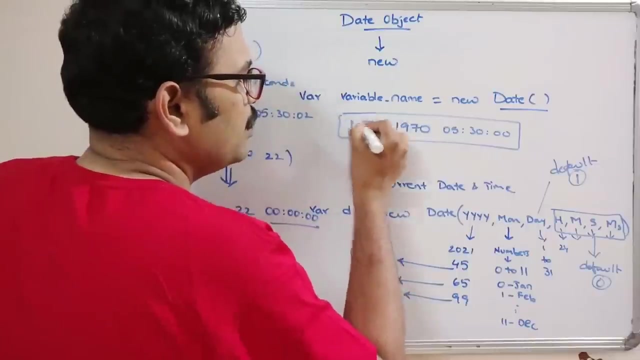 here. uh, by default date is first january 1970, 거예요 5, 30.. so this is the default date in a javascript right. this is the default date. so if you give only one parameter, that is, 2021, that will be treated as a. 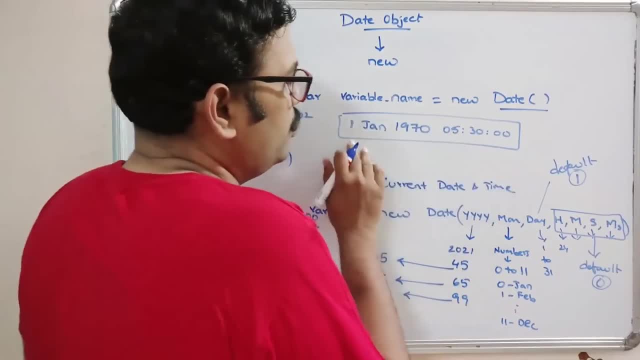 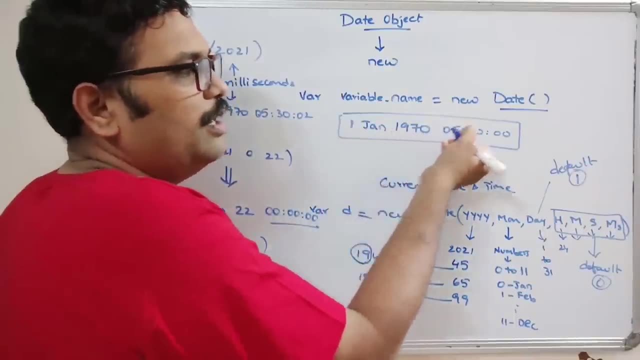 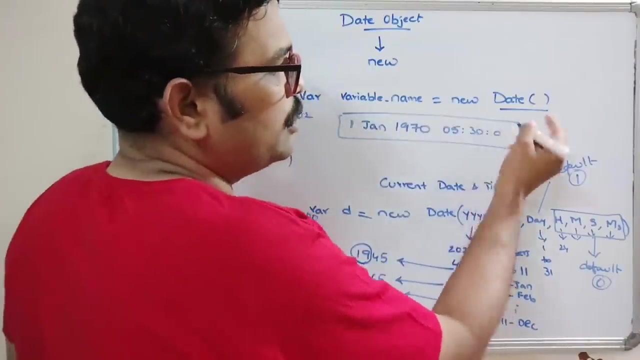 millisecond and that milliseconds will be set in here, so you are not giving any other parameters. automatically. it will go for this default date. so 1 january 1970, 5, 30 and instead of 0, 0, we are giving some 2021 milliseconds. that is equal to 2 seconds, so it will come as a 2 right, so minimum. 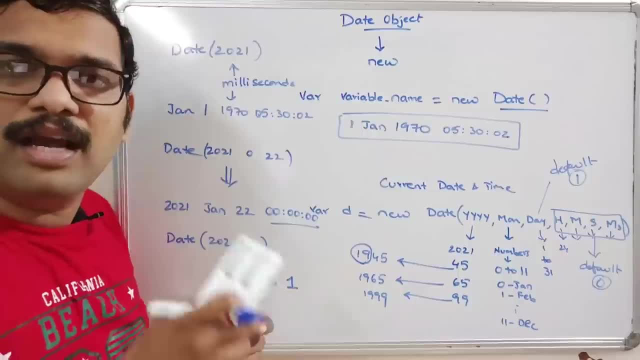 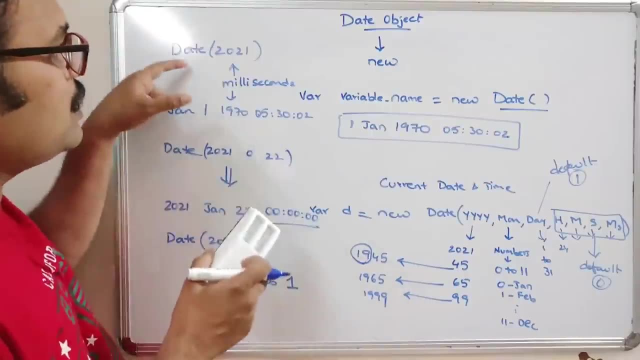 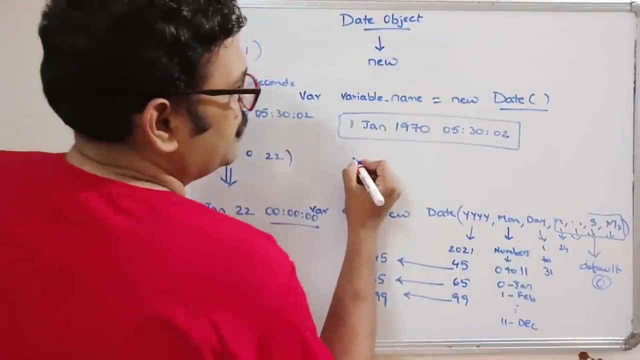 we have to give two parameters: one is a month and another one is a year, right? so if you are not giving like that, it will consider as a millisecond. so this is the third way of creating a data object. this is the third way of creating the data object. see where d is equal to new. 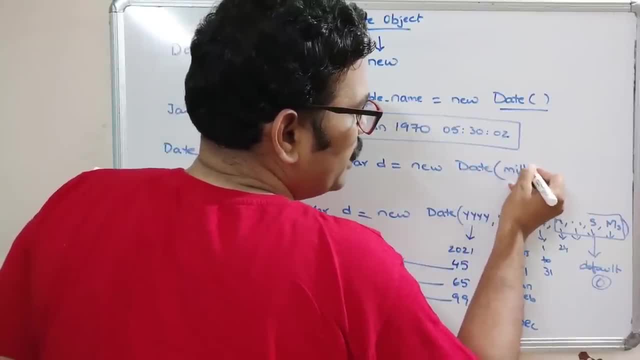 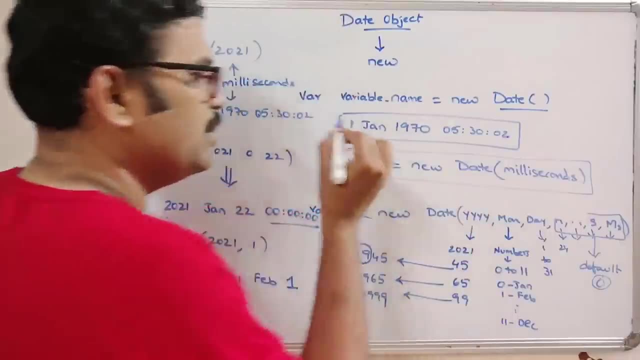 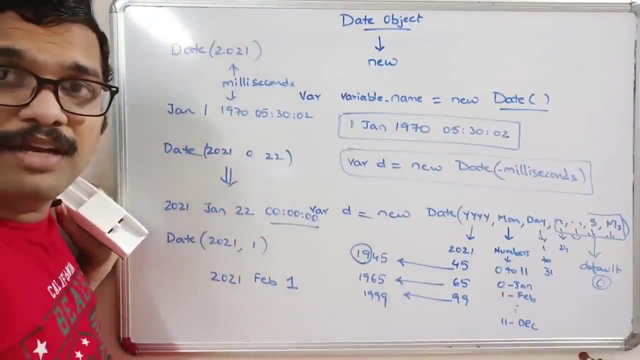 date and here it will be the milliseconds. so we need to give the milliseconds here. so this is the third way. this is the third way to create the date right. so if you give negative to the milliseconds, okay, if you give the negative milliseconds, so that milliseconds will be. 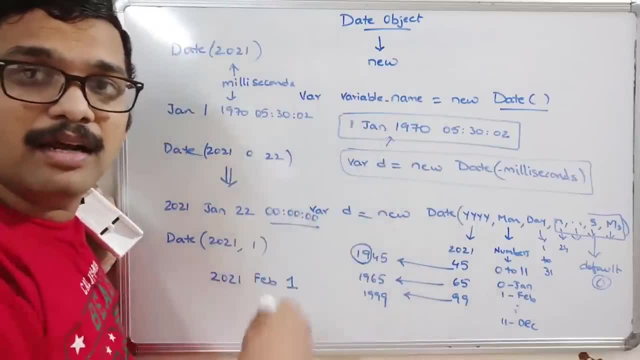 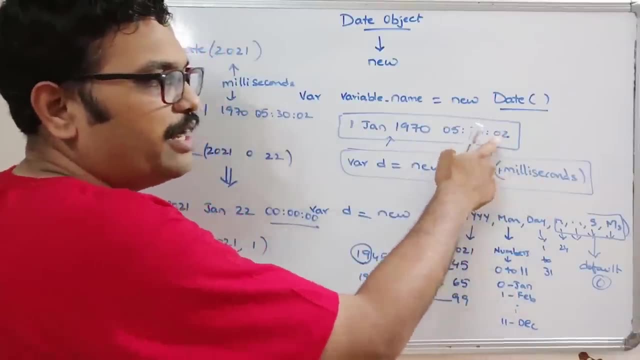 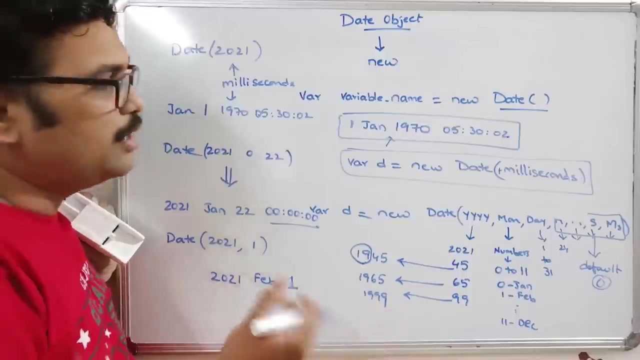 decreased from this date and the resultant date will be displayed. okay, so if you give plus milliseconds, that many milliseconds will be added to this date and the resultant date will be displayed. so i will show you an example for positive and negative. okay, don't worry about that. so default date will be this one. default date will be this one. so if you 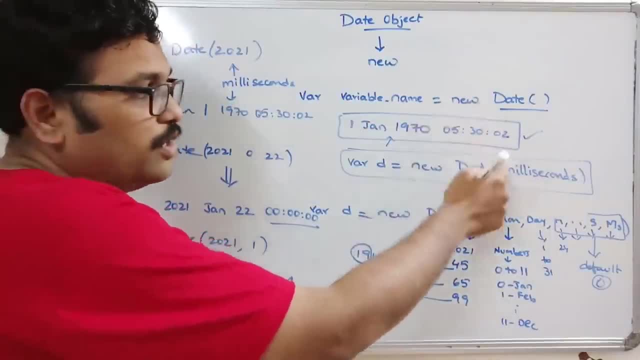 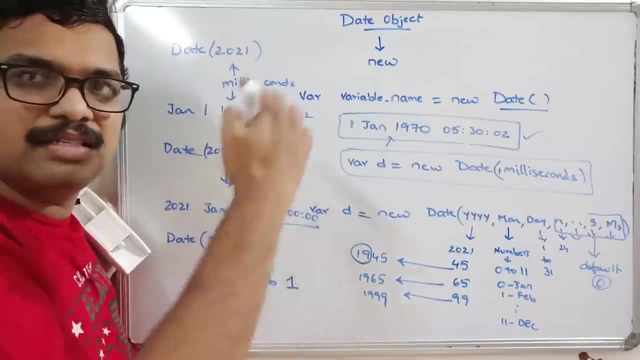 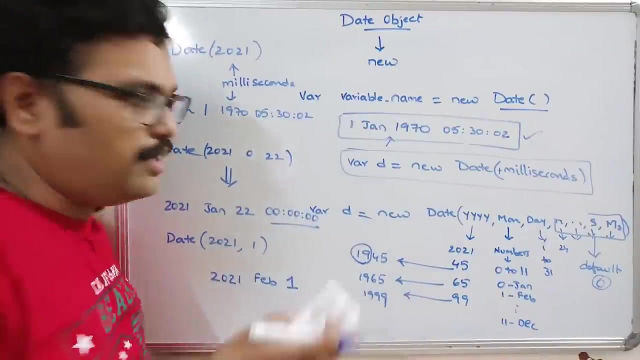 add here. this will be modified if you minus here. so if you give some negative milliseconds, it will be reduced from this date. okay, so we may get the previous years- 1969, 1966, like that- right. so, and there is a one more way to create the date object, that is by taking the date string. okay, by taking 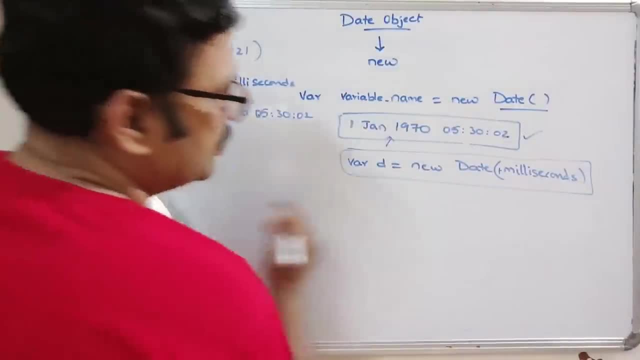 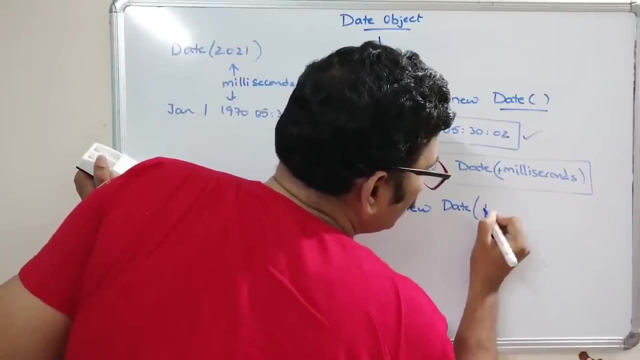 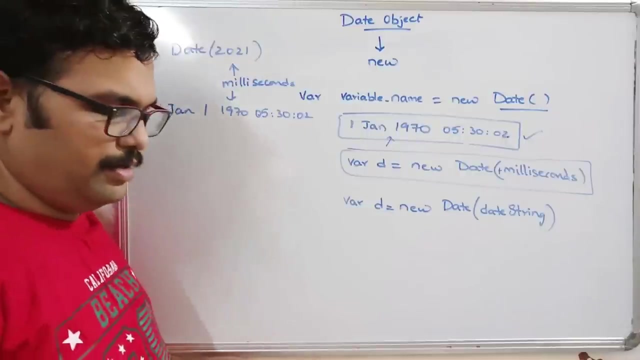 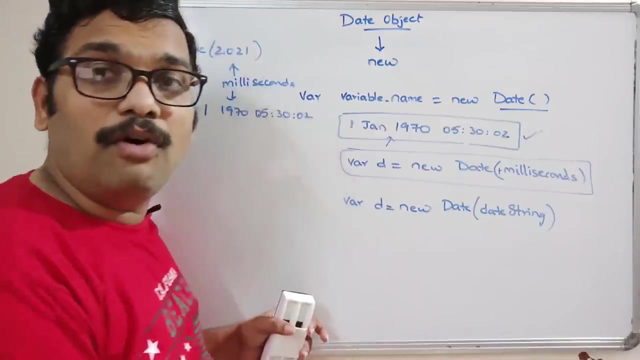 the date string. so where d is equal to new date of date string. so we need to pass a string date string. okay, we have to pass the date string. so here in the date string we have to give all the parameters. okay, in the this date string we have to give all the parameters. 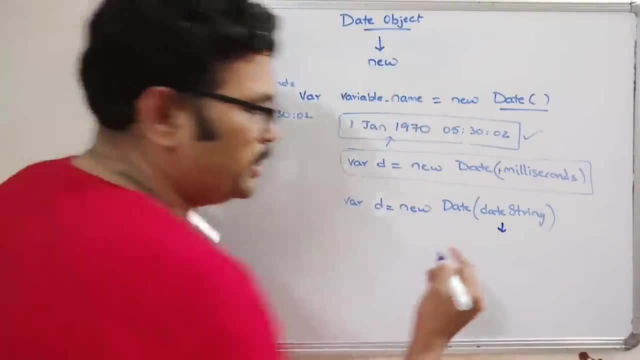 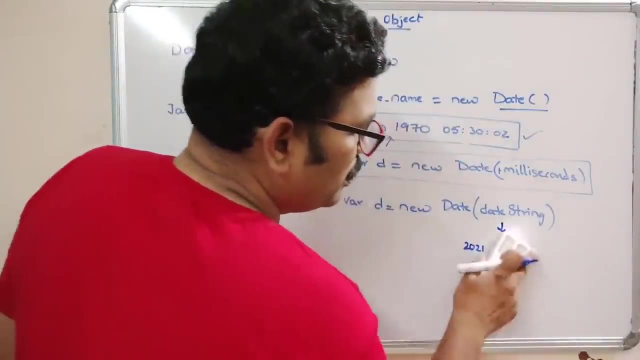 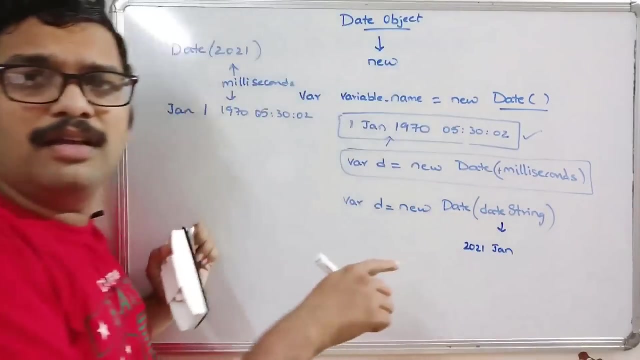 so all the parameters in terms of year, month and all these things. so 2021, 22. sorry, we need to give the. so we can also give some name like january, february, like that. okay, we may not represent in in the form of a new maker, so we can also give the name some 22 and see. 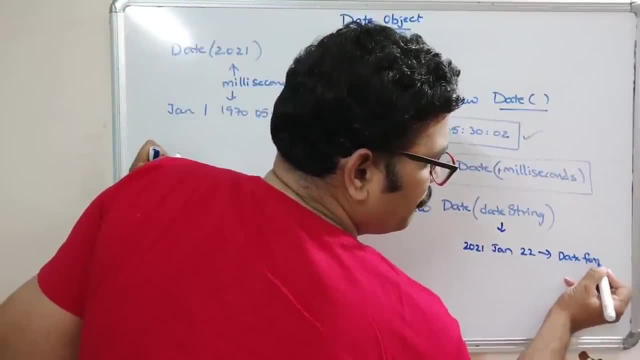 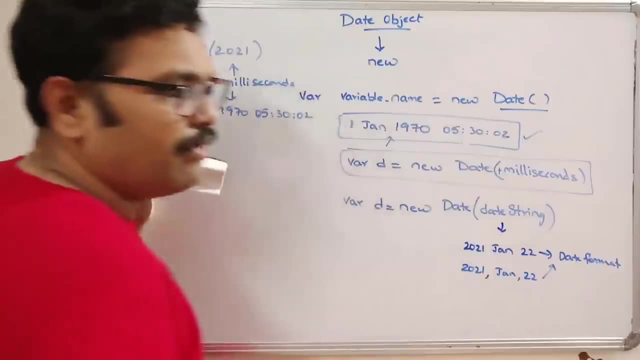 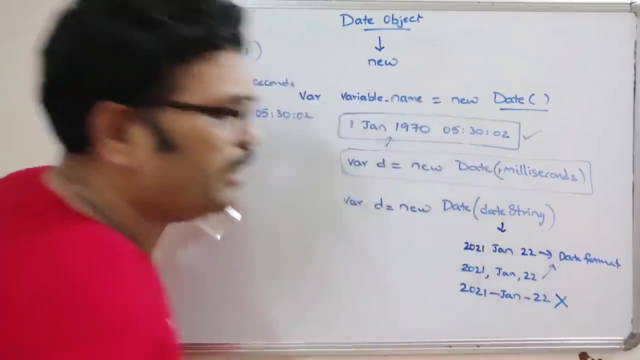 this is the date format. okay, this is the date format. this is the date format. or you can also give comma jan, comma 22, so this: this is available, okay, and 2021- hyphen jan, hyphen 22. this is the invalid date format. we'll get the result as invalid date. 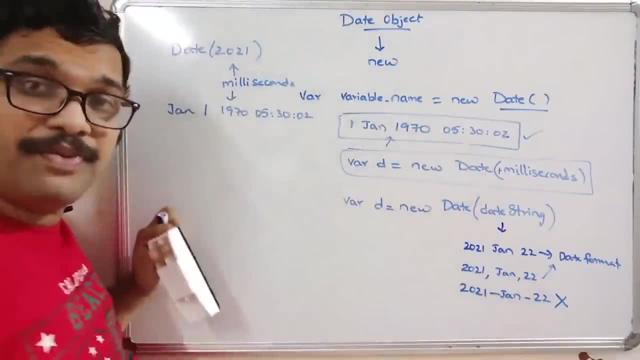 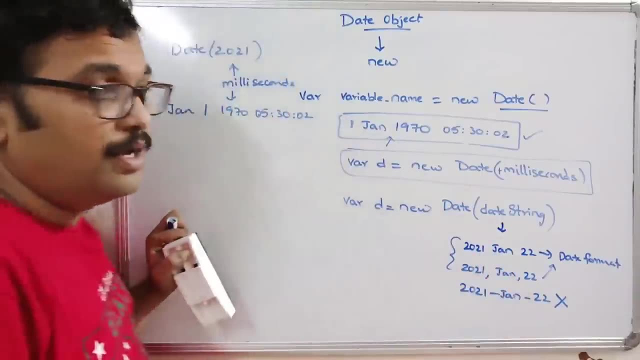 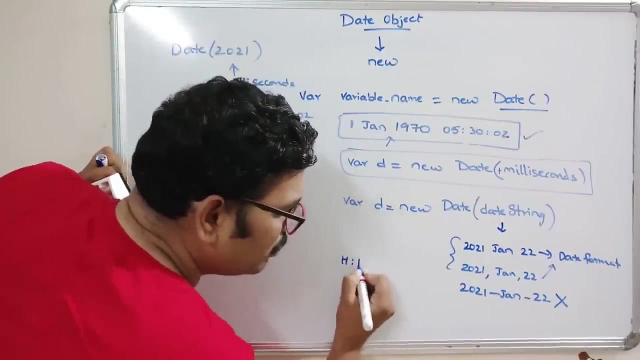 format. so we have to insert the. i mean we have to specify the date in either one among these two formats. you can use either comma or space. and coming to the time format, we have to go with this: colons hit hours, colons minutes, colon seconds, colon milliseconds. so other than these format, 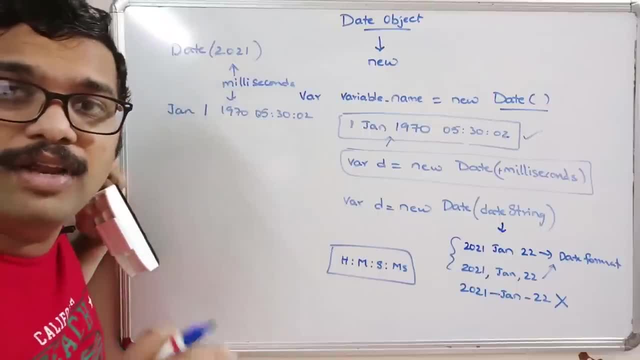 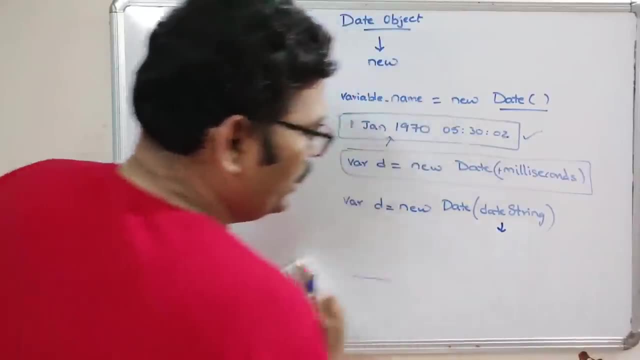 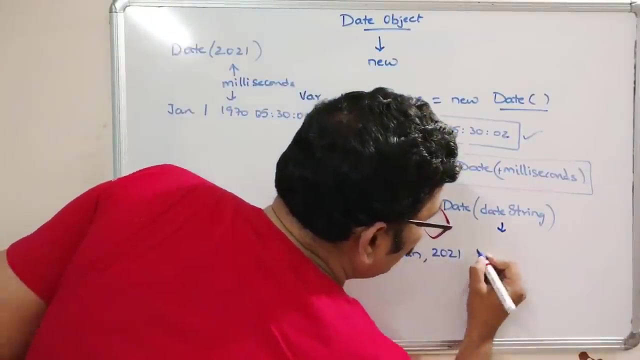 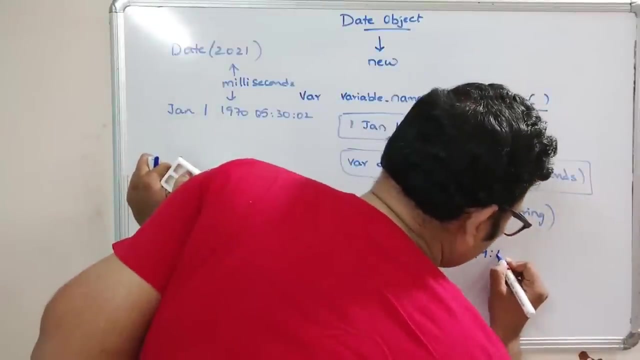 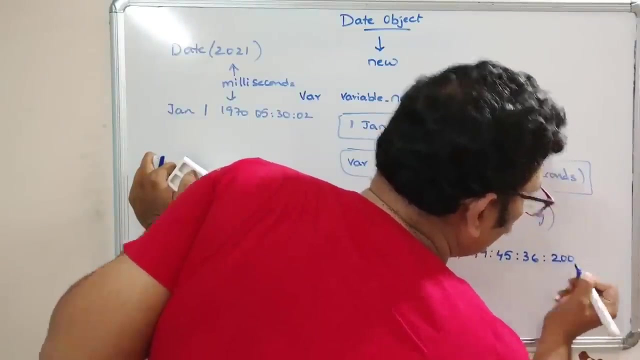 if you follow other than this format, in this date string again you'll get the invariant, okay. so if you want to specify the date string here, we can specify 22nd january 21, okay, some 19- 19 hour. that means 7, 45, 36, 200, right? so in this format we have to pass the date in in the in the 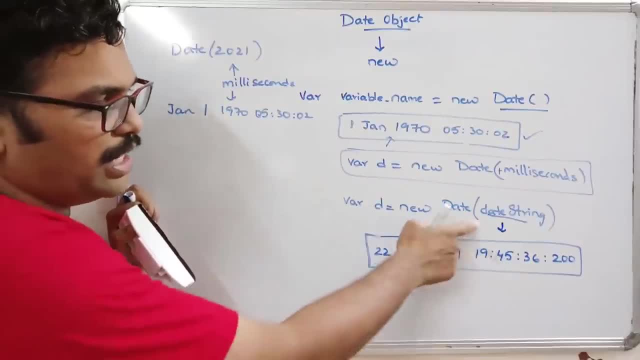 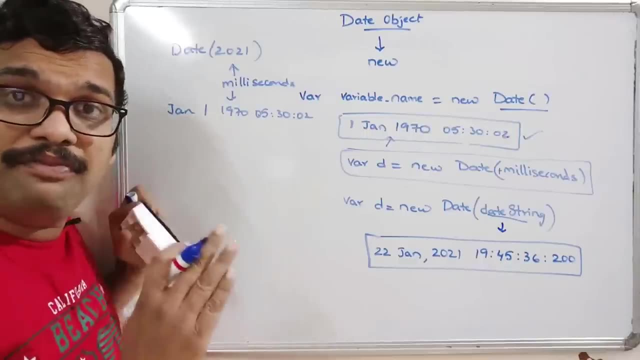 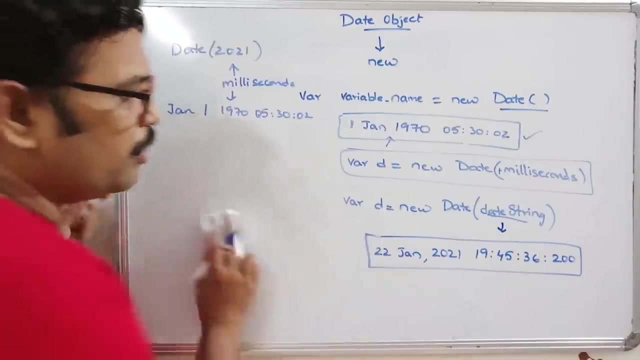 place of date string right. so this is another way to create the date object right. so in this session we have seen four different ways to create the date right. so i will demonstrate all these things by executing a small code. so now i will show you the four ways. i will write just the four ways: how 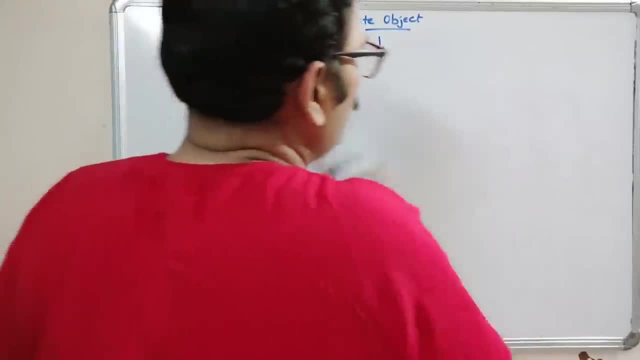 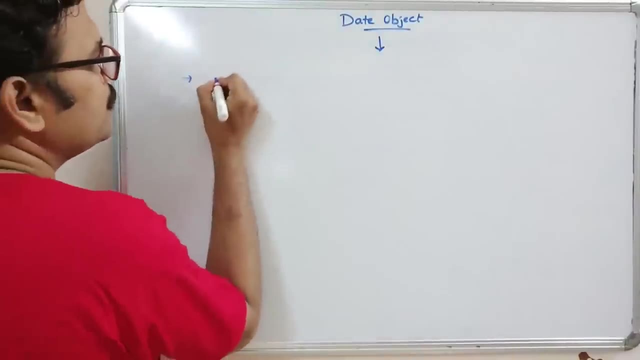 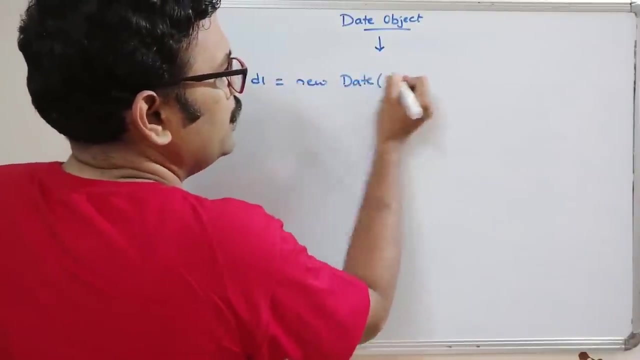 to create the date object, right, and then we move on to the computer and i will demonstrate these things. we will. we will create the date objects. so first way is where d1 is equal to new date. so so here, if you are not giving any parameters, we get the correct date and time. the second way: 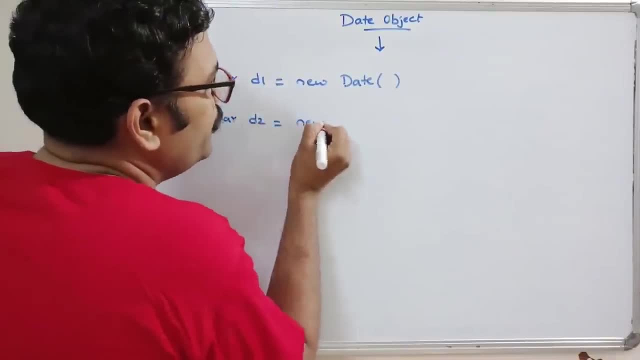 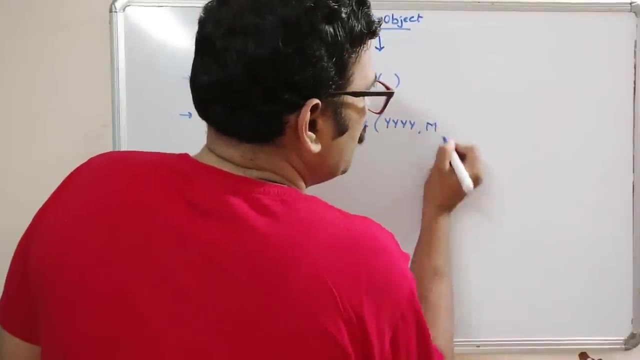 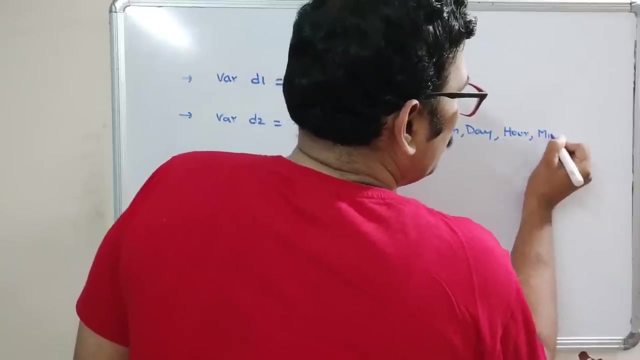 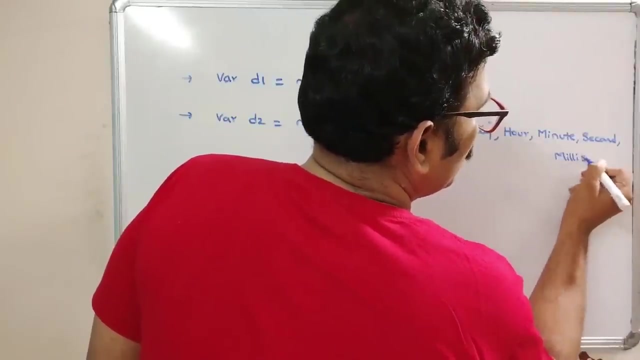 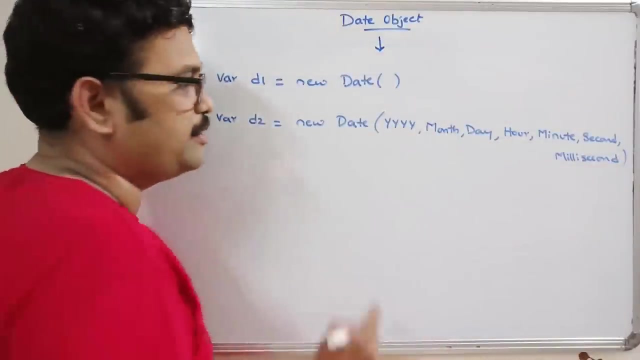 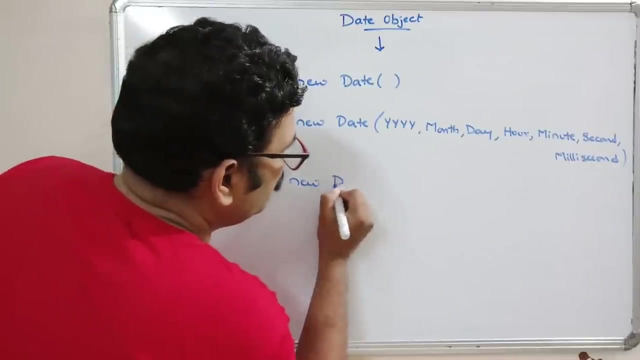 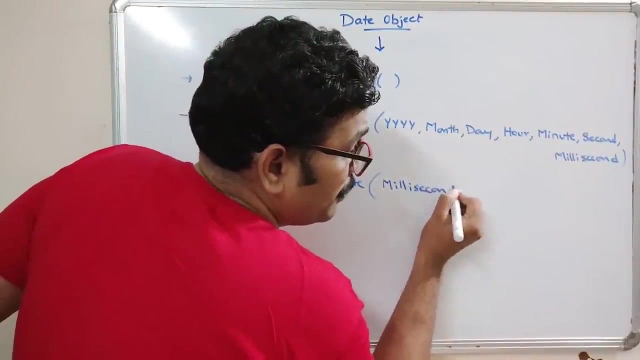 where d2 is equal to new date of year, comma, month, day, hour, minute, second millisecond right. so this is another way we need to pass all those seven parameters: d3, new, go with the date and here we can go with the milliseconds, milliseconds only. we will give the milliseconds automatically. the date will be forwarded. next, the 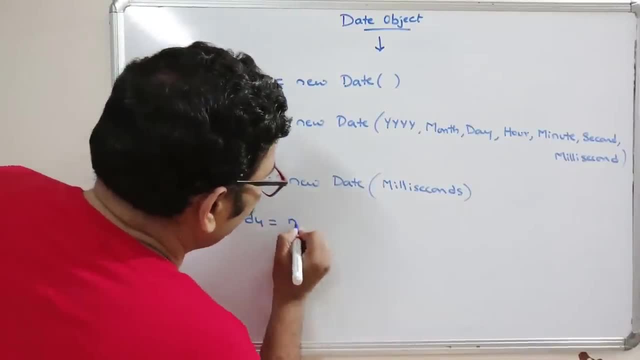 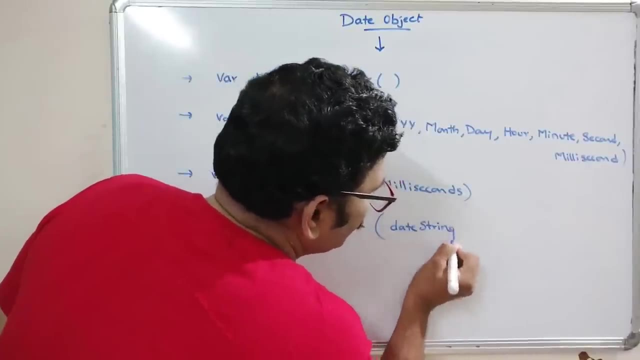 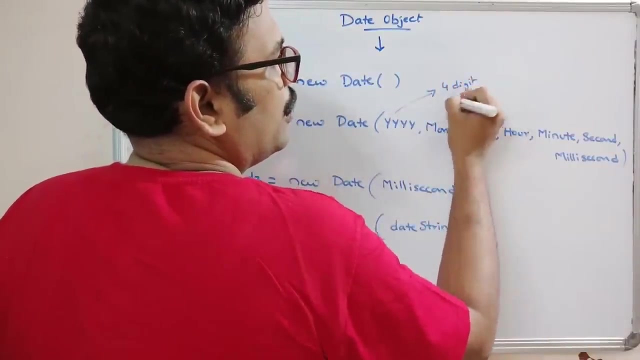 fourth one, where d4 is equal to d1, introduces it should NOT collaboration. where 4 is equal to 7 kiloseconds, equal to new date, and here we will pass the date string, date stick. so here this can be four digit and two digit. if it is two digit it will be nineteen, nineteen. 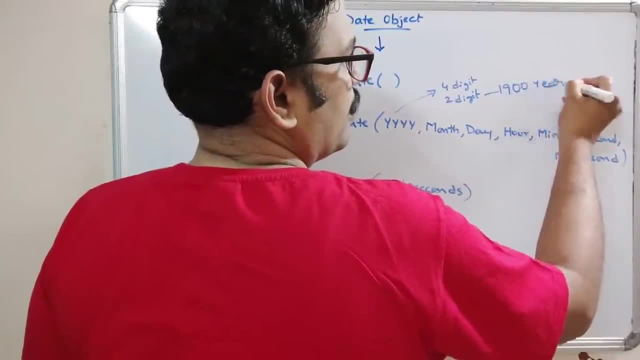 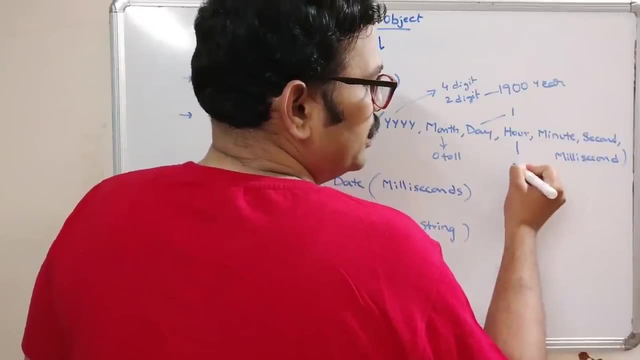 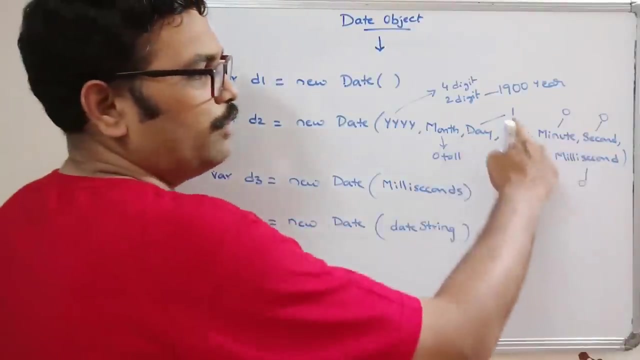 series. okay, nineteen hundred years, and a month will be from zero to eleven. they will be, by default, one, our zero minutes, zero seconds, zero, milliseconds, zero, right, so these are the different values: one zero, zero, zero. all these are the default values. okay, and this is a millisecond, and default date will be: 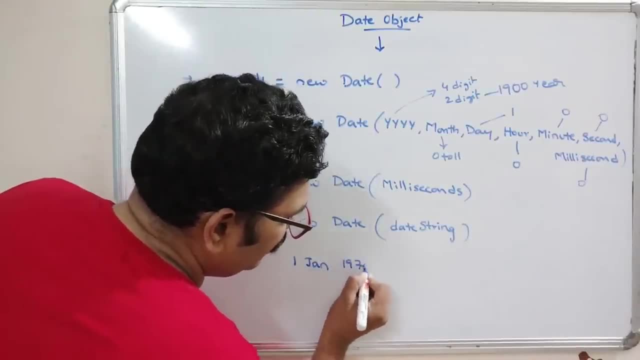 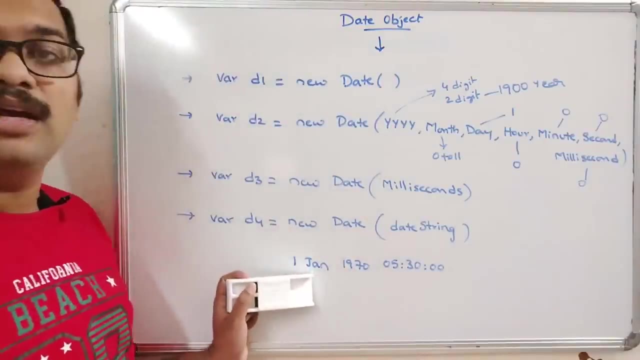 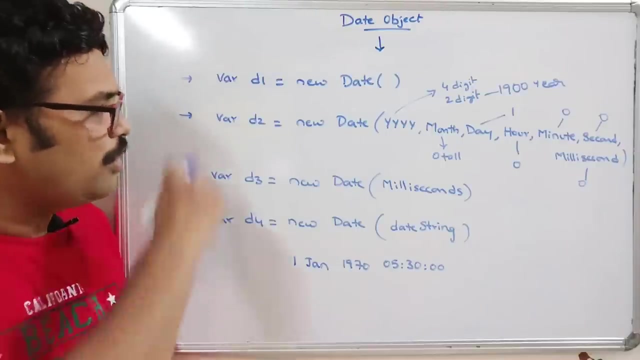 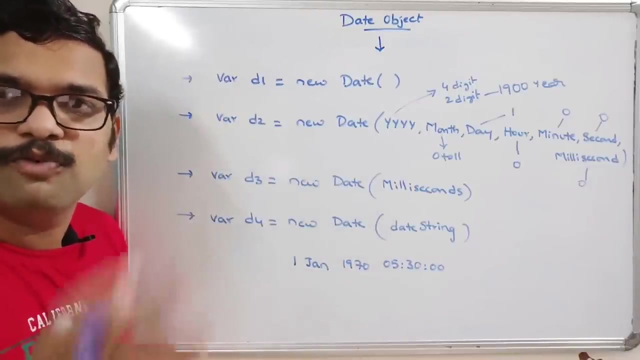 first Jan 1970, 0530. this is a default date. okay, so these are the four cases how we can create the date object. so let's talk here. I will demonstrate all these ways of creating the data object by executing a small code on the system. so let's move. 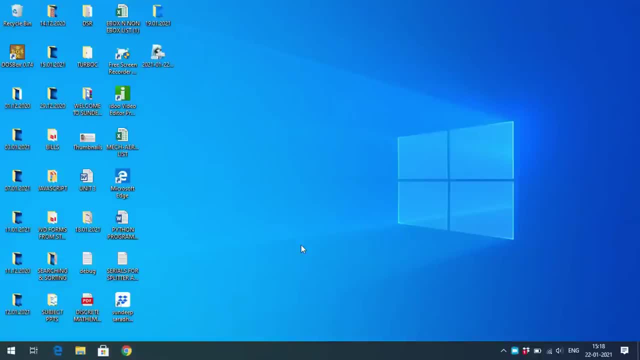 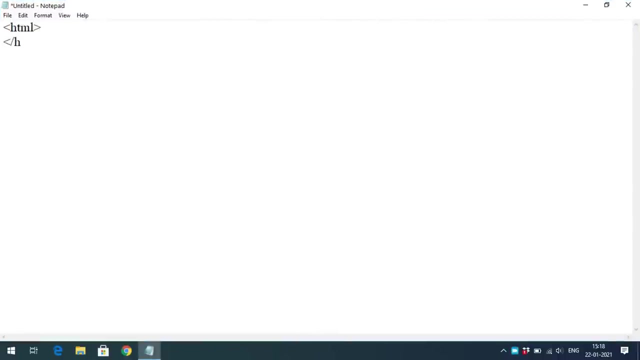 on to the system. hello friends. so just now we have seen how to create the date object right, so I will demonstrate by Medium code: HTML tag. so inside the HTML to write search table heading and we'll write the script right. so inside the body we'll write some heading. 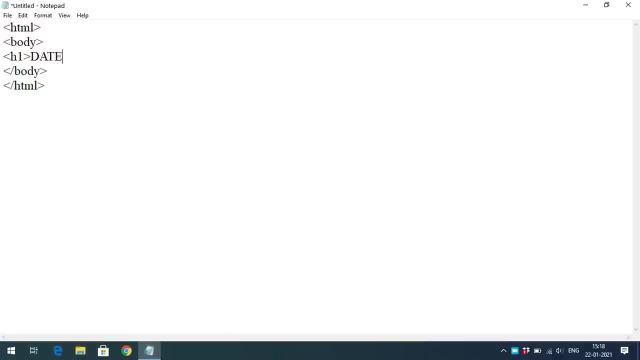 so this is for date object, right? so date object. now i will write the script here. so inside the script we'll create some dates. so we'll choose the dates in this script say: just fine, so this one we now use is second. so first one is directly by using the date function, so we'll see where D1 is equal to. 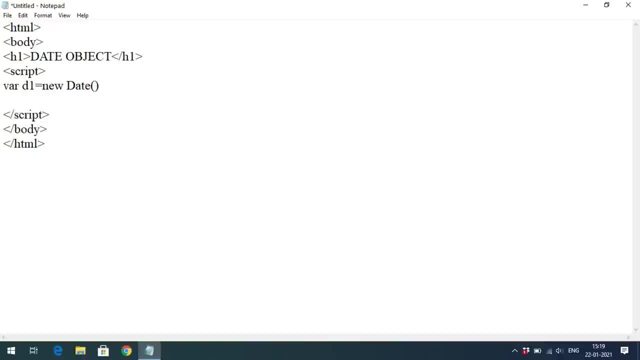 so a new late function. right, so date function. so if you are not giving any parameter here directly, it will give the current date and time. present date and time. it will give the current time. now we will print and check. so document dot write ln of d1 and I will also give the br for the next row. now let us check so. 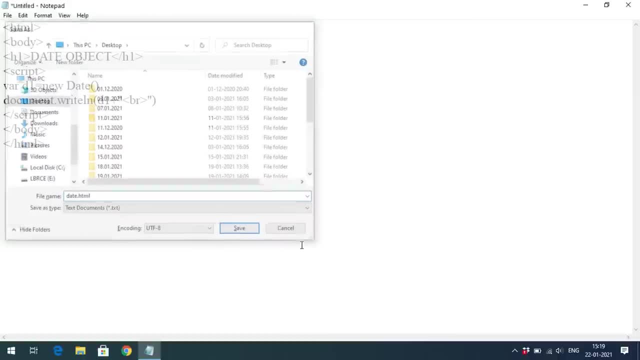 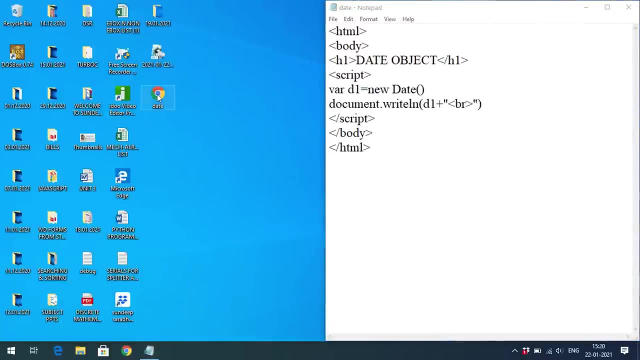 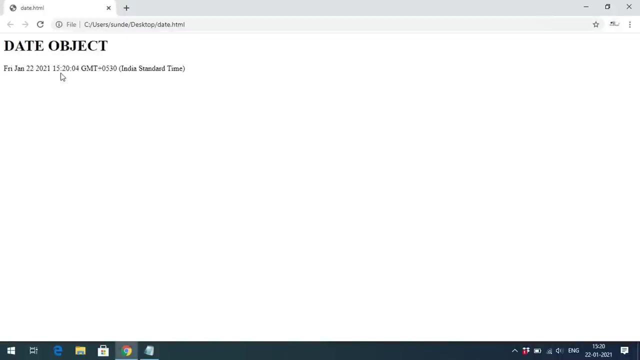 first of all, we save it: date dot HTML. so here you can get the date dot HTML page. so here you can observe, and if you double click on that, we will get see. so this is the current date and time. so this is 22 January 2021- 1520. so now the time is 1520, so we will. 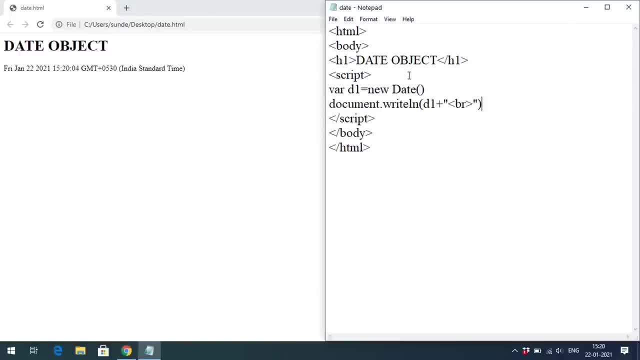 getting this date now, so let us increase the size. okay, write ln- go with some h2. okay, yeah, so this is d1. now we will go with another creation, so date 2. so see, you can observe here. so after every refresh it will be giving the current date and time. 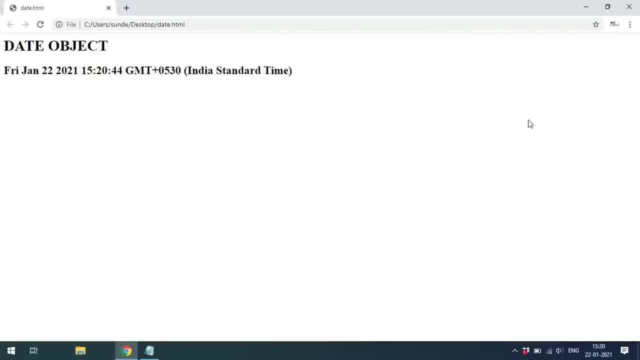 so if you observe here 15, that means 15 hours, 20 minutes, that means 3, 20, 44 seconds. if you refresh now again, it will be changed. see so 56 seconds. after 4 seconds, again minutes will be changed. I am refreshing, right, so I am just refreshing the page. so you can observe 21, so that means 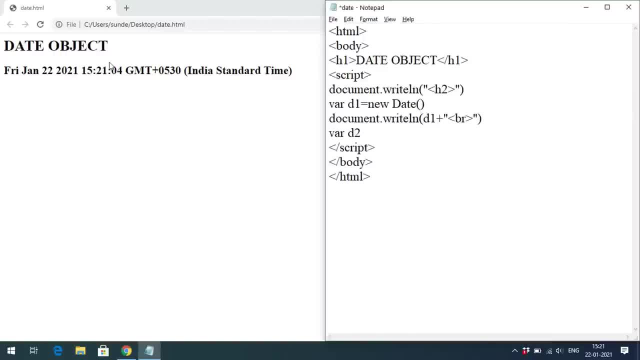 if you are not giving any parameters inside the date function, automatically it will give the current date and time, updated date and time. okay, and now we will go with one more thing. so date 2 is equal to new. we can set the date right. so date here we have to give. 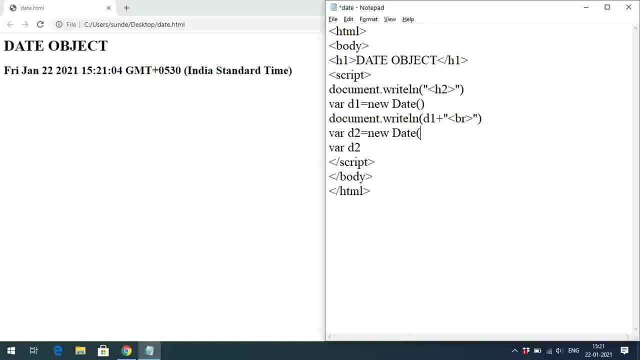 the seven parameters. what is the seven parameters? first, one gives the year, second, one gives the month. Third, one gives the day. fourth, one gives the hours. fifth, one minutes, sixth, one seconds and seventh, one milliseconds. so thousand milliseconds is equal to one second. so that also we have 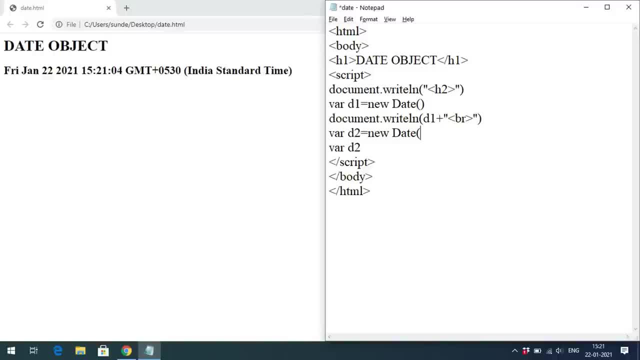 to mention right? so first I will go with the year. so I will give the year some 2021 comma and also month. let us go with the 01 month and again day. so what is it today? so here, month. So here the numbers from 0 to 11 represents the month from January to December, if you. 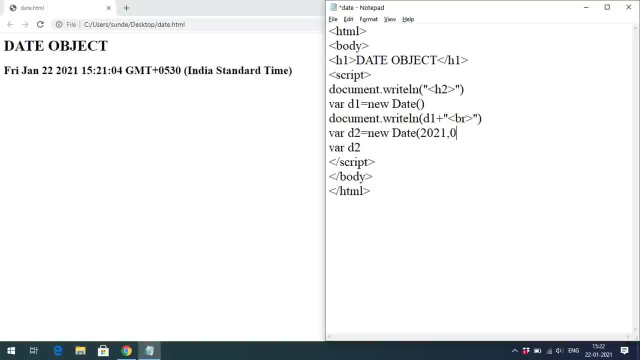 want to give the January, we have to go with a 0 and if you want to give the December, we have to specify 11. so the month category, month numbers will be from 0 to 11. so 0 is January and give the date. today's date is a 22 and you can observe here. we will observe here. 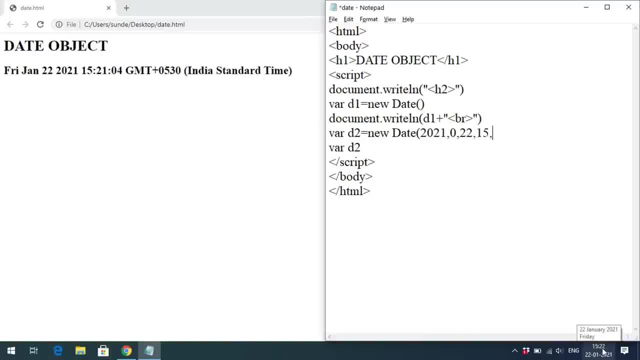 the time and we will give. so the time is 15 minutes and the next one is sorry, 15 hours 22 minutes. So we will give the time and give the second some 50 seconds and some hundred milliseconds. so I am given I have given some seven parameters. first, one gives the year, month number representing 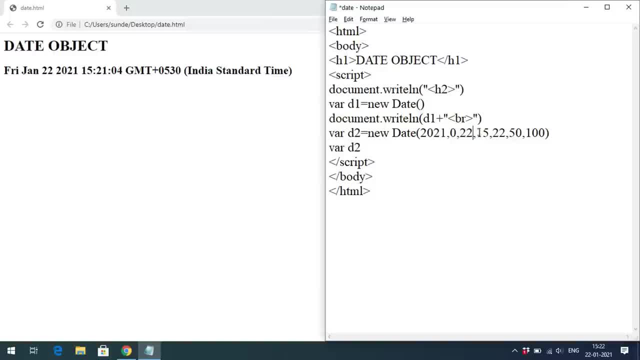 the month, date, okay, the day, day, hours, minutes, seconds and milliseconds. now let us print the same: So document, So document, So document, dot Right Total length: D2 plus again we give the BR for the next output and observe here. you can observe here. 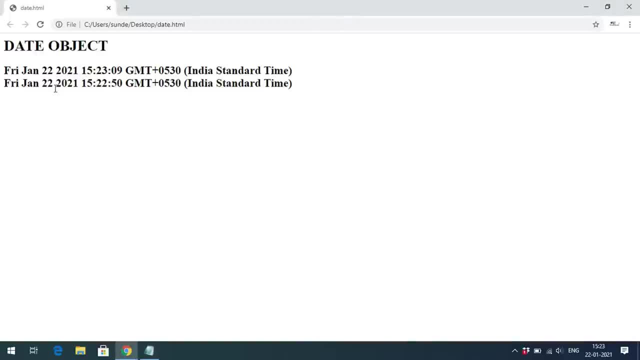 So we have given here some 50 will be here 25 and all these things. we can get the same time and keep on refreshing. you will get the same. the time and date will not be changed. you can observe here: the first one is a date we have given with the no arguments, so that 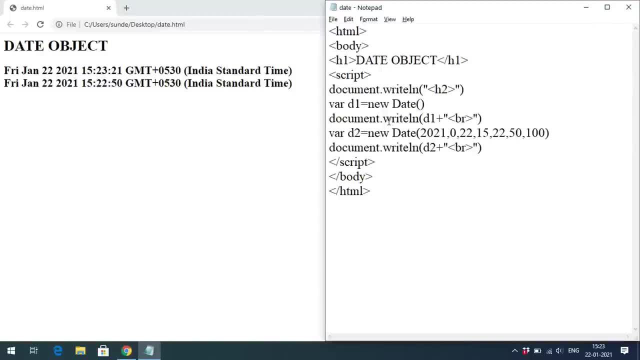 will give the current working date. date and time. i connections. but in second case, we are specifying some parameters here, so it will be a static. it doesn't change itself. if you, whenever you refresh, the first one will be changed and the second one will not be changed. you can observe here. so if you observe here. so 15, 23, 21, 15 1 to 50. 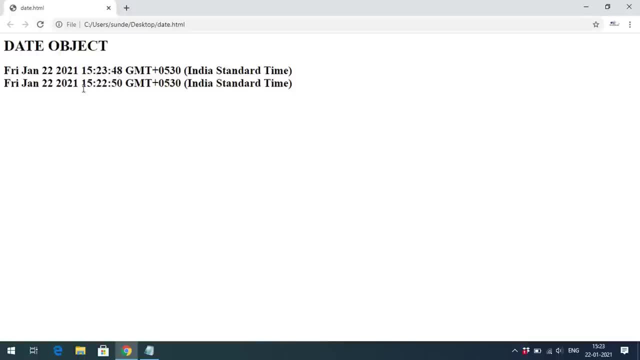 if you refresh the page, you can observe 15, 23, 48 and 15 20 to 50. this doesn't change because we are giving the date time and all the things as a parameters to the date function. so this is one more way we can create the date. and also, if you want to give specify, see date- only month. 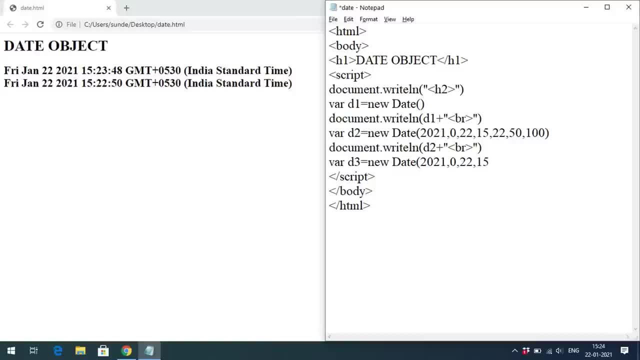 0, 22, 15, okay, and 24.. so i have given some only six, oh sorry, five parameters. i have given some five parameters. so here: month, month, day, hours and minutes. what is the? what about the seconds and milliseconds by default? if you are not giving any value by default, it will be treated as a zero, so you can. 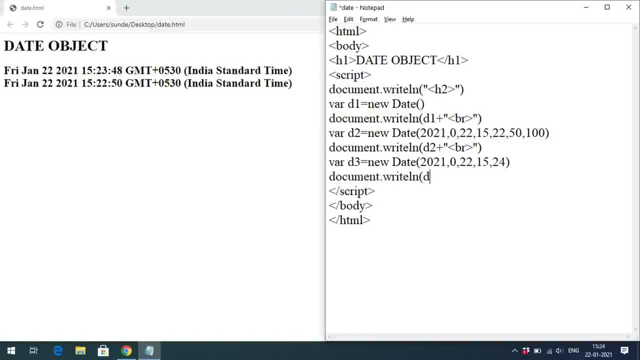 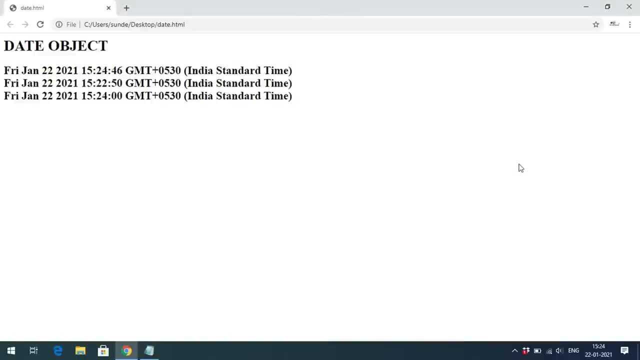 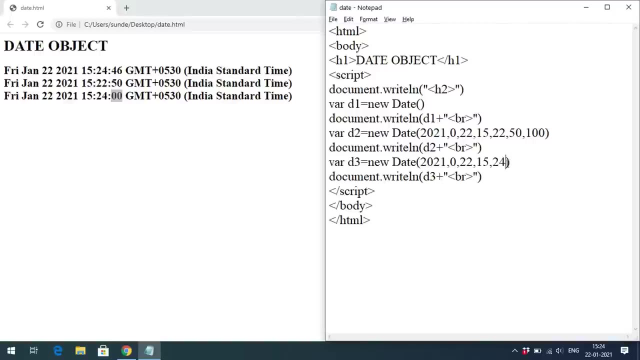 observe here: document dot. write ln d3 plus give the br function so you can observe here: see, the seconds is a zero because we are not specifying any seconds. okay, here we are not specifying any seconds. so that's why we get seconds as zero. and the same thing. same thing if you use the same thing. 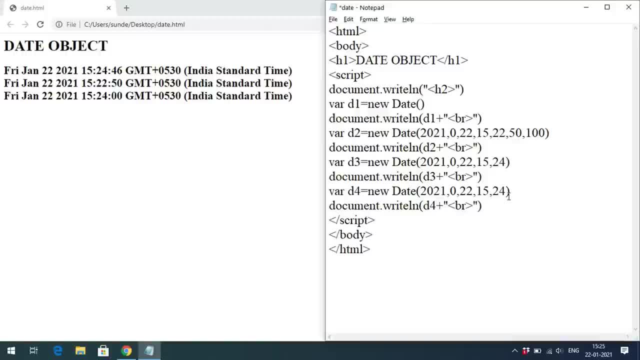 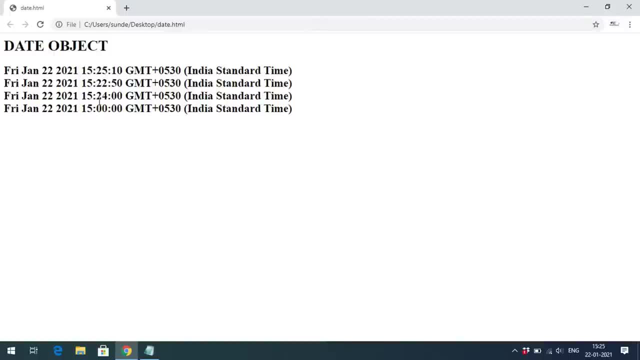 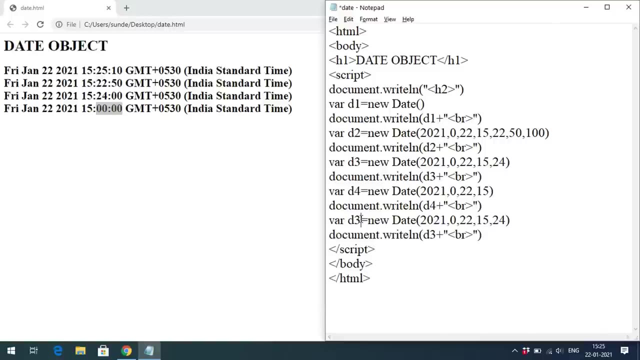 but reducing the parameters. reduce the parameter, that means take over the minutes. only. we are specifying the hours immediately. we'll get the hours as 15 and the all the remaining as zeros. and also and also, if you give, if you still reduce the parameters, if you still reduce the parameters. 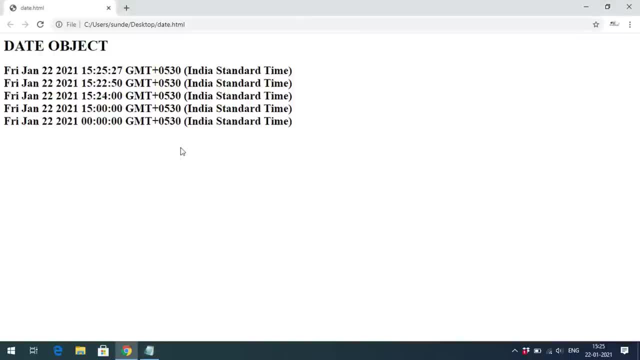 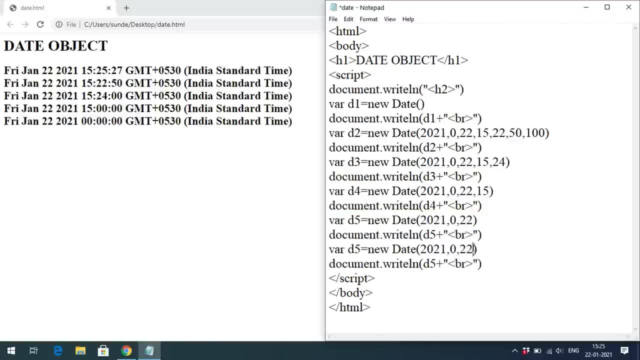 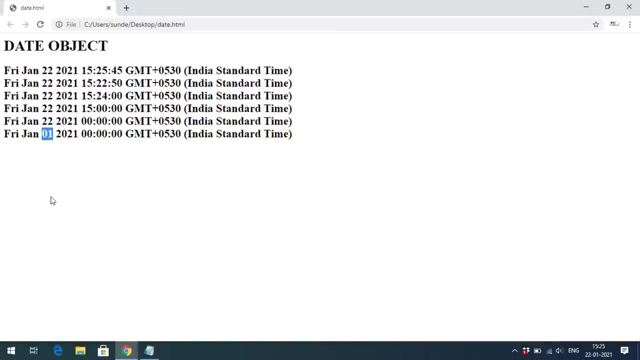 so you get 3, 3, so we are giving only date, so the time will be zero. the time will be zero and similarly. similarly, if you give the day and year and a month, just you are skipping the day. then also we'll get the same thing. see january first. by default it will be taken as first, okay, if? 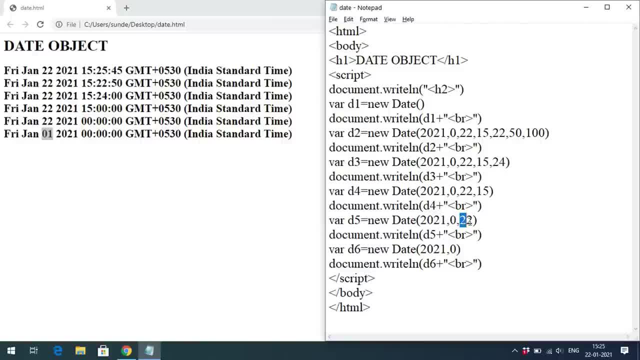 you are not specifying any day. so previously we were not specifying any option before we are giving, only Previously. we are specifying the day as 22.. So that is why we got a 22. And here, if you are not specifying any day, automatically, by default it will be considered as a 01.. And this is a special case. 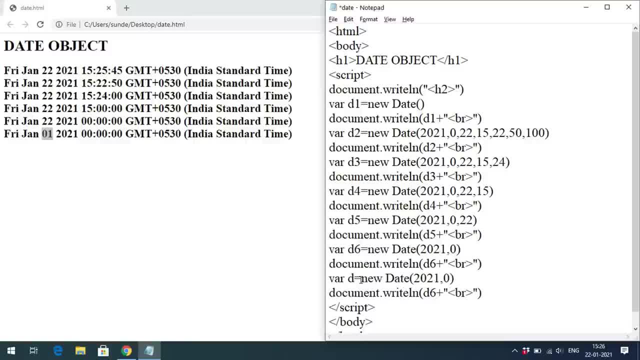 If you still reducing the parameters, so if you give only one parameter, if you give only one parameter, so that is 2021, 2021.. So that will be considered as a milliseconds. Okay, that will be considered as a milliseconds. So we know that. So 2021 means 2 seconds. 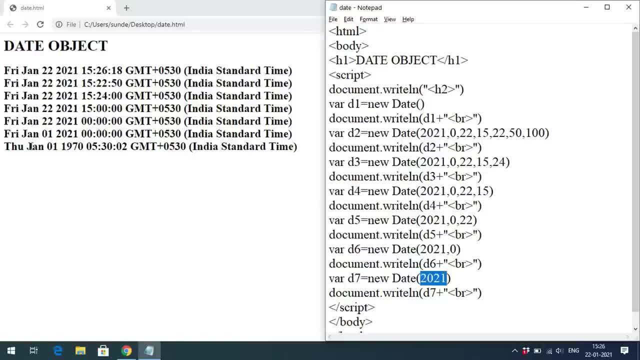 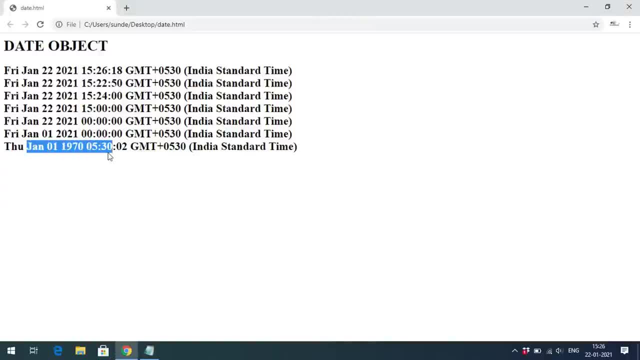 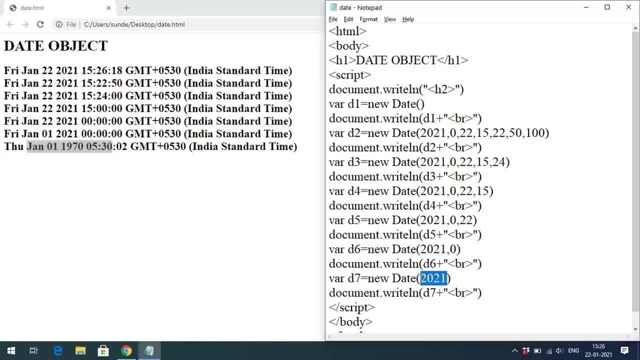 So, by default, the date will be starting from January 1st 1970, 5.30. Right. So this is the default time. This is the default time. So here the date object will start from this date and time. So if you are giving this 2021, in our perception we are giving the year, but the JavaScript will consider it as a milliseconds. 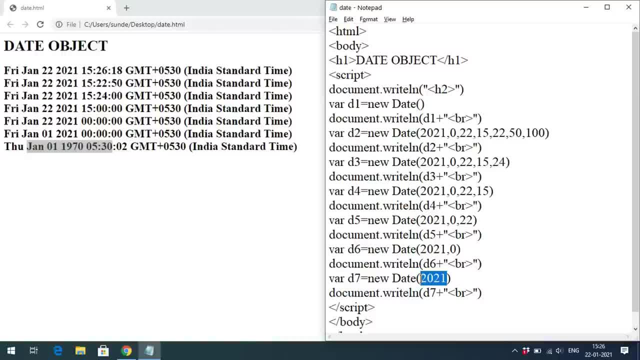 So 2021 milliseconds is equal to 2 seconds, So here we will get 2.. Okay, Hope you understood. So if you give 3000. Then it will give the 3 milliseconds here, So you can observe here: 3 milliseconds. Okay, So this will be considered as milliseconds And this is the way we can create the date by using milliseconds. 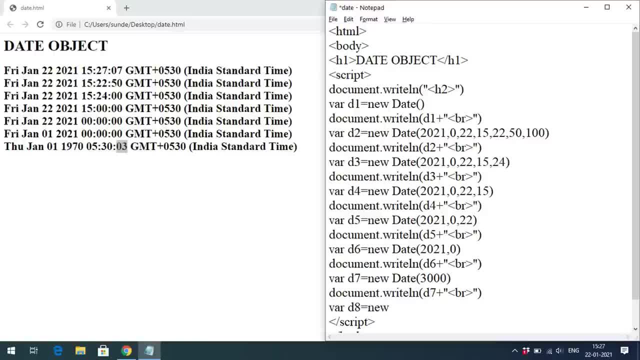 So date is equal to new date. Give the milliseconds here. So, whatever the milliseconds you can give, everything we can give, And it will be updated from this date: January 1st 1970, 5.30. Right. 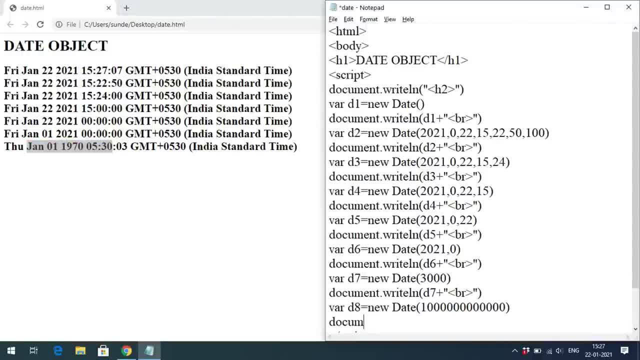 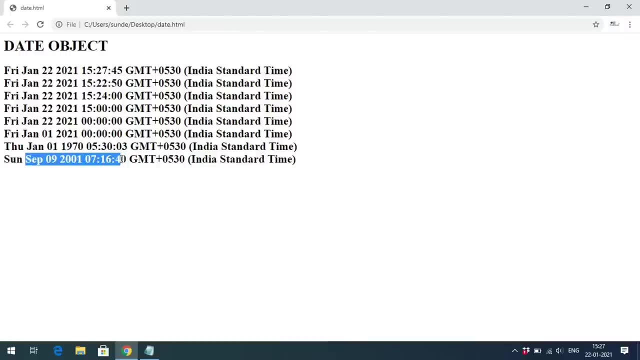 So if you observe here, I will print here document dot. write LN D8 plus BR. You can observe, See. So this is the date we got, So September 9th 2001, 7.16.40.. So after calculating these milliseconds and applying to this year, we will get this one. 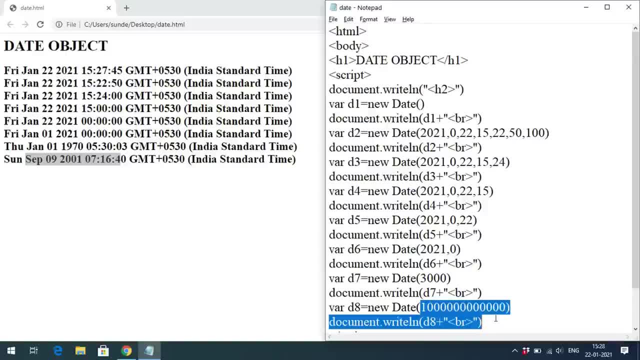 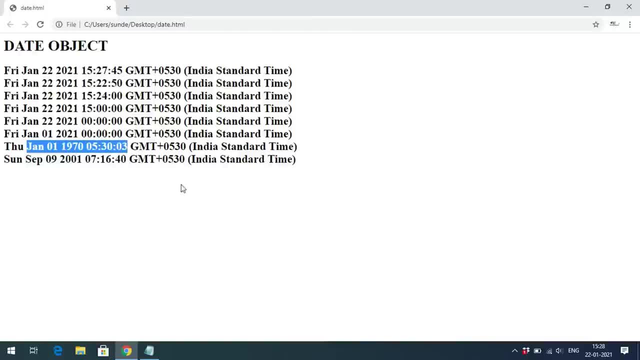 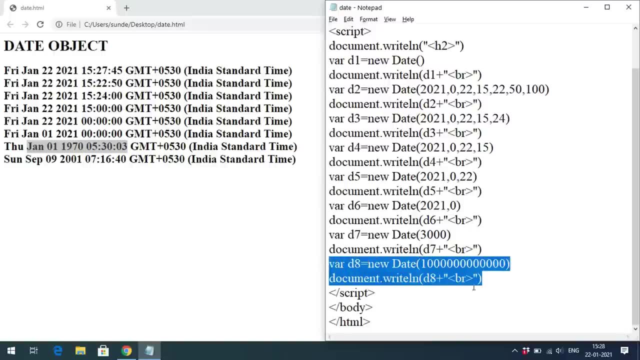 Okay, This is the milliseconds, This is the milliseconds, Right? So these milliseconds, These milliseconds will be added to this date. These milliseconds will be added to this date And we will get this one. And if, for example, so here the milliseconds is of positive, 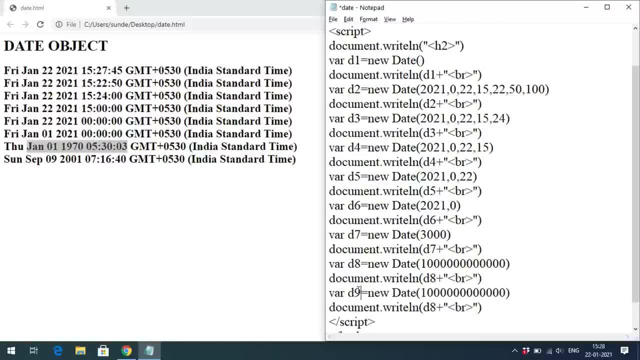 And if you give the negative, automatically it will minus from the 1970 and we will get less than 1970.. So let us check. So if you give here minus milliseconds, we will get. it will be minus from 1970.. 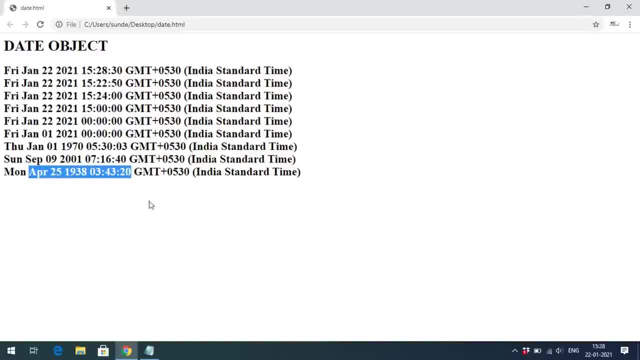 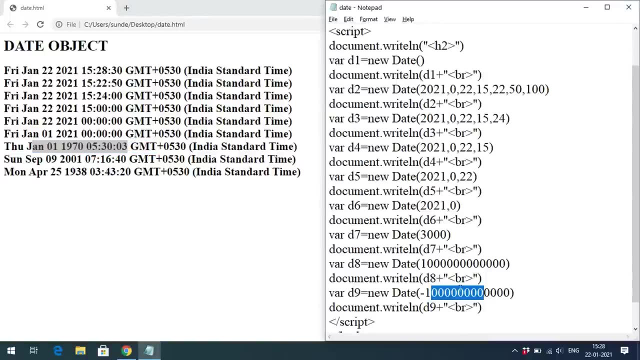 So we will get the date as 19,, 38,, 3,, 43,, 20 seconds. So these milliseconds will be minus from subtracted from this date. Okay, This date Automatically we will get. So that means first this will be converted into milliseconds and these milliseconds will be subtracted from these milliseconds. 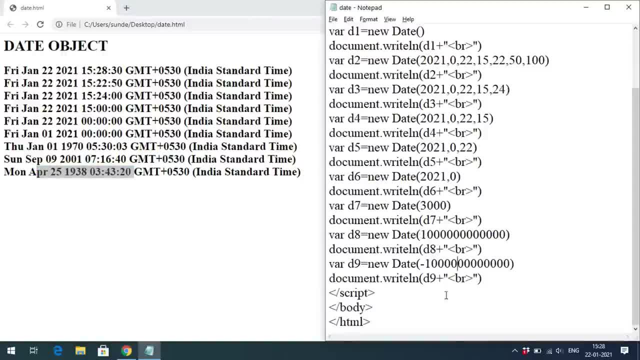 So automatically we will get the date as this one Right. So this is how we can use, And also if the year, if the year is displayed Here. if so, obviously we should give two parameters, That is, one is month and another one is year. So if we are giving only year, only one parameter, automatically- we have seen that that will be considered as milliseconds. 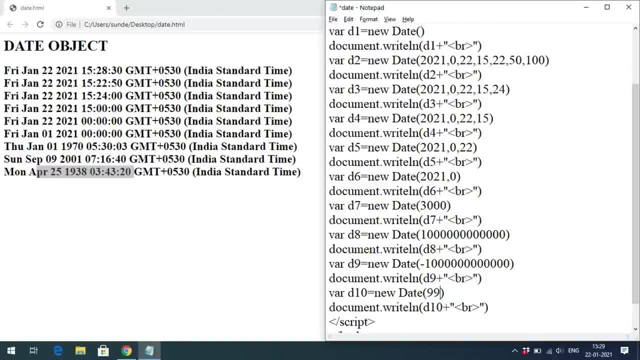 Now I will give some 99.. So if I am giving some two-digit number, so in the year, in the year, if you are giving some two-digit number, that will be considered as a 19th century. I mean 20th century. 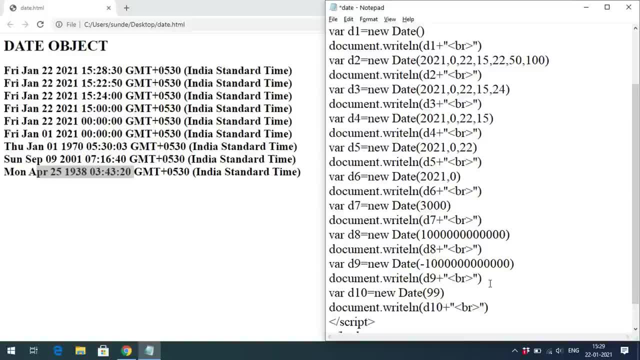 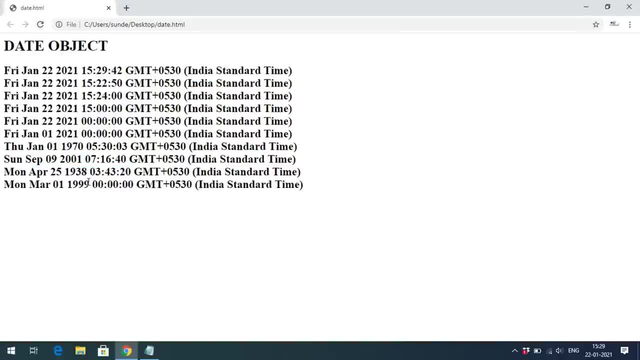 Okay, That is 1999, 1999, 22.. That is 1999, 1999, 22.. That is 1999, 1999, 22.. like that, ok, see 20, 99 and 2. if you execute this one, we will get see 19- 99. it will be considered. 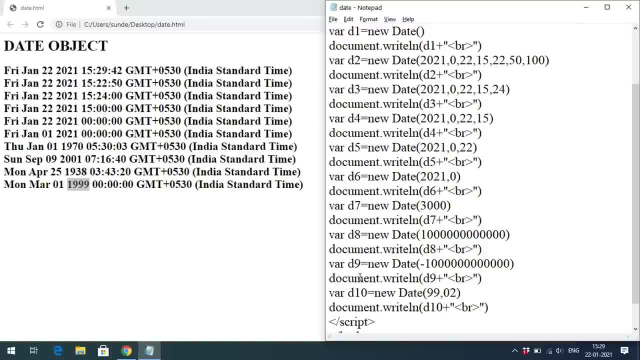 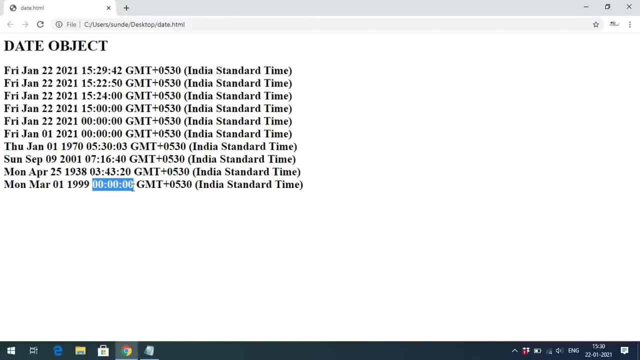 as a 19, 99. so here the second one. that means march, because here the months will start from 0, right, so we are not spacing any day. so that is why we by default we will get 0, 1, and seconds, milliseconds, hours and minutes will be considered as a zeros, and if you here you give some 90 and 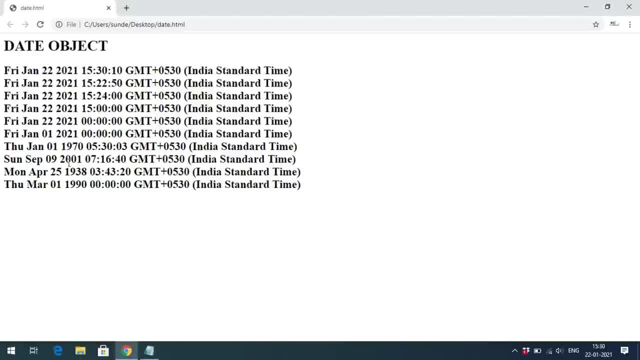 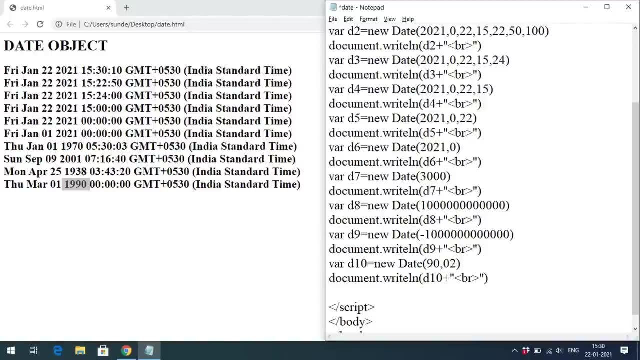 again, we will get some 1990, ok, you can observe here. so we need to give four digits, otherwise it will consider as a 19 1990, 1991, right? so this is how we can use. and one more way to create the date object is by giving a date string so we can pass as a date string. so instead of giving the 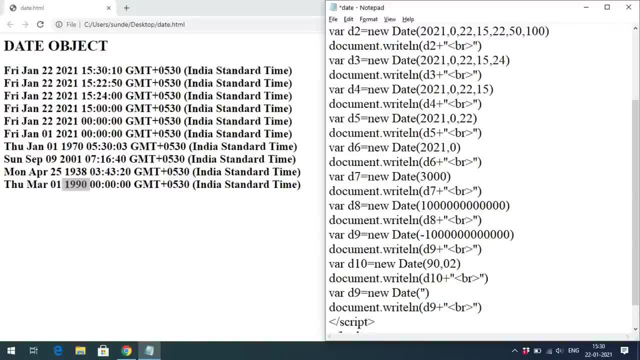 milliseconds, we can give the date string. so date string means give the date string here: 2021, january 22. so here you can give some 11 and also again go with 11. so you can observe here: so like this also we can give, so we can give this. 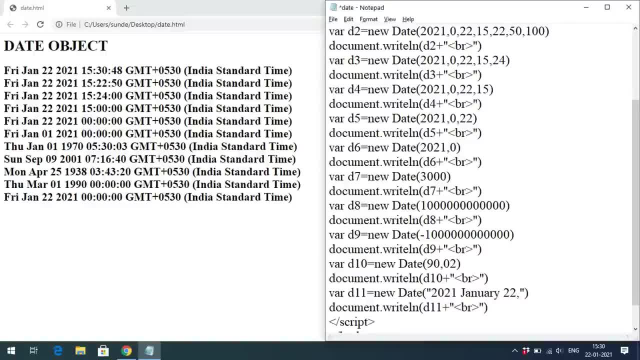 date strings. ok, date string some 10, 50, 40, 43. you can observe 10, 50, 43, so we can give like this: ok, so use the semicolons. use- sorry, use- the columns. so if you are not using the column and if you put the comma, we will get the invalid date. so 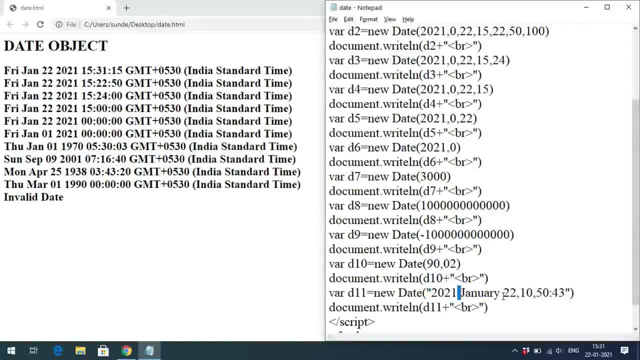 because so here the date can be. you can use a space or a comma in the dates, but coming to the time, we need to go with this. this format: use a column, ok. 10, column 50, column 43. that means hours, column minutes, column seconds. so if you are not giving this one so automatically, we will get a zero right. so this is. 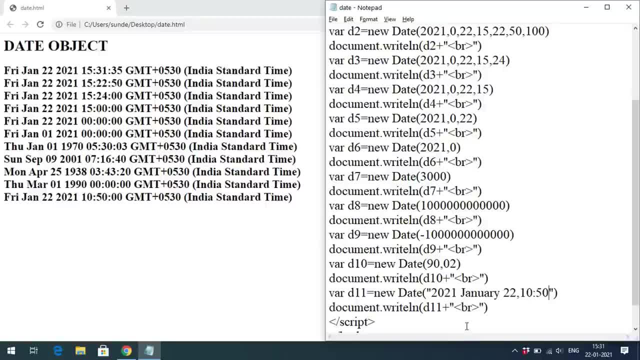 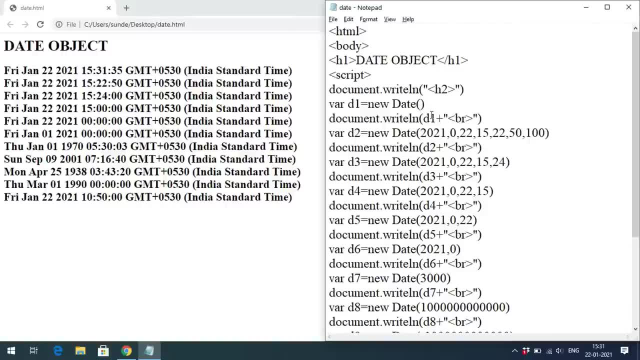 how we can create a date object. we can create the date object. so one thing we have to remember: if you are not giving any parameters, that will give the current date and time, the current date and time, and if you want to give the parameters, we have to give at least two parameters. that is a year. 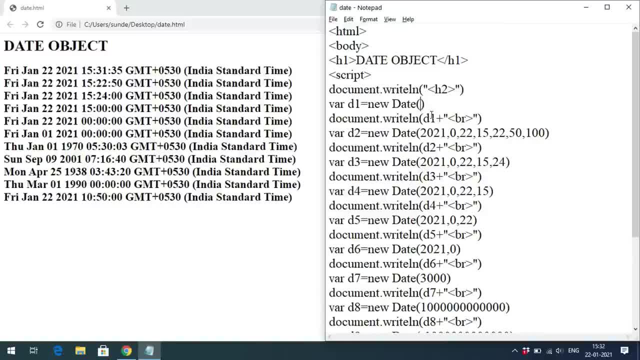 and month, and if you are giving only one parameter, that will be considered as a milliseconds, and also we can give number of milliseconds so that that in javascript the date object will always start from january 1st 1975, 30.. right, so it will add the milliseconds to that particular. 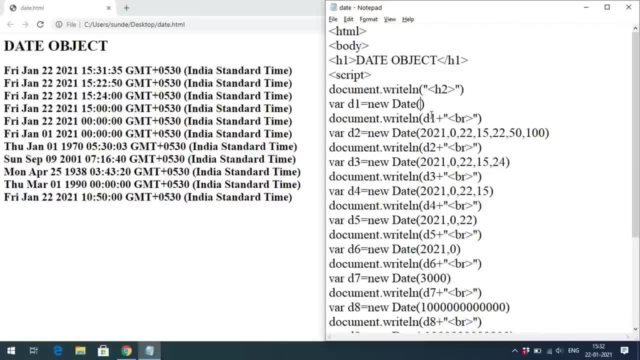 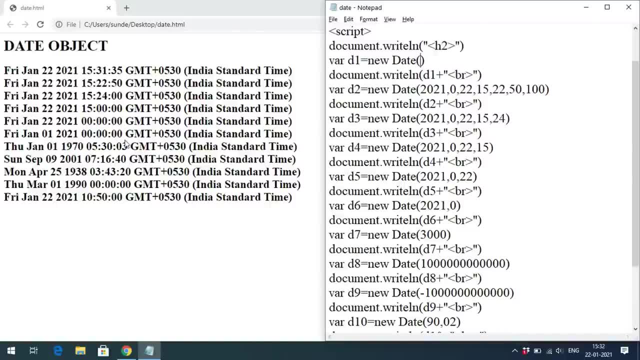 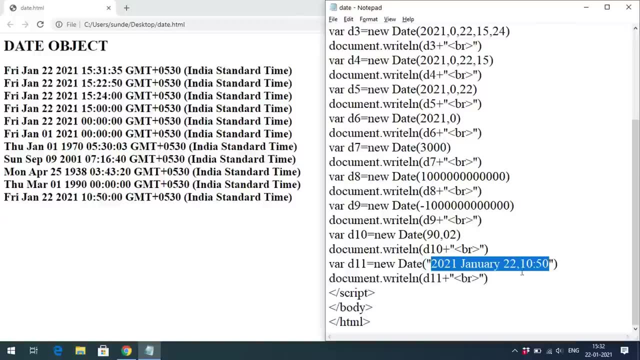 date and we get the updated date. or else we can give you the milliseconds in terms of negative, so that it will subtract the milliseconds from the given date and we will get the corresponding date, or else we can also pass the date string, so use the format. you remember the format, so 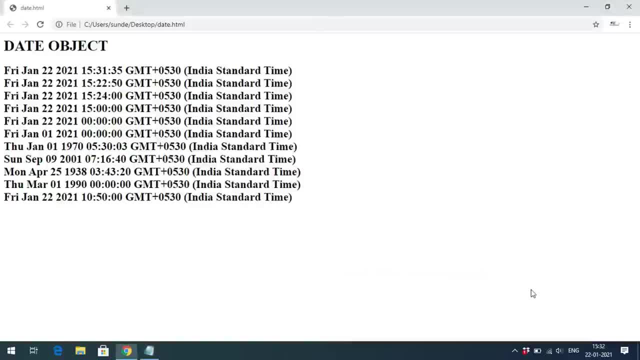 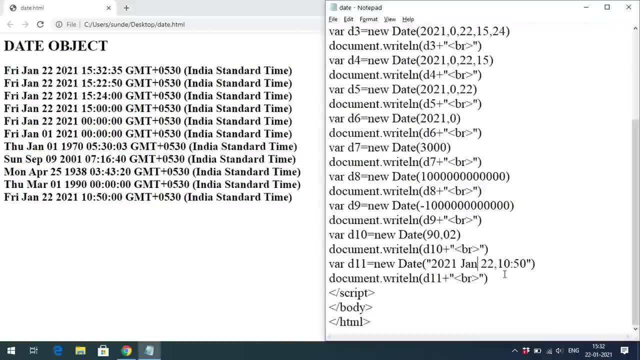 you can remember any format. you need not go with the full name. you can also go with the normal rain name, january, so that we will get the same thing here. okay, so this is how we can create the date object, how these many ways we can create the date objects. right, so hope you understood and 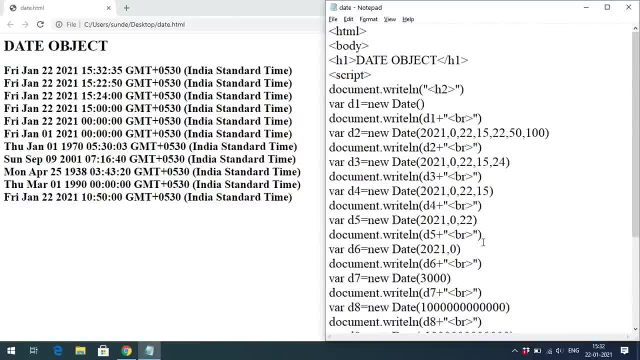 one more thing. we have to remember the mem, the months. the months will be represented in terms of numbers and the months will be starting from 0 to 11.. so 0 for january, 1 for february, similarly for december, right, so hope you understood. 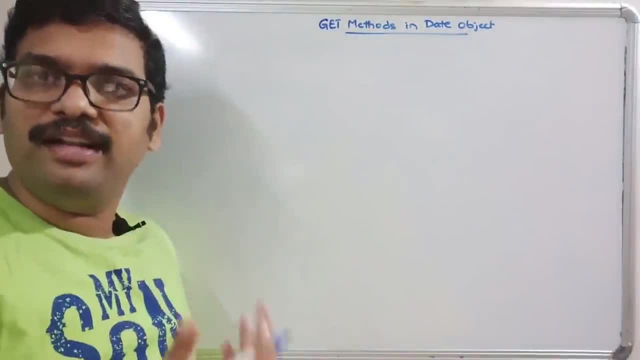 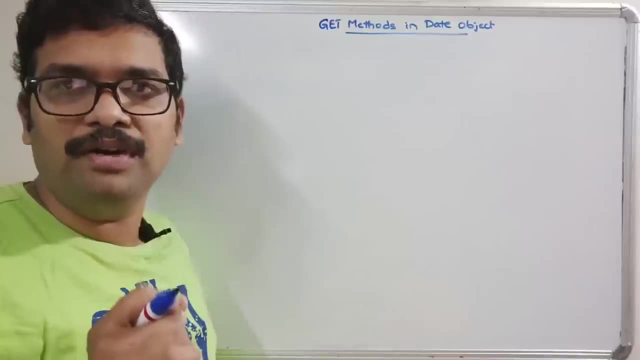 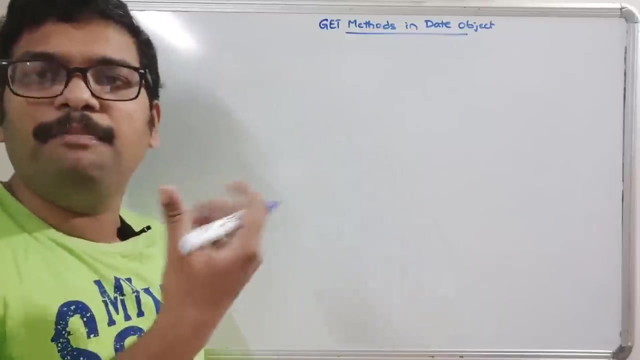 so in the previous session we have seen how to create the data object right. so whenever we say about the object, that object should be created with the help of new keyboard right. so first of all we'll create a date object and so that after that we can get different parameters from that date right. so in the previous session we 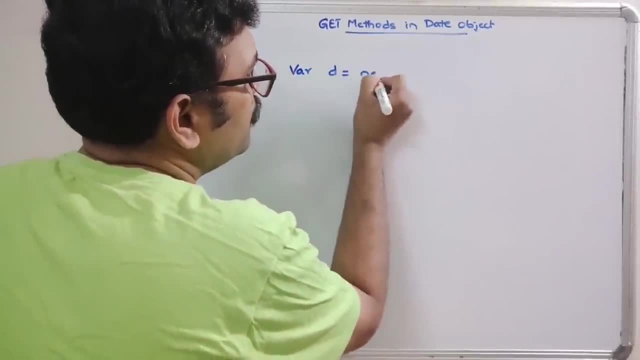 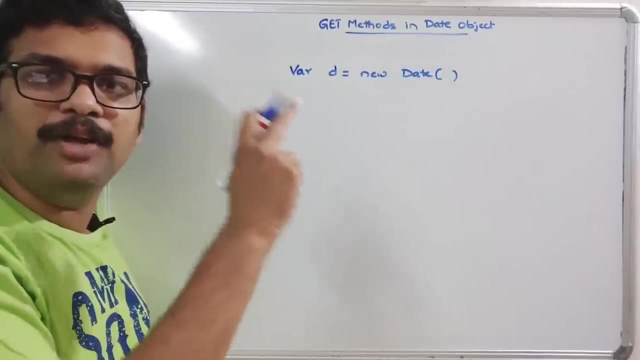 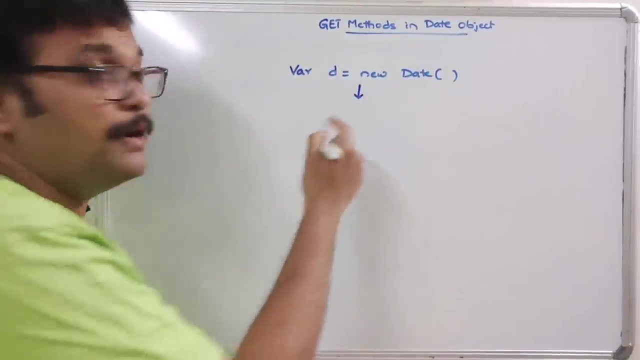 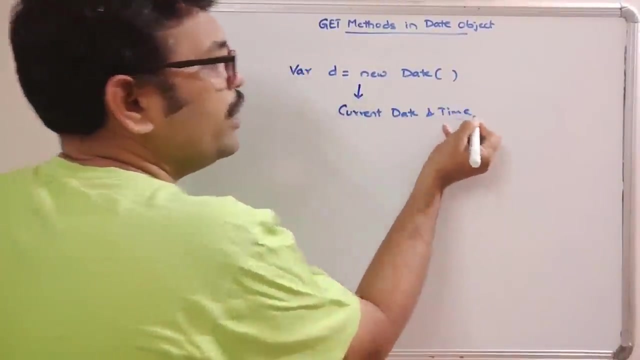 have seen somewhere. d is equal to new date, so this is the one way to create the data object. so if you create in this way, by using this statement, that means if you are not passing any parameters inside the date function, this will retrieve. this will give the current date and time. current date and time. so we have. we know that date can be. 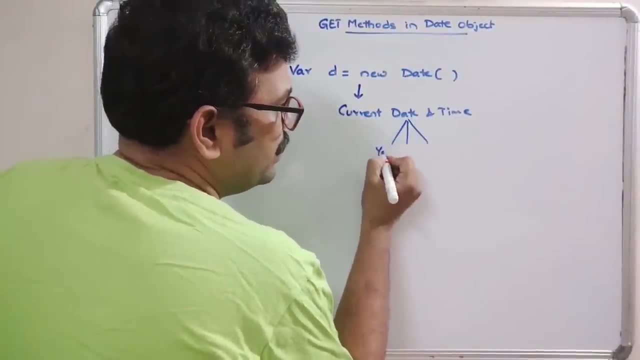 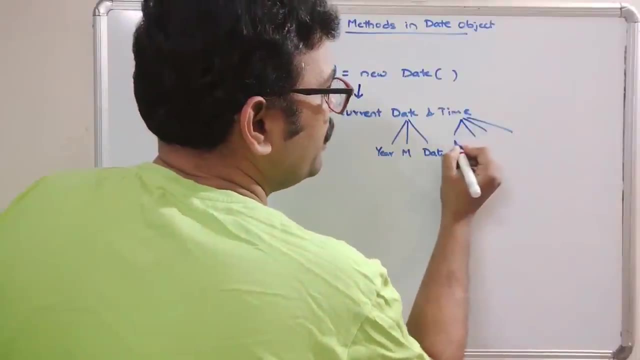 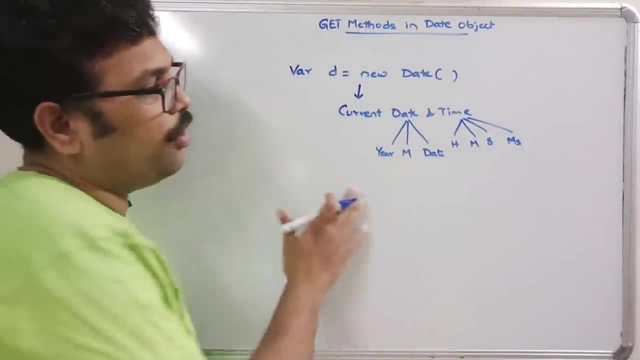 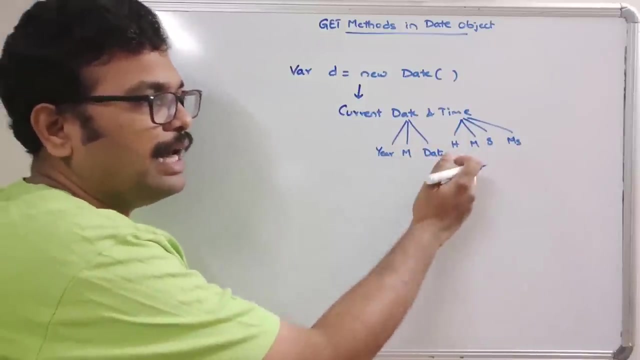 represented in three parameters, that is, year, month and date. okay, and time can be of four parameters: hours, minutes, seconds and milliseconds. so we need to get all these parameters right so we can get the year, we can get the month, we can get the date, we can get the hour, we can get the minute, seconds. 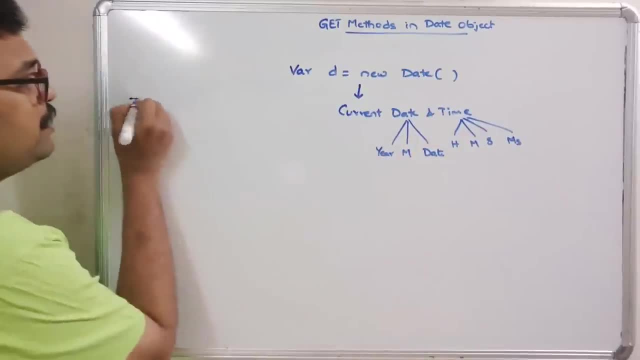 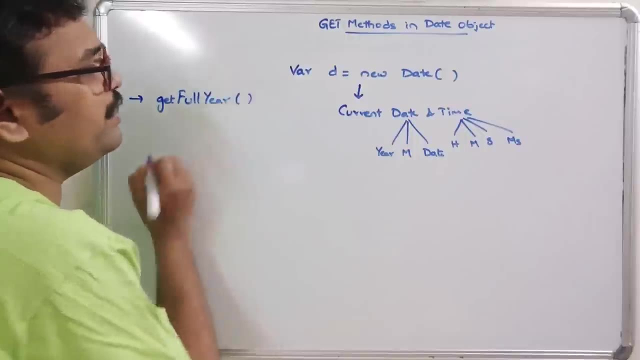 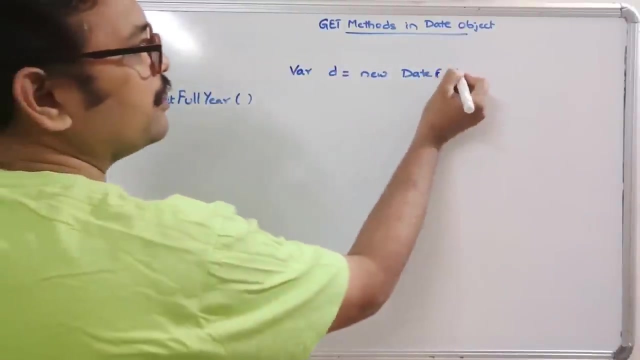 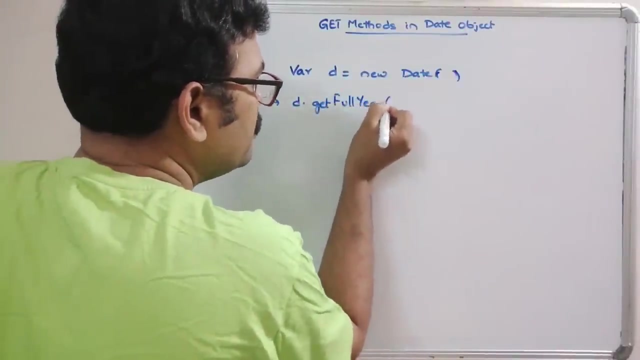 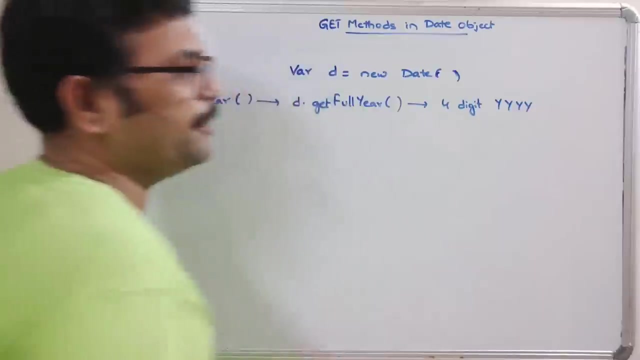 and the milliseconds. so, for this purpose, the first function is get full year. get full year, okay. so the syntax for this one is: we need to call this with the help of this date. okay, so d dot get full year, right. so this will give the four digit year the four digit year. so y y, y y, okay. 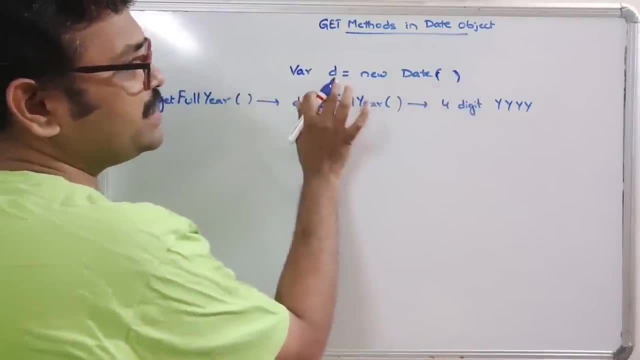 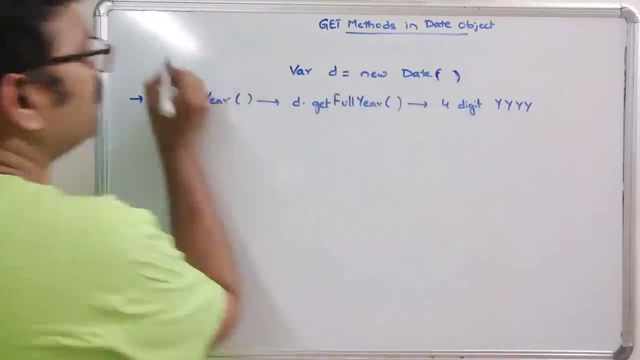 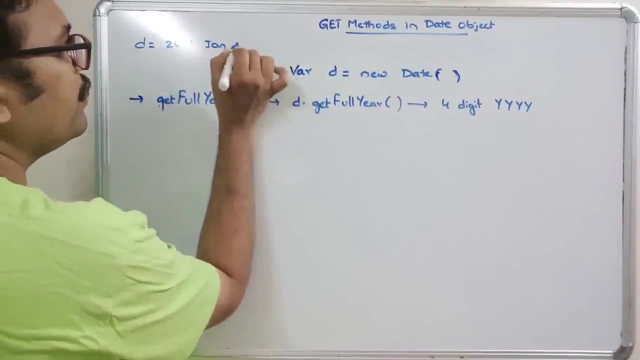 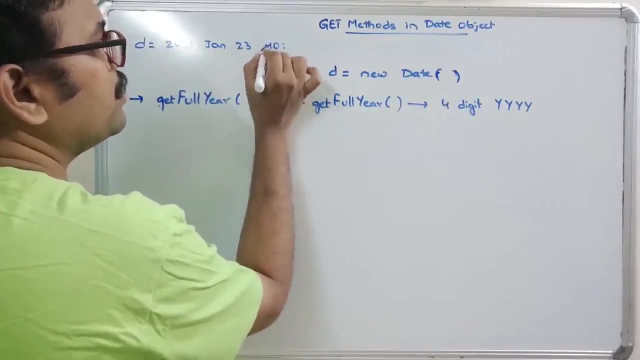 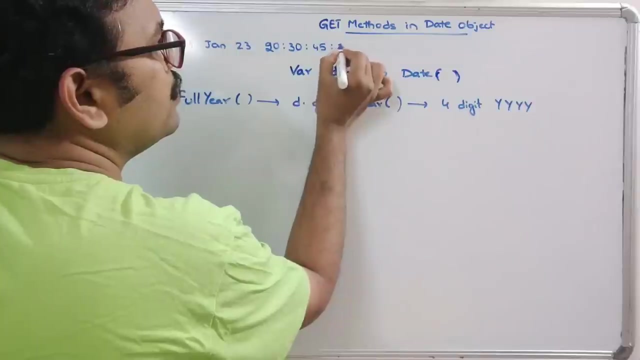 four digit here. so now, from this date, we'll get the year. for example, if it is, if, if you after, if executing this one, the d will be some 2021, january 23, 10 hour or something: 20 hour, 30 minutes, 45 seconds, 200 milliseconds. so this is the day now, after getting this function, after executing this. 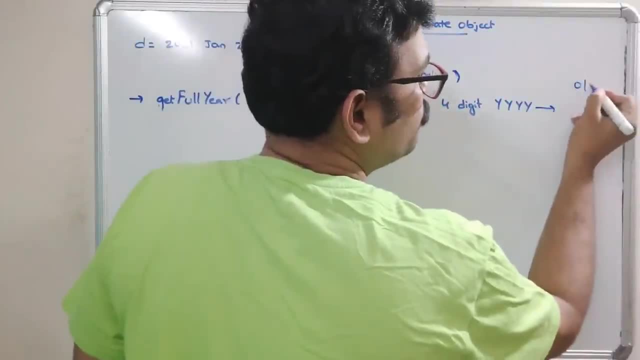 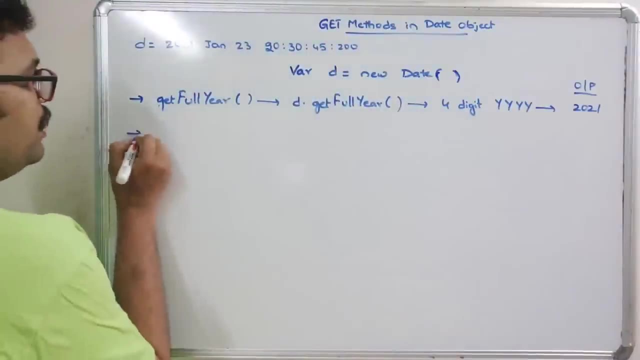 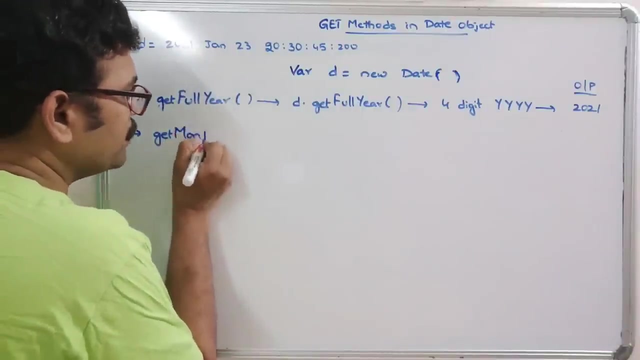 function d dot get full year, we will get the year after executing this function. after executing this function d dot get full year, the result, the output, will be 20, 21, 20, 21 and similarly get. the second one is month get month. so this is also the syntaxes we should call with the help of a date object. so d dot. 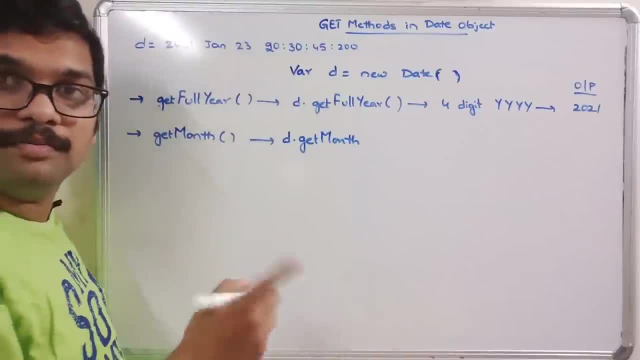 get month, so i will execute each and every function by execute, by showing the code right, so by writing the code, we will execute the code by using the code located in the function right to writing the code, we'll execute. and when it sits right, so by doing each and every function by walnut, by showing the code right, so by writing the code, we. 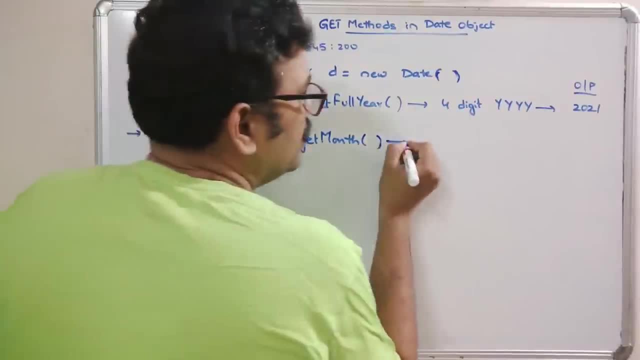 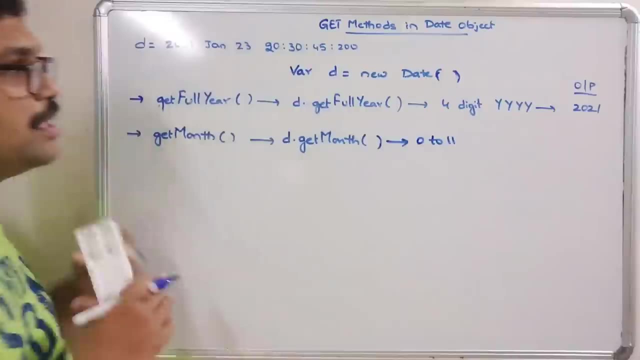 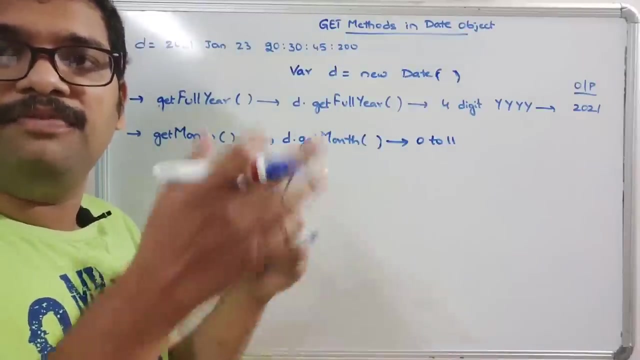 will execute each and every function. let's see the syntax now. so this will return. this will return 0 to 11, because a month can be represented in a numbers from 0 to 11.. so if it is 0, that implies the month is january. if it is 11, the month is december. so the output for this one. 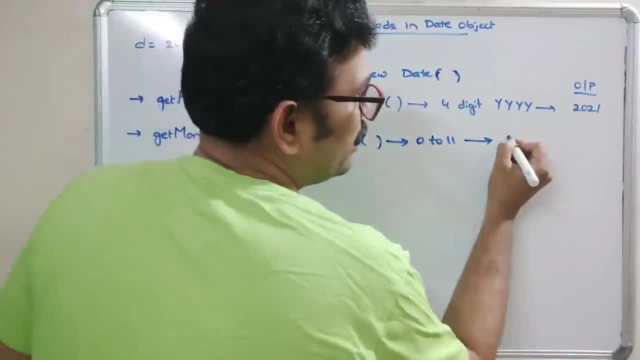 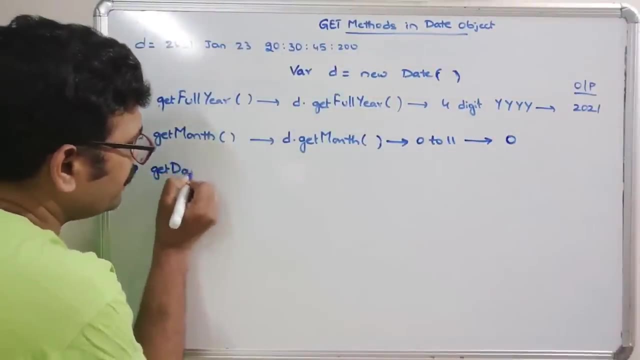 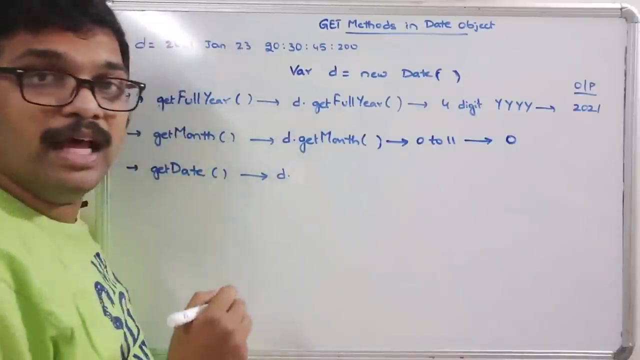 the output for this one is: so here it is a january, so we'll get zero as a output. okay, 0 as a output. and the next one: get date, get date. so get date means this is also we have to call with the help of data object, so d dot get. 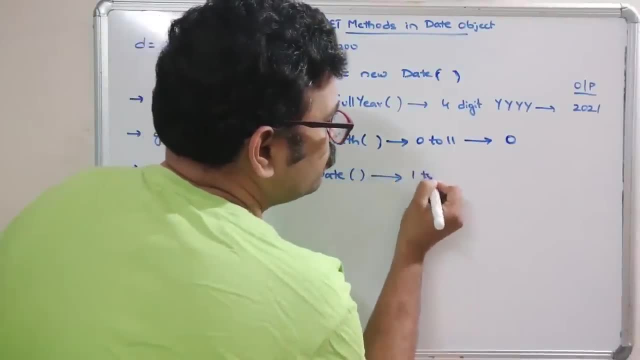 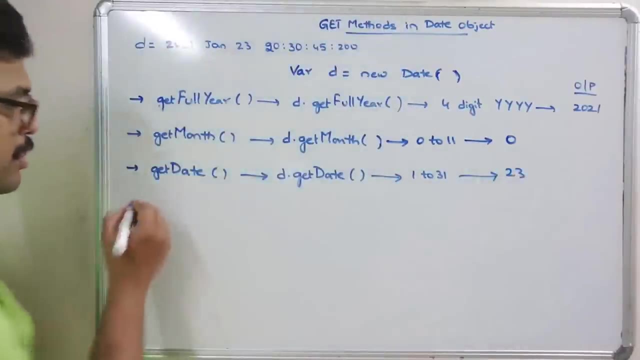 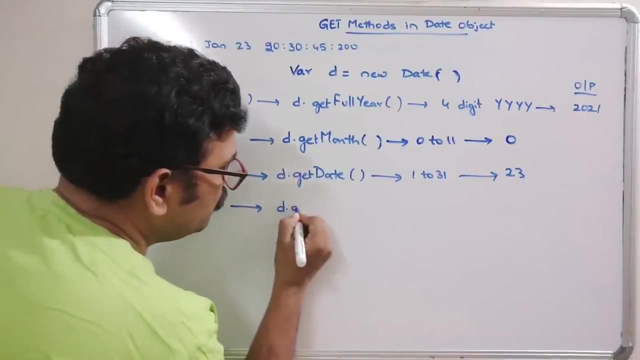 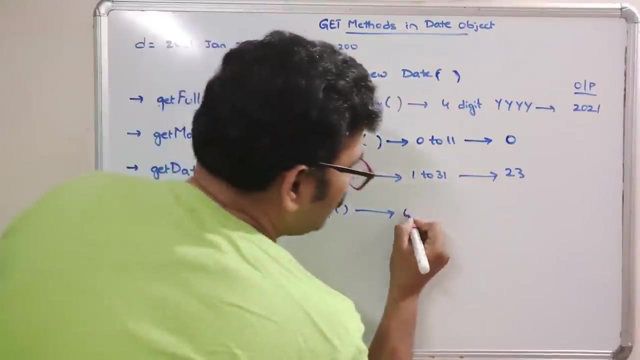 date. so here the date can be from 1 to 31, so from this we'll get the result as 23. okay, next get day. so this is also d? dot get day, so it will give the number for days. okay, so it returns from 0 to 6. 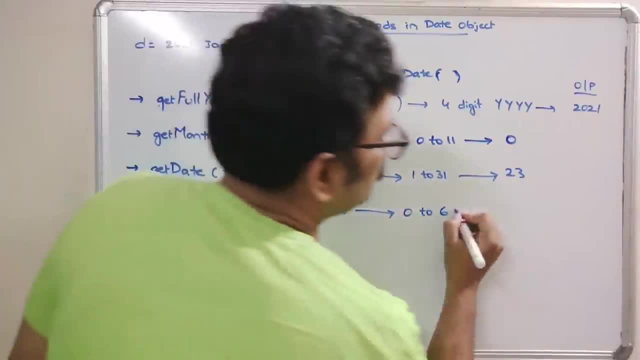 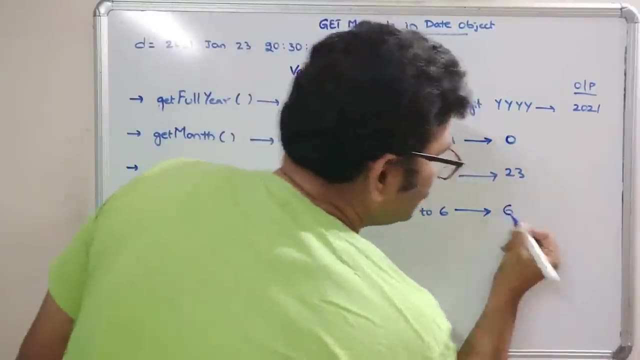 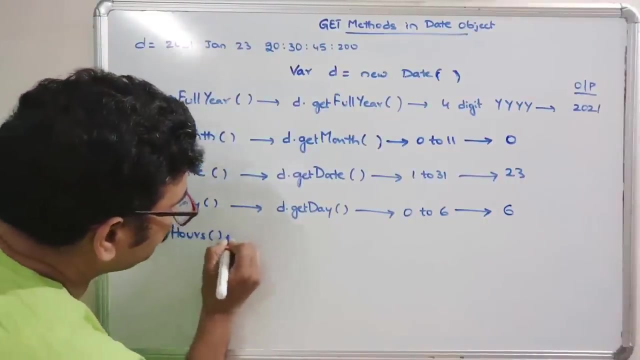 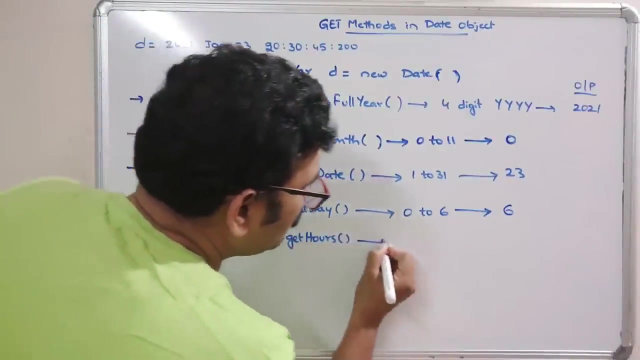 so 0 starts from sunday and 6 will be saturday, so this will return. so as as of now, 23rd january, that means today it's a saturday, so the result will be 6 here, okay, and get hours, hours, get hours. so d dot get hours. it will return the hours from 0 to 23 and here we'll get the. 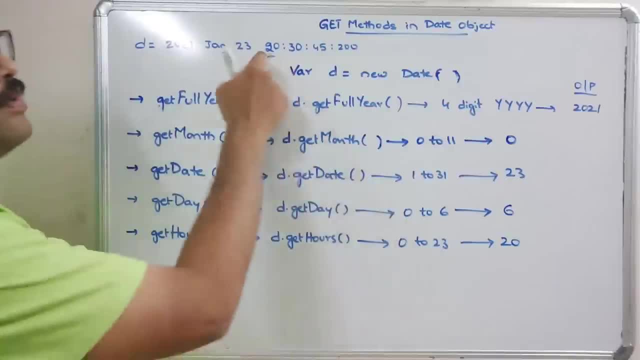 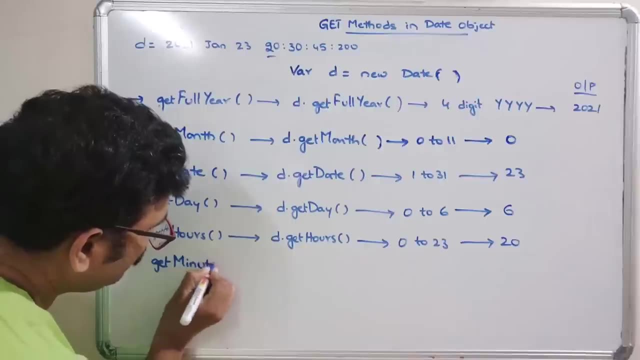 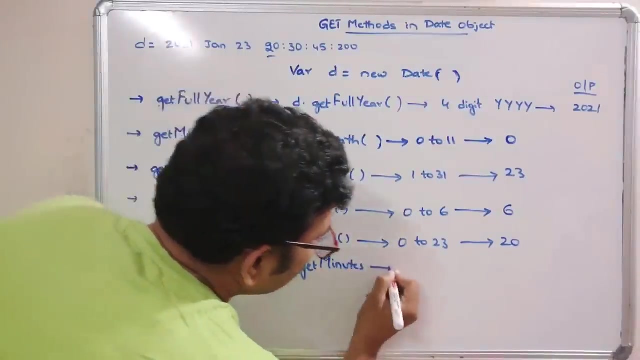 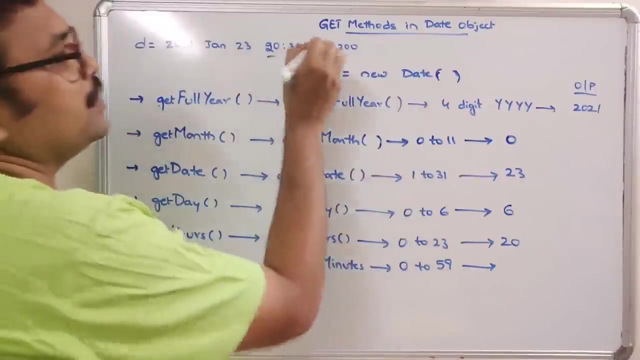 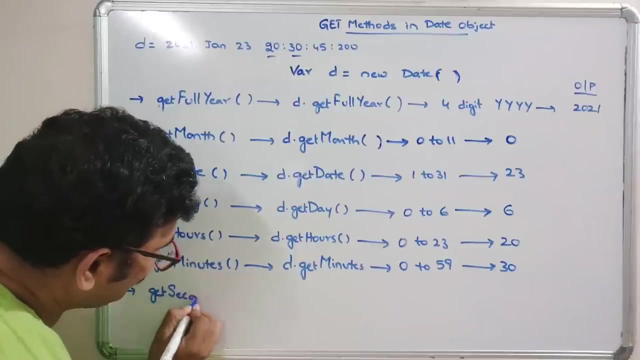 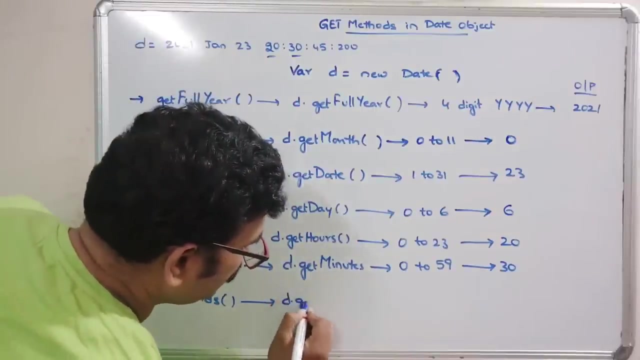 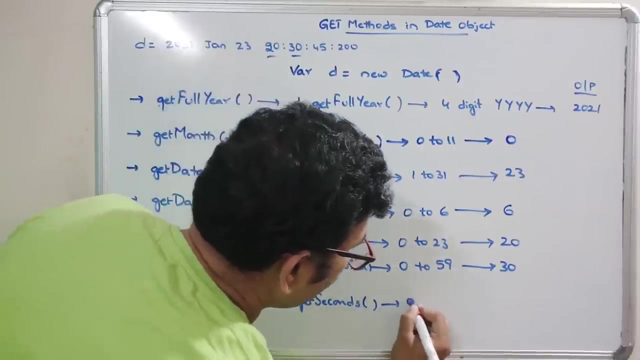 hours as 20. 20 will be the output for this data object and the next one: get minutes- get minutes, so d dot get minutes, minutes, so that the minutes will be from 0 to 59. right, the result will be see 30. and similarly: get seconds- get seconds, so we'll get D dot get seconds. and here: 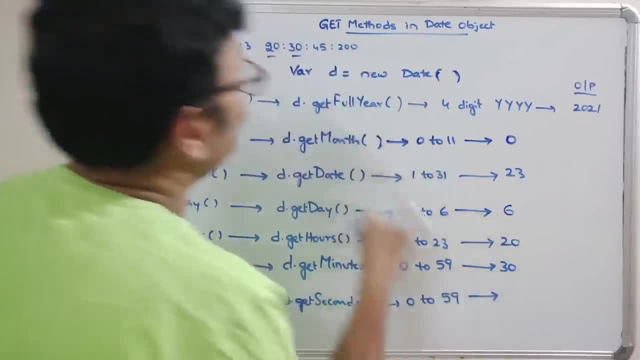 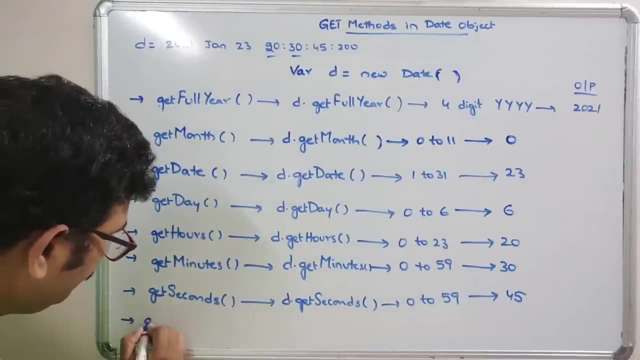 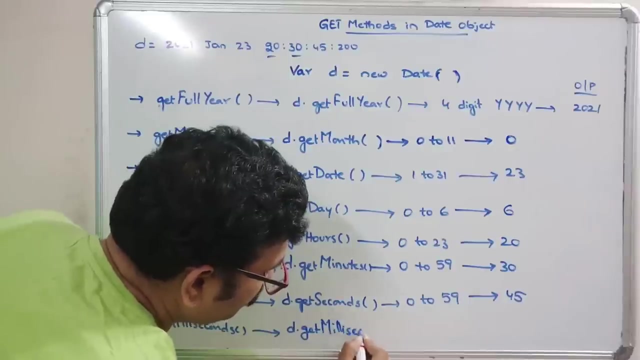 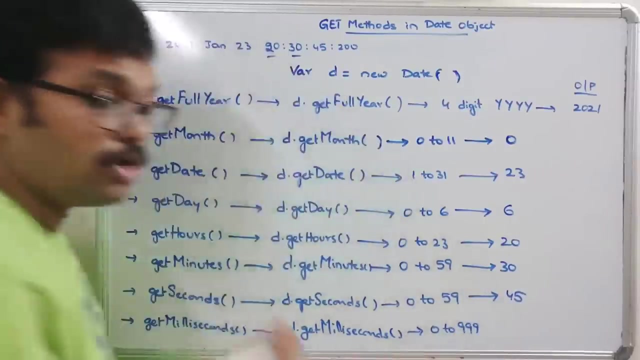 also it will be 0 to 59, so that we will get here as a 45 and the next one get milliseconds. so we know that there is a 7 property. so D dot get milliseconds, so which will return from 0 to 999, because thousand milliseconds will be. 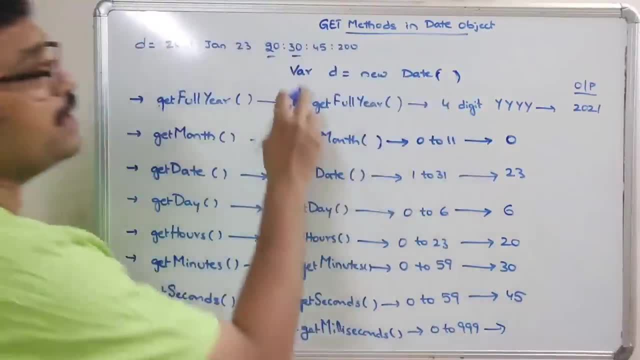 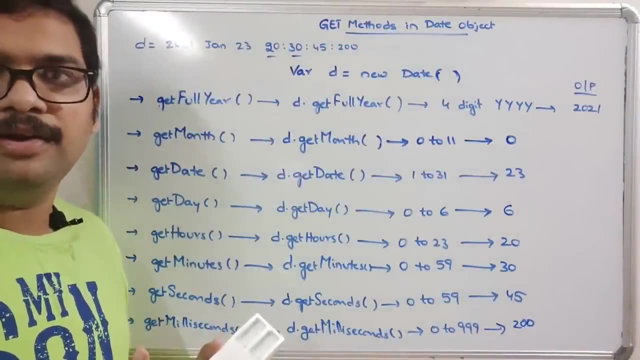 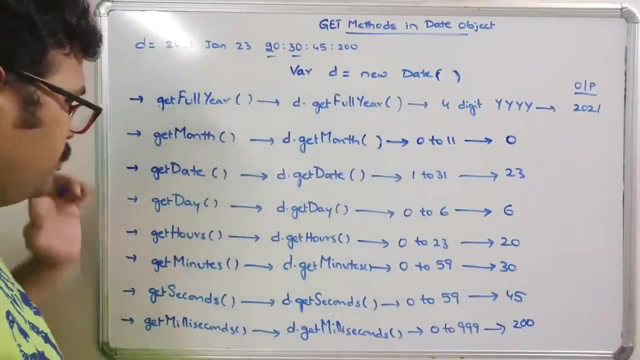 given as a 1 second. so here we get the result as 200. so this is how we can get different properties from the date. okay, different attributes from the date. so we can retrieve all the seven properties, seven attributes. right? so this is. these are the get methods. these are all called get methods in order to retrieve the 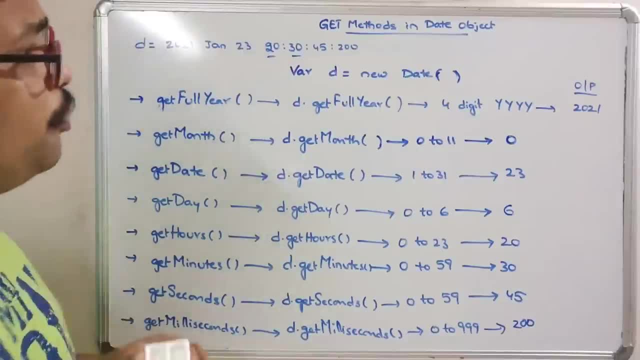 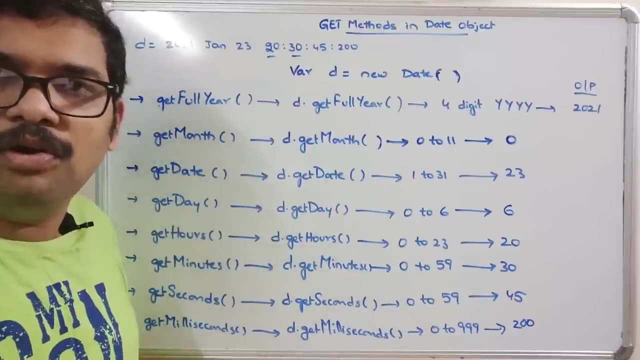 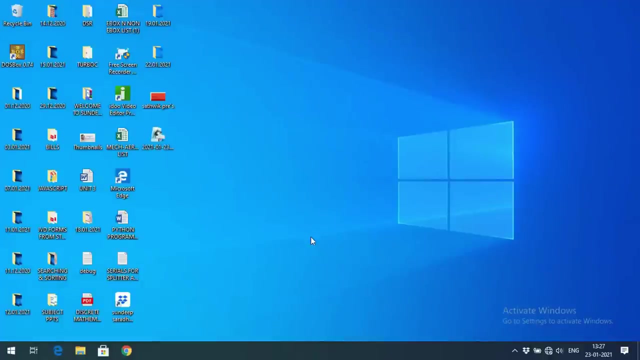 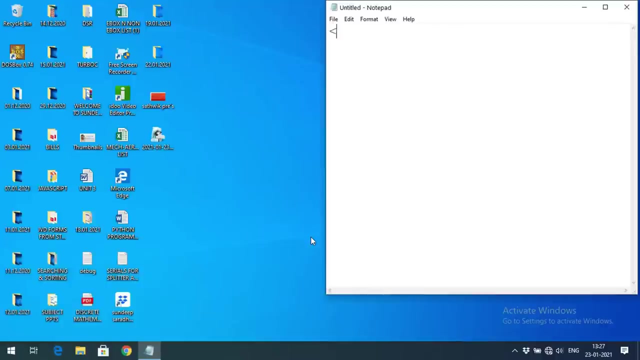 existing data, right, so hope you understood this one. so I will execute the same thing. I will demonstrate each and every method by executing a code. so we move on to the system. hello friends, so just now we have seen various get methods of a data object. now I will demonstrate each and every method by writing a small code. so first let us 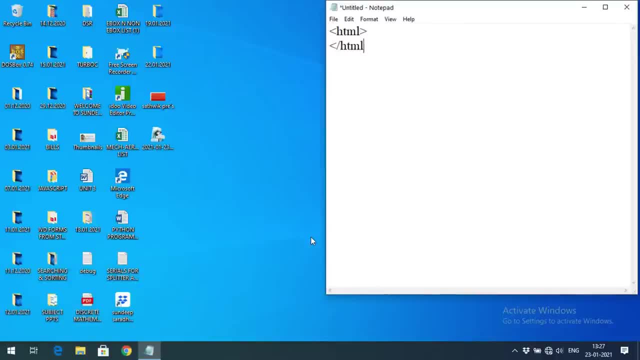 begin with the HTML tags. so I will give the start and end tags of HTML and inside that we will go with the body tag and inside the body will give some title and then we'll write the script. right, so I will go with the h1 get methods. 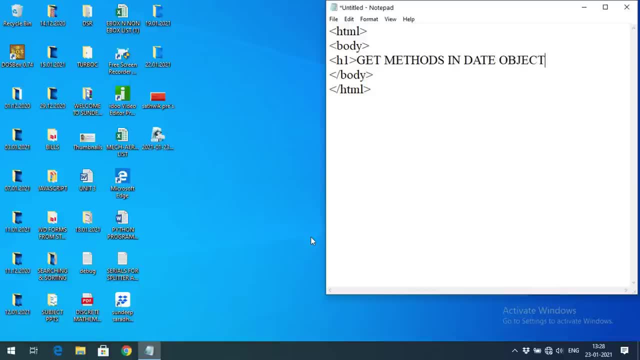 in data object. right now we'll write the script here. so inside this script start and end tag, you need to write it. first of all we have to create some date. so in the previous session we have seen how to create the date by using the date function without having any parameters. we will get the current date and time. so 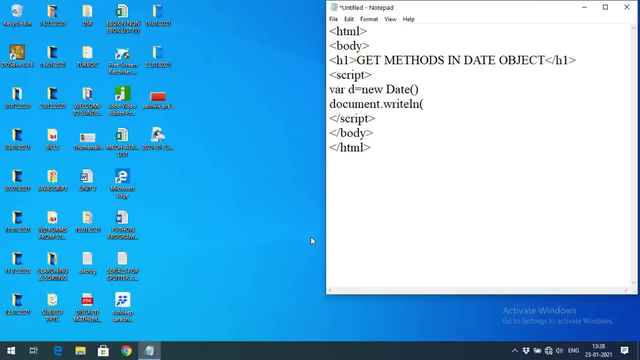 first let us print that current date and time and then we will use the get method, write Ln D plus break line for the next output. so I will save this file by using a name called get methods dot HTML. okay, so you can observe this created and you. 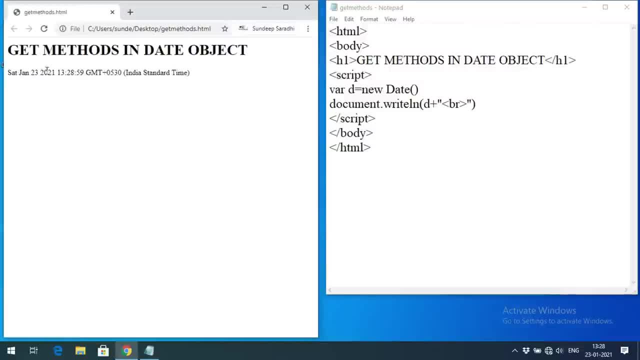 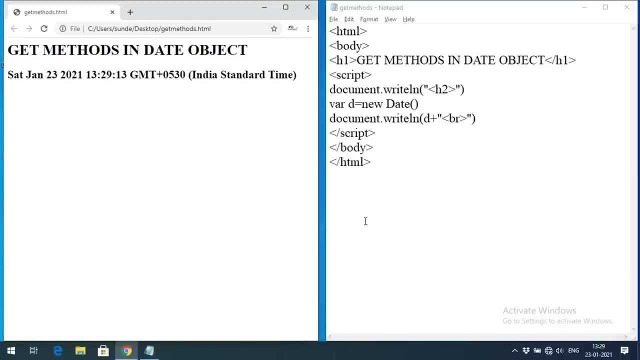 can observe the icon here, so just double click on that, we will get the date right. so before going to that, we increase the size. okay, write Ln H to so that the output will be of: right now let us start with the. as we knew that date and time, we are having some seven parameter. so seven parameters are first one is the year. 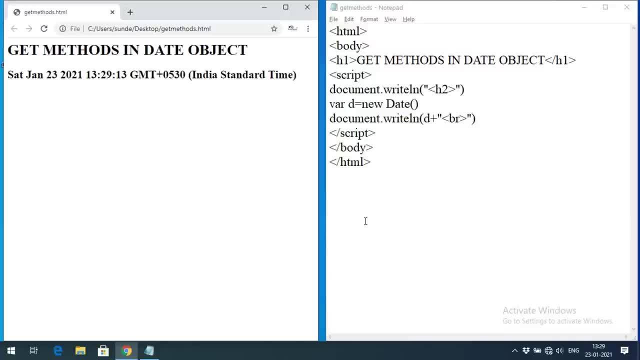 month, date, hours, minutes, seconds and milliseconds. so for for extracting each thing, we are having a separate get function. so, in order to get the complete year, in order to get the complete year, so we need to implement get full year method. so let us start write ln year. so d dot, sorry d dot. 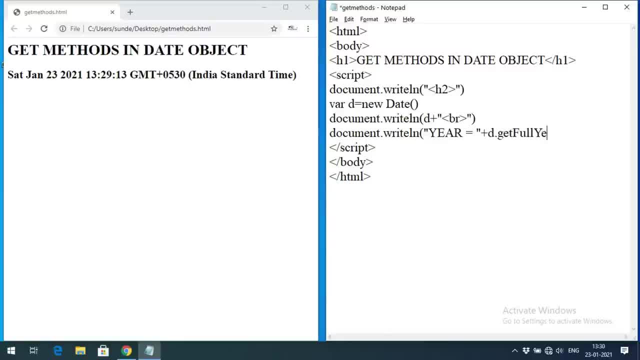 d dot. get full year method right. yeah, now execute this one so you can get the year. year is equal to 2021, so from the current date and time. so here we are taking the current date and time to the d. d is a data object and from the 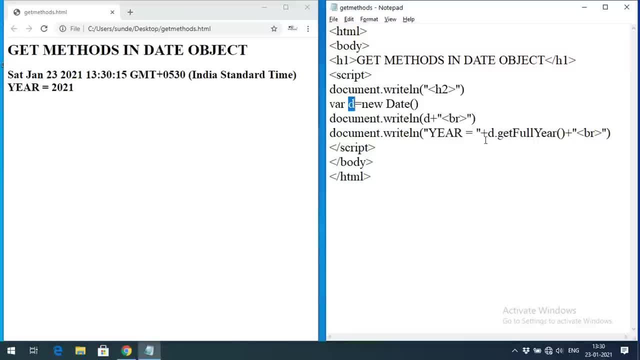 data object: we are getting the full year- full year- right. so get full year will give the four digit year right. similarly, we can copy the same thing, we will execute, so get full year is equal to. in order to get the month, in order to get the month, month is equal to go with the function called get month, get month. so 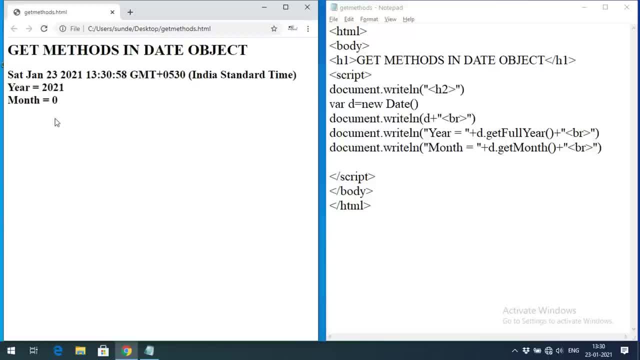 automatically we will get the month zero. so here the month is represented as numbers from 0 to 11.. so 0 represents january and 11 represents the december. so in order to get the month, we'll get get month. so if it is zero, that means january. so this is a january right. 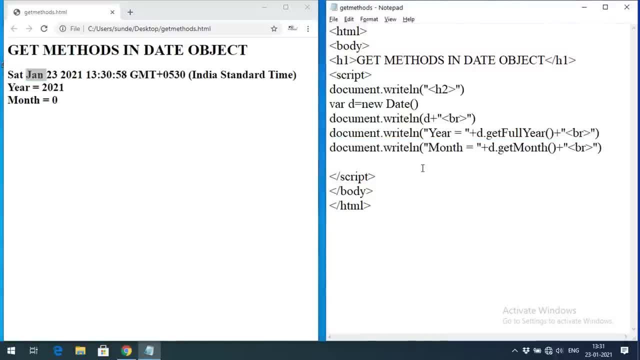 yeah, and there is a one more function, uh, in order to retrieve the date. okay, in order to retrieve the date, so get date. so here date will be from one to thirty one. here the date will be from one to thirty one, so we'll get the date 23, so today date is 23, so this is the current date and time. okay. 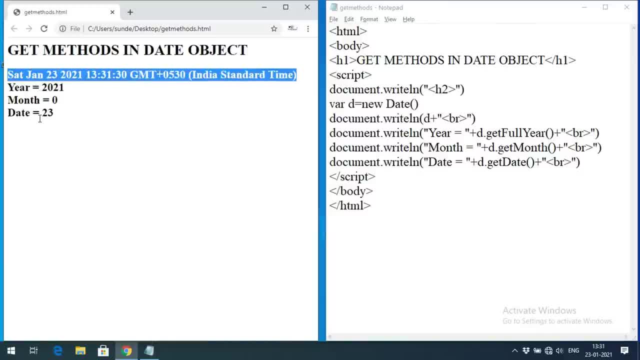 this is the current date and time. so from this we are extracting each and every property, okay, each and every argument right. first year, then month, then date, and also we can get the day. what is the day? okay, document, dot. write l. and day is equal to plus D, dot get day. so here also it will represent the numerical value, will. 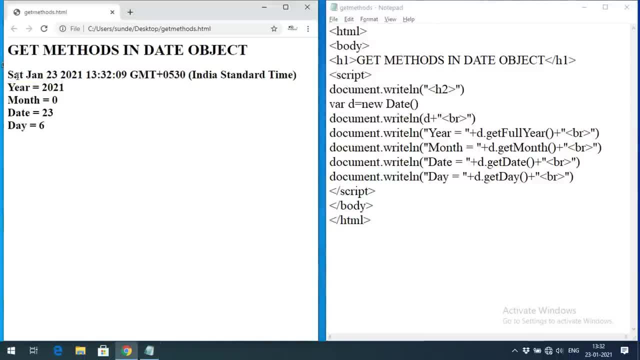 represent the numerical value you can observe. day 6. so today is a Saturday, so it is a day 6, so Sunday it will be 0. right from Sunday to Saturday. the numbering from 0 to 6, right then? and one more thing: that is hours. so we got a. 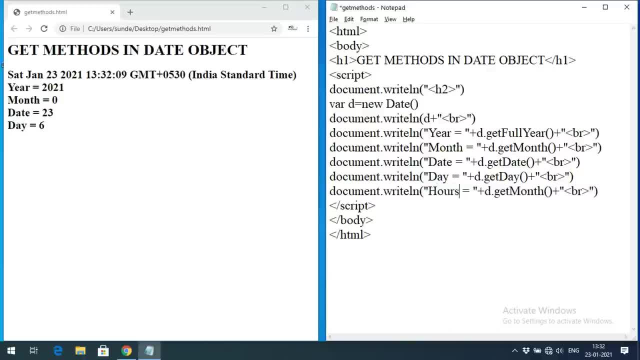 year, month, date, day and now hours in the current time. okay, can get it. okay, see, hours is equal to 13. we can observe here 13, so we'll get the result as 30. similarly, minutes, so get minutes. so we'll get the minutes. can observe here 32. 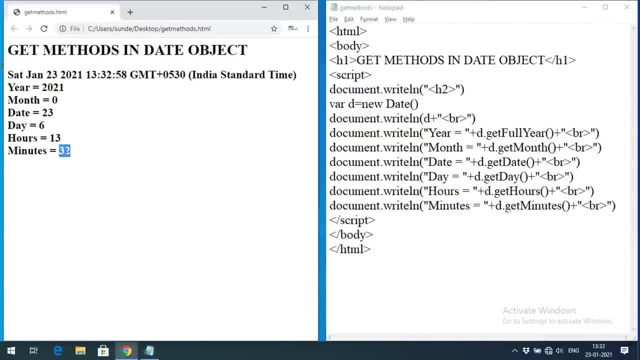 is the minutes, so 32 will be get okay, we are getting some 32, and similarly seconds: get seconds. so you'll get the seconds. so what are the seconds you can observe here? 19 is the seconds, 19 seconds okay, and then milliseconds, so we can also get the milliseconds. milliseconds, so get milliseconds is the. 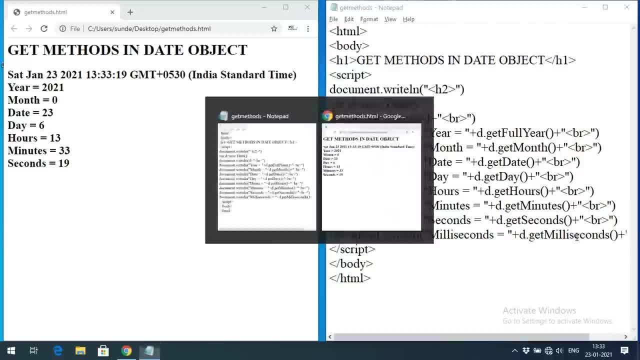 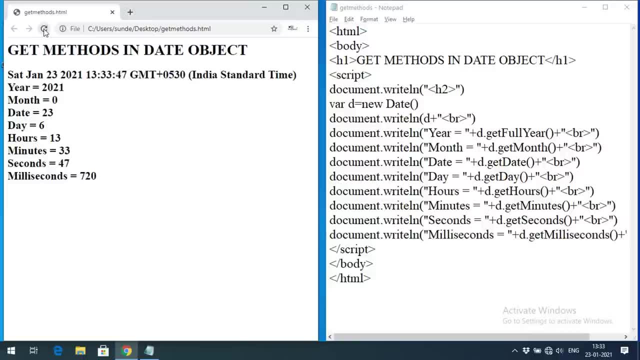 milliseconds. so get milliseconds. is the second method? okay, in order to get the second method. okay, in order to get the millisecond. so this is the milliseconds millisecond. so this is the milliseconds. if you refresh it again, the milliseconds, if you refresh it again, the milliseconds will be changed. okay, we cannot again it. 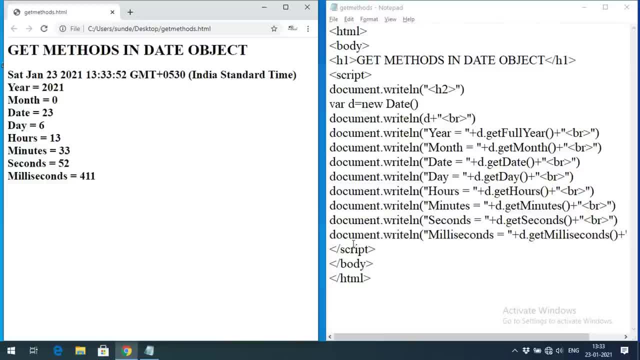 will be changed. then, after the milliseconds, we can also, we can also get the time. so what is the time in terms of milliseconds? okay, so default date will be January 1970 and from that we'll get the milliseconds. okay, get high. so we get till now. till now, what are the milliseconds until? 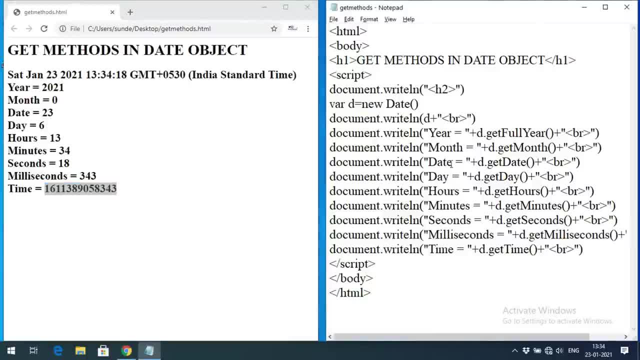 the date, how many milliseconds we are getting, so that will be displayed here. okay, so this is. these are all the different get methods. so in order to get the year that were getting, that was time, that was七 Nos, but it is also 0 minutes or second. N is nap word расп 1985. 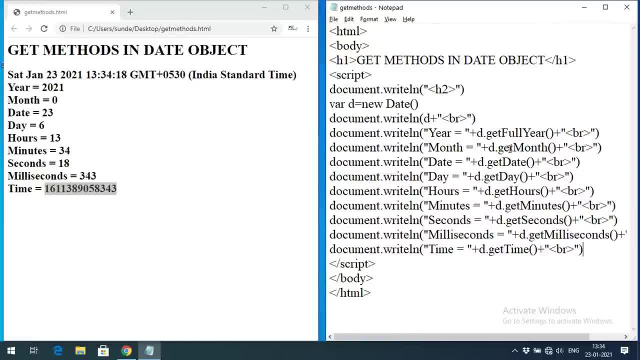 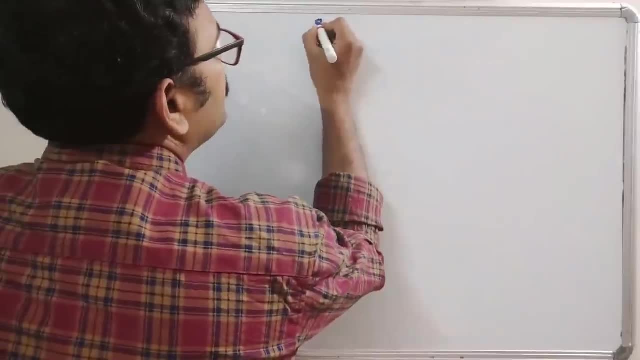 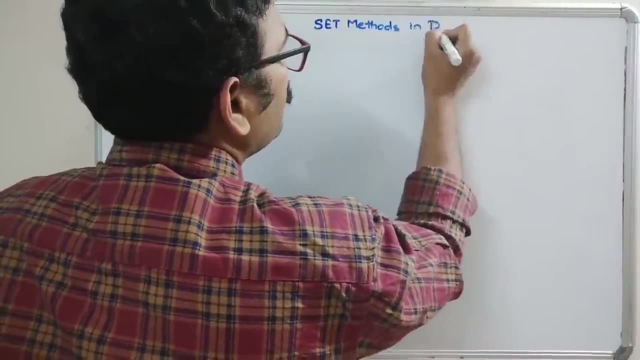 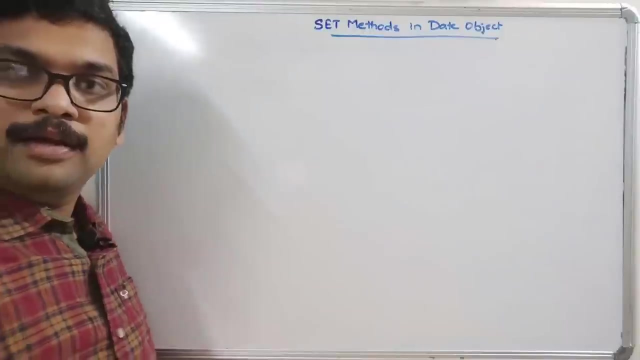 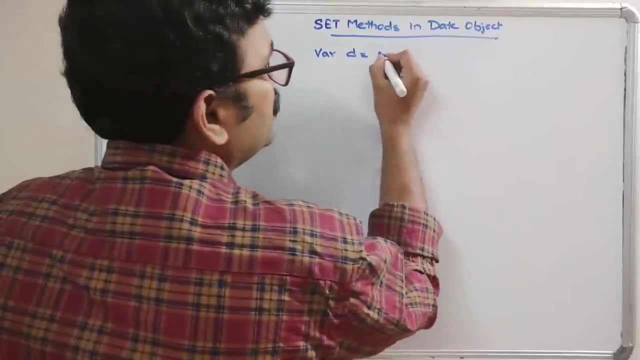 month, date, day, hours, minutes, seconds, milliseconds and time. so we can get all these things right. so we can get all these things set: methods in date object right now. here also we can go with the same thing. so we'll create some b, that means we'll get the current date and time. so d is equal to mu. 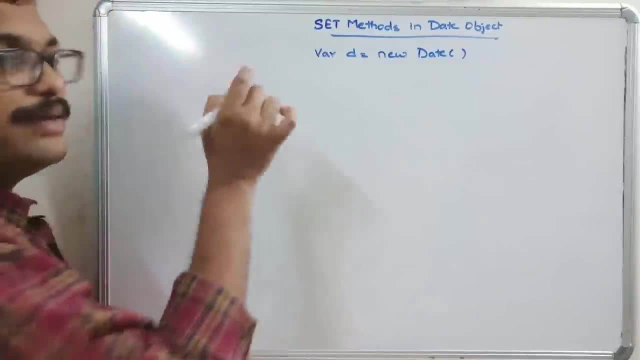 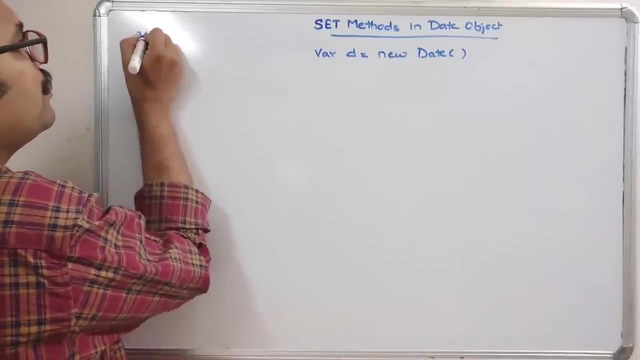 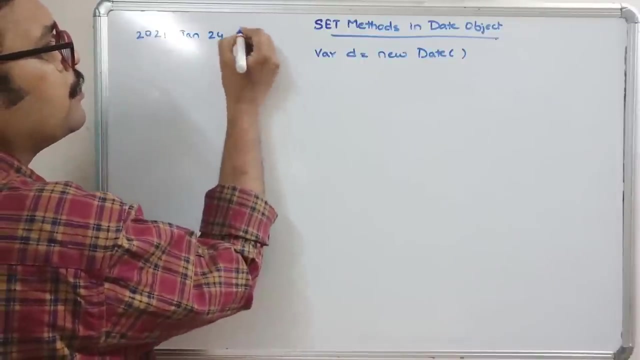 so we can go with the same thing. so we'll create some b. that means we'll get the current date and time, so that we'll get the current date and time. current date and time. so current date and time. it is some sorry. yeah, 2021, january 24 and then uh hours. 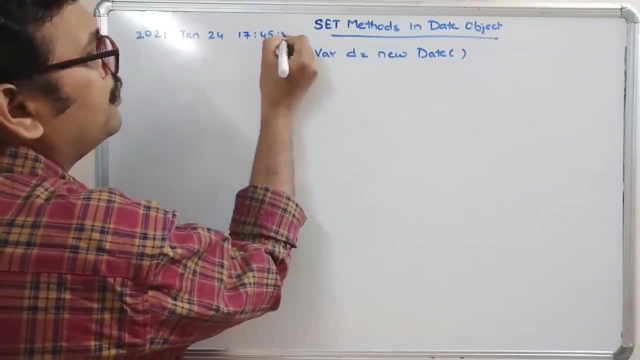 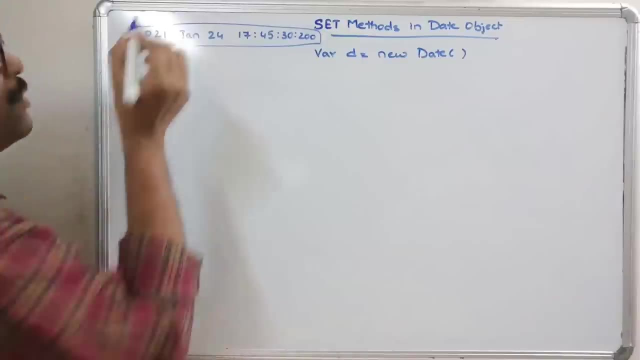 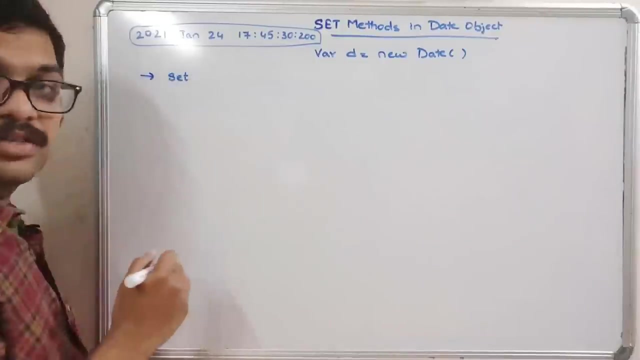 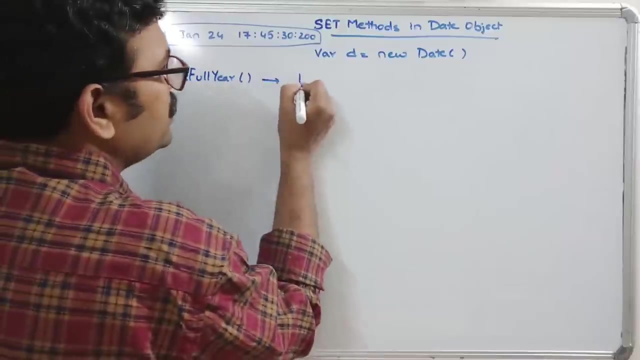 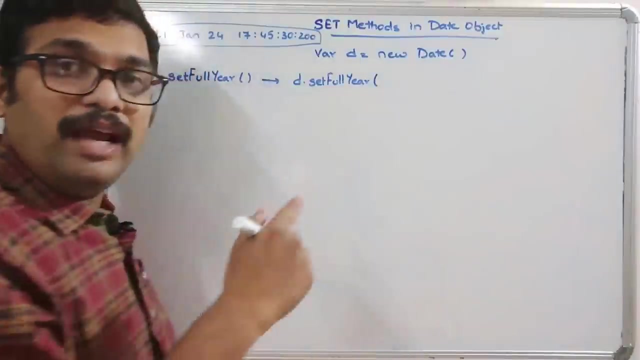 17, 45, 30, 200. so this is the date, current date and time, for example. right, so we need to set the year and all these things. in order to set that, we are having a different methods called set full year. so the syntax for this one is d dot set full year. here we need to give either month and year. okay, 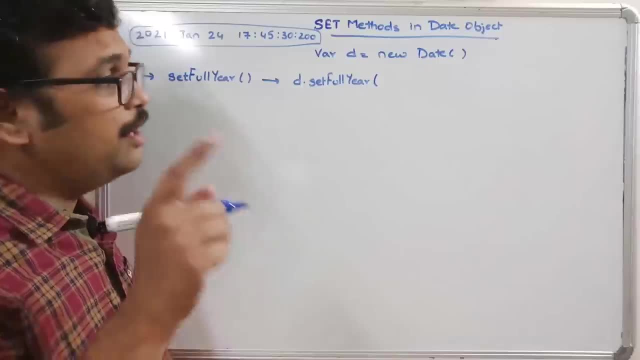 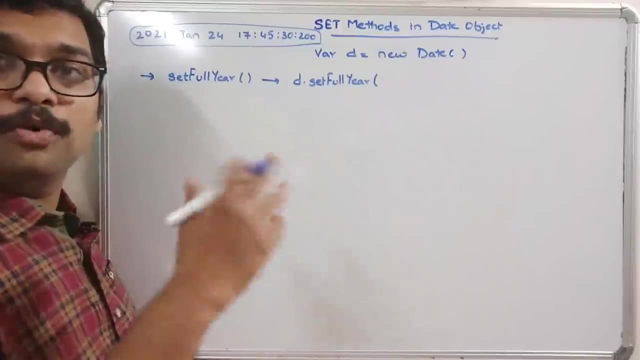 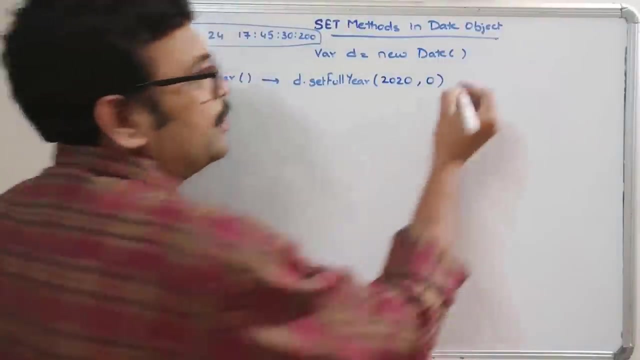 so during the creation of a date. we have seen so if you give only the four digit year, that will be considered as a millisecond. so here we are supposed to give both the year and month. so here i will go with the 2020 comma zero. zero stands for january, so automatically the result. 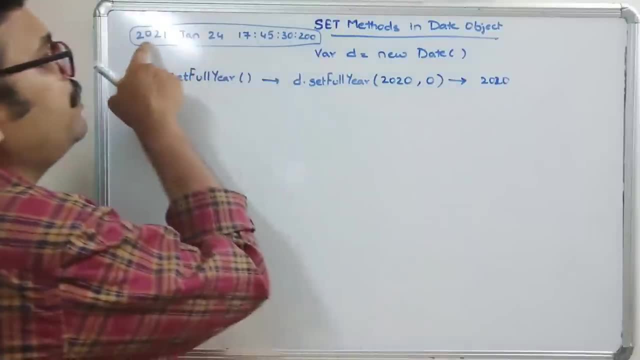 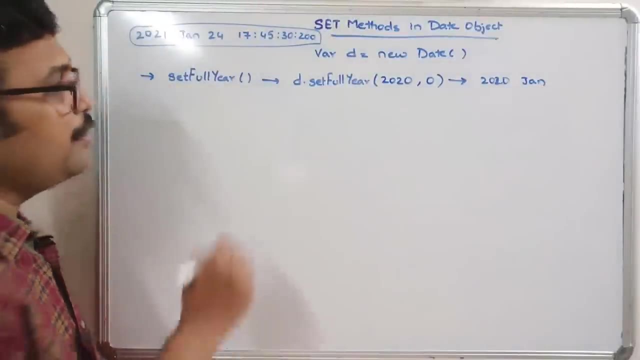 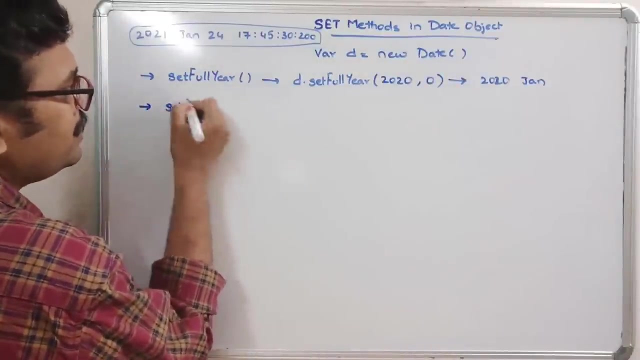 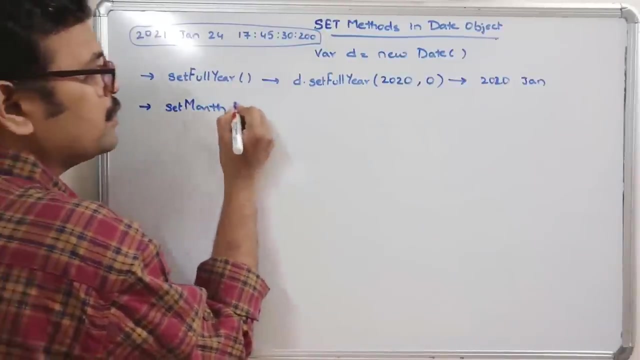 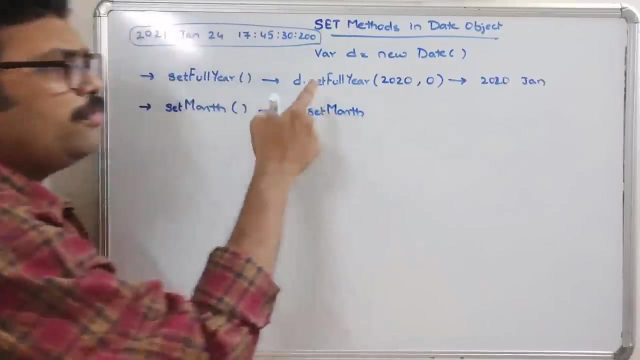 will be 2020, the the year for the given date will be set to 2020 and the month will be january. okay, so, so, so, so, instead of 2021, we are setting the date as 2020, then set month. so we need to set month. okay, so, set month. and if you after that, after that. 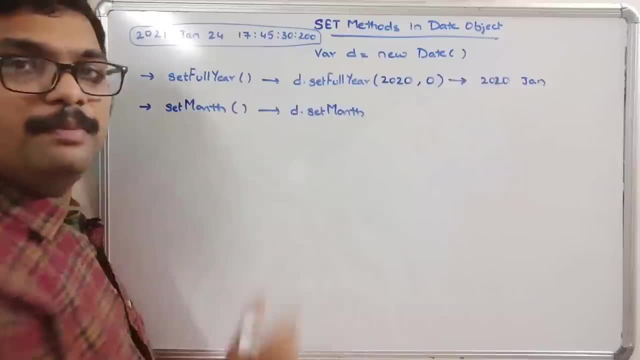 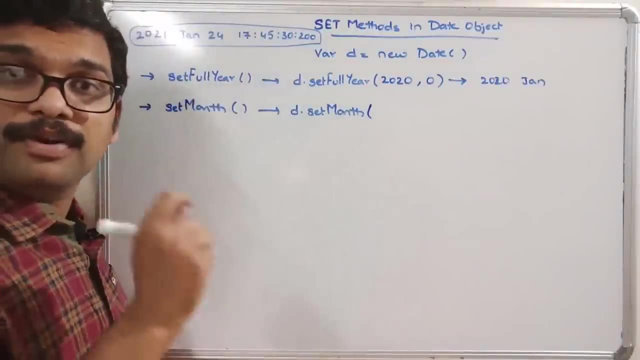 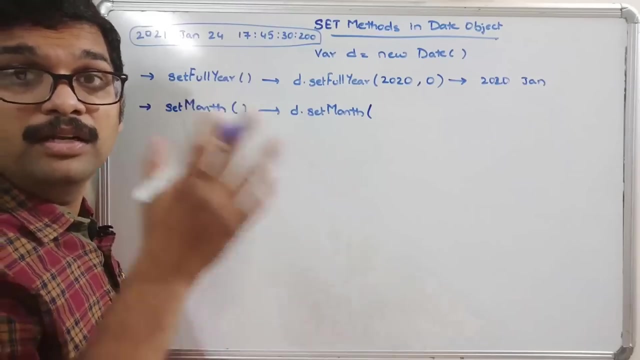 if you print the d, automatically the updated will be coming up. okay, now, set month, set month, and here we need to give from either 1 to 31, right? so the month, sorry, 0 to 11. here the month will be from 0 to 11. so 0 for january, 11th for december. so here here we have to give that month. 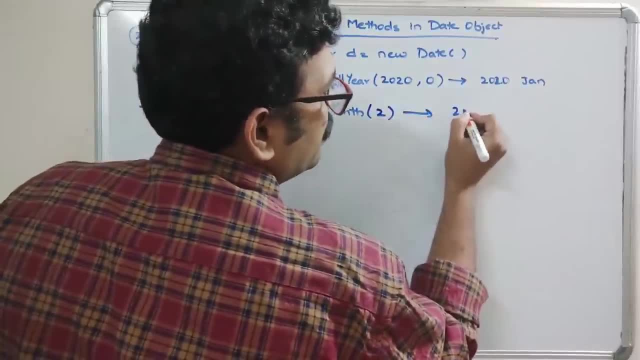 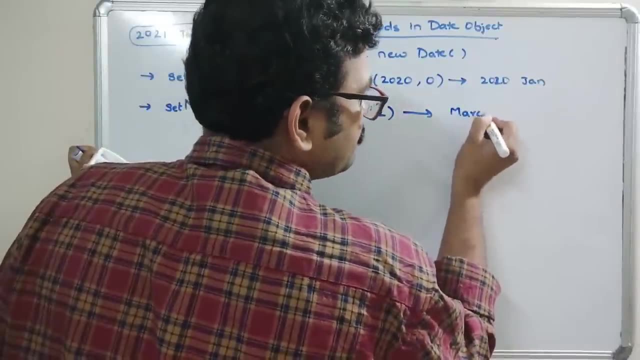 i will give 2. okay, automatically, that the month will be set to 2. 2 means march, 2 means march, set month, and here we need to give from either 1 to 31, right? so the month, sorry, 0 to 11. here the month will be from 0 to 11. so 0 for january, 11 for december. so here we have to give that month. i will give 2. okay, automatically, that the month will be set to 2. 2 means march, 2 means march, 2 means month. 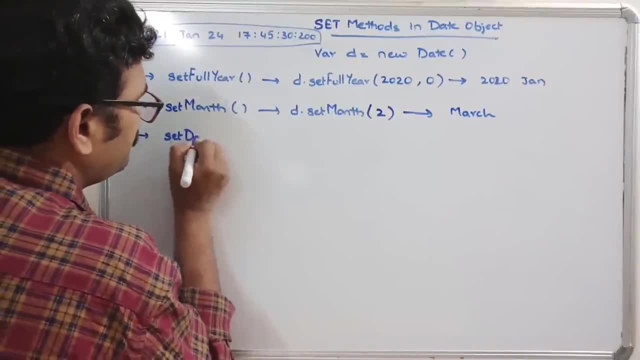 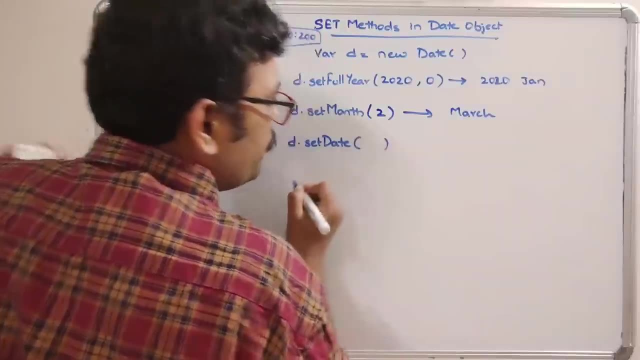 so here we have to give that month. i will give 2. okay, automatically that the month will be set to 2. 2 means march. 2 means march 2 means month. similarly, set date. so here, set date. here we need to pass from 1 to 31 because 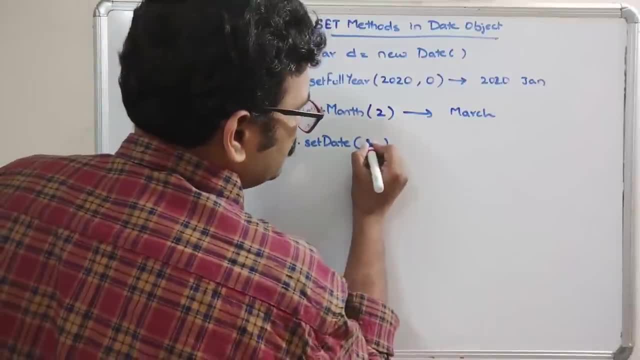 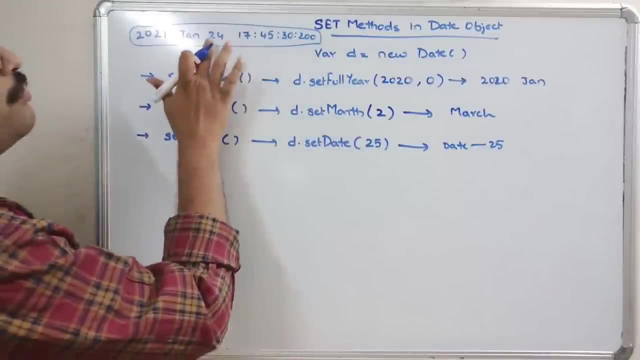 the date will be from 1 to 31. so we can set here some 25 so that the date will be 25. it will be set to 25. so instead of 24 we'll get 25 here. so i will execute each and every. 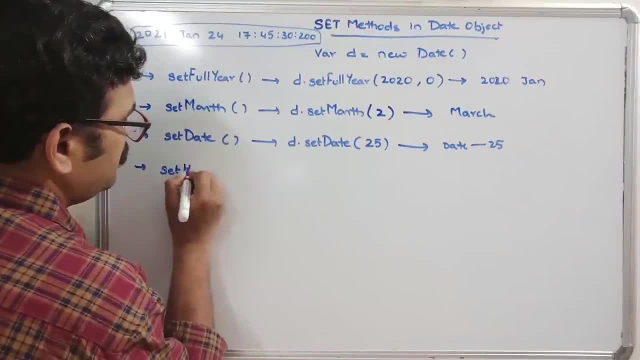 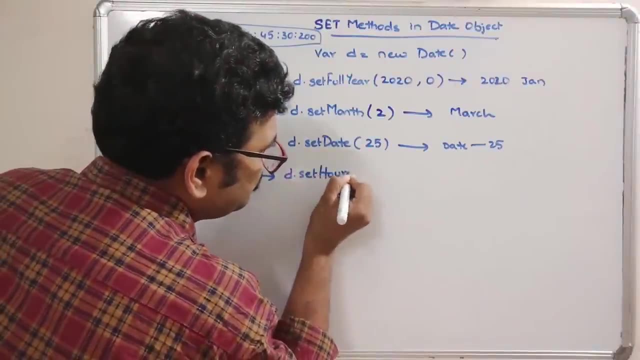 we'll get 25 here, so i will execute each and every method, don't worry. set hours, set hours: so d dot set hours. set hours, set hours, so d dot set hours. set hours, set hours, so d dot set hours. and here we need to give from 0 to 23. 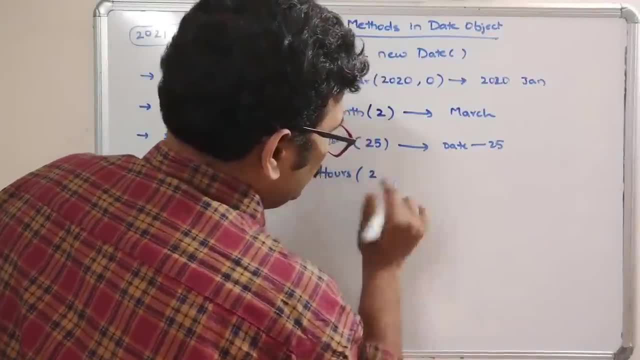 and here we need to give from 0 to 23. and here we need to give from 0 to 23. okay, i will give with 24. oh, sorry, okay, i will give with 24. oh, sorry, okay, i will give with 24. oh sorry, 22. so automatically, the hours will be. 22. so automatically the hours will be 22. so automatically the hours will be set to. set to set to hours will be set to 22. so instead of 17, hours will be set to 22. so instead of 17, hours will be set to 22. so instead of 17, we'll get 22 here. 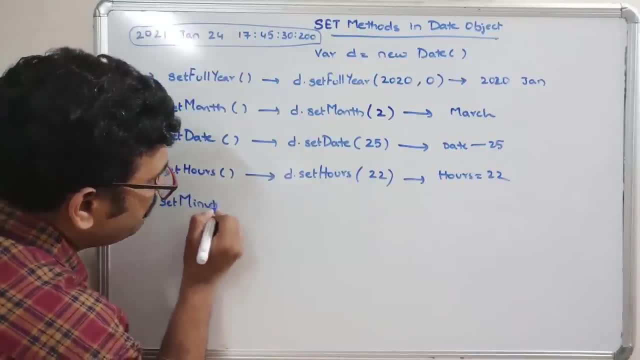 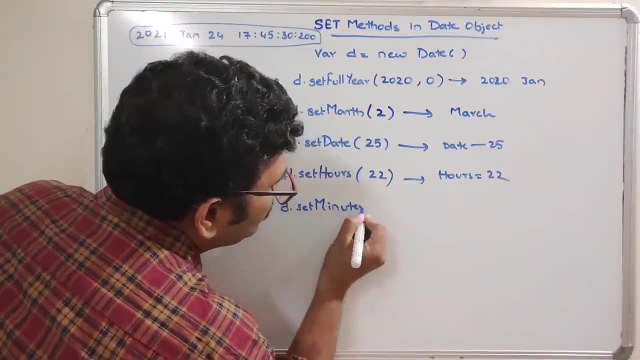 we'll get 22 here. we'll get 22 here. next set: next set: next set set hours will be set to hours will be set to 22. so instead of 17, we'll get 22 here. next set minutes: so we can also set the minutes d dot set minutes. okay, so here we need to give from 0 to 59. 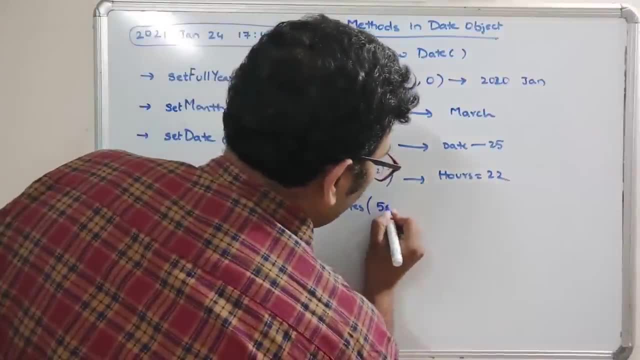 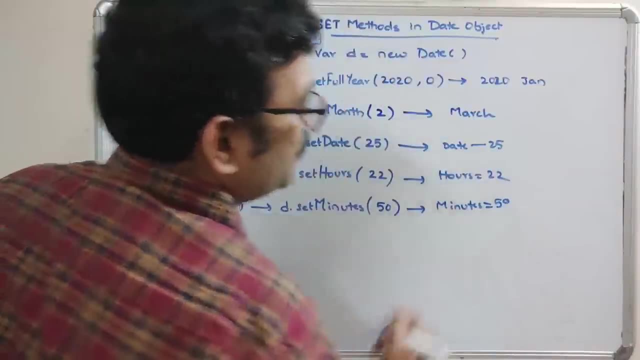 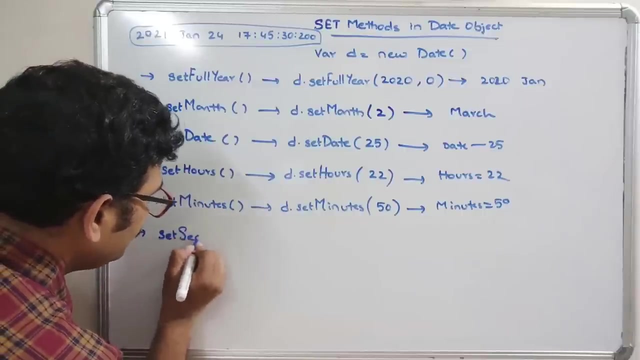 because minutes will be varying from 0 to 59, I will go with a 50 so that the minutes will be set to 50- 50, right. so here instead of 45 we get a 50 set seconds. so here also the seconds will be from. 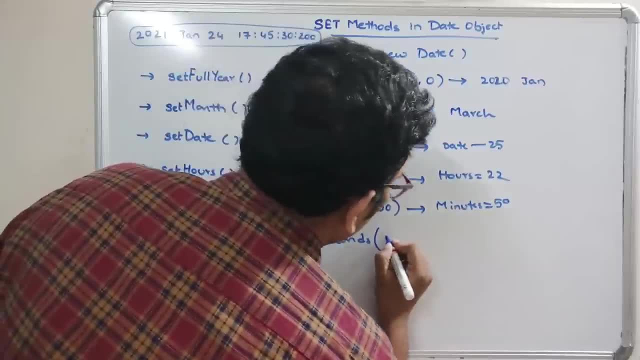 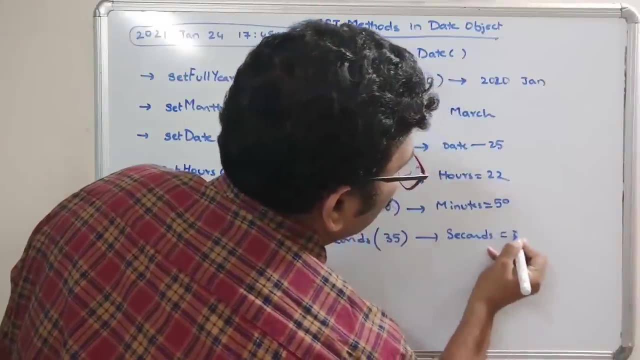 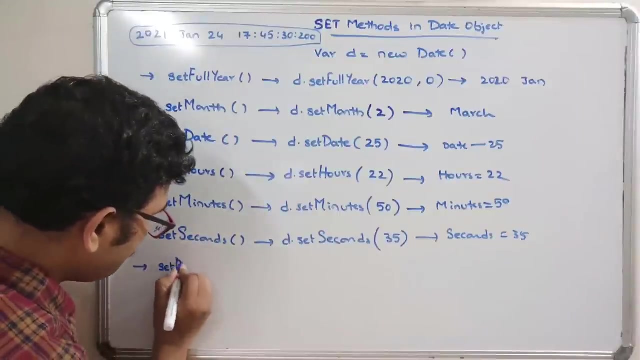 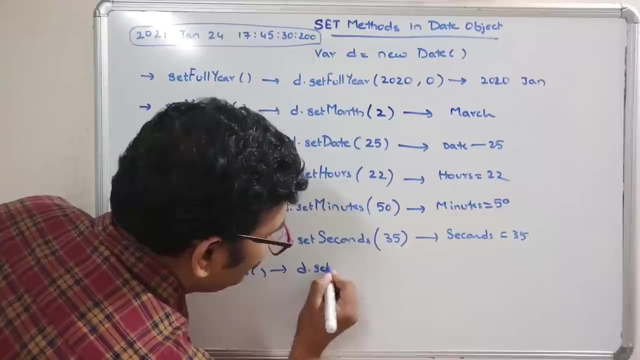 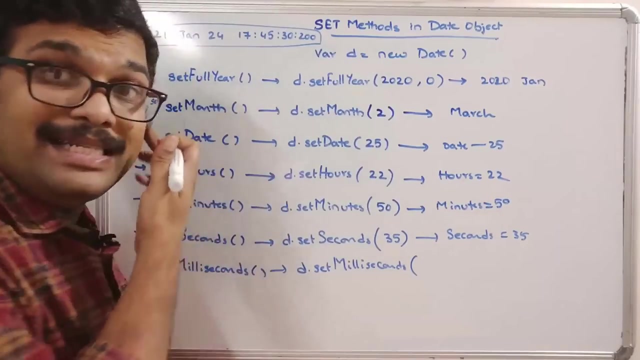 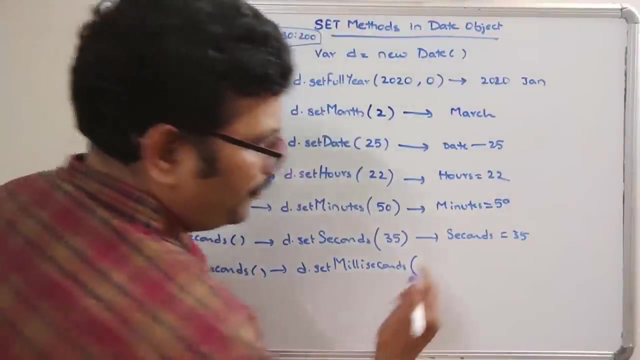 0 to 59. okay, so here also I will go with the. some 35 will get. the seconds will be set to 35, so instead of 30 will get 35 as a result. similarly set milliseconds. milliseconds we can represent in a millisecond, so set milliseconds. and here we need to give the milliseconds the number of milliseconds. okay, from 0 to 999. okay, so I will give some 400. 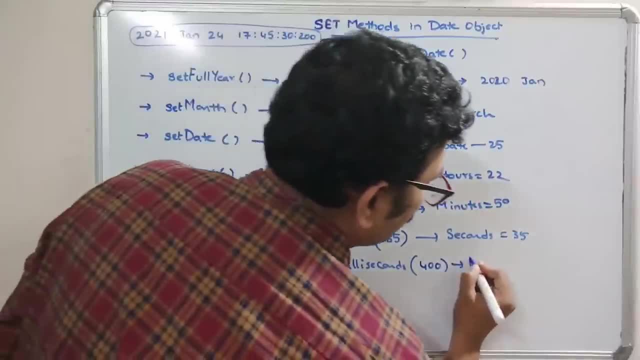 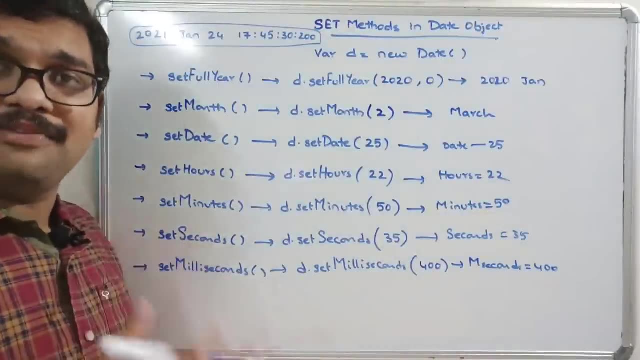 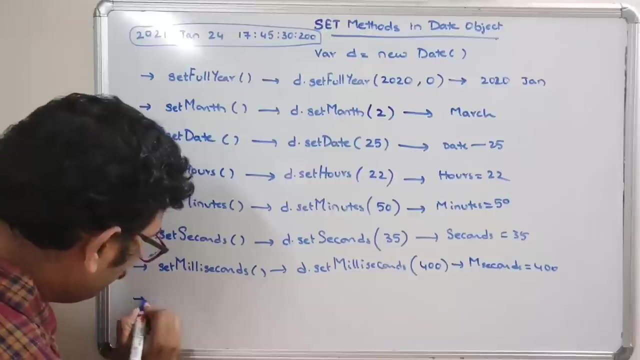 so automatically the milliseconds. the milliseconds will be set to 1 minute seconds will be set to 400. so like this we can set all the seven attributes like year, month, date, hours, minutes, seconds and milliseconds. and there is a one more thing called set time, so we can also. 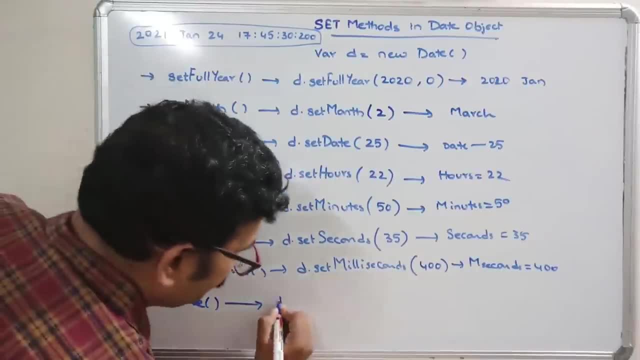 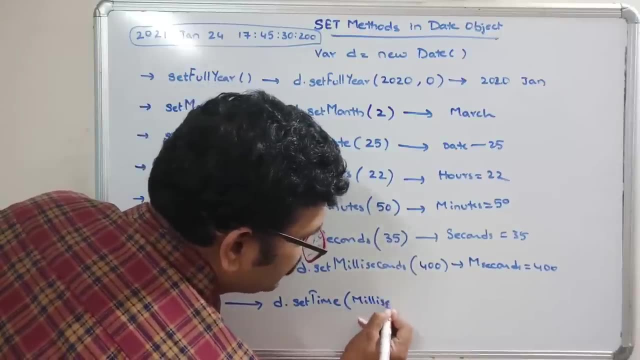 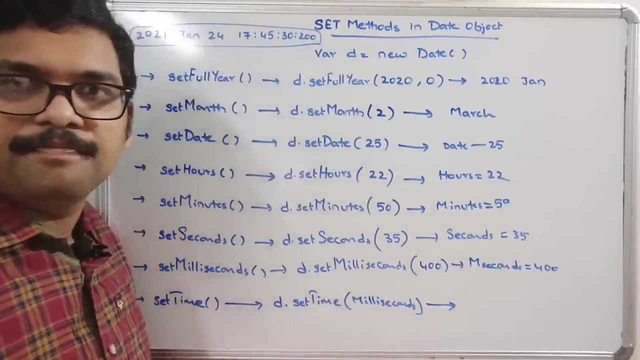 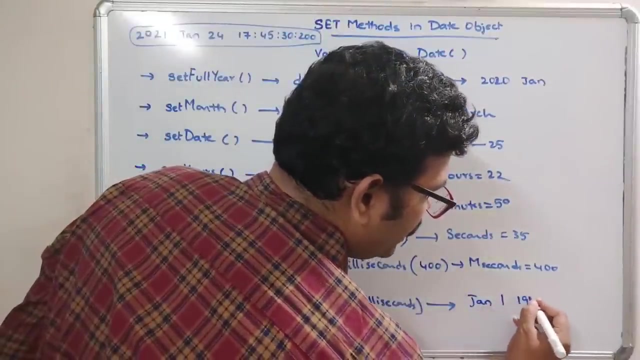 set the time. okay, we can also set the time. so d dot set time. and here we need to pass the milliseconds, the number of milliseconds. okay, so that it will return the date applying with this milliseconds. okay, so the default date is january 1 1970, january 1 1970. so from this date, 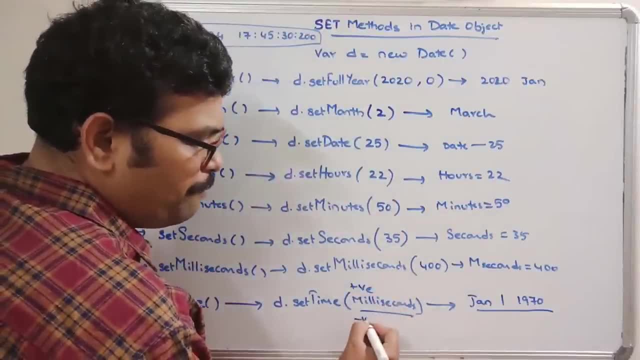 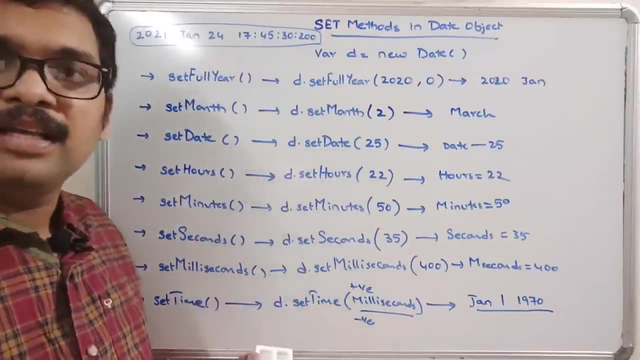 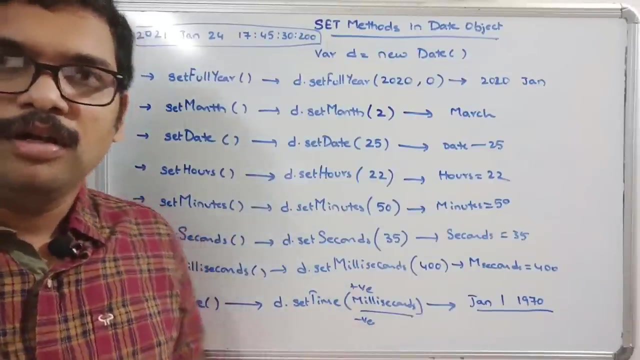 it will add the milliseconds if it is positive and it will minus the milliseconds if it is negative. right, so this is how we can apply the set methods. right? so i will demonstrate each and every method by executing a small code, so we'll see. we'll execute the same on the system. 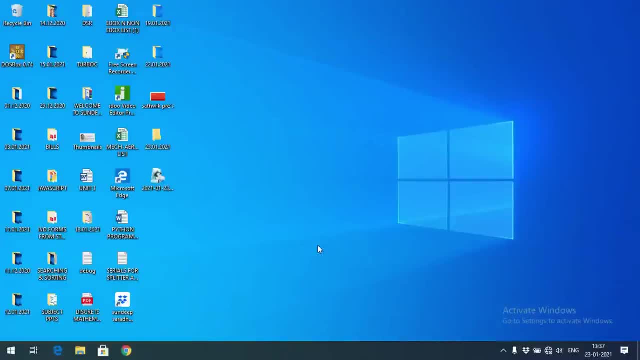 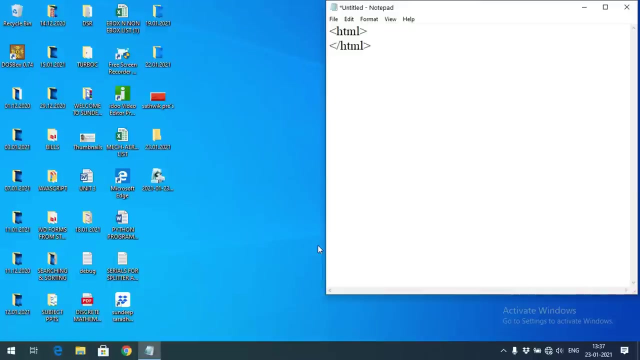 so let's move on to the system. hello friends. so just now we have seen a different set methods of data object. so now i will demonstrate each and everything by executing a small code. so let us start writing the code by from the html tags. so inside the html tag we write the body and 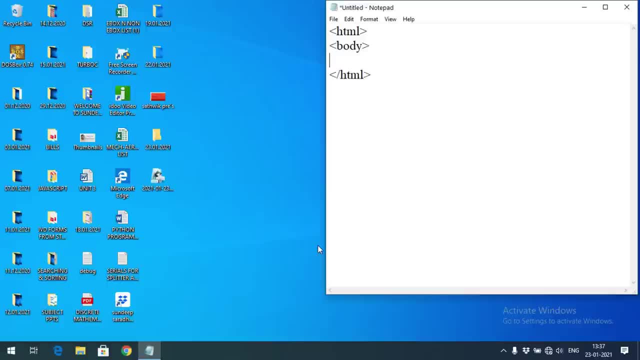 we use some title for that and then we'll write the script. yeah, now give the title. so: h1 set methods in date object. so here also we'll create one date object and then we'll start fixing the different parameters right now. so let us take some document, dot write ln, h2. yeah, so where d is equal to. so we'll take the current time. 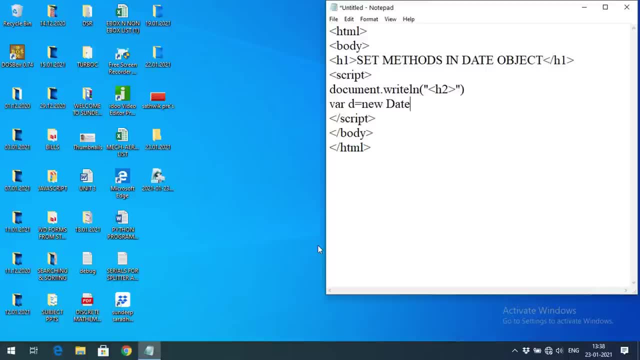 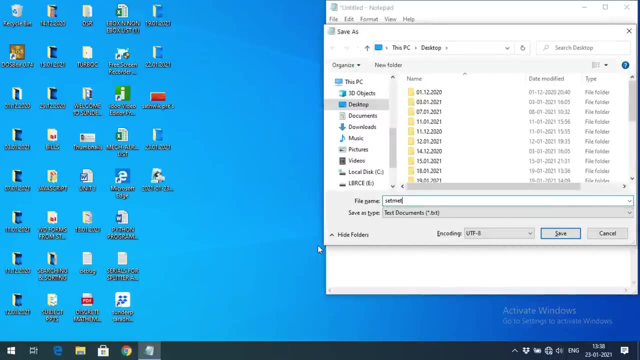 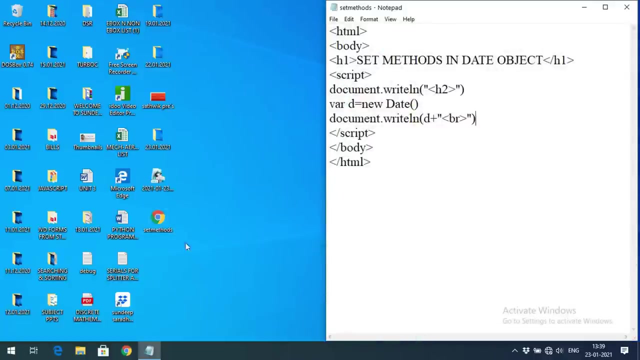 okay, d is equal to new date, so that it will give the current date and time. so document dot write ln d plus cr. so let us save this one with the set methods. the name was the set methods dot html, so you can observe here the icon and we'll double click on that so that we will get the 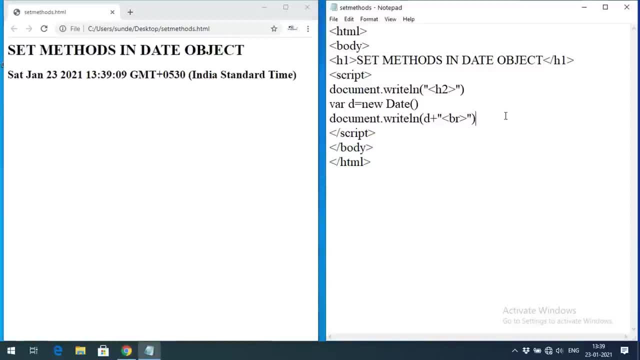 current date and time. see, this is the current date and time and now we'll set each and every date so we can set our own date. so you can observe here. so this is the current date and time right now. let us go with the date. so here the date is 23, but we are setting here, so d dot set. 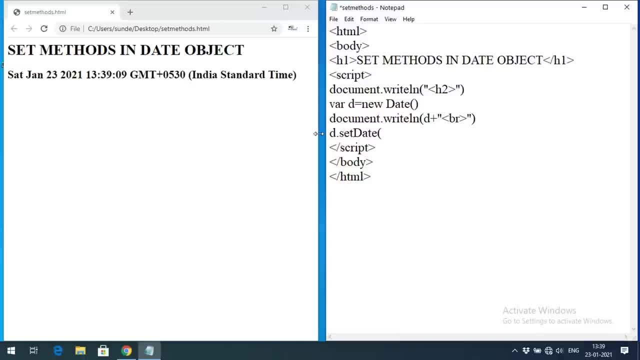 date of. here the date values will be from 1 to 31. that should be given as a parameter here, so i will go with the 24 or 28. okay, so i have set the date for 28. now i will display here new date plus d plus dr. right now we will execute here you can observe the new date is 28th january. 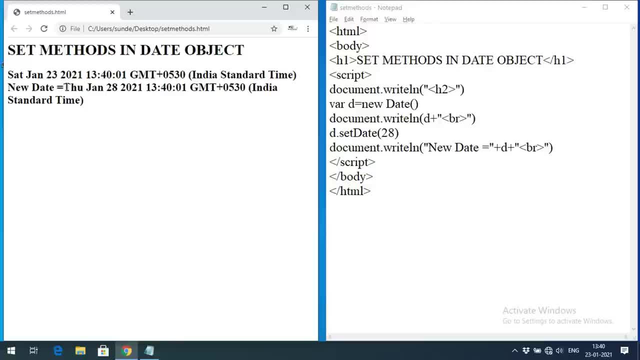 so obviously the day will also be changed. okay, then the date- i mean the day is- also- has been changed. i will show you. so now you can observe the completely printed in the next line so you can observe here. see, if you observe here, january 28 is thursday, so automatically we got it as a thursday now. 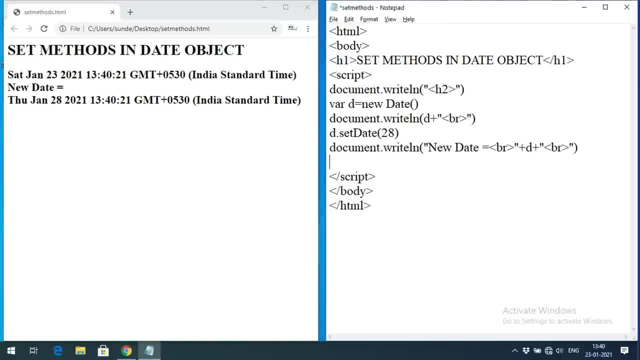 the next one is: we can set the year also. so let us set the year, set full year. so here we need to give a month and year. okay, month and year. i will give the month, as i will give the year as a 2020 and zero. that means i have changed the year from 2021 to 2020 and now let us check the date. okay, so. 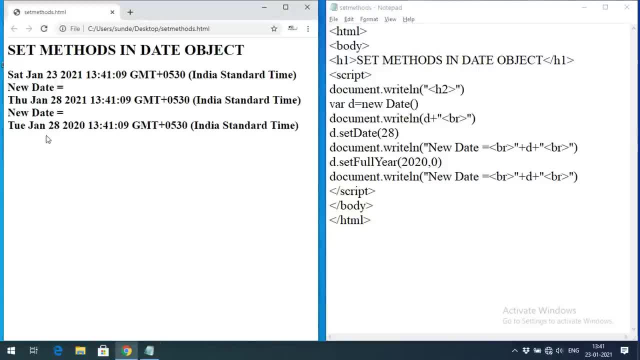 new date. let us check. you can observe here: 2020 january 28th. okay, so because here we have given 2020, so previously it was 2021. i have set the date to 2020, so we got the result as 2020 jan 28. so this is how we can set the full year we can set. 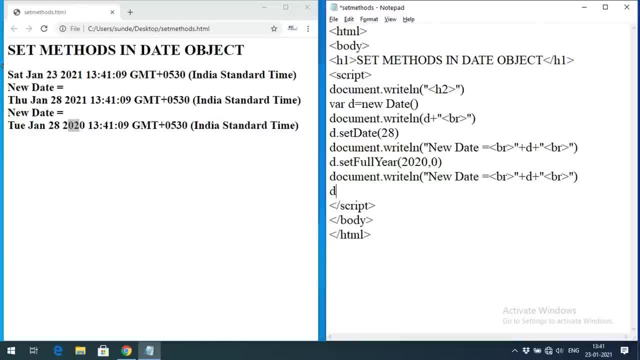 the date and also we can set the time also. so go with this one d dot set hours. so you can observe: previously it was hours is 13, so we can change the date from 0 to 23. okay, the values of hours will be from 0 to 23. we can give any one value, so that will be replaced with the current value. 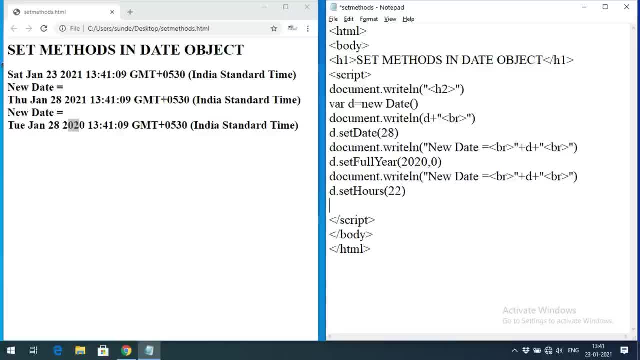 so i will go with 22 right now, again, you can observe the new date. see here you can observe 22 is the new updated hours: updated hours. and then next we can also set the minutes. so i will set the minutes, set minutes, and this minutes can be of values from: 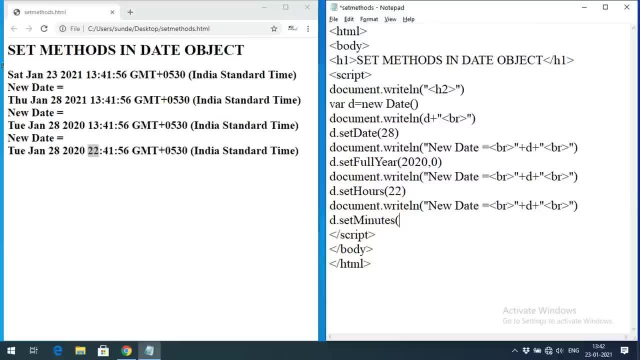 0 to 59. okay, 0 to 59, so previously we can have. it says a 41, i will go with some 50, 52, right, so? and again, see you can observe here, so it is a 52 now. okay, the change it as 52, so you can observe the date. 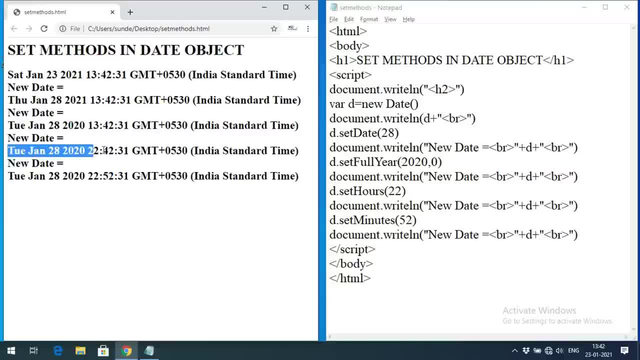 has been changed, the year has been changed, that the minutes has been changed and, sorry, the hours has been changed and now the minutes we have changed and similarly, we can also change the second minutes. we have changed, the second minutes we have changed and now the minutes we have changed. 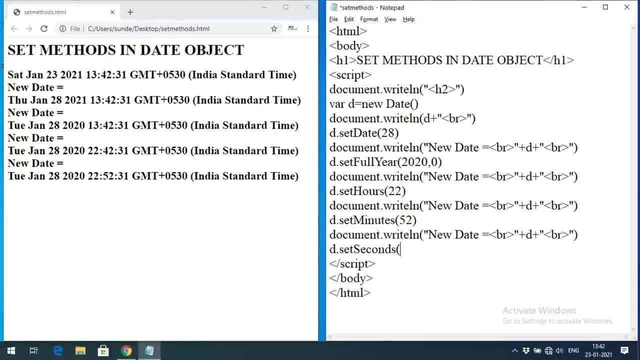 So d dot set seconds. So seconds will also be having the values from 0 to 59, right. So I will go with the 50 minutes seconds as a 50, right? So now again check you. 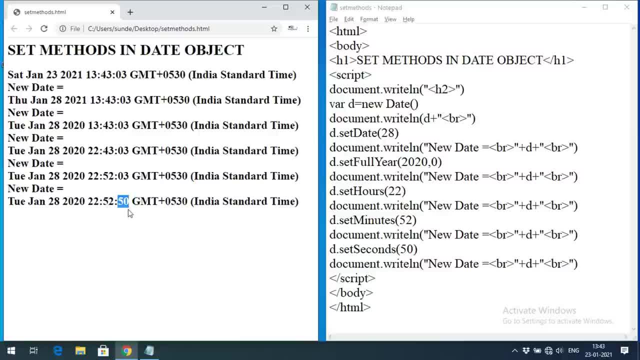 can observe, it was set to 50,. okay, It was set to 50.. And similarly we can also change the milliseconds. We can also change the milliseconds D dot, set milliseconds and give the milliseconds. here The milliseconds range will be from 0 to 999.. So I will give some 500 here and 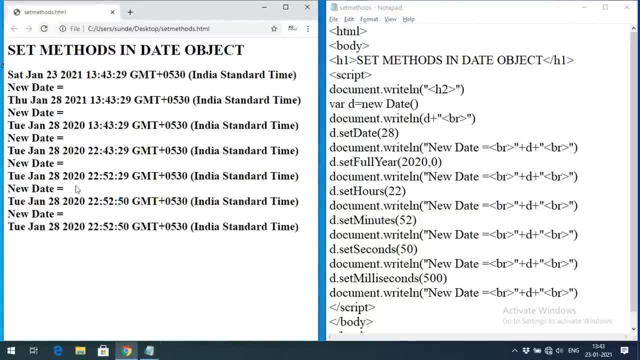 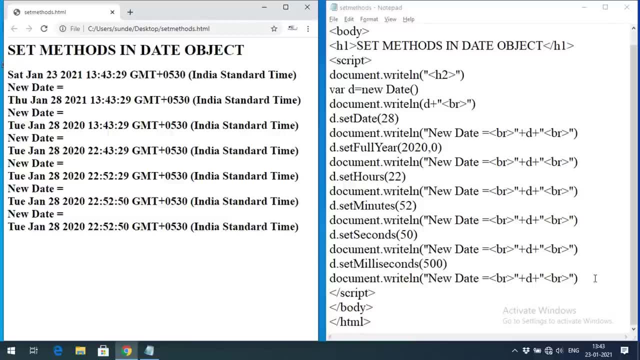 we will get the result so that you can observe here. So here we are not having the milliseconds. If you get the milliseconds automatically, we will get it right. So immediately that will be changed And also we can set the time with the help of milliseconds. that already we have seen. 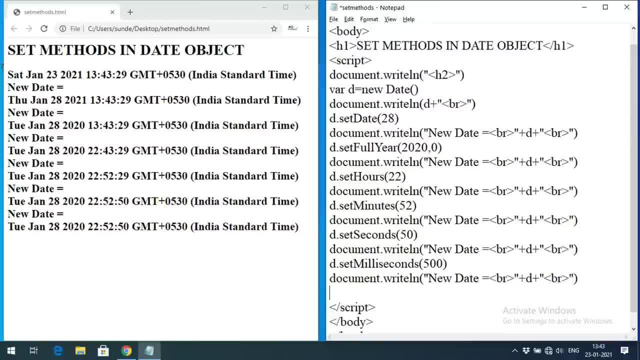 by using the date function. So we are passing some number of milliseconds as a parameter to the date function. Automatically it will be changing the date. Similarly, here also we are having some set time- set time in terms of milliseconds, So I will go with this: milliseconds. 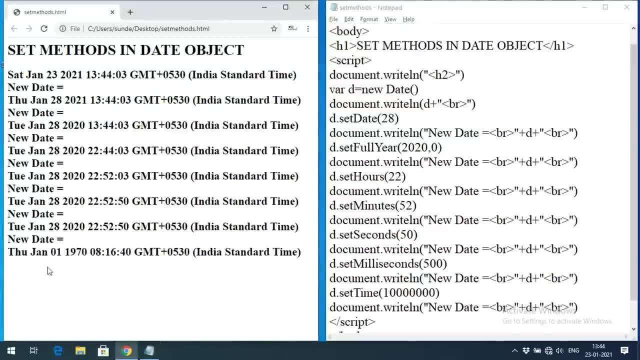 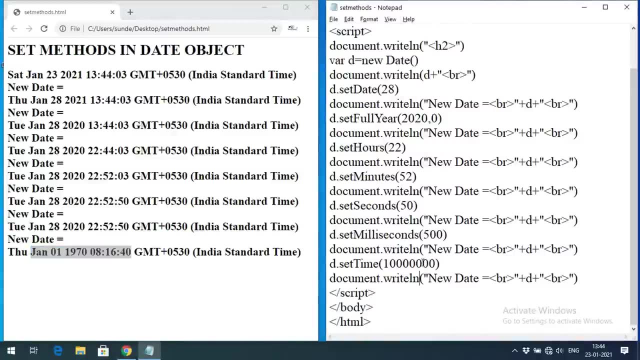 and let us check here So you can observe. So the default date will be from January 1, 1970, 530. From that these milliseconds are added and the updated date is this one. Hope you understood this one. And also we can add the dates. We can add the dates See. So here we are. 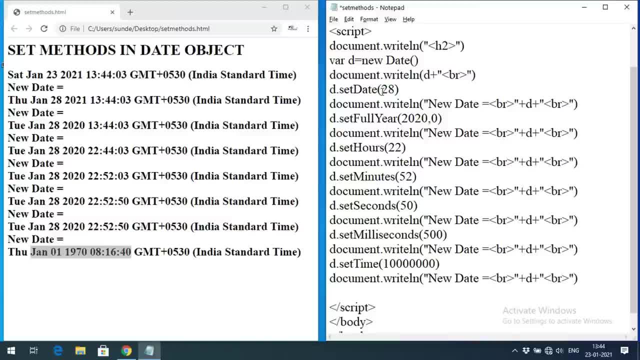 adding some date 28.. So here we can add more number of dates, See D dot. instead of writing here, I will write the same thing here instead of writing all these things. so d dot, getDate will give the number of days here. so I will give the number of days, getDate and plus some. 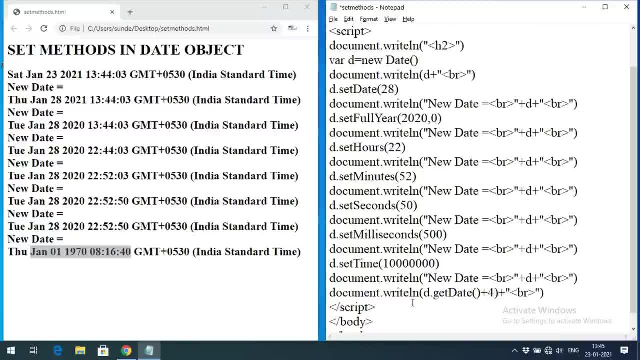 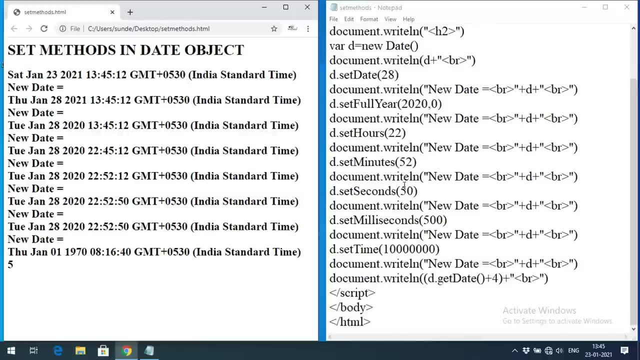 I will add some 4 days. now you can observe here: see getDate plus 4. automatically it will return the updated dates. so this is how we can implement the set methods in date update. so by default the date will be having 7 parameters, that is, year, month, day, hours, minutes. seconds and milliseconds, So all those things we can implement. So, by default, the date will be having 7 parameters, that is, year, month, day, hours, minutes, seconds and milliseconds. so all those things we can implement. So all those things we can implement. 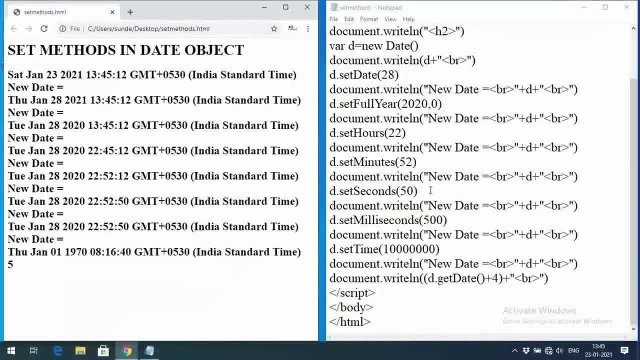 We can set this with the user defined values. so whatever the values we can give. so here the date represents the number from 1-31 and the hours from 0-23, milliseconds with 0-999, minutes with 0-59 and month from 0-11 and seconds from 0-59, right. 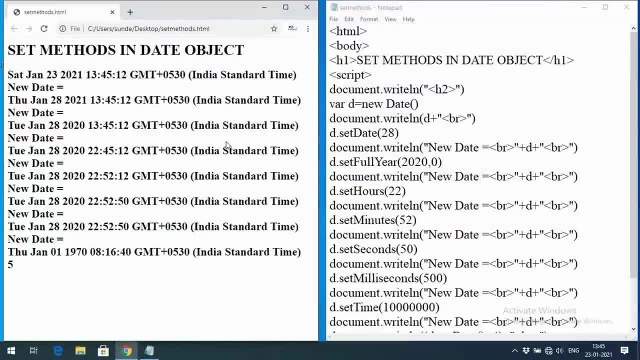 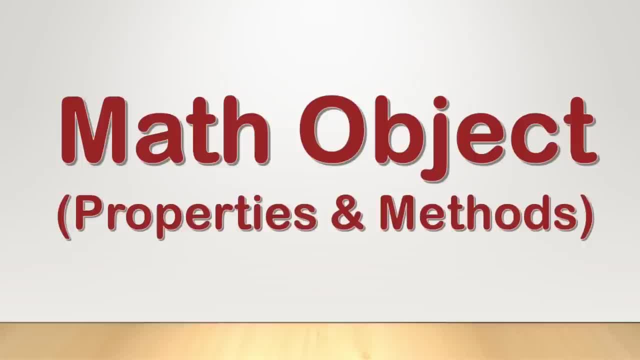 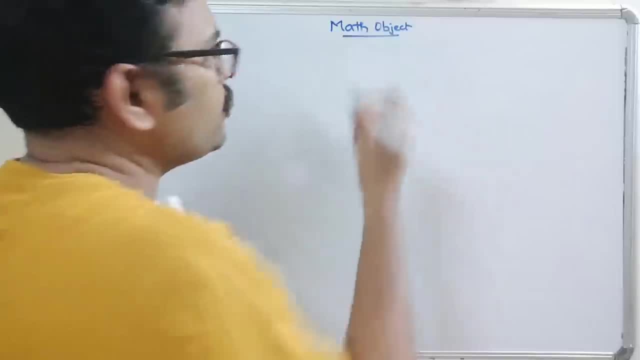 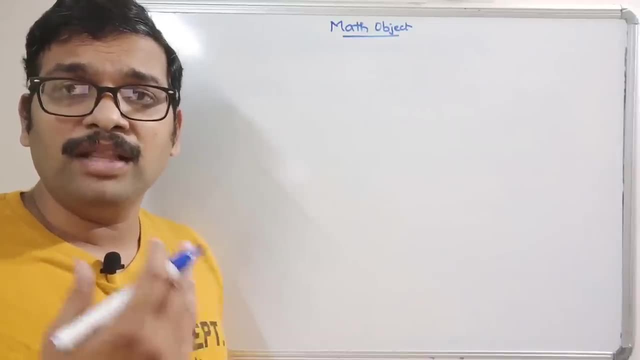 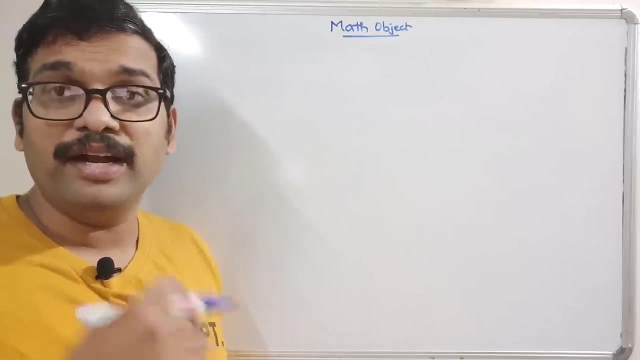 So this is all about our set methods in date object, math object. so here, if here also we will be having the methods and properties, but one thing: we need not create the object with the use of a new keyword before using those methods, so we can directly call those methods and also we are having some properties for this math. 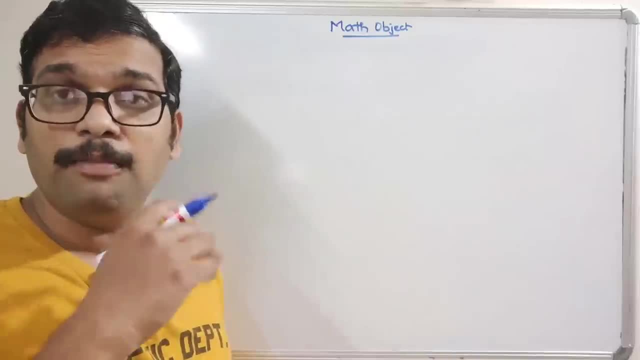 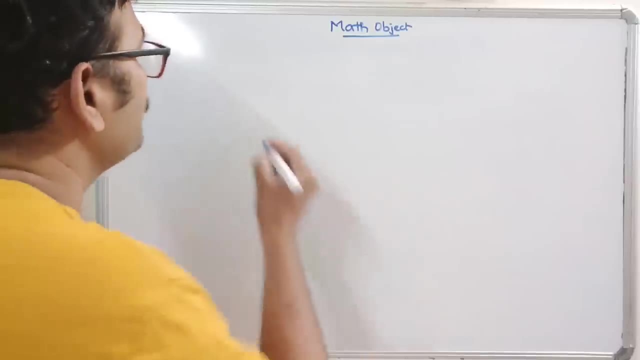 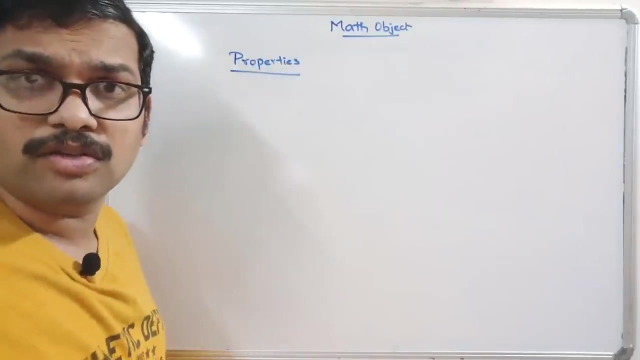 object. so those properties can also be used with the help of math name, right? so first we'll see the properties of math and then we'll go with the methods. so first one is the properties, properties or constants- we can call also constants- right? so the first one is. 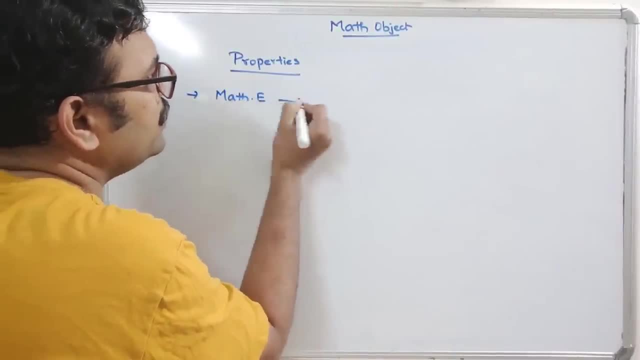 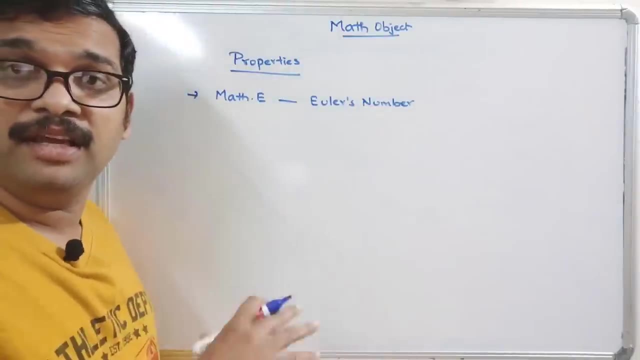 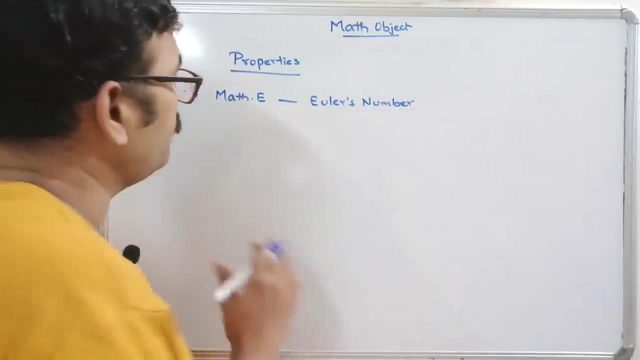 math dot e is nothing but euler's number, so it will return the euler's number. so i will execute each and everything and i will show you right. so i will demonstrate each and every method and property and by you executing them, by using some code, right? so don't worry about that. now we'll see the syntax and 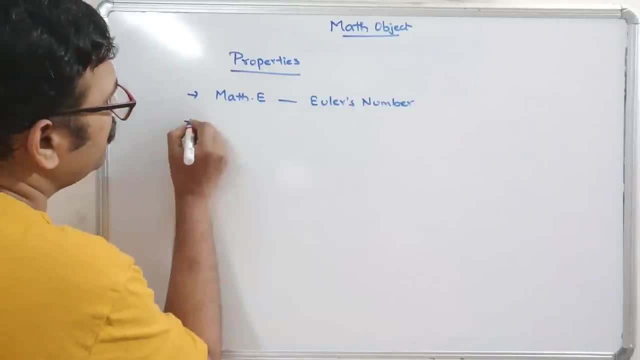 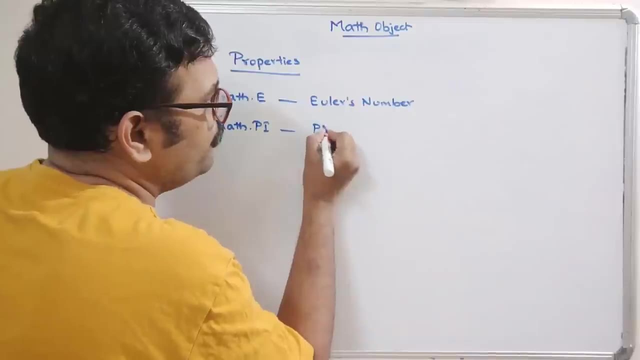 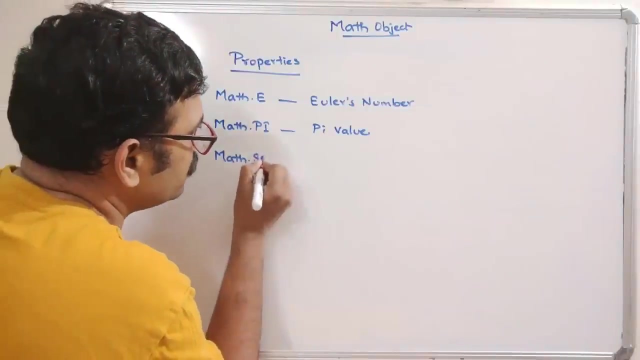 then we'll move on to the system and i will execute all those things. the next one is math dot pi, p and i should be capital letters, so it will return the pi value, the value of a pi, okay. and the next one: math dot square root sqrt, so sqrt are in capital letters. 2 that implies it will. 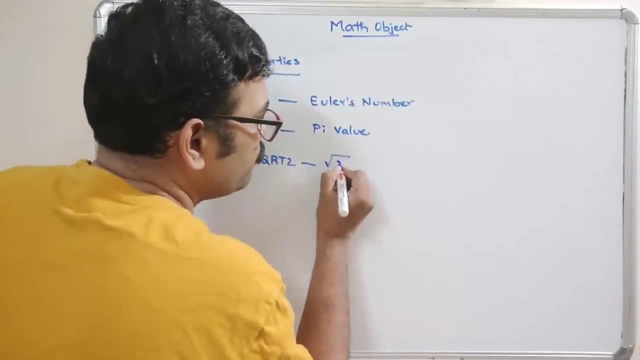 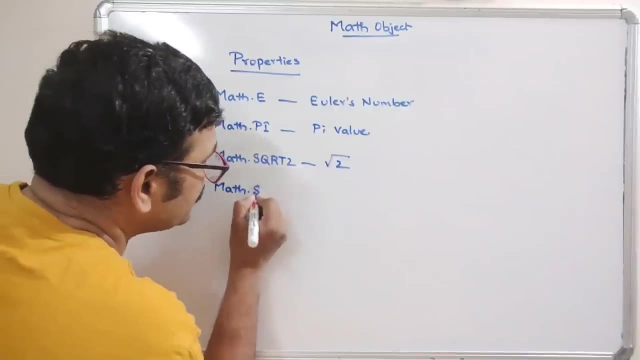 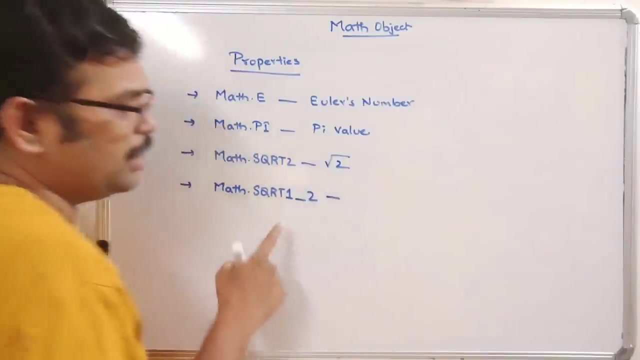 return the result of root 2, so square root of 2. okay, it will return the square root of 2. similarly, there is a one more property called math dot, sqrt 1. so this is a 1 underscore 2 underscore 2: 1 underscore 2. it will. 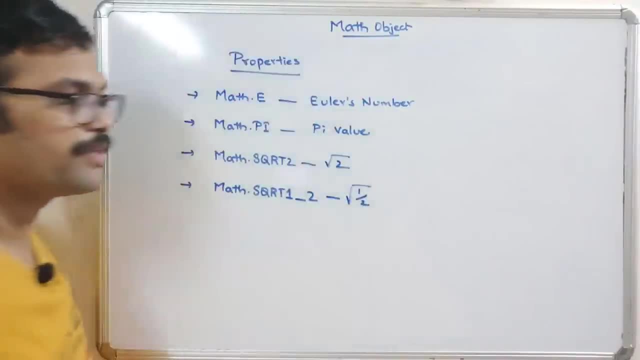 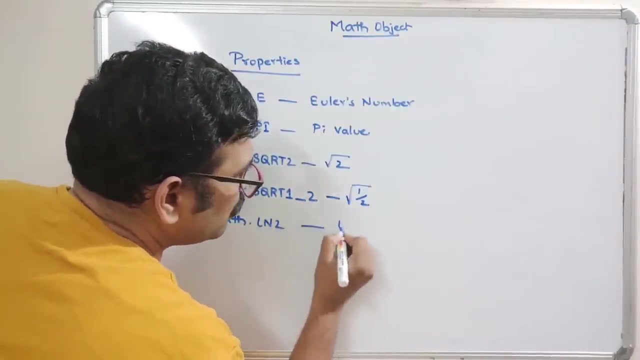 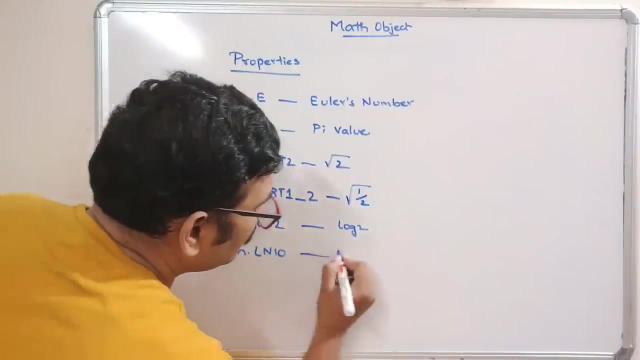 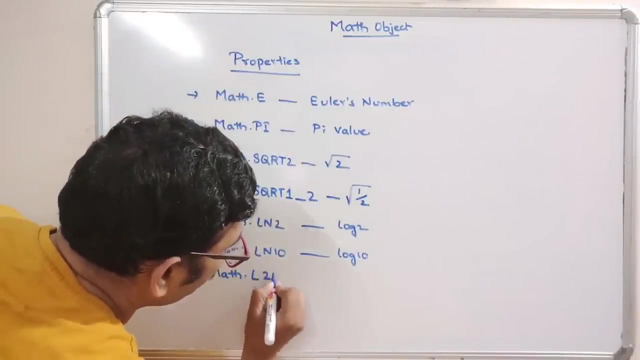 give square root of 1 divided by 2, square root of 1 by 2. okay, and then the next one: math dot l n 2: it gives log 2. similarly, math dot l n 10: it gives log 10. and also math dot l 2 e. 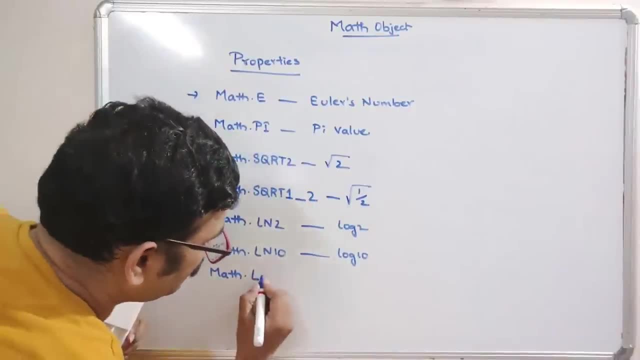 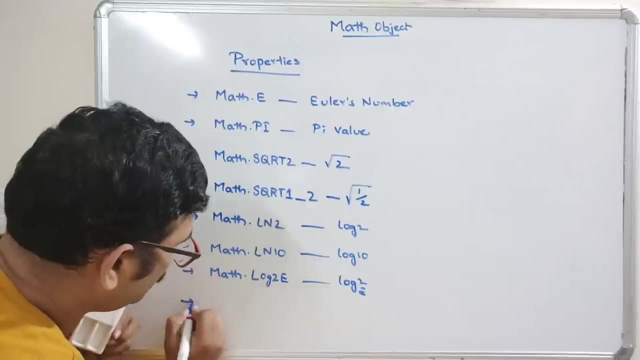 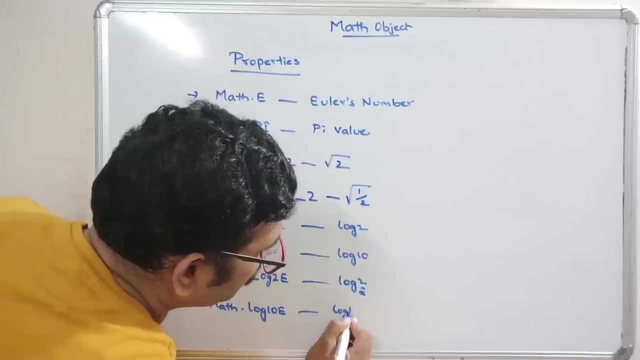 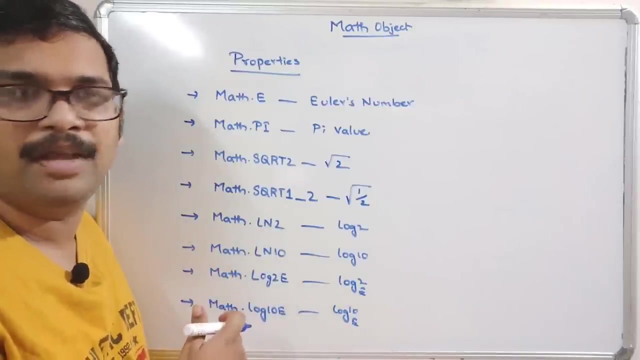 sorry, sorry. log 2 e: it will give log 2 base e. similarly, math dot log 10 e: it will give log 10 base e. so this, these are the properties available in math object, so we can directly use them. okay, if you want to use a pi value, we need to give this. 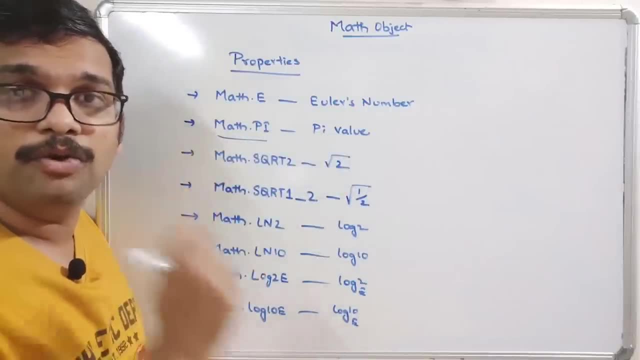 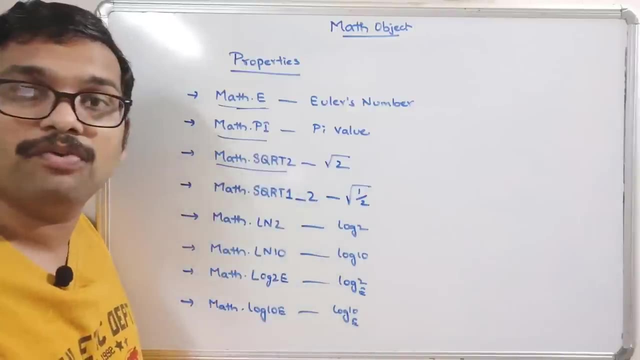 math dot pi. if you want to give, give the euler's number, we need to give math dot e. if you want to some some square root, we are supposed to give the math dot square root of 2, so we are supposed to. we are also having a method called square root. so if you directly want to use this square root, 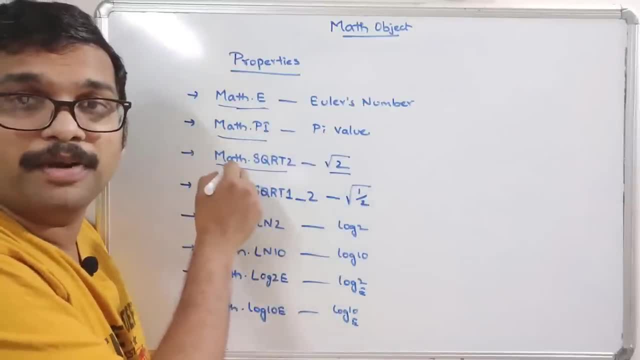 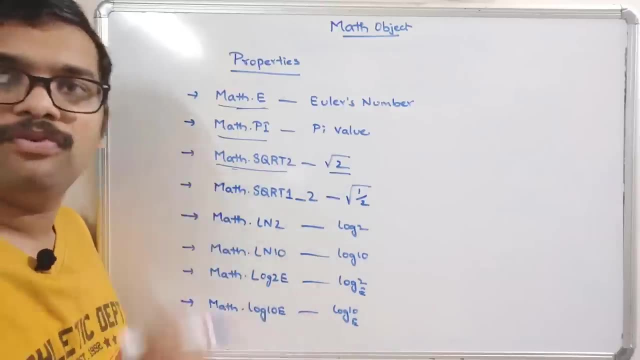 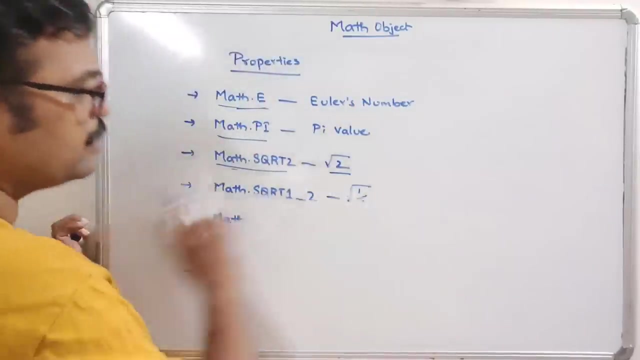 root of 2, then directly we can go with this, this property. okay, we need not go with the function directly, we can use this property, right? so these are all the properties of math object. now i will execute all these things. okay, so now we'll see the methods and then we'll move on to the system. 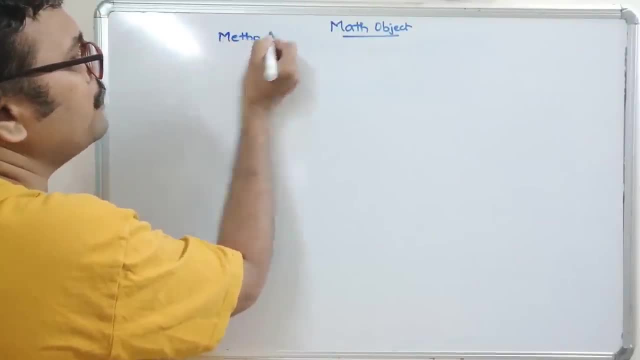 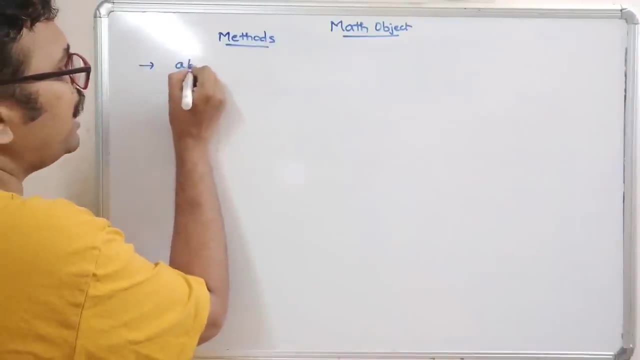 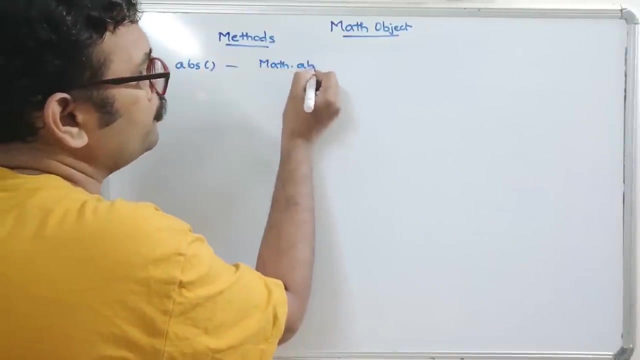 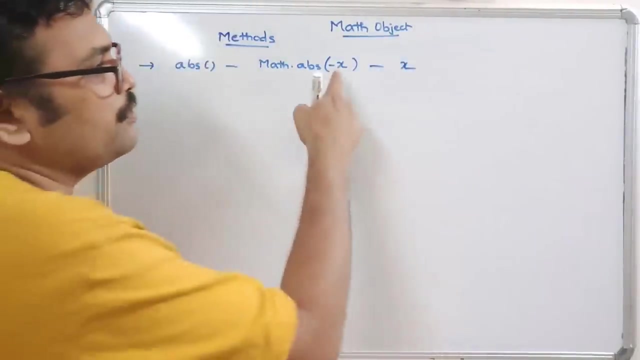 now we'll see the methods. so what are the methods available? so we'll see the method and i will execute them in the system. so first one is absolute, absolute. so the syntax is math dot: absolute of some x. if you give the minus x, we will get the x as a result. okay, if you give the negative value. 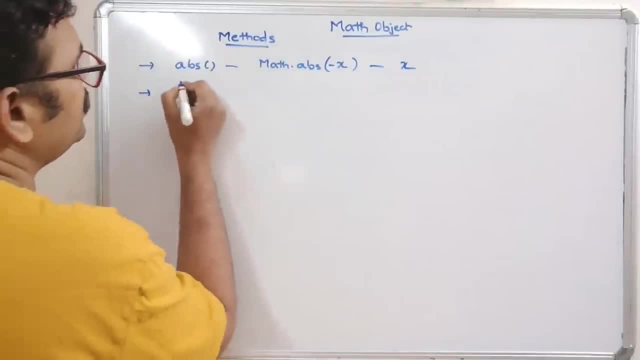 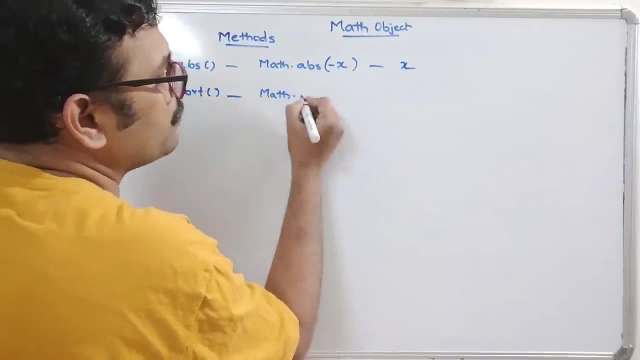 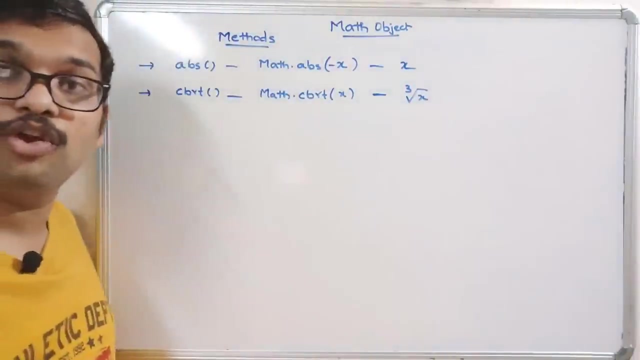 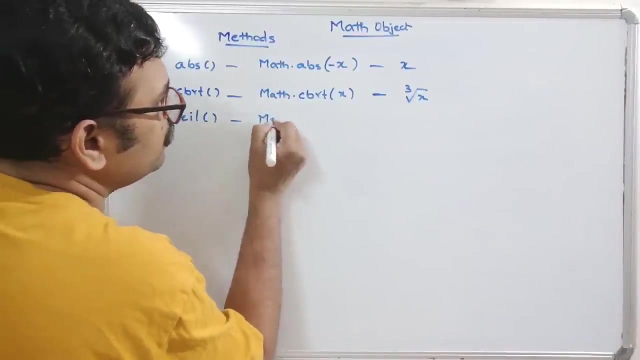 we'll get the positive value, and the second one is cbrt. so for that also we have to call, with the help of math, math dot, cbrt of x. this gives the cube root of x. it gives the cube root of x, similarly seal function, so that also math dot. 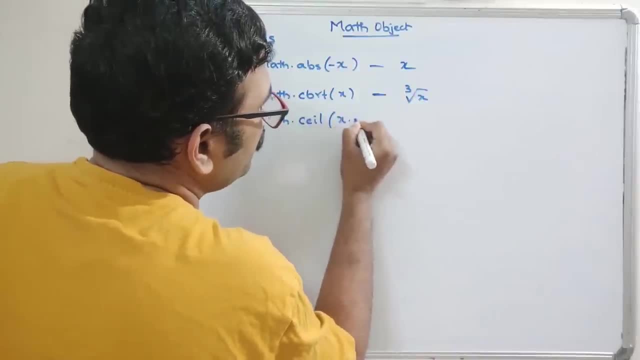 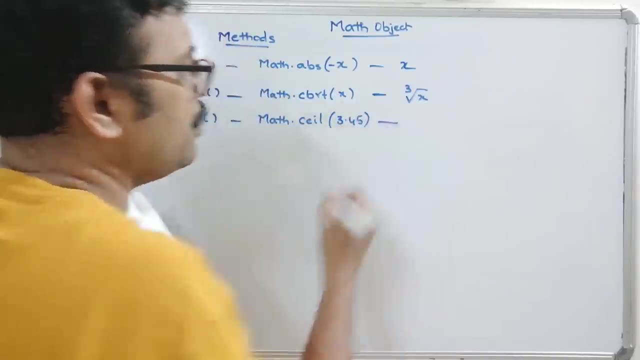 seal of x. point. let us take directly number 3.4, 5: okay, so automatically it will round down. so let us take x: okay, we'll see the example there. so x, then it will automatically round. seal. round up of x. it will return. round up of x. 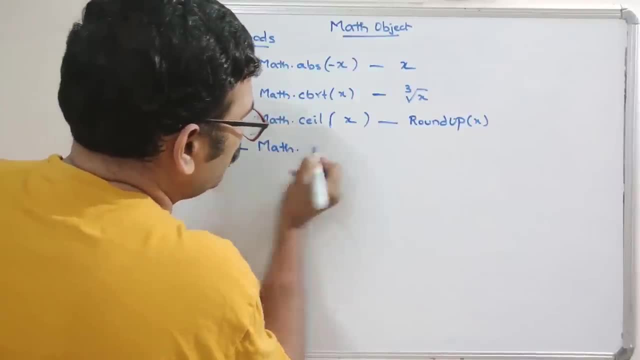 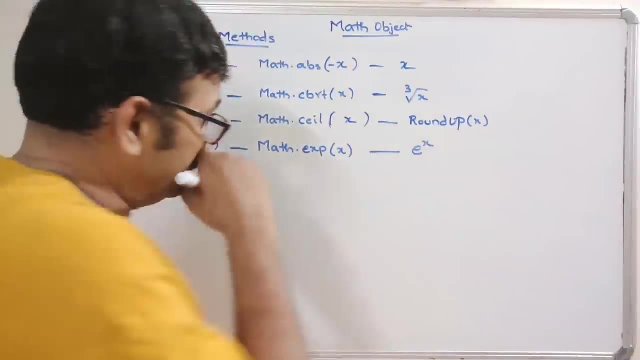 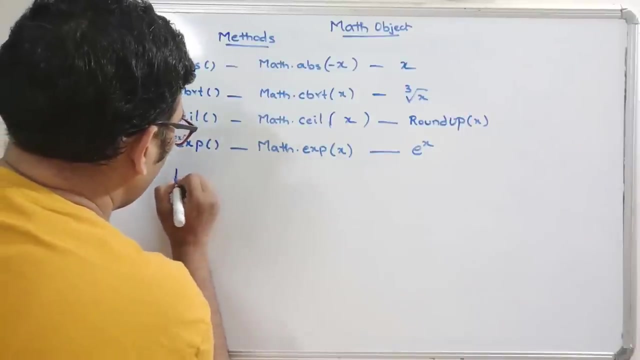 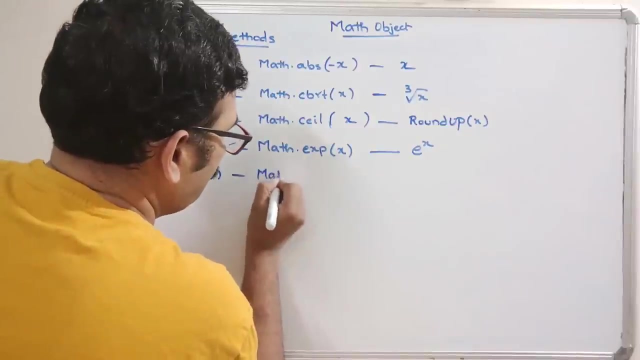 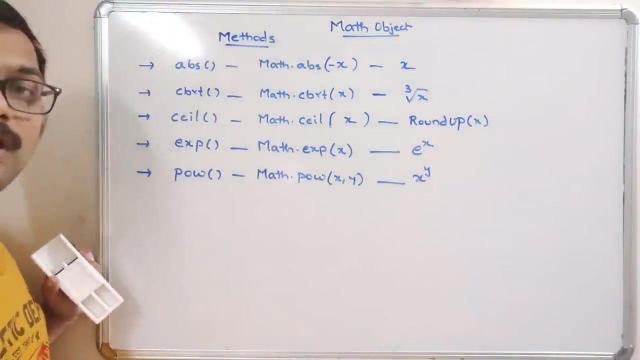 exponential. so again, math dot exponential of x. it will give e. exponential of x. it will give e power x. okay, exponential, yes, power power function. so here, math dot power of x, comma y. it will return x power y. okay, it will give x power y. it will return x power y. okay, it will give x power y. 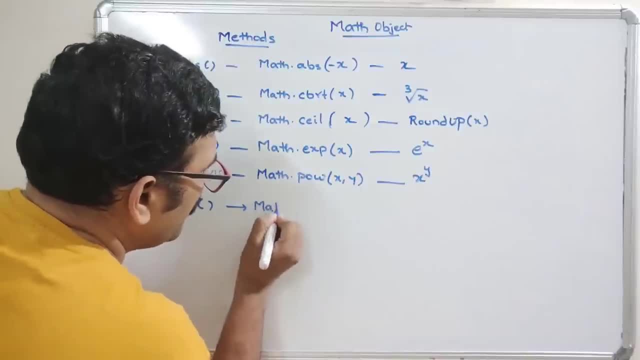 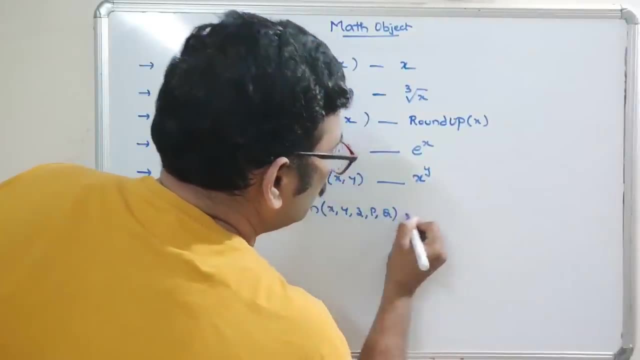 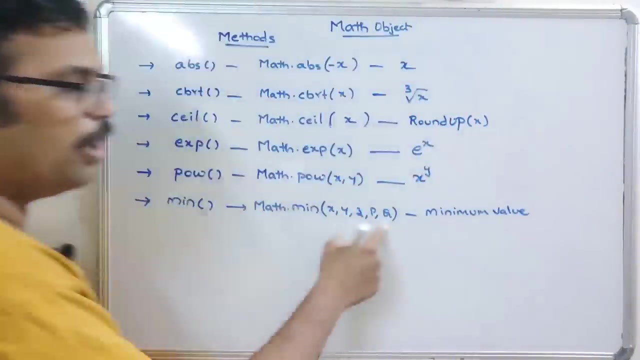 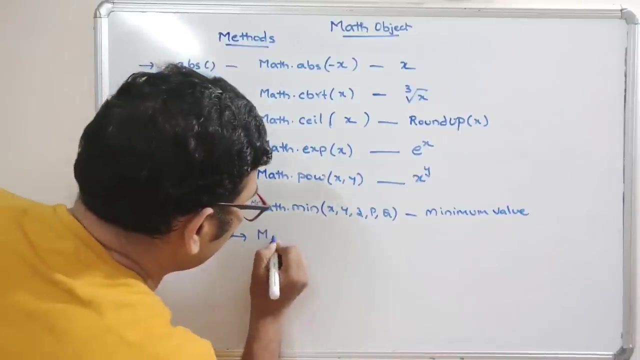 minimum function, math dot Hay, minimum value. above all these numbers dot at royable value. among all these numbers, number, and along with all these numbers, similarly, we are having another function called max. we to well to it is. in this one we need to call math dot max of x: 1 or x 2. x is equal to a. 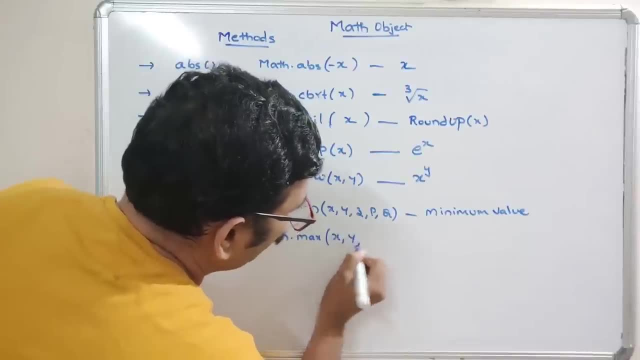 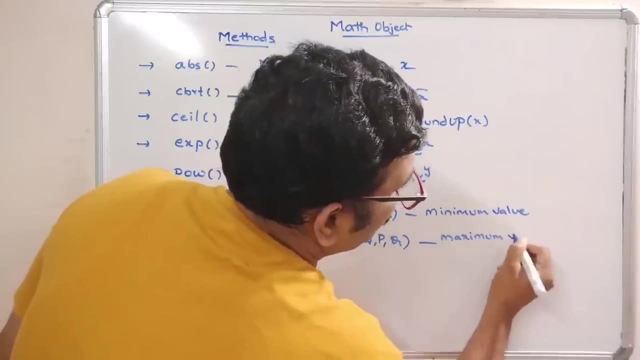 triangle from x to 0. x goes with c. We have left the skill function. we will use isλα, coololl, the, the superscripts we will use for that max of x, y, z, p, q. It will give the maximum value. It will give the maximum value. 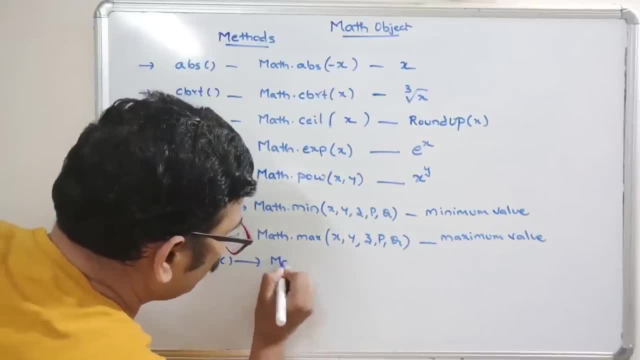 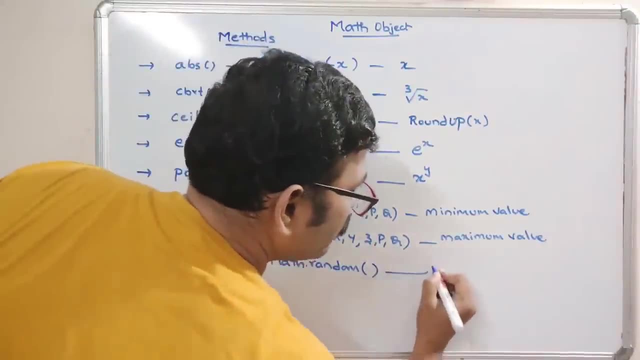 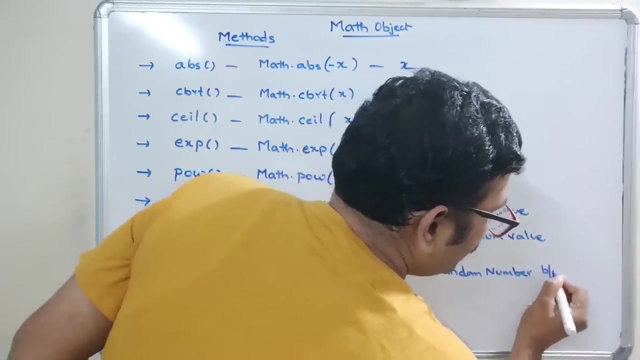 Random. For this also we have to call, with the help of math, math dot. random. Okay, This will give random number, random number between 0 and 1.. So in between 0 and 1, we will get the random. 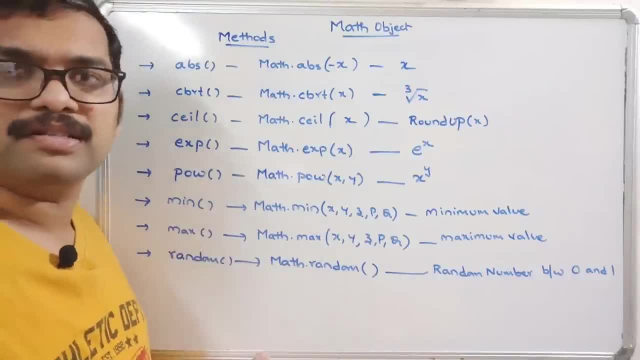 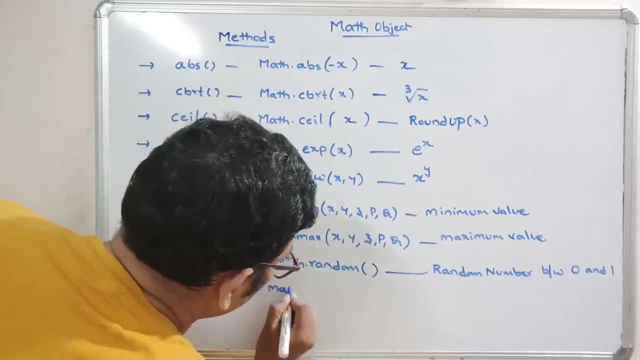 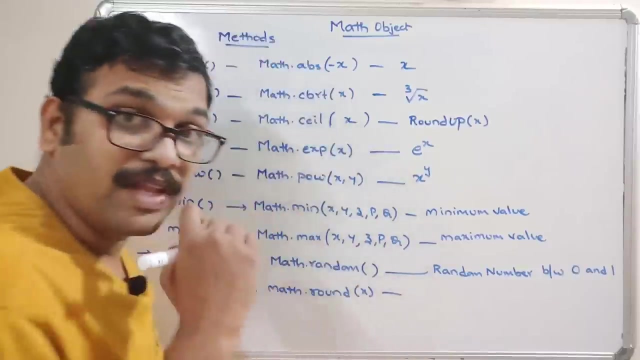 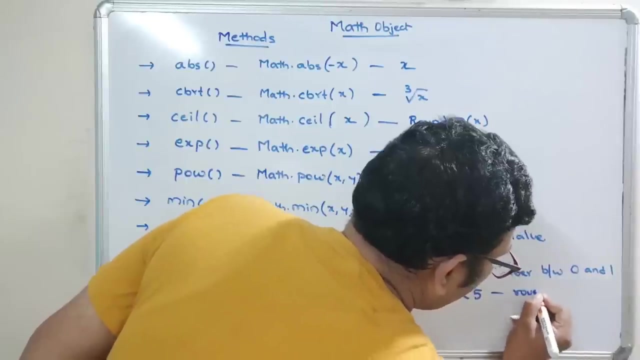 number. So keep on executing this one. we will get a different results. Okay, Next one round function. So math dot round of x. So if the decimal value, the decimal, is less than 5, it will be applying round down, round down. If 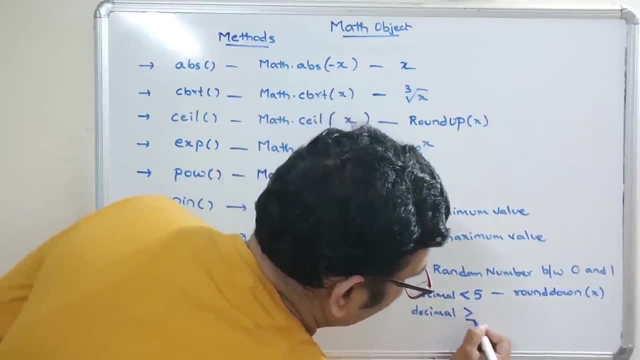 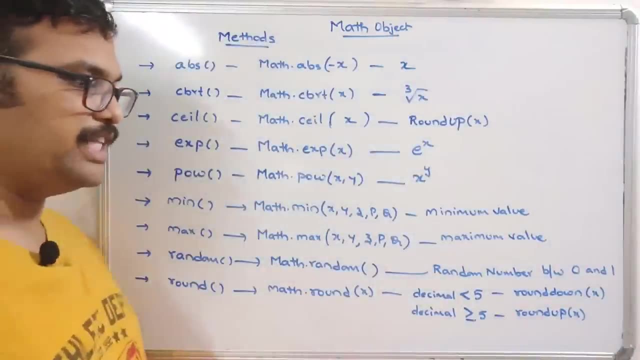 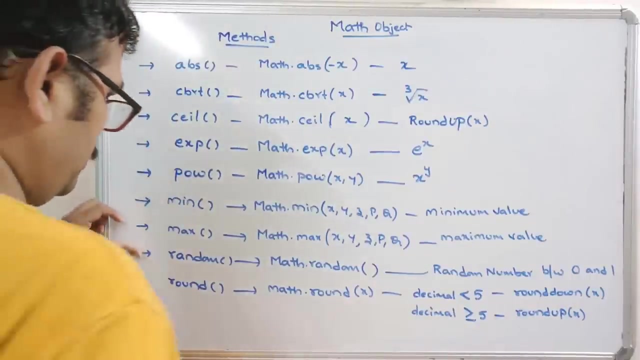 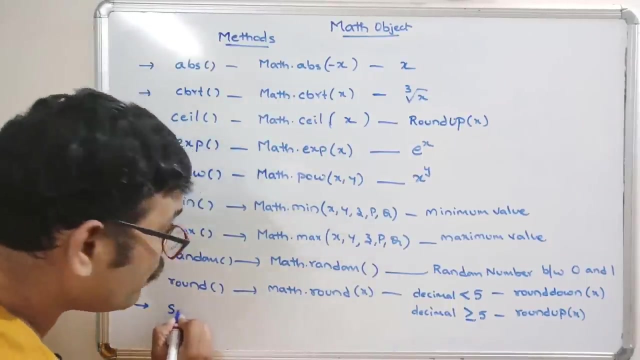 the decimal. if the decimal greater than or equal to 5, then automatically we will get the result as round up of x. So based upon the decimal value we will get the result either round up or round down. Okay, Square root, Square root function. For this also we will go with the math dot. 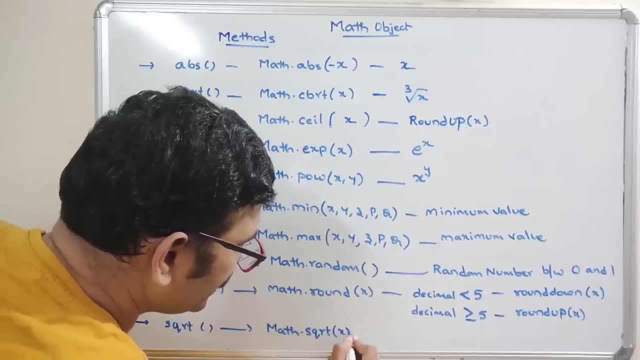 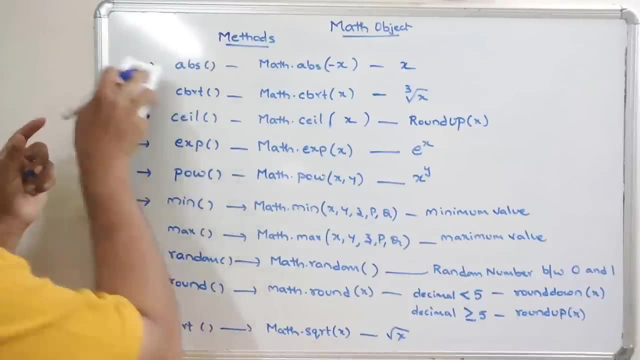 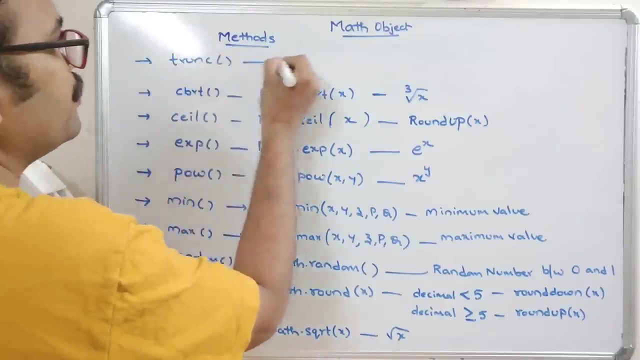 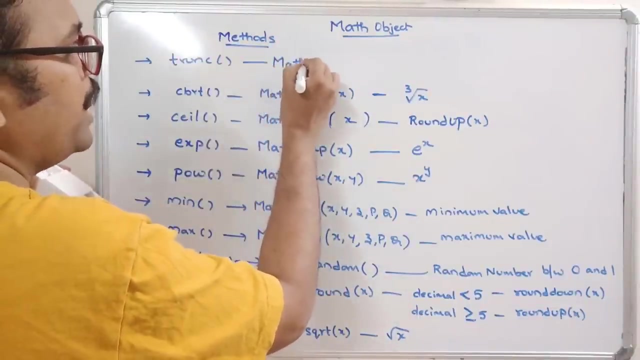 square root of x. Automatically we will get square root of x value, square root of x value. Okay, After that, truncate, Truncate. So for this again we need to call, with the help of math, math, dot. 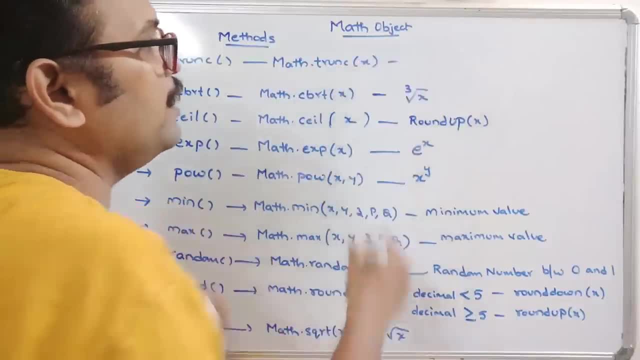 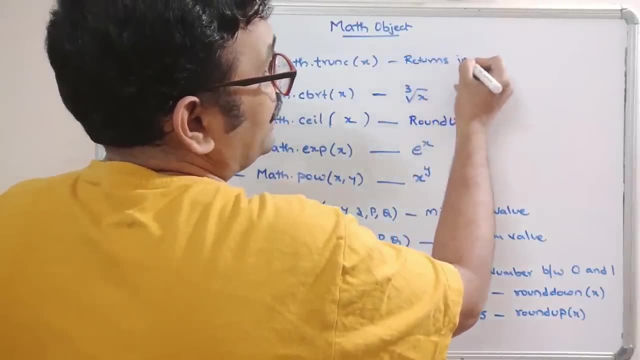 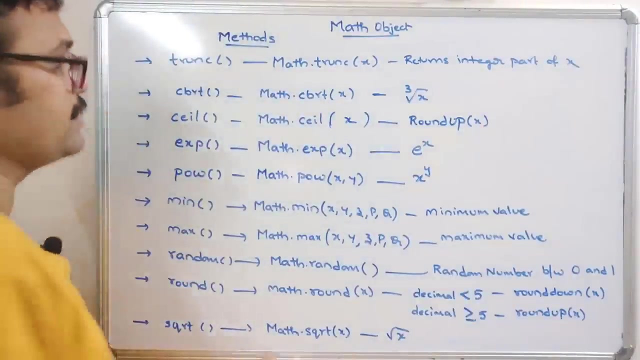 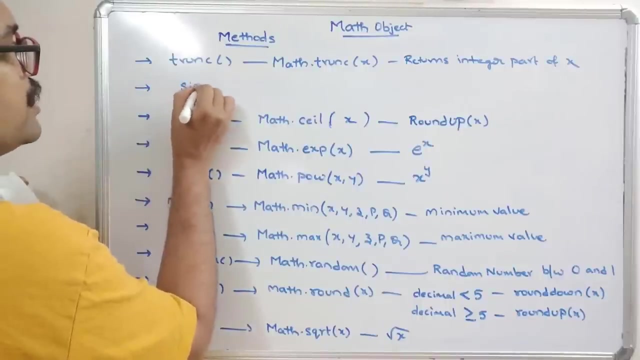 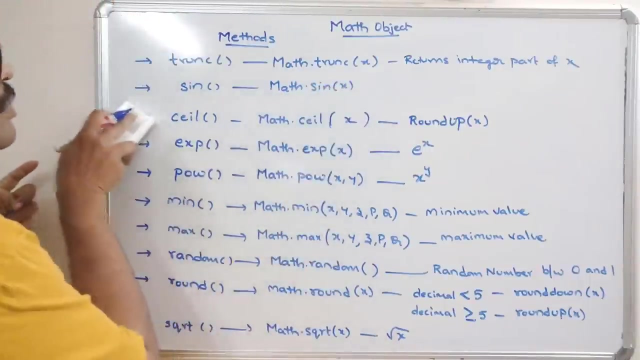 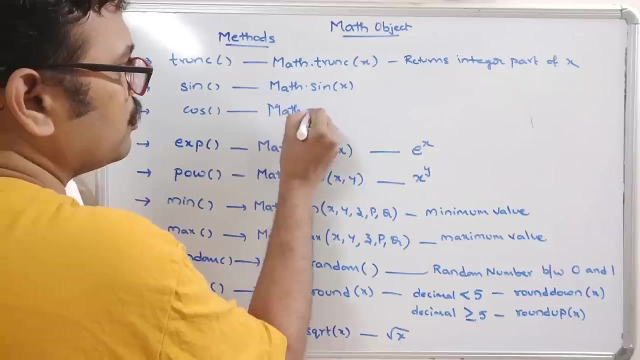 truncate of x, Automatically it will return only the integer part. It returns integer part of x And then the trigonometric functions sine. So for this we will go with the math dot sine of x. Okay, Similarly cos. So the syntax is: math dot cos of x, Similarly tan. 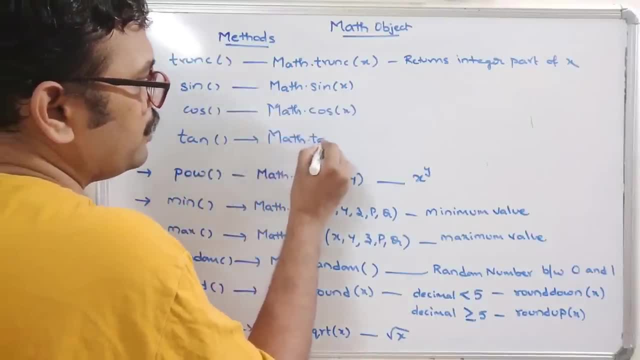 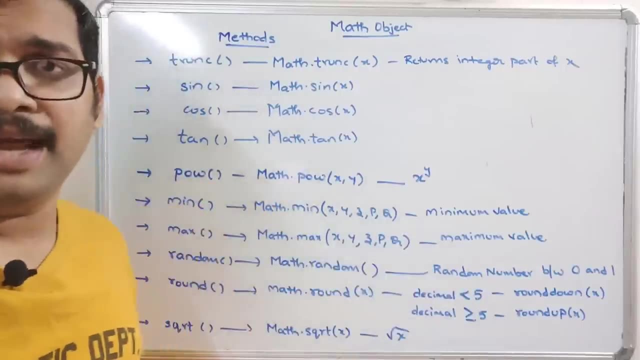 of x. So math dottan of x. So apart from these we can also find hyperbolic sine, hyperbolic cos and hyperbolic tan. So all these things we can apply. So these are the 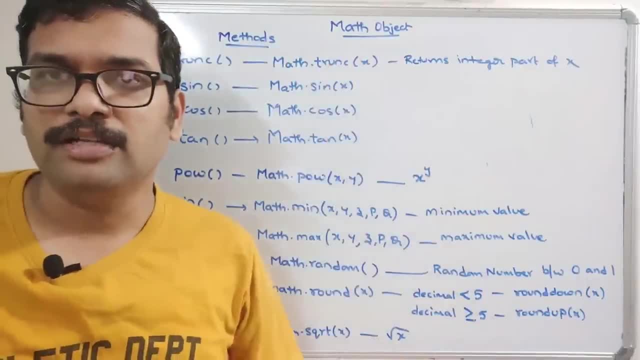 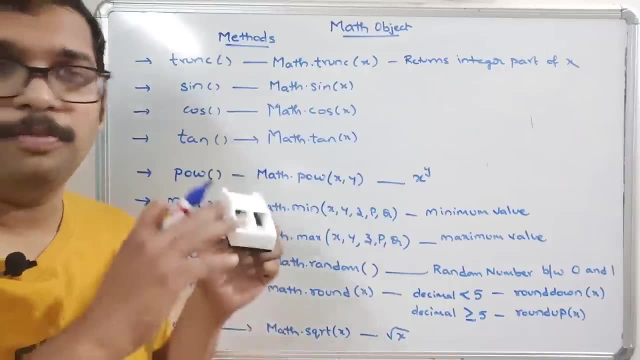 a few methods available in math object. So I will execute and I will demonstrate each and every function by executing a small code on the system, Right? So hope you understood the syntax for all these things. So if you are having any doubts still, 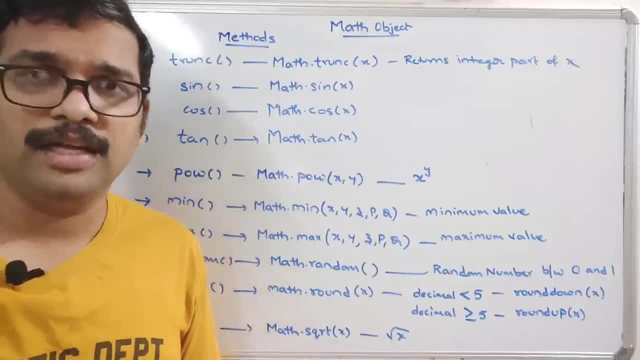 experiment with this, So I will see you in the next video. Bye, Bye, Bye. Come back on the system, Right? So hope you understood the syntax for all these things. So after after watching the execution, your notes will be clarified, right? so let's. 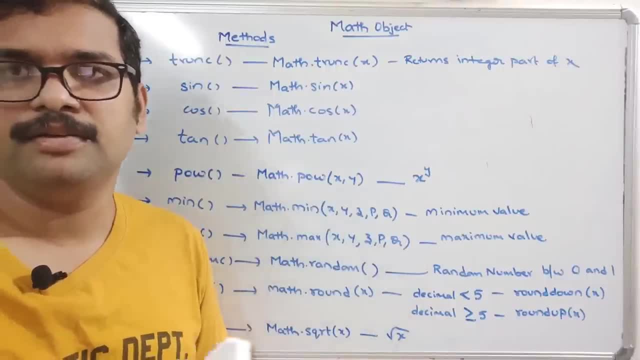 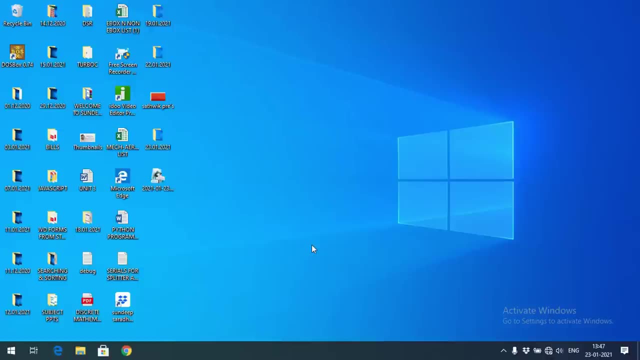 move on to the system and execute all these methods. hello friends, so just now we have seen about the math object methods and the math property. so I will demonstrate each and every or method of a math object and properties by executing a small code. so let us start writing the code. so first we will begin. 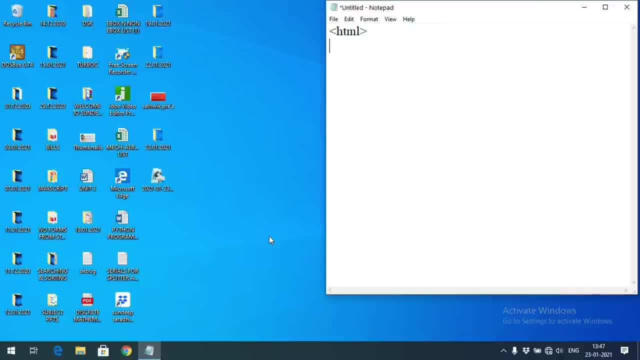 with the HTML tags. so in between the HTML tags will write the body and we'll write some title and then we'll start writing the script. so body, so inside the body will do the title as a math object. right, which one math object or math properties? first let us see the math properties and then we'll go with the 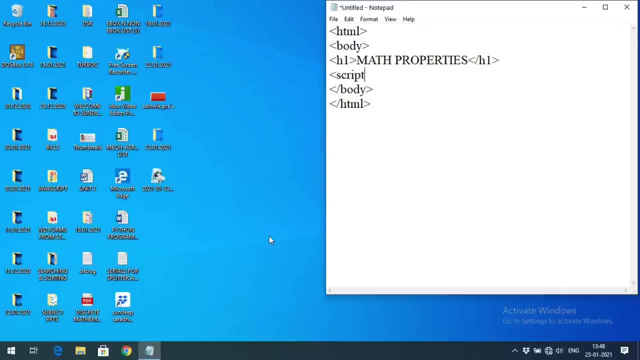 math methods. so script, and inside the script we can write, and actually we have created the objects for the previous thing. that is, if you observe the data object, we are using the objects with the help of new keyword. but here math is a special thing, that we need not create the math object first, but directly we can use the. 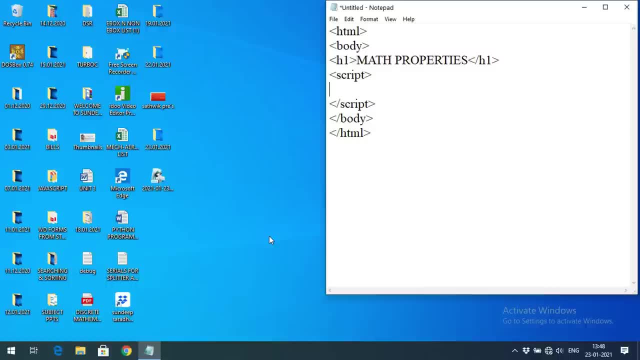 methods or properties with the help of math name, right, so let us start here. so there are a few properties which we have seen just now, so I will demonstrate this. so document, let us take document, dot, write LN. so let us give the some other heading so that the display will be good now. so 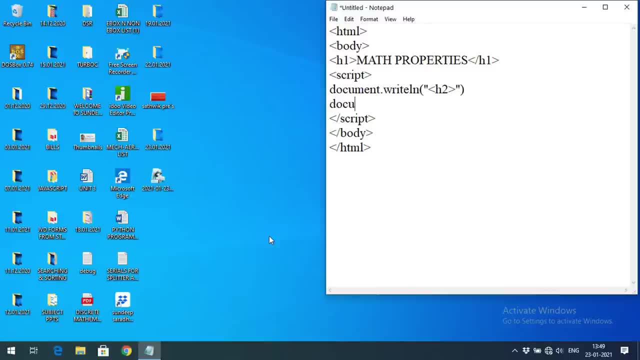 first, first property. so all the properties and methods should be called with the help of math, right. so right line, write LN, math dot E. E means a Euler's number. it will print the Euler's number. okay, see, I will go this one plus and go with the br for the output to be displayed in the next. okay, so I am. 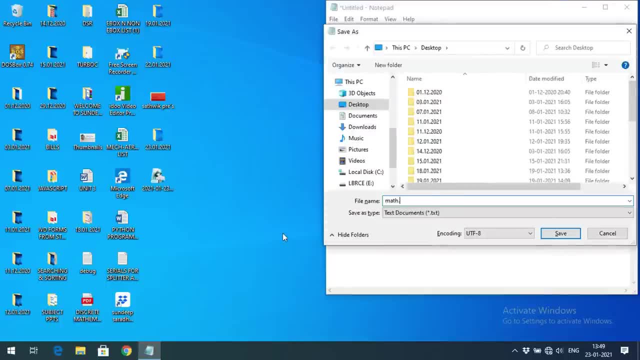 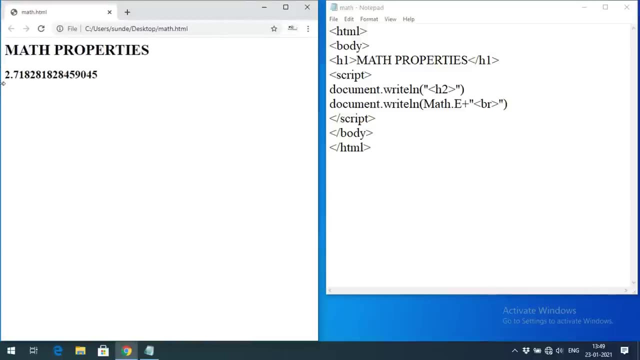 saving this one for math dot HTML. so we have got this one. so by double-clicking on this we'll get the. this is the Euler's number, Euler's number right, and we'll save this. one will go with another property. These are all the properties. These are all, not a method. 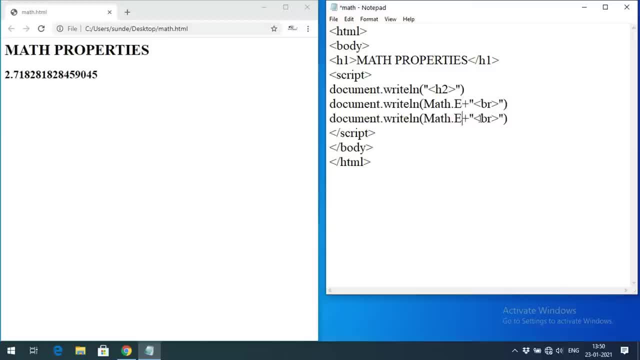 If it is a method, you have to use the parentheses. This is a property, So properties are nothing but a constant. This is a pi value. The next one is a pi value. We know that 3.14 is a pi value, So in order to use the pi in JavaScript, we have to call that pi with the math object. 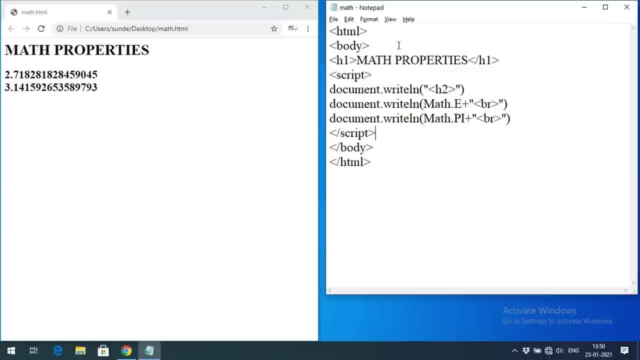 mathpl. So here you can observe, we have not created any math object with the use of new keyword. So this is a special thing, So we need not go with the math object. And again, there is one more constant called square root, sqrt2, square root of 2.. The result: 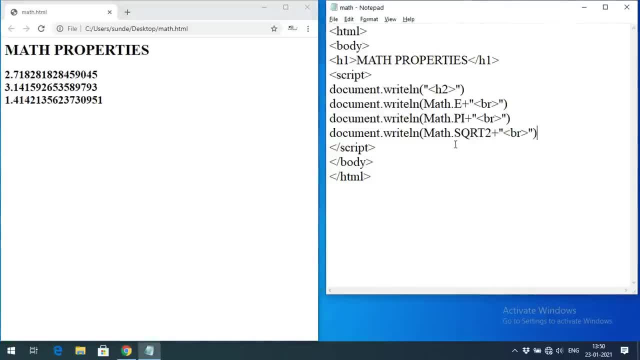 of square root of 2 will be getting here right. So sqrt is in capital letter And similarly there is one more thing called one more property, called sqrt1, underscore 2.. That means 1 by 2, the square root of 1 by 2, okay, You can observe. So the square. 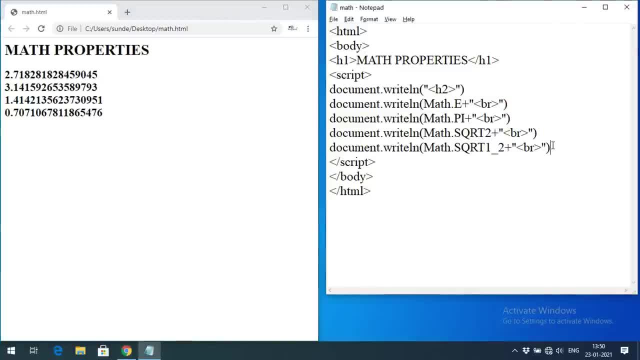 root of 1 by 2.. So sqrt2 is like this: square root of 2, square root of 1 by 2.. And similarly, math dot log 2, log 2.. So this is the result for log 2.. And similarly there is a one more. 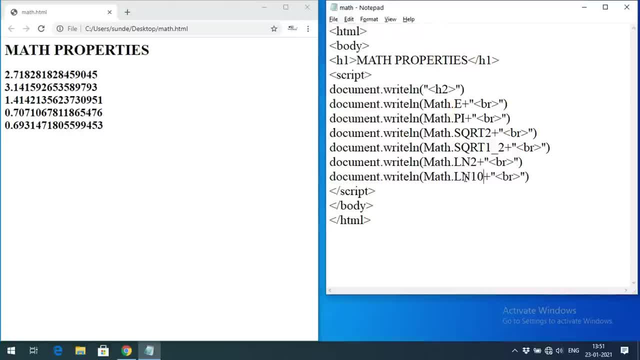 thing called log 10,, log 10.. So you will get the value for log 10.. And all these are the constants. We can go with the constants, right. So next one is log 2e, log 2 base. 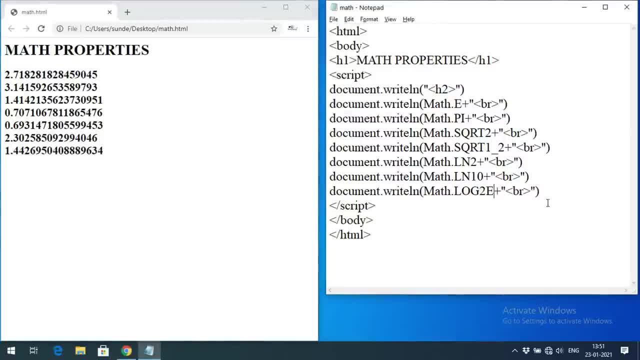 e. So this is the result for log 2 base e. So this is the result for log 2 base e. So this is the result for log 2 base e. And similarly, we are having one more thing called. 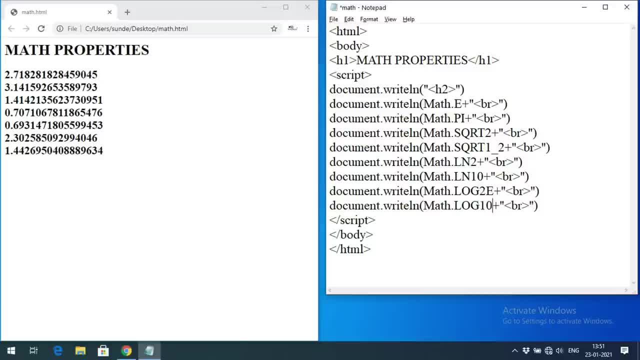 log 2, log 10 base e. okay, Log 10, base e. All these are the constants we can use in our scripting, right? So let us close this one document. dot write ln- And I am closing here, So h2.. And now again, I am writing one more title. 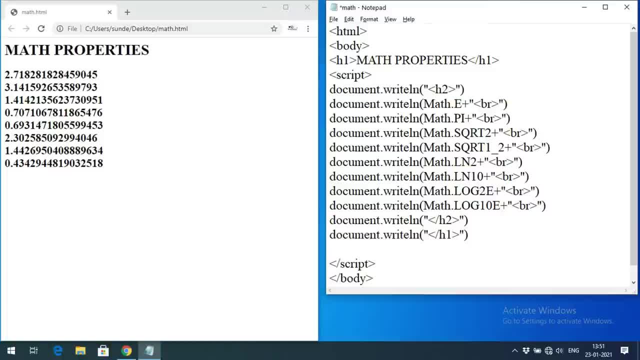 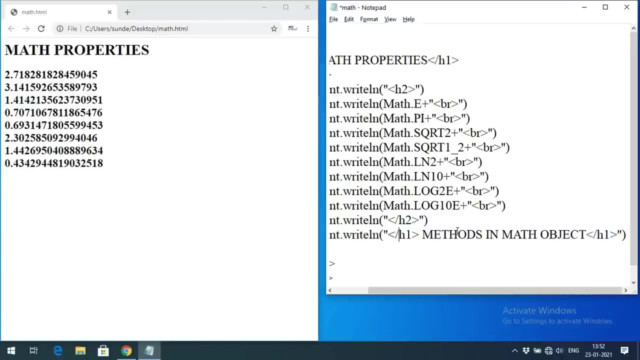 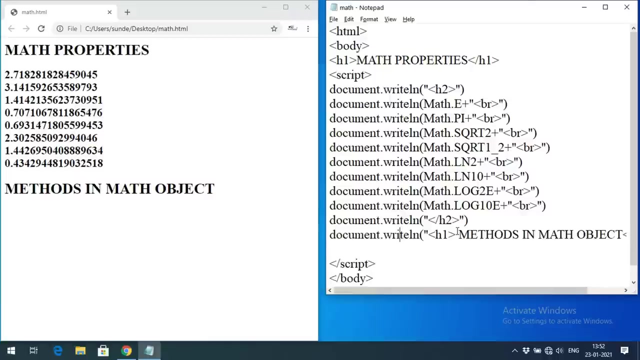 So h1 with property: math object methods. okay, Methods, Methods in math object. right, You can observe again. we have given certain title right Now we will start. So document dot write ln. First one is absolute. So let us take the absolute function. Let us take 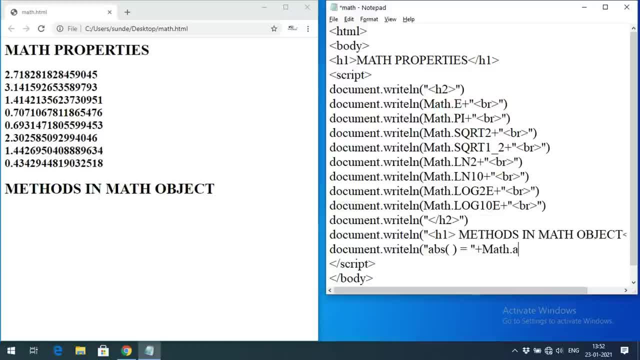 the absolute function, And those functions are the ones that we are going to use. So let us take the absolute function, And those functions are the ones that we are going to use. So let us take the absolute function, And those functions should be called with the help of mathname. 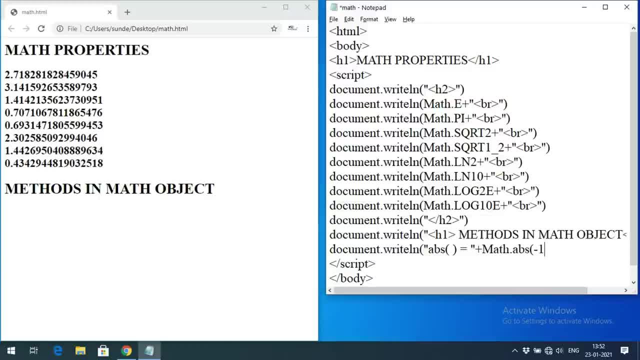 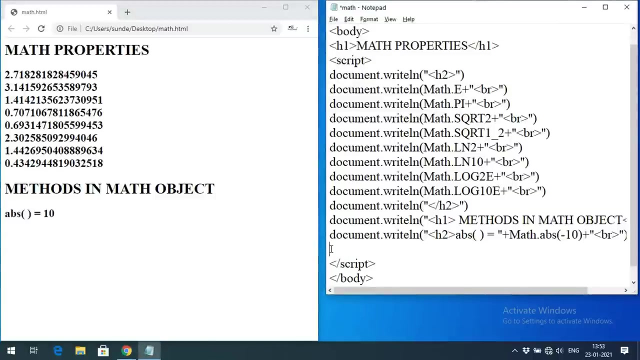 So math avvolute of some minus 10.. Automatically it will give the positive result, right? You can observe here: abs 1.. Or and again h2. H2. See abs 2.. abs of 10, that means even though you are giving some negative value, we will get the positive value. even though we are giving negative value, we will get the positive value. that is the absolute value. it is an absolute value, yeah. 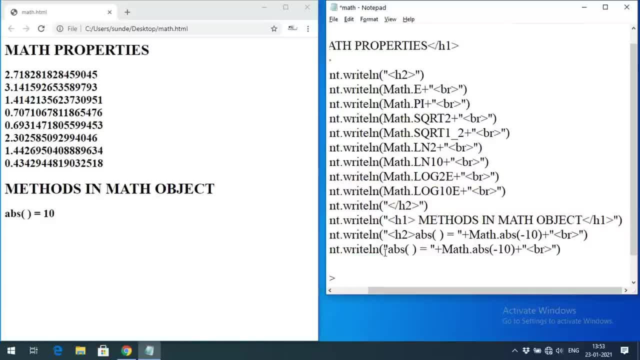 Now the next method. the next method is CBRT. CBRT means a cube root, cube root. so if it is a cube root, CBRT, if you go with the 27,. right, we have to get the 3 as a result, right, 3 as a result. so let us take some here, the values. we will take the values so that it will be displayed and you will not get confused. 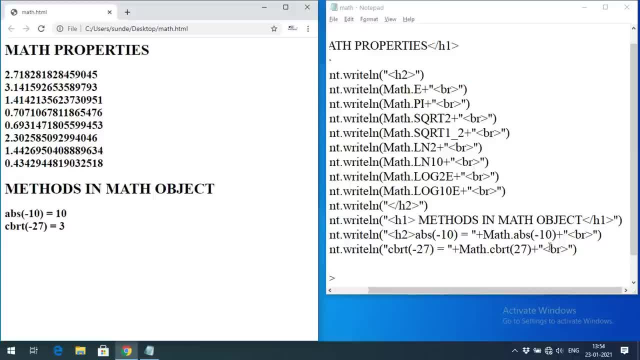 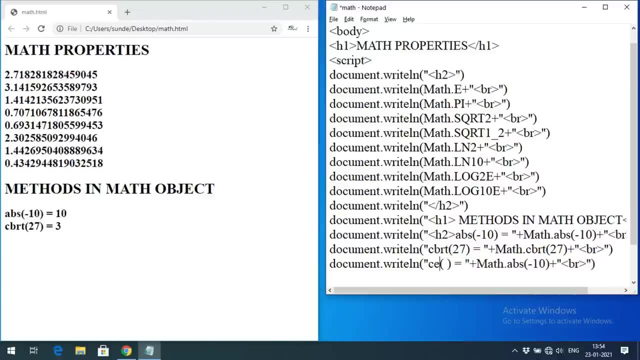 Yeah, yes, now this is a cube root and again we can have the third one, that is, seal function. seal, seal means round up, seal means round up, so 3.5, round up 3.5, and this is also a seal. okay, seal function. 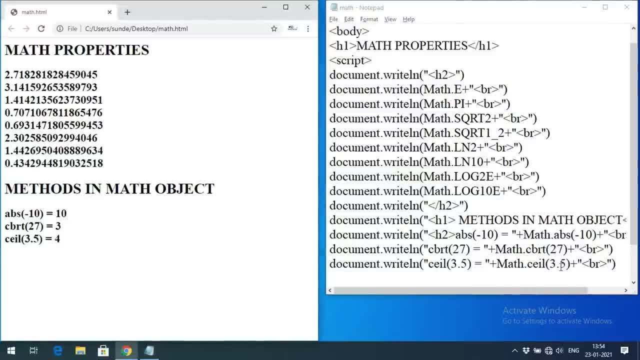 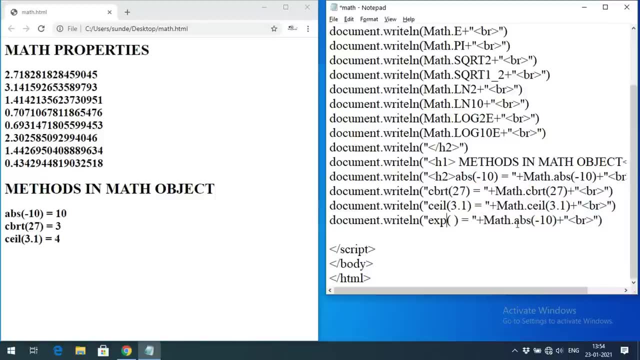 It is a round up, that means it will be moving with a 4, even though if it is 3.1,, even though it is 3.1, we will get the round up automatically. 4 we will get okay. and then there is one more function. the next function is exponential. exponential. so here you can observe exponential exp, okay, exp of 3, and here also you can go with the 3, so that we will get the result exponential 3 by 3.. 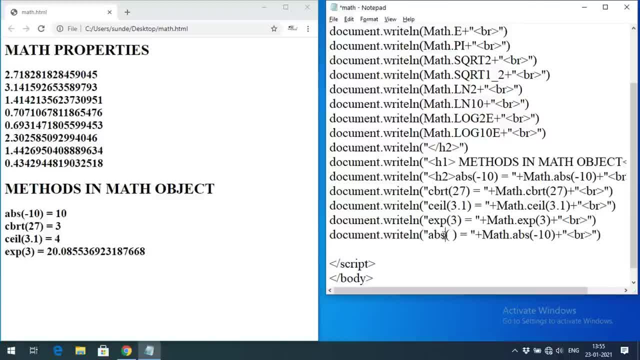 Okay, so this is the value. this one, right. and then next function or next method is a floor. it is a round down. round down 3.9 will also give the round down function. okay, 3.9 means it rounds down. okay, floor. we will get a 3 as a result. even though it is a 3.9,. we will get the result as 3,. okay, it is a round down. 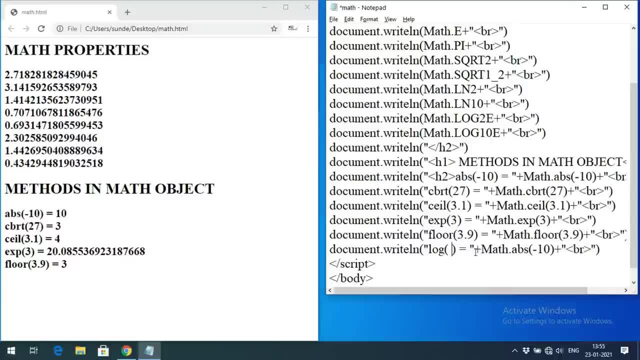 And then log, so logarithmic value some log log 2 will take, will take log 2.. So math dot log of 2. So it will give the value of log 2, log 2 value here And then the next function is a maximum. So it will take it. 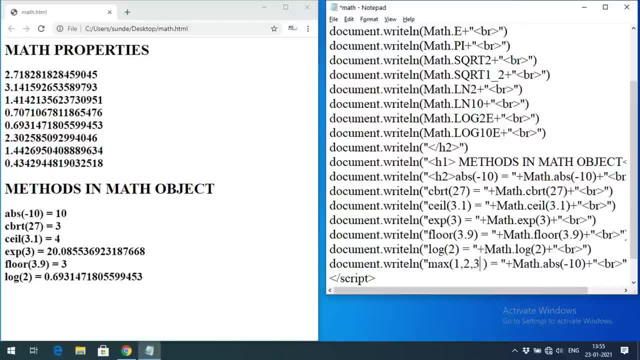 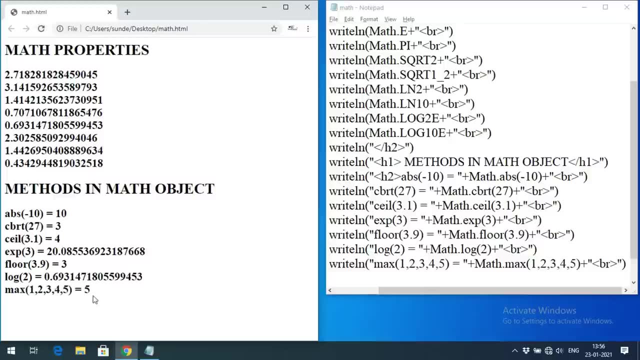 will return the maximum value from the given number of values. You can take 1,, 2,, 3,, 4,, 5.. And the same thing I am writing here: you will get the maximum value from the given elements. So the in the maximum value of given elements is 5.. So automatically we 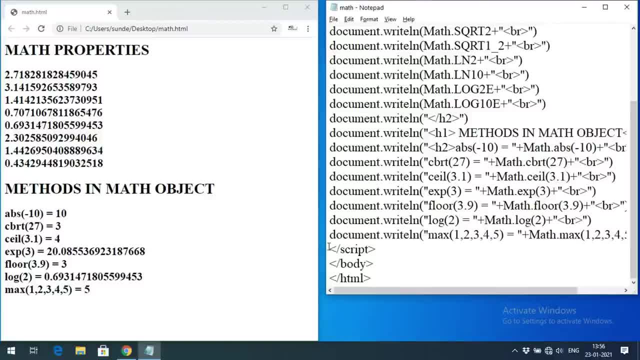 will get the result as 5.. And then similarly minimum. So if you write minimum, we will get the minimum value. So what is the minimum value? 1.. So we need to get the result as a 1.. 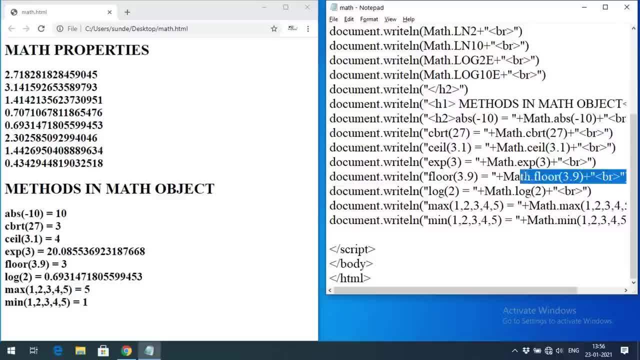 So you can get the result as 1.. And now the next one is a power power function power. So power function 2 comma 3.. And here also I will go with the power function 2 comma 3, 2 comma 3.. So automatically it will give the result as 2 power 3,, that is 8.. You can. 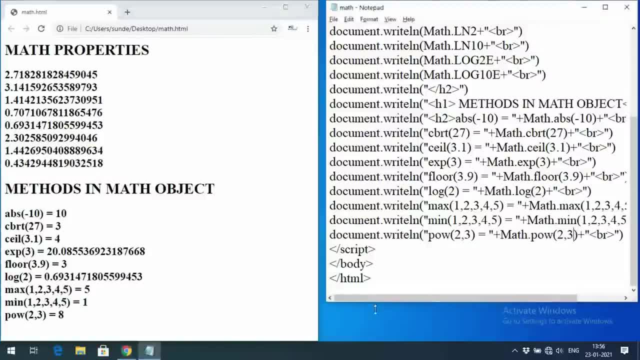 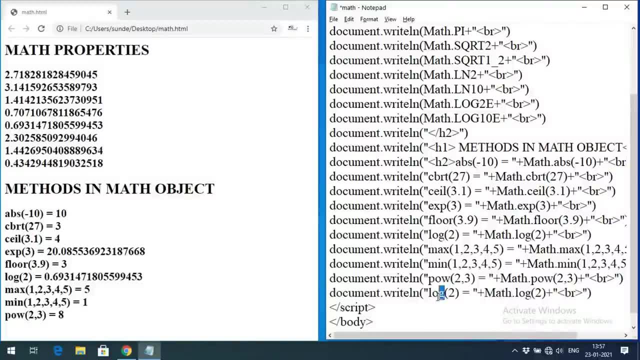 observe here: 2 power 3, it is 8.. Hope you understood this one power function. And similarly, the next function is a random function. So there is a function called random function which does not take any parameter right, any value as a parameter, And it will. 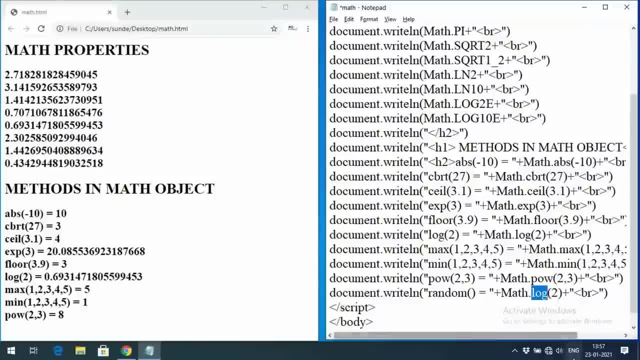 return the result: a random value between 0 and 1, a random value between 0 and 1.. We need not give any parameter here. see Once again: if you execute this one, the value of this one will be changed. So you can observe here, see Immediately whenever you refresh. 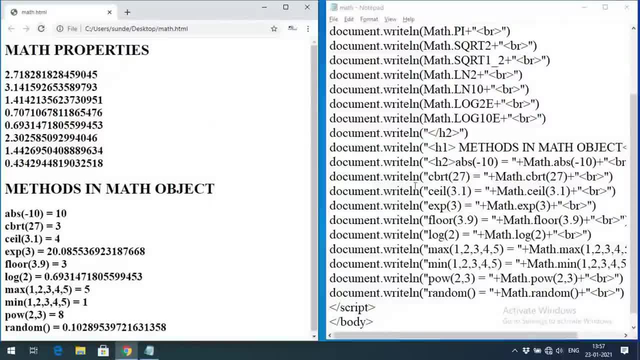 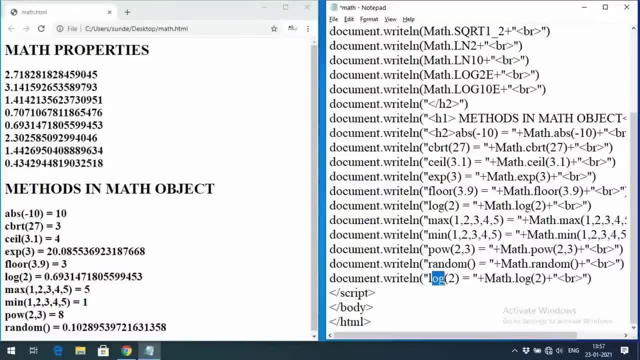 upon refreshing the page, we will get the random value, but it will be in between 0 and 1.. And then round function. The next function is round function. So round you go with a 2.3,, round 2.3, you will get the round function based upon the precision right. 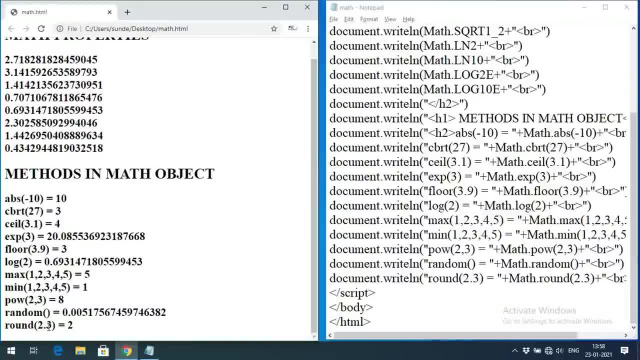 So if it is less than the decimal value, if it is less than 0.5, it will go with the round down. If it is greater than or equal to 0.5, it will be round up. So you can observe it is a less than 0.5.. So we will get the. 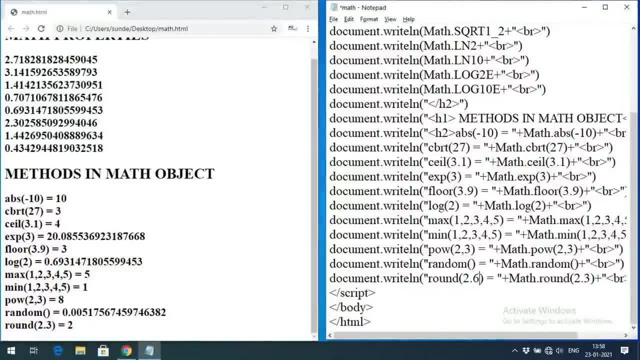 round down And if the value is greater than 0.5, we will get a round up. you can observe here. Here it is a 6,. ok, Yeah, Now we can observe. so it is a 3,, right, So if it is. 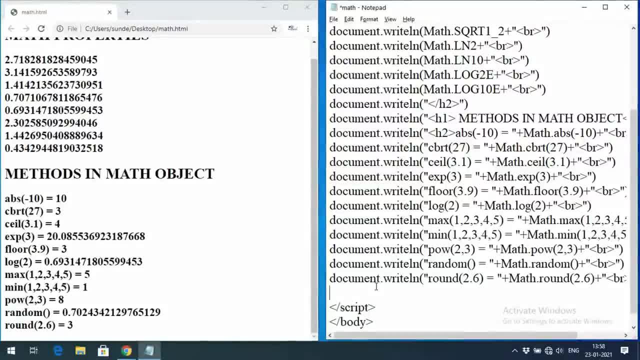 greater than or equal to 0.5, it is also, it will be round down. So, again, if you consider, it will be round up. If it is a less than 0.5, it will be round up. And the next one. 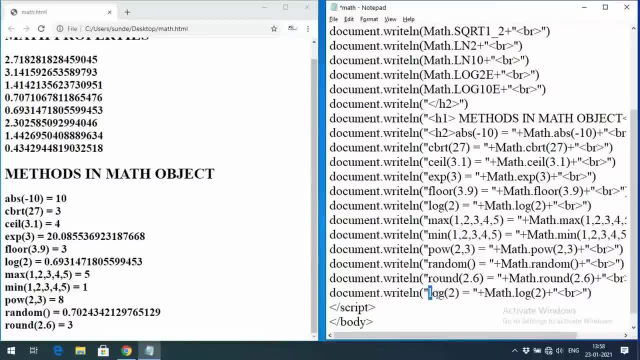 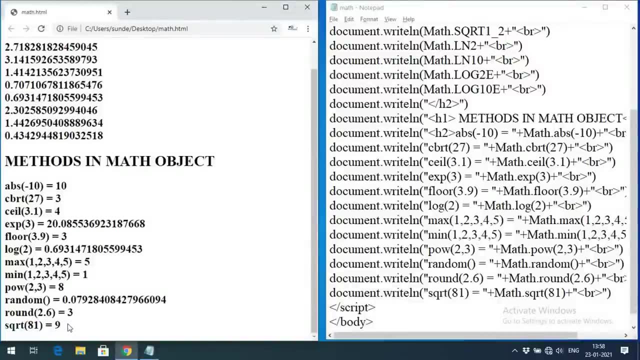 is a square root function, So square root SQRT of 81.. Similarly, SQRT of 81.. So we will get the result as a 9.. So you can observe here: Result as a 9.. Square root of 81 is. 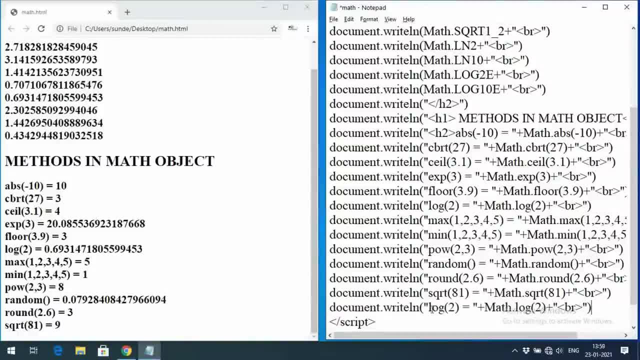 9. Next, truncate. Truncate, That means it will omit the decimal values. It will give only the integer path: Trunc Point 2.12345.. Similarly, trunc 2.12345.. So automatically. 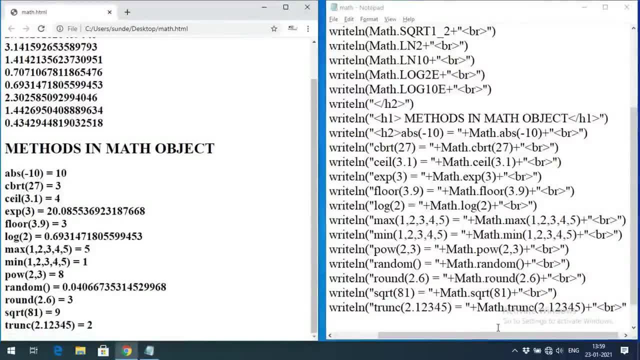 we will get the only integer value. So you can observe here Point 2.12345.. So if you give the value, then also we will get the same thing. See, it will omit the decimal values and will get only the integer value. Similarly, apart from: 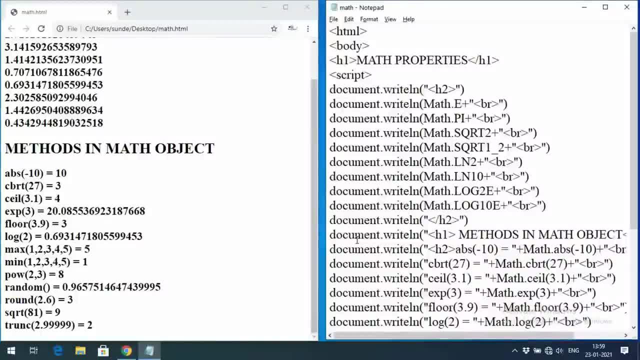 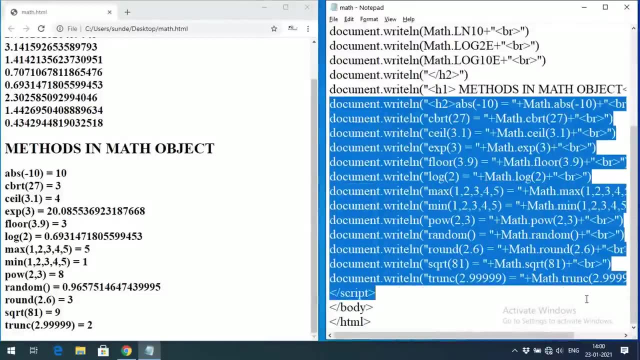 all these methods, there are a few methods of trigonometric functions like sine cos, tan, hyperbolic, sine hyperbolic. So all these functions are also available in math object. So these are the few object methods, A few methods available in math object. So hope you understood this one. So if you, 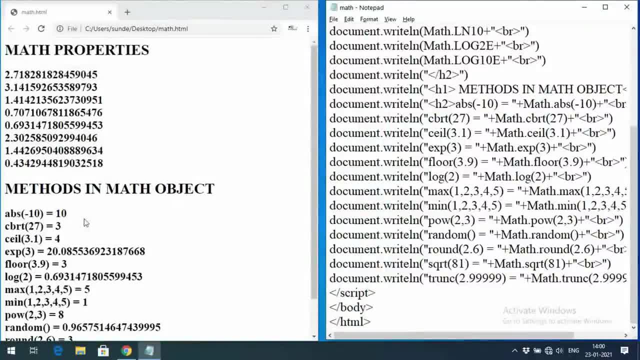 are having any doubts regarding these properties, either properties or methods, so feel free to post your doubts in the comment section. Definitely, I will try to clarify all your doubts And if you really understood my session like my session, share my session with your. 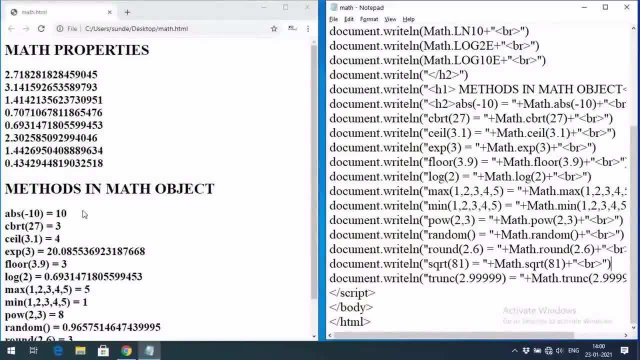 friends, and don't forget to subscribe to my channel. So thank you. Thanks for watching. Thank you very much.